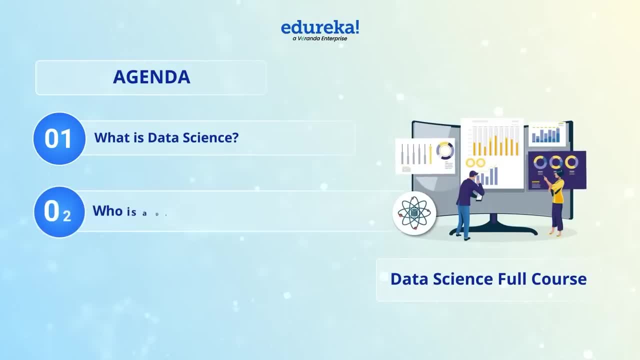 to know. Followed by this, we have the topic: who is a data scientist? Now, once we understand who a data scientist is, we'll then see the roadmap to becoming a data scientist. We'll also see some salary statistics after that. 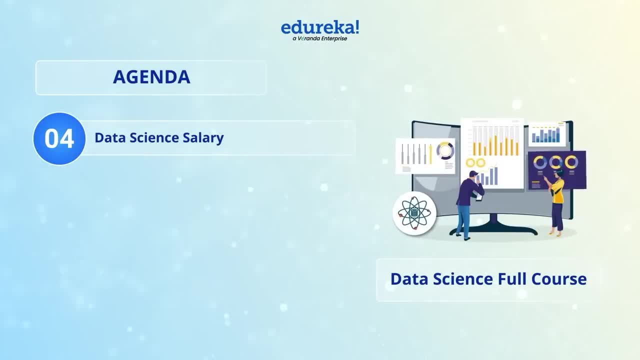 Next we'll discuss the data science core concepts. In this we'll begin by seeing the data life cycle. This topic discusses the stages in acquisition and processing of data. After that we have statistics and probability. These are three important concepts, which sets your foundations, So take your time understanding. 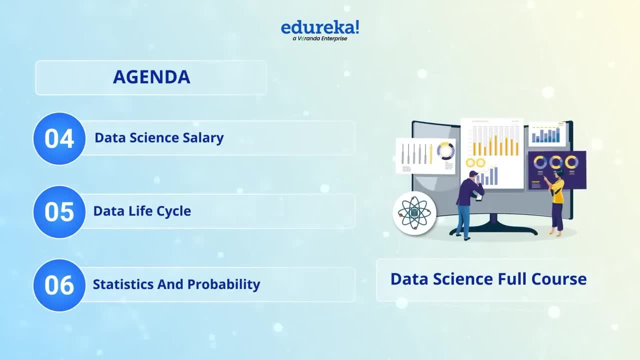 this part. Once we're done with statistics and probability, we'll cover what is machine learning. Followed by this topic, we have some core algorithms in data science, which includes Linear Regression, Logistic Regression, Decision Tree Algorithm, Random Forest, KNN. 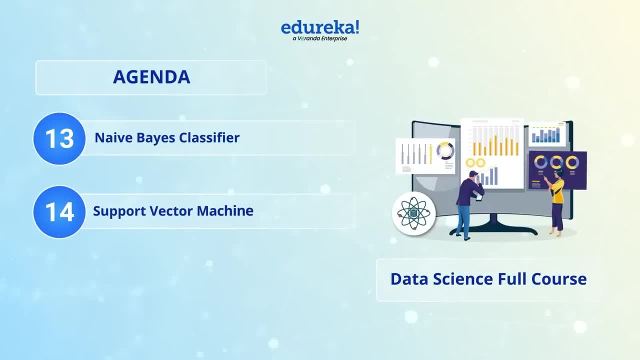 Algorithm, Naive, Bayes, Classifier, Support, Vector Machine, K-Means, Clustering Algorithm, Pre-Priori Algorithm, Reinforcement Learning, Q-Learning, etc. Now I know this list looks intimidating, but trust me, we'll ease you in And guess what? 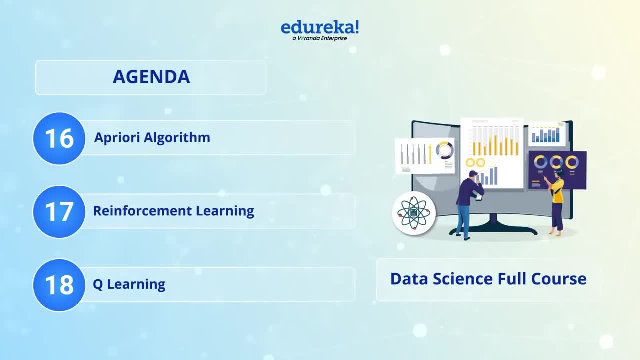 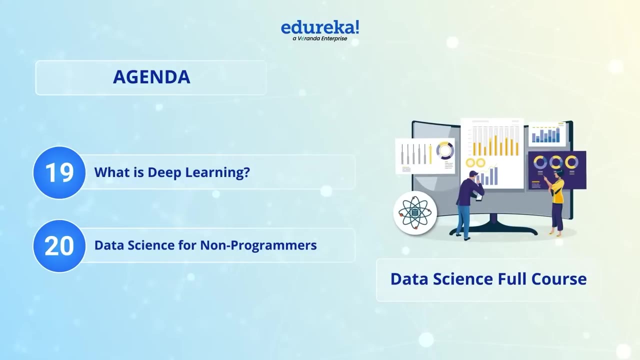 we're still not done. After learning all these algorithms, we'll discuss what is deep learning. Next, we have data science for non-programmers. This answers most of the questions that non-programmers have on data science. Now, after all this, we really do hope that you build a successful 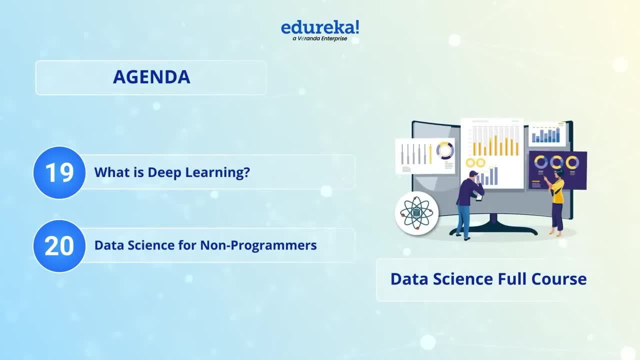 career in this domain. For that reason, we have included two bonus sections. This includes content on how data scientists should create their resume, and data science interview questions and answers. So let's not waste any more time and get started with the first section. 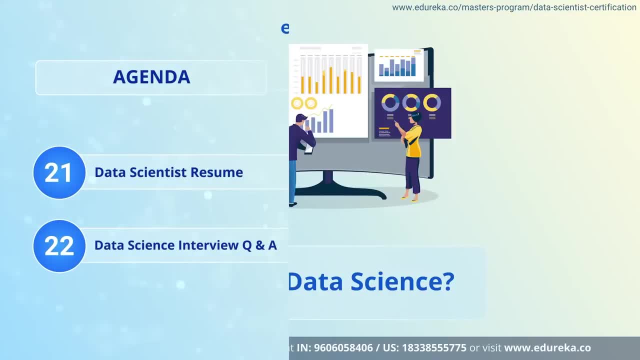 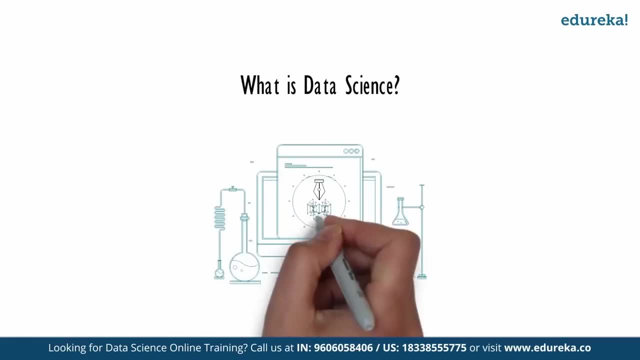 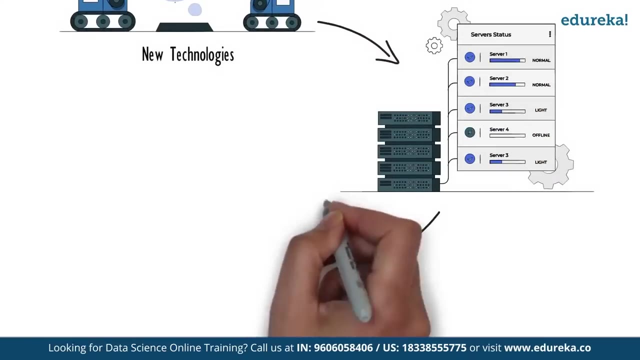 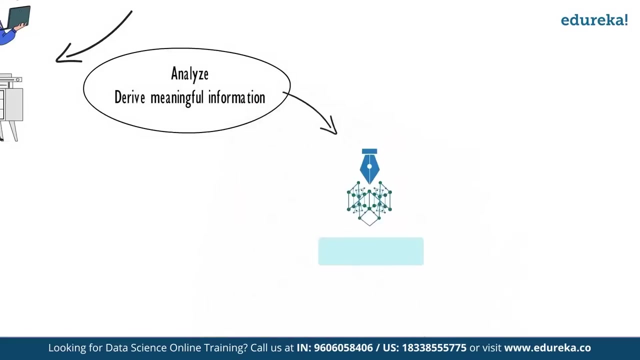 which is what is data science. What is data science? With the development of new technologies, there has been a rapid increase in the amount of data. This has created an opportunity to analyze and derive meaningful information from all this data. This is where data science comes into the picture. Technically, data 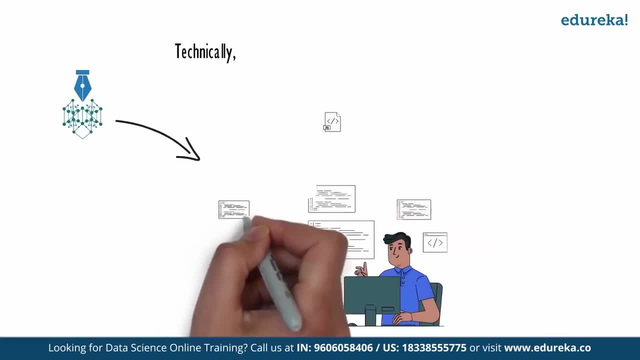 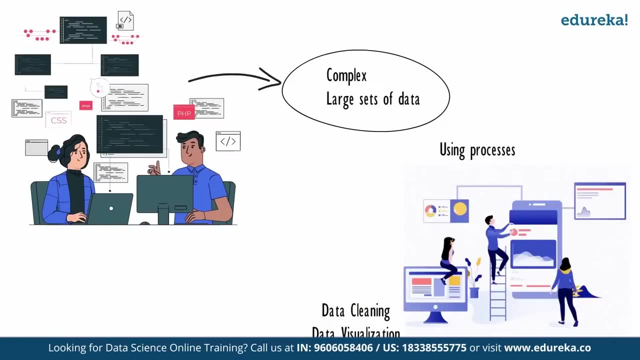 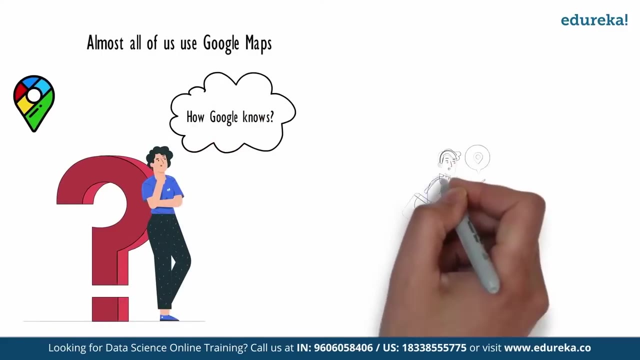 science is defined as the process of extracting knowledge and insights from complex and large sets of data by using processes like data cleaning, data visualization. Almost all of us use Google Maps, But have you ever wondered how Google knows the traffic conditions between where you are? 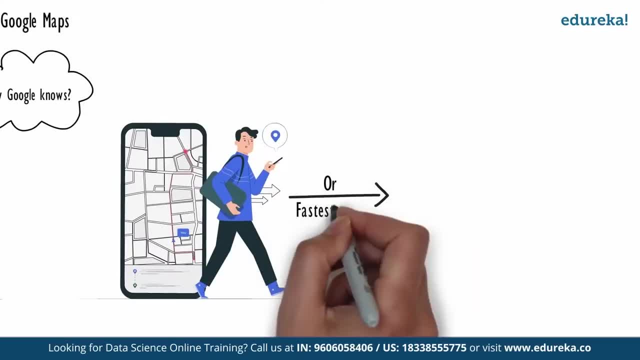 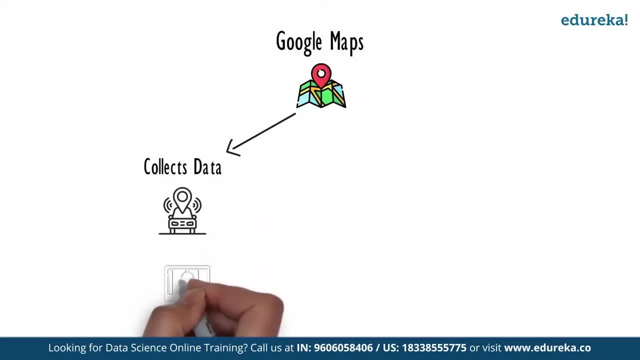 and where you're trying to go, Or how does it determine the fastest way to your destination? The answer is data science. Google Maps collects data every day from a multitude of reliable sources. that primarily includes smartphones. It continuously combines the data from drivers. 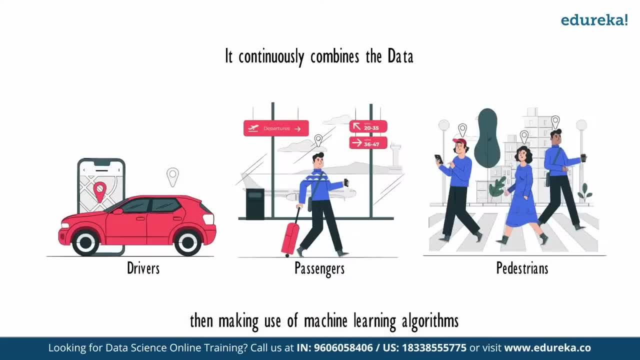 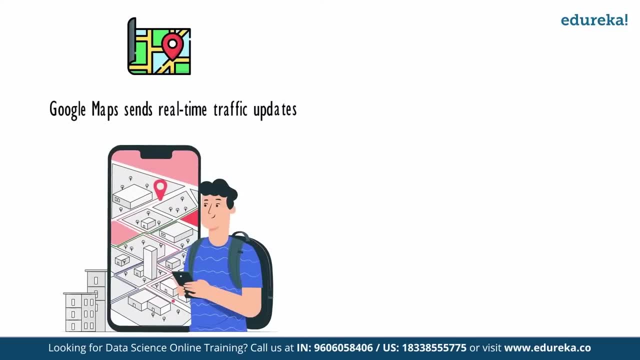 passengers and pedestrians, And then, making use of machine learning algorithms, Google Maps sends real traffic updates by way of colored lines on the traffic layers. This helps you find your optimal route and even determine which areas should be avoided due to roadwork or accidents. Isn't that amazing? 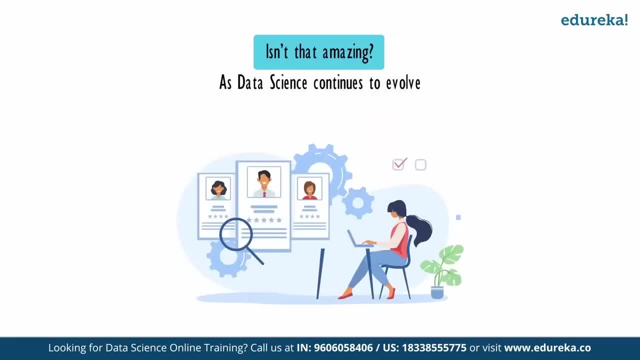 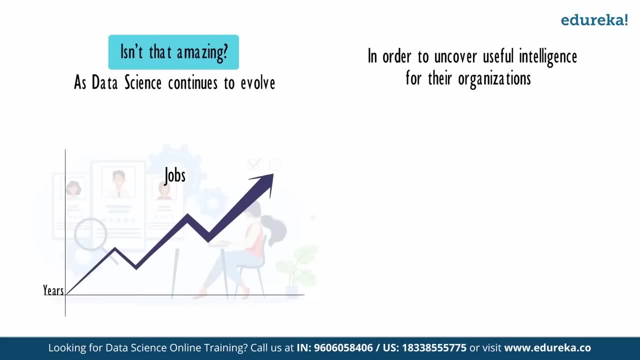 As data science continues to evolve, the demand for skilled professionals in this domain is also increasing drastically. In order to uncover useful intelligence for their organizations, data scientists must master all the skills they have acquired in the field of data science. So what is data science? 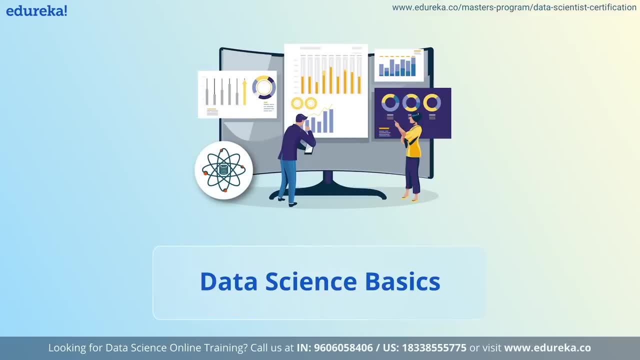 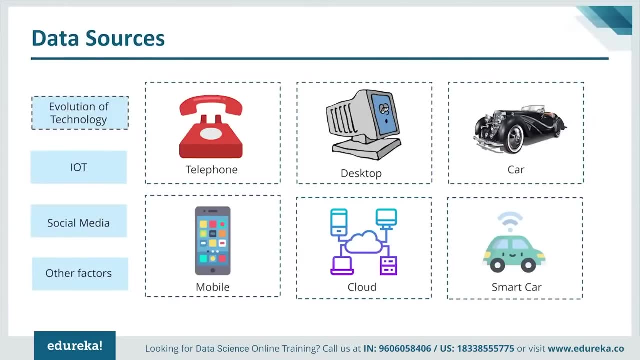 Do you guys remember the times when we had telephones and we had to go to PCO booths in order to make a phone call? Now, those times were very simple because we didn't generate a lot of data. But these days we have smartphones which store a lot of data. So there's everything. 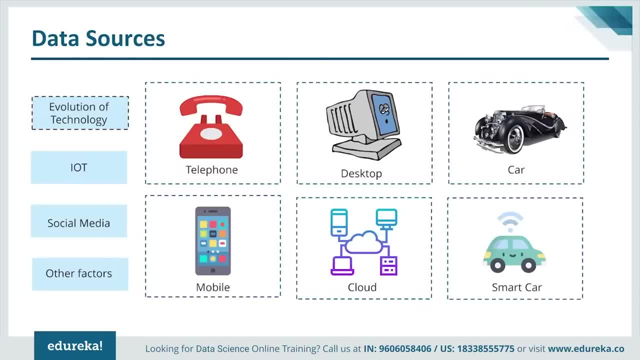 about us in our mobile phones, Similarly the PCs that we use. in the earlier times it used to process very little data. all right, There was not a lot of data processing needed because technology wasn't evolved that much. So, if you guys remember, we used floppy disks back then and floppy disks was used to store. 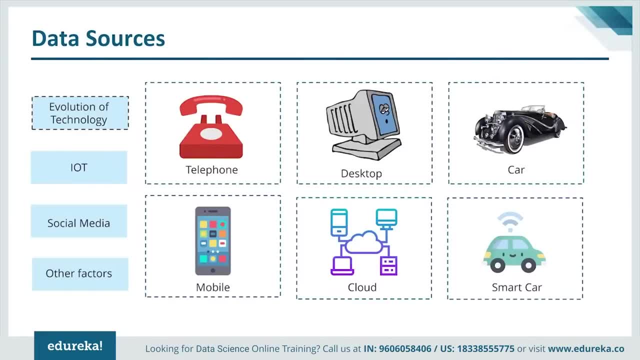 small amounts of data, But later on, hard disks were created and those used to store GBs of data. But now, if you look around, there's data everywhere around us. all right, We have data stored in the cloud. We have data in each and every appliance at our houses. 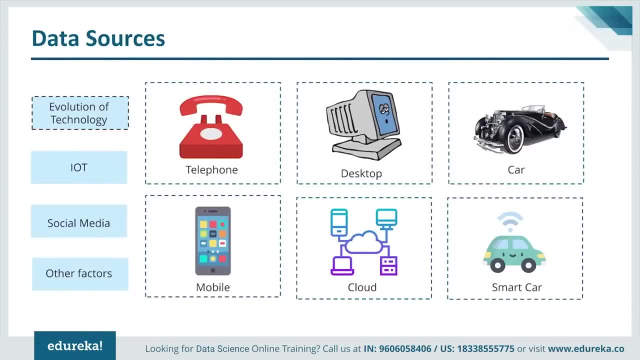 Similarly, if you look at smart cars, these days they're connected to the internet, they're connected to our mobile phones And this also generates a lot of data. In order to process this much data, we need more complex algorithms. We need a better 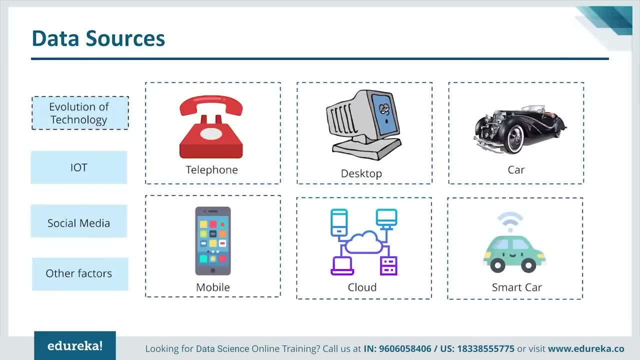 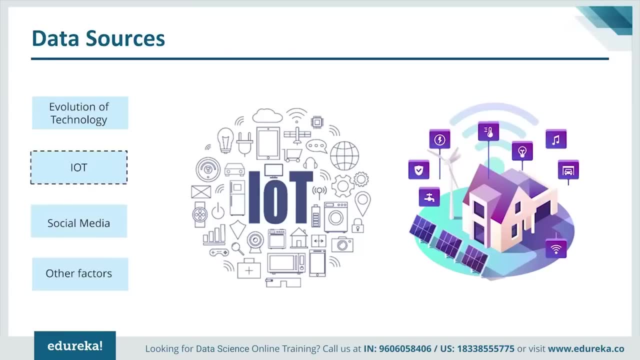 process all right, And this is where data science comes in Now. IoT or Internet of Things is just a fancy term that we use for network of tools or devices that communicate and transfer data through the internet. Guys, IoT data is measured in zettabytes And one. 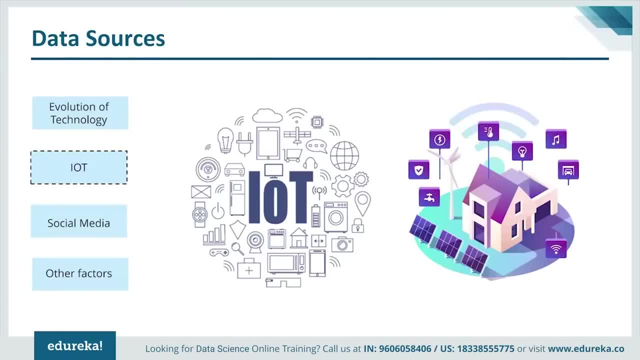 zettabyte is equal to trillion gigabytes. So according to a recent survey by Cisco, which is almost here, the IoT will generate more than 500 zettabytes of data per year. Moving on, let's see how social media is adding on to the generation of data. Now the fact. 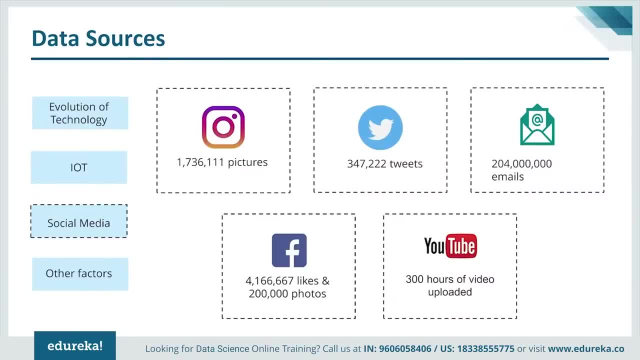 that we are all in love with social media. it's actually generating a lot of data for us. okay, It's certainly one of the fuels for data creation. Now, all these numbers that you see on the screen are generated every minute of the day. 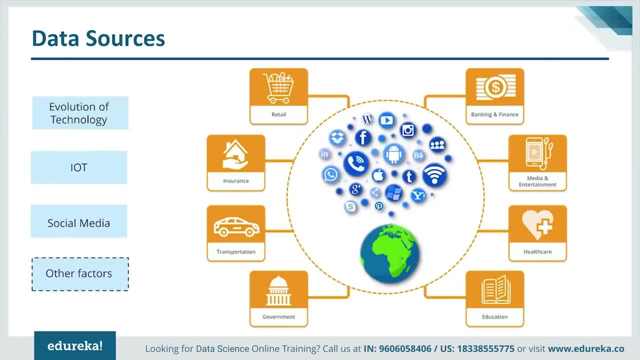 Now, guys, apart from social media and IoT, there are other factors as well which contribute to data generation. These days, all our transactions are done online, right? We pay bills online, we shop online, we even buy homes online. these days, You can even sell your pets on OLX. these 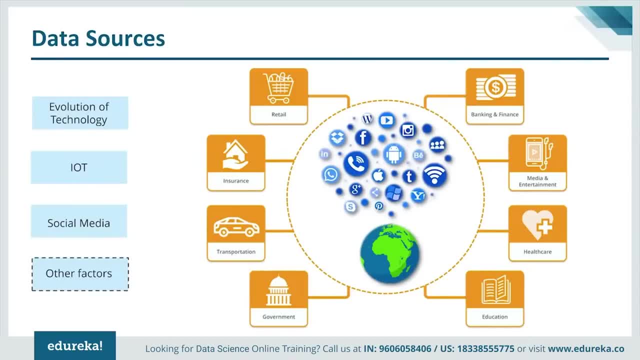 days, Not only that, when we stream music and we watch videos on YouTube. all of this is generating a lot of data. So, with the emergence of the internet, we now perform all our activities online. okay, Obviously this is helping us, but we are unaware of 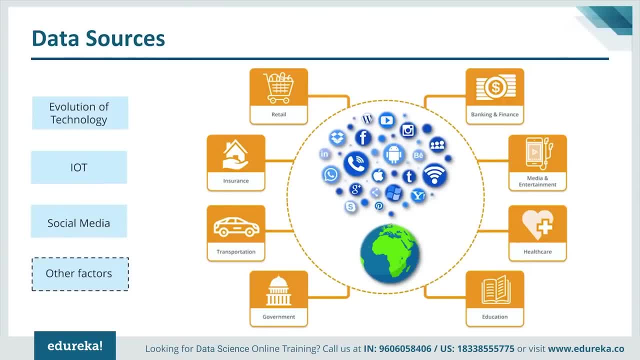 how much data we are generating, What can be done with all of this data And what if we could use the data that we generated to our benefit. Well, that's exactly what data science does. Data science is all about extracting the useful insights from. 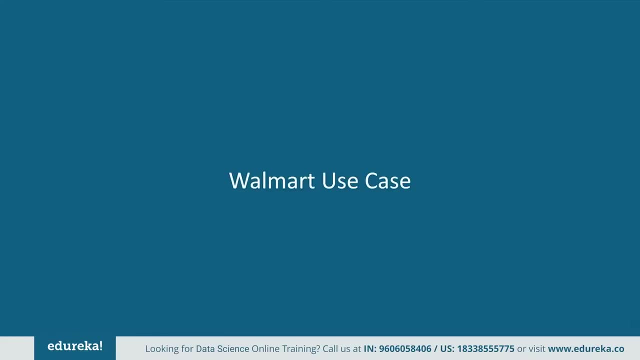 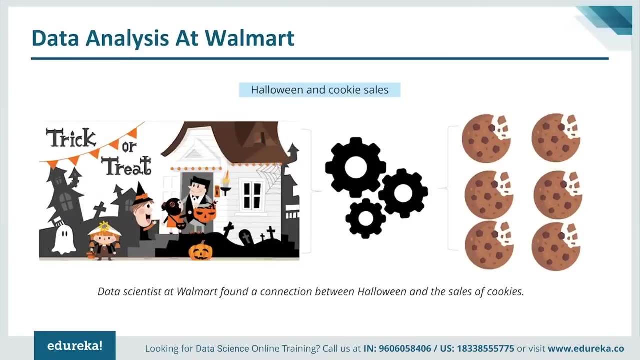 data and using it to grow your business. Now, before we get into the details of data science, let's see how Walmart uses data science to grow their business. So, guys, Walmart is the world's biggest retailer, with over 20,000 stores in just 28 countries. Okay, now it's. currently building the world's biggest private clothing store in the United States. Now it's currently building the world's biggest private clothing store in the United States. Let's have a look at the data science industry, So let's get started with this first thing. 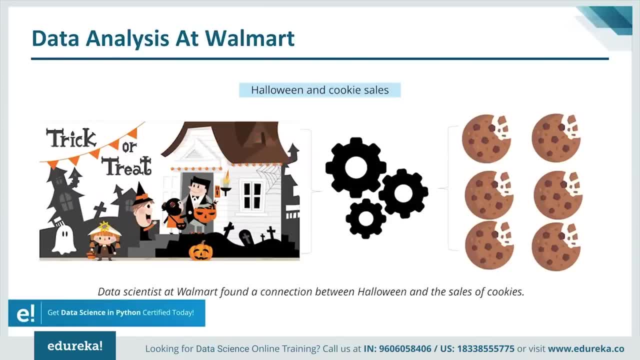 This is the Cloud which will be able to process 2.5 petabytes of data every hour. Now, the reason behind Walmart's success is how they use the customer data to get useful insights about customers' shopping patterns. Now the data analysts and the data scientists at Walmart- 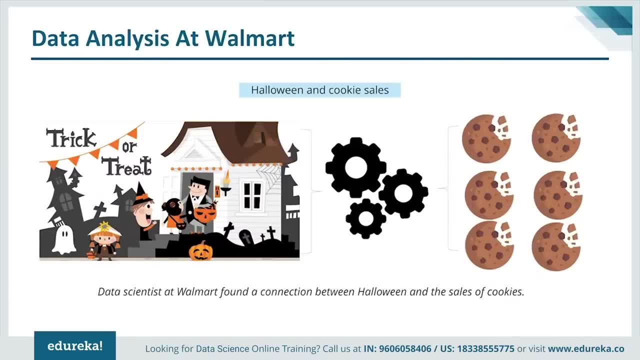 they know every detail about their customers. They know that if a customer buys Pop-Tarts, they might also buy cookies. How do they know all of this, Like? how do they generate information like this? Now they use the data that they get from their customers and they know all. 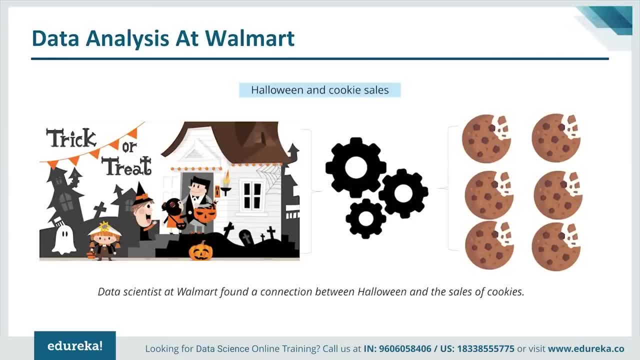 customers and they analyze it to see what a particular customer is looking for. Now let's look at a few cases where Walmart actually analyzed the data and they figured out the customer needs. So let's consider the Halloween and the cookie sales example. Now, during Halloween, sales analyst. 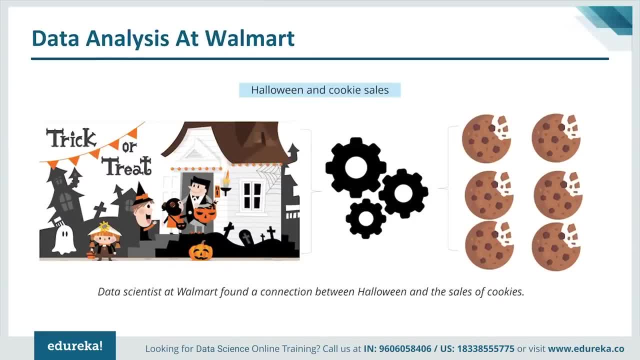 at Walmart took a look at the data, okay, and he found out that a specific cookie was popular across all Walmart stores, So every Walmart store was selling these cookies very well, but he found out that there were two stores which were not selling them at all. Okay, so the situation was immediately. 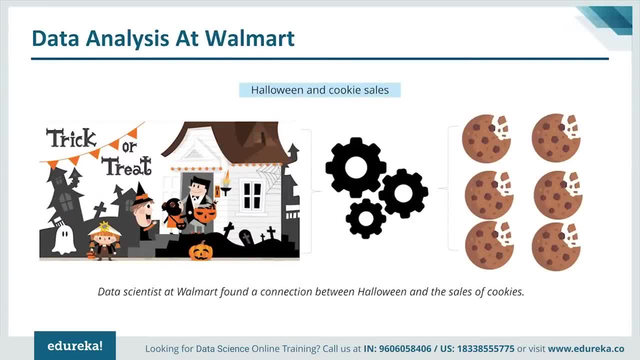 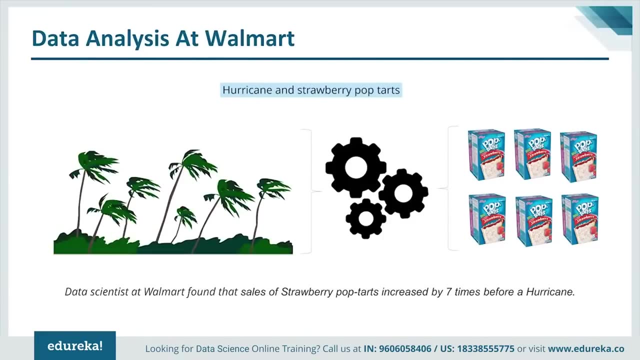 investigated and it was found that there was a simple stocking oversight okay, because of which the cookies were not put on the shelves for sale. So, because this issue was immediately identified, they prevented any further loss of sales. Now, another such example is that, through association rule mining, Walmart found out that strawberry pop tart sales increased by seven times before a 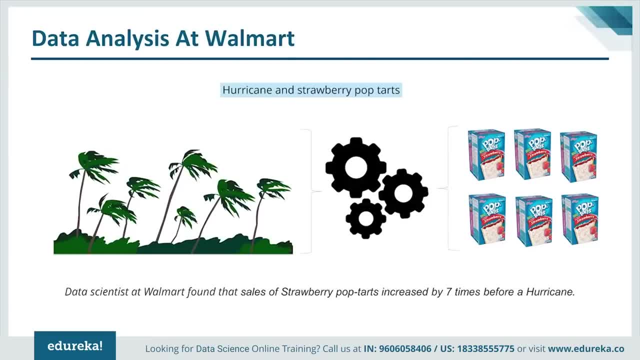 hurricane. So a data analyst at Walmart found out that strawberry pop tart sales increased by seven times before a hurricane, and Walmart identified the association between hurricane and strawberry pop tarts through data mining. Now guys, don't ask me the relationship between pop tarts and hurricane. 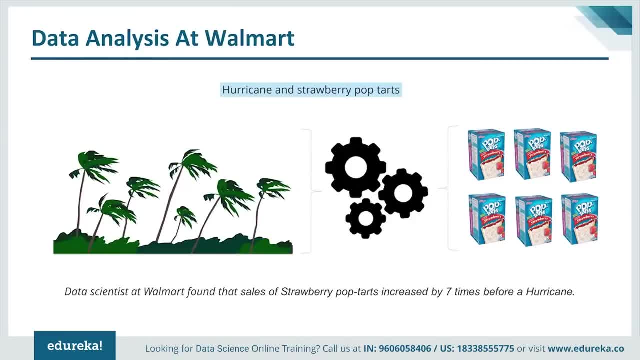 but for some reason, whenever there was a hurricane approaching, people really wanted to eat strawberry pop tart. So what Walmart did was they placed all the strawberry pop tarts as a checkout before a hurricane would occur. So this way, they increased sales of their pop tarts. Now, guys, this 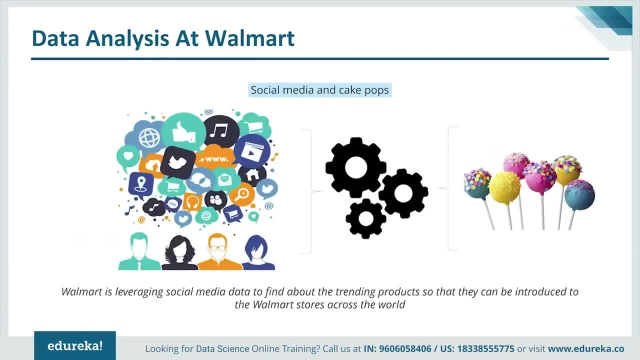 is an actual thing. I'm not making it up. you can look it up on the internet. Not only that, Walmart is analyzing the data generated by social media to find out all the trending products. So, through social media, you can find out the likes and dislikes of a person, right? So what Walmart did? 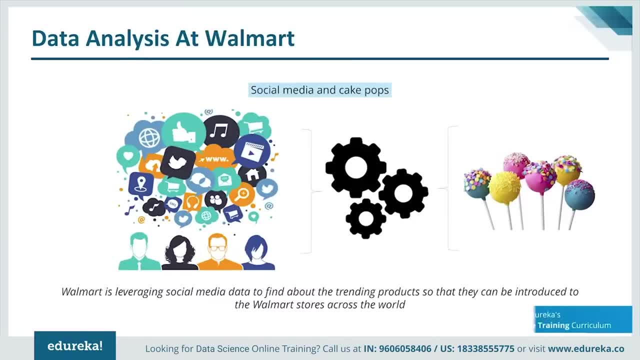 is they're quite smart. they use the data generated by social media to find out what products are trending or what products are liked by customers. Okay, an example of this is Walmart. analyzed social media data to find out that Facebook users were crazy about cake pops. Okay, so Walmart immediately. 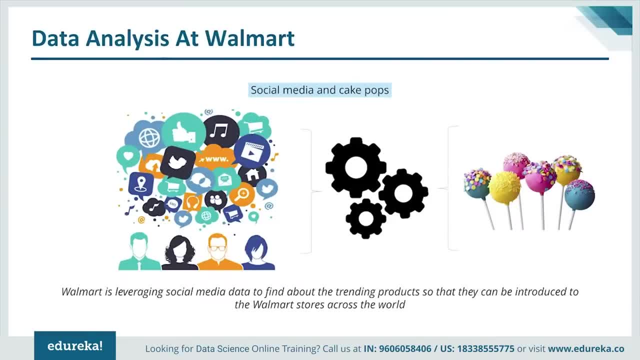 took a decision and they introduced cake pops into the Walmart stores. So, guys, the only reason Walmart is so successful is because the huge amount of data that they get, they don't see it as a burden. Instead, they process this data, analyze it and then they try to draw useful insights from it. Okay, so they invest a lot of money, a lot of effort. 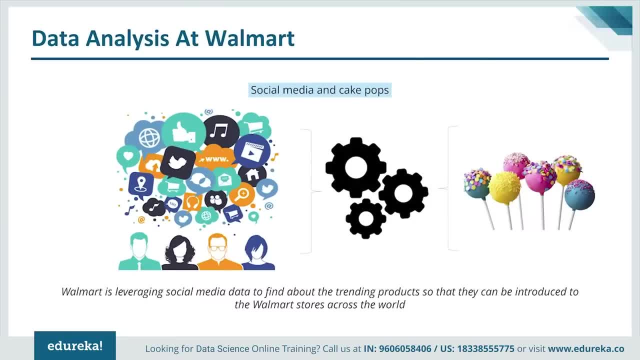 and a lot of time in data analysis. Okay, they spend a lot of time analyzing data in order to find any hidden patterns. So as soon as they find out hidden pattern or association between any two products, they start giving out offers or they start giving discounts or something along that line. 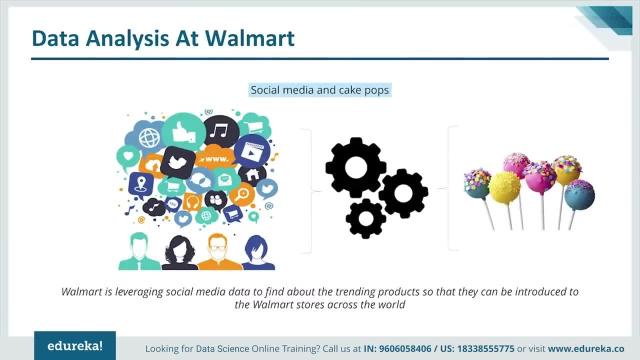 So, basically, Walmart uses data in a very effective manner. They analyze it very well, they process the data very well and they find out the useful insights that they need in order to get more customers or in order to improve their business. So, guys, this was all about how Walmart uses data. 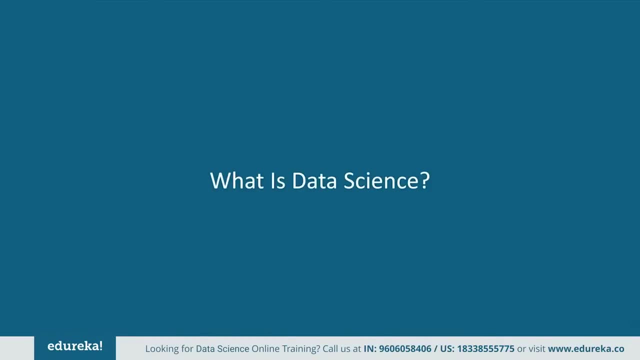 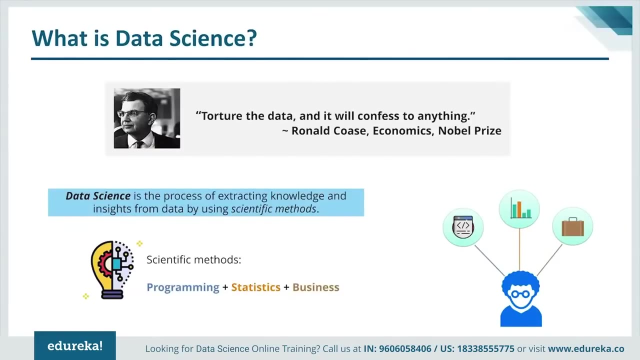 science. Now let's move ahead and look at what is data science. Now, guys. data science is all about uncovering findings from data. It's all about surface science. It's all about data science. It's all about using the hidden insights that can help companies to make smart business decisions. So all these 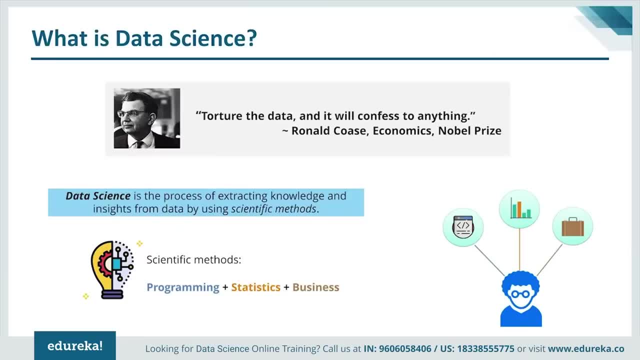 hidden insights, or these hidden patterns, can be used to make better decisions in a business. Now, an example of this is also Netflix. So Netflix basically analyzes the movie viewing patterns of users to understand what drives user interest and to see what users want to watch. And then, once they 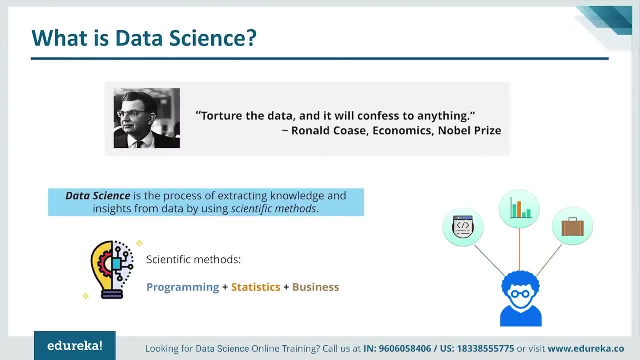 find out, they give people what they want. So, guys, actually data has a lot of power. You should just follownyt to mobile phones. Sometimes you can even find out the best ways to uncover data using data science, So perhaps you can imagine a simple, continually following the insights that Google. 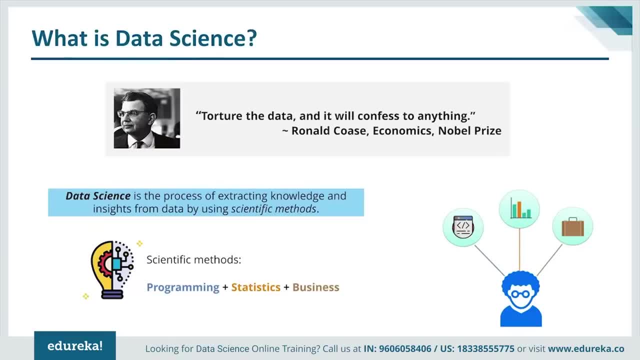 shows you. It can even give you better information. Maybe you don't even know the exact Christ called CPR or what's called insights. So how this is how this whole thing can be done in digital- is data science. What's this kind of split blend using data science? So these are called Data science. 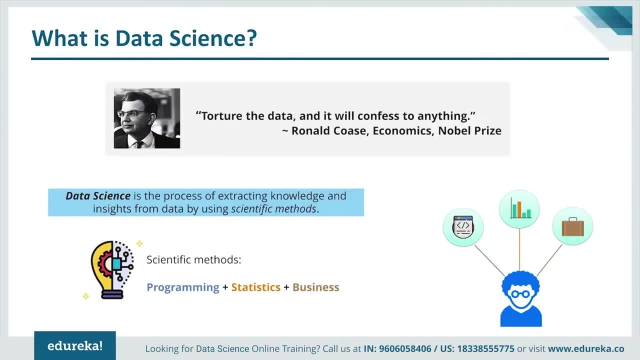 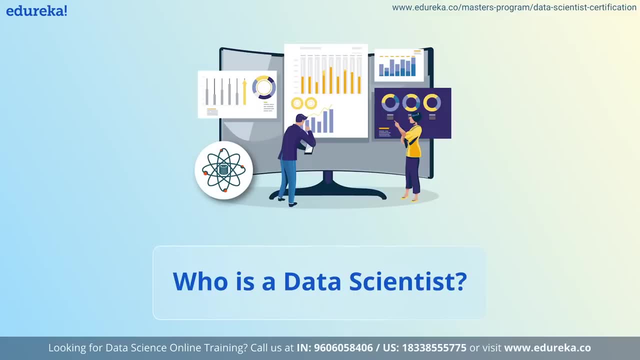 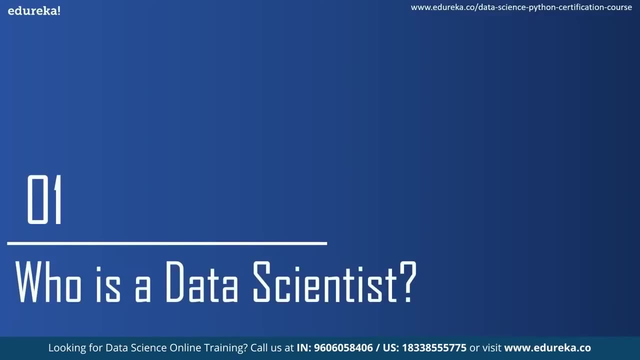 and i'm sure that you're familiar with Data science, Data science right. So you have to do all the information that they can from the data and then they use it for the betterment of the organization or the business. Now let's get started and understand who is a data scientist. 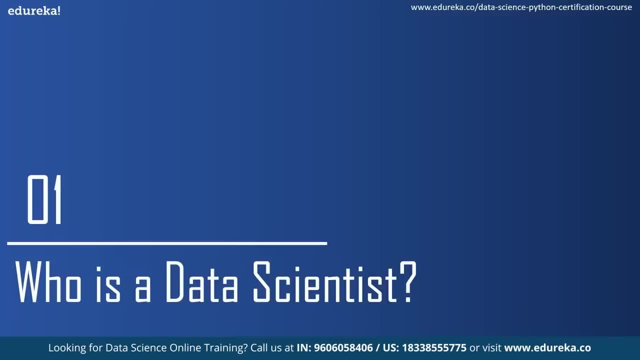 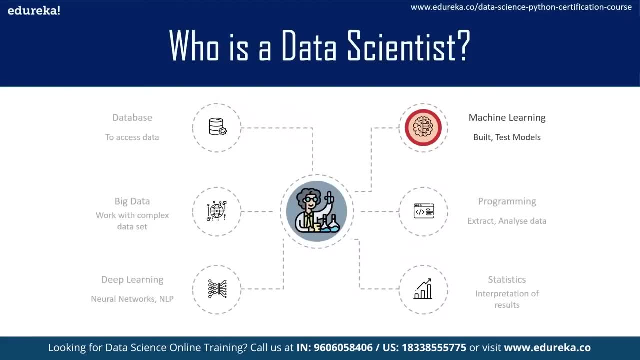 Well, when the term scientist comes to our mind, the first thing is experiments. So scientists are related with experiments and a data scientist is related with data and experimenting with that data. So a data scientist is someone who experiments with data and has certain tools and 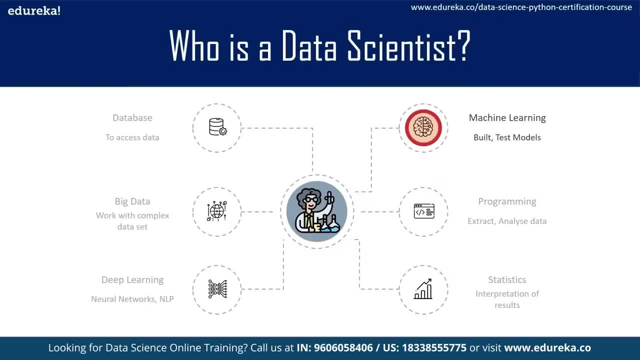 technologies at his disposal to draw insights and meaningful patterns from this data. So these tools and technologies have been listed here and we will cover first machine learning. Now, this machine learning is very important tool for a data scientist to build and test models. Also another. 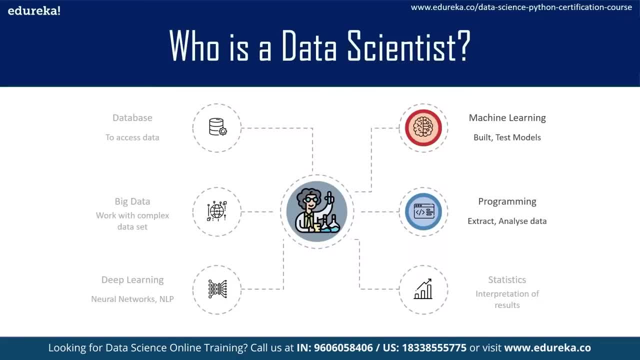 tool is programming language to extract, analyze and manipulate the data. A data scientist also uses yet another important tool And that is statistics. So now statistics is used to make predictive analysis, to understand and interpret the results from the data. So statistics is really important tool for a data 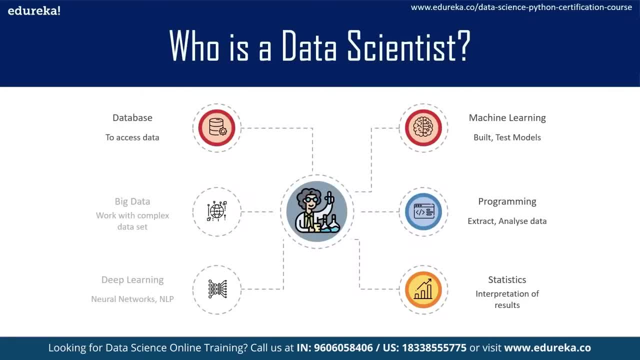 scientist. So another tool is database. So database is yet another important tool, which means to access the data. Yet another tool is big data to work with complex data set, and big data technologies are really required now in a data scientist. We will cover all these technologies in detail in the 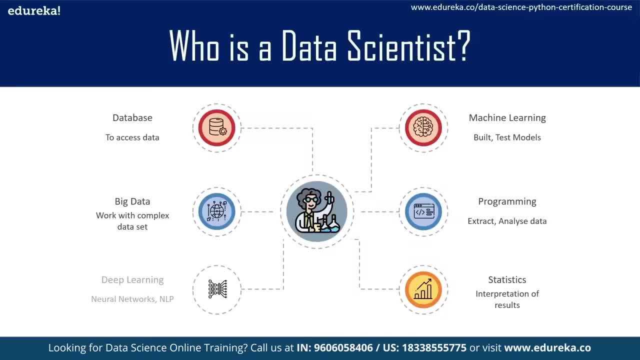 coming up slides. Be patient a little. And this is just a coverage of giving you a brief gist of the tools and technology techniques. So another technique is deep learning. So a data scientist is also required to have the knowledge of neural networks, NLP, to draw meaningful insights from. 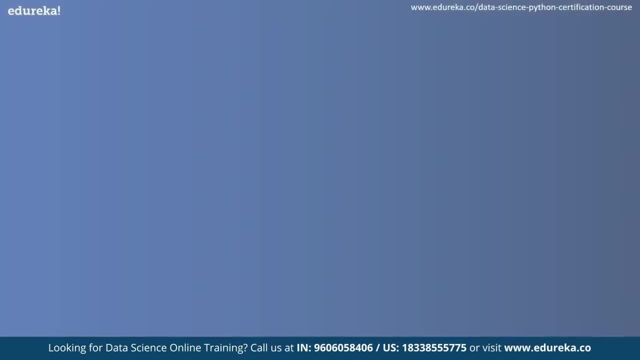 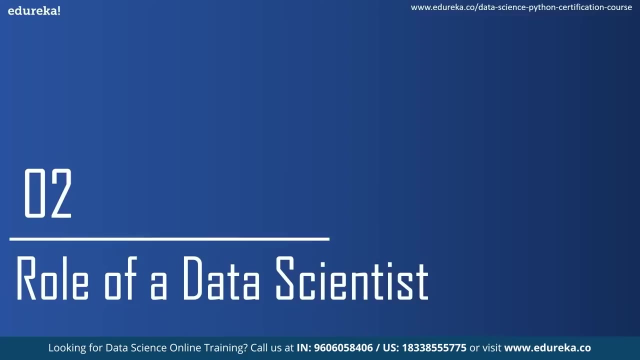 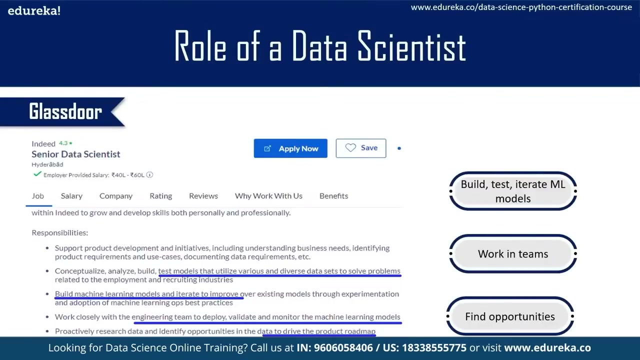 unstructured data and also to process such data. Now let's move on to discussing about the role of a data scientist. So what exactly does a data scientist do, And this will be clear once we go through a few job responsibilities of a data scientist. Now this data has been taken from: 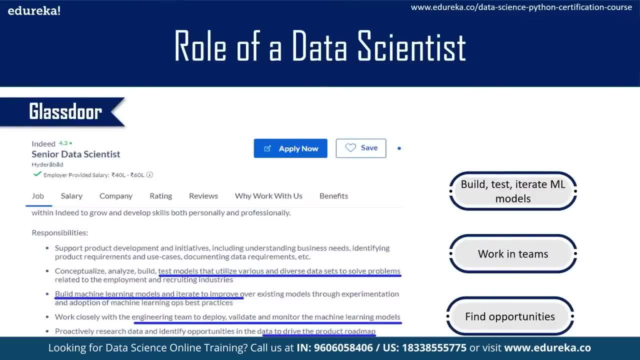 Glassdoor. So let us look at the role that a data scientist needs to perform And, as you can see in the right hand side, just the gist of the role is being listed. So a data scientist is required to build and test and iterate on the machine learning model. So we've already covered the machine. 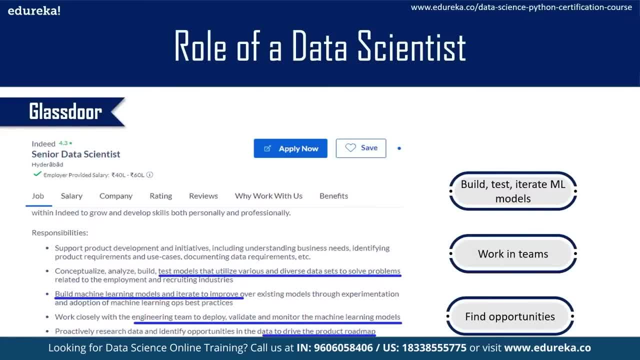 learning is the indispensable tool of a data scientist. So iteration requires a lot of repetition, Repetitive experiments with the data, and it is quite a complex process- and repartition is done to improve the results of the models. So a data scientist is really required to iterate again and 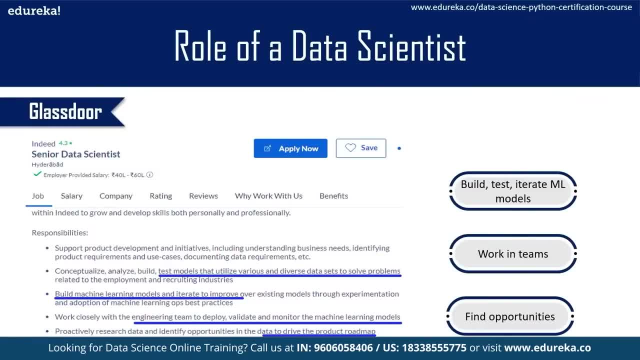 again with the machine learning models, although the billing part is not so much, because already the companies are working under predefined, predesigned coded softwares. So testing an iteration becomes the indispensable part of a data scientist. Now another role if we look at here. 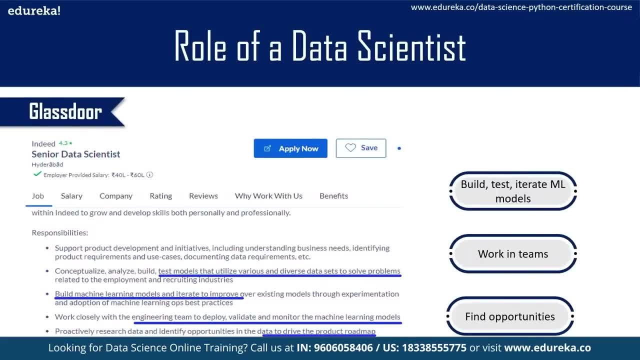 is that they're working in teams, So working in team with the engineer team to deploy, validate and monitor the machine learning models. so this is very important, because once a model goes to the production state, so you have to monitor it and also you have to undertake the deployment of it. how to? 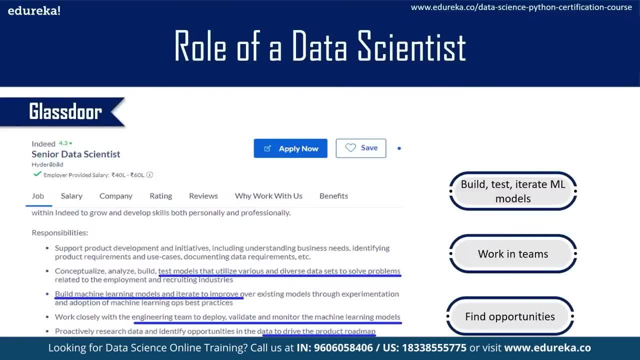 really connect it with the front end and see how is it really working, what accuracy is it giving. and then, most importantly, a data scientist is required to research data, identify opportunities now. this means that drawing useful insights from the data by using various techniques, as we have seen earlier. so a 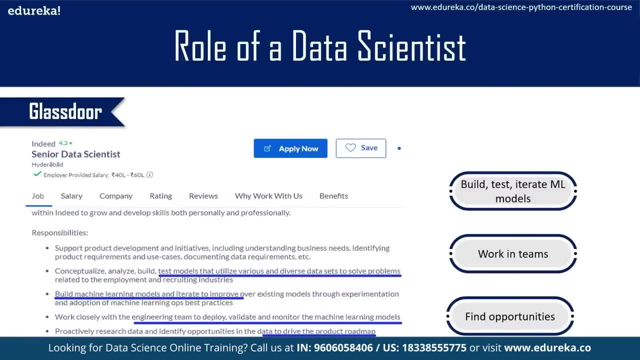 data scientist applies all these techniques together to draw meaningful insights from the data. and now let us understand what all to learn to become a data scientist, so that this role is suited for a data scientist and one can perform this very well. so the technologies to learn for a data: 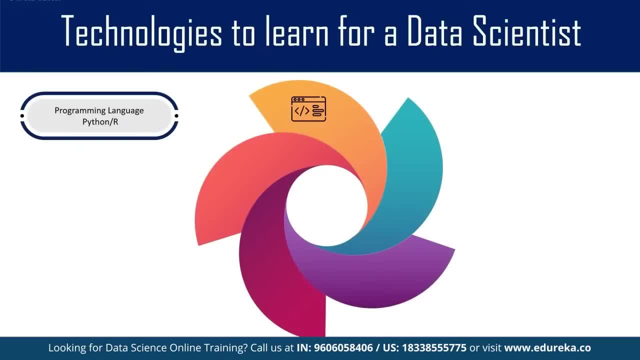 scientist are programming language. it could be either Python or R, machine learning, deep learning and NLP concepts, which need to be really very clear. you can use a lot of different technologies to learn and solid foundation of the same another technology to learn a statistics that is both descriptive and 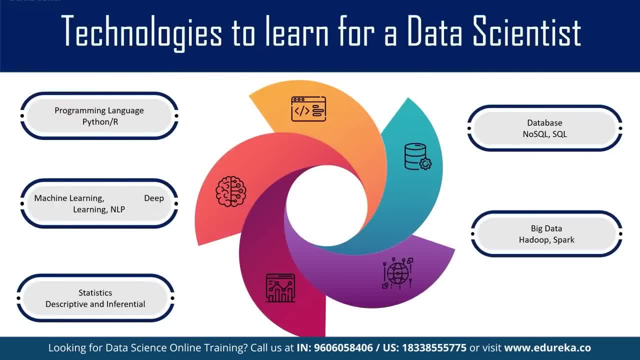 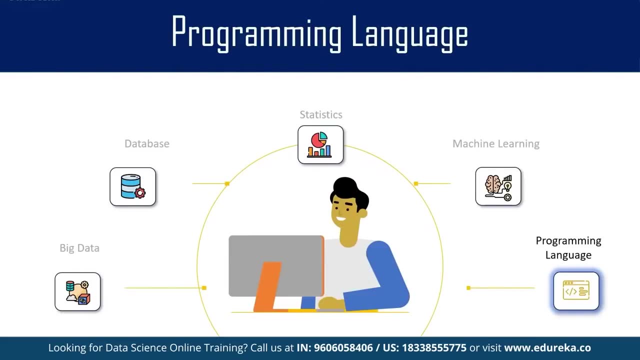 inferential. another technology is database knowledge of sequel and no sequel, and big data. big data, the knowledge of Hadoop, spark- any one of them is required. so now let's cover these technologies in detail. now, moving on forward to the programming language. now why a programming language is really. 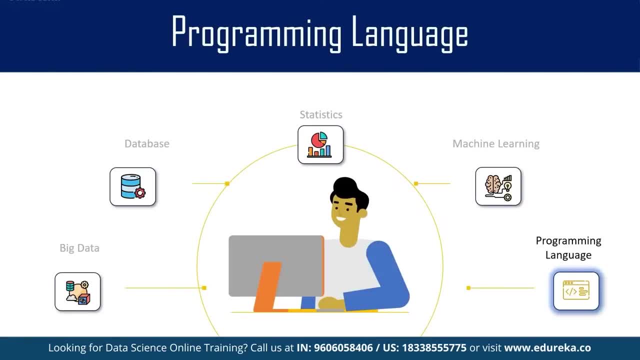 required by a data scientist is to analyze huge volumes of data and also to before 커�- medias of the need to perform analysis of the data. so programming language really each in better analysis, manipulation of the data. so programming language: generally used our Python, R, Scala or Java, but generally 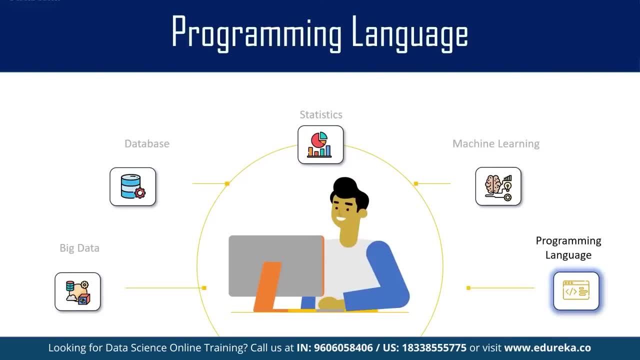 preferred is Python and is the most popular language which is now being used in the data science community. R is also there, but on the production side it becomes little tough, okay, so now we will cover what the languages and the important libraries to study for these languages. so now moving on forward to 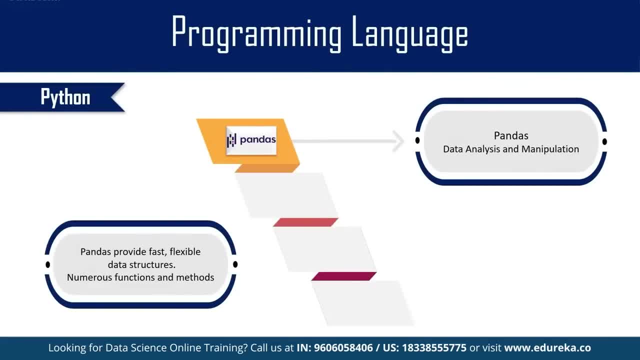 programming language Python. So in Python, what all needs to be covered? First library is Pandas. Now, this library is very important because this is used for data analysis and manipulation, and Pandas also provide very fast, flexible data structures. This means that numerous functions and methods are available in 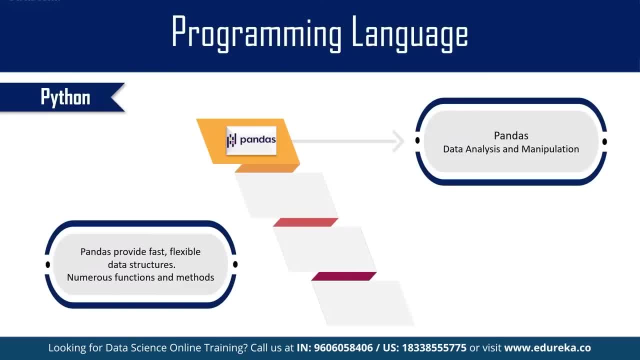 Pandas, which allows you to perform data analysis and manipulation of the data very quickly and very fast, and time series analysis is also possible with the help of Pandas. So the examples like when you're forecasting, when you're forecasting weather predictions or stock prices predictions, or houses predictions- 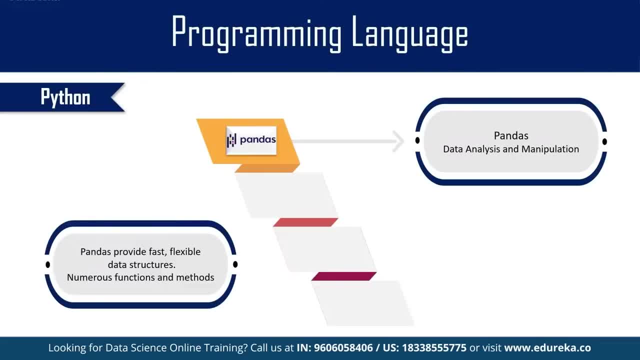 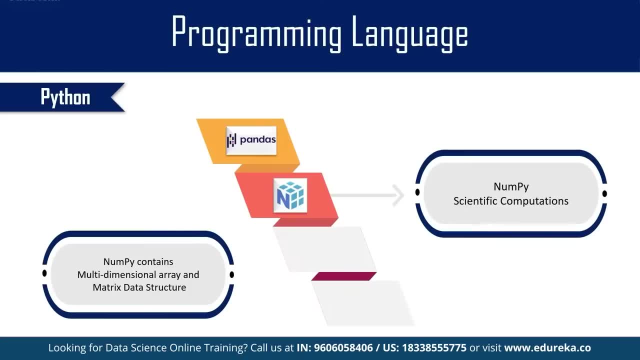 then Pandas really help, you know, in data analysis and manipulation. So that's an example of that. Now coming to NumPy, This is another library which is numerical Python, and this is used for scientific computations. Now, numerical calculation and machine learning is done with the help of NumPy, and this is the 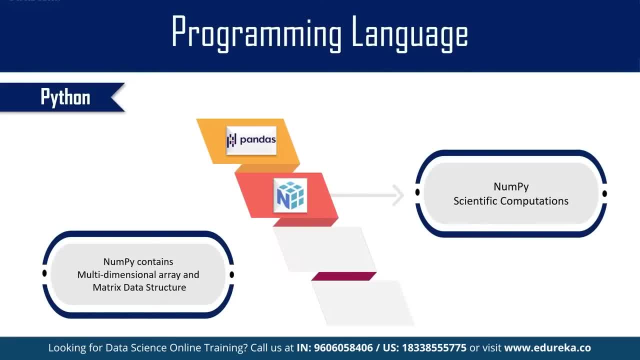 foundation, I would say the building block, of Python, And all the calculations, mathematical calculations, scientific computations, is possible because of NumPy, and NumPy contains multi-dimensional array and matrix data structure. With these powerful data structures one can really perform efficient calculations in Python. Alright, now, moving on forward, we have 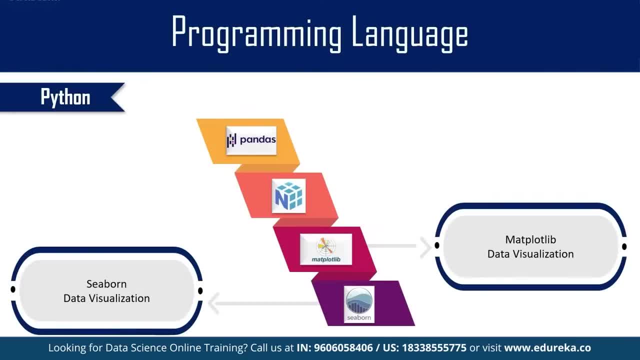 the visualization libraries, like Seaborn and Mathplotlib. These two libraries are used for visualizing the plots, looking at the spread of the data and seeing how does the data look like, Whether are there any outliers or what is the spread of the data. Is it? 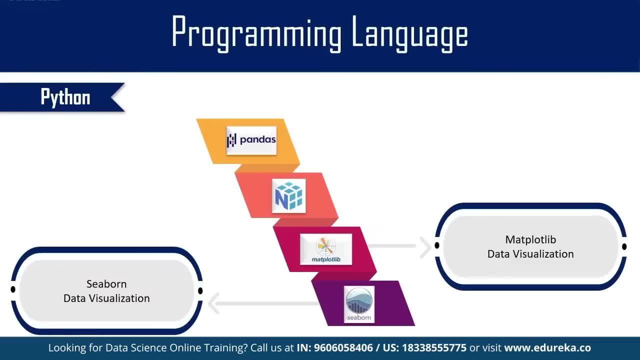 normally distributed or it is only unevenly distributed. So these visualization libraries really help us to visualize the data. And also another thing is that Seaborn is built over Mathplotlib. That means that it derives functionality methods from Mathplotlib, but offers more flexibility in 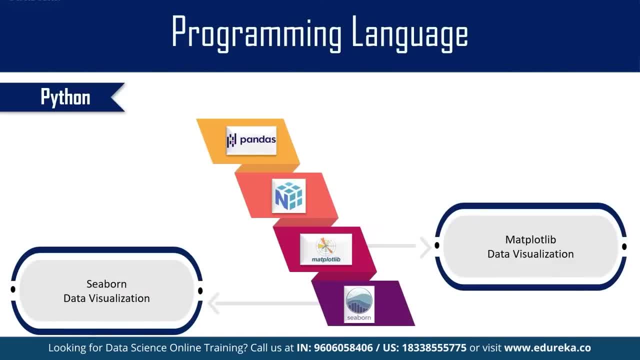 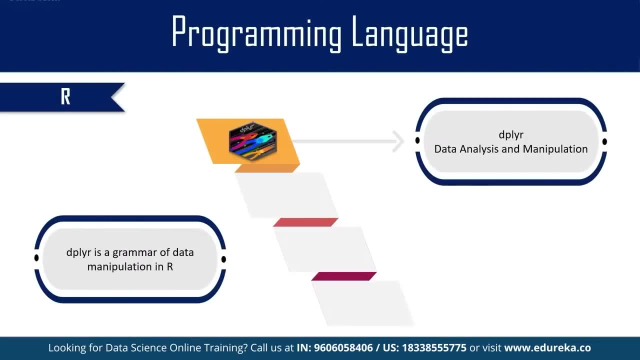 terms of plotting the graphs and better representation in terms of color, and aesthetically beautiful plots can be plotted with the help of Seaborn. So now we are moving forward to another language, which is R. So R is also preferred in the data science community, and data scientists work with R. R has 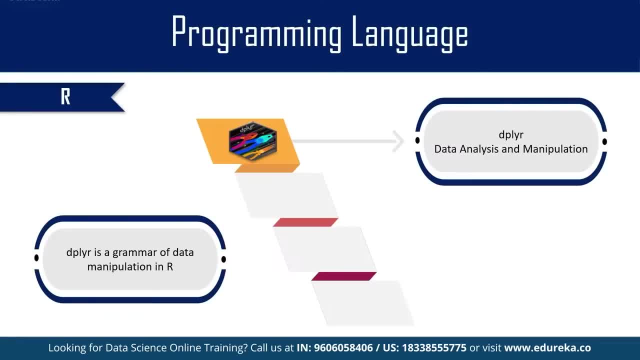 very strong statistical packages as it was developed by statisticians, and R is really good for data analysis. but when you take next step into machine learning, R has its limitations too, as we have discussed earlier also. So now for R. if you're using R, then we can use the plier package. Now this is used for data analysis and manipulation. 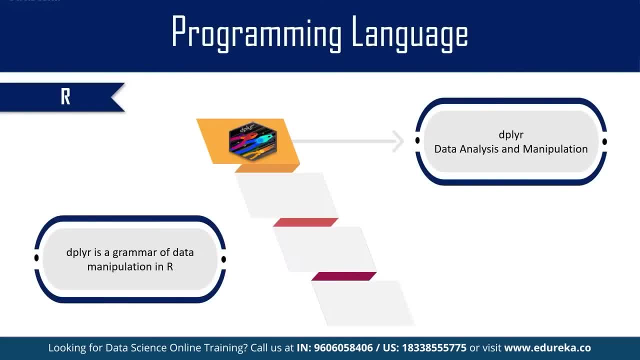 Now this is used for data analysis and manipulation. Now this is used for data analysis and manipulation And for the exploration of data. The plier is a very strong packet and it is a grammar of manipulation. This means that the plier provides us a consistent set of 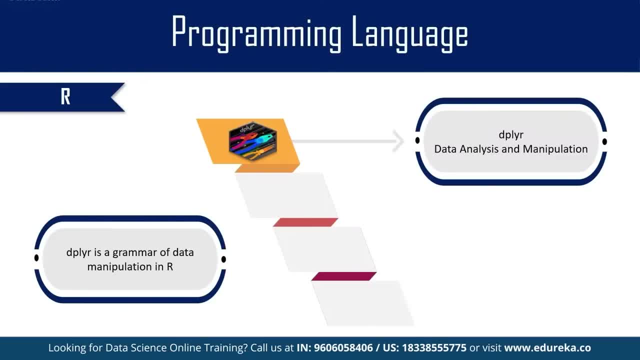 functions, Then these functions are called verbs. So R has a defined language and that language has to be preserved, so we use verbs here. So functions are called verbs here and they help to perform the manipulation on the data. So now, moving on forward, we have another package and that is janitor. Janitor is basically a. 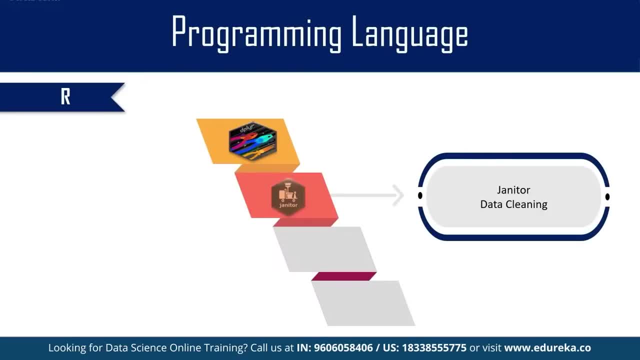 And this is used for data cleaning, like removing empty values or removing duplicates from your data, and so on. So one thing to note here is that data scientists really spend most of the time in data cleaning, in transforming the data, in just removing the missing values or empty values, or cleaning. 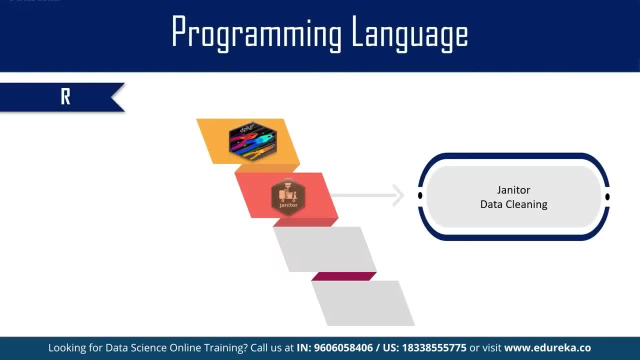 Cleaning is the most part that data scientists spend too. So these libraries can be really helpful when one is building models or one is working on various complex kind of data. So now, moving on further, to another library, that is LubriDate, And this LubriDate is for date and time manipulation in R. 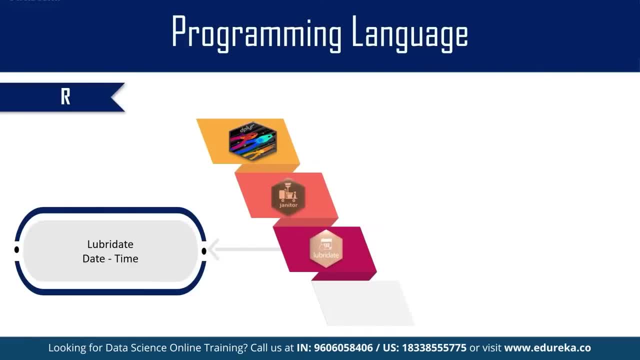 And for Python we have Pandas All right for date and time analysis And this really helps because it already has functions and methods predefined, which understands date and time analysis, and manipulation can be done very easily with the help of LubriDate. 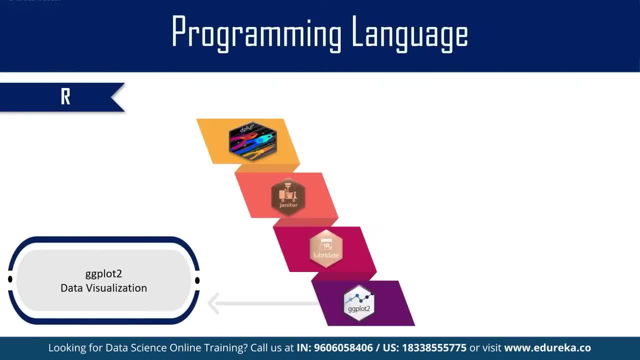 Now, another library that we would cover is ggplot2 for data visualization in R. Now, this gg stands for grammar of graphics. Now in R, ggplot2 is used to make the graphs, plots, and we work with layers in ggplot2.. 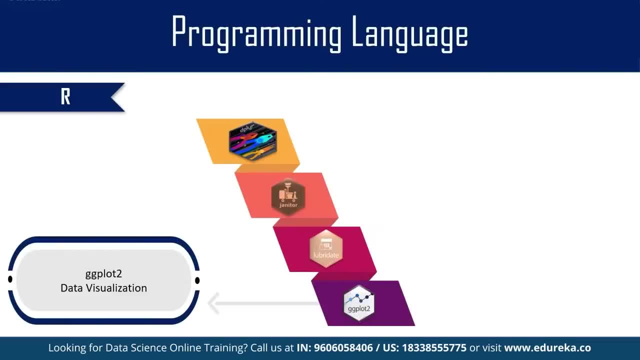 So, with the help of these layers, we can plot a very complex plot with the help of ggplot2.. And we can say that ggplot2 has very aesthetically appealing plots and it gives us the flexibility to show our data in various structures and various formats. 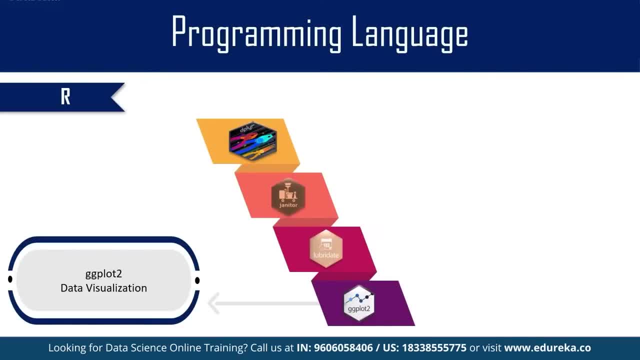 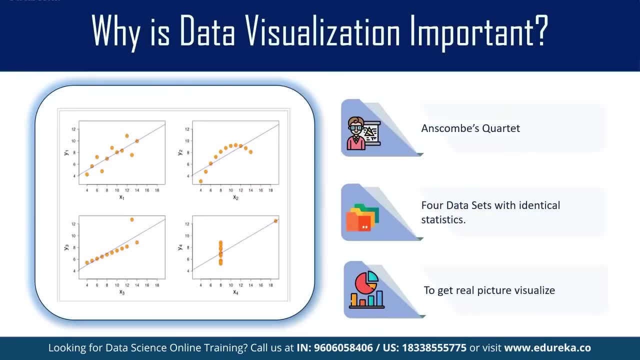 And we can always see what the data is. So we visualize the data with the help of ggplot2 in R. Now I want to tell you something really very interesting, as why is data visualization important? And now let us just uncover this thing. 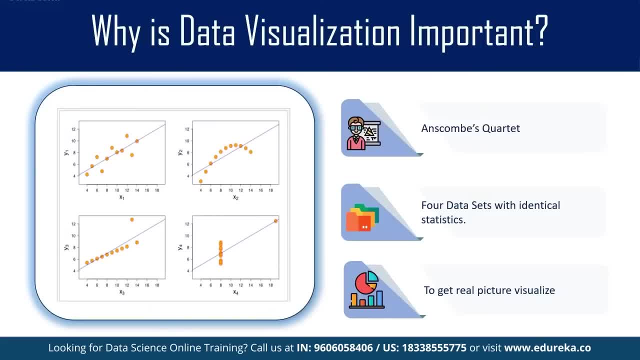 The significance of data visualization can be understood with the help of the image here on the left hand side, And this is known as Anscombe Quadrate. Now, Anscombe was an English mathematician and he developed this quadrate to demonstrate the importance of data visualization. 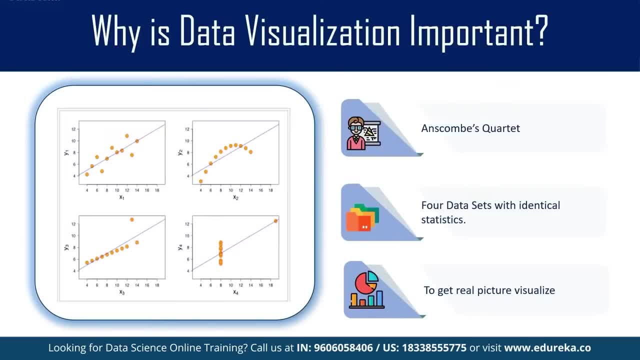 Now this comprises Of four, as we can see, four data sets, and these data sets have the same or identical, simple descriptive statistics. right, But when they were being plotted, we get different graphs of each data set. Now, this is the importance of visualization: that the numbers and figures will appear same, but when they are plotted they would be different. 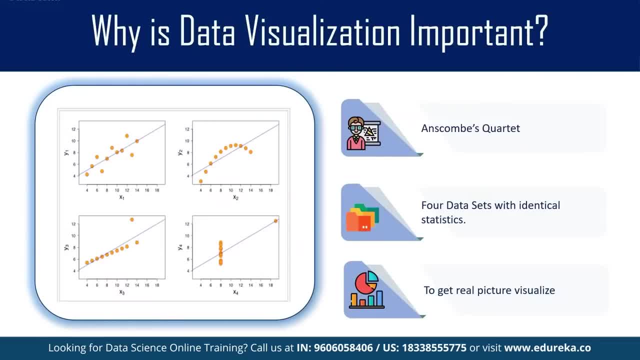 So to get the real picture and the meaning of your data, your data needs to be plotted to get the true picture, All right. So it's always been said that numbers will not reveal the true picture, but the, but the visualization of that data would definitely reveal it. 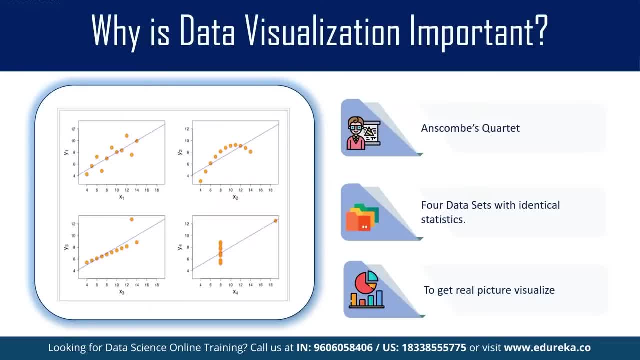 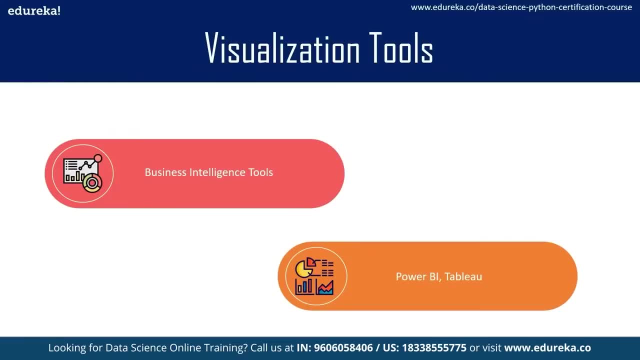 So this was a very important Anscombe Quadrate to visualize that rest data visualization. why is it really important? So, moving on further, linked with this is data visualization tools that a data scientist uses, and one can learn these tools. It could be very handy. 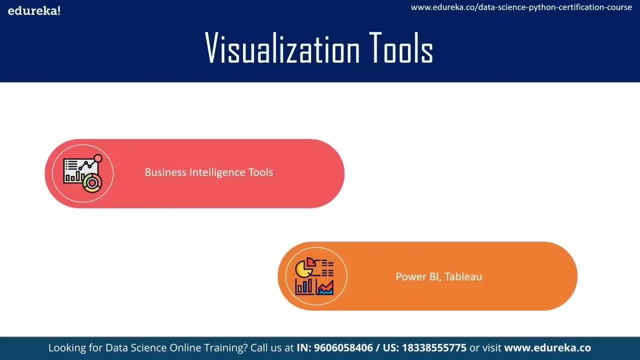 So few visualization tools or softwares are Now. these tools really help you to visualize large data sets. and these powerful softwares- They can connect with multiple data sources. in no time You can build dashboards, interactive dashboards, powerful visualization and even you can go on creating applications with these tools. 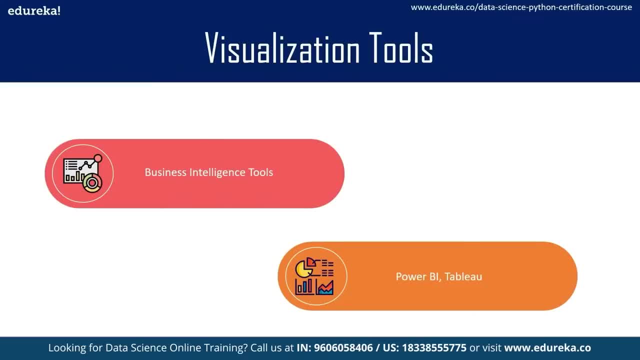 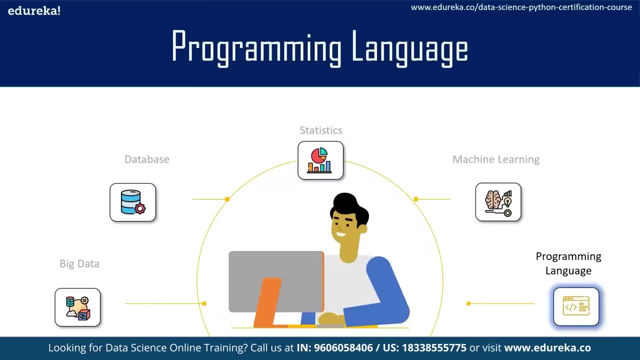 So business intelligence tools. knowledge is one of the requirements, but it is not that necessary. It's easy to learn and it's fun too. Okay, Now move coming on to another concept After programming language, and that is machine learning. Now, machine learning, this is the ability to understand algorithms, both supervised and unsupervised machine learning algorithm. 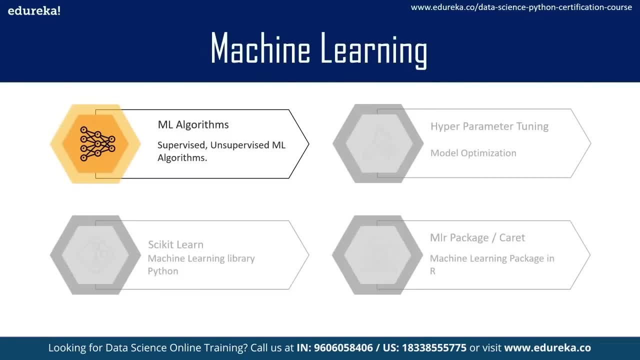 So now we will discuss about supervised- unsupervised machine learning algorithms. So supervised is something when we work with labeled data- that means the output is known- and unsupervised is when we don't know the output and the algorithm has to make a guess. 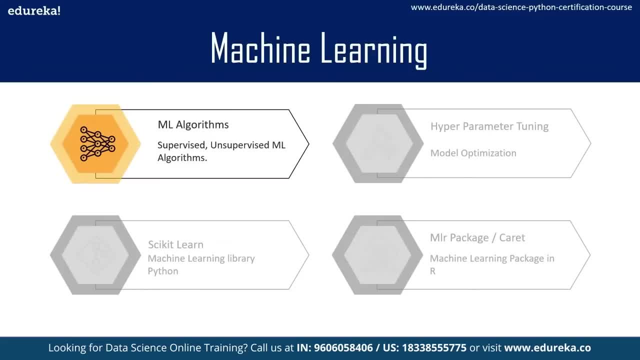 Okay, What is this, and which category or which class cluster will the data fall into? So primarily we deal with supervised machine learning, and there are two types of supervised machine learning. that is, classification and regression. And in unsupervised machine learning we will see dimensionality reduction and then various algorithms like clustering, and in clustering there are so many algorithms, like hierarchical clustering of k-means and so on. 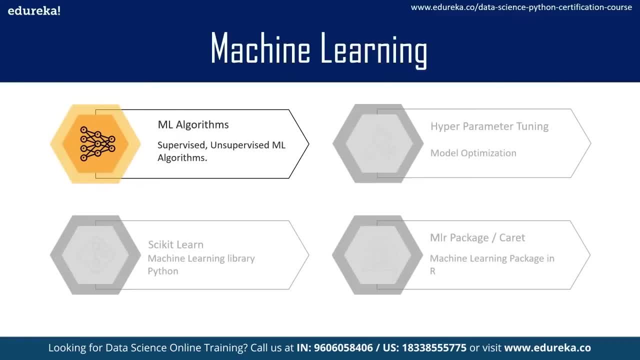 So a data scientist has to know about the algorithms, different kinds of algorithms that can be applied to a data to give good results. That's why it's a little vast, but it is really very interesting. So various algorithms like SVM, NAV, random, forest- k-means good command over the supervised and unsupervised machine learning is required by a data scientist. 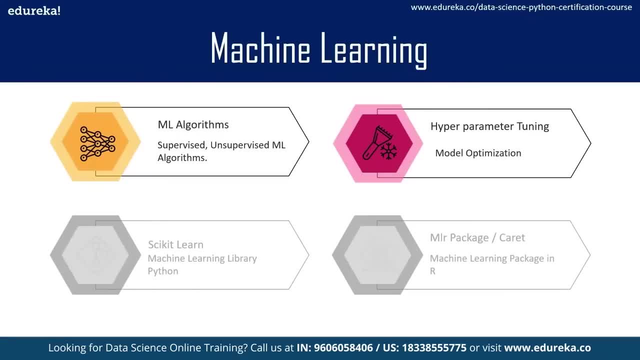 Hyperparameter tuning. Now this is again important because hyperparameters are nothing but they control the behavior of an algorithm. So you can say that if a hyperparameter tuning is being done or performed on any algorithm, that is done to improve the results. Okay, 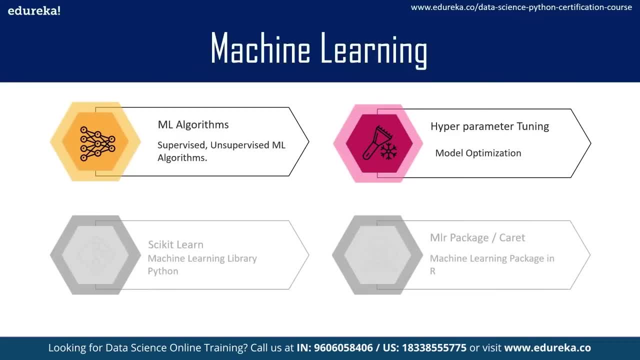 So for model optimization, this is required. So to improve the predictions by tweaking a few parameters via hyperparameter tuning. that is what a data scientist also does. So to learn machine learning. moving on forward now, to learn machine learning in Python, what libraries are required? is that scikit-learn is a package for machine learning library in Python? 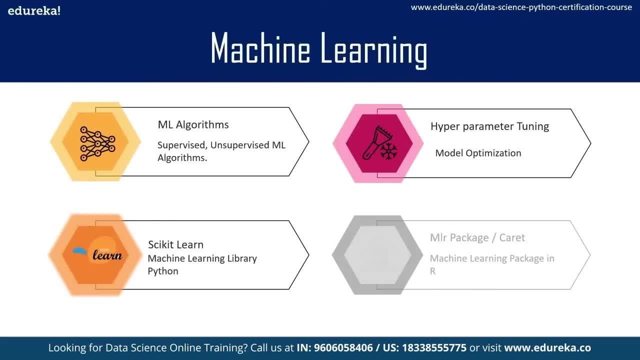 So the scikit-learn is the machine learning library and this supports both supervised and unsupervised learning, and it also provides various tools for model fitting, data pre-processing, model selection, model evaluation and other utilities. So if you, if you're making any model or you're importing any of the algorithms, scikit-learn package would be used. 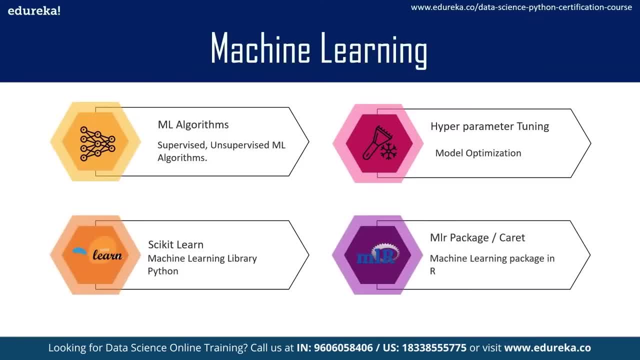 Okay Now, moving on further to R. So in R, if one wants to build machine learning models, so MLR is the package or carrot is the package. So here MLR has all the important and useful algorithms to perform machine learning tasks, and carrot stands for classification and regression. 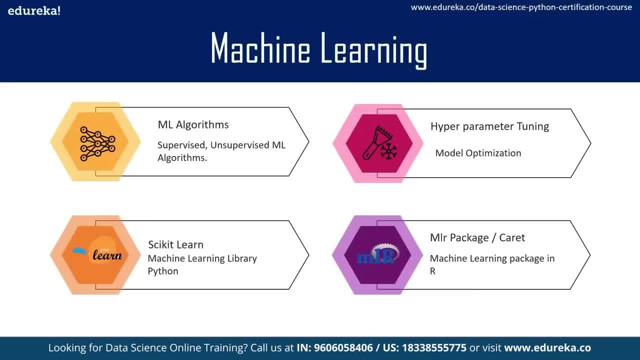 Training. So with carrot one can process and streamline model building and evaluation process. Also, feature selection could be done and other techniques are also can be applied with the help of these libraries. These are very strong and powerful libraries which have consolidated packages and you just need to import it in your project and use it. 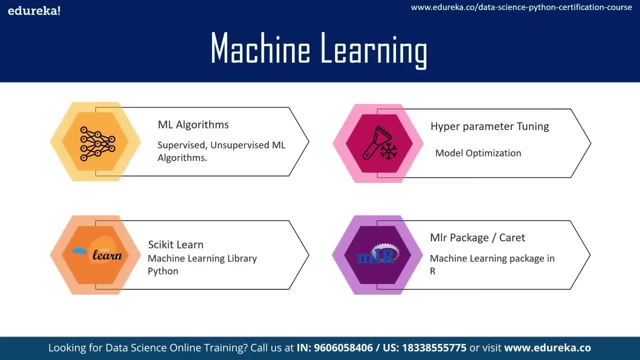 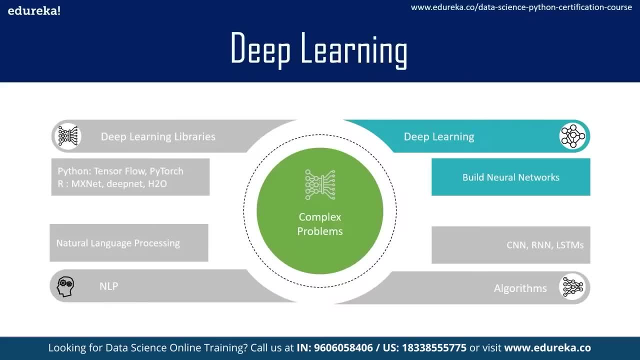 But the knowledge of how to use it, where to use it, is what the data scientist knows. So now, moving on further to another technique and technology, That is deep learning techniques. So now, when we want to work with complex data sets, when the data set size is huge, then traditional machine learning algorithms, they are not preferred. 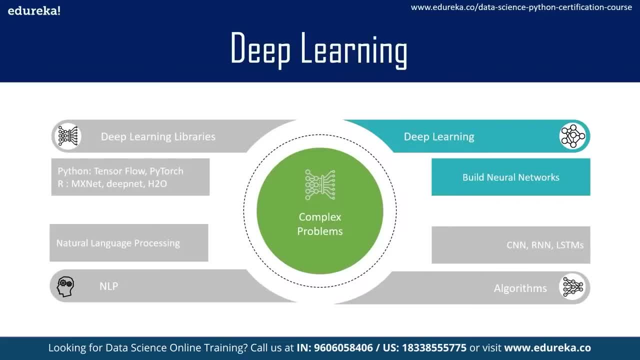 And generally we move on to deep learning. So gradually, from machine learning one moves to deep learning. That is a gradual shift. So when we talk about deep learning, what comes to our mind is neural networks. So when you're working with various kinds of layers and neural networks, then deep learning. 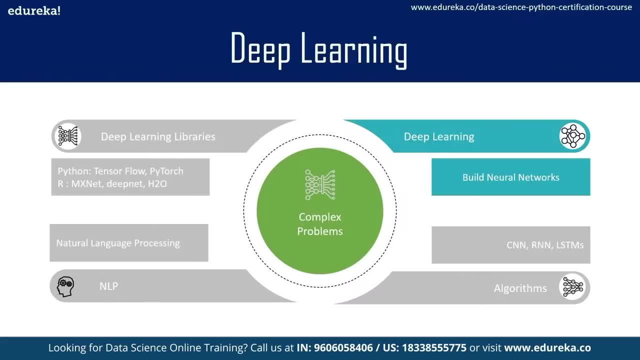 And neural networks are neural. There are a set of algorithms which are modeled loosely after the human brain to recognize patterns, So just as to make it, the system, more intelligent by just understanding the patterns and predicting. So deep learning is more advanced than machine learning, I can say. 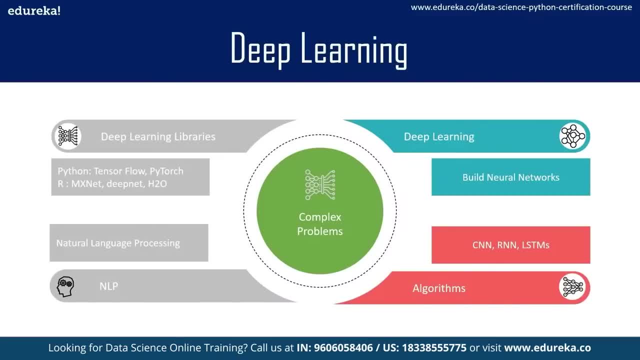 So a few deep learning algorithms are convolution neural networks, RNN, that is, recurrent neural networks, or LSTMs, which is long, short term memory networks. So a few deep learning algorithms are convolution neural networks, RNN, that is, recurrent neural networks, or LSTMs, which is long, short term memory networks. 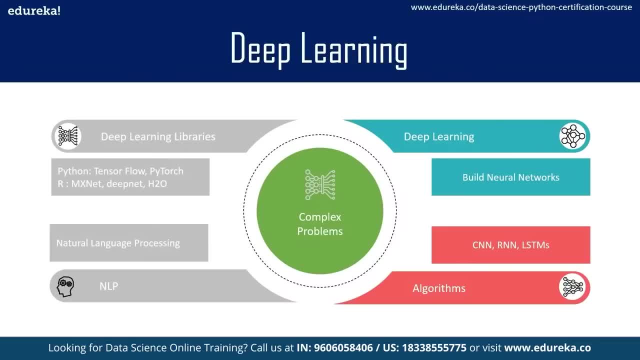 and there are many other deep learning techniques or algorithms. so these algorithms they help to solve complex problems like image classification or text to speech or language translation. so these are really very powerful algorithms which are deployed to solve real world challenges and how to really life, make life simple. so now, moving on forward to natural language processing and what if? 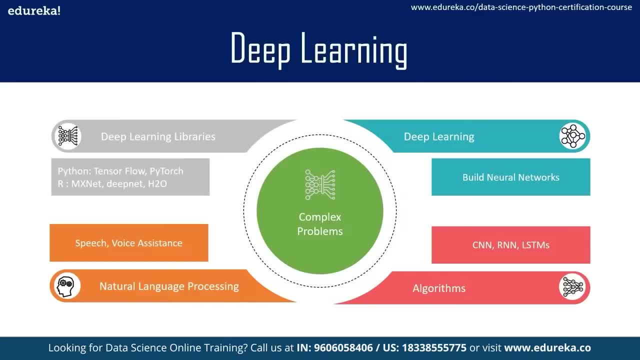 i say that we all have, some time or the other, had experienced with nlp and we know the end result. how remember siri and alexa? yes, i'm talking about natural language processing and this is a subfield of artificial intelligence, and this is concerned with interaction between machines and humans. 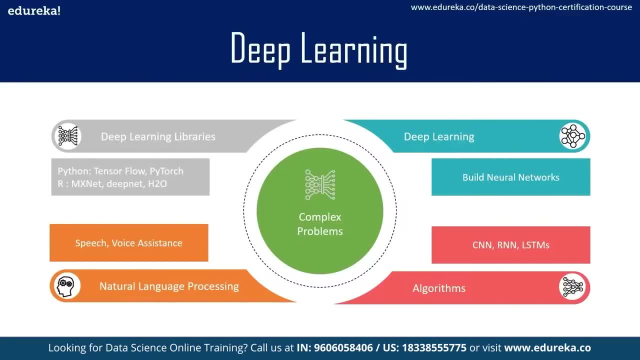 so it is used for speech recognition, reading text, voicemail virtual assistants like alexa or siri, and these are also the examples of nlp. so for python, the deep learning libraries are used for speech recognition, reading text, voicemail virtual assistants like alexa or siri. 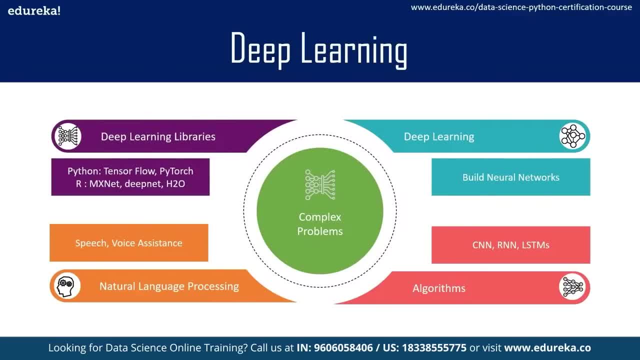 are mx net, r, deep net, deep r, h2o. so, talking about mx net, art is used for feed forward, neural network, convolution neural network, whereas h2o can also be used for the same, but h2o is for deep auto encoders. so when we move on to deep learning, there are more sophisticated terms and technologies that 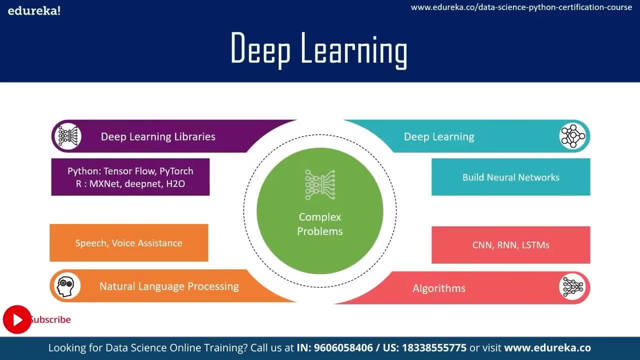 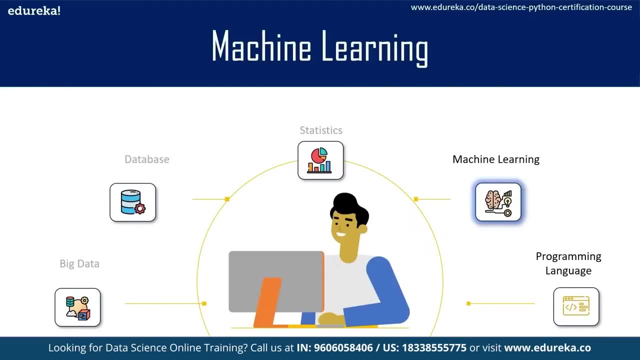 needs to be learned and to puff. to improve the model performance, one needs to understand the working of algorithm, the limitation of these algorithms and how one can really improve upon the model by iterating over these models. so now moving on forward from machine learning, deep learning and another tools and technique, and that is statistics. so yet this 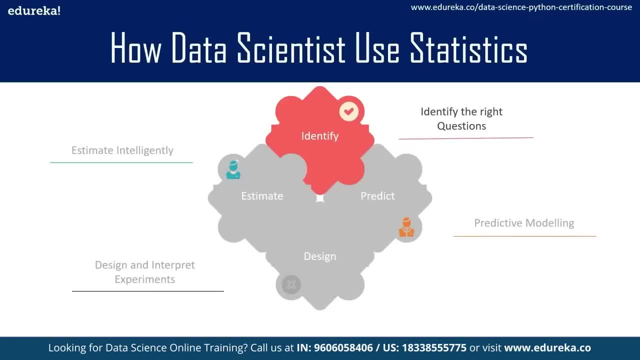 is yet another important tool. now, how does a data scientist use statistics? so it has been used to identify the right questions. so data scientists also use statistics to apply it to the data and ask the right questions, and once they know what the question is, they can use statistics. 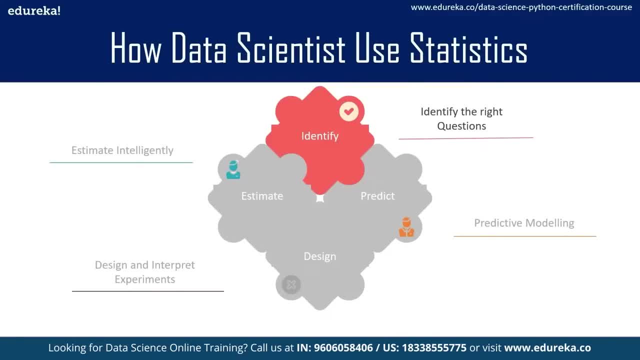 to find answers. so statistics also help them to understand how reliable their results are and how likely is it that the findings can be changed. now, moving on further, the statistics help data scientists to do predictive modeling. this means that using the past data to create models, and that 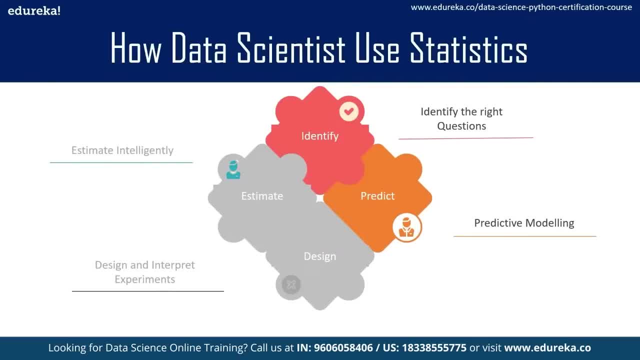 can be used for predicting the future events. that is, predictive modeling. now, another importance of statistics is that it will help a data scientist to understand how reliable their results are and scientists to design and interpret experiments to make informed decisions. so now let us understand this with the help of an example. an observation was made that an advertisement x suppose an 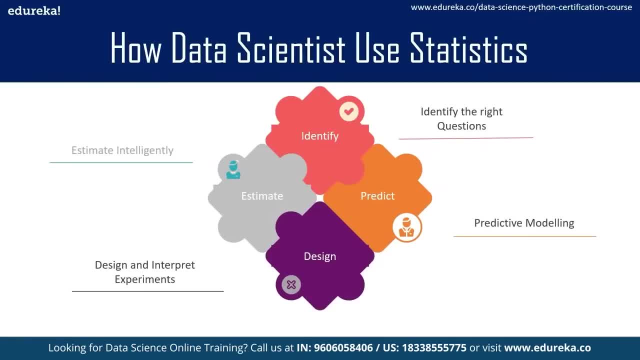 advertisement x has a seven percent higher click-through rate than an advertisement b, so a data scientist would determine whether or not this difference is significant enough to warrant any increased attention, focus and investment. now this statistics would help us to experiment and design the frequency statistics, or hypothesis testing and confidence intervals. 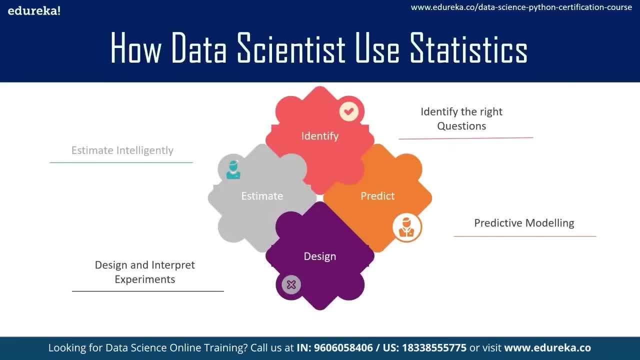 so data scientists would work with these tools like frequency statistics and hypothesis testing to understand whether this is really important or not, whether advertisement x requires more attention or advertisement b requires more attention, focus and investment or not. so statistics helps to determine these important and crucial decisions. all right, so now another use of 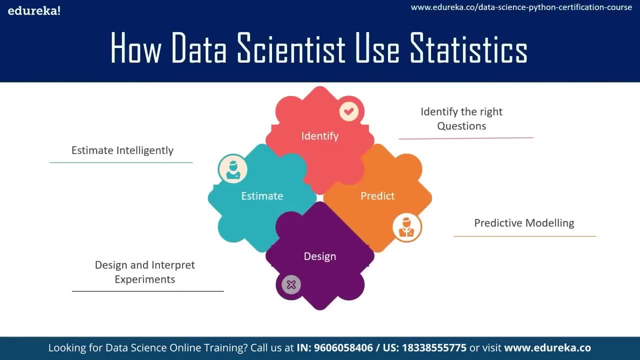 statistics is to estimate intelligently. so data scientists estimate intelligently. that means by using bayesian theorem. there are various theorems which help to estimate intelligently, because a bayesian theorem takes the result from the past experiences and observations and then make predictions. so this is estimating intelligently and they can also summarize what estimates are. 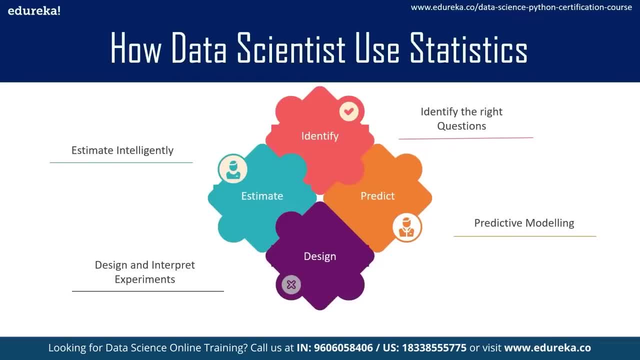 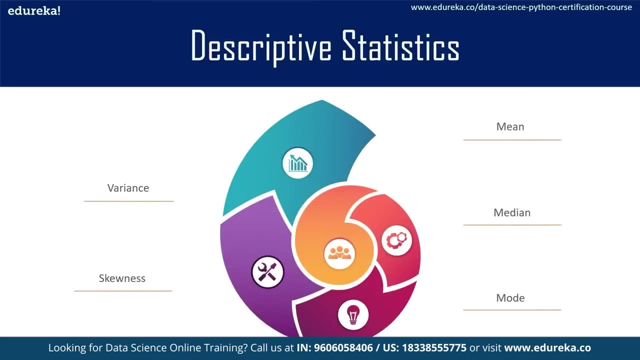 and mean with the help of bayesian theorem. so now statistics equip a data scientist to solve problems and make data driven decisions. and now moving on forward to most common statistical methods, and this is descriptive statistics. so we talked about descriptive statistics. now let us understand what is descriptive statistics. so descriptive means it is a summary statistics that quantitatively, 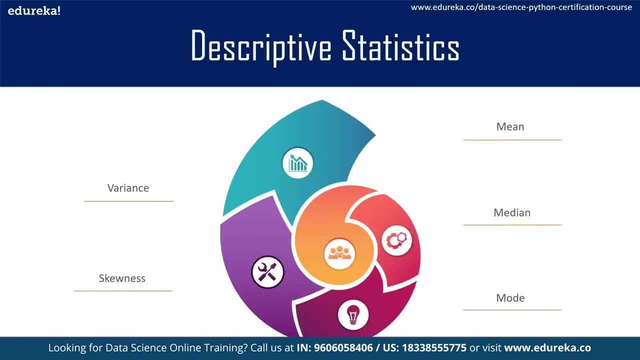 summarizes features and some measures include. these are the central tendency measure, measures which are being listed on the right hand side, like mean, median and mole, and on the left hand side- the left hand side- it is skewness and variability which are measures of standard deviations, and variance is nothing but knowledge of like. how much is the spread of the data right? skewness is where 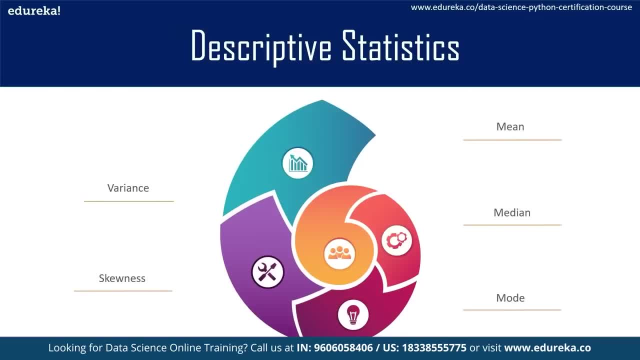 the data is inclined, whether it is right, towards the right or left, and determining the normal distribution of the data. we understand that. are there any outliers in the data, what, how the data really is spread? so these descriptive statistics, they help us from through the numbers that they. 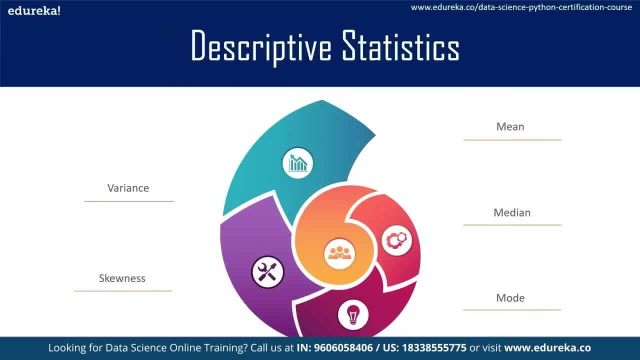 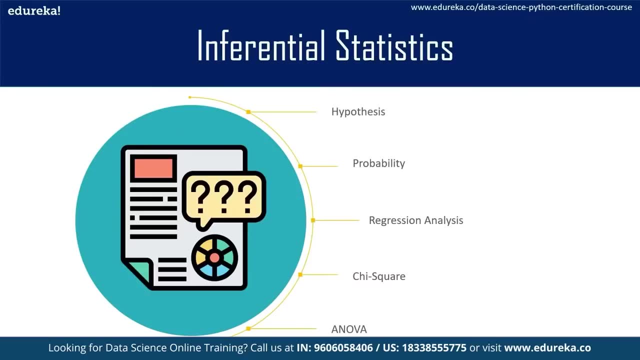 give so we understand what the data is. now moving on further to understanding what is inferential statistics. so a data scientist must also be able to use inferential statistics, because here inferential means we are taking a small sample from the entire data and we are making 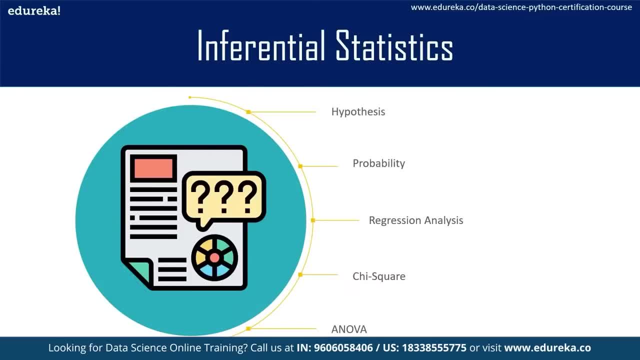 generalization about the entire data. so this is inferential statistics, inferencing something from a small data, assuming that this is this will also apply to a data. okay, so we make inferences from a sample about the population. now, the methods for this includes hypothesis testing, probability. now probability is used to predict the likelihood. 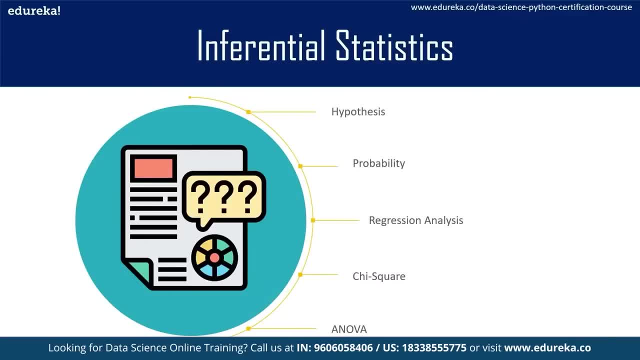 of an event. regression analysis is yet another method. so regression what we do is we model the relationship between variables. like anova is yet another, which is analysis of variance. this is a test to compare the means of different groups and how different they are, and based on the results, we take decisions. another method is chi-square, and this chi-square is used. 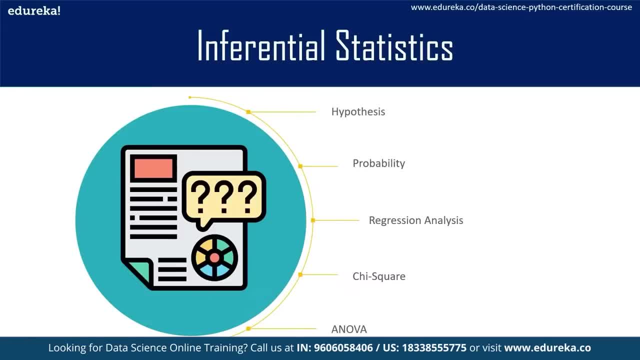 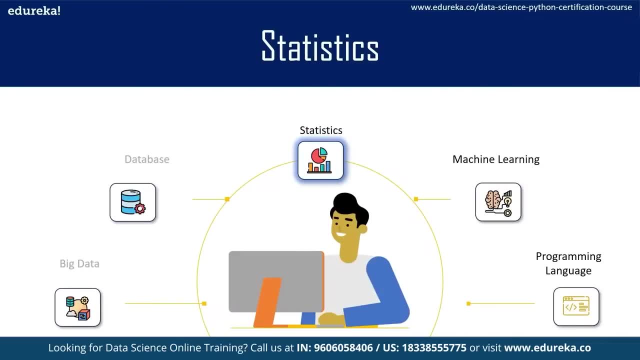 to determine any relationship between variables or compare the result between an expected and observed values. so this is inferential statistics. and now we will move on to another technique, and that is from statistics to databases. so let's understand what are databases. so now data has to be stored before analyzing or making predictions, and to store the data we have databases. 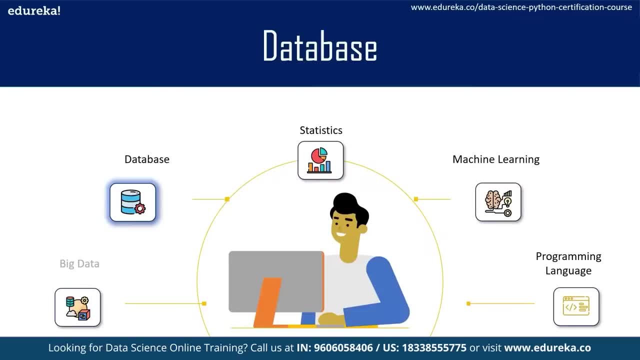 we know to store data. these databases are instances of data, so database must be rapidly stored before a person studies a new study. for example, if somebody is studying a new research project, then they have to write an interview where they study data. so you can consider this in the data. 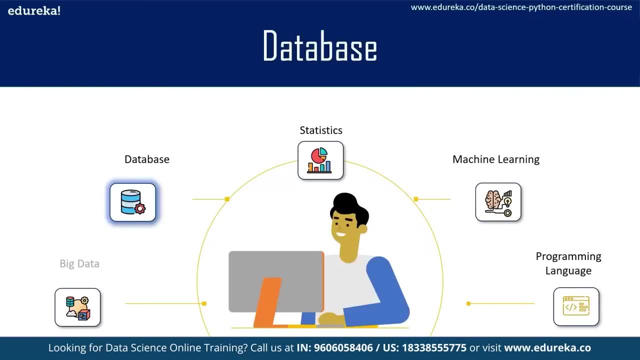 too right. what this is? what viral data is. they use it to collect data and traded as related documents so they can use this to rundown and process data in a way that internationally supported and labor-intensive eleven, buscar and strawberry draußen, and they use it to code the data. today. data can be processed by a database, and loading a database can be done on a database, can be done in an any of these databases. so in a database or other, anytime you want to, Hanson, data is handled. this is not as easy as data was created or developed better because we find data, so we need to understand the. 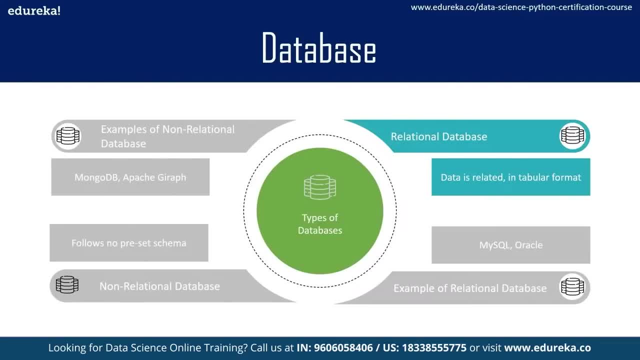 course, but again, information solutions, are것 게임 and data science are most important. so is relational database, was we'll be talking about. so, as it is said, relational that means the data has some relation between itself or between each other, so the data is related and it is stored in. 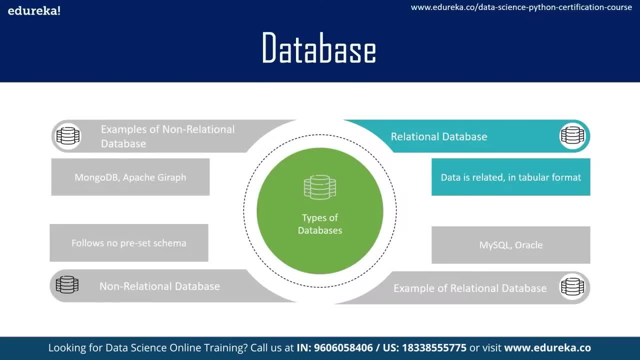 a tabular format in some predefined schema in the databases. so what happens is that when it is in a tabular format, when it is in a clean format, the retrieval becomes quite easy. it's smooth, it is not complicated and this data is related somehow. so the example i can say of relational databases: 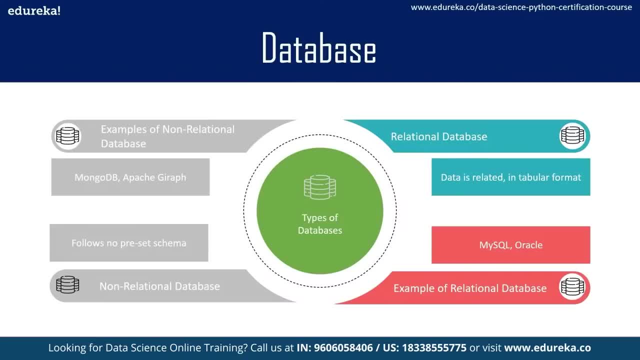 are my sql, microsoft sql server or oracle databases. and now another type of a database is non-relational database. now, non-relational that means it is not having any relation, and this database is. it does not follow any preset schema and also it is not in a tabular format. this is 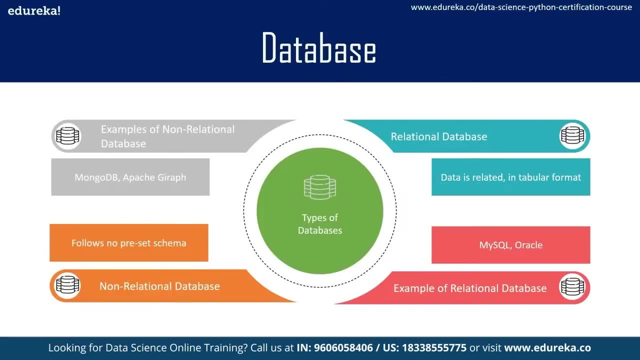 not important and we can store any kind of a complicated data in a tabular format and we can store any kind of a complicated data in a data. whatever complex data we have and an unstructured data we have, that goes into non-relational database, and few examples of non-relational database are, as we can see, here. 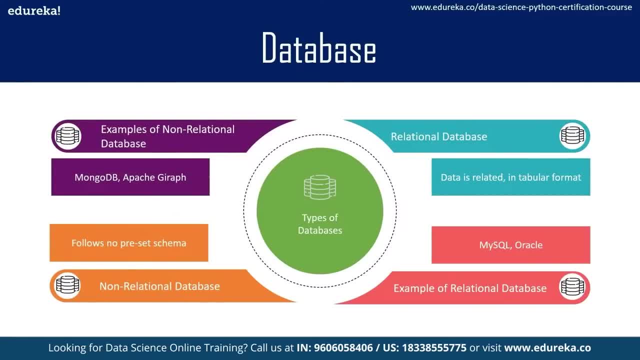 mongodb apache gdraft. now let me tell you something about apache gdraft. it is optimized for storing relationship between nodes. so why is it important? because this shows connection between entities in, and this software really makes social network data more informative and it provides real-time graph processing. so when you are analyzing huge volume of data from social network sites, 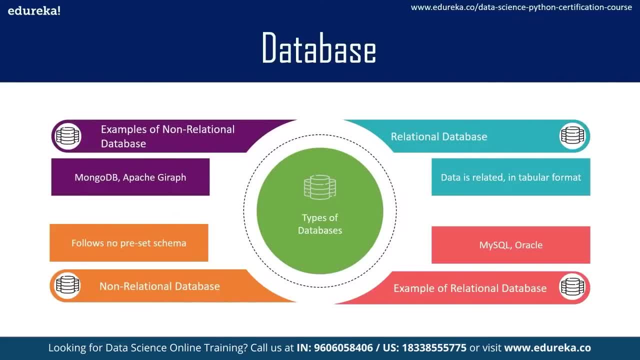 these non-relational database really help you to understand, analyze, store the data and find some relation between them. so that is why it is really important to have the knowledge of these databases. no sql databases and mongodb is optimized to store the documents right, so there are various. 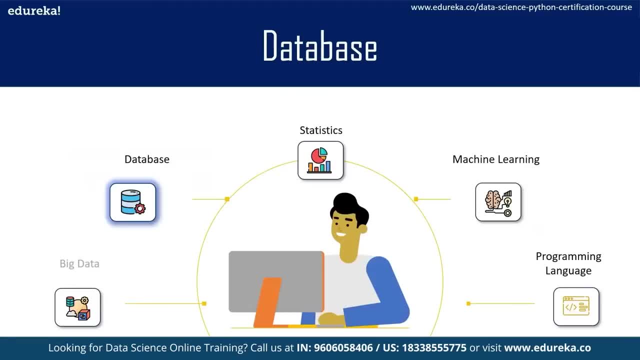 non-relational databases. i've just listed a few here. now let's move on from database to another technology, and that is big data. now to understand, or the ability to analyze the unstructured data. this is relevant in the context of big data. so big data: we are moving forward, and big data, what? 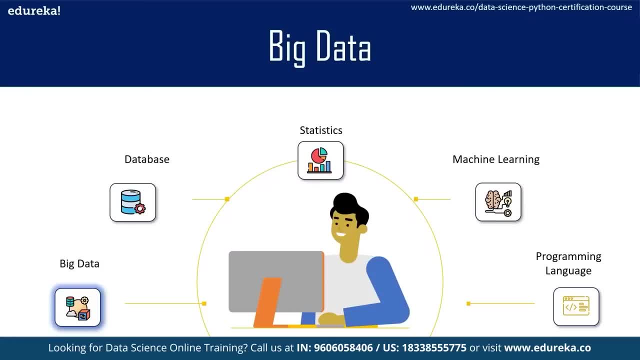 happens here is that we are dealing with larger and more complex data set day by day, and companies are dealing with huge volumes of data, especially from new data sources. so these data sets, they're so voluminous that traditional data processing softwares cannot manage them. that's why the 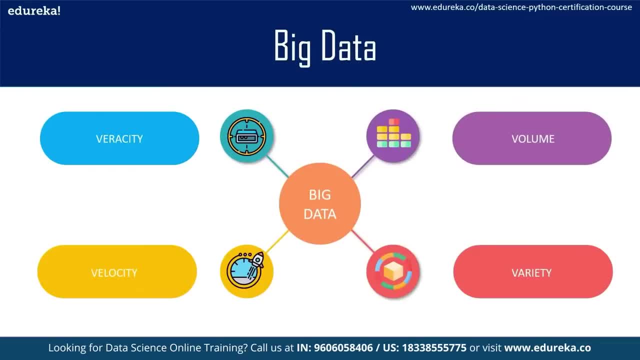 big data technology is really helpful. and big data, it is a collection of data from diverse data sources and it has certain characteristics like volume, variety, velocity and veracity. so these are certain characteristics of big data. now moving on forward to big data technologies. now why they are needed? because to manage big data we have to use big data technologies and they are classified. 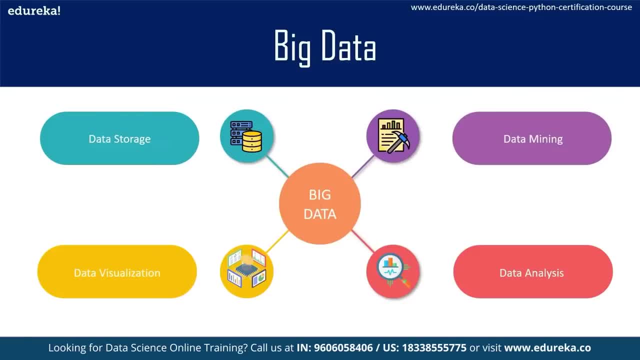 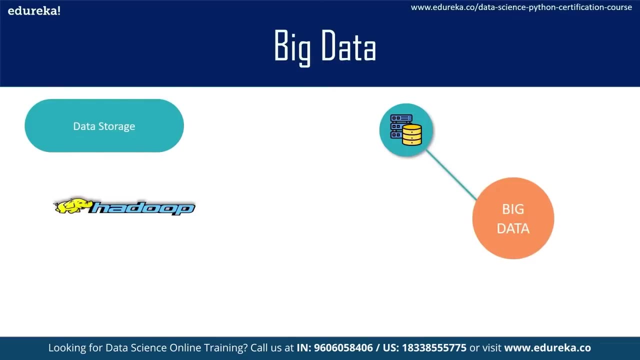 into data mining, data analysis, data visualization and data processing. so these are the characteristics of big data technologies. so all these big data technologies are not required by a data scientist. we will particularly deal with data storage, which is required and which is really important to know by a data scientist. so for data storage we have hadoop. so we will cover first hadoop. what is this? 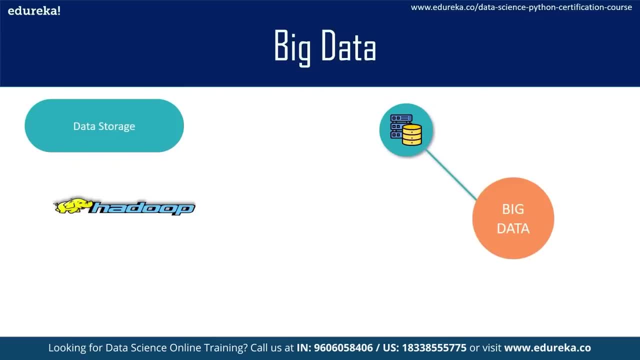 hadoop. so hadoop framework is there to store and process the data in a distributed environment, so which means that it can store and analyze the data, but it can also store and analyze the data which is present in different machines and it also comes with very high speed and very low cost. 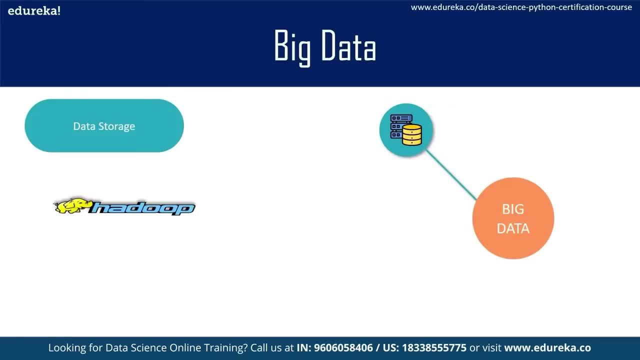 so the companies like microsoft or intel, ibm- they use hadoop to store and process data. so when you're working with huge volumes of data, you need to even store and analyze it also at very quick speed and at low cost. so hadoop gives you that flexibility and power and those features which you really need. 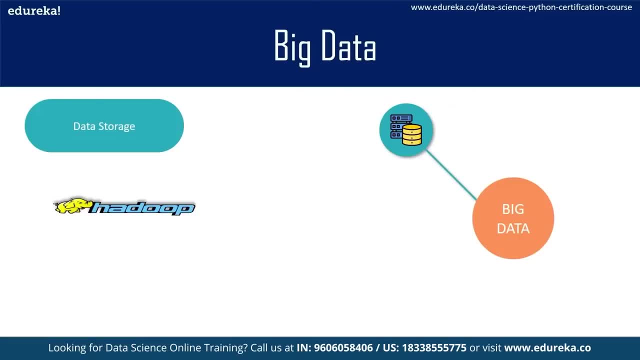 so now coming on forward to another big data: data storage is mongodb. now, this is again a no sql database and it offers what a direct alternative to rigid schema, which is used in relational databases, but mongodb. another flexibility is that, while handling a wide variety of data types and at large volumes, you can use mongodb, and it also can be used for 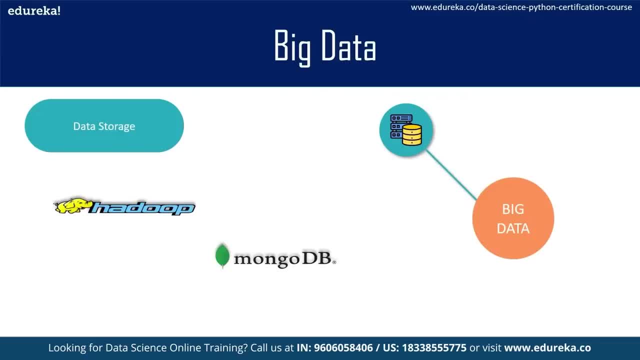 distributed architectures. so again, mongodb can be used and companies like mysql sql server. they use mongodb to handle data. another big data storage is apache spark. now apache spark is again used for large-scale data processing. now both- i would say that- the apache spark and apache hadoop. they are both open source frameworks. 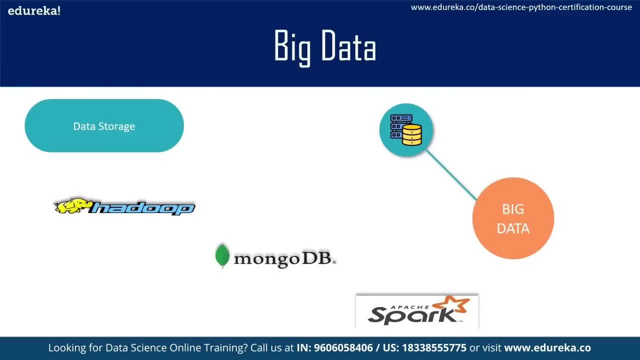 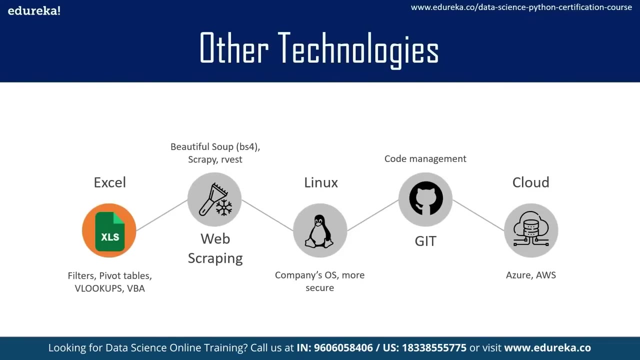 for big data processing. there are some key differences, like: hadoop uses map reduce to process data, while spark uses resilient distributed data sets, rdds. so now moving on further, for other technologies which are recommended for a data scientist is excel. now, excel is used since decades for analysis, but now more advanced languages and more simple. 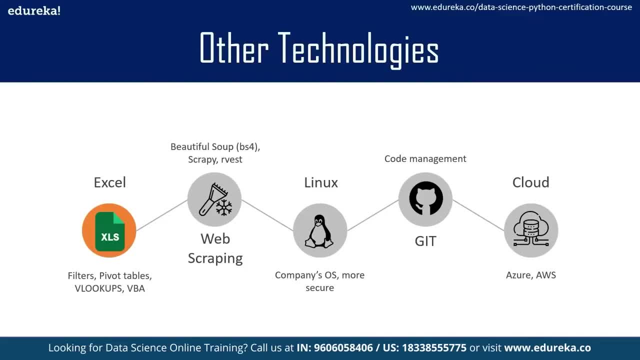 languages are there out, like python and r, but excel is here to stay. so using excel for basic analysis, like formulas, pivot tables, vlookups or vbas- this can be used by data scientists, so vba is nothing, but you know visual basic for application and this can help automate repetitive 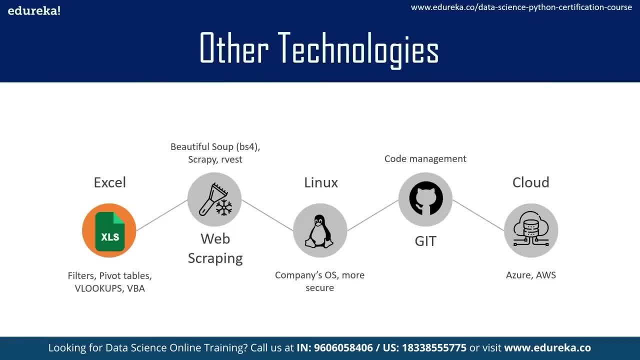 word and data processing functions, and it could also help you to do a lot of other things like creating web staples to generate a set of such custom essences, to help you generate custom graphs, forms and reports. so excel is really a very powerful tool which is yet even today, which is 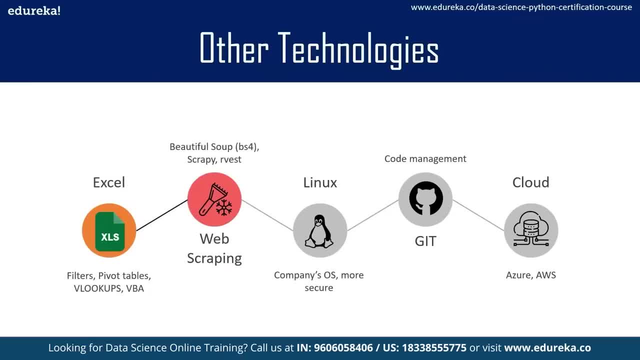 being used. so now we are moving on forward to web scraping. so scraping libraries like beautiful soup in python. it is also known as bs4 or scrapey. these are popular libraries in python, but if one is using r then rwest package is useful in extracting information from the web. so web scraping is not. 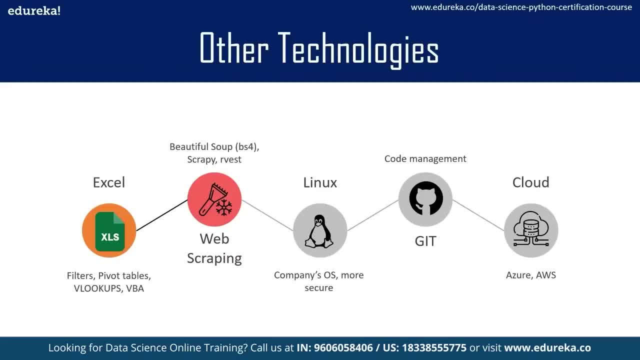 there in most of the libraries, but it is still used by data scientists. so that's why we have the Most of the job responsibilities are for data scientists, but if one is equipped with this and have a knowledge of how to use various APIs and get the data from that various resources, 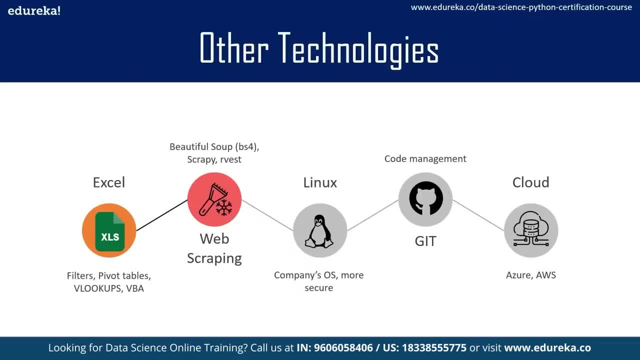 over internet, then this could be a real help. Now moving on forward to Linux. Now, why is Linux required? Because the company operate on various operating systems, not necessarily Windows. So Linux is the most recommended language, I would say, or the commands need to be learned. 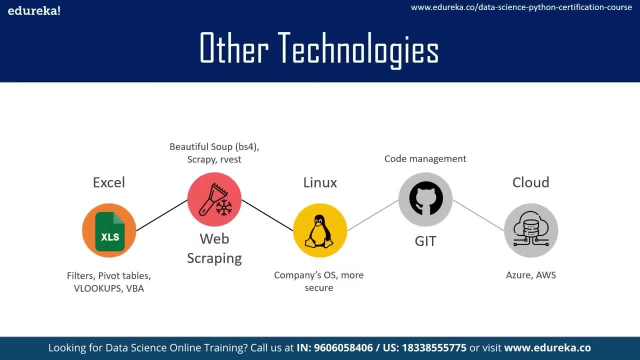 from Linux for a data scientist, because anyways, when you're joining a company you have to learn those commands. So basic knowledge, not much, just basic concepts to how to operate Linux, the commands- And this would be really helpful as Linux is considered more secure as compared to other. 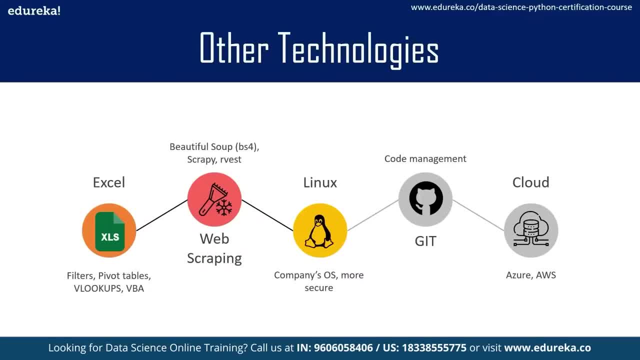 OS and companies really want that their data should be secured, their information should be secured, So a different operating system is used. So that is the entire idea about learning Linux. But this is not essential, But this is an option. Now, moving on forward to another technology, that is Git. 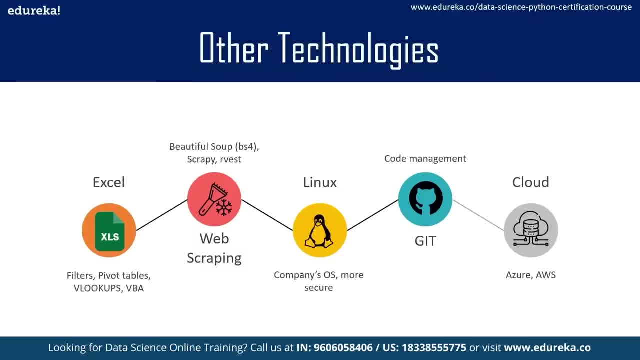 Now Git is for code management, or your source code management when you're working in teams and you're sharing the code. So various versions of various changes could be made in that code by various people. So Git provides one source wherein all the changes could be merged into just one source. 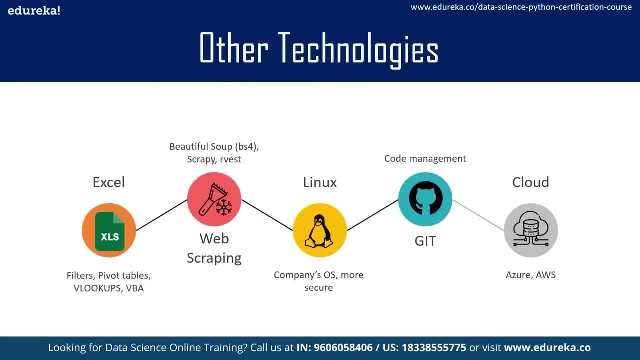 and one gets an edited version. So this is very, very handy and it saves a lot of time And making collaboration is very easy here. You can also allow multiple changes to be merged into a single source, And it is basically a version control system. 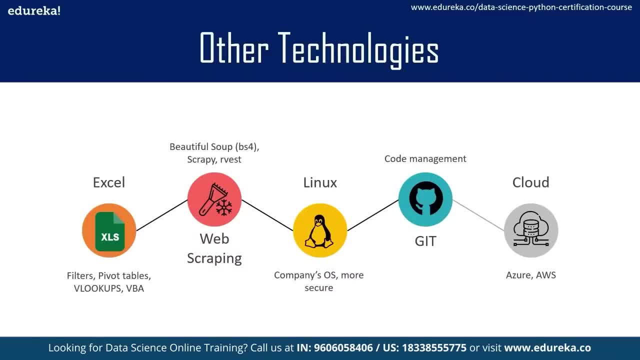 Very useful Git. So Git commands and Git knowledge- not commands, but at least you know how to really work with Git for code management. Now moving on further to another, this is again an option, that is cloud technology. But few companies really now are looking for data scientists who also know the knowledge. 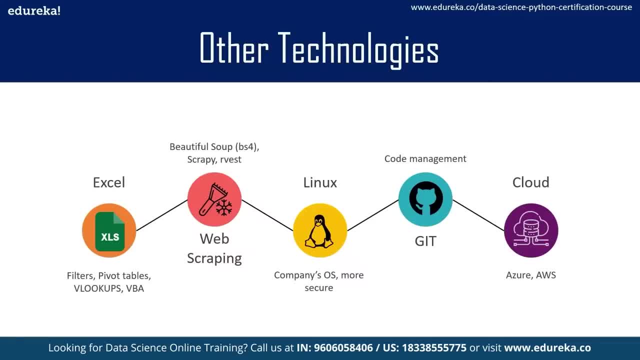 of cloud technology And now cloud technology like Azure or AWS, so that you can gain access over or to the storage of software or servers over the internet. So how do you really access that? How do you retrieve information from cloud by using AWS or Azure or different technologies? 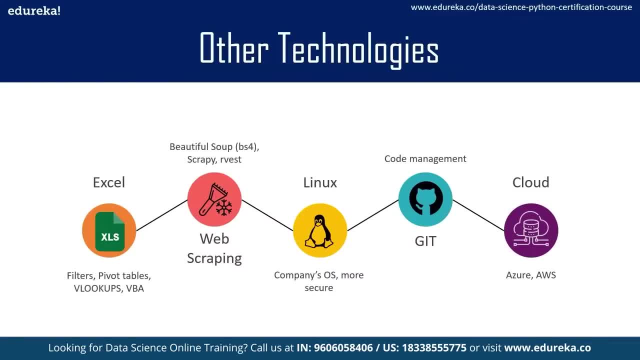 that the company is using. So the benefit of by company or sorting to cloud is that it provides unlimited storage space and very high speed. The backup So create is good and it restores the data. It is also cost effective and it saves much of the infrastructure cost of the companies. 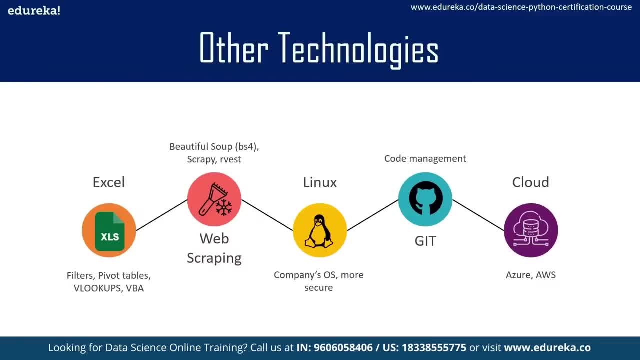 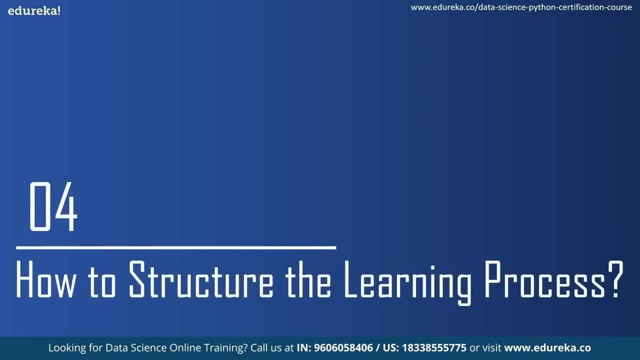 too. So that's why companies are really moving forward to cloud, and they need people who can really access cloud along with deploying machine learning models. So this is preferred. Sometimes it becomes important too Okay now. so moving on further to how to structure the learning process, 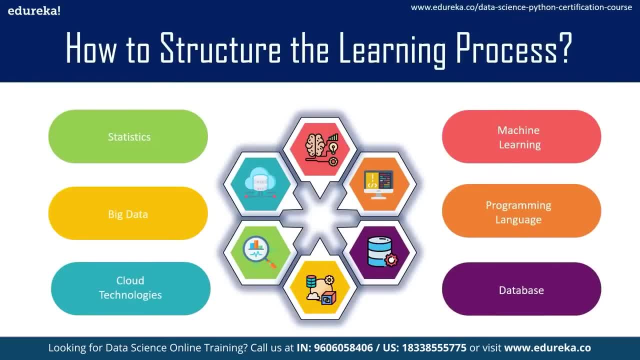 Now, the above list of subjects could be really overwhelming And can really, you know, demotivate a serious learner in the long run. So how one should structure the learning process to scale up the ladder of a data scientist. Now, all these topics need not be learned at one go, but parallel learning is recommended here. 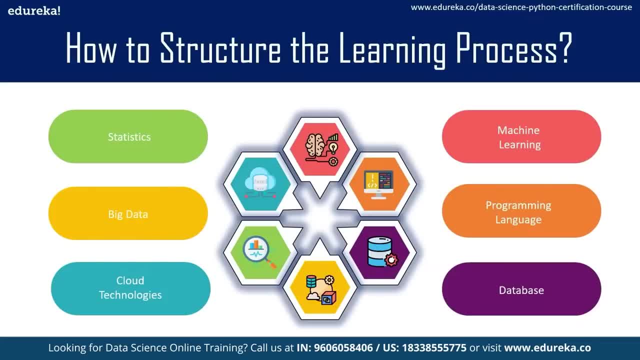 By parallel learning I mean that learning Python first and then moving on to data analysis, visualization with the help of various projects, building machine learning models with the help of one programming language. That will give the Idea of how really algorithms work on data understanding the answers or the outputs from 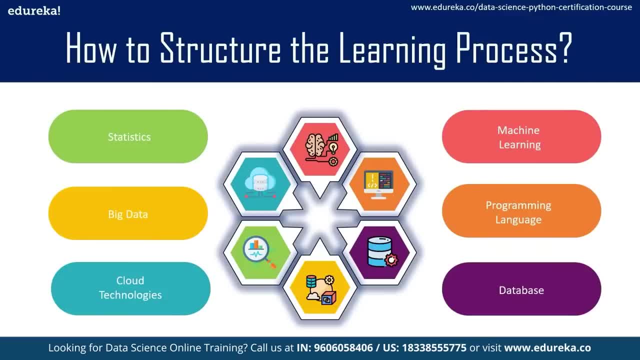 the data and then tweaking in with certain hyper parameters and improving those results. Once you are done with machine learning, move on to deep learning and apply those statistical analysis, the status inferential statistics and diff and descriptive statistics, because we find the description, the statistical bar from the data and understand how does 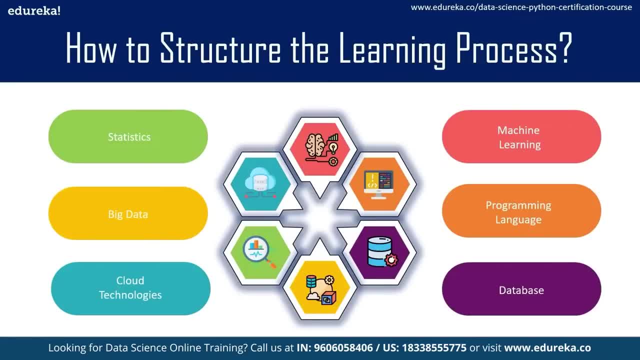 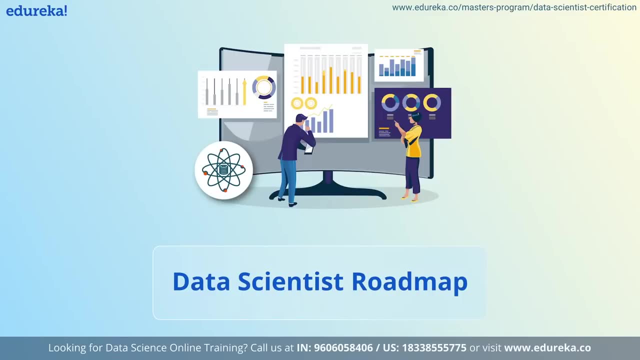 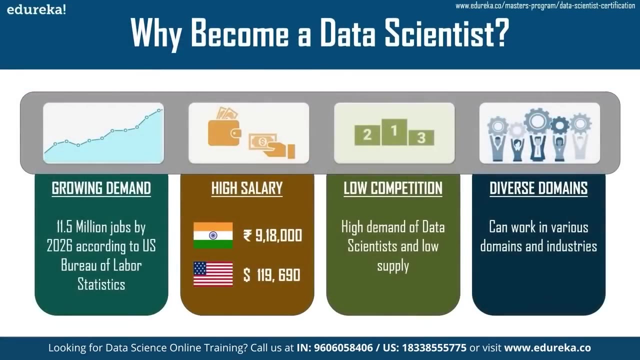 it work by various plots also, So statistics really is helpful in understanding the results. So these learnings are being used in unison, not individually. So the knowledge of all these things are really required. Why become a data scientist? So there are several reasons why somebody should become a data scientist. 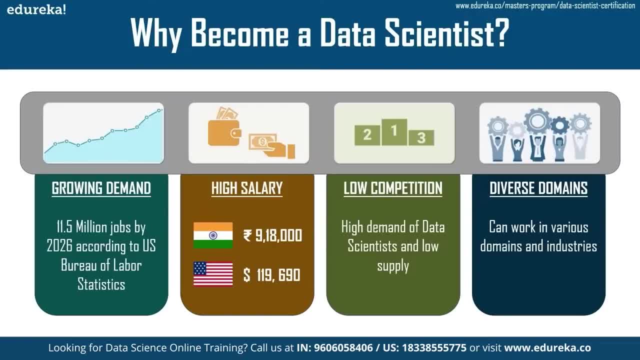 But we're going to take a look at the most compelling ones, which are growing demand, high salary, low competition and diverse domains. So let's go over them one by one. First up, growing demand. US Bureau of Labor Statistics estimates that there'd be around 11.5 million data scientist. 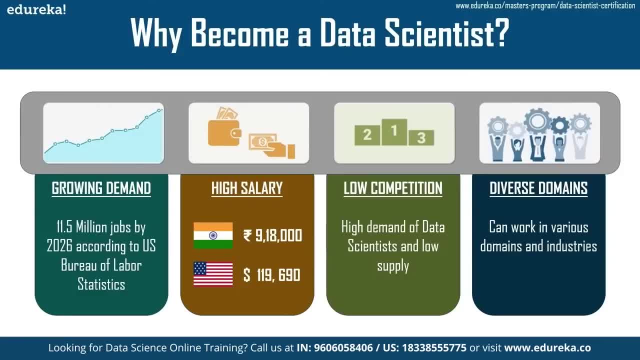 jobs by the year 2026.. That says a lot about the field itself, And the reason behind such a humongous growth rate is that organization all across the globe have realized that data science is pertinent and very important In crucial decision making. 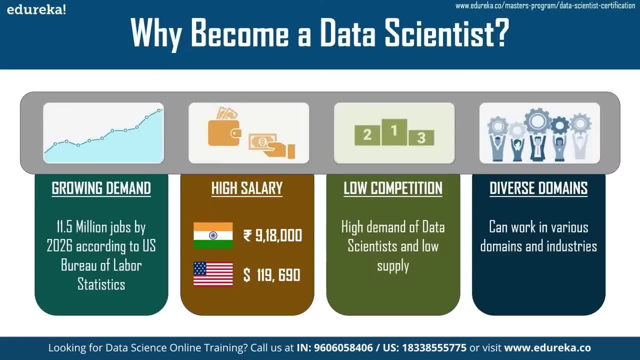 And so all the big organizations across the world are willing to pay hefty salaries to data scientists. That brings us to the second reason why somebody should become a data scientist, And that is high salary. In India alone, a data scientist can easily make, on an average, over nine lakhs. 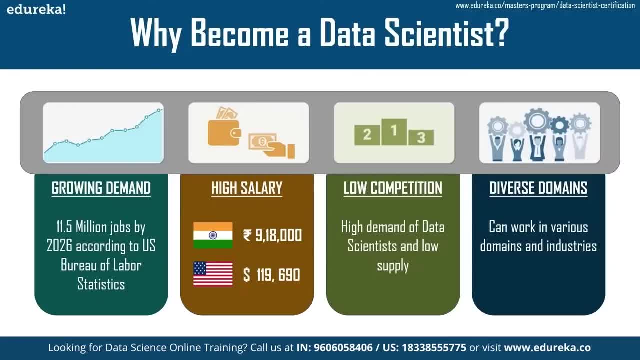 In the United States, that number is 120,000 US dollars. Data scientists with experience of more than five years can make 20 to 30 lakhs, or even over that, And in the United States they can make over 200 to 500,000 dollars per annum. 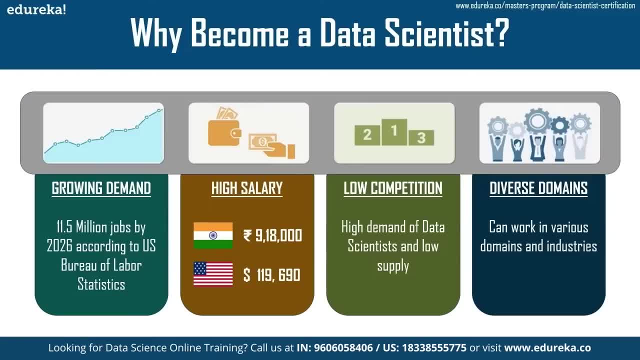 So those are some attractive figures. And keep in mind they don't include bonuses, incentives, benefits and allowances, So those are some crazy good figures. The third reason is low competition. Organizations all across the globe have realized the importance of data science. 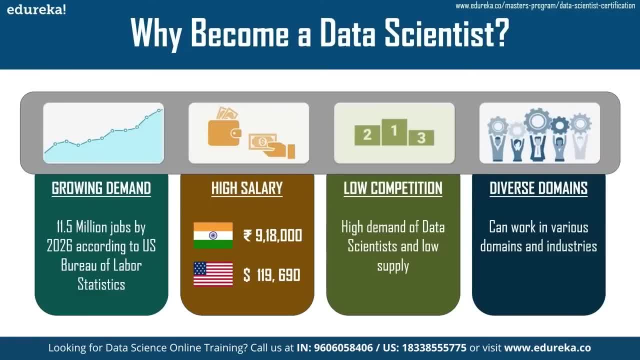 And so they're hiring data scientists left, right and center, But the problem for them is it's hard for them to Find good data scientists. So, in other words, the demand for data scientists is very high and the supply of good data scientists. 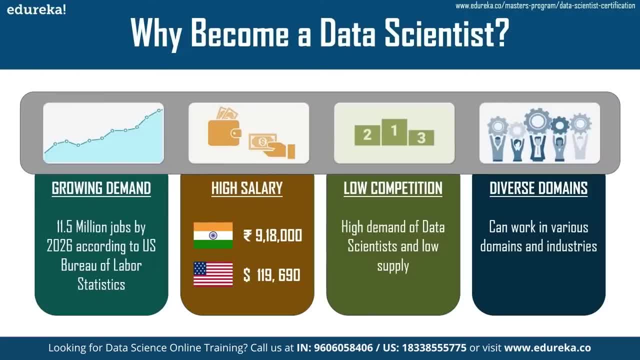 is considerably low. The fourth reason is diverse domains. If you choose to become data scientists, you can actually end up in any domain, For example, product manufacturing, energy, retail, marketing, health care and a dozen more, And the implementation of data science is increasing day upon day. 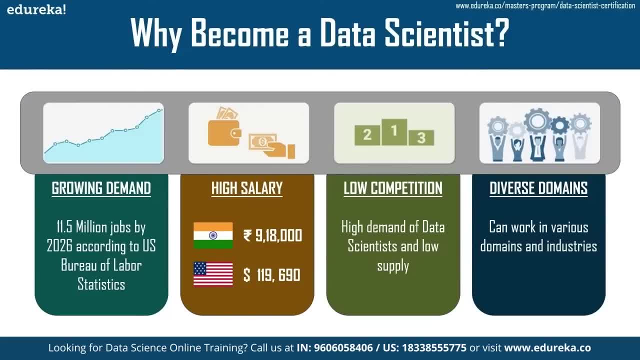 And As each day passes by, people are discovering more ways to use data science in different ways in different domains, And so data scientist job is never going to be boring, because they can move between domains and help different sorts of industries, So it's always going to be challenging and it's always going to be fun. 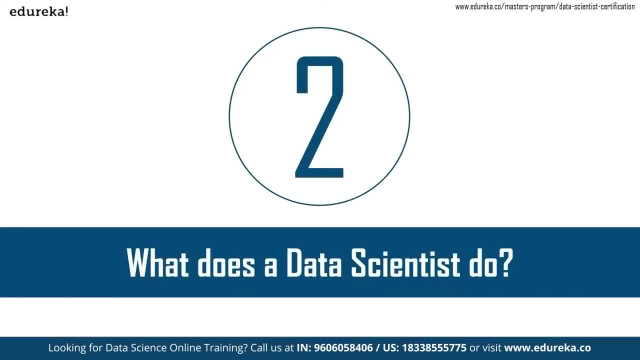 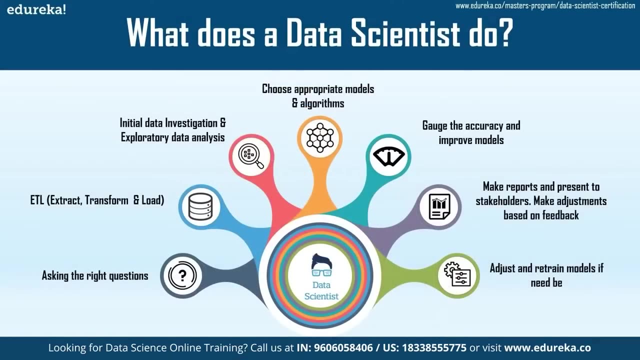 So, now that we have seen that it's a good idea to become a data scientist, if you're data oriented, let's now find out. what does a data scientist do, as in, what are their roles and responsibilities? Okay, So the first thing that they do is ask the right questions to begin the discovery process. 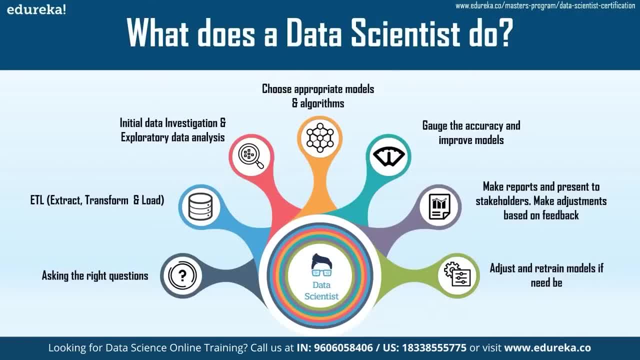 So what I mean by that is, data scientists are hired to solve problems for a company or to help them make crucial decisions. In order to solve any big problem, they have to ask the right questions, which will lead them to the right data to collect and the processes and models they need to use or build. 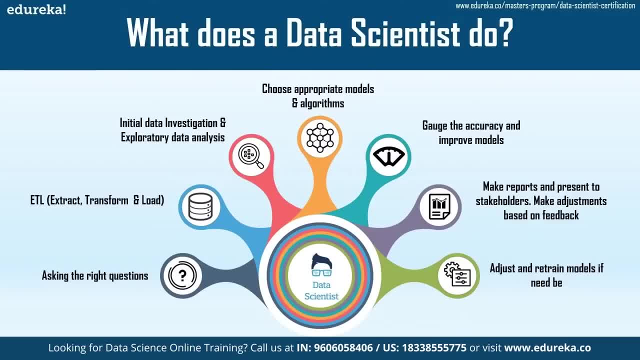 to eventually pull the right answers that will help a business grow or get rid of its problems. So after figuring out what data to collect, now they actually have to clean and prep the data for analysis. So this is referred to as ETL, which stands for extract, transform and load. 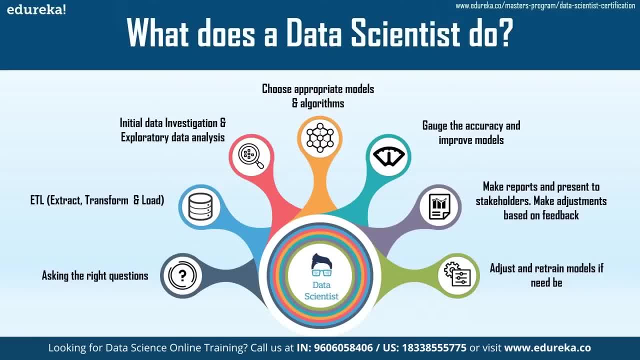 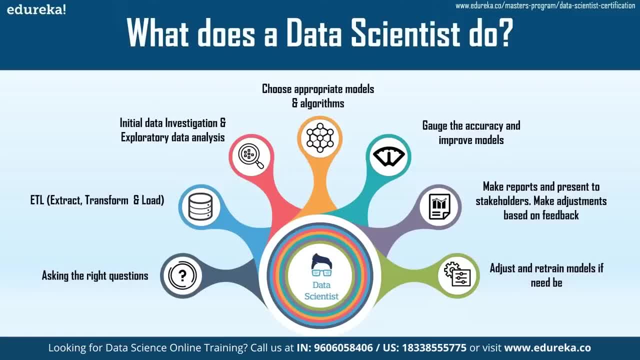 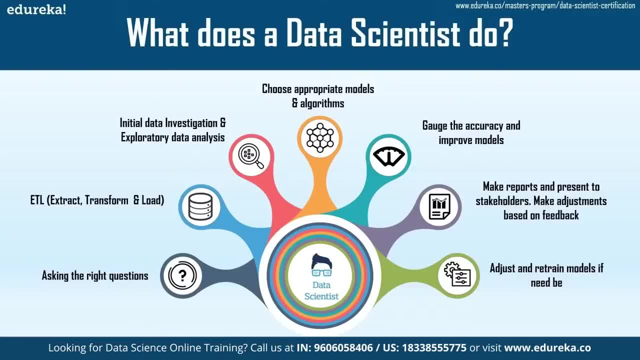 be integrated and stored in the organization's existing database systems. So what would be next? Loading. So loading refers to the process where the data is integrated and stored in the organization's databases. So after ETL they have data that is ready and stored to perform analysis and investigation. 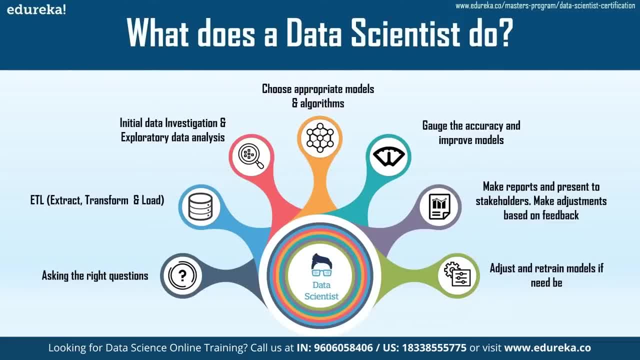 exploration on. So what do they do next? Well, of course, they perform initial data investigation and exploratory data analysis to make sure that everything that they collected is useful in the context of solving that problem, And this also gives them an idea as to which models and algorithms they need to use in. 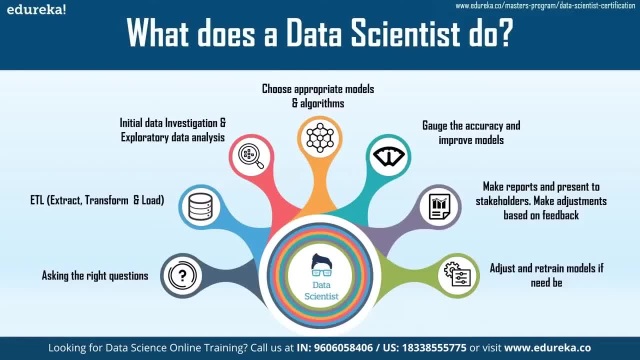 order to extract the meaningful insights. So obviously, after they perform this investigatory and exploratory data analysis, they choose the appropriate models and algorithms that will identify patterns and trends in the data. so they use different data science techniques, such as machine learning, statistical modeling. 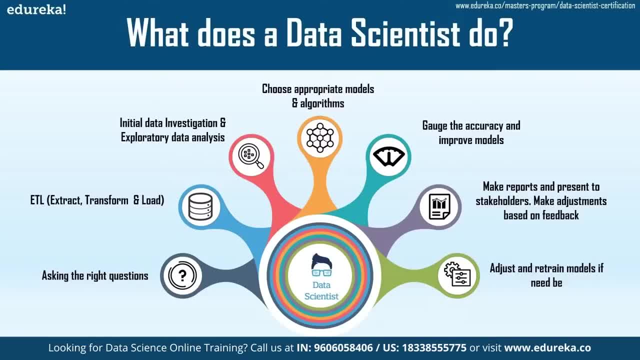 and deep learning, sometimes as well, in order to make these models that gives the appropriate results that they're looking for. After that, they move on to checking the accuracy of the models and improve the models if needed, Once they are satisfied with the models and its accuracy and the answers that they're. 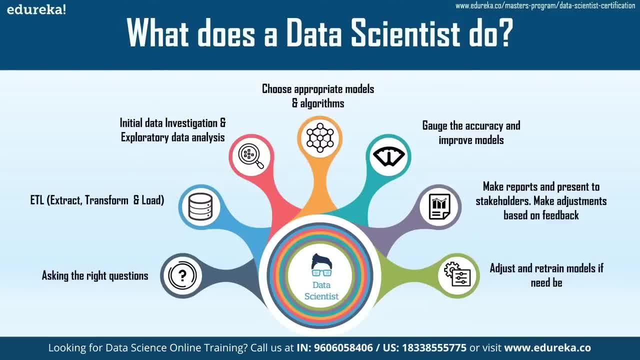 getting they move on to making reports so that they can extract all of these insights- insights into a report form that can be presented to the stakeholders. And so this is usually the last step, where a decision is made, using the insights and recommendations from the data scientists and their reports. 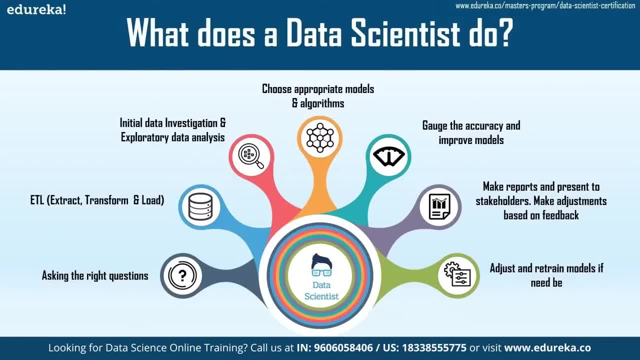 It is also at this stage that data scientists may make some adjustments based on the feedback that they get from stakeholders. Even after the decision is made and the problem is solved, they continue to adjust and retrain the models if needed, So they continue to provide the desired results. 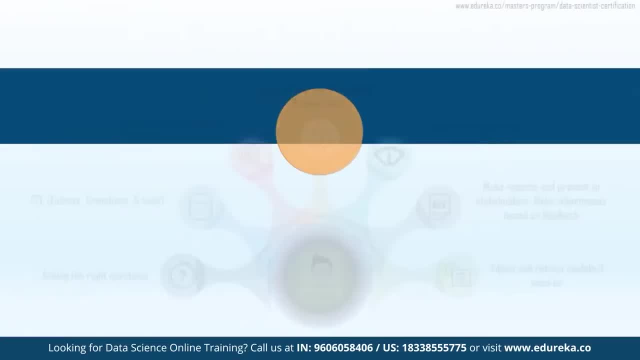 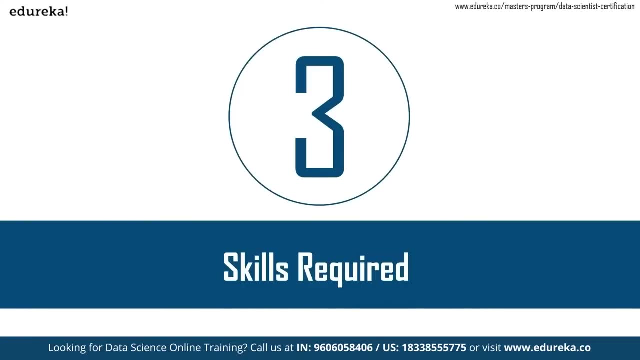 That will help guide the business. So I hope this was clear. Why don't we move on to the next section, which is skills required for a data scientist? So, after going through a lot of job descriptions on sites like Indeed, Glassdoor and more, 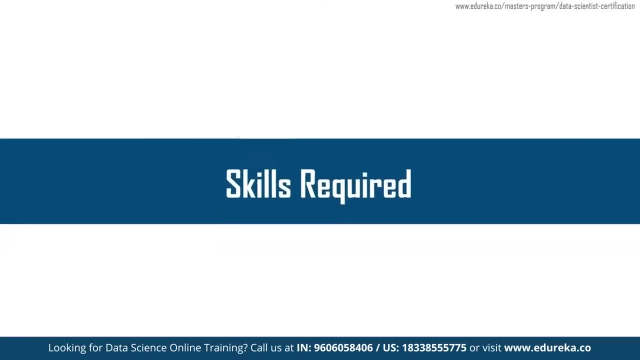 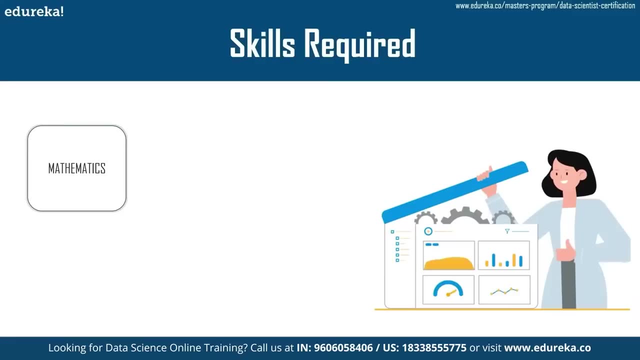 we found that these are the basic skills required if you want to make it as a data scientist. So first up, mathematics. Mathematics forms the foundation for data science. In mathematics you should know statistics and probability, And if you want to become the best data scientist possible, you will also learn linear algebra. 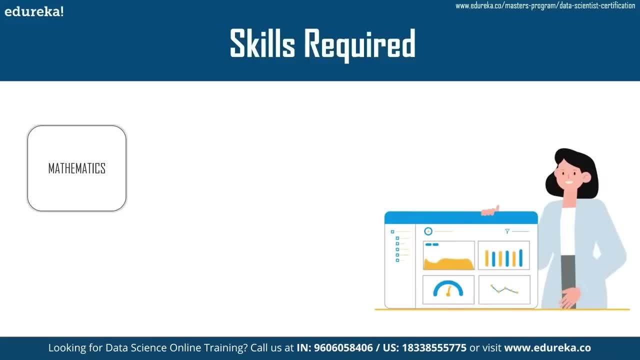 and calculus. We're going to dive into details of what you should learn in mathematics, But for now let's move on. Second skill that you need is programming. You don't have to be a master at programming. You need to know enough in order to use the libraries, handle files and process data. 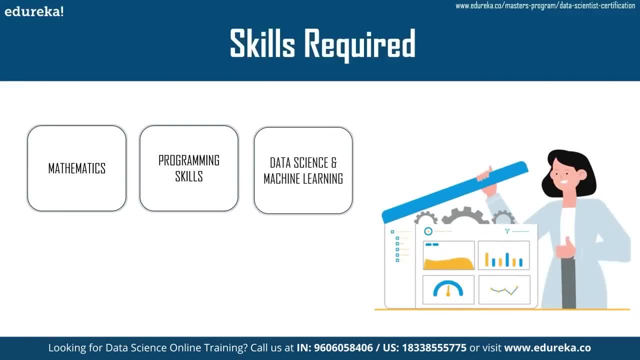 Then the third skill that you should have is data science and machine learning. So you should know all the concepts of data science and machine learning and you should know which concepts to implement in which scenarios. Moving on, the fourth skill is deep learning. 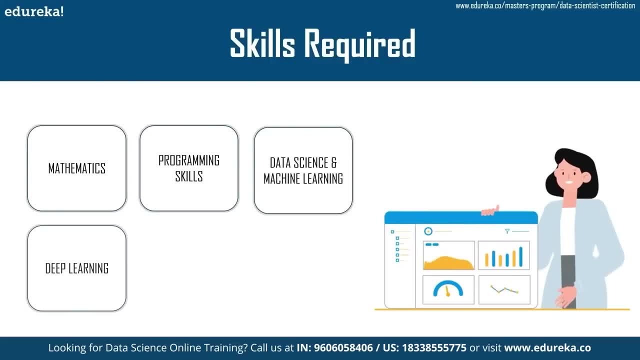 So it is very useful for an aspiring data scientist to not only know the concepts of data science and machine learning, but they should know deep learning so they are able to replicate neural networks to produce predictive models. The fifth skill that a data scientist does need to have is data visualization. 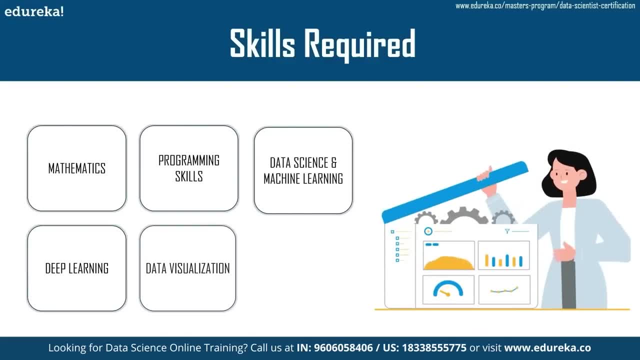 They should be able to take all the insights from models and systems that they've built and they should be able to apply them to their work. They should be able to put that in a form of a report where they can explain the insights in the simplest way possible, so even a layman who doesn't know technical terms is able. 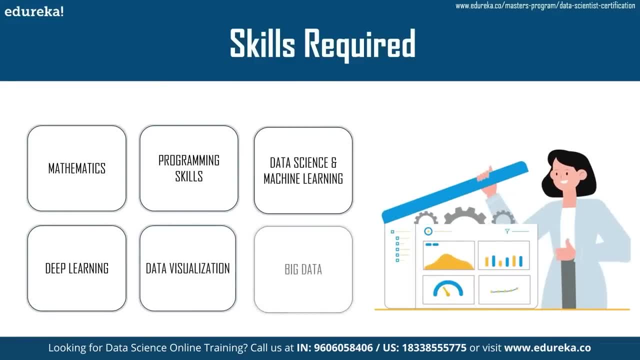 to understand what the data is trying to show. And the last skill that data scientists should know is big data. Data is all around us and we are producing more and more data every day, Data that is so huge that it's hard for normal people to comprehend. 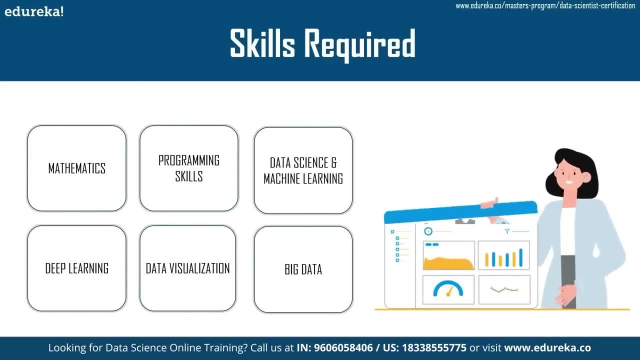 But data scientists need to know how to process big data. So processing big data and drawing insights from it requires different set of tools than processing normal data sets. So it is essential for data scientists to know how to work with big data. So I hope you got a picture of what kind of skills are required in order to fulfill the 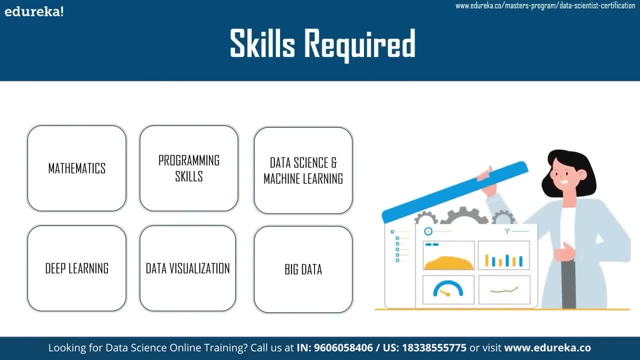 roles and responsibilities that we went over. Apart from these sort of technical skills, there are some soft skills that you need to be very good at as well, For example, good communication- Being able to abstract the complex ideas and explain them. And then the last skill that you need to be very good at is good communication. 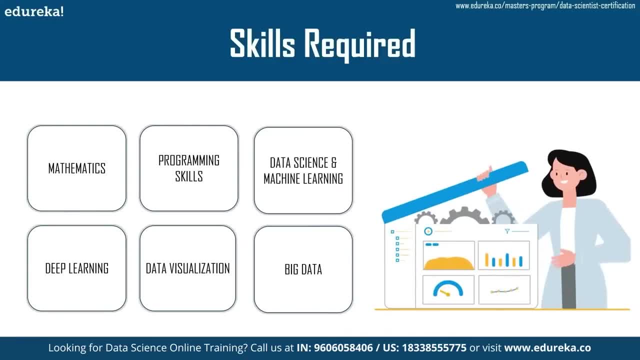 Being able to abstract the complex ideas and explain them. And then the last skill that you need to be very good at is great communication: Being able to abstract the complex ideas and explain them to stakeholders and business clients. And the last one is being familiar with the big data. 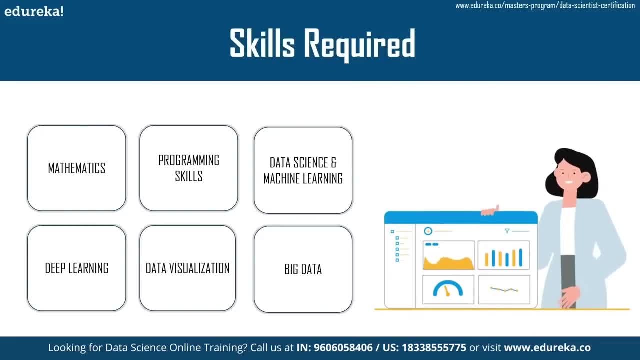 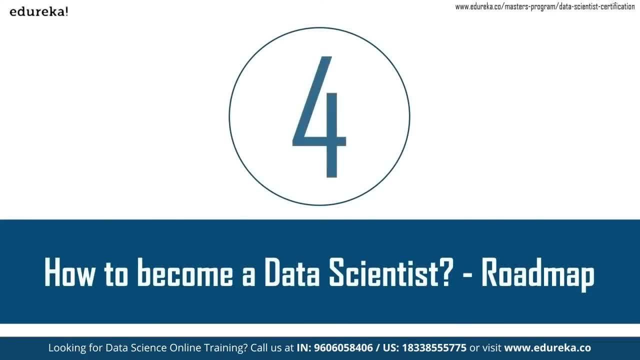 So, now that we got a good picture of roles and responsibilities of a data scientist, and what kind of skills are required in order to fulfill those roles and responsibilities, let's quickly find out how to become a data scientist by showing you a road map. So the first point on the journey to become a data scientist: 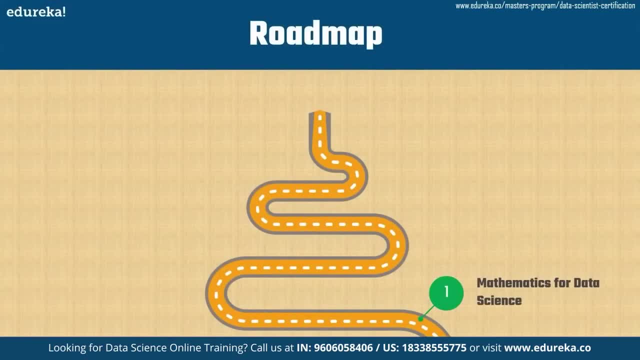 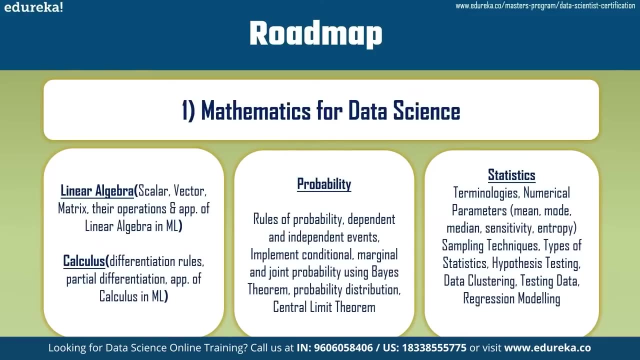 The first point I want to point out is to be well versed in the mathematics for data science. So what do I mean by mathematics? Well, not all mathematics is essential in order to become data scientists, but it's very useful to know four different, distinct concepts of math, namely linear algebra. 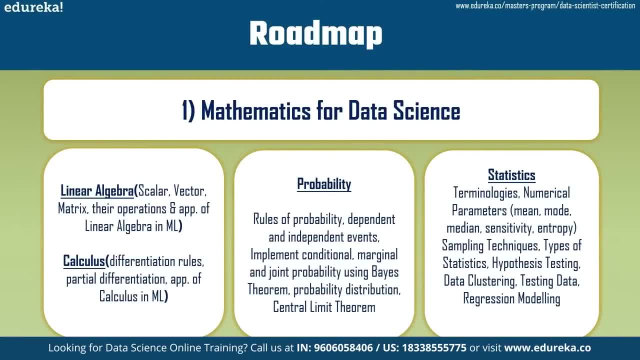 calculus, probability and statistics. You can probably get away with just learning probability and statistics, but if you want to become a really good data scientist, you will have to incorporate machine learning math, which entails linear algebra and calculus. So what do we need to learn in these topics? 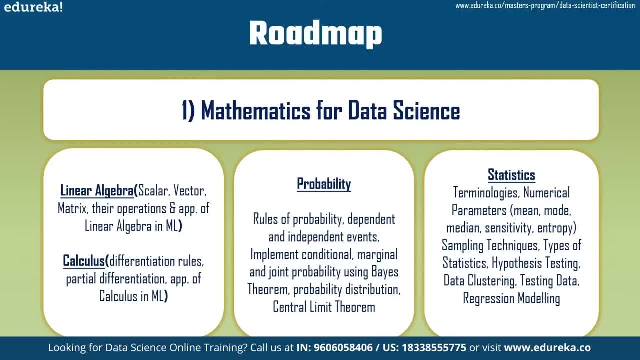 So in linear algebra you should know what a scalar vector matrix is and how to perform different types of operations on each one of these. Then you should also learn the application of linear algebra in machine learning. How is this subject- linear algebra- used in machine learning? 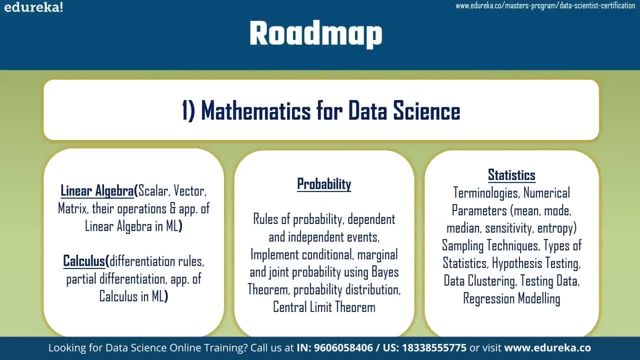 There would be no point of learning linear algebra without knowing its application in machine learning. It's like having a tool not knowing what that tool does. Next subject that you should learn is calculus. In calculus, please learn differentiation rules, partial differentiation and how all of these apply in machine learning. 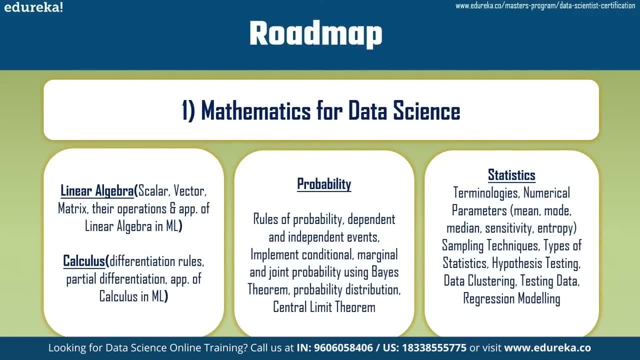 But those two topics that we just talked about- linear algebra and calculus- are relatively optional. if you just want to become an entry-level data scientist, The two of the most important topics are probability and statistics. So let's take a look at probability now. You should know rules of probability: dependent and independent events. 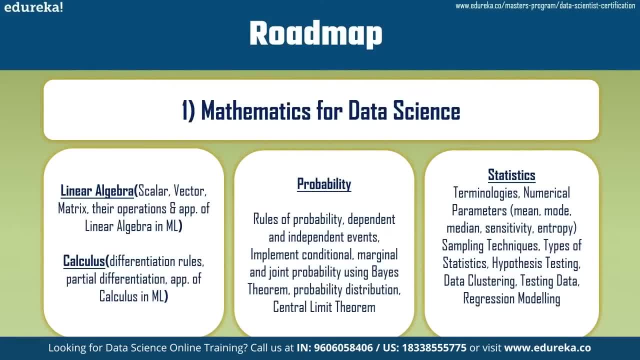 implement conditional, marginal, marginal and joint probability using Bayes' Theorem, probability distribution and central limit theorem, And in statistics you should know all the terminologies, Numerical parameters like mean mode, median sensitivity, entropy, sampling techniques, types of statistics. 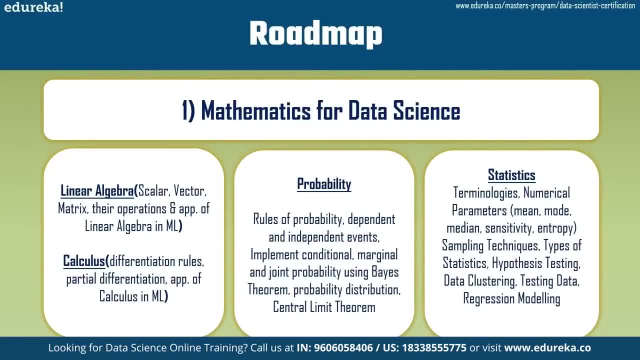 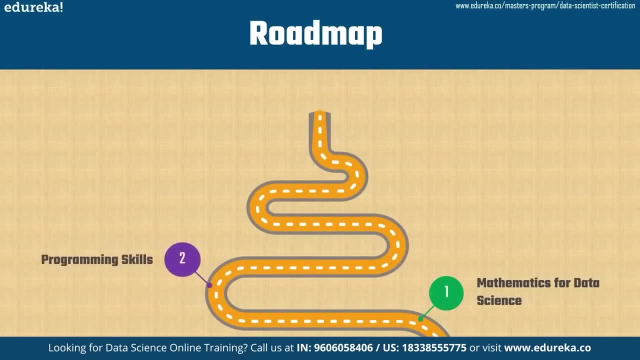 hypothesis testing, data clustering testing, data regression modeling. So the concepts that we just talked about of probability and statistics will form the basis that you will use to process data and gain insights. So as you're learning mathematics for data science, it's also a good idea to start acquiring programming skills. 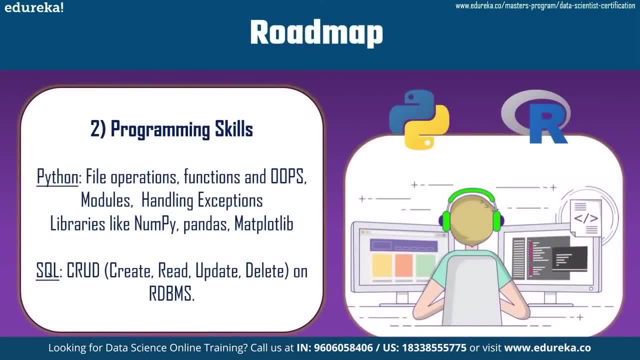 So, in programming skills, what do you need to know? Well, two of the most famous programming languages are R and Python, But especially Python is used in the entire world. In India, both Python and R are used heavily. Go with either one of them and you shouldn't have any problems. Remember earlier I mentioned that you don't have to be a programming wizard. 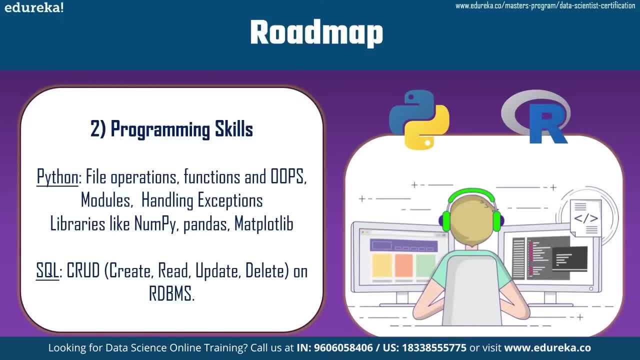 in order to get good at data science. Well, that is absolutely true. Let's now say that you're learning Python programming, So you start with the basic syntax and what data structures are. After that, you should start learning file operations, functions and object-oriented. 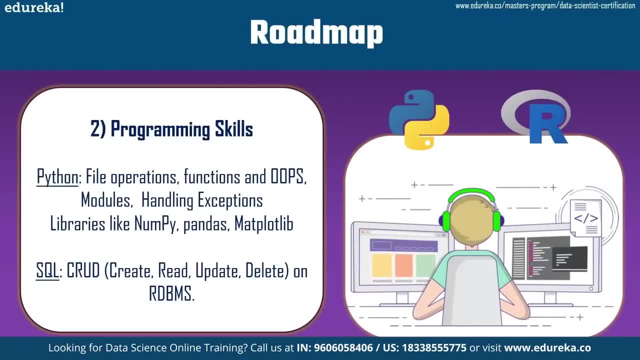 programming and how to use different modules in order to process data. You should also know how to handle exceptions and as you're learning the math, it's very good to start learning the libraries like NumPy, Pandas, Matplotlib. if you're learning the programming languages, R, learn the same concepts And for libraries, it is essential to learn. 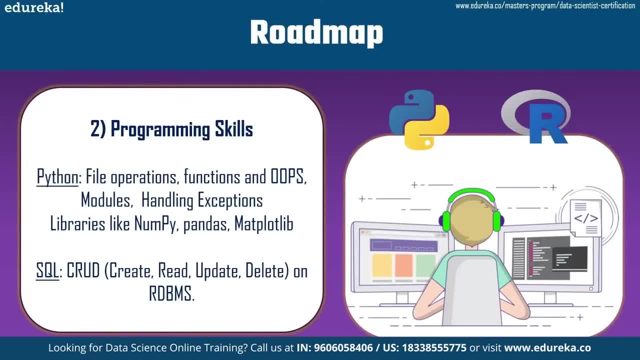 E1071 and POT or R programming. Apart from Python or R, you should also know a bit of SQL, as it forms the basis to understand any type of databases. You don't have to master SQL, just try to understand the CRUD, which is create, read, update and delete data in relational database systems. 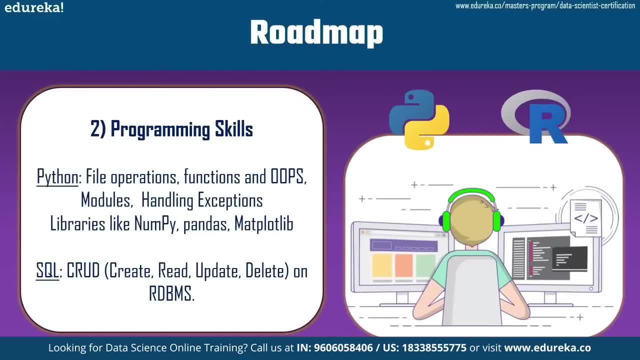 This is going to give you a good idea how databases work and how to query them, how to modify data, transform data and extract data. So let's say you've been learning math and programming skills and you've done some practical examples or real-world scenarios. 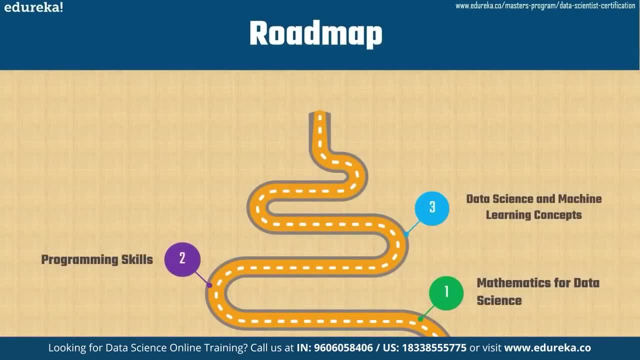 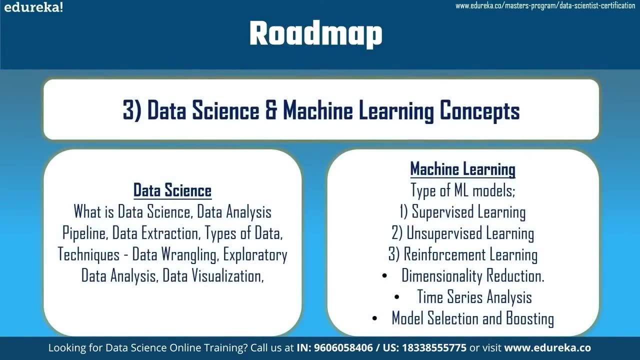 Now would be a good time to start learning different concepts in data science and machine learning. So why don't we take a look at data science? In data science, you should first obviously understand what data science is. You should know what data analysis pipeline is. then data analysis. 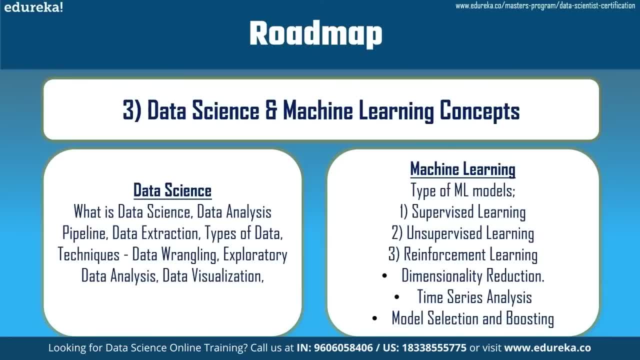 extraction, types of data techniques like data wrangling, exploratory data analysis, data visualization. And when it comes to machine learning, you should definitely know what type of machine learning models are there, namely supervised learning, unsupervised learning, reinforcement learning, And there are various algorithms within each one of them, So you should 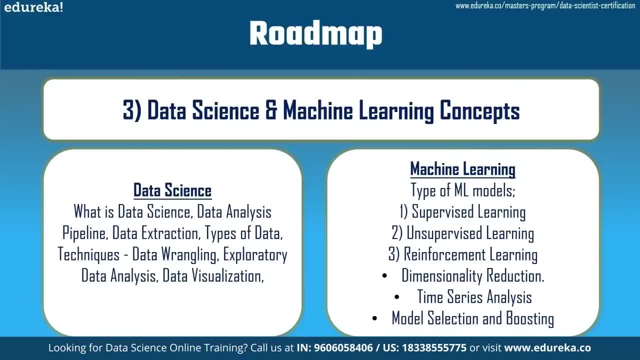 know them as well. Apart from these, you should also learn dimensionality reduction concepts, time series analysis And then, depending on the kind of situation and problem at hand, you should also learn how to do model selection and boosting. So at this point you're getting. 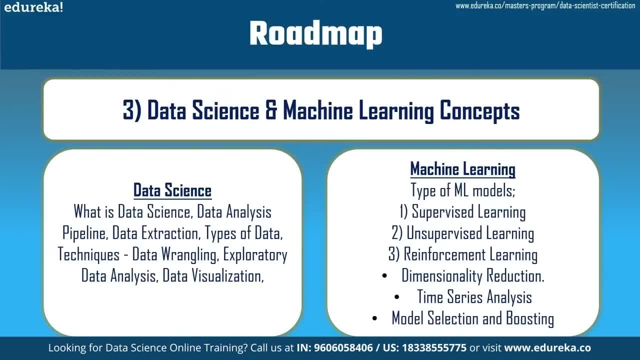 quite good and deep into data science, And as you learn all of these topics one by one, you should do practical examples using Python or R and make sure that you really have a grasp of all these concepts, Because these are the core concepts that will help you get your foot in the door. 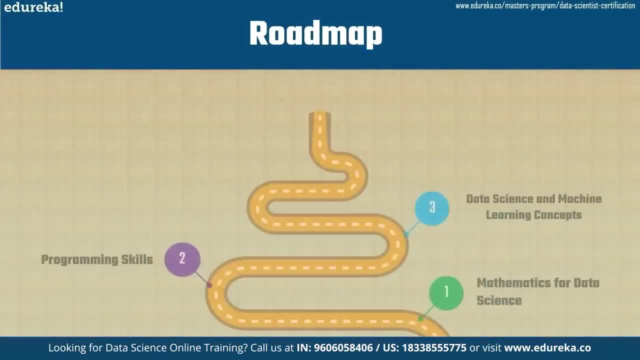 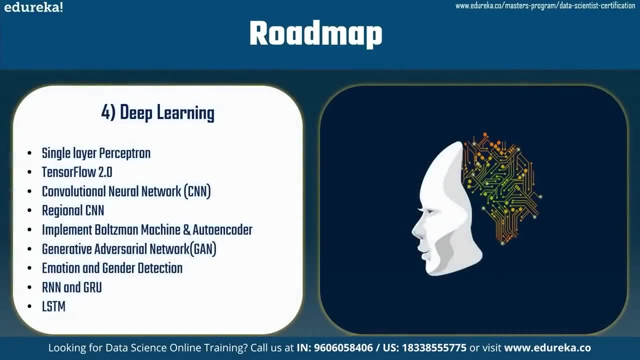 and help you become a data scientist. So what is next? So the fourth skill is deep learning concepts and know how to implement them. So in deep learning you should know single layer perception, TensorFlow 2.0, convolutional neural networks, regional CNN, implement Boltzmann machine and autoencoder generative adversarial network. 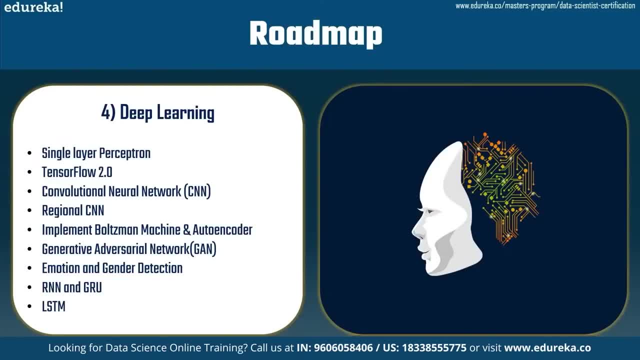 emotion and gender detection, RNN and GRU, LSTM. If you haven't heard about these concepts, then you must be feeling overwhelmed. Let me put your mind at ease. These are not too difficult. especially after learning machine learning and data science concepts, You should be able to pick them up quite easily. So a big 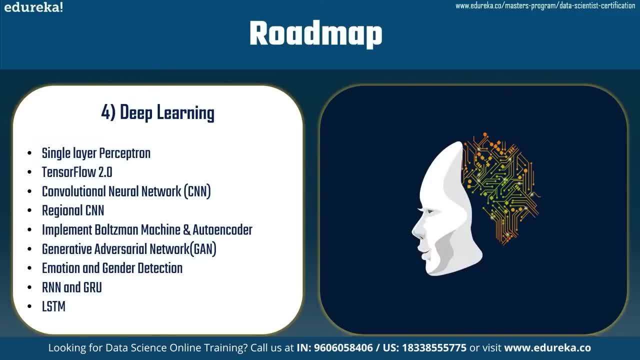 part of becoming a data scientist is to make sure that whatever you're learning conceptually, you should be able to implement it in real life scenarios, And so just learn the basics and know how to implement them. Moving on to the next skill that you should have is big data and its tools. 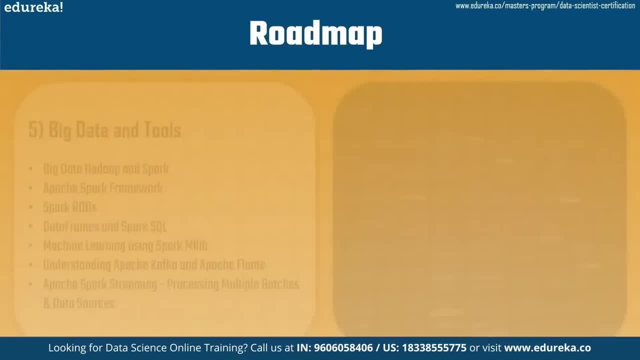 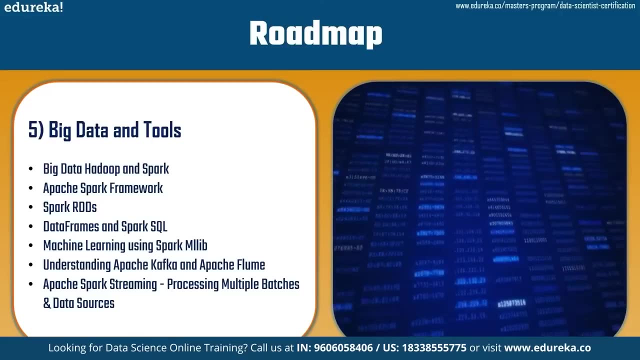 like PySpark, Hadoop And so on. Now we're entering the realm of big data. For a data scientist, it is very essential, especially these days, to know how to handle big data. So you might ask: what are the different? 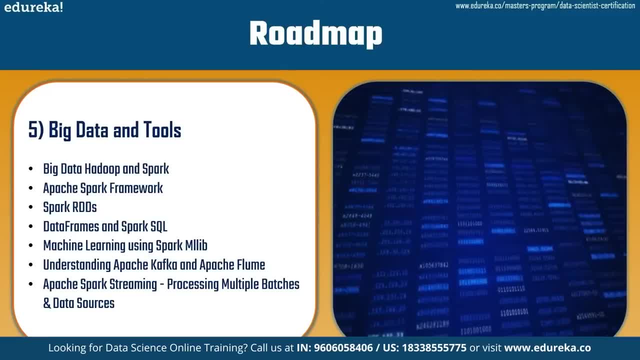 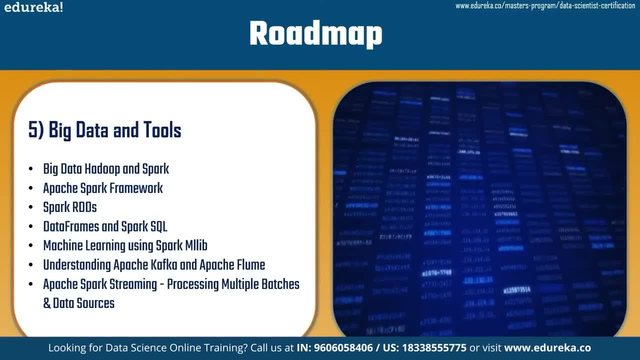 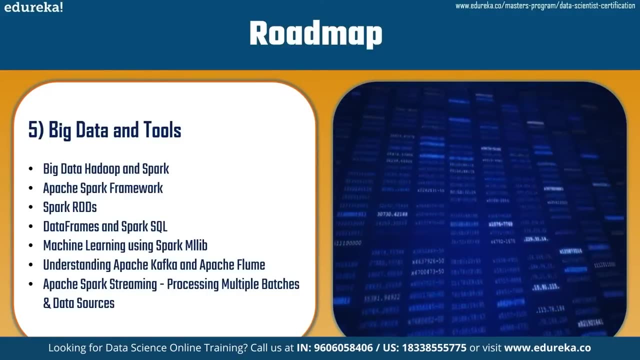 big data tools and concepts. So here they are: Big data Hadoop and Spark, Apache, Spark framework, Spark RDDs, DataFrames and Spark SQL machine learning using Spark MLlib, understanding Apache, Kafka and Apache Flume, Apache Spark streaming, processing multiple batches and. 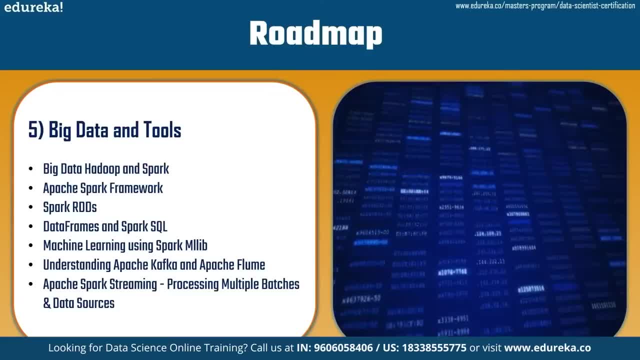 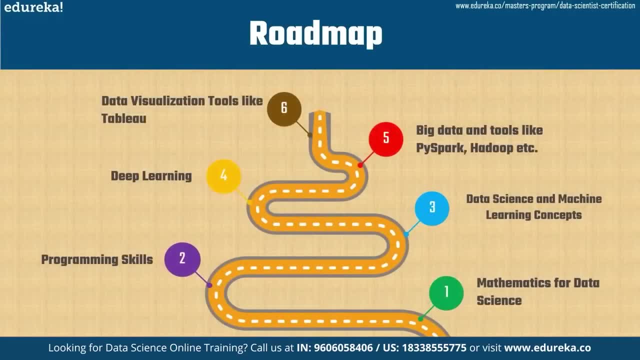 data sources. Again, don't dive too deep into these topics. You should just know the basics, Don't be overwhelmed and move on to the next thing, Last skill to acquire, which is data visualization, And so you should know tools like Tableau. So in data visualization, you should learn basic visual. 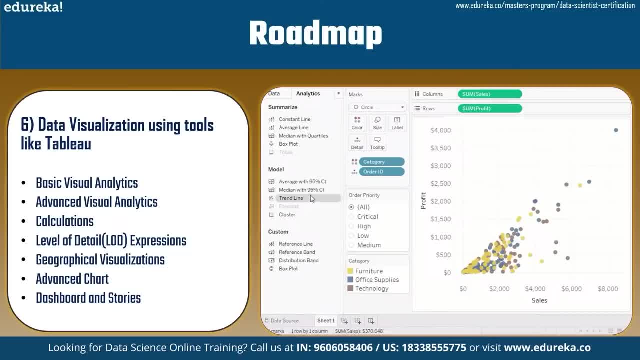 analytics, advanced visual analytics, calculations, level of detail, LOD expressions, geographical visualizations, advanced charts, dashboard and stories, And so obviously you can use different tools. The tools that are used most widely across the world are Tableau and Power BI, So these are very 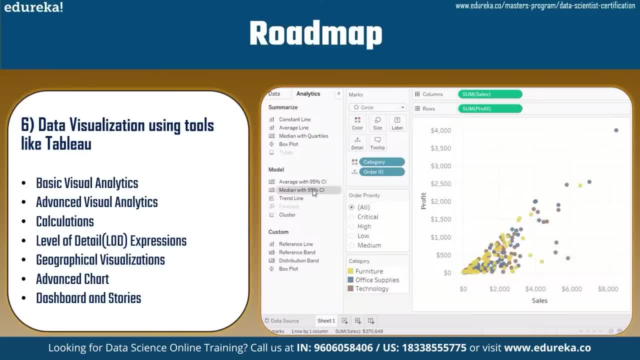 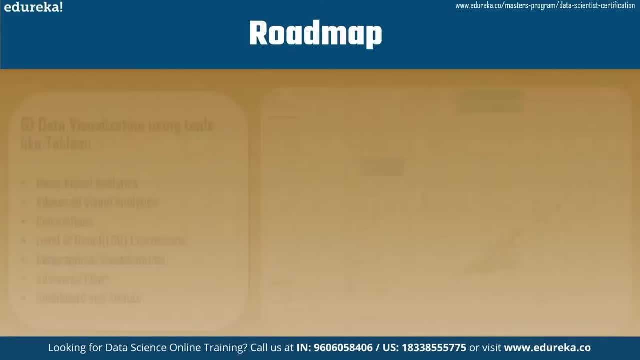 powerful tools and they're very easy to use, very user friendly, and learning them will enable you to represent data in a very spectacular fashion. So, wrapping up, so you should start your journey with mathematics for data science. Along with that, you can start learning programming skills. 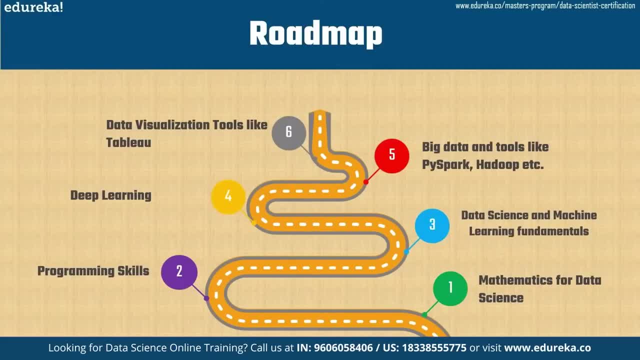 as well. Then learn data science and machine learning fundamentals and concepts. Know how to implement with data science as well. Know how to implement with software and other software, and know how to implement with software and other software and other software and other software and concepts using Python or R. Then move on to learning deep learning concepts and 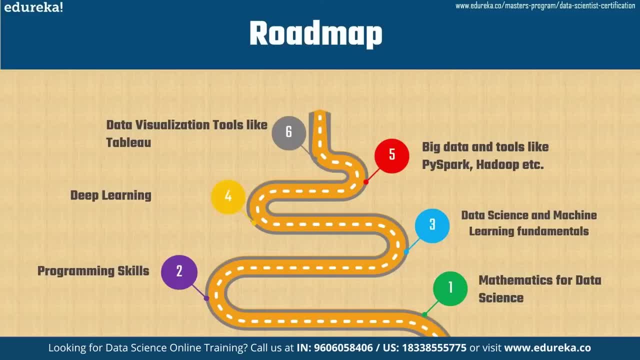 know how to implement those as well. After that, you should know how big data works and what are the tools that are industry standard, like we discussed. And, finally, you should learn how to visualize the different insights, patterns and trends that you have gathered by implementing different 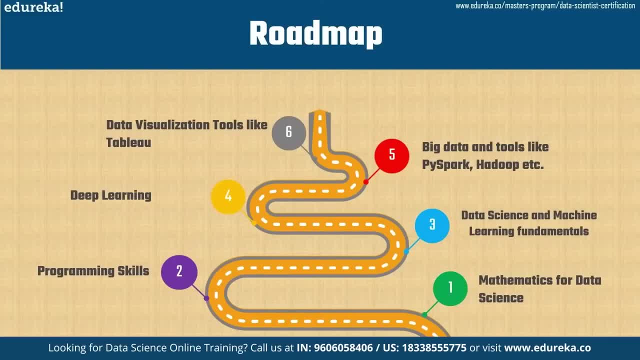 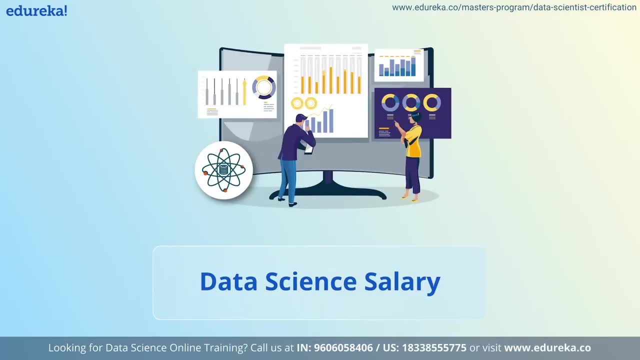 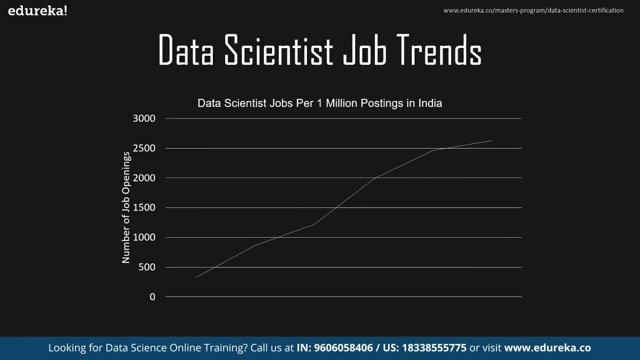 models and systems, And I can guarantee that if you follow this roadmap judiciously, then you will become a data science wizard Moving ahead. let's look at data scientist job trends. This is a graph of number of job openings for data scientists. per 1 million postings, What? 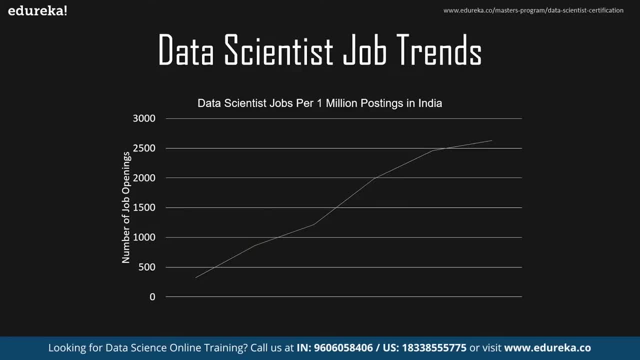 we can infer from the graph is that data scientist jobs have a growing trend and this trend is expected to continue in the coming years. Apart from this, statistics also show that data scientist jobs are growing in the coming years. Also say that 97% of data scientist jobs are on full-time basis. 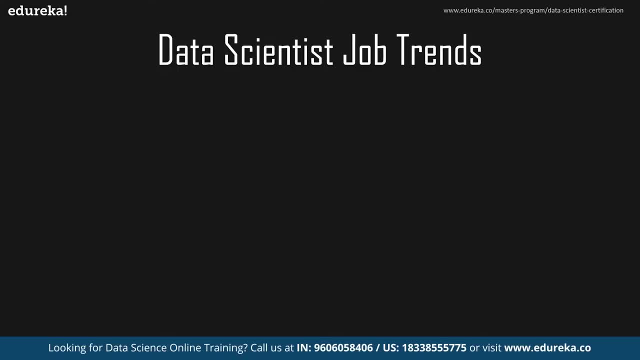 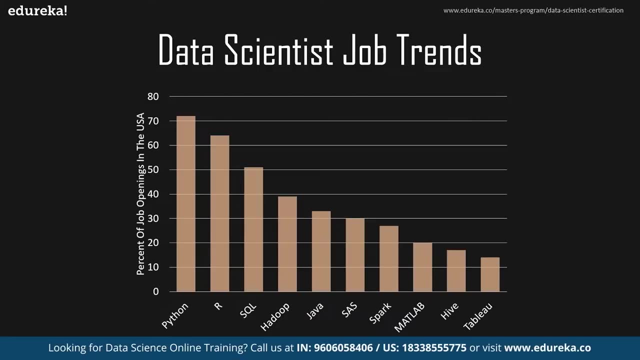 whereas only 3% are part-time. Also, one of the important things to get a job is mastering the required skills. The most in-demand skills that every company looks for in a data scientist are listed here, along with the corresponding percentage of job openings. This doesn't necessarily mean you need to master all. 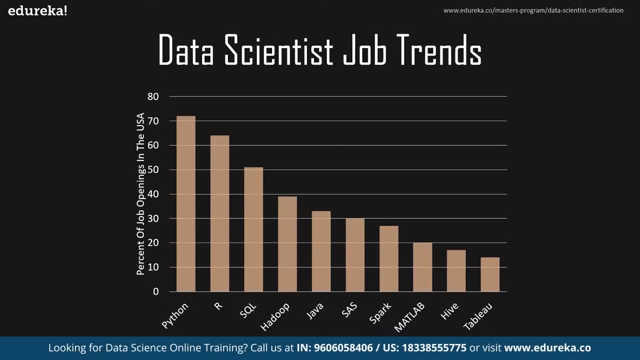 these skills in order to find a job as a data scientist. In fact, mastering job openings is just 3 core skills, which are Python, R and SQL, can provide a solid foundation for 7 out of 10 job openings today as data scientist. 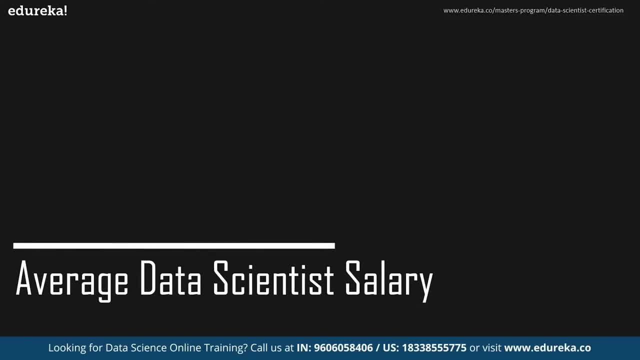 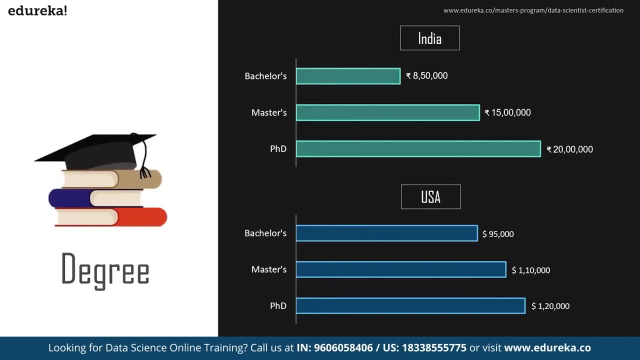 Now let's look at the average data scientist salary based on different criterias. First, let's look at the salary based on degree. As we can see, both in India and the United States, there is a clear correlation between degree level and the associated salary: Higher the degree. 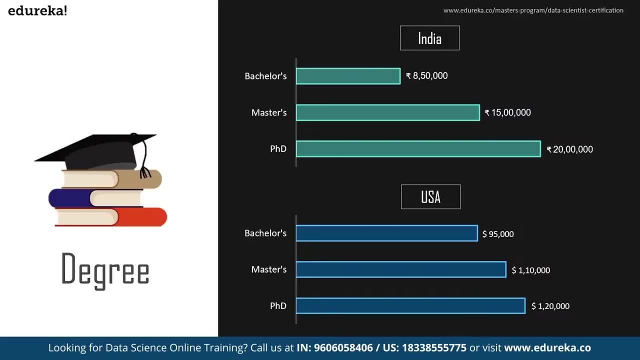 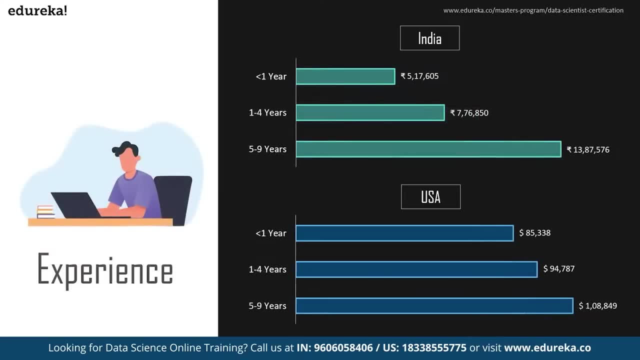 better the salary. Hence PhD holders earn the highest as a data scientist compared to others. The next criteria is experience. Your experience plays a crucial role in deciding your salary, Be it India or the United States. typically, more experience in the relevant field results in higher. 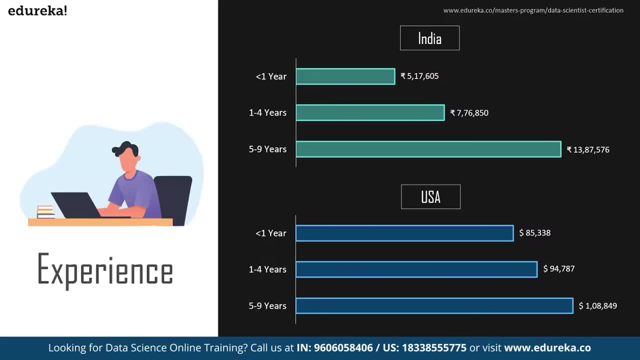 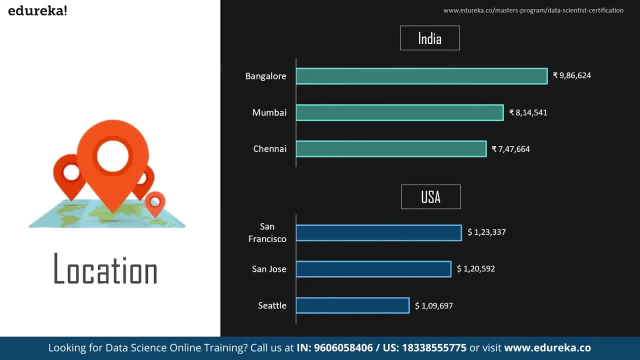 pay, but definitely up to a certain point. In case of stagnant salary, even with a great experience, consider learning new skills to outstand in the job market. The next criteria we are going to discuss is location. Not surprisingly, geographic location is one of the biggest factors. 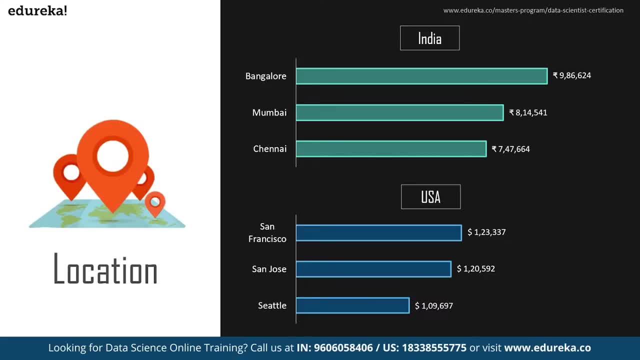 when it comes to how much you can earn in a given profession. As a rule of thumb, salaries are going to be higher in larger cities such as Mumbai in India or New York in the United States than they are in rural locations. However, it's important to remember that cost of living in rural areas is much less than in big cities. Considering these factors, we have found out cities like Bangalore in India and San Francisco in the United States still top the list of providing a high salary- The last criteria. we are going to look. 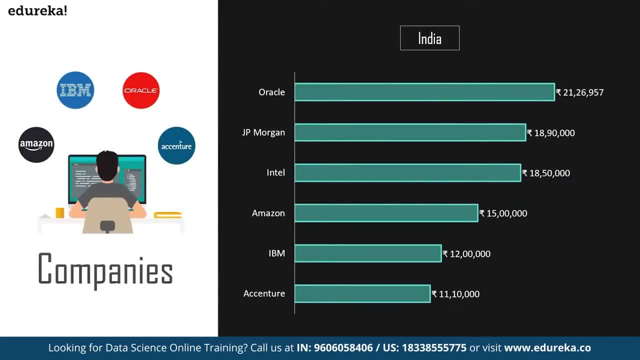 at includes companies. There are a large number of companies that are now looking for data scientists, but it's essential to find companies that commonly hire data scientists and also provide them withading salary so that they can keep a good pay. Hence we have made a list of companies that are ranked similar in India. and the United States for data scientist salary. The companies include Oracle, JP Morgan, Intel, Amazon, IBM and Accenture. Similarly, you can see the salary in each company for a data scientist in the United States. Now let's quickly discuss the future scope for data scientists. 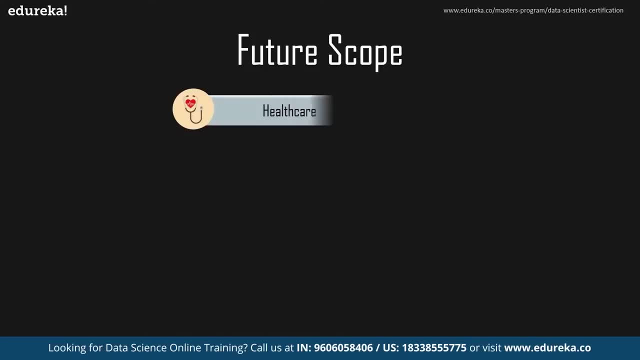 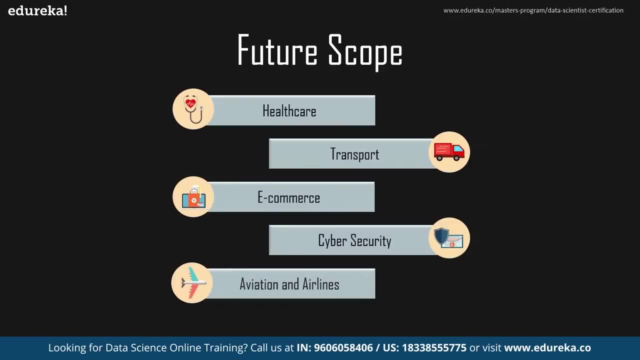 Data scientists are high in demand in industries like healthcare, transport, e-commerce, cyber security. along with aviation and airlines, The healthcare industry is extensively making use of data scientists to develop a system that can predict health risks. They are also being hired for the process of drug discovery, to provide insights into optimizing and increasing the 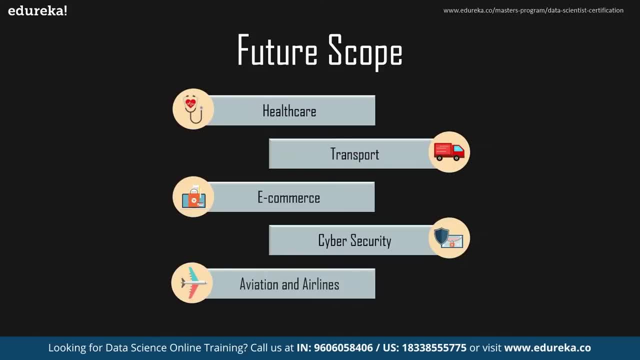 success rate of predictions. The travel and transportation industry is one of the most important industries in India. The transport industry always had to handle large amount of data. Conventional ways of handling data is no more enough. Hence using data scientists, efficient data analysis and prediction. 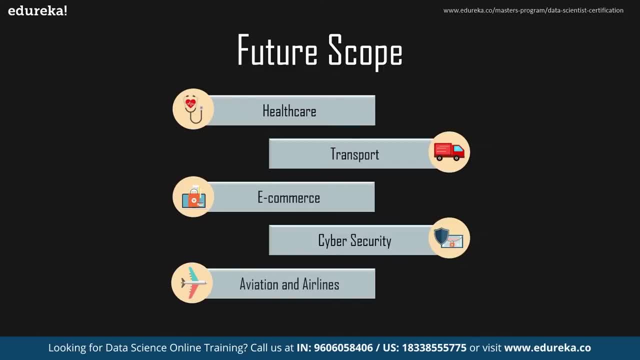 can be done to improve business process and customer service In the e-commerce industry. to improve user experience and personalize service and suggestion, they use customer data. For handling this, user data companies need data science professionals to understand customer behavior and then market them the correct product. 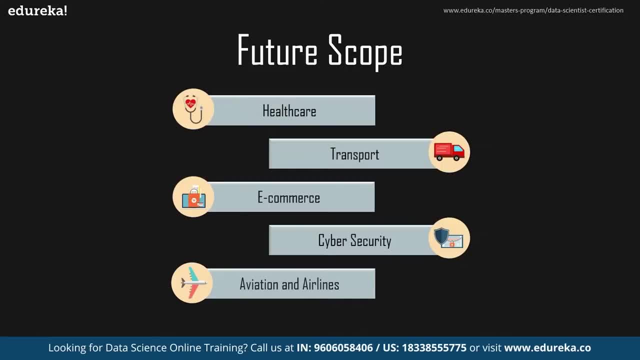 The next industry is cyber security. Due to an increase in online transactions and internet usage, fraudulent activities have also increased. Organizations are now adopting data scientists to apply techniques to detect such fraudulent activities and to prevent losses. The last industry that we are going to discuss is aviation and airlines. 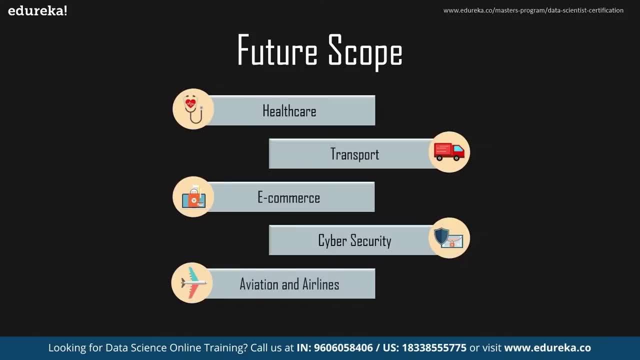 In the aviation and airlines industry, companies use data for putting up their prices, optimizing routes and carrying out pre-emptive maintenance. To develop each of this system requires knowledge in the field of data science. This leads to substantial increase in the need of data scientists. 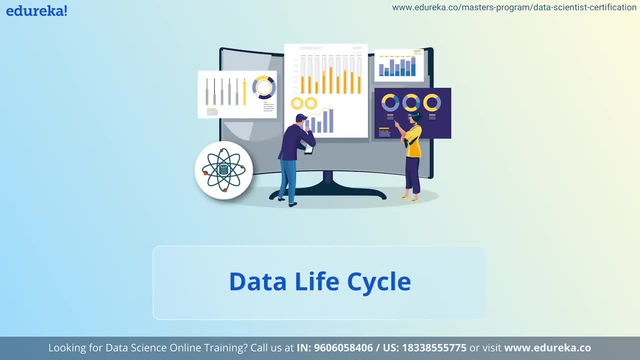 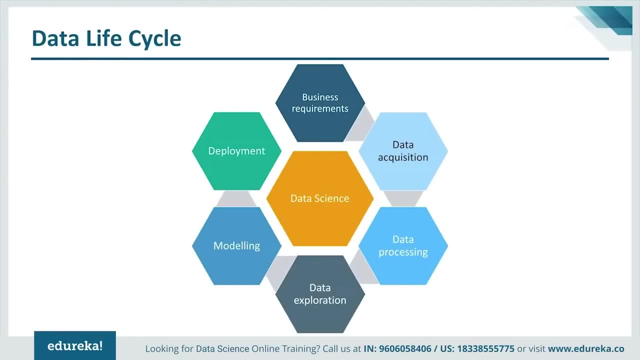 Now let's move ahead and look at the data life cycle. So, guys, there are basically six steps in the data life cycle. It starts with a business requirement. Next is the data acquisition. After that you'll process the data, which is called data processing. 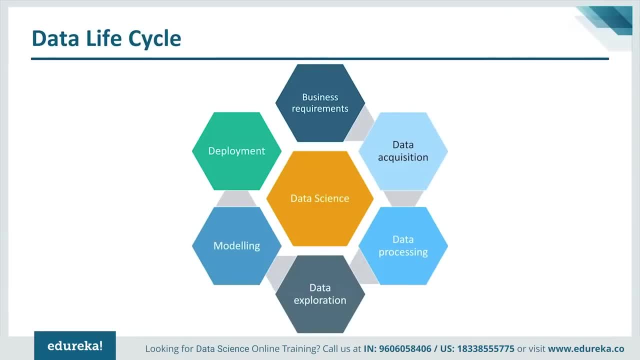 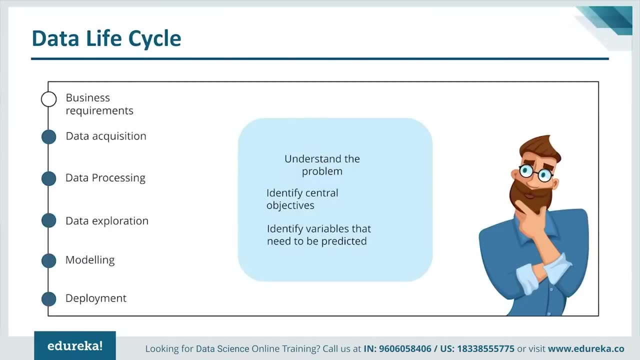 Then there is data exploration, modeling and, finally, deployment. So, guys, before you even start on a data science project, it is important that you understand the problem you're trying to solve. So, in this stage, you're just going to focus on identifying the central objectives of the project. 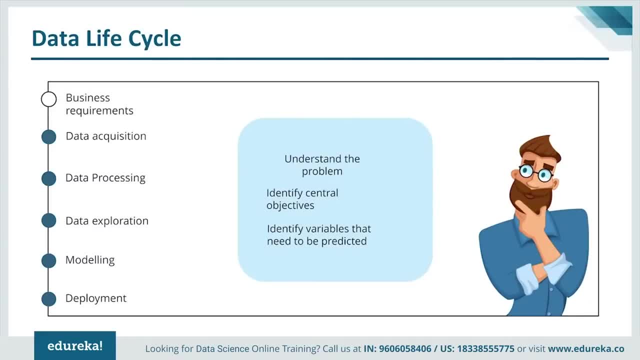 And you'll do this by identifying the variables that need to be predicted. You'll also need to identify the things that need to be predicted. Next up, we have data acquisition. Okay, so, now that you have your objectives defined, it's time for you to start gathering the data. 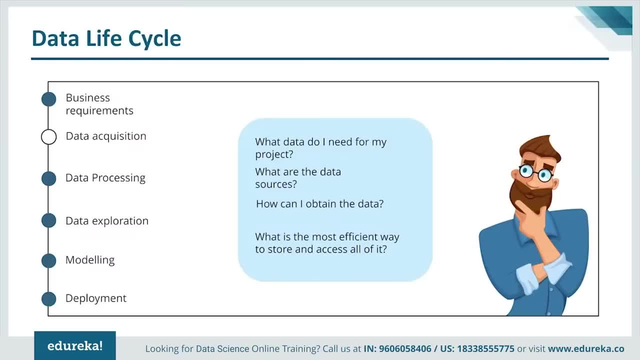 So data mining is the process of gathering your data from different sources. At this stage, some of the questions you can ask yourself is: what data do I need for my project, Where does it live, How can I obtain it And what is the most efficient way to store and access? 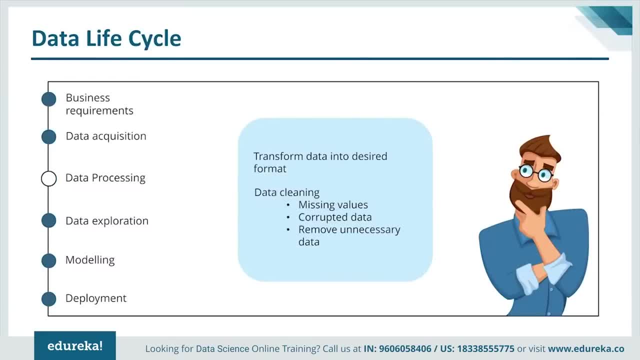 all of it. Next up, there is data processing. Now, usually all the data that you collect is a huge mess. Okay, it's not formatted, it's not structured, it's not cleaned. So if you find any data set that is cleaned and it's packaged well for you, then you've actually won the lottery. 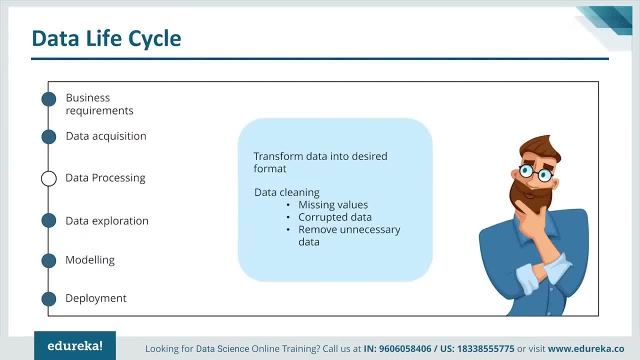 because finding the right data takes a lot of time and it takes a lot of effort, And one of the major time consuming tasks in the data science process is data cleaning. Okay, this requires a lot of time. it requires a lot of effort because you have to go through the entire data set to find 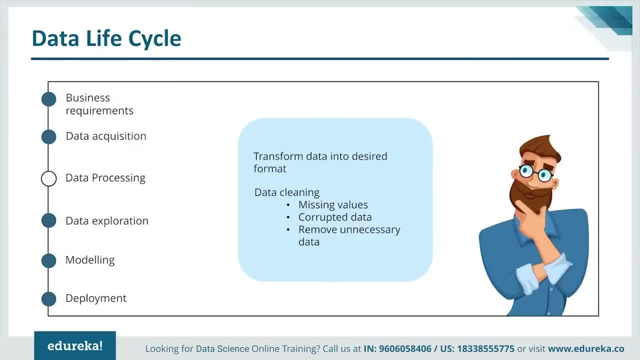 out any missing values or if there are any inconsistent values or corrupted data, And you also find the unnecessary data over here and you remove that data. So this was all about data processing. Next we have data exploration. So now that you have sparkling clean set of data, 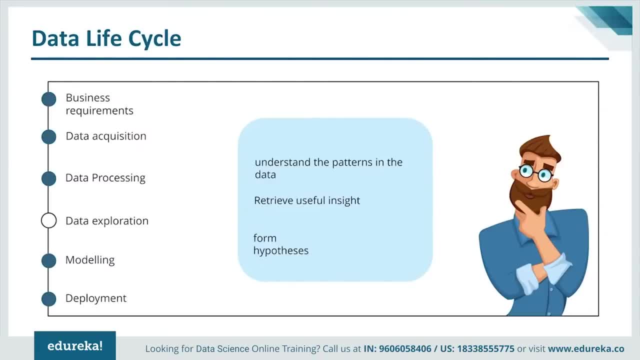 you are finally ready to get started with your analysis. Okay, the data exploration stage is basically the brainstorming of data analysis. So, in order to understand the patterns in your data, you can use histogram. you can just pull up a random subset of data and plot a histogram. you can even create interactive visualizations. 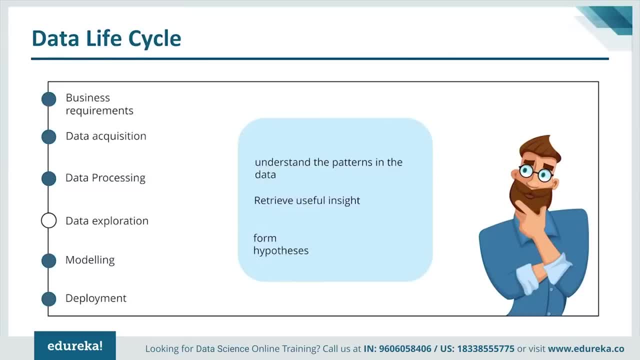 This is the point where you dive deep into the data and you try to explore the different models that can be applied to your data. Next up, we have data modeling. So, after processing the data, what you're going to do is you're going to carry out model training. Okay, now, model training is. 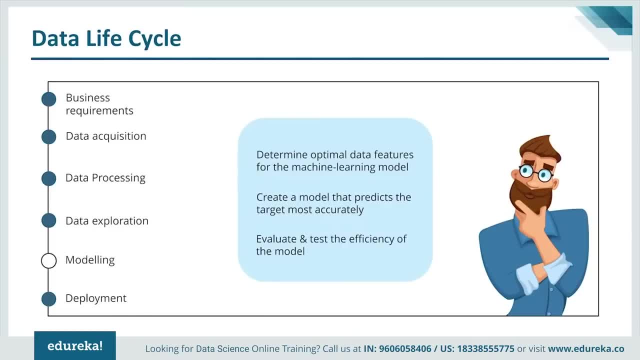 basically about finding the model that answers the questions more accurately. So the process of model training involves a lot of steps. So firstly, you'll start with the model training. you'll start by splitting the input data into the training data set and the testing data set. 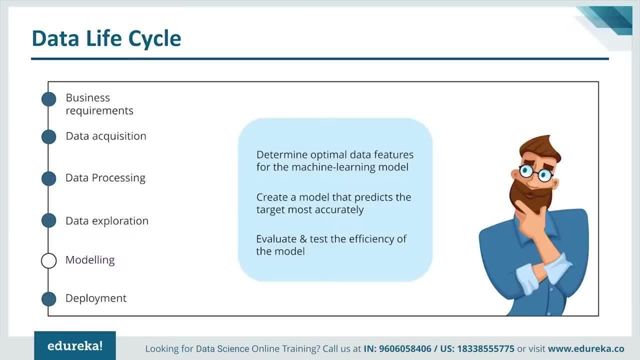 Okay, you're going to take the entire data set and you're going to separate it into two parts: One is the training and one is the testing data. After that, you'll build a model by using the training data set And once you're done with that, you will evaluate the training and 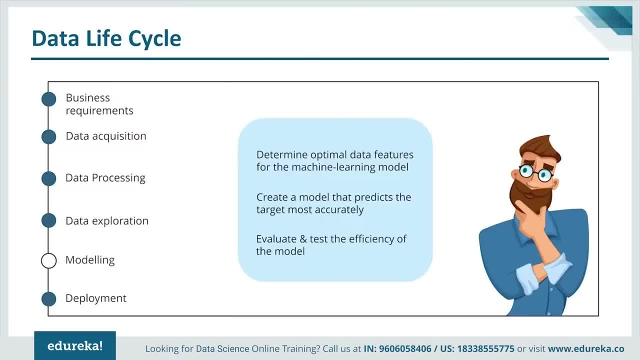 the test data set. Now, to evaluate the training and testing data, you'll be using a series of machine learning algorithms. After that you'll find out the model which is the most suitable for your business requirement. So this was mainly data set. 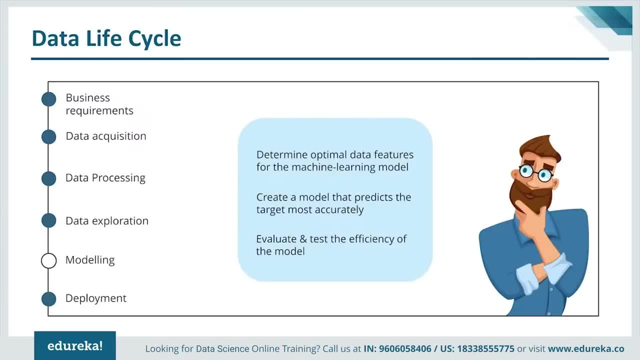 modeling. okay, this is where you build a model out of your training data set and then you evaluate this model by using the testing data set. next we have deployment. so there's a goal of the stage is to deploy a model into a production, or maybe a production like environment. so this is basically done. 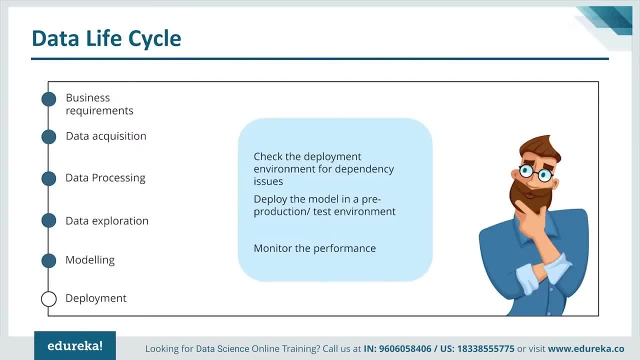 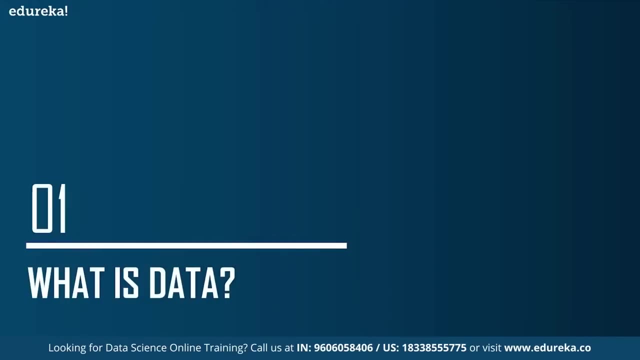 for final user acceptance, and the users have to validate the performance of the models, and if there are any issues with the model or any issues with the algorithm, then they have to be fixed in this stage. let's move ahead and take a look at what is data now? this is a quite simple question. if I ask any of you what, 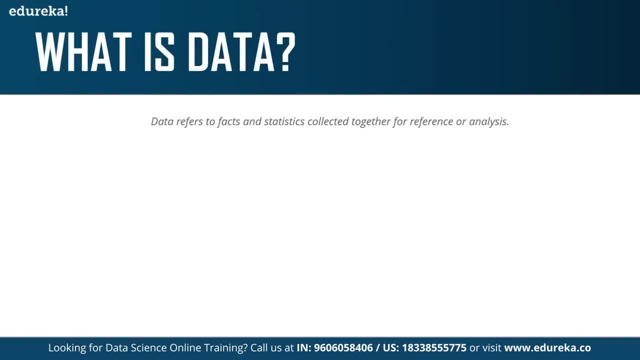 is data. you'll see that it's a set of numbers or some sort of documents that I've stored in my computer. now, data is actually everything. all right, look around you: there is data everywhere. each click on your phone generates more data than you know you now. this generated data provides insights for analysis and helps us make 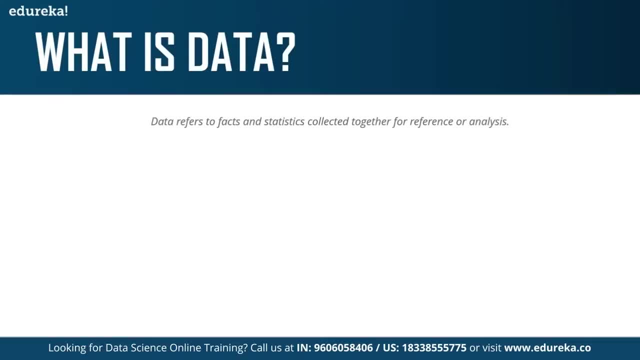 better business decisions. this is why data is so important. to give you a formal definition, data refers to facts and statistics collected together for reference or analysis. all right, this is the definition of data in terms of statistics and probability. so, as we know, data can be collected, it can be measured. 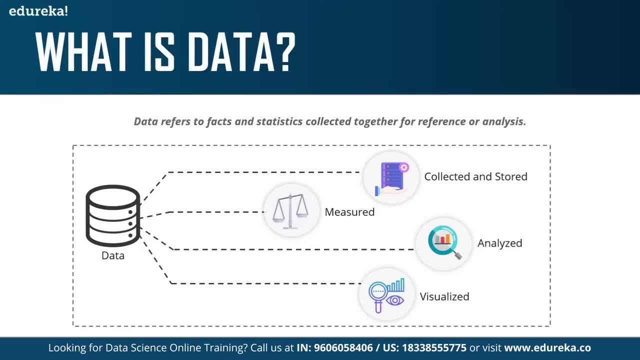 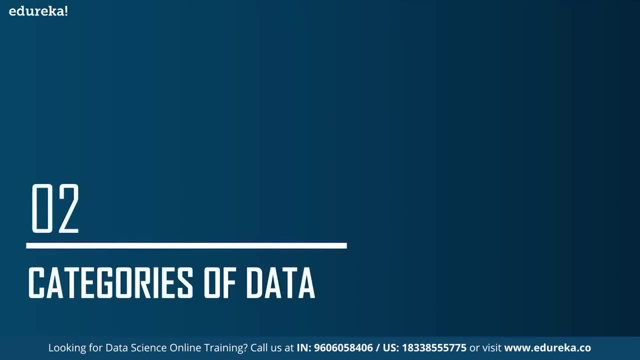 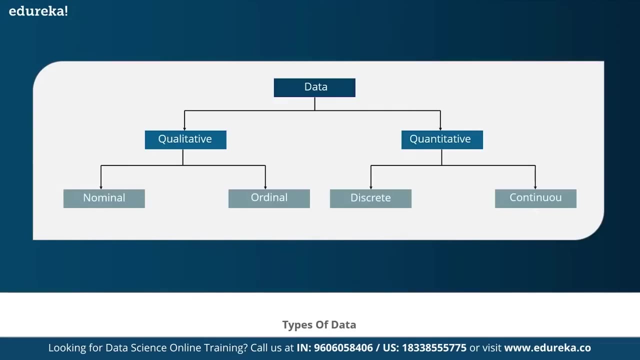 and analyzed. it can be visualized by using data, STATISTICAL MODELS and graphs. now, Data is divided into two major subcategories, alright, so first we have qualitative data and quantitative data. these are the two different types of data. under qualitative data, we have nominal and ordinal data, and under quantitative data we have discrete and 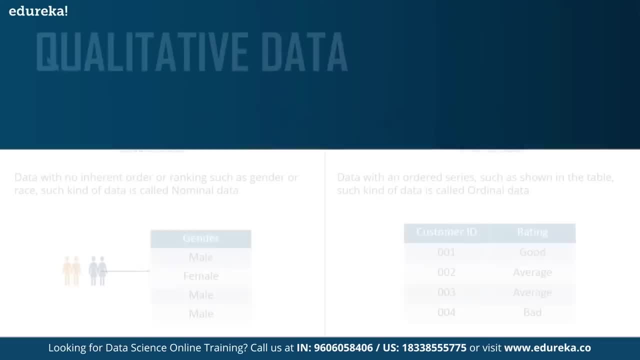 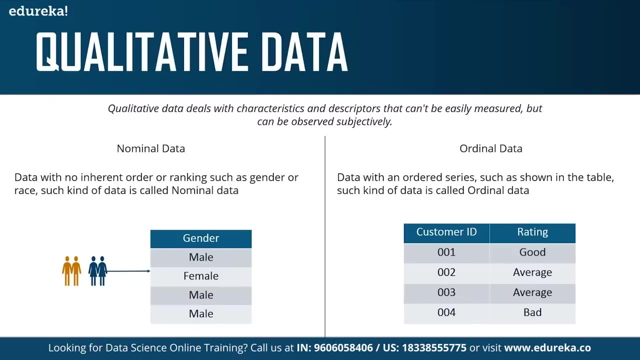 continuous data. now let's focus on qualitative data. now. this type of data deals with characteristics and descriptors that can't be easily made measured, but can be observed subjectively. now qualitative data is further divided into nominal and ordinal data, so nominal data is any sort of data. 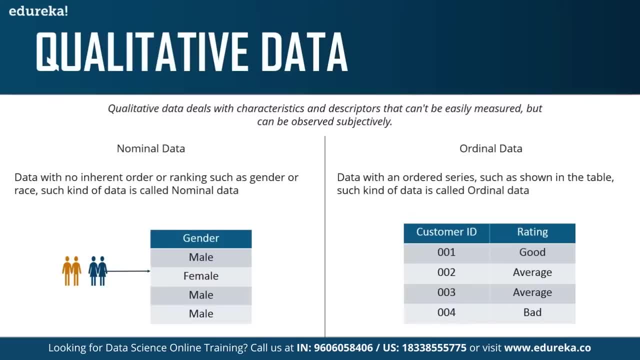 that doesn't have any order or ranking. okay, an example of nominal data is gender. now, there is no ranking in gender. there's only male, female or other right. there is no one, two, three, four or any sort of ordering in gender. race is another example of nominal data. now, ordinal data is basically an ordered 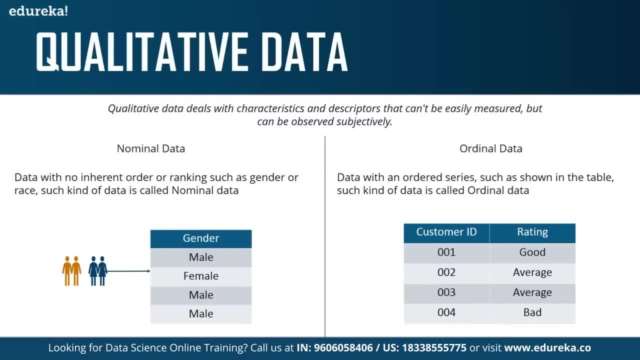 series of information. okay, let's say that you went to a restaurant. okay, your information is stored in the form of customer ID, all right. so basically, you are represented with a customer ID. now you would have rated their service as either good or average. all right, that's how an ordinal data is, and 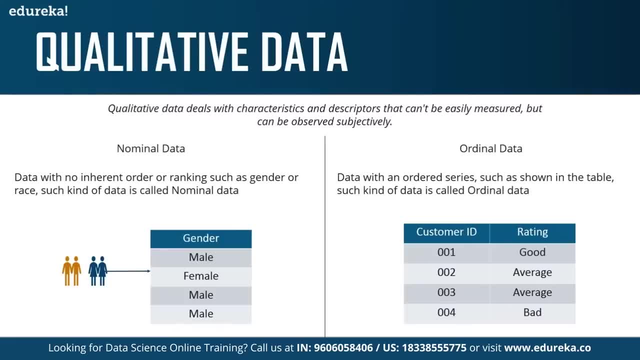 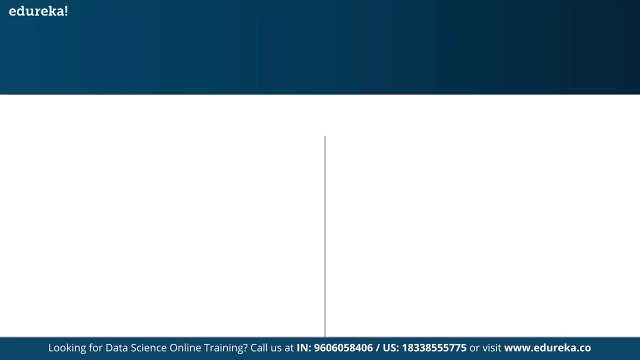 similarly, they'll have a record of other customers. who was it. the rest is along with their ratings. all right, so any data which has some sort of sequence or some sort of order to it is known as ordinal data. all right, so, guys, this is pretty simple to understand. now let's move on and look at quantitative data. so 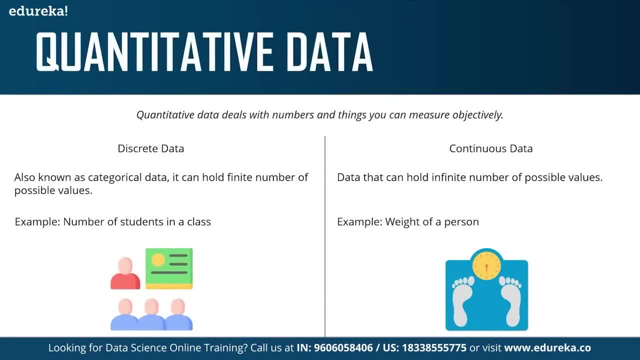 quantitative data basically deals with numbers and things. okay, you can understand that by the word quantitative itself. quantitative is basically quantity, right? so it deals with numbers. it deals with anything that you can measure objectively. all right, so there are two types of quantitative data. there is discrete and 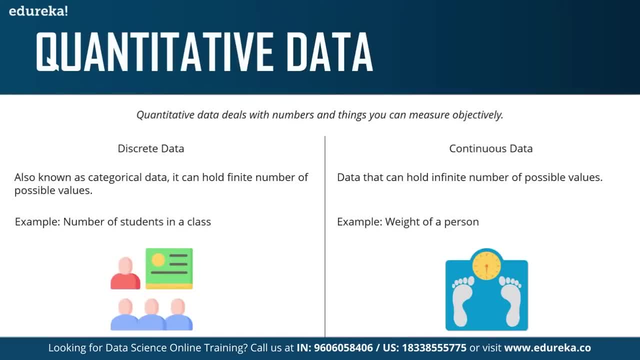 continuous data. now discrete data is also known as categorical data- and it can hold a finite number of possible values. now the number of students in a class is a finite number. all right, you can't have infinite number of students in a class. let's say in your fifth grade there were hundred students in your 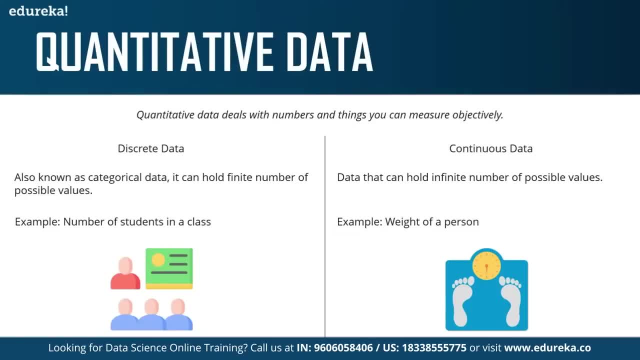 class. all right, there weren't infinite number, but there was a definite finite number of students in your class. okay, that's. Medicaid doesn't mean that you obtain infinite number of students per step. okay, yeah, you need to have two common sources. for me, someone who does that. 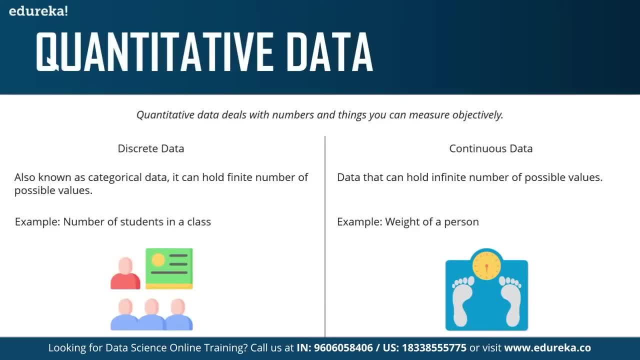 seems like a pretty easyitted question. you can say that students rating your academic list also depends primarily on the time period of the school year. if students are on a midterm andilian tour, if students are on ltr- students up to three or four years of age- then theЧ hel Gobm of well write higher level. 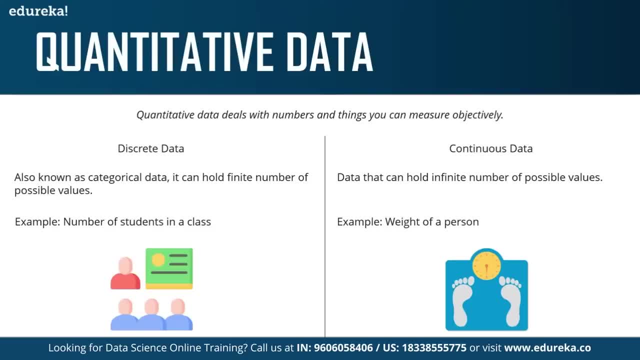 of studentuchtiож勉 aufgere ganhar am somebody decent is considered a delivery values, right? so this is what I mean by continuous data. all right, this is the difference between discrete and continuous data, and also I'd like to mention a few other things over here. now there are a couple of types of variables. 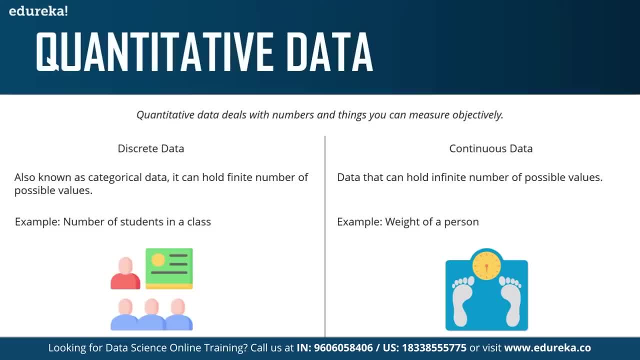 as well. all right, we have a discrete variable and we have a continuous variable. discrete variable is also known as a categorical variable. all right, it can hold values of different categories. let's say that you have a variable called message and there are two types of values that this variable can hold. let's 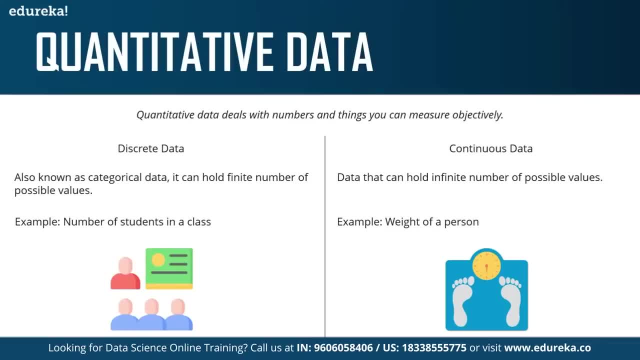 say that your message can either be a spam message or a non spam message. okay, that's when you call a variable as discrete or categorical variable, all right, because it can hold values that represent different categories of data. now, continuous variables are basically variables that can structure the data in a particular way. so let's say, for example: if I want to, 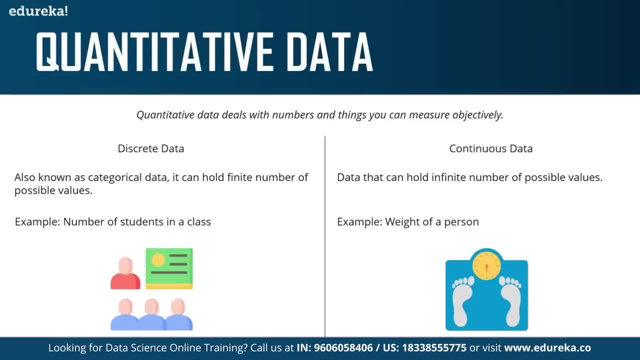 store infinite number of values. so the weight of a person can be denoted as a continuous variable. all right, let's say there is a variable called weight and it can store infinite number of possible values. that's why we'll call it a continuous variable. so, guys, basically, variable is anything that can store a. 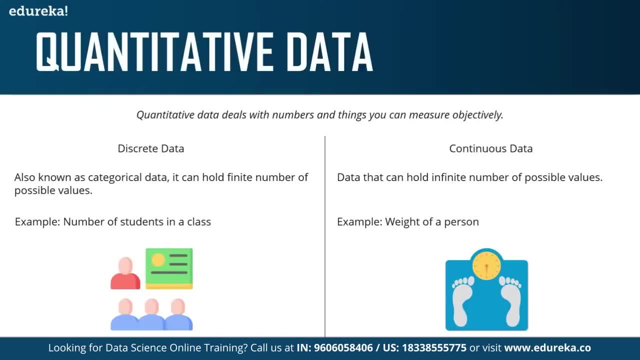 value right. so if you associate any sort of data with a variable, then it will become either discrete variable or continuous variable. that is also dependent and independent type of variables. now we won't discuss all of that in depth because that's pretty understandable. I'm sure all 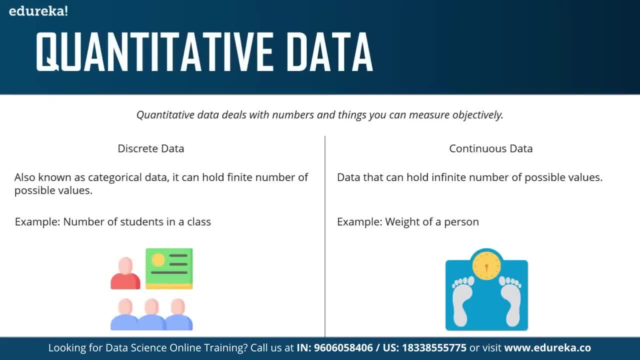 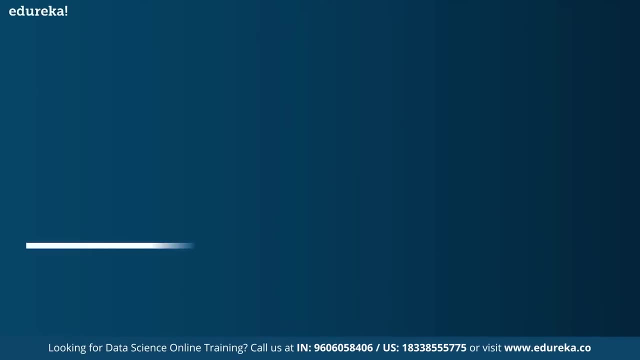 of you know what is independent variable and dependent variable, right, dependent variable is any variable whose value depends on any other independent variable. so, guys, that much knowledge I expect all of you to have. all right. so now let's move on and look at our next topic, which is: what is statistics now? 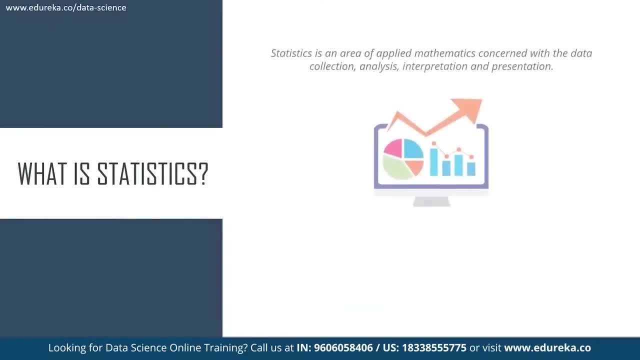 coming to the formal definition of statistics. statistics is an area of applied mathematics which is concerned with data collection, analysis, interpretation and presentation. now, usually when I speak about statistics, people think statistics is all about analysis. but statistics has other parts to it. it has data collection is also a part of statistics- data interpretation. 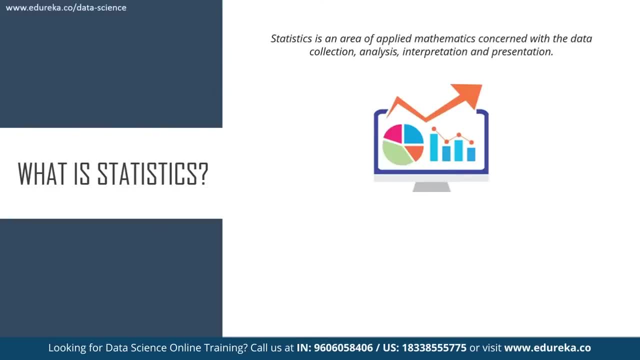 presentation visualization. all of this comes into statistics. all right, you're going to use statistical methods to visualize data, to collect data, to interpret data, all right. so the area of mathematics deals with understanding how data can be used to solve complex problems. okay, now I'll give you a couple of examples that 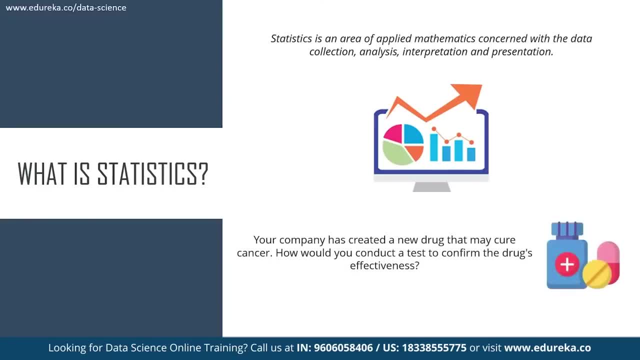 can be solved by using statistics. okay, let's say that your company has created a new drug that make your cancer. how would you conduct a test to confirm the drugs effectiveness? now, even though this sounds like a biology problem, this can be solved with statistics. all right, you will have to create a test which can 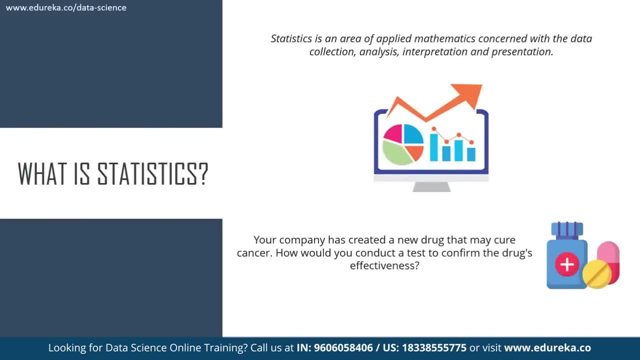 confirm the effectiveness of the drug. all right, this is a common problem that can be solved using statistics. let me give you another example. you and a friend are at a baseball game and, out of the blue, he offers you a bet that neither team will hit a home run in that game. should you take the bet all? 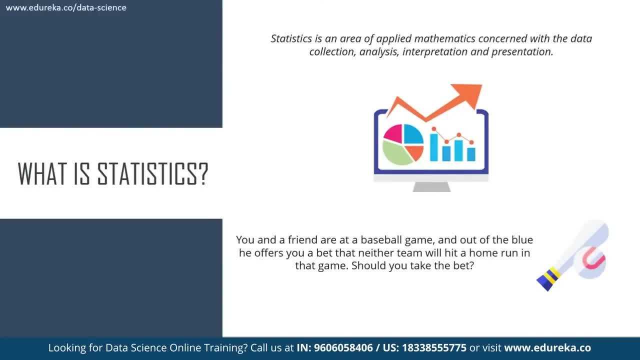 right, here you'll just discuss the probability of whether you'll win or lose. all right, this is another problem that comes under statistics. let's look at another example. the latest sales data has just come in and your boss wants you to prepare a report for management on. 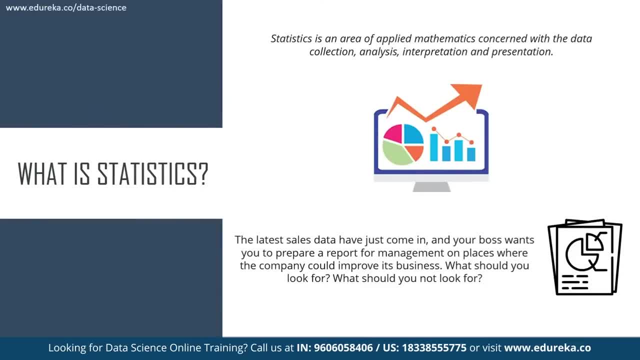 places where the company could improve its business. what should you look for and what should you not look for? now, this problem involves a lot of data analysis. we'll have to look at the different variables that are causing your business to go down or that. you have to look at a few variables that are 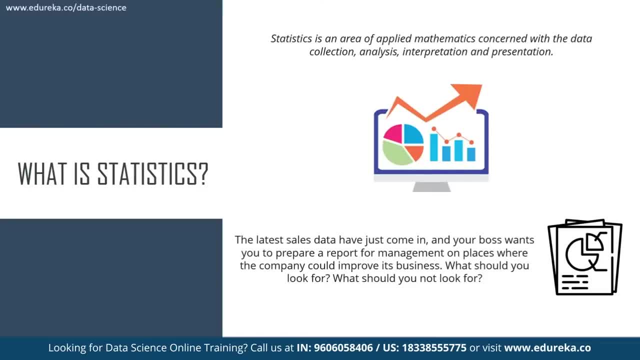 increasing the performance of your models and thus growing your business. alright, so this involves a lot of data analysis, and the basic idea behind data analysis is to use statistical techniques in order to figure out the relationship between different variables or different components in your business. okay, so now let's move on and look at our next topic, which is basic. 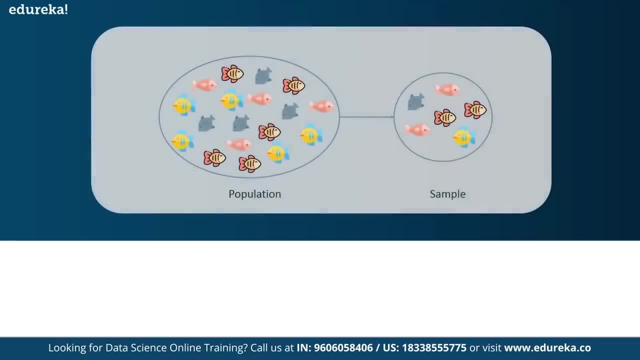 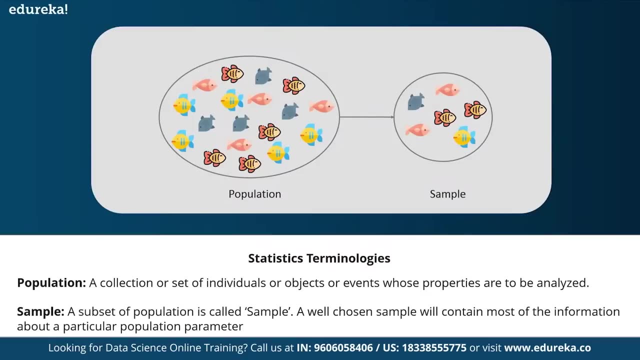 terminologies in statistics. now, before you dive deep into statistics, it is important that you understand basic terminologies used in statistics. the two most important things that you need to know about statistics is that you need to know. most important terminologies in statistics are population and sample. so 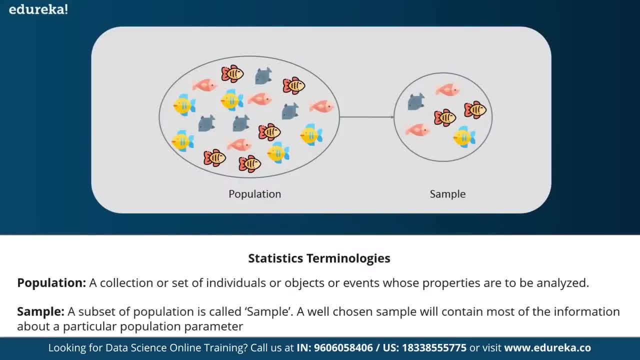 throughout the statistics course, or throughout any problem that you're trying to solve with statistics, you will come across these two words, which is population and sample. now, population is a collection or a set of individuals or objects or events whose properties are to be analyzed. okay, so basically you can. 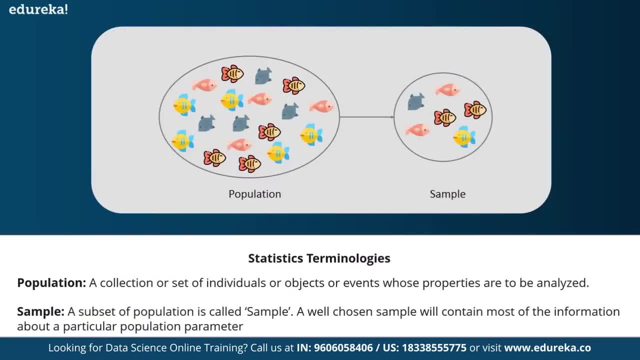 refer to population as a subject that you're trying to analyze now. a sample is just like the word suggests: it's a subset of the population. so you have to make sure that you choose the sample in such a way that it represents the entire population. alright, it shouldn't focus at one part of. 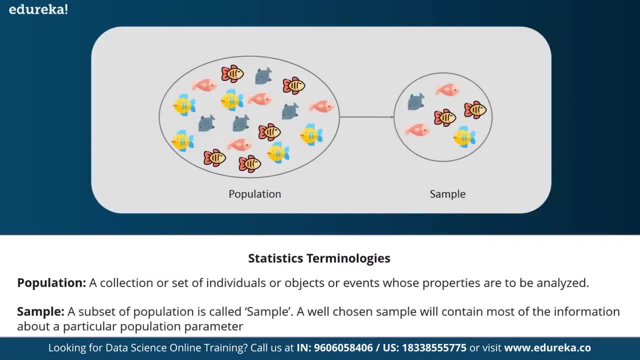 the population. instead, it should represent the entire population. that's how your sample should be chosen. so a well chosen sample will contain most of the information about a particular population parameter. now you must be wondering: how can one choose a sample that is more specific to your particular population? 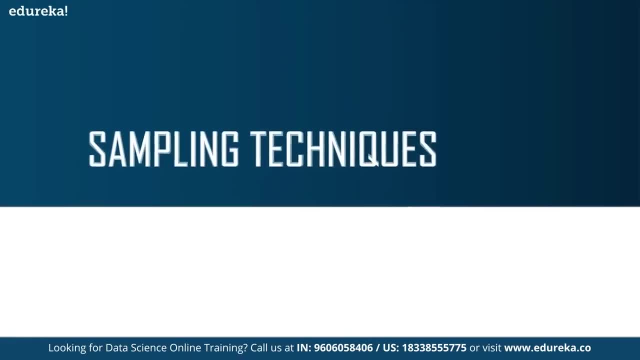 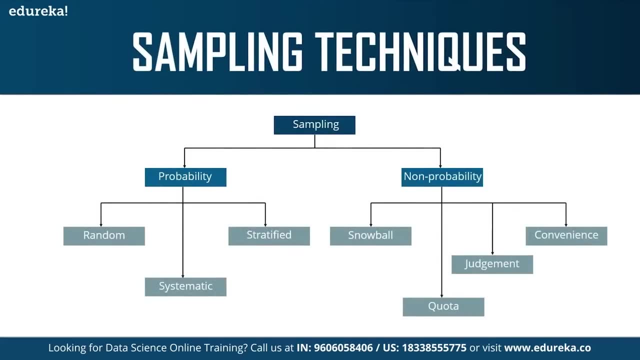 that best represents the entire population. Now, sampling is a statistical method that deals with the selection of individual observations within a population. So sampling is performed in order to infer statistical knowledge about a population. Alright, if you want to understand the different statistics of a population, like the mean, the median, the mode or the standard deviation, or 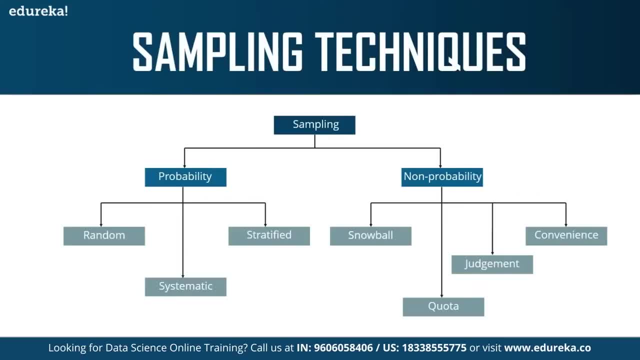 the variance of a population, then you're going to perform sampling. Alright, because it's not reasonable for you to study a large population and find out the mean, median and everything else. So why is sampling performed? You might ask: what is the point of sampling? We can just study the 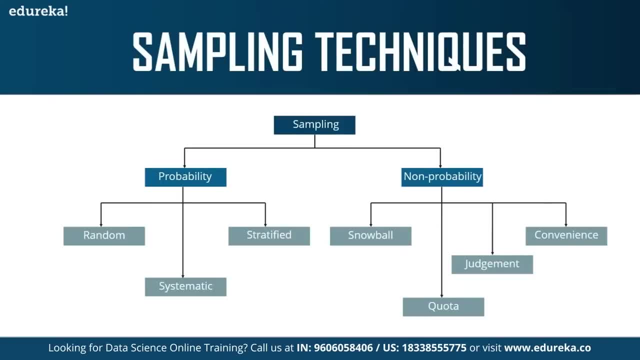 entire population. Now, guys, think of a scenario wherein you're asked to perform a survey about the eating habits of teenagers in the US. So at present, there are over 42 million teens in the US, and this number is growing as we are speaking right now, correct? 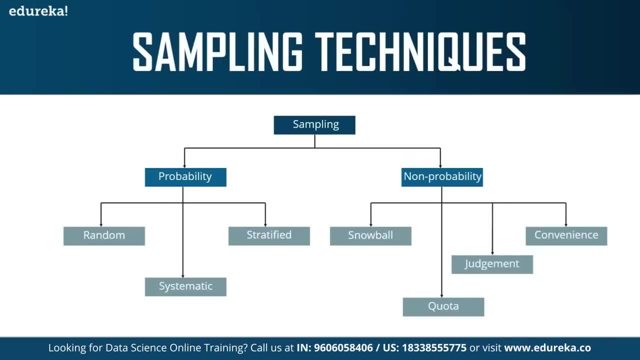 Is it possible to survey each of these 42 million individuals about their health? Is it possible? Well, it might be possible, but this will take forever to do Now. obviously it's not. it's not reasonable to go around knocking each door and asking for what does your teenage son eat? and 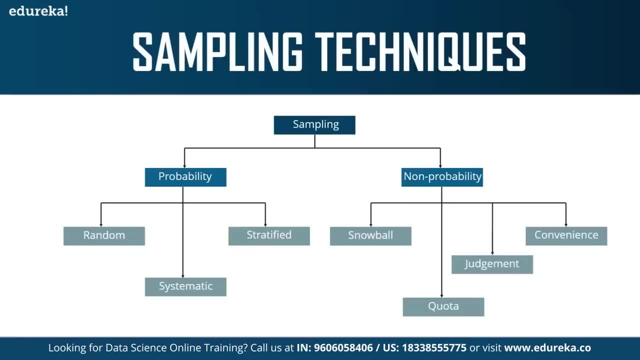 all of that, alright. This is not very reasonable. that's why sampling is used. It's a method wherein a sample of the population is studied in order to draw inference about the entire population, so it's basically a shortcut to studying the entire population, instead of taking the entire 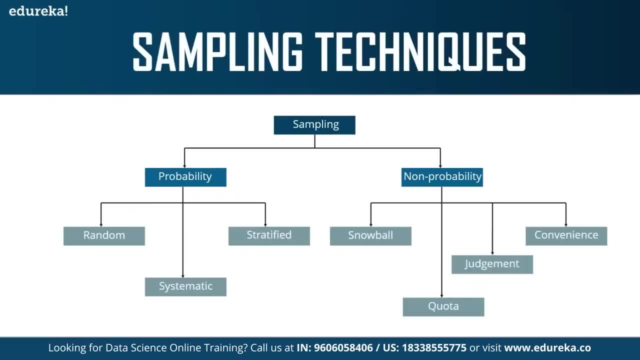 population and finding out all the solutions. you're just going to take a part of the population that represents the entire population and you're going to perform all your statistical analysis, your inferential statistics, on that small sample, all right, and that sample basically represents the entire population, all right. so i'm sure i've made this clear to y'all: what is sample and what. 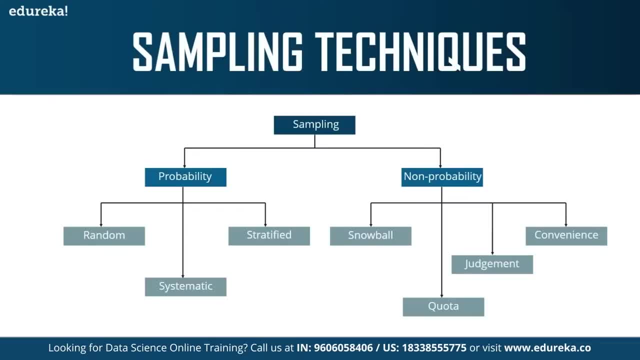 is population. now there are two main types of sampling techniques that i'll discuss today. we have probability sampling and non-probability sampling. now, in this video, we'll only be focusing on probability sampling techniques, because non-probability sampling is not within the scope of this video. all right, we'll only discuss the probability part, because we're focusing on. 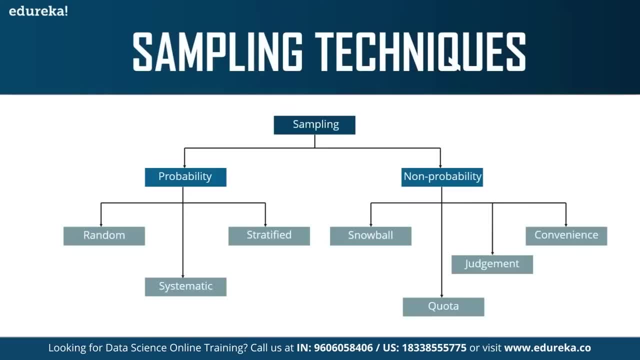 statistics and probability correct. now again, under probability sampling, we have three different types. we have, we have. we have random sampling, systematic and stratified sampling. all right, and just to mention the different types of non-probability samplings, we have snowball quota judgment and convenient. 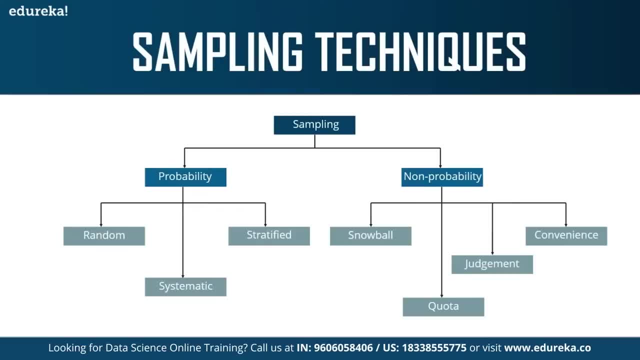 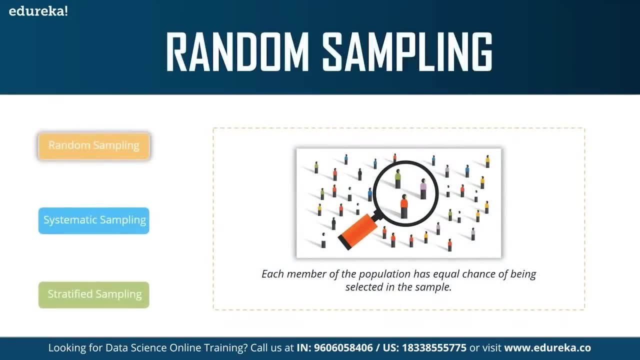 sampling. all right now, guys. in this session i'll only be focusing on probability, so let's move on and look at the different types of probability sampling. so what is probability sampling? it is a sampling technique in which samples from a large population are chosen by using the theory of probability. all right, so there are three types of probability. 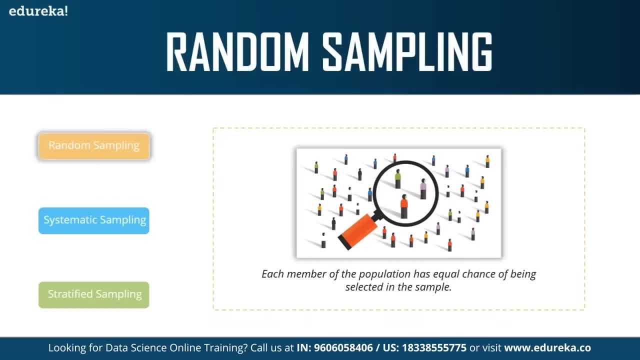 sampling. all right. first we have the random sampling now. in this method, each member of the population has an equal chance of being selected in the sample, all right. so each and every individual or each and every object in the population has an equal chance of being a part of the sample. 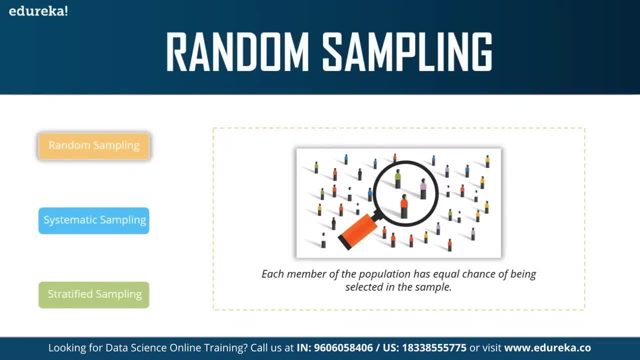 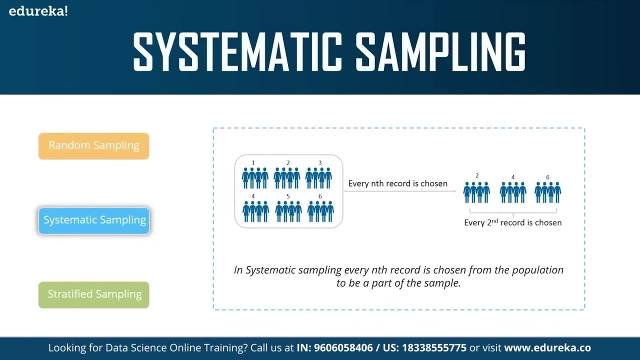 that's what random sampling is all about. okay, you're randomly going to select any individual or any object, so this way, each individual has an equal chance of being selected correct. next we have systematic sampling. now, in systematic sampling, every nth record is chosen from the population to be a part of the sample. all right, now refer this image that i've shown over here. out of these, 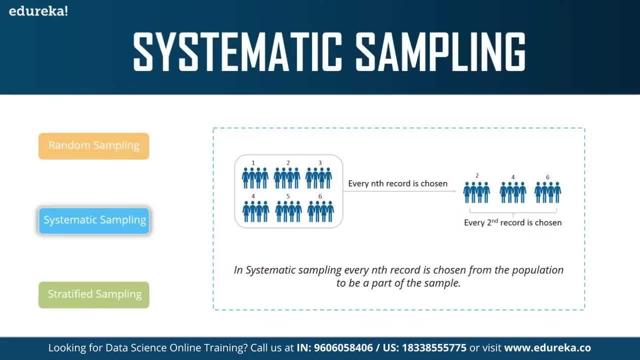 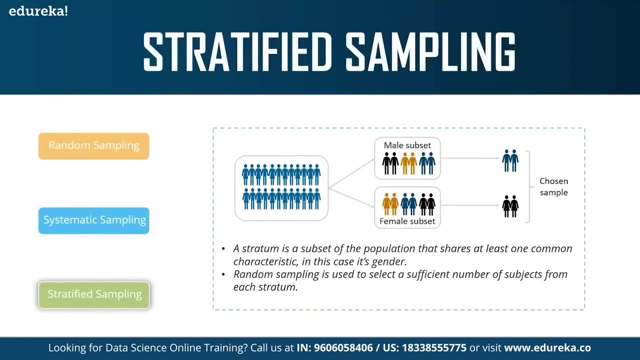 six groups. every second group is chosen as a sample. okay, so every second record is chosen here, and this is our system. systematic sampling works. okay, you're randomly selecting the nth record and you're going to add that to your sample. next we have stratified sampling now, in this type of technique, a stratum. 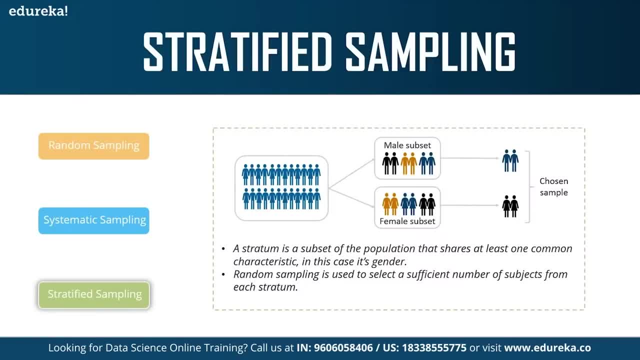 is used to form samples from a large population. so what is a stratum? a stratum is basically a subset of the population that shares at least one common characteristics. so let's say that your population has a mix of both male and female. so you can create two stratums and you can 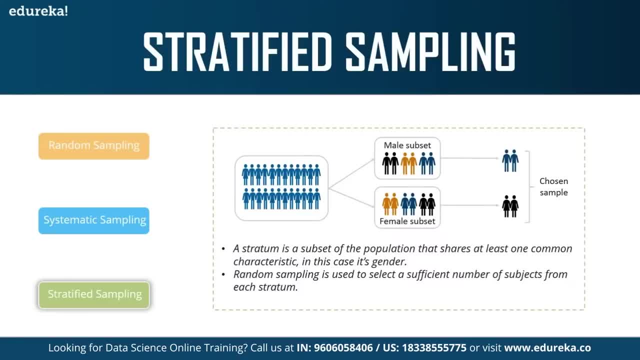 create two stratums out of this. one will have only the male subset and the other will have the female subset. all right, this is what stratum is. it is basically a subset of the population that shares at least one common characteristics. all right, in our example, it is gender. so after you've created 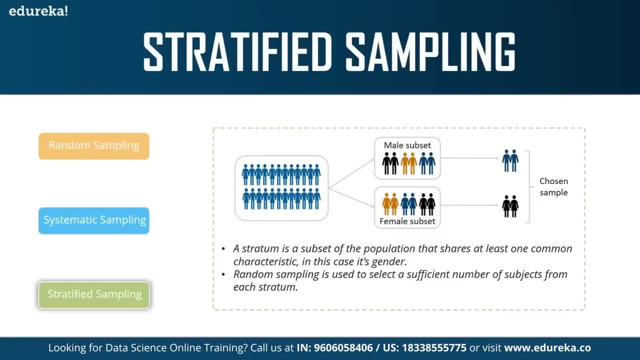 a stratum. you're going to use random sampling on these stratums and you're going to choose a final sample. so random sampling meaning that all of the individuals in each of the stratum will have an answer being selected in the sample, correct? so, guys, these were the three different types of 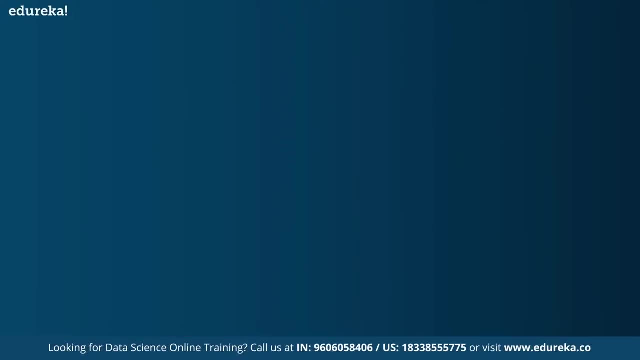 sampling techniques. now let's move on and look at our next topic, which is the different types of statistics. so after this, we'll be looking at the more advanced concepts of statistics. all right, so far we discussed the basics of statistics, which is basically what is statistics. the different 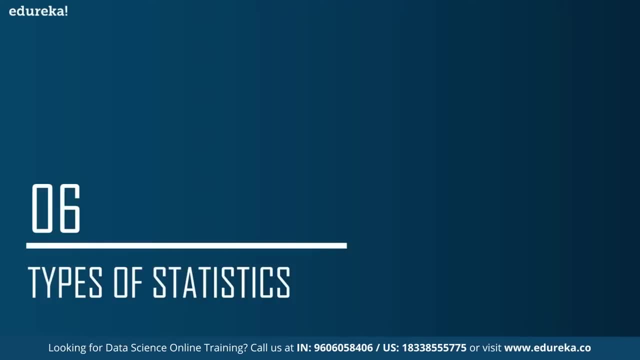 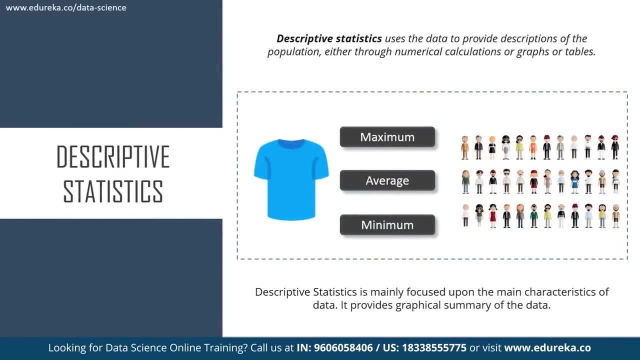 sampling techniques and the terminologies and statistics. all right, now we look at the different types of statistics. so there are two major types of statistics: descriptive statistics and inferential statistics. in today's session we'll be discussing both of these types of statistics in depth. all right, we'll also be 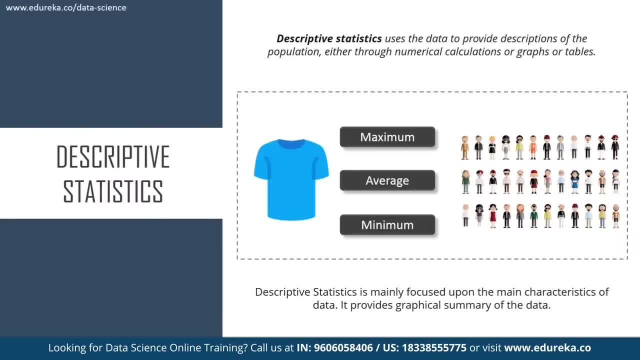 looking at a demo which i'll be running in the r language in order to make you understand what exactly descriptive and inferential statistics is. so, guys, we're just going to look at the basics, so don't worry if you don't have much knowledge. i'm explaining everything from the basic level. 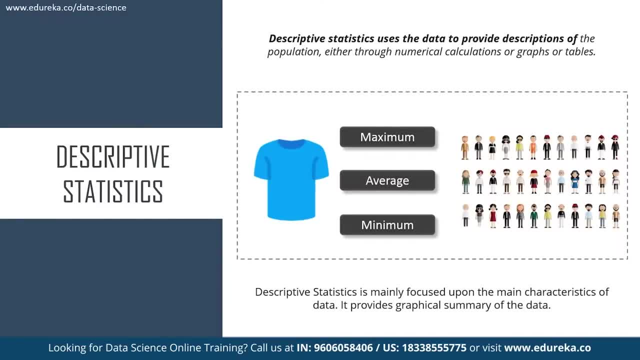 all right. so, guys, descriptive statistics is a method which is used to describe and understand the features of specific data set by giving a short summary of the data. okay, so it is mainly focused upon the characteristics of data. it also provides a graphical summary of the data. now, in order to make you understand what. 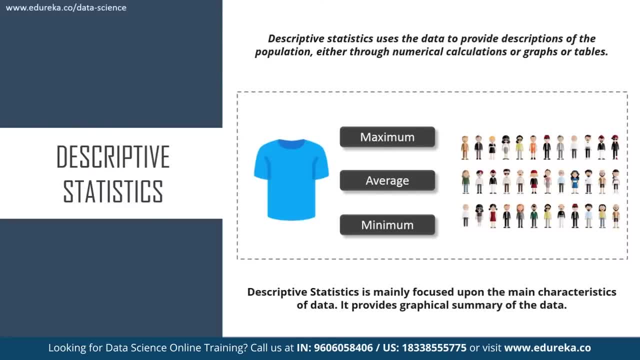 descriptive statistics is: let's suppose that you want to gift all your classmates a t-shirt, so to study the average shirt size of a student in a classroom. so if you were to use descriptive statistics to study the average shirt size of students in your classroom, then what you would do is you would record the shirt size of all students. 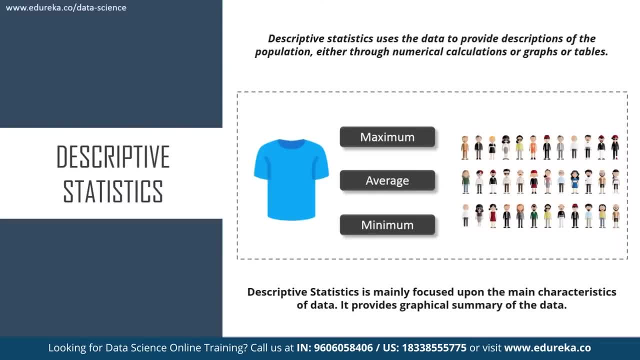 in the class and then you would find out the maximum, minimum and average shirt size of the class. okay, so, coming to inferential statistics, inferential statistics makes inferences and predictions about a population based on the sample of data taken from the population. okay, so, in simple words, it generalizes a large data set and it applies probability to draw a. 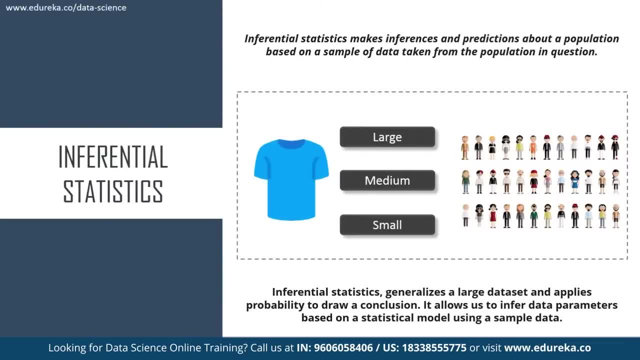 conclusion: okay, so it allows you to infer data parameters based on a statistical model by using sample data. so if we consider the same example of finding the average shirt size of students in a class, in inferential statistics you will take a sample set of the class, which is basically a few. 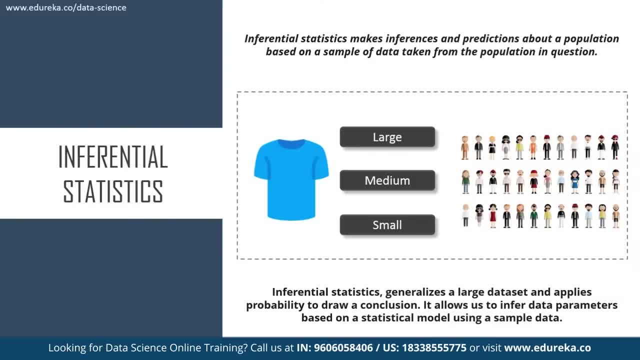 people from the entire class. all right, you already have had. group the class into large, medium and small, all right. in this method, you basically build a statistical model and expand it for the entire population in the class. so, guys, there was a brief understanding of descriptive and inferential statistics. so that's the difference between descriptive and 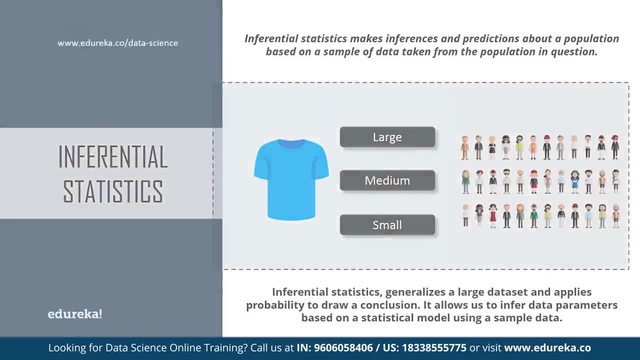 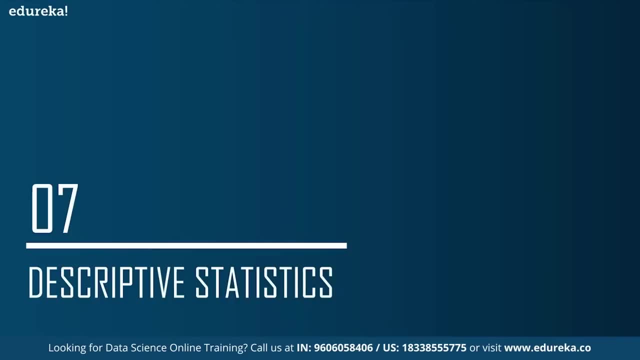 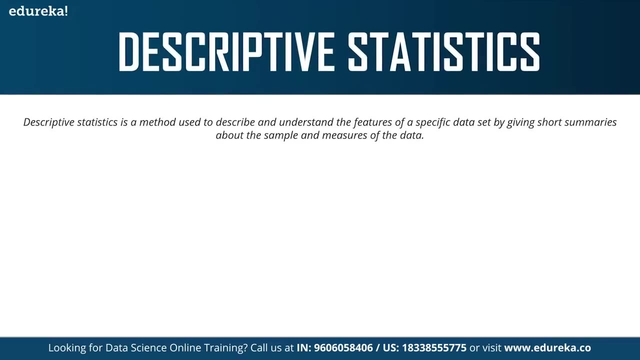 inferential. now, in the next section, we'll go in depth about descriptive statistics. all right, so let's discuss more about descriptive statistics. so, like i mentioned earlier, descriptive statistics is a method that is used to describe and understand the features of a specific data set by giving short summaries about the sample and measures of the data. there are two important 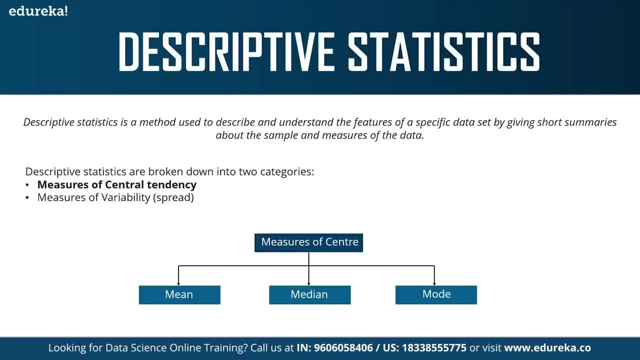 measures in descriptive statistics. we have measure of central tendency, which is also known as measure of center, and we have measures of variability- this is also known as measures of spread. so measures of center include mean, median and mode. now what is measures of center? measures of the center are statistical measures that represent the summary of a data set. 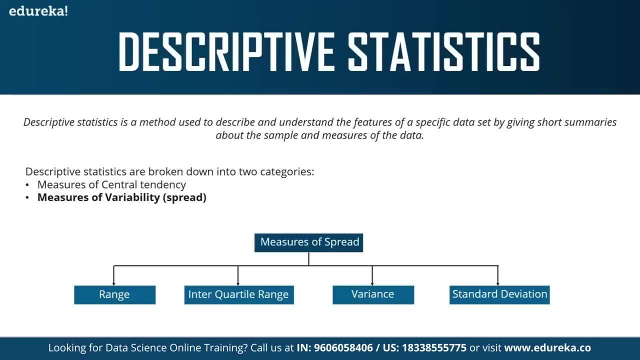 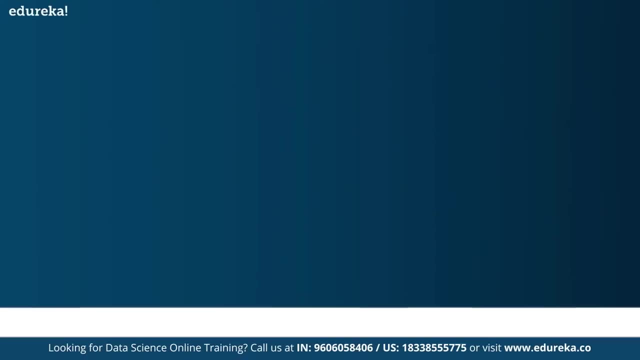 okay, the three main measures of center are mean, median and mode. coming to measures of variability, or measures of spread, we have range, interquartile range variance and standard deviation. all right, so now let's discuss each of these measures in a little more depth, starting with the measures of 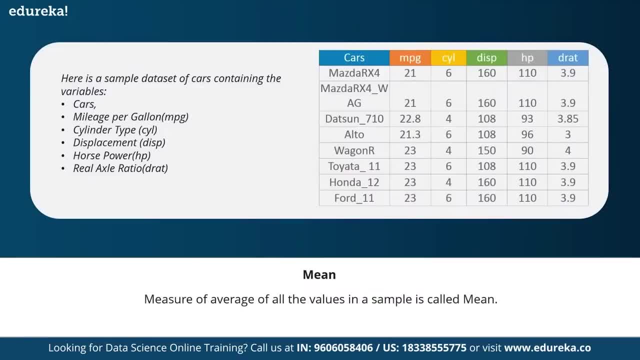 center. now, i'm sure all of you know what the mean is. mean is basically the number of measures of center. it's basically the measure of the average of all the values in a sample. okay, so it's basically the average of all the values in a sample. how do you measure the mean? i hope all of you know how the 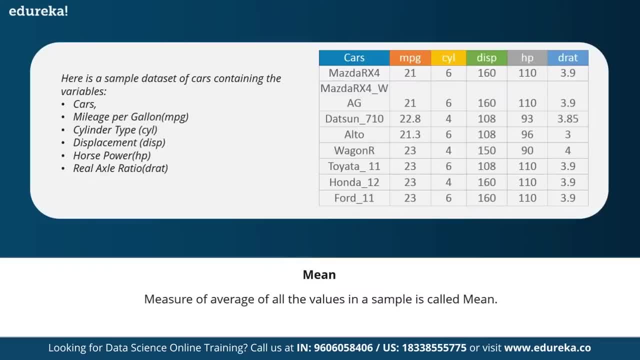 mean is measured. if there are 10 numbers and you want to find the mean of these 10 numbers, all you have to do is you have to add up all the 10 numbers and you have to divide it by 10.. 10 here represents: 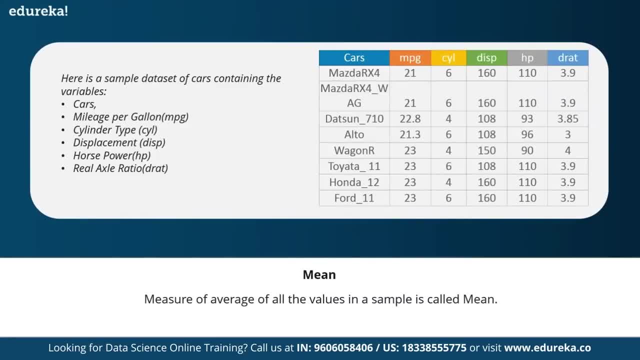 the number of samples in your data set. all right, since we have 10 numbers, we're going to divide this by 10.. all right, this will give us the average or the mean. so to better understand the measures of central tendency, let's look at an example now. the data set over here is basically the cars data set. 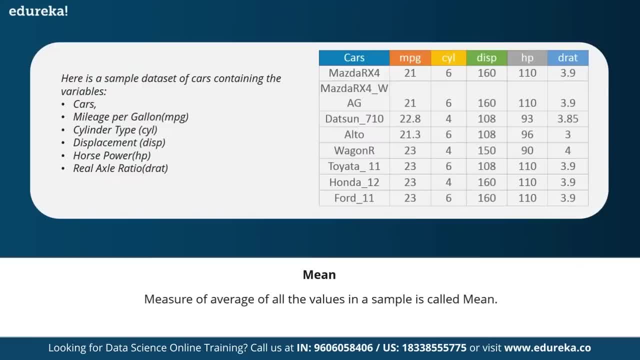 and it contains a few variables. all right. it has something known as cars. it has mileage per gallon, cylinder type, displacement, horsepower and real axle ratio. all right, all of these measures are related to cars, okay, so what you're going to do is you're going to use descriptive analysis and you're going to analyze each of the variables in the sample. 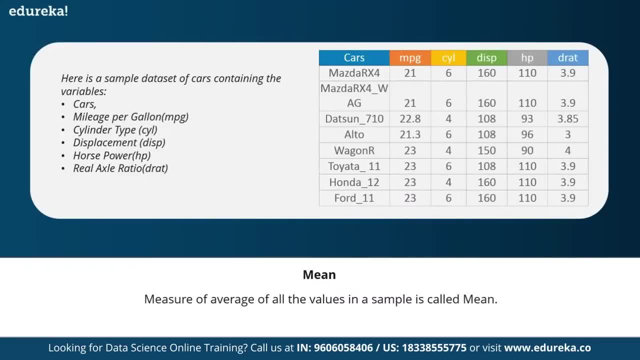 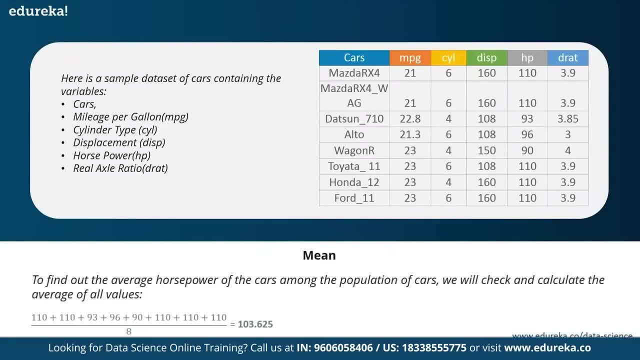 data set for the mean standard deviation, median, more and so on. so let's say that you want to find out the mean or the average horsepower of the cars among the population of cars, like i mentioned earlier. what you do is you'll check the average of all the values, so in this case we'll take the sum. 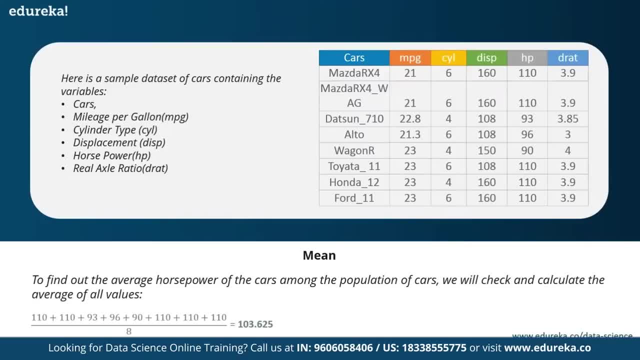 of the horsepower of each car and we'll divide that by the total number of cars. okay, that's exactly what i've done here in the calculation part. so this 110 basically represents the horsepower for the first car. all right? similarly, i've just added up all the values of horsepower for each of. 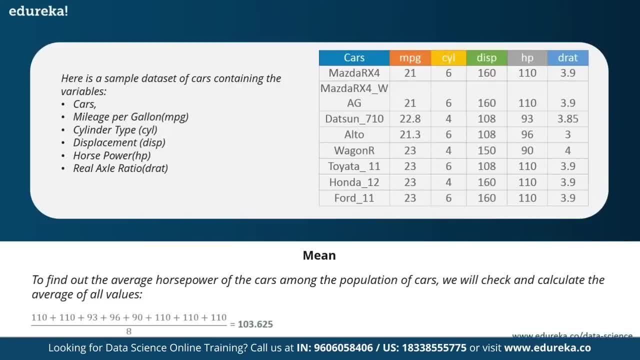 the cars and i've divided it by 8.. now, 8 is basically the number of cars in our data set. all right, so 103.625 is what our mean is, or the average of horsepower is. all right. now let's understand what median is with an example. 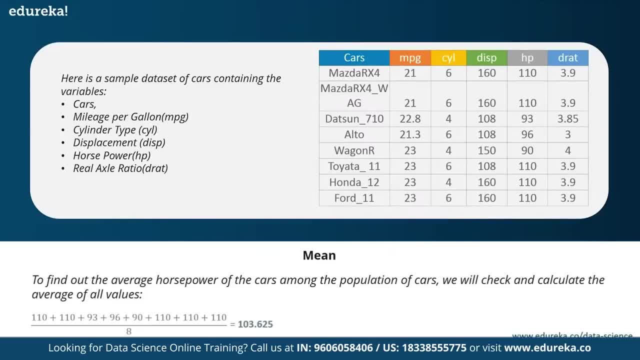 okay, so to define median. median is basically a measure of the central value of the sample set is called the median. all right, you can say that it is a middle value. so if you want to find out the center value of the mileage per gallon among the population of cars, 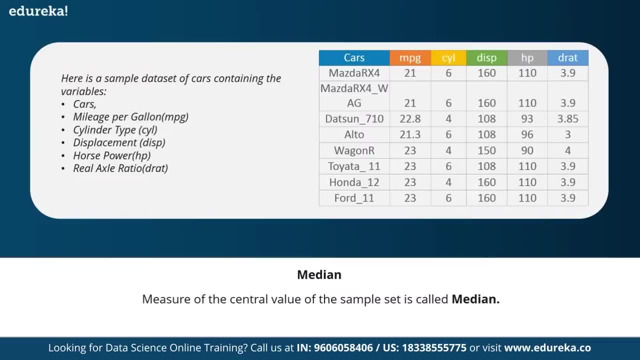 first, what we'll do is we'll arrange the mpg values in ascending or descending order and choose a middle value. all right in this case, since we have eight values. right, we have eight values, which is an even entry. so whenever you have even number of data points or samples in your data, 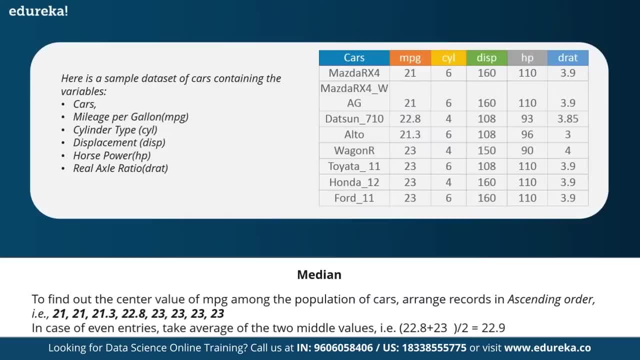 set, then you're going to take the average of the two middle values. if we had nine values over here, we can easily figure out the middle value and, you know, choose that as a median. but since there are even number of values, we're going to take the average of the two middle values. all right, so 20.625. 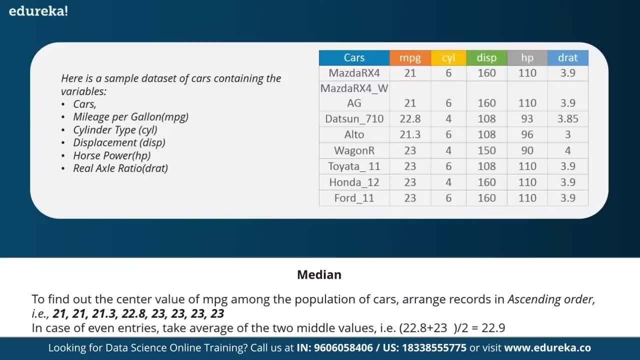 22.8 and 23 are my two middle values and I'm taking the mean of those two and hence I get 22.9, which is my median. all right, Lastly, let's look at how mode is calculated. 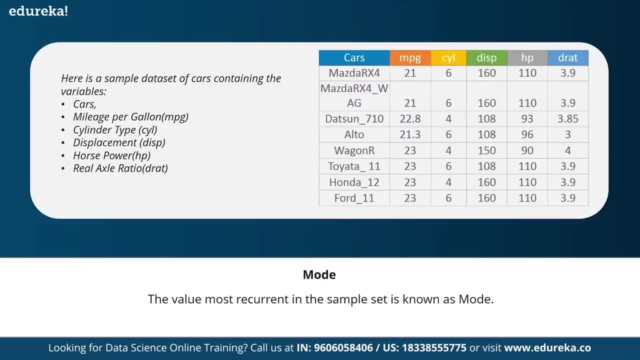 So what is mode? Now, the value that is most recurrent in the sample set is known as mode, or basically, the value that occurs most often. okay, That is known as mode. So let's say that we want to find out the most common type of cylinder. 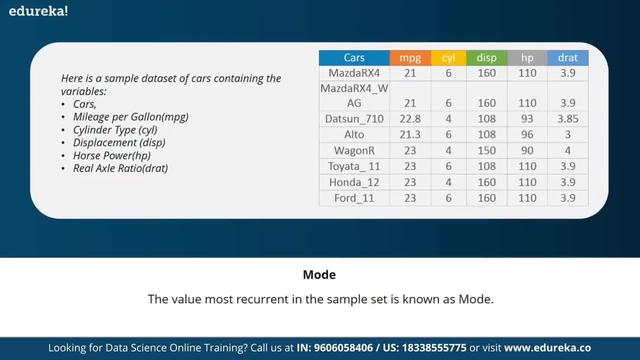 among the population of cars. All we have to do is we will check the value which is repeated the most number of times. Here we can see that the cylinders come in two types. We have cylinder of type four and cylinder of type six. right. 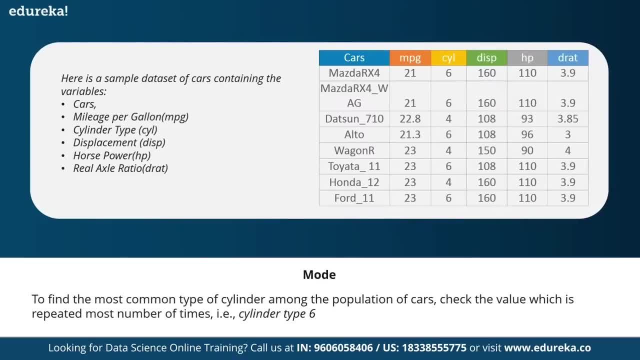 So take a look at the data set. You can see that the most recurring value is six. right, We have one, two, three, four and five. We have five, six. and we have one, two, three. Yeah, we have three, four. type cylinders. 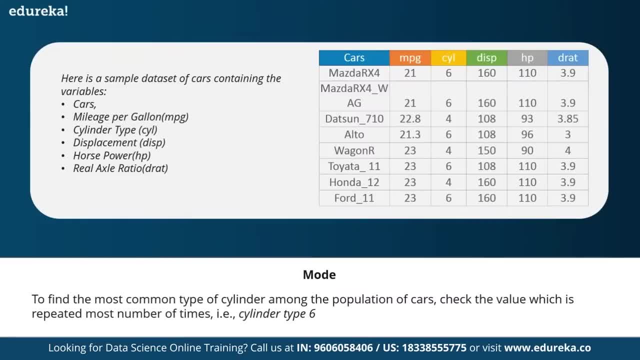 and five six type cylinders. So, basically, we have three four type cylinders and we have five six type cylinders. all right, So our mode is going to be six, since six is more recurrent than four. So, guys, those were the measures of the center. 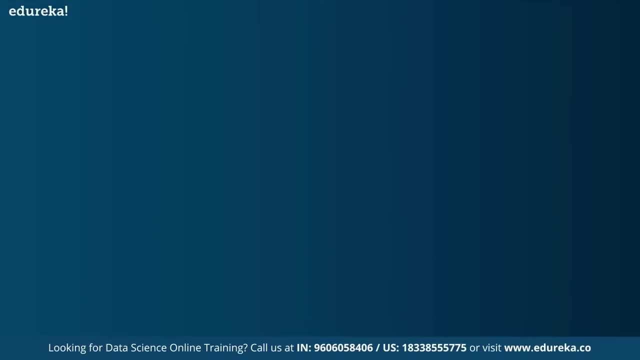 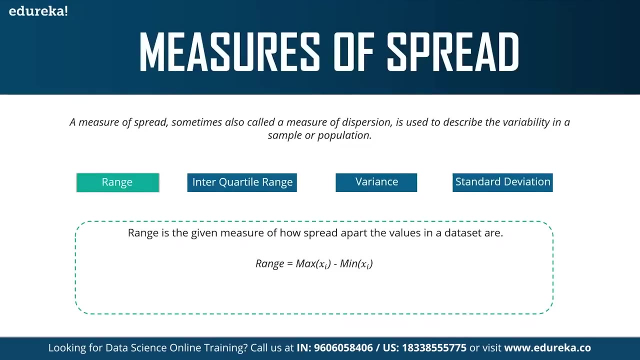 or the measures of central tendency. Now let's move on and look at the measures of the spread. All right, Now, what is the measure of spread? A measure of spread, sometimes also called as measure of dispersion, is used to describe the variability. 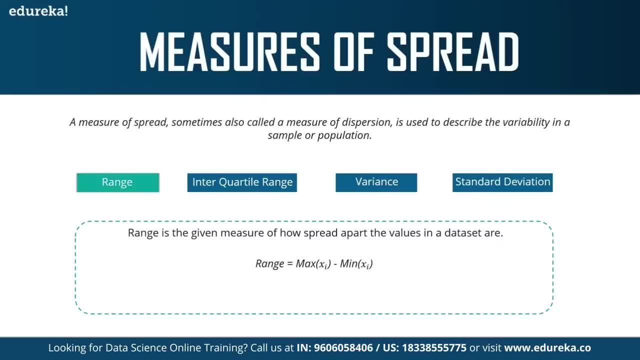 in a sample or population. Okay, you can think of it as some sort of deviation in the sample. all right, So you measure this with the help of the different measure of spreads. We have range, interquartile range variance and standard deviation. 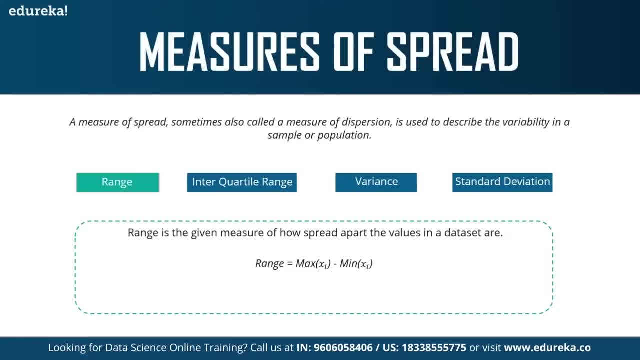 Now, range is pretty self-explanatory, right. It is the given measure of how, spread apart, the values in a data set are. The range can be calculated as shown in this formula. So you're basically going to subtract the maximum value in your data set. 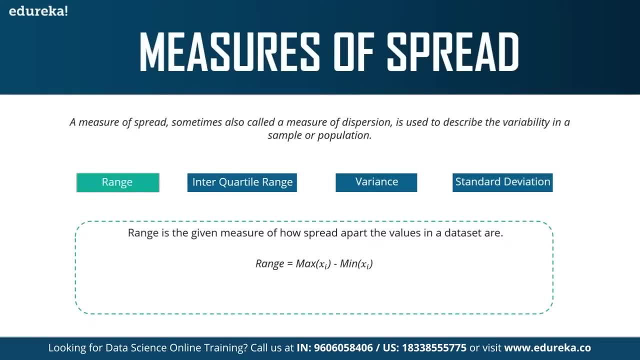 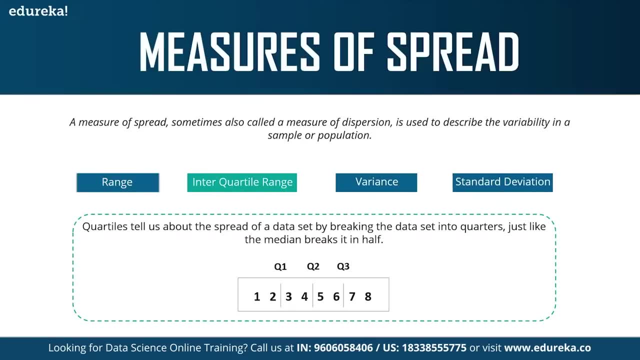 from the minimum value in your data set. That's how you calculate the range of the data. all right. Next we have interquartile range. So before we discuss interquartile range, let's understand what a quartile is. 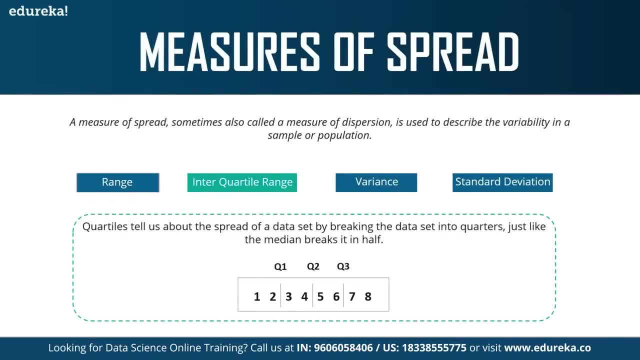 All right. so quartiles basically tell us about the spread of a data set by breaking the data set into different quartiles. Okay, just like how the median breaks the data into two parts, the quartile will break it into different quartiles. 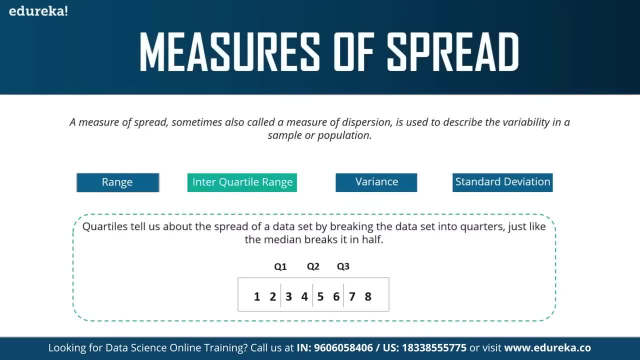 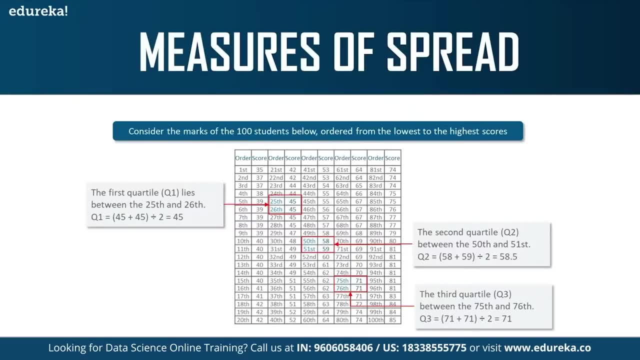 So to better understand how quartile and interquartile are calculated, let's look at a small example Now. this data set basically represents the marks of 100 students, ordered from the lowest to the highest scores. all right, So the quartiles lie in the following ranges: 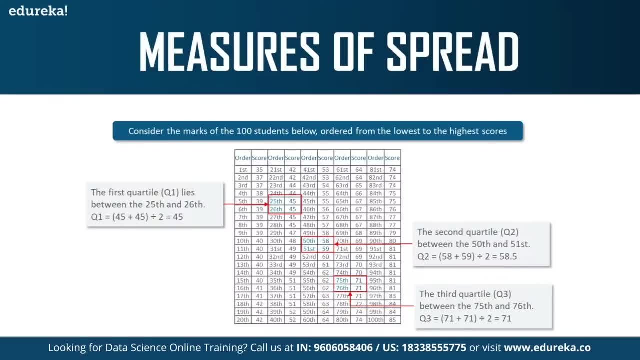 Now the first quartile, which is also known as Q1,. it lies between the 25th and the 26th observation. all right, So if you look at this, this have highlighted the 25th and the 26th observation. 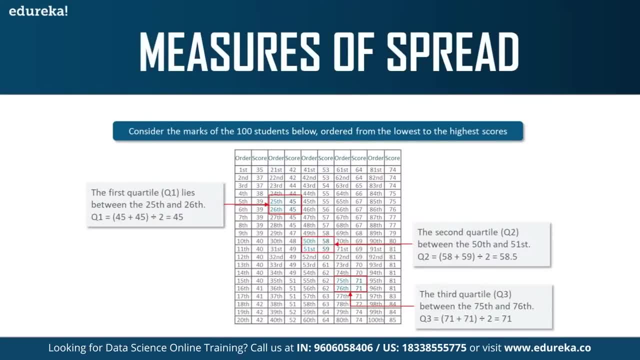 So how you can calculate Q1, or first quartile, is by taking the average of these two values. all right, Since both the values are 45, when you add them up and divide them by two, you'll still get 45.. 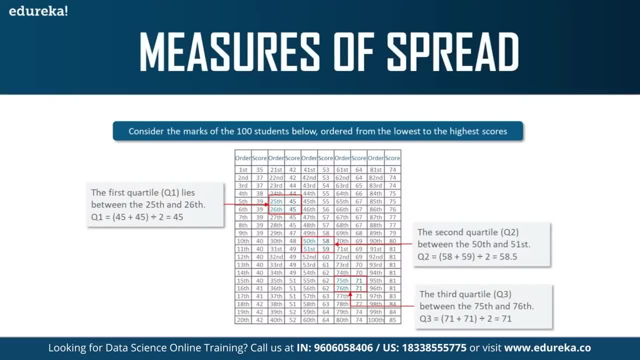 Now the second quartile, or Q2, is between the 50th and the 51st observation. So you're going to take the average of 58 and 59, and you'll get a value of 58.5.. Now this is my second quarter. 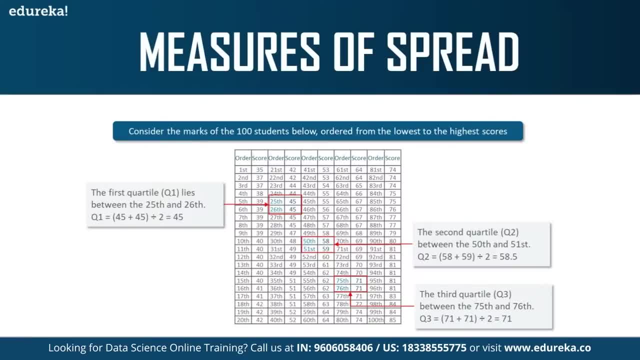 The third quartile, or Q3, is between the 75th and the 76th observation. Here again, you'll take the average of the two values, which is the 75th value and the 76th value. all right. 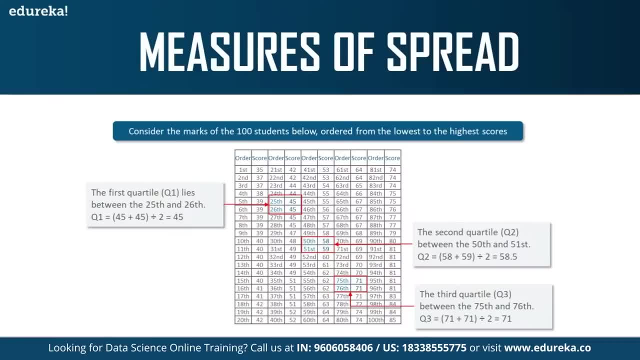 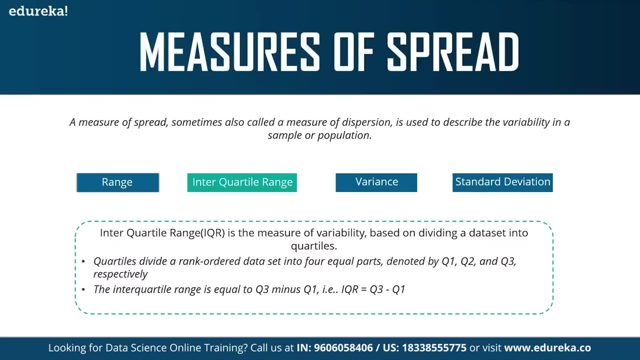 And you'll get a value of 71,. all right, So, guys, this is exactly how you calculate the different quartiles. Now let's look at what is interquartile range, So IQR or the interquartile range. 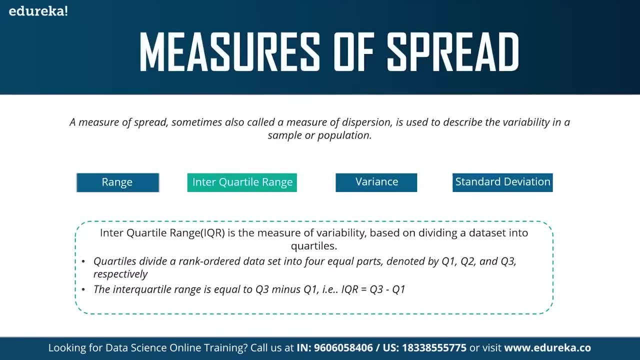 is a measure of variability based on dividing a data set into quartiles. Now the interquartile range is calculated by subtracting the Q1 from Q3.. So basically, Q3 minus Q1 is your IQR. So your IQR is your Q3 minus Q1, all right. 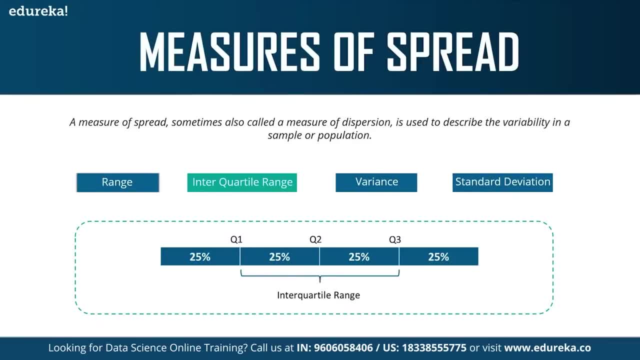 Now this is how each of the quartiles are. Each quartile represents a quarter, which is 25%. all right, So, guys, I hope all of you are clear with interquartile range and what are quartiles. Now let's look at variance. 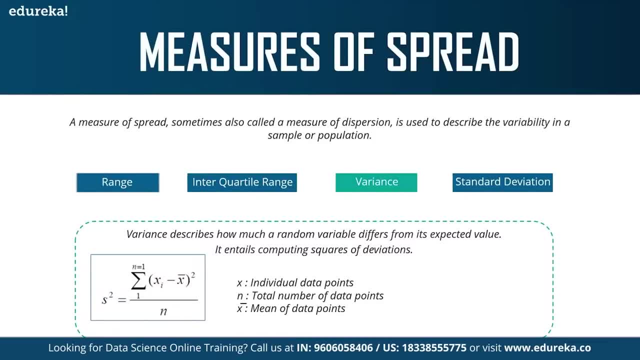 Now, variance is basically a measure That shows how much a random variable differs from its expected value. okay, It's basically the variance in any variable. Now variance can be calculated by using this formula Right here. X basically represents any data point in your data set. 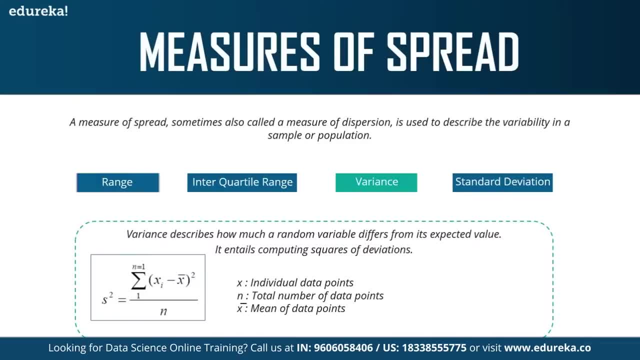 N is the total number of data points in your data set and X bar is basically the mean of data points. all right, This is how you calculate variance. Variance is basically computing the squares of deviations. Okay, So X bar is S squared there. 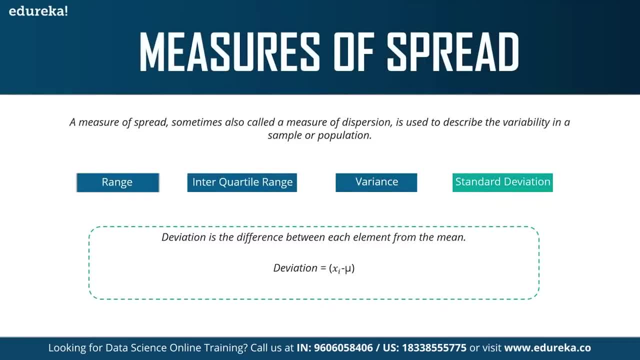 Now let's look at what is deviation. Deviation is just the difference between each element from the mean. okay, So it can be calculated by using this simple formula, where XI basically represents a data point and mu is the mean of the population. all right. 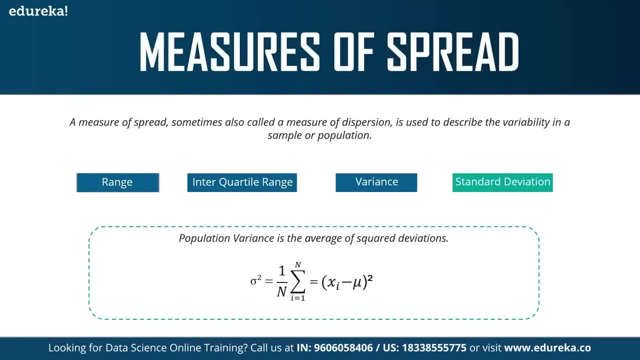 This is exactly how you calculate deviation. Now, population variance and sample variance are very specific to whether you're calculating the variance in your population data set or in your sample data set. That's the only difference between population and sample variance, So the formula for population variance is pretty explanatory. 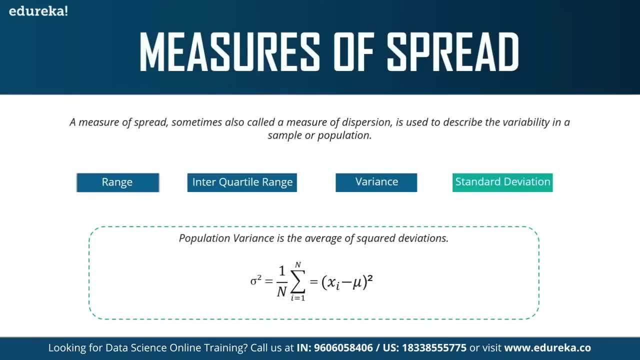 So XI is basically each data point. Mu is the mean of the population, N is the number of samples in your data set. all right, Now let's look at sample variance. Now, sample variance is the average of squared differences from the mean. all right, 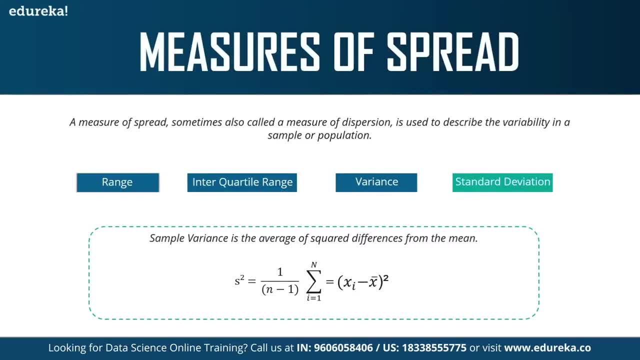 Your XI is any data point or any sample in your data set. X bar is the mean of your sample. all right, It's not the mean of your population, It's the mean of your sample. And if you notice N, here is a smaller N. 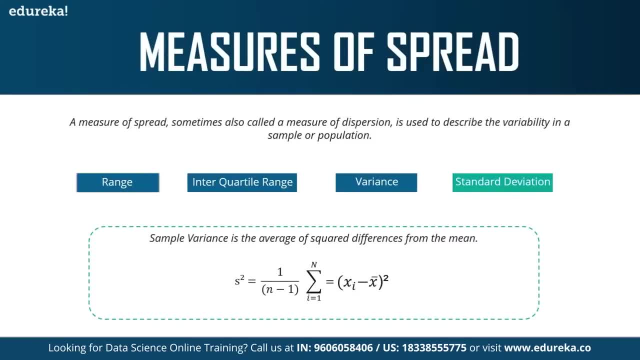 It's the number of data points in your sample And this is basically the difference between sample and population variance. I hope that is clear. Coming to standard deviation is the measure of dispersion of a set of data from its mean. all right, So it's basically the deviation from your mean. 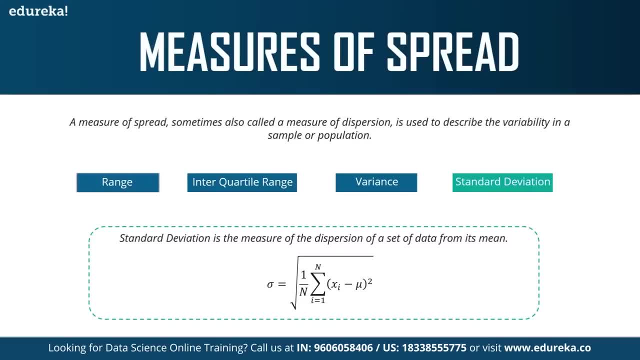 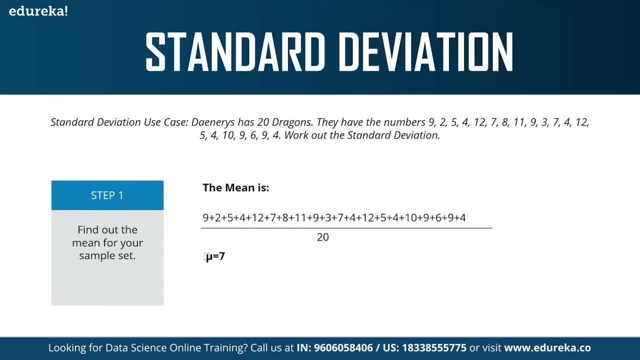 That's what standard deviation is. Now, to better understand how the measures of spread are calculated, let's look at a small use case. So let's say Daenerys has 20 dragons. They have the numbers nine, two, five, four and so on. 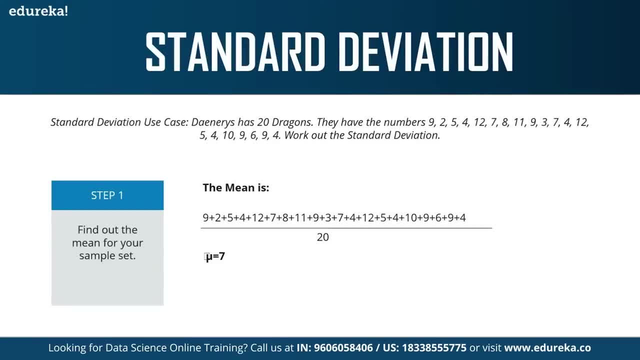 as shown on the screen. What you have to do is you have to work out the standard deviation. all right, In order to calculate the standard deviation, you need to know the mean right. So first you're gonna find out the mean of your sample set. 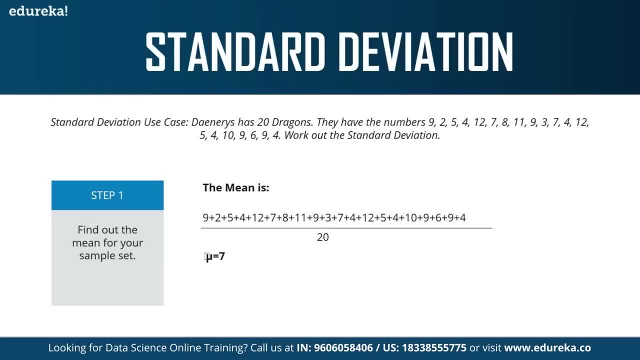 So how do you calculate the mean? You add all the numbers in your data set and divide it by the total number of samples in your data set. So you get a value of seven here. Then you calculate the RHS of your standard deviation formula. 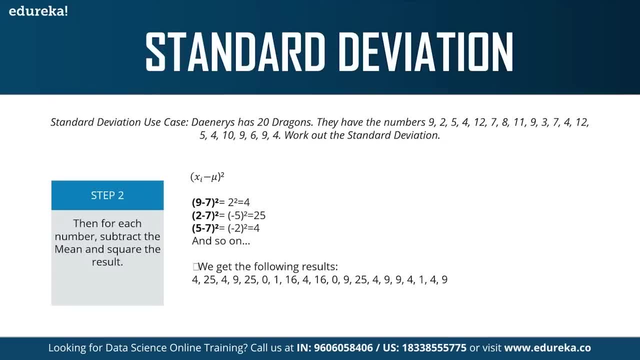 All right. so from each data point you're going to subtract the mean and you're going to square that. all right. So when you do that, you'll get the following result: You'll basically get this: 425,, 4925, and so on. 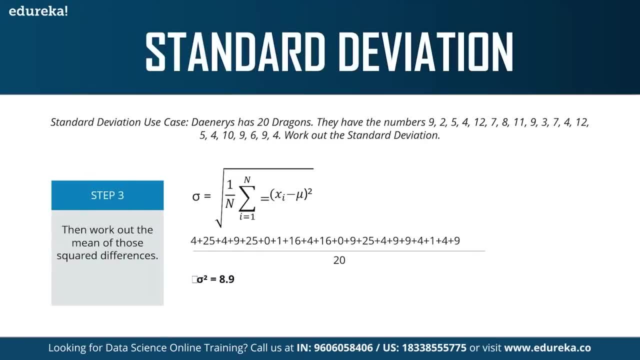 So, finally, you'll just find the mean of these squared differences, all right. So your standard deviation will come up to 2.983 once you take the square root. So, guys, this is pretty simple. It's a simple mathematic technique. 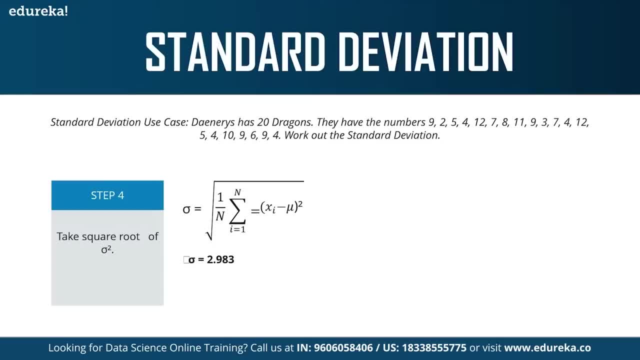 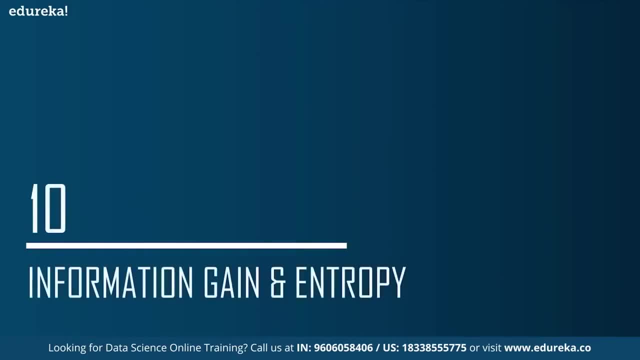 All you have to do is you have to substitute the values in the formula. all right, I hope this was clear to all of you. Now let's move on and discuss the next topic, which is information gain and entropy. Now, this is one of my favorite topics in statistics. 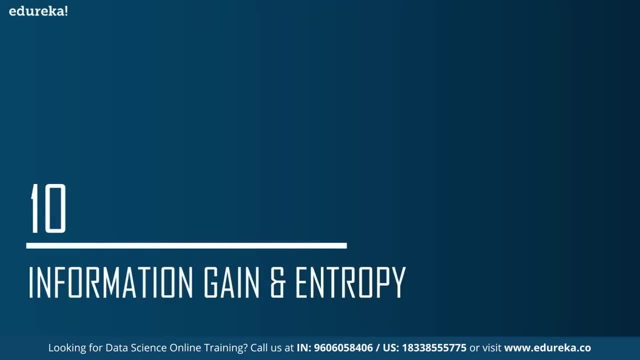 It's very interesting, and this topic is mainly involved in machine learning algorithms like decision trees and random forest. all right, It's very important for you to know how information gain and entropy really work and why they're so essential in building machine learning models. 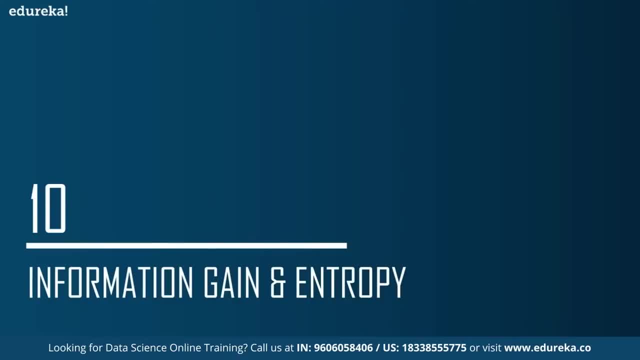 We'll focus on the statistic parts of information gain and entropy, and after that we'll discuss a use case and see how information gain and entropy is used in decision trees. So for those of you who don't know what a decision tree is, 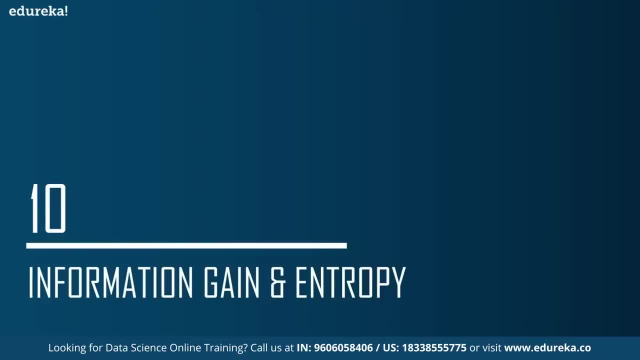 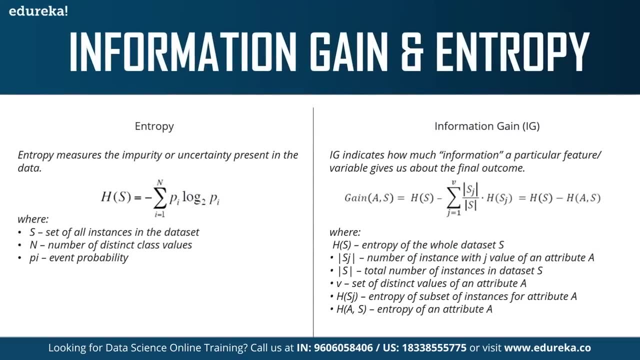 it is basically a machine learning algorithm. You don't have to know anything about this. I'll explain everything in depth, so don't worry. Now let's look at what exactly entropy and information gain is. Now, guys, entropy is basically the measure. 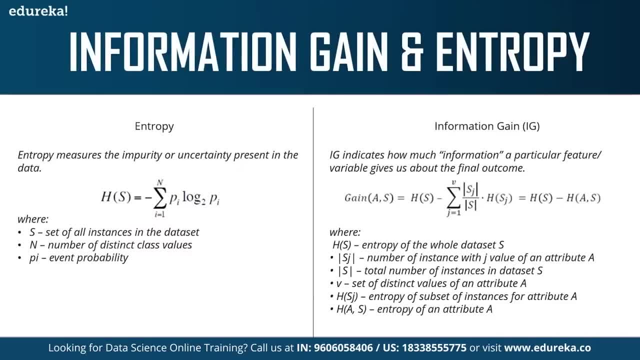 of any sort of uncertainty that is present in the data. All right, so it can be measured by using this formula. So here: S is the set of all instances in the data set or all the data items in the data set. N is the different type of classes in your data set. 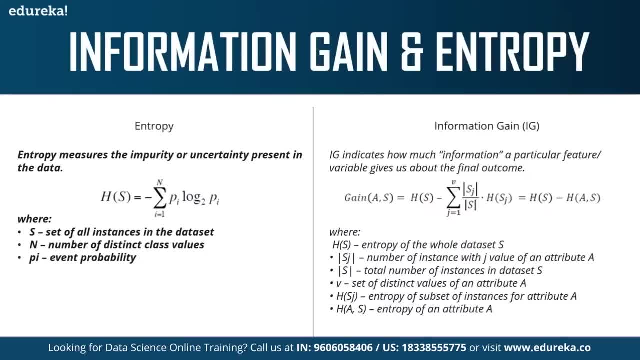 Pi is the event probability. Now, this might seem a little confusing to you all, but when we go through the use case you'll understand all of these terms even better. All right, coming to information gain. As the word suggests, information gain indicates: 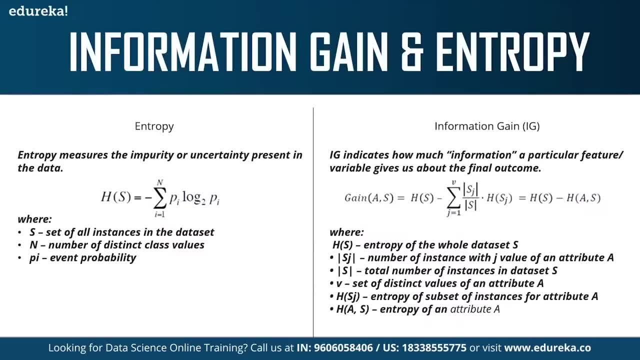 how much information a particular feature or a particular variable gives us about the final outcome. Okay, it can be measured by using this formula. So again here. H of S is the entropy of the whole data set, S, Sj is the number of instances. 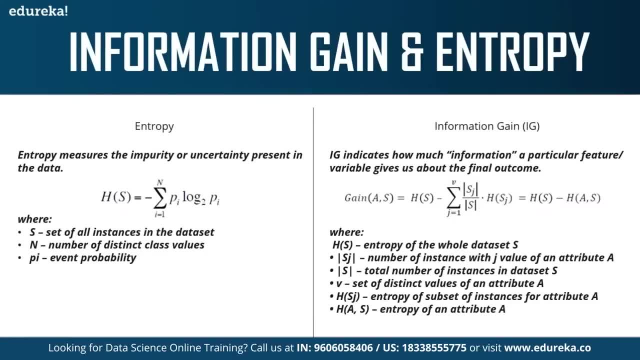 with the j value of an attribute A. S is the total number of instances in the data set. V is the set of distinct values of an attribute A. H of Sj is the entropy of subset of instances And H of A? S is the entropy of an attribute A. 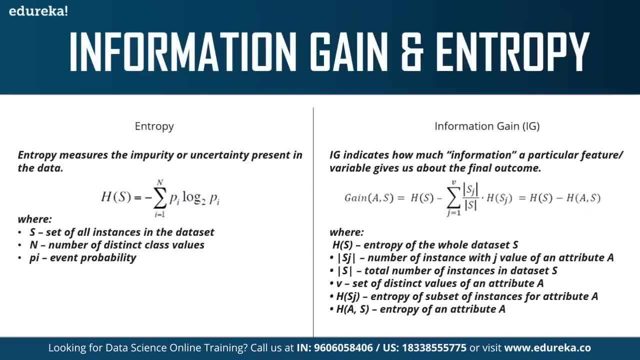 Even though this seems confusing, I'll clear out the confusion. All right, let's discuss a small problem statement where we'll understand how information gain and entropy is used to study the significance of a model. So, like I said, information gain and entropy. 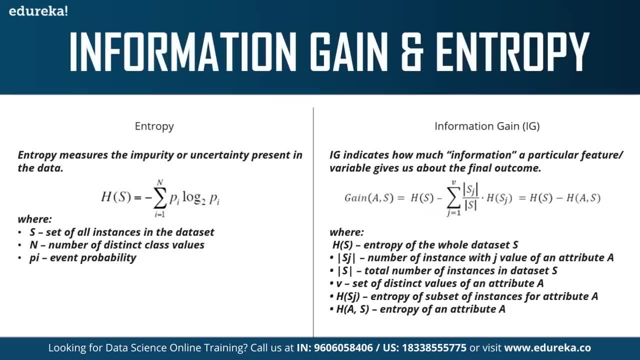 are very important statistical measures that let us understand the significance of a prediction. So, like I said, information gain and entropy are very important statistical measures that let us understand the significance of a prediction. So, like I said, information gain and entropy are very important statistical measures that let us understand the significance of a prediction. 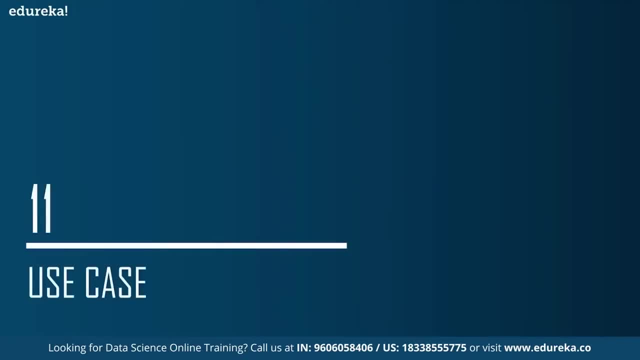 So, like I said, information gain and entropy are very important statistical measures that let us understand the significance of a prediction. To get a more clear understanding, let's look at a use case. All right, now suppose we're given a problem statement. 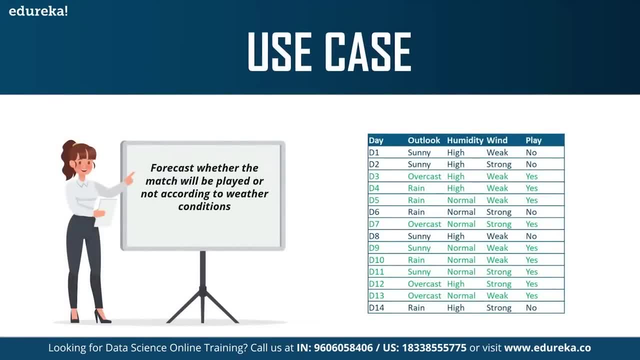 All right. the statement is that you have to predict whether a match can be played or not by studying the weather conditions. So the predictor variables here are outlook, humidity, wind Day is also a predictor variable. The target variable is basically play. 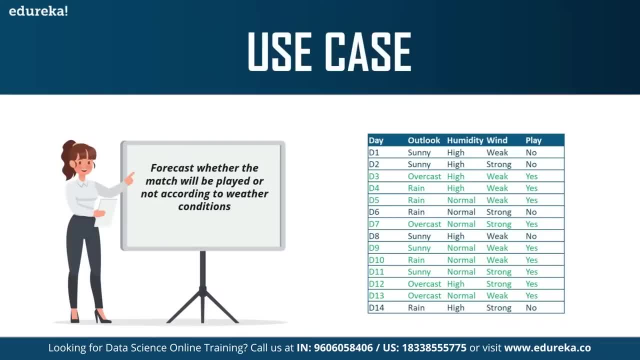 All right, the target variable is the variable that you're trying to predict. okay, now, the value of the target variable will decide whether or not a game can be played. all right, so that's why the play has two values. it has no and yes. no meaning that the weather conditions are not. 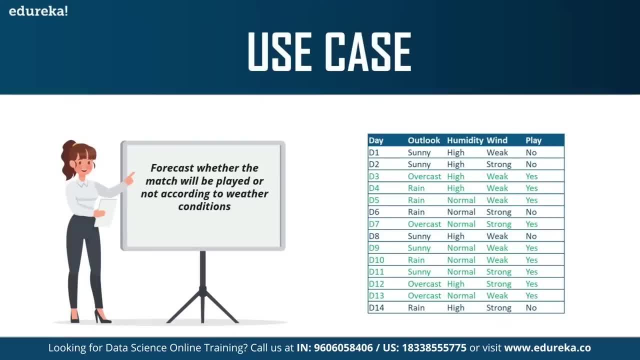 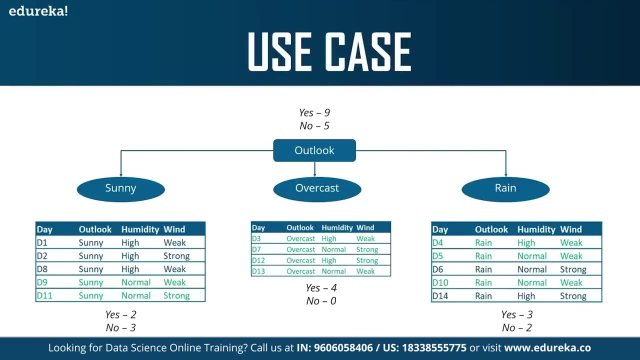 good and therefore you cannot play the game. yes, meaning that the weather conditions are good and suitable for you to play the game. all right, so that was a problem statement. i hope the problem statement is clear to all of you now. to solve such a problem, we make use of something known as. 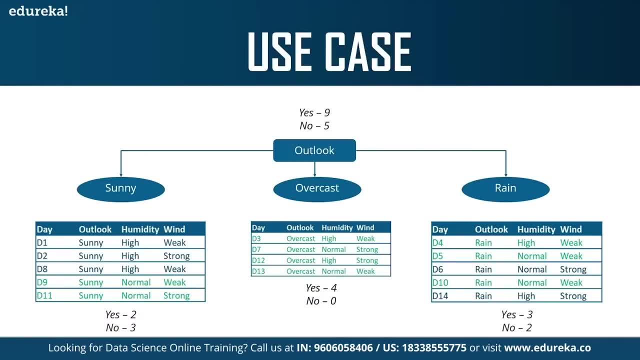 decision trees. so guys think of an inverted tree and each branch of the tree denotes some decision. all right, each branch is known as the branch node, and at each branch node you're going to take a decision in such a manner that you'll get an outcome at the end of the branch. all right now. 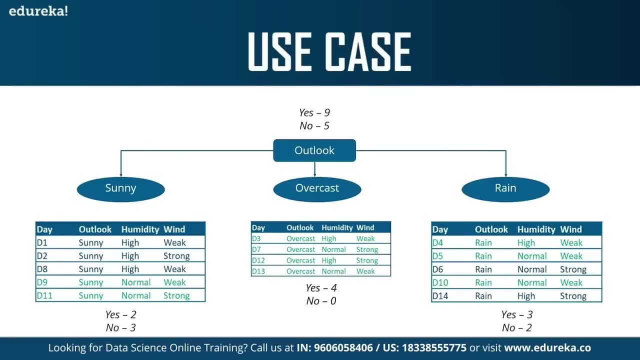 this figure here basically shows that out of 14 observations, nine observations result in a yes, meaning that out of 14 days, the match can be played only on nine days days. all right, so here, if you see, on day 1, day 2, day 8, day 9 and day 11, the 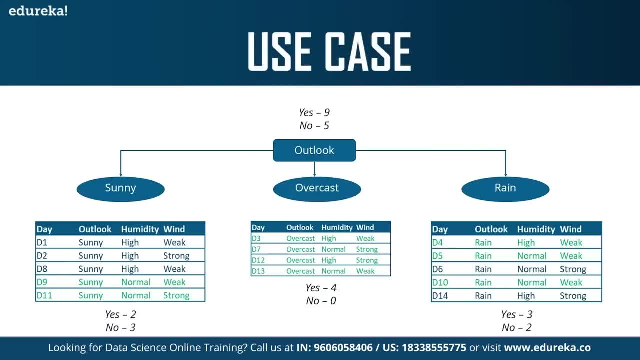 outlook has been sunny, all right. so basically, we're trying to cluster our data set depending on the outlook. so when the outlook is sunny, this is our data set. when the outlook is overcast, this is what we have, and when the outlook is rain, this is what we have, all right. so when it is sunny, we have two. 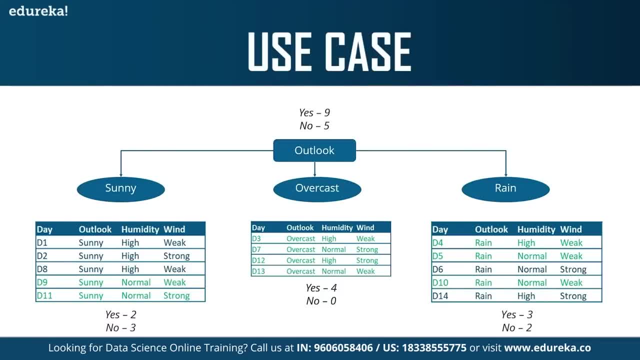 yeses and three no's. okay, when the outlook is overcast, we have all four as yeses, meaning that on the four days when the outlook was overcast, we can play the game all right. now, when it comes to rain, we have three yeses and two no's- all. 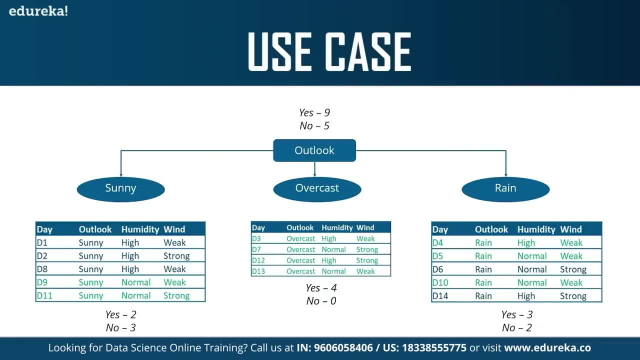 right. so, if you notice, here the decision is being made by choosing the outlook variable as the root node. okay, so the root node is basically the topmost node in a decision tree. now, what we've done here is we've created a decision tree that starts with the outlook node. all right, then you're. 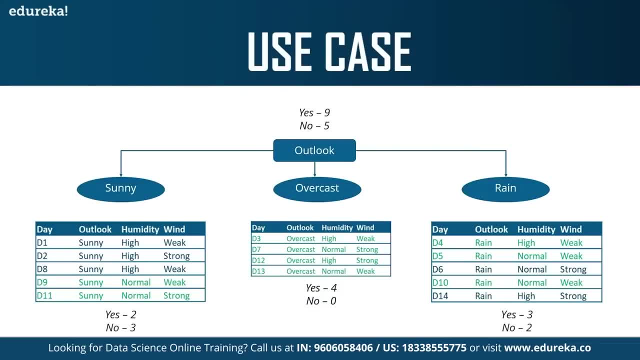 splitting the decision tree further depending on other parameters like sunny, overcast and rain. all right now, like we know, that outlook has three values- sunny, overcast and rain- so let me explain this in a more in-depth manner. okay, so what you're doing here is you're making the decision tree by choosing the outlook. 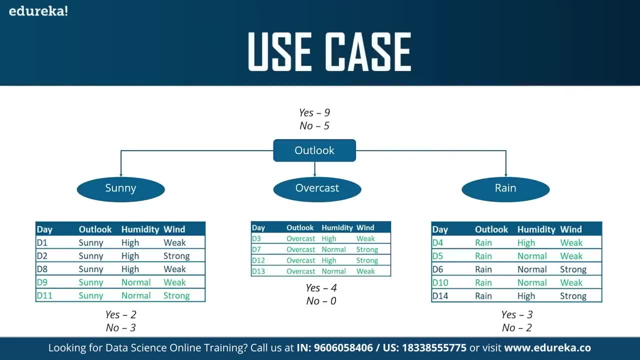 variable at the root node. the root node is basically the topmost node in a decision tree. now the outlook node has three branches coming out from it, which is sunny, overcast and rain. so basically Outlook can have three values: either it can be sunny, it can be 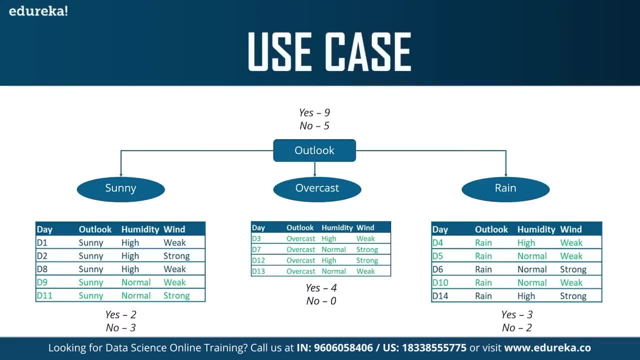 overcast or it can be rainy. okay now, these three values are assigned to the immediate branch nodes and for each of these values, the possibility of play is equal to. yes is calculated, so the sunny and the rain branches will give you an impure output, meaning that there is a mix of yes. 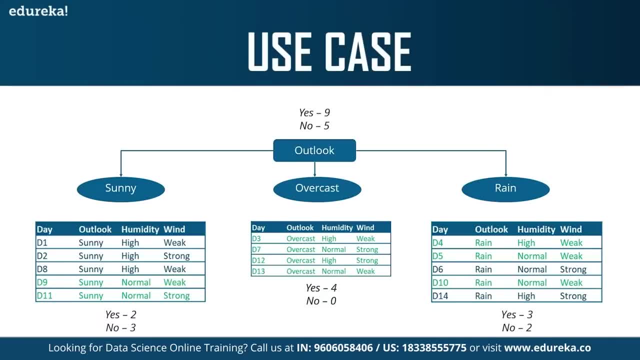 and no right. there are two Yeses here and there is no equal to yes here. there is no equal and there are two Yeses here. fit in between a yes and a right, no right. there are two yeses here, three no's here. there are three yeses here and two nodes over here. 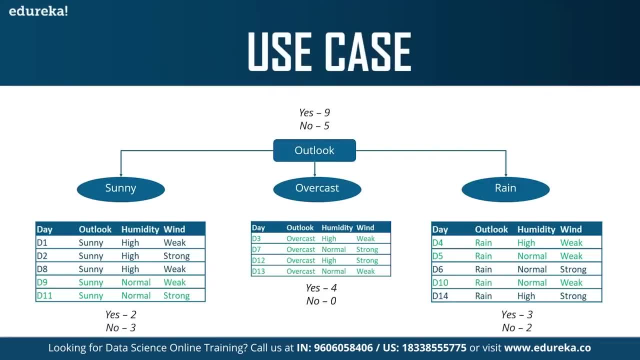 but when it comes to the overcast variable, it results in a hundred percent pure subset. all right, this shows that the overcast variable will result in a definite and certain output. this is exactly what entropy is used to measure. all right, it calculates the impurity, or. 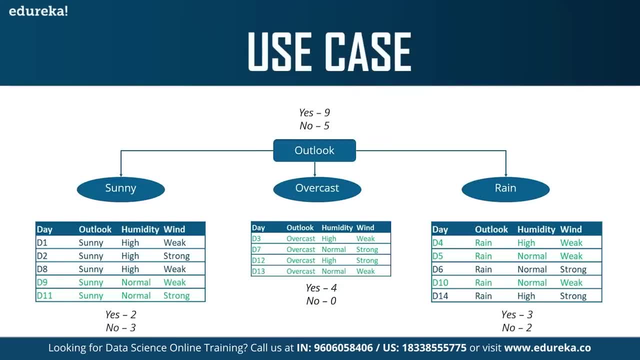 the uncertainty, all right. so the lesser the uncertainty or the entropy of a variable, more significant is that variable. so when it comes to overcast, there's literally no impurity in the data set. it is a hundred percent pure subset, right. so we want variables like these in order to build a 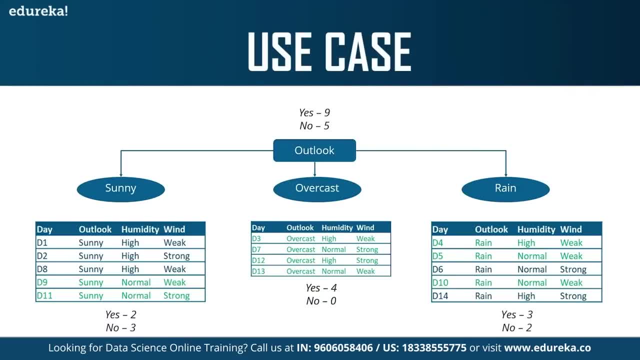 model. all right now, we don't always get lucky and we don't always find variables that will result in pure subsets. that's why we have the measure entropy. so the lesser the entropy of a particular way variable, the most significant that variable will be. so in a decision tree the root node is assigned. 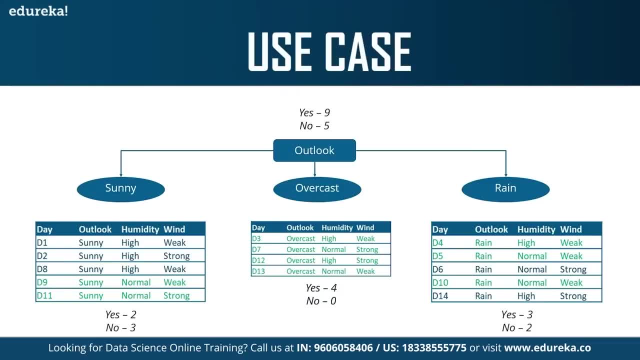 the best attribute, so that the decision tree can predict the most precise outcome, meaning that, on the root node, you should have the most significant variable. all right, that's why we've chosen outlook, all right. now, some of you might ask me: why haven't you chosen overcast? now guys, overcast is not a 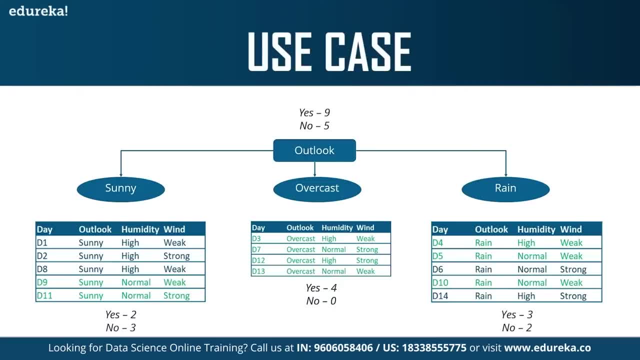 variable. it is a value of the outlook variable, all right, that's why we've chosen outlook here, because it has a hundred percent pure subset which is overcast. all right now. the question in your head is: how do i decide which variable or attribute best splits the data? now, right now, i know i looked at the 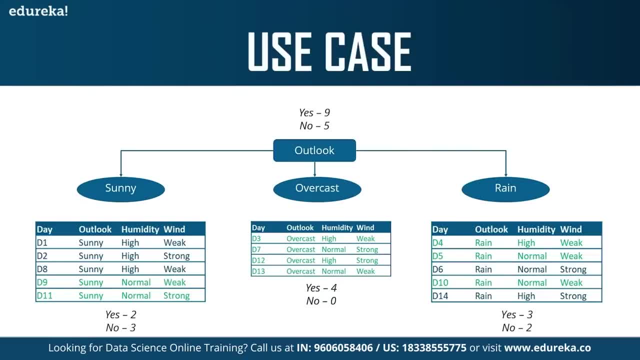 data and i told you that you know, uh, here we have a hundred percent pure subset, but what if it's a more complex problem and you're not able to understand which variable will best split the data? so, guys, when it comes to decision trees, information and gain and entropy will help you. 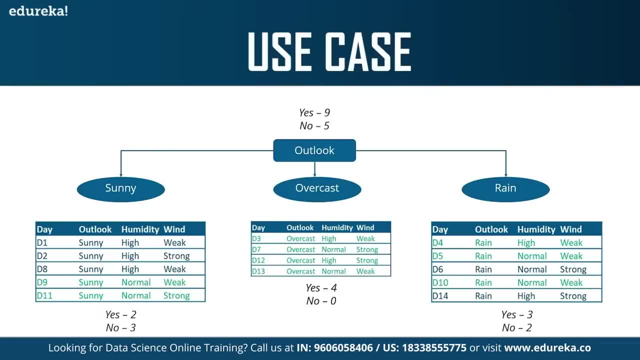 understand which variable will best split the data set- all right- or which variable you have to assign to the root node, because whichever variable is assigned to the root node, it will best split the data set, and it has to be the most significant variable, all right. so how we can do this is we need 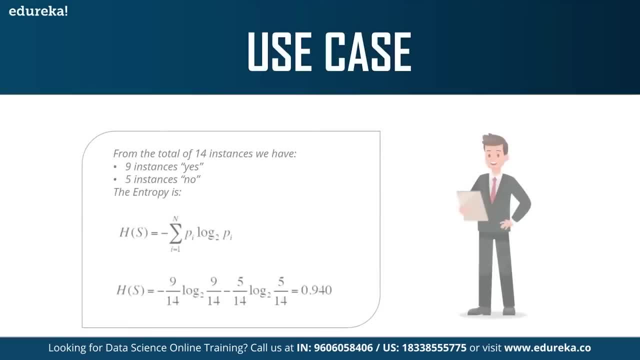 to use information gain and entropy. so from the total of the 14 instances that we saw, nine of them said yes and five of the instances said no, that you cannot play on that particular day. all right, you calculate the entropy. so this is the formula. you just substitute the values in the formula. so 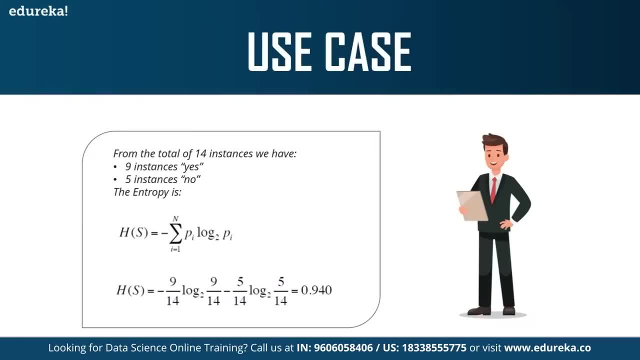 when you substitute the values in the formula, you'll get a value of 0.940. all right, this is the entropy, or this is the uncertainty, of the data present in our sample. now, in order to ensure that we choose the best variable for the root node, let us look at all the possible combinations that you. 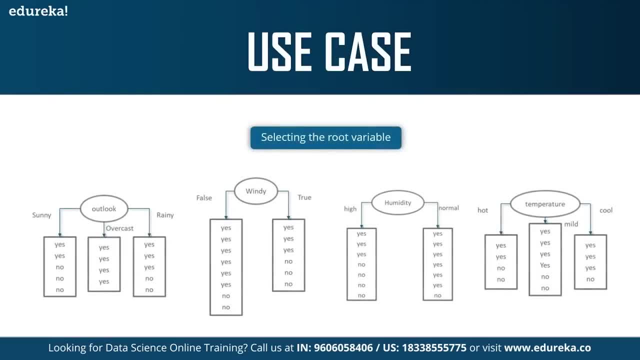 can use on the root node. okay, so these are all the possible combinations. you can either have outlook, outlook outlook humidity or temperature. okay, these are our four variables and you can have any one of these variables as your root node. but how do you select which variable best fits the root node? 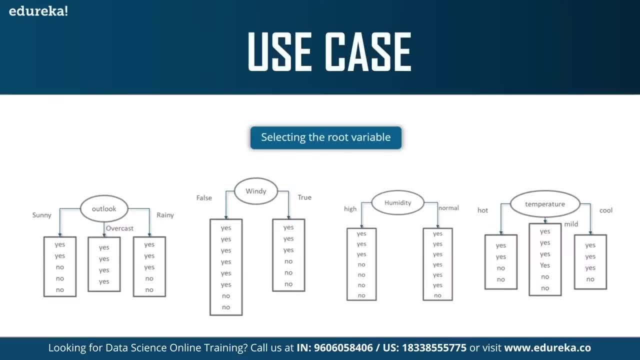 that's what we're going to see by using information gain and entropy. so, guys, now the task at hand is to find the information gain for each of these attributes. all right, so for outlook, for windy, for humidity and for temperature, we're going to find out the information gain. all right, now a point. 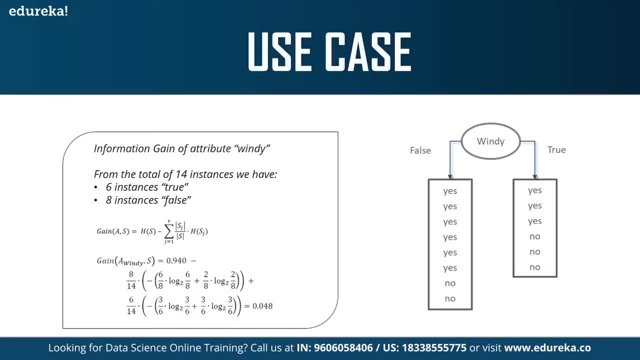 the variable that results in the highest information gain must be chosen because it will give us the most precise and output information. all right, so the information gain for attribute windy, we'll calculate that first. here we have six instances of true and eight instances of false. okay, so when you substitute all the 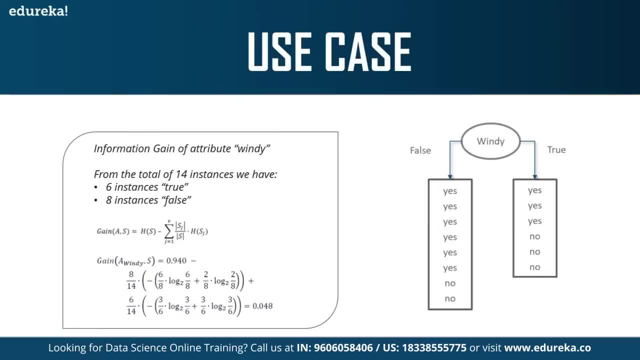 values in the formula, you'll get a value of 0.048. so we get a value of 0.048. now, this is a very low value for uh information gain. all right. so the information that you're going to get from windy attribute is pretty low, so let's. 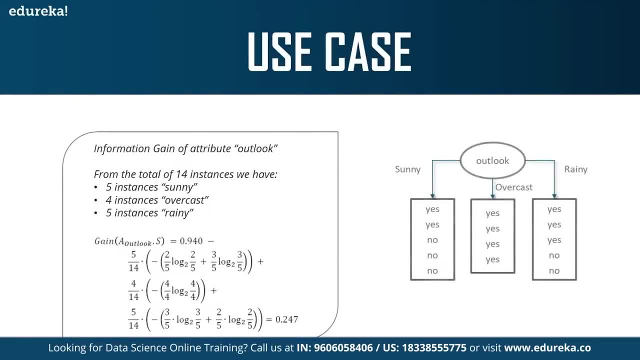 calculate the information gain of attribute outlook. all right, so from the total of 14 instances, we have five instances which say sunny, four instances which are overcast and five instances which are rainy. all right, for sunny, we have three yeses and two no's. for overcast, we have all the four as yes. for rainy, we have three yes and two. 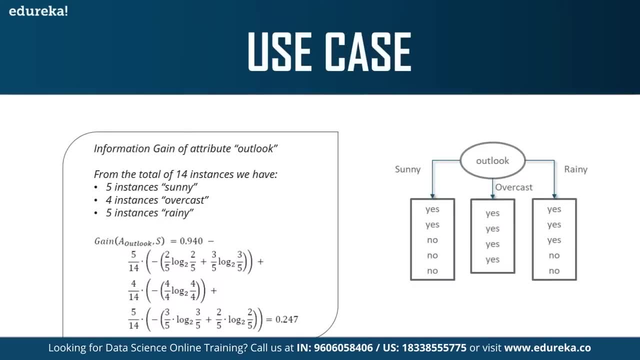 no's okay. so when you calculate the information gain of the outlook variable, we'll get a value of 0.247. now compare this to the information gain of the windy attribute. this value is actually pretty good. right? we have 0.247, which is a pretty good value for information gain. 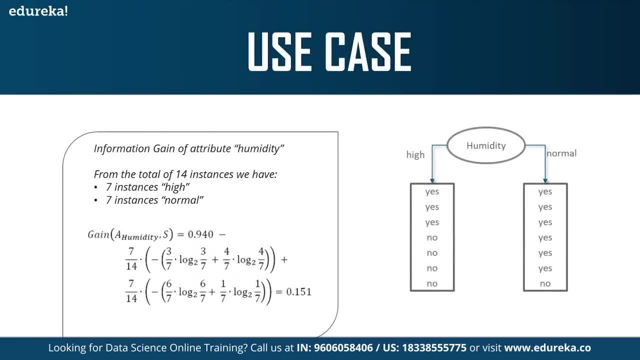 now let's look at the information gain of attribute humidity. now over here we have seven instances which say high and seven instances which say normal. right and under the high branch node we have three instances which say yes and the rest four instances which say no. similarly, under the normal branch we have 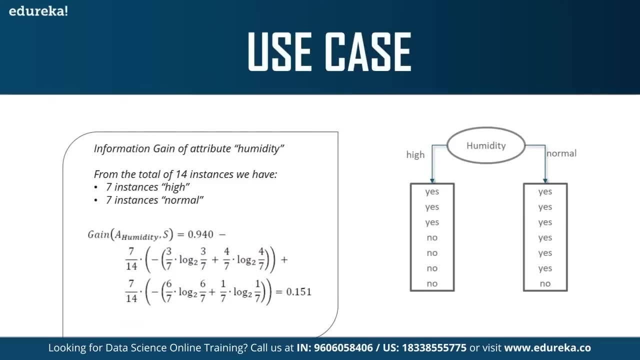 one, two, three, four, five, six, seven instances which say yes and one instance which says no. all right, so when you calculate the information gain for the humidity variable, you're going to get a value of 0.151. now, this is also a pretty decent value, but when you compare it to the 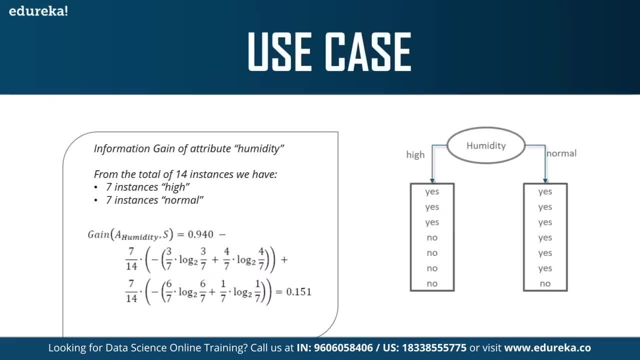 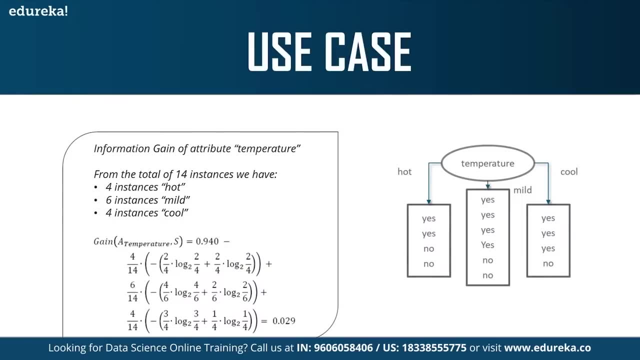 information gain of the attribute outlook. it is less right now. let's look at the information gain of attribute temperature. all right, so the temperature can hold. repeat. so basically the temperature attribute can hold. hot, mild and cool. okay, under hot, we have two instances which says yes and two instances for no. under mild, we have four instances of. 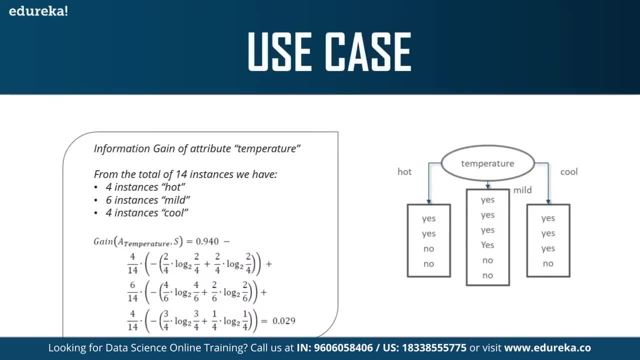 yes and two instances for no. so under mild we have four instances of yes and two instances for no, and under cool we have three instances of yes and one instance of no. all right now, when you calculate the information gain for this attribute, you'll get a value of 0.029, which is again very 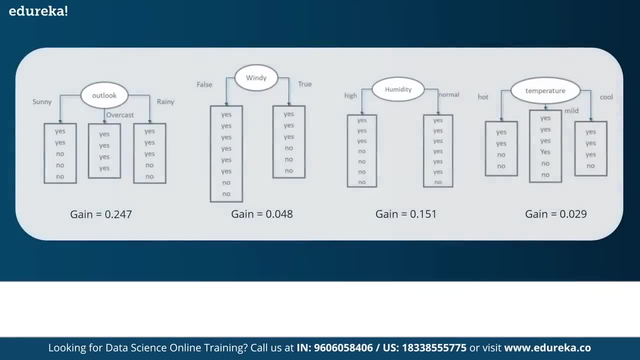 less so. what you can summarize from here is, if we look at the information gain for each of these variables, we'll see that for outlook, we have the maximum gain. all right, we have 0.247, which is the highest information gain value, and you must always choose a variable with the highest information gain to split the data at the 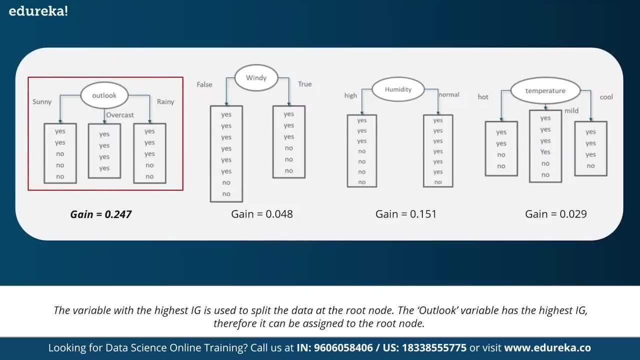 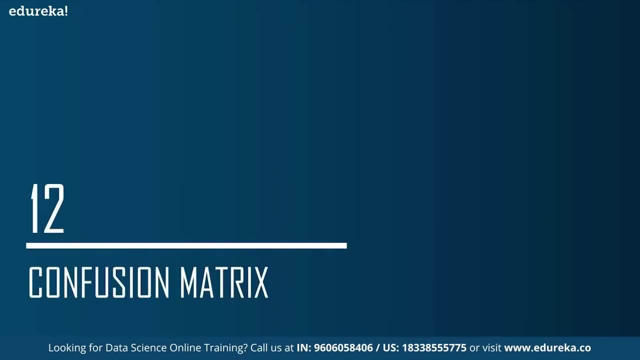 root node. so that's why we assign the outlook variable at the root node. all right, so, guys, i hope this use case was clear. if any of you have doubts, please keep commenting those doubts. now let's move on and look at what exactly a confusion matrix is. now the confusion matrix is the last. 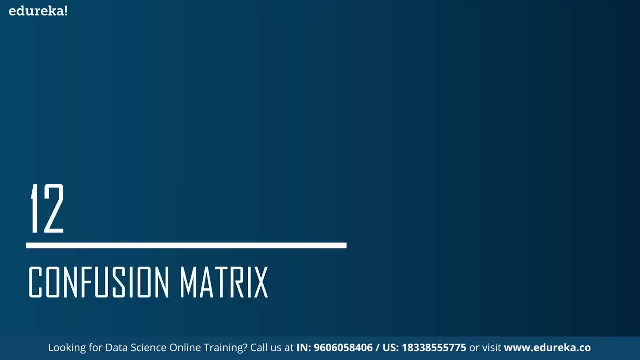 topic for descriptive statistics. all right, after this, i'll be running a short demo where i'll be showing you how to use a confusion matrix. and i'm going to show you how to use a confusion matrix, how you can calculate mean, median mode and standard deviation variance, and all of those. 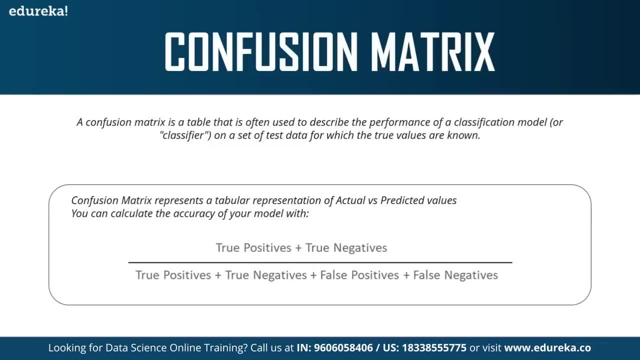 values by using r. okay, so let's talk about confusion matrix now, guys, what is a confusion matrix? now, don't get confused. this is not any complex topic now. confusion matrix is a matrix that is often used to describe the performance of a model. all right, and this is specifically. 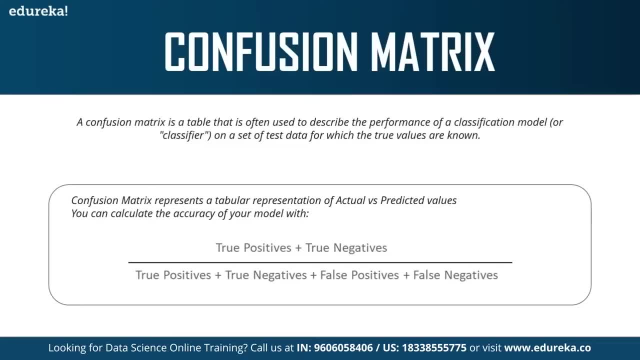 used for classification models or a classifier, and what it does is it will calculate the accuracy or it will calculate the performance of your classifier by comparing your actual results and your predicted results. all right, so this is what it looks like: two positive plus true negative and all of that. now, this is a little confusing. i'll get back to. 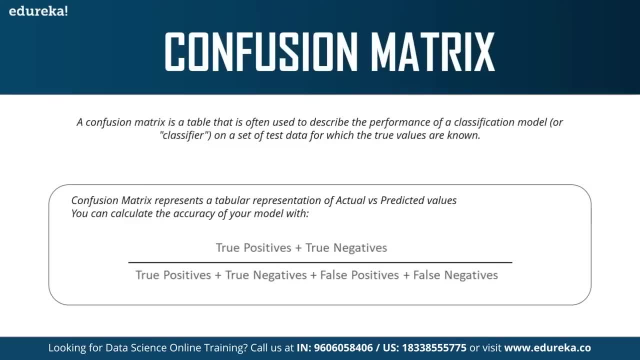 what exactly true, positive, true, negative and all of this stands for. for now, let's look at an example and let's try and understand what exactly confusion matrix is. so, guys, i made sure that i put examples after each and every topic because it's important you understand the practical part of statistics. all. 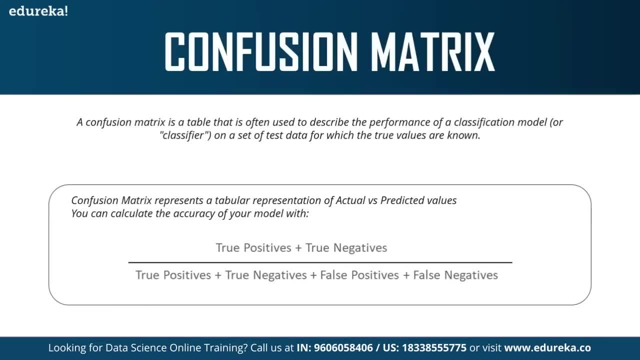 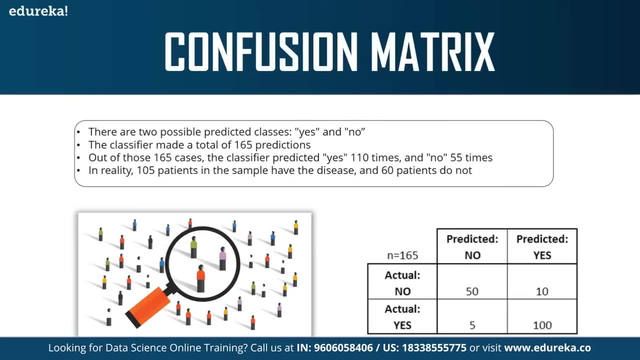 right. statistics has literally nothing to do with theory. you need to understand how calculations are done in statistics. okay, so here, what I've done is now let's look at a small use case. okay, let's consider that you're given data about hundred and sixty five patients, out of which hundred and five patients have a. 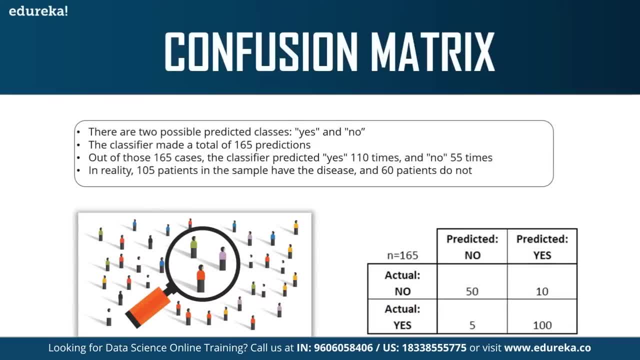 disease and the remaining fifty patients don't have a disease. okay, so what you're going to do is you will build a classifier that predicts by using these hundred and sixty five observations. you'll feed all of these 165 observations to your classifier and it will predict the output every time a new. 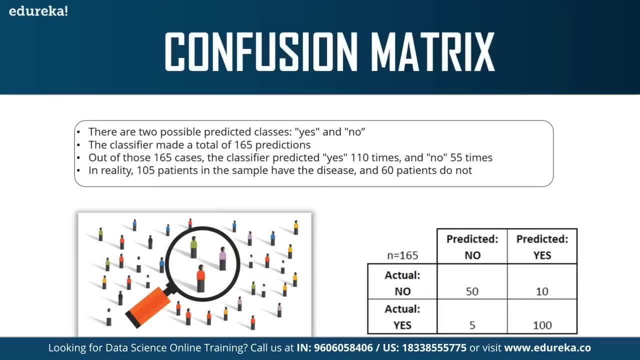 patient's detail is fed to the classifier right now, out of these 165 cases, let's say that the classifier predicted yes 110 times and no 55 times. all right, so yes basically stands for yes- the person has a disease, and no stands for no- the person does not have a disease. all right, that's pretty. 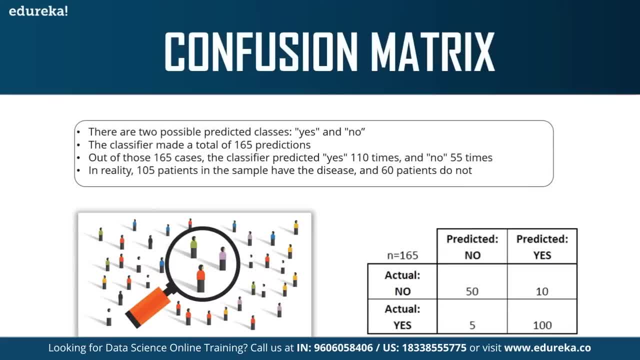 self-explanatory, but yeah, so it predicted that one hundred and ten times the patient has a disease and 55 times that, no, the patient doesn't have a disease. however, in reality, only 105 patients in the sample have the disease and 60 patients who do not have the disease, right? so how do you calculate? 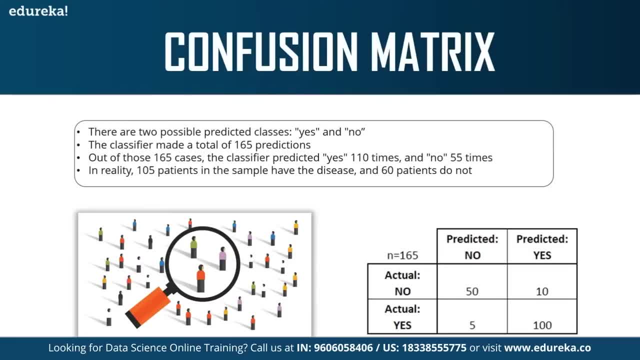 the accuracy of your model. you basically build the confusion matrix, alright, this? This is how the matrix looks like and basically denotes the total number of observations that you have, which is 165 in our case. Actual denotes the actual values in the data set and predicted denotes the predicted values. 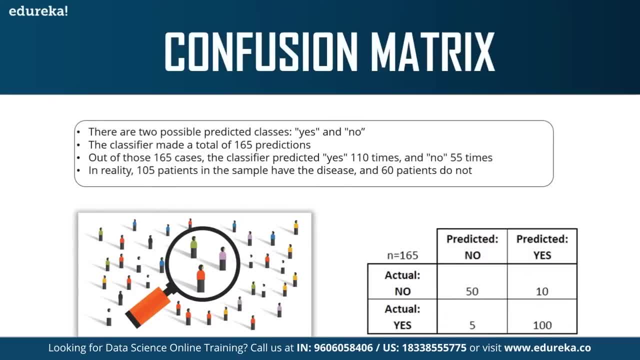 by the classifier. So the actual value is no here and the predicted value is no here. So your classifier was correctly able to classify 50 cases as no, Since both of these are no. so 50 it was correctly able to classify but 10 of these cases. it. 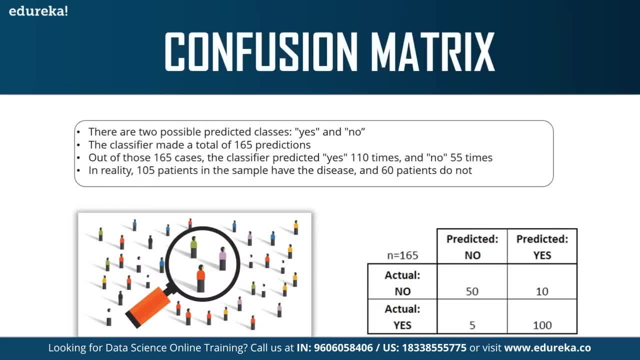 incorrectly classified, meaning that your actual value here is no, but your classifier predicted it as yes. Alright, that's why there's 10 over here. Similarly, it wrongly predicted that 5 patients do not have diseases, whereas they actually did have diseases, and it correctly predicted 100 patients which had the disease. 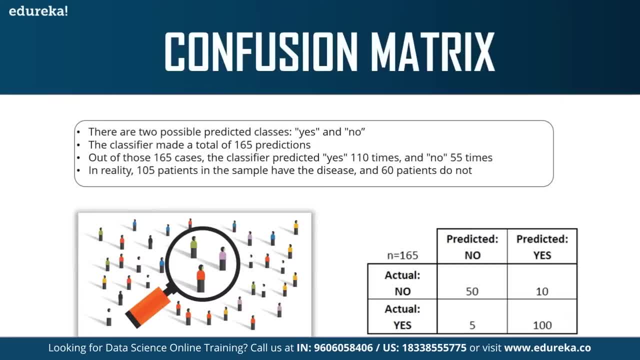 Alright, I know this is a little bit confusing, But if you look at these values- no, no, 50, meaning that it correctly predicted 50 values- No, yes means that it wrongly predicted yes for the values that it was supposed to predict. 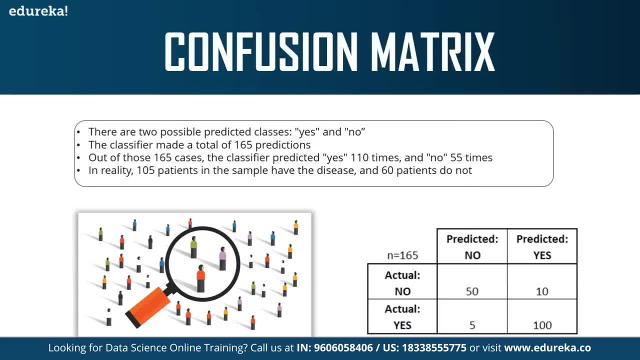 no. Alright. now, what exactly is this? true positive, true negative and all of that. I'll tell you what exactly it is So true positive are the cases in which we predicted a yes and they do not actually have the disease. Alright. 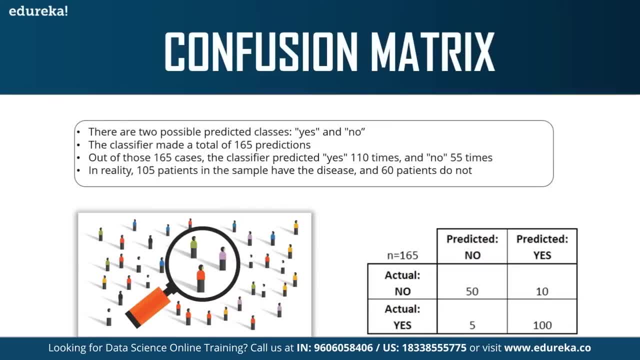 So it is basically This value. Alright, we predicted a yes here, even though they did not have the disease. So we have 10 true positives Right. Similarly true negative is we predicted no and they don't have the disease, meaning that: 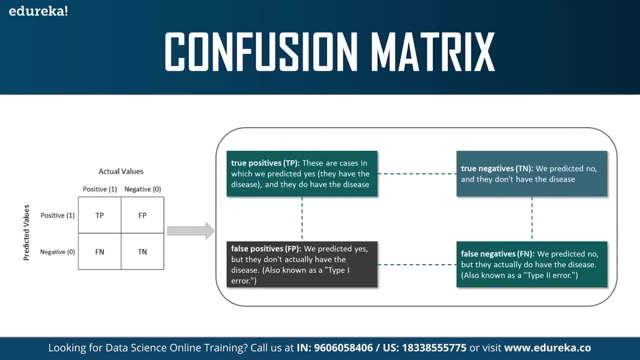 this is correct. False positive is: we predicted yes, but they do not actually have the disease. Alright, this is also known as type 1 error. False negative is we predicted no, but they actually do not have the disease. So, guys, basically false negative and true negative. 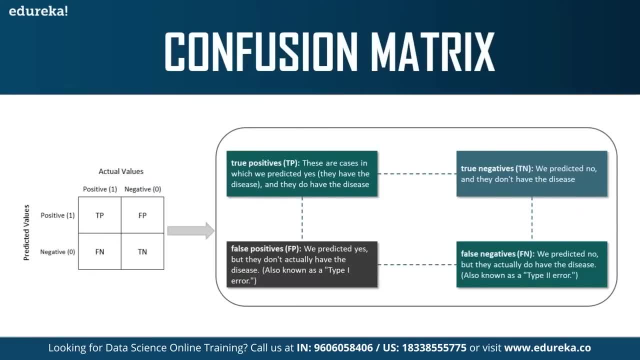 Okay And true negatives are basically correct classifications. Alright, So this was confusion matrix and I hope this concept is clear. So, guys, that was descriptive statistics. Now, before we go to probability, I promised you all that we'll run a small demo in R. 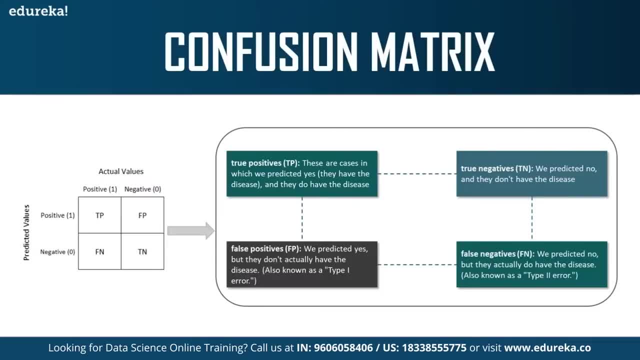 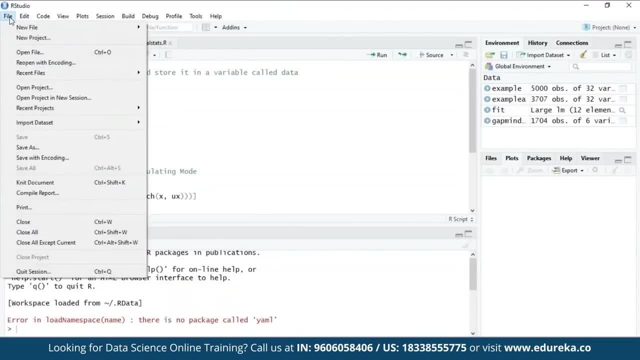 Alright, we'll try and understand how mean median mode works in R. Okay, so let's do that first. So, guys, again, what we just discussed so far was descriptive statistics. Alright, Next We'll discuss probability and then we'll move on to inferential statistics. 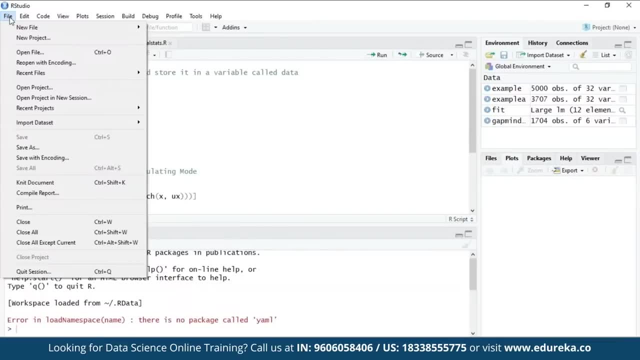 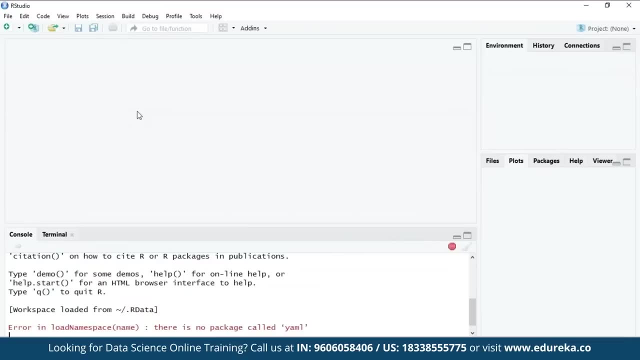 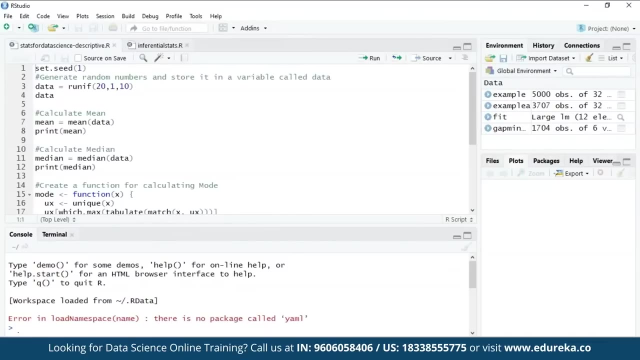 Okay, Inferential statistics is basically the second type of statistics. Okay, Now, to make things more clearer for you, Let me just zoom in. So, guys, it's always best to perform practical implementations in order to understand the concepts in a better way. 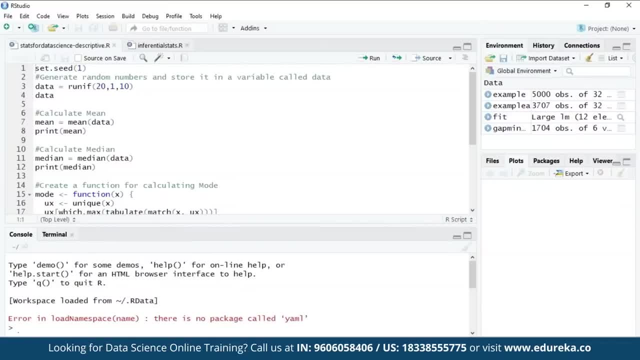 Okay, So here we'll be executing a small demo that will show you how to calculate the mean, median mode, variance, standard deviation and how to study the variables by plotting a histogram. Okay, Don't worry if you don't know what a histogram is. it's basically a frequency plot. 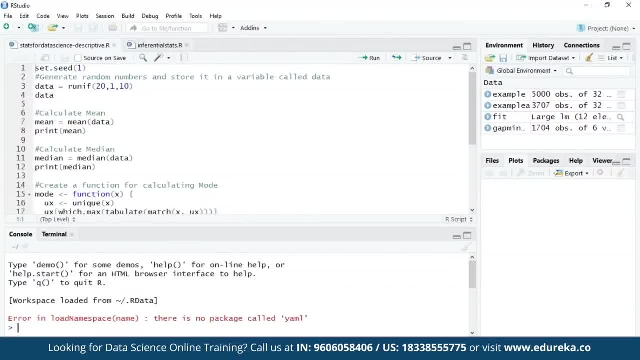 There's no big science behind it. Alright, This is a very simple demo, but it also forms a foundation that every machine learning algorithm is built upon. Okay, you can say that most of the machine learning algorithms- actually all the machine learning algorithms and deep learning algorithms- have this basic concept behind them. 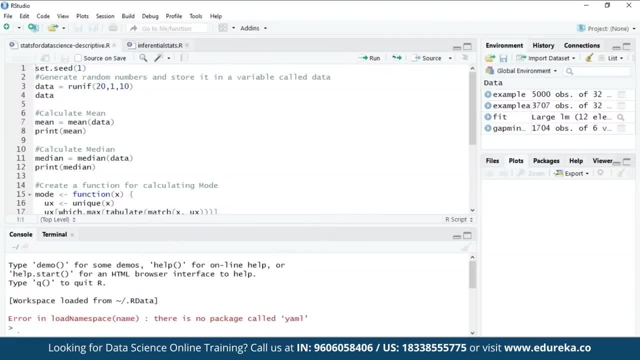 Okay, You need to know how mean median mode and all of that is calculated. So, guys, I'm using the R language to perform this and I'm running this on R studio. For those of you who don't know R language, I will leave a couple of links in the description. 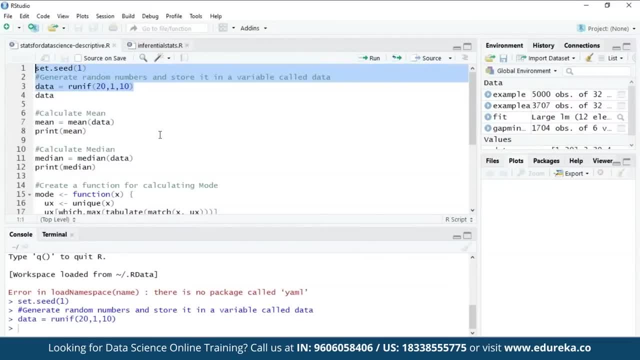 box, You can go through those videos. So what we're doing is we're randomly generating numbers and we're storing it in a variable called data Alright. So if you want to see the generated numbers, just run the line data Alright. 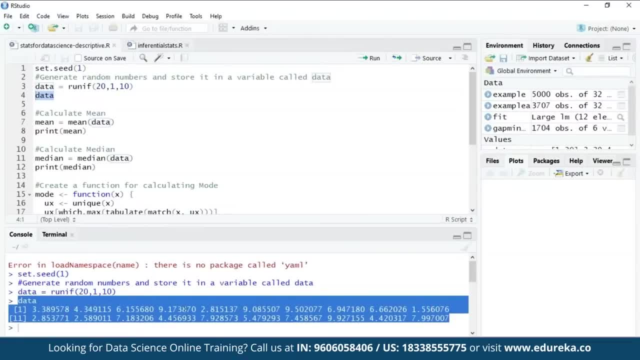 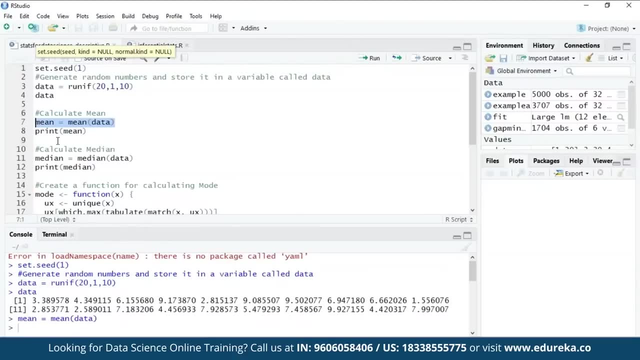 This variable basically stores all the variables. Okay, All our numbers. Alright, Now what we're going to do is we're going to calculate the mean. Now, all you have to do in R is specify the word mean along with the data that you're. 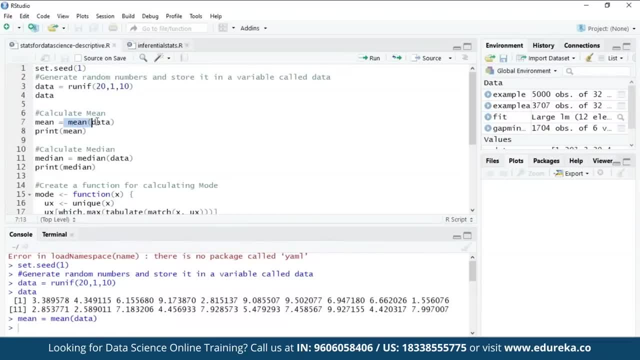 calculating the mean of, And I've assigned this whole thing into a variable called mean, which will hold the mean value of this data. So now let's look at the mean. For that I've used a function called print and mean. Alright, 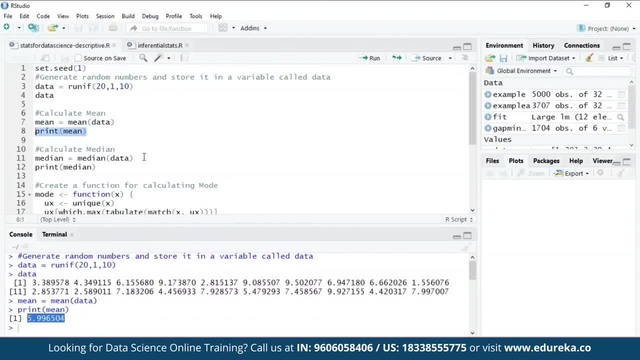 So our mean is around 5.99.. Okay, Next is calculating the median. It's very simple, guys. All you have to do is use a function- median Alright- And pass the data as a parameter to this function. That's all you have to do. 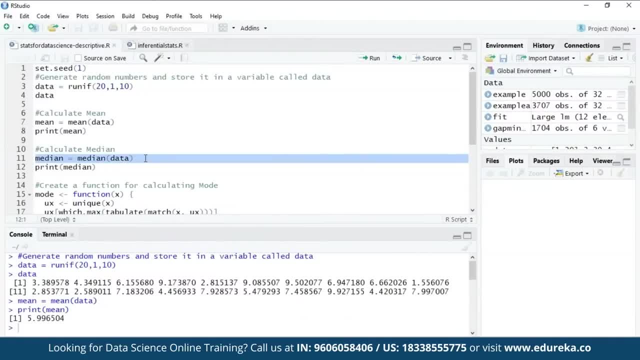 So R provides functions for each and everything. Alright, Statistics is very easy when it comes to R, because R is basically a statistical language. Okay, So all you have to do is just name the function, And that function is already inbuilt in your R. 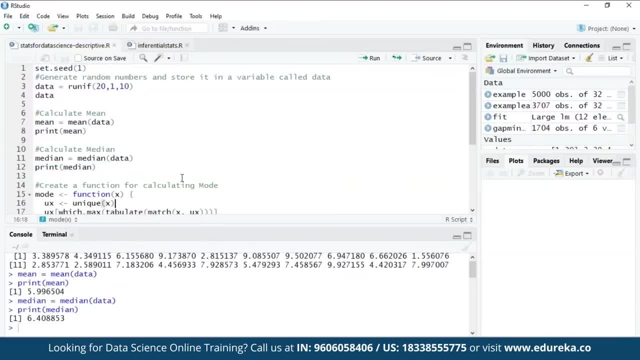 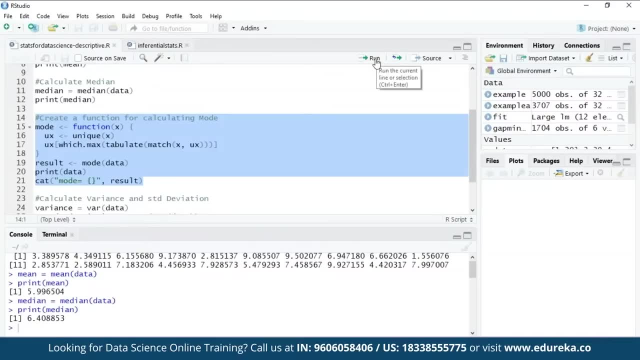 Okay, So your median is around 6.4.. Similarly, we'll calculate the mode. Alright, Let's run this function. I've basically created a small function for calculating the mode. So, guys, this is our mode, meaning that this is the most recurrent value. 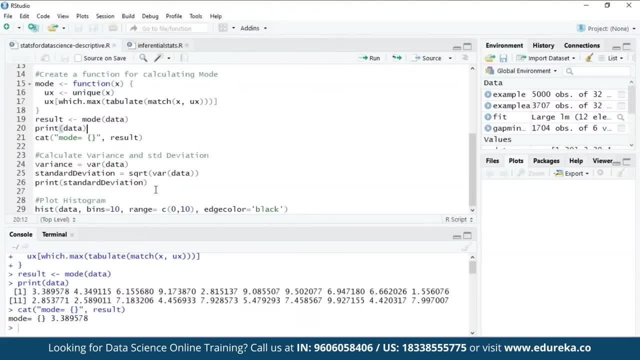 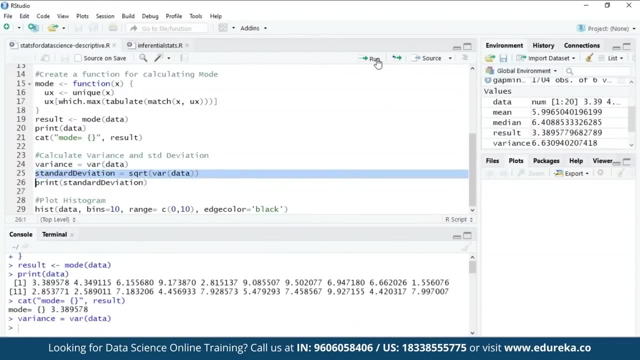 Right Now we're going to calculate the variance and the standard deviation. For that, again, we have a function in R called as var. Alright, So what we're going to do is pass the data to that function, Okay, Similarly, we'll calculate the standard deviation, which is basically the square root of your. 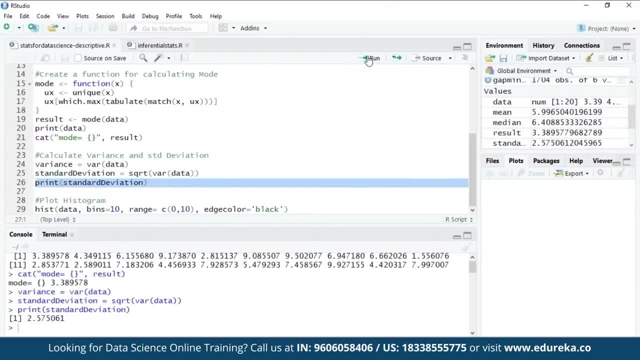 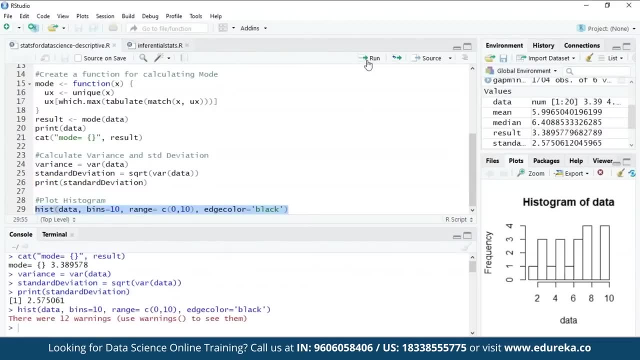 variance. Right Now we'll print the standard deviation. Right, This is our standard deviation value. Now, finally, we'll just plot a small histogram. Histogram is nothing, but it's a frequency plot. Alright, It'll show you how frequently a data point is occurring. 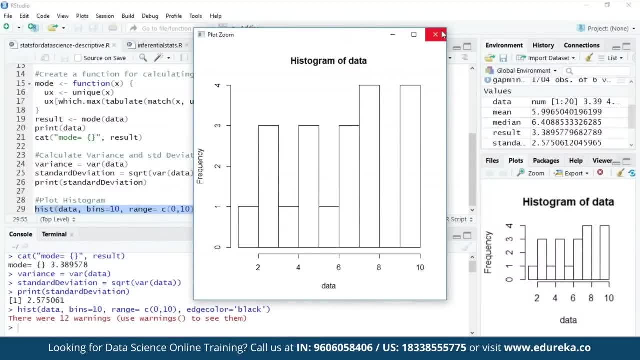 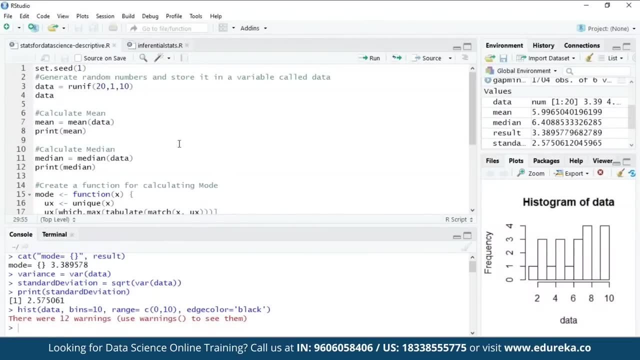 So this is the histogram that we've just created. It's quite simple in R, Because R has a lot of packages and a lot of inbuilt functions that support statistics. Alright, It is a statistical language that is mainly used by data scientists or by data analysts. 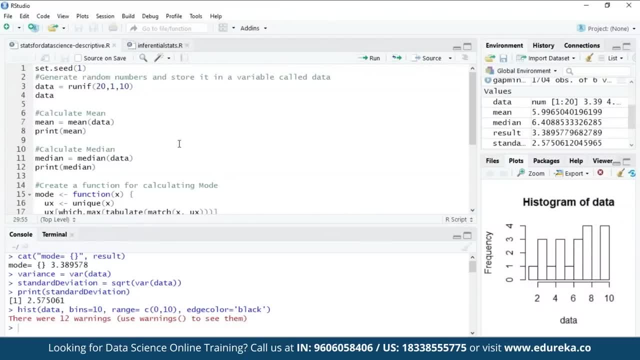 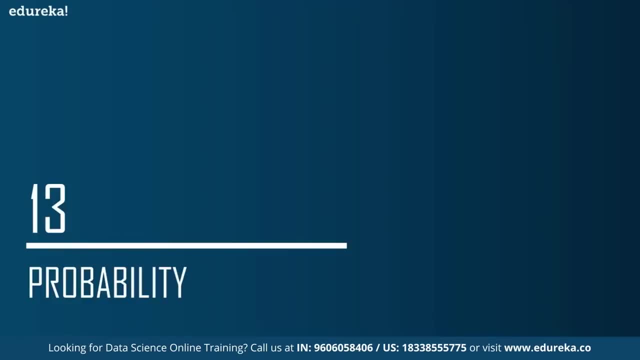 and machine learning engineers, because they don't have to sit and code these functions. All they have to do is they have to mention the name of the function and pass the corresponding parameters. So, guys, that was the entire descriptive statistics module, And now we'll discuss about probability. 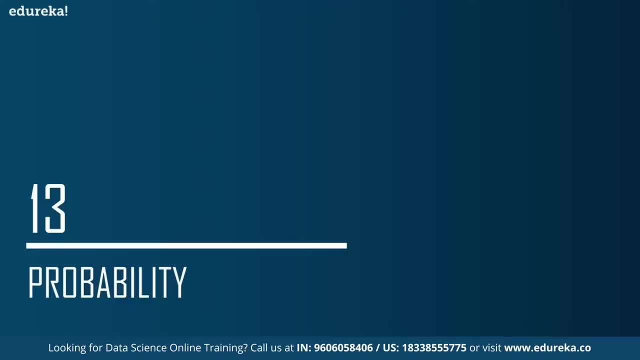 Okay, So before we understand what exactly probability is, let me clear out a very common misconception. People often tend to ask me this question: What is the relationship between statistics and probability? So probability and statistics are related fields? Alright, So probability is a mathematical method used for statistical analysis. 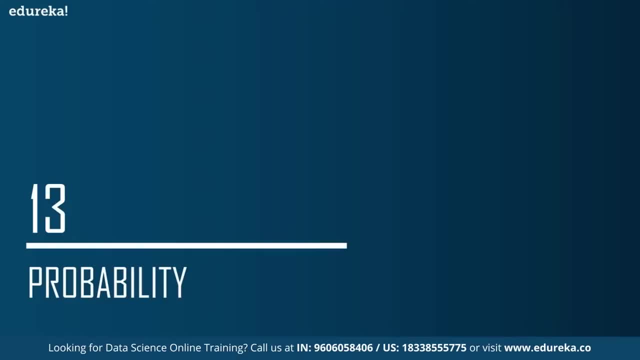 Therefore we can say that a probability and statistics are interconnected branches of mathematics That deal with analyzing The relative frequency of events. So they're very interconnected fields. and probability makes use of statistics and statistics makes use of probability. Alright, They're very interconnected fields. 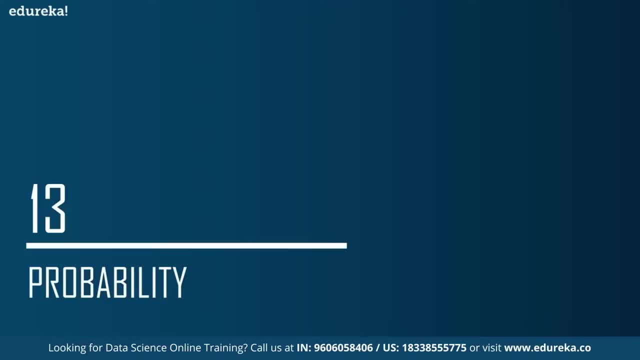 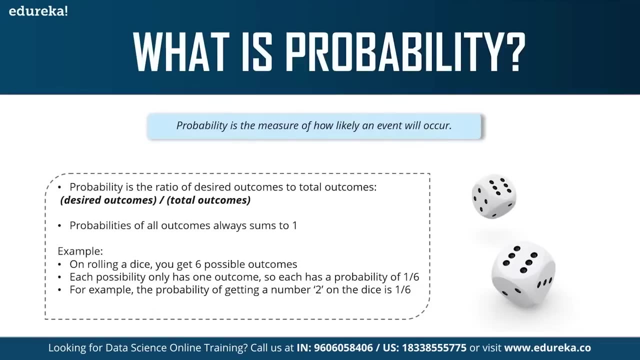 So that is the relationship between statistics and probability. Now let's understand what exactly is probability. So probability is the measure of how likely an event will occur. To be more precise, it is the ratio of desired outcome to the total outcome. Now, the probability of all outcomes always sum up to 1.. 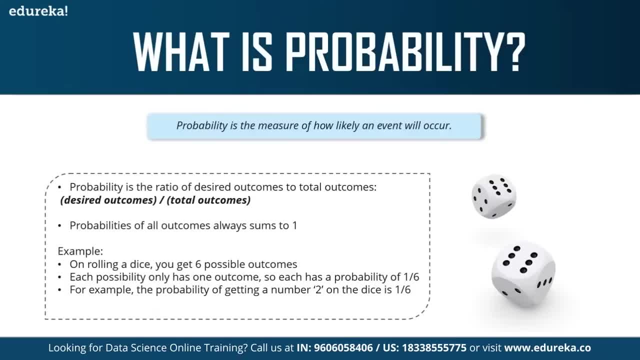 Now, the probability will always sum up to 1.. Probability cannot go beyond 1.. Okay, So either your probability can be 0, or it can be 1, or it can be in the form of decimals, like 0.52 or 0.55, or it can be in the form of 0.5, 0.7, 0.9.. 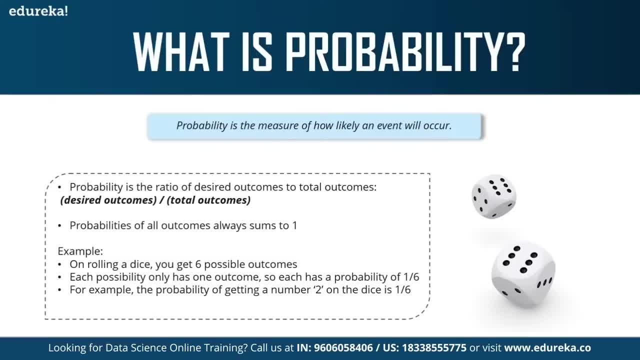 But its value will always stay between the range 0 and 1.. Okay, Another example of probability is rolling a dice example. So when you roll a dice, you get 6 possible outcomes. right, You get 1,, 2,, 3,, 4, and 5,- 6 phases of a dice. 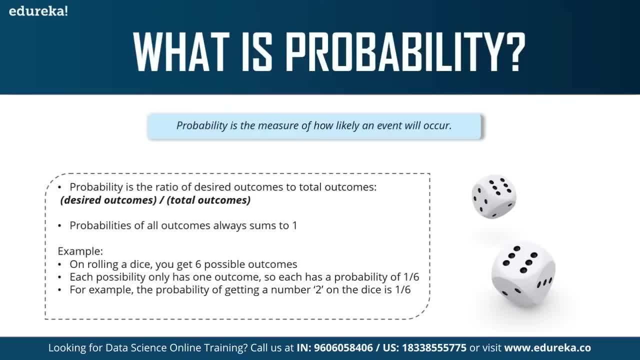 Now, each possibility only has one outcome. So what is the probability that, on rolling a dice, you'll get 3?? The probability is 1 by 6, right, Because there's only one phase which has the number 3 on it. 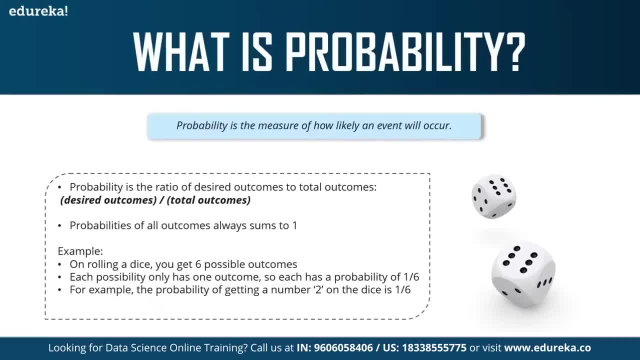 Out of 6 phases, there's only one phase which has the number 3.. So the probability of getting the number 3.. Okay, So the probability of getting 3 when you roll a dice is 1 by 6.. Similarly, if you want to find the probability of getting a number 5, again the probability. 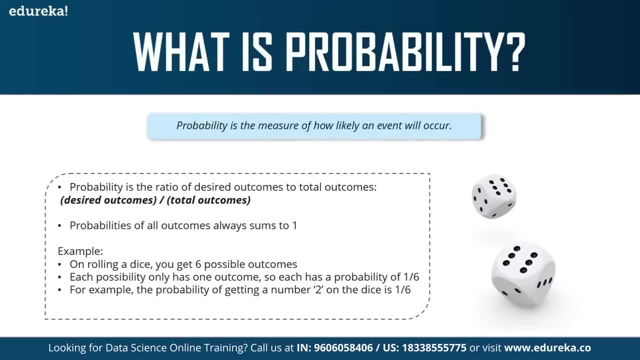 is going to be 1 by 6.. Alright, So all of this will sum up to 1.. Alright, So, guys, this is exactly what probability is. It's a very simple concept. We all learnt it in 8th standard onwards, right. 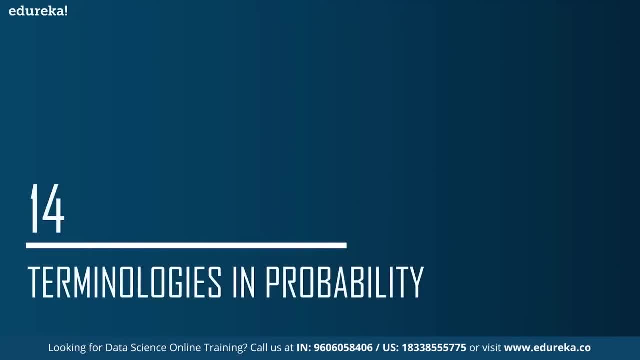 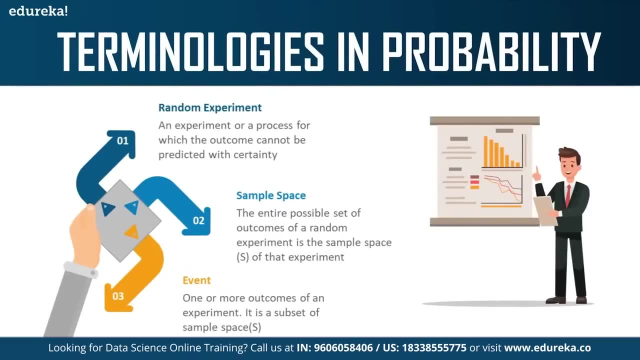 Now let's understand the different terminologies that are related to probability. Now there are 3 terminologies that you often come across when we talk about probability. We have something known as a random experiment. It's basically an experiment or a process for which the outcomes cannot be predicted. 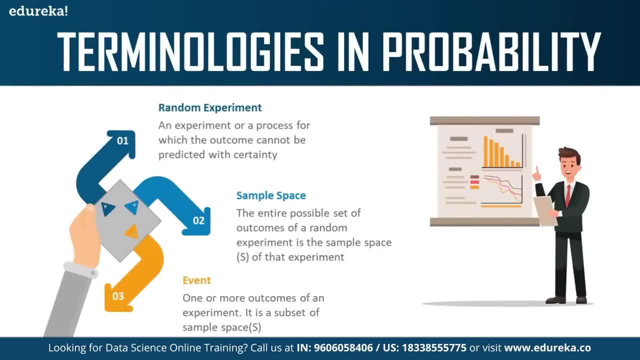 with certainty. Alright, That's why you use probability. You're going to use probability in order to predict the outcome with some sort of certainty. Sample space is the entire possible set of outcomes of a random experiment. An event is one or more outcomes of an experiment. 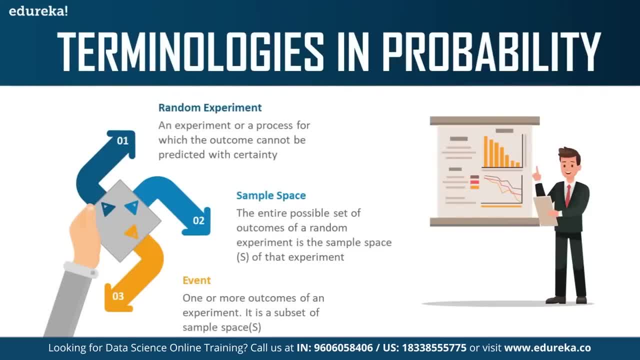 So if you consider the example of rolling a dice Now, let's say that you want to find out the probability of getting a 2 when you roll a dice. Okay, So finding this probability is the random experiment. The sample space is basically your entire possibility. 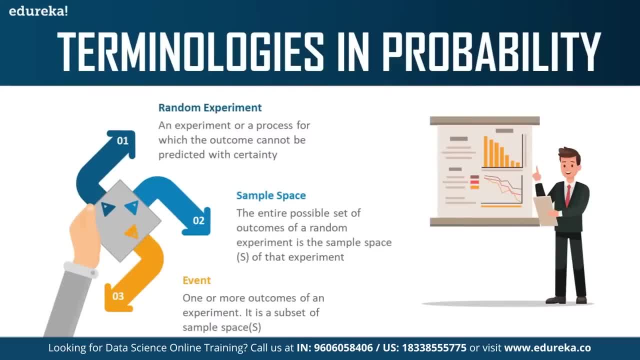 Okay, So 1,, 2,, 3,, 4,, 5, 6 phases are there, and out of that you need to find the probability of getting a 2. Right, So all the possible outcomes will basically represent your sample space. 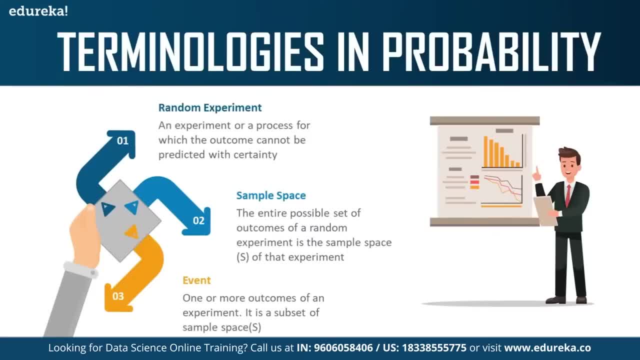 Okay, So 1 to 6 are all your possible outcomes. This represents your sample space. Now, event is one or more outcome of an experiment. So in this case, my event is to get a 2 when I roll a dice, Right, 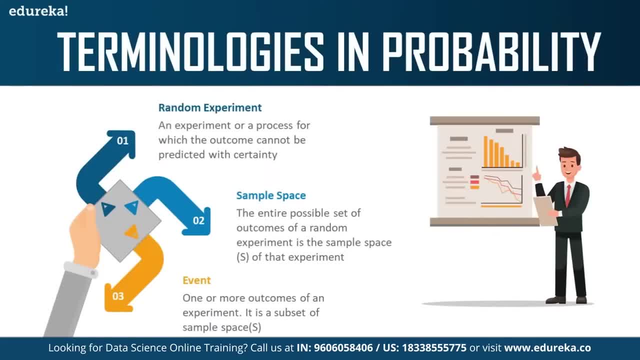 So my event is the probability of getting a 2 when I roll a dice. So, guys, this is basically what random experiment, sample, space and event really means. All right, Now let's discuss the different types of events. There are two types of events that you should know about. 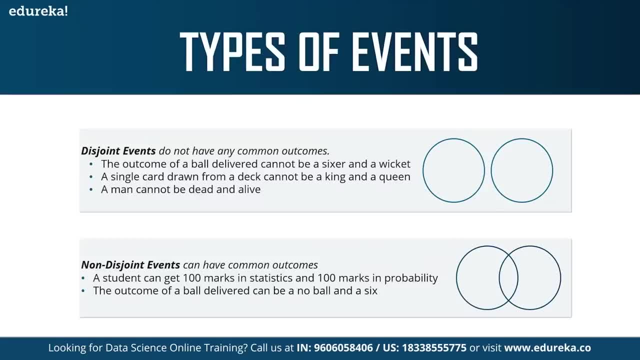 There is disjoint and non disjoint events. Disjoint events are events that do not have any common outcome. For example, if you draw a single card from a deck of cards, it cannot be a king and a queen. Correct, It can either be king or it can be queen. 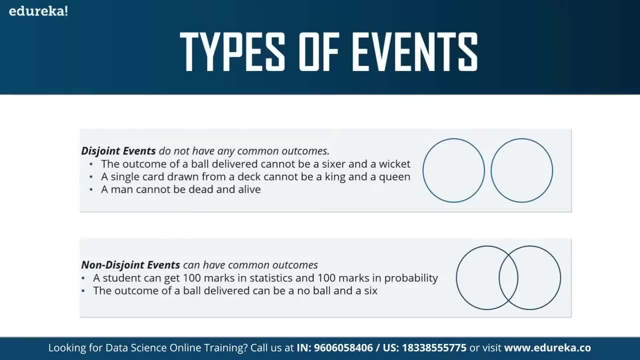 Now, non disjoint events are events that have common outcomes. For example, a student can get 100 marks in statistics and 100 marks in probability, All right. And also the outcome of a ball delivered can be a no ball and it can be a 6.. 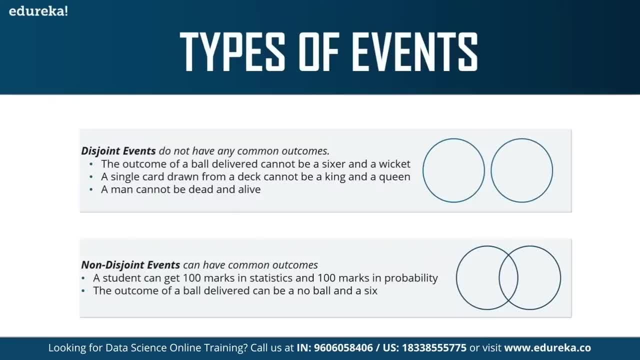 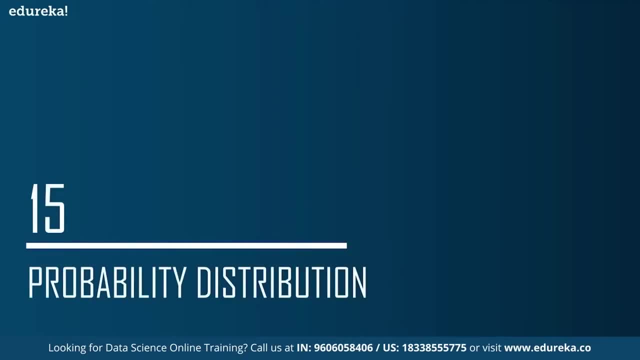 Right. So this is what non disjoint events are. All right, These are very simple to understand Right Now. let's move on and look at the different types of probability distribution. All right, I'll be discussing the three main probability distribution functions. 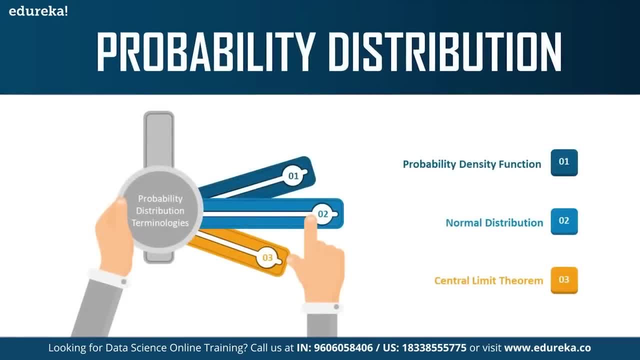 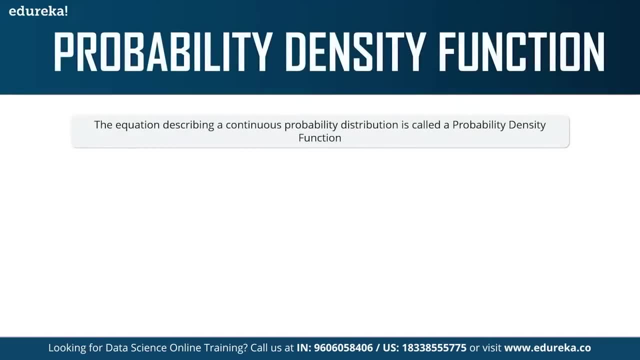 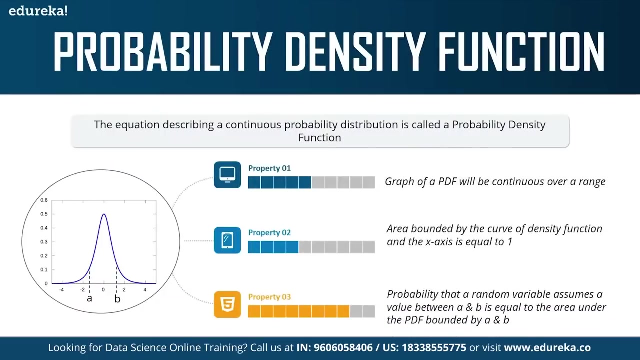 I'll be talking about probability density function, normal distribution and central limit theorem. Okay, Probability density function, also known as PDF, is concerned with the relative likelihood for a continuous random variable to take on a given value. All right, So the PDF gives the probability of a variable that lies between the range A and B. So basically, 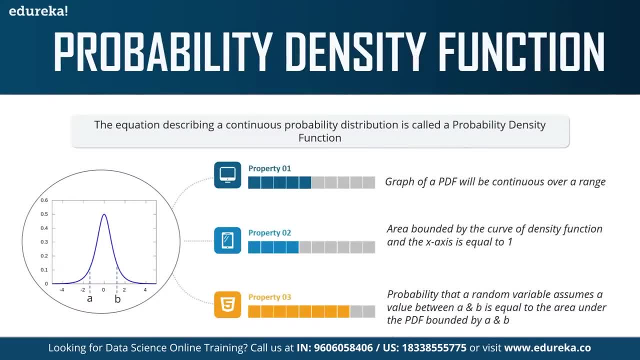 what you're trying to do is you're going to try and find the probability of a continuous random variable over a specified range. Okay, Now this graph denotes the PDF of a continuous variable. Now, this graph is also known as the bell curve. All right, 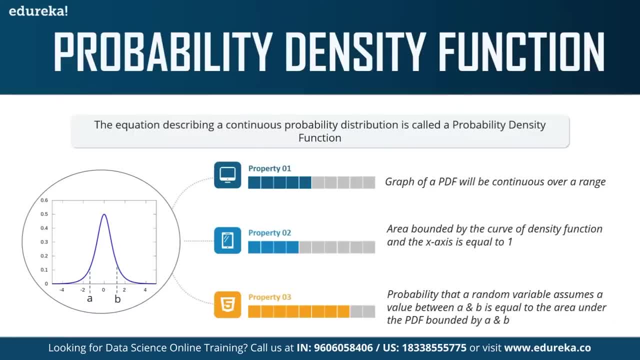 We call the bell curve because of its shape, and there are three important properties that you need to know about: a probability density function. Now the graph of a PDF will be continuous over a range. This is because you're finding the probability that a continuous variable lies between the 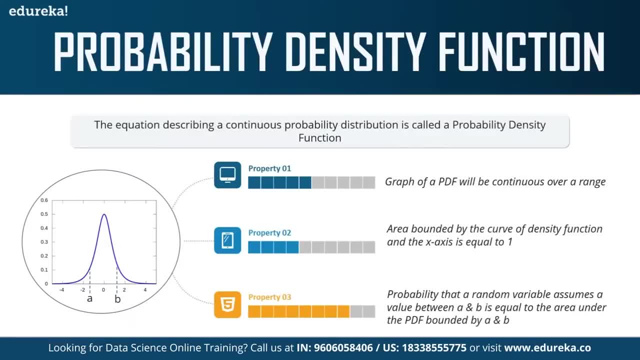 ranges A and B Right. The second property is that the area bounded by the curve of a density function and the X axis is equal to one. Basically, the area below the curve is equal to one. All right, Because it denotes probability. Again, the probability cannot range more than one. 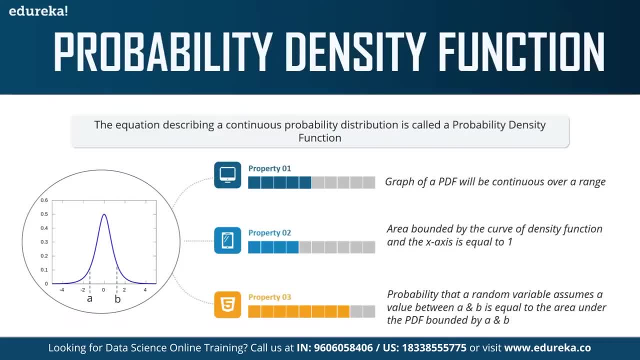 It has to be between zero and one Property. number three is that the probability that a random variable assumes a value between A and B is equal to the area under the PDF bounded by A and B. Okay, Now, what this means is that the probability value is denoted by the area of the graph. 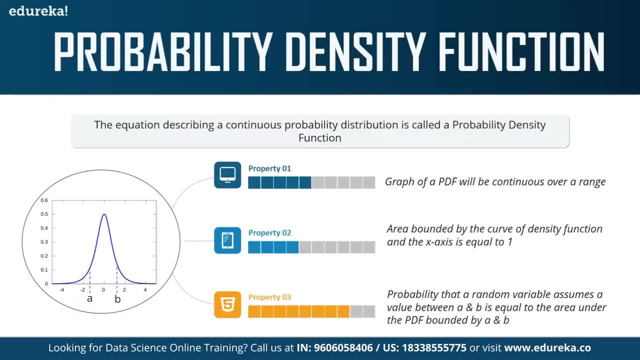 All right. So whatever value that you get here, which is basically one, is the probability that a random variable will lie between the range A and B. All right, So I hope all of you have understood the probability density function. It's basically the probability of finding the value of a continuous random variable. 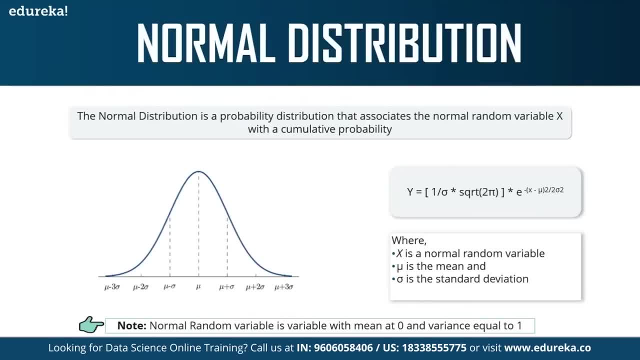 between the range A and B. All right, Now let's look at our next distribution, which is normal distribution. Now, normal distribution, which is also known as the Gaussian distribution, is a probability distribution that denotes the symmetric distribution. It denotes the symmetric property of the mean. 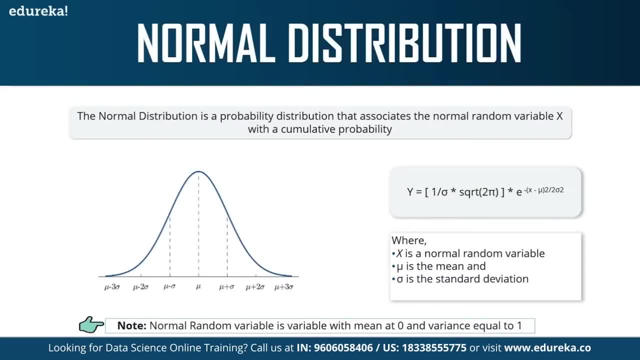 All right, Meaning that the idea behind this function is that the data near the mean occurs more frequently than the data away from the mean. So what it means to say is that the data around the mean represents the entire data set. Okay, So if you just take a sample of data around the mean, it can represent the entire data. 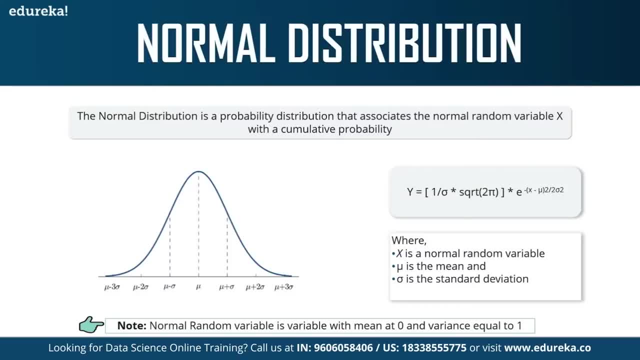 set Now, similar to the probability density function, the normal distribution appears as a bell curve, All right. So when it comes to normal distribution, there are two important factors. All right, We have the mean of the population and the standard deviation. 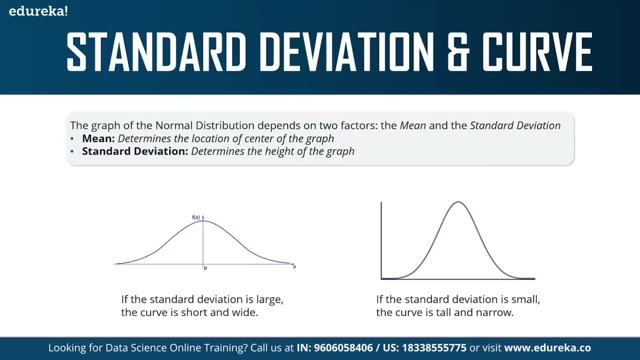 Okay, So the mean and the graph determines the location of the center of the graph, All right. And the standard deviation determines the height of the graph. Okay, So if the standard deviation is large, the curve is going to look something like this: 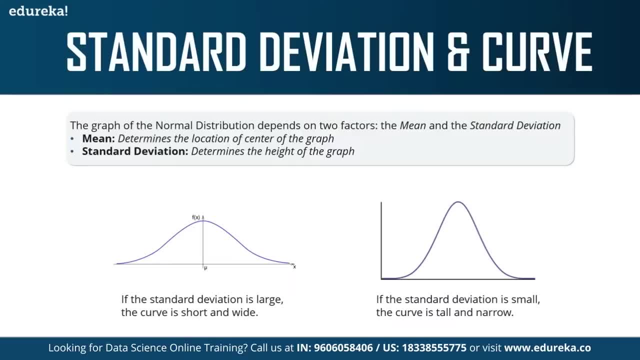 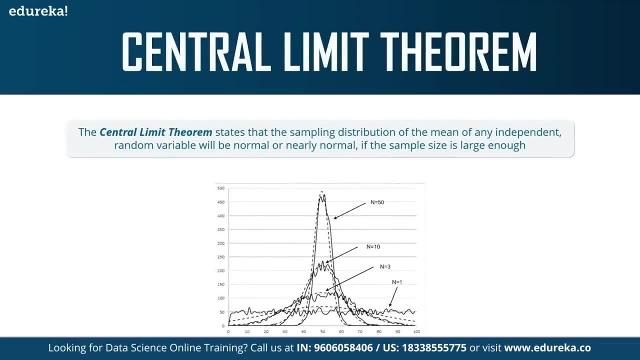 All right, It'll be short and wide, And if the standard deviation is small, the curve is tall and narrow. All right. So this was it about normal distribution. Now let's look at the central limit theory. Now, the central limit theory states that the sampling distribution of the mean of any independent 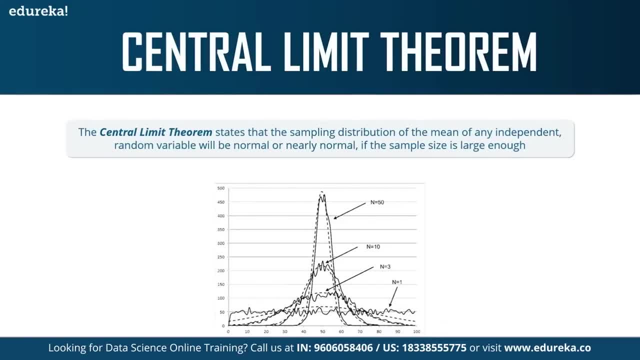 random variable will be normal or nearly normal if the sample size is large enough. Now that's a little confusing. Okay, Let me break it down for you Now in simple terms. if we had a large population and we divided it into many samples, then 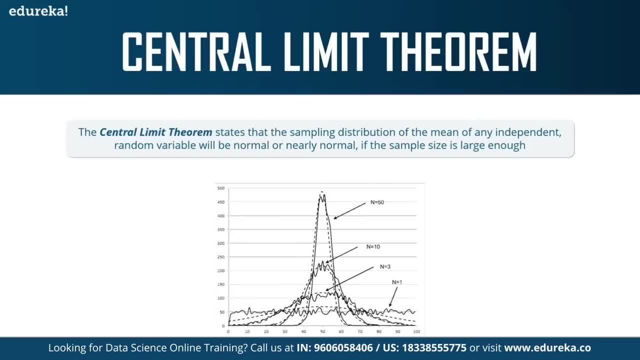 the mean of all the samples from the population Will be almost equal to the mean of the entire population. All right, Meaning that each of the sample is normally distributed Right. So if you compare the mean of each of the sample, it will almost be equal to the mean. 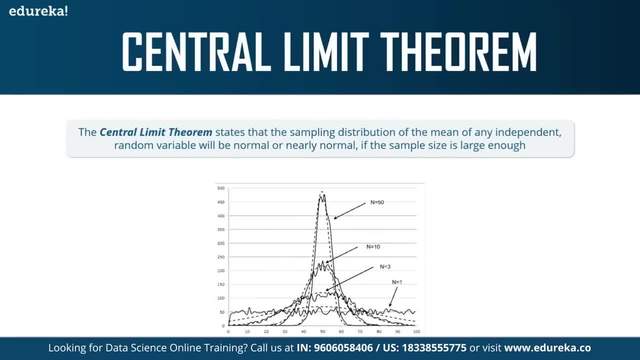 of the population, Right? So this graph basically shows a more clear understanding of the central limit theorem. Right? You can see each sample here, and the mean of each sample is almost along the same line, Right? Okay, So this is exactly what the central limit theorem states. 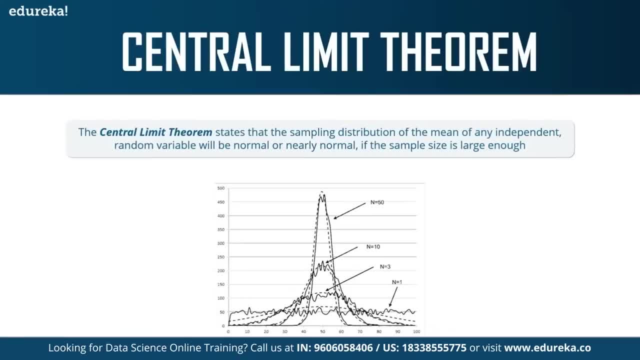 Now, the accuracy or the resemblance to the normal distribution depends on two main factors, Right? So the first is the number of sample points- that you consider All right- And the second is the shape of the underlying population. Now, the shape obviously depends on the standard deviation and the mean of a sample. 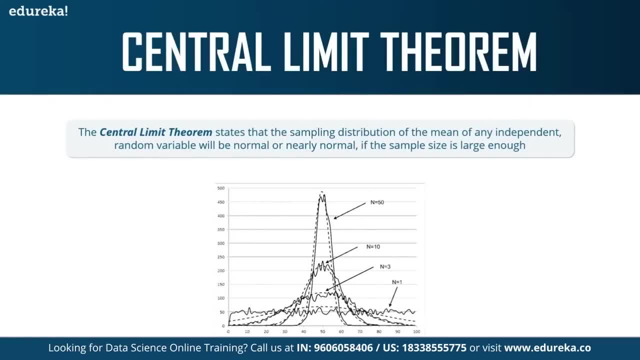 Correct. So, guys, the central limit theorem basically states that each sample will be normally distributed in such a way That the mean of each sample Sample will coincide with the mean of the actual population. All right, In short terms, that's what central limit theorem states. 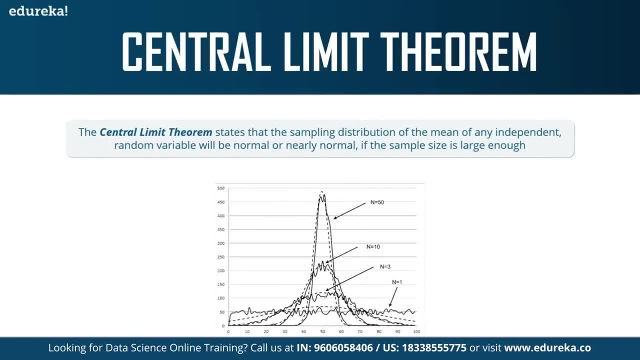 All right, And this holds true only for a large data set. Mostly for a small data set there are more deviations when compared to a large data set. It's because of the scaling factor Right. The smallest deviation in a small data set will change the value very drastically. 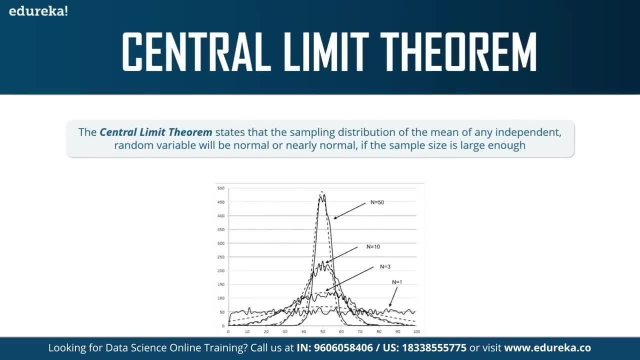 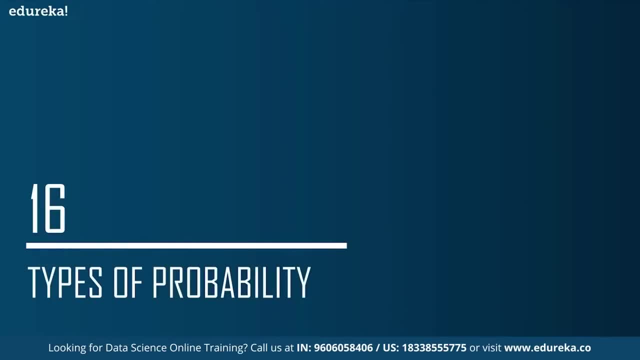 But in a large data set, a small deviation will not matter at all. Now let's move on and look at our next topic, which is the different types of properties. Now, this is an important topic because most of your problems can be solved by understanding. 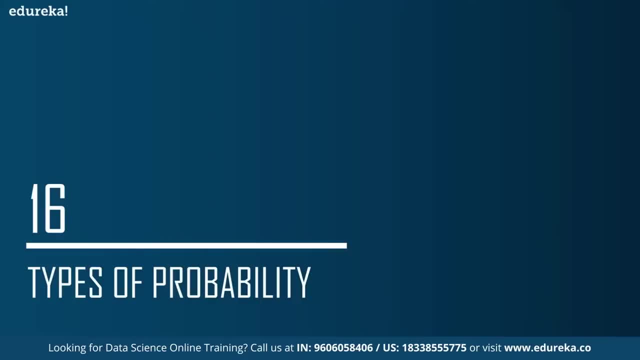 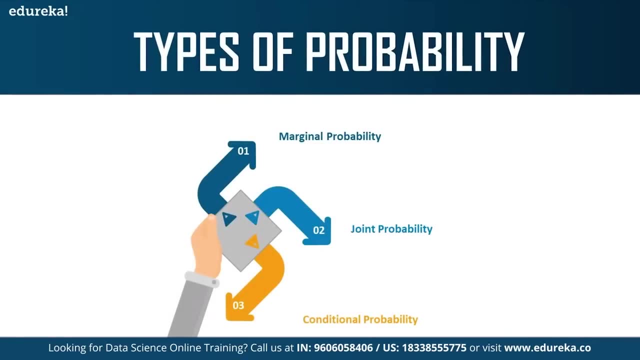 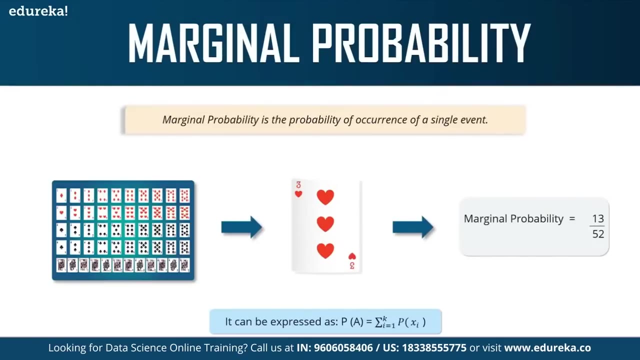 which type of probability should I use to solve this problem? Right, So we have three important types of probability. We have marginal, joint and conditional probability, So let's discuss each of these Now. the probability of an event occurring unconditioned on any other event is known. 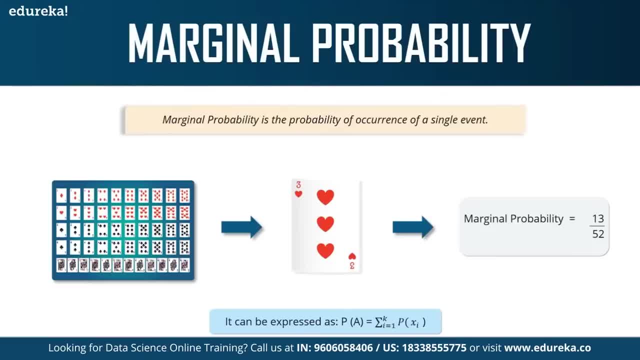 as marginal probability or unconditional probability. So let's say that. So let's say that you want to find the probability that a card drawn is a heart, All right. So if you want to find the probability that a card drawn is a heart, the probability will. 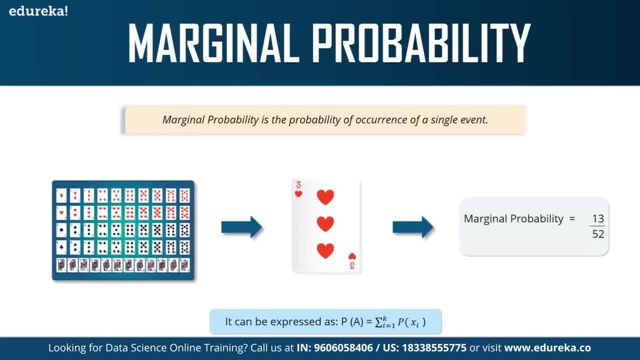 be 13 by 52.. Since there are 52 cards in a deck and there are 13 hearts in a deck of cards, Right, And there are 52 cards in a total deck, So your marginal probability will be 13 by 52.. 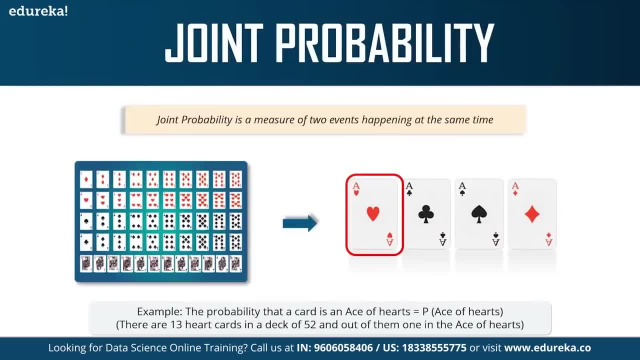 That's about marginal probability. Now let's understand what is joint probability? Now, joint probability is a measure of two events happening at the same time. Okay, Let's say that the two events are A and B, So the probability of event A and B occurring. 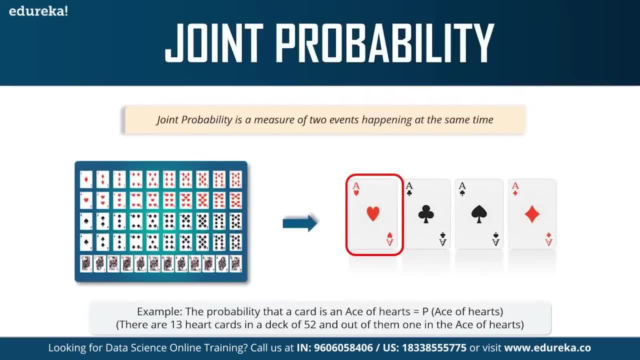 is the intersection of A and B. So, for example, if you want to find the probability that a card is a 4 and a red, that would be joint probability- All right, Because you're finding a card that is 4 and the card has to be red in color. 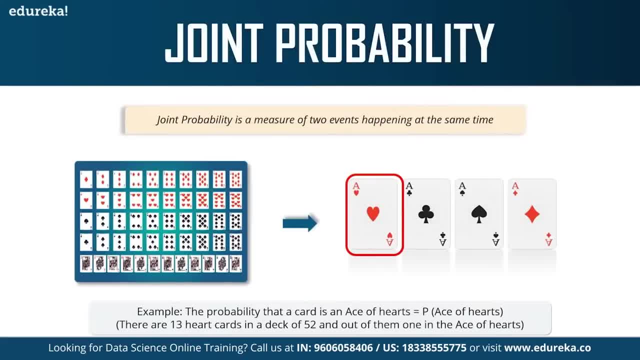 So for the answer, this will be 2 by 52.. Right, Because we have 1, 2 in hearts and we have 1, 2 in diamonds, Correct? So both of these are red in color. Therefore, our probability is 2 by 52.. 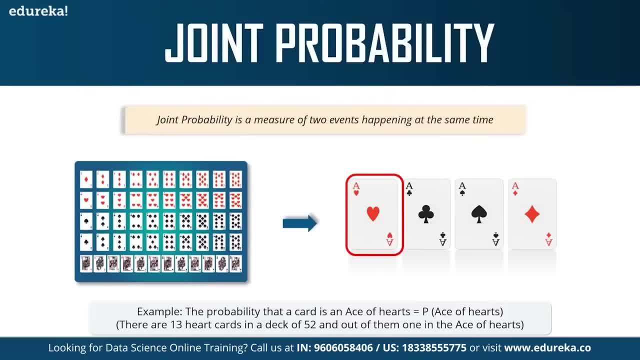 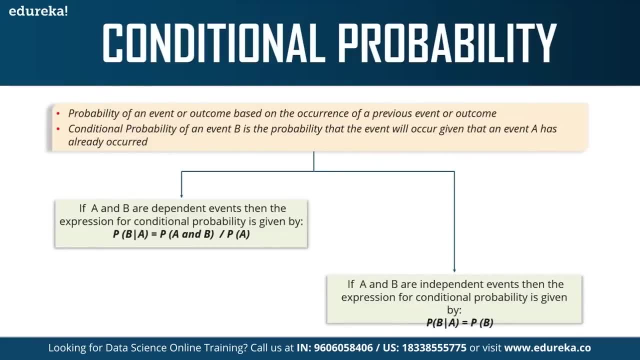 And if you further down it, it is 1 by 26.. Right, So this is what joint probability is all about. Moving on, let's look at what exactly conditional probability is. So if the probability of an event or an outcome is based on the occurrence of a previous event, 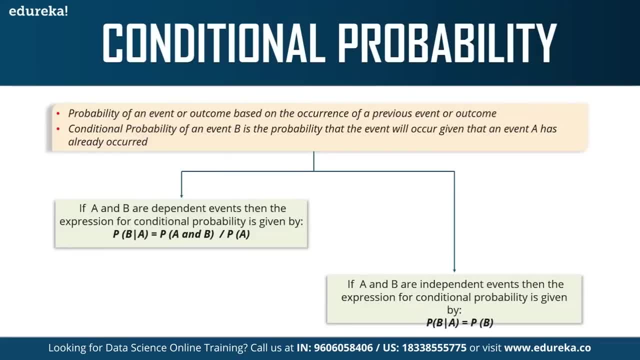 or an outcome. Then you called it as a conditional probability. Okay, So the conditional probability of an event B is the probability that the event will occur, given that an event A has already occurred. Right? So if A and B are dependent events, then the expression for conditional probability 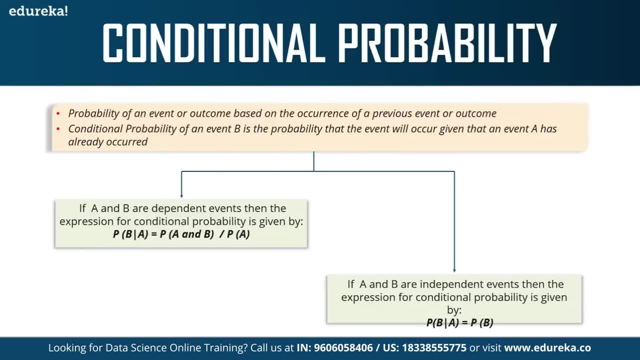 is given by this. Now, this first term on the left hand side, which is P, B of A is basically the probability of event B occurring, given that event A has already occurred. All right, So, like I said, if A and B are dependent events, then this is the expression. 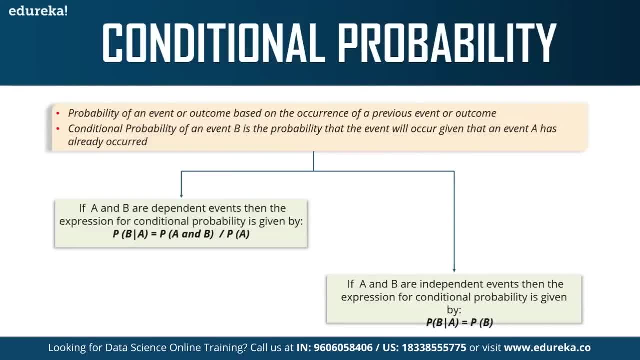 But if A and B are independent events, then the expression for conditional probability is like this: Right, So, guys, P of A and P of B is obviously the probability of A and probability of B. Right Now, let's move on. 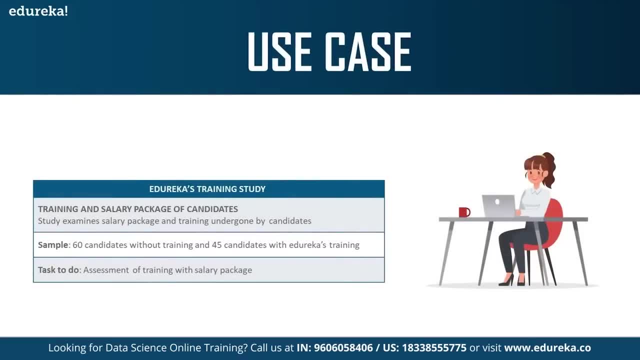 Now, in order to understand conditional probability, joint probability and marginal probability, let's look at a small use case. Okay, Now, basically, we're going to take a data set which examines the salary package and training undergone by candidates. Okay, 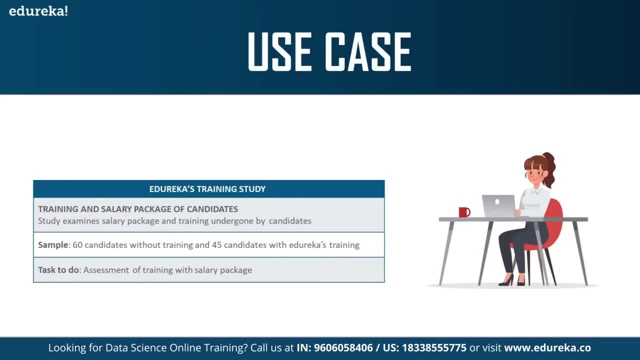 Now in this there are 60 candidates without training and 45 candidates which have enrolled for Edureka's training Right Now. the task here is you have to assess the training with a salary package. Okay, Let's look at this in a little more depth. 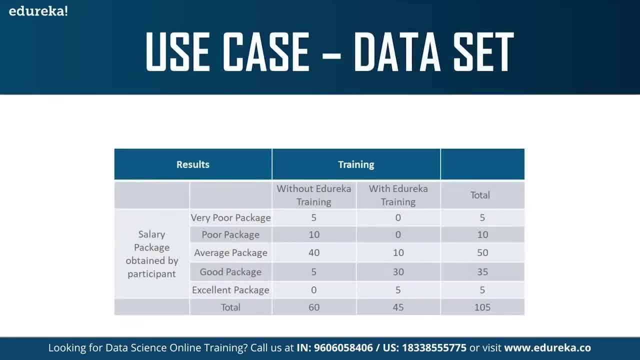 So in total, we have 105 candidates, out of which 60 of them have not enrolled for Edureka's training. All right, This is a small survey that was conducted and this is the rating of the package or the salary that they got. 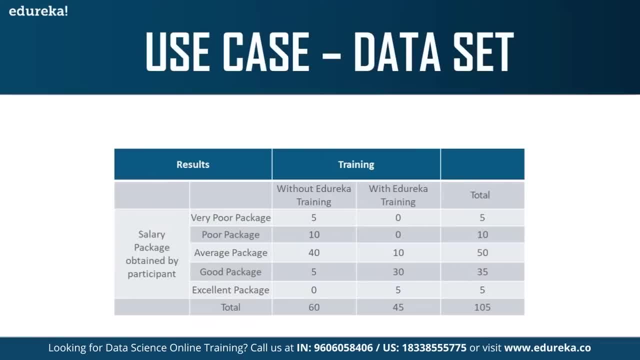 Right. So if you read through the data, you can understand. There were five candidates without Edureka training who got a very poor salary package- Okay. Similarly, there are 30 candidates with Edureka training who got a good package Right. 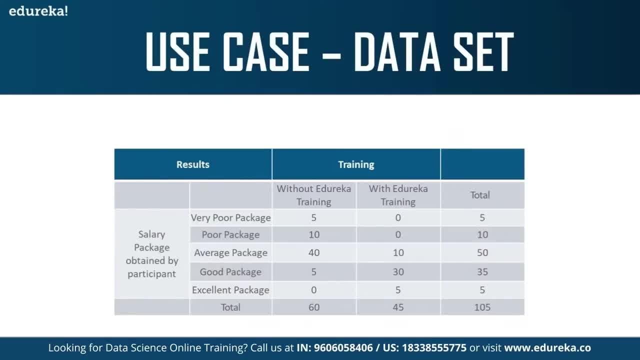 So, guys, basically you're comparing the salary package of a person depending on the salary package. So you're comparing the salary package of a person depending on whether or not they've enrolled for Edureka training Right, This is our data set. 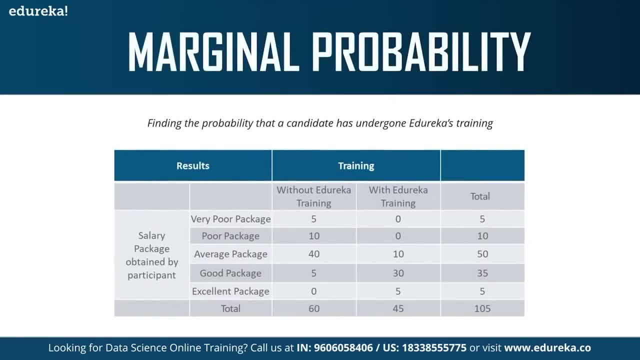 Now let's look at our problem statement. Find the probability that a candidate has undergone Edureka's training Quite simple. Which type of probability is this? This is marginal probability, Right? So the probability that a candidate has undergone Edureka's training is obviously 45 divided. 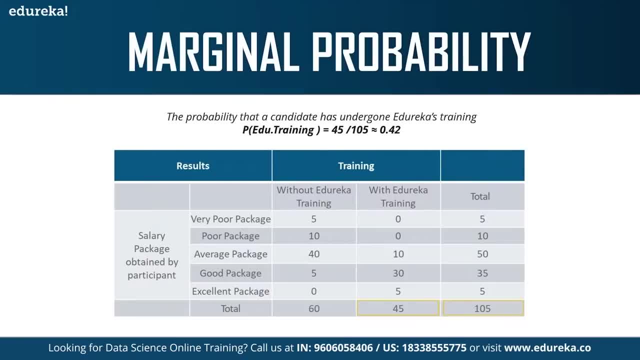 by 105.. Since 45 is the number of candidates with Edureka training and 105 is the number of candidates with Edureka training And 105 is the total number of candidates, So you get a value of approximately 0.42. 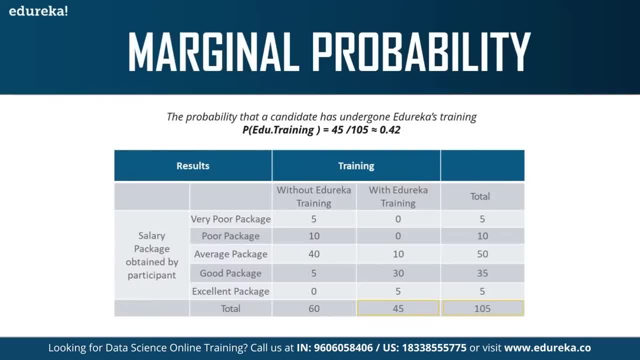 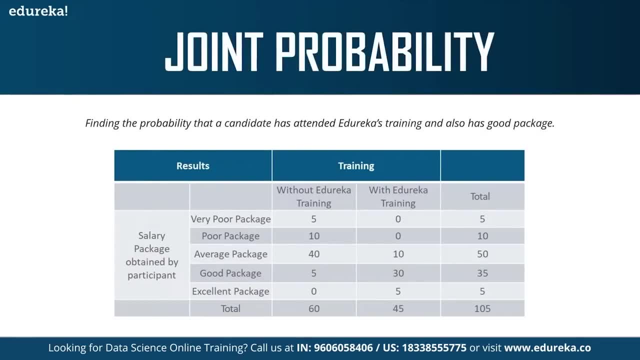 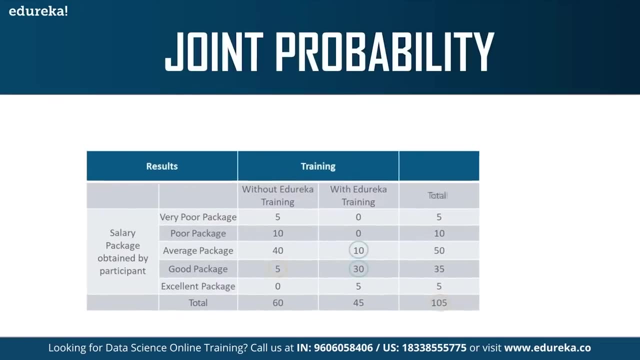 Alright, That's the probability of a candidate that has undergone Edureka's training. Next question: Find the probability that a candidate has attended Edureka's training and also has good package. Now, this is obviously a joint probability problem, Right? So how do you calculate this? 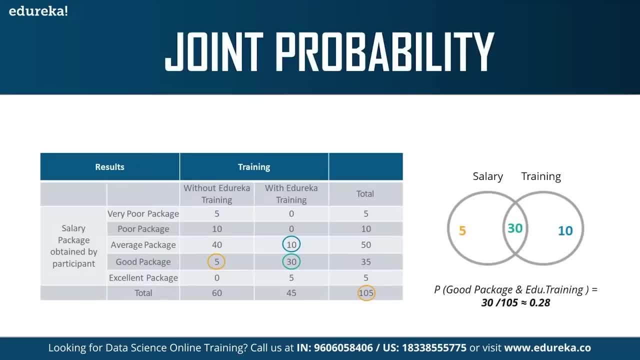 Now, since our table is quite formatted, we can directly find that people who have gotten a good package along with Edureka training are 30. Right, So out of 105 people, 30 people have Edureka training and a good package. 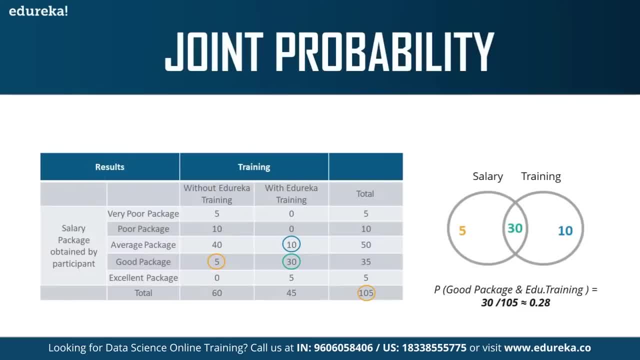 Right. They are specifically asking for people with Edureka training. Remember that Right. The question is: find the probability that a candidate has attended Edureka's training and also has a good package? Alright, So you need to consider two factors. 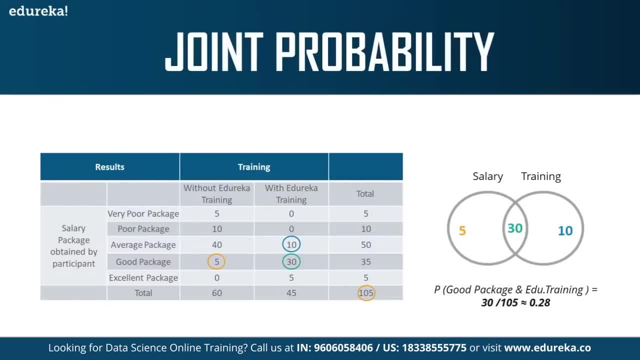 That is a candidate who has attended Edureka's training and who has a good package. So clearly, that number is 30.. 30 divided by total number of candidates, which is 105.. Right, So here you get the answer clearly. 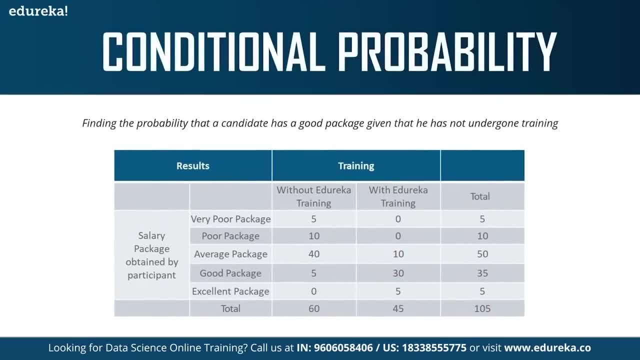 Next, we have find the probability that a candidate has good package given that he has not undergone training. Okay, Now, this is clearly conditional probability, because here you are defining a condition, You are saying that you want to find the probability of a candidate who has a good package given. 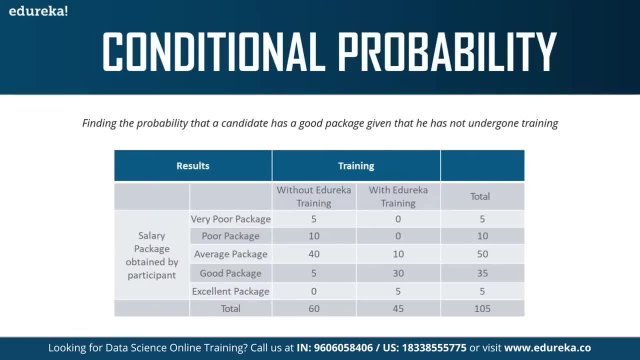 that he has not undergone any training. Right, The condition is that he has not undergone any training, Alright. So the number of people who have not undergone training are 60, and out of that, 5 of them have got a good package. 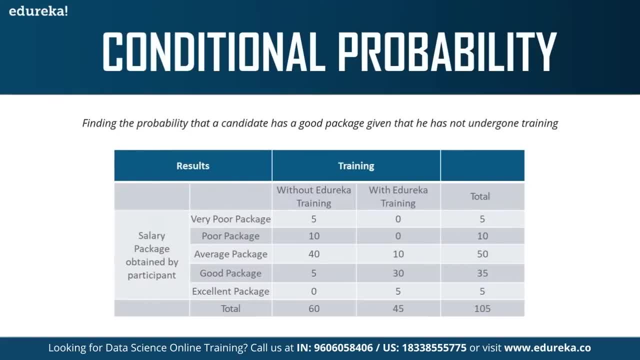 Right. So that's why this is 5 by 60 and not 5 by 105, because here they have clearly mentioned has a good package, given that he has not undergone training. So you have to only consider people who have not undergone training. 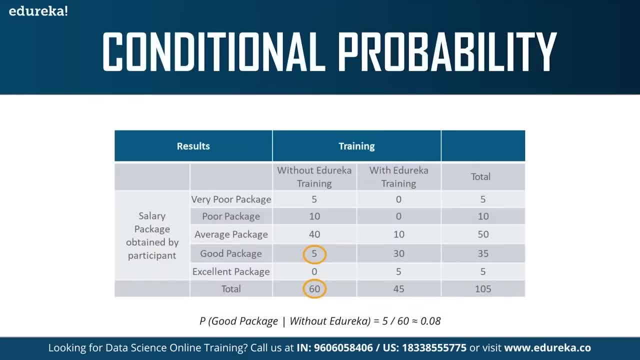 Right. So only 5 people who have not undergone training. Right, They have gotten a good package Right. So 5 divided by 60, you get a probability of around 0.08, which is pretty low, Right. 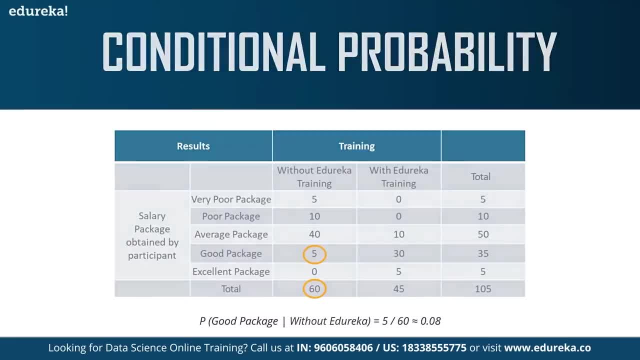 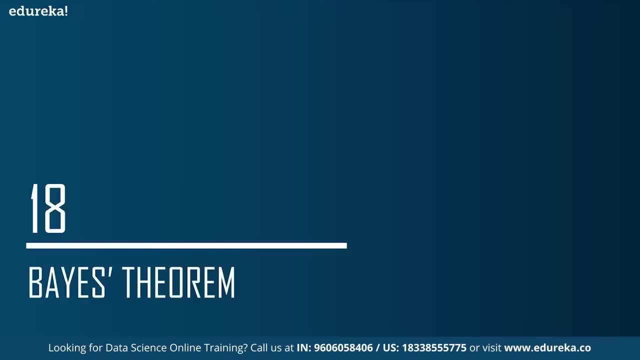 Okay, So this was all about the different types of probability. Now let's move on and look at our last topic in probability, which is Bayes theorem. Now, guys, Bayes theorem is a very important concept when it comes to statistics and probability. 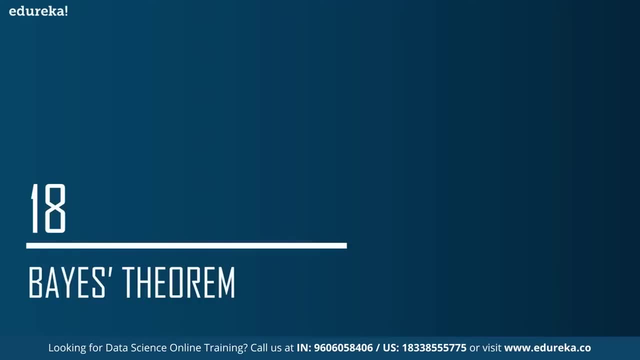 It is majorly used in naive bias algorithm. those of you who aren't aware, Naive bias is a supervised learning classification algorithm and it is mainly used in Gmail spam filtering Right. A lot of you might have noticed that if you open up Gmail, you'll see that you have a 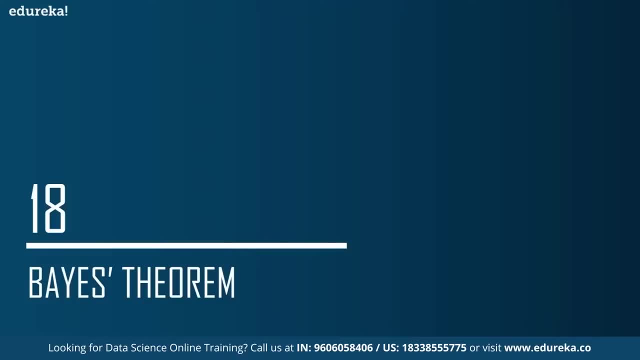 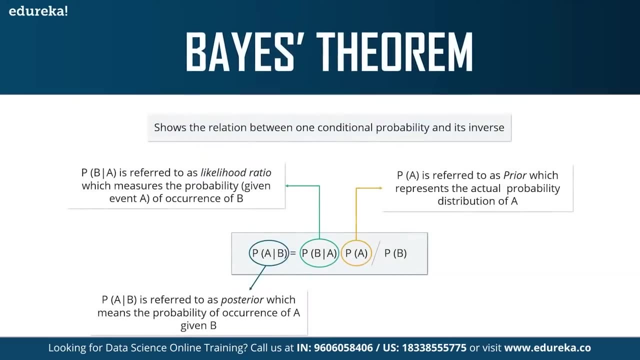 folder called spam Right. All of that is carried out through machine learning and the algorithm used. there is naive bias Right. So now let's discuss what exactly the Bayes theorem is and what it denotes. So the Bayes theorem is used to show the relation between one conditional probability. 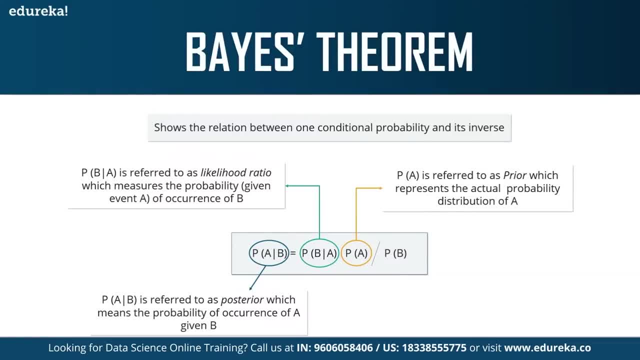 and its inverse. All right, Basically, it's nothing but the probability of an event occurring, based on prior knowledge of conditions that might be related to the same event. Okay, So mathematically, the Bayes theorem is represented like this: 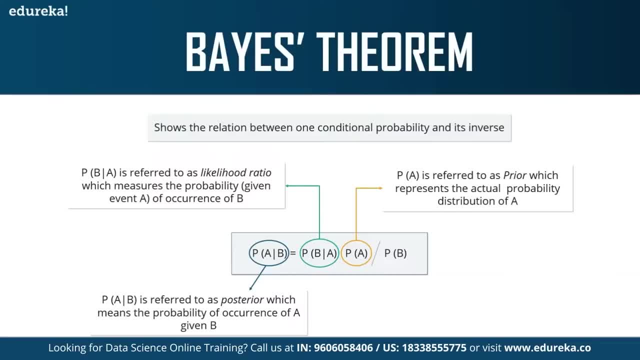 Right, Like shown in this equation. The left-hand term is referred to as the likelihood ratio, which measures the probability of occurrence of event B Okay Given an event A Okay. On the left-hand side is what is known as the posterior. 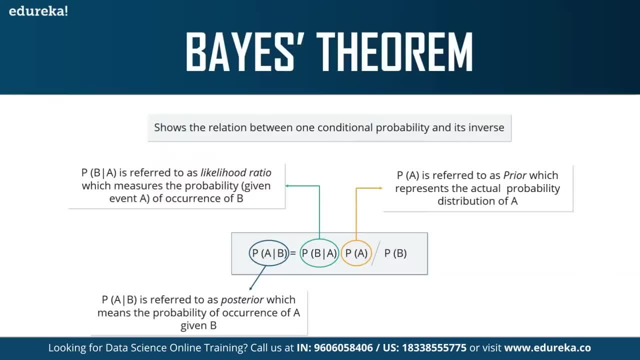 All right, It is referred to as posterior, which means that the probability of occurrence of A given an event B Right. The second term is referred to as the likelihood ratio. All right, This measures the probability of occurrence of B given an event A. Now P is also. 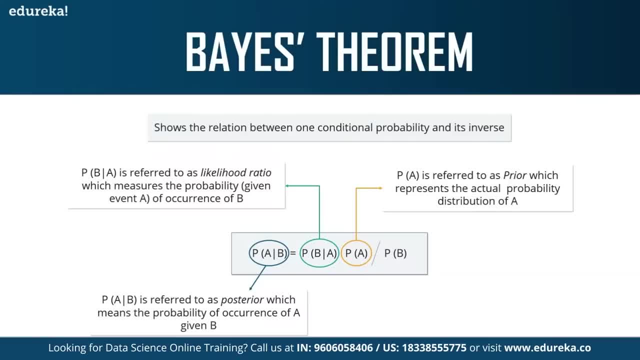 known as the prior, which refers to the actual probability. distribution of A and P is again the probability of B. Okay, All right, This is the Bayes theorem. Now, in order to better understand the Bayes theorem, let's look at a small example. 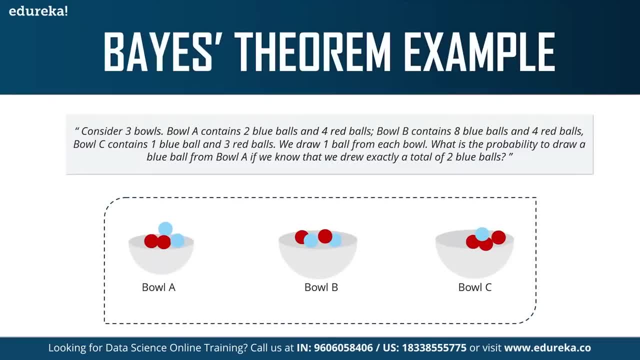 Let's say that we have three bowels. We have bowel A, bowel B and bowel C. Okay, Bowel A contains two blue balls and four red balls. Bowel B contains eight blue balls and four red balls. Bowel C contains one blue ball and three red balls. 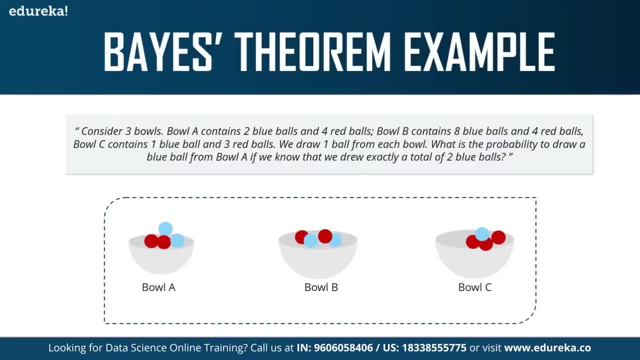 Now, if we draw one ball from each bowel, what is the probability to draw a blue ball? If we draw a blue ball from a bowel A, if we know that we drew exactly a total of two blue balls, Right? If you didn't understand the question, please reread it. 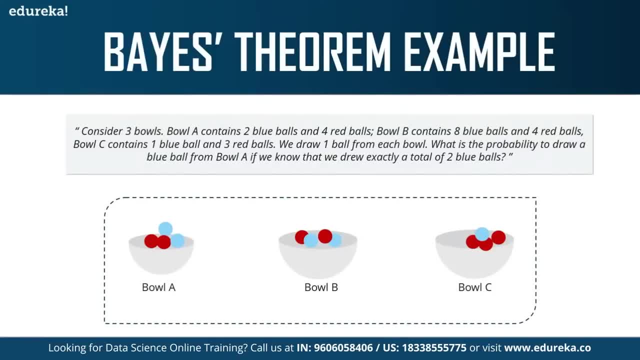 I shall pause for a second or two, Right? So I hope all of you have understood the question. Okay, Now what I'm going to do is I'm going to draw a blueprint for you and tell you how exactly to solve the problem. 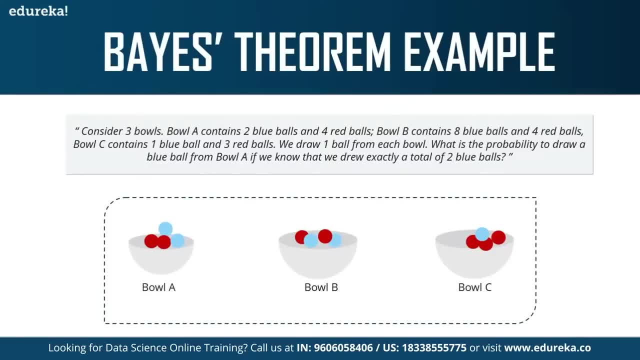 But I want you all to give me the solution to this problem. Right, I'll draw a blueprint, I'll tell you what exactly the steps are, but I want you to come up with a solution on your own Right. The formula is also given to you. 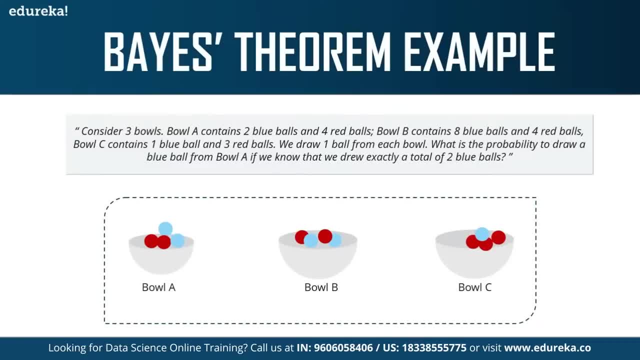 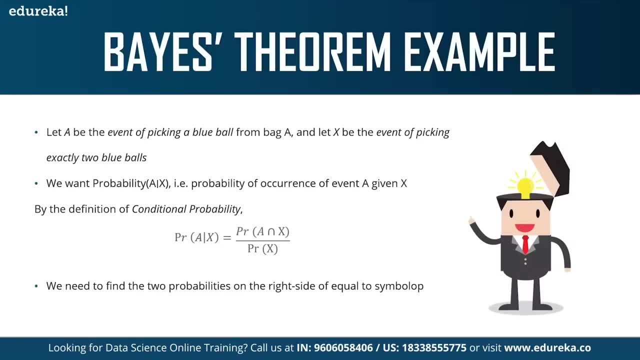 Everything is given to you. All you have to do is come up with a final answer. Right, Let's look at how you can solve this problem. So, first of all, what we'll do is: let's consider A. All right, Let A be the event of picking a blue ball from bag A, And let X be the event of picking. 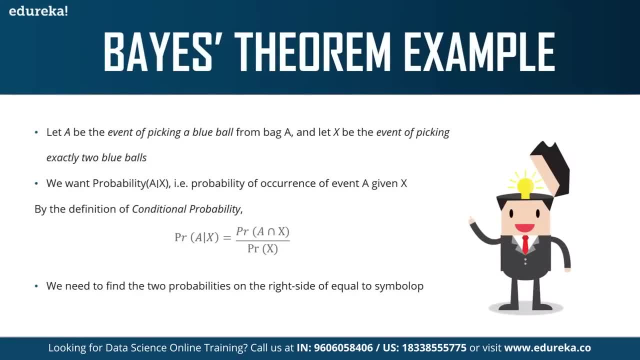 exactly two blue balls. Right, Because these are the two events that we need to calculate the probability of. Now. there are two probabilities that you need to consider here. One is the event of picking a blue ball from bag A and the other is the event of picking 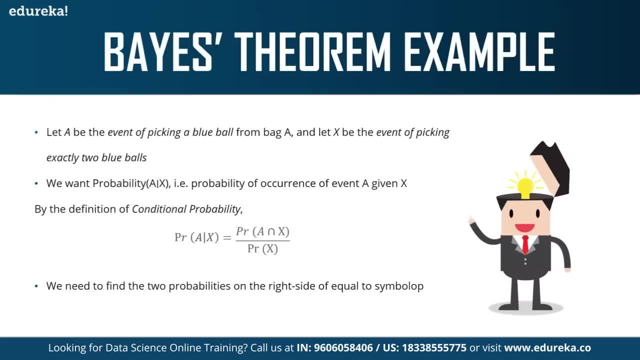 exactly two blue balls. Okay, So these two are represented by A and X respectively. So what we want is the probability of occurrence of event A given X, which means that, given that we're picking exactly two blue balls, what is the probability that we are picking? 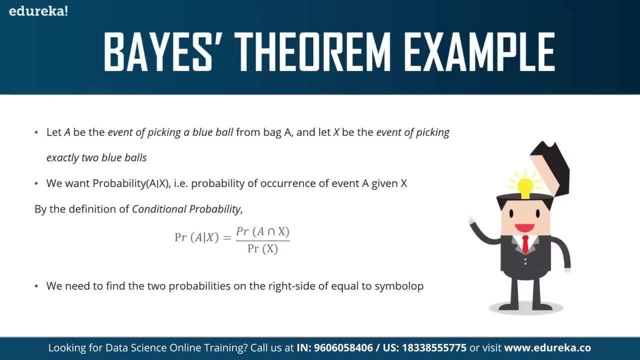 a blue ball from bag A. So, by the definition of conditional probability, this is exactly what our equation will look like, Correct. This is basically occurrence of event A given an event X, And this is the probability of A and X, And this is the probability of X alone. 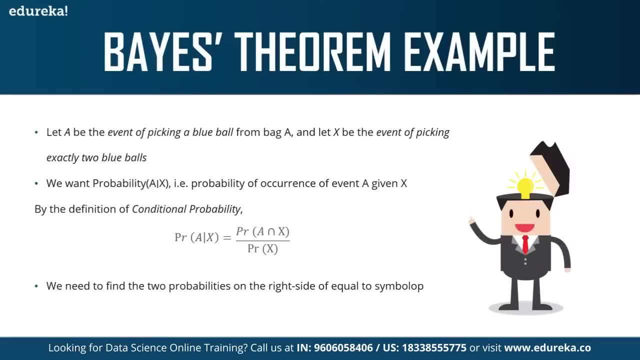 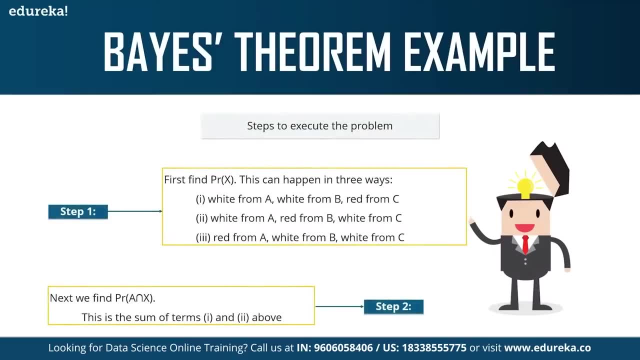 Correct. Now what we need to do is we need to find these two probabilities, which is probability of A and X occurring together and probability of X. Okay, This is the entire solution. So how do you find the probability of X? Okay, 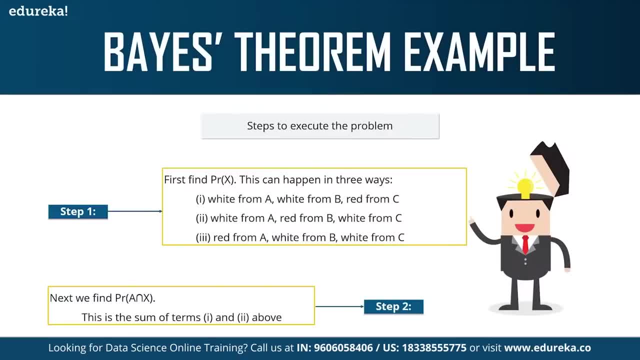 This you can do in three ways. So first is white ball from A, either white from B or red from C. Now, first is to find the probability of X. X basically represents the event of picking exactly two blue balls, Right? So these are the three ways in which it is possible. 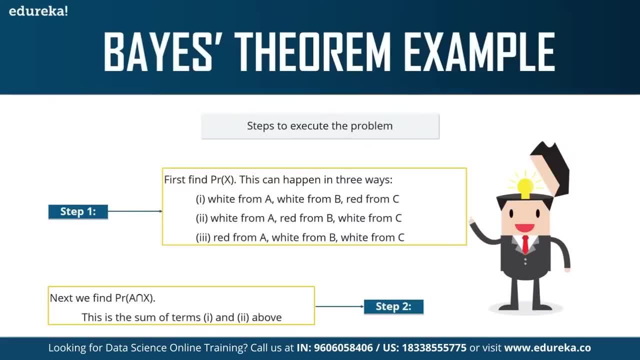 So you'll pick one blue ball from bowl A and one from bowl B. In the second case, you can pick one from A and another blue ball from C. In the third case, you can pick one from B. In the fourth case, you can pick a blue ball from bag B and a blue ball from bag C, Right. 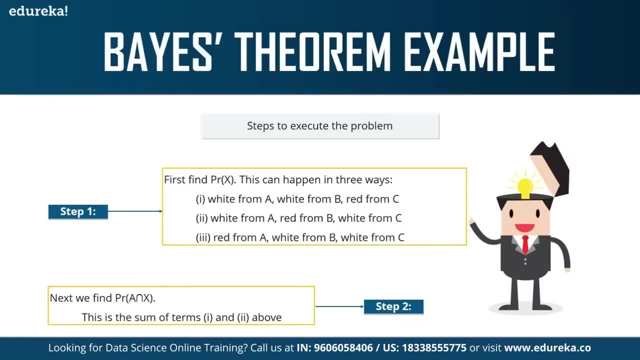 These are the three ways in which it is possible, So you need to find the probability of each of this. Step two is that you need to find the probability of A and X occurring together. This is the sum of terms one and two. Okay, 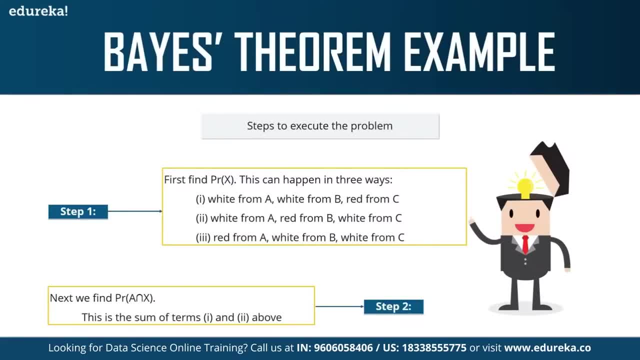 This is because in both of these events, you're picking a ball from bag A, Correct? So, guys, find out this probability and let me know your answer in the comment section. All right, So bag C. if you get the answer right, I gave you the entire solution to this. 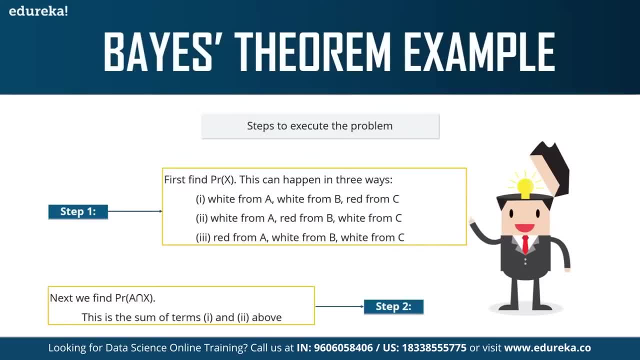 All you have to do is substitute the value, right? If you want a second or two, I'm going to pause on the screen so that you can go through this in a more clear way, right? Remember that you need to calculate two probabilities. 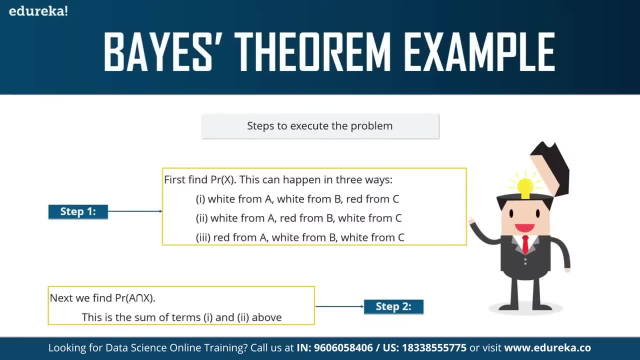 The first probability that you need to calculate is the event of picking a blue ball from bag A. given that you're picking exactly two blue balls, Okay, The second probability you need to calculate, It is the event of picking exactly two blue balls. 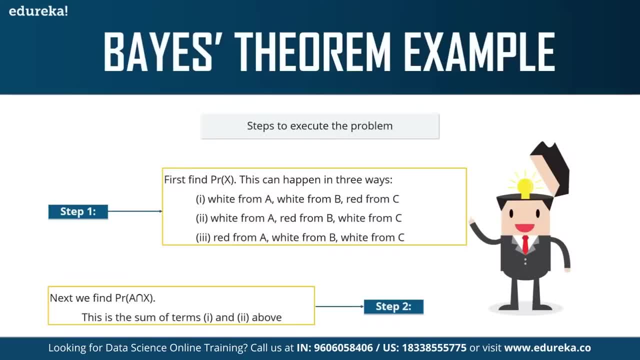 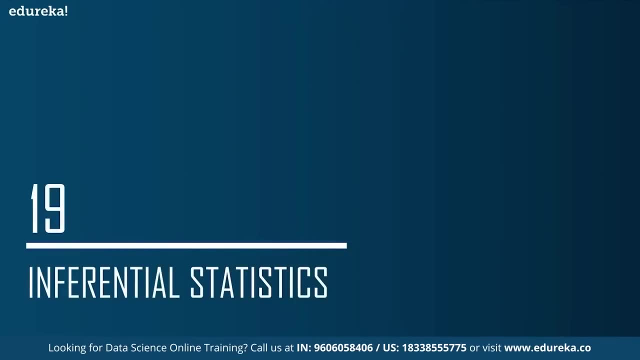 All right, These are the two probabilities you need to calculate. So remember that, And this is the solution, All right. So, guys, make sure you mention your answers in the comment section. For now, let's move on and look at our next topic, which is the inferential statistics. 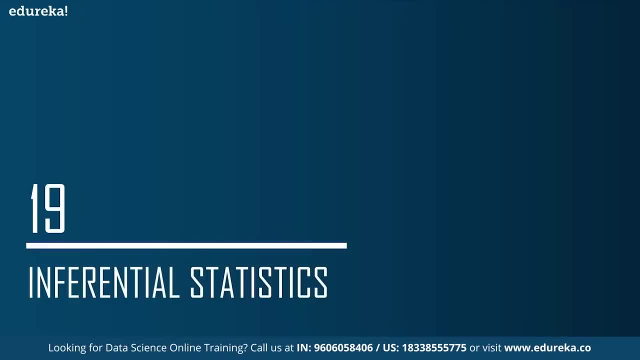 So, guys, we just completed the probability module. right Now we'll discuss inferential statistics, which is the second type of statistics. We discussed descriptive statistics earlier. all right, So, like I mentioned earlier, inferential statistics, also known as statistical inference, is a 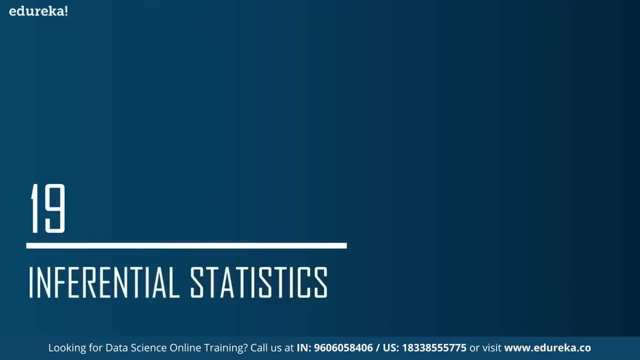 branch of statistics that deals with forming inferences and predictions about a population based on a sample of data taken from the population. All right, And the question you should ask is: how does one form inferences or predictions on a sample? The answer is: you use point estimation. 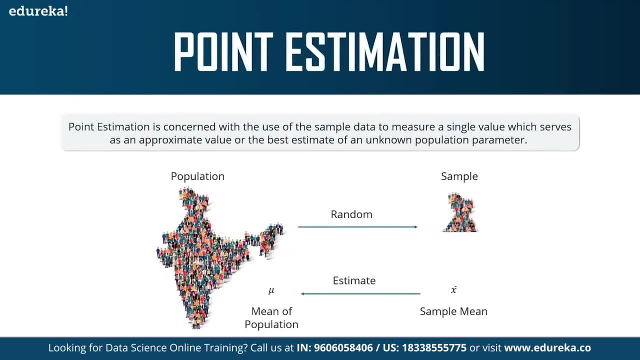 Okay. So you might be wondering what is point estimation? Point estimation is concerned with the use of the sample data to measure a single value which serves as an approximate value or the best estimate of an unknown population parameter. That's a little confusing. 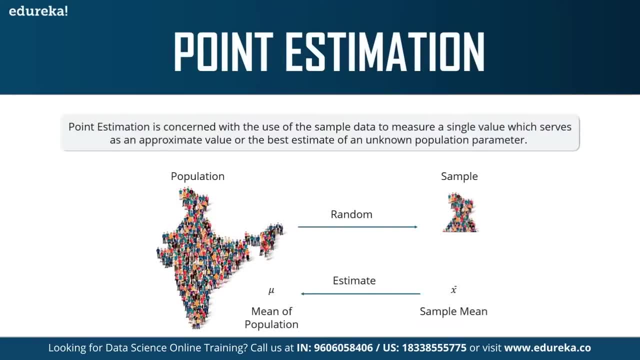 Let me break it down to you. For example, in order to calculate the mean of a huge population, what we do is we first draw out the sample of the population and then we find the sample mean right. The sample mean is then used to estimate. 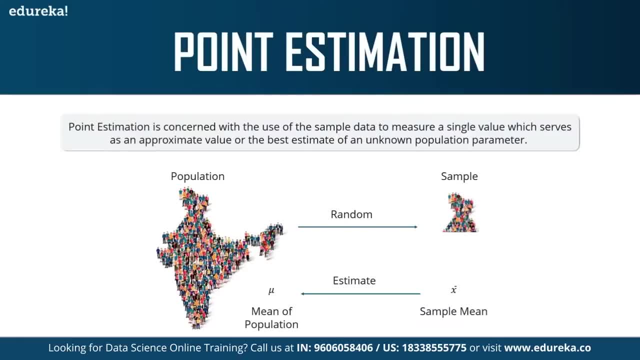 Okay. The sample mean is then used to estimate the population mean. This is basically point estimate. You're estimating the value of one of the parameters of the population, right, Basically the mean. you're trying to estimate the value of the mean. 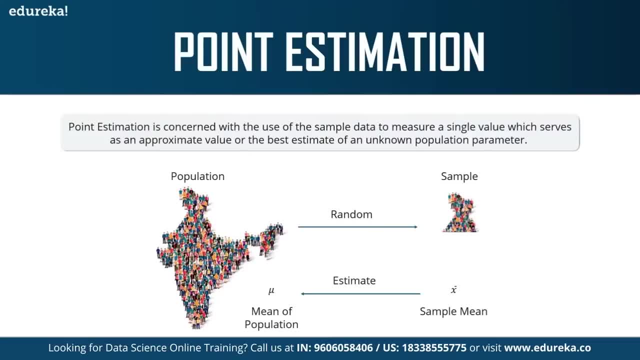 This is what point. estimation is The two main terms in point. estimation, there's something known as the estimator and there's something known as the estimate. Estimator is a function of the sample that is used to find out the estimate. all right, 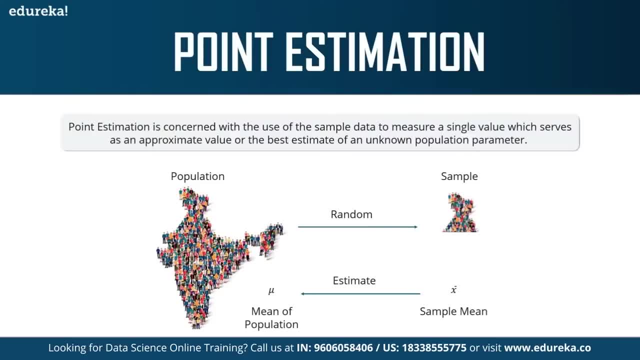 In this example it's basically the sample mean, Right. So a function that calculates the sample mean is known as the estimator, and the realized value of the estimator is the estimate Right. So I hope point estimation is clear. Now, how do you find the estimates? 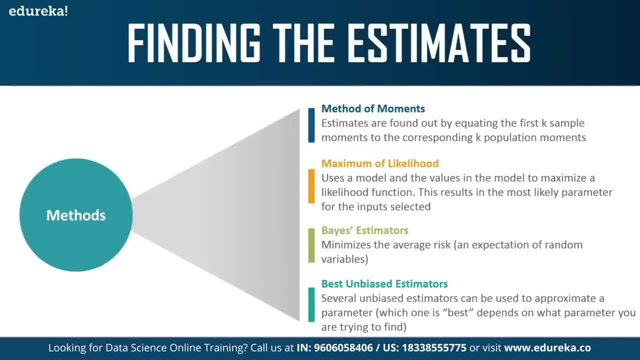 There are four common ways in which you can do this. The first one is method of moments. Here what you do is you form an equation in the sample data set and then you analyze a similar equation in the population data set as well. 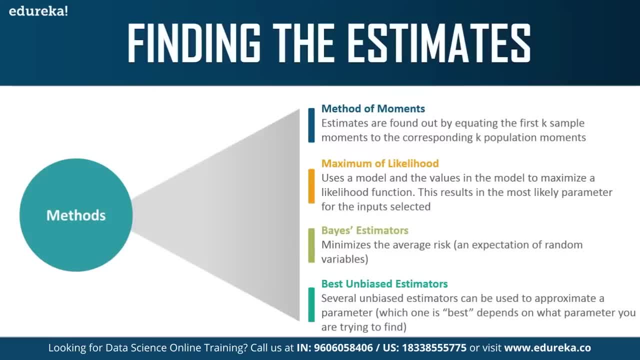 Like the population, mean population mean Okay. Like the population variance, and so on. So, in simple terms, what you're doing is you're taking down some known facts about the population and you're extending those ideas to the sample. 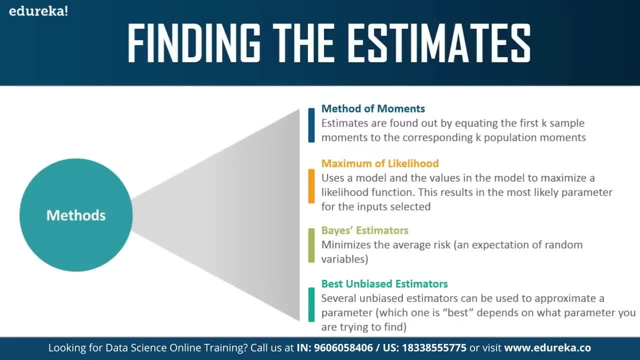 All right. Once you do that, you can analyze the sample and estimate more essential or more complex values Right. Next, we have maximum of likelihood. Now, this method basically uses a model to estimate a value. All right Now. maximum of likelihood is majorly based on probability, so there's a lot of probability. 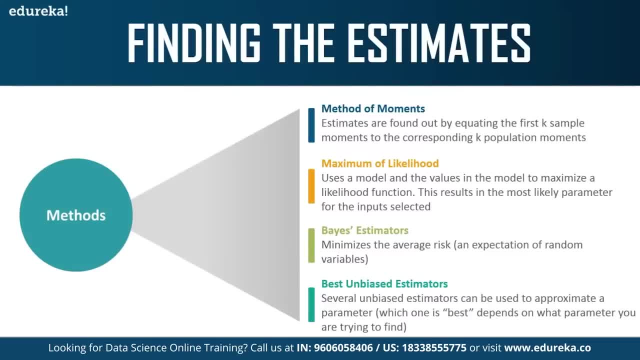 involved in it In this method. Next, we have the base estimator. This works by minimizing the errors or the average risk. Okay, The base estimator has a lot to do with the bias theorem. All right, Let's not get into the depth of these estimation methods. 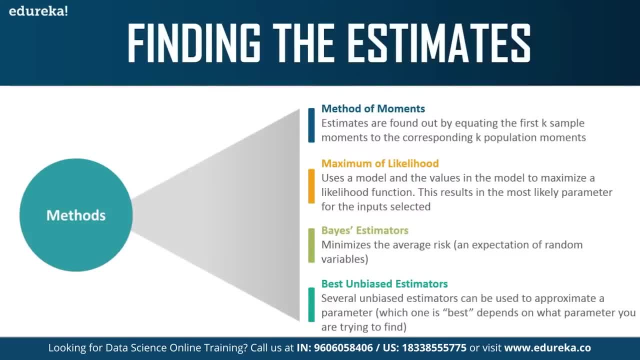 Finally, we have the best unbiased estimators. In this method. there are several unbiased estimators that can be used to approximate a parameter. Okay, So, guys, these were a couple of methods that are used to find the estimate, But the most well-known method to find the estimate is known as the interval estimation. 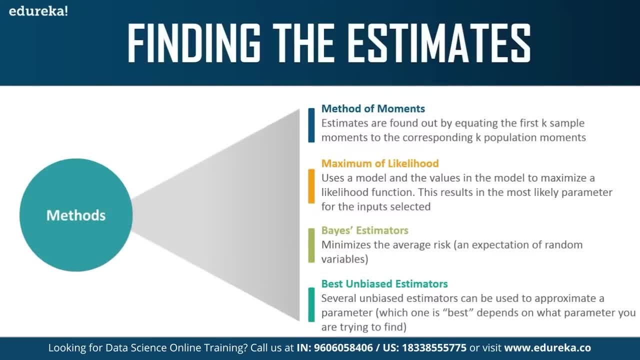 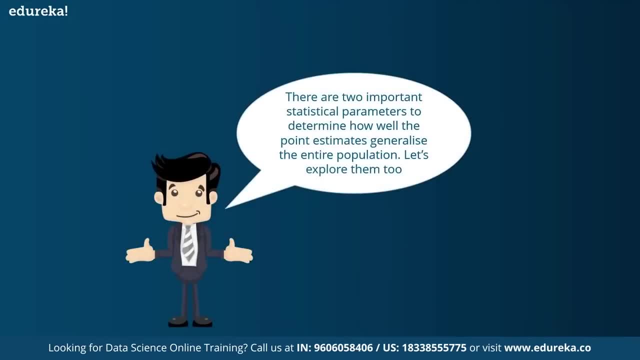 Okay, This is one of the most important estimation methods. All right, This is where confidence interval also comes into the picture. Right Apart from interval estimation, we also have something known as margin of error, So I'll be discussing all of this in the upcoming slides. 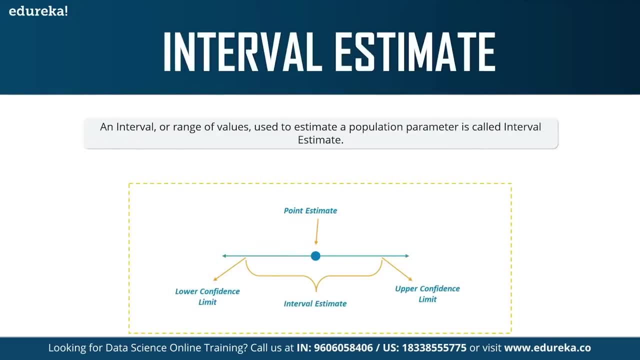 So first let's understand what is interval estimate. Okay, An interval or range of values which are used to estimate a population parameter is known as an interval estimation. All right, That's very understandable. Basically, what they're trying to say is: you're going to estimate the value of a parameter. 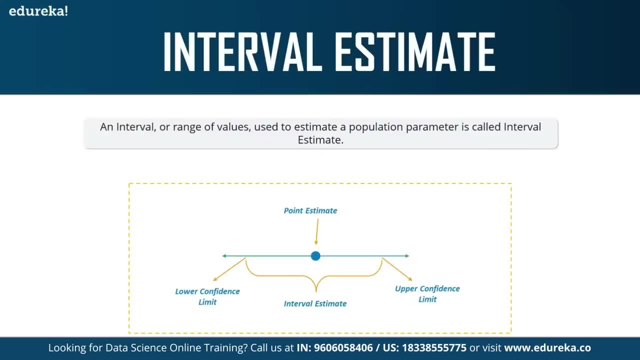 Let's say you're trying to find the mean of a population. What you're going to do is you're going to build a range and your value will lie in that range or in that interval. All right, So this way your output is going to be more accurate, because you've not predicted a point. 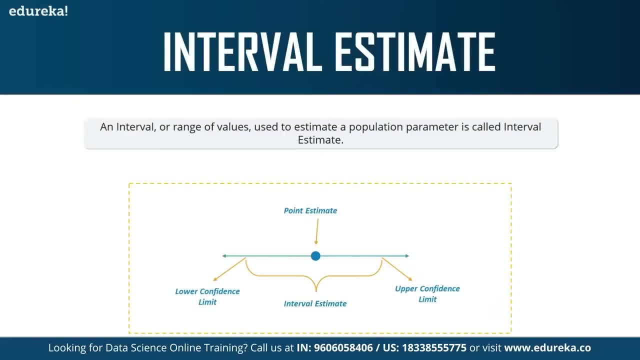 estimation. Instead, you have estimated an interval within which your value will lie Right. Okay, Now this image clearly shows how point estimate and interval estimate are different. So, guys, interval estimate is obviously more accurate because you're not just focusing. 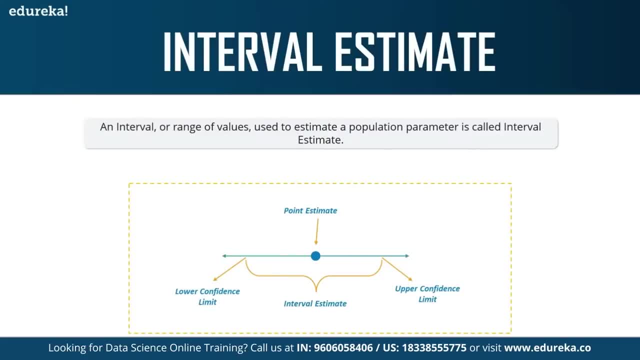 on a particular value or a particular point in order to predict the probability. Instead, you're saying that the value might be within this range between the lower confidence limit and the upper confidence limit. All right, This just denotes the range or the interval. 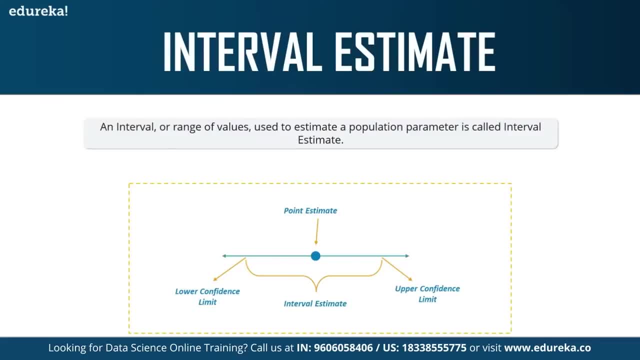 Okay. If you're still confused about interval estimation, let me give you a small example. If I stated that I will take 30 minutes to reach the theater, this is known as point estimation- Okay. But if I stated that I will take between 45 minutes to an hour to reach the theater, this 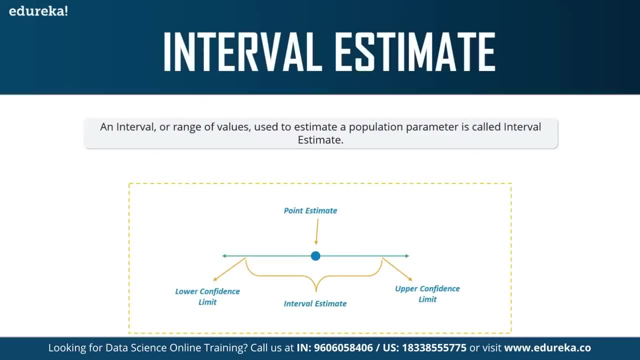 is an example of interval estimation. All right, I hope it's clear now. Now, interval estimation gives rise to two important statistical terminologies. One is known as confidence interval And the other is known as margin of error. All right, So, guys, it's important that you pay attention to both of these terminologies. 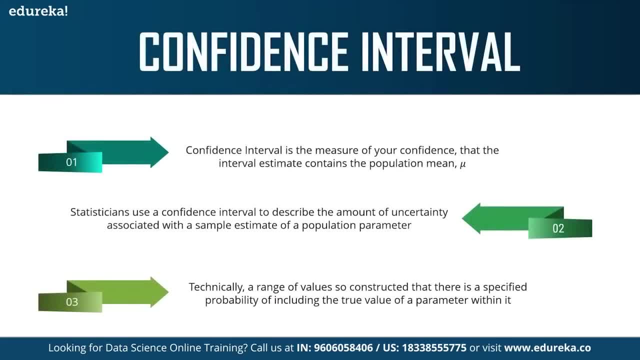 Confidence interval is one of the most significant measures that are used to check how essential a machine learning model is. All right. So what is confidence interval? Confidence interval is the measure of your confidence that the interval estimated contains the population parameter or the population mean or any of those parameters. 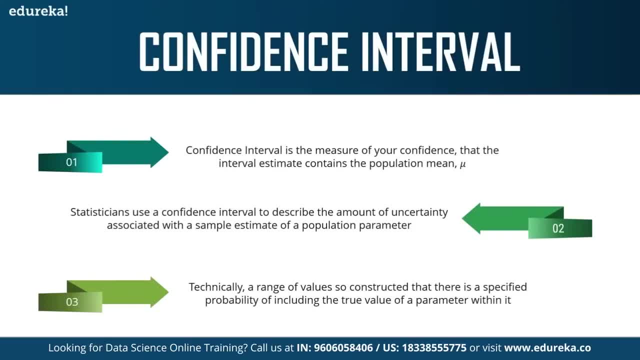 Right Now, statisticians use confidence interval to describe the amount of uncertainty associated with a sample estimate of a population parameter. Now, guys, this is a lot of definition. Let me just make you understand confidence interval with a small example. Okay, let's say that you perform a survey and you survey a group of cat owners to see. 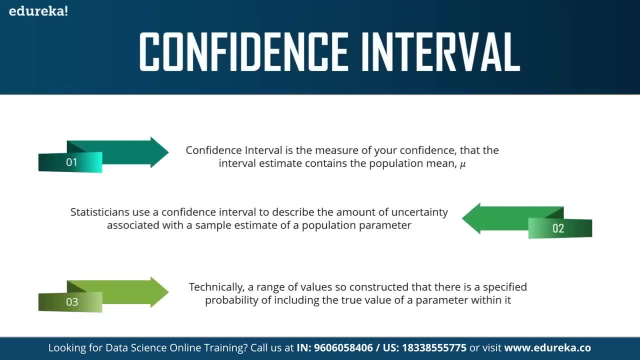 how many cans of cat food they purchase in one year. Okay, You test your statistics at the 99% confidence level- Okay, And you get a confidence interval of 100, 200. This means that you think that the cat owners buy between 100 to 200 cans in a year. 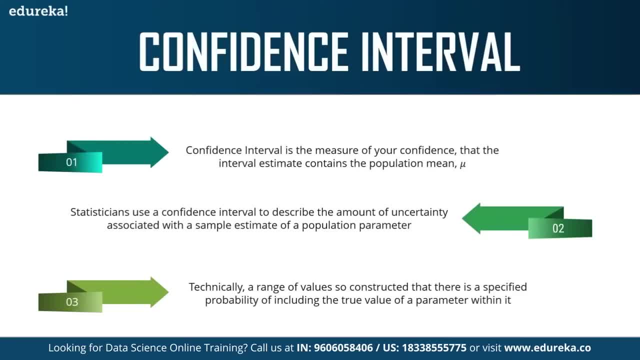 And also, since the confidence level is 99%, it shows that you're very confident that the results are correct. Okay, I hope all of you are clear with that. All right, So your confidence interval here will be 100 and 200.. 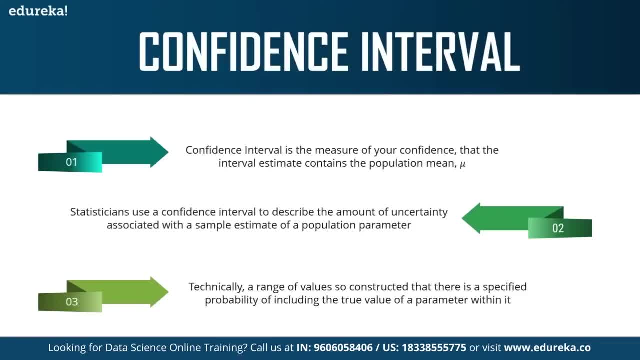 And your confidence level will be 99%. Right. This is the difference between confidence interval and confidence level. So within your confidence interval, your value is going to lie And your confidence level will show how confident you are about your estimation Right. 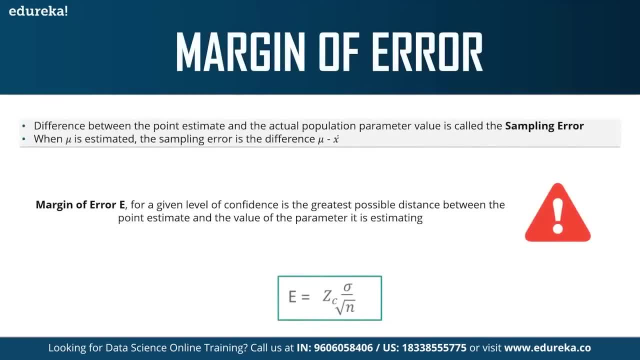 I hope that was clear. Let's look at margin of error Now. margin of error for a given level of confidence is the greatest possible distance between the point estimate and the value of the parameter that it is estimating. You can say that it is a deviation from the actual point estimate. 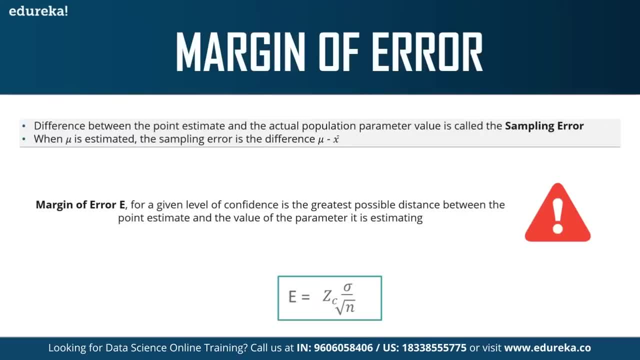 Right Now, the margin of error can be calculated using this formula. Now, ZC here denotes the critical value or the confidence interval, And this is multiplied by standard deviation, divided by root of the sample size. All right, N is basically the sample size. 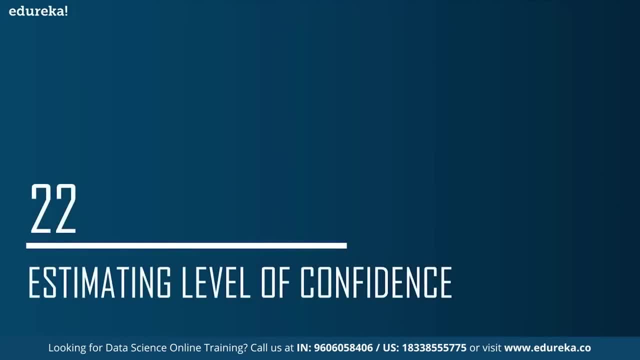 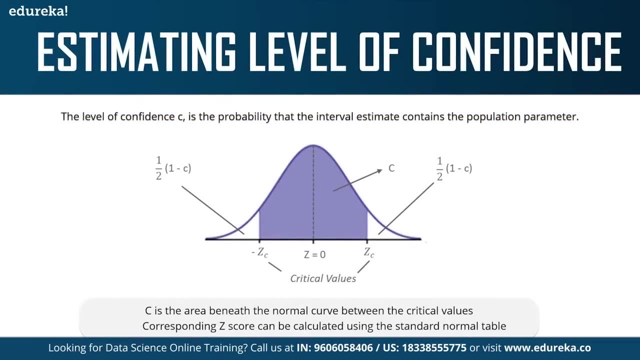 Now let's understand how you can estimate the confidence intervals. So, guys, the level of confidence which is denoted by C is the probability that the interval estimate contains a population Parameter. Let's say that you are trying to estimate the mean. 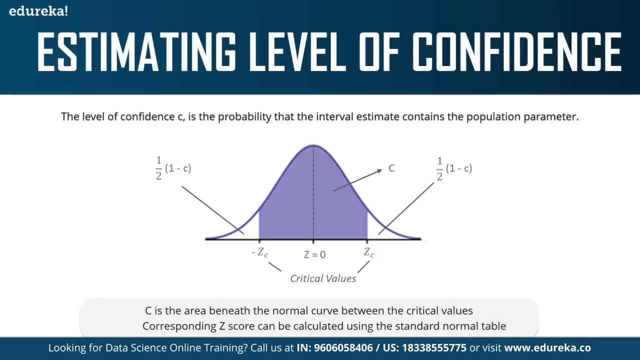 All right. So the level of confidence is the probability that the interval estimate contains a population parameter. So this interval between minus ZC and ZC, or the area beneath this curve, is nothing but the probability that the interval estimate contains a population parameter. 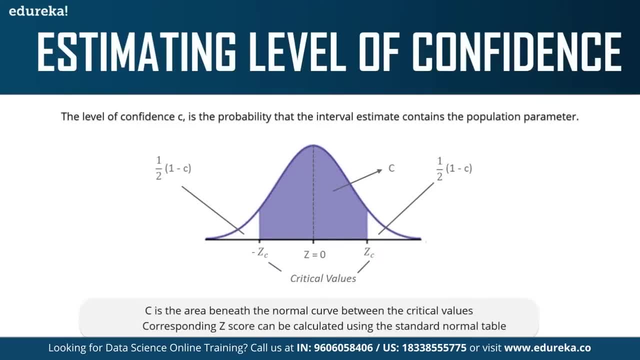 All right. It should basically contain the value that you are predicting Right Now. these are known as critical values. This is basically your lower limit and your higher limit confidence level. Also, there's something known as the Z score. Now this score can be calculated by using the standard normal table. 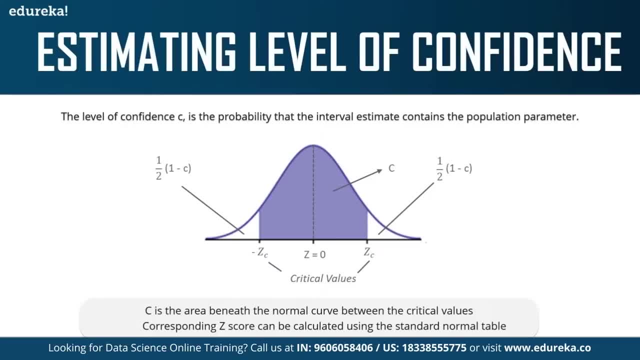 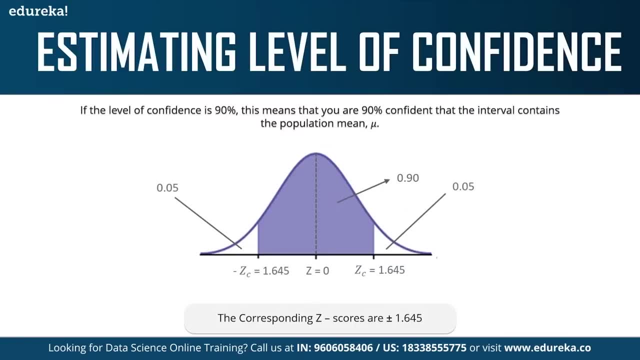 All right, If you look it up anywhere on Google, you'll find the Z score table or the standard normal table. Okay, To understand how this is done, let's look at a small example. Okay, Let's say that the level of confidence is 90%. 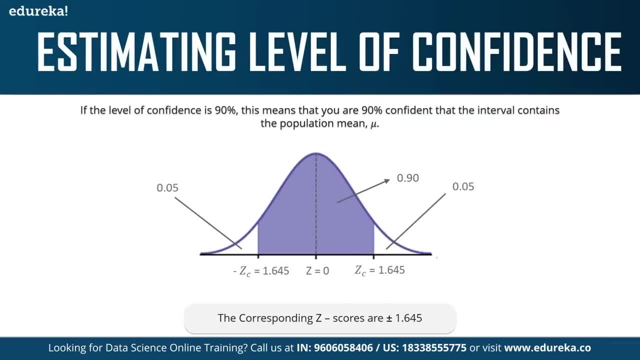 This means that you are 90% confident that the interval contains the population mean. Okay, So the remaining 10%, which is out of 100%, the remaining 10% is equally distributed on these tail regions. Okay, So you have 0.05 here and 0.05 over here. 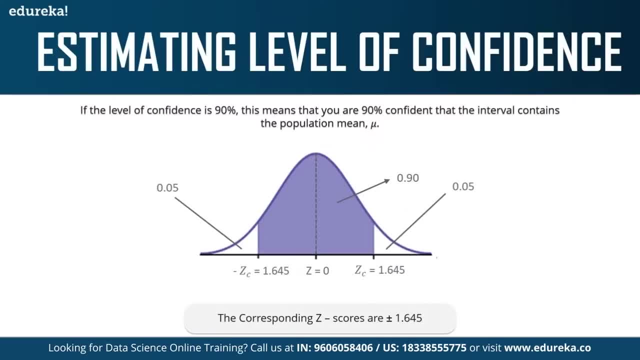 Right. So on either side of C you'll distribute the other left over percentage. Now these Z scores are calculated from the table, as I mentioned before. All right, 1.645 is calculated from the standard normal table. Okay. 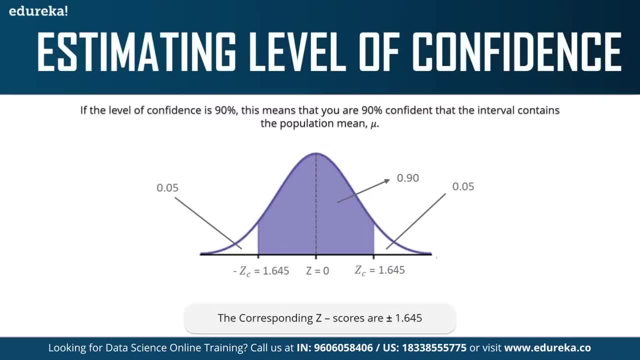 So, guys, this is how you estimate the level of confidence. So, to sum it up, let me tell you the steps that are involved in constructing a confidence interval. First, you'll start by identifying a sample statistic. Okay, This is the statistic that you will use to estimate a population parameter. 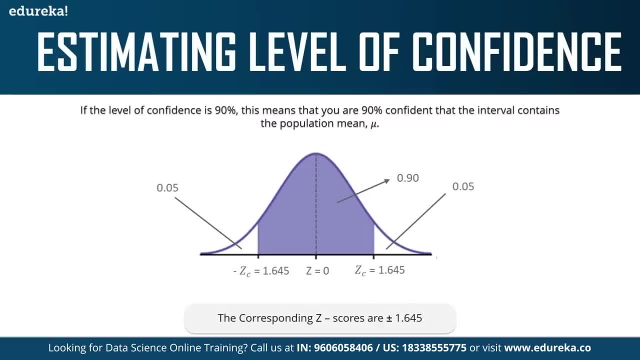 This can be anything like the mean of the sample. Next, you will select a confidence level. Now, the confidence level describes the uncertainty of a sampling method. Right After that, you'll find something known as the margin of error. Right. 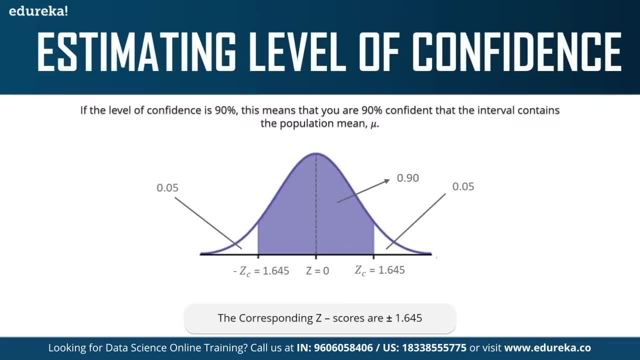 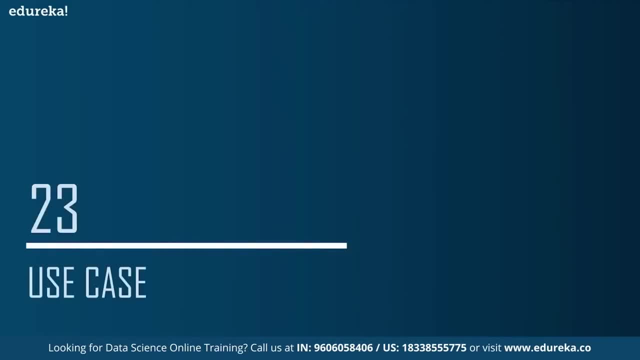 We discussed margin of error earlier, So you find this based on the equation that I explained in the previous slide. Then you'll finally specify the confidence interval. All right, Now let's look at a problem statement to better understand this concept. 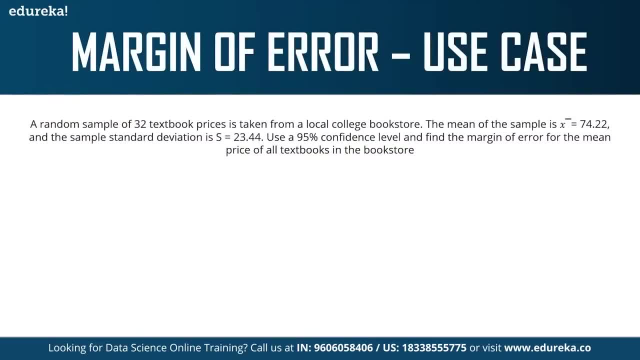 A random sample of 32 textbook prizes is taken from a local college bookstore. The mean of the sample is so, so and so, And the sample standard deviation is this: Use a 95% confident level And find the margin of error for the mean prize of all textbooks in the bookstore. 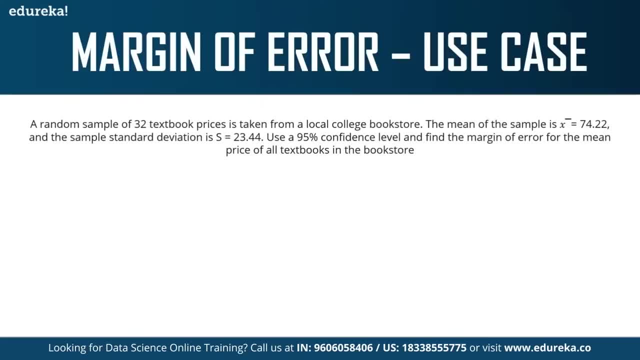 Okay, Now, this is a very straightforward question. If you want, you can read the question again. All you have to do is you have to just substitute the values into the equation. All right, So, guys, we know the formula for margin of error. 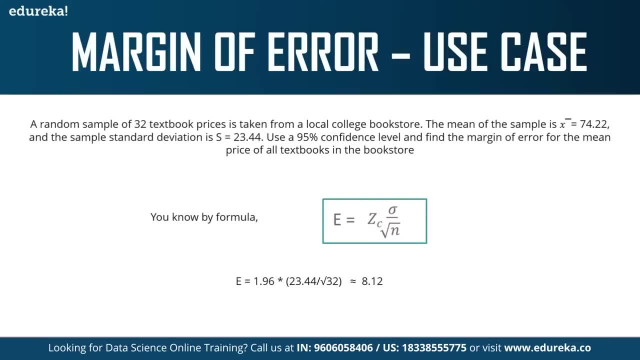 You take the z-score from the table. After that we have deviation, which is 23.44.. Right, That's standard deviation, And n stands for the number And n stands for the number of samples. Here the number of samples is 32.. 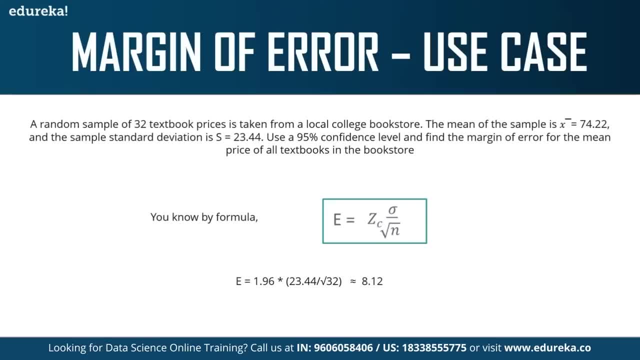 Basically 32 textbooks, So approximately your margin of error is going to be around 8.12.. This is a pretty simple question, All right, I hope all of you understood this. Now that you know the idea behind confidence interval, let's move ahead to one of the most 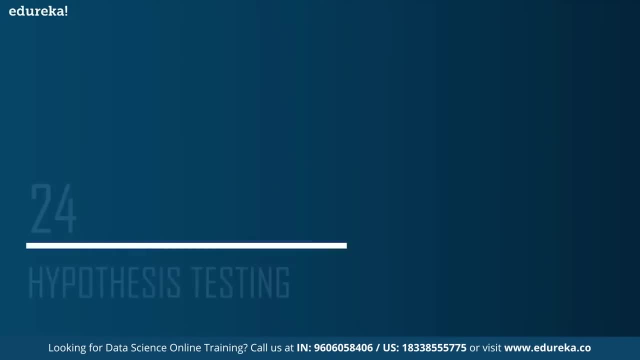 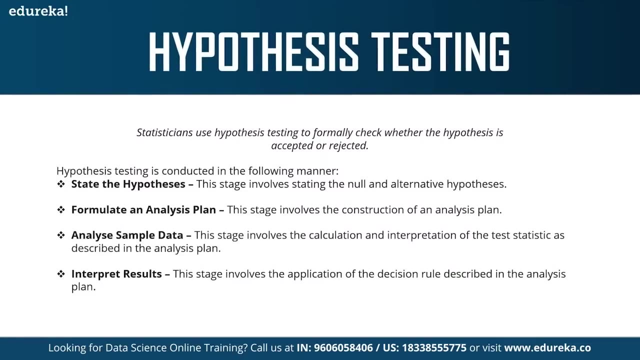 important topics in statistical inference, which is hypothesis testing, Right? So basically, statisticians use hypothesis testing to formally check whether the hypothesis is accepted or rejected. Okay, Hypothesis testing is an inferential statistical technique used to determine whether there is enough evidence in a data sample to infer that a certain condition holds true for an 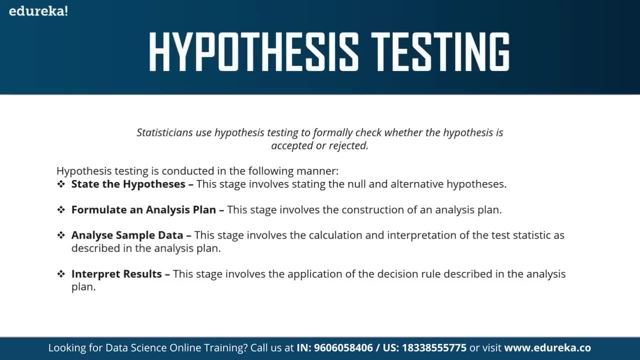 entire population. So to understand the characteristics of a general population, we take a random sample and we analyze the properties of the sample Right. We test whether or not the identified condition is true, The identified conclusion represents the population accurately And finally, we interpret their results. 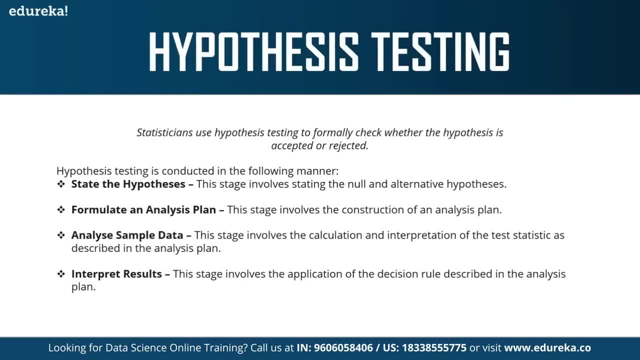 Now, whether or not to accept the hypothesis depends upon the percentage value that we get from the hypothesis. Okay, So to better understand this, let's look at a small example. Before that, there are a few steps that are followed in hypothesis testing. 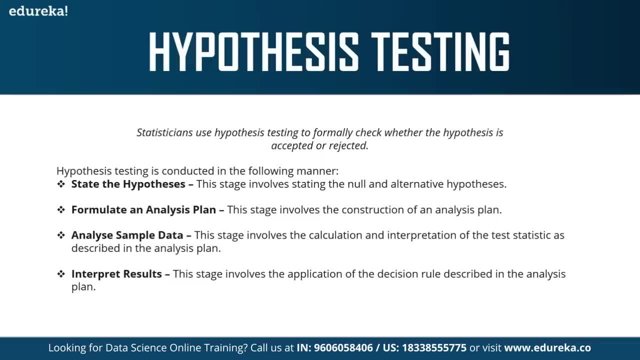 You begin by stating the null and the alternative hypothesis- All right, I'll tell you what exactly these terms are. And then you formulate an analysis plan. All right. After that, you analyze the sample data and finally, you can interpret the results. 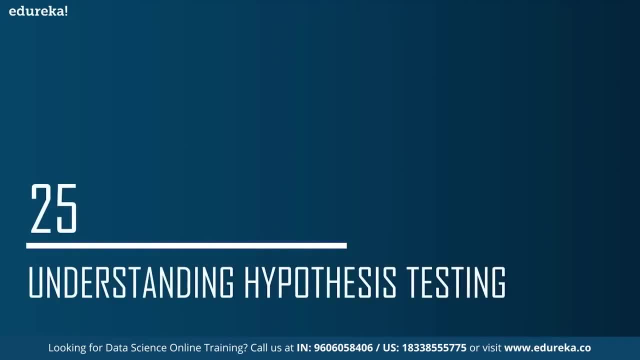 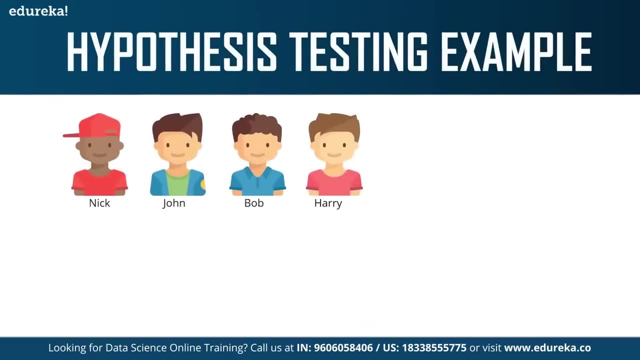 Right Now, to understand the entire hypothesis testing, we'll look at a good example. Okay, Now consider four boys: Nick, John, Bob and Harry. These boys were caught bunking a class and they were asked to stay back at school and 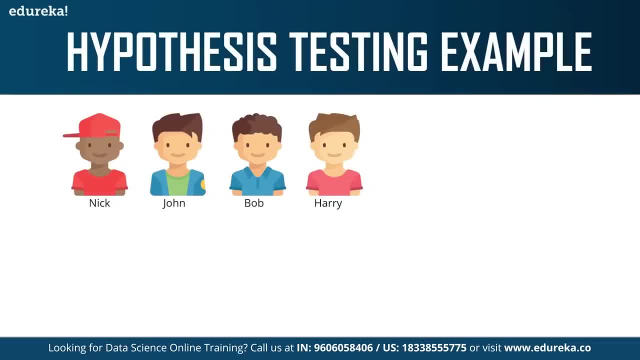 clean their classroom as a punishment, Right? So what John did is he decided that four of them would take turns to clean their classrooms, Right? So he came up with a plan of writing each of their names on chits and putting them in. 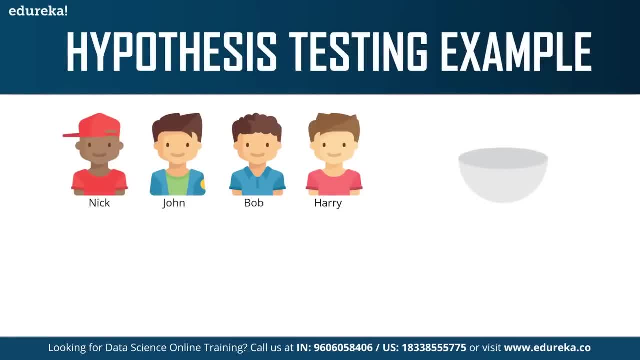 a bowl. Now every day they had to pick up a name from the bowl and that person had to clean the class, Right? That sounds pretty fair enough. Now it has been three days and everybody's name has come up except John's. 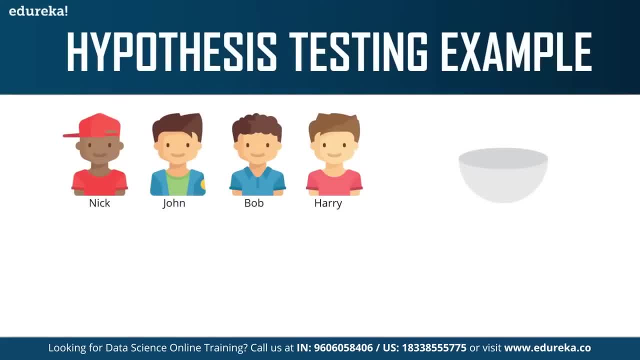 Assuming that this event is completely random and free of bias, what is the probability of John not cheating, Right? What is the probability that he's not actually cheating? This can be solved by using hypothesis testing. Okay, So we'll begin by calculating the probability of John not being picked for a day. 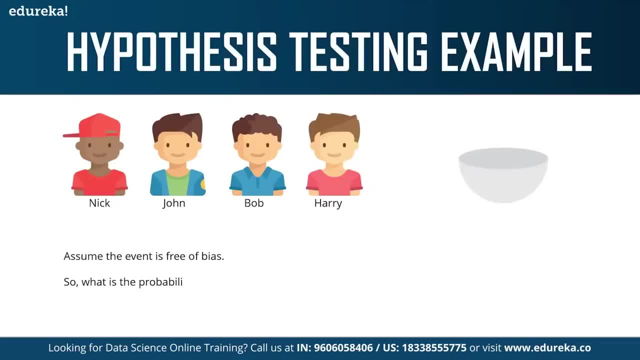 Right. So we're going to assume that the event is free of bias. So we need to find out the probability of John not cheating Right First. we'll find the probability that John is not picked for a day Right. 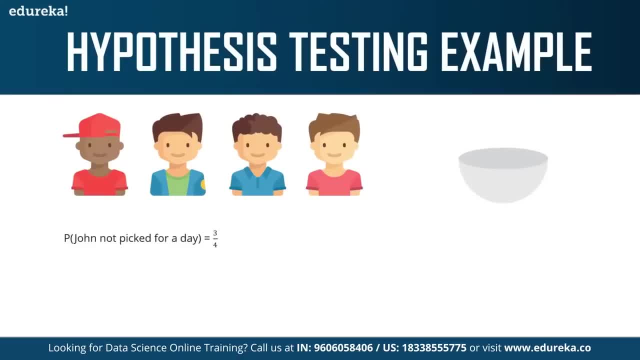 We get three out of four, Which is basically 75 percent. Now, 75 percent is fairly high, so if John is not picked for three days in a row, the probability will drop down to approximately 42 percent. okay, so three days in a row meaning. 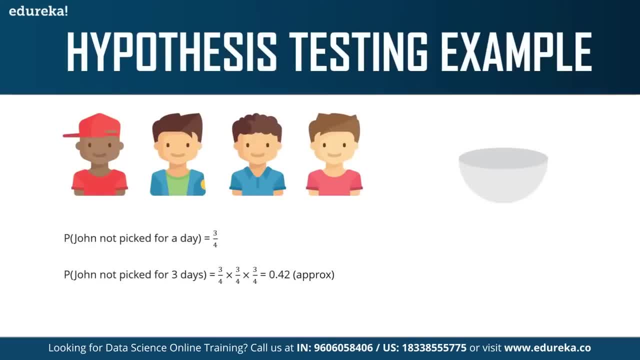 that is, the probability drops down to 42 percent. now let's consider a situation where john is not picked for 12 days in a row. the probability drops down to 3.2 percent. okay, that's, the probability of john cheating becomes fairly high, right? so, in order for statisticians to come to a conclusion, 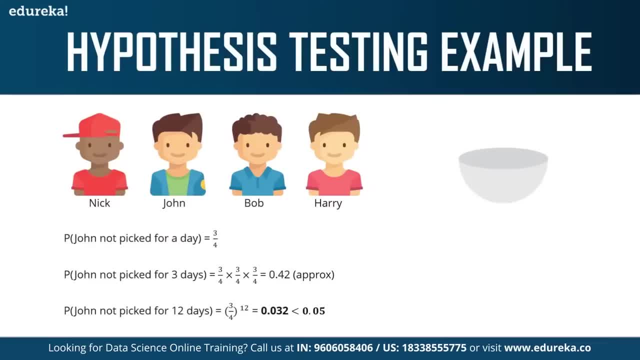 they define what is known as the threshold value right. considering the above situation, if the threshold value is set to five percent, it would indicate that if the probability lies below five percent, then john is cheating his way out of detention. but if the probability is above threshold value, then john is just lucky and his name isn't getting picked. so the probability and hypothesis. 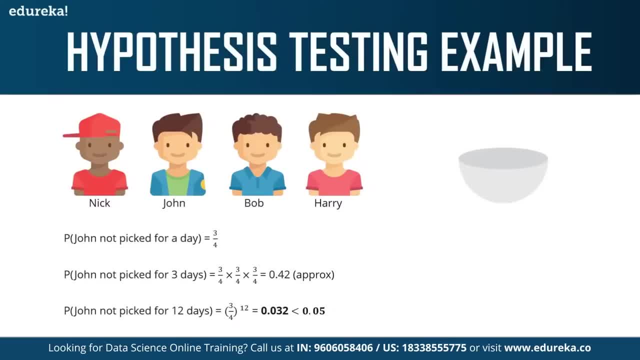 testing give rise to two important components of hypothesis testing, which is null hypothesis and alternating hypothesis. null hypothesis is basically approving the assumption. alternate hypothesis is when your result disapproves the assumption right. therefore, in our example, if the probability of an event occurring is less than five percent, which it is, then the event is biased, hence it proves the. 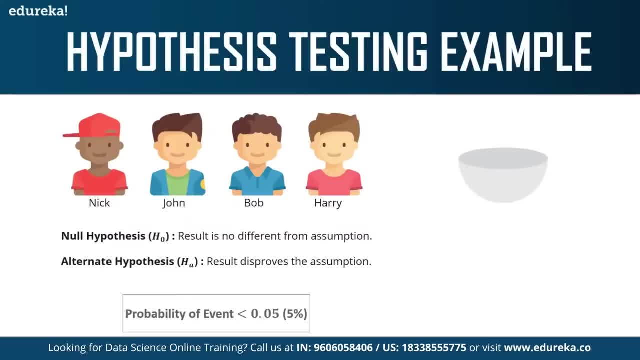 alternate hypothesis. so, guys, with this we come to the end of this session. so, before i wrap up, we're going to run a quick demo which is based on inferential hypothesis, and then we're going to run a quick demo which is based on inferential hypothesis, and then we're going to run a quick. 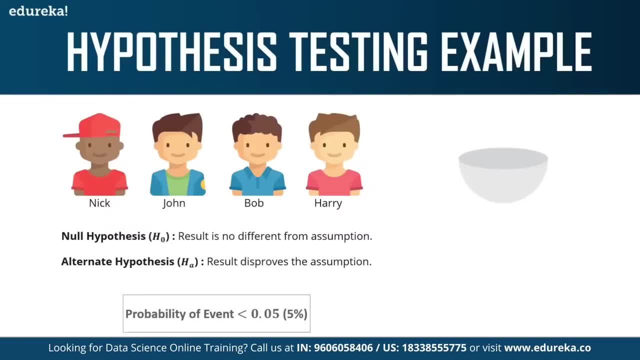 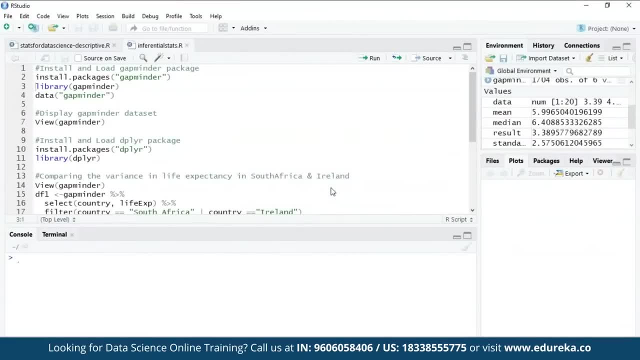 demo, which is based on inferential statistics. let's quickly open up our studio again. i'll be running this in our language and those of you who don't know are it's okay. i'm going to leave a couple of links in the description, and this is pretty understandable. this is just basic math. 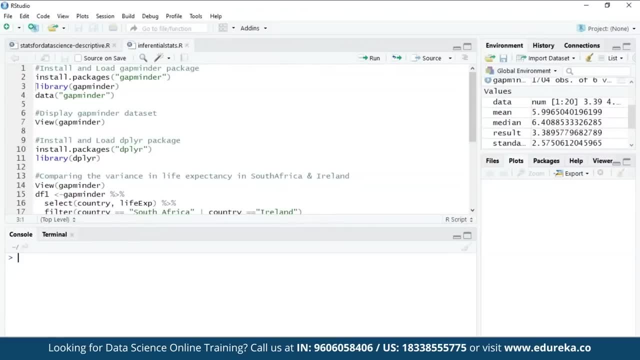 right now, in this demo, what we'll be doing is we'll be using the gapminder data set to perform hypothesis testing. now, guys, the gapminder data set contains a list of 142 countries with their respective values for life expectancy, and then we're going to run a quick demo, which is based on. 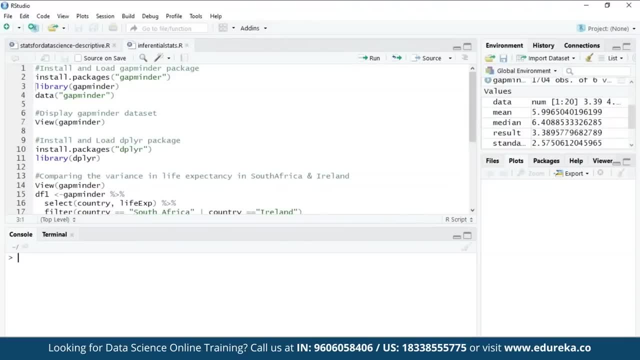 inferential hypothesis, and then we'll be using the gapminder data set to perform hypothesis testing. now, guys, the gapminder data set contains a list of 142 countries with their respective values for life expectancy, a gdp per capita and population every five years from 1952 to 2007. okay, don't worry, i'll show you the data set. so what we'll do is we'll begin by 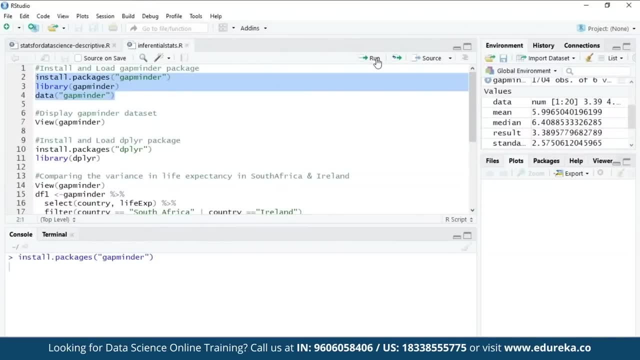 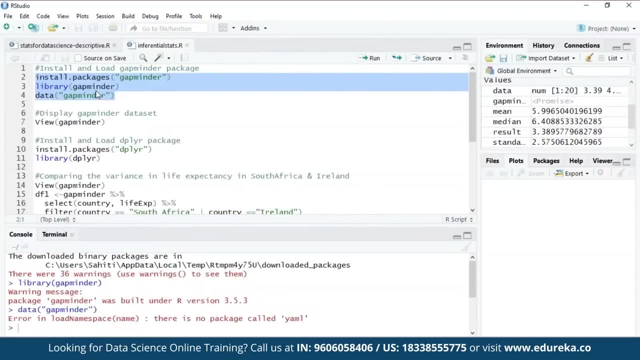 installing and downloading the gapminder data set. so these installpackages will basically install the gapminder package and this library. gapminder will just load the gapminder library. all right, so we've successfully loaded our gapminder package. now let's view the 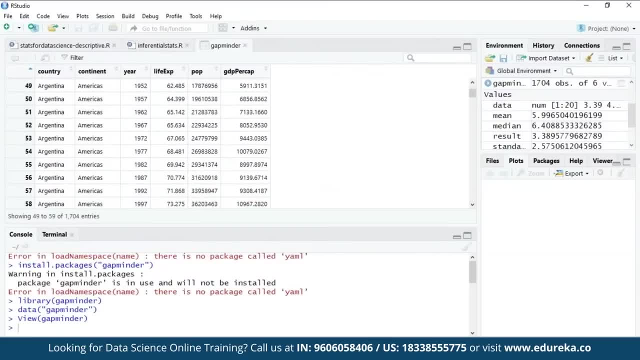 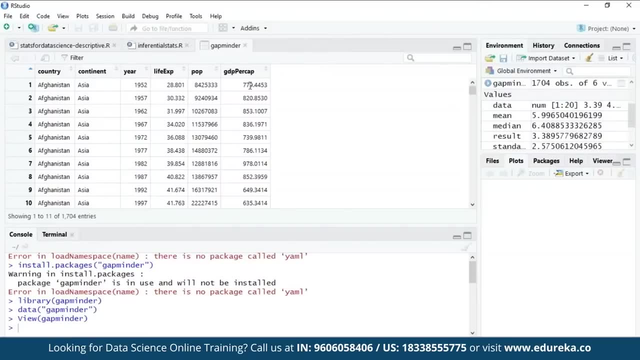 data set. these are the countries. all right, different countries, and you have the continents, the year, the life expectancy, the population and the gdp per capita. okay, so, each of these countries. we have this information right now. the next step is to load the famous deployer package provided. 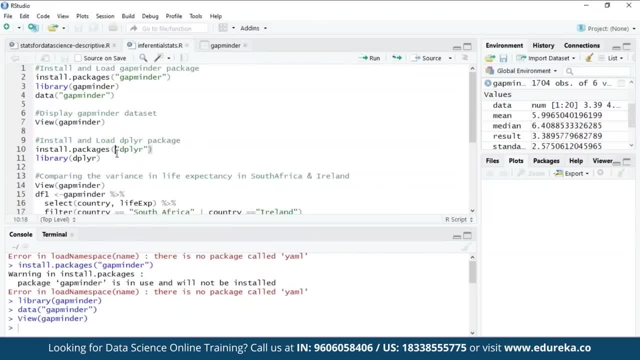 by our. we're specifically looking to use the pipe operator in this package. okay, now for those of you who don't know what the pipe operator does, this is a pipe operator. right now, the pipe operator allows you to pipe your data from the left hand side into the. 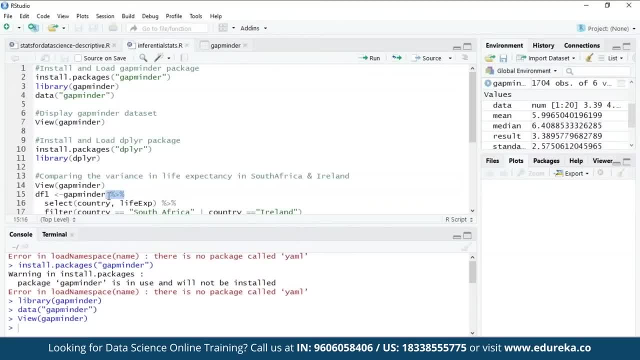 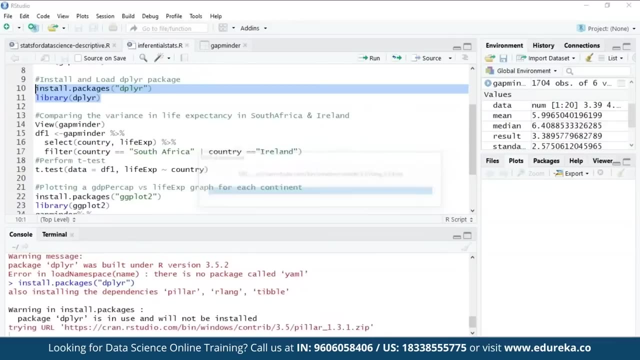 data at the right hand side of the pipe. okay, it's quite self-explanatory: it's a pipe which connects two data points, right? so let's install and load this package. all right. now our next step. what we're going to do is we're going to compare the life expectancy of two places. 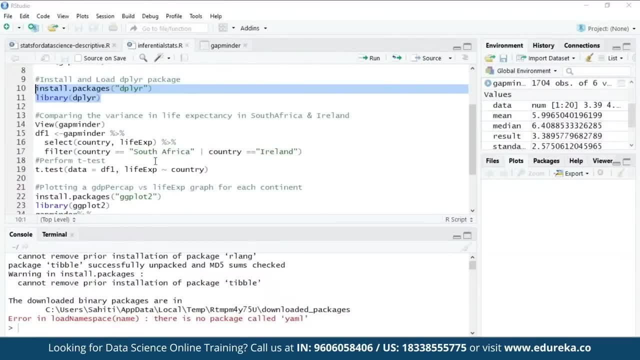 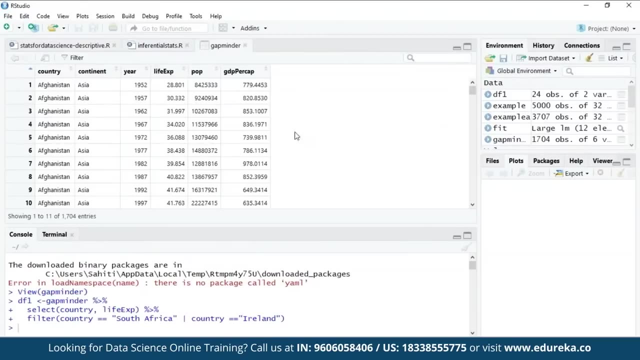 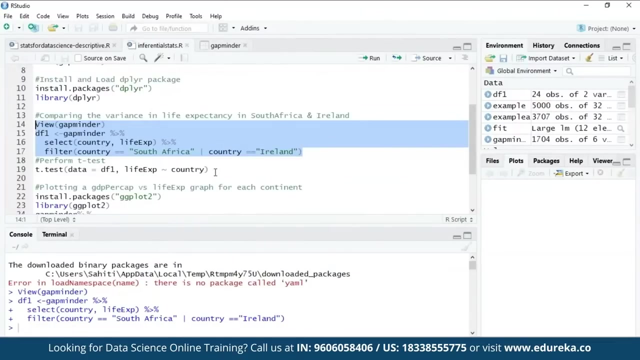 okay, we're going to compare the life expectancy of ireland and south africa and we're going to perform the t test to check if the comparison follows a null hypothesis or an alternate hypothesis. okay, so let's run the code. okay, so now we'll apply the t test and we'll compare the life expectancy of these two places. 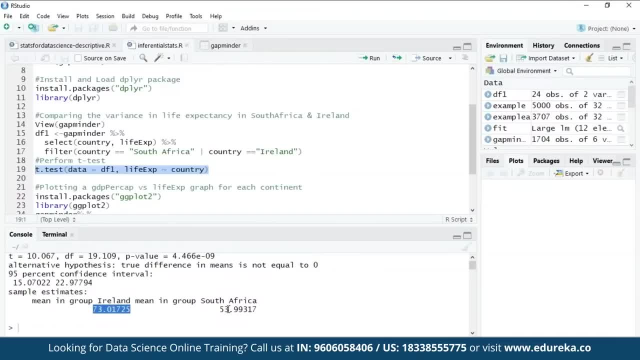 all right, let's run this: notice: the mean in group ireland and south africa. right here is the mean. you can see that the life expectancy almost differs by a scale of 20.. now we need to check if this difference in the value of life expectancy in south africa and ireland is actually valid and not. 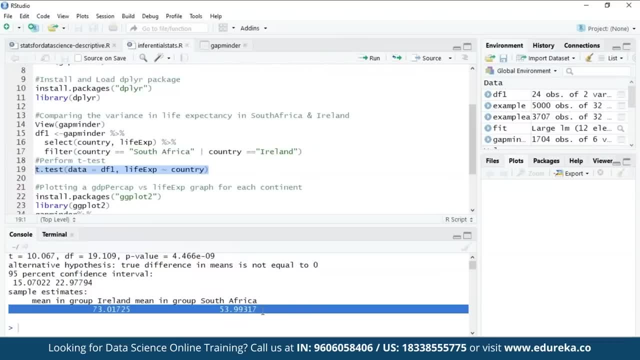 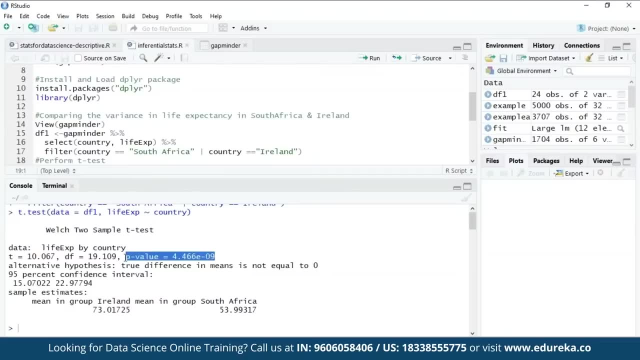 just by pure chance, okay. for this reason, the d test is carried out. so pay special attention to this p value over here. this is also known as the probability value right. the p value is very important measurement when it comes to ensuring the significance of a model. a model is said to. 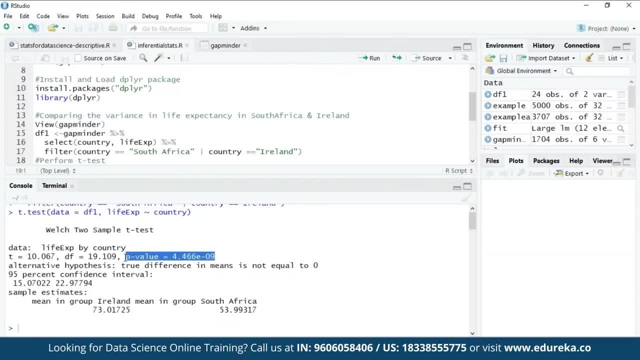 be statistically significant only when the p value is less than the predetermined statistical significance level, which is ideally 0.05. right, so your p value has to be much lesser than 0.05. as you can see from our output, the p value is very, very lesser when compared to 0.05. 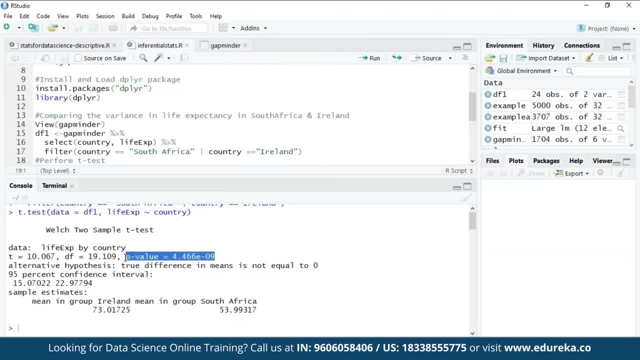 right, it is an extremely small value, which is a good thing. now, in the summary of the model, notice another important parameter called the t value. right, i've been talking about the t test. and what exactly is this t value? you can see it over here: it is 10.067. now a larger t. 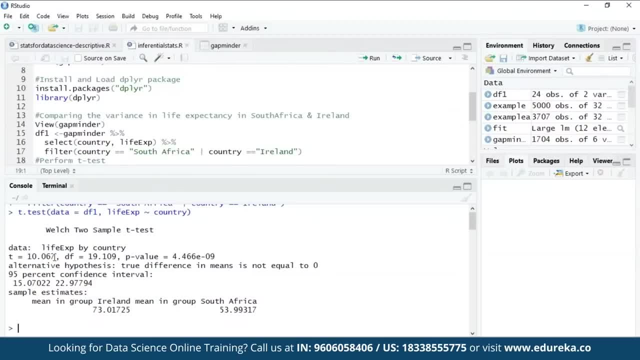 value suggests that the alternate hypothesis is true and that the difference in life expectancy is not equal to 0 by pure luck. hence, in our case, the null hypothesis is disapproved. so to conclude the demo, we'll be plotting a graph for each continent, such that the graph shows how the 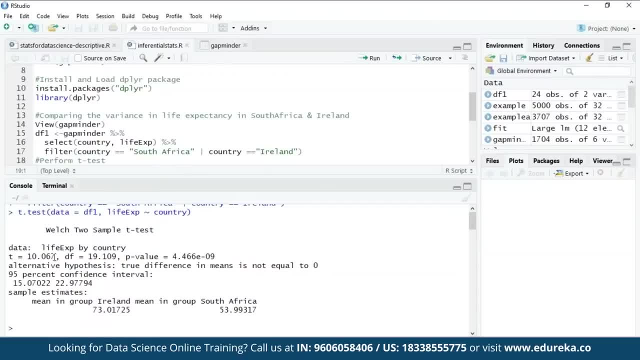 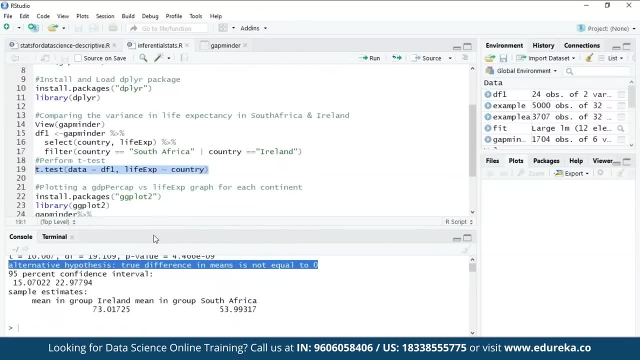 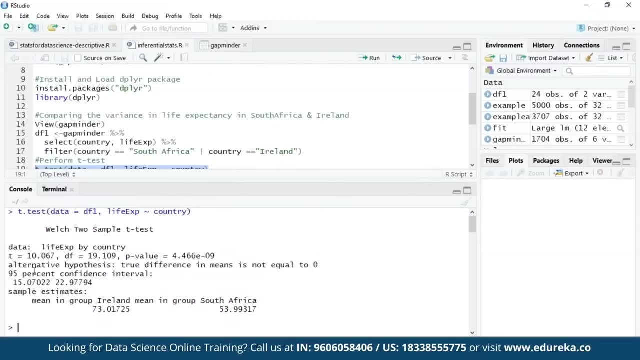 life expectancy for each continent varies with the respective gdp per capita. just to add a little bit data visualization. i am performing this last step. so, guys here, we can clearly see from the output that the alternate hypothesis is true, all right. and also, this is the is calculated with a 95 confidence interval, right? you get what i'm saying when i'm talking about. 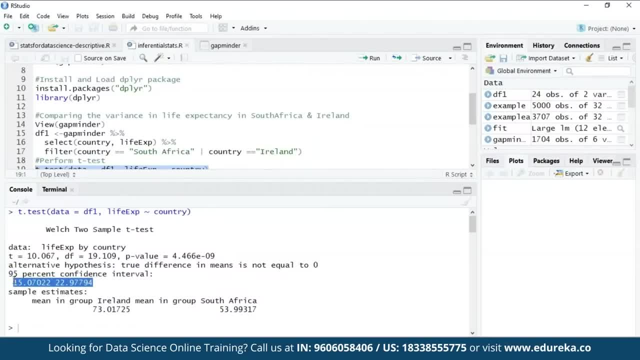 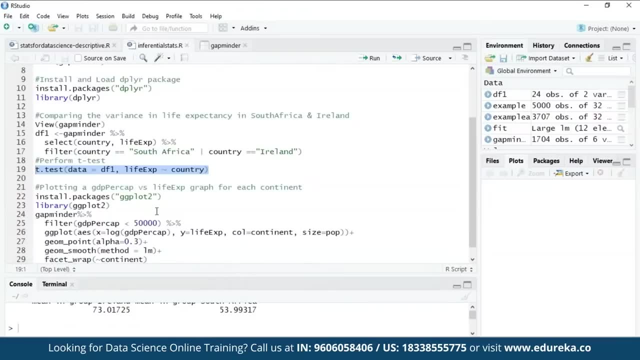 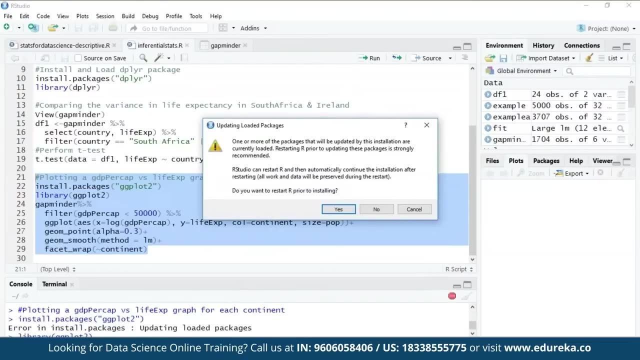 95 confidence interval. right, this is our confidence interval: 15 to 22, and our confidence level is 95. this is exactly what we discussed a couple of minutes ago. now, just to end the demo, i'll show you a small visualization here. what we're doing is we're. 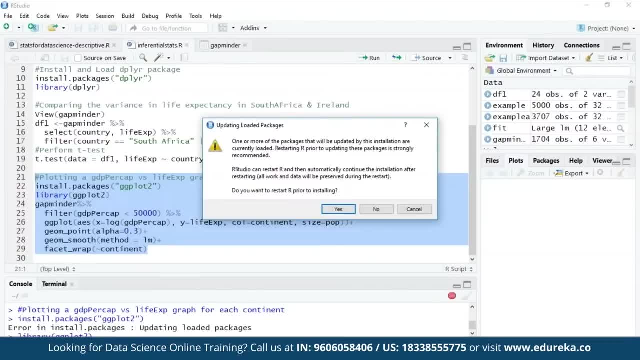 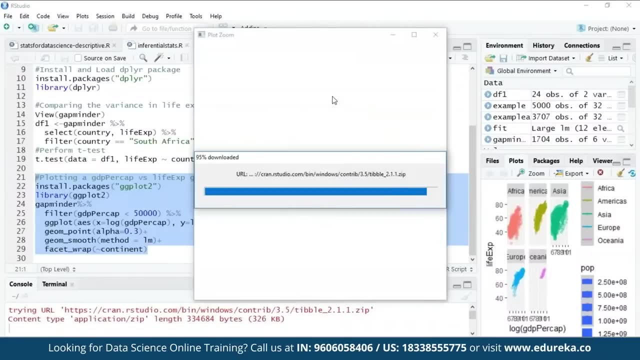 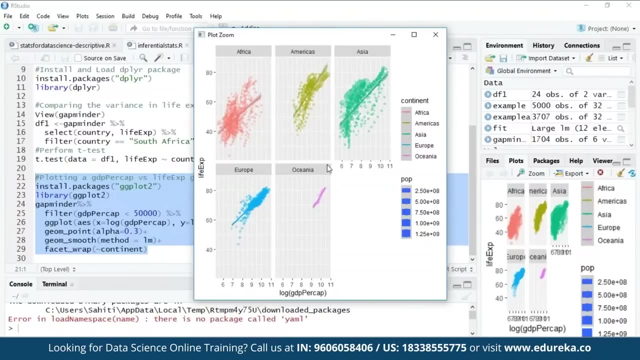 showing how the life expectancy for each continent varies with respect to the gdp per capita for that continent. okay, so this is our plot. okay, if you look at the illustration, you can almost see a linear variance. right, you can almost see a linear line in the life expectancy for each of. 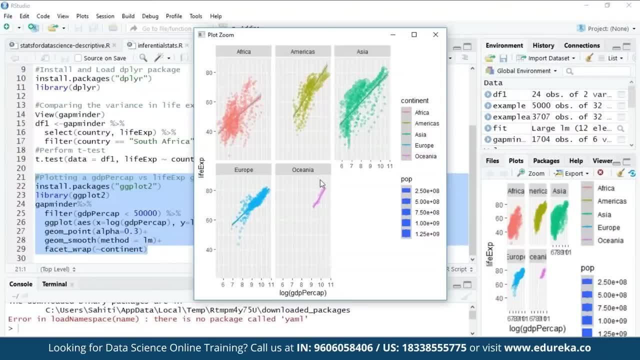 the continent with respect to the gdp per capita right. this also shows how well the r language can be used for statistical analysis right? look at how pretty the graph looks. and also how well they show that there is almost a linear dependency between the gdp per capita and the gdp per capita right. 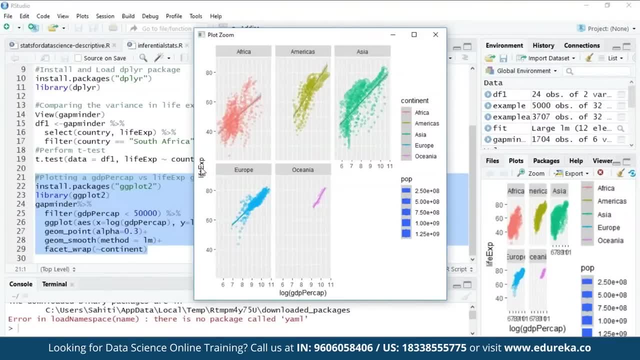 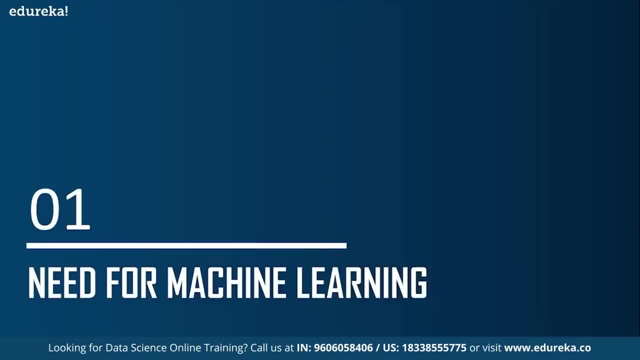 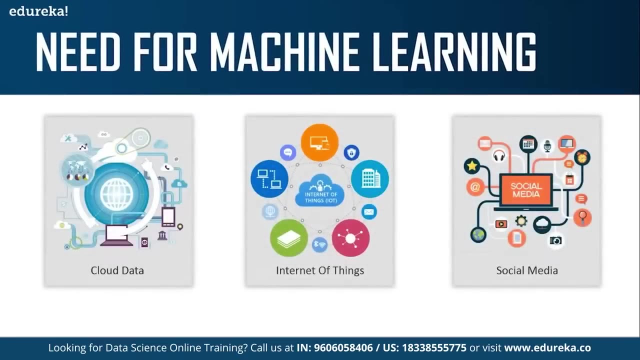 between the gdp per capita and the life expectancy. so what is the importance or what is the need for machine learning now? ever since the technical revolution, we've been generating an immeasurable amount of data, as, per research, we're generating around 2.5 quintillion bytes of data every single day, and it is estimated that 1.7 mb of data. 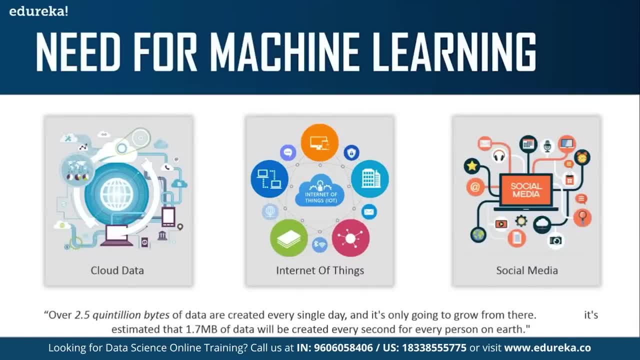 will be created every second for every person on earth. now, that is a lot of data. right now, this data comes from sources such as the cloud, iot devices, social media and all of that, since all of us are very interested in the internet. right now, we're generating a lot of data. 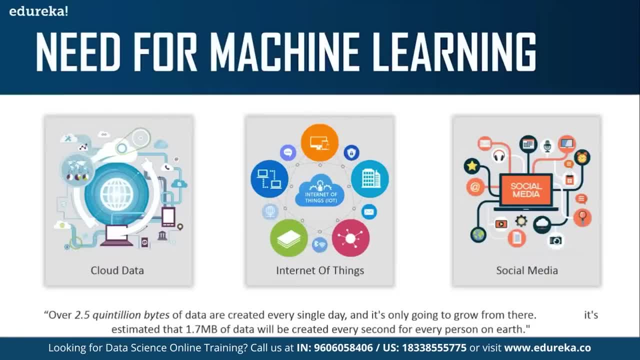 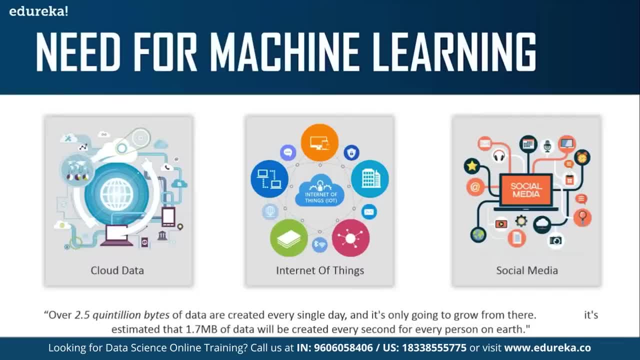 all of this generates a lot of data. all of this generates a lot of data. now, how does machine learning fit into all of this? since we're producing this much data, we need to find a method that can analyze, process and interpret this much data. all right, and we need to find a. 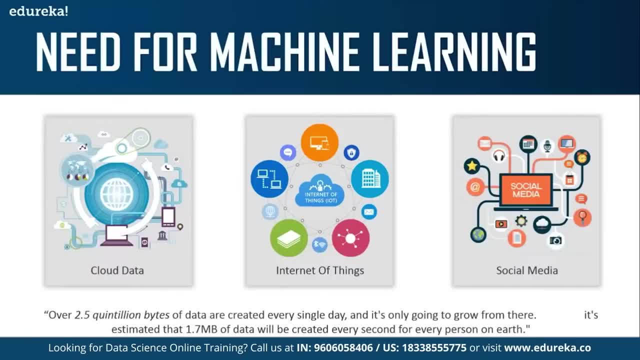 method that can make sense out of data, and that method is machine learning. now there are a lot of top-tier companies and data-driven companies, such as netflix and amazon, which build machine learning models by using tons of data in order to identify any profitable opportunities for machine learning. 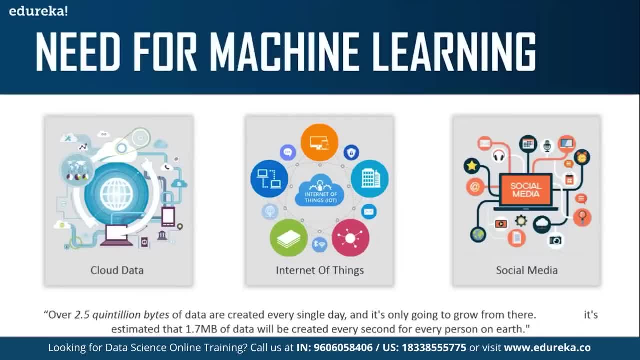 and if they want to avoid any unwanted risk, they make use of machine learning. all right, so through machine learning you can predict risks, you can predict profits, you can identify opportunities which will help you grow your business. so now i'll show you a couple of examples wherein machine 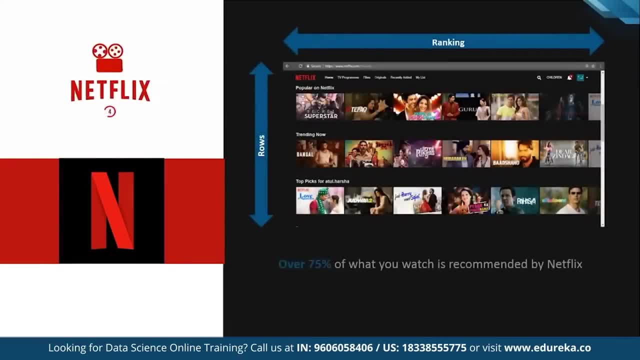 learning is used, all right, so i'm sure all of you have binge watch on netflix now. the most important thing about netflix is its recommendation engine. all right, most of netflix's revenue comes from its recommendation engine, so the recommendation engine basically studies the movie viewing. 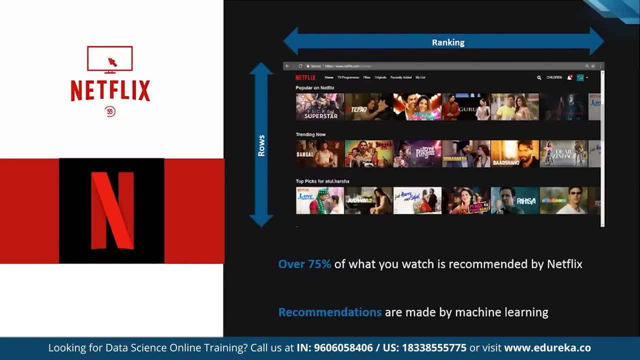 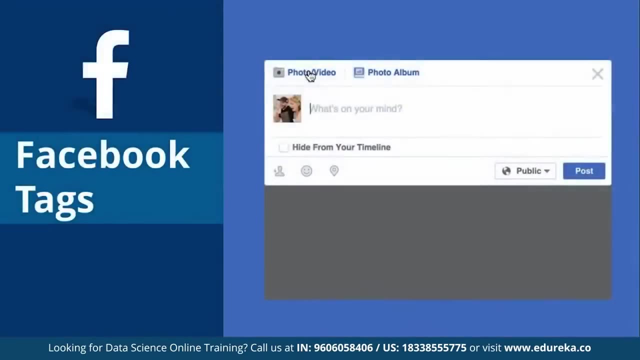 patterns of its users and then recommends relevant movies to them. all right. it recommends movies depending on users interests, depending on the type of movies the user watches, and all of that all right. so that is how netflix uses machine learning. next we have facebook's auto tagging. 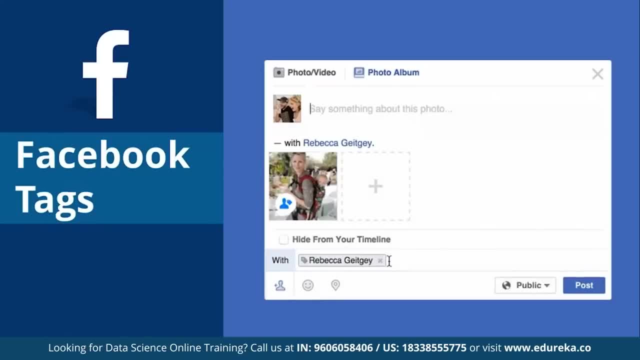 feature. now, the logic behind facebook's uh auto tagging feature is machine learning and neural networks. i'm not sure how many of you know this, but facebook makes use of deep mind face verification system, which is based on machine learning, natural language processing and neural networks. so deepmind basically studies the facial features in an image and it tags your friends and 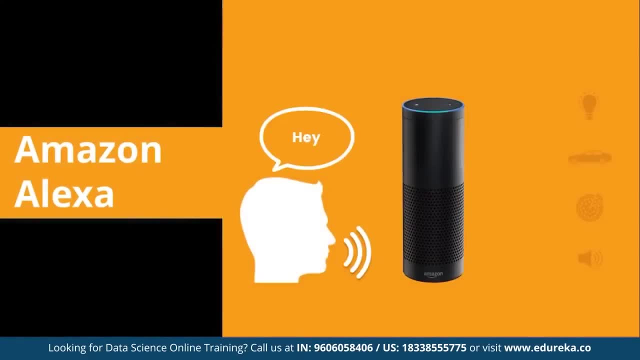 family. another such example is amazon's alexa. now alexa is basically an advanced level virtual assistant that is based on natural language processing and machine learning. now it can do more than just um play music for you. all right, it can book your uber, it can connect. 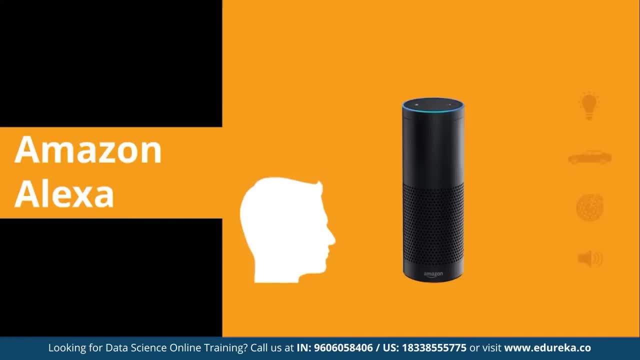 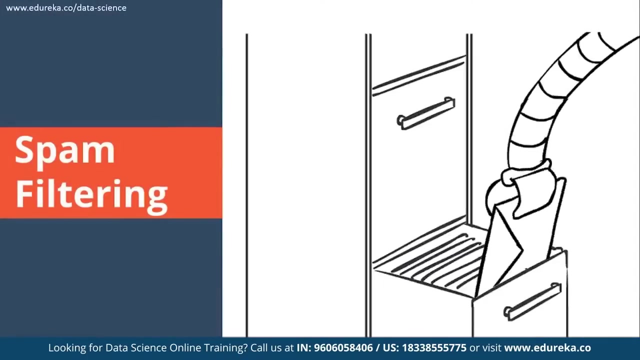 with other iot devices at your house. it can track your health, it can order food online and all of that okay. so data and machine learning are basically the main factors behind alexa's power. another such example is the google spam filter. so, guys, gmail basically makes use of machine. 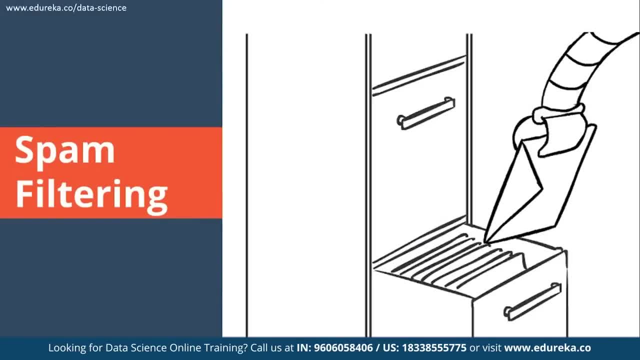 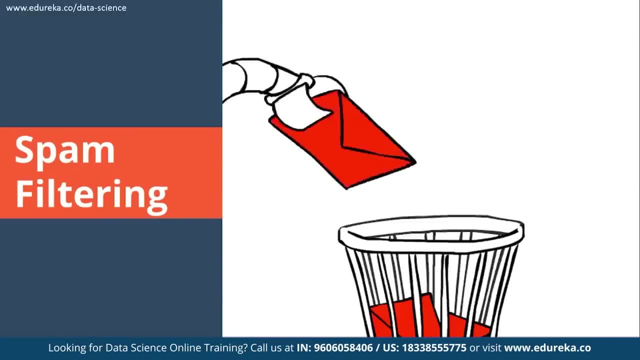 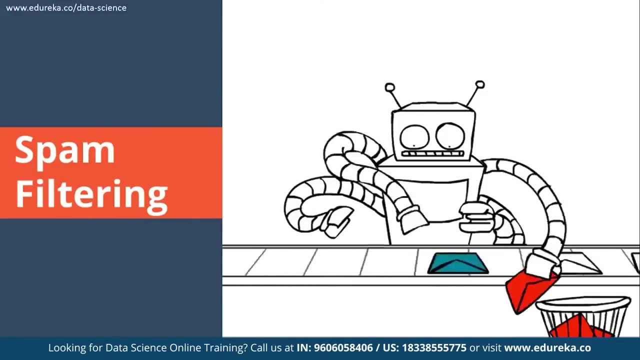 learning to filter out spam messages. if any of you just open your gmail inbox, you'll see that there are separate sections: there's one for primary, there's social, there's spam and there's your general mail. now, basically, gmail makes use of machine learning, algorithms and natural language processing to analyze emails in real time and then classify them as either spam. 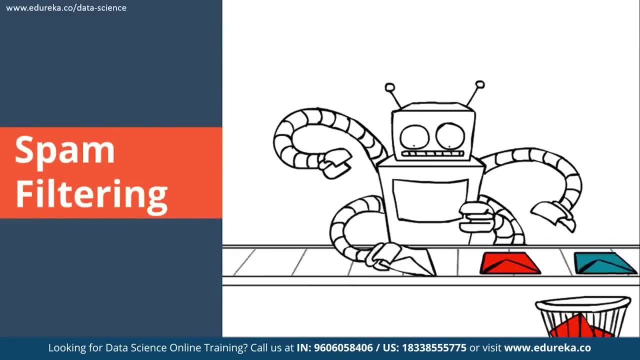 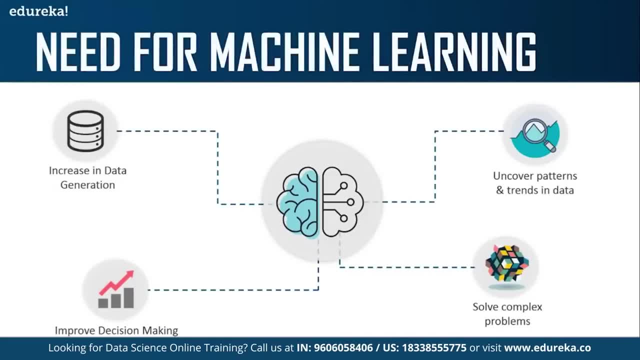 or non-spam. now this is another famous application of machine learning. so, to sum this up, let's look at a few reasons why machine learning is so important. so the first reason is obviously increase in data generation. so, because of excessive production of data, we need a method that can be used to structure, analyze and draw useful insights from data. this is where 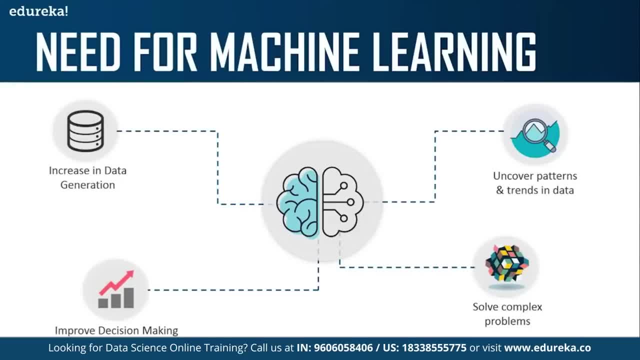 machine learning comes in. it uses data to solve problems and find solutions to the most complex tasks faced by organizations. another important reason is that it improves decision making. so, by making use of various algorithms, machine learning can be used to make better business decisions. for example, machine learning is used to forecast sales. it is used to predict any downfalls. 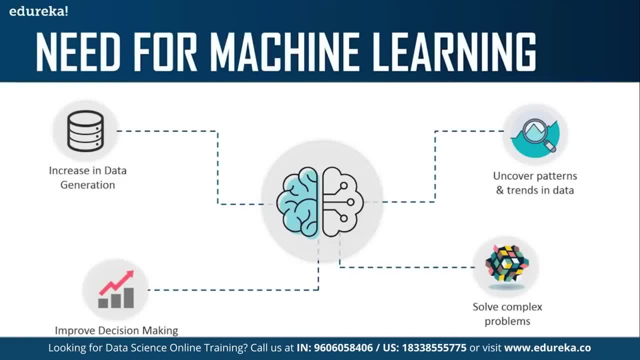 in the stock market. it is used to identify risks, anomalies and so on. now the next reason is it uncovers patterns and trends in data. finding hidden patterns and extracting key insights from data is the most essential part of machine learning. so by building predictive models and using statistical techniques, machine learning allows you to dig beneath the 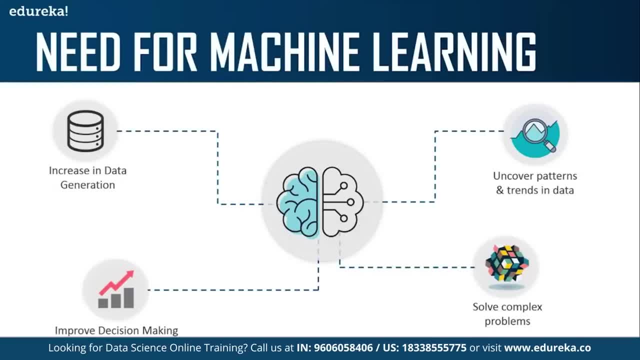 surface and explore the data at a minute scale. now, understanding data and extracting patterns manually will take a lot of days. now, if you do this through machine learning algorithms, you can perform such computations in less than a second. another reason is that it solves complex problems, so from detecting genes that are linked to deadly als diseases to building self-driving. 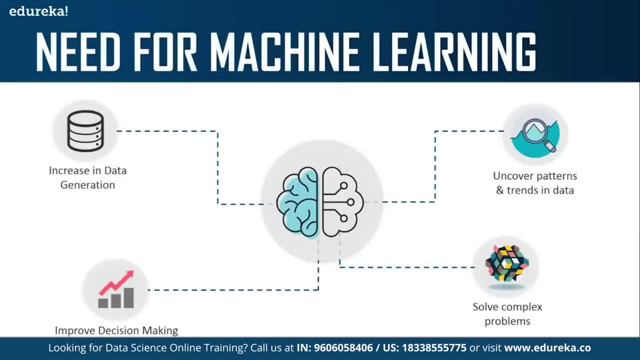 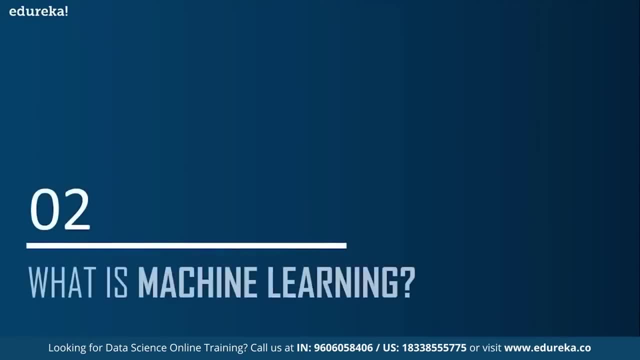 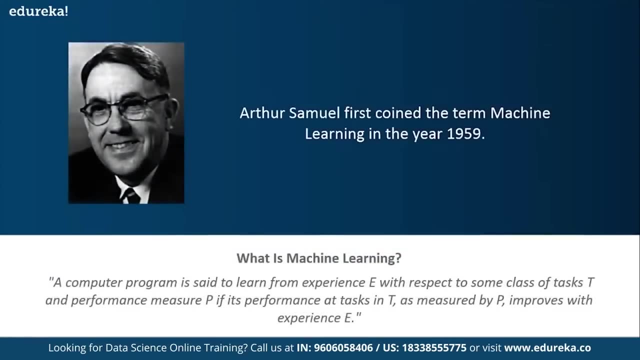 cars and building phase detection systems, machine learning can be used to solve the most complex problems. so, guys, now that you know why machine learning is so important, let's look at what exactly machine learning is. the term machine learning was first coined by arthur samuel in the year 1959. now, looking back, that year was probably the most significant in 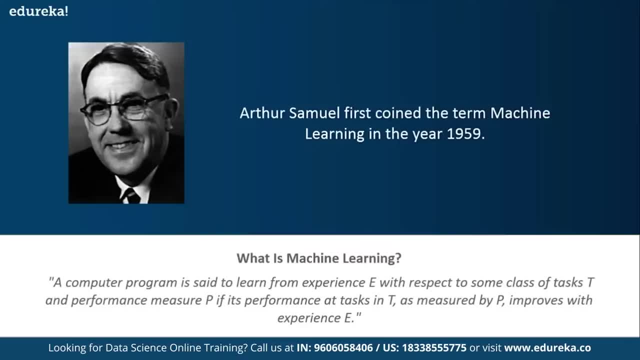 terms of technological advancements. guys, if you browse through the net about what is machine learning, you'll get at least 100 different definitions. now the first and very formal definition was given by tom m mitchell. now the definition says that a computer program is said to learn from experience e with respect to some class of task t and performance measure p if its 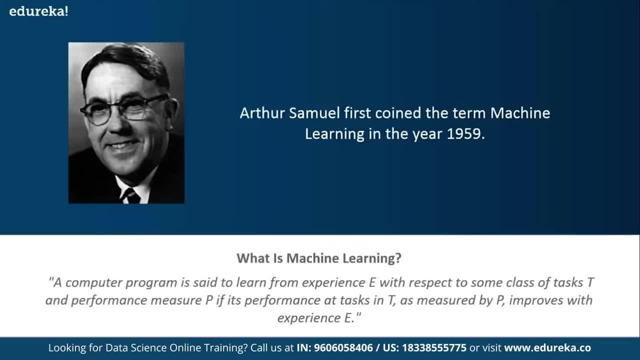 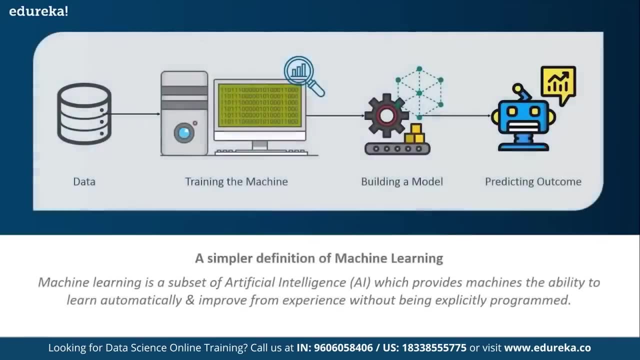 performance at tasks in t, as measured by p, improves with experience, e. all right now, i know this is a little confusing, so let's break it down into simple words now. in simple terms, machine learning is a subset of artificial intelligence. it provides machines the ability to learn automatically and improve from experience. 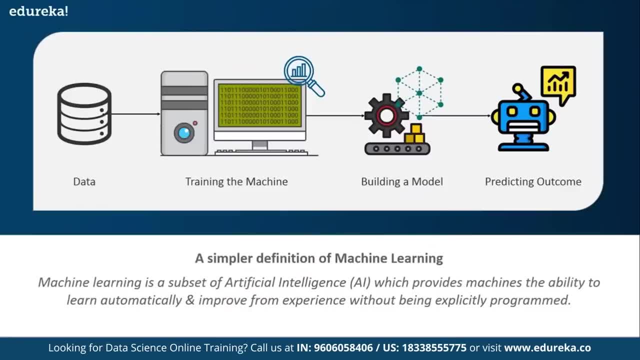 without being explicitly programmed to do so. in the sense, it is the practice of getting machines to solve problems by gaining the ability to think. but wait now. how can a machine think or make decisions? well, if you feed a machine a good amount of data, it will learn how to interpret. 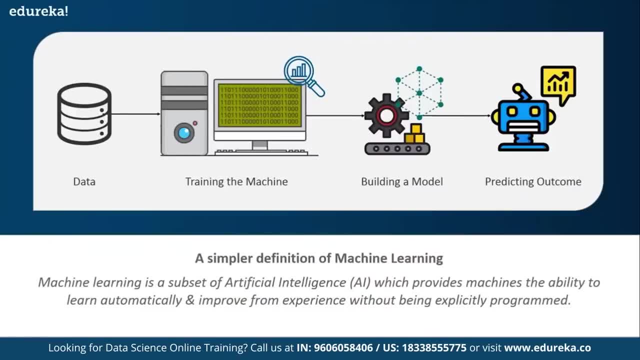 process and analyze this data by using machine learning algorithm. okay, now guys, look at this figure on top. now. this figure basically shows how a machine learning algorithm, or how the machine learning process, really works. so the machine learning process begins by feeding the machine lots and lots of data. okay, by using this data, the machine is trained to detect hidden insights. 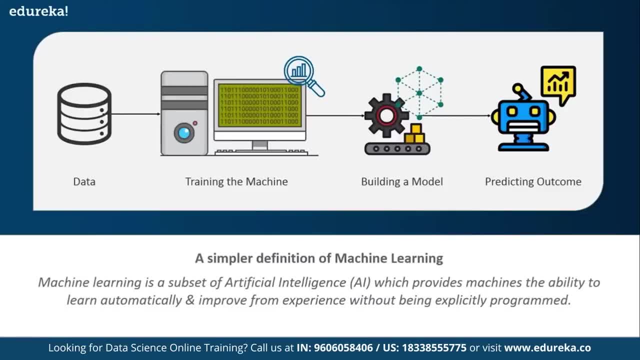 and trends. now, these insights are then used to build a machine learning model by using an algorithm in order to solve a problem. okay, so basically, you're going to feed a lot of data to the machine. The machine is gonna get trained by using this data, It's going to use this data and it's gonna draw. 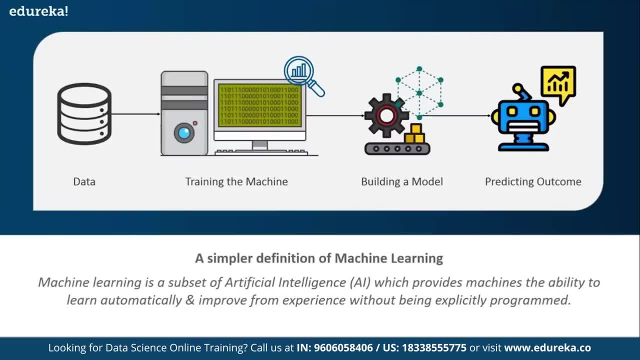 useful insights and patterns from it, And then it's going to build a model by using machine learning algorithms. Now this model will help you predict the outcome or help you solve any complex problem or any business problem. So that's a simple explanation of how machine learning works. 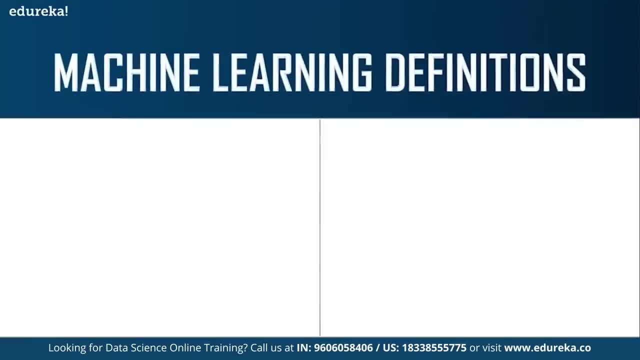 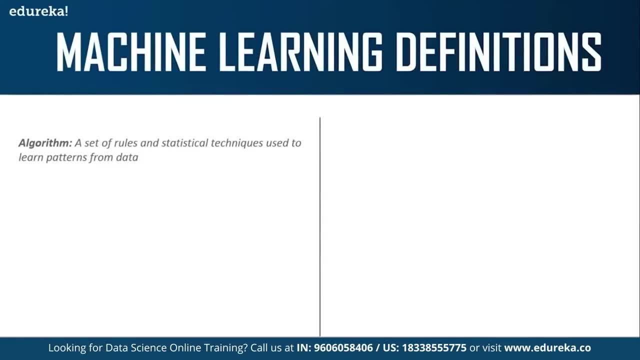 Now let's move on and look at some of the most commonly used machine learning terms. So first of all, we have algorithm. Now this is quite self-explanatory. Basically, algorithm is a set of rules or statistical techniques which are used to learn patterns from data. 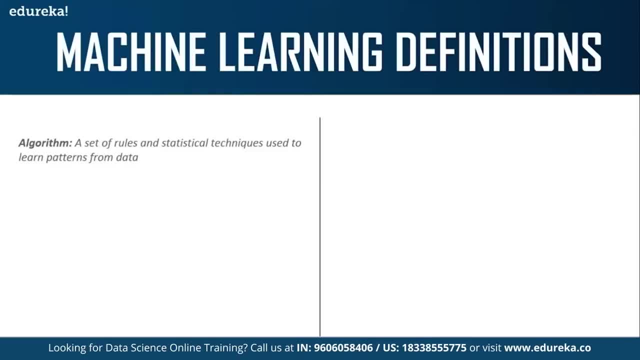 Now, an algorithm is the logic behind a machine learning model. all right, An example of a machine learning algorithm is linear regression. I'm not sure how many of you have heard of linear regression. It's the most simple and basic machine learning algorithm. 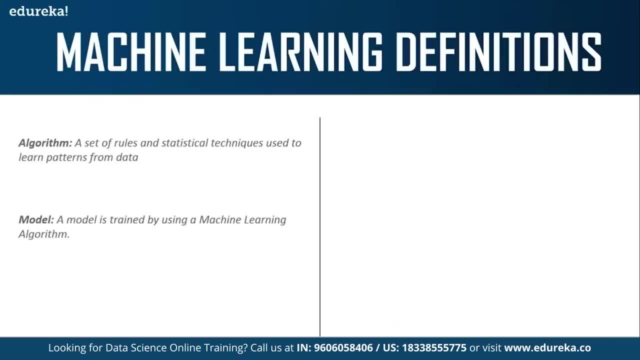 All right, next we have model. Now model is the main component of machine learning. all right, So model will basically map the input to your output by using the machine learning algorithm and by using the data that you're feeding the machine. So basically, the model is a representation. 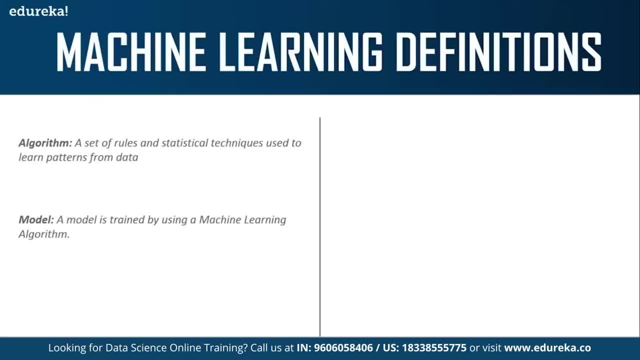 of the entire machine learning process. So the model is basically fed input, which is a lot of data, and then it will output a particular result or a particular outcome by using machine learning algorithms. Next, we have something known as predictor variable. Now, predictor variable is a function of machine learning. 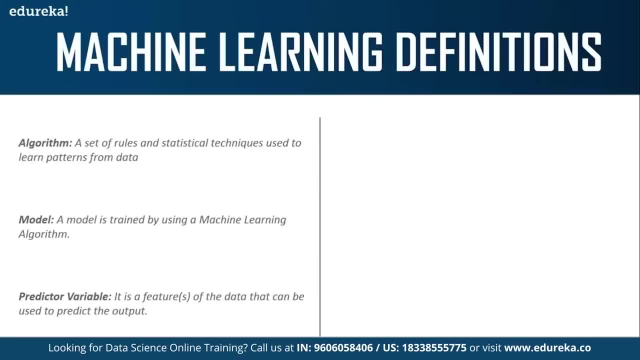 Now, predictor variable is a feature of the data that can be used to predict the output. So, for example, let's say that you're trying to predict the weight of a person depending on the person's height and their age. all right, So over here, the predictor variables. 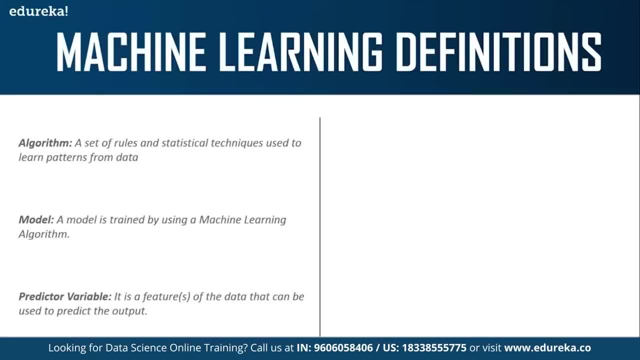 are your height and your age, because you're using height and age of a person to predict the person's weight, all right. So the height and the age are the predictor variables Now. weight, on the other hand, is the response or the target variable. 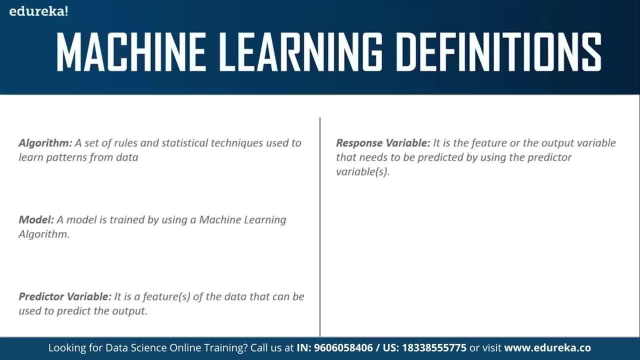 So response variable is a feature or the output variable that needs to be predicted by using the predictor variables. all right, After that we have something known as training data. So, guys, the data that is fed to a machine learning model is always split into two parts. 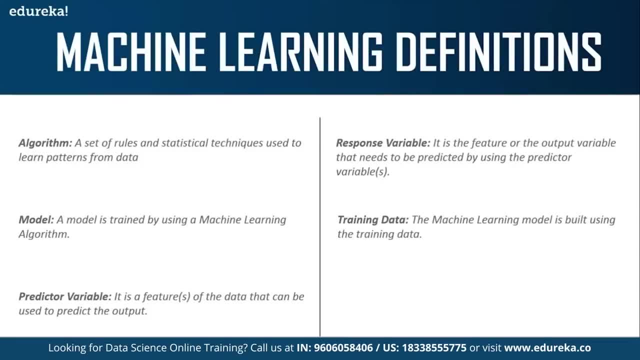 First we have the training data and then we have the testing data. Now training data is basically used to build the machine learning model. So usually training data is much larger than the testing data because obviously if you're trying to train the machine, then you're gonna feed it a lot more data. 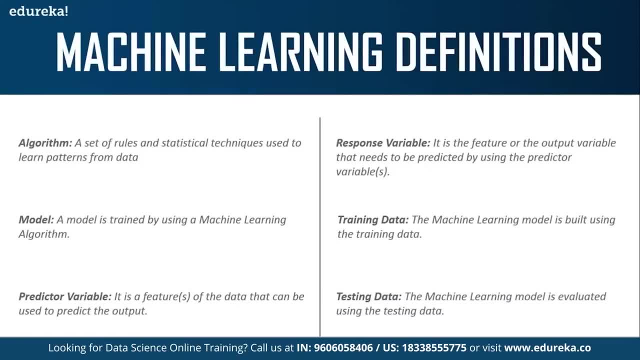 Testing data is just used to validate and evaluate the efficiency of the model. all right, So that was training data and testing data. So, guys, these were a few terms that I thought you should know before we move any further. Okay, now let's move on. 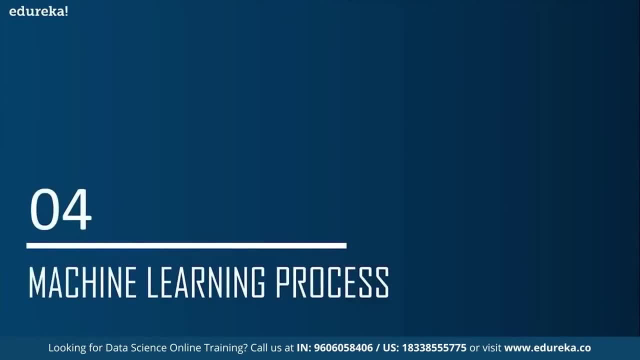 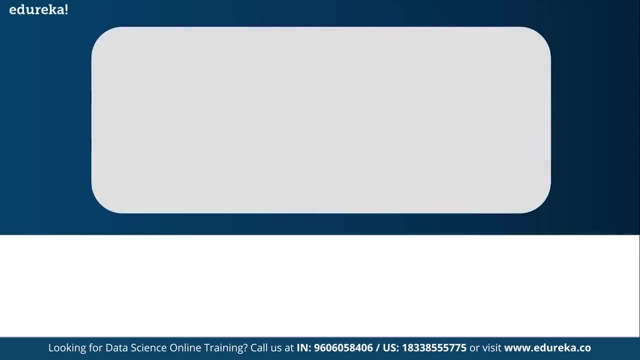 and discuss the machine learning process. Now this is gonna get very interesting because I'm gonna give you an example and make you understand how the machine learning process works. So, first of all, let's define the difference between the different stages or the different steps involved. 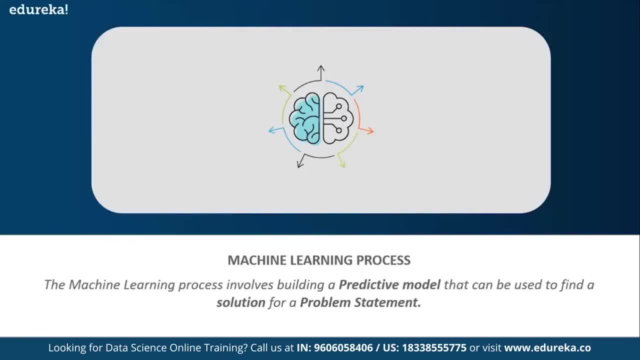 in the machine learning process. So a machine learning process always begins with defining the objective, or defining the problem that you're trying to solve. Next stage is data gathering, or data collection. Now the data that you need to solve this problem is collected at this stage. 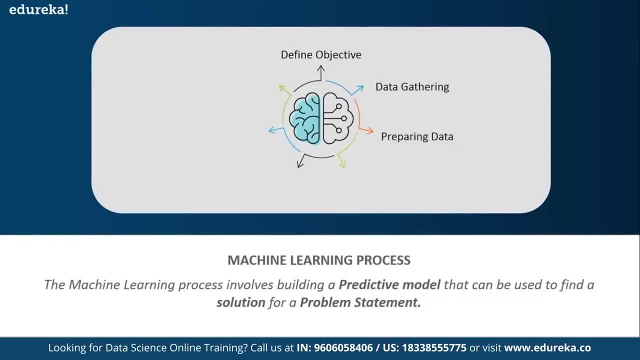 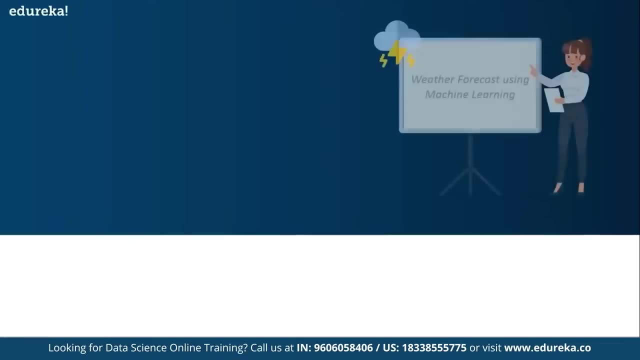 This is followed by data preparation or data processing. After that, you have data exploration and analysis, And the next stage is building a machine learning model. This is followed by model evaluation And finally you have prediction, or your output. Now let's try to understand. 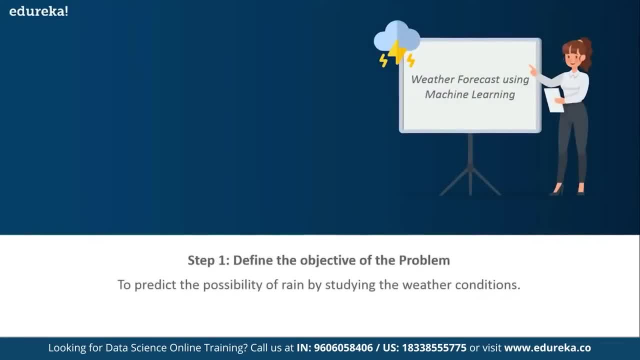 this entire process with an example. So our problem statement here is to predict the possibility of rain by studying the weather conditions. So let's say that you're given a problem statement and you're asked to use a machine learning process to solve this problem statement. 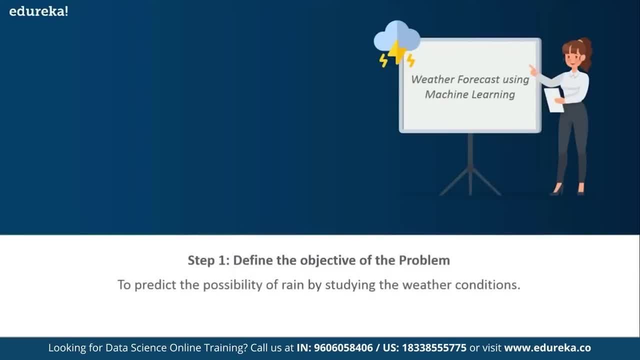 So let's get started. all right. So the first step is to define the objective of the problem statement. Our objective here is to predict the possibility of rain by studying the weather conditions. Now, in the first stage of a machine learning process, you must understand what exactly needs to be predicted. 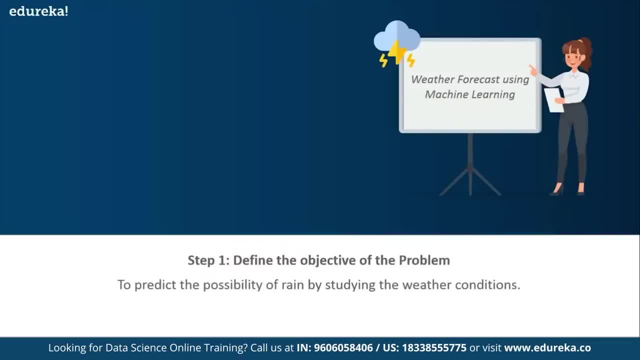 Now. in our case, the objective is to predict the possibility of rain by studying weather conditions, So at this stage, it is also essential to take mental notes on what kind of data can be used to solve this problem or the type of approach that you can follow. 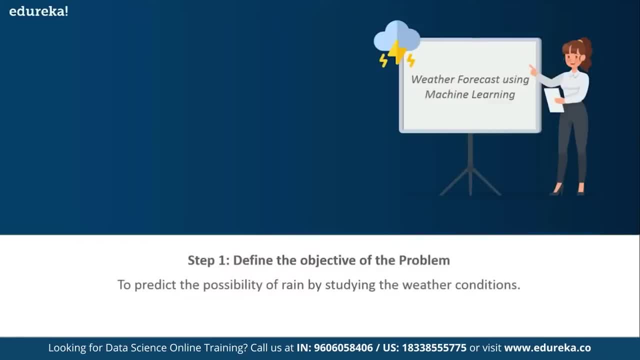 to get to the solution. A few questions that are worth asking during this stage is: what are we trying to predict, What are the target features or what are the predictor variables? What kind of input data do we need And what kind of problem are we facing? 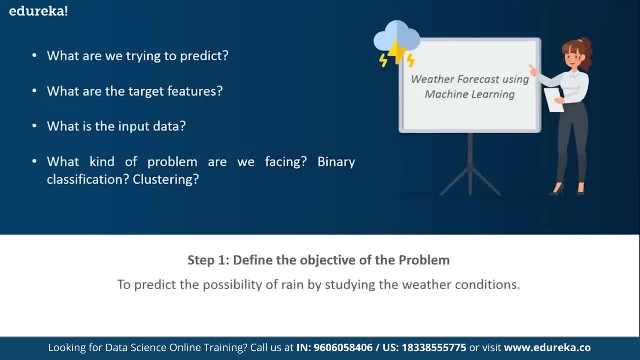 Is it a binary classification problem or is it a clustering problem? Now, don't worry, if you don't know what classification and clustering is, I'll be explaining this in the upcoming slides. So, guys, this was the first step of a machine learning process. 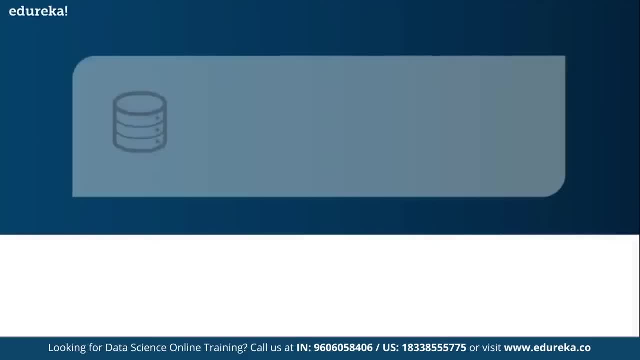 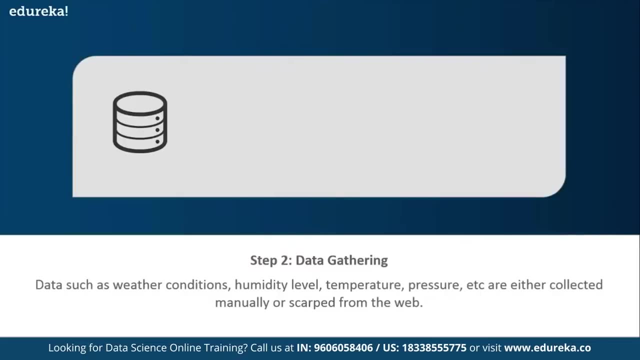 which is define the objective of the problem. All right, Let's move on and look at step number two. So step number two is basically data collection, or data gathering. Now, at this stage, you must be asking questions such as what kind of data is needed to solve the problem? 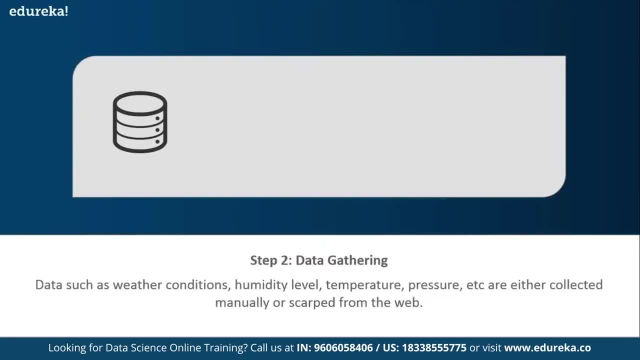 Is the data available And if it is available, how can I get the data? Okay, So once you know the type of data that is required, you must understand how you can derive this data. Data collection can be done manually or by web scraping. 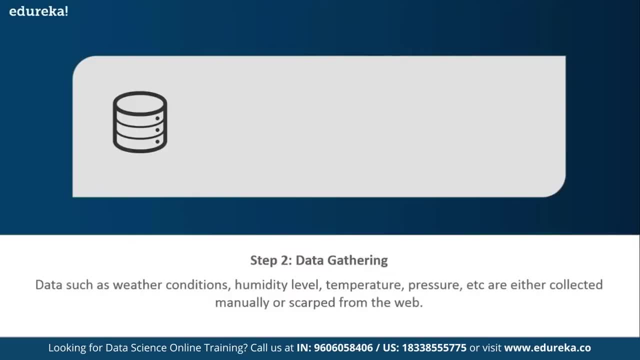 But if you're a beginner and you're just looking to learn machine learning, you don't have to worry about getting the data okay. There are thousands of data resources on the web. You can just go ahead and download the data sets from websites such as Kaggle, okay. 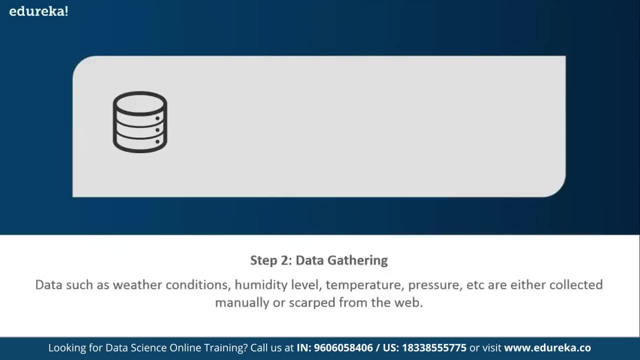 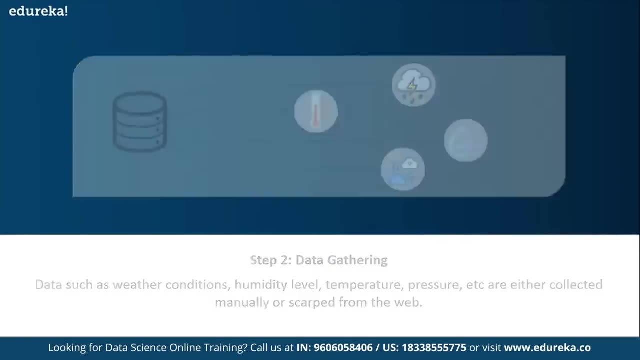 Now coming back to the problem at hand. the data needed for weather forecasting includes measures such as humidity level, temperature pressure, locality, whether or not you live in a hill station, and so on. So, guys, such data must be collected and stored for analysis. 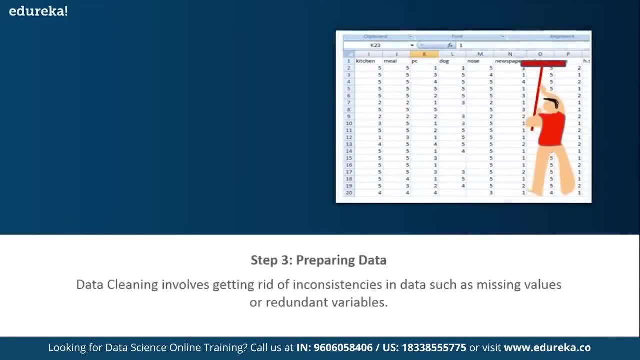 Now the next stage in machine learning is preparing your data. The data you collected is almost never in the right format, So basically, you'll encounter a lot of inconsistencies in the data set. Okay, this includes missing values, redundant variables, duplicate values and so on. 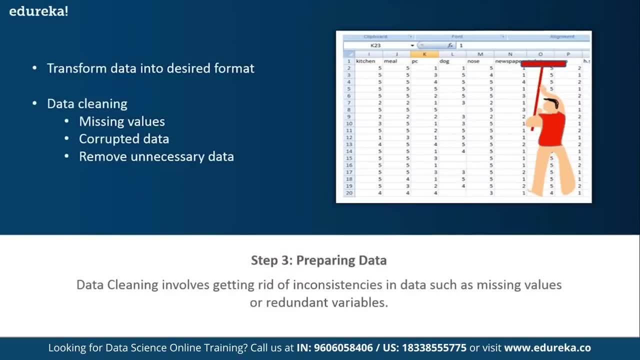 Removing such values is very important because they might lead to wrongful computations and predictions. So that's why, at this stage, you must scan the entire data set for any inconsistencies, and you have to fix them at this stage. Now the next step is exploratory data analysis. 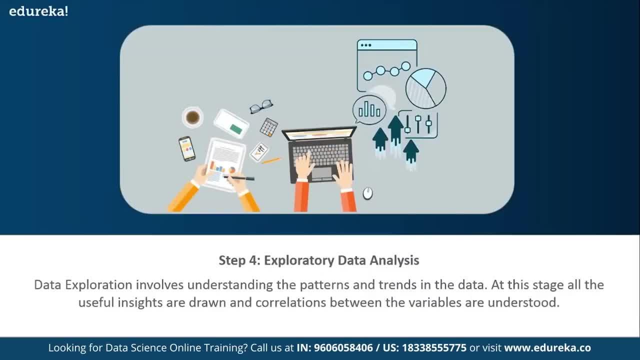 Now, data analysis is all about diving deep into data and finding all the hidden data mysteries. Okay, this is where you become a detective. So EDA, or exploratory data analysis, is like the brainstorming of machine learning. Data exploration involves understanding the patterns. 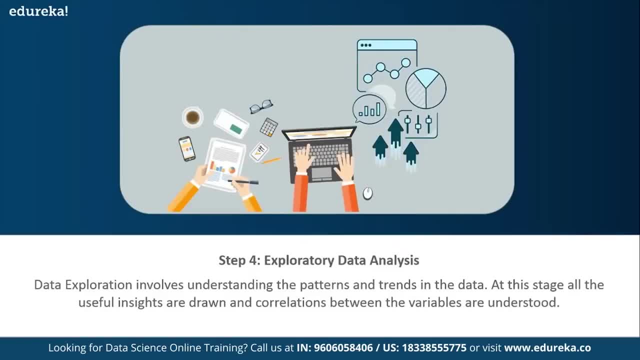 and the trends in your data. So at this stage, all the useful insights are drawn and all the correlations between the variables are now included, understood. so you might ask: what sort of correlations are you talking about? for example, in the case of predicting rainfall, we know that there is a strong 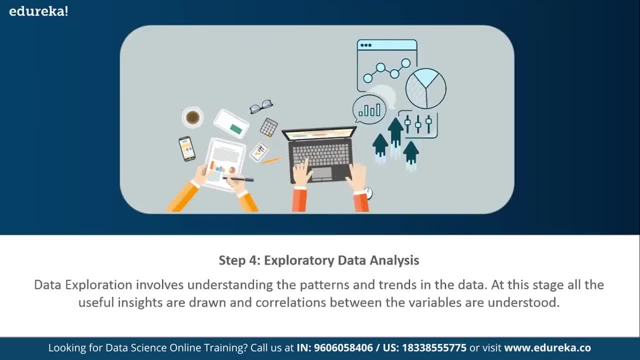 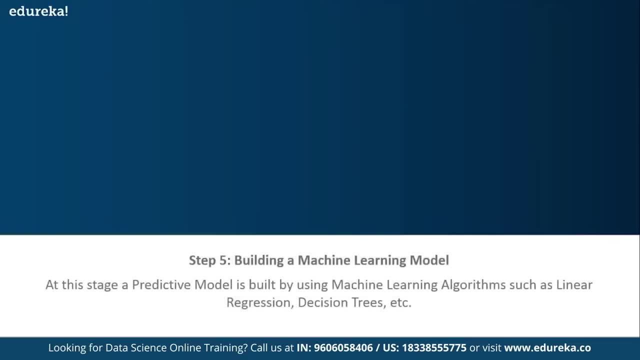 possibility of rain if the temperature has fallen low. okay, so such correlations have to be understood and mapped at this stage. now, this stage is followed by stage number five, which is building a machine learning model, so all the insights and the patterns that you derive during data exploration are used. 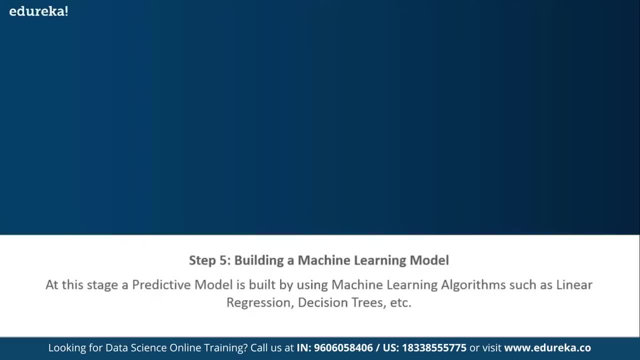 to build the machine learning model. so this stage always begins by splitting the data set into two parts: training data and the testing data. so earlier in this session I already told you what training and testing data is. now the training data will be used to build and analyze the model and the logic of the 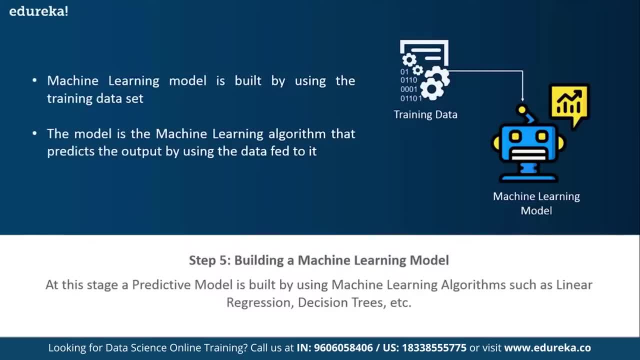 model will be based on the machine learning algorithm that is being implemented. okay, now in the case of predicting rainfall, since the output will be in the form of true or false, we can use a classification algorithm to predict the rainfall and we can also use the classification algorithm to predict the rainfall, and we can also use the classification. 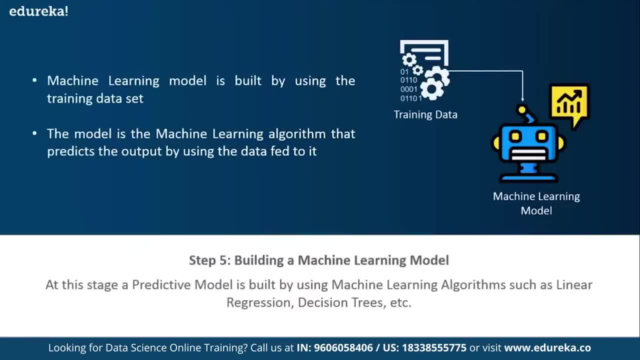 algorithm like logistic regression. Now, choosing the right algorithm depends on the type of problem you're trying to solve, the data set you have and the level of complexity of the problem. So in the upcoming sections we'll be discussing different types of problems. 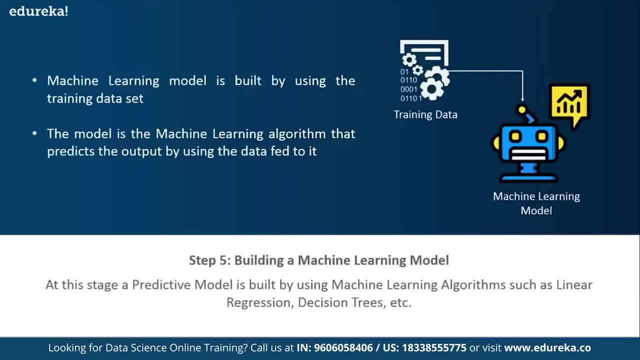 that can be solved by using machine learning. So don't worry. if you don't know what classification algorithm is and what logistic regression is okay. So all you need to know is, at this stage, you'll be building a machine learning model by using machine learning algorithm. 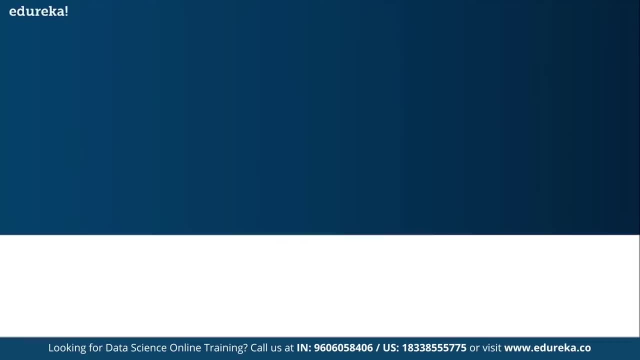 and by using the training data set. The next step in a machine learning process is model evaluation and optimization. So, after building a model by using the training data set, it is finally time to put the model to a test. okay, So the testing data set is used to check the efficiency. 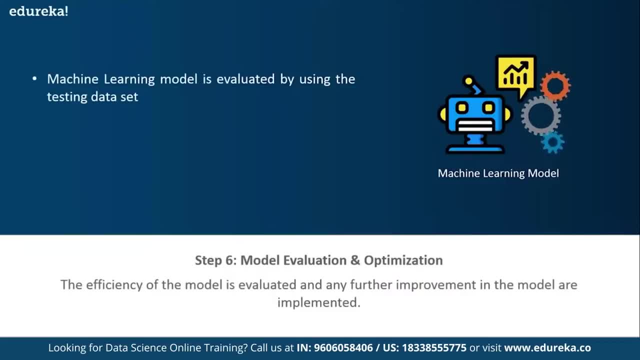 of the model and how accurately it can predict the outcome. So, once you calculate the accuracy, any improvements in the model have to be implemented in this stage. okay, So methods like parameters, data tuning and cross-validation can be used to improve the performance of the model. 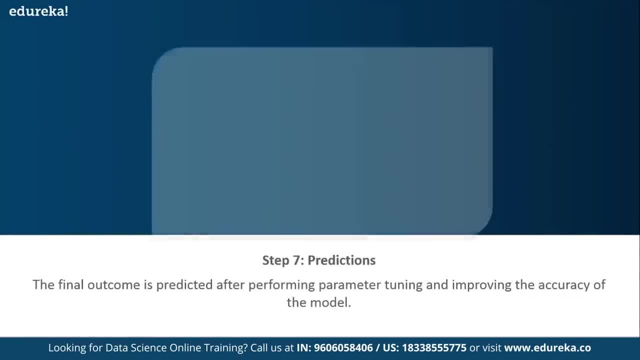 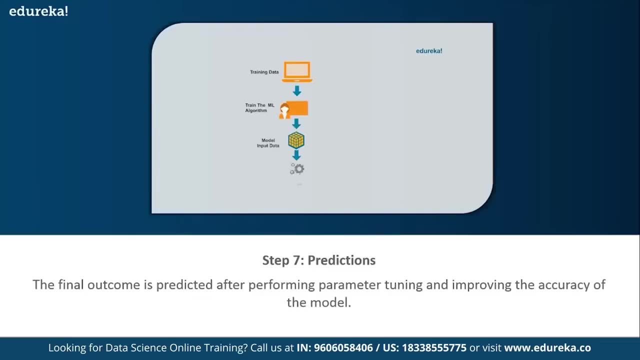 This is followed by the last stage, which is predictions. So once the model is evaluated and improved, it is finally used to make predictions. The final output can be a categorical variable or it can be a continuous quantity, In our case for predicting the occurrence of rainfall. 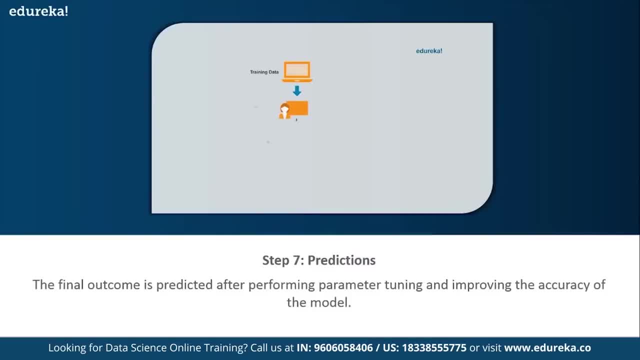 the output will be a categorical variable, In the sense our output will be in the form of true or false, yes or no. Yes basically represents that it's going to rain, and no will represent that no, it won't rain okay. 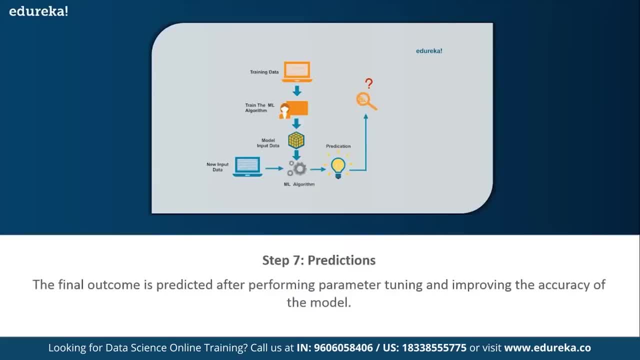 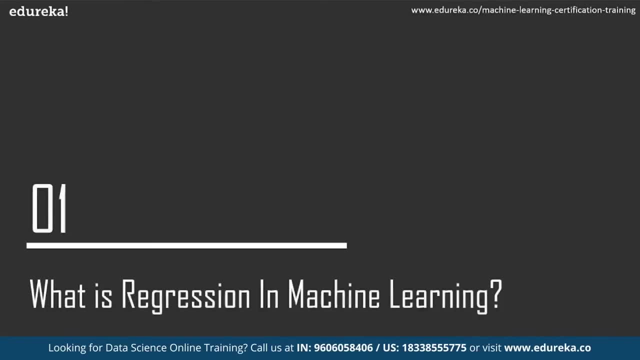 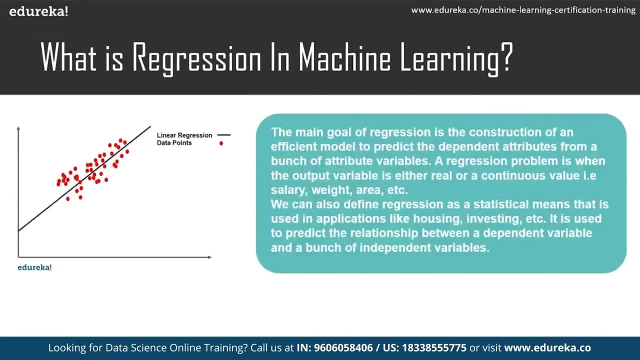 As simple as that. So, guys, that was the entire machine learning process. Now, without wasting any more time, let us understand what regression in machine learning is. So what exactly is regression? The main goal of regression is the construction of an efficient model to predict the dependent attributes. 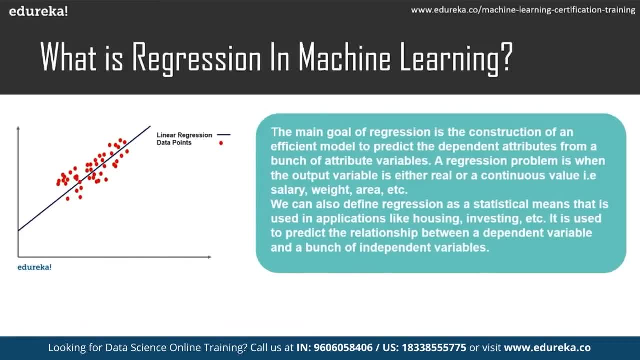 from a bunch of attribute variables. Regression problem is where the output variable is either real or a continuous value, like salary, weight area, Etc. We can also define regression as a statistical means that is used in applications like housing investing, Etc, to predict the relationship. 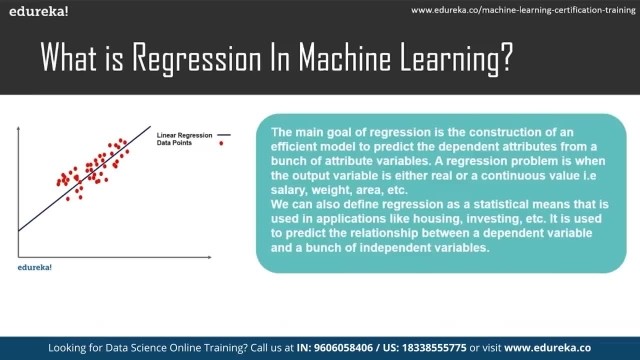 between a dependent variable and a bunch of independent variables. For example, let's say, in the finance application or investing, we can actually predict the values of certain stock prices, or you know those values depending on the independent variables, like how many years it takes. 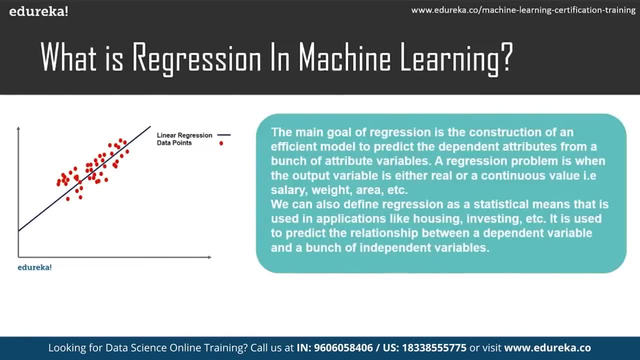 For a stock to you know actually mature, or how many days will it take to grow, or those variables that you have in investing, and depending upon that we can make a possible outcome or a possible prediction of how our stock is going to be invested in a profit state or a loss state. 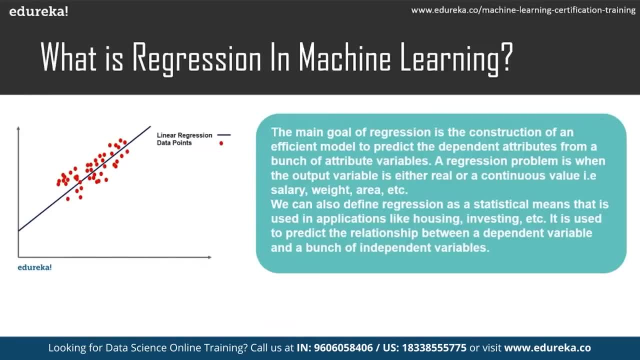 or all those things. or we can take another example like housing. we can take different parameters like number of years It's been there, how many people have used it or what is the area of the house. depending on all these factors, or how many rooms to the house have, we can predict. 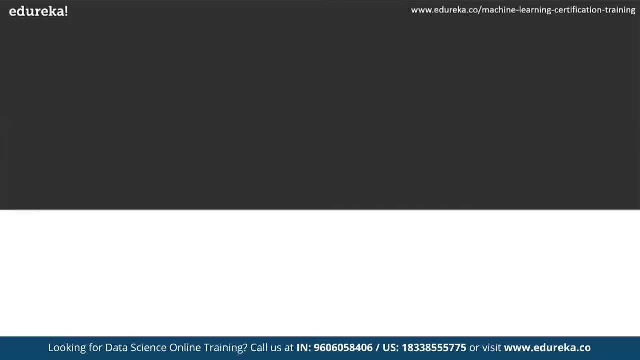 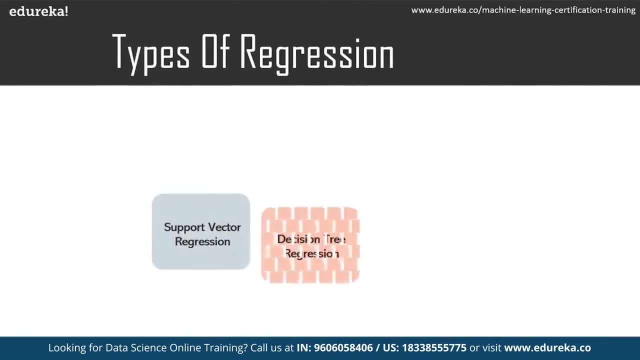 What is the price of a house. So this is basically what regression really is. So let us take a look at a various types of regression techniques that we have. We have simple linear regression. when we have polynomial regression, support vector regression, decision to regression. 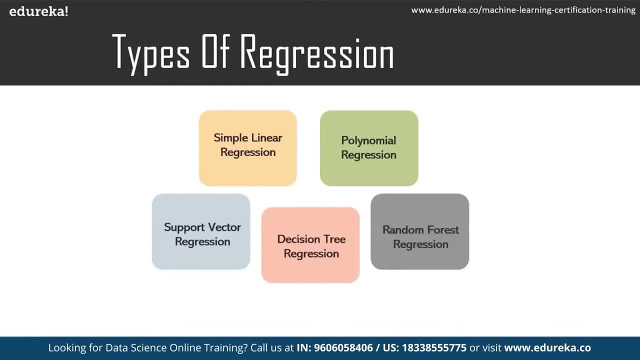 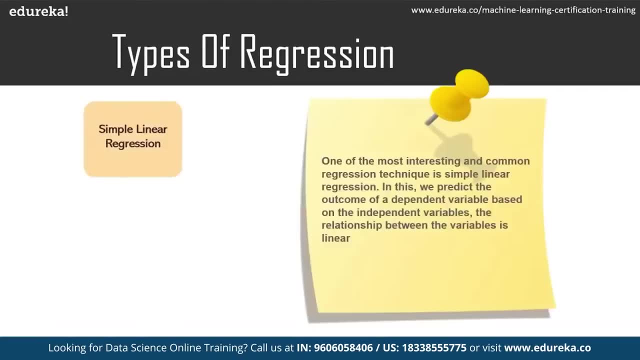 We have random forest regression and we have logistic regression as well. That is also a type of regression that we have, but for now we'll be focusing on simple linear regression. So let's talk about how or what exactly. simple linear regression first. So one of the most interesting. 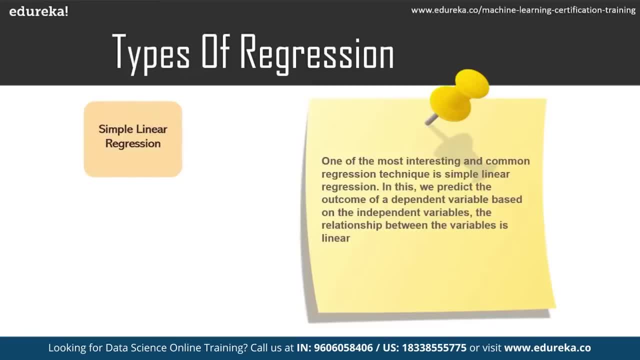 and common regression technique is a simple linear regression and this way predict the outcome of a dependent variable Y based on the independent variables X. So the relationship between the variables is linear, Hence the word linear regression. then comes the polynomial regression. So in this regression technique, 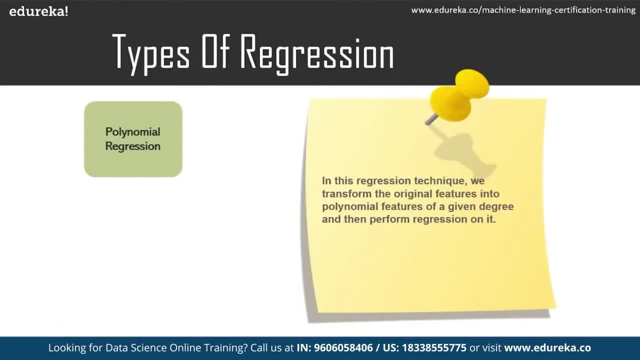 we transform the original features into a polynomial feature of a given degree and then perform regression on it. So this is basically polynomial regression. after this We have support vector machine regression, or we can also call it SVR. We identify a hyperplane with maximum margin, such 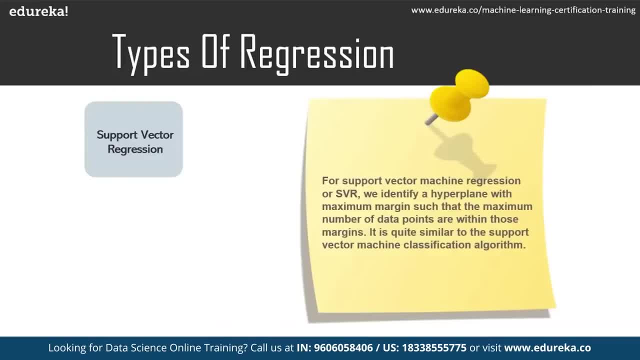 that the maximum number of data points are within those margins. It is also quite similar to the support vector machine classification algorithm. Then we have decision tree regression. a decision tree can be used for both regression and classification, But in this case of regression we use the ID three algorithm. 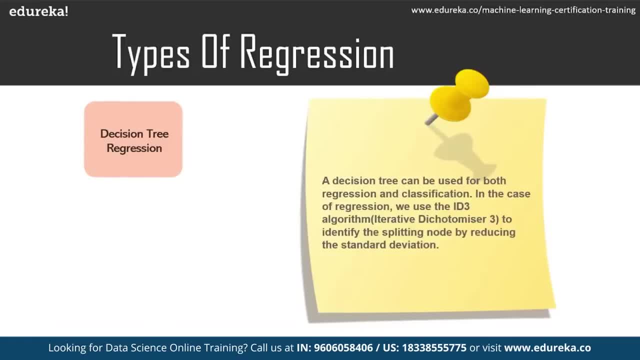 which is iterative dichotomizer three, to identify the splitting node by reducing the standard deviation. after this we have a random forest regression which is basically an ensemble of predictions of several decision tree regressions. So this is all about the types of regressions for now. 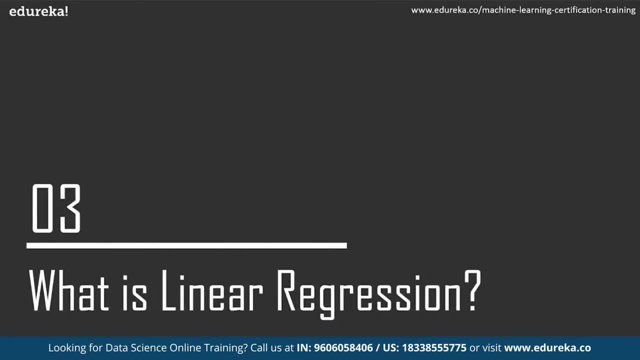 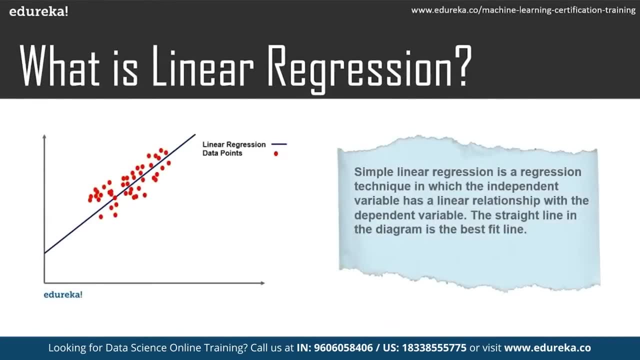 We are going to focus on simple linear regression. So let's take a look at what exactly is the simple linear regression. simple linear regression is a regression technique in which the independent variable has a linear relationship with the dependent variable. straight line in the diagram is the best fit line. 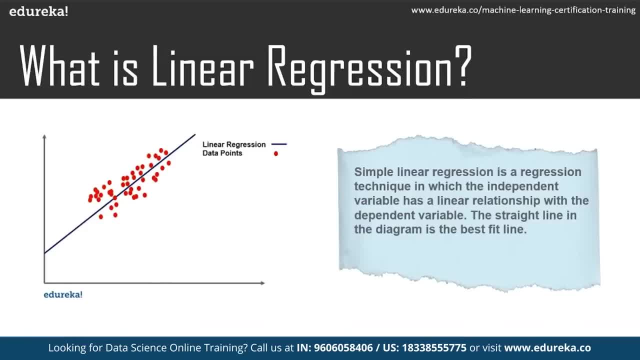 and the main goal of the simple linear regression is to consider the given data points and plot the best fit line For the model in the best way possible. So if you talk about a real-life analogy to explain linear regression, we can take an example of a car resale value. 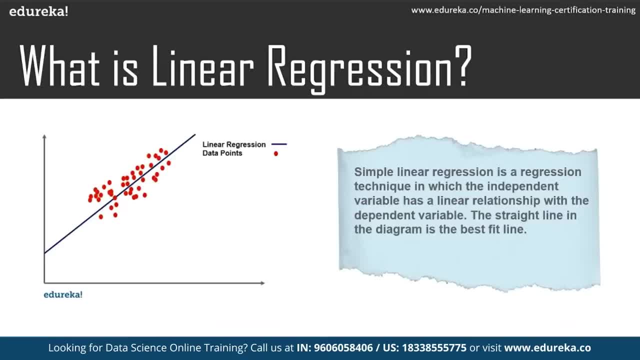 So we have different parameters. you know, when we are talking about a resale value of a car, like how many years the car has been there in the market and how many kilometers it has been written, the kind of mileage the car gives, and then we have different parameters we can focus upon. 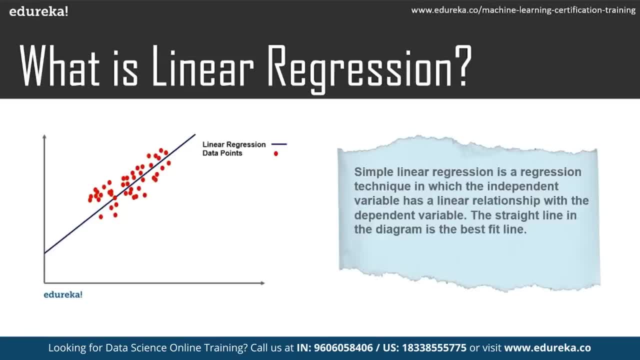 and all these independent variables somehow are linearly connected or interconnected to the price of the car. So that is one example to understand linear regression. We'll be doing that in the use case. I'll be telling you about how you can predict the price of car. 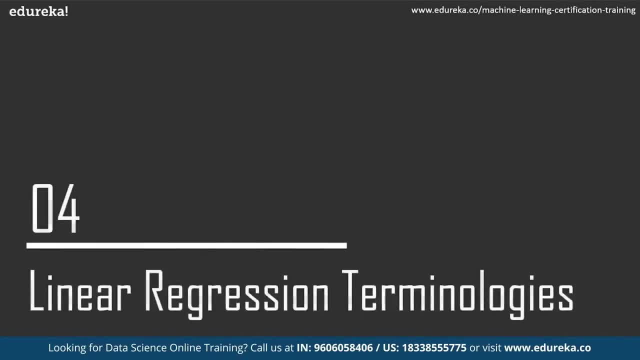 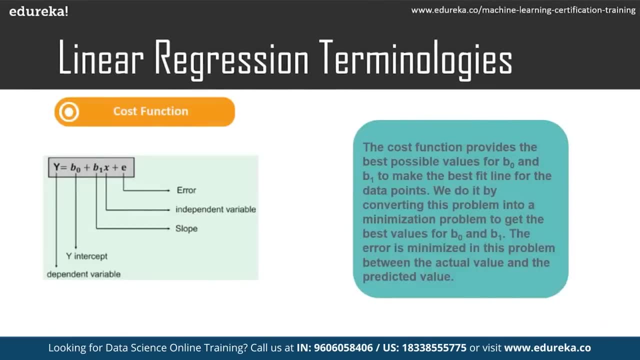 now talking about linear regression terminologies. There are a few terminologies They had you have to be thorough with to begin with, linear regression. So first of all we have talked about cost function, So the best fit line can be based on the linear equation that is given here. 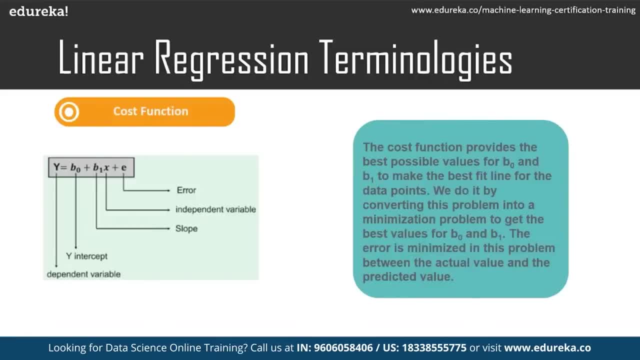 So in this the dependent variable that is to be predicted is denoted by Y. a line that touches the y-axis is denoted by the intercept B 0, the B 1 is the slope of the line and X represents the independent variables that determine the prediction of Y. the error. 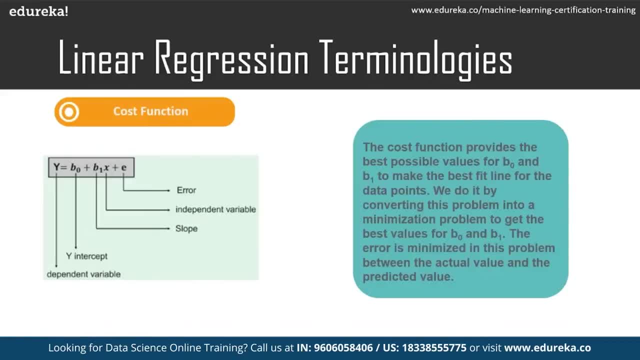 in the resultant prediction is denoted by E, not talking about cost function. the cost function provides the best possible values for B 0 and B 1 to make the best fit line for the data points. We do this by converting this problem into a minimization problem to get the best values for B 0. 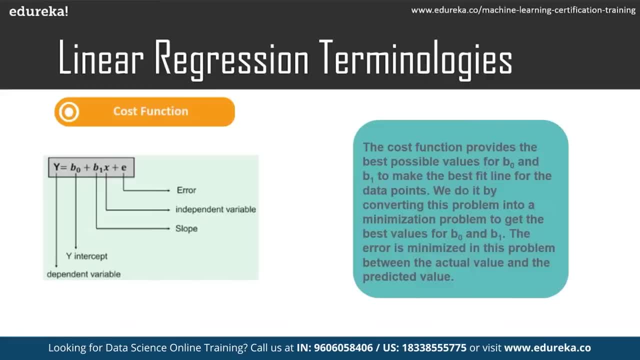 and B 1. so with this the error is minimized in this problem between the actual value and the predicted value and we choose the function to above to minimize. now we square the error difference and some the error over all the data points, the division between the total number of data points. 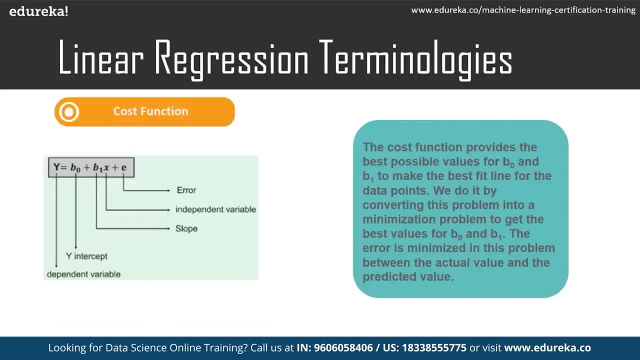 and the produced value provides the average square error for all the data points. It is also known as mean squared error and we can change the values of B 0 and B 1 so that the MSE or the mean squared error value is settled at the minimum. 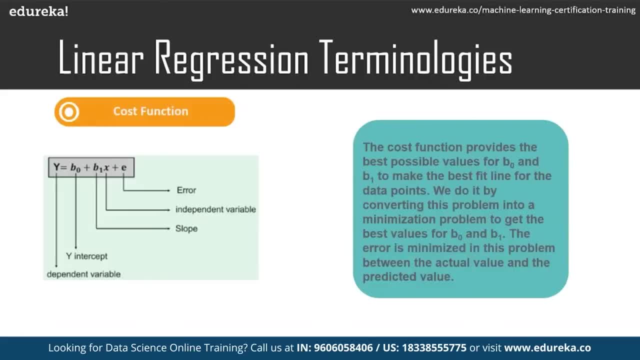 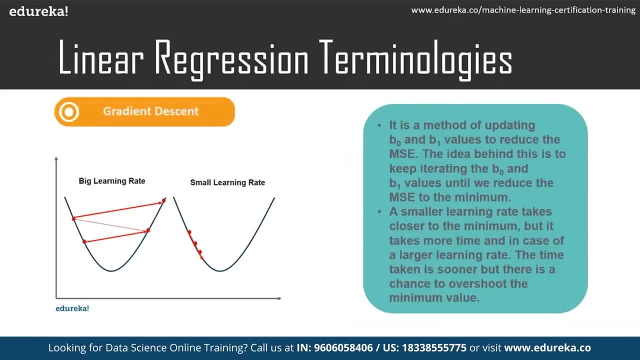 So this is one terminology that is cost function that we use in linear regression. Then we have the grade and descent. so the next important terminology to understand linear regression is gradient descent, of course, and it is a method of updating B 0 and B 1 value to reduce the MSE. 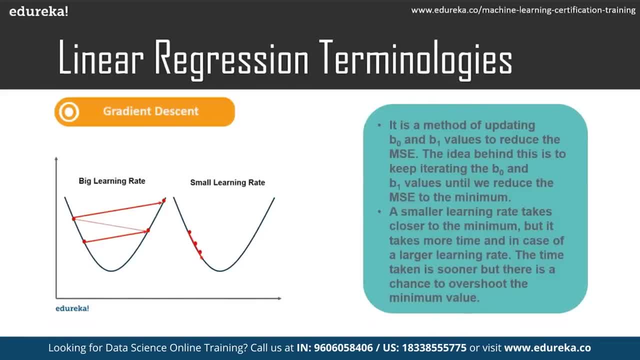 which is the mean squared error. The idea behind this is to keep iterating the B 0 and B 1 values until we reduce the MSE to the minimum. now to update B 0 and B 1. We take the gradient from the cost function. 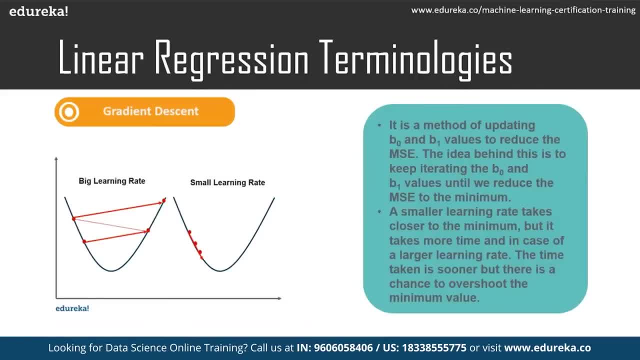 and to find these gradients, We take partial derivatives with respect to B 0 and B 1 and these partial derivatives are the gradient and are used to update the values of B 0 and B 1.. I'm sure that this is might be a little confusing for you guys. 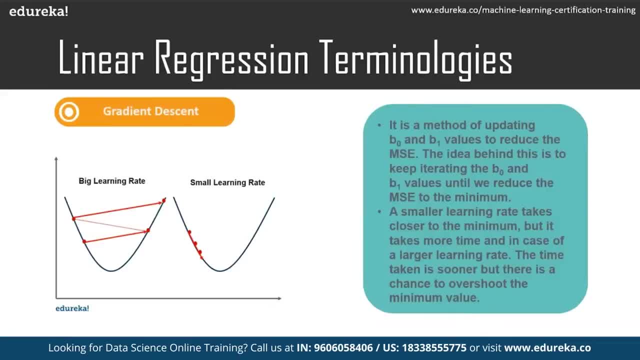 If you are new to this- the gradient, descent and cost function. but you don't have to worry about this, because in Python, when we're using a linear regression, we're going to be using the sklearn or the scikit-learn library, So you don't have to worry about this. 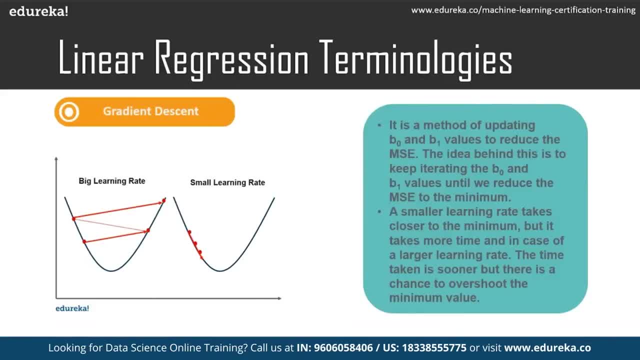 You just have to integrate your model with the linear regression model that we have already over there and you will be down with, and when I'm implementing the linear regression model, you'll see how easy it is to actually implement linear Regression invite. So after this, let's talk about a few advantages. 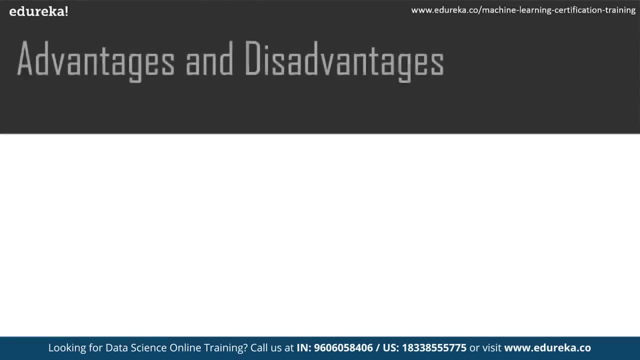 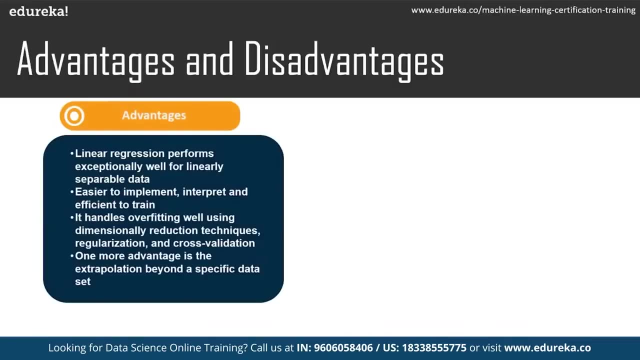 and disadvantages of linear regression. So talking about the advantages, first, linear regression performs exceptionally well for linearly separable data and it is actually very easy to implement, interpret and very efficient to train as well. And even though the linear regression is prone to overfitting, 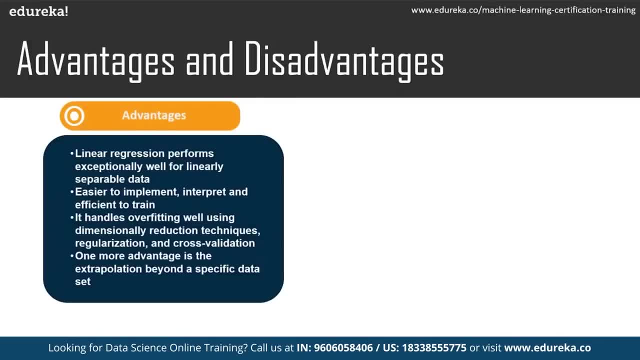 it handles it pretty well using dimensionally reduction techniques, regularization and cross validation, and one more advantage is that the extra population beyond a specific data set. So these are all the advantages that we have with linear regression. Let's talk about a few disadvantages as well. 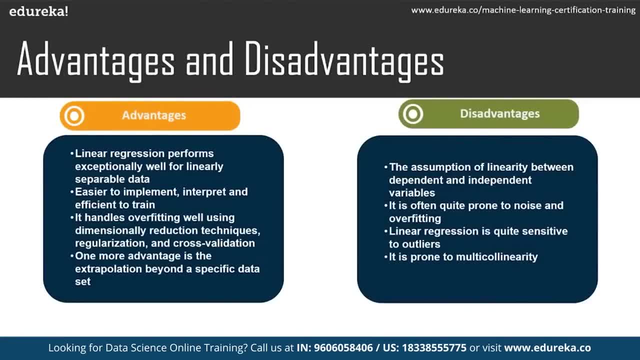 So one of the most common disadvantage with linear regression is that it takes the assumption of linearity between dependent and independent variables. The next disadvantage is it is often very prone to noise and overfitting as well, which is not a very good sign for any model. 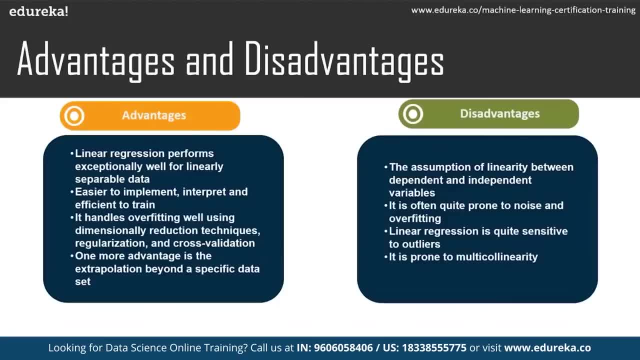 If you are doing regression or classification in machine learning. the next disadvantages: It is very, quite sensitive to outliers as well, And the last one is that it is very prone to multicollinearity. So these are all the advantages and disadvantages of linear regression. 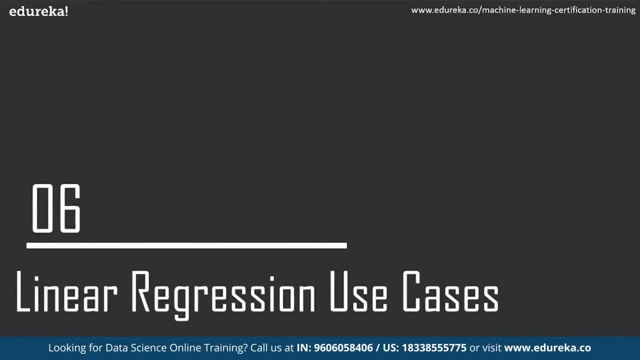 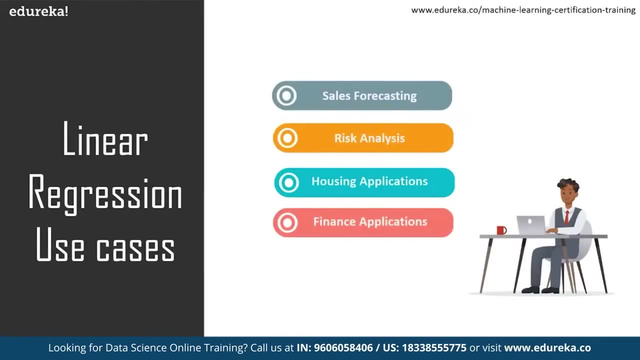 Now let's also take a look at a few use cases that we can use linear regression for. so we can use it for sales forecasting depending upon the features, like we can actually predict the price of a item or, in sales, We can forecast the price. 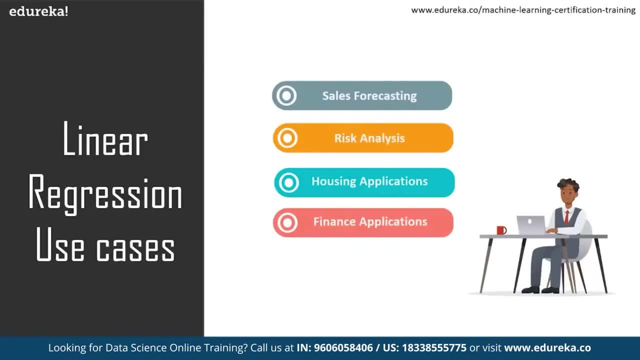 or make assumptions over there, like predictions. obviously, then we can use it for risk analysis, for disease predictions, Like we can take our disease data set and, depending upon several features that are linearly connected with one risk detection, We can use it for risk analysis as well. 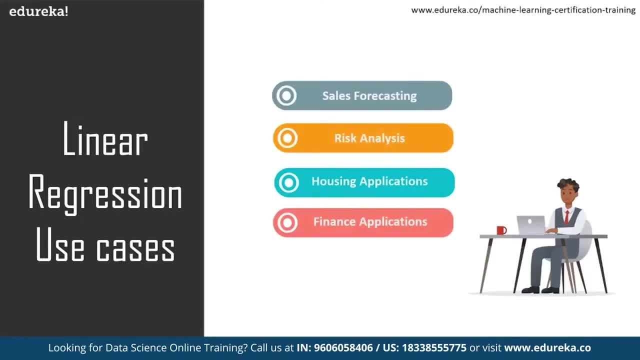 We can obviously use it for housing applications to predict the prices and other factors, like what are the different aspects that are going to be decisive in the price of a house, all those features using the linear regression. and then, of course, we can use it for finance applications. 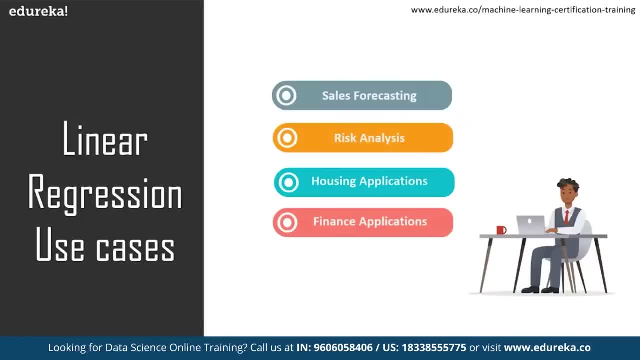 to predict the stock prices, investment evaluation, etc. The basic idea behind linear regression is to find the relationship between the dependent and independent variables to get the best fitting line that would predict the outcome with the least error. So we can use linear regression in simple real life situations. 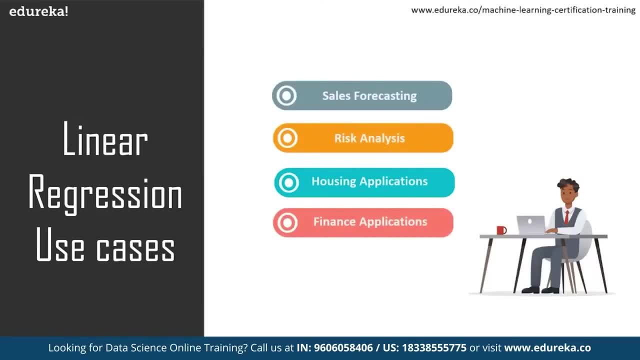 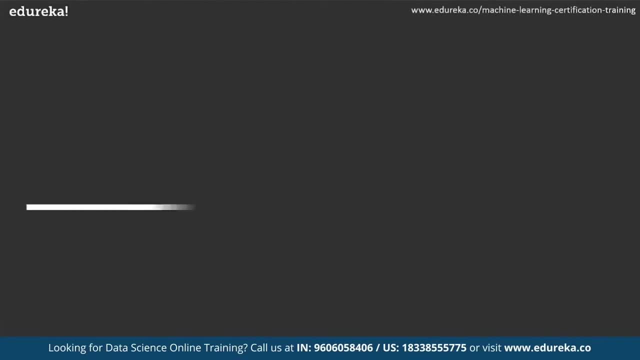 as well, like predicting the SAT scores with regard to the number of hours of study and other decisive factors that we can use it for. now that we are done with the use cases as well, Let's take a look at specific use case that I'm going to show you in sklearn. 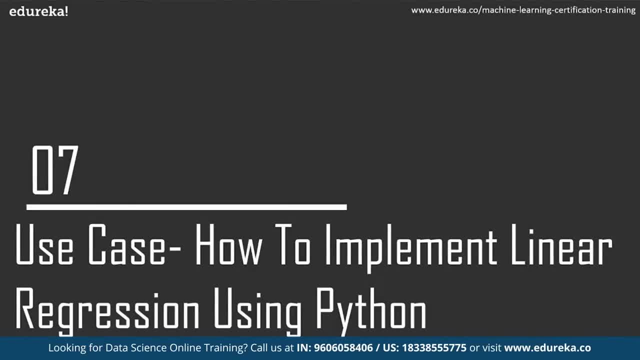 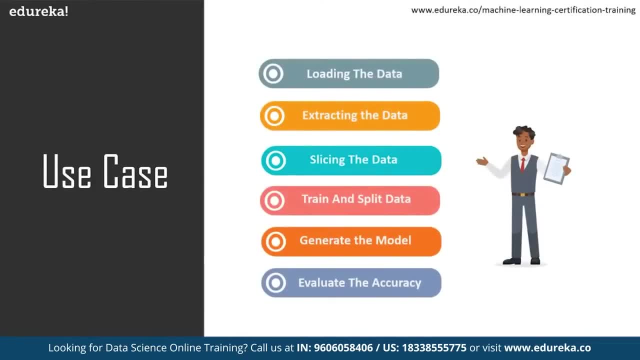 or scikit-learn library, and we're going to implement the linear regression model over there. So let me take you through the steps that are going to take place over there. So, first of all, we are going to load the data. after that, 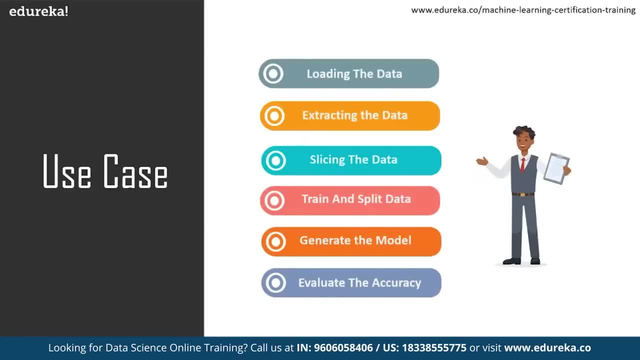 We'll explore the data, So we'll take a look at how our data is, What are the different features and what are the data points that we have in the data set of. that will slice the data according to our requirements and then we'll train and split the data using the fit. 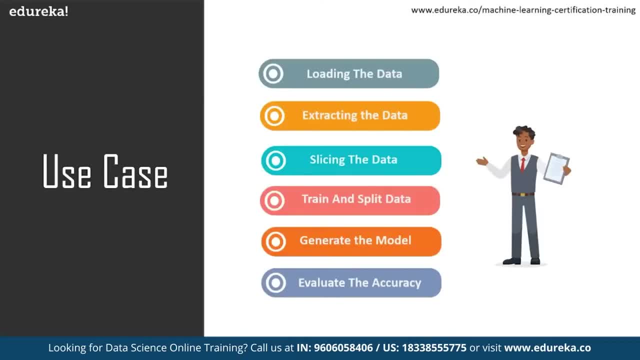 and predict method that we have in scikit-learn, and then we generate the model from scikit-learn and after we are done Taking the model, will evaluate the accuracy. So let's take it up to PyCharm guys. I'll show you a very simple example. 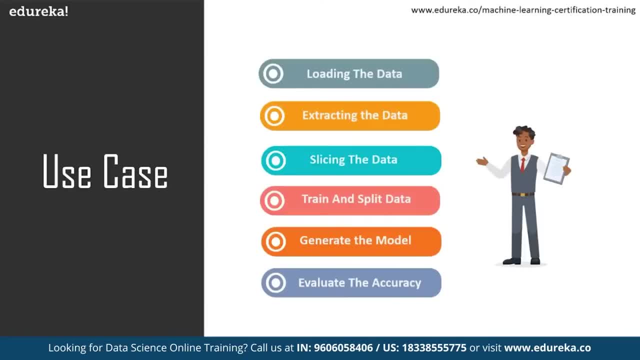 First of all, with the diabetes data set that we have in scikit-learn, we can simply import it from the data sets module that we have in scikit-learn. and after this simple example, I'm going to show you a custom data set that is a car resale value. 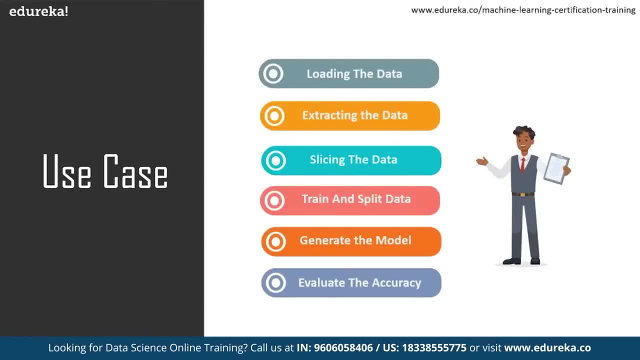 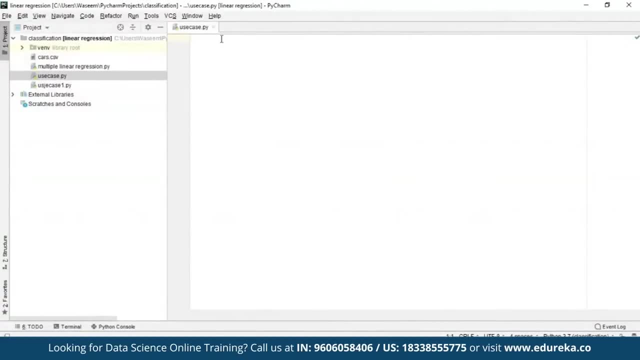 and we're going to predict some prices for car resale values. So, without wasting any more time, let's take it up to PyCharm. So now that we are in PyCharm, guys will try to implement linear regression using simple data set that we have in a skill on library. 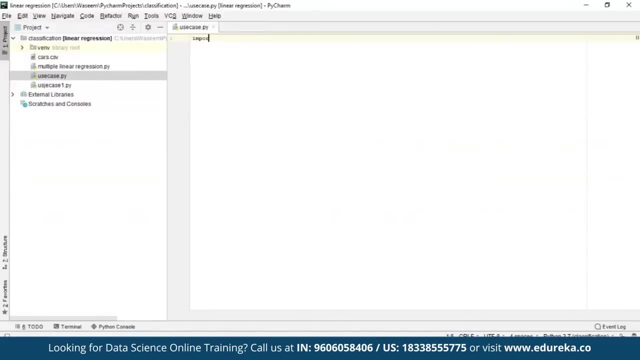 So first of all we'll have to import basic libraries like matplotlib. I'll make it a little bigger for visibility. So first I'll import matplotlib Dot by plot, as let's say PLT, and after that I'll import numpy as NP. 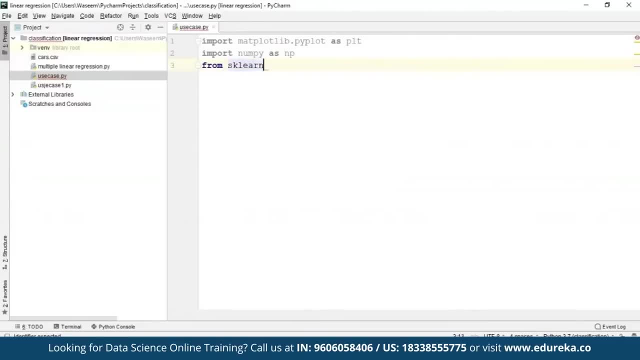 So from a skill, and we'll have to import data sets because we are going to use the data set from the data sets module And we are going to import linear model as well, for linear regression can made a mistake over here And again we have to import metrics for accuracy evaluation. 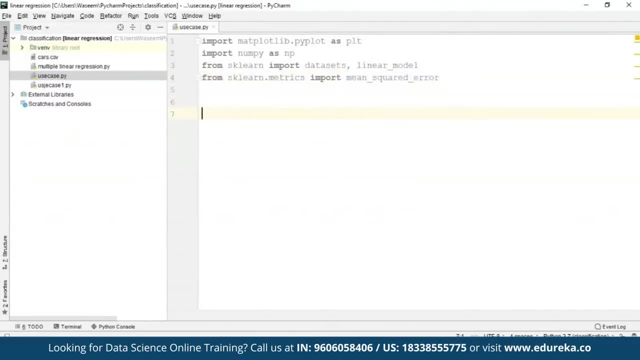 and we'll be importing mean squared error. So these are all the libraries that I'm going to use to show you how you can implement linear regression. But before that, don't make a mistake of using these libraries just as it is, because I have already installed all these libraries. 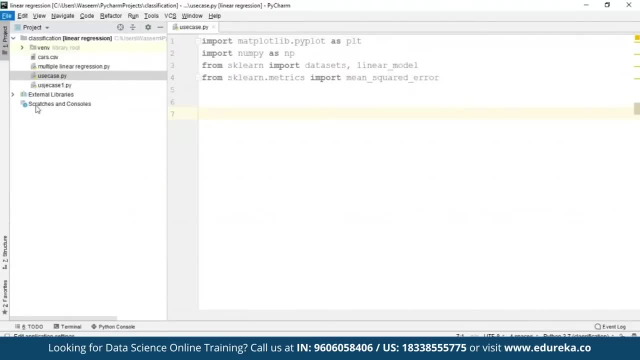 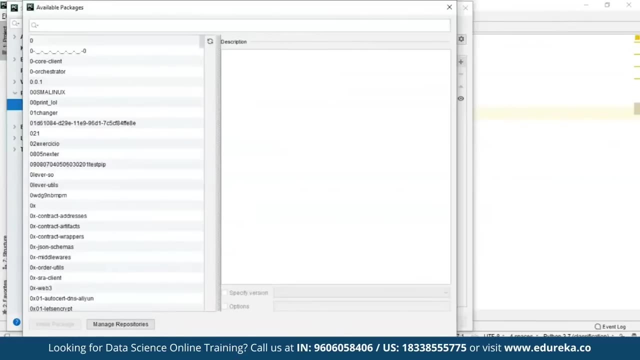 So for that you can just go to the project interpreter that you'll find in the settings, and over here you can just install all the packages that you need. So this is the add button. there You can add all the libraries that you need. So for a skill on, you can just type a skill on: 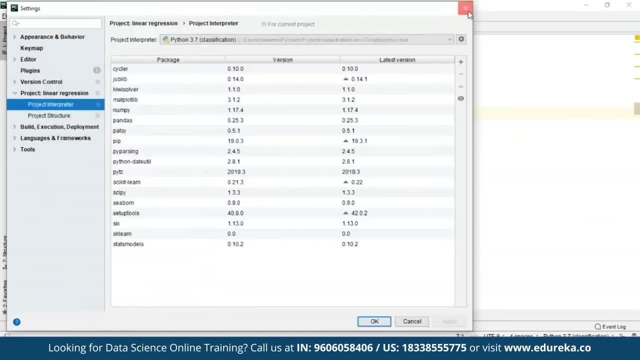 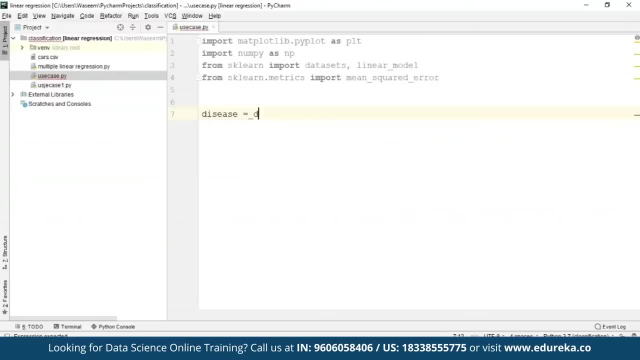 and install that library. I'm not doing that again because I've already done it. So after this, first thing that you have to do is import your data set. So for that I'm taking a variable disease and data sets: dot load data sets or I'm just going to load. 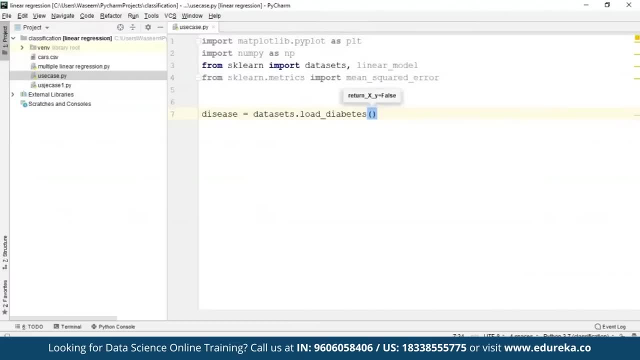 Diabetes, because that's the data set that we are going to use in this and let's just see what all we have in the data set that we have over here. So I'm just going to print this to know what all we are dealing with right now. 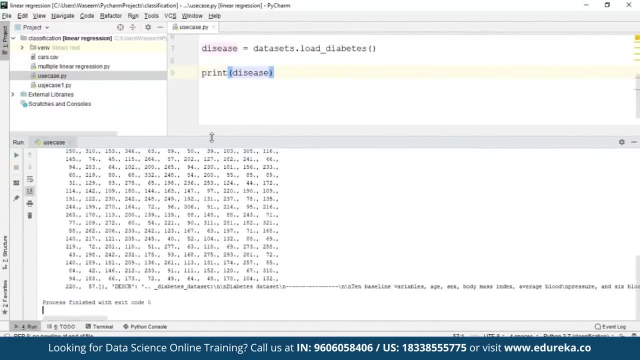 It's going to take a while. So this is our data set guys. We already have a data over here. I'm sure we'll be having a target. We have description over here. So this is our data set guys. We have a target also. 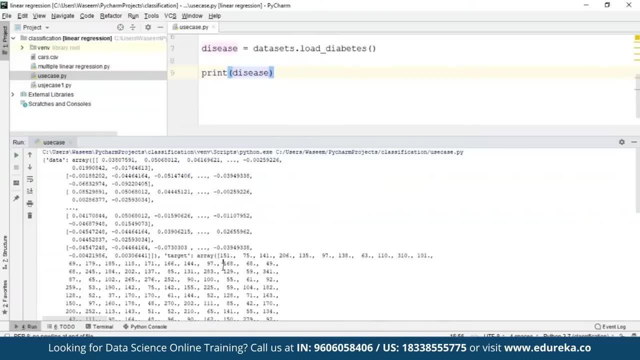 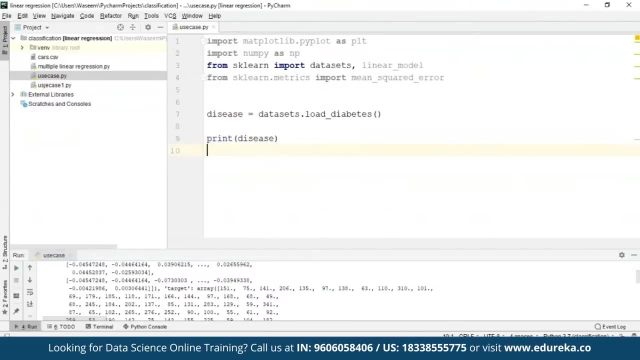 So this is a very sliced up data, which is actually pretty good for our use right now, because I'm showing you a simple implementation of linear regression. So this is going to be very easy. So what I'll do is I'll comment this line. 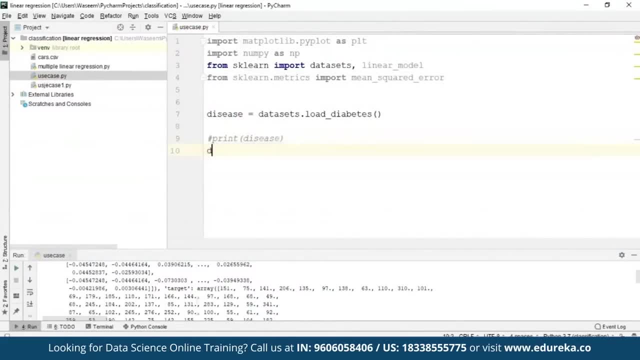 because we don't need this right now. And after this, I'll just take one more variable, as just say disease X, and inside this I am going to take disease dot data. Now, after this, I'm going to split my data into train and test. 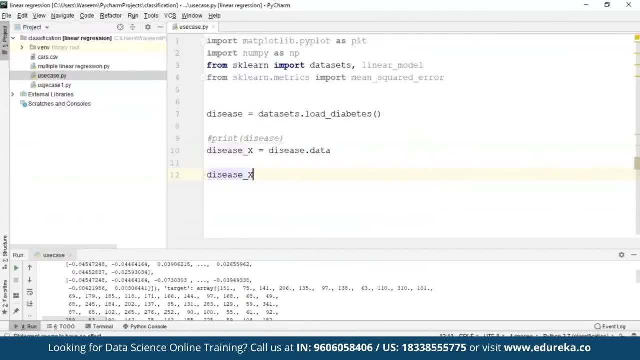 So what I'll do is I'll just write disease X. After this I'll write train. And let me take another variable, that is the X test, And we'll have to take this same variable for Y as well, because we need two variables. 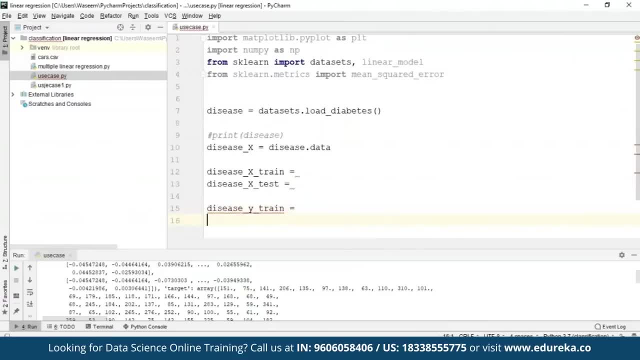 So I'll take it as Y train and disease Y test. now, inside this I'll have to split my data into training and testing data. So I'll use the disease over here, or we can just call it data also disease X, and I'm going to split the data from the starting until minus 30.. 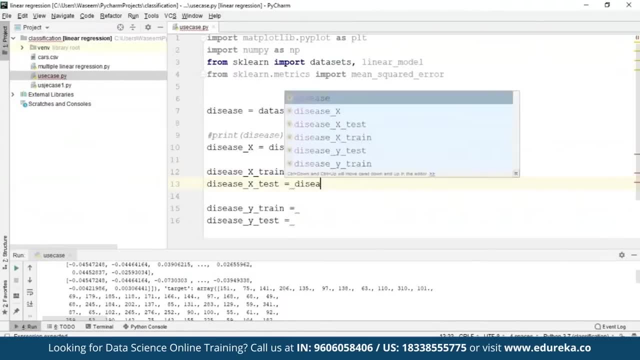 So I'll leave the last 30 data entries inside the data set which I'm going to use in the training set. So I'll use for the training set the minus 20, that is, from the last the 20 entries that we have over here. 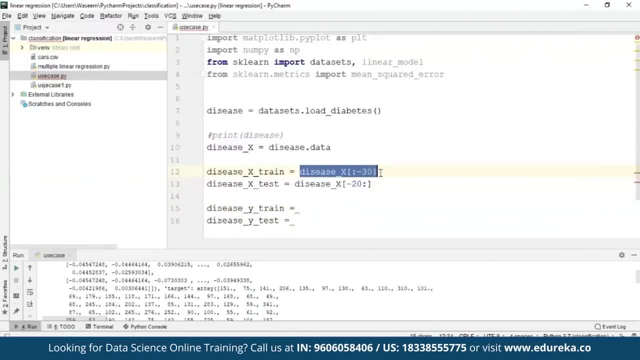 and similarly in the same thing we are going to do for the white train and y test as well. So we are just right. why so? before doing this, I'm just going to me as Target, because we're using the target variable over here. This is your Target again. 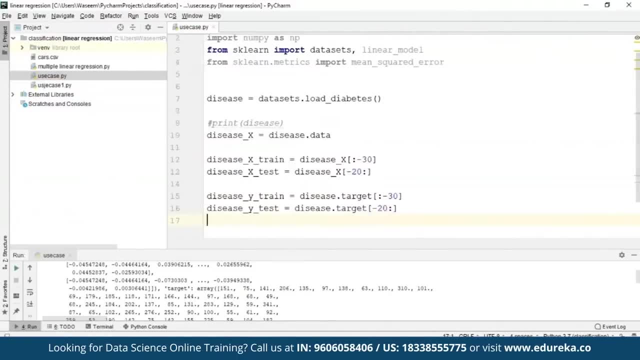 and in this I am going to use the last 20 entries. So we have successfully split our data. Now what happens is, after splitting your data, you have to generate your model for that. I'm just going to take one variable. So I'm just going to take it as reg or regression. 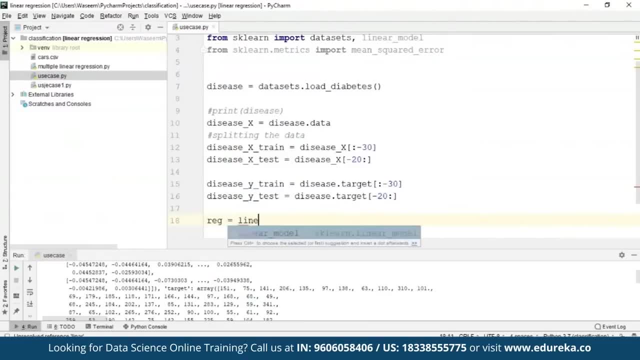 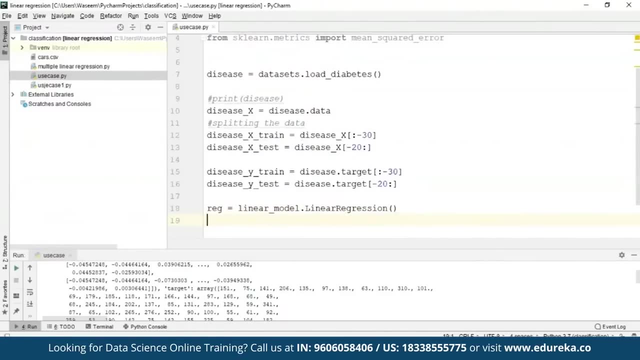 We can call it as regression as well. So I'm going to use linear model and I'm going to call linear regression. So this is how you can generate your model. So after this, you have to fit your training data inside the model using the fit function. 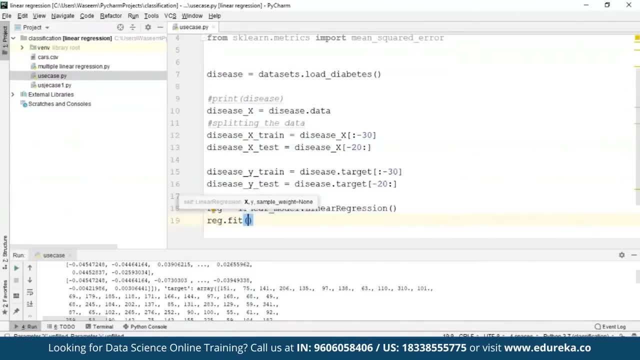 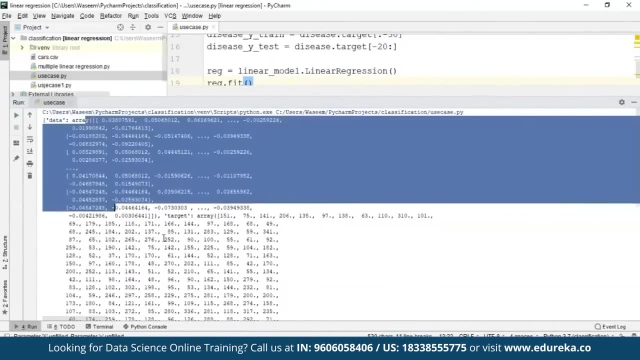 So I'll use fit over here and to fit the data I'm going to use disease X train that has the data variables, all those values that we have over here. That is this one. This array is going to be in the training one and we're going to use the target one for the disease Y. 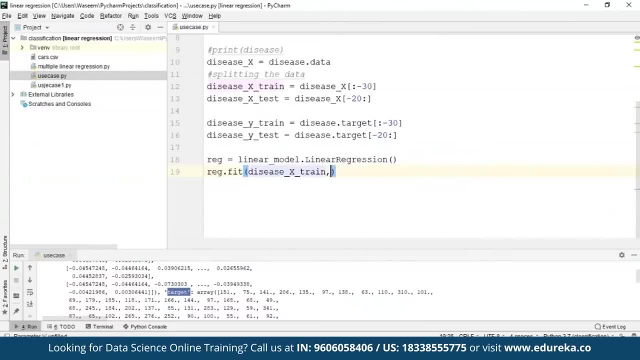 So I'll just do that. This is X train and disease Y train as well. So we're done. after this, I have to make a prediction variable as well. I'll make it as my predict and inside this I am going to use the predict function. 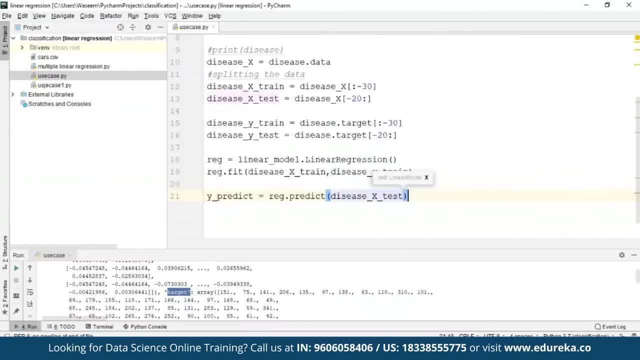 So for this we are going to use a disease X test, because this is what we are testing right now. So our model is actually done. guys, I'll just write some code for checking the accuracy as well. So I'll use the mean squared arrow over here. 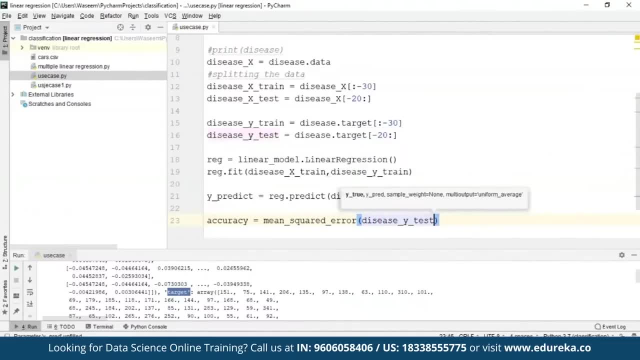 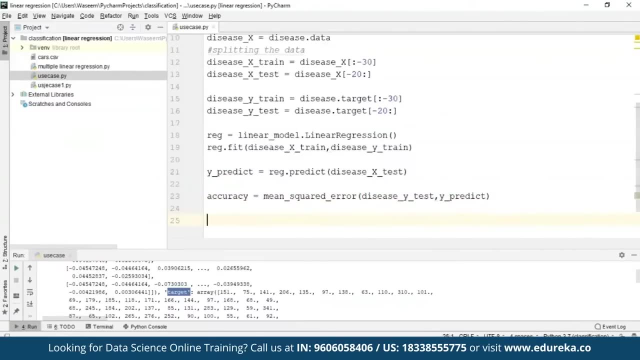 and inside this I'll pass disease Y Test and the y predict that we are going to get after the prediction. So we're almost done. after this, I'll print the accuracy as well, Whatever we will get, and let's just print the weights. 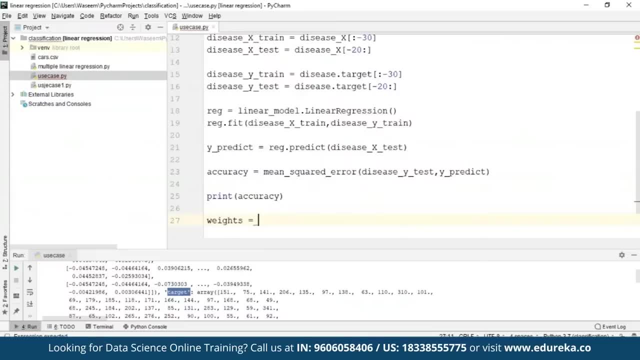 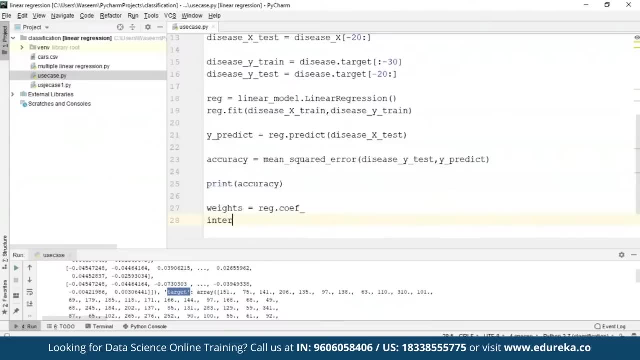 and the coefficients as well. So let's just say weights is equal to reg dot. So you have a function for this as well, to calculate the coefficient, that is, the weights, and intercept as well. So I'll name it as intercept and RG dot intercept. 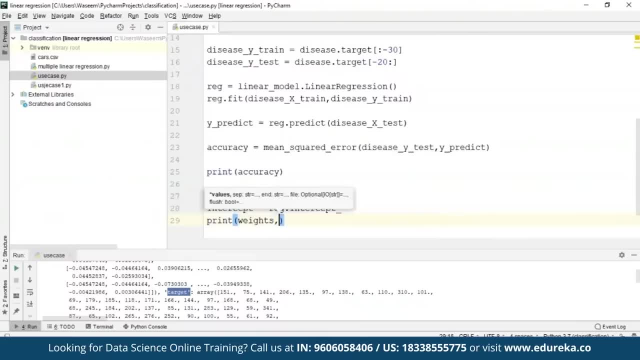 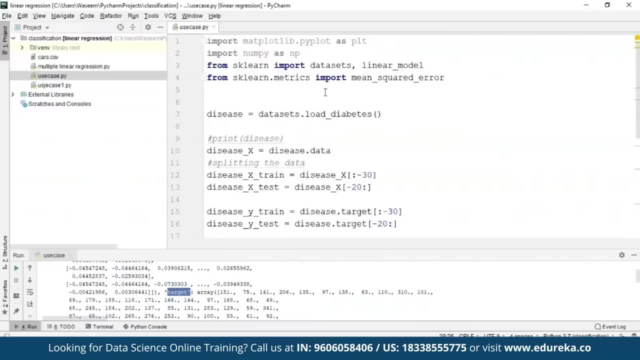 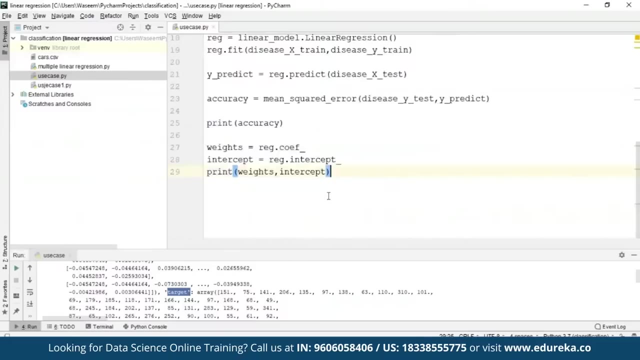 We'll print these as well. Wait and intercept. So we are. model is done, guys. So I successfully used all these libraries, We have load the data set and after that we have generated the model by splitting the data and everything. So I'll just run this code and see what the output is. 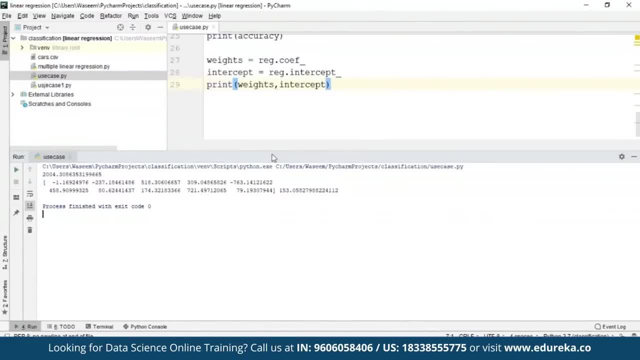 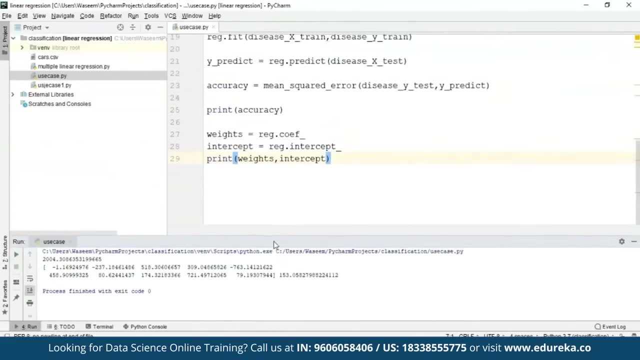 Okay, so we have the accuracy. that is a mean square error. That is 2004, and then we have the intercept and the weights as well. So this might sound a bit confusing for you guys, So I'll just add a few things over here. 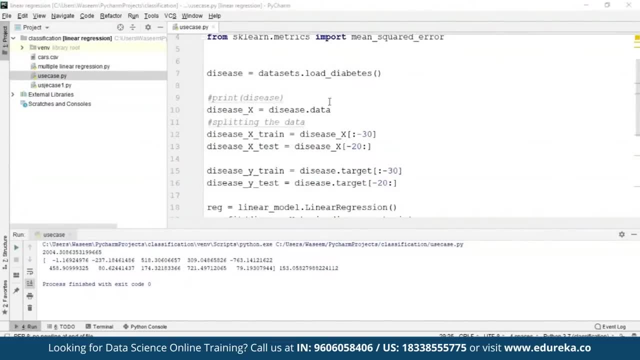 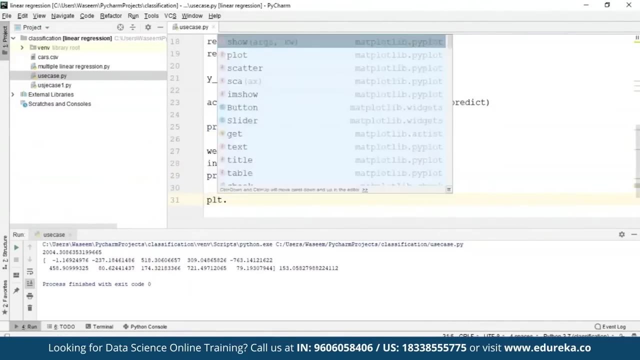 to make you understand this better. So what I do is I will make a few changes over here. So I'll just write it like: NP dot- new axis lighted as to over here, and we'll plot the graph also. So for that I'll just write plot scatter inside this: 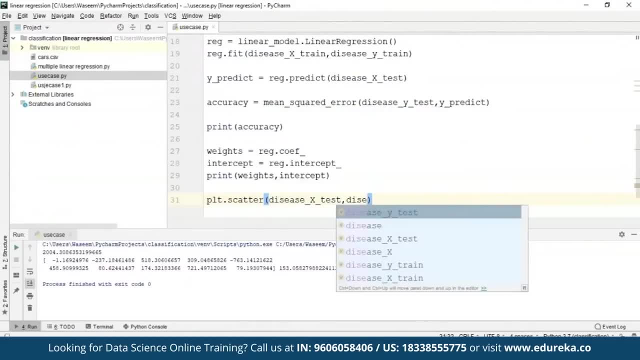 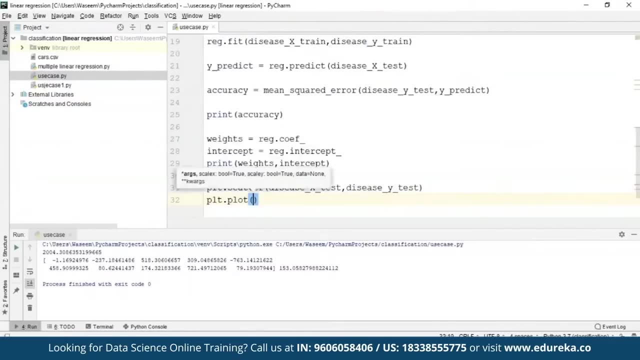 I'll use disease dot X test disease, not white test, PLT dot plot for the line and inside this I'm going to use disease X test and Y predict. So now when I run my code, you will be able to see the graph. 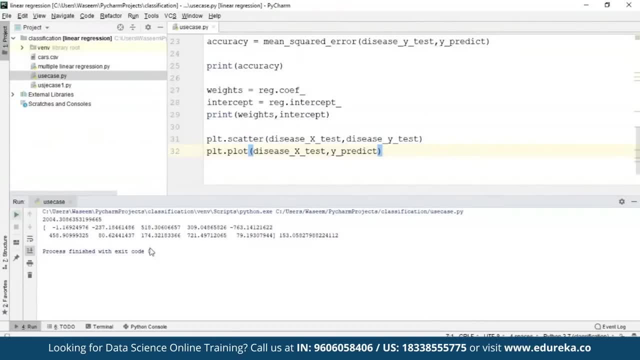 which will have the data entries And you'll be able to see the graph which has the data points, and there will be an intercept as well, with a line plotted which is the best fit line over here. Okay, we have not written. PLT dot show. 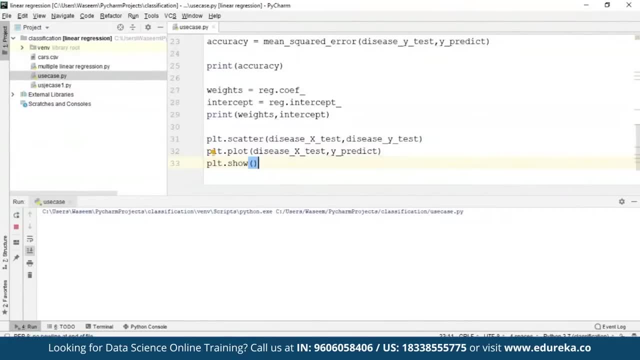 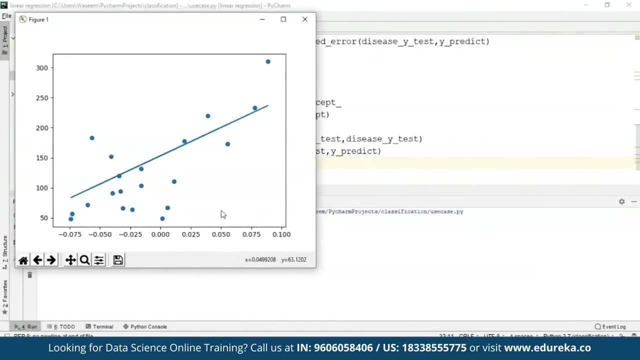 That's how you're not getting the graph. now It should be fine, and we'll be able to see the graph as well. So this is our best fit line, guys. So we have successfully implemented linear regression using python for this disease data set. 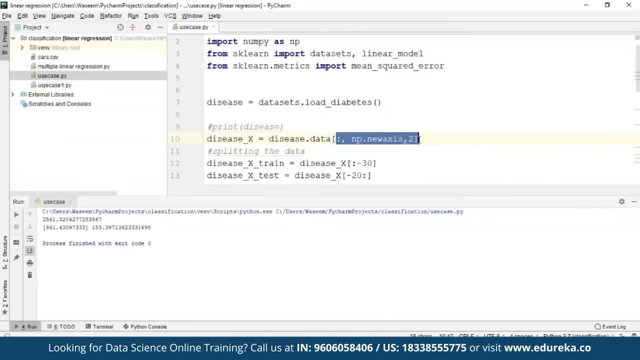 But to do this I had to segregate this data All separately and if you implemented using all the columns that you have in over here in the data, it's not going to be fine. I mean, it's going to throw you an error. 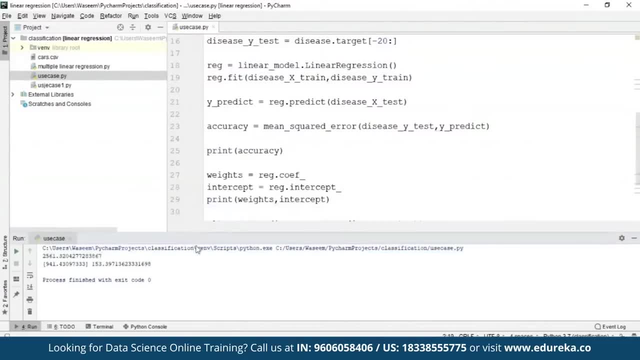 and with not show you a best fit line. So now that we are done with this one, I'll show you one more use case. inside We are going to use the custom data set which has the car resale value. So let's get done. 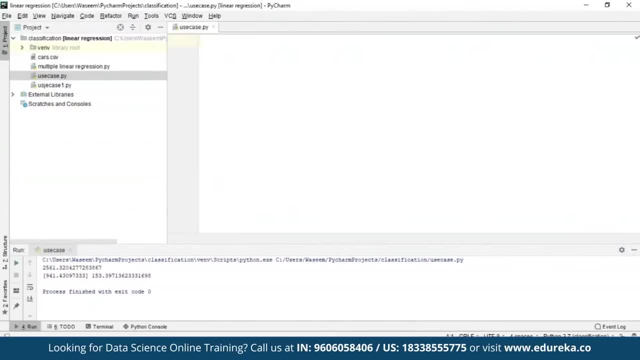 So I just remove all this. So first of all, I will import, as you can see over here in the directory, guys, you can already see this: cars X- CSV. This is my custom data set that I'm going to use inside this one. 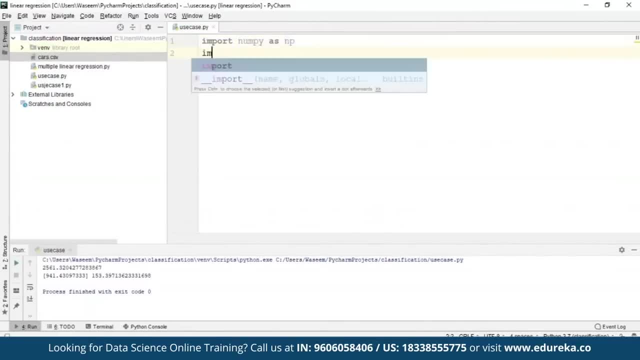 So I'll just import numpy as NP, Import pandas, because we are using a custom data set. I'm going to have to use pandas to import or to actually load the CSV file that I have over there, and after this I'll use my part- lip dot pi plot- as PLT. 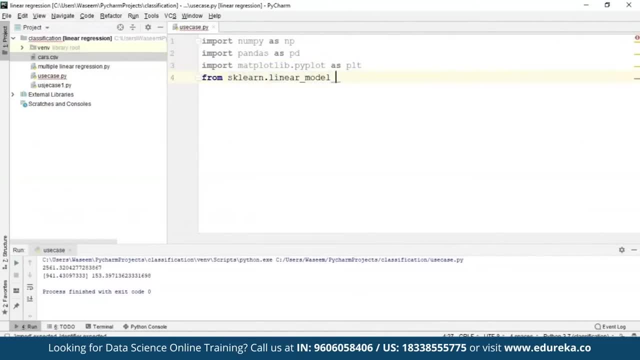 and from a scale on linear model. We are going to use linear regression And after this I'll just import a scale on dot matrix and import the R2 score, or we're not going to use that, So I'll just remove this one for now. 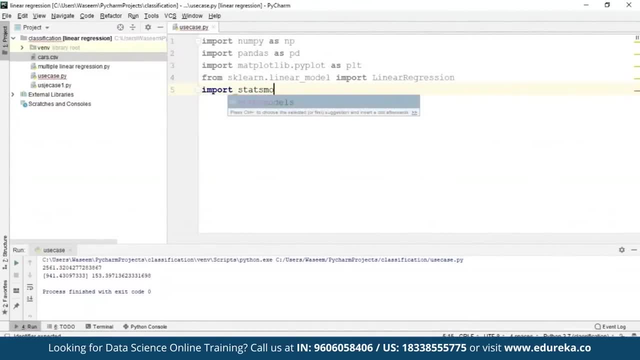 and we'll use import stats model. We'll leave this one for later as well. So first of all I have to load the data. So I'm naming it as cars. So for this I'll just write PD, rotary CSV. And if you don't know how you can import the CSV files, 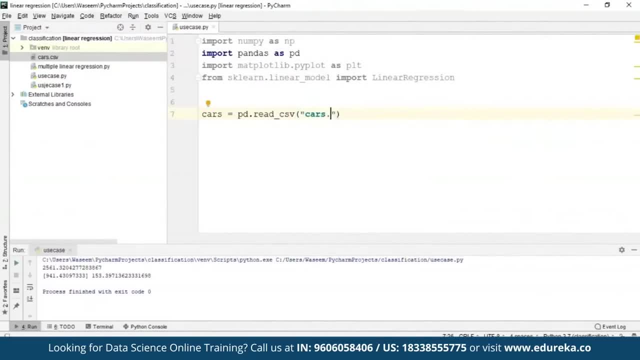 the custom made CSV files inside your program you can check out other tutorials on the end. You're a cop, So we have a tutorial in detail how you can do CSV files. So first of all, let me just get a quick exploration of the data. 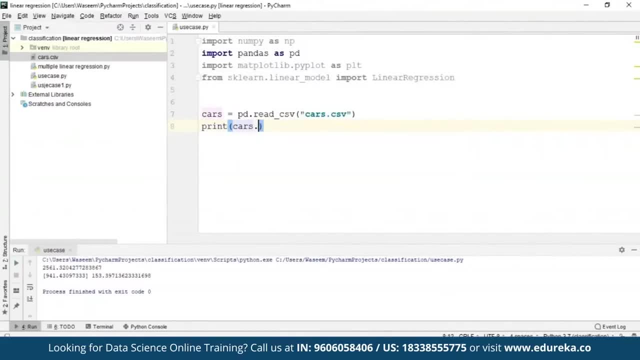 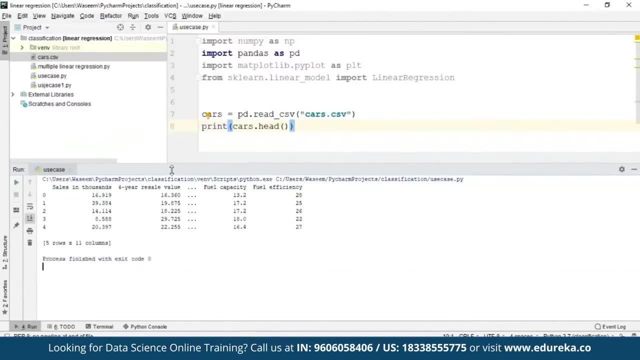 what we have over here. So I'll just write the print statement. I'll get the head. So this is what my data set looks like. guys, It's loading still. so we have all these values and to get the better picture over here, 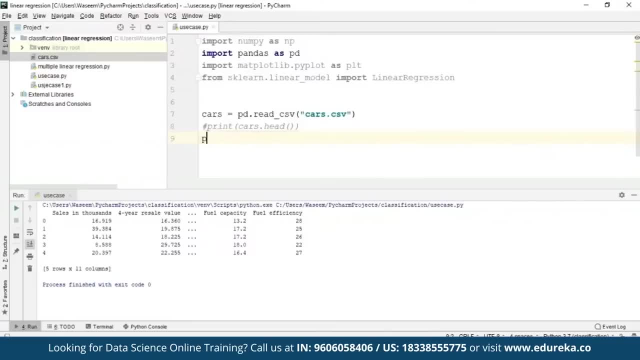 I will try to print The columns as well. So I just write cars or columns, So it will give me the name of all the columns that I have in this data set. Okay, so we have all these values. It's in thousands. 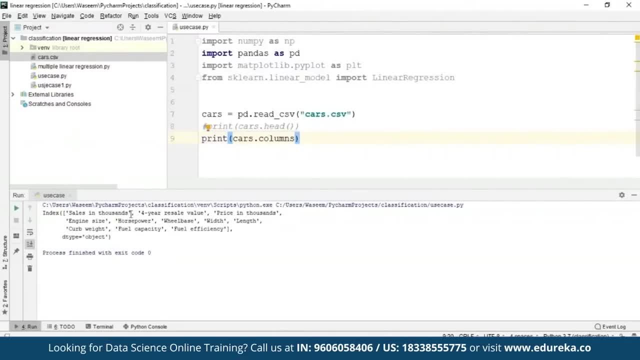 We have a four-year resale value, Then we have price in thousands, and we have engine size, horsepower, wheelbase width, length, Then we have cup weight. We have fuel capacity, fuel efficiency as well. Okay, so this is what our data looks like, guys. 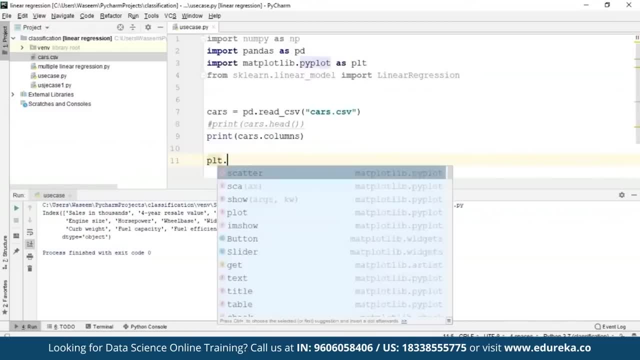 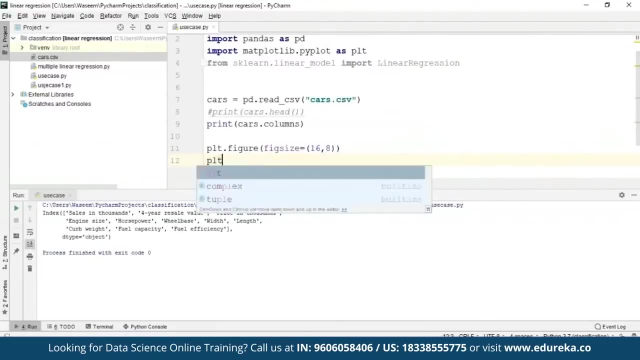 So let me just plot a graph first of all. So I'll just write PLT And you're going to use the figure size, For figure size is equal to, let's just say, 16 by 8, and after this I will use a scatter plot. 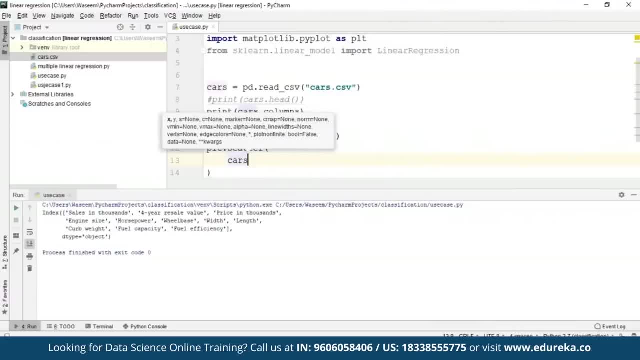 And inside this I'm going to give a few values. So I'm going to use cars. So first of all I want to check the relationship between a horsepower and then I'll check what is the relation between a horsepower and the price of the car, which is in thousands. 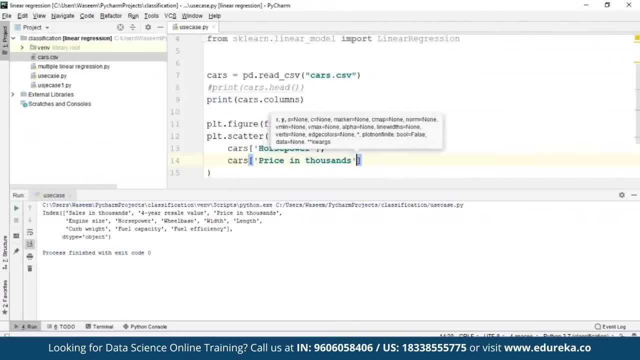 of course, And let's just Set it as black, Yes, And let's just put a few labels as well. So X label is going to be, let's say, horsepower, And we will write the Y label as, let's just say, price. 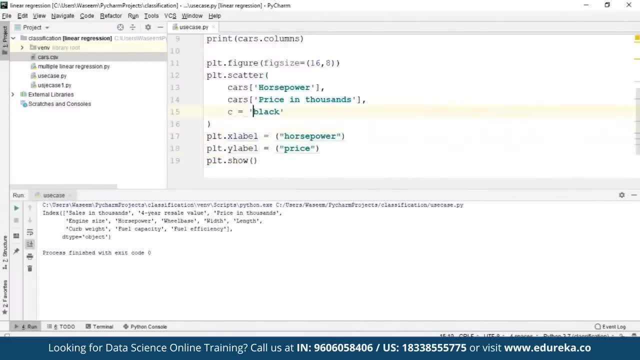 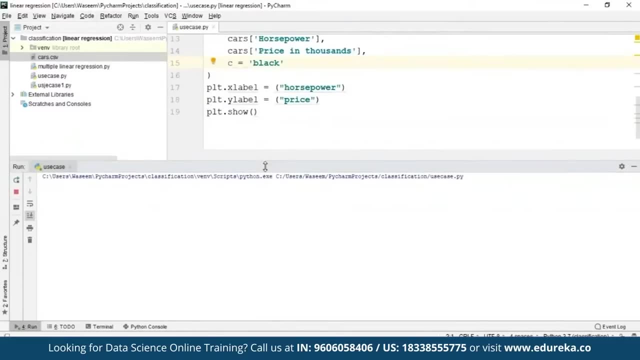 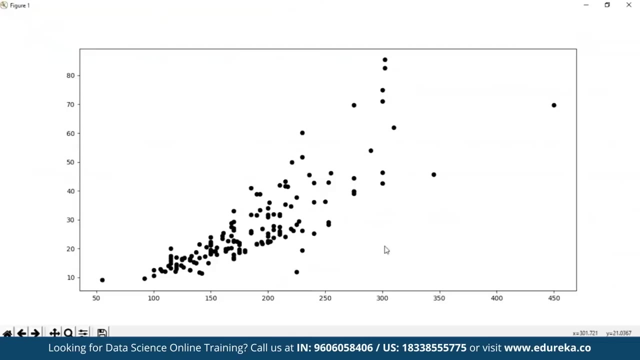 And let's just plot this graph for now. We'll put it over here only Now, when I run this, let's see what I'm getting over here. So I'm getting a graph like this So you can see all the data points. 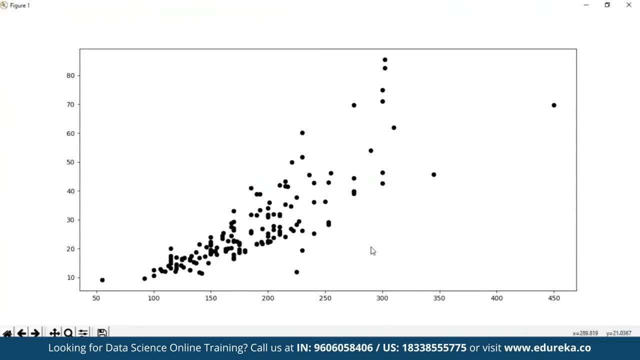 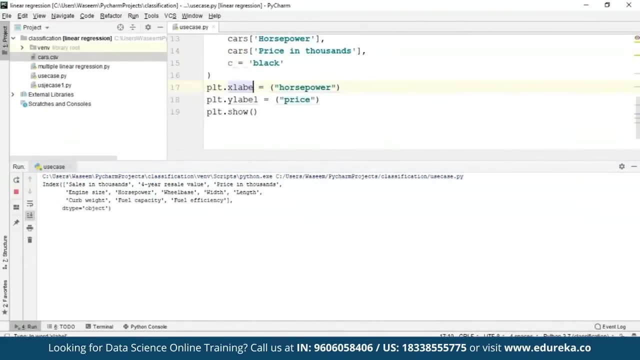 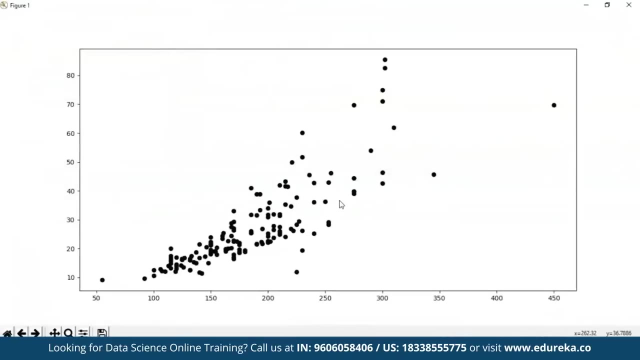 and as we go further, the values are actually increasing. We're not getting the Y labels over here somehow. I think there's some problem. Just check it out. Give me leave it for now And let's check the image of over here. 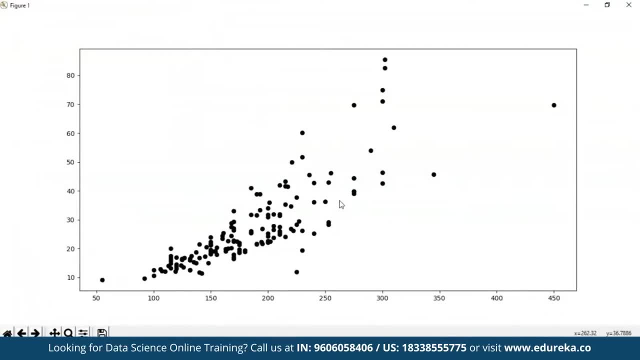 So on the x-axis we have the horsepower, which is going until 450.. So a car with the horsepower 450 is ranging around 70,000.. That is the price and that's going to be in dollars, guys. and all these values, like a 150 horsepower car is going. 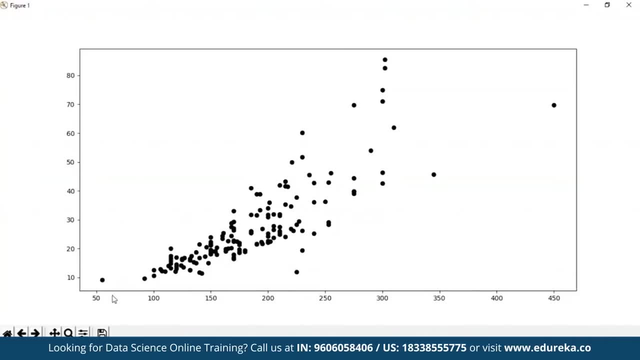 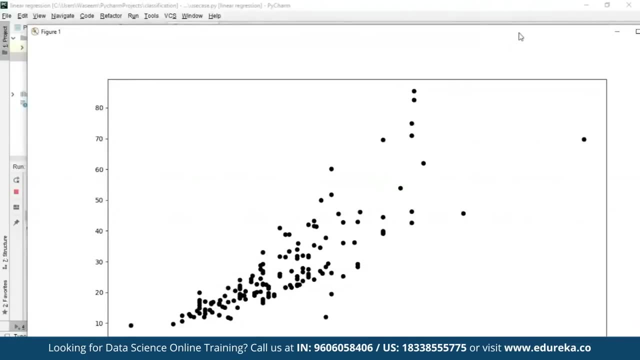 to be around 20,000 bucks and a simple 50 horsepower car is going to be around 10,000 bucks. So this is our data, guys. I think it's pretty evident that we have a relation between a horsepower and the price of the car. 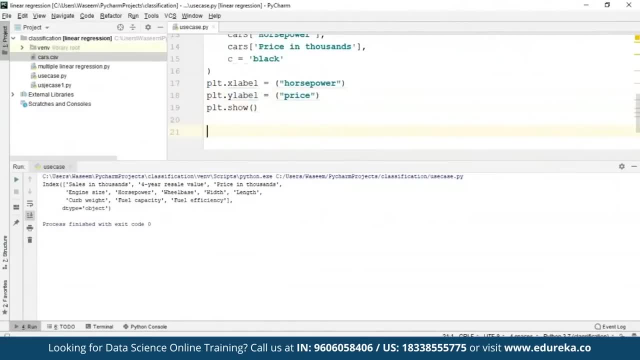 that we are actually looking at right now. So we'll build a model around this for now. So I'll take one variable, Let's just say X, and inside this I'm going to put cars- horsepower, because we are going to take horsepower as our independent variable. 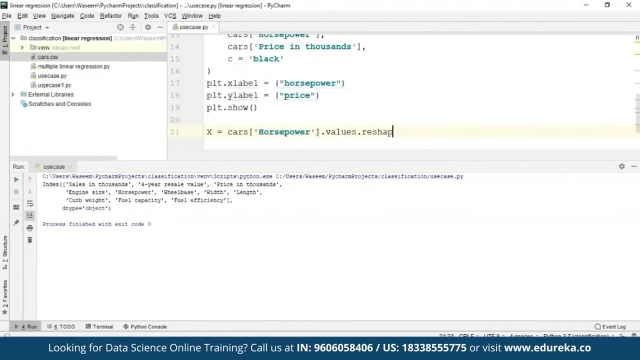 and all these values. I'm going to reshape them into minus one and one. I'm going to take one more independent variable. Why that's going to be my price In thousands, guys, I'm going to do the reshaping again. Is this basically to avoid the errors? guys reshaping? 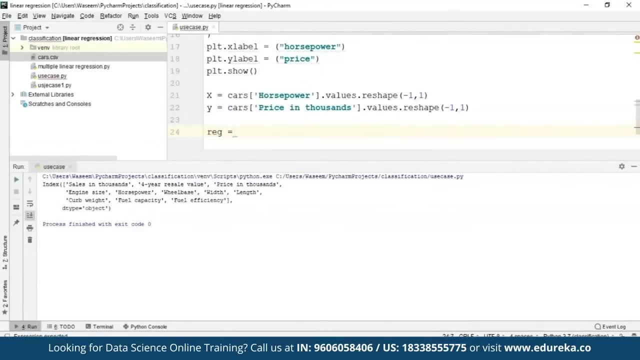 that I'm doing over here and I'll just generate my model right now. So I'll use linear regression And after this I'll try to fit my X and Y over here using the fit method. So just write X and Y. Now I'm going to print the coefficient. 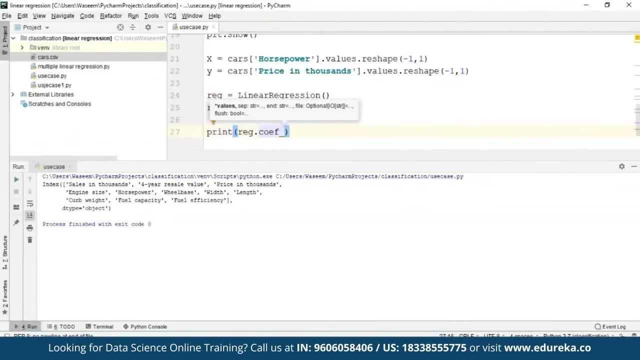 using the coefficient function that I've shown you before. I'm going to take the values as 0 and 0.. Again, for the same thing, I want the intercept as well. So instead of coefficient, I'll write as intercept and I'll remove this one. 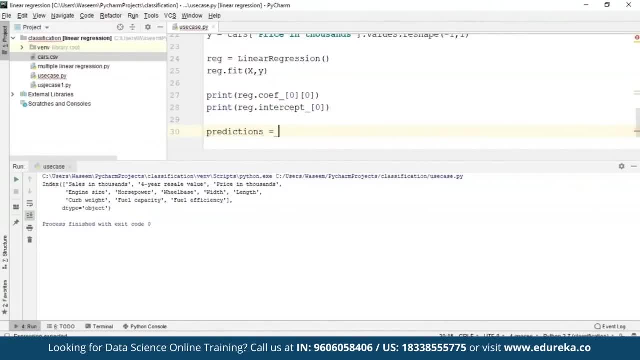 After this, let's make one variable, Let's just say predictions- that's going to store the predicted value and we're going to use the predict function over here. So I'm just going to put X over here in the predict function and let's just plot a graph again. 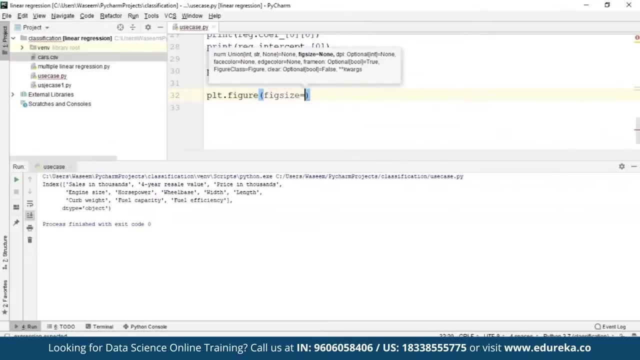 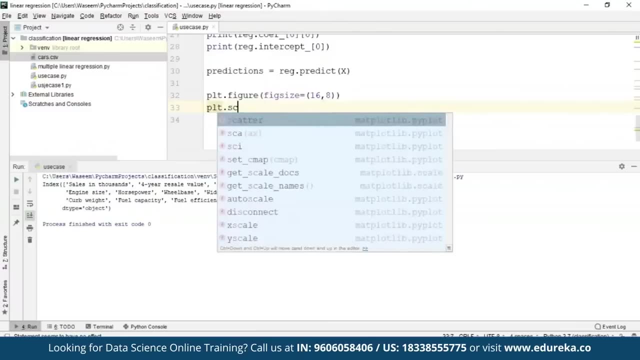 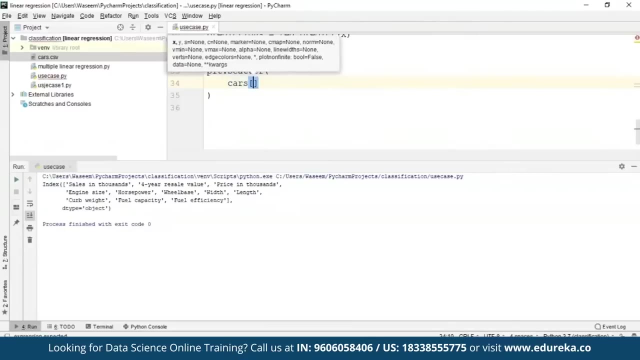 So right, figure figure size again. Let's just take 16 by 8.. We'll use the scatter plot again. We just write it again. First of all we have cars and horsepower. Then we have cars rise in thousands. after this: 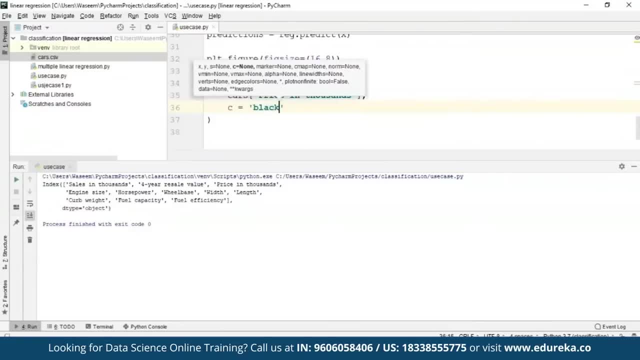 I'm just going to write: C is equal to black. Now we have one more plot for the line, So I'm going to use PLT dot plot. inside this We'll have cars, horsepower, We'll use the predictions as well, And let's just make it blue. 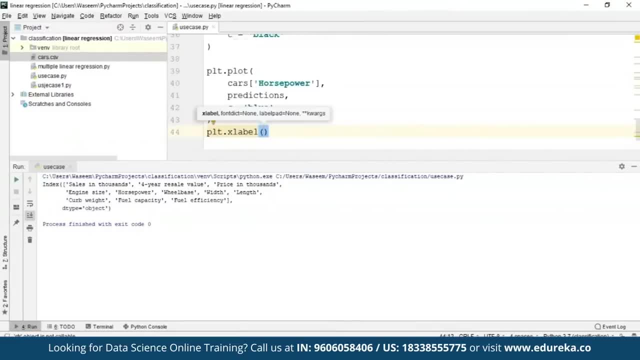 We'll put the label again, So the X label is going to be the horsepower And the Y label is going to be prices or just price. I'll write PLT dot show. now when I run this I should be getting a. okay, we'll get the first plot. 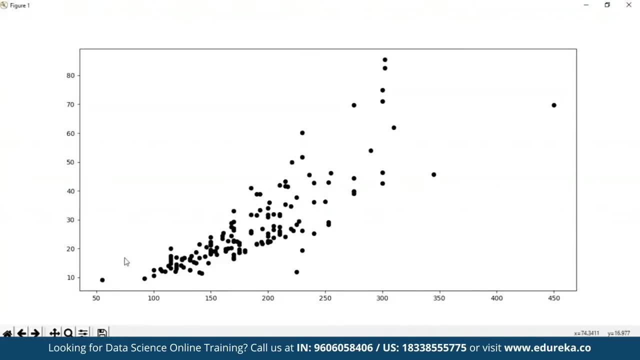 before getting the second blood. So we have a plot like this: So actually the horsepower is over here, That is going up till 450 horsepower, And this is actually our price Now when I close this. Okay, I've made a mistake somewhere. 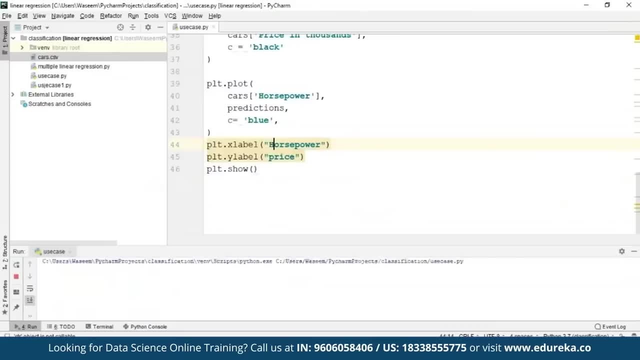 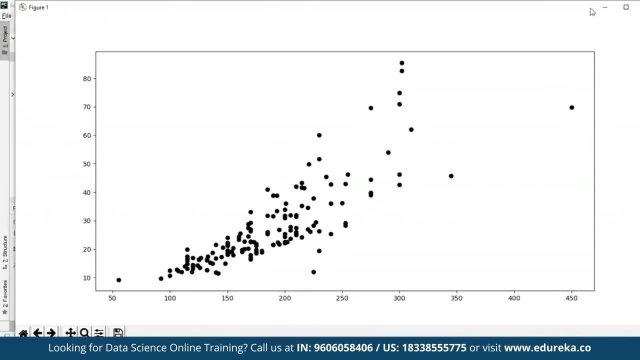 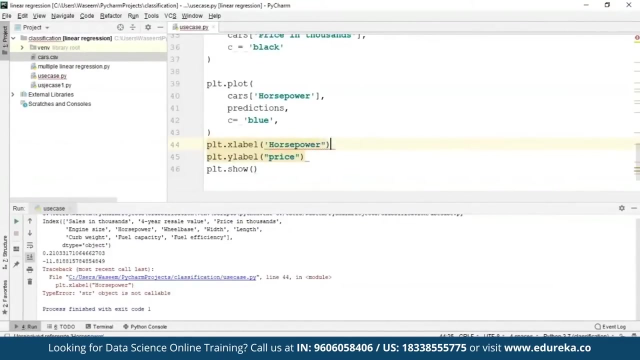 Okay, this is actually now when I run this again, I should be fine. I close this and after this: Okay, so I've got the mistake that I was making. So before running this program, I'll add the line width as well. 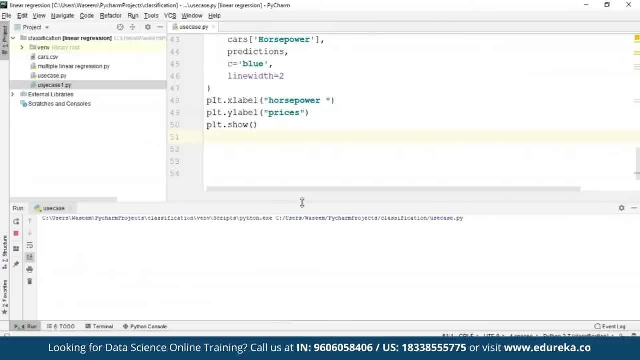 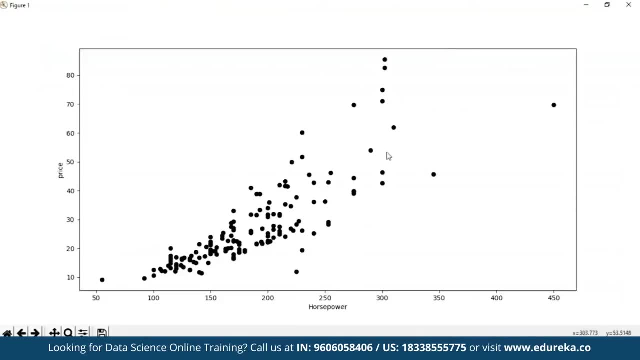 And let's just run this again. So first I'm getting this, which is horsepower, right here, and we have the price right over here. after this, Let's see. So we have a best-fit line over here, as you can see, guys. So this is a simple linear regression implementation. 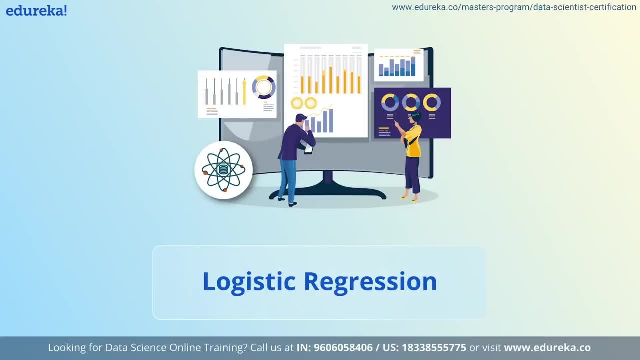 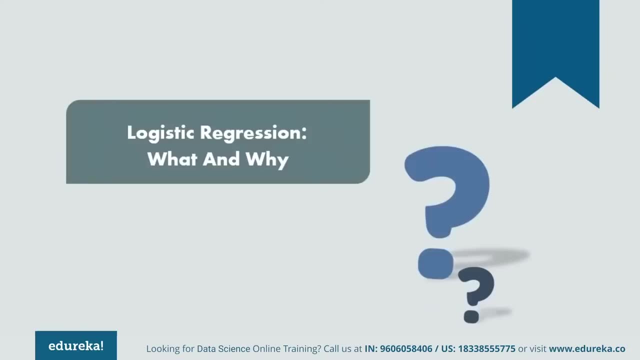 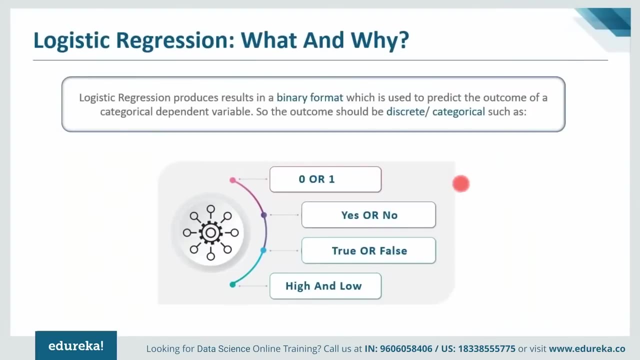 on a custom data set. So today we'll be discussing logistic regression. So let's move forward and understand the what and why of logistic regression. Now. this algorithm is most widely used when the dependent variable, or you can say the output, is in the binary format. 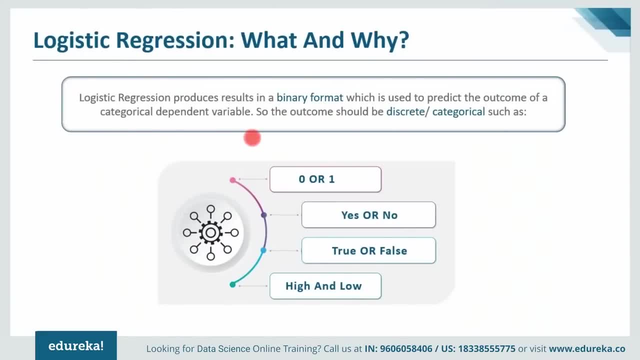 So here you need to predict the outcome of a categorical dependent variable. So the outcome should be always discrete Or categorical in nature. now by discrete I mean the value should be binary, or you can say you just have two values. It can either be 0 or 1. it can either be yes. 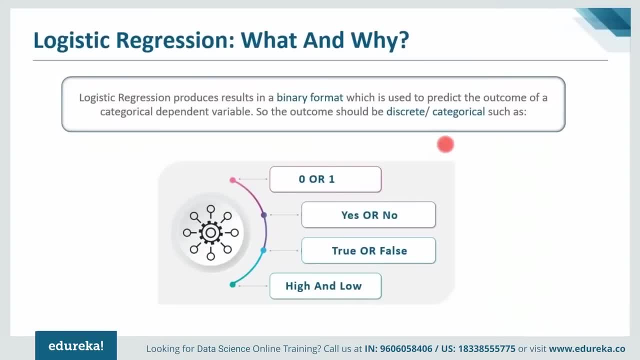 or no, either be true or false, or high or low, So only these can be the outcomes. So the value which you need to predict should be discrete, or you can say categorical in nature. Whereas in linear regression we have the value of y, or you can say the value need to predict is in a range. 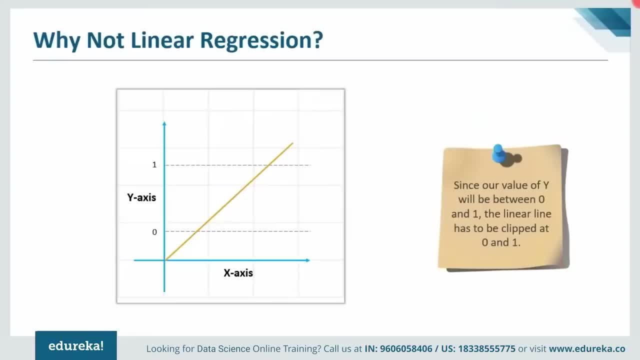 So that is how there is a difference between linear regression and logistic regression. Now you must be having question: Why not linear regression? Now, guys, in linear regression, the value of y, or the value which you need to predict, is in a range. But in our case, as in the logistic regression, 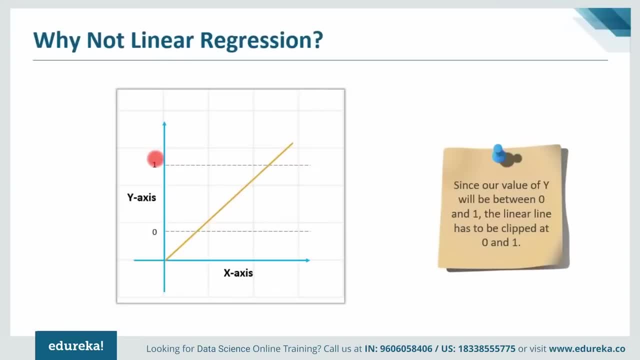 we just have two values. It can be either 0 or it can be 1.. It should not entertain the values which is below 0 or above 1.. But in linear regression we have the value of y in the range. So here, in order to implement logistic regression, 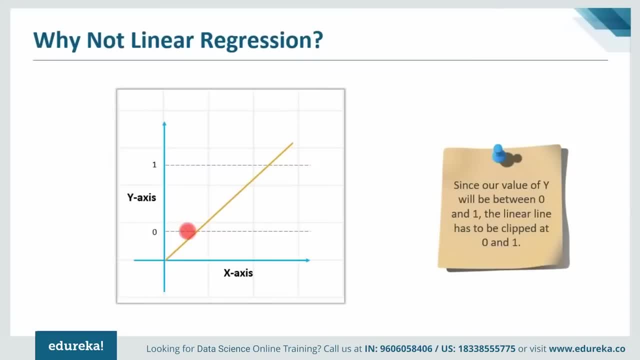 we need to clip this part, So we don't need the value that is below 0, or we don't need the value which is above 1.. So, since the value of y will be between only 0 and 1, that is the main rule of logistic regression. 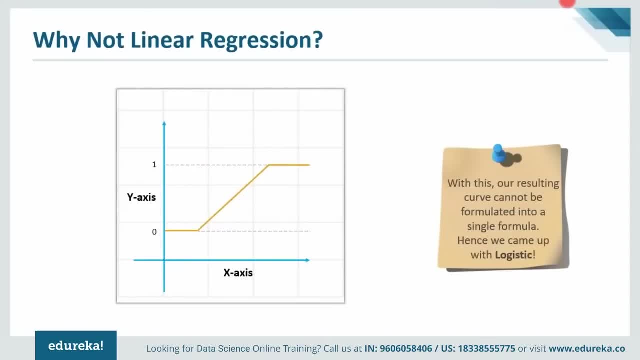 the linear line has to be clipped at 0 and 1.. Now, once we clip this graph, it would look somewhat like this: So here you are getting the curve, which is nothing but three different straight lines. So here we need to make a new way to solve this problem. 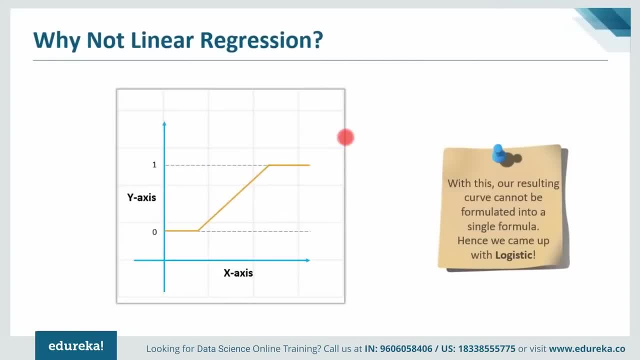 So this has to be formulated into equation, and hence we come up with logistic regression. So here the outcome is either 0 or 1, which is the main rule of logistic regression. So with this our resulting curve cannot be formulated. So hence our main aim, to bring the values to 0 and 1, is fulfilled. 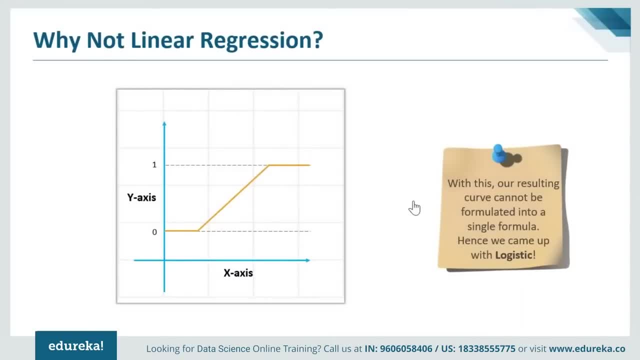 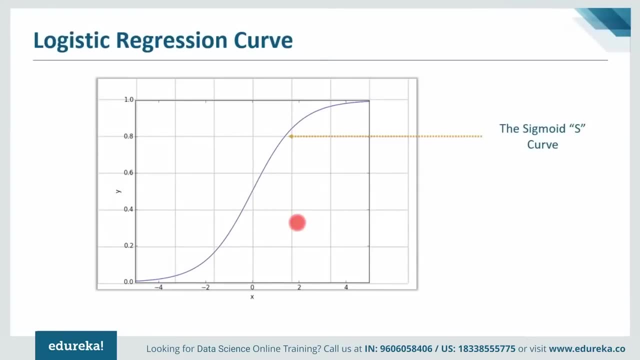 So that is how we came up with logistic regression. Now here, once it gets formulated into an equation, it looks somewhat like this: So, guys, this is nothing but a S curve, or you can say the sigmoid curve, or sigmoid function curve. So this sigmoid function basically converts any value. 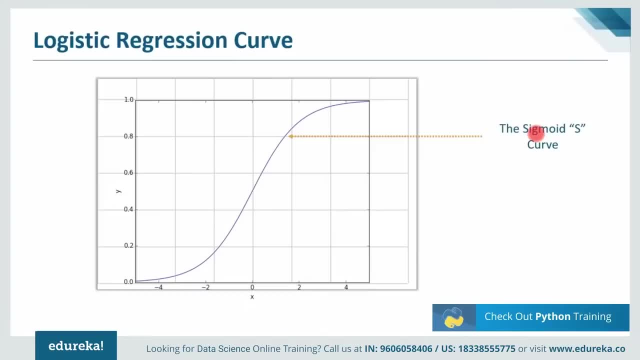 from minus infinity to infinity, to your discrete values, which a logistic regression wants. or you can say the values which are in binary format, either 0 or 1.. So if you see here the values are either 0 or 1, and this is nothing but just the transition of it. 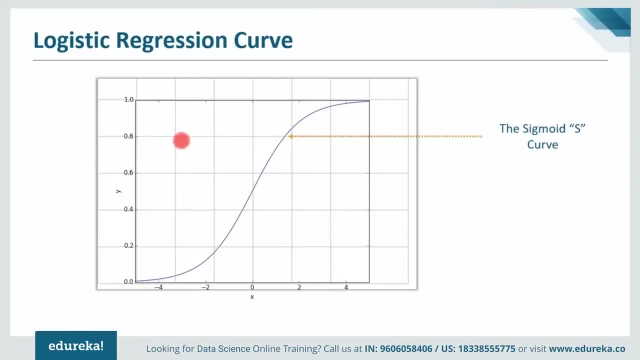 But, guys, there's a catch over here. So let's say, I have a data point that is 0.8.. Now how can you decide whether your value is 0 or 1? Now, here you have the concept of threshold, which basically divides your line. 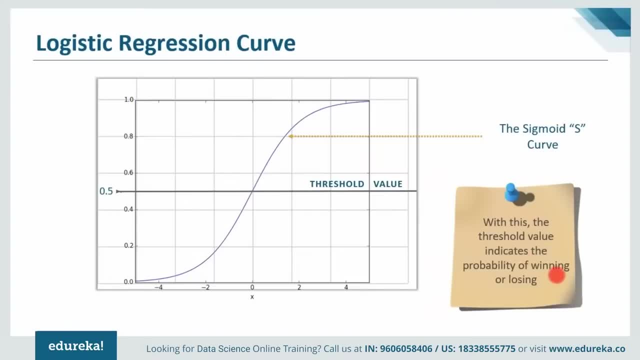 So here threshold value basically indicates the probability of either winning or losing. So here, by winning I mean the values equals to 1, and by losing I mean the values equals to 0. But how does it do that? Let's say I have a data point which is over here. 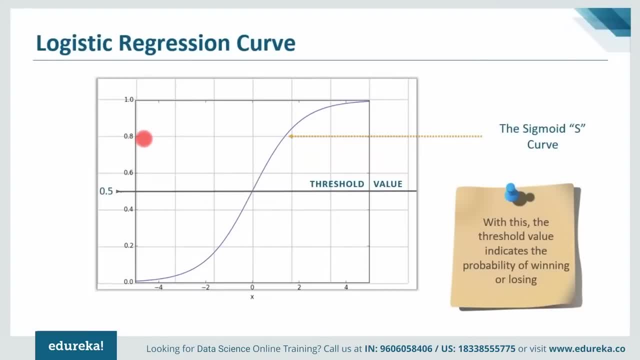 Let's say, my cursor is at 0.8.. So here I'll check whether this value is less than my threshold value or not. Let's say, if it is more than my threshold value, it should give me the result as 1.. 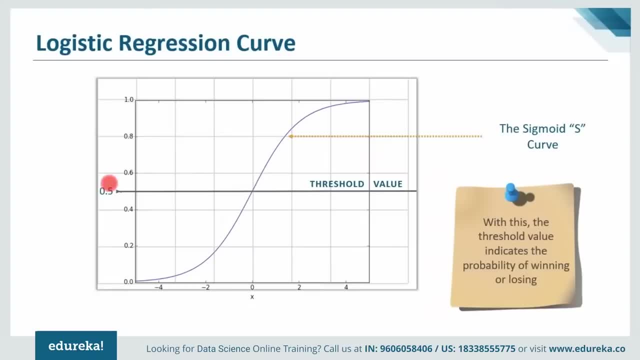 If it is less than that, then should give me the result as 0.. So here, my threshold value is 0.5.. Now I need to define that if my value, let's say 0.8.. It is more than 0.5.. 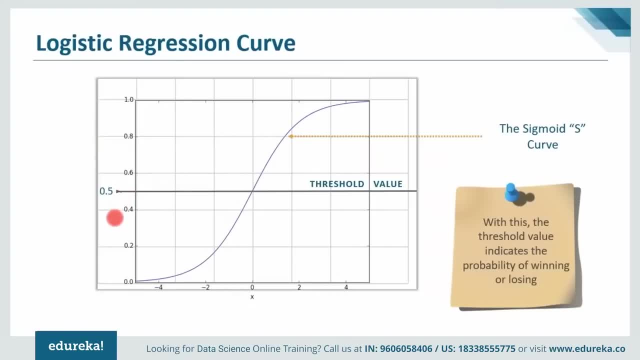 Then the value shall be rounded off to 1, and let's say if it is less than 0.5.. Let's say I have a value 0.2.. Reduce it to 0. So here you can use the concept of threshold value. 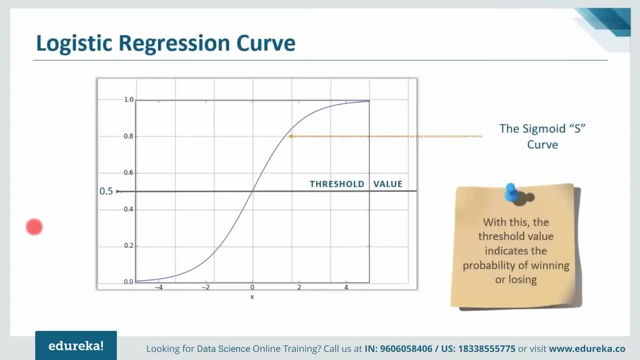 to find your output. So here it should be discrete, It should be either 0 or it should be 1.. So I hope you caught this curve of logistic regression. So, guys, this is the sigmoid S curve. So to make this curve we need to make an equation. 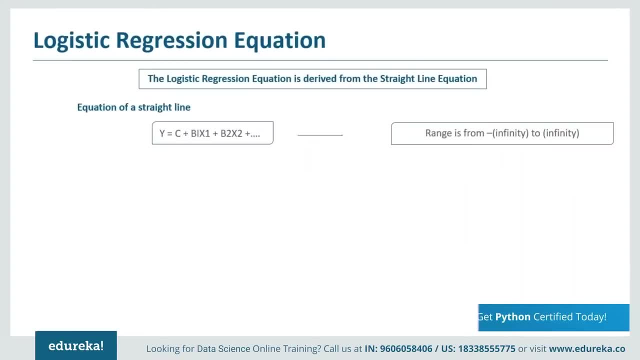 So let me address that part as well. So let's see how an equation is formed to imitate this functionality. So over here we have an equation of a straight line which is: y is equals to MX plus C. So in this case, 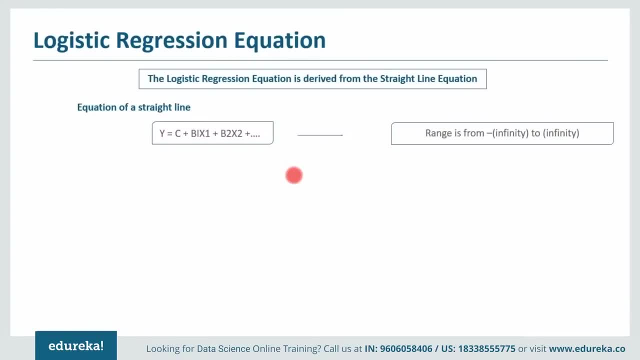 I just have only one independent variable. but let's say, if we have many independent variable, then the equation becomes m1, x1 plus m2, x2 plus m3, x3 and so on till mn xn. Now let us put in b and x. 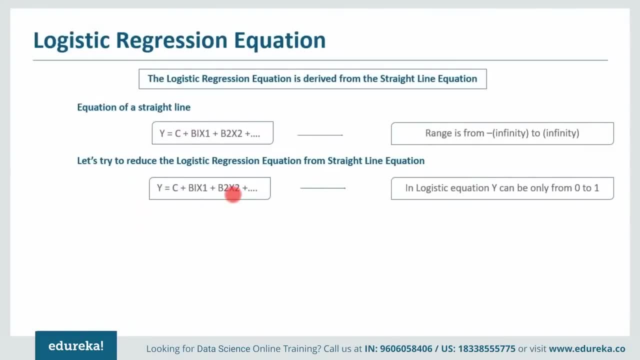 So here the equation becomes: y is equals to b1, x1 plus b2, x2 plus b3, x3 and so on, till bn, xn plus C. So, guys, your equation of the straight line has a range from minus infinity to infinity, But in our case, or you can say in logistic equation, the value. 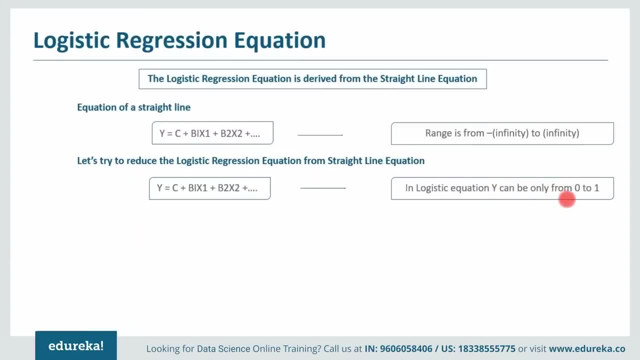 which we need to predict, or you can say the y value. It can have the range only from 0 to 1.. So in that case we need to transform this equation So to do that what we had done, we have just divide the equation. 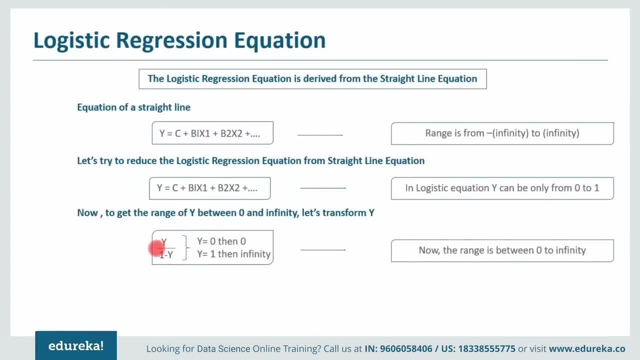 by 1 minus y. So now our y is equals to 0. so 0 over 1 minus 0, which is equals to 1, so 0 over 1 is again 0 and if we take y is equals to 1. then 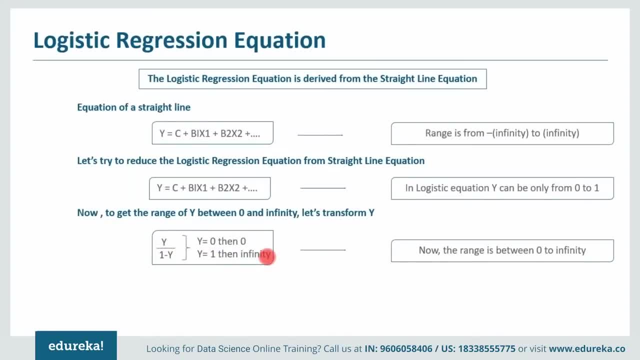 1 over 1 minus 1, which is 0. so 1 over 0 is infinity. So here my range is now between 0 to infinity. But again, we want the range from minus infinity to infinity. So for that, what we'll do will have the log of this equation. 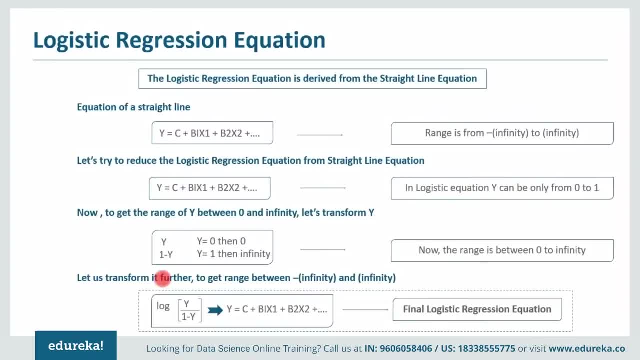 So let's go ahead and have the logarithmic of this equation. So here we have this. transform it further to get the range between minus infinity to infinity. So over here we have log of y over 1 minus 1 and this is your final logistic regression equation. 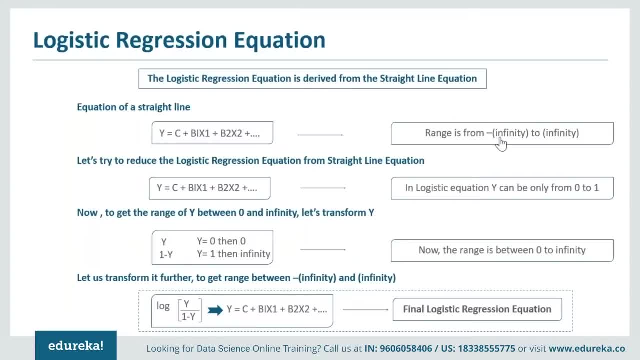 So, guys, don't worry, You don't have to write this formula or memorize this formula in Python. You just need to call this function, which is logistic regression, and everything will be automatically for you. So I don't want to scare you with the. 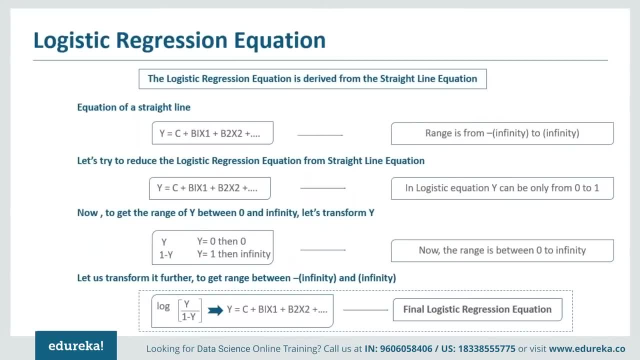 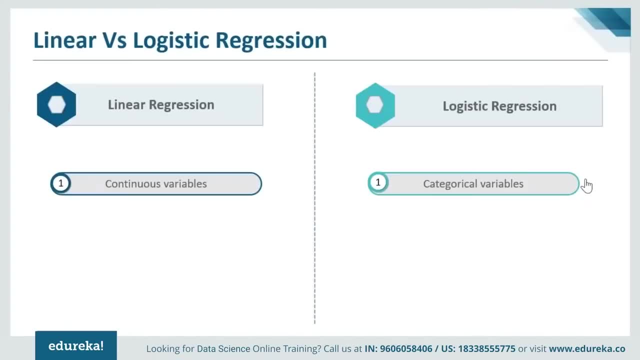 maths and the formulas behind it, but it's always good to know how this formula was generated. Let's let us see What are the major differences between linear regression versus logistic regression. Now, first of all, in linear regression we have the value of y as a continuous variable, or the variable. 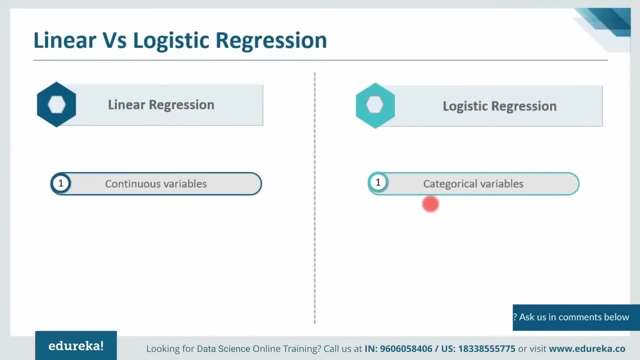 which we need to predict a continuous nature, whereas in logistic regression we have the categorical variable. So here the value which you need to predict should be discrete in nature. It should be either 0 or 1 or it should have just two values to 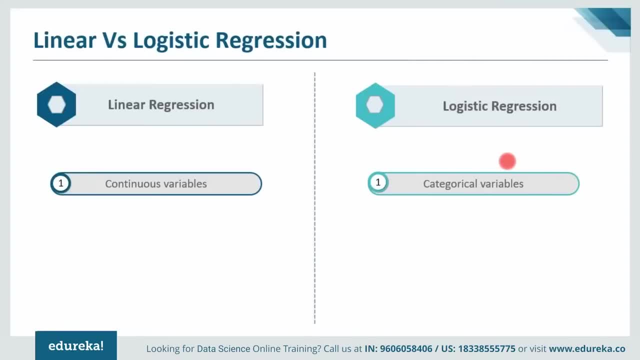 it, For example, whether it is raining or it is Not raining. Is it humid outside or it is not humid outside? now, Does it going to snow or it is not going to snow? So these are the few example where you need to predict where. 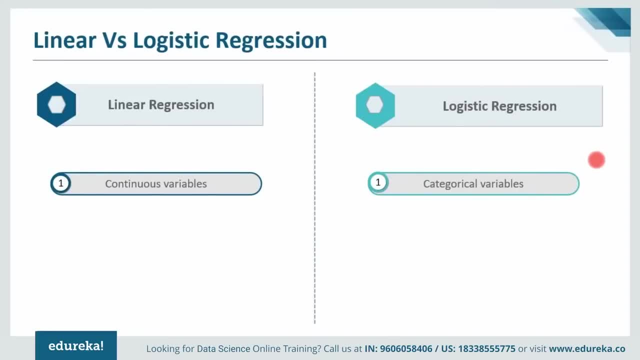 the values are discrete, or you can just predict whether this is happening or not. next, linear regression solves your regression problems. So here you have a concept of independent variable and a dependent variable. So here you can calculate the value of y which you need to predict. 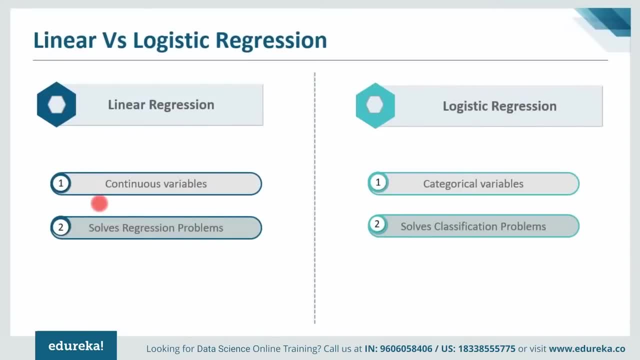 using the value of x. So here your y variable, or you can say the value that you need to predict, are in a range, But whereas in logistic regression you have discrete values. So logistic regression basically solves your classification problem. So it can basically classify it and it can just give you result. 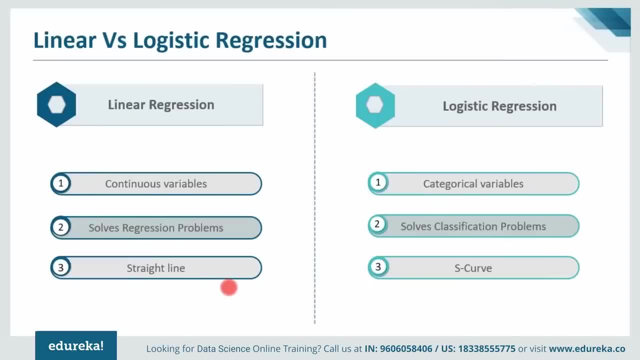 whether this event is happening or not. next, in linear regression, the graph that you have seen is a straight line graph, So over here you can calculate the value of y with respect to the value of x, whereas in logistic regression the curve that we got was a s curve, or you can say the sigmoid. 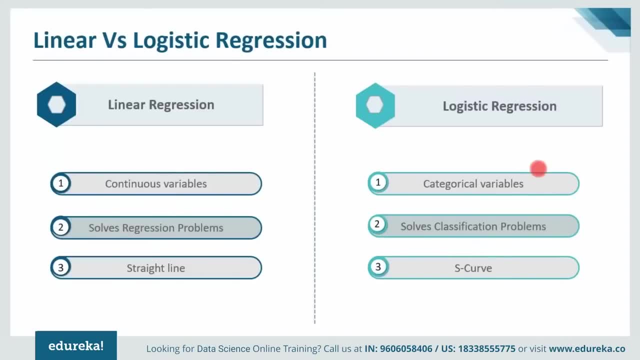 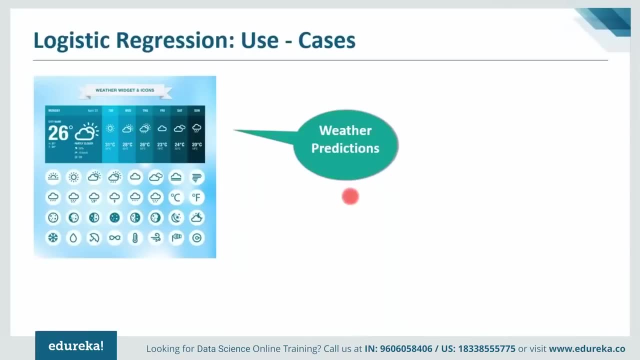 curve. So, using the sigmoid function, you can predict your y values Moving ahead. Let us see the various use cases wherein logistic regression is implemented in real life. So the very first is weather prediction. Now logistic regression helps you to predict your weather. 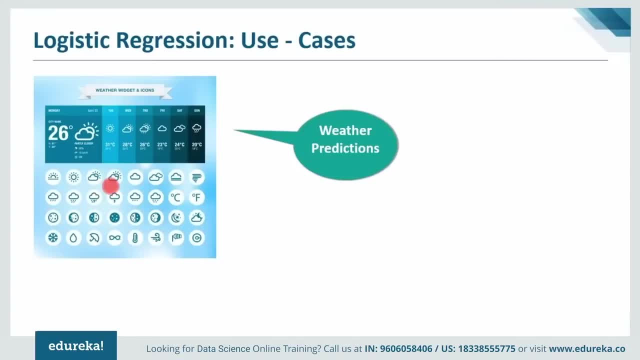 For example, it is used to predict whether it is raining or not, whether it is sunny, Is it cloudy or not. So all these things can be predicted using logistic regression, whereas you need to keep in mind that both linear regression and logistic regression can be used in predicting the weather. 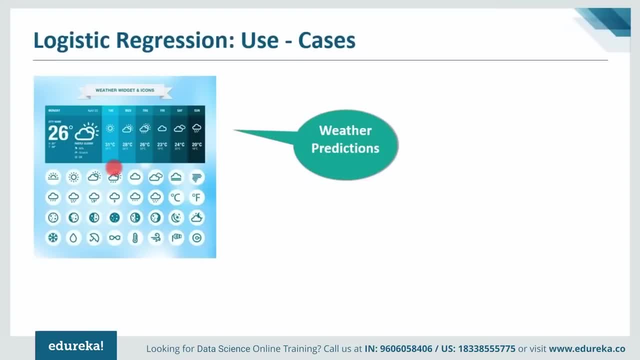 So in that case, linear regression helps you to predict what will be the temperature tomorrow, Whereas logistic regression will only tell you whether it's going to rain or not, or whether it's cloudy or not, which is going to snow or not. So these values are discrete. 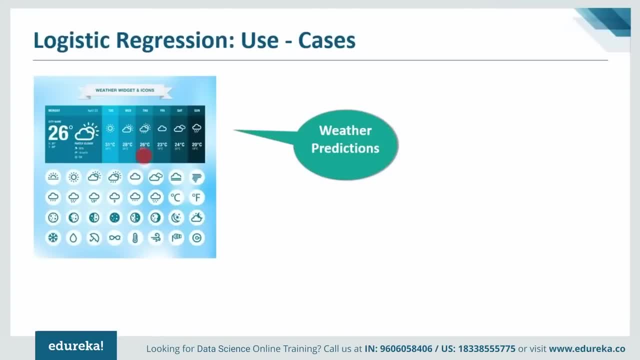 Whereas if you apply linear regression, you will be predicting things like what is the temperature tomorrow or what is the temperature day after tomorrow, and all those things. So these are the slight differences between linear regression and logistic regression. Now moving ahead, we have classification problem. 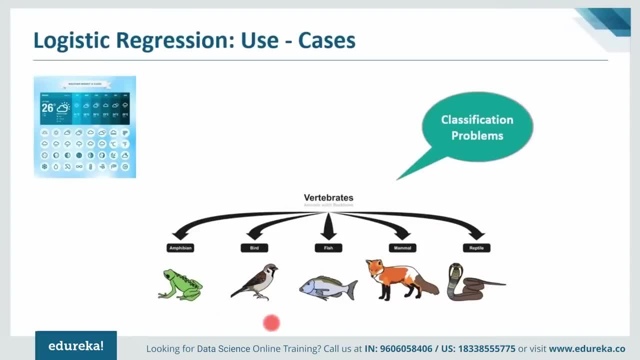 So python performs multi-class classification, So here it can help you tell whether it's a bird or it's not a bird. Then you classify different classifications, Let's say whether it's a dog or it's not a dog. Similarly, you can check it for reptile, whether it's a reptile or not. a. 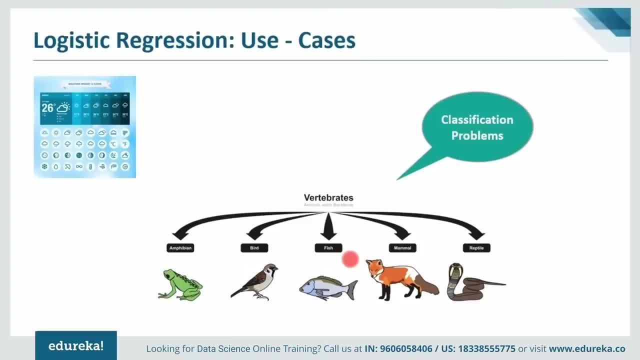 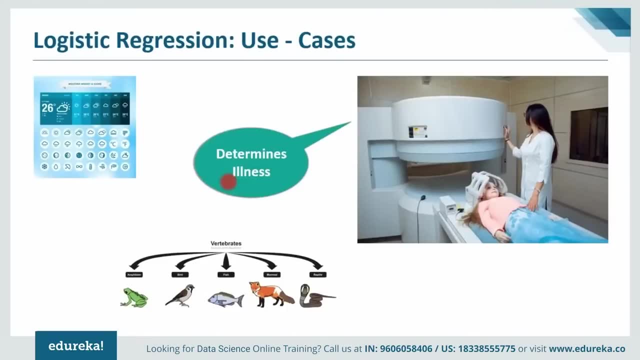 reptile. So in logistic regression it can perform multi-class classification. So this point I have already discussed, that it is used in classification problems. Next, it also helps you to determine the illness as well. So let me take an example. Let's say a patient goes for routine checkup in hospital. 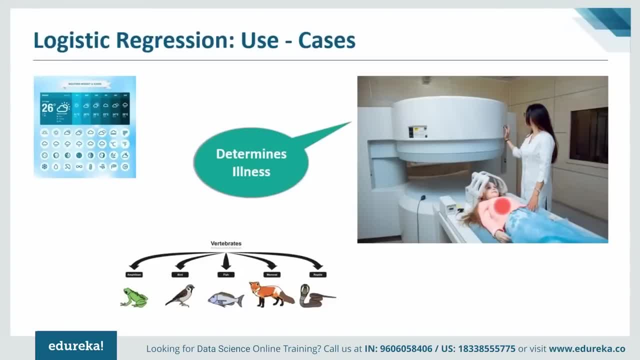 So what doctor will do? it will perform various tests on the patient and will check whether the patient is actually ill or not. So what will be the feature? So doctor can check the sugar level, the blood pressure. then what is the age of the patient? 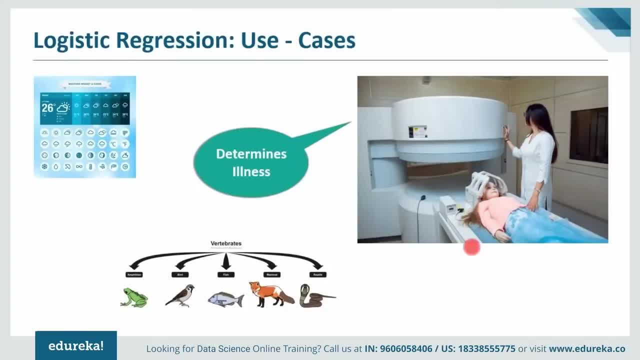 Is it very small or is it an old person? then, what is the previous medical history of that patient? and all of these features will be recorded by the doctor. and finally, doctor checks the patient data and determines the outcome of an illness and the severity of illness. 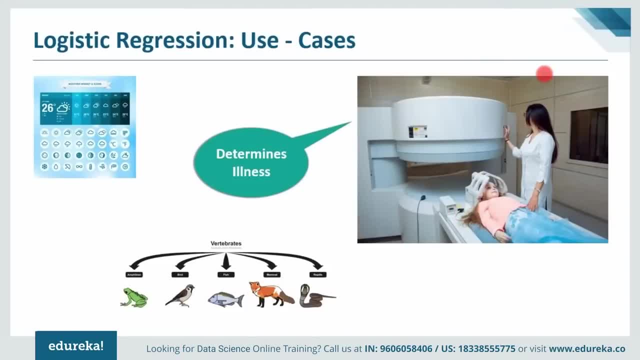 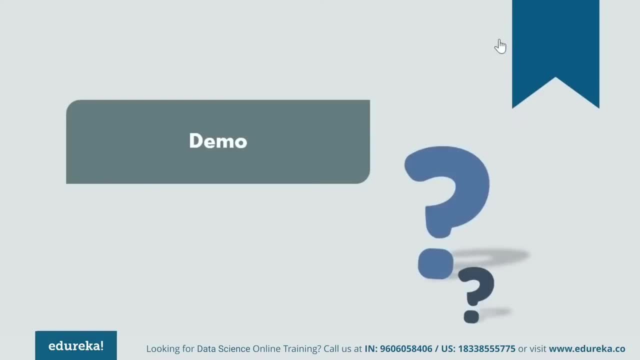 So, using all the data, a doctor can identify whether a patient is ill or not. So these are the various use cases in which you can use logistic regression. Now, I guess, enough of theory, But so let's move ahead and see some of the practical implementation. 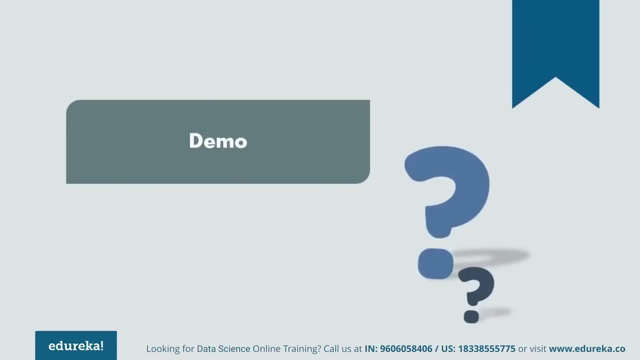 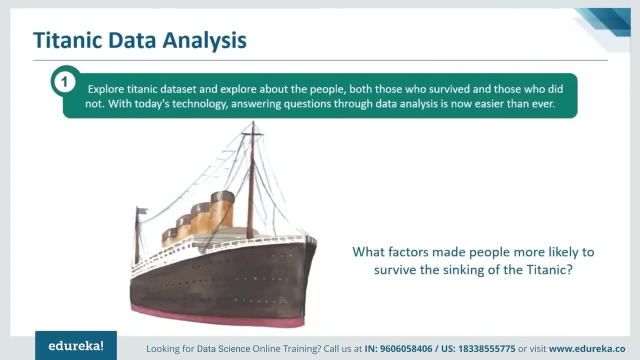 of logistic regression. So over here I'll be implementing two projects wherein I have the data set of a Titanic. over here will predict what factors made people more likely to survive the sinking of the Titanic ship and in my second project will see the data analysis on the SUV cars. 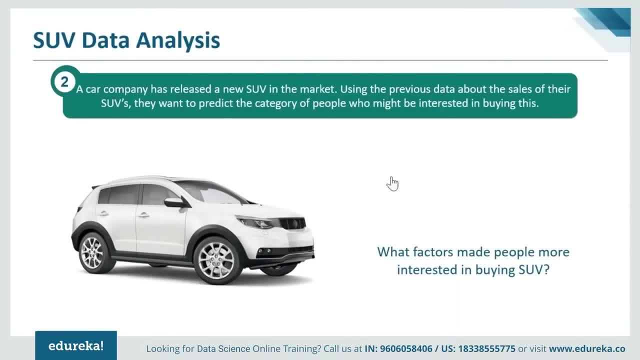 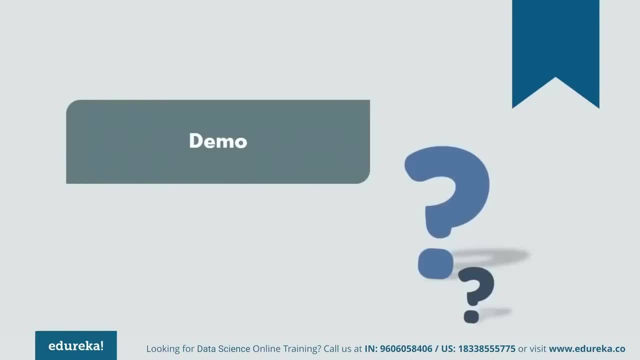 So over here we have the data of the SUV cars, who can purchase it and what factors made people more interested in buying SUV. So these will be the major questions as to why you should implement logistic regression and what output will you get by it. 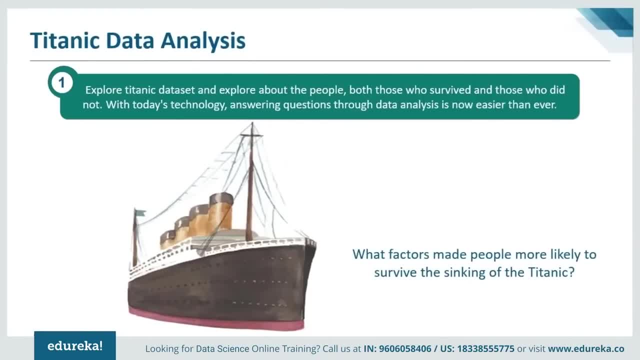 So let's start by the very first project, that is, Titanic data analysis. So some of you might know that there was a ship called as Titanic, which basically hit an iceberg and it sunk to the bottom of the ocean and it was a big disaster at that time because it was the 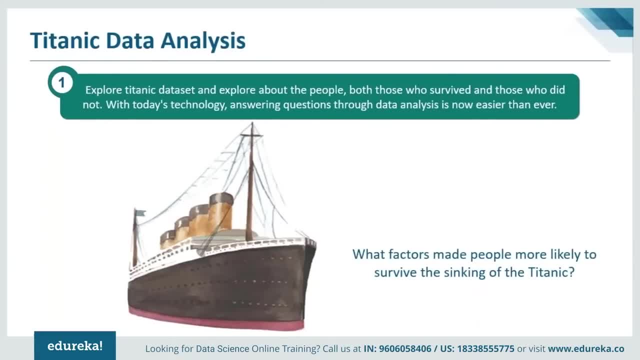 first voyage of the ship and it was supposed to be really, really strongly built and one of the best ships of that time. So it was a big disaster of that time And, of course, there's a movie about this as well, So many of you might have watched it. 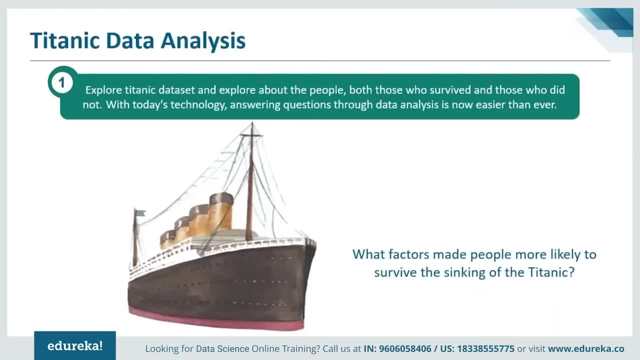 So what we have? we have data of the pattern Passengers, those who survived and those who did not survive in this particular tragedy. So what you have to do, you have to look at this data and analyze which factors would have been contributed the most to the chances. 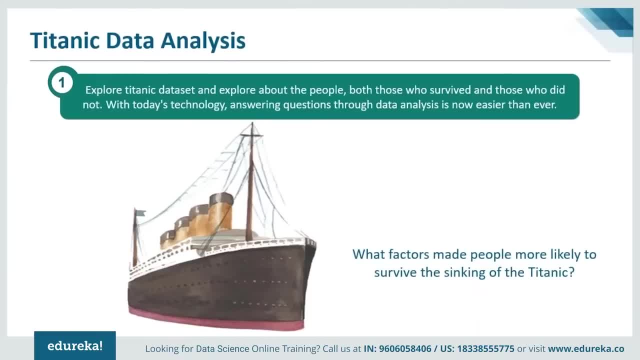 of a person, survival on the ship or not. So, using the logistic regression, we can predict whether the person survived or the person died. now, apart from this, we also have a look with the various features along with that. So first let us explore the data set. 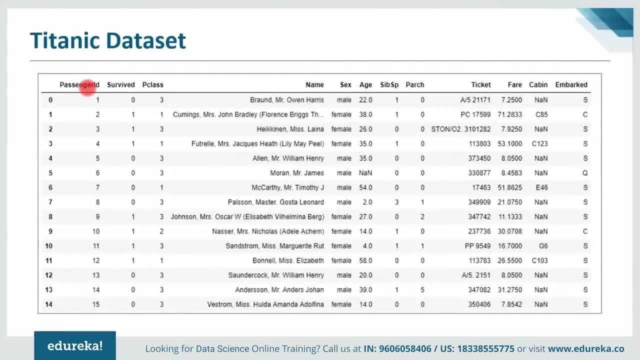 So over here we have the index value, then the first column is passenger ID, Then my next column is: So over here we have two values, a zero and a one. So zero stands for did not survive and one stands for survive. So this column is categorical, where the values are discrete. next, 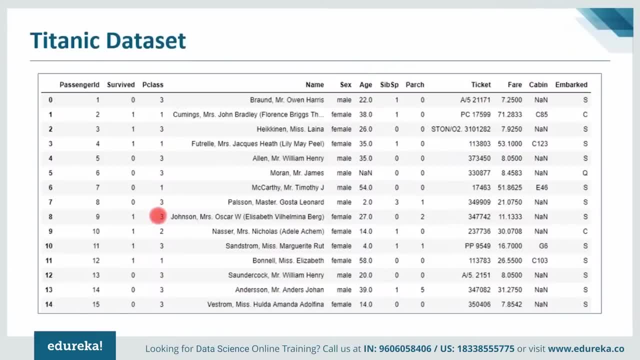 We have passenger class over here. We have three values: one, two and three. So this basically tells you that whether a passenger is traveling in the first class, second class or third class, then we have the name of the passenger, We have the sex or you can say the gender of the passenger. whether 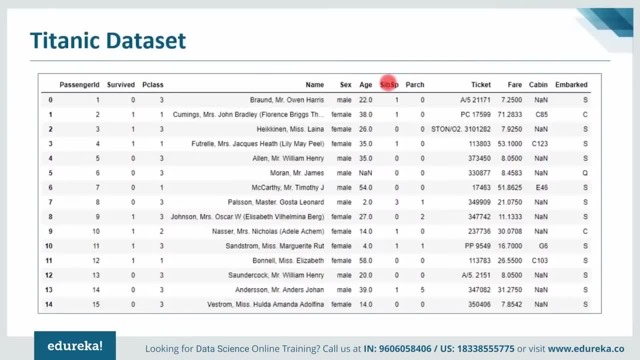 passenger is a male or female, then we have the age, we have the gender of the passenger, So this basically means the number of siblings or the spouses aboard the Titanic. So over here we have values such as one, zero and so on. then we have patch. 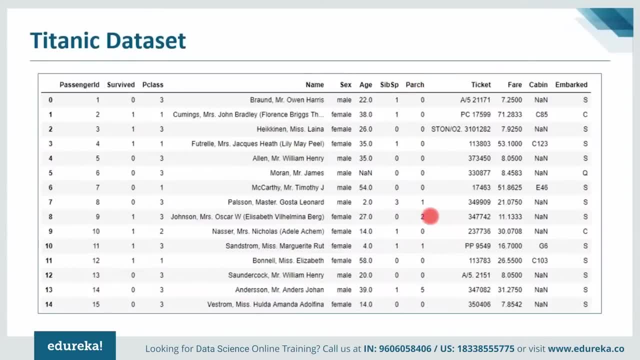 So patch is basically the number of parents or children aboard the Titanic over here. We also have some values. then we have the ticket number, We have the fare, We have the cabin number and we have the embarked column. So in my embarked column we have three values. 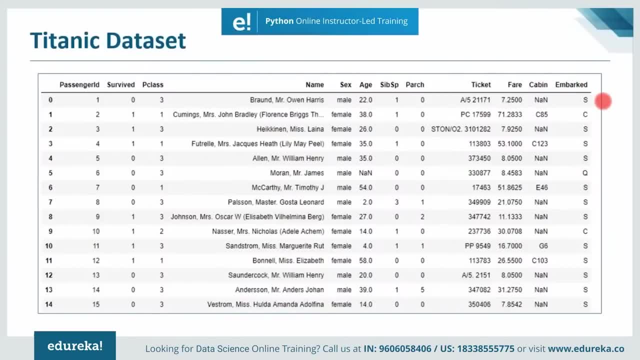 We have S, C and Q, so S basically stands for Southampton, C stands for Cherbourg and Q stands for Kuenstown. So these are the features that we'll be applying our model on, So here we will perform various steps and then we'll be implementing. 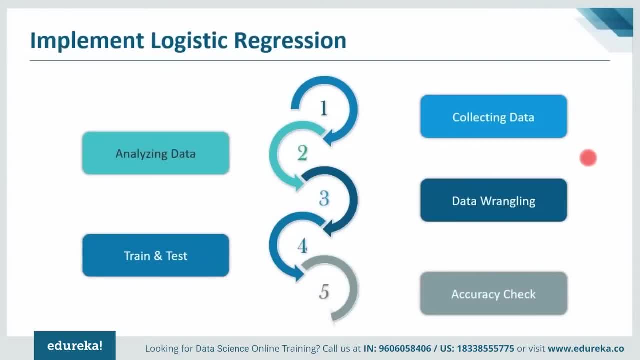 logistic regression. So now, these are the various steps which are required to implement any algorithm. So now, in our case, we are implementing logistic regression. So our very first step is to collect your data, or to import the libraries that are used for collecting your data and then taking 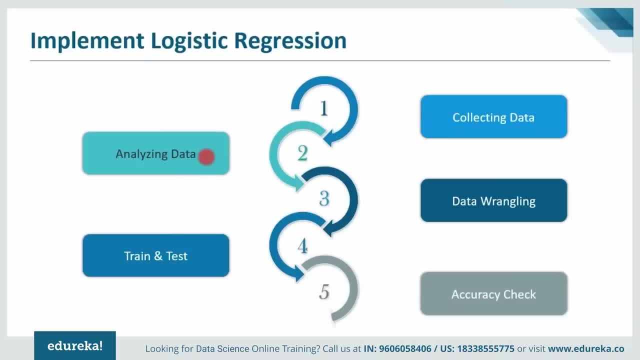 it forward. Then my second step is to analyze your data. So over here I can go through the various fields and then I can analyze the data. I can check: did the females or children survive better than the males, or did the rich passenger survive more than the poor passenger, or did 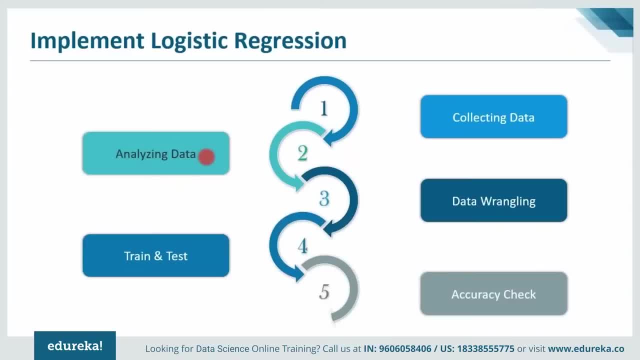 the money matter, as in who paid more to get into the ship, what they evacuated first and what about the workers? does the worker survived, or what is the survival rate if you were the worker in the ship and not just a traveling passenger? So all of these are very, very interesting questions and you would 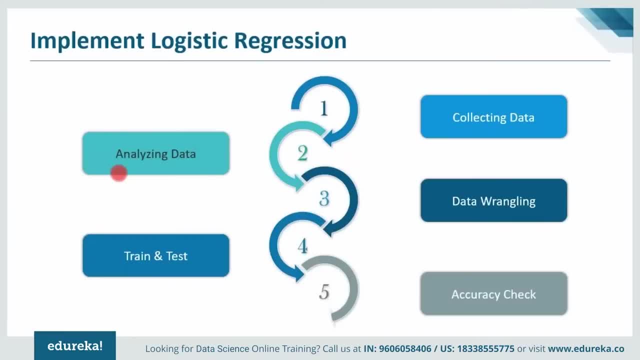 be going through all of them one by one. So in this stage you need to analyze your data and explore your data as much as possible As you can. then my third step is to wrangle your data Now. data wrangling basically means cleaning your data. 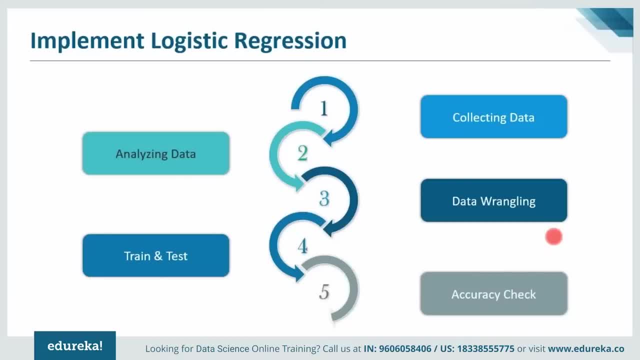 So over here you can simply remove the unnecessary items, or if you have a null values in the data set, you can just clear that data and then you can take it forward. So in this step you can build your model using the train data. 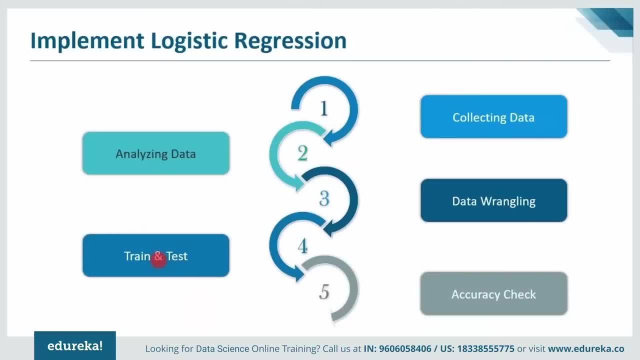 set and then you can test it using a test over here. You will be performing a split, which basically split your data set into training and testing data set, and finally, you will check the accuracy so as to ensure how much accurate your values are. So now let's go into all these steps in detail. 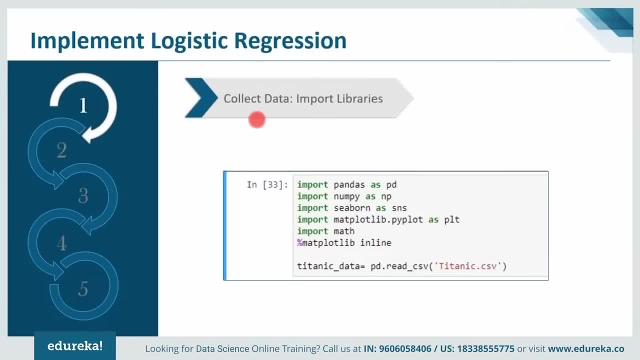 So, number one, we have to collect your data, or you can say, import the libraries. So it may show you the implementation part as well. So I'll just open my Jupiter notebook and I just implement all of these steps side by side. So, guys, this is my Jupiter notebook. 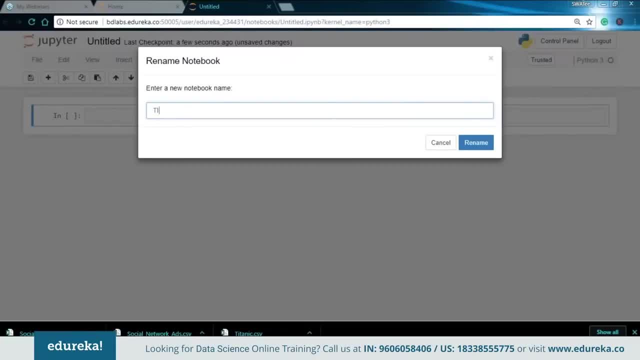 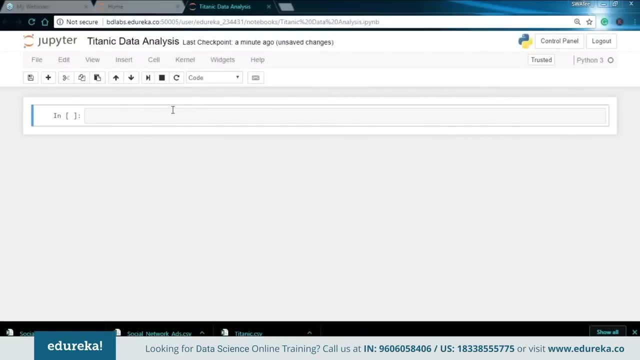 So first let me just rename Jupiter notebook to, let's say, Titanic data analysis. Now our first step was to import all the libraries and collect the data, So let me just import all the libraries first. So first of all I'll import pandas. 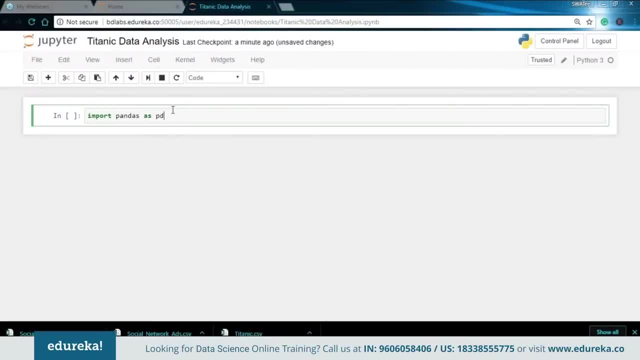 So pandas is used for data analysis. So I'll say: import pandas as PD. then I'll be importing numpy, So I'll say: import numpy as NP. So numpy is a library in Python which basically stands for numerical Python and it is widely used to perform any scientific 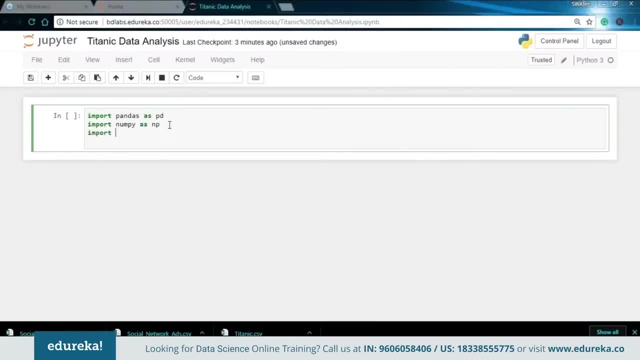 computation. Next we will be importing Seaborn. So Seaborn is a library for statistical plotting. So I'll say: import Seaborn as SNS. I'll also import matplotlib, So matplotlib library is again for plotting. So I'll say: import matplotlib, dot by plot, as PLD. 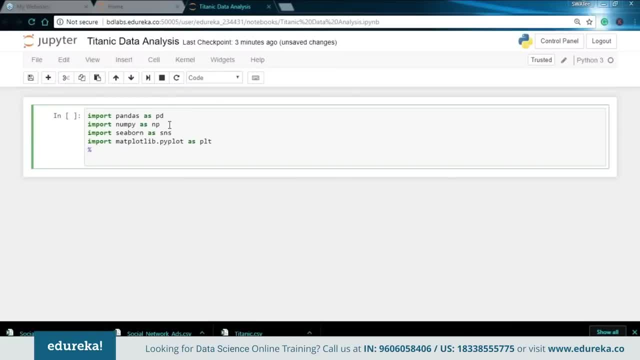 Now to run this library in Jupiter notebook, All I have to write in is percentage matplotlib inline. Next, I'll be importing one module as well So as to calculate the basic mathematical functions. so I'll say: import maths. So these are the libraries that I'll be needing in this Titanic. 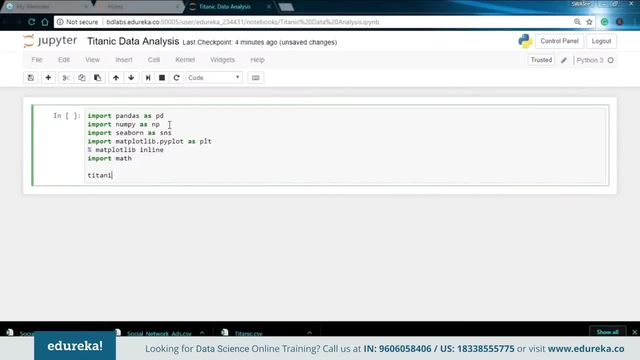 data analysis. So now let me just import my data set. So I'll take a variable, Let's say Titanic data, and using the pandas I will just read my CSV, or you can say the data set. I'll write the name of my data set, that is, Titanic dot CSV. 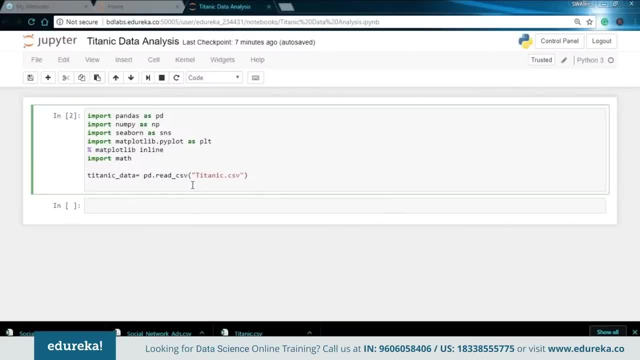 Now I have already showed you the data set, So over here let me just print the top 10 rows. So for that I'll just say: I'll take the variable Titanic data dot head and I'll say the top 10 rows. So now I'll just run this. 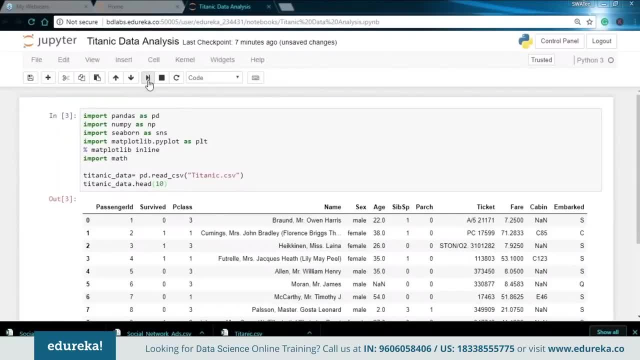 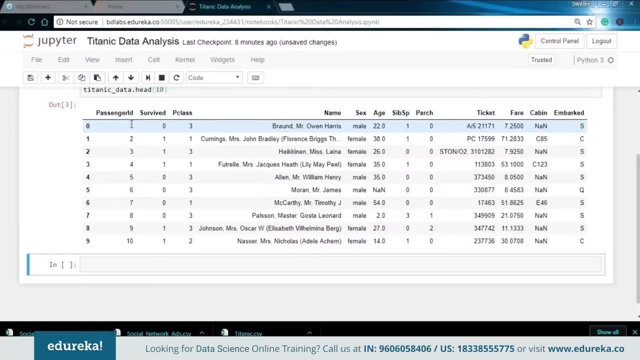 So to run this I just have to press shift plus enter, or else you can just directly click on the cell. So over here I have the index, We have the passenger ID, which is nothing but again the index which is starting from 1. then we have the survive column, which 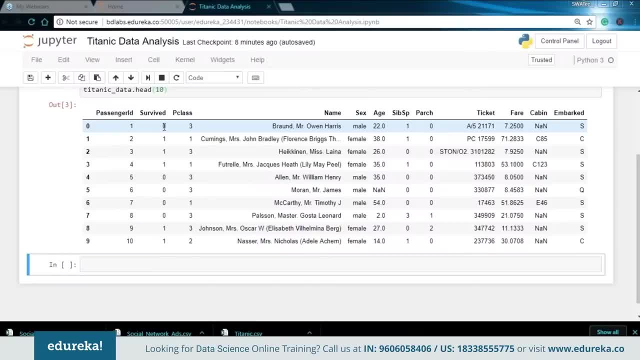 has the categorical values, or you can say the discrete values, which is in the form of 0 or 1. then we have the passenger class, We have the name of the passenger, sex, age and so on. So this is the data set that I'll be going forward with next. 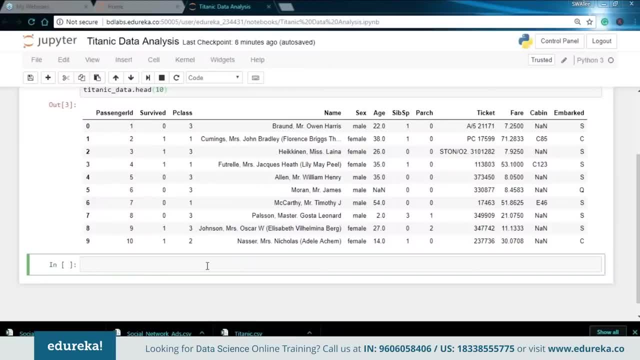 Let us print the number of passengers which are there in this original data set. for that I'll just simply type in print. I'll say number of passengers And using the length function I can calculate the total length. So I'll say length and inside this I'll be passing this variable. 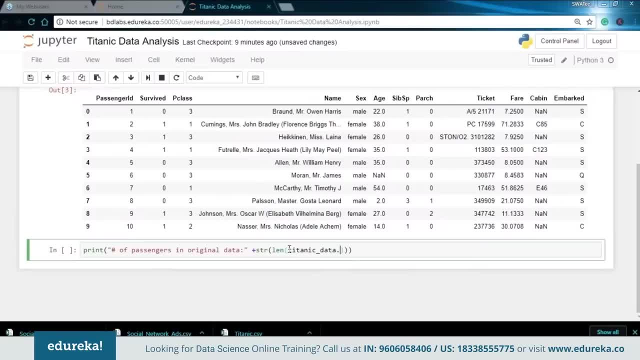 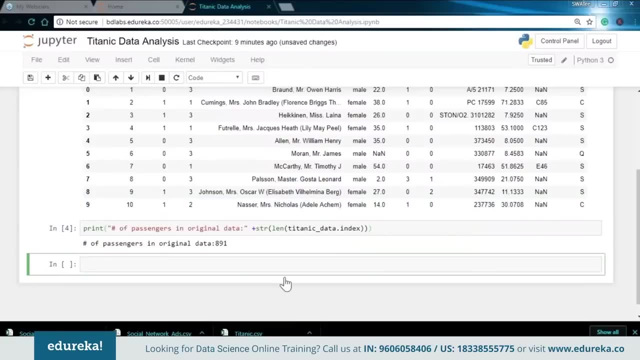 which is Titanic data, So I'll just copy it from here. I just paste it dot index and next let me just print this one. So here the number of passengers which are there in the original data set we have is 891.. So around this number were traveling in the Titanic ship. 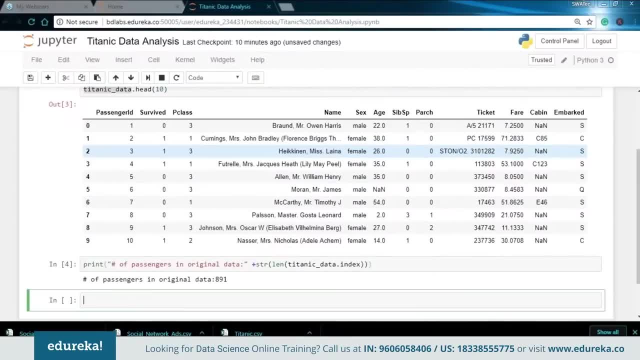 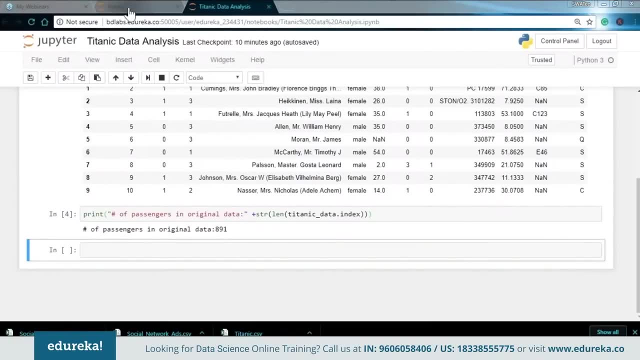 So over here, my first step is done, where you have just collected data, imported all the libraries and find out the total number of passengers which are traveling in Titanic. So now let me just go back to presentation and let's see what is my next step. 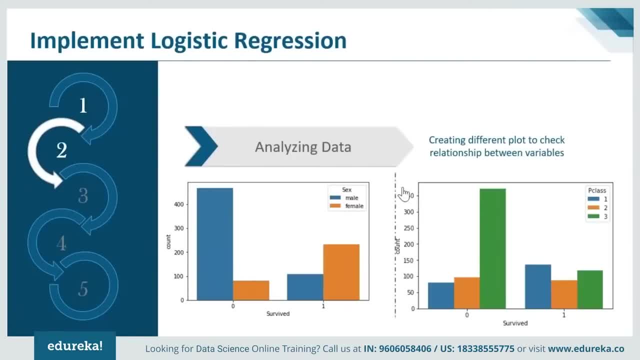 So we're done with the collecting data. Next step is to analyze your data. So over here we'll be creating different plots to check the relationship between variables, as in how one variable is affecting the other. So you can simply explore your data set by making use of. 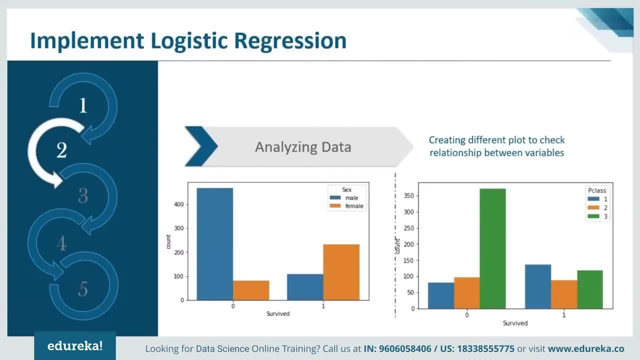 various columns and then you can plot a graph between them. So you can either plot a correlation graph, You can plot a distribution graph. It's up to you guys. So let me just go back to my Jupyter notebook and let me analyze some of the data over here. 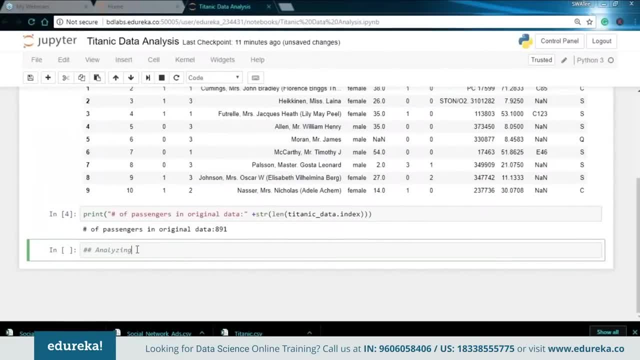 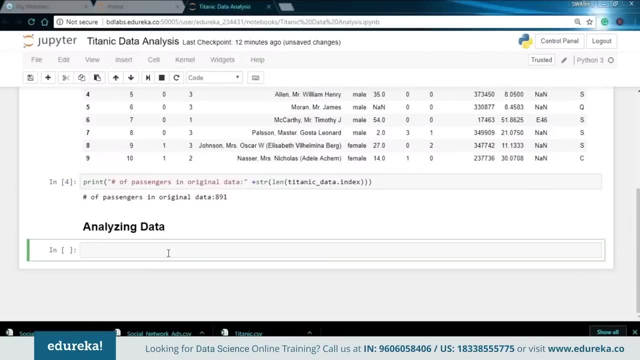 My second part is to analyze data, So I just put this in header 2.. Now, to put this in header 2, I just have to go on code, click on markdown and I just run this. So first let us plot a count. plot where you compare between the 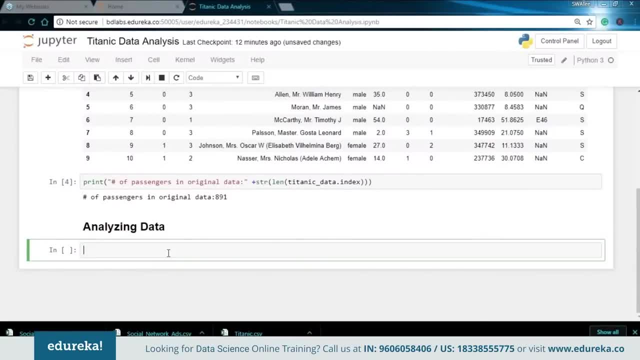 passengers who survived and who did not survive. So for that I'll be using the seaborn library. So over here I have imported seaborn as SNS, So I don't have to write the whole name. I'll simply say SNS dot count plot. 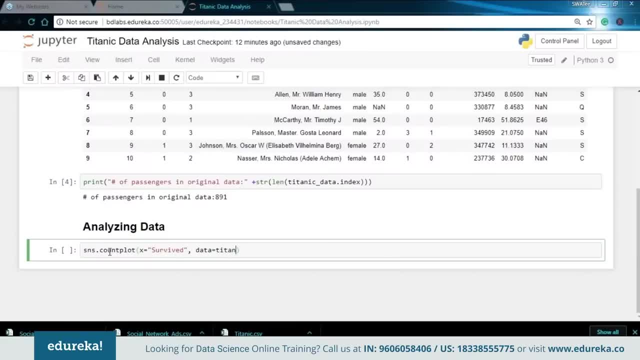 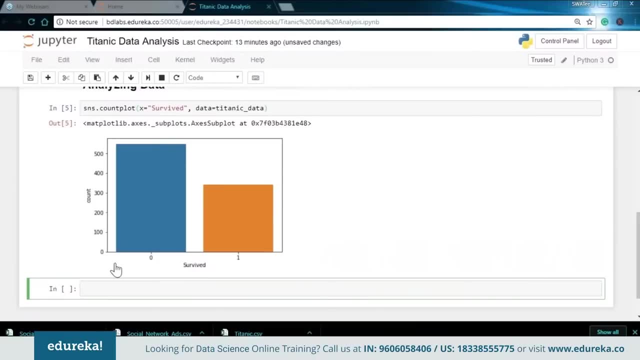 I'll say X is who survived, And the data that I'll be using is the Titanic data, or you can say the name of variable in which you have stored your data set. So now let me just run this So over here. as you can see, I have survived. column on my x-axis. 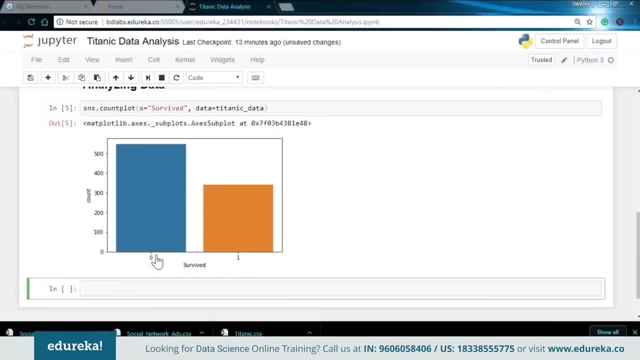 and on the y-axis I have the count. so 0 basically stands for did not survive and one stands for the passengers who did survive. over here You can see that around 550 of the passengers who did not survive and they were around 350 passengers who only survive. 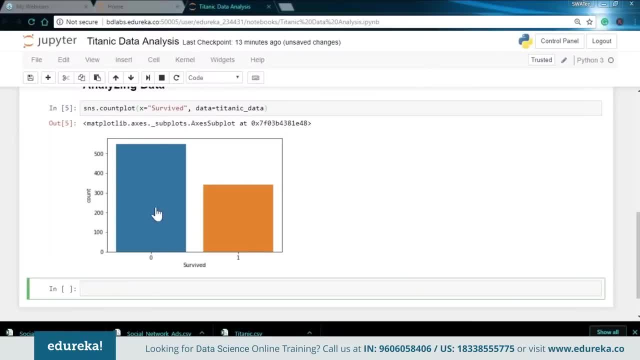 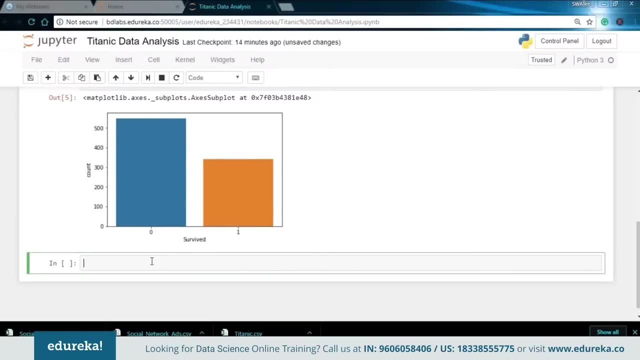 So here you can basically conclude that there are very less survivors And non-survivors. So this was the very first plot. Now there is not another plot to compare the sex as to whether, out of all the passengers who survived and who did not survive, how many. 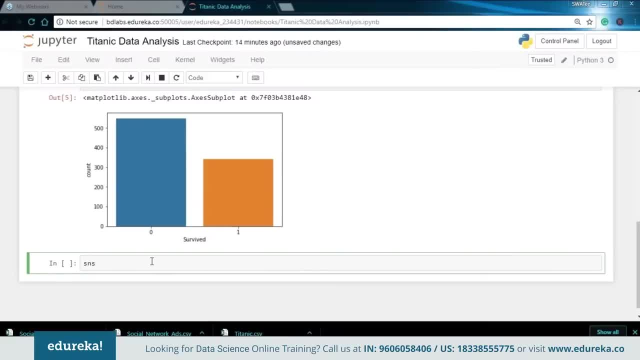 were men and how many were female. So to do that, I'll simply say SNS dot count plot. I add the hue as sex. So I want to know how many females and how many males survive. then I'll be specifying the data. 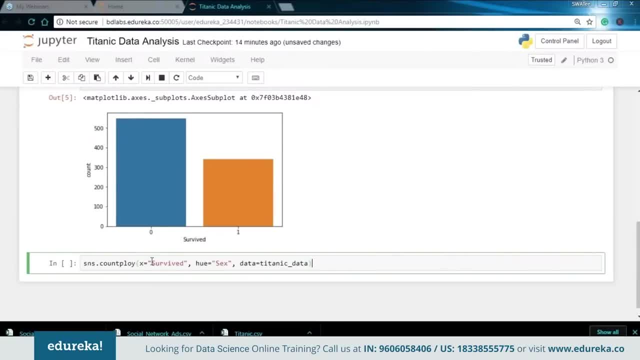 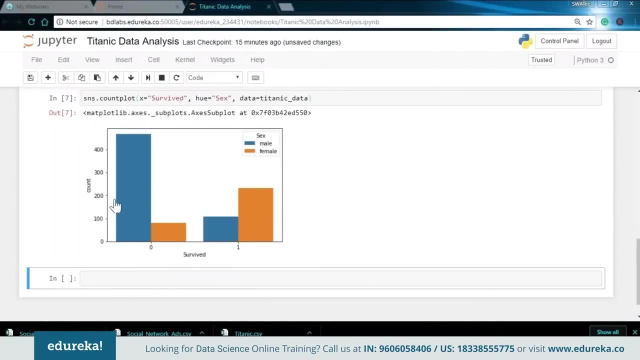 So I am using Titanic data set And let me just run this. Okay, I've done a mistake over here, So over here you can see I have survived column on the x-axis and I have the count on the Y now. So here your blue color stands for your male passengers, and orange. 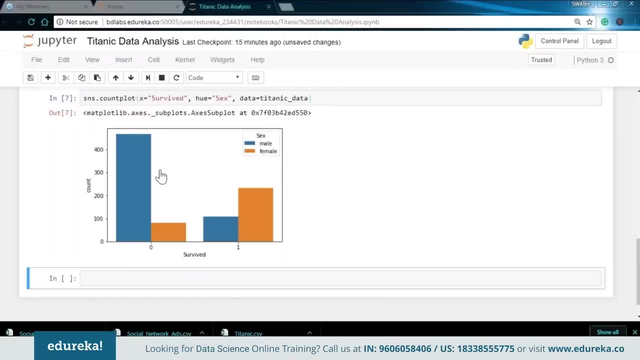 stands for your female. So, as you can see here the passengers who did not survive, that has a value 0. so we can see that majority of males did not survive and if we see the people who survived here, we can see the majority of females. 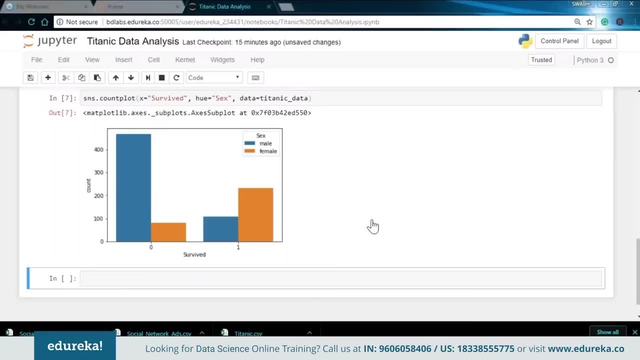 survive. So this basically concludes the gender of the survival rate. so it appears, on average women were more than three times more likely to survive than men. next Let us plot another plot where we have the hue as the passenger class. So over here we can see which class at the passenger was traveling in. 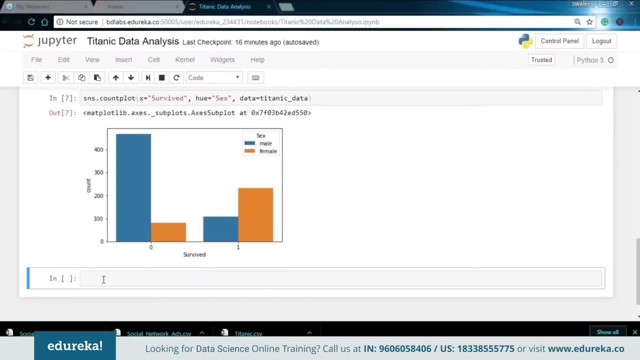 whether it was traveling in class 1, 2 or 3.. So for that I'll just write the same command. I'll say SNS dot count plot. I'll keep my x-axis as sub, only I'll change my hue to passenger class. 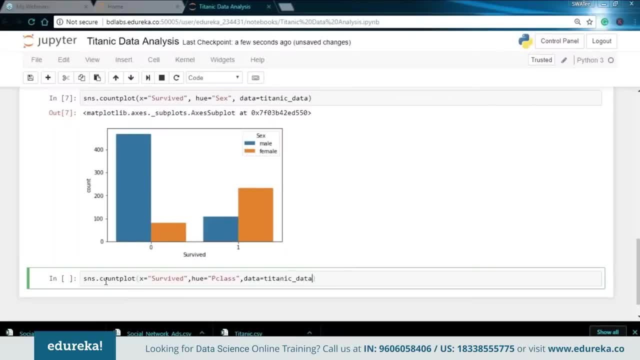 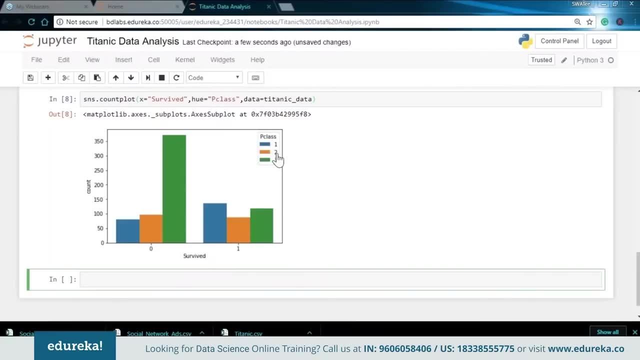 So my variable is named as P class And the data said that I'll be using this Titanic data. So this is my result. So over here you can see I have blue for first class, orange for second class and green for the third class. 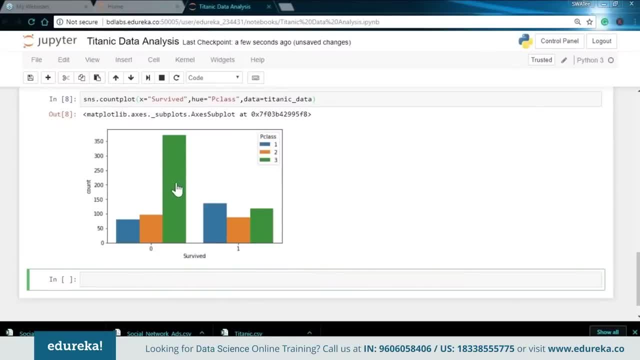 So here the passengers who did not survive were majorly of the third class, or you can say the lowest class or the cheapest class to get into the Titanic, and the people who did survive majorly belong to the higher classes. So here one and two has more rise than the passenger who were traveling. 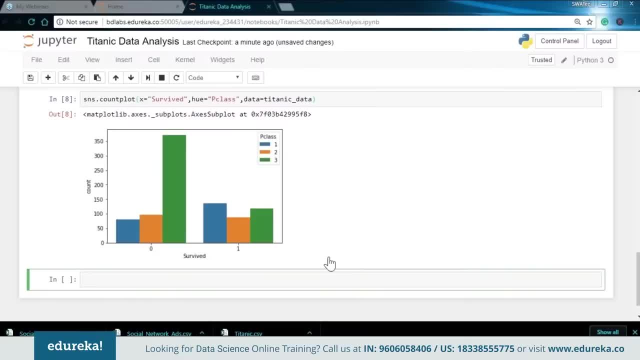 in the third class. So here we have concluded that the passengers who did not survive were majorly of third class, or you can say the lowest class, and the passengers who were traveling in first and second class would tend to survive more. next Let us plot a graph for the age distribution over here. 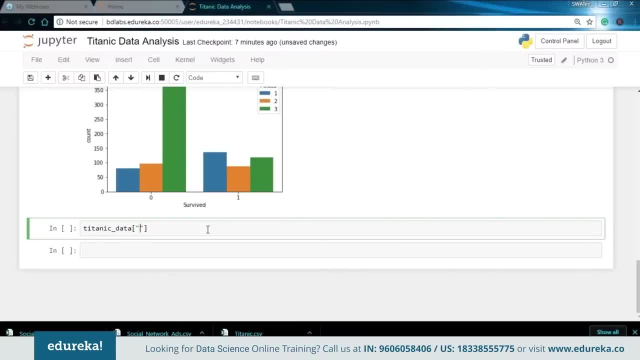 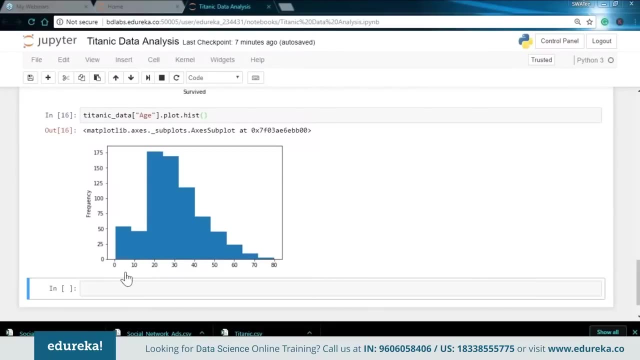 I can simply use my data. So we'll be using pandas library for this. I'll declare an array and I'll pass in the column. that is age, So I plot and I want a histogram, So I'll say plot dot hist, So you can notice over here that we have more of young passengers, or you. 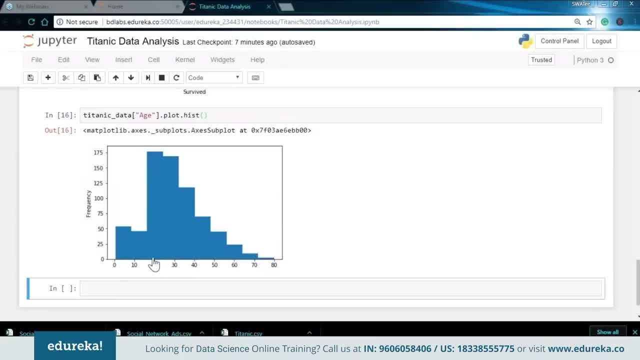 can see the children between the ages 0 to 10, and then we have the average age people and if you go ahead, lesser would be the population. So this is the analysis on the age column. So we saw that we have more young passengers and more mediocre age. 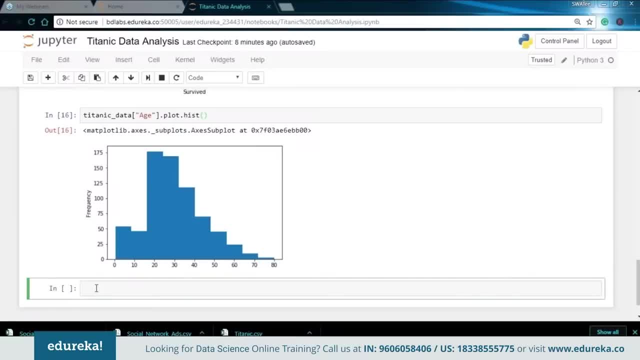 passengers which are traveling in the Titanic. So next let me plot a graph of air as well, So I'll say Titanic data. I'll say fair, and again I'll plot a histogram, So I'll say hist. So here you can see, the fair size is between: 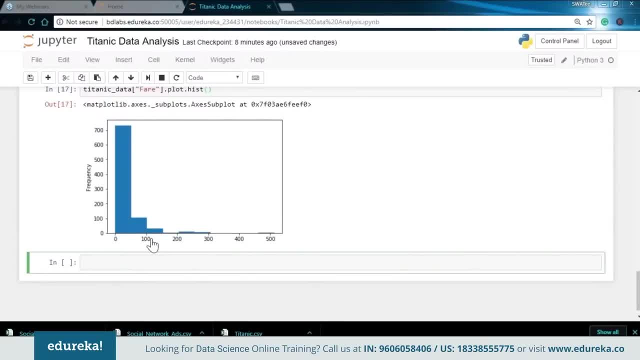 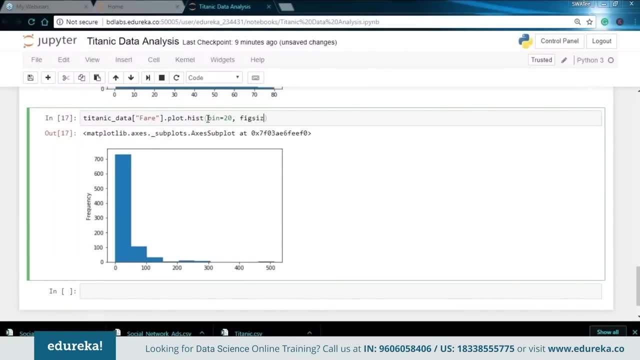 0 to 100.. Now let me add the bin size so as to make it more clear over here. I'll say bin is equals to, let's say, 20, and I'll increase the figure size as well, So I'll say fig size. 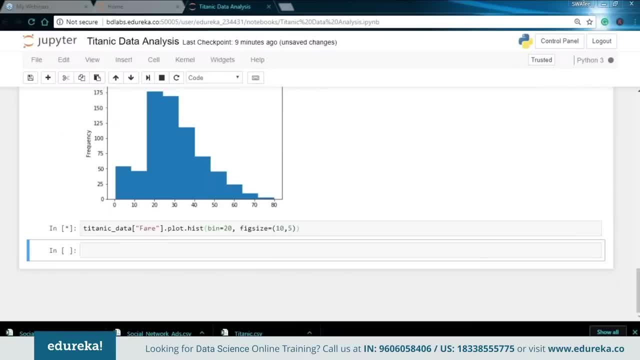 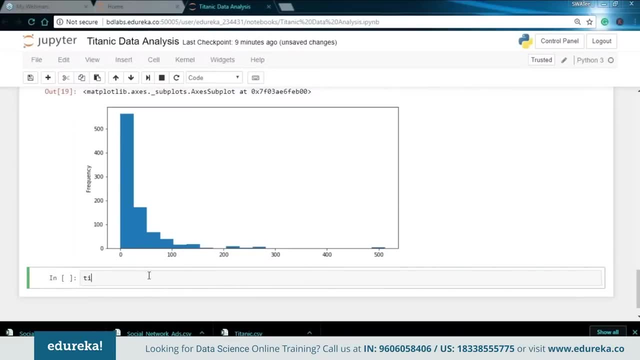 Let's say I give the dimensions as 10 by 5. So it is bins. So this is more clear now. next Let us analyze the other columns as well. So I'll just type in Titanic data, and I want the information as to what. 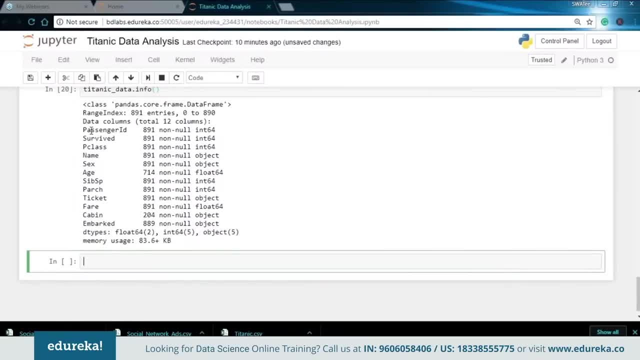 all columns are left. So here we have passenger ID, which I guess it's of no use. then we have see how many passengers survived and how many did not. we also see the analysis on the gender basis. We saw when the female tend to survive more or the men tend to survive. 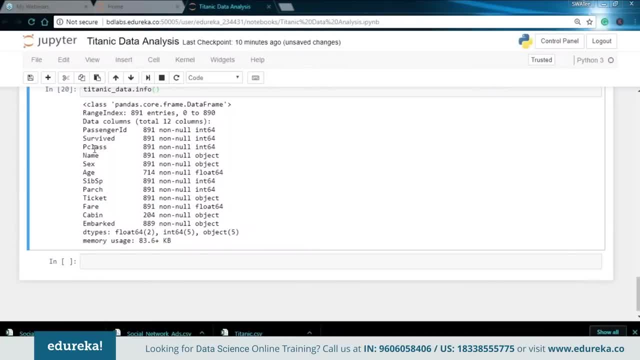 more. then we saw the passenger class, where the passenger is traveling in the first class, second class or third class. then we have the name. So in name we cannot do any analysis. We saw the sex. We saw the age as well. Then we have Sib SP. 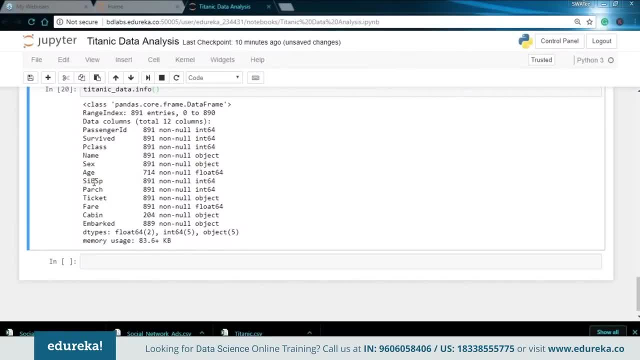 So this stands for the number of siblings, or the spouses, Which are aboard the Titanic. So let us do this as well. So I'll say snscom plot, I'll mention X as Sib, SP And I'll be using the Titanic data. 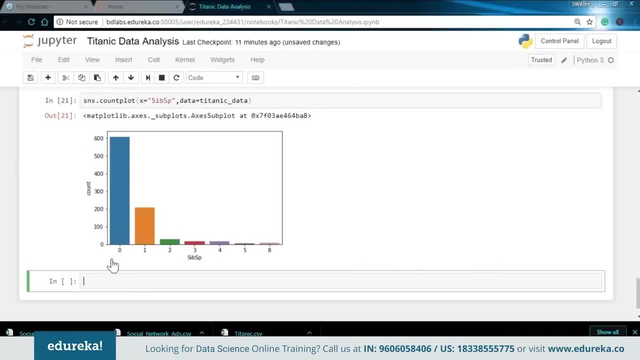 So you can see the plot over here. So over here you can conclude that it has the maximum value on zero. so you can conclude that neither a children nor a spouse was on board the Titanic. now, second most highest value is one, and then we have very less values for. 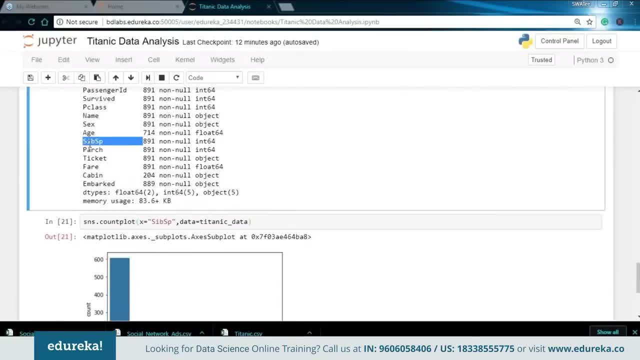 two, three, four and so on. Next, if I go above, we saw this column as well. Similarly, you can do for part, So next we have parts. or you can say the number of parents or children which were aboard the Titanic. So you, similarly, can do this as well. 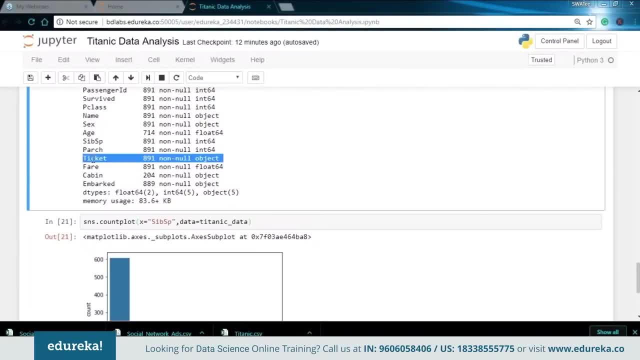 Then we have the ticket number, So I don't think so Any analysis is required for ticket. Then we have fair, so fair. We have already discussed as in, the people who tend to travel in the first class usually pay the highest fare. Then we have the cabin number and we have embarked. 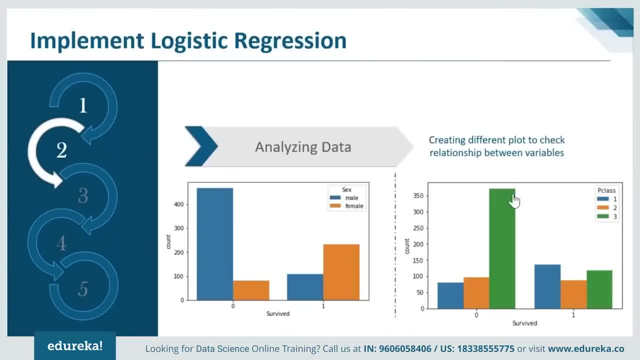 So these are the columns that will be doing data wrangling on. so we have analyzed the data And we have seen quite a few graphs in which we can conclude which variable is better than another or what is the relationship they hold. So third step is my data wrangling. 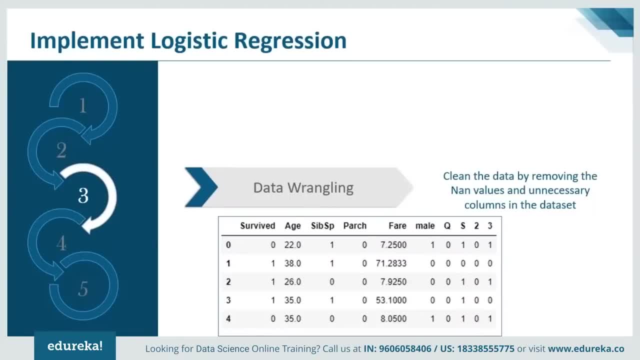 So data wrangling basically means cleaning your data. So if you have a large data set, you might be having some null values or you can say any and values. So it's very important that you remove all the unnecessary items that are present in your data set. 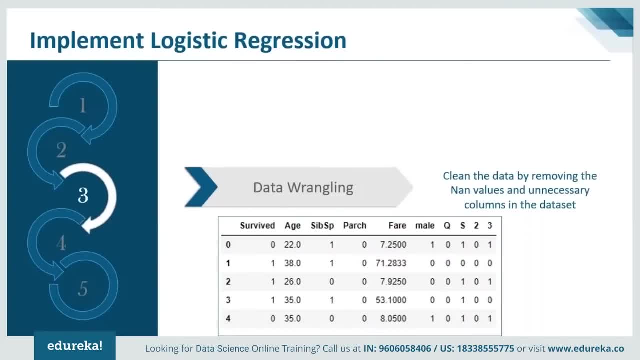 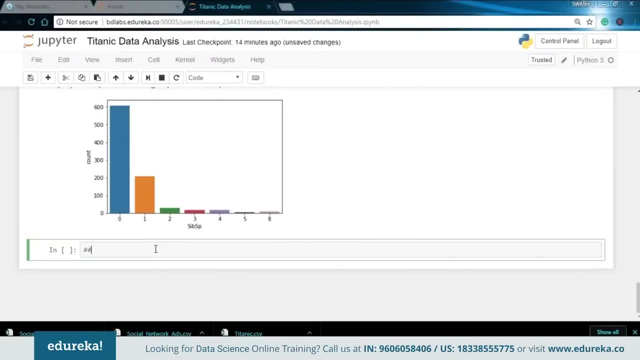 So removing this directly affects your accuracy. So I'll just go ahead and clean my data by removing all the NAN values and unnecessary columns, which has a null value in the data set. So next I'll be performing data wrangling. So first of all, 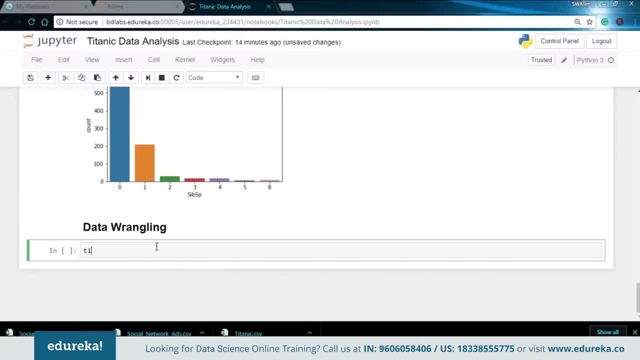 I'll check whether my data set is null or not. So I'll say Titanic data, which is the name of my data set, and I'll say is null. So this will basically tell me what all values are null and it will return me a boolean result. 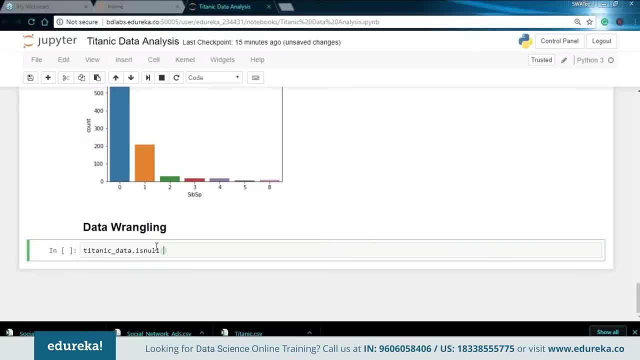 So this basically checks the missing data and your result will be in boolean format. as in, the result will be true or false. So false mean if it is not true, not none. and true means if it is null. So let me just run this. 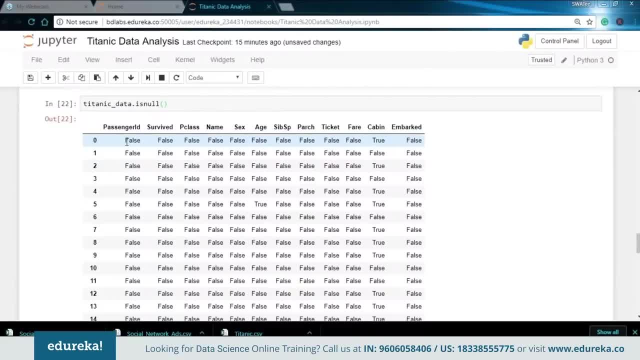 Over here you can see the values as false or true. So false is where the value is not null and true is where the value is none. So over here you can see, in the cabin column We have the very first value, which is null. 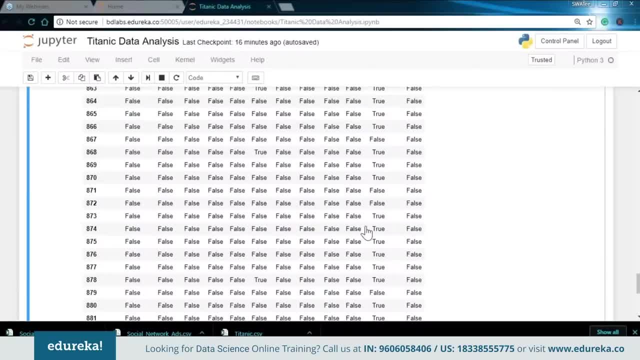 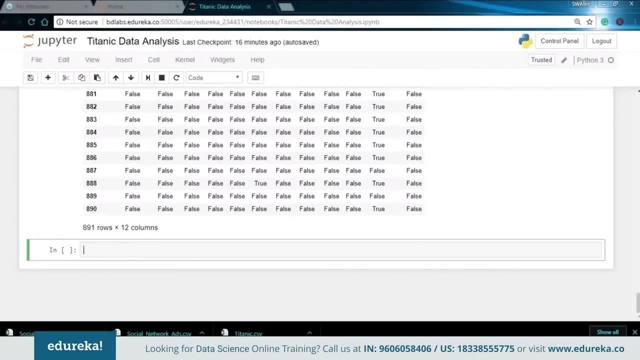 So we have to do something on this So you can see that we have a large data set, So the counting does not stop and we can actually see the sum of it. We can actually print the number of passengers who have the NAN value. 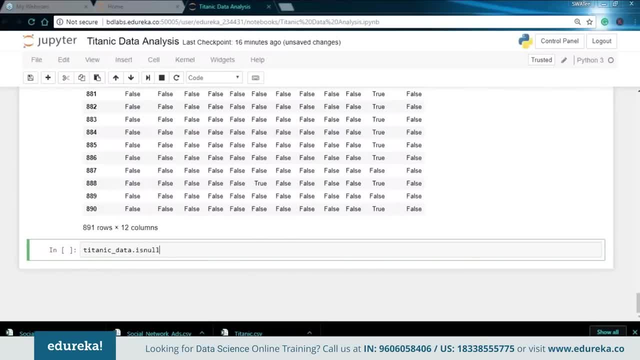 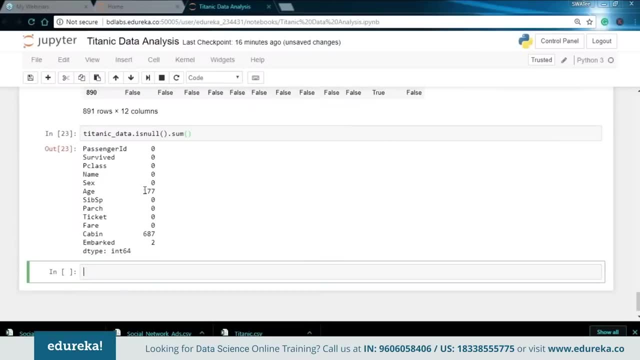 In each column. So I'll say: Titanic underscore data is null and I want the sum of it. Well, say dot sum. So this will basically print the number of passengers who have the NAN values in each column. So we can see that we have missing values in each column. 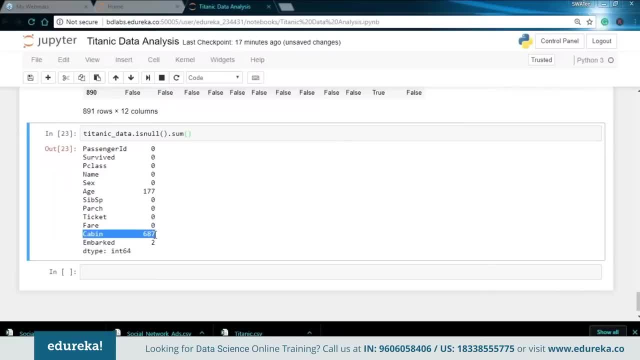 That is 177.. Then we have the maximum value in the cabin column and we have very less in the impact column, That is 2.. So here, if you don't want to see this numbers, you can also plot a heat map and then you can visually analyze it. 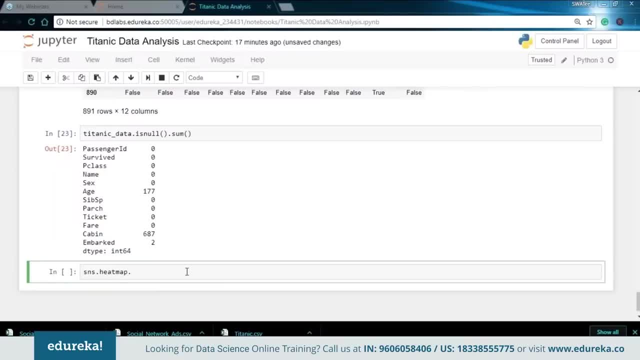 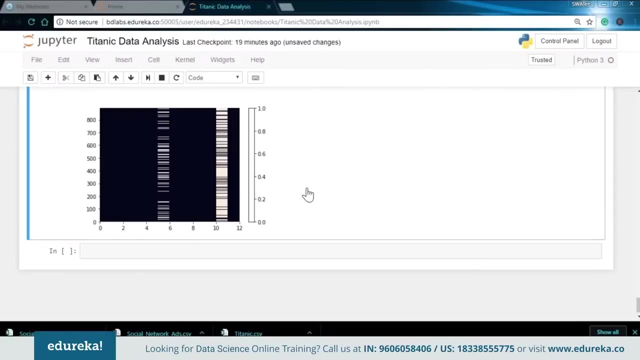 So let me just do that as well. So I'll say sns, Not heat map. I'll say why tick labels falls. So I'll just run this So, as we have already seen that there were three columns in which missing data value was present, 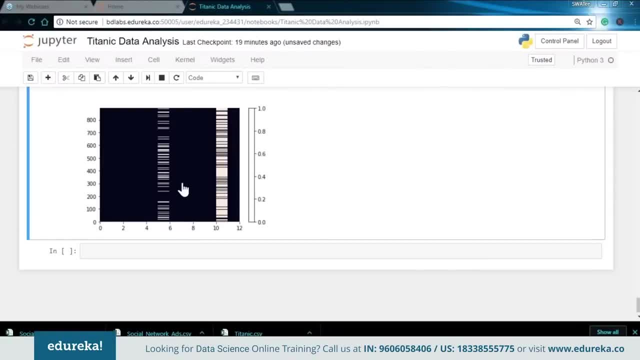 So this might be age. So over here, almost 20% of age column has a missing value. Then we have the caping columns. So this is quite a large value, and then we have two values for impact column as well. Add a C map for color coding. 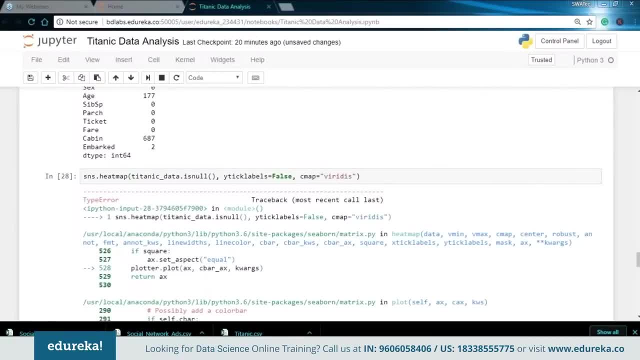 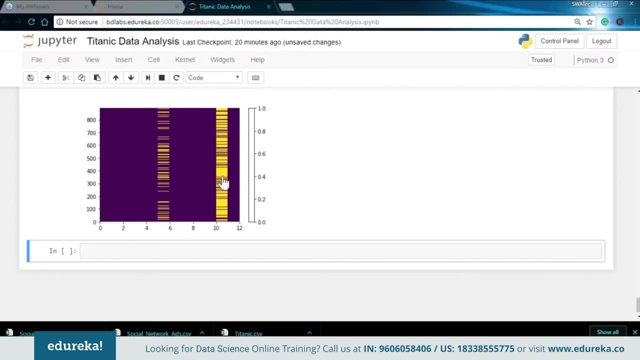 So I'll say C map. So if I do this, so the graph becomes more attractive. So over here your yellow stands for true, or you can say the values are null. So here we have concluded that we have the missing value of age. 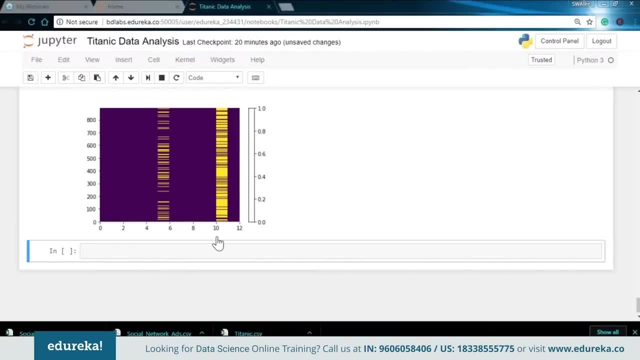 We have a lot of missing values in the cabin column and we have very less value which is not even visible in the embark column as well. So to remove these missing values, you can either replace the values and you can put in some dummy values to it, or you can simply drop the. 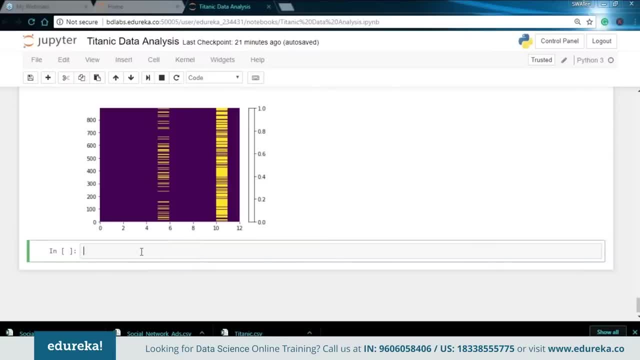 column. So here let us first pick the age column. So first let me just plot a box plot and they will analyze with having a column as age. So I'll say SNS dot box plot. I'll say X is equals to passenger class. 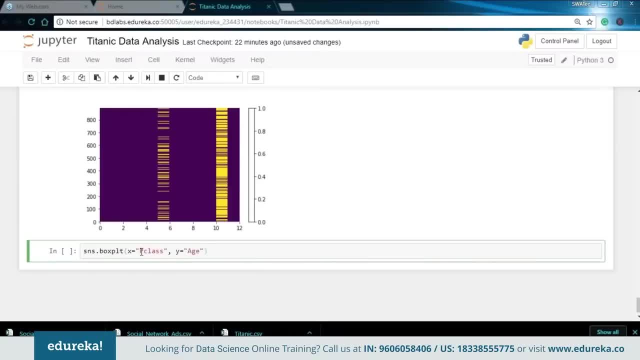 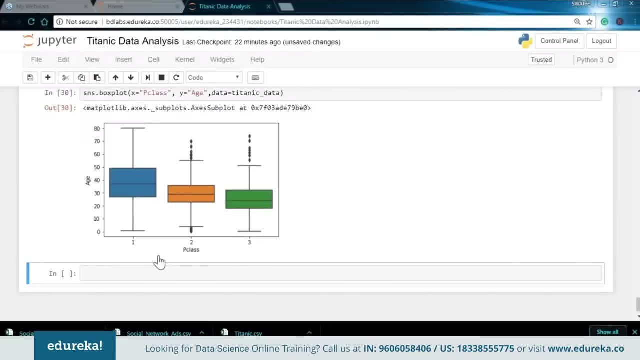 So it's P class. I'll say Y is equals to age and the data set that I'll be using is Titanic set. So I'll say data is equals to Titanic data. You can see the age in first class and second class tends to be more older. 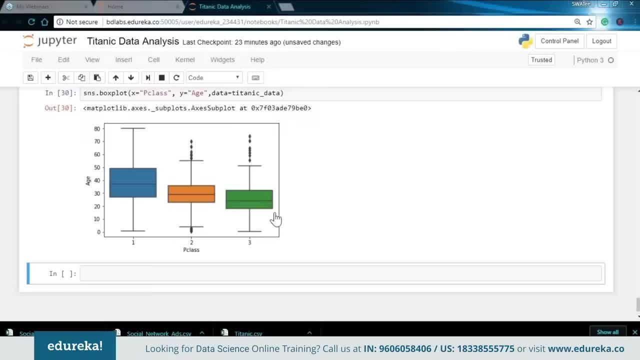 rather than we have it in the third class. Well, that depends on the experience, how much you own or might be. there n number of reasons. So here we concluded that passengers who were traveling in class 1 and class 2 are tend to be older than what we have in the class 3.. 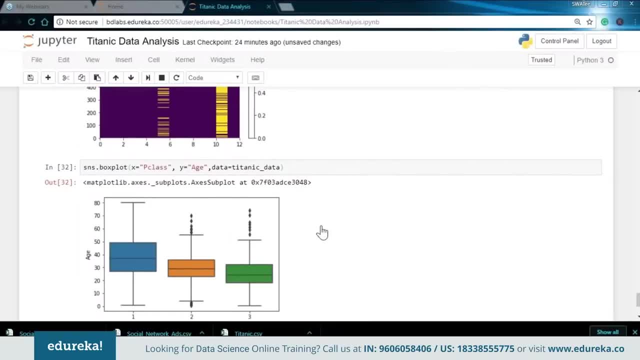 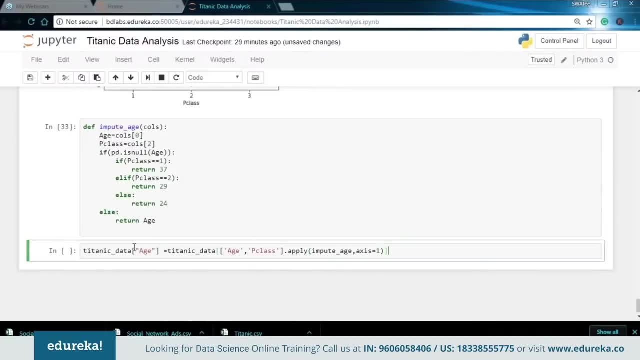 So we have found that we have some missing values in M. Now one way is to either just drop the column or you can just simply fill in some values to them. So this method is called as imputation. now to perform data wrangling or cleaning: 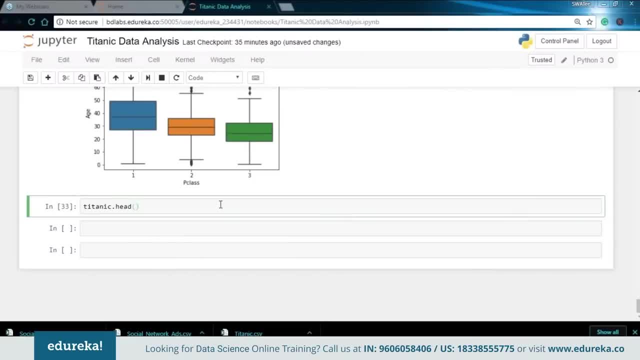 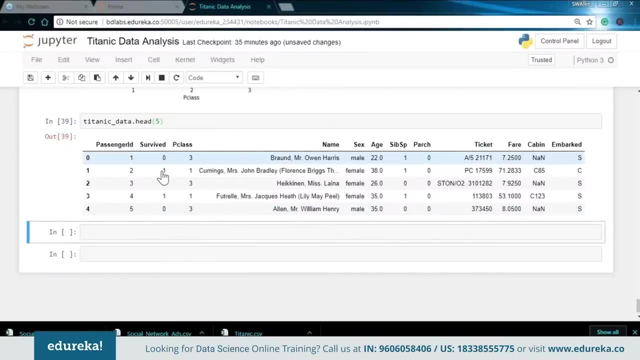 It is supposed to print the head of the data set. So I'll say Titanic, not head, So it's Titanic underscore data. Let's say I just want the five rows. So here we have survived, which is again categorical. So in this particular column I can apply logistic regression. 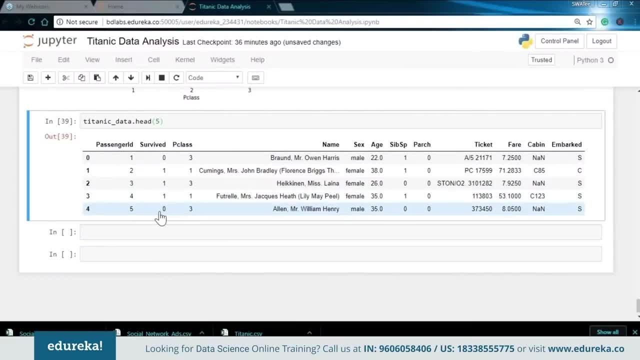 So this can be my Y value or the value that you need to predict. Then we have the passenger class, We have the name, then we have ticket number pair, cabin. So over here we have seen that in cabin We have a lot of null values or you can say the NAN values is quite visible. 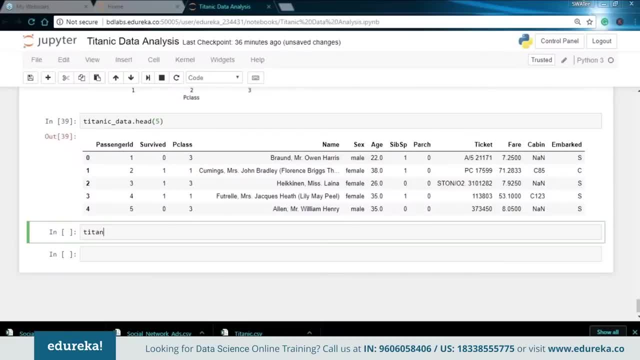 as well. So, first of all, we'll just drop this column. So, dropping it, I'll just say Titanic underscore data and I'll simply type and drop and the column which I need to drop. So I have to drop the cabin column. 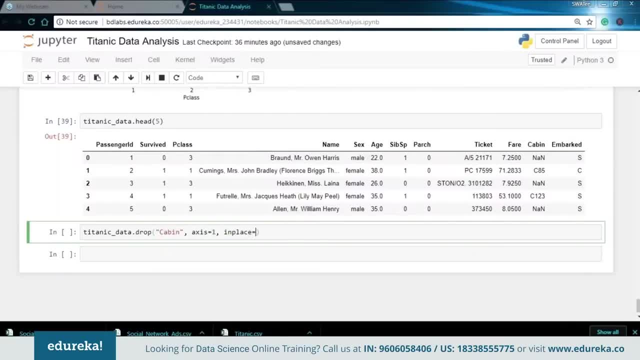 I'll mention the axis equals to one and I'll say in place also to true. So now again, I'll just print the head and let us see whether this column has been removed from the data set or not. So I'll say Titanic, not head. 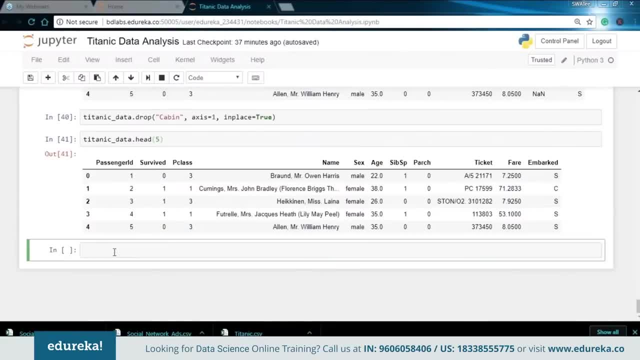 So, as you can see here, we don't have cabin column anymore. Now you can also drop the NA values. So I'll say: Titanic, data Dot, drop all the NA values. or you can say NAN, which is not a number, and I'll say: in place is equals to true. 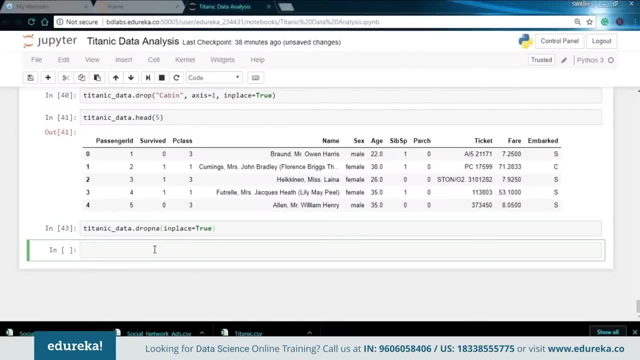 It's Titanic. So over here let me again plot the heat map and let's say what the values which are before showing a lot of null values. has it been removed or not? So I'll say SNS dot heat map, I'll pass in the data set. 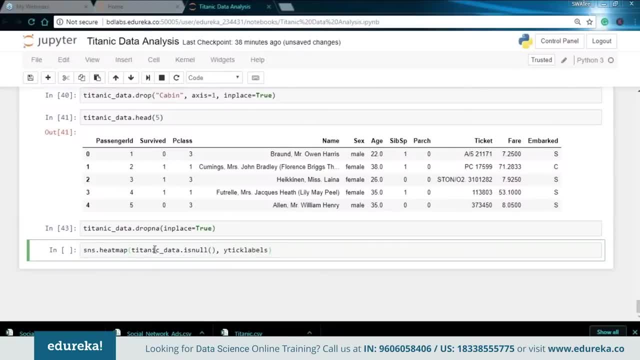 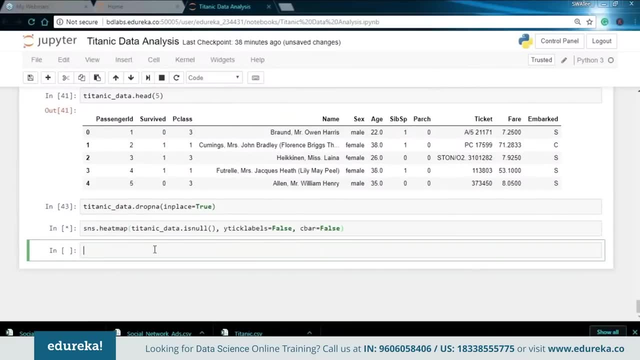 I'll check. it is null, I'll say y tick labels is equals to false And I don't want color coding, So again I'll say False. So this is basically helped me to check whether my values has been removed from the data set or not. 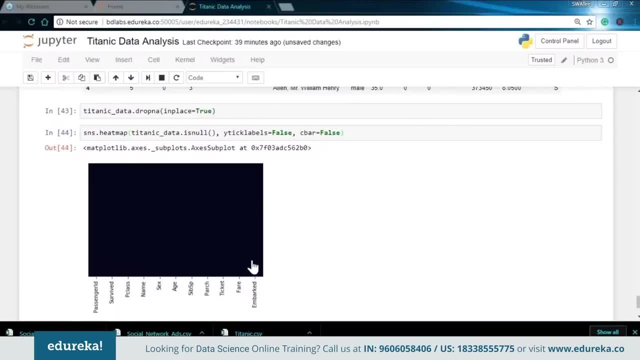 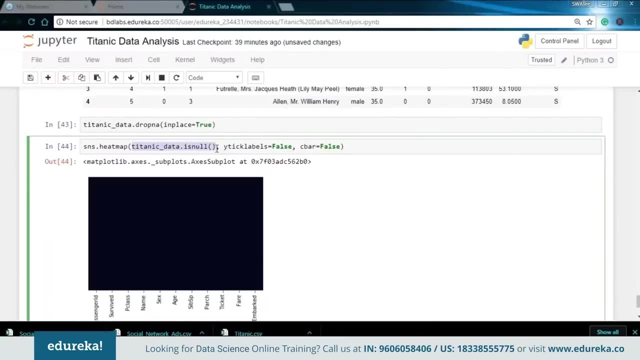 So, as you can see, here I don't have any null values, So it's entirely black. Now you can actually know the sum as well, So I just go above. So I'll just copy this part and I just use the sum function to calculate the sum. 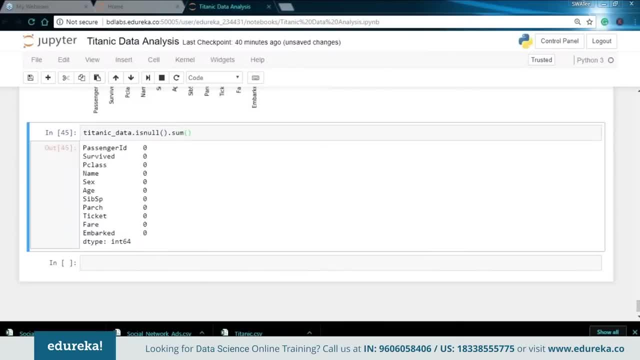 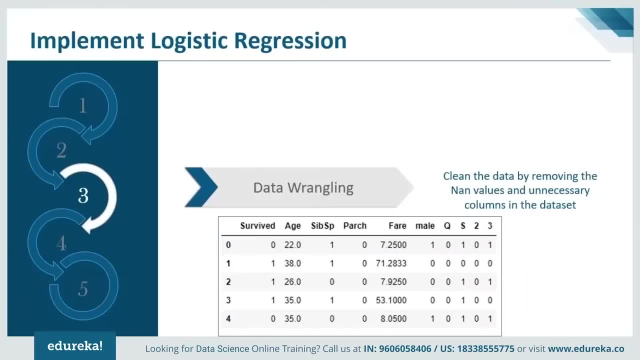 So here that tells me that data set is clean, as in, the data set does not contain any null value or any NAN value. So now we have Rangel Data. you can say cleaner data. So here we have done just one step in data Rangling, that is, just removing one column. 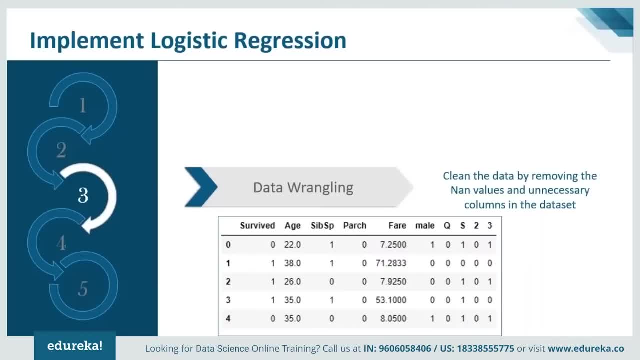 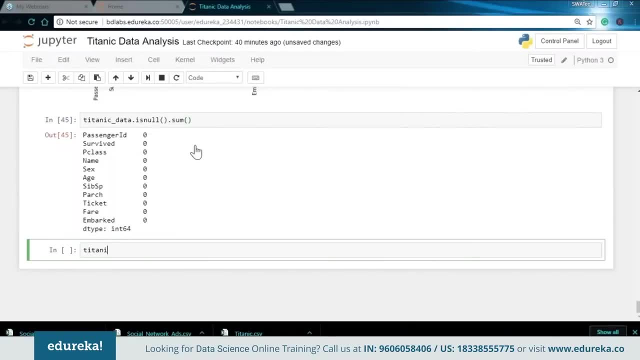 out of it. Now you can do a lot of things. You can actually fill in the values with some other values, or you can just calculate the mean and then you can just put in the null values. But now if I see my data set, so I'll say Titanic data dot head. 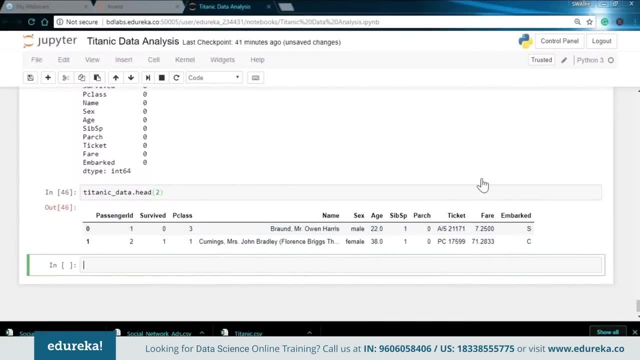 But now, if I see over here, I have a lot of string values, So this has to be converted to categorical variables in order to implement logistic regression. So what we will do, We will convert this to categorical Variable into some dummy variables, and this can be done using pandas, because logistic regression 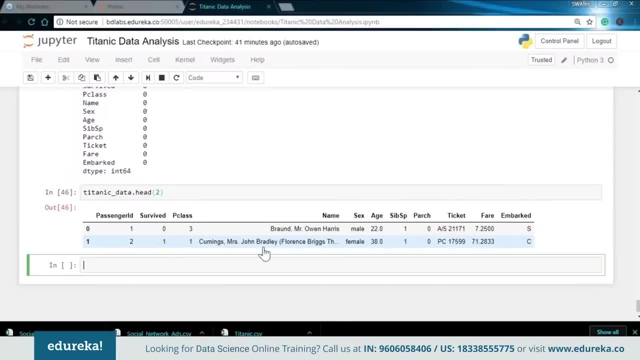 just take two values. So whenever you apply machine learning, you need to make sure that there are no string values present, because it won't be taking these as your input variables. So using string, you don't have to predict anything. but in my case I have the survive column. 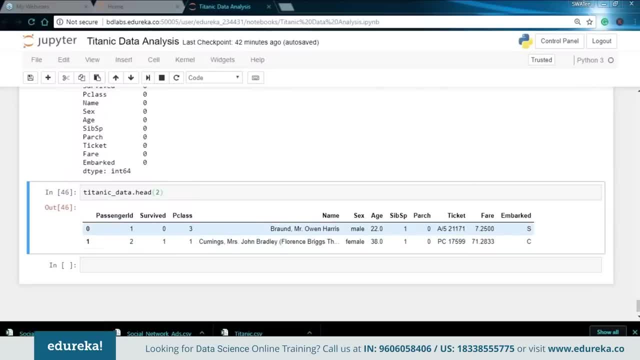 So I need to play to how many people tend to survive and how many did not. so zero stands for did not survive and one stands for survive. So now let me just convert these variables into dummy variables. So I'll just use pandas and I'll say: PD dot get dummies. 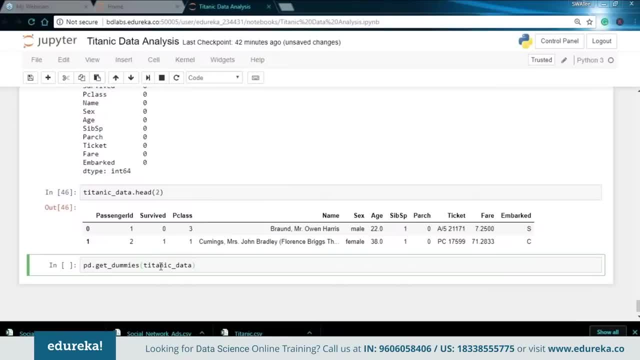 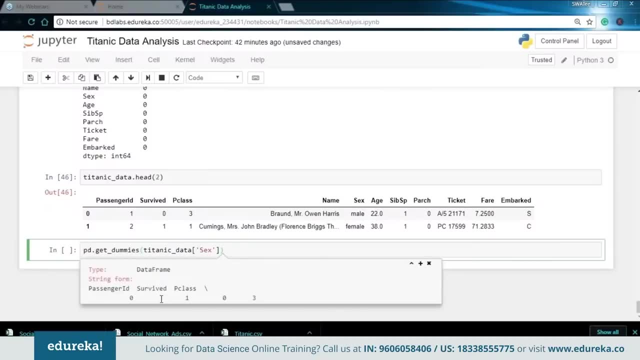 You can simply press tab to autocomplete and say Titanic data and I'll pass the sex. So you can just simply click on ship plus tab to get more information on this. So here we have the type data frame and we have the passenger ID survived and passenger class. 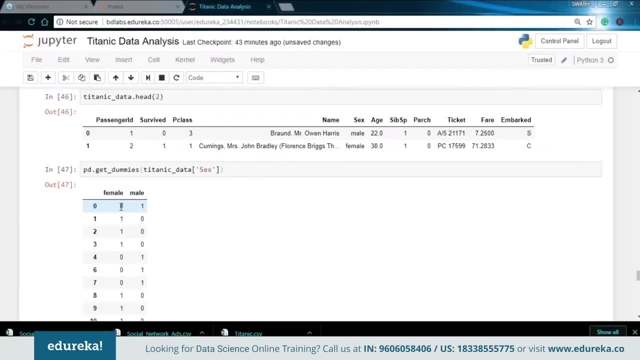 So if you run this, you'll see that zero basically stands for not a female and one stand for it is a female. Similarly for male: zero stands for it's not male and one stand for male. Now we don't require both these columns, because one column itself is enough to tell us whether it's male. 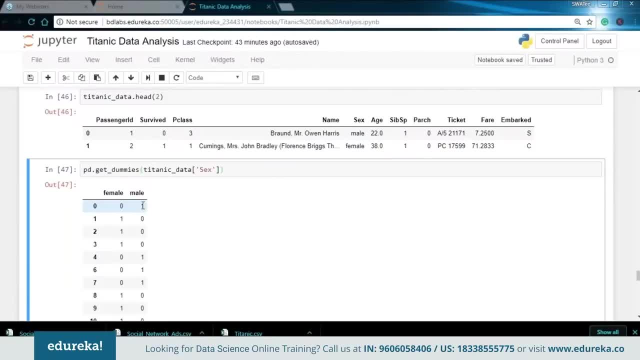 or you can say female or not. So let's say, if I want to keep only male, I'll say: if the value of male is one, so it is definitely a male and it is not a female. So that is how you don't need both of these values. 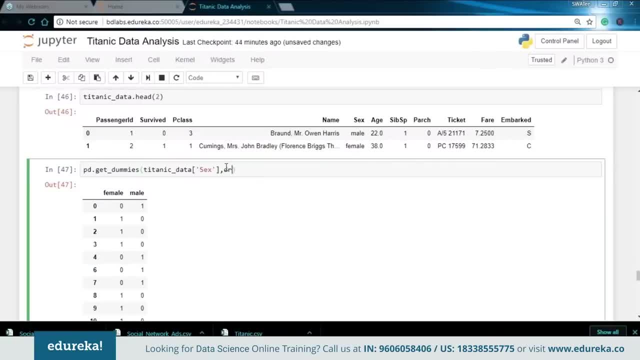 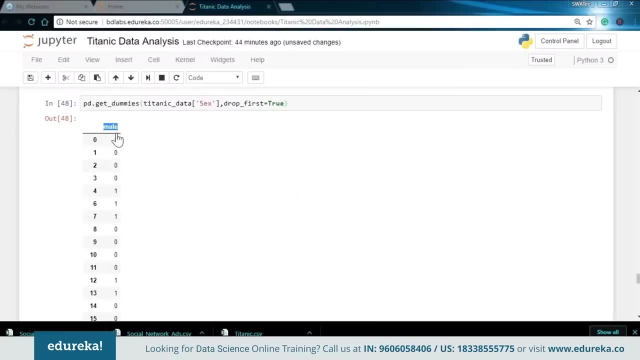 So for that I just remove the first column, that same female. So I'll say, drop first, and true. So over here it has given me just one column which is male and has the value zero And one. let me just set this as a variable. 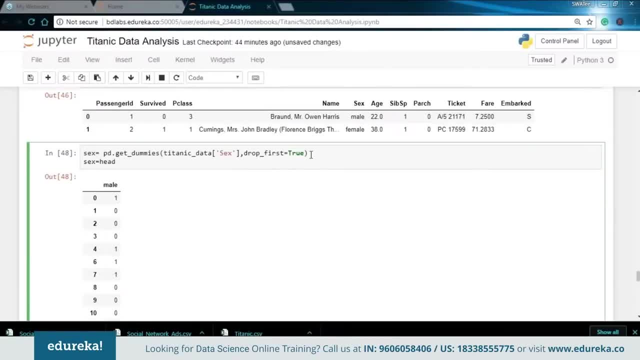 It says sex over here. I can say sex dot head. I just want to see the first five rows. Sorry, it's not So. this is how my data looks like. Now, here we have done it for sex. Then we have the numerical values in age. 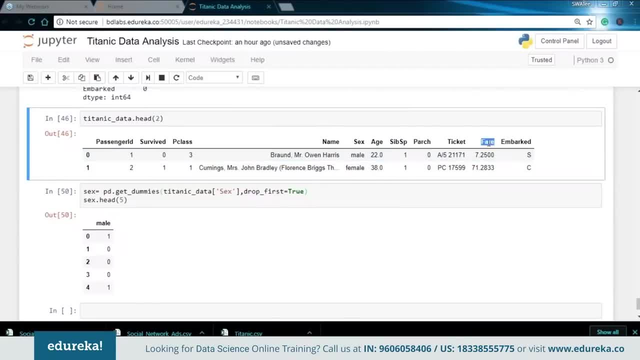 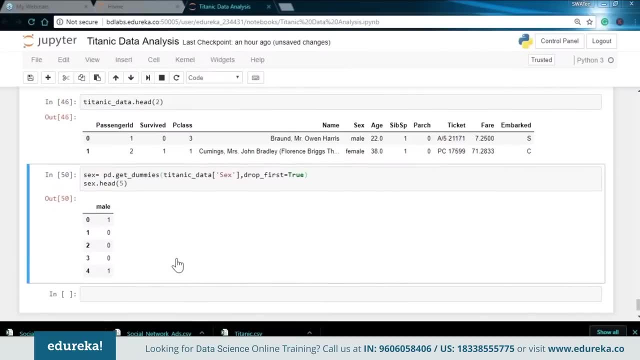 We have the numerical values in spouses, Then we have the ticket number, We have the pair and we have embarked as well. So in embarked the values are in SC and Q. So here also we can apply this get dummy function. So let's say I'll take a variable. 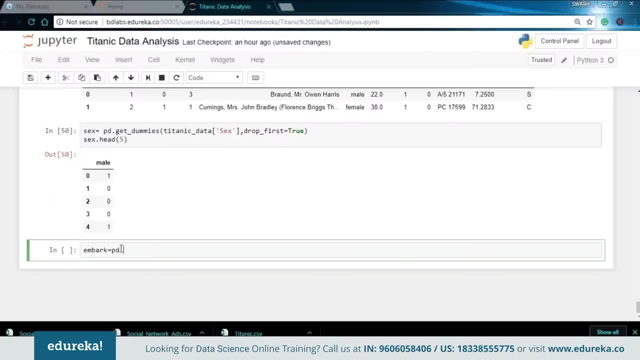 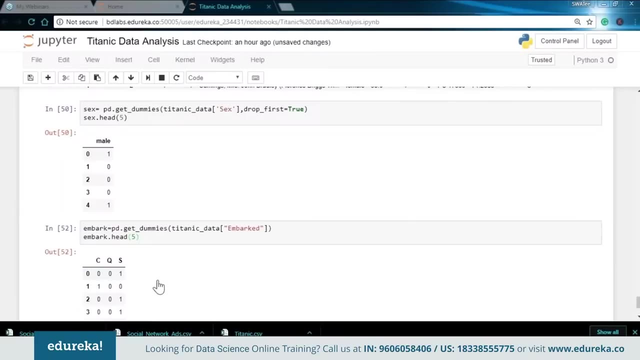 Let's say embark. I'll use the pandas library, I'll enter the column name that is embarked. Let me just print the head of it. So I'll say embarked dot head. So over here we have CQ and S. Now here also we can drop the first column because these two values are enough. 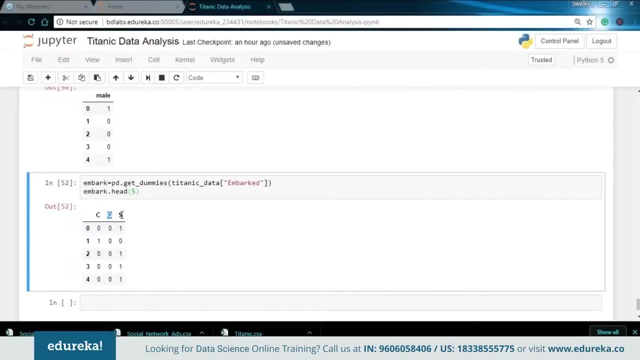 whether the passenger is either traveling for Q, that is, Kuenstown, S for Southampton, And if both the values are zero, then definitely the passenger is from Cherbourg. That is the third value. So you can again drop the first value. So I'll say drop. 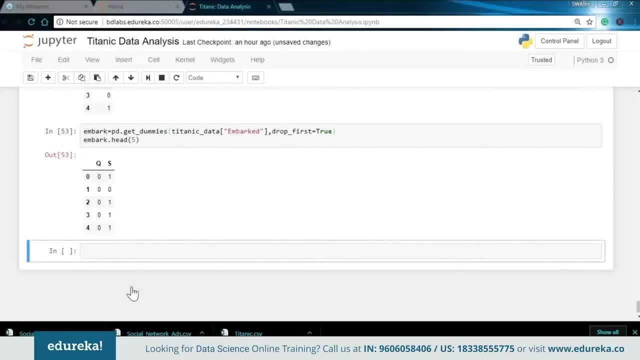 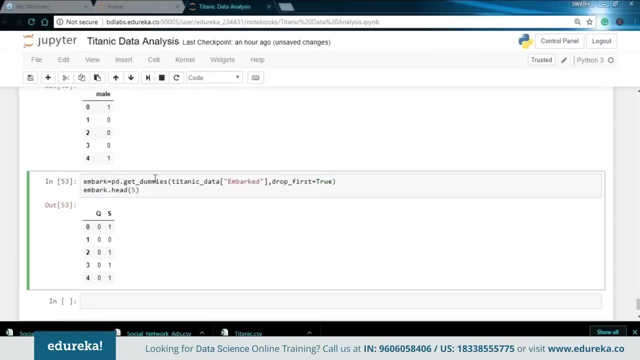 And true, Let me just run this. So this is how my output looks like now. Similarly, you can do it for passenger class as well. So here also we have three classes: one, two and three. So I just copy the whole statement. 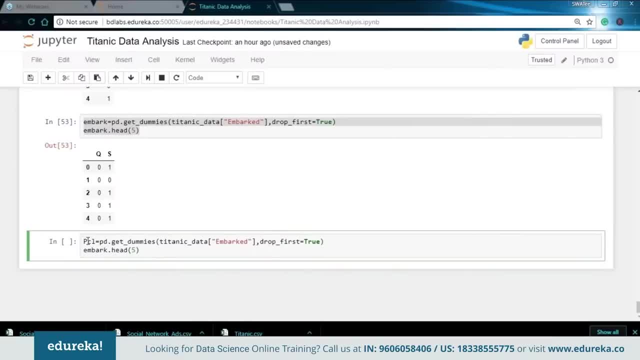 So let's say I want the variable name, Let's say PCL. I'll pass in the column name, that is, P class, And I'll just drop the first column. So here also the values will be one, two or three and I'll just remove the first column. 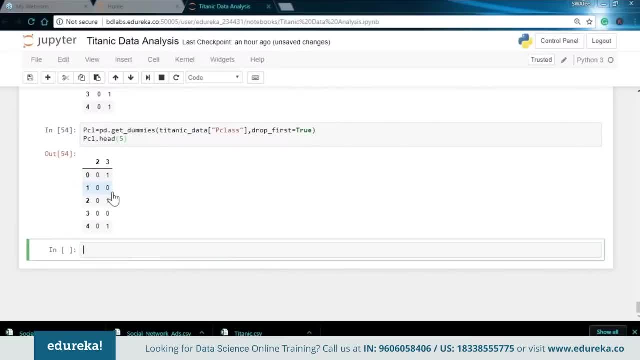 So here we just left with two and three. So if both the values are zero, then definitely the passengers traveling in the first class. Now we have made the values as categorical. Now my next step would be to concatenate all these new rows into a data set. 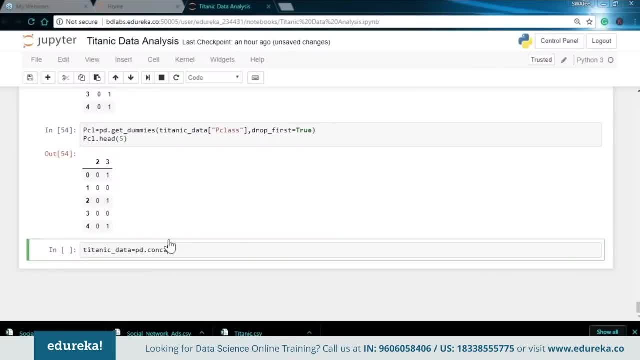 I can say Titanic data using the Pandas, will just concatenate all these columns. So I'll say P dot concat. And I'll say we have to concatenate sex, We have to concatenate Embark and PCL, and then I'll mention the access to one and just run this: 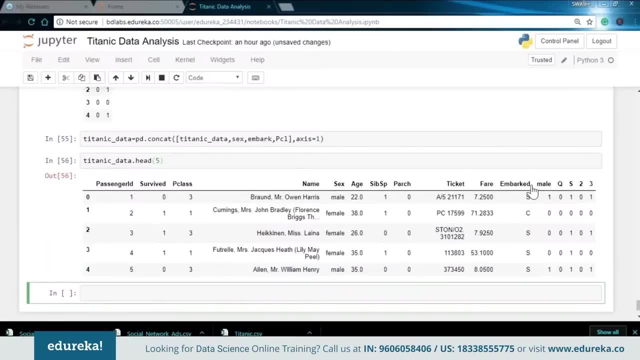 I need to print the head, So over here you can see that these columns have been added over here. So we have the mail column, which basically tells whether person is male or it's a female. then we have the Embark, which is basically Q and S. 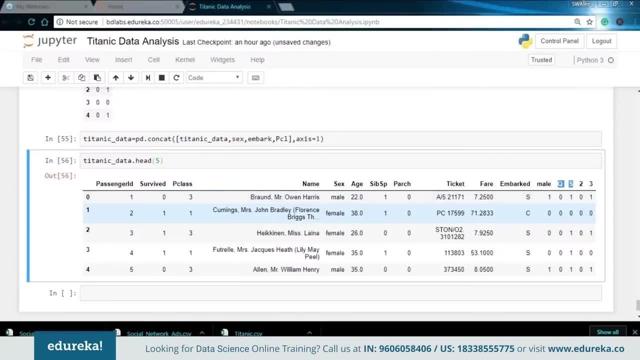 So if it's traveling from Cunestown, value would be one, else it would be zero. and if both of these values, As you know it is definitely traveling from chair Bob, then we have the passenger class as two and three. So the value of both these is zero. then the passengers traveling in class one: 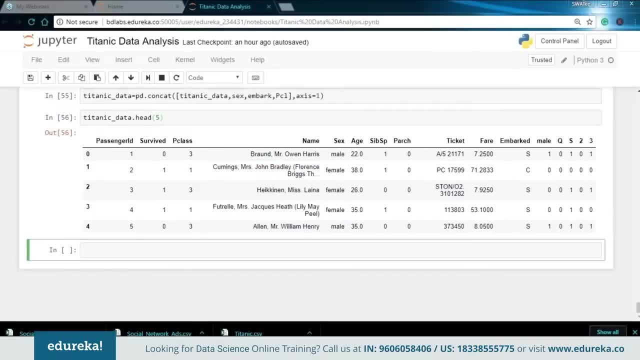 So I hope you got this till now. Now These are the irrelevant columns that we have it over here So we can just drop these columns. will dropping P class, the Embark column and the sex column. So I just type in Titanic data dot drop and mention the columns that I want to drop. 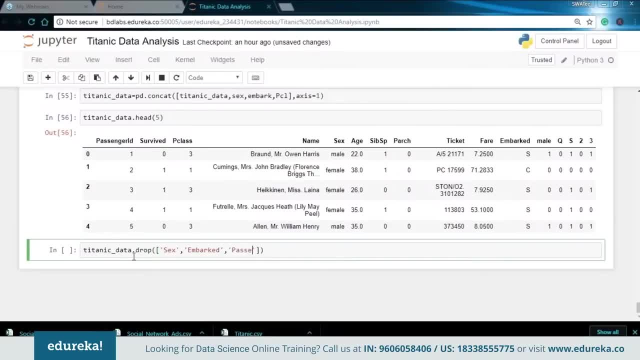 So I'll say I'll even delete the passenger ID, because it's nothing but just the index value which is starting from one, So I'll drop this as well. Then I don't want name as well, So I'll delete name as well. 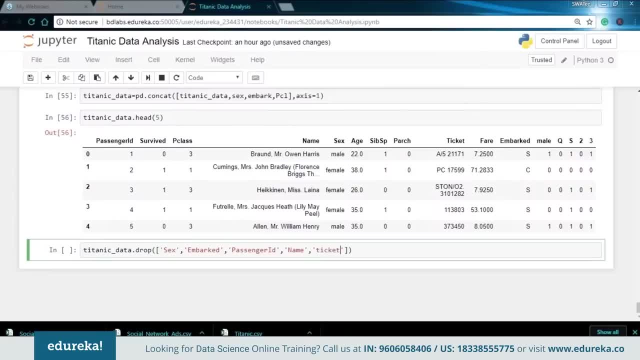 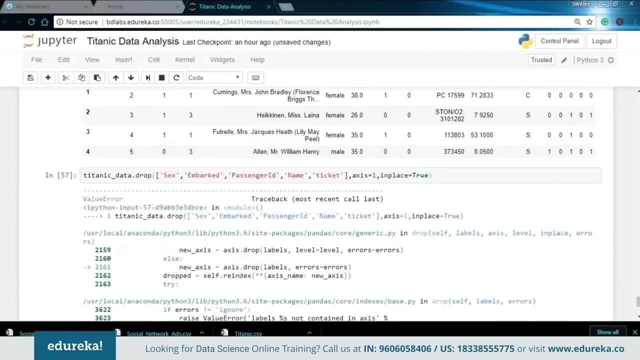 Then what else we can drop. we can drop the ticket as well, And then I'll just mention the access and I'll say: in place is equals to true. Okay, so my column name starts from uppercase, So these has been dropped. now Let me just print my data set again. 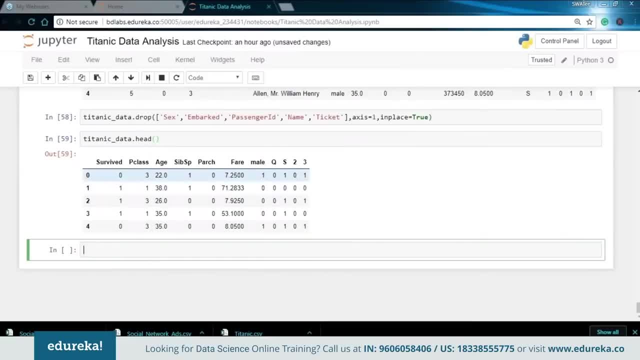 So this is my final data set, guys. We have the survived column, which has the value 0 and 1. then we have the passenger class. Oh, we forgot to drop this as well, So, no worries, I'll drop this again. So now let me just run this. 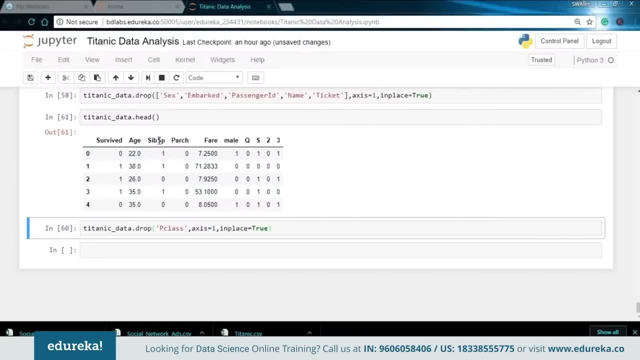 So over here we have the survive, We have the age, We have the Sib SP, We have the part, We have fair meal and these we have just converted. So here we have just performed data wrangling, or you can say: clean the data. 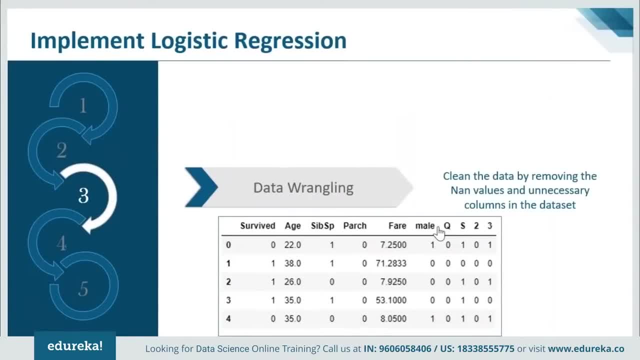 and then we have just converted the values of gender to mail, then embarked to Q and S and the passenger class to 2 and 3.. So this was all about my data wrangling, or just cleaning the data. Then my next step is training and testing your data. 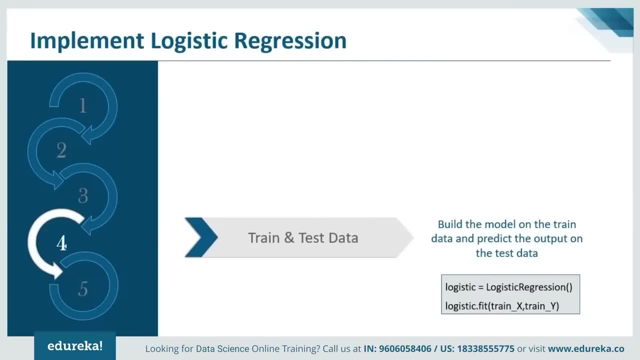 So here we will split the data set into train subset and test subset, and then what we'll do will build a model on the train data and then predict the output on your test data set. So let me just go back to Jupiter and let us implement this as well over here. 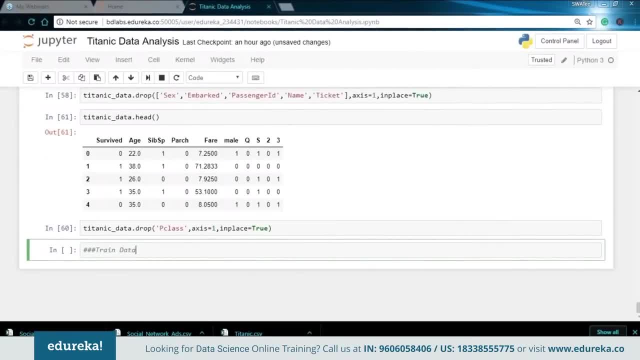 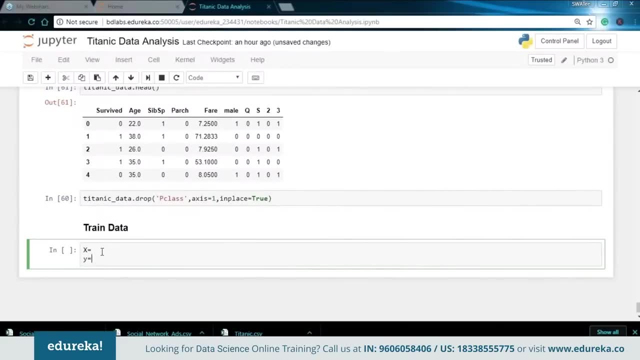 I need to train my data set, So I'll just put this in the heading 3.. So over here you need to define your dependent variable and independent variable. So here my Y is the output. I can say the value that I need to predict over here. 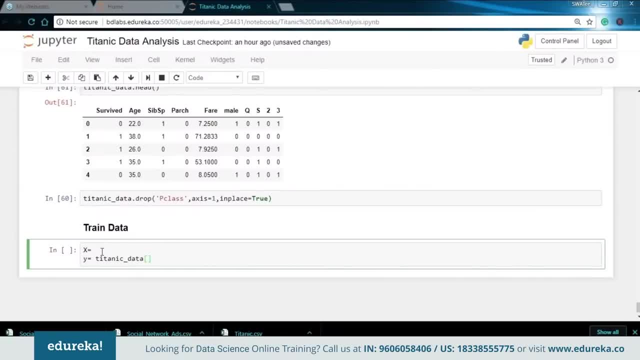 I'll write Titanic data. I'll take the column which is survive. So, basically, I have to predict this column, whether the passenger survived or not, and, as you can see, we have the discrete outcome, Which is in the form of 0 and 1 and rest, all the things we can take it. 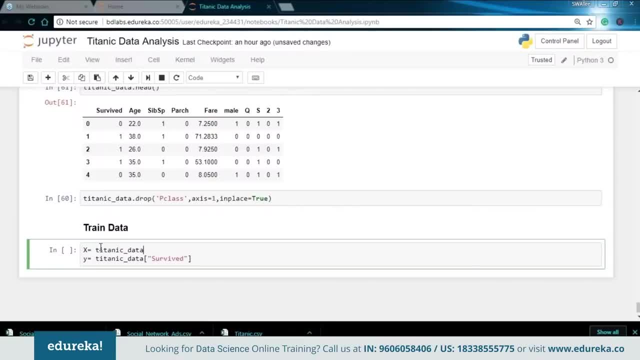 as a features, or you can say independent variable. So I'll say Titanic data, not drop. So we'll just simply drop the survive and all the other columns will be my independent variable. So everything else are the features which leads to the survival rate. 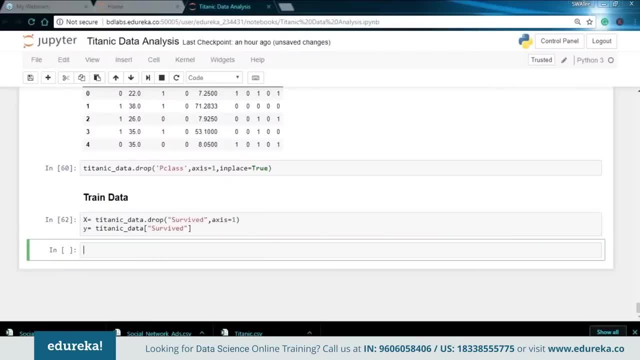 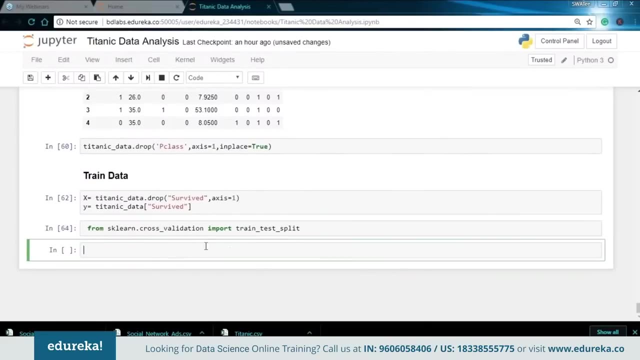 So once we have defined the independent variable and the dependent variable, next step is to split your data into training and testing subset. So for that we'll be using sklearn. I just type in from sklearn: dot: cross validation: Import train test plate. Now here, if you just click on shift and tab, you can go to the documentation. 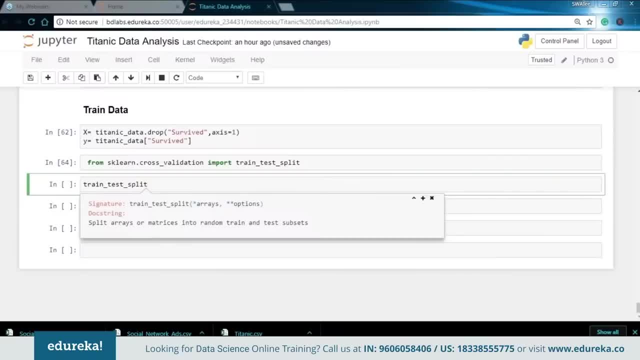 and you can just see the examples over here. I'll click on plus to open it and then I just go to examples and see how you can split your data. So over here you have X train, X test, Y train, Y test and then, using this train test plate, you can just pass in your independent 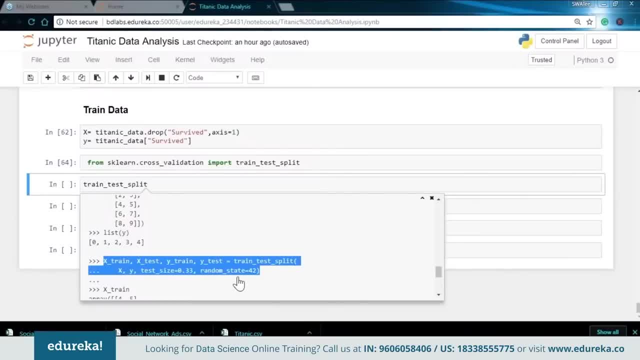 independent variable and dependent variable and just define a size and a random state to it. So let me just copy this and I'll just paste it over here. Over here will train test, then we have the dependent variable, train and test and using the split function will pass in the independent. 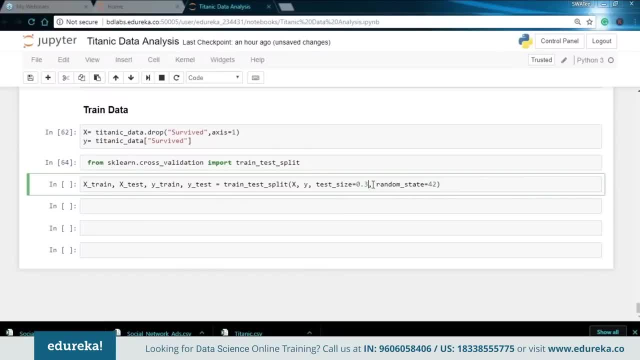 and dependent variable, and then we'll set a split size. So let's say I'll put it at 0.3.. So this basically means that your data set is divided in 0.3. That is in 70-30 ratio, and then I can add any random state to it. 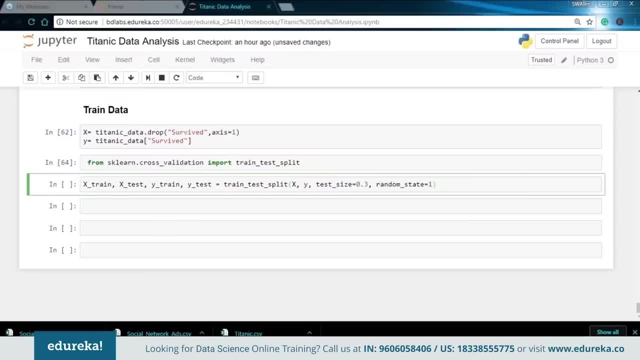 So let's say I'm applying one. This is not necessary. If you want the same result as that of mine, you can add the random state. So this will basically take exactly the same sample every time. Next, I have to train and predict by creating a model. 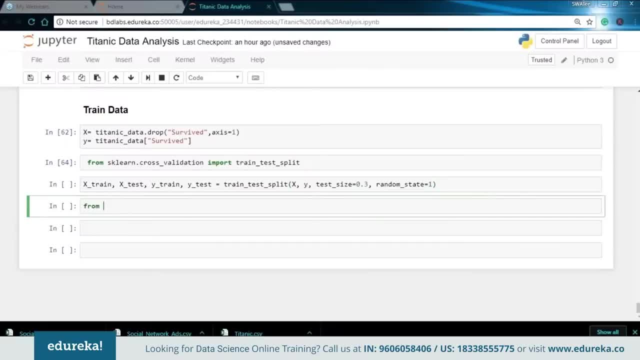 So here logistic regression will grab from the linear regression. So next I'll just type in from sklearnlinear model import logistic regression. Next I'll just create the instance of this logistic regression model. So I'll say log Model is equals to logistic regression. 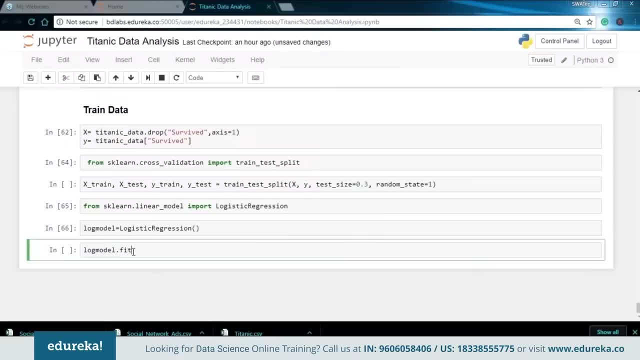 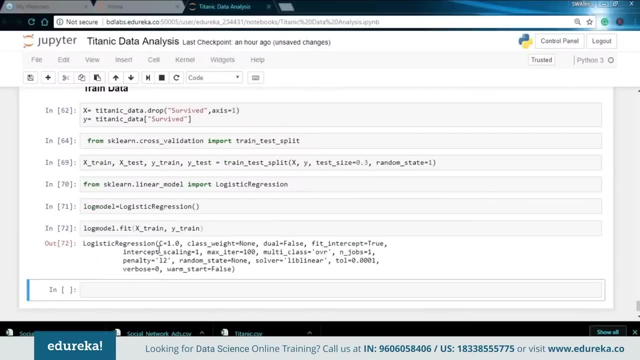 Now I just need to fit my model. So I'll say log model, dot fit, and I'll just pass in my x-train And y-train, All right. So here it gives me all the details of logistic regression. So here it gives me the class weight, dual fit, intercept and all those things. 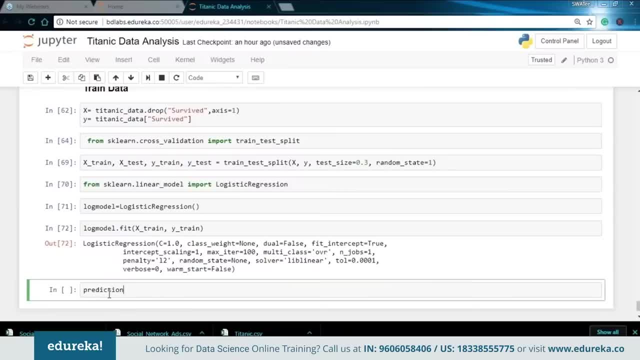 then what I need to do. I need to make prediction. So I'll take a variable, let's say predictions, and I'll pass on the model to it. So I'll say log model, dot predict, and I'll pass in the value, that is, X test. 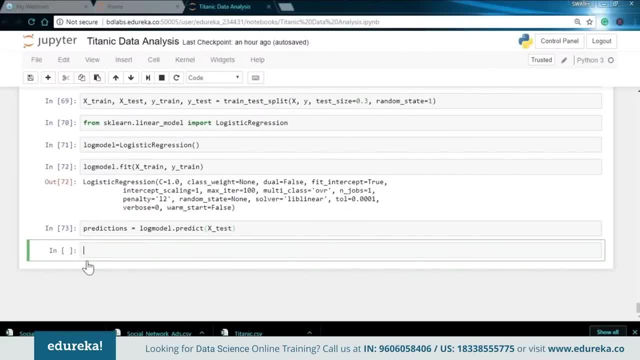 So here we have just created a model. fit that model, and then we had made predictions. So now to evaluate how my model has been performing. so you can simply calculate the accuracy, or you can also calculate a classification report. So don't worry guys, I'll be showing both of these methods. 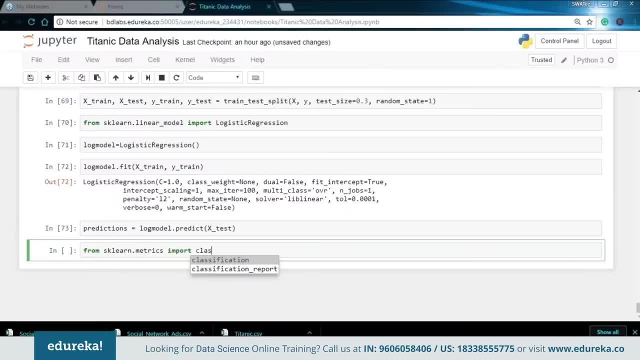 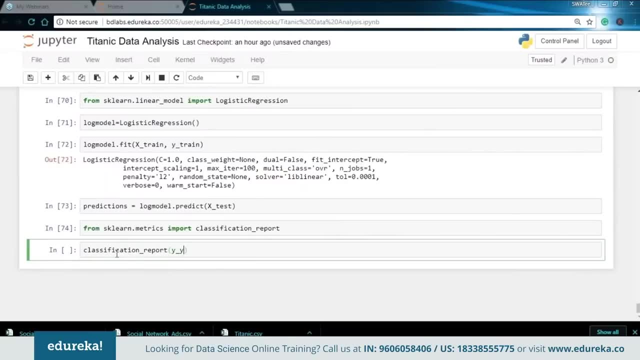 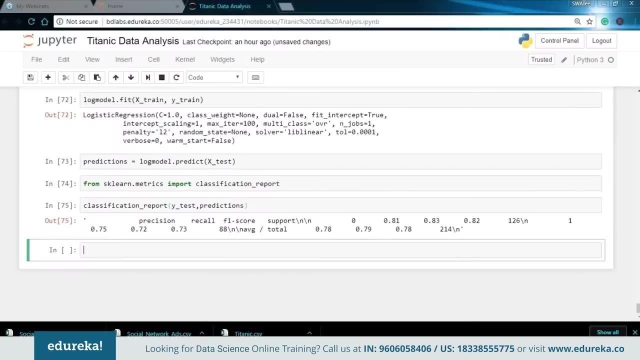 So I'll say from sklearnmetrics import classification report. Over here I use classification report And inside this I'll be passing in y test and the predictions. So, guys, this is my classification report. So over here I have the precision. 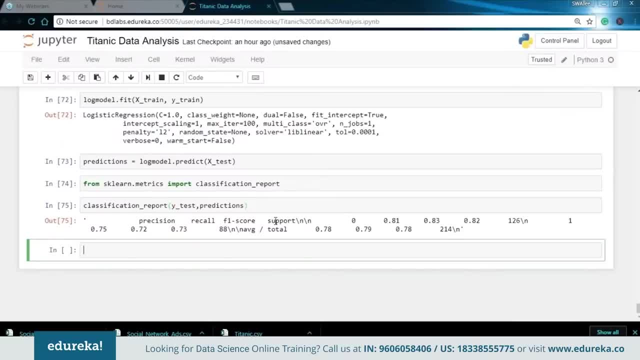 I have the recall We have the F1 score and then we have support. So here we have the value of precision as 75, 72 and 73, which is not that bad. now, in order to calculate the accuracy as well, You can also use the concept of confusion matrix. 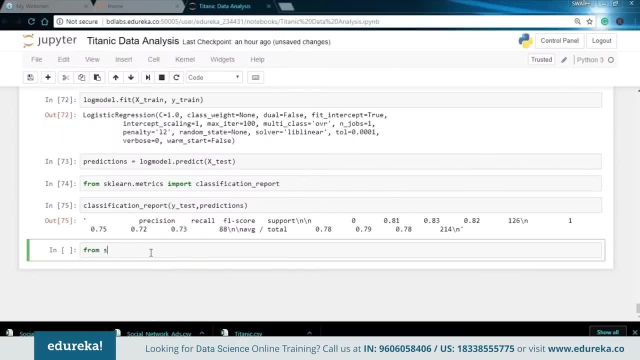 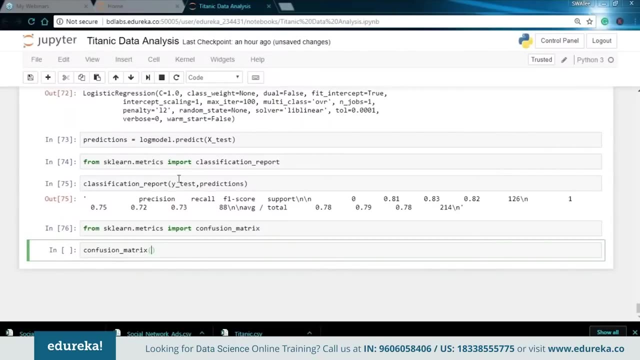 So if you want to print the confusion matrix, I will simply say: from sklearnmetrics, import confusion matrix first of all, and then we'll just print this. So here my function has been imported successfully. So I'll say confusion matrix And I'll again pass in the same variables, which is y test, and 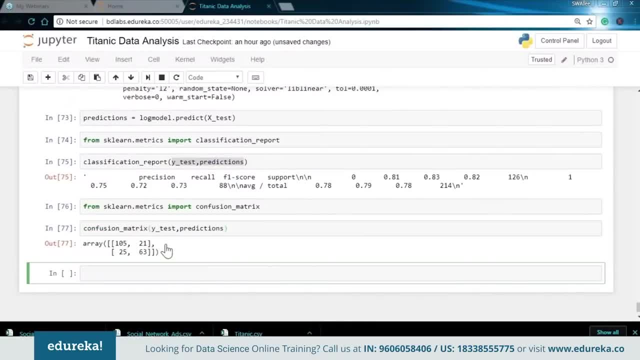 predictions. So I hope you guys already know the concept of confusion matrix. So can you guys give me a quick confirmation as to whether you guys remember this confusion matrix concept or not? So if not, I can just quickly summarize This as well. 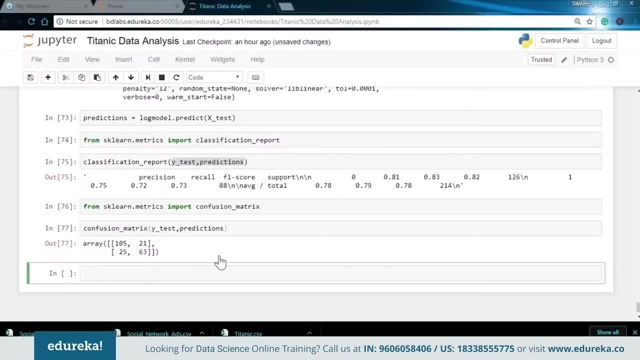 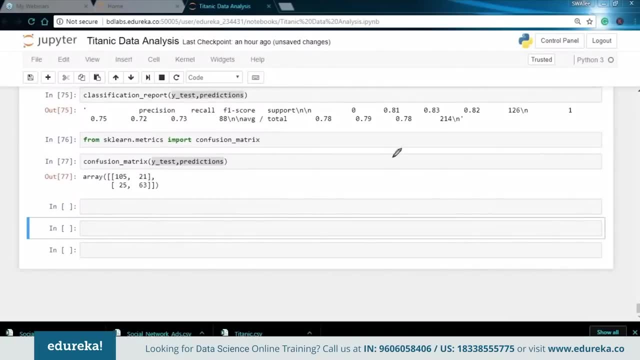 Okay, Jagruti says a yes. Okay, Swati is not clear with this, So I'll just tell you in a brief what confusion matrix is all about. So confusion matrix is nothing but a two by two matrix which has a four outcomes. 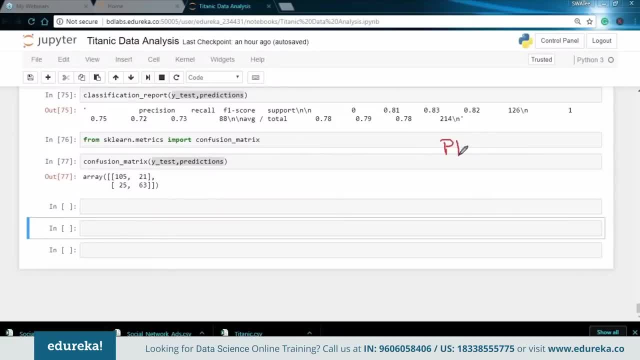 This basically tells us that how accurate your values are. So here we have the column as predicted No, predicted Why, And we have actual no and an actual yes. So this is the concept of confusion matrix. So here let me just 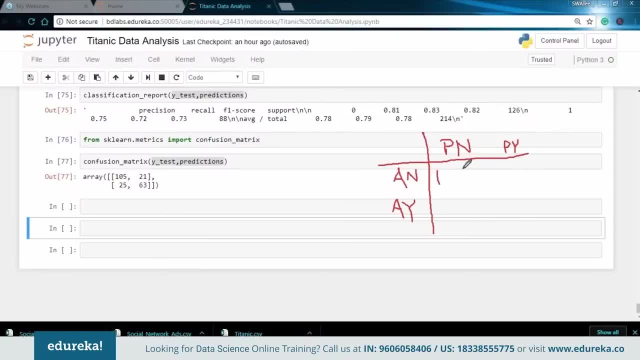 Get in these values which we have just calculated. So here we have 105.. 105, 21, 25 and 63.. So, as you can see, here we have got four outcomes. Now, 105 is the value where a model has predicted. 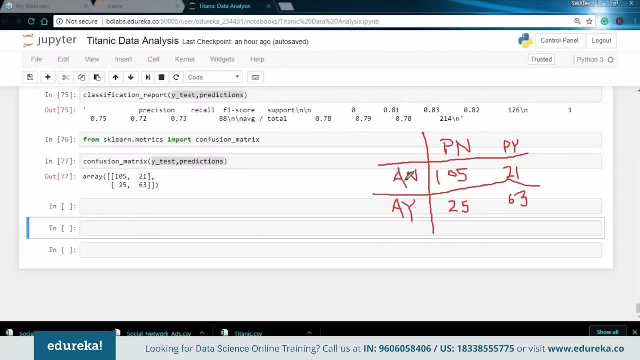 No and in reality it was also a no. So here we have predicted no and an actual no. Similarly, we have 63 as a predicted Yes. So here the model predicted Yes and actually also it was a yes. 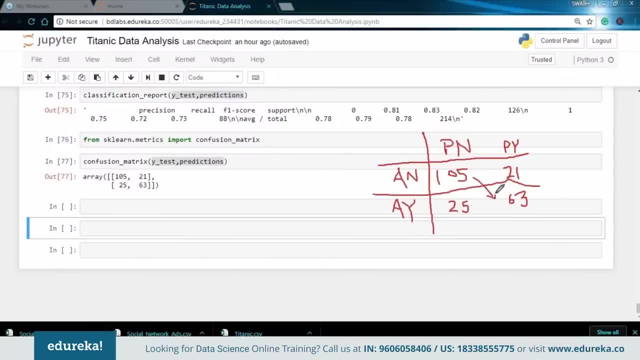 So in order to calculate the accuracy, you just need to add the sum of these two values and divide the whole by the sum. So here these two values tells me where the model has actually predicted the correct output. So this value is also called as true- negative. 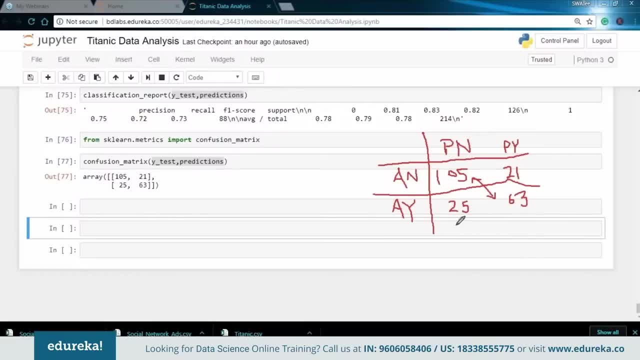 This is called as false positive, This is called as true positive and this is called as false negative. Now, in order to calculate the accuracy, you don't have to do it manually. So in Python you can just import accuracy score function and you can get the results from that. 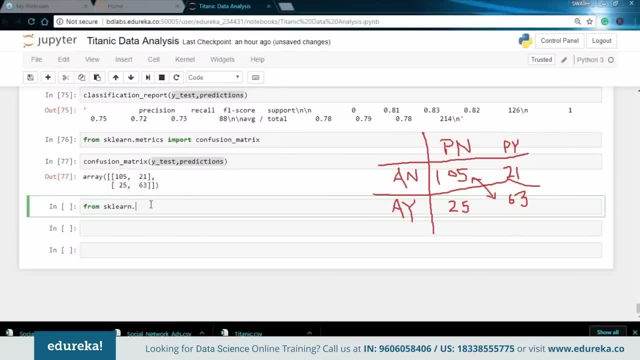 So I'll just do that as well. So I'll say from sklearnmetrics import accuracy score and I simply print the accuracy. I'll pass in the same variables, that is, y test and predictions. So over here it tells me the accuracy as 78, which is quite 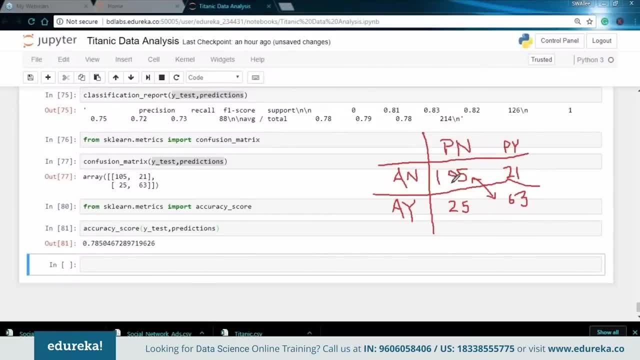 good. So over here, if you want to do it manually, you have to plus these two numbers, which is 105 plus 63. So this comes out to almost 168, and then you have to divide by the sum of all the four numbers. 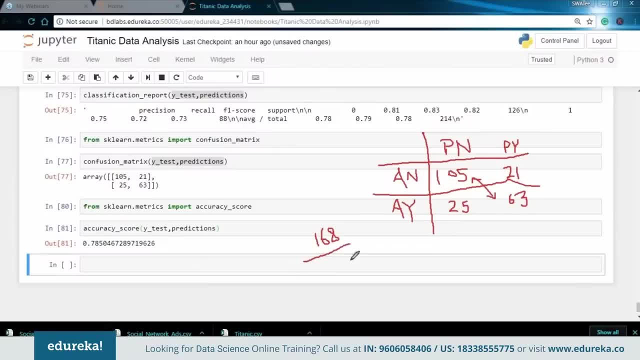 So 105 plus 63 plus 21.. Plus 25.. So this gives me a result of 214.. So now, if you divide these two number, you'll get the same accuracy, that is 78%, or you can say 0.78.. 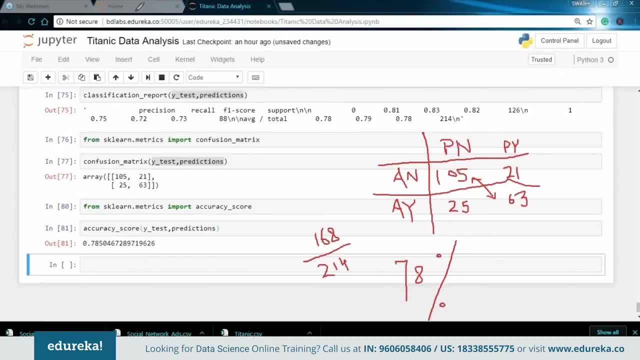 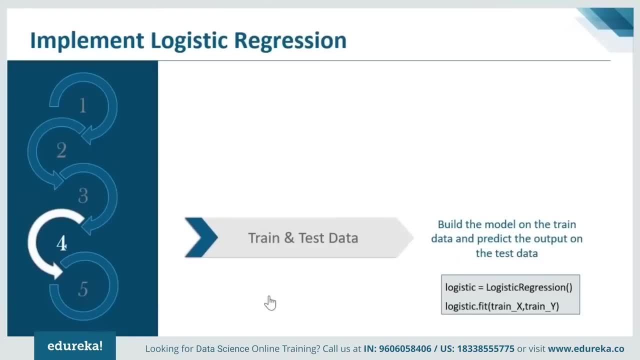 So that is how you can calculate the accuracy. So now let me just go back to my presentation and let's see what all we have covered till now. So here we have first split our data into train and test subset. Then we have build our model on the train data and then predicted. 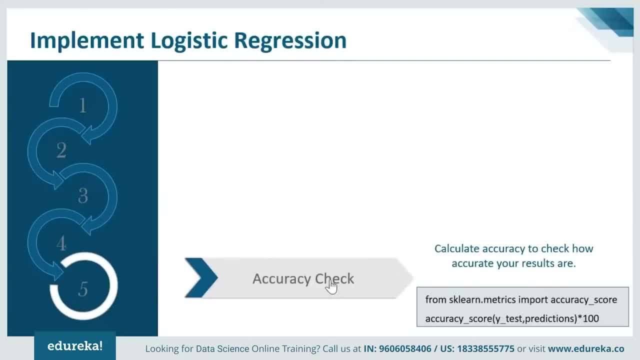 the output on the test data set. and then my fifth step is to check the accuracy. So here we have calculated accuracy: Accuracy to almost 78%, which is quite good. You cannot say that accuracy is bad. So here it tells me how accurate your results are. 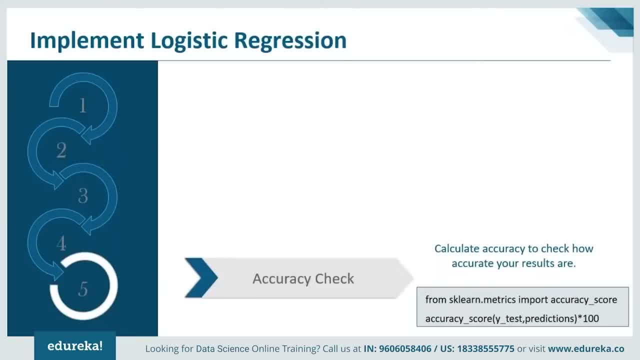 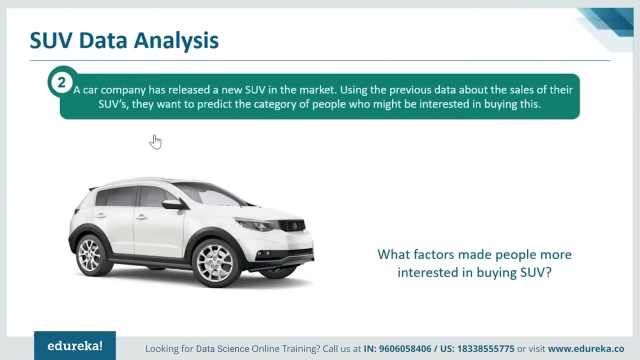 So here my accuracy score defines that, and hence we got a good accuracy. So now moving ahead. Let us see the second project, that is, SUV data analysis. So in this, a car company has released new SUV in the market and using the previous data about the sales of their SUV, 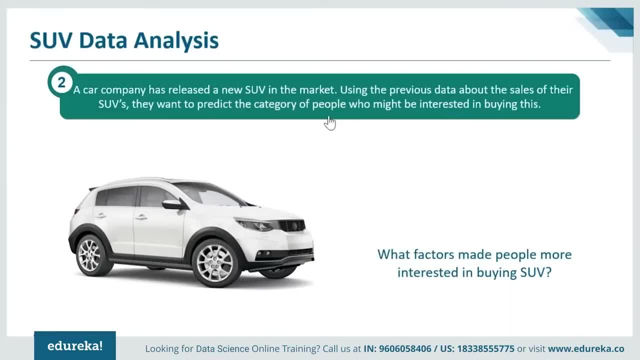 They want to predict the category of people who might be interested in buying this. So, using the logistic regression, You need to find what factors made people more interested in buying this SUV. So for this, let us see a data set where I have user ID. 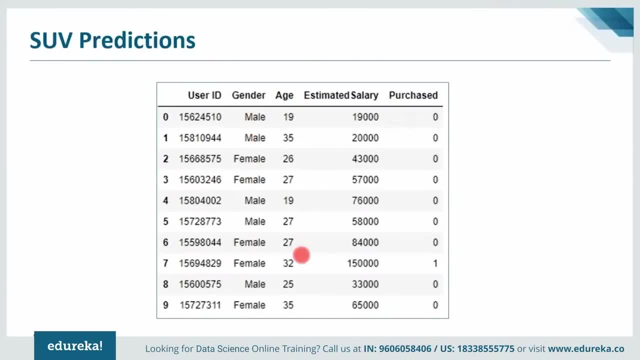 I have gender as male and female, then we have the age, we have the estimated salary and then we have the purchase column. So this is my discrete column, or you can say the categorical column. So here we just have the value, that is, 0 and 1, and this column. 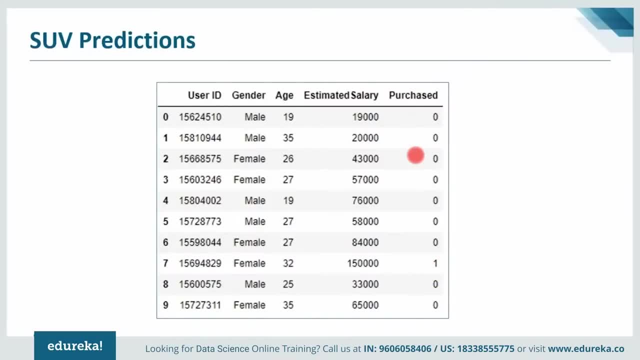 we need to predict whether a person can actually purchase a SUV or not. So, based on these factors, we will be deciding whether a person can actually purchase. We are not, so we know the salary of a person, We know the age and using these, we can predict whether person 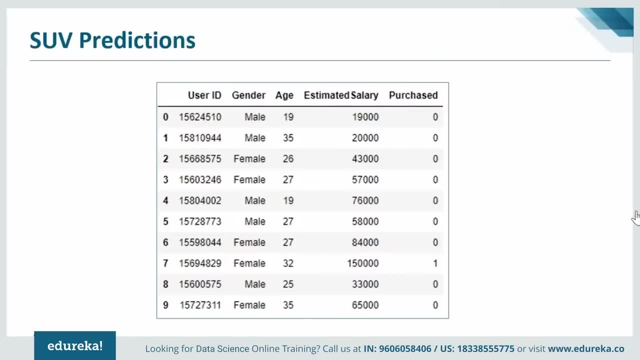 can actually purchase SUV or not. So let me just go to my Jupiter notebook and it is implement logistic regression. So, guys, I will not be going through all the details of data cleaning and analyzing the part. that part, I'll just leave it on you. 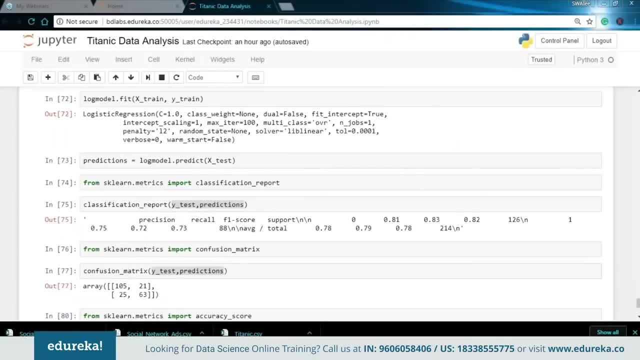 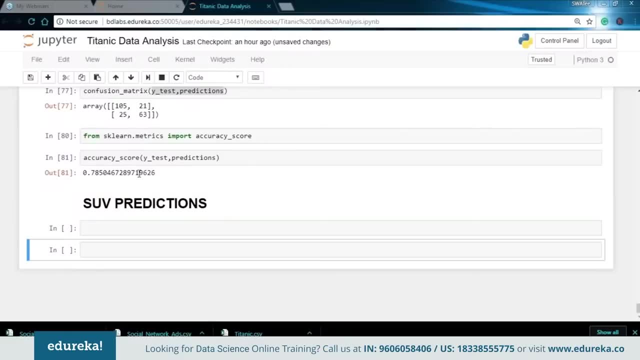 So just go ahead and practice as much as you can, All right. So the second project is SUV predictions- All right. So first of all I have to import all the libraries. So I say import Import numpy as NP and similarly I'll do the rest of it. 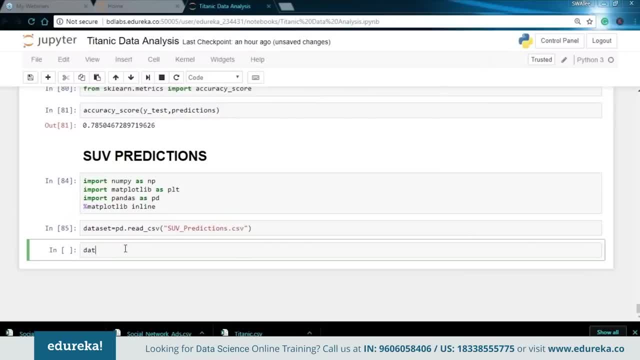 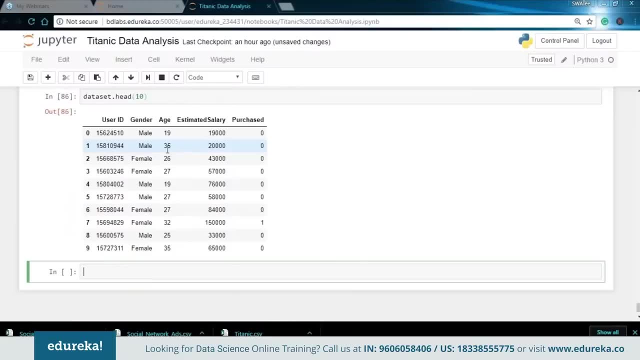 All right. So now let me just print the head of this data set. So this: we've already seen that we have columns as user ID, We have gender, we have the age, we have the salary and then we have to calculate whether person can actually purchase a SUV. 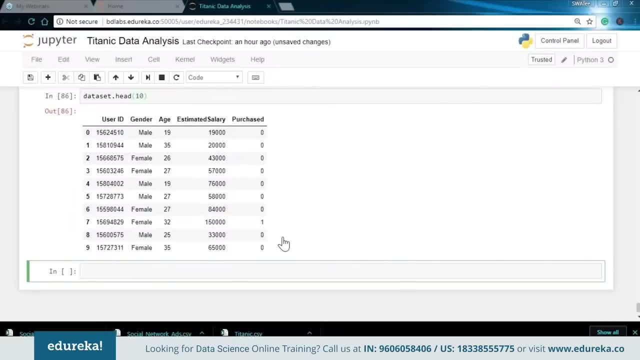 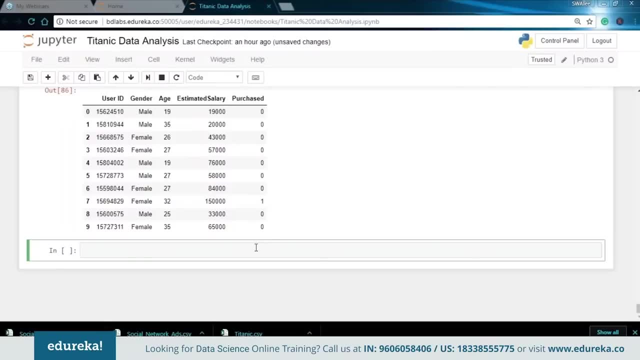 or not. So now it is just simply go on to the algorithm part, So we'll directly start off The logistic regression or how you can train a model. So for doing all those things, we first need to define your independent variable and dependent variable. 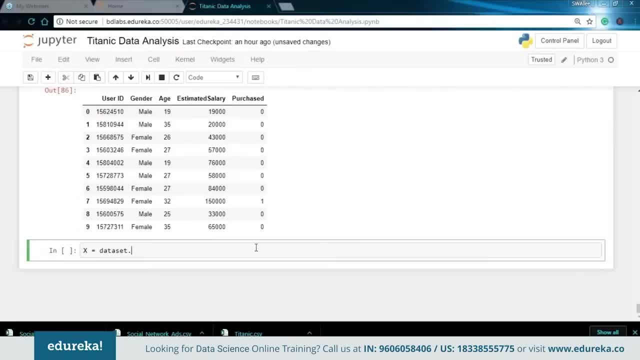 So in this case I want my X. that is an independent variable. I said data set, dot, I lock, So here I'll be specifying all the rows. So colon basically stands for that and in the columns I want only two and three dot values. 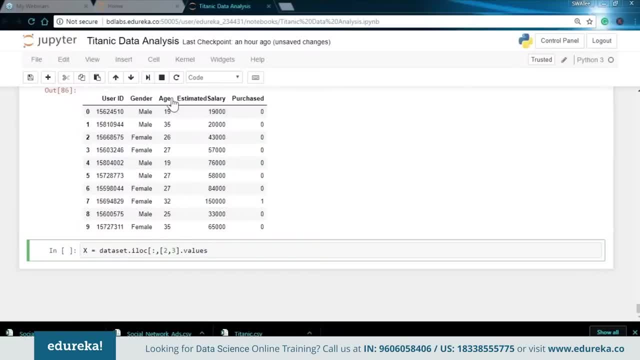 So here should fetch me all the rows and only the second and third column, which is age and estimated salary. So these are the factors which will be used, Suppose, to predict the dependent variable that is purchase. So here, my dependent variable is purchase and independent. 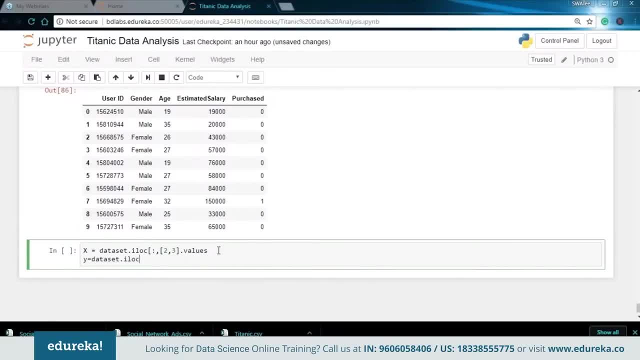 variable is of age and salary. So I'll say data set, dot. I love, I'll have all the rows and I just want fourth column, That is, my purchased column: dot values. All right, So I've just forgot one, one square bracket over here. 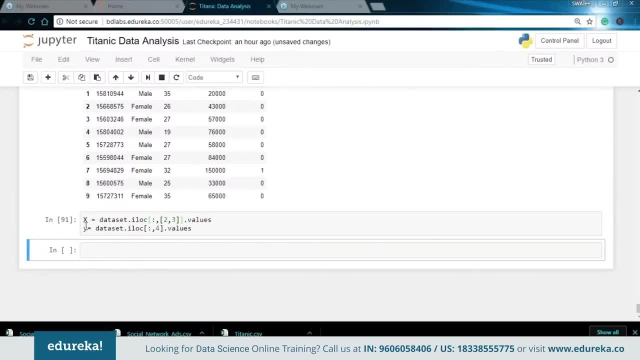 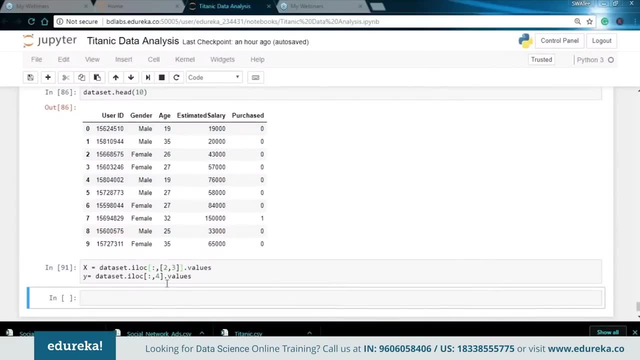 All right. So over here I have defined my independent variable and dependent variable. So here my independent variable is age and salary, and dependent variable is the column purchase. Now you must be wondering: what is this? I log function, So I love. function is basically an indexer for pandas data frame. 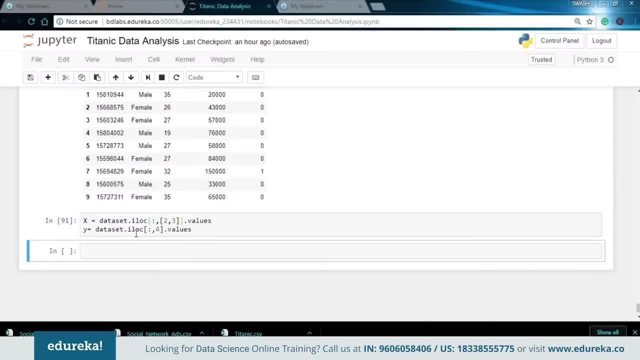 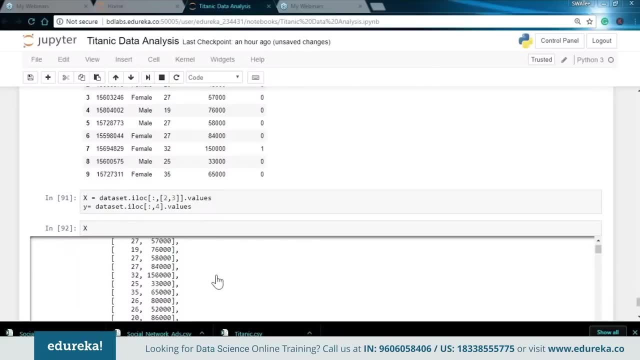 and it is used for integer based indexing. I can also say selection by index. Now let me just print these independent variables and dependent variable. So if I print the independent variable, I have the age as well as the salary. next Let me print the dependent variable as well. 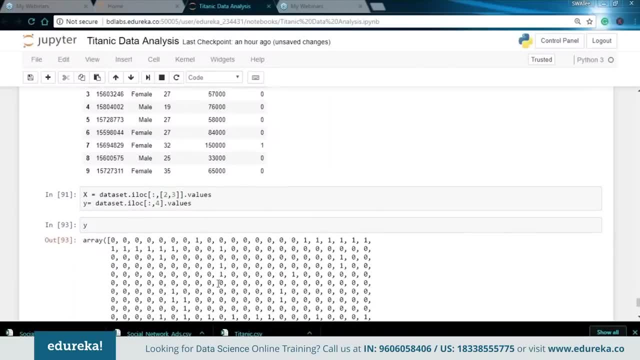 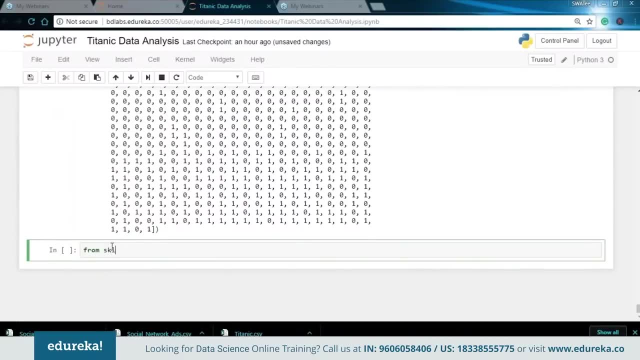 So over. here you can see I just have the values in 0 and 1, so 0 stands for did not purchase. next, Let me just divide my data set into two Training and test subset, So I'll simply write in from sklearn dot cross, split dot cross. 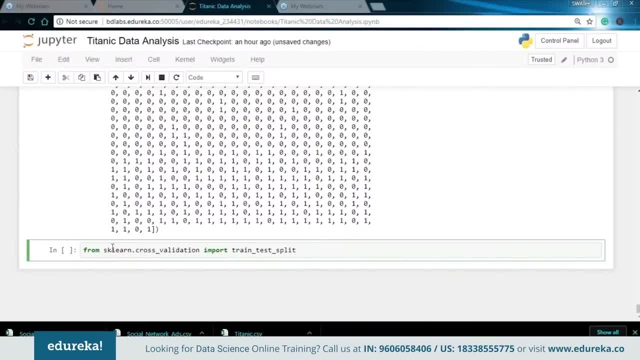 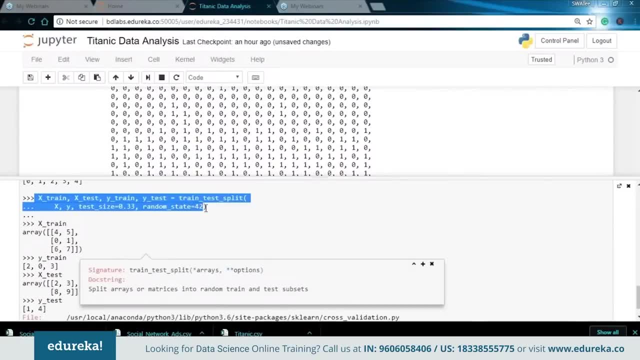 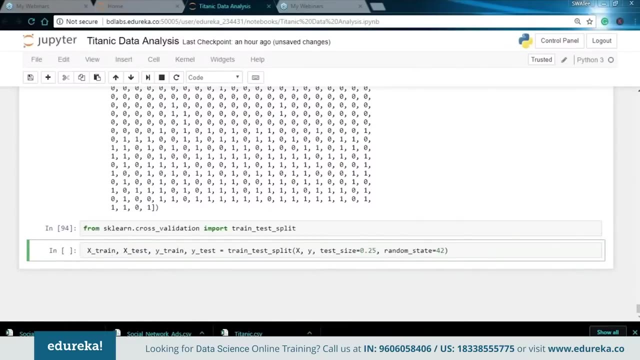 validation: Import train test. Next, I just press shift and tab and over here I'll go to the examples and just copy the same line. So I'll just copy this. I'll remove the points. Now. I want the text size to be, let's say, 25.. 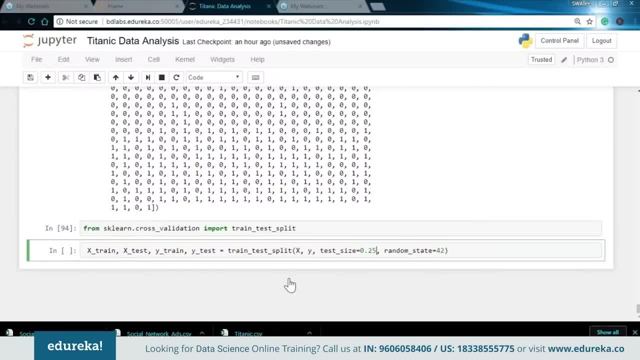 So I have divided the train and test it in 75: 25 ratio. Now let's say I'll take the random Set as 0, so random state basically ensures the same result. or you can say same samples taken whenever you run the code. 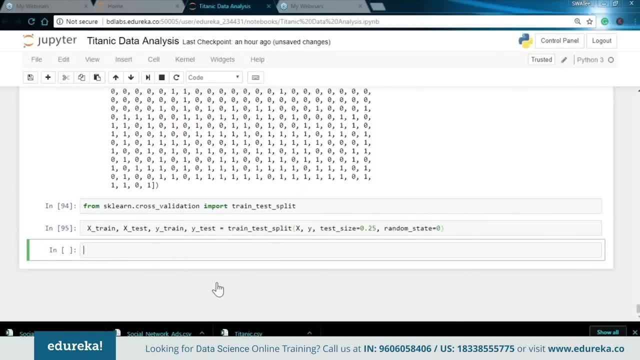 So let me just run this now. You can also scale your input values for better performing, and this can be done using standard scalar, So let me do that as well. So I'll say: from sklearn dot pre-processing Import standard scalar. Now, why do we scale it now? 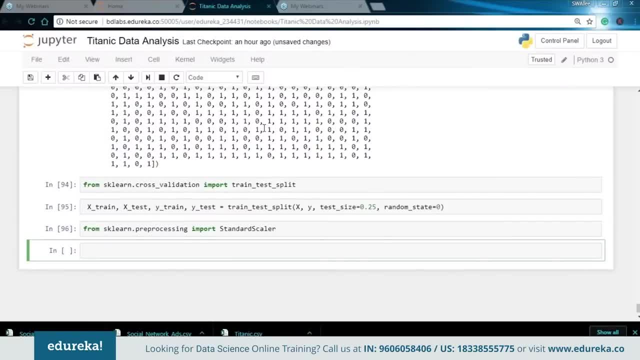 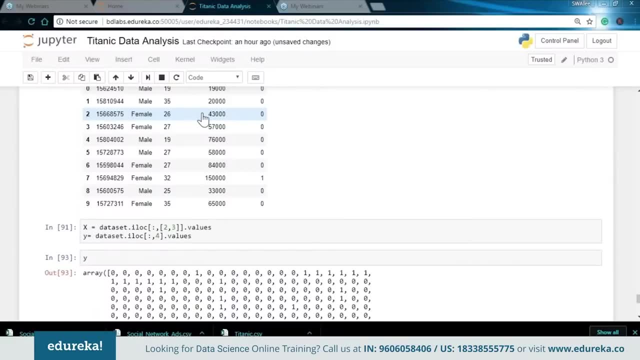 If you see our data set, we are dealing with large numbers. Well, although we are using a very small Data set. whenever you're working in a broad environment, you'll be working with large data set, where you'll be using thousands and hundred thousands of tuples. 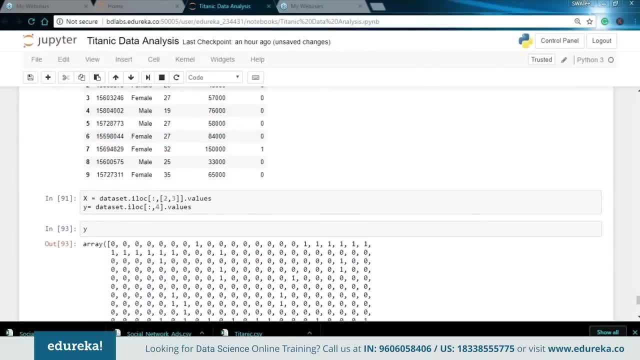 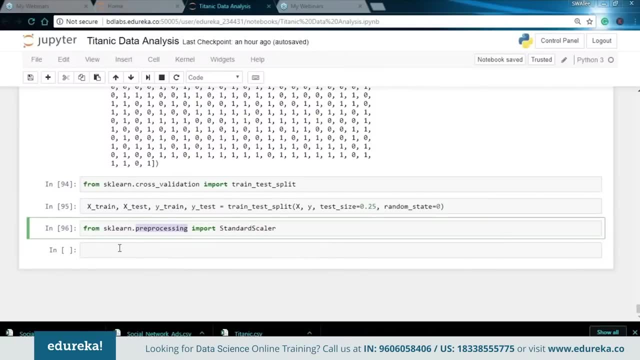 So they're scaling down will definitely affect the performance by a large extent. So here let me just show you how we can scale down these input values. and then the pre-processing contains all your methods and functionality which is required to transform your data. So now that is scaled down for test as well as a training data. 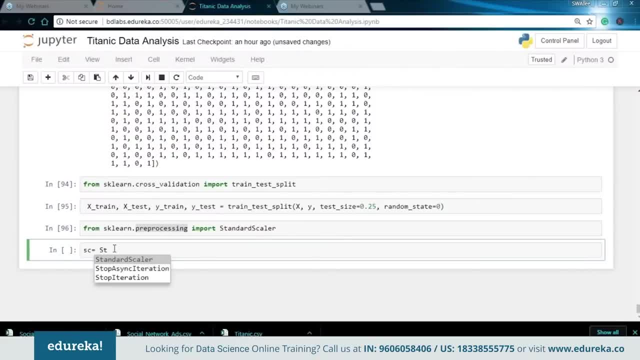 set. So I'll first make an instance of it. So I'll say standard scalar, then I'll have extreme. I'll say scfit, fit, underscore, transform, I'll pass in my extreme variable. And similarly I can do it for test, where in I'll pass the X test. 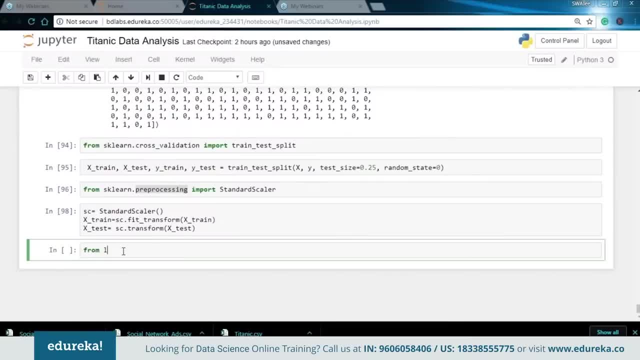 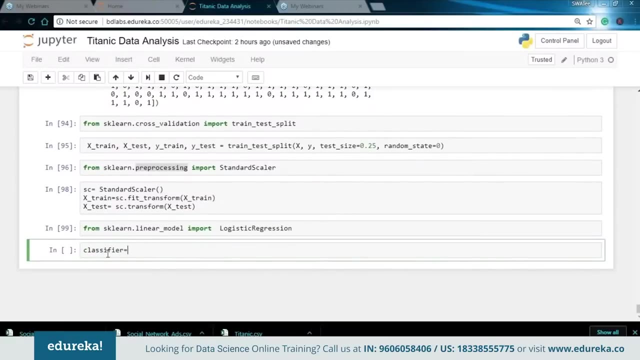 Now my next step is to import logistic regression. So I'll simply apply logistic regression by first importing it. So I'll say: from sklearn, sklearn dot linear model, import Logistic regression. Over here I'll be using classifier, So I'll say: classifier dot is equals to logistic regression. 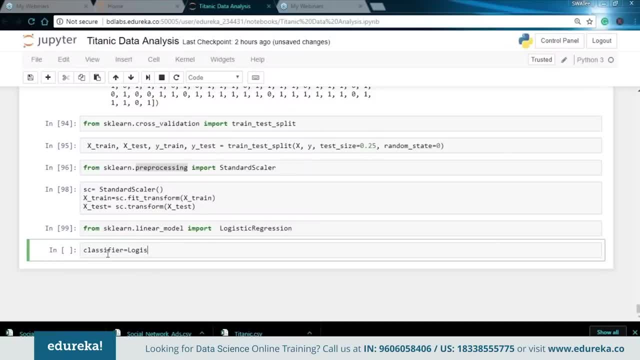 So over here I just make an instance of it. So I'll say logistic regression, and over here I just pass in the random state which is zero, And now I'll simply fit the model And I simply pass in extreme and y-train. 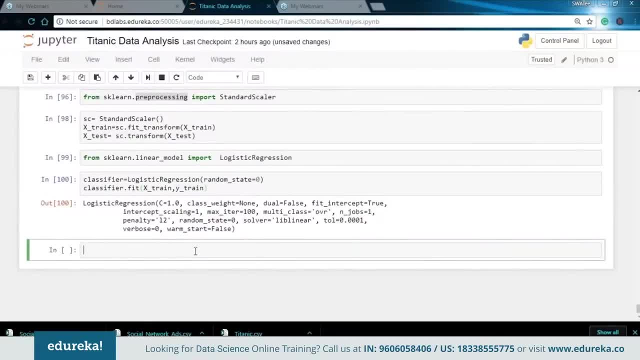 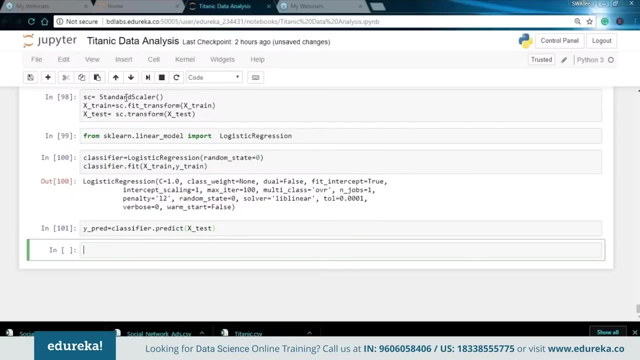 So here it tells me all the details of logistic regression. Then I have to predict the value. So I'll say y-train, it's equals to classifier, Then predict function and then I just pass in X test. So now we have created the model. 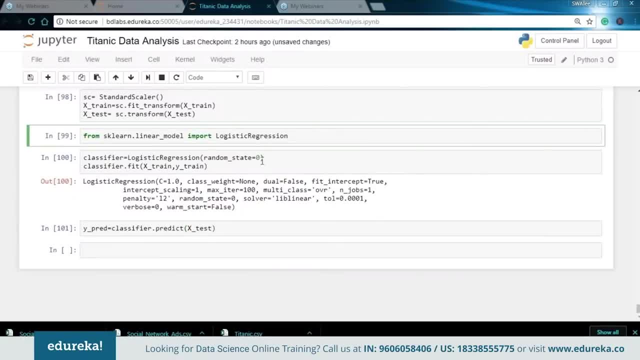 We have scaled down our input values, Then we have applied logistic regression, We have predicted the values and now we want to know the accuracy. So to know the accuracy, first we need to import accuracy score. So I'll say, from sklearn dot metrics, import accuracy score and using this function, 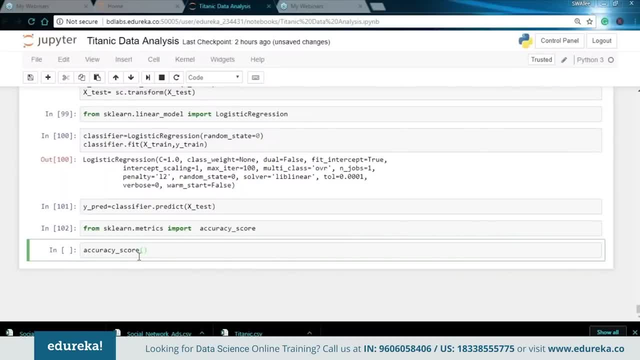 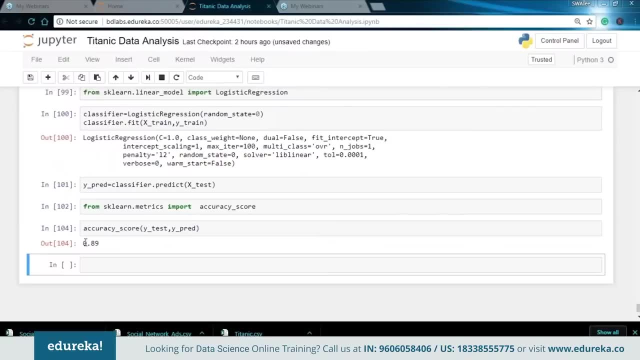 We can calculate the accuracy or you can manually do that by creating a confusion matrix. So I just pass in my y test and my y predicted All right. So over here I get. the accuracy is 89%. so we want to know the accuracy in percentage. 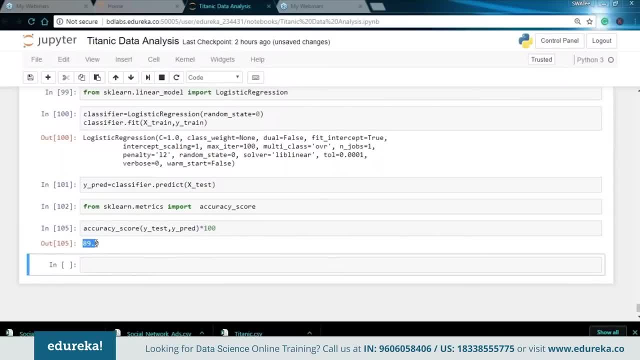 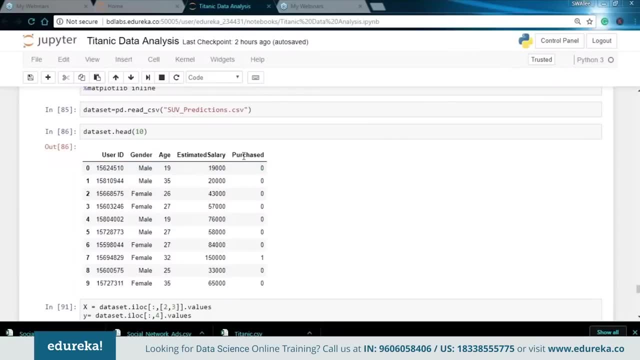 So I just have to multiply it by hundred, and if I run this, so it gives me 89%. so here I have taken my independent variables as age and salary, and then we have calculated that how many people can purchase the SUV, and then we have calculated our model. 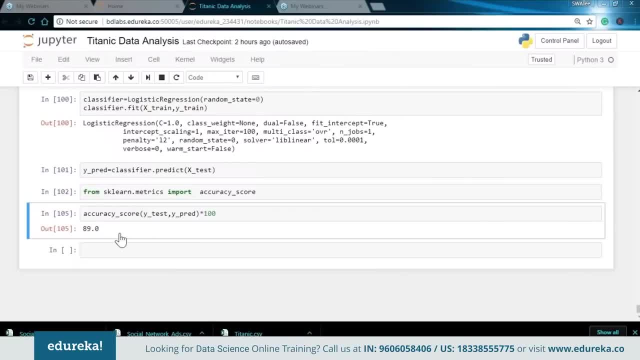 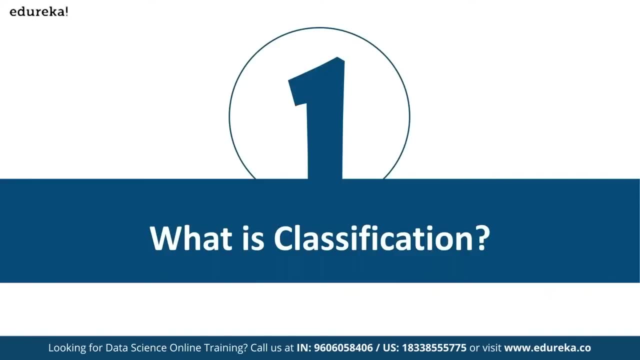 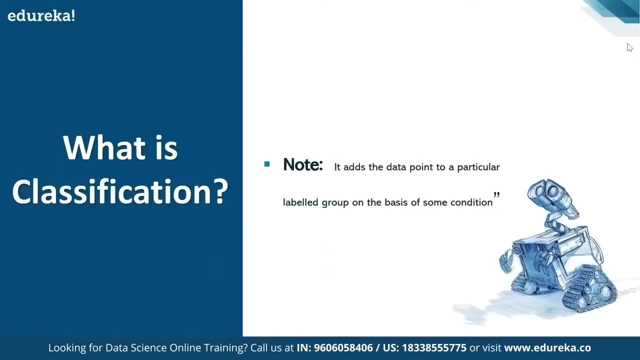 By checking the accuracy. So over here we get, the accuracy is 89, which is great. So what is classification? And if I have to tell you about classification like, for example, what happens is like we have two type of when we talk about machine learning. machine learning is nothing, but you know. 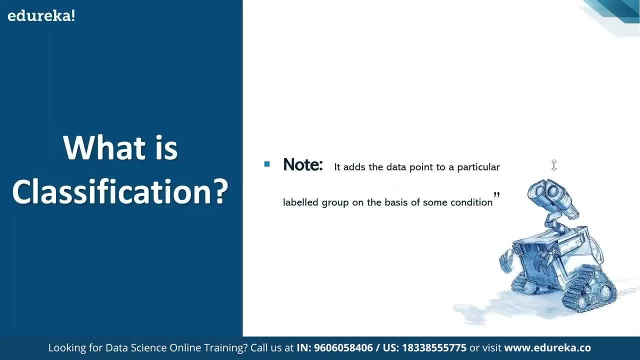 like a series of much instructions. you give it to the computer so that it can learn The patterns from your data set right. to give you an example, Imagine that there is a trending topic, For example. you found it. you want to find it out whether prime minister Modi will be. 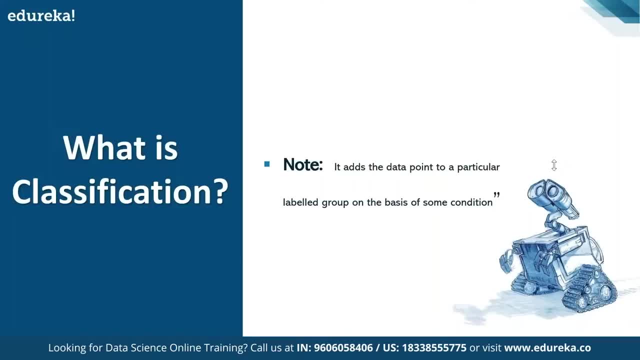 the second prime minister, once again the prime minister for the country, or not? Okay, So now what you will do is you will collect the data set from multiple different sources and you will, you will actually build it a like a algorithm, where you you will get a. 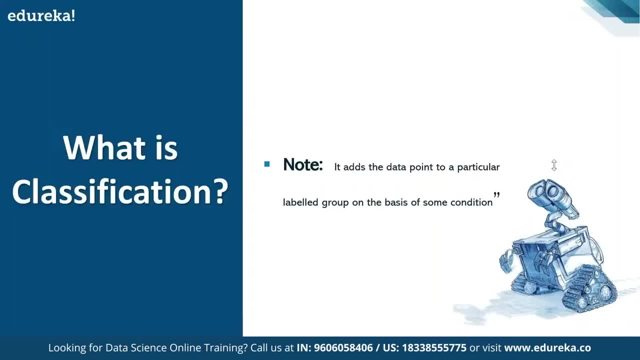 label as yes or no. Yes, he will continue as the next prime minister or no, He will not continue as a next prime minister. So you will collect the data set and you will feed this data set to the computer, and this process is called as a machine learning right. 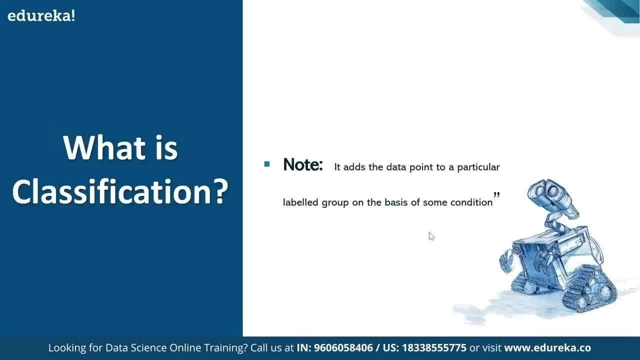 So now, in this case, what happens is so this: this is about the classification, right? So now machine learning is basically of two type. one is called as a supervised machine learning, another is called as a unsupervised machine learning and the third one is a rain. 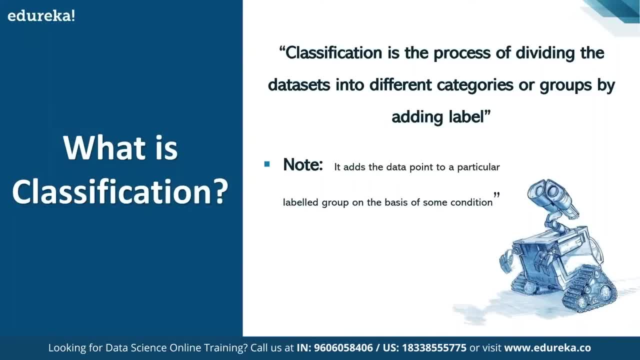 enforcement machine learning. So when we speak about supervised machine learning, As the name suggests, it provides some supervision right. For example, the teacher teaching the kid is a supervised machine learning right. So we will give the trained examples, We will give the train data set with a pure label on top of that. 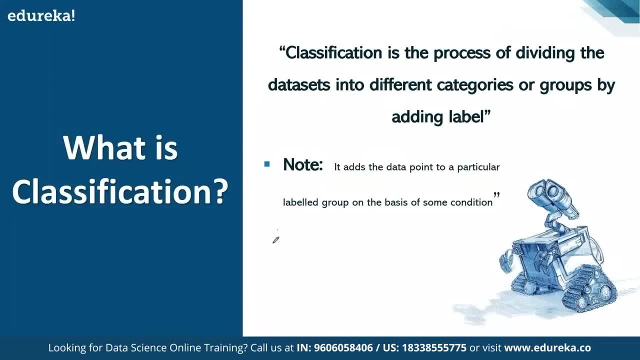 This is called as a supervised machine learning. So if I draw in front of you this type of machine learning, look like this supervised machine learning where what happens is like you would have the data set, which is a structured data set, and you would have one column, which is called as a label. 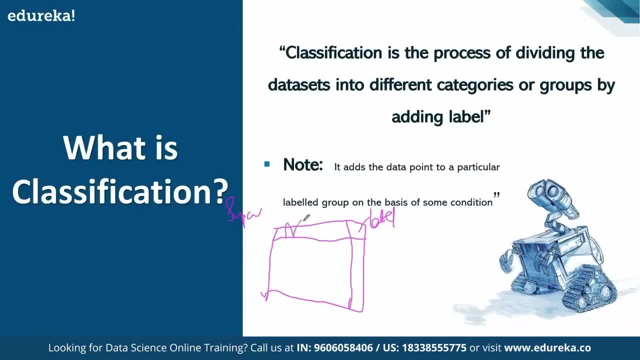 What you want to predict. Okay, and you would have a various predictors by which you want to predict. to give you an example, Imagine that you want to predict a pricing of a community. Okay, you want to predict what would be the pricing of apartment in a particular community. 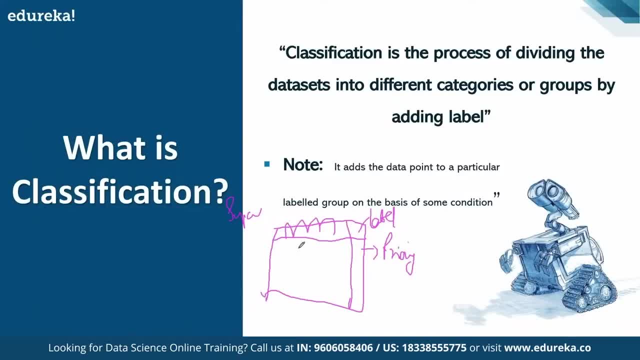 right now This can be the variable. like you can see that, what would be the number of how many floors it has? you can have a variable like: what is a pollution level? how many educational institution are nearby right? So based upon that, the pricing will change. 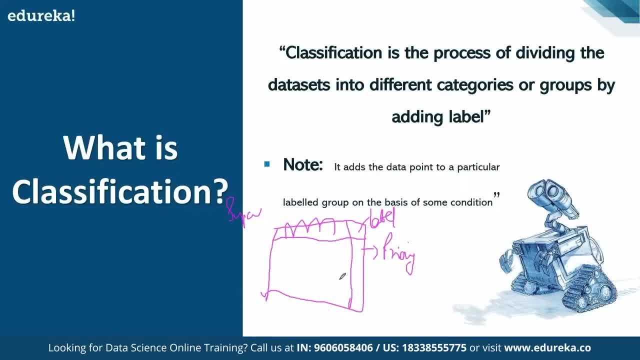 This type of supervised machine learning. why it is called supervisor machine learning? because we provide the independent variable or we provide the predictors. Also, we provide the label data set. Okay, Now, this supervised machine learning is basically of two type. this supervised machine learning- one type, one first, is called, as the, you know, regression based supervised machine learning. 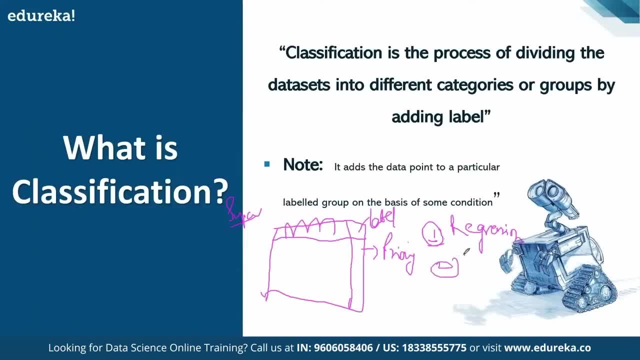 Okay, and the second one is called as a classification based supervised machine learning. Now, what is the difference between regression based and a classification based supervised machine learning? regression based supervised machine learning is that machine learning where what you want to predict is continuous in nature. 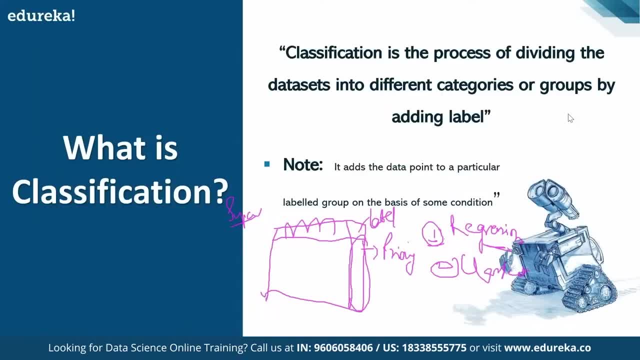 Okay, imagine the. you want to predict the community prices, right, which is a continuous value. If it is a continuous value, then we will go ahead with regression based supervised machine learning- Okay. whereas if you want to predict something which is the discrete. 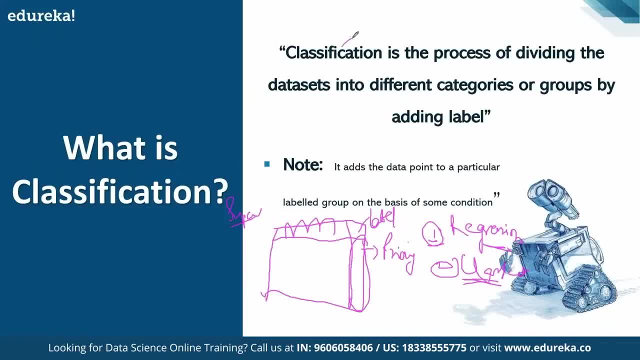 Outcome. to give you an example, you want to predict that, whether I will win the match or not, Okay, I want to predict whether the particular employee will churn out from the company or not. You want to predict, you know, like, whether the person will have a cancer or not. 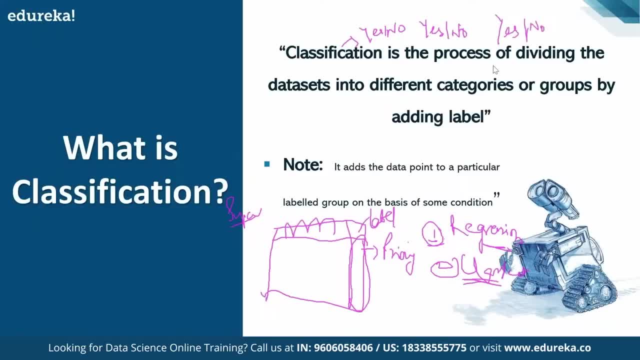 You're getting the point right. So if you have the output which you want to predict is in the form of yes or no, or true or false, right, This is called as the supervised machine learning, But a classification based supervised machine learning. 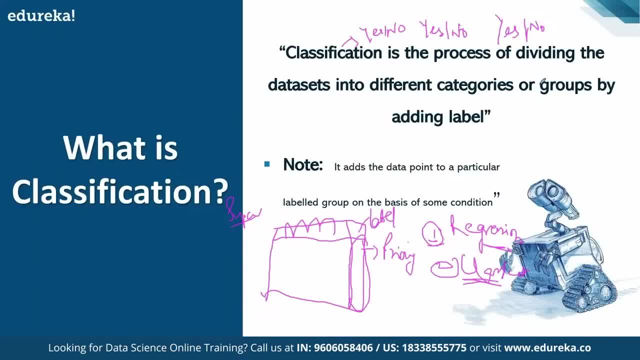 Okay so classifications based supervised machine learning is the process of dividing the data set into different categories or group by adding a label. Okay, So always remember that whenever you guys want to predict the classes in the data set, whenever you want to predict, you know, like, whether this will happen or not, whether the 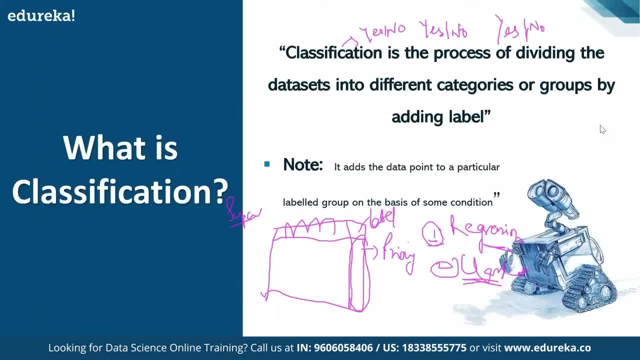 whether a person will do a credit card fraud or not, you're getting a point right. whether the employee will churn out from The company or not, right? whether the particular person will have a diabetes as a disease or not- all these questions wherever you want to find it out. 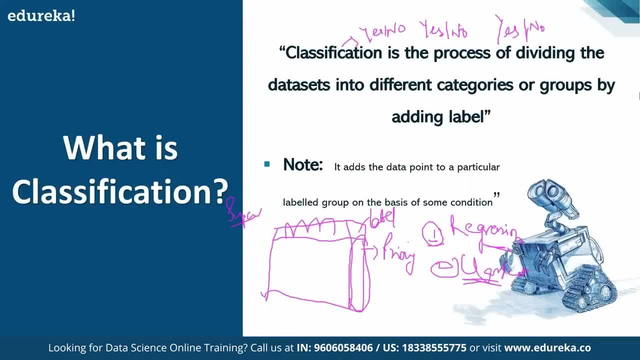 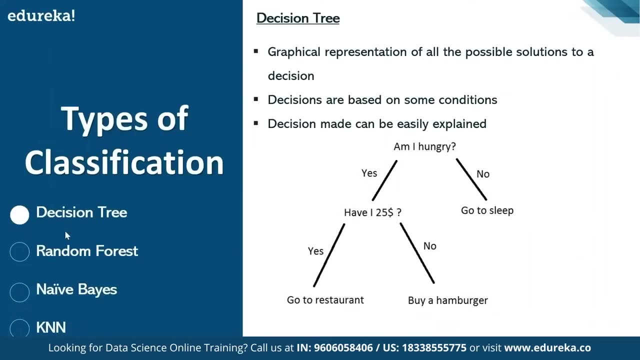 Yes or no, or true or false, or you want to predict classes in the data set. This is called as a classification based supervised machine learning. Okay, So this is what is called as a classification based supervised machine learning, and today I will teach you, you know, I will tell you about various form of classification based 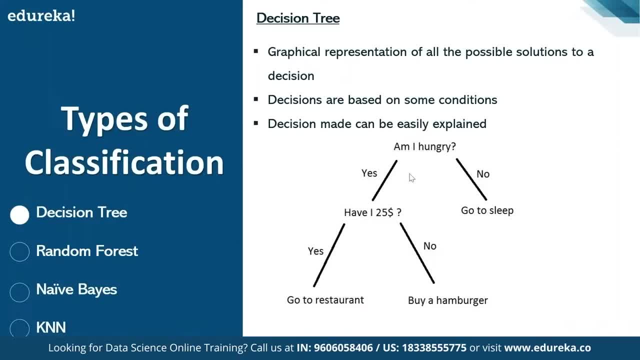 supervised machine learning. Although We will do a deep dive into decision tree right now, You will be able to understand that decision tree, how decision tree is connected to the network, what we are learning today with classification based supervised machine learning. Okay, So now we have various algorithms. algorithm is nothing but set of mathematical equations. 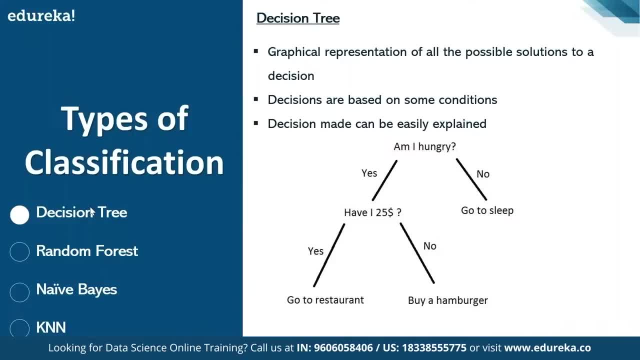 for classification based supervised machine learning. We, first of all, we have something called as decision tree, then we would have something called as random Forest, then knife base, and then KNN, which is called as a K- nearest neighbors. Okay, So let me give you a few statements about this algorithm- and we have many others, but 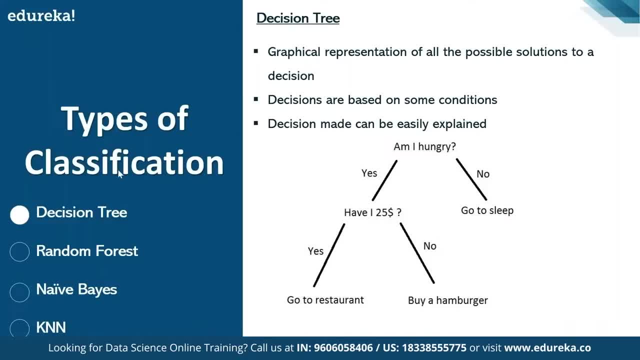 today we will focus on one of them, which is decision tree. So now, first, let's start with decision tree. Now, what is a decision tree? What I was telling you is, believe me or not, decision tree is something you use every day in your in your daily life. 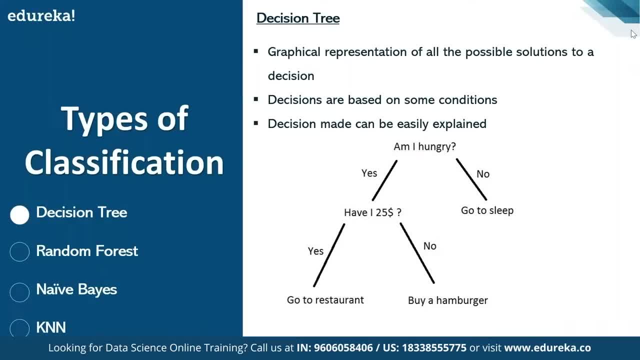 For example, you take decisions and, for example, today Also, you took a decision to attend this webinar, right? But how do you decide a decision based on various further decisions, right? For example, for today joining the webinar? you have seen that, okay, when this webinar. 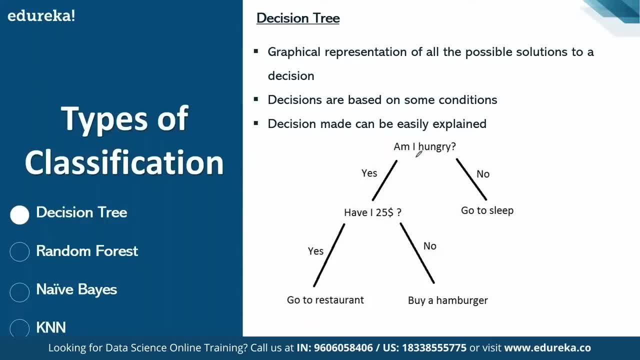 is about okay, So you said it is weekday or weekend. then you might have said, check it out, right, What is the time of the webinar? then you might have checked it out. What is the topic of the webinar, right? So, and who is conducting this webinar? 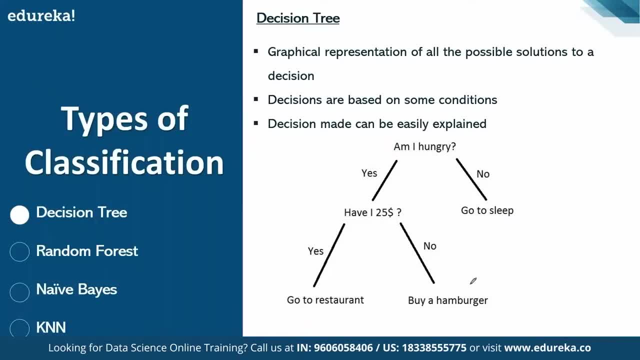 So, based upon this, you took a decision: Shall I go ahead or not Go ahead? You're getting my point right. So this is what is called as a decision tree. We call it as decision tree because it is a graphical representation of all the possible. 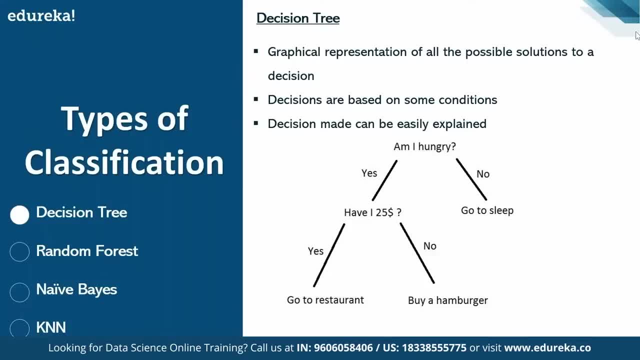 solution to a decision. It's like a tree, like decision tree is like a tree. Why? because a tree also start with a root and then it emerged into various branches. Similarly, you have a decision tree, which I am showing to you here as a simplest algorithm. 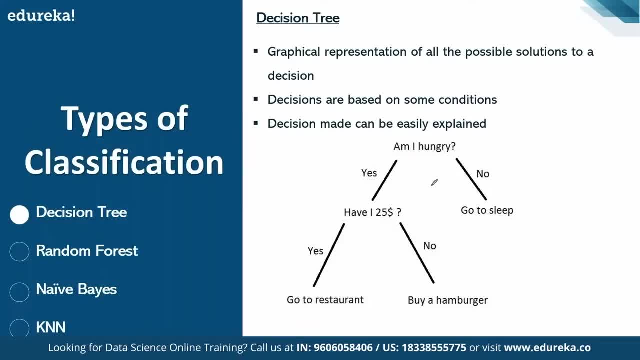 which is being used for machine learning purposes. Now, it is something like this: Imagine that You want to find it out that you know like: do you want to go to a restaurant or do you want to buy an hamburger? Okay, So you have two choices: either you can go for a restaurant or either you can buy a hamburger. 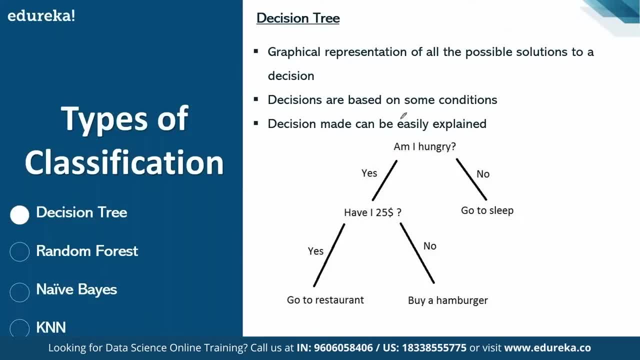 Now how would you decide which one you would follow? So you will start with what is called as a root note. You will start with a root note that, whether I am hungry or not, right, If I am hungry right, then only I will go for all these activity. if I am not hungry at all, 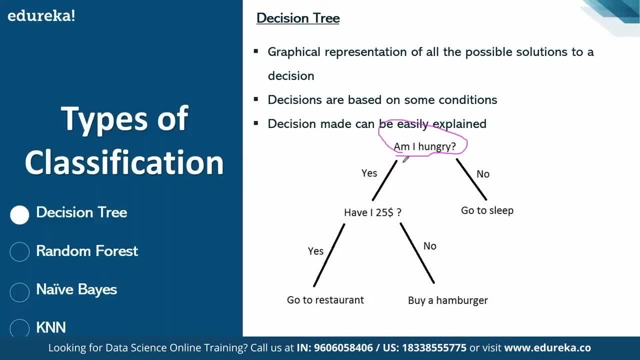 Then simply go and sleep. You got my point right, So this is how you will start with the first note, which is to find it out whether I'm feeling hungry or not. If I'm feeling hungry, then I will decide that. well, I do. I have money which is around $25 worth. 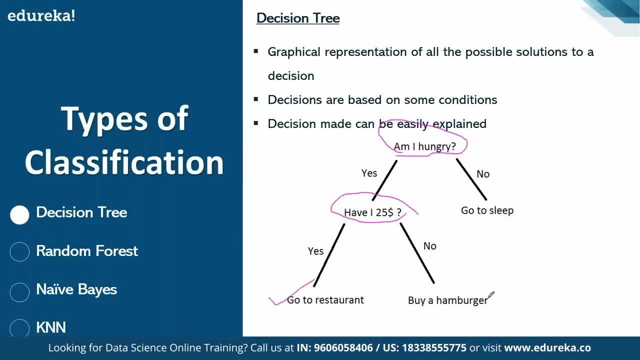 If I have money, then I will go for a restaurant. If I don't have a money, then I will buy an hamburger. You understood this. This is simplest representation of decision tree. Basically, you decide something on the basis of the previous. 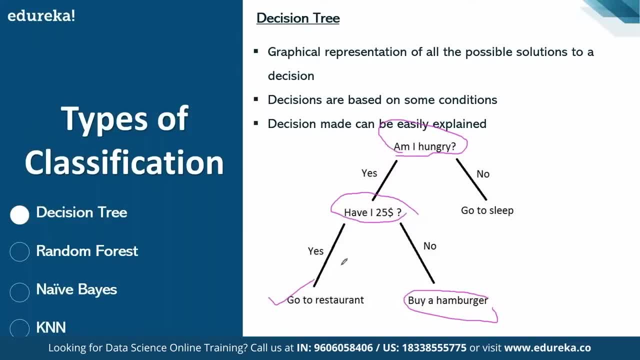 Outcomes, and you can imagine any sort of example here. Imagine that you want to find it out whether the person will do a credit card fraud or not. Again, It will depend upon the previous circumstances that you know. for example, it will depend upon how much 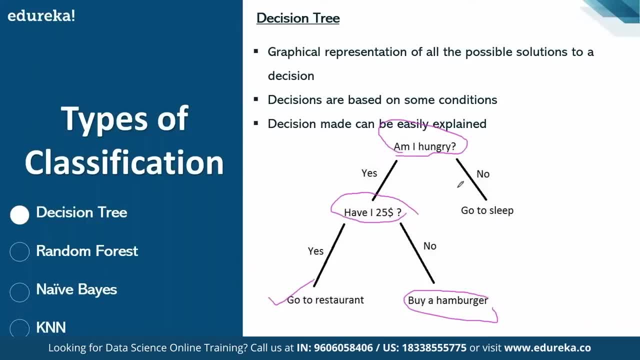 is the salary of the person, you, it will depend upon what is the job profile of the person. It will depend upon the fact that you know like, for example, how many fraud or how many cards this person have right. So on basis of you will decide that whether this will do a credit card fraud or not, 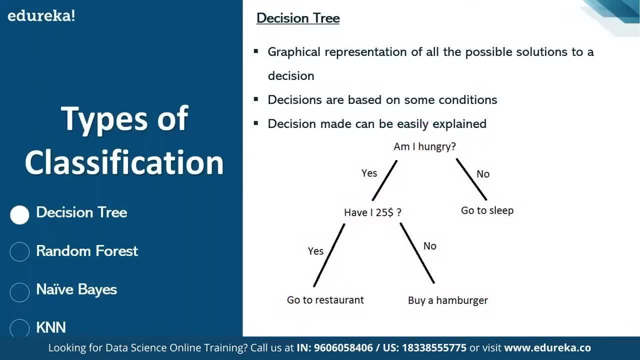 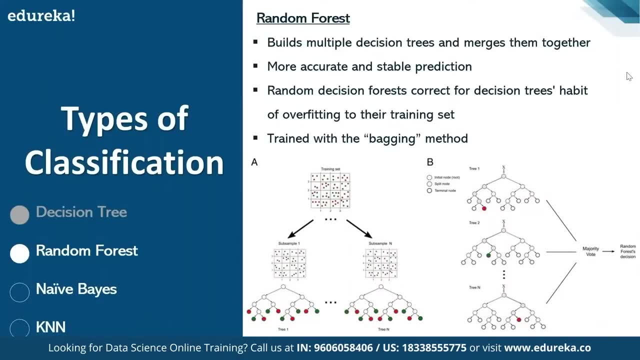 So this is the simplest form of classification based algorithm. Then we have the next algorithm, which is called as a random forest. Now, what is a random forest? as a name suggests, you built one decision tree in the last example, right? But one decision tree can sometime be overfitting as a case, right? 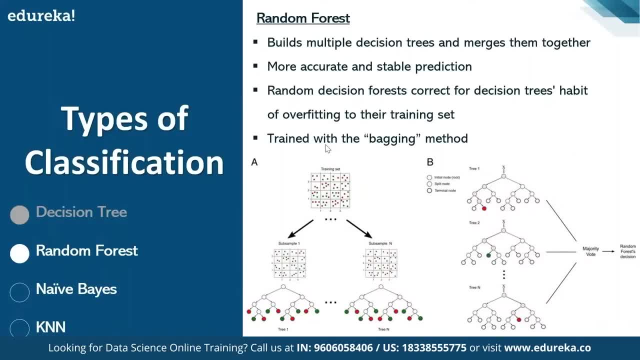 So people said that you know, like, why should I only trust one decision tree? For example, whenever you take a bold decision in your life, you don't trust only a single voice, Right? You want to hear it from multiple different people to make your decision more stronger, right? 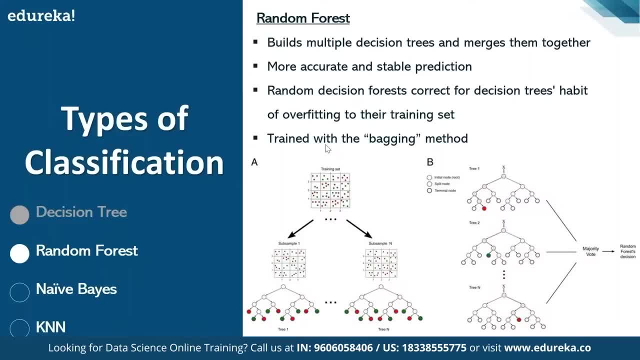 Go to a doctor. If the doctor says to you that you have this type of a disease, you don't believe in that, What you do is you also talk to second doctor, third doctor, fourth doctor to confirm that this is true or not. Okay, 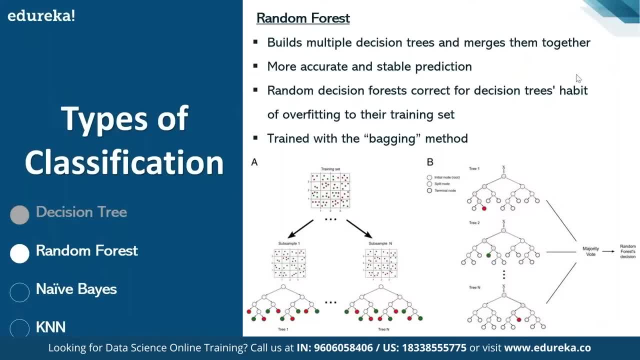 So this is what is called as a random forest, as the name suggests why it is called random forest. It is called random forest because now you are building the various number of decision trees Here. It's like a forest of all the trees, right? 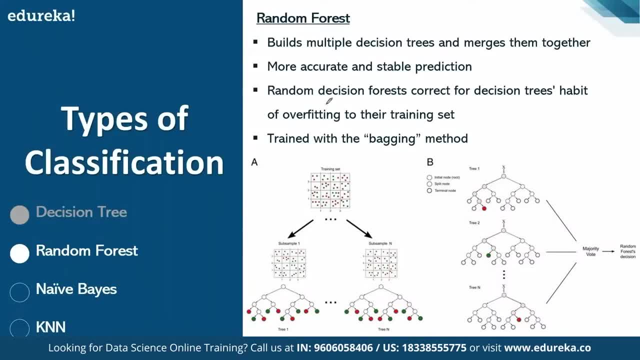 It is no longer a single tree, It is a forest of complete trees. So, for example, you can imagine that if it is my training data set, I will. I will split my training data set into multiple examples. multiple decision trees will be built and then, based upon the majority, 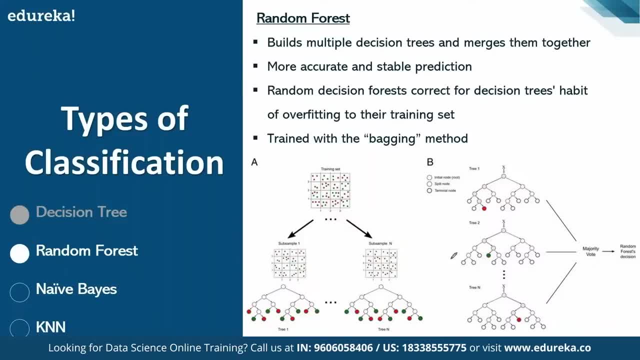 I will decide whether should I do this or not. Okay, So it is also called as a bagging sort of methodology, where we bring the outcome of various models, or we bring the outcome of various trees all together to make the, to make our powerful decision. 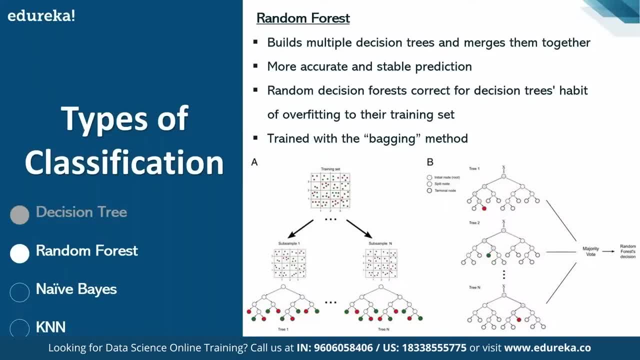 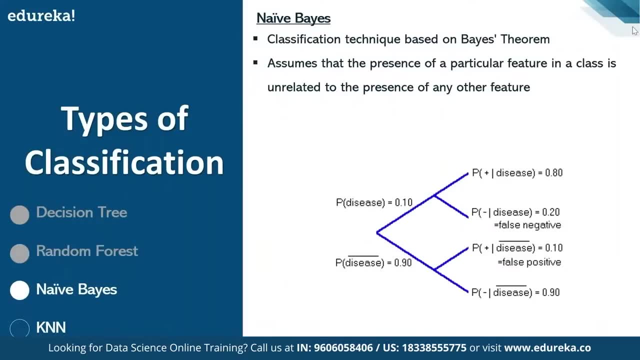 Okay, This is another algorithm which is called as a random forest. Then, after random forest, we have something called as knife base. Okay, Now, what is a knife base algorithm? Knife base is a also a simplest algorithm, but knife base is basically based on the base theorem. 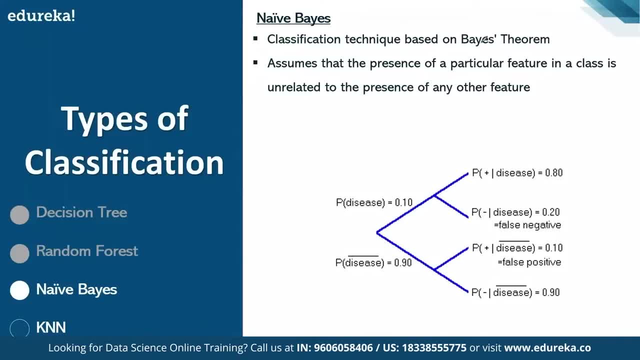 Okay, so this algorithm is basically based on the base Theorem, and base theorem is based on the conditional probability, right? So it is based on the conditional probability, which is your knife base. Now, in the name name base, What happens is like we decide that, whether something will happen or not, on the basis of probability. 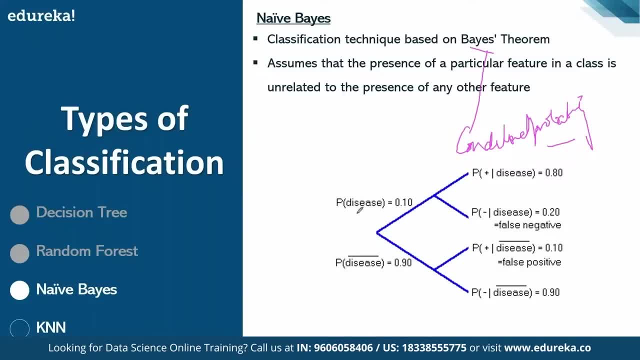 So let me illustrate you with this example. Imagine that you want to find it out whether I would have a disease or not. Okay, So first of all, the probability of having a disease is 0.10 and the probability of not having a disease is 0.90.. 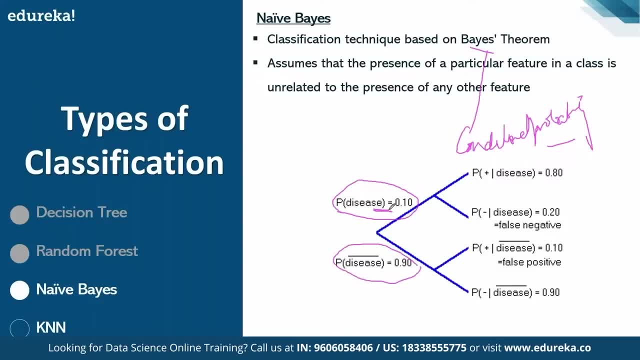 Okay, So if there is a probability of having a disease is 0.10, you will further find it out that what is the probability that my test will be positive, given I am diseased? What is the probability that my test to diagnose the disease is negative, given I have a disease, right? 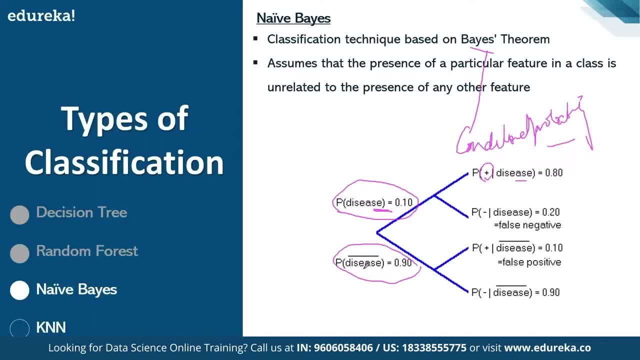 Similarly, if you go into this direction, if there is a probability of not having a disease is 0.90, you will find it out that what is the probability of having a disease test being positive with having with no disease And what is the probability of no disease given. 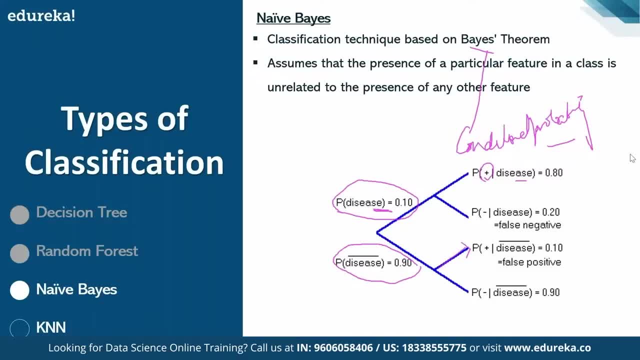 I don't have the disease, which is 0.90.. So, basically, here you check the outcomes, here You check the outcome of all the party, all the possible combinations. This is what is called as the Base algorithm, or base theorem, or, you know, conditional probability based theorem. 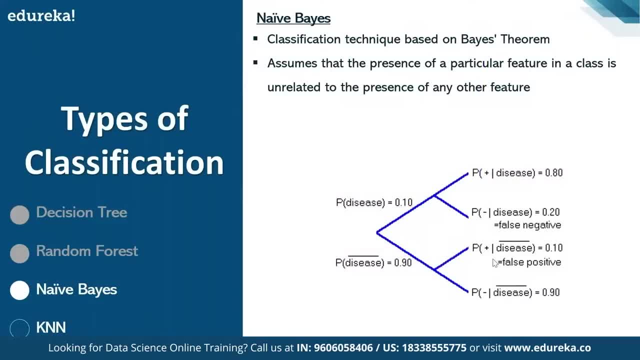 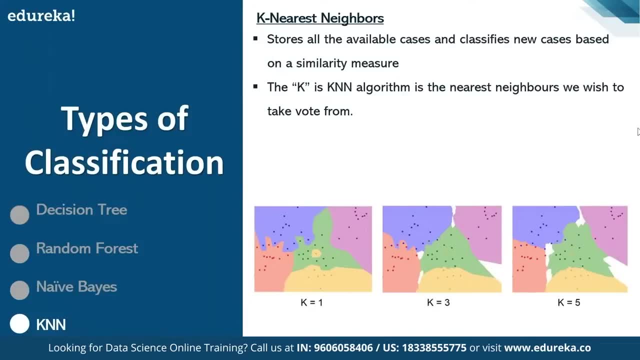 Okay, Then we also have something which is called as a key nearest neighbor, which is the one of the finest algorithm, which also helps you in deciding the classification right now. What is K nearest neighbor? K nearest neighbor, as the name suggests. what happens in this case is we try to build. 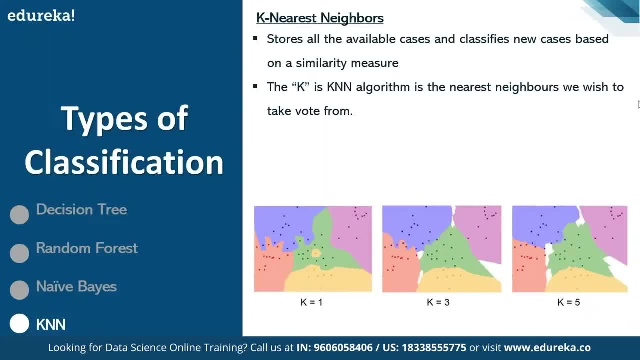 you know we try to build Basically it's like a neighbor. So it's something like this: Like if I give you the data set, say I give you the customer data set, Okay and I it is a transaction data set. 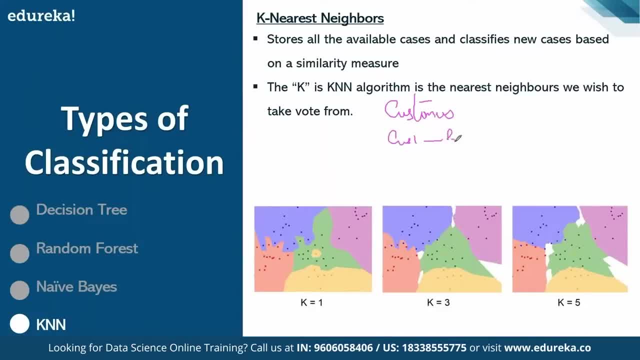 So customer number one has bought a product number one right from a particular vendor at a particular rate And this is a profit This customer has given to us and this is the revenues. Okay, this is my class customer number one. Similarly, you would have customer number two, customer number three customer. 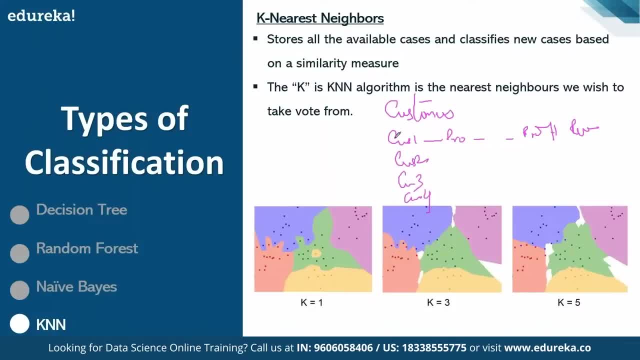 Customer number four: right now, if I ask you that which customer profiling is same, is nearby, same right. So what you can do is you can group your customers or you will get to know that which customer behave in the similar way, So you can say that customer one, customer three and customer for they behave in a similar way because they are giving us the high profit and high revenue margins. 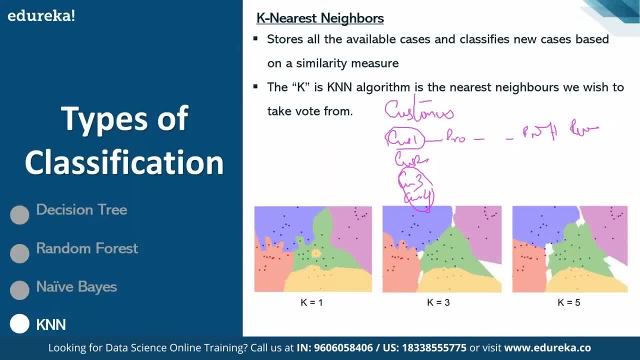 You understood. So this is what happens in the case of K nearest neighbor. So, K nearest neighbor, What you generally do is you find it out that what I would be able to you know, find it out Who is my nearest neighbor. 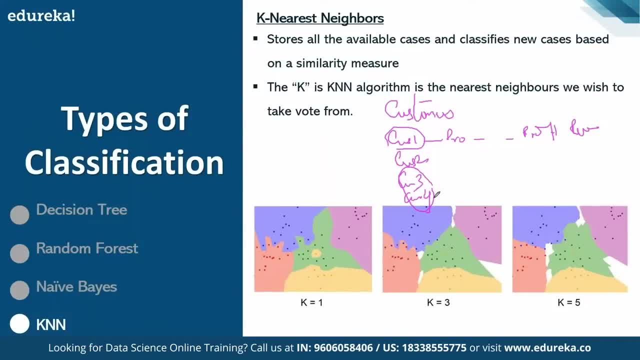 Like: what are the similarities in the patterns? We have right, This is what we use for K- nearest neighbors and this you can see that, for example, the algorithm based on the distance based mechanism find it out that how many people or what type of audience is similar to the outcomes. 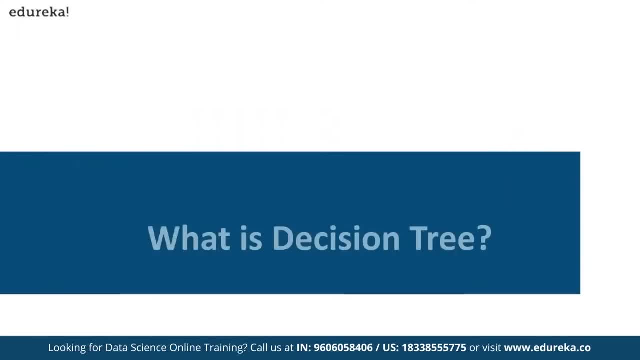 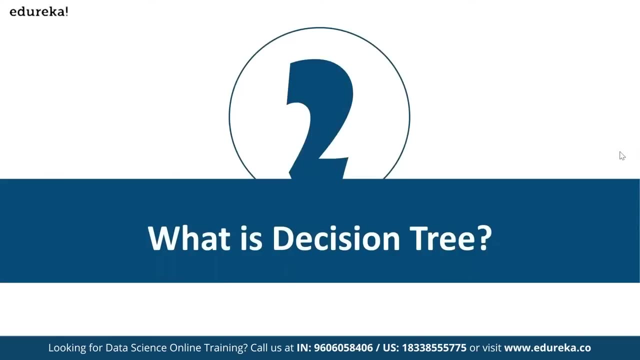 right? So then, moving further here with the second topic, let's go into detail about what is decision tree all about, right? So so far I have touched base on classification based algorithm, right, And I was teaching you different type of classification based algorithm. 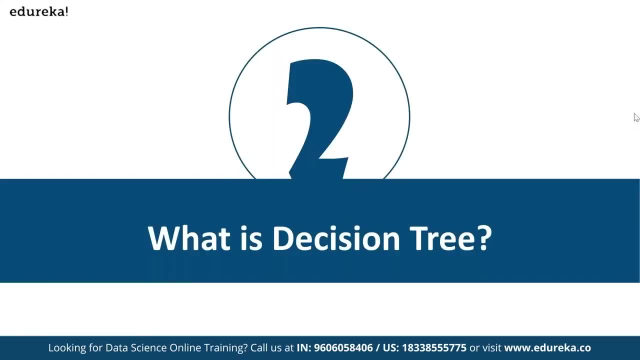 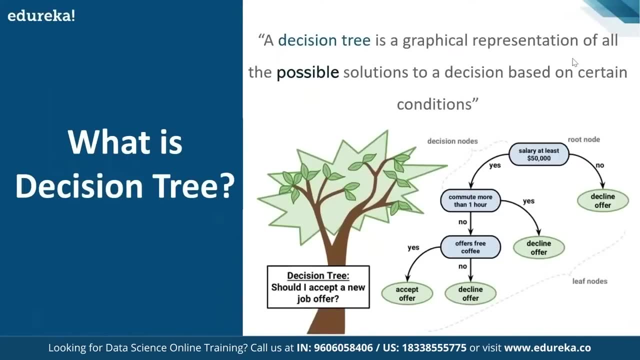 But since the focus of today's class is decision tree, let's take a deep dive into the decision tree. Okay, so let's get started with decision tree. A decision tree is a graphical representation of all possible solution To a decision, based on a certain condition. 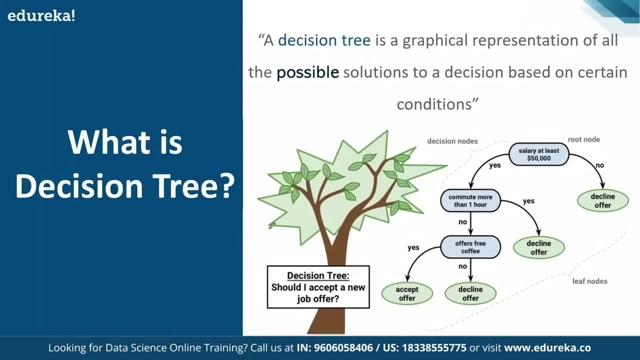 What does it mean? It means that it is as simple as that. Imagine that this is a tree, right? So it is like a tree where you have a problem. statement that: should I accept a job offer or not. Imagine that you want to find it out that should I accept a job offer or not. 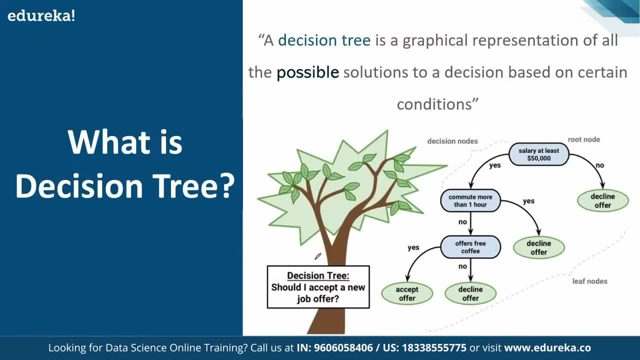 This is a problem statement which is there in your mind. Now, how would you solve this problem statement with the help of our decision tree? First of all, you will start with what we call as a root node. We will start with a root node, starting with: you know. 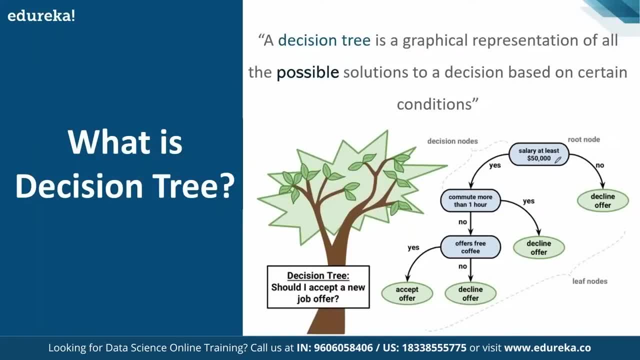 to find it out. What is a salary? Okay, what I'm, what I, what is the salary I'm getting? So if my salary is equal to or greater than equal to 50,000, I'll go here If my salary is not greater than equal to 50,000.. 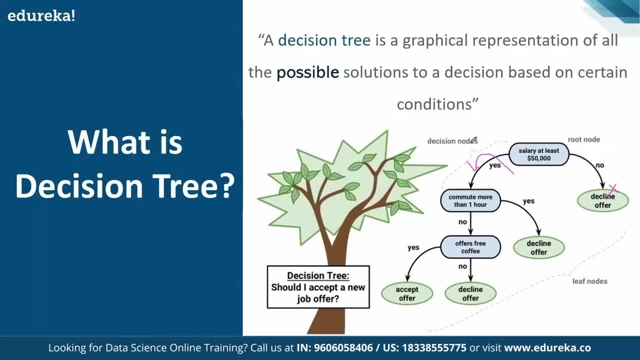 I will say I will not accept this offer. Okay, Now imagine that you say that your salary is greater than 50,000.. Then you will check another, another variable here. You will check it Out better. I have to commute more than one hour. 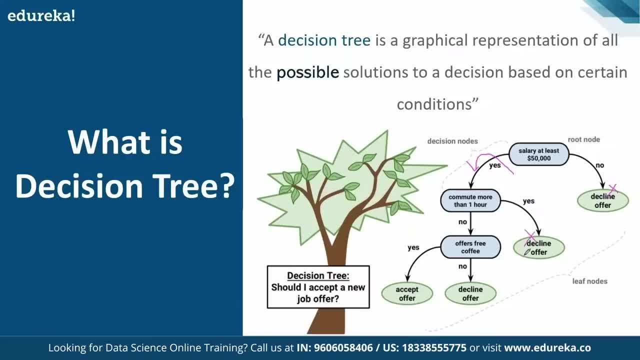 If I have to commute more than one hour, I will decline the offer. Then, if you don't have to commute more than one hour, then you will still consider this option and then you will check it out, For example, in this case, 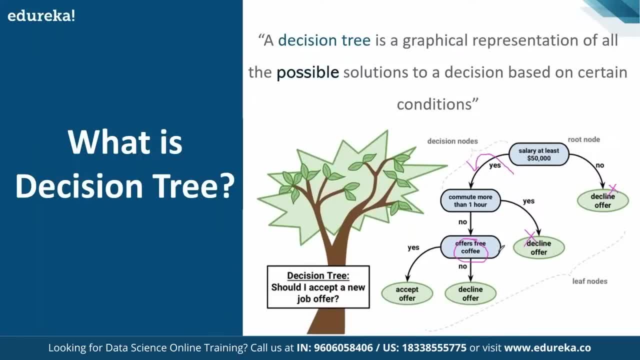 we are checking it out whether you are getting the free offers also like coffee or some snacks or other things like that. If yes, then you will accept finally the offer. Otherwise you will decline the offer. You got my point. This is how our decision. 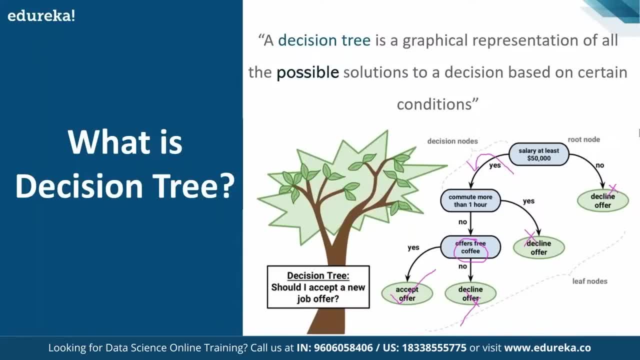 Tree works Basically. decision tree will keep on splitting, keep on splitting unless and until you are able to find it out your decision. Okay, So here the decision was. shall I accept this or not? Right, So it will keep on splitting. keep on splitting unless and until you. 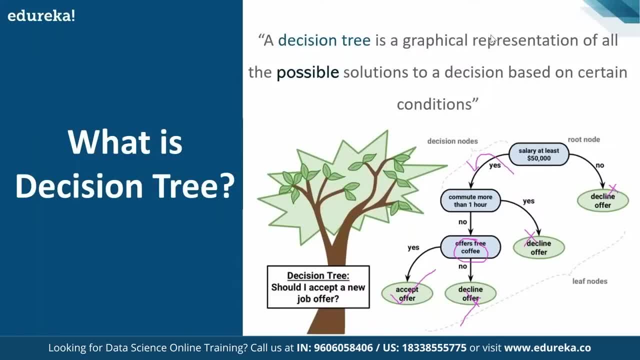 get your decision. whether you do this or not. like this example which I have to, I have explained you. Okay. Now, with this, what happens is like: let me, if I go further and explain you further on this. Let's understand this more importantly. 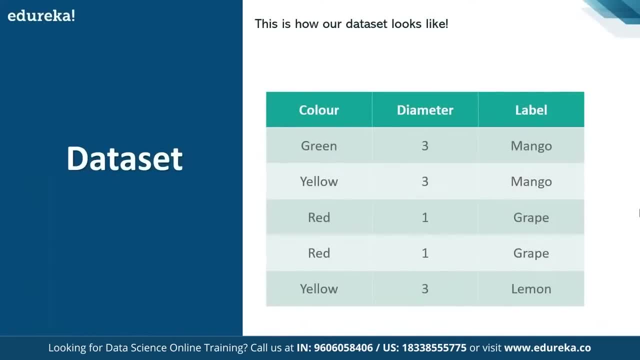 right, Let's understand this one by one. So imagine that this is my data set. Okay, Now in my data set you can see that I have various colors given to you. It's like a green color, yellow color, red color, red color and a. 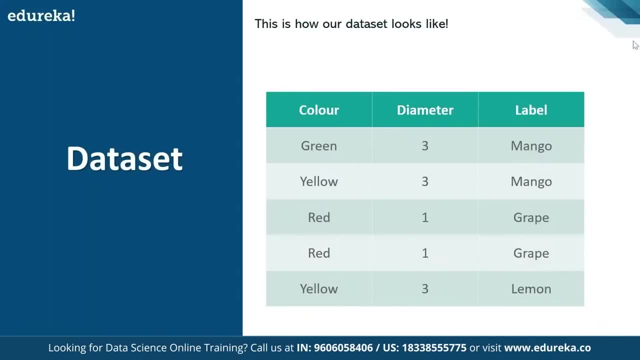 yellow color. I am saying if this is a, if there is a green color fruit with a diameter of three, right and I can say it is a mango, where, as I am saying, if it is a yellow color and a diameter three, still will be called as a mango. if it is a red color with one diameter, then it is. 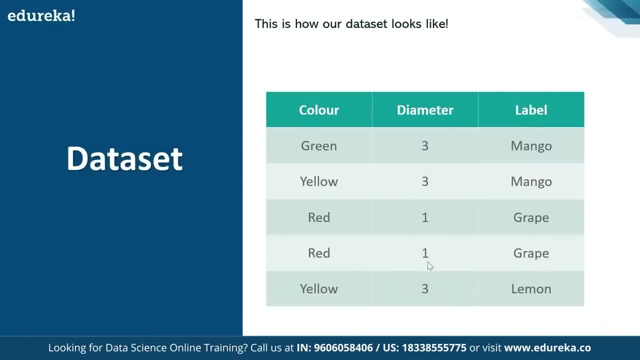 a grape, and it can be. a red color with a diameter of one still can be a grape, but even a yellow with a diameter of three can be lemon. Now, what is happening in this case is if you have this type of a data set where you want to predict the label of the fruit right, 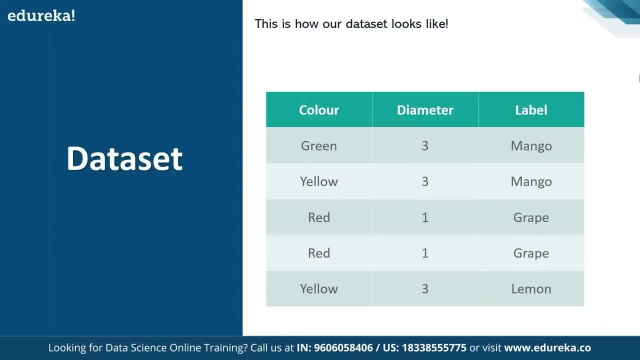 You want to predict whether a fruit will be mango, whether a fruit will be lemon right, Or whether a fruit, in this case, is mango and lemon or grape. I have to build a classifier, which is a decision tree classifier, on the basis of this data set. 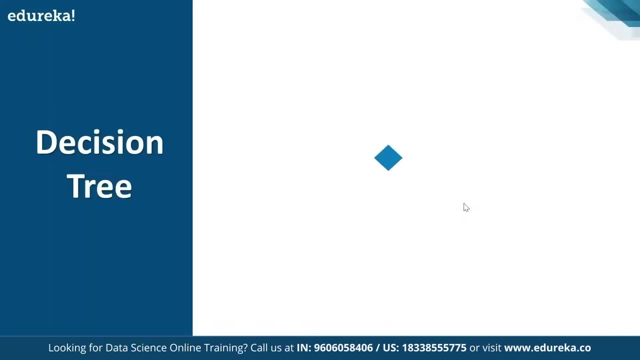 Imagine this is a problem statement given to you Now. First of all, what you will do here is you will take this data set right. You will take this data set and you will start with a root node. root node Imagine here is like: is my diameter of the fruit greater than? 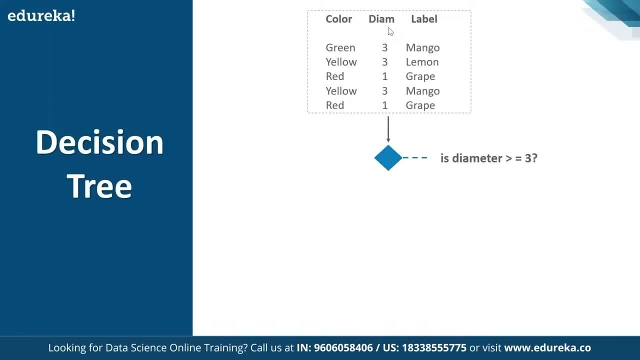 equal to three or not? Okay, is my diameter of the fruit Greater than equal to three or not? If it is greater than equal to three, right now, if it is greater than equal to three, you can see that you have three fruits here. 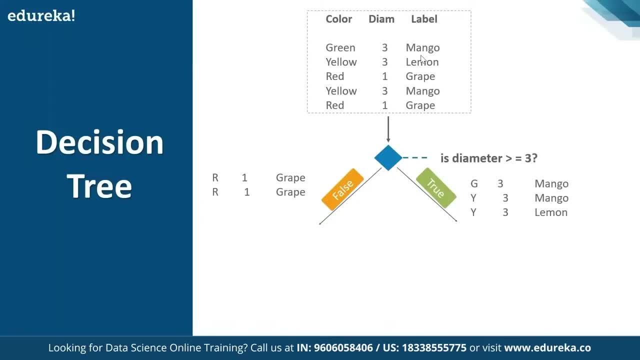 three rows of the data set here. One is green with three mango, yellow with three, lemon yellow with three mango. and wherever it fails in the condition you are left with, where the diameter is not greater than equal to three, It is less than equal to three. then, which are the data set? 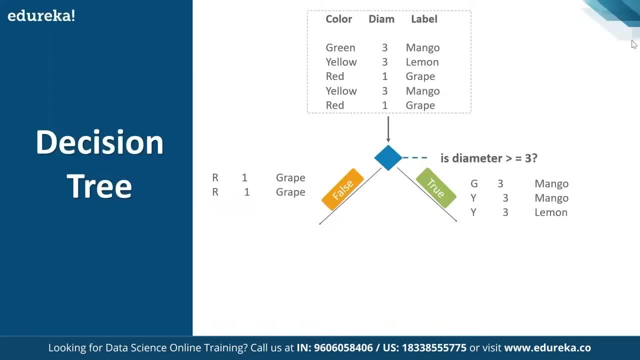 We have red one grape And red one grape, Okay, so I hope you are understanding this right, how we have starting with the decision tree, with the based on one condition here, right, which is diameter. now, based upon this, What I will do is I have to split it further here, in this case. 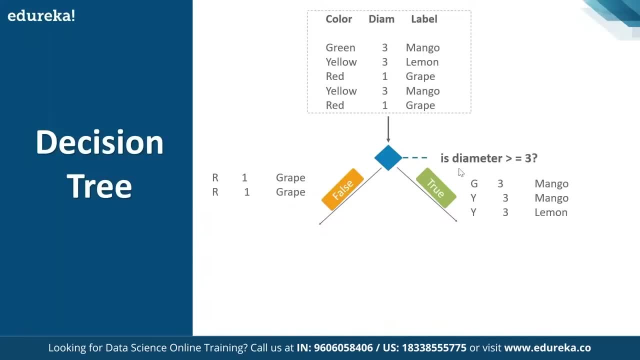 I don't have to split it because I already got the result. So, if my diameter is greater than equal to three in my data set, if the diameter is not equal to greater than equal to three- I know it is a grape right- Whereas 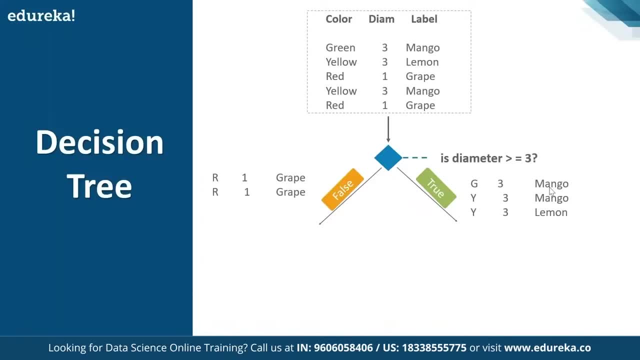 If the diameter is greater than equal to three, then it can be a mango or it can be a lemon, I'm not sure in my decision. So what I will do here is I will split it further. So I have to split this further here. 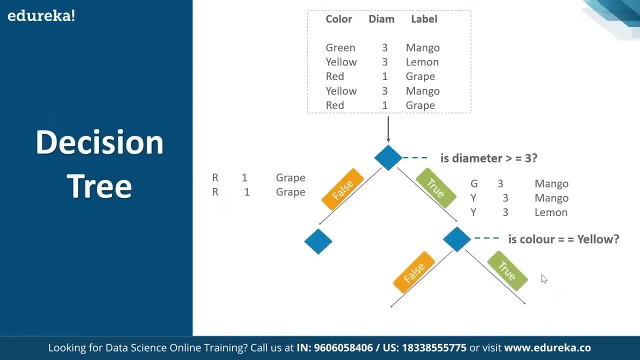 The splitting is not required. But if I split this further, I may check it out Now. is the color equal to yellow or not? Now, if the color is equal to yellow, then I have two fruit, which is your, this row, which is you know. 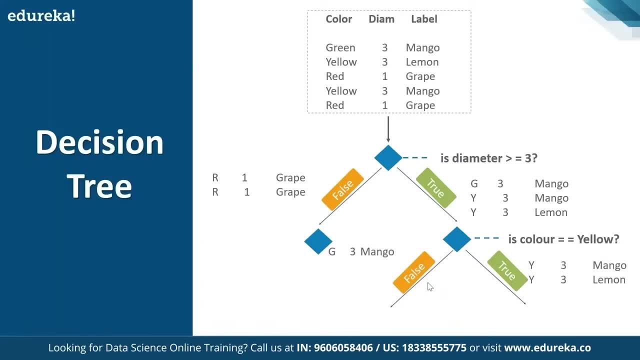 your mango or lemon, And if the color is not equal to yellow, then you will have the another row of the data set, which is you know, which is you are left with right. So this is how you have done this work in the case of your. 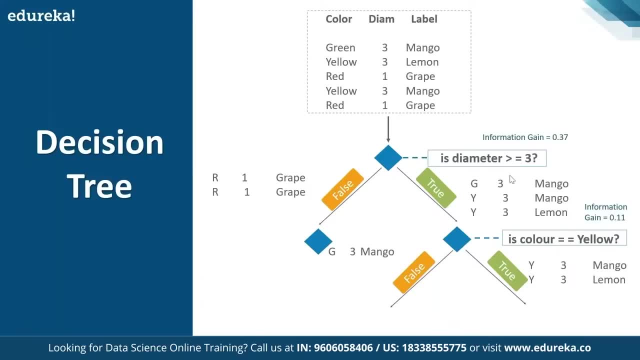 decision tree. Okay, and how you will find it out at which type of the criteria or which type of the algorithm I should, or which type of criteria or variable I should choose here. to split the tree is on the basis of Gini index, Andy. 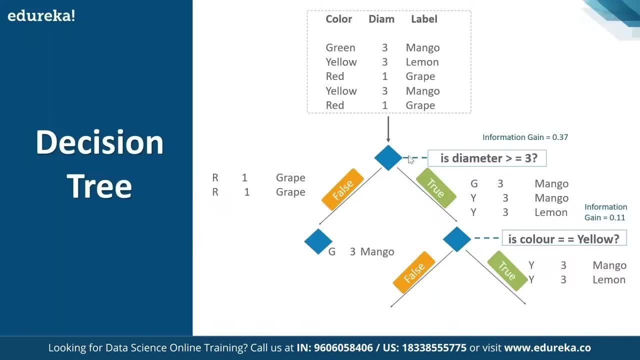 Formation gain how your decision tree works, basically on the basis of the condition, and if you get a pure subset, then no need to split it further. If there is no pure subset, you will keep on splitting. keep on splitting unless and until you get a pure subset. 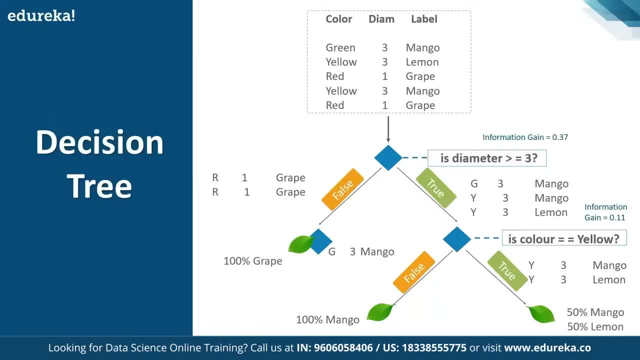 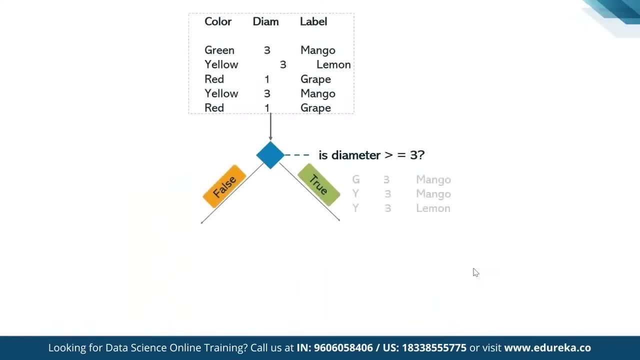 So in this case, what has happened is you got hundred person mango here. You got 50% mango and 50% lemon. So now this is what like. how does it work? right Now? this all depend upon the Gini index basis right now in the 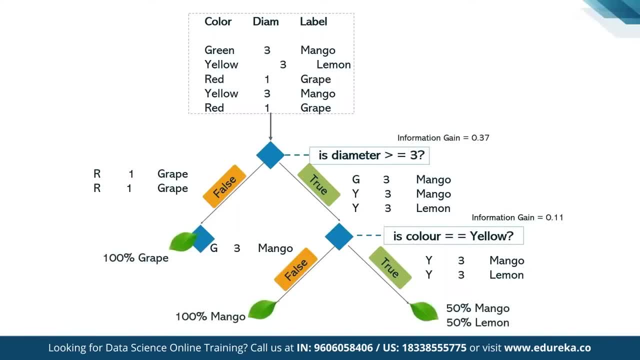 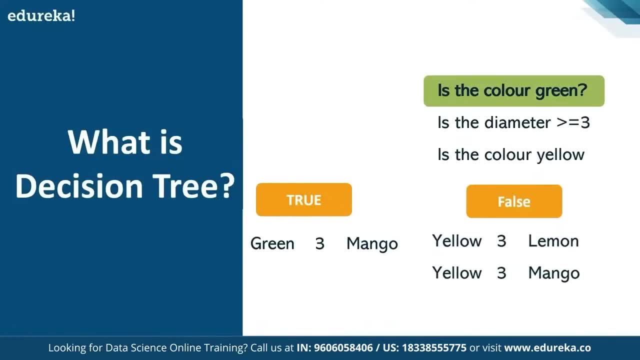 next subsequent slide. Let me tell you and explain you about Gini index and information gain. How does it work? Right? How does that something works on the basis of your Gini index. So imagine that you know like, imagine that I have a feature. 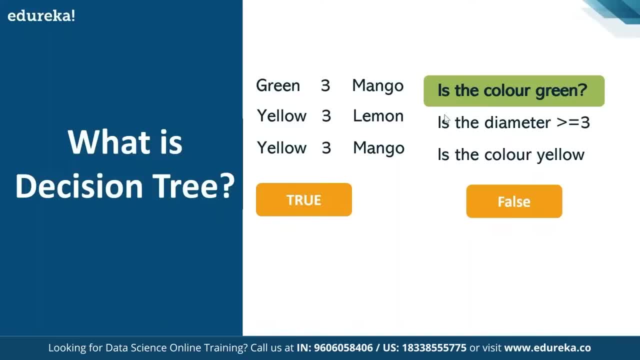 here is the color green or not, right basis of whether the feature, whether you have a color green or not. What would happen here is, if the color is green, you will get this row here. If it is not, you will get this, these two rows here, right in the 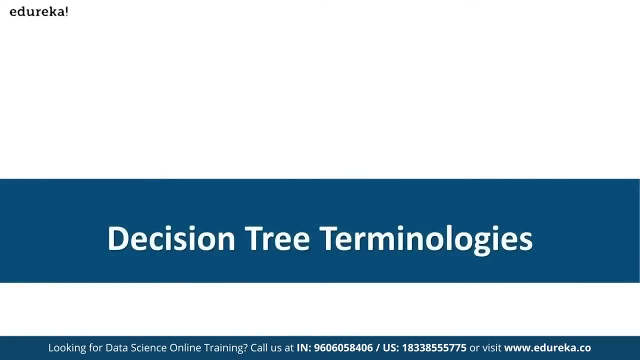 next, it may decide on the other basis- right, It can be. is the diameter which is greater than equal to 3 or not, and many other things. Okay, Now let's go ahead. the example and the questions which is coming to your mind, which is related to you know, decision tree. 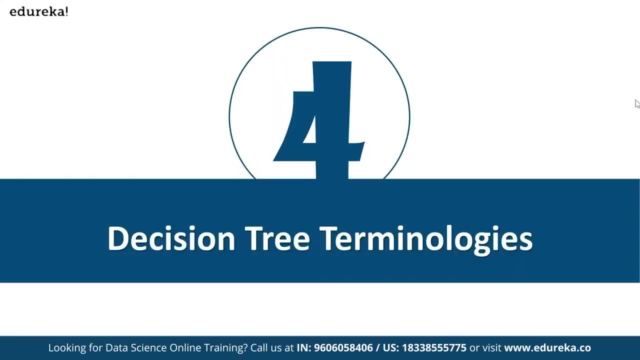 terminologies. I'm pretty sure you would have these questions in your mind And you would be thinking that how should I decided which feature I should use and which feature shouldn't I be using? This is a question which you had, and this is an excellent question. 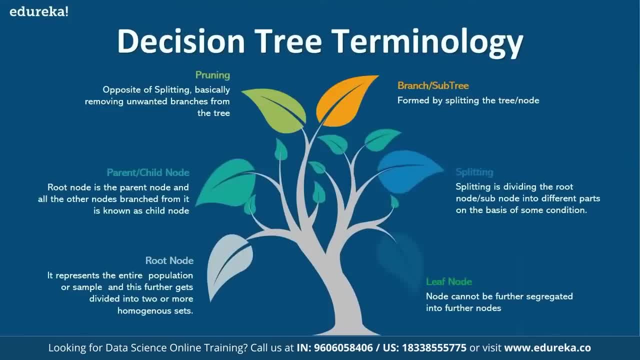 for understanding the decision tree. But before I go on to that, I have to tell you about some of the terminologies which we commonly use while we build the decision tree. So first of all, decision tree looks like this type of a tree based structure: 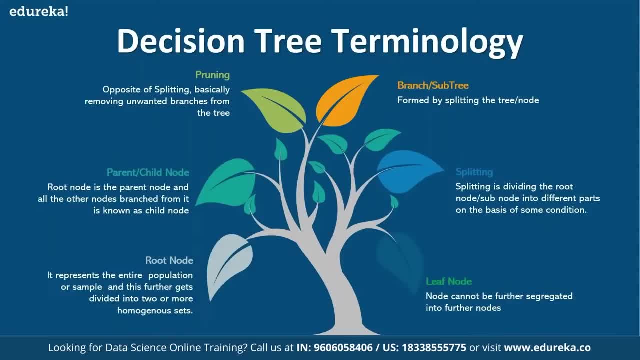 Okay, So every decision tree will have it root node. So root node is where the decision tree will start, So it represent the entire population or sample, and it is further get divided or into two or more homogeneous sets. as you know that this will be the first feature on the basis of your 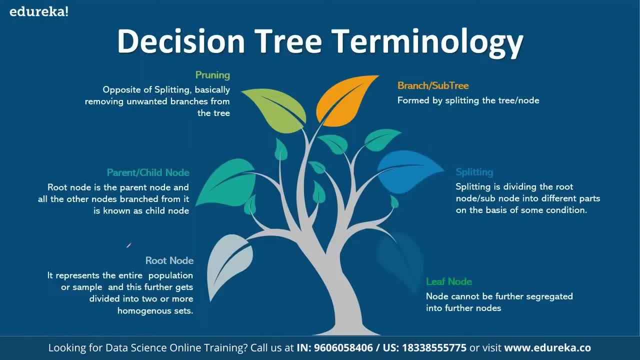 tree will start, like tree, start, with a root. your, in this case, your decision tree will also start with a root node. Okay, Now, once you have the root after that in a tree, what happens is you will start getting the branches right. I hope you understand what is branches in this case. 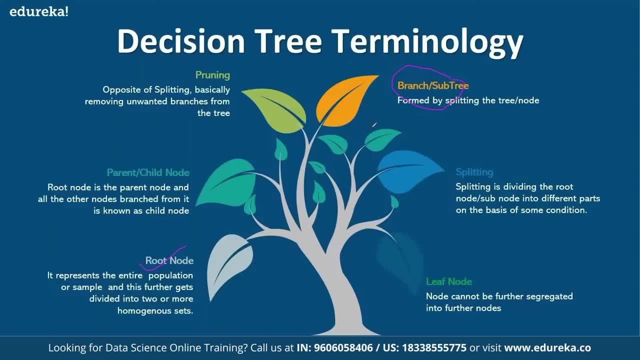 We will keep on splitting, keep on splitting unless and until we get a decision whether this will happen or not. So it's like a branches. Okay, then we would also have a parent or a child node. So child node is nothing, but when you have a branches, then 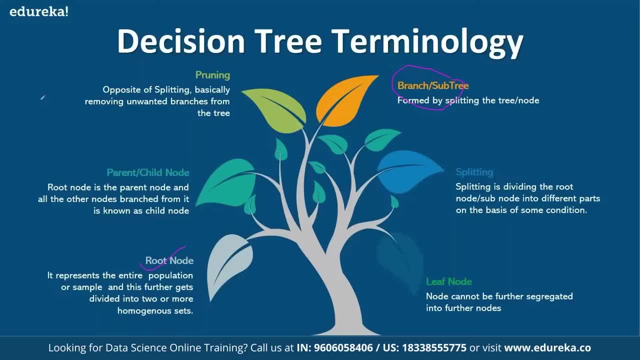 the branches can also have the outcomes. So in the previous example, like, for example, we have whether the diameter is greater than equal to 3 or not. You remember whether the diameter is greater than equal to 3 or not. if it is true, what is happening if it is a false? 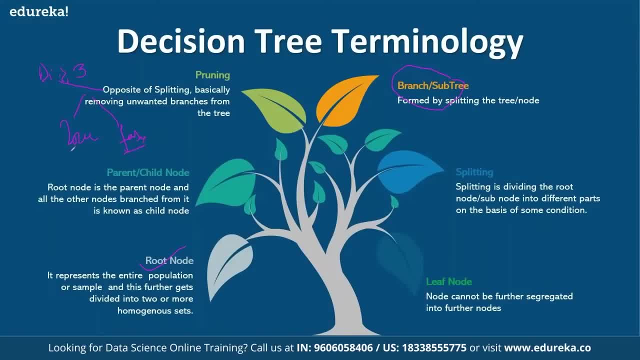 what is happening. So this is a child or child node. Basically, this is an intermediate node. This is not the final decision which is being made, So this is called as a parent or the child node. Then we also have other terminology here which is splitting. 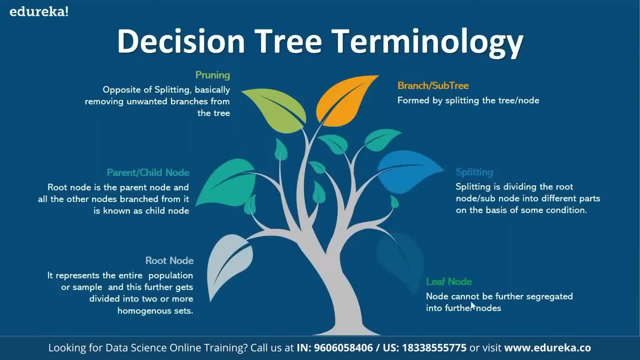 which you know that we will keep on splitting unless and until you get a desired node, and finally the tree, and with the leaf node. So always remember one thing: you will start your tree with a root node. root node is a node with which we will start the 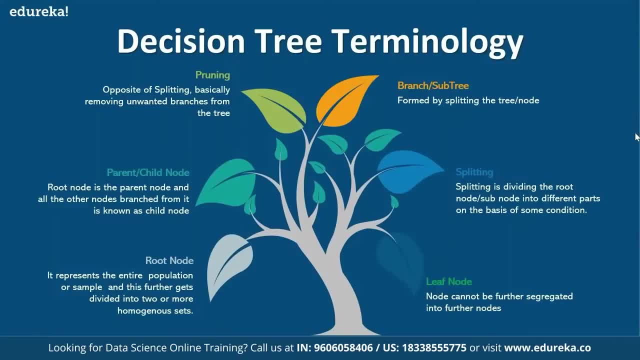 decision tree and you will end your decision as decision tree at a Leaf node where you will get a decision that you should do this or not. Okay, and now pruning is the activity where you will cut down the decision tree if it is pruned lot amount of times. 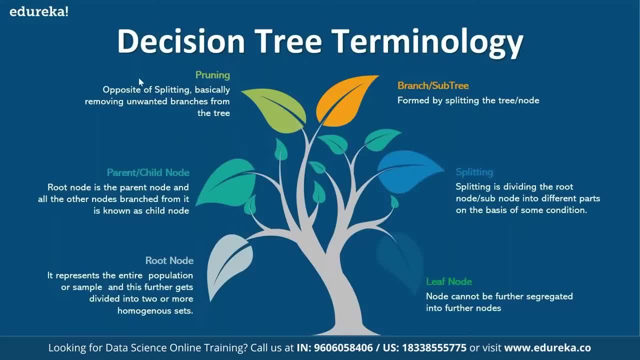 I will even explain you this. It is a case of overfitting. You shouldn't build thousand. You can shouldn't build thousand branches of the tree when it is not even required. So I'll explain you this point. Now let's move further. 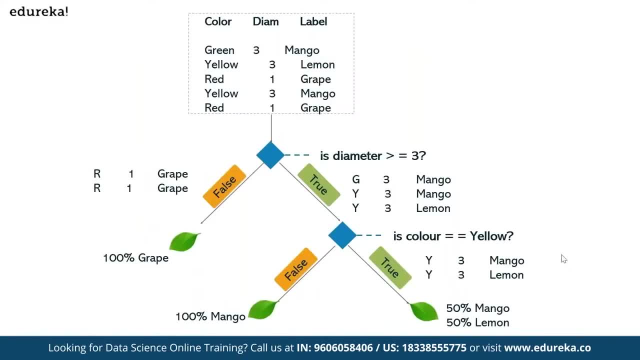 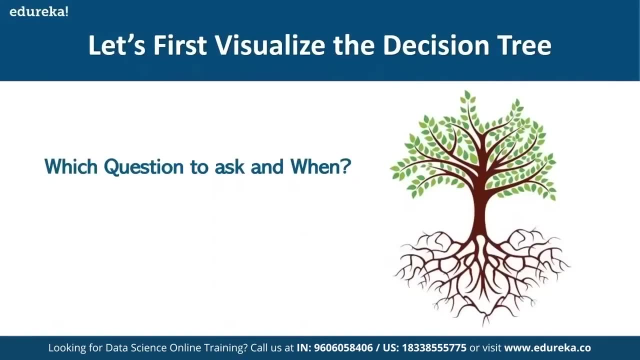 Here- and let's see this with the help of an example, which was your genie index and your information gain, right? So this is where you were asking me that which question to ask and when? right? how would you decide that which feature has to be taken first, right? 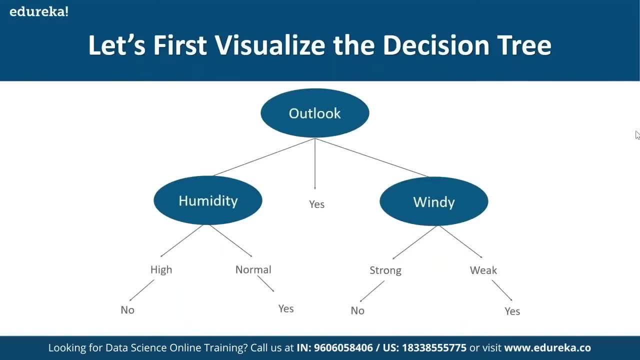 Let's take up an example here- and I would encourage everyone of you to hear me really fine here, because this is on the basis- how would you decide, or how the algorithm decide, to break this further, and I'm explaining you with the help of one simplest example, and we will do some maths over it. 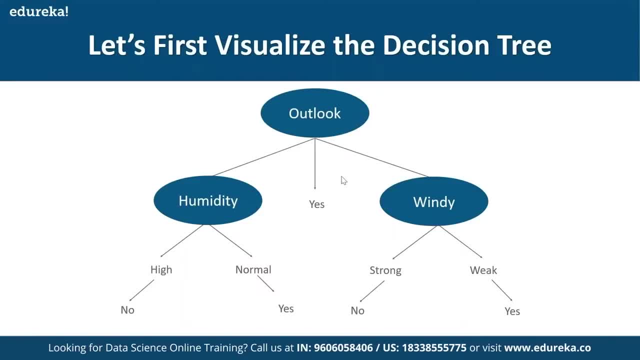 So imagine that there is a data set where I want to find it out whether I will play the match or not. Okay, there is a cricket match, or there is a football match, or whatever it is. I want to find it out whether I will play the match or not. 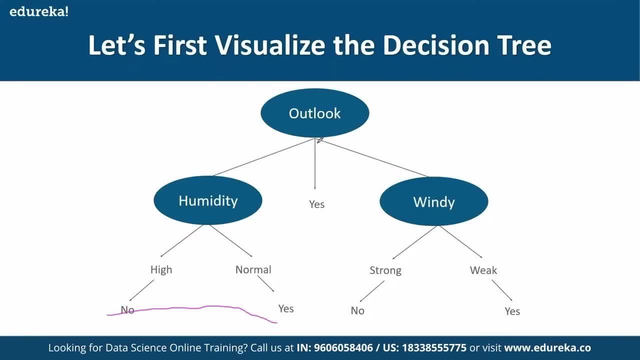 Okay now, How do the decision tree look? like this didn't look like this. if the outlook, if the outlook is humid, if the outlook is humid, and if the outlook is humid and humidity is very high, then I will not play the match. on the other hand, if the outlook is, 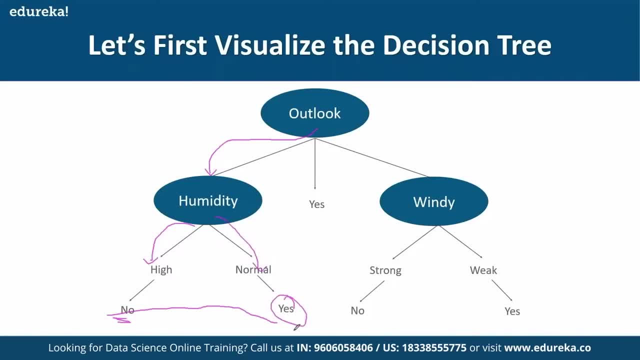 humid and humidity is normal, I may play the match. Okay, if the outlook is absolutely clear, then I will always play. on the other hand, If outlook is windy And the winds are very strong, I may not play the match. on the other hand, if the outlook is. 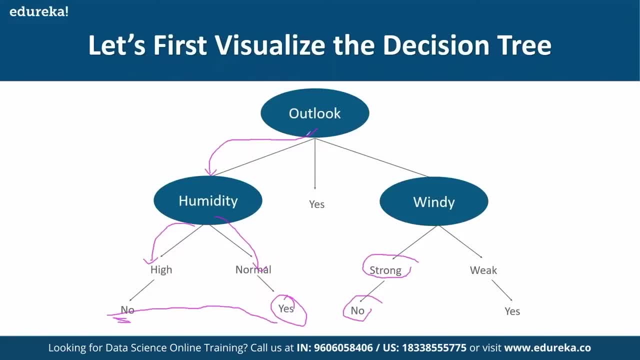 windy and the winter week I may play the match. So now what is happening again is that you are not sure how you decided with outlook, how you decided with these notes here, how you decided with these features here. Let me try to show you this entire data set. 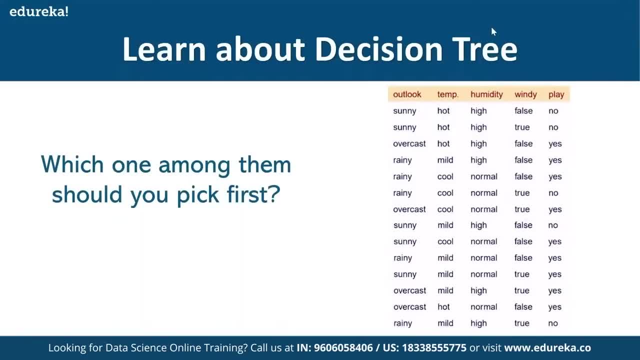 So this entire data set look like this: Okay, So this is basically your 14 days data set, and this exactly happens in the case of your Classification based algorithm. You will get a data set like this, So you can imagine that you want to find it out. 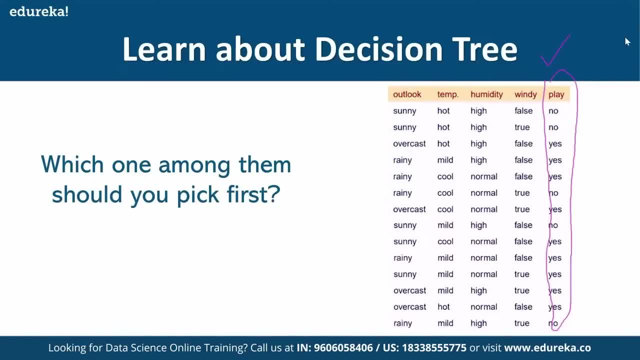 I would like whether I will play or not. right, This is what you want to essentially find. it want to find it out whether I would play or not. on basis of what? on basis of four different variables. You have four different variables or features in the data. 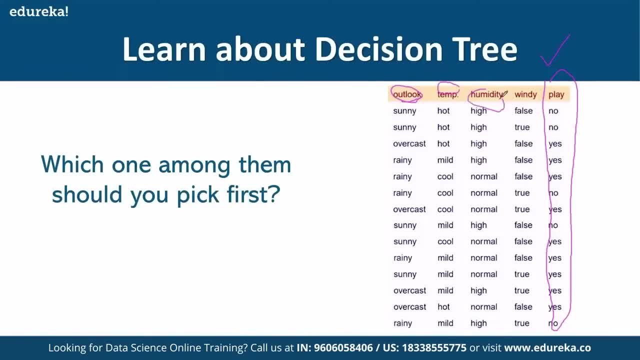 set is outlook, temperature, humidity and wind 9.. So now it can be like: The outlook is sunny, temperature is hot, humidity is high, wind is not there. I will not play the match. This is how you will read this one data point, right. 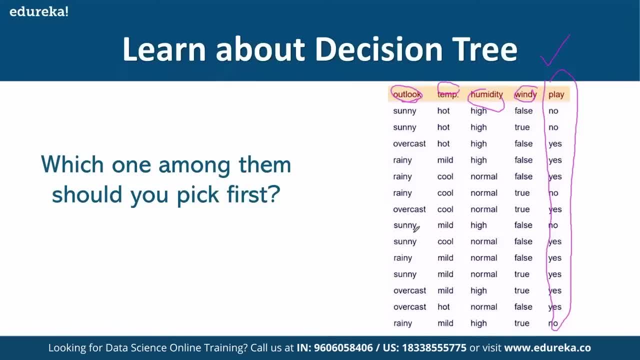 Similarly, I have multiple data point. now I have to decide: how can I build a decision tree and out of these four features, which feature should I use first as my root node, right? So this is what I have to decide, and let's do it accordingly. 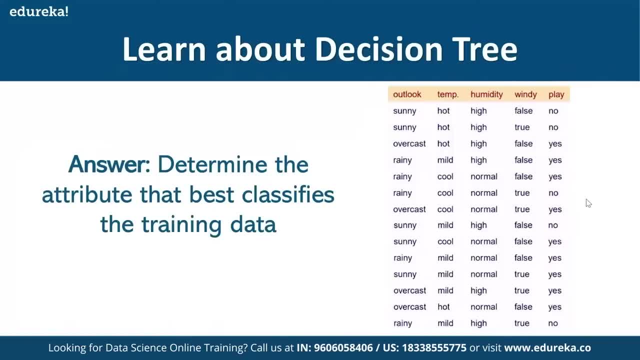 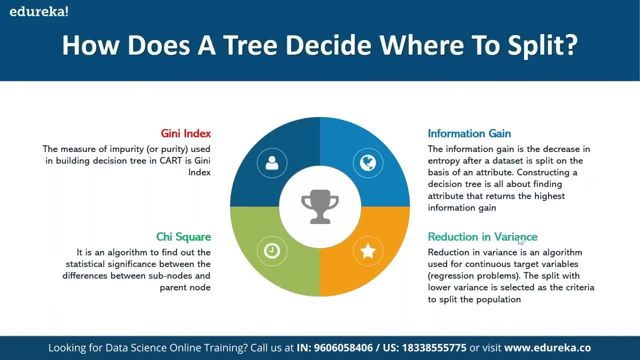 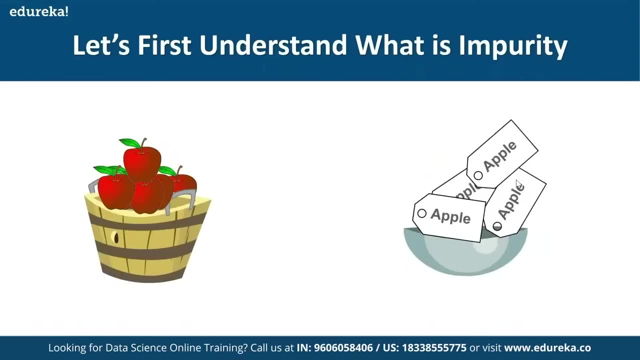 right. So now what I'll do is: from here is We. I will illustrate you What is genie index, What is information gain and how does this happens right, And this is basically used to build your decision tree. So, before I make you understand about genie index or information, 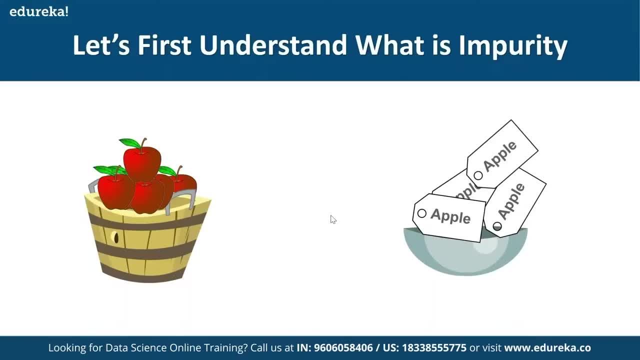 gain. one thing which you should always remember is to understand the concept of impurity. What is impurity? impurity is nothing, but you can see there is a basket, You have apples right now. If you have a basket which is of Apple and another tray it. 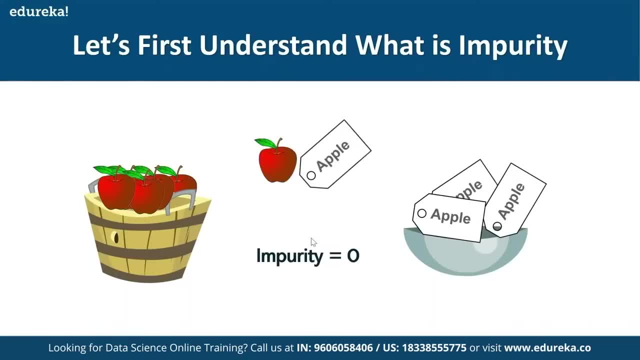 is written the label as Apple. Now, in this case, you will never make a mistake. You will never make a mistake because here you have an apple, here You have only one label, So everything will be perfect, It will be 100%, basically. 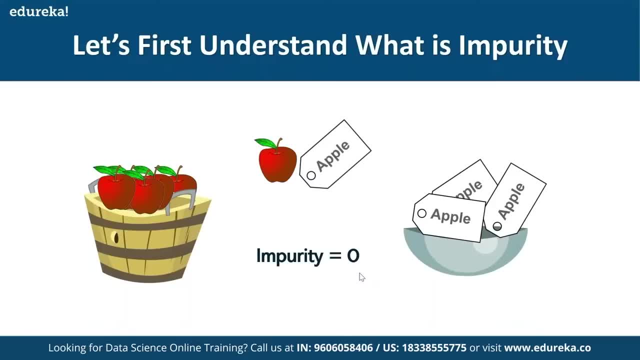 There is no impurity, There is no problem in your data set right. on the other hand, Let me flip the story in this case, Imagine that I have different fruits in the basket, which is like Apple. You have a banana, You have a grapes. 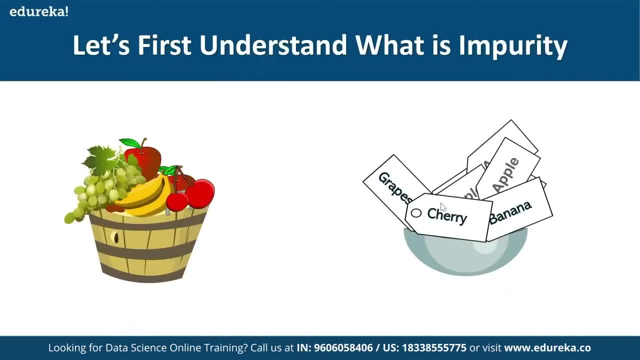 You have a, you know cherries and many other things, right, and you have many apples, many labels here in this case. Try imagining you have to match each fruit with its label right now. in this case, the impurity cannot be equal to 0 the impurity. 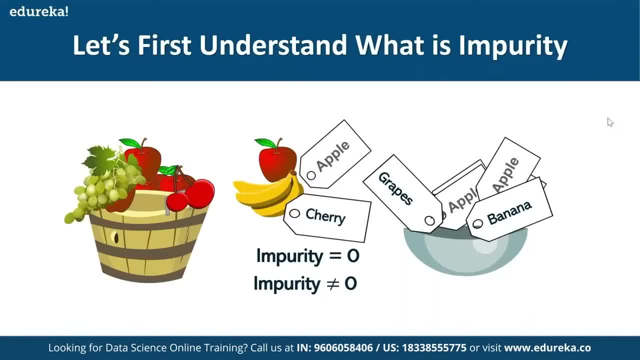 will not be equal to 0 in this case, because what would happen here is that you have a chance Is of misclassification. right? This is a very important concept. right, when you have perfect thing, the misclassification will not happen. But whereas if you have a multiple labels with multiple fruit, 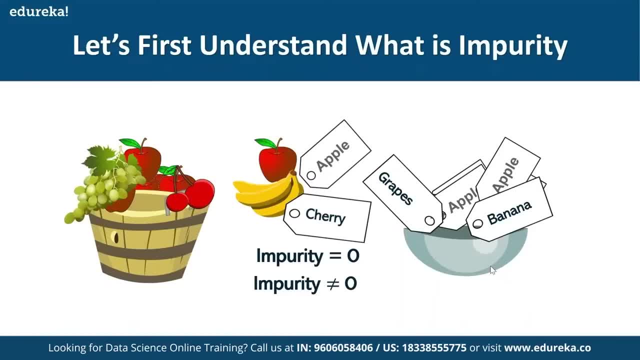 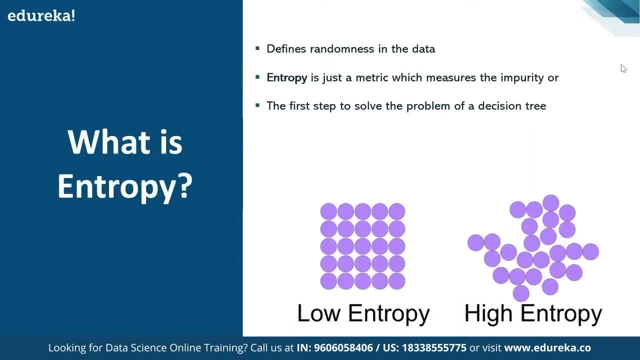 misclassification or impurities will not be equal to 0 right. So this is associated with a term called as entropy. Maybe in your childhood days you have learned about entropy in your chemistry class in a simple sense: What is entropy? Entropy is a randomness. 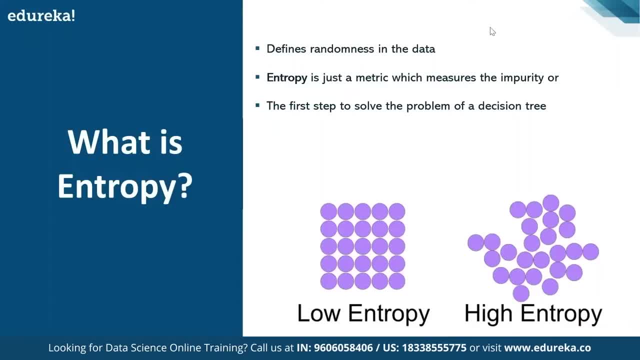 Of the space, sample space. whenever you are not sure on your decision, then entropy will be more. imagine that I'm giving you the data set where it is like: 51% of doing this thing, 49% of not doing this thing, 51% chance at the employee may leave the organization. 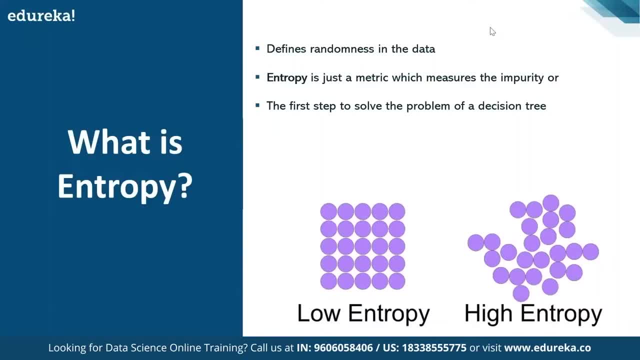 49% chance that employee may not leave the organization. So, basically, you are not sure on your decision. If you are not sure on your decision, then the entropy will be very high on the other, And if you are very sure on your decision, then the entropy 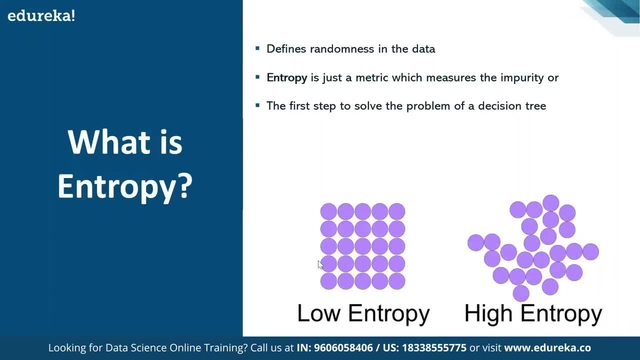 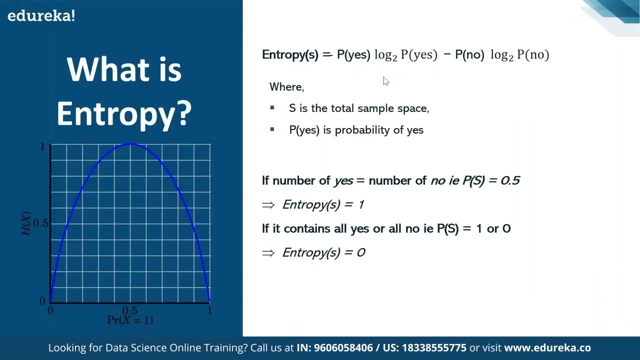 will be very low. So basically, we need that feature which can provide us lowest entropy rather than the highest entropy to select as that as a good feature. So we generally find it out entropy by the help of this formula. What we simply do is: don't get scared with this formula, because 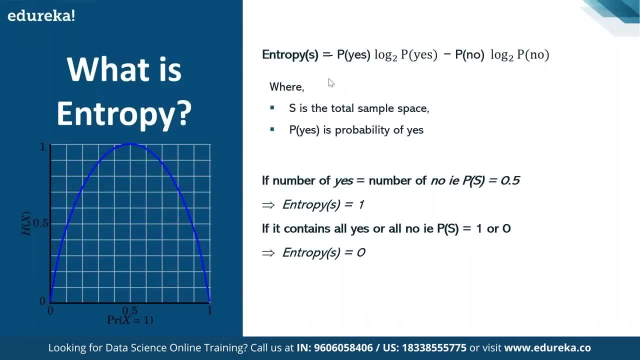 everything happens automatically in our or python right. imagine. just look at this formula. What is this formula? This formula says that what is the probability that something will happen? x log base 2: probability that something will happen. subtract this with probability that something will not happen into log. 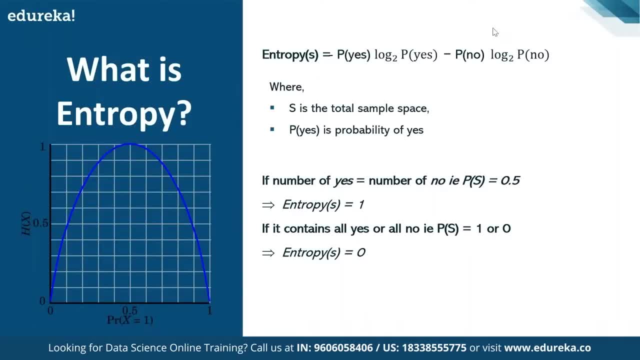 base 2 probability that something will not happen. Okay, let's take up an example. Don't worry about it. Let's take up an example: that probability that I will win the match, you will apply here. and probability that I will not play the match or win the match, you will apply here. 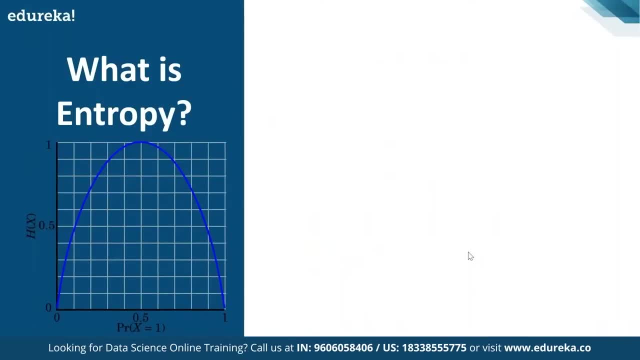 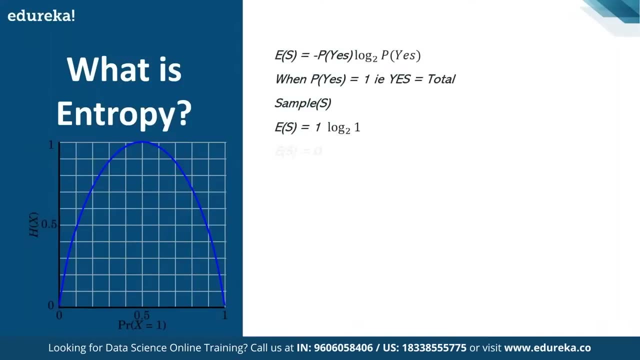 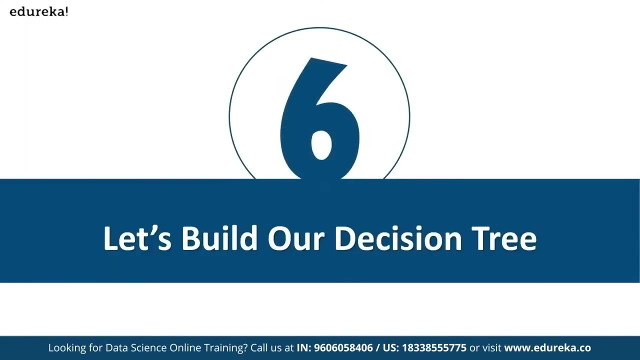 and then you will calculate the entropy. Let's take, you know, an example: how you can do this in our case. So, in our case, let me show you, Yeah, how we will build the decision tree in our case, in our case, You just see here. 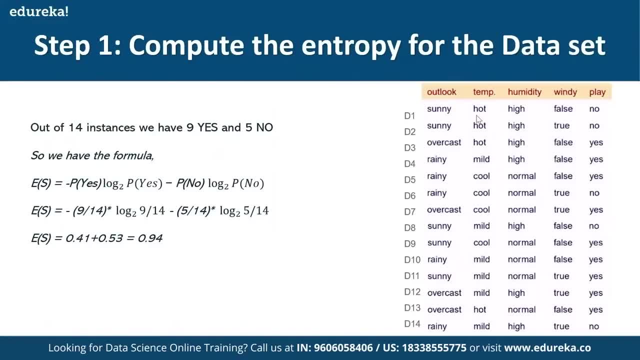 What is happening is that we have 14 instances, Or 14 rows of the data set, where nine times, If you see it, I will play the match and five times I will not play the match. Okay, So, if you see carefully, there are nine labels where I'm playing. 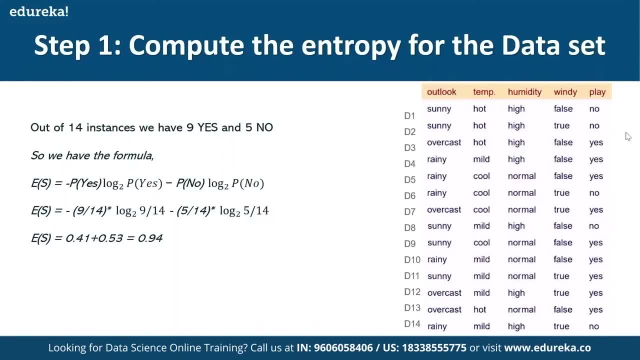 the match and there are five levels where I'm not playing the match right. So first of all I have to find it out the total entropy. how I will find the total entropy? This is being determined by probability that I will play the match. 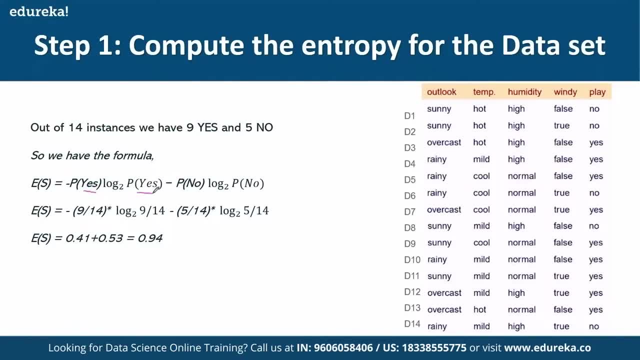 sub. multiply this with log base, power 2: probability that I will play the match. What are the chances that I will play the match? 9 out of 14?. All of you will be with me, right? This is 9 out of 14. multiply with log base to 9 out of 14 subtract. 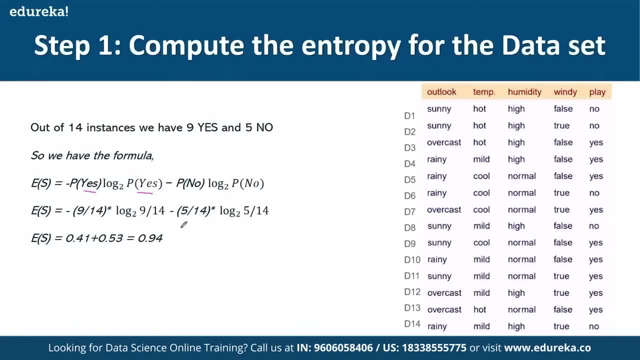 this with: what is the probability that I will not play the match? 5 out of 14. multiply this with log base to 5 out of 14.. So once you calculate this, you will find it out the entropy of this entire system. Entropy: 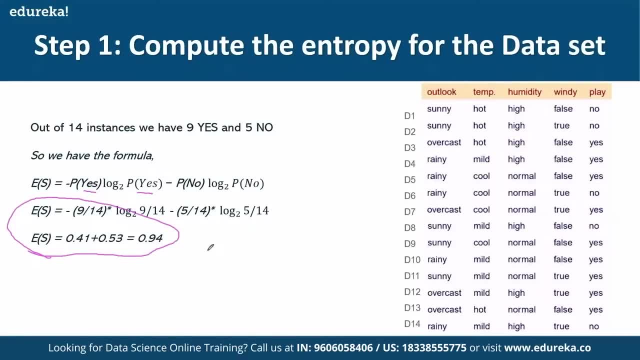 Of this entire system is 0.94.. Okay, So this is the entropy of your entire sample space. This is the first thing. now, how this entropy will help you in selecting which features you will take or not. So let's go further. 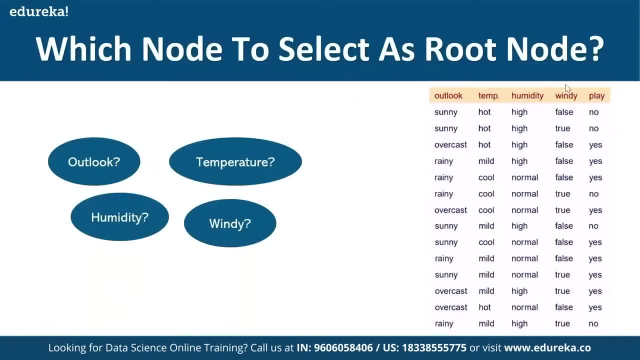 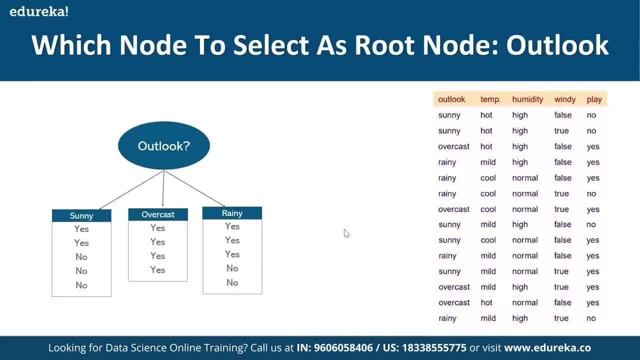 So now we will take each feature one by one: whether I should take Outlook, whether I should take temperature, whether I should pick up humidity, or whether should I pick up windy right, Let's go one by one now. First I'm plotting for Outlook. 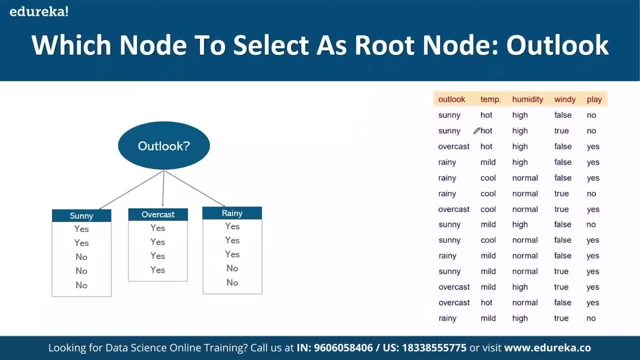 Imagine for Outlook how many times. so what are the distinct value of Outlook? Outlook can be sunny, Outlook can be overcast or Outlook can be rainy. right, These are the three different combinations you can have for Outlook. Now, if the Outlook is sunny two times, I'm playing three times. 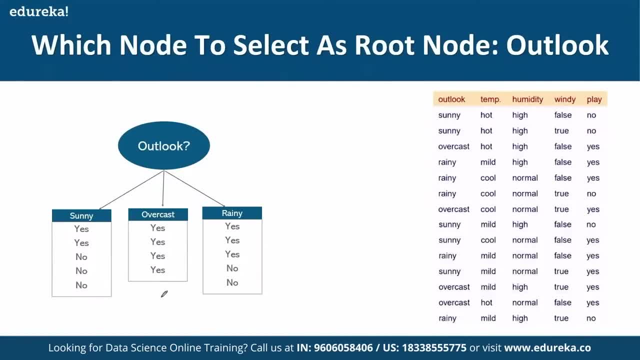 I'm not playing the match if the Outlook is overcast. I'm always playing the match if the Outlook is rainy: three times. I'm playing two times. I'm not playing the match. right? This is how I have bifurcated. 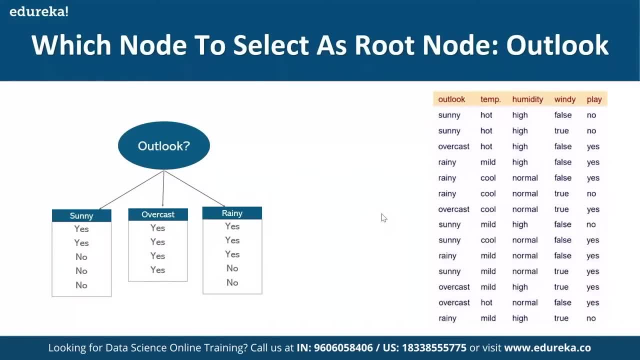 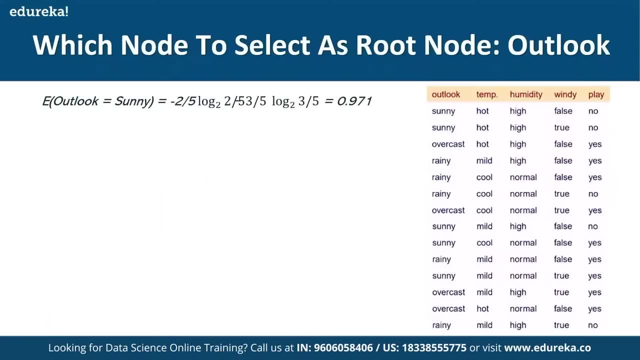 What I will do in the next iteration is, let me point it out, the entropy of Outlook. Okay, so, if we start with Outlook, remember this formula, which is, you know, probability that I will play, multiply with the probability that I will play right and subtract with probability. 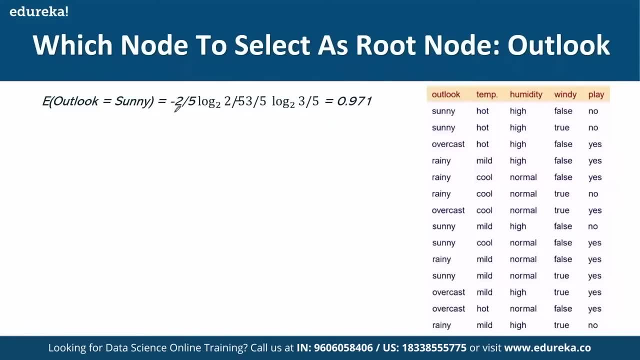 which I will not play, and log base 2 of not playing. So 2 by 5 is the chances that I will not. I will play into log base 2, 2 by 5.. This is a subtraction Here, right with I will play and log 3 by 3 by 5.. 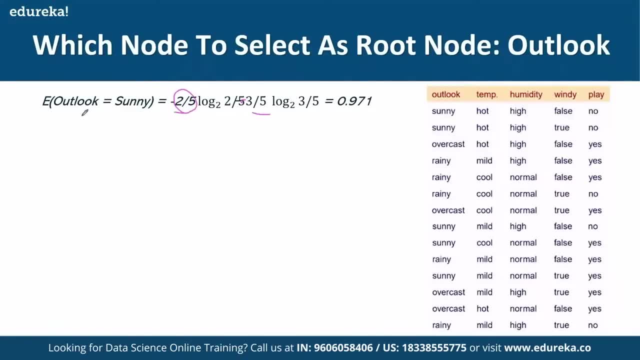 I will play right. So you will calculate this entropy when Outlook is sunny. Yeah, so you got this. entropy when the Outlook is sunny is point 971. accordingly, you will proceed with calculating the entropy when the Outlook is overcast. Outlook is overcast. 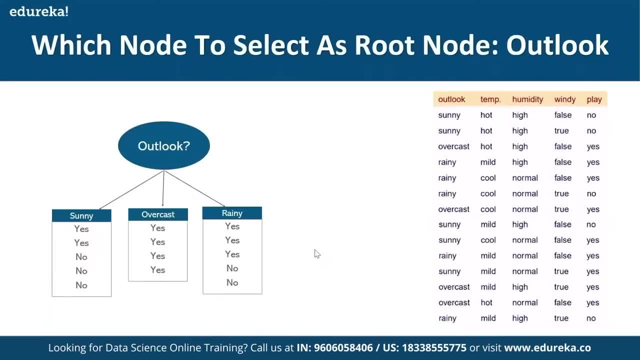 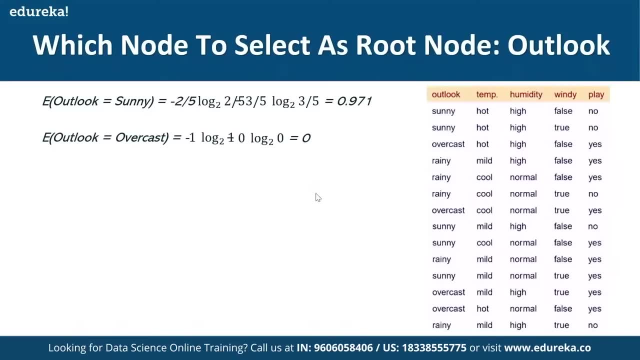 always you are playing right. if the Outlook is overcast every time you are playing, So means that you will get a probability of 0. if you apply in that formula, you will get 0. and third, what, what? what would happen if the, if the Outlook is sunny? in that case you will. 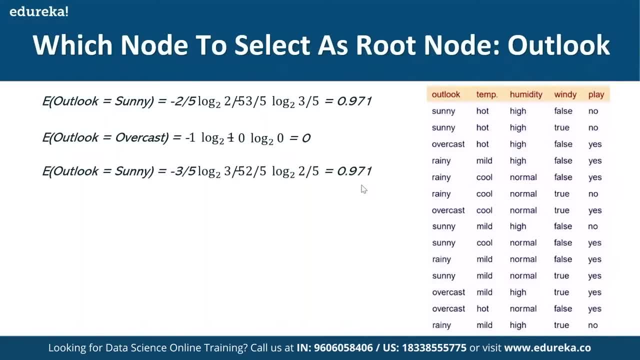 again, multiply and you will put the formula and you will get it out- point 971,. right, So you will find it out. entropy for each and every distinct combination of your feature. You got my point right: Outlook being sunny, Outlook being overcast, Outlook being sunny. 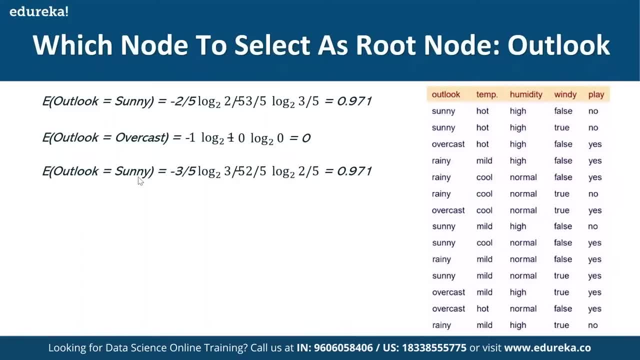 You know, overcast, sunny and rainy. This should be replaced here, right. and then what you will do is you will finally calculate the information gain. information gain is nothing, but what you will do is you will pick it up the chances, you will pick it up the entire chances when you 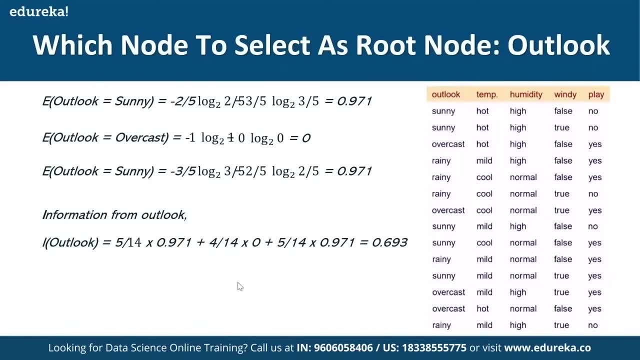 are playing right, which is 5 out of 14. you remember 5 out of 14 were the total chances that I will play into. if it is sunny, plus 4 out of 14.. If it is overcast, 5 out of 14. if it is rainy right and you. 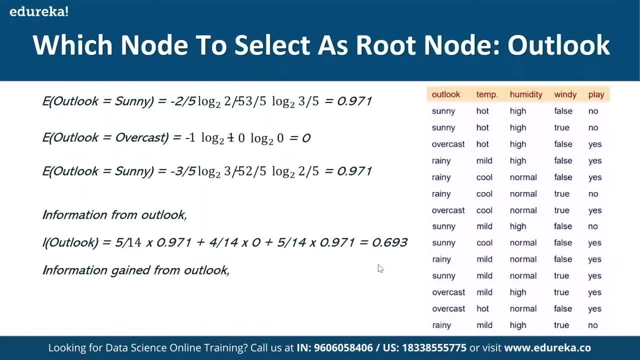 will calculate the information from this Outlook and once you calculate the information, you will subtract this information from your total entropy, which I found it out in the last slide, which was 0.94. you will subtract this and you will get the information gain, or this is also called as a information gain. 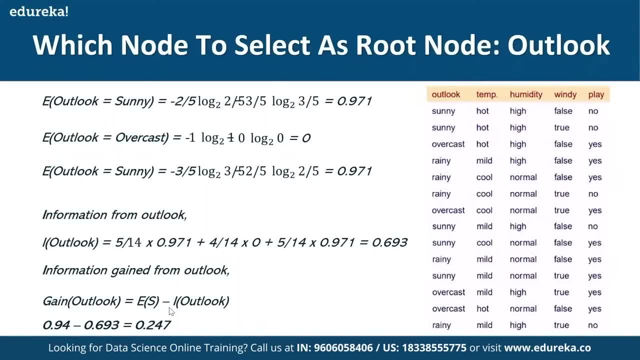 from a particular feature. So, basically, these type of a calculation. first of all, don't get scared The way that you have to do this calculation, but what I'm trying to explain you is: this is how your algorithm will work for each and every feature. 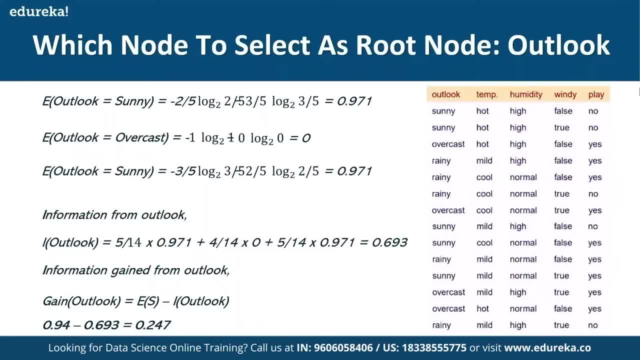 It will calculate the information gain from your feature. Right, if you have the more information gain, it means that this variable is of very, very important in predicting that something will happen or not. Okay, so for Outlook, I got the information gain as 0.247 with 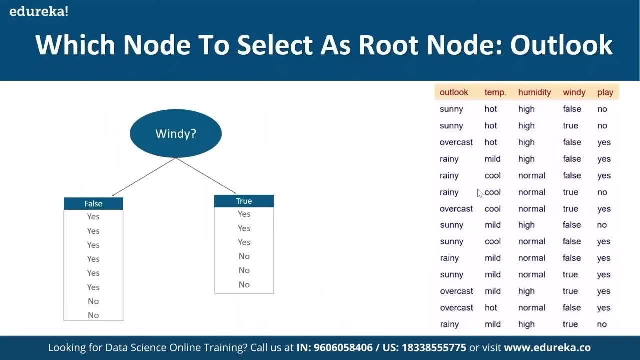 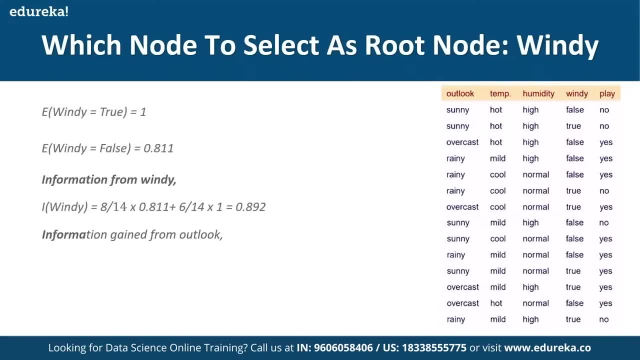 all the calculation, Remember. then we will proceed with wind, if the wind is there or not, right, and then I will proceed with wind and I will calculate the information gain and say information gain I found it out is 0.048. Right. 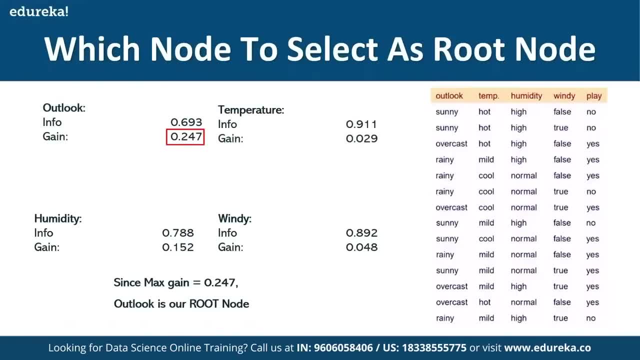 Similarly, we will calculate for all the four of them. Let me put it together for all of you. So this is what happens here Now. if I put in front of all of you these were the four different variable, I have Outlook. 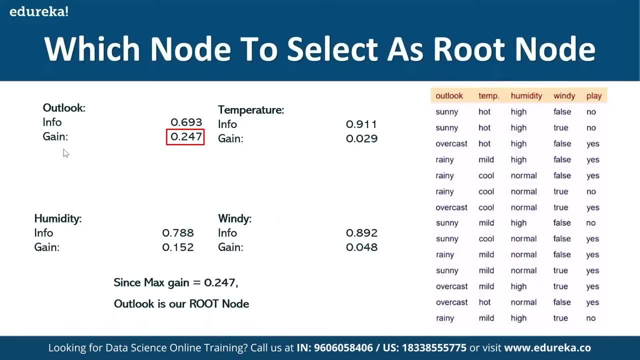 Temperature, humidity and wind. right, I am calculating the information gain for each one of them, and the information gain I got for Outlook is 0.247.. So if the information gain is highest in a particular feature, that feature will become your root node. You got my point. 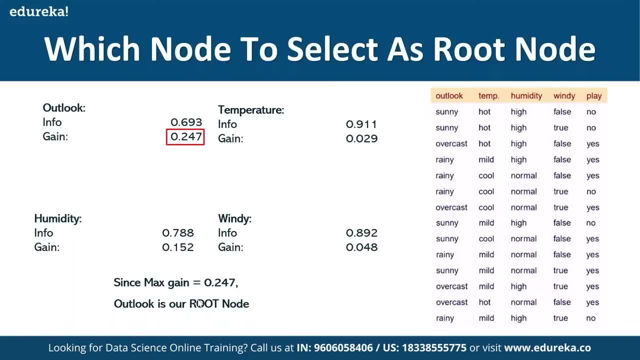 So therefore we will pick it up- Outlook as our root node, Similarly for when the tree get started, later on, as a branch node Also, your information gain will be calculated and wherever, whichever feature is giving you more information gain, that will be picked up later in the. this is your tree also. 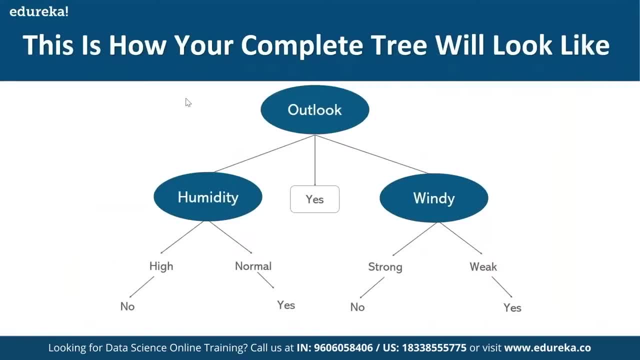 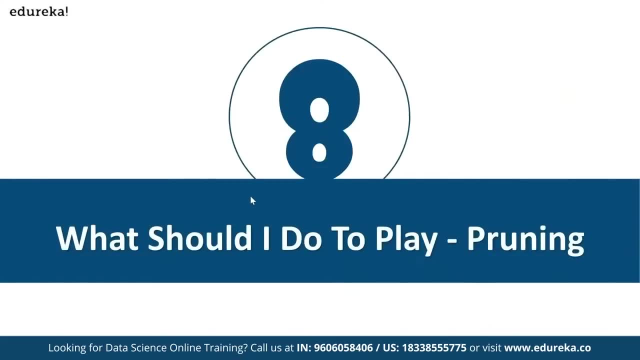 So this is how you will build your decision tree, and you will finally get a decision tree like this. Okay, So now what I will do is you know like I will quickly show you how do we do the decision tree in your python. 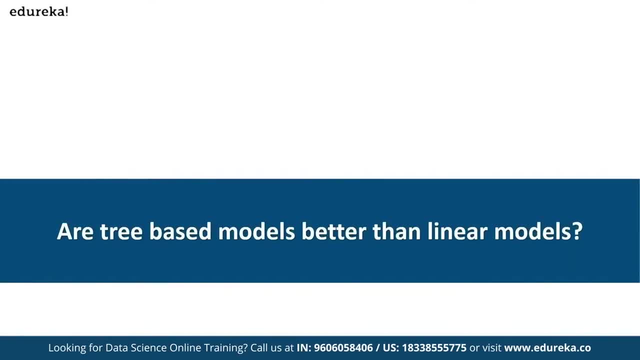 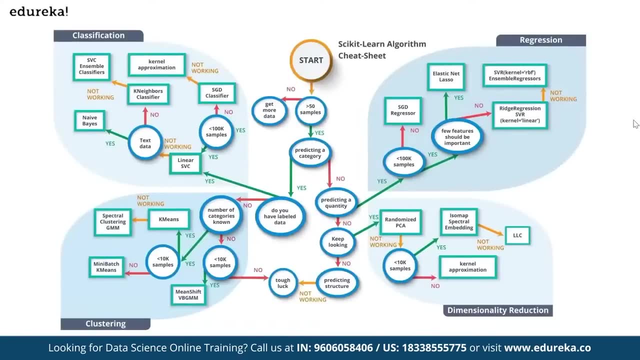 Okay, so I'll show you how do you do this in python and then I will Summarize for all of you that why decision trees or tree based algorithms are better than your other algorithm. Okay, so how do you choose, basically, that which algorithm? 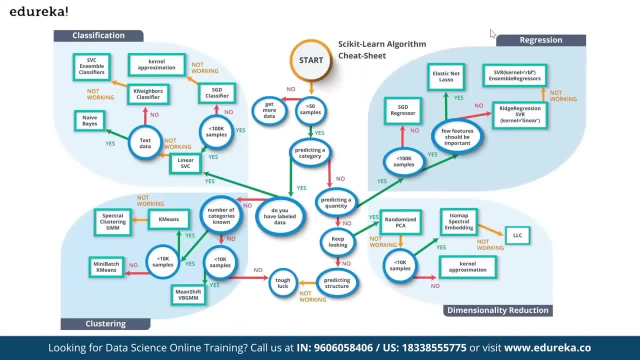 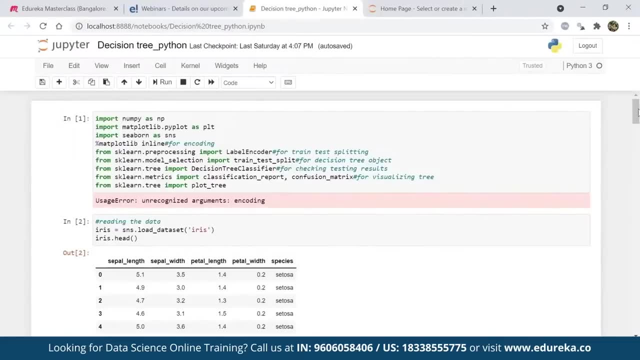 you will select and when. okay, so I'll describe you this, but before let's jump on to python and go there. So what I have done here is like I had built the decision tree in front, like you know already. so quickly I will. 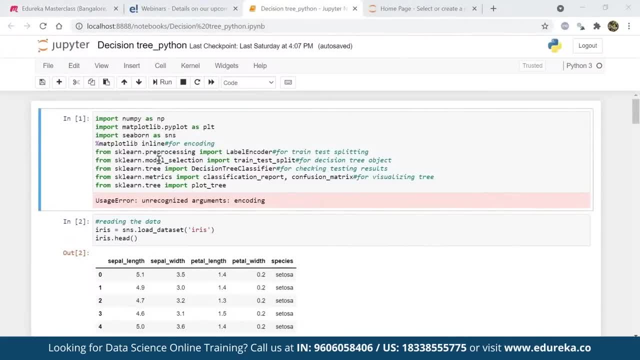 Check you through the commands. Okay, So what happens here is that in python- as you would be well versed with this- that we generally import packages in python. So I'm importing numpy, I'm importing matplotlib for plotting the chart, I'm importing various packages from your sklearn, which is for 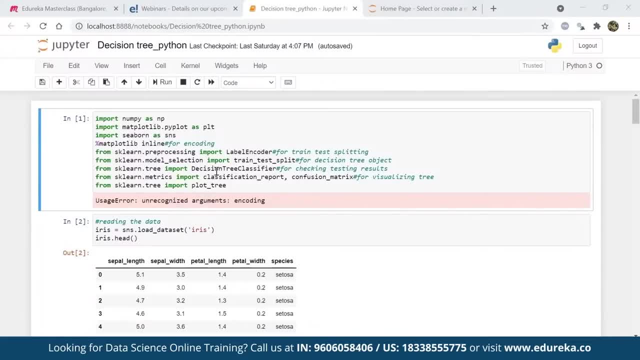 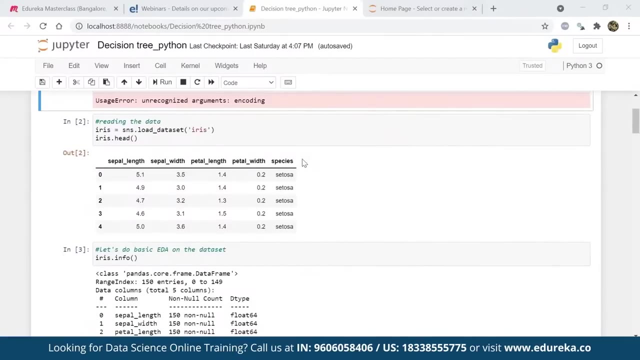 machine learning purposes, right, So I am importing your label and quarter your decision tree, classifier, classification report, and I also I'm importing your decision tree. right, So we have all this, which I am importing right after I import, what I will do is I'm reading my data set. 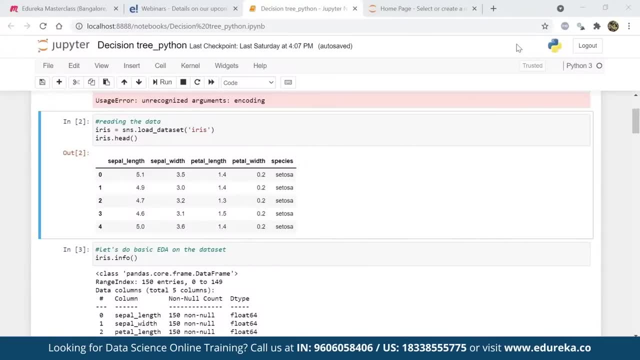 So I'm showing you this with the help of our iris data set, which is one of the very popular data set for building the decision tree rights for any particular source. So imagine that this is my data set and I'm just showing you six rows of the data set where you know like I want to find. 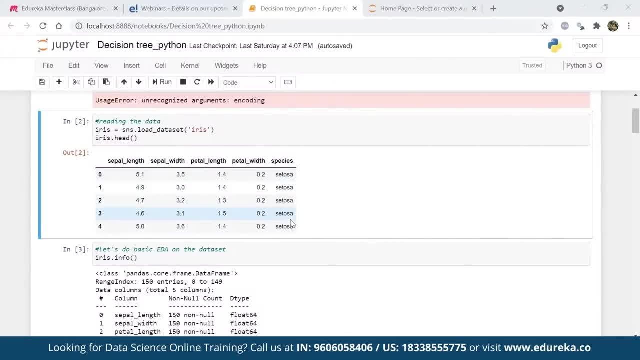 it out whether a particular flower species will be sitosa versicolor or virginica. I have three different flowers which I want to predict, and on the basis of sepal length, petal length, sepal width and petal width. So basically, I have different dimensions of flowers. length: 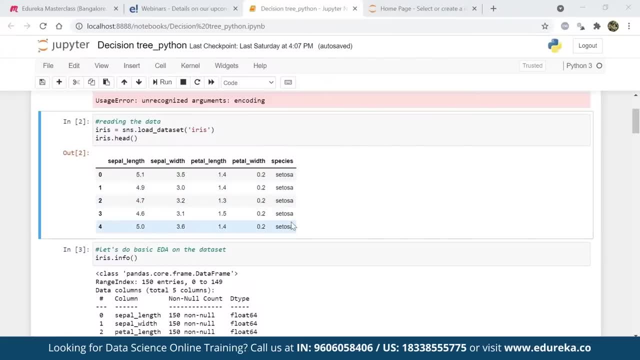 and width and, based on that, I want to find it out whether the particular species will be sitosa versicolor or virginica. You got my point right. So this is a data set. So what I will do is I, as you know, with every machine learning. 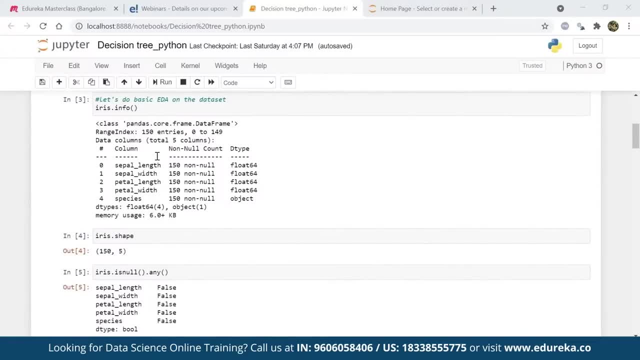 data set. we play with the data set, So I'm checking the information here. I like what type of the data type it is. So sepal length: it is a float, petal length: It is a float and species is a object. Why object? because this is a categorical column. 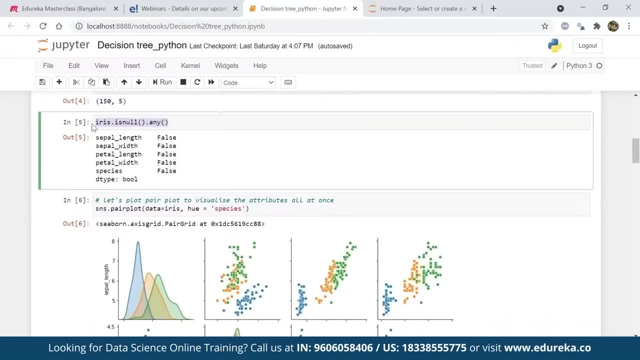 So after this, I'm also checking whether there is any null value present in the data set or not, because if there is any null value, then we have to get rid of that null value or we have to replace that null value with some imputed value, right? 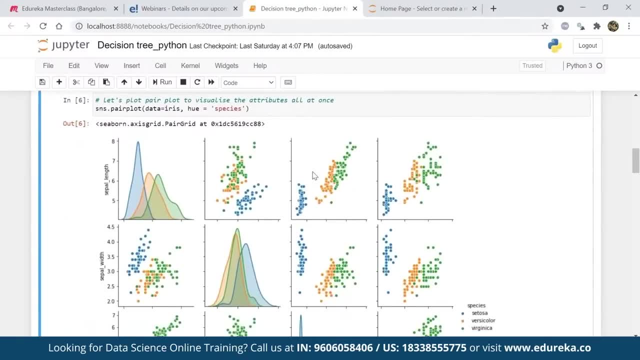 This is what I'm checking here. Once I do that, I'm also plotting this, Because we usually do visualization right to understand the data set better. So what I'm doing here in the, with the help of SNS, which is your SNS dot pair plot. 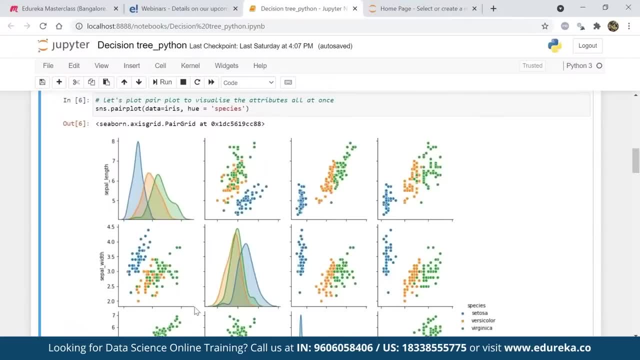 I'm plotting all the possible plots. So basically, sepal length with sepal width, what type of the combination look like? so, sitosa, versicolor and virginica: There are three different species You can see in the data set and this is what I'm getting: a trend. 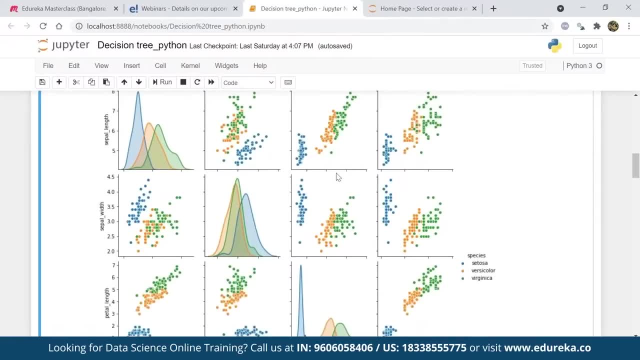 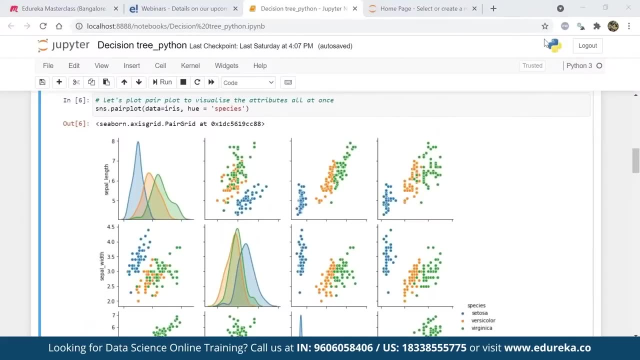 between your sepal length and sepal width. Similarly, This is basically from sepal width to petal length, right? So this is how I am understanding the patterns, or I'm understanding the relationship between the variables in the data set. So this is what I am understanding here. 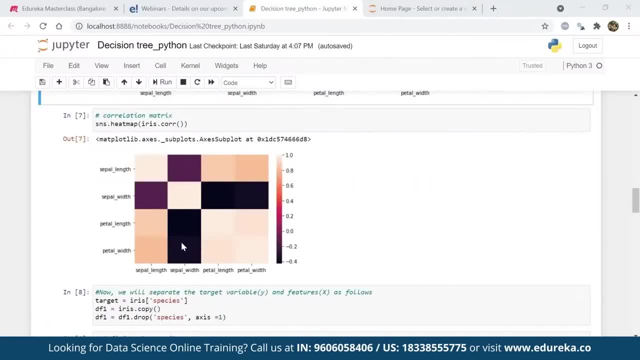 I am also checking whether there is a correlation or not. higher the shade It means there will be a strong correlation. So all of these things is being done as a part of exploratory data analysis, before even you start your machine learning model, right? 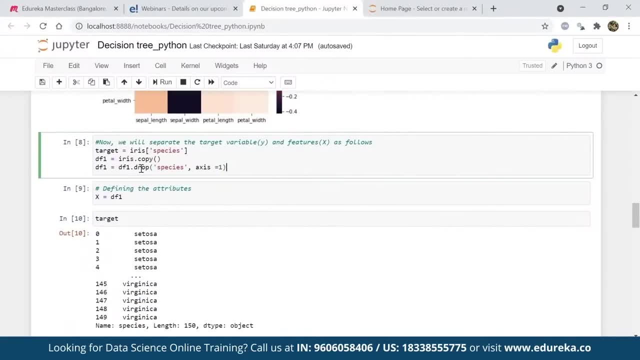 Once you do this, after that, what I have to do is, after that, what I'm trying to do is I am taking your species column, what I want to predict, as my Target variable, which is your dependent variable and what I. so this is my the dependent variable and, with the help of what I want, 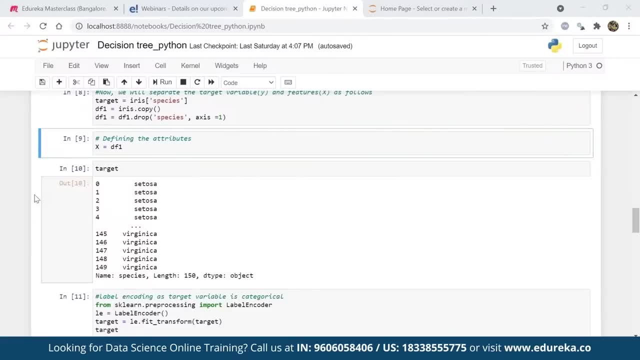 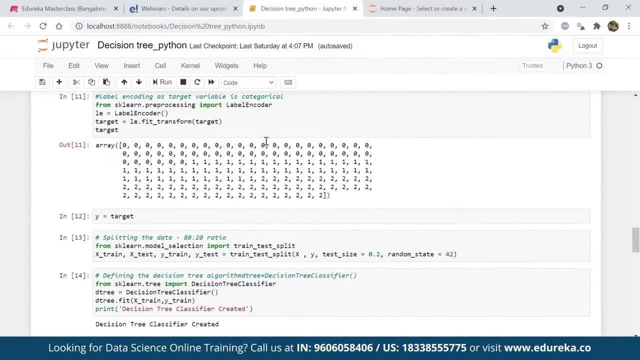 to predict will be my independent variable. So I'm calling X all my independent variable and I'm calling target as my dependent variable. Once I do this, then you will also think about it at your. the variable which I want to predict is the flower species, right? 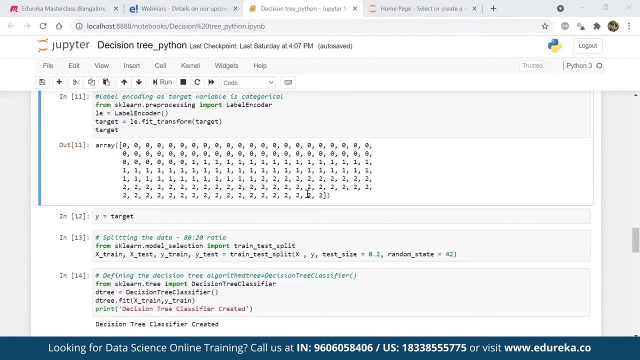 But I want to convert this into 0 and 1 class, 0, 1, 2 class, because your computer cannot understand text, right? computer can only understand the numbers. So what I am doing here is I am changing it to the, I'm changing it to the class. 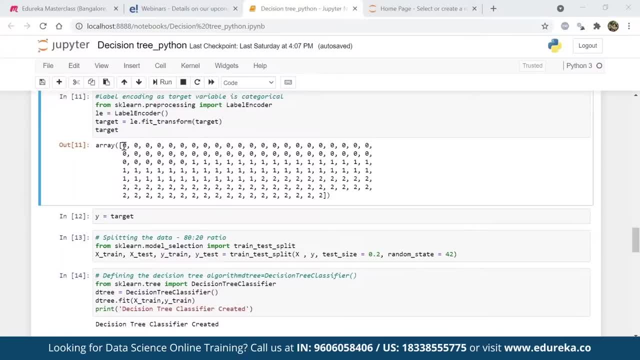 Right. So what I am trying to do here is I am saying: wherever it is sitosa, it will become 0, wherever it is virginica, It will become 1, and it is versicolor, as a third category to become 2.. So now imagine my data set, my label to predict, becomes 0, 1 or 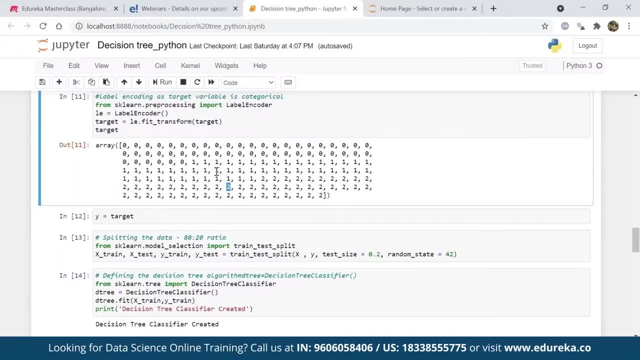 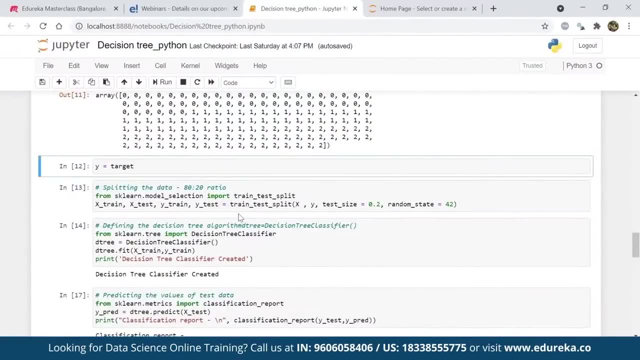 2 instead of 3 flower, which was sitosa, Tosa versicolor and virginica. This is what I am doing with the encoder here. Once I convert this and this become my target, What I will do is I, as I told you, that I will split this data. 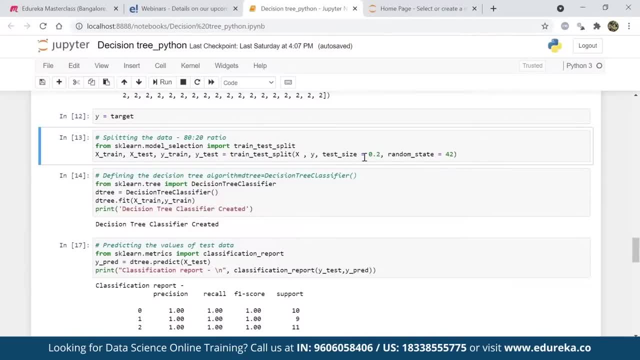 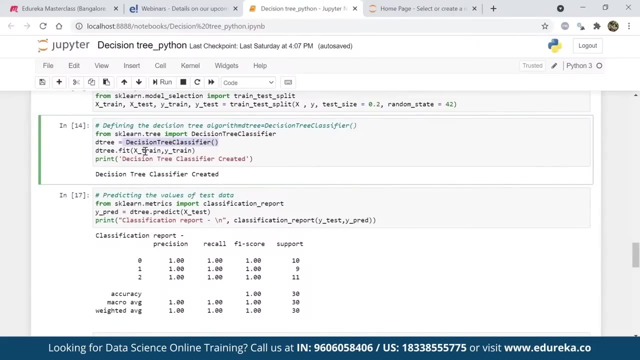 set into training and test data set. So basically, 80% of the data is going into the training data set and remaining 20% I am taking as a test data set. Okay, now I will call decision-free classifier. you know like I want to make our decision tree and I want to fit this. 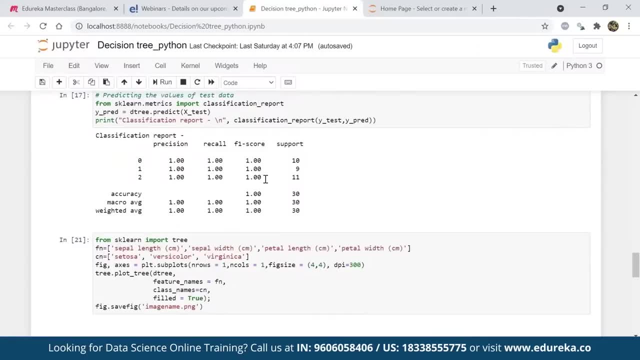 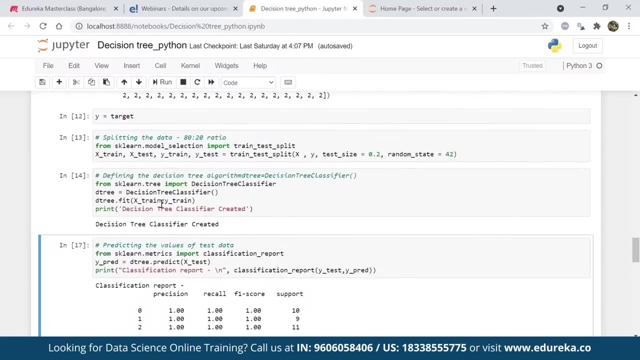 on my training data Set and the test data set and I will start building the decision tree and, with the help of you, know from. so here is when I have created the decision tree and here is when I am checking the prediction: how accurate my decision tree is. 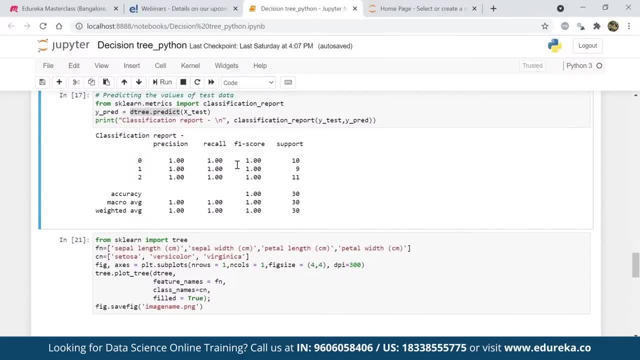 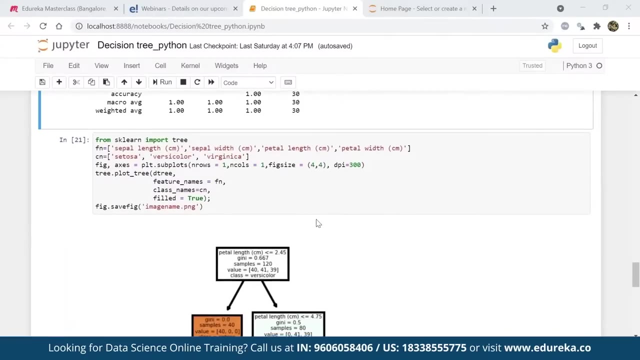 So I got my precision, which is good, I got my recall, I got my f1 score and I also get the support right. So all these matrices are being used to calculate your, how accurate your predictions are. so higher the precision, better The results would be right. and finally, I am showing to you 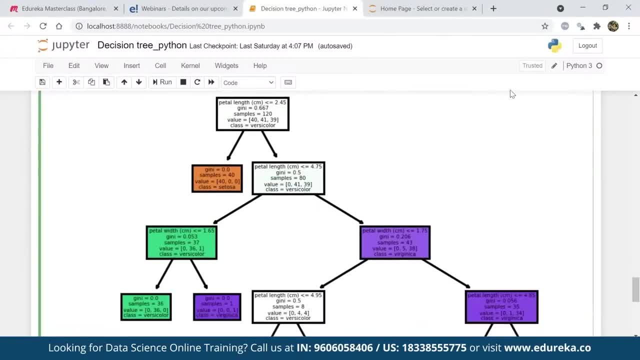 that? how does the tree look like? so I had tried to plot this decision tree in front of you. So basically it start with Peter length and you can see the Gini index coming up here, or the information gain, which is information gain and Gini index are reciprocal to each other. 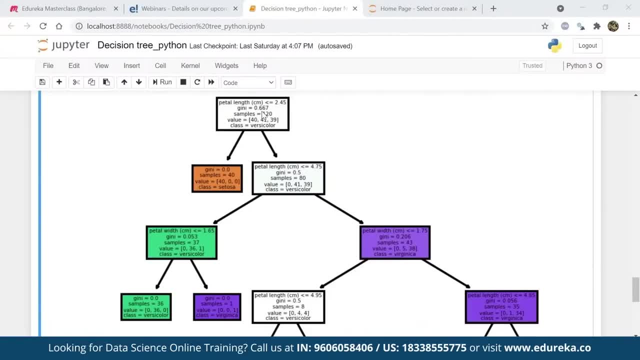 If you want to use information gain, you will get that score. If you don't want to use information gain, you will get Gini index. So they are both reciprocal of each other. It is one and the same thing. you use Gini index or you use 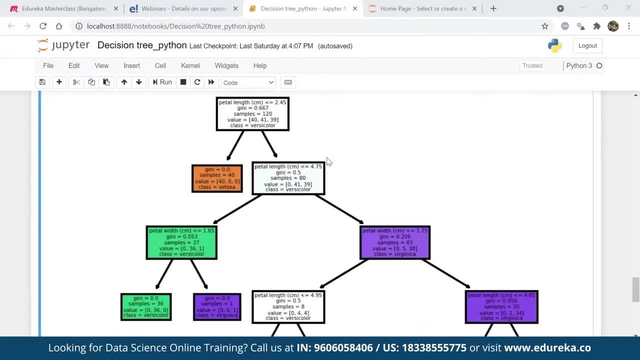 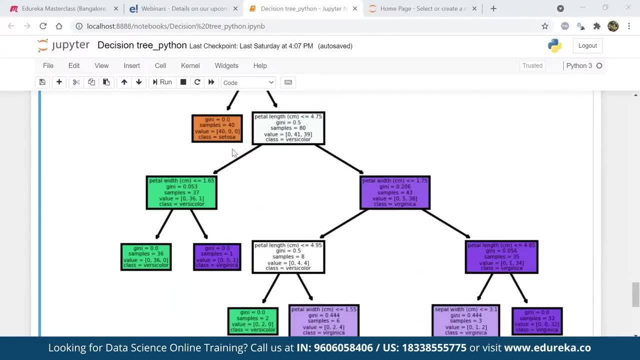 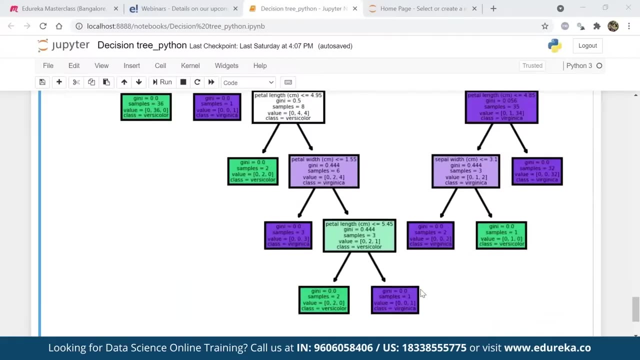 information gain. They are the two different metrics to build your decision tree. So you can see that, based on a Peter length, the tree gets splitted like this: then, based on the Peter length of different dimensions, your tree further split, then it further split, then it further split. and finally, you get to know that, whether the 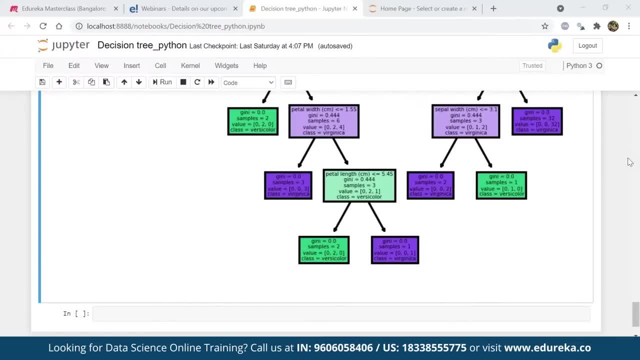 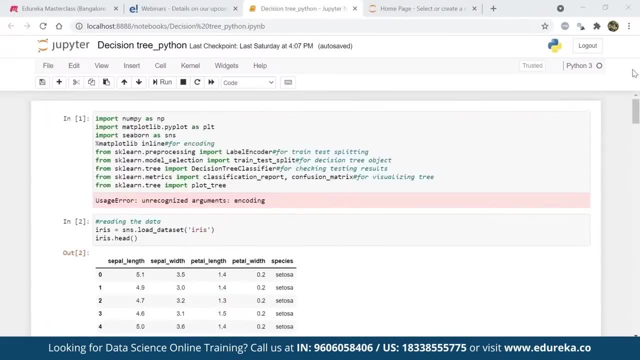 particular species will be versicolor or virginica. Okay, so this is how your entire decision tree is built in Python. Okay, so this is how it's so simple. I know it takes time to build this thing, But once you are a good data scientist and you understand all. 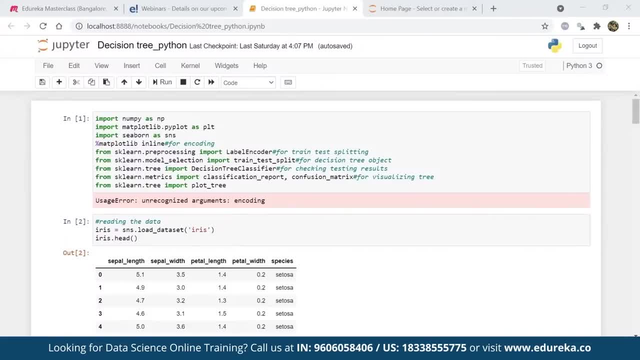 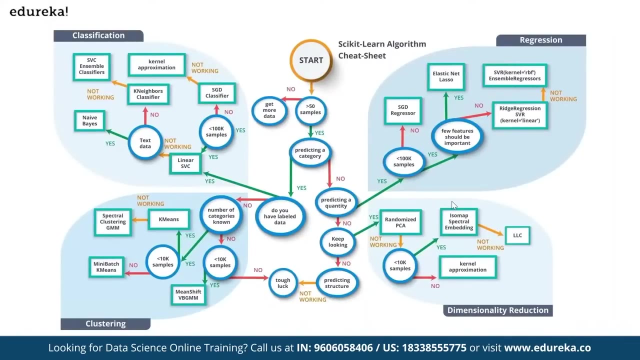 these things. it is very simple to build all these things very easily in Python, or are right? So now, finally, going back, how would you decide? how would you decide that? which algorithm? you know which algorithm will be taken when? so What happens is? this is on the basis of scikit-learn. 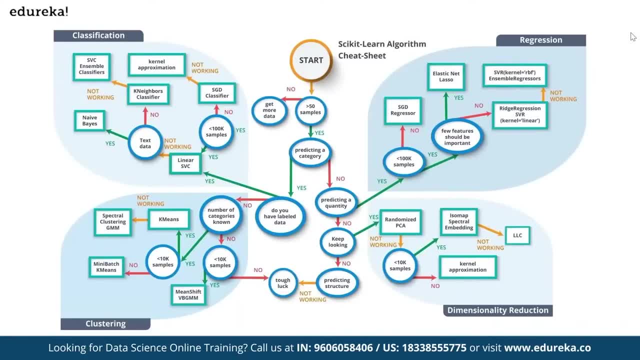 So it starts something like this: Okay, so it is on the basis of like this that, first of all, you see here that, whether how many samples you have, how many data points you have in the data set, right, If you have more than 50 samples, then you will go here. 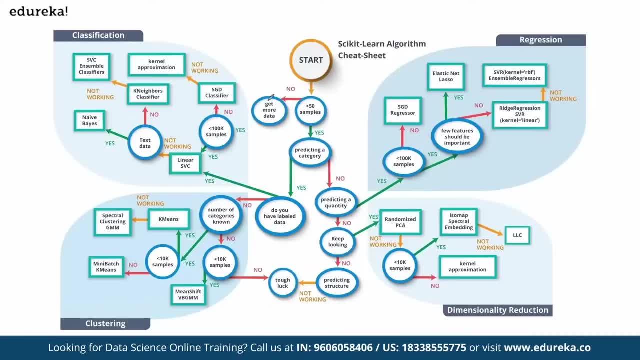 If you have less than 50 data point, then you know you will go here, So you will get more data set right. So if you have more data, If you have greater than 50 data point, then you will go further. 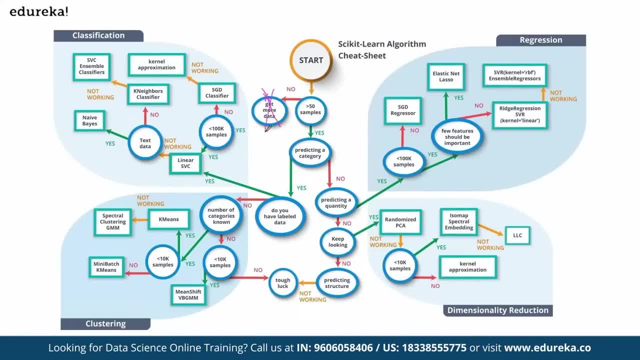 you split on your data set. If it is not, then you will. you just the kind advice: it get more data set. Okay. so then you will decide at what you want to predict. If you have a label data set, then you will go here right and 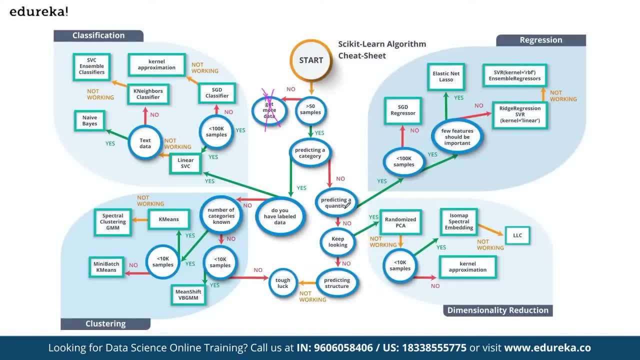 do clustering. If you don't have the label data set, then you will see whether you want to predict a quantity. If yes, you will go in regression. If you want to predict, if you just want to do exploratory analysis, you can do dimensional reduction. 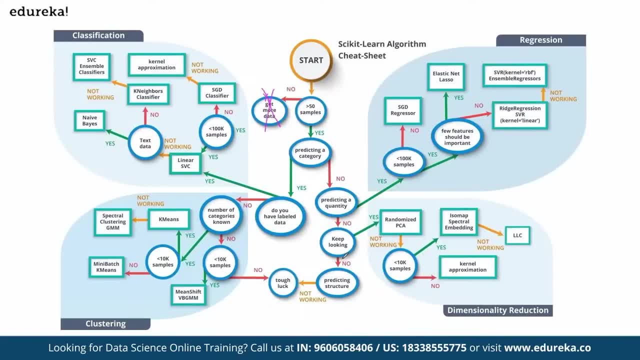 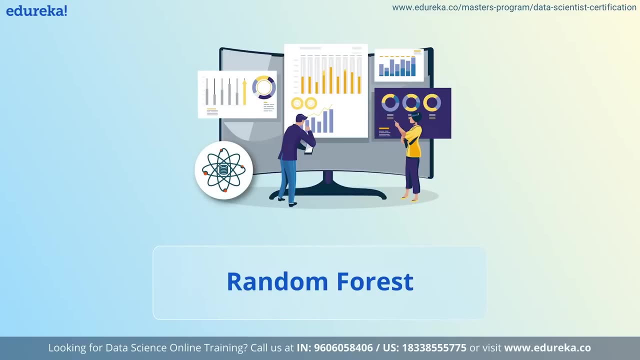 If you have a label, data set, you know, for classification, you can do all this classification. So, basically, this is a cheat sheet which we generally use to decide that what we have to do with the data set and when. So now let's understand what is a random forest? 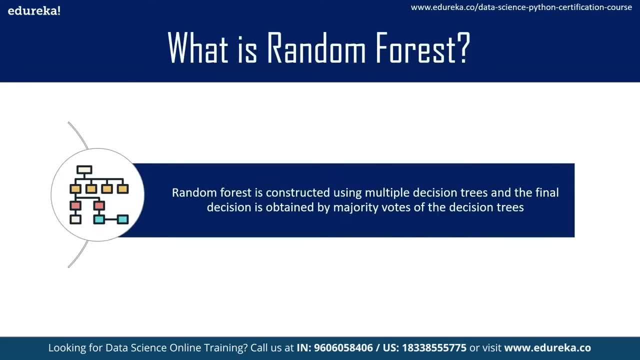 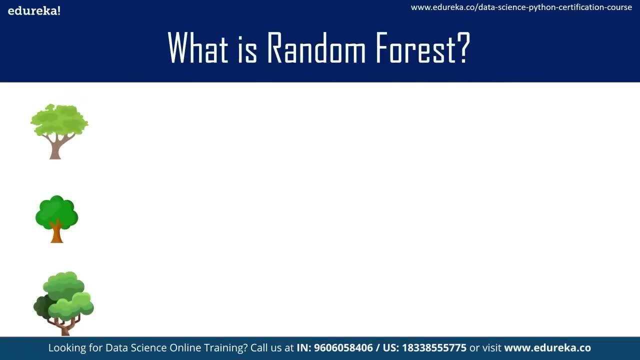 So random forest is constructed by using multiple decision trees and the final decision is obtained by majority votes Of these decision tree. So let me make things very simple for you by taking an example. Now suppose we have got three independent decision trees here. 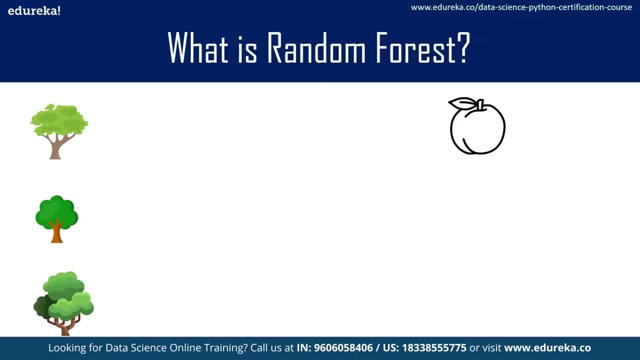 We are just taking three decision trees and I have got an unknown fruit and I want that these trees would give me a result of what exactly this fruit is. So I pass this through to the first decision tree, the second decision tree and the third decision tree. 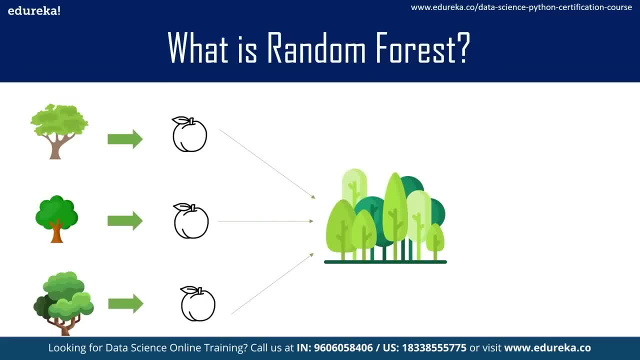 Now, a random forest is nothing but a combination of these decision trees, So the results are being fed Into the random forest algorithm. So what it sees is that, okay, the first decision tree classifies it as peach, The second decision tree says that it is an apple and the third 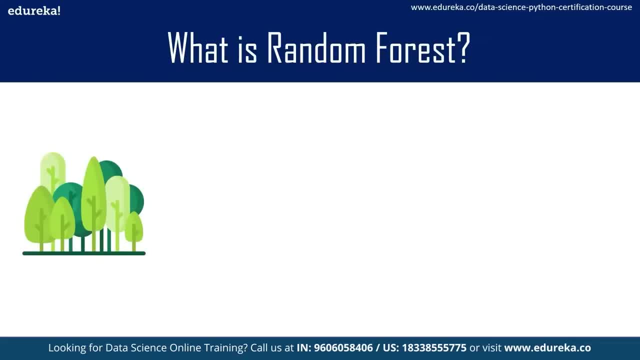 one says that it is a peach, So random forest classifier says that. okay, I've got the result as two peach and one for an apple, So I would say that the unknown fruit is an peach. All right, So this is based on the majority voting of the decision trees and: 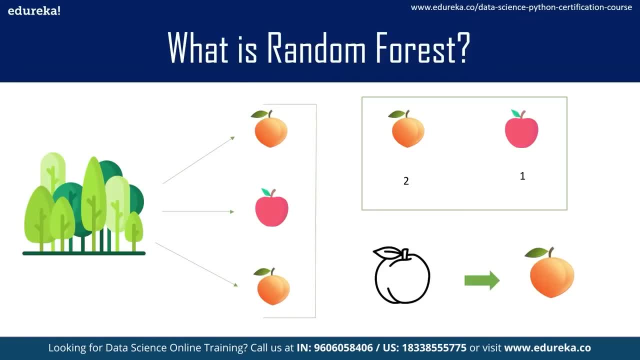 that is how a random forest classifier comes to a decision of predicting the unknown value. Okay, So this was a classification problem, So it took the majority vote. Now suppose if it was an regression problem it would have taken mean of it. Okay, 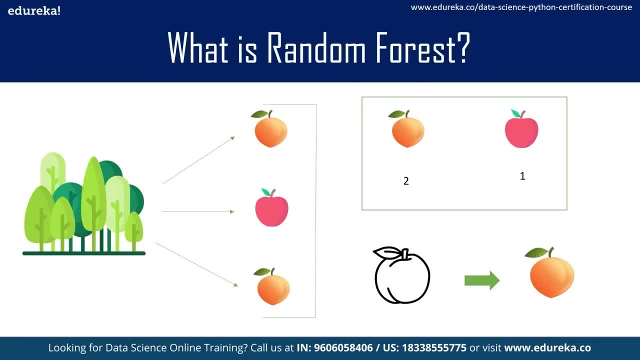 So now let's move on further to understanding what is a decision tree, But before that, we should understand that random forest. the building blocks are decision trees, and that's why studying decision tree becomes important, because if you understand one decision tree, We can apply. 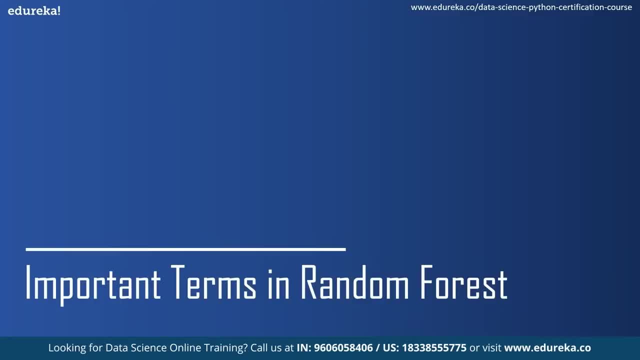 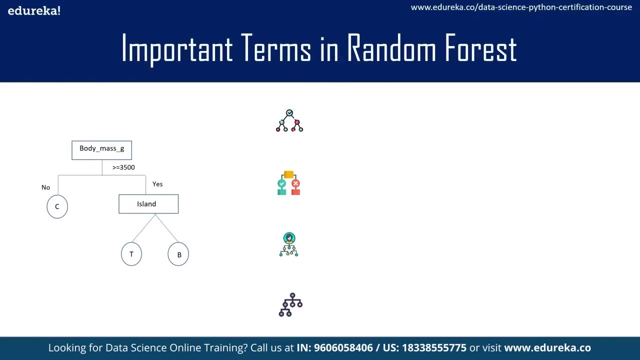 The same concept to random forest. So now let's move on forward and understand the important terms and random forest, and this will also help us to consolidate whatever we have learned so far. So we've taken the same small decision tree of the previous example and let's understand these are also the important terms which will 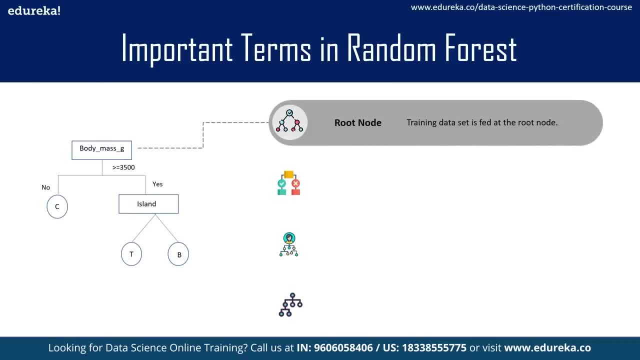 be relevant to random forest also. So the first is the root node. Now here, what happens is that the entire training data is being fed to the root node, and then we've got here that each node will ask either true or false question with respect to one of the feature. 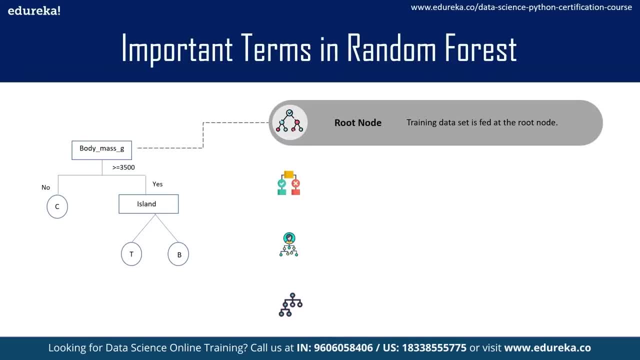 and then, in response to that question, it will partition the data set into different subsets. That's what it is It is doing here, based on the condition that if the mass body mass is greater than equal to 3500, it ask a question either. yes, 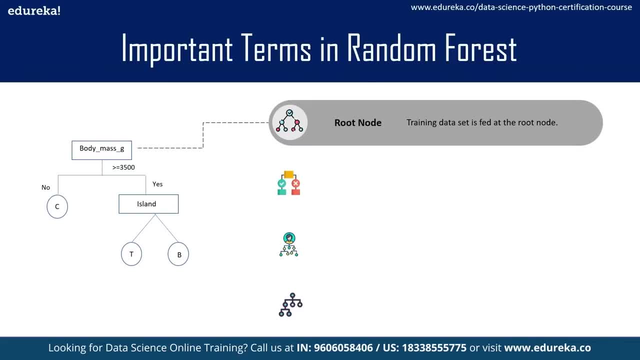 or no, and based on that again, for the partition is done, and if not, then it just classifies the species and then again what happens is that the splitting- now this is very important here- the splitting takes place either with the help of a genie or entropy methods, and 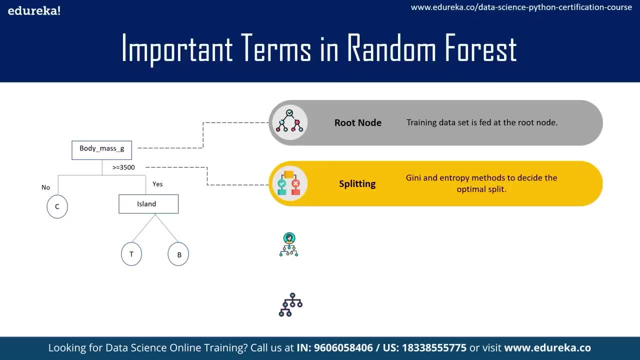 these helps to decide the optimal split, and we will be discussing about splitting methods very soon, right, Okay, and then we've got the decision nodes, which provide the link to the leaf nodes, and these are really important because then only the leaf nodes will tell us what actually the real predictions, or to 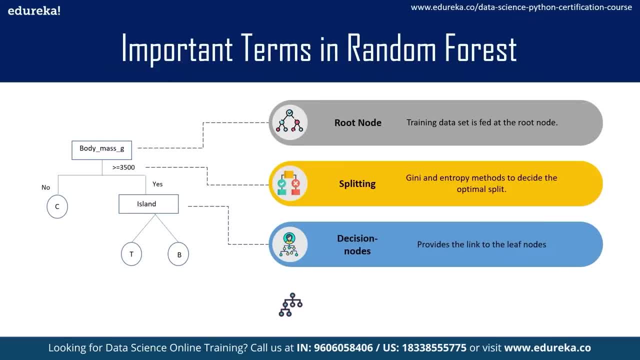 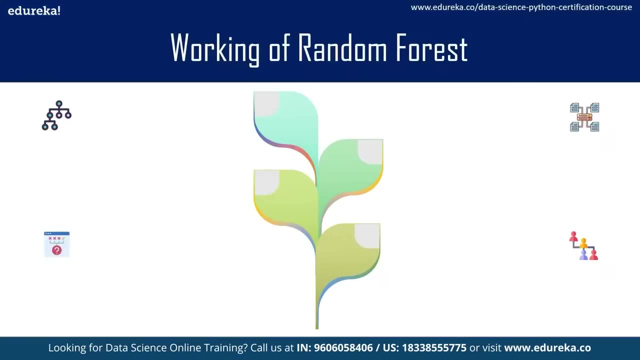 which class does the species belong? So now coming to the leaf node, and these are the endpoints where no further division will take place and we will obtain our predictions. Okay, So now coming up to another important thing here is working of random Forest. So now for working of random Forest. we will have to understand a few. 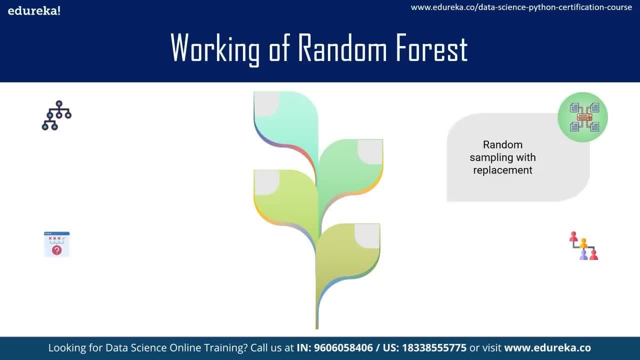 important concepts like random sampling with replacement, feature selection and also the ensemble technique which is used in random Forest and that is bootstrap aggregation, which is also known as bagging. So we will understand this with the help of an example which will be very simple, and then we will go on understanding how feature selection. 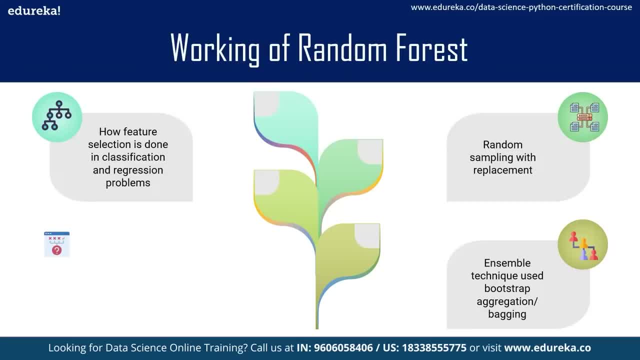 is done in both the classification and the regression problem. Actually, how random Forest select features for the construction of decision trees? Well, in random Forest the best split is chosen based on genie, impurity or information gain methods. So this also we will understand. Now let us first understand random sampling with replacement. 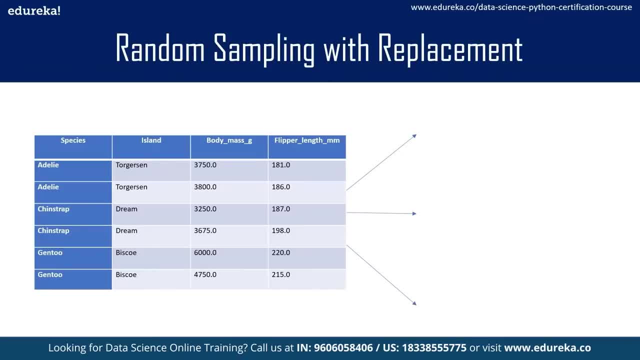 Now, what happens here is that we have got a small subset of the same penguin data set wherein we have got some six rows and four features. that means four columns and the arrows. that you can see is that now we will be creating three subsets from this small subset. right, and these three. 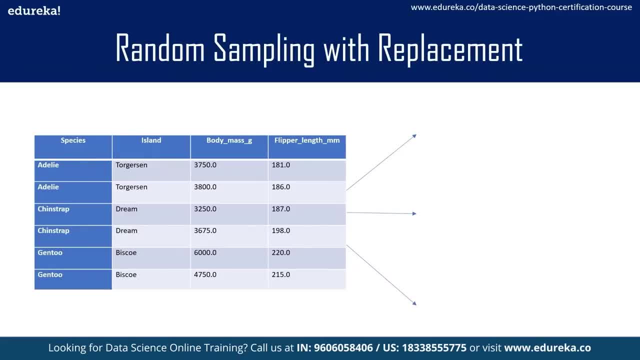 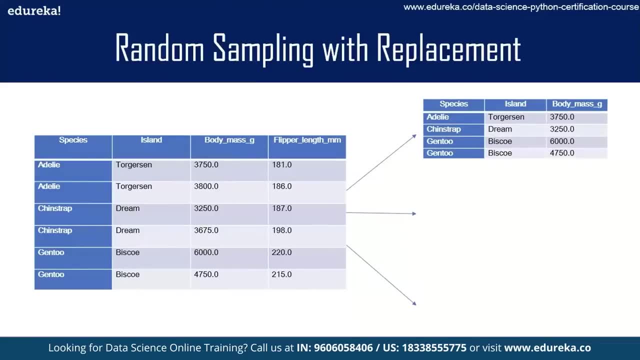 subsets will become our decision trees and then we'll be constructing decision trees from these subsets. So let us create our first subset, and you can see here that the subset is randomly been created. and for convenience sake, let me just also show you the different subsets here. 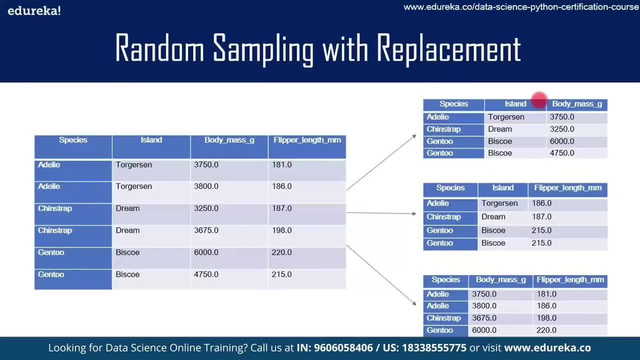 Okay, So now for better understanding, let us understand this: that in the first subset, if we focus, we've got certain random rows here and we've got certain feature, but we do not know how this feature has been selected. We got island and we got body mass, but in the second subset, we got island. 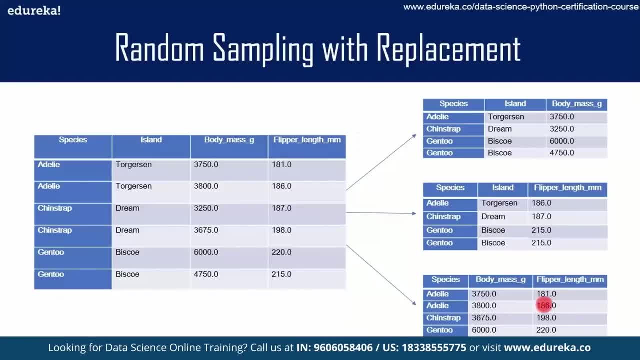 and flipper length, and in the third subset we got body mass and flipper length. right now, Let's look at the rows. Now, when I am talking about these features, I will say: this is feature selection and remember this term. now coming to the second, 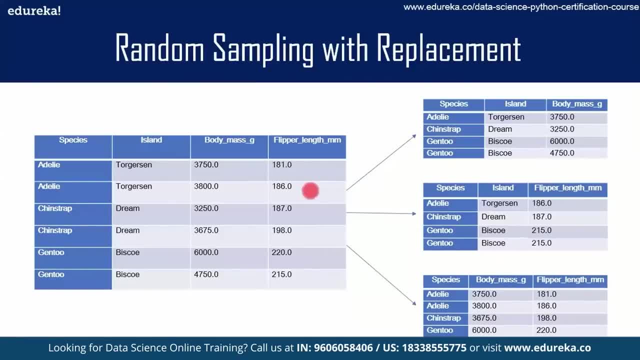 concept that is random sampling. now, random sampling is nothing but selecting randomly from your subset. So I'm selecting randomly certain rows from my subset and creating further subset. Okay, So what is replacement here? Replacement is can be seen here and can be understood with this second. 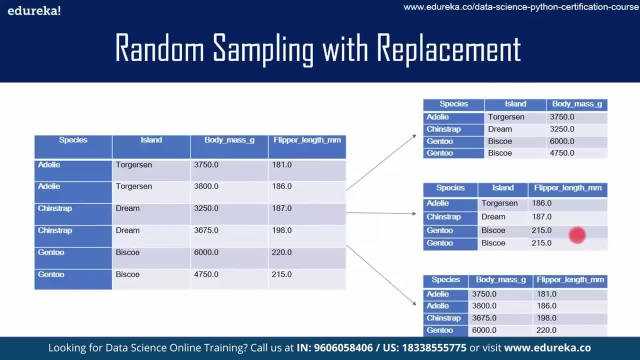 subset. We see here that the Gento species- this row is being repeated again and this is replacement. that means that when we are working with repeated rows and this row can be repeated again in the second or the third subset, then this is random sampling with replacement. 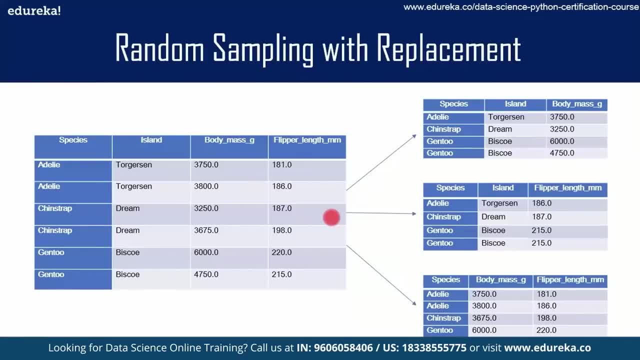 That means my random Forest can use a row multiple times in multiple decision trees. right, So this is the basic concept of random sampling, with replacement and feature selection in random Forest. another important term which I would like to bring into the note, This is that when we are working with these type of small subsets, 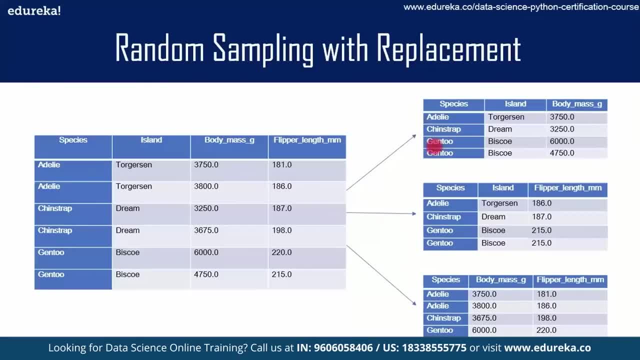 These are also known as a bootstrap data sets, and when we aggregate the results of all these data set, it becomes bootstrap aggregation. So just filling in the gaps so that later on the concepts become more clear. So now let's move on to drawing decision trees of these subsets. 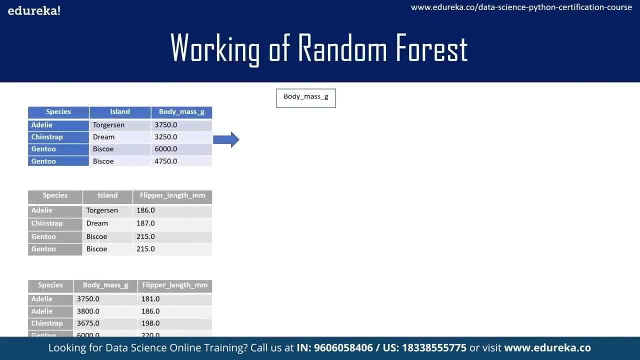 Okay, So let's draw the decision tree of the first subset again. We are taking body mass as the first root, Not, and then based on a decision like if the mass is greater than equal to 3500, then take a decision: either yes or no. 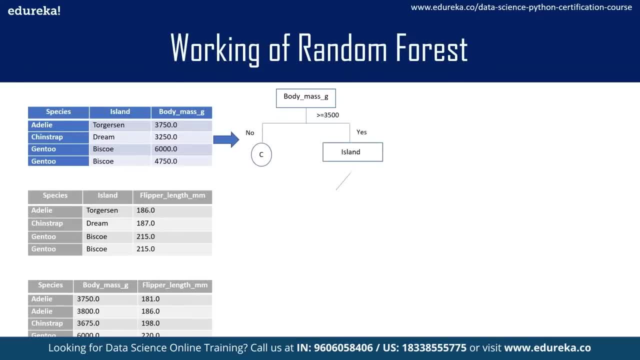 If it is no, then the species is chinstrap, and if it is yes, then again you partition based on Island, and if it is togracin, then it is early, and if it is visco, then it is again to species. Okay, So this is how we will construct two more decision trees of the remaining. 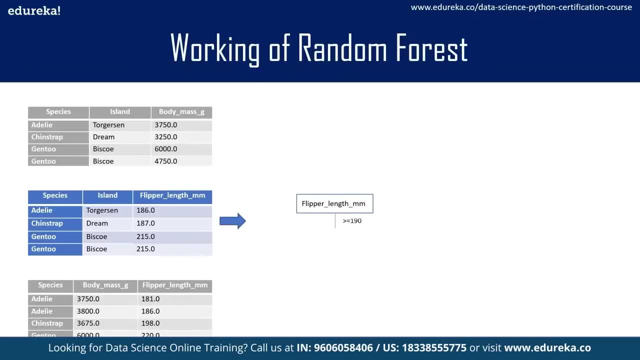 subsets. on the second subset, Let us just again create decision tree, And here now we are taking flipper length and then, based on a condition, that if the flipper length is greater than equal to 190, then make a split. if it is yes, then the species become Gentoo, and if it is no, that means 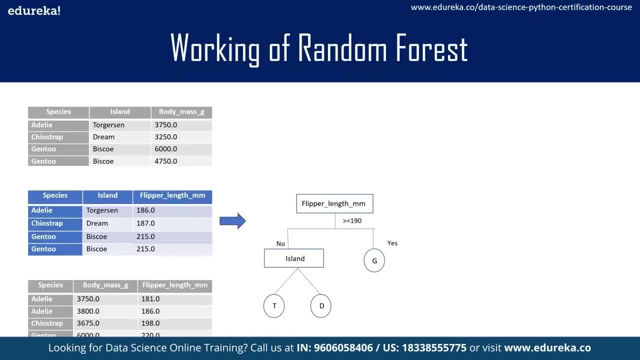 again make a decision based on Island, and if it is togracin, it is edeli, and if the Island is dream Island and it is a chinstrap species. So this is how the decision tree of the second subset has been created and this is how it will take. 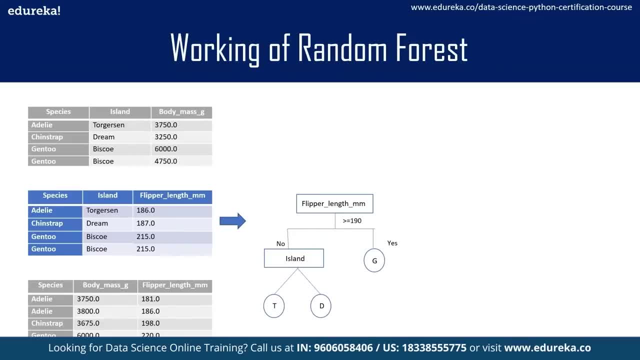 Decisions right, based on the tree length, depth and also the features it is selecting. Okay, So now let's create the third decision tree of the third subset and we get a decision tree something like this: where, in body mass, if it is greater than 4000 and if it is yes, then clearly it is again to species. 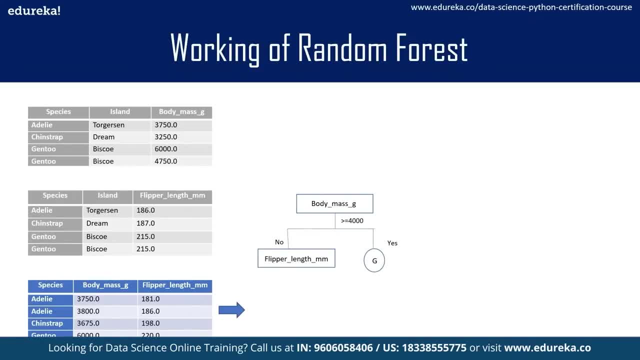 and if it is no, then again make a partition with the with respect to flipper length- another feature here- and then if it is again greater than equal to 190. Then the species would be edeli, as it would be chinstrap. So this is how decision tree three will make a decision. 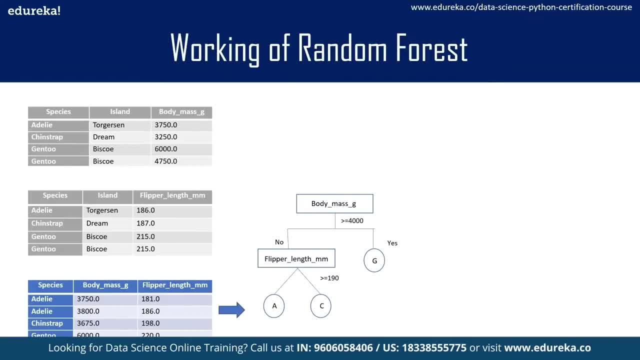 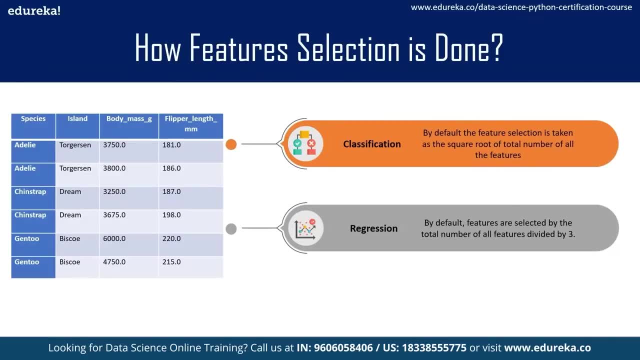 Now let's just keep these decision trees with us, Okay, and we will make sense of these trees just in a while. Okay, but before that, let us understand how feature selection is done in a random forest. How am I selecting the columns? 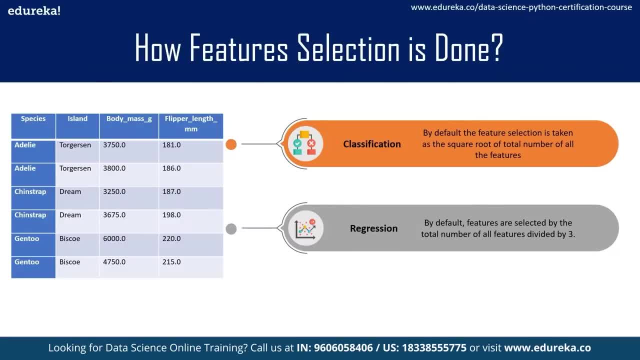 So for classification, by default the feature selection is taken as the square root of total number of all the features. now suppose we have a I've got here for features, So it is a classification problem. I will take the square root of these four features, which becomes two. so 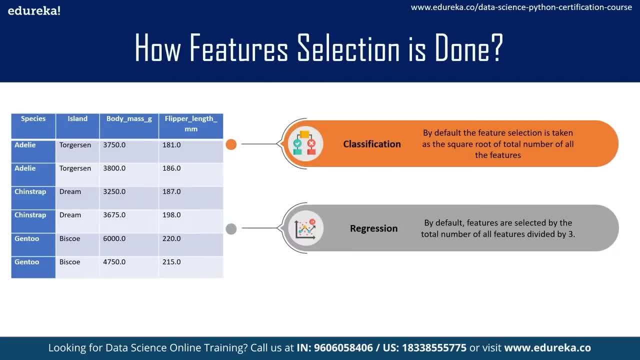 decision tree would be constructed based on two features each. is suppose I had 16 features, then it would be square root of 16, that would be four. so four features would be taken in each decision tree. All right, and suppose if this would have been a regression problem then. 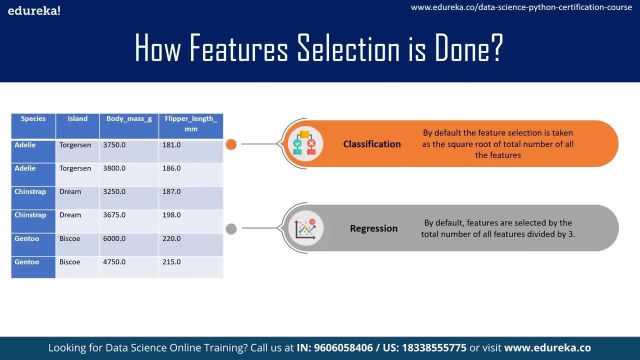 by default. what would happen? the features would be selected by taking the total number of features and dividing them by three. Okay, So this is how, by default, the feature selection is being done by a random forest. Okay, Now let us move on forward to consolidating our learning. 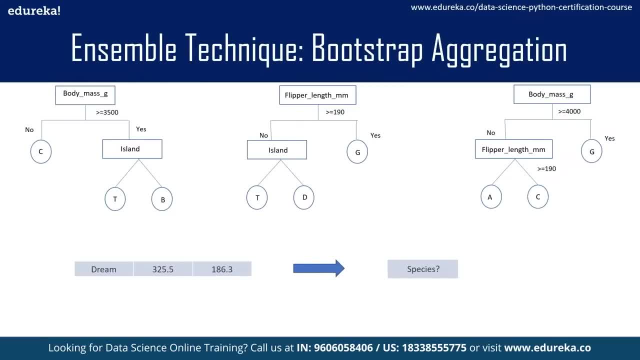 So now we are coming to ensemble techniques. that is also known as bootstrap, aggregation, random forest uses, ensemble techniques. and what is assembling? it just means that you are aggregating the result of the decision trees and taking the majority vote in case of classification and the mean in case of regression problems and giving the output. 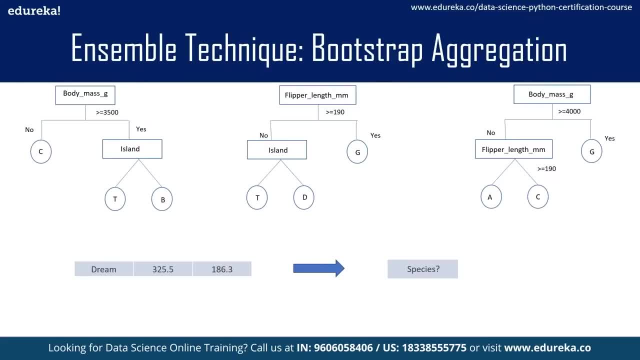 Okay. So now we have again plotted all our decision trees here and below, we can see that there's an unknown data, and I want to predict the species of this data. So what will happen is that, again, let us just feed this problem to each. 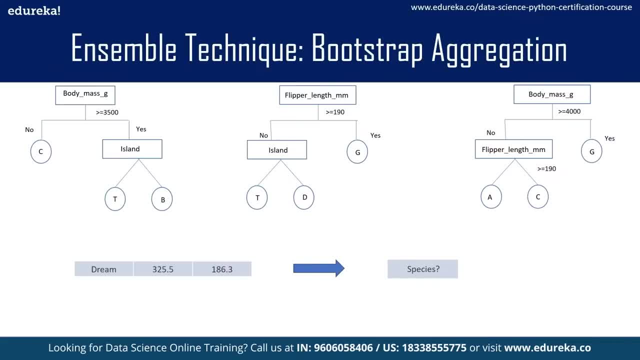 of the decision tree and let's see what each decision tree makes the prediction. So I just feed this unknown data to decision tree one and it says that, okay, the species seems to be chinstrap. Okay. and then decision tree To says that, based on the data, it has been found that the species is. 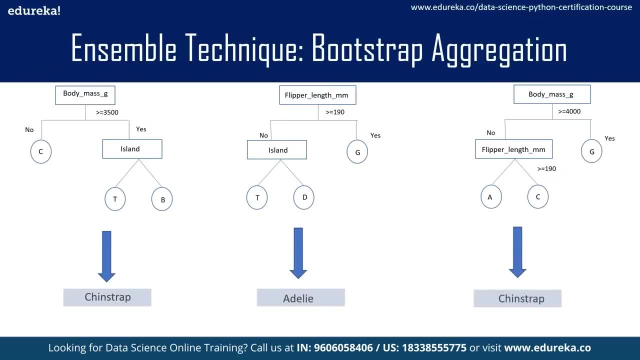 elderly and then decision trees. He says that, no, I with my decision tree, This species is chinstrap. Okay, Now all these data has been fed to random forest classifier and it says that: okay for chinstrap. I've got two votes for elderly. 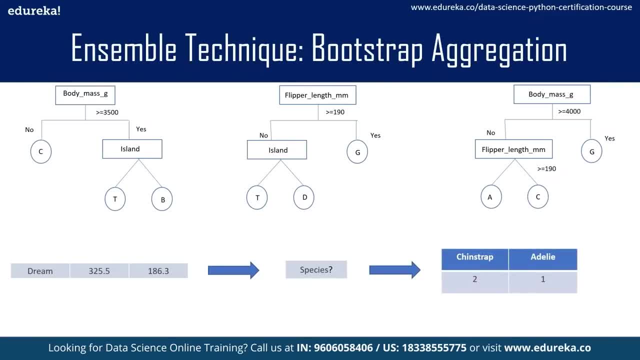 It's got one vote, So the new species would be chinstrap, right. So this is how the bootstrap aggregation is done: Based on the majority voting and decisions taken by different decision trees, They have been combined together, aggregated and we get an ensembled. 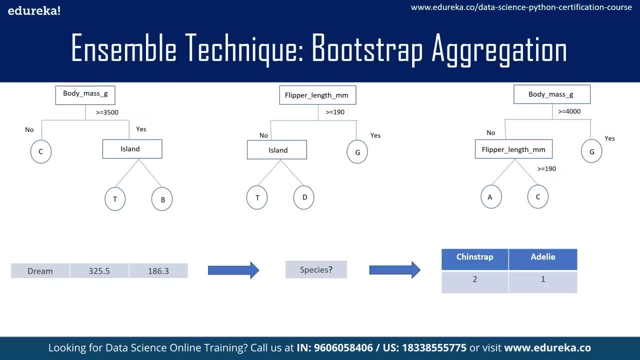 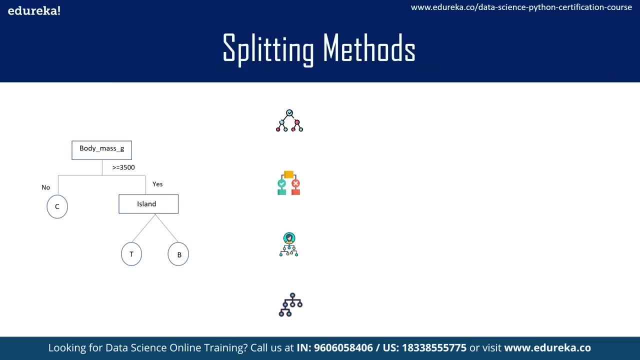 result in the random forest. Okay, So this was very simple concept of ensemble techniques which has been used in random forest. Okay, So now let's move on forward to splitting methods. So what are the splitting methods that we use in random forest? 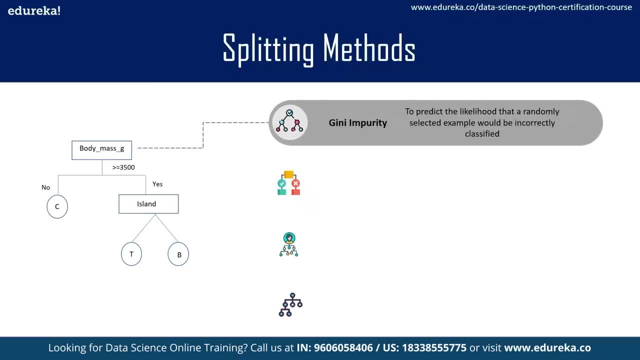 So splitting methods are many, like gene impurity, information gain Or chi-square. So let's discuss about gene impurity. So gene impurity is nothing, but it is used to predict the likelihood that a randomly selected example would be incorrectly classified by a specific. 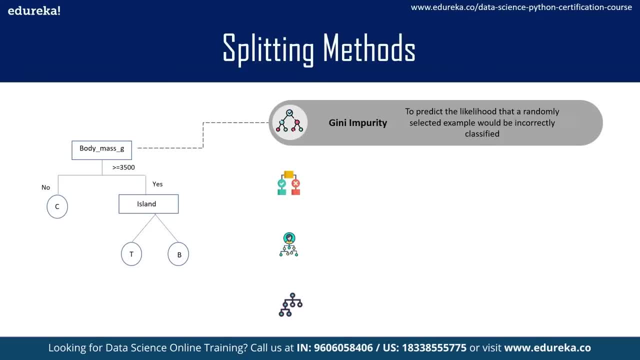 node and it is called impurity metric because it shows how the model differs from a pure division right. And another interesting fact about gene impurity is that the impurity ranges from 0 to 1, with 0 indicating that all of the elements belong to. 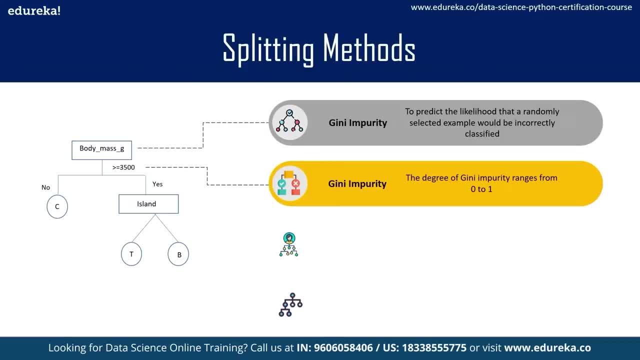 a single class and 1 indicates that Only one class exists. now, value which is like 0.5.. This indicates that the elements they are uniformly distributed across some classes right now. moving on forward to information gain, Now this is another splitting method which random forest can use and 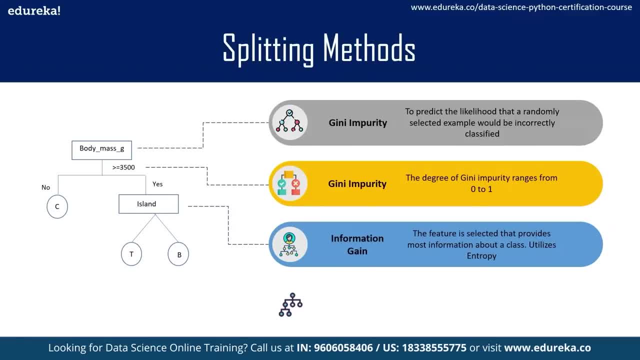 information gain utilizes entropy. So entropy is nothing but it is a measure of uncertainty. So information gain, Let's talk about that first. So the features: they are selected. that provides Most of the information about a class right and this utilizes the entropy concept. 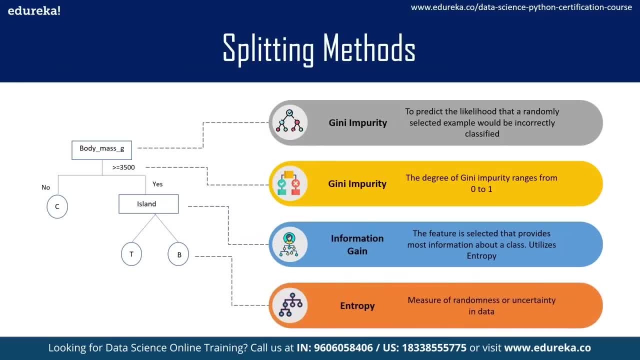 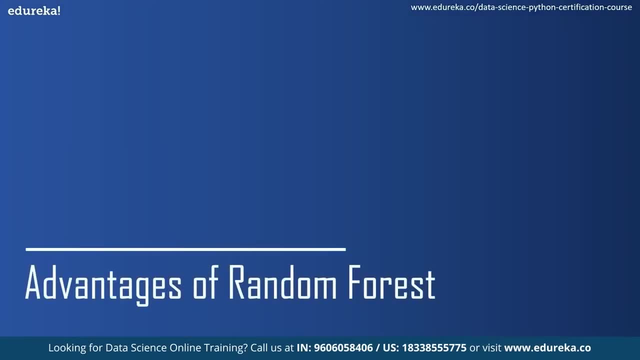 So let's see what is entropy. This is a measure of randomness or uncertainty in the data, right? So now let's move on to understanding the advantages of random forest, and we see here various advantages, So let's focus on, firstly, low variance. 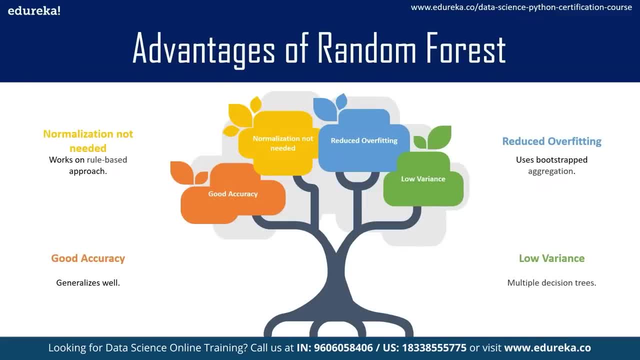 Now, since random forest overcomes the limitations of decision tree and it also has the advantage of low variance because it Combines the result of multiple decision trees and each decision tree is being trained on limited data set that we have seen earlier also, so each tree was making its own subset of data and training. 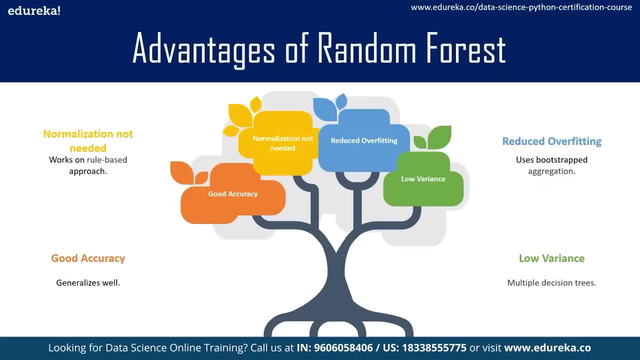 the data on that limited length of the tree. So there's less step, There's less overfitting and low variance of the data. So, coming to the next point, that is, reduced overfitting again, since we were working with multiple decision trees, hence reduce depth of. 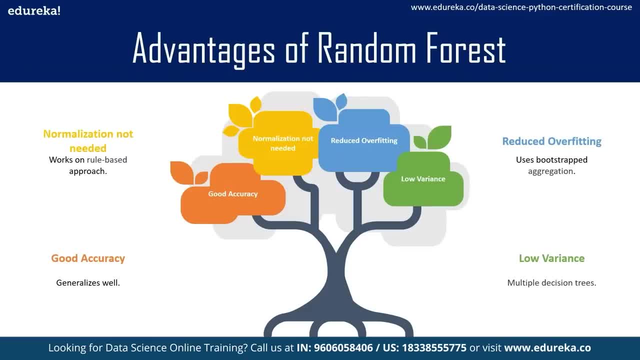 the tree. So we get reduced overfitting. That means the model is fitted Well and it does not tries to learn even the noises right. So we use the bootstrap, aggregation or bagging here in random forest And that is why we also get reduced overfitting in random forest. 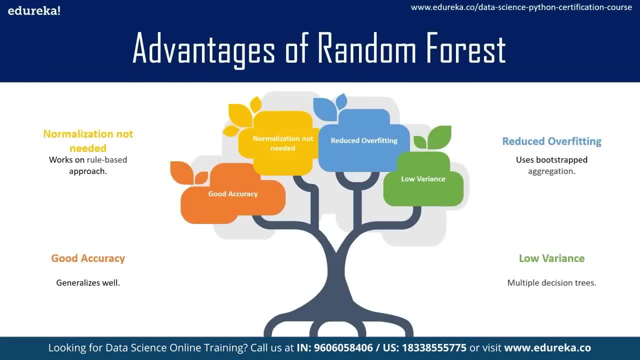 And this is one of the reasons that. why is it so popular? because you don't have to worry about overfitting of the data, right, All right. Now moving on forward to the another advantage is that the normalization is not required in random forest, because it works on rule-based approach. 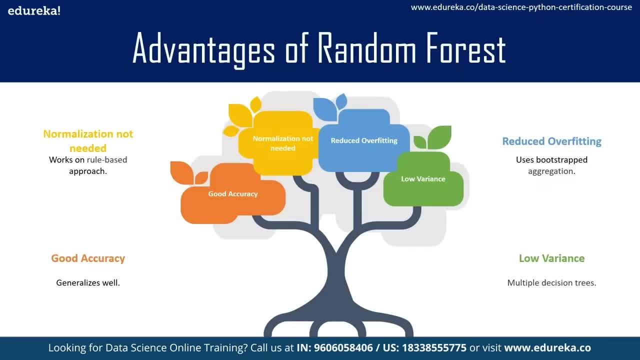 Right, And another advantage is that it gives really good accuracy, which we will also see in our hands-on. It really gives a very nice predictions, either precision or recall, and generalizes well on unseen data as compared to other classifiers or machine learning classifiers which are present, like Naive Bayes or 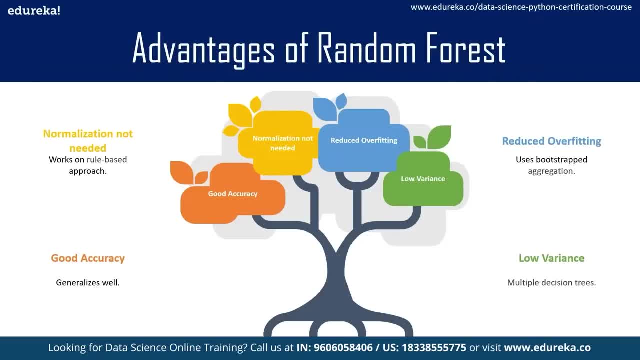 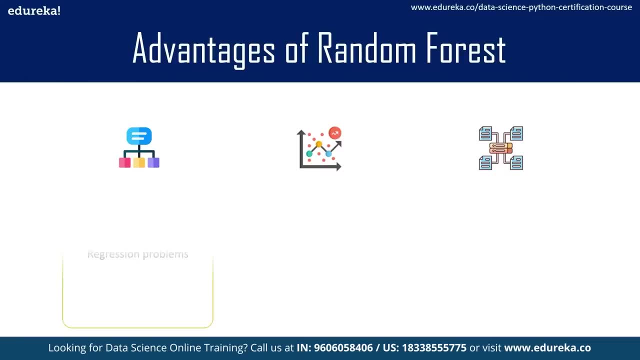 SVM or KNN, Random forest really outperforms other classifiers right. So let's move on to understanding. few more advantages of random forest is that it is suitable Both classification and regression problems, and also it works well with both categorical and continuous data. 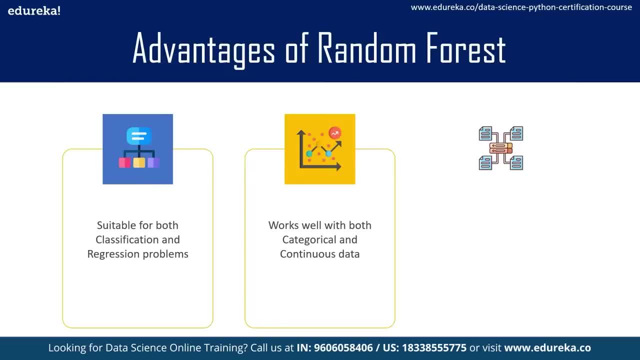 So you can use it well with any of the data sets right, And it performs well on large data sets right, So it solves most of the problem. That's why random forest is largely been used in machine learning problems. Now moving on forward to certain disadvantages of random forest: 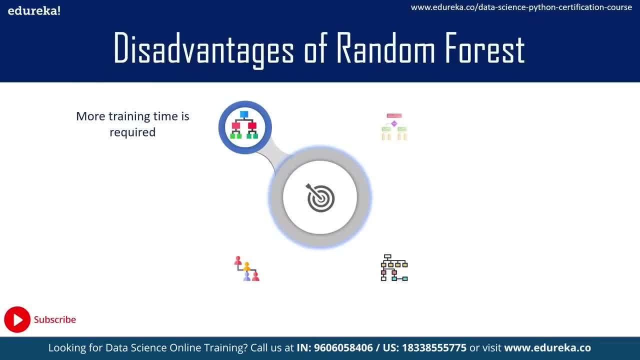 So the first disadvantage is that it requires more training time because of the multiple decision trees. If you've got a huge data set, you would be constructing hundreds and hundreds of decision trees and that requires a lot of training time. and here comes one more disadvantage is that the interpretation becomes 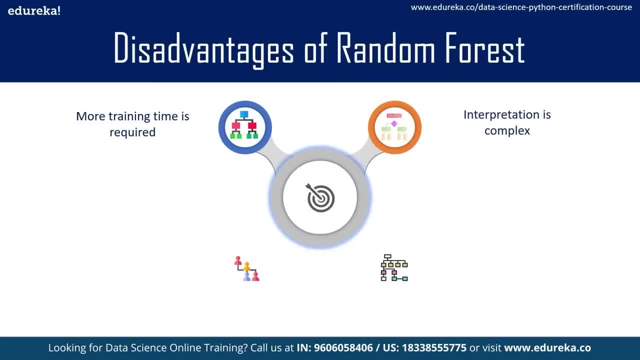 really complex when you've got multiple decision trees. So decision tree interpretation is easy because it is an individual decision tree, But when you combine hundreds of decision tree to form a random forest, the interpretation is really very difficult to understand and becomes quite complex to apprehend. 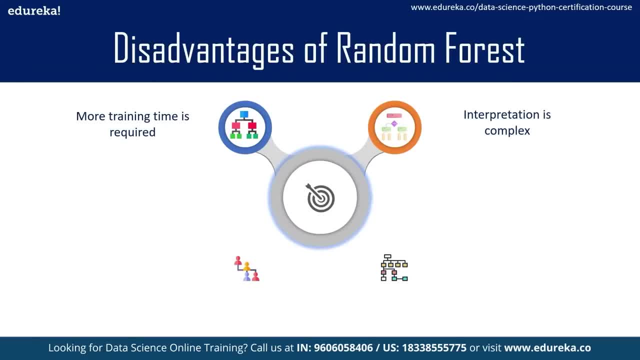 What exactly the model is trying to predict and where the splitting occurs and what features are being selected and so on. And another disadvantage is that it requires more memory. So memory utilization is really heavy in case of random forest because we are working with multiple decision trees. and another disadvantage is 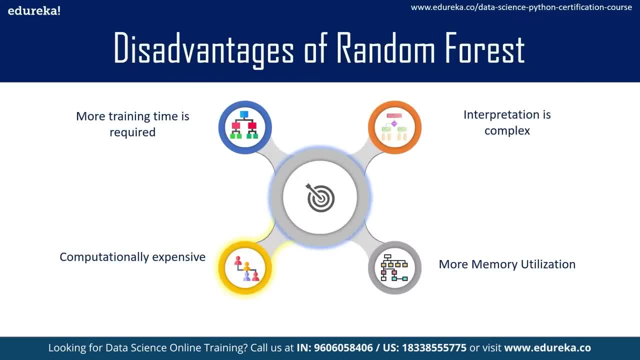 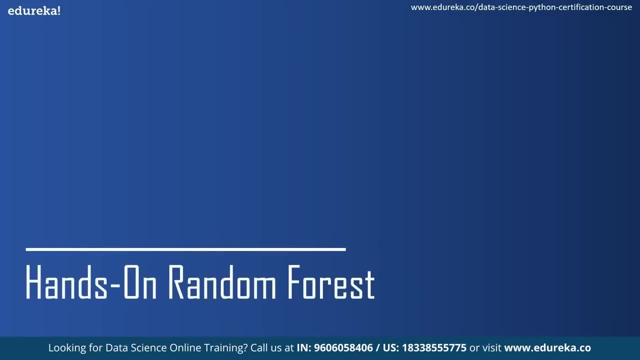 that it is computationally expensive and requires a lot of resources because of the training of multiple decision trees and also storing them All right. So this was all About random forest, the theory part of it, And now let us just move on to the practical demonstration or a hands-on. 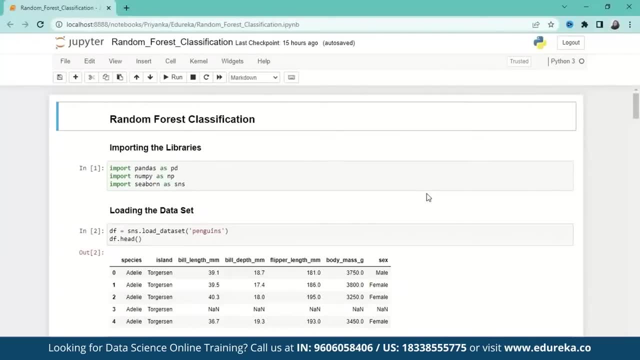 on random forest. Okay, So now it's time for a hands-on on random forest. So let us just import a few basic libraries of python in our jupyter notebook and we will run this. We will import pandas as pd, numpy as np and seaborn as sns. 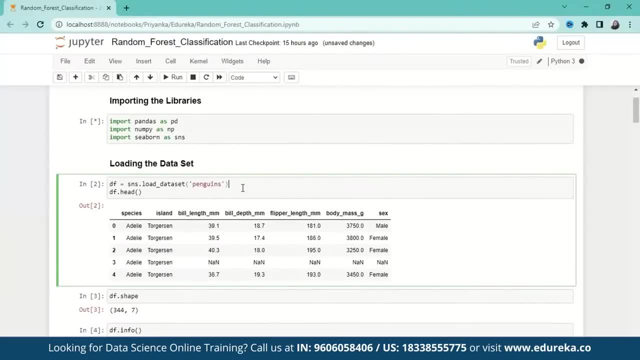 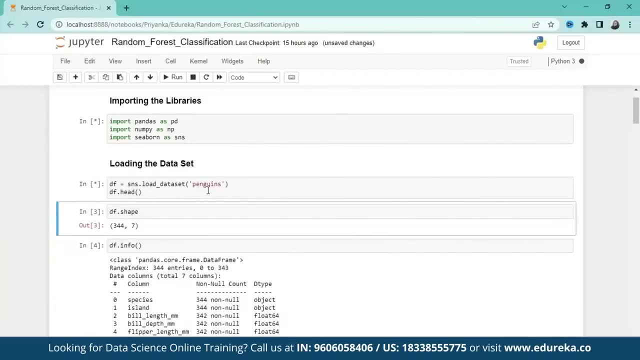 Now seaborn is needed here because we want to load a data set, that is, a penguins data set, with the help of seaborn. And this is already been preloaded in seaborn. This is already loaded data set and seaborn has got multiple data sets, you know, for practice, for beginners. 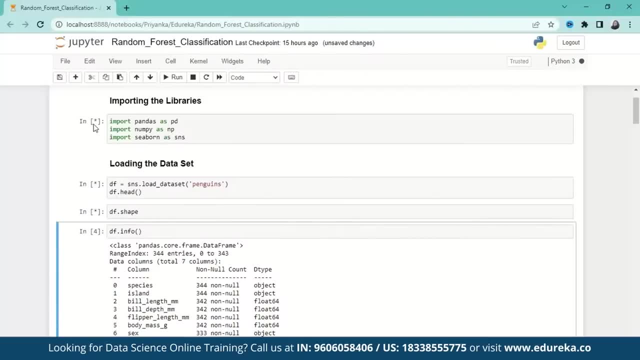 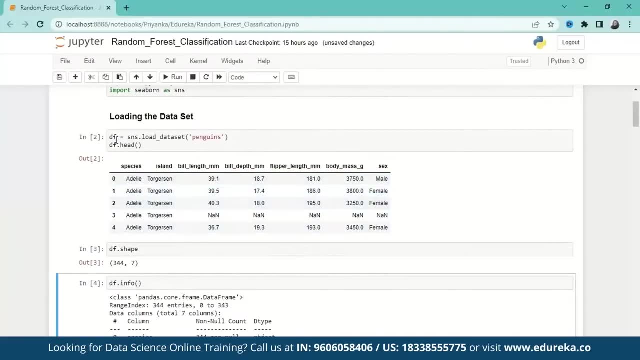 So it is a good way to practice for data sets. Now you can see this asterisk sign. That means it is telling us to wait, So let us just let it get loaded. So we get got our data in an object called DF and we can see the first. 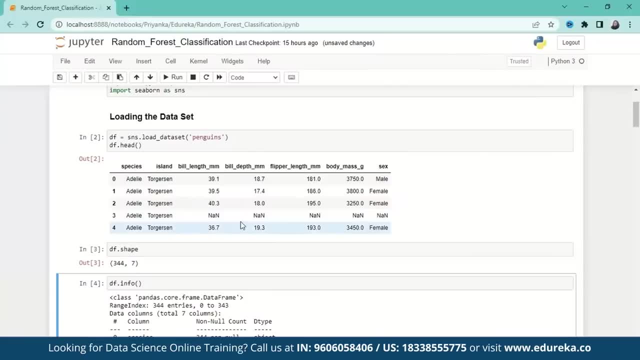 five entries here and this data frame is shown in the form of a table, rows and columns, and we see here some species are in bill length, Bill depth, flipper length, body mass and the sex of the penguin. So our task is to specify or to classify these species of penguins and 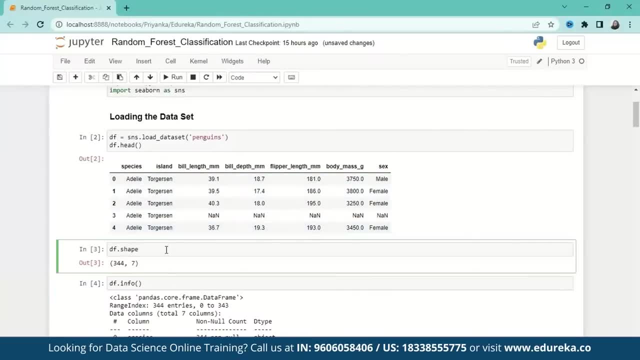 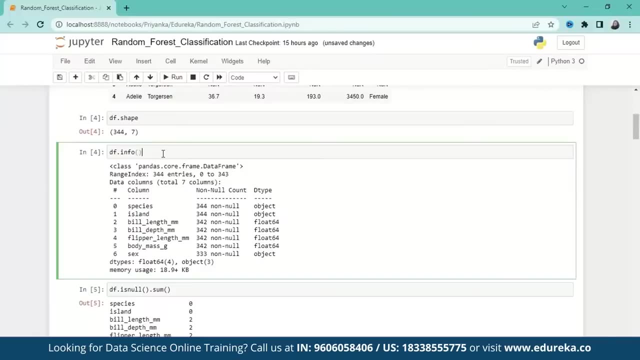 do the respective correct species right. So we see the shape of our data and we see that it is like three, 44 rows and seven columns, and we will see the info. So we see DF dot info and this gives us, along with the non null count. 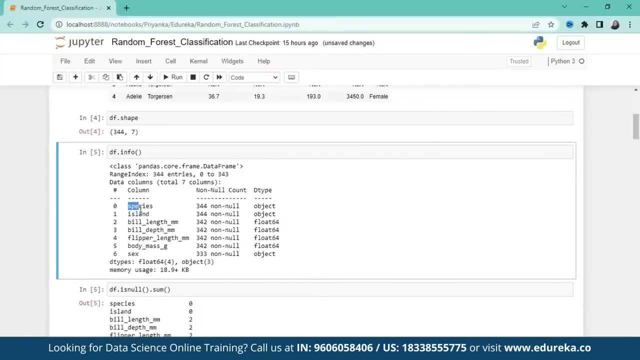 We also get the data type of the values. So we have got species island as the object data type, Whereas the bill length, bill depth, flipper length and body mass are in floating point, or you can say floating data type, and the sex is in. 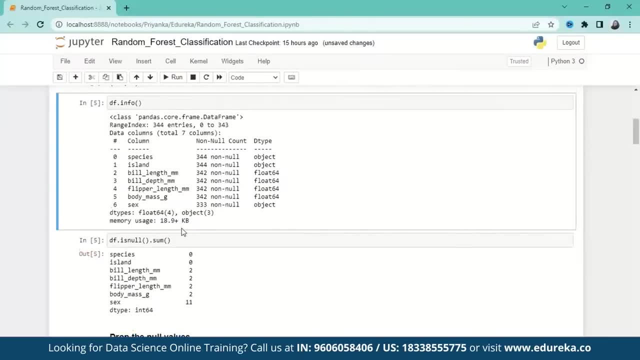 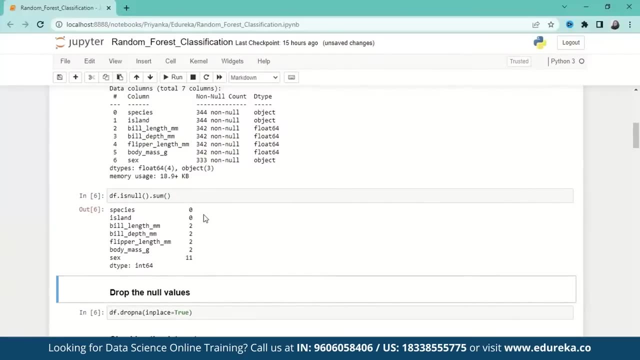 object: data type: right, So now moving on forward to calculating how many null values are there with the help of DF. dot is null dot sum, So we get certain, like some, around two null values in all these columns. as you can see the features like bill length, bill depth, flipper. 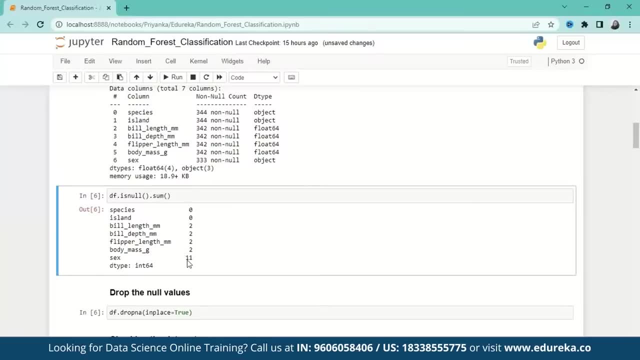 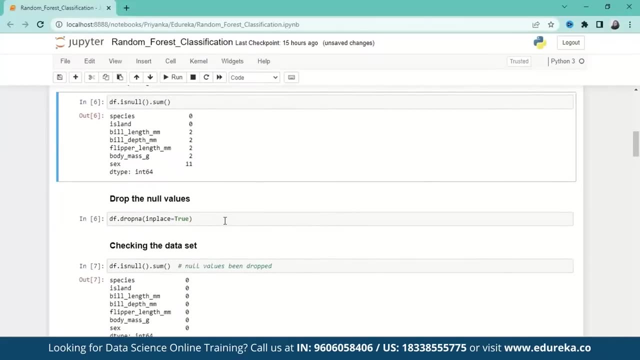 length and body mass, whereas there are 11 null values and sex features, Sure right. So what we do is, since they are very small null values, we can just drop it or you can also ignore them. So here in this data frame, what I'm doing is I'm just dropping these. 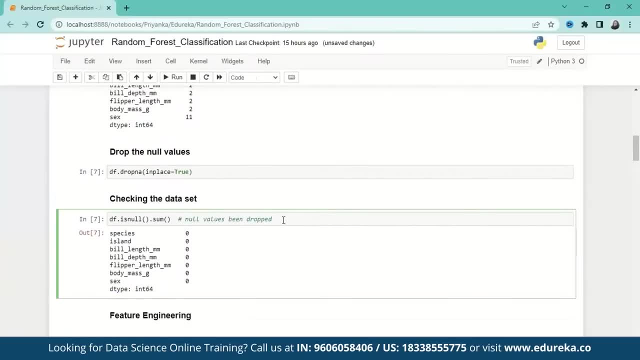 null values and let us just check whether they are being dropped or not with the help of again the same function: dot is null, dot sum, and then we see that, yes, they have been dropped from our data frame. Now let us do some feature engineering with our data. 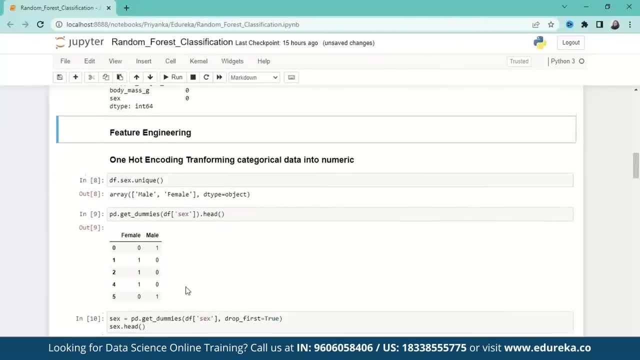 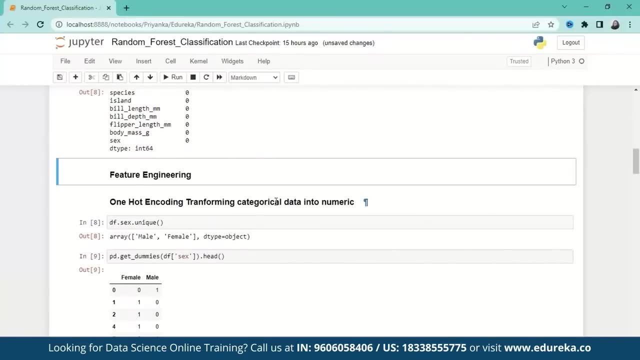 Now we have seen that we have got some object data type in our data frame and before feeding it into algorithm That is random Forest, We have to transform the categorical data or the object data type into the numeric. So we are using here one hot encoding to convert the categorical data. 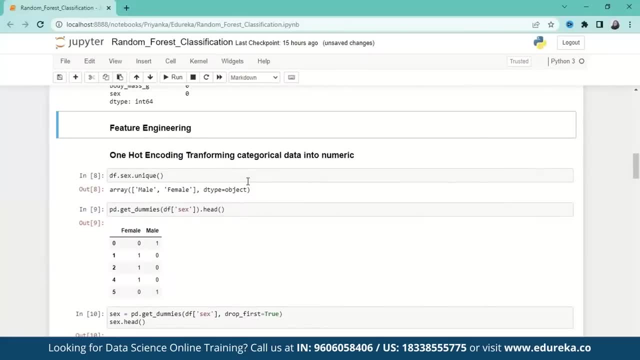 into numeric. Now there are various ways in Python which we can do that, like one not encoding, or you can also use the mapping function in python, But here we are using one hot encoding, So let us just do that and we find here. first of all, let us apply it. 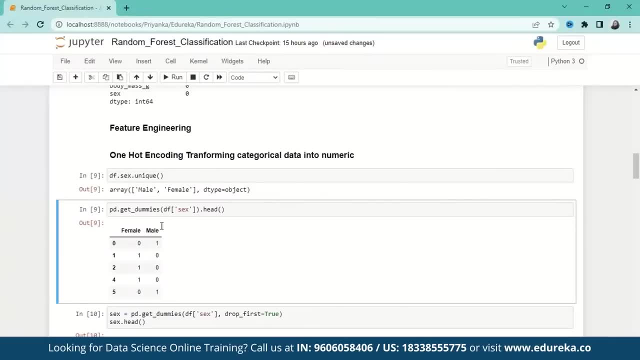 on the sex column and here we see that we have got two unique values in sex, that is, male and female, And we use pandas here to get dummies. That is how we will apply this one hot encoding, because this is how get dummies work. 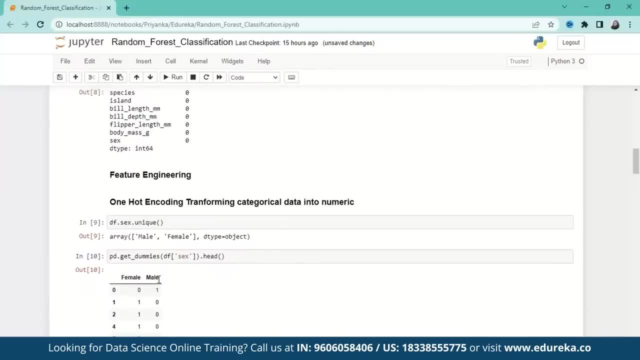 So what happens is here is that the new unique values are converted into the respective columns in the data frame. So we see, here We have got two unique values, males and females, and they are being converted into the columns. Okay. So one thing to note here is that we also get a problem of dummy trap. 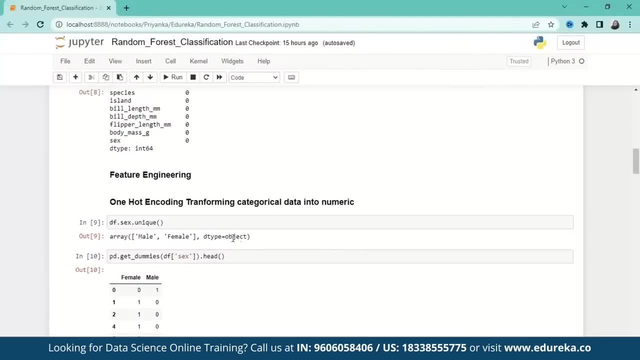 because here we see only two unique values. Now, Suppose if I had six or seven unique values and I do this one hot encoding, I would have lots of features in my data frame and that would lead to several complexities. So what I do is to keep things simple. 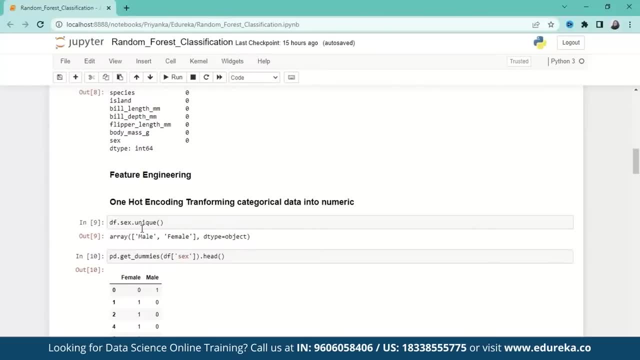 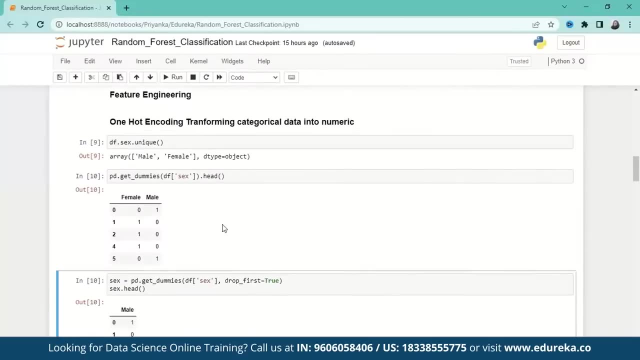 I can use one hot encoding when my data frame or my unique counts are low, when my unique values are less. So since I had just two or three, I can use it, So I'm using here. So what I do is again now one row, one column, as we can see here that 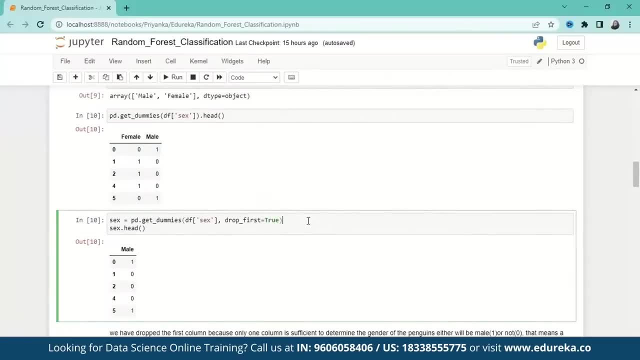 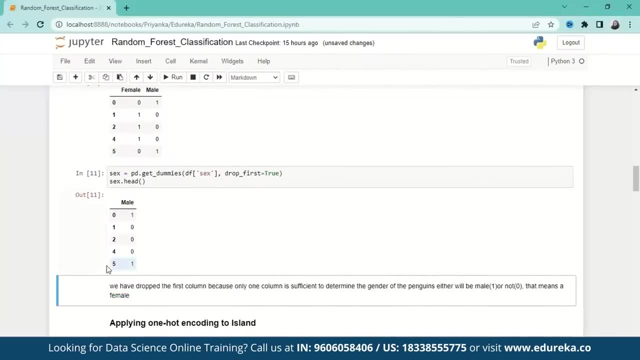 it is redundant Giving me extra information, So I will just drop it. So I drop this first column and what I get in this data frame is only male. So let us just infer whether I can also infer females from this or not. So if the value is one, that means the penguin is a male, and if the 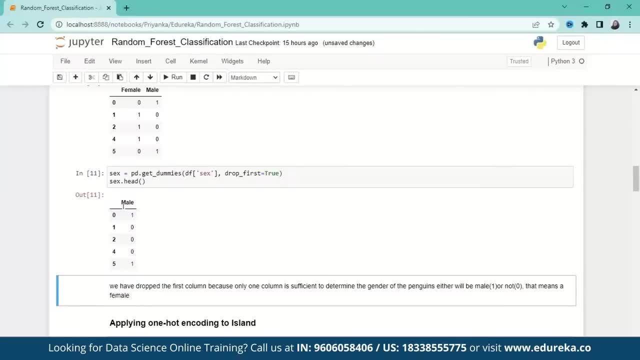 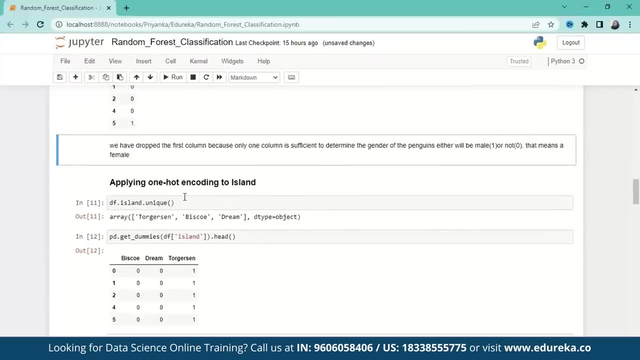 value 0, that means the penguin is a female. Okay, so only one column is needed for this data frame, So I just kept one and drop the other one. Okay, now apply again one hot encoding to the island feature. So in island, if we check the unique values, we've got three unique. 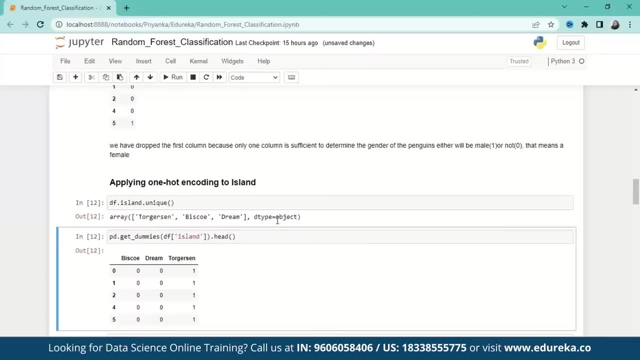 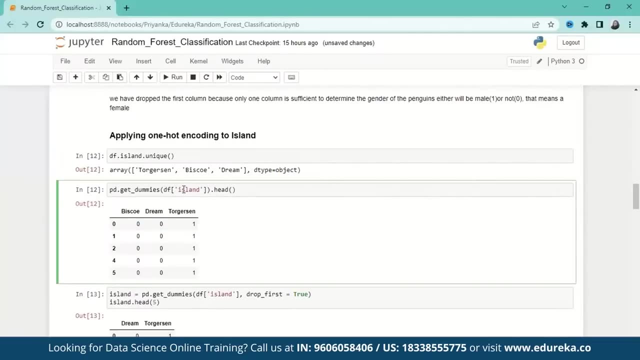 values here- Togerson, Biscoe and dream island- and the object is the data type right. So again, we will use pandas, PD dot, get dummies and we will use apply it on the feature Island and let's get the head of it. 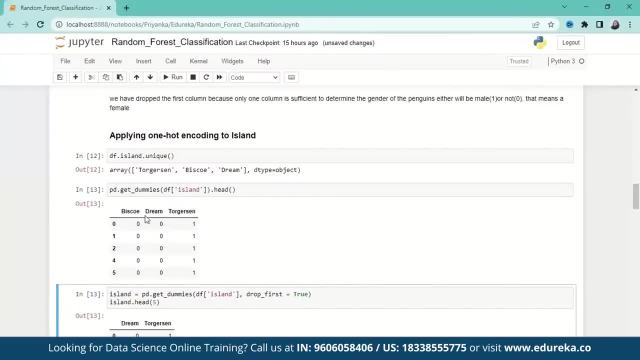 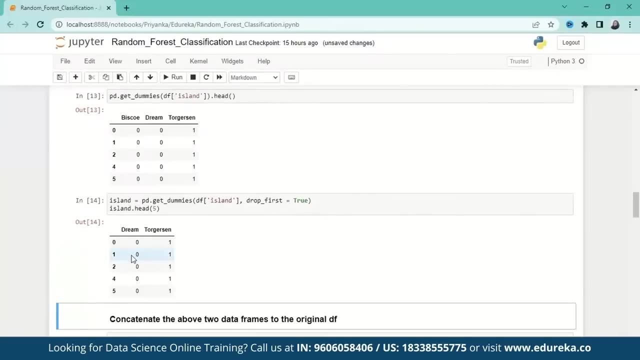 So we get here again. the unique values were converted into columns and we get your respective three columns and then again we will just drop the first column to get the remaining two columns. So here Here also, we can infer that if the island is Togerson, if it is one, 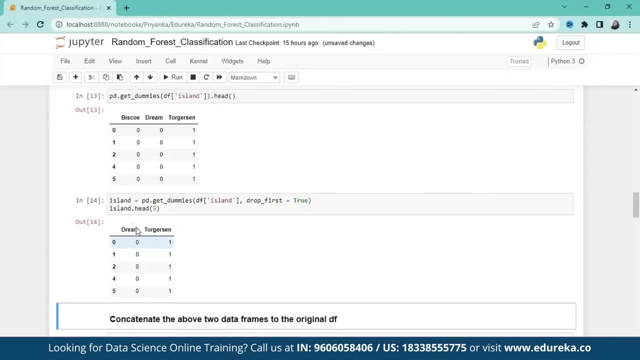 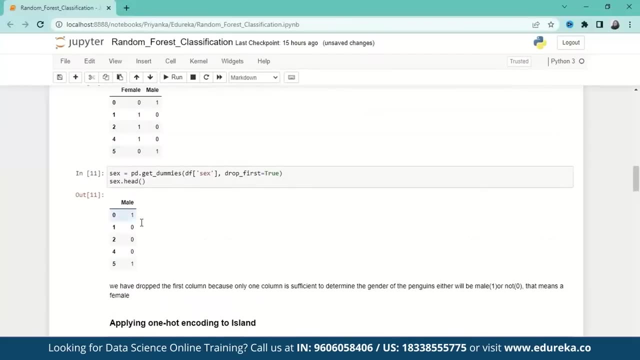 then it is not dream, neither Biscoe, right? So this is how we can read it from the data frame and understand that. now remember this thing: that these two Island and here sex. These are two independent data frames. These are not yet included in the main data frame. 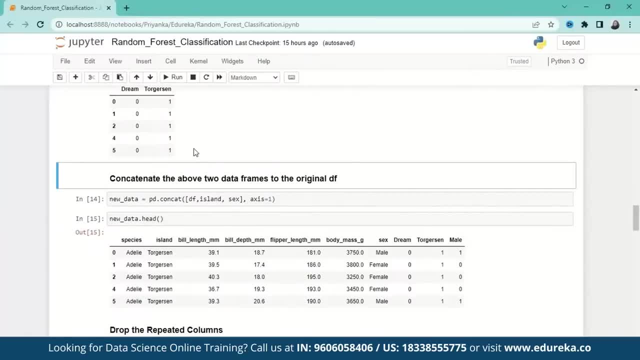 So what we will do now is we will concatenate the above two data frames into the original data frame. So what we do, we again create a new data frame, that is, new data, and let us just concat with the help of PD dot concat Function and we will concat what DF, Island and sex and access is. 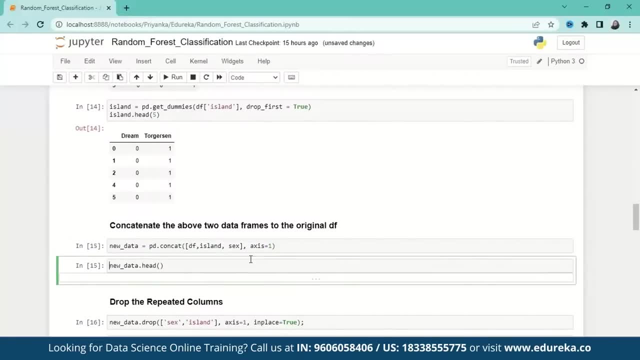 one that means in the column. Okay, so when we will run this, let's see the head of it. So everything gets concatenated in a single data frame, which is good for the feeding this data into, or splitting the data into, test and train data. 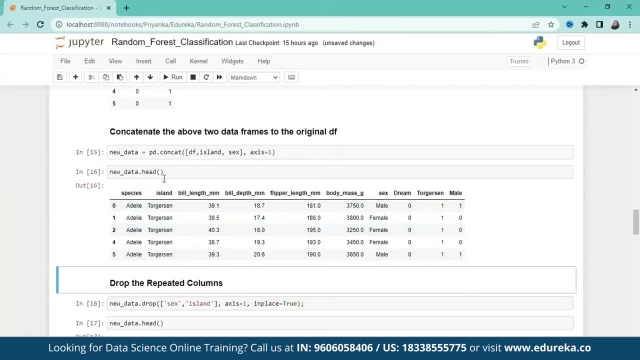 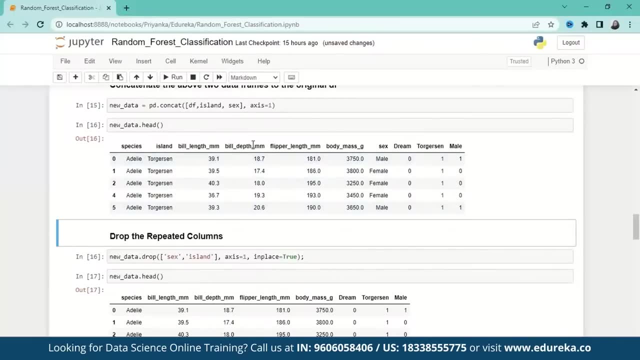 So now we have this new data frame and we've got some repeated columns here which needs to be deleted. So what we do is we will delete sex and Island here, which are just repeating, Because we've got here male and we have also got here dream and 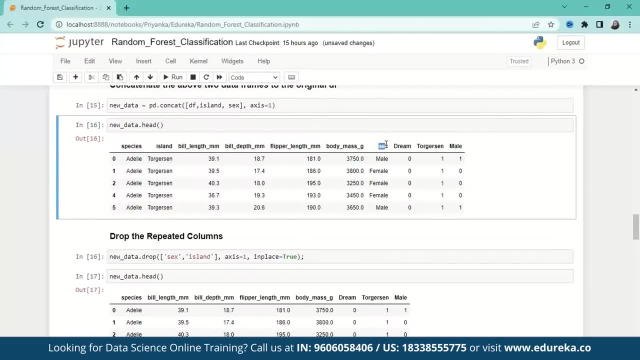 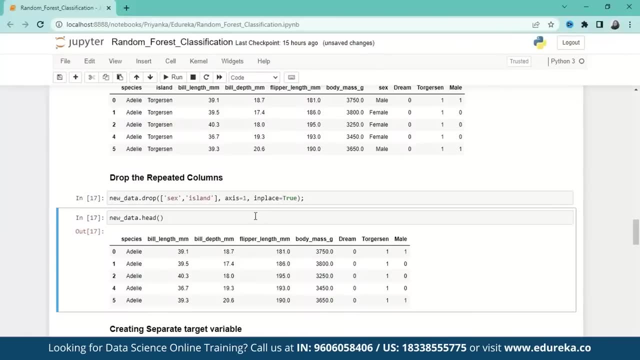 Togerson. So we do not require this Island column, neither the sex. So we just drop it with the help of new data drop and the column names. X is one in place, equals to true right. and let's see the head of this data frame. head of the data frame gives me five unique values. 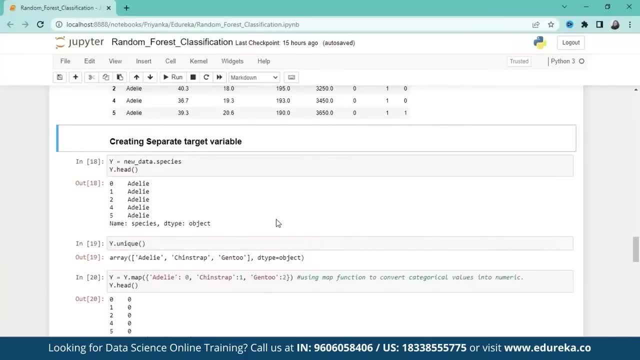 right, and now it is time to create a separate target variable, and what we'll do is we will store in a variable called by only species. So what we do Is, from this new data dot, species, We will just store the species in this by- and we see this- by a dot. 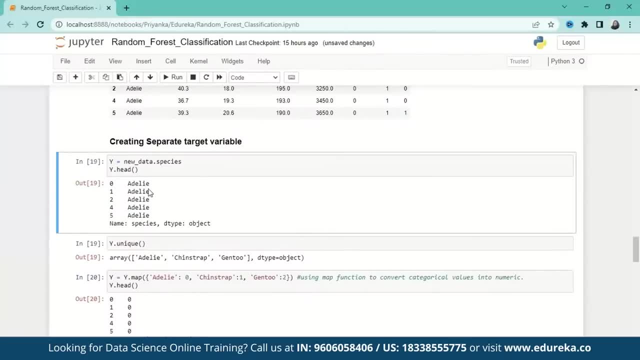 head. that is the first five species and we got the values here. That means another target variable is being created now. So and you can also see the y dot unique values as a deletion strap and get into. so now we see here three unique values of the penguin. 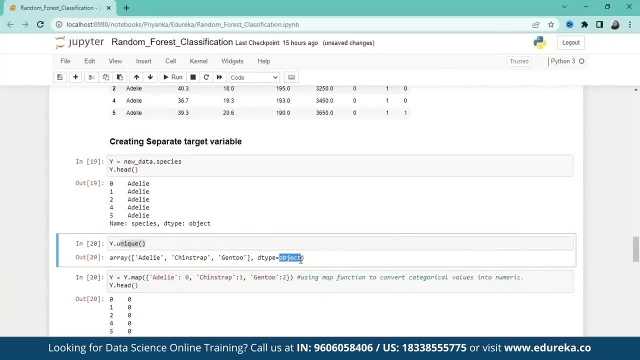 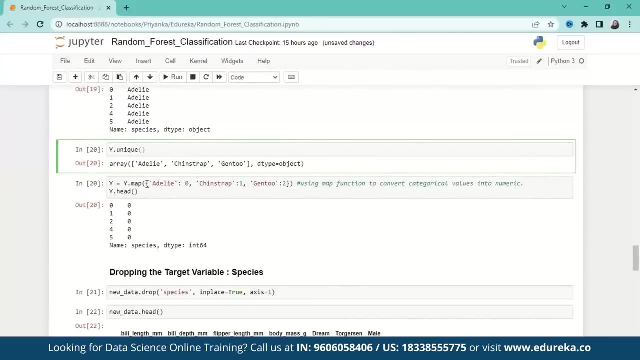 that is chin strap Italy and get into and the data type is object here. So again, we need to convert this object into the numeric data type. So now what we are doing is we are using the map function in python and what we do is we map Italy to zero, chin strap to one, and can do to: 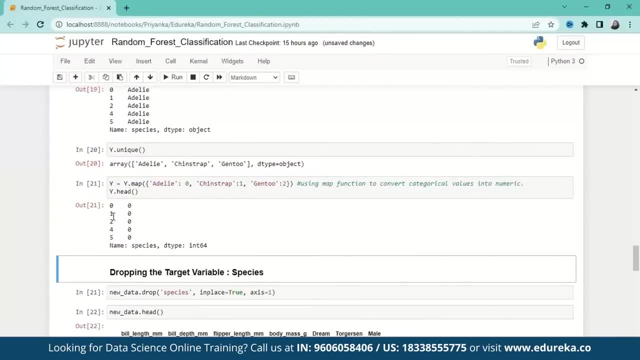 two. So this is how we see, then all the values have been mapped to numeric. This is another way to convert a categorical value into a numeric value in python. Now what we do is let us just drop the target value species from our main data frame. 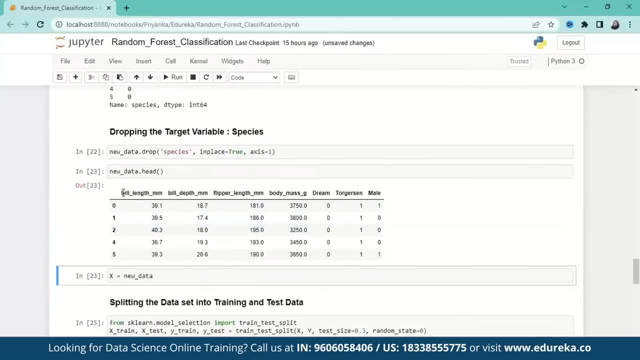 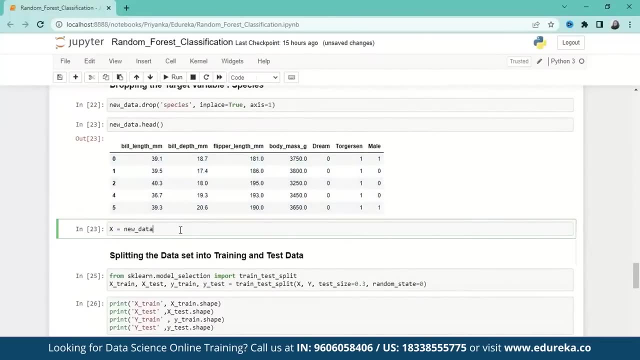 So we just drop it and let's see a new data frame. So we see that we don't have any target species here, right, Okay? So in X, let's store this new data and perform the splitting of the data. So what we do is from sklearnmodel selection. 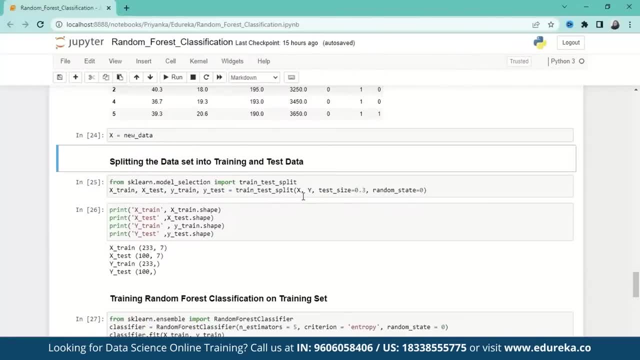 we will import our train test split and we will split our training data into 70% and 30%, or test data becomes 30% and training data is some 70% and this random state is zero, which means that I'm not fixing any random state, and this is also. 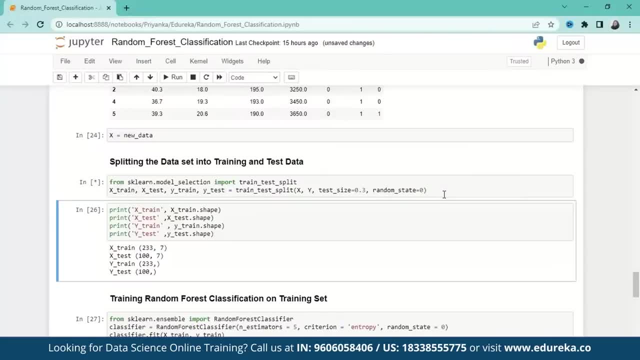 used for the code reproducibility. Now suppose if I again run this code I will get the same result. It will not change. You can set this random state to any of the random number as per your choice, and result would differ, Okay. 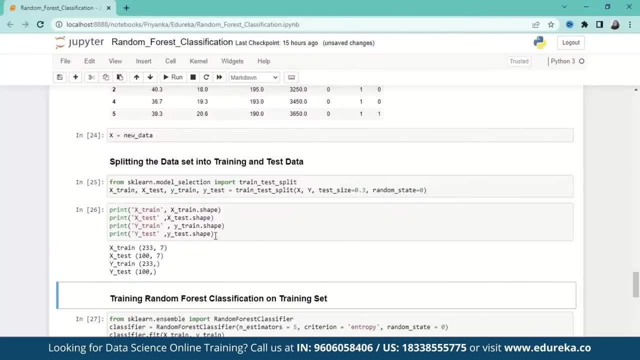 So now let us print the shape of X train by train: X test and Y test. So we see here that it has been split it into 70 and 30% and we get X train as 233 values here and seven features and X test has. 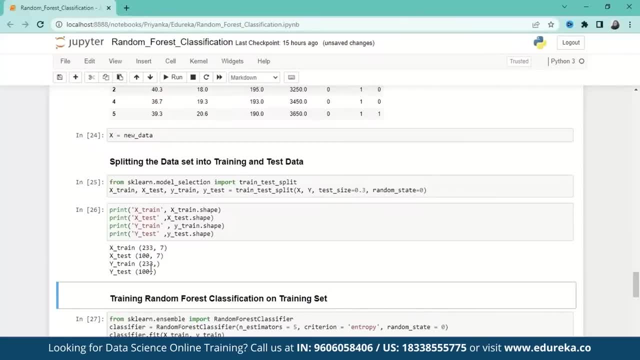 hundred values and seven features. Similarly, Y train, you can see 233 values and Y test as hundred values. That means the Species. Okay, so that has been perfectly. split it into 70 and 30%. now What we do is we will train the random forest classifier on the. 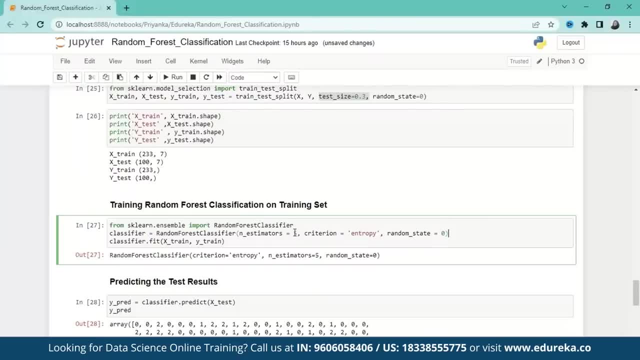 training set. How do we do it? We will import the random forest classifier from a skill on dot ensemble, So we've already dealt with what is ensemble, and then in classifier we will store this random forest and this n estimator is nothing but decision trees. 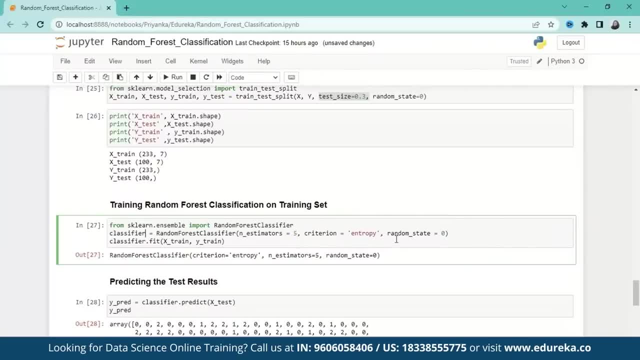 So we are creating some five decision trees here and the criteria is entropy and again random status. So let's see, and then we will fit this X train and Y train. So this has been fitted and the criteria is entropy here. All right, So now let's make some predictions and let's create a variable. 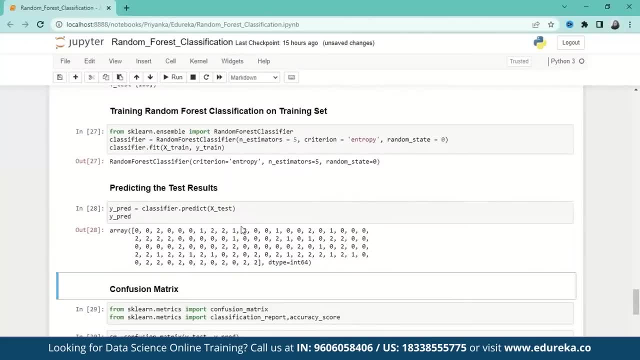 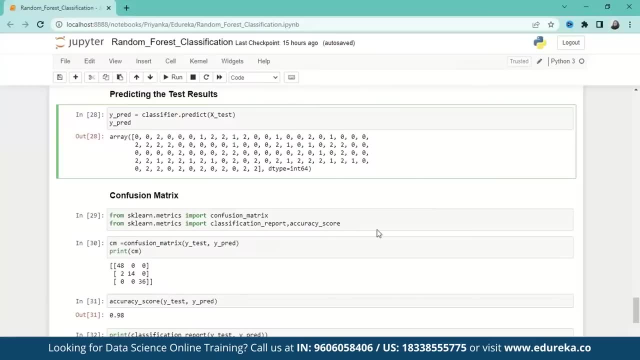 called by predict and we will just predict it on X test and we have also printed this by prediction. and now let's bring the confusion matrix to check the accuracy of random forest algorithm and what we do is from matrices, that skill and matrices. we will import classification report and confusion matrix and also the 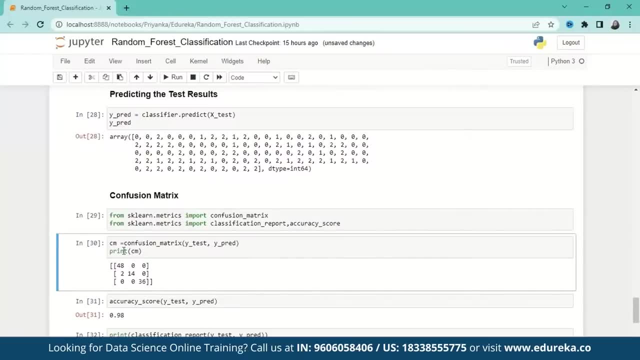 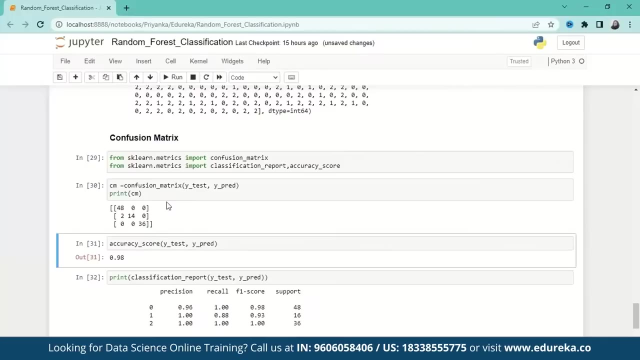 accuracy score. So we will just import them and then in CM variable We will print the confusion matrix of by test and by predictions. So we will print it and we see here the accuracy score also, which is 98%. So our random forest classifier is giving us a very good accuracy. 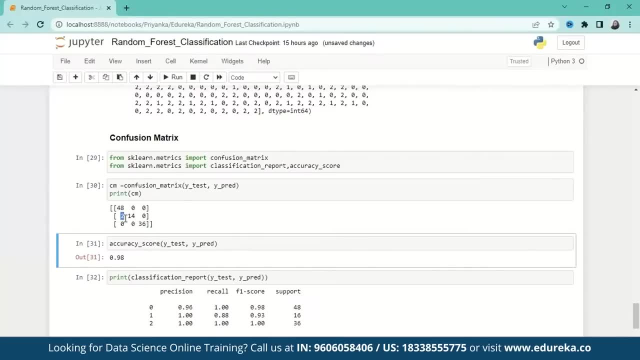 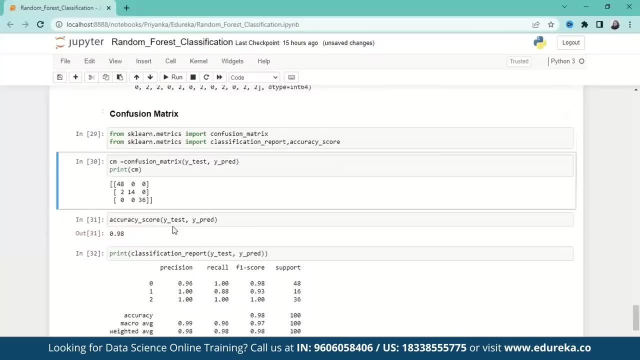 of 98% and you can see a confusion matrix that only two cases have been misclassified. rest: All the cases have been correctly classified by random forest classifier. Okay, So now let's move on to printing the classification report of my test and by prediction: 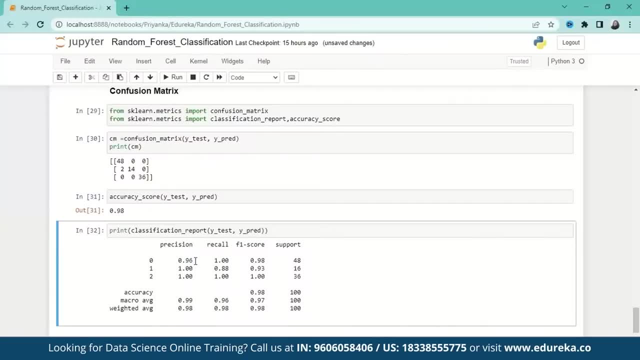 Let's see. and we get the precision as 96%. that means the two predictions by the algorithm is 96%. the recall, or the true prediction rate is hundred percent, which is very nice, and Evan score is also good, which is 98%. 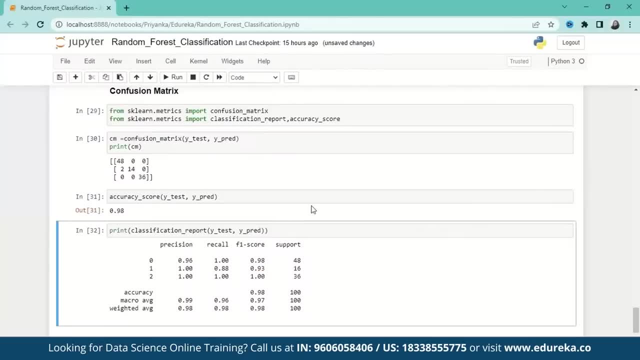 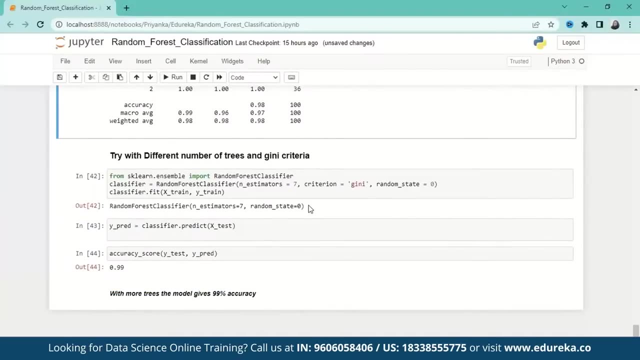 So this is giving us a good result. But what if? if we change the criteria from entropy to Ginny? So let's just experiment with that too. So let's try this with the different number of trees and change The criteria to Ginny: coefficient. 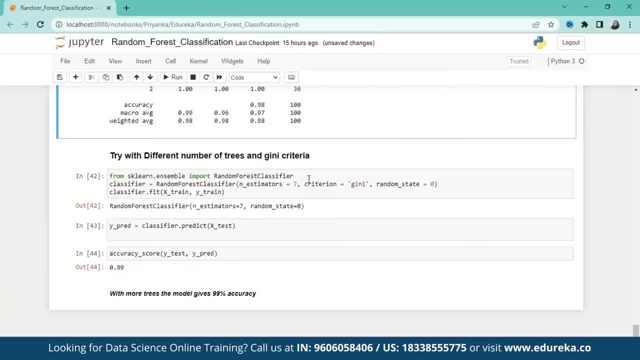 So now again from Escalon dot ensemble, we will import random forest classifier and fit it Okay. and here what we are doing is just we are using seven trees, previously We used five and now in the criteria we will use Ginny coefficient and random state is zero. 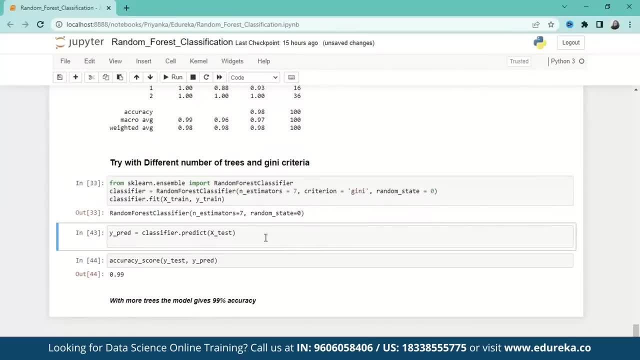 So let's run this and see whether there is a change in accuracy or not, and let's predict this. and let's check the accuracy score. What is the accuracy score for this random forest classifier with seven trees? So we get 99% accuracy with changing the criteria and changing. 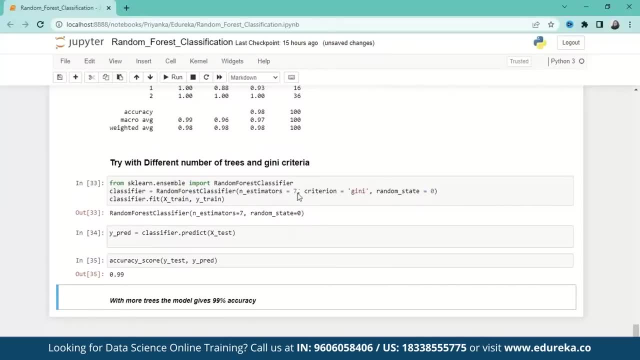 the number of trees, So you can just experiment with different number of trees and different number of decision trees. Let's just experiment with, you know, 12 decision trees and see what happens. So you can see the accuracy reduced to 98%. Okay, but seven, we were getting 99. 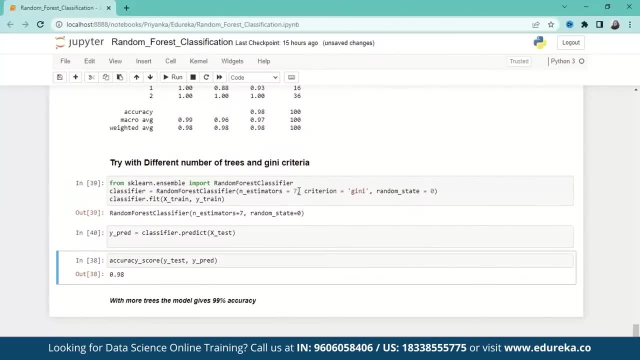 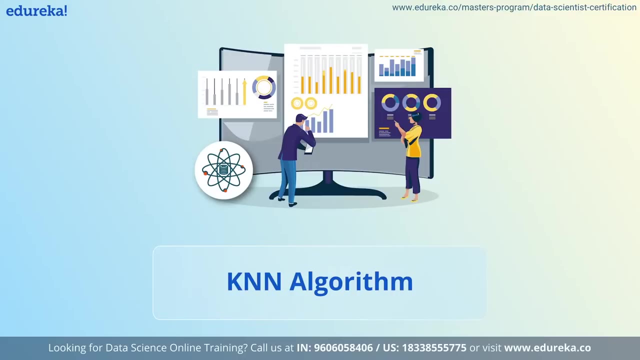 So they'll just keep seven because it is giving us really good accuracy. So this is about random forest classifier and how it works with several trees and different criteria To give us very good accuracy on our training and test data. What is KNN algorithm? 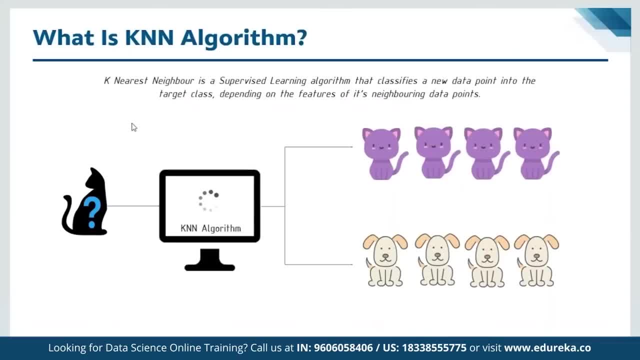 So, as we said, KNN algorithm is K nearest neighbors algorithm and it is an example of supervised learning algorithm where, basically, you try to classify a new data point based on the neighbors of that data point, which is basically which data points are closer to it. 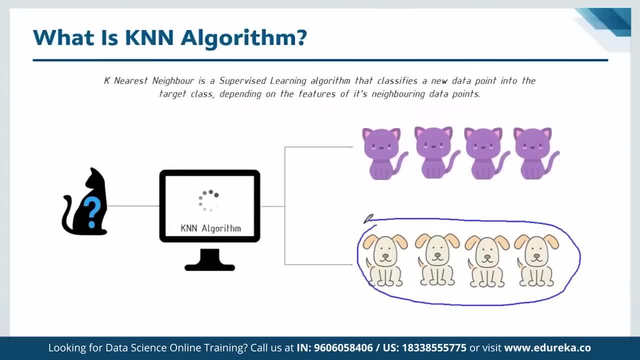 For example, here, as you can see, on one side you have dogs and on the other side you have cats. Right now, if a new data point is given to us, there is a picture of a new animal, and if it is lying somewhere here, right, then we know that it is nearer to the cats, right? 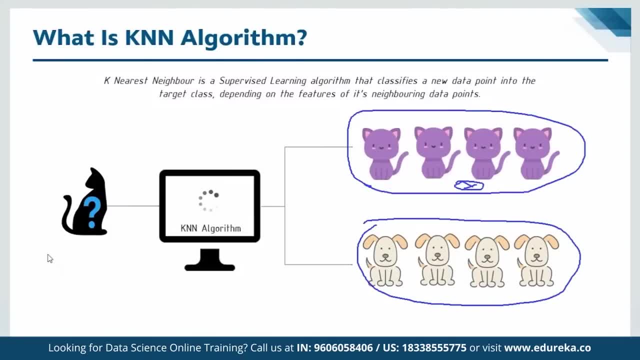 and therefore we will classify it as cat, whereas if it is sort of nearer to the dogs then we classify it as dog, right? So that's the like, you know neighborhood for the dog and therefore we sort of classified that new animal or the new 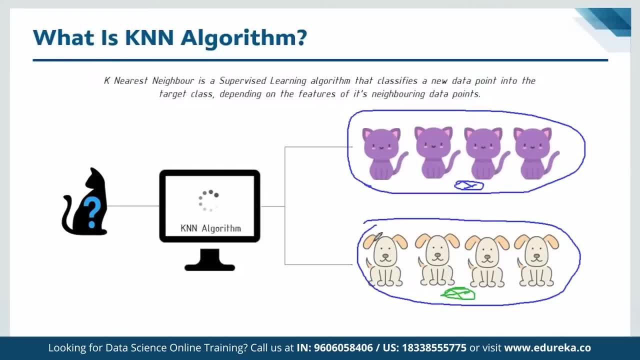 picture as as being or that of a dog, and this is quite, you know, this is something which is even seen our in our regular day-to-day life. right, You know, we have had examples where our parents keep telling us: Okay, don't play with those kinds of, you know, children or 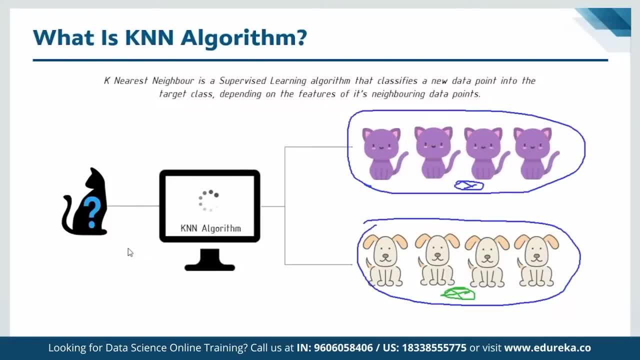 something because they are not good in their studies, or probably they are not so good in their behavior because you would become like them, right? So it's again an example from real life of classifying a particular person based on the company that they keep right, or from the 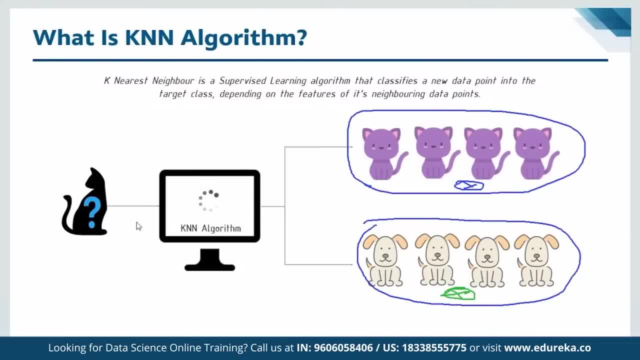 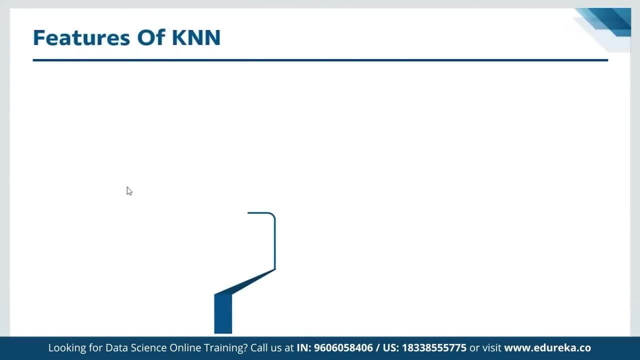 with the kind of people that they are. So that's, that's sort of the example. and now let me actually go back. Okay, What are the features of of K- nearest neighbors algorithm? Okay, So let's talk about the features of KNN. 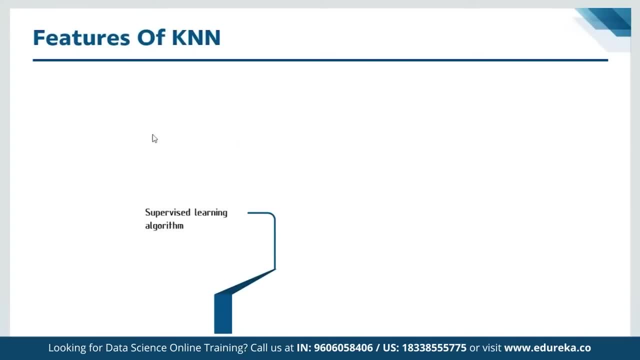 So, as I said, KNN is a supervised learning algorithm. Typically it is, you know, used for supervised learning kind of problems. It's very simple, as we mentioned: intuitively, you can, you know it's about. you know what kind of neighbors do you have, so your class is predicted. 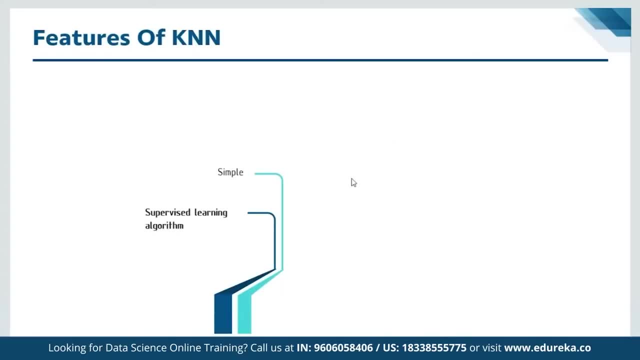 based on the your nearest neighbors, as the name suggests, and then it's a non-parametric technique. So I would like to spend a couple of minutes here to discuss about what we mean by by non-parametric. So typically, you know, the supervised machine learning algorithms are. 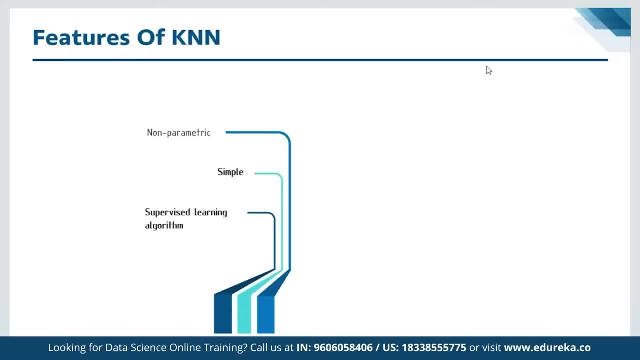 of two kinds right. one is the parametric types and the second one is the non-parametric type. when we say parametric, what we mean is basically that the machine or the algorithm assumes that there is an underlying function or a distribution that is known of the particular data set. 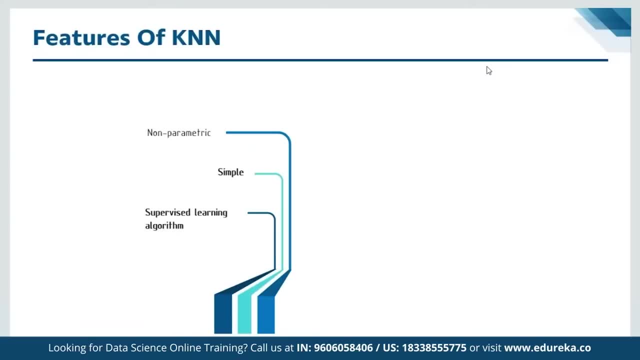 like, for example, the linear regression would assume that the relationship between two, two things- X and Y is- is linear in nature, right And and and. similarly, for a distribution, a Gaussian distribution, It would assume a normal distribution Of the data points, and so on. 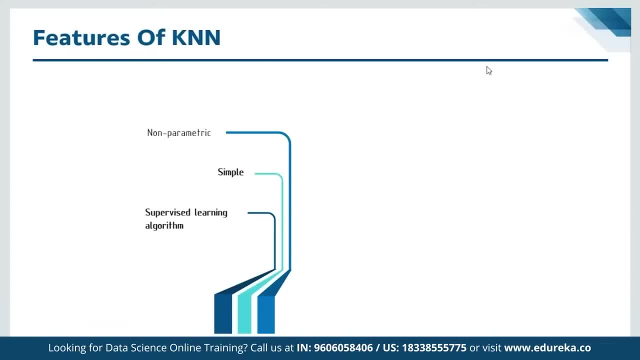 So a lot of the supervised machine learning algorithms, They assume some kind of function association between the predictor- which is basically the root causes which help you in predicting- and variable that you are trying to predict, whereas there are certain algorithms like the KNN or the person window or the linear discriminant analysis. 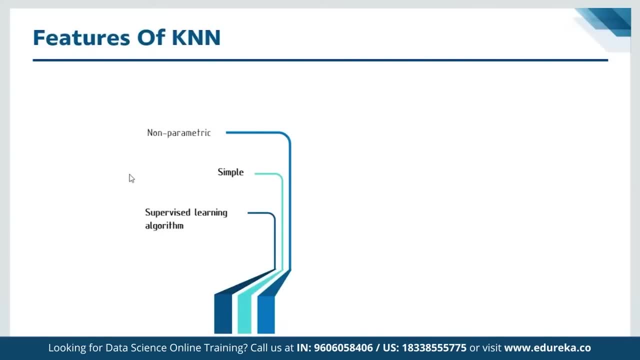 which is of the kind which is called non-parametric, because it does not assume any particular kind of distribution or any particular kind of functional relationship of the data that you are trying to- you know- predict, or you're trying to learn the pattern of. so KNN is one. 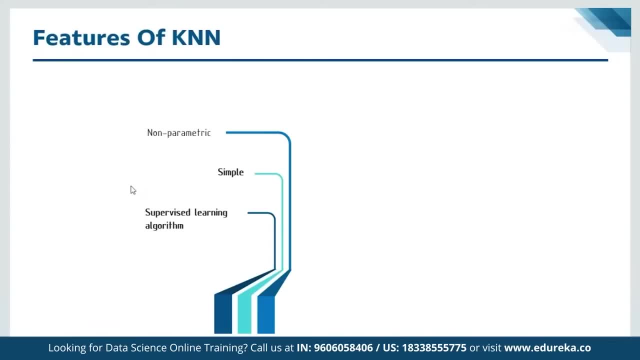 of the kind, as I said, Parson window is another one, which is basically where you, in Parson window, essentially you know the, the volume of the data set or the area that the data Set covers, is known, whereas you're trying to find the K there. 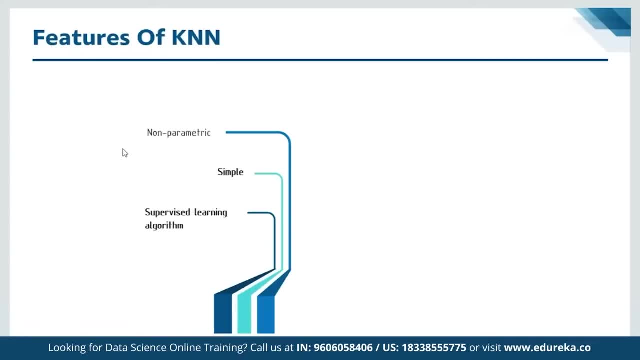 where which is the number of data points within that area or the volume right, whereas in case of non-parametric technique like KNN, it's the opposite. where the K is known, which is basically, you would like to associate the class of the data point that you are trying to predict based. 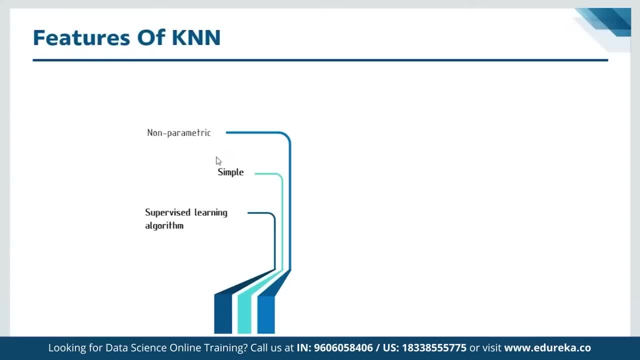 on the K number of neighbors around it. Now K can be three, four, five, whatever right, 10, 20 and so on. essentially, the difference between Parson window and KNN is that in KNN you already know the K and then from the K you try to find out the volume. 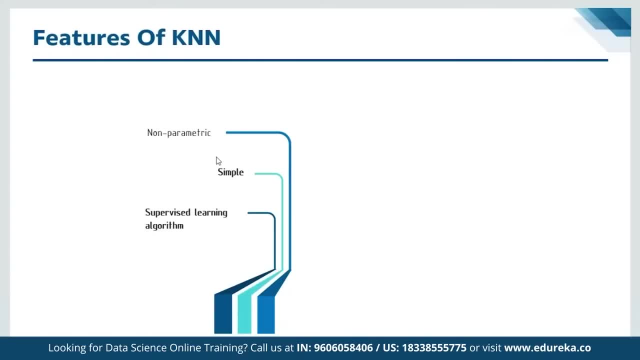 and therefore then you try to find the probability or the density underlying distribution. And then there is the, the discriminant analysis which is off, again two kinds: linear discriminant and multiple discriminant analysis, where basically what you do is you, you transform the underlying data, the features, 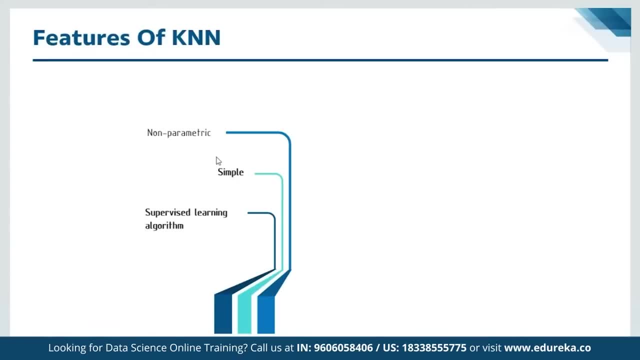 into a higher dimension and in such a way that in the new feature space, after you have transformed the data, you now try to apply a parametric approach. like, for example, you will try to project the features onto a line or, if it is on a subset, subspace. 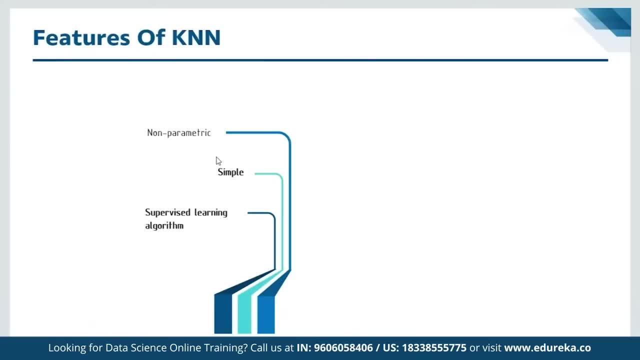 which is higher dimension than a line, then essentially it becomes multiple discriminant analysis. So basically, those are the three kinds of non-parametric techniques. So, even if you were not able to sort of get the full hang of what these three types are, what you need to keep in mind. 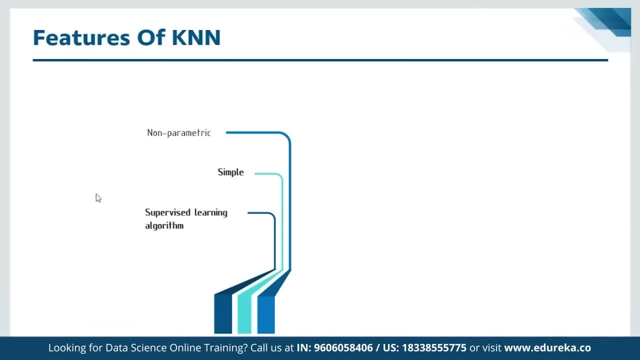 is that non-parametric technique does not assume any kind of distribution or any kind of functional relationship of the underlying data and therefore it gives us a lot of flexibility, whereas the parametric techniques, They basically assume some kind of functional relationship between the data points or they assume some kind. 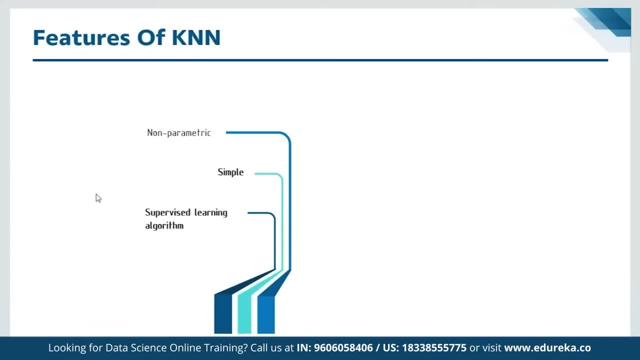 of distribution. So where would you use a non-parametric versus a parametric technique, right? So basically, you would use non-parametric technique. you know where you do not know about the functional relationship. that is one. second is that you know there is maybe, let's say, large amount of data and so on. 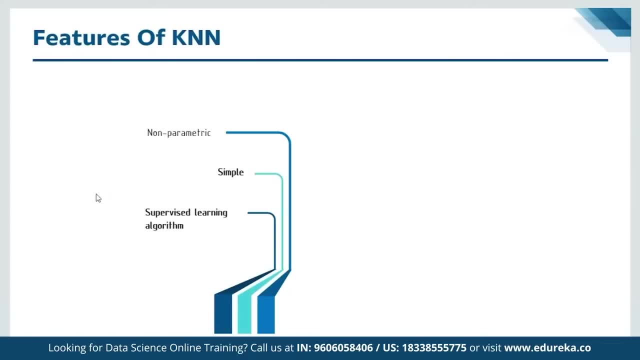 and thirdly, non-parametric technique, like KNN, does not work in very high dimensional data, So you would also use parametric techniques in that case, Whereas if you have, you know, smaller data sets, you would use, you know, typically non-parametric techniques, and then also 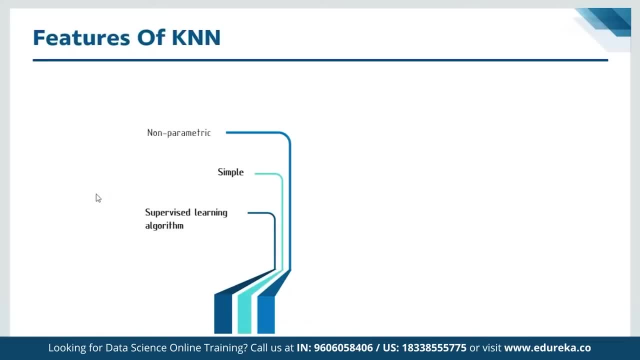 if you know, understand that the relationship between the data points might be, for example, linear or something like that, You would use a parametric technique. So you are assuming that there is some kind of relationship, like a linear relationship or something like that, and between the data point. 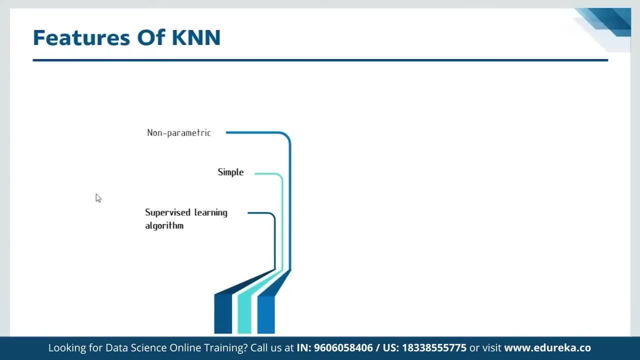 So that's where you will use the parametric technique. So again, just to summarize, basically, non-parametric is an approach where you do not assume any kind of distribution or functional relationship, whereas parametric assumes a functional relationship or basically a distribution between the data points. 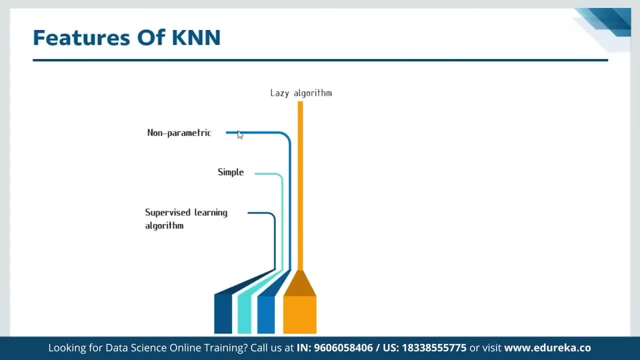 The other feature of Canon is that it is a lazy algorithm. So what do we mean by lazy algorithm? actually, in most of the supervised learning algorithms, you basically train your model on the training data set, Then you have your model And then you apply this particular model. 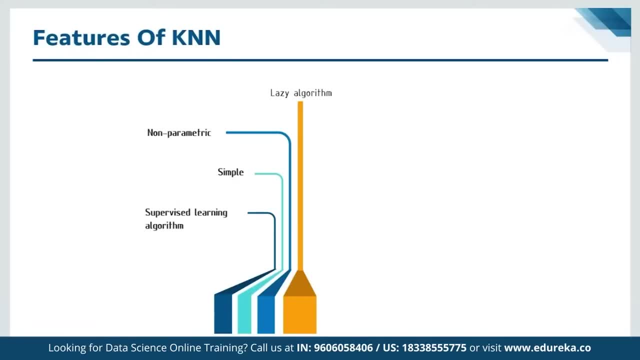 to the test data set to then classify or predict. you know, for example, whether a new image is that of a cat or a dog, right? So this can be. you know some kind of algorithm like support vector machine or regression or logistic regression or whatever, right? 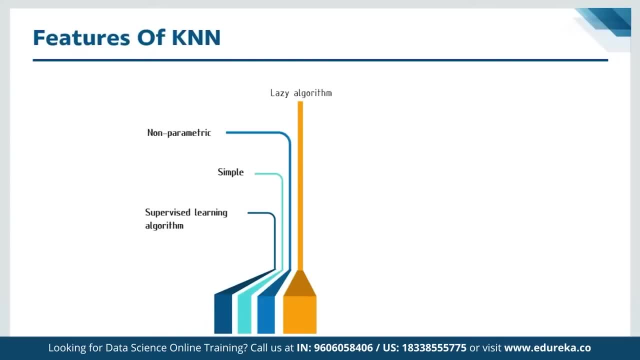 So you run this logistic regression or you run this regression or support vector machine on the training data set and it learns the features or it learns the parameters Of the model from that data set and then applies this learnt model on the test data set, Whereas in case of Canon, actually 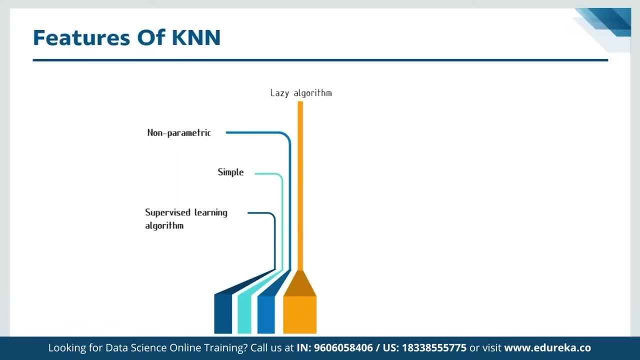 there is no training step at all. That's why it's called a lazy algorithm, because what it does is at the time that you are actually now want to predict. at that point in time, actually, it will go and it will do all the calculations of the distance. 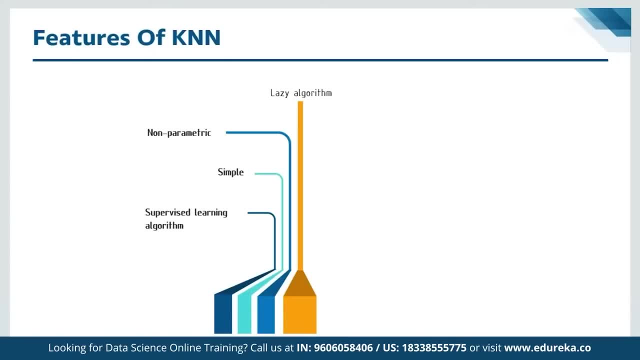 of the new data point, Like, for example, the new image of the cat or dog from all the other data points that you have. so it will calculate all the distances and then we'll check for the those data points which are, or the K data points which are nearest to this. 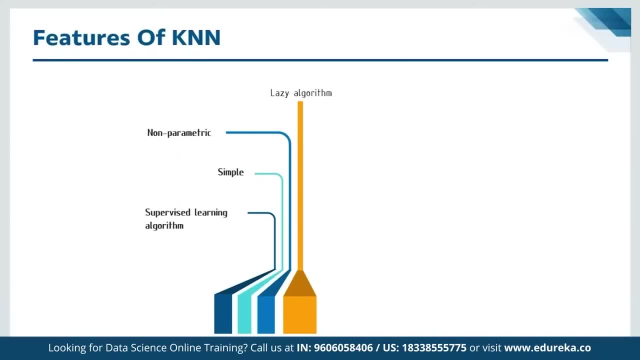 So that's why it's called lazy algorithm, because nothing happens till the point, or no calculations happen till the point. You are actually trying to predict something. So there is no training step involved, Okay, and then it's used for both classification and regression. 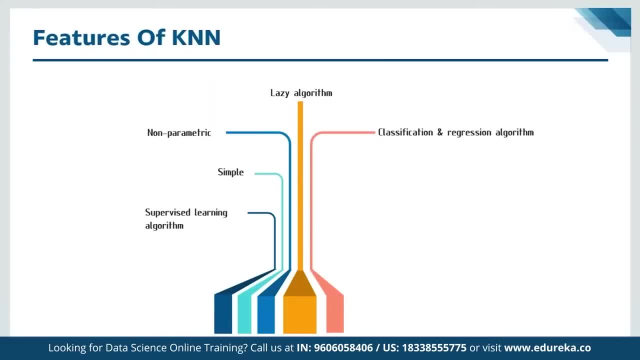 as we just mentioned. So it can be used to predict the values as well as be able to classify something like you know, okay, whether it is a cat or dog, or if you're trying to, let's say, predict some value, some forecast or something that for that also you can use it. 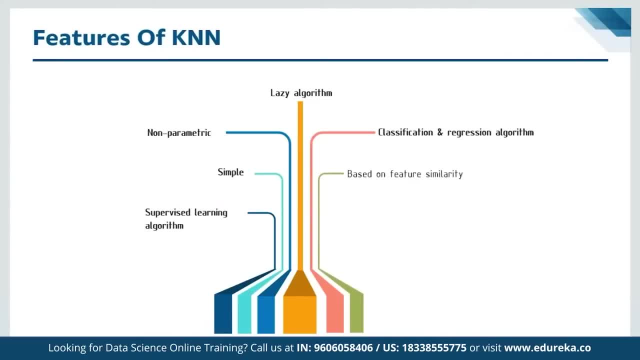 and then it is based on feature similarity, which is basically what do we mean by feature similarity. So feature can be things like: if, for example, you know you are looking at classifying cats versus dog, right, So is the eyes like a dog. 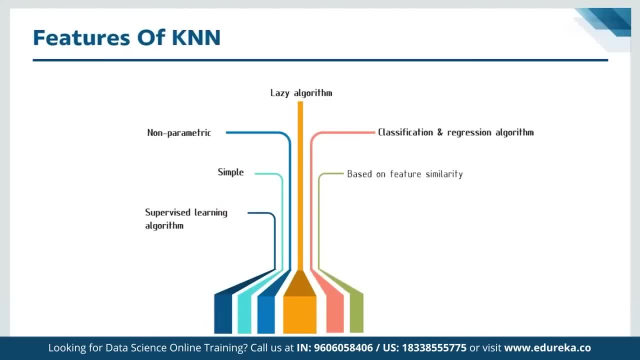 That can be one of the features. is the war? How do the ears look? that can be one of the features. What about the tongue, the face and so on? so there can be multiple such features and how similar it these features are between two data points. 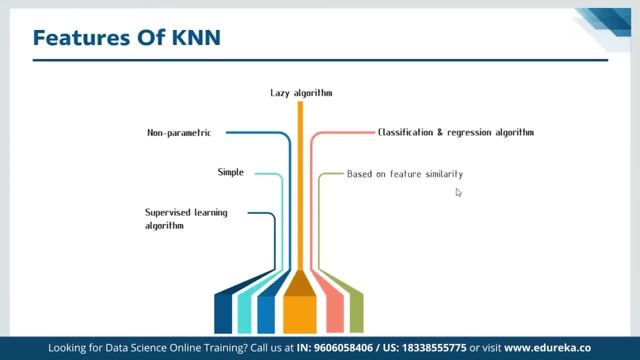 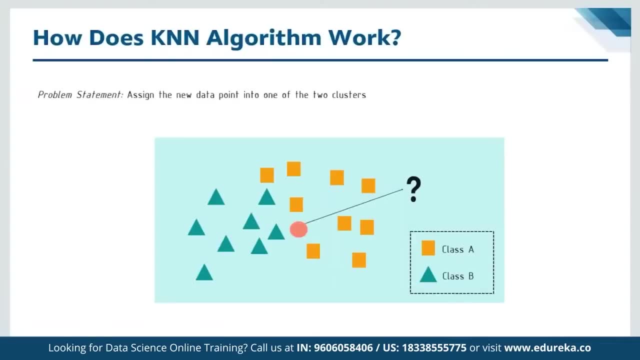 which is used basically by the K and an algorithm, and then, as I said, there is no training step involved. So these are the features of K and an algorithm and therefore now let's look at actually just some simple examples of how it works. So, as you can see here in this slide, 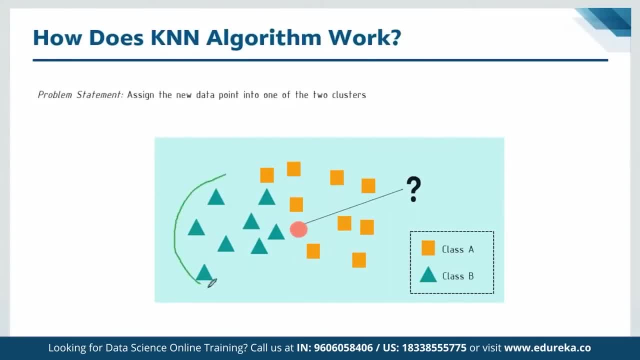 we have two classes of data. So one is the all this blue data points, and there is another one which is the orange data points. Now, if you have a new data point, which is this pink one here, which class should it belong to? should it belong to class a? 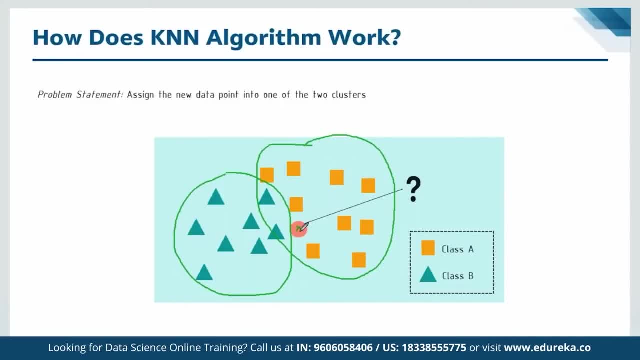 or should it belong to class B? So what you would do is you would actually start calculating the distance of this pink data point from every square or blue triangle data point, and then you will decide. you will have to assume a particular K. Let's say K is 3, right? 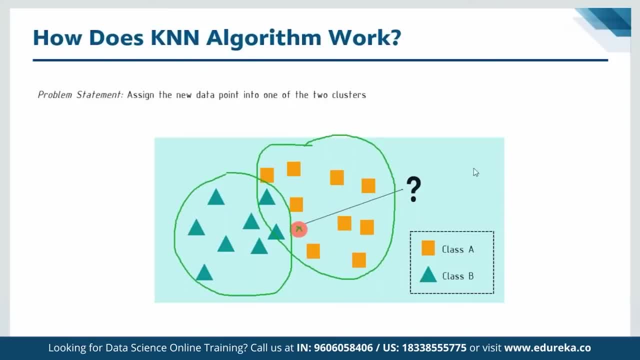 which is I'm looking at the nearest three data points and in that case, basically, as you can see, if we draw this circle right, then we see that two of the nearest data points within that circle is of the square orange Kind. So basically, we will predict. 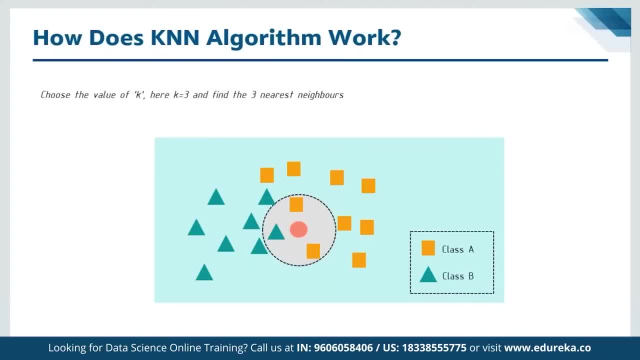 that this particular new data point belongs to class A, whereas K value was 7, right as in this particular example. Now you would see that 4 out of the 7 is actually of the blue triangle kind, and therefore we will now classify it as belonging to class B. 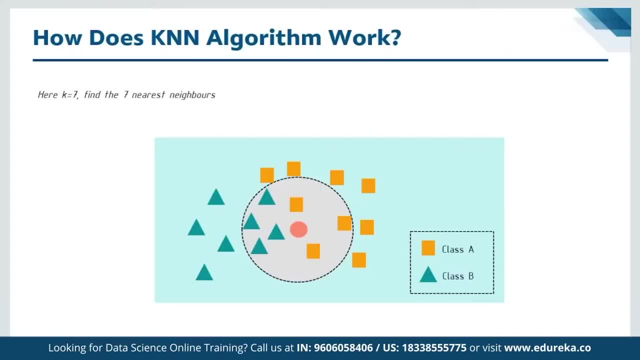 So, essentially, this prediction changes, as you can see here, depending on what is the K value. So therefore, the question is: what should be the value of K? right? And typically what happens is you run a trial and error and basically you come up with: okay. 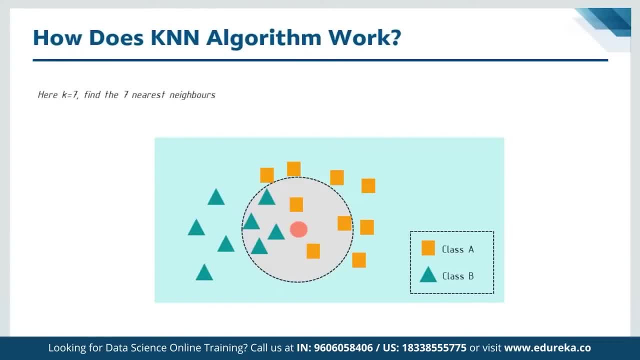 What is the best K value? But essentially, what one needs to understand is that as the value of K increases, basically the partition line starts moving towards becoming more and more linear, So it starts becoming less flexible and it starts assuming some kind of a linear dividing line. 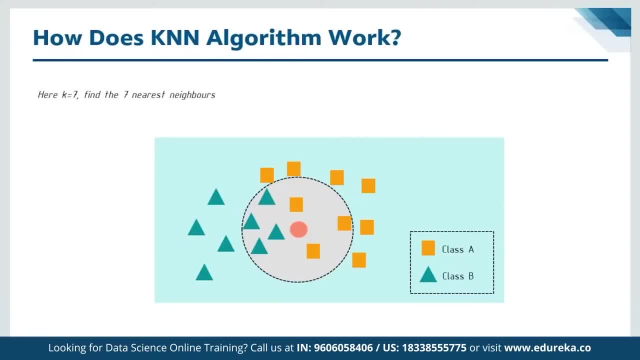 or something like that. So What happens is that in that as you increase the K, your bias basically increases, but your variation reduces. So we know that in classification problems or in machine learning problems, bias and variance are two things that we are trying to manage right. bias is basically how close you are. 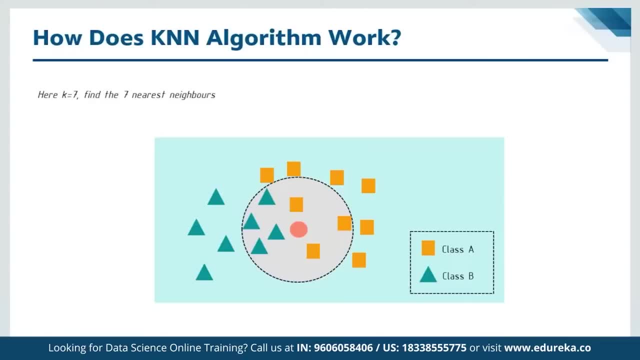 to the actual class or how, or to the actual value, Whereas variation is: how much variability Is there in your prediction? So as the K increases, the bias sort of increases, but the variance reduces, and then it is vice versa. So if your K decreases, 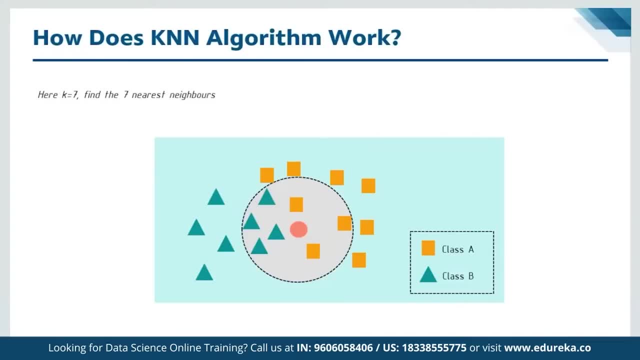 let's say at, K is equal to 1, where you are only looking at just one nearest neighbor and then predicting based on that. actually, the bias is the least, which means it is the most flexible. K is going to. one is the will give you the most flexible sort. 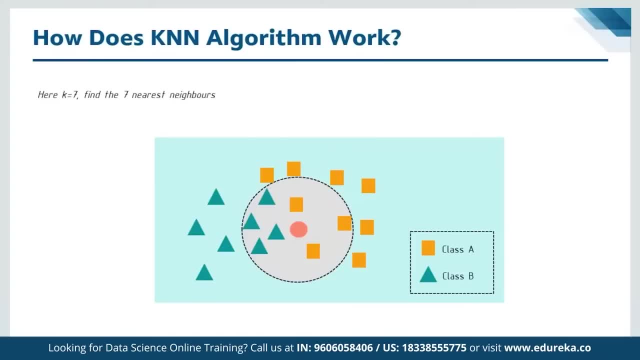 of demarketing line or function, Whereas the variability will be the maximum. so that that's the sort of the trade-off And that's how we actually determine K. So we have to get a K value in such a way, based on trial and error, that sort of maximizes our sort of or reduces the bias as well as the variance. 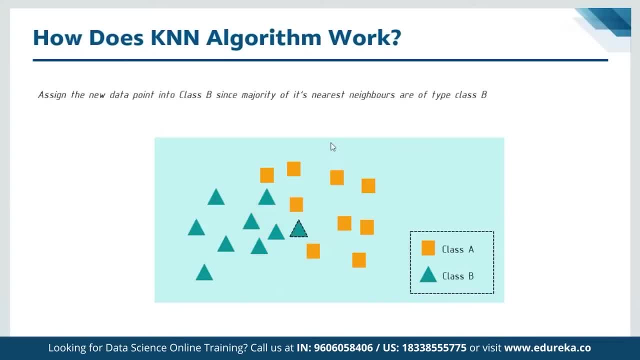 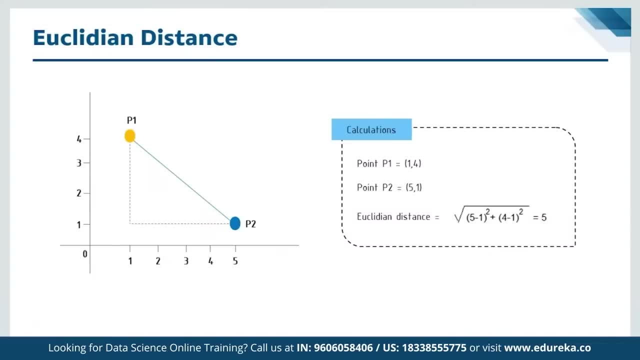 and, and that's the kind of optimization we are trying to do. Okay, So how do we calculate the distance itself? Right, and distance typically can be of many kinds. So you know, the example here is of the Euclidean distance, but you can have other kinds of distances, like Manhattan distance. 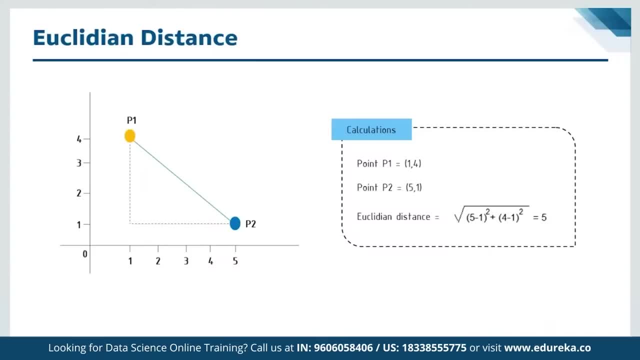 or Mahalan obese distance, and you can look up references for other kinds of distances. Now Euclidean distance is calculated for the point P 1 and P 2 as given here. essentially Euclidean distance is nothing but the, you know, square root of sum of the x coordinates of these two points, P 1 and P 2. 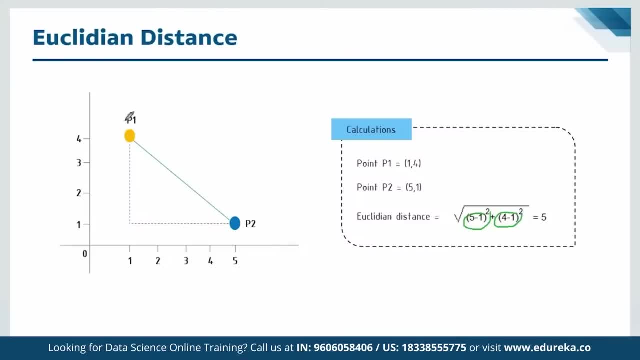 and then y coordinate square of Of these two points, P 1 and P 2, and this is just an example of one kind of distance, and other kinds of distances, like Manhattan or Mahalan obese, are also there, and then this calculating this distance becomes quite challenging. 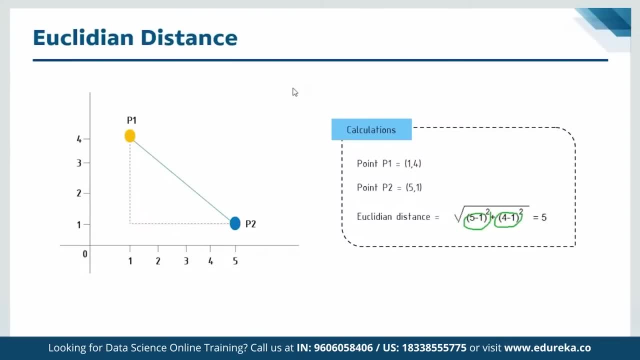 especially in cases where you know you are trying to, for example, calculate, let's say, how close to LinkedIn profiles are right, or trying to classify the category of electrocardiogram, and so on, so forth. So there, we have to bring in more creativity to just decide what kind of distance to use. 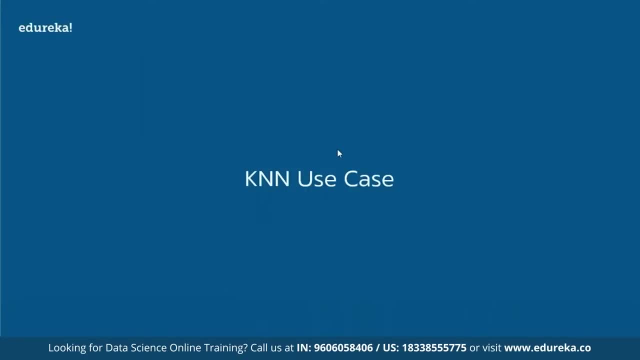 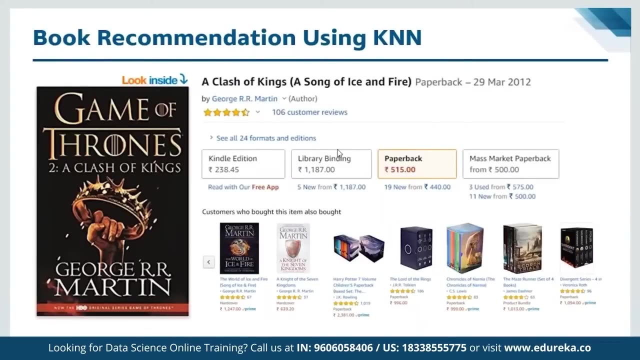 Okay, Now let's move ahead. We will now talk of some use cases where Canon can be used, and this is an example of how Canon can be used for book recommendation. So if you have purchased books on Amazon or wherever right, some of these recommendations are based on on Canon algorithm. 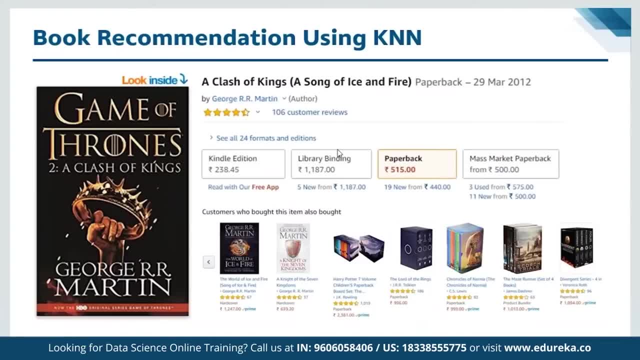 and then you know, as we said, you know, Canon is like based on features, right? So maybe let's say what will be the nearest neighbor. So a particular book it can be based on: who is the author, What is the topic, and so on, so forth. 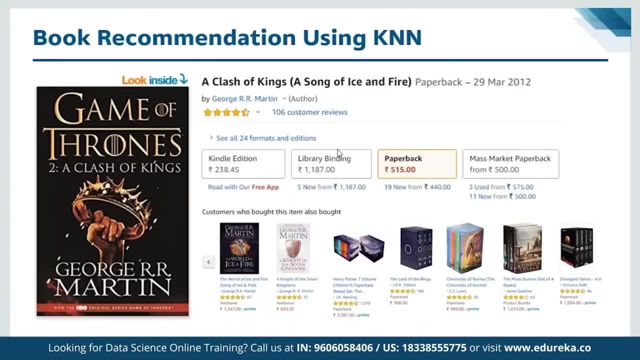 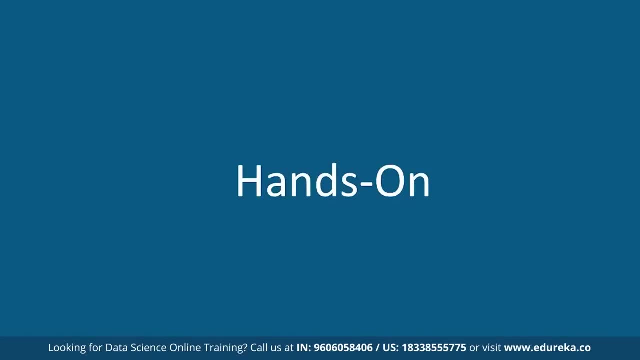 And then there are other use cases, like I mentioned. So for classifying satellite images, for classifying handwritten digits on image analytics, or for classifying electrocardiograms, Etc. You know, typically Canon can be used, Okay, So now actually we will get into some hands-on. 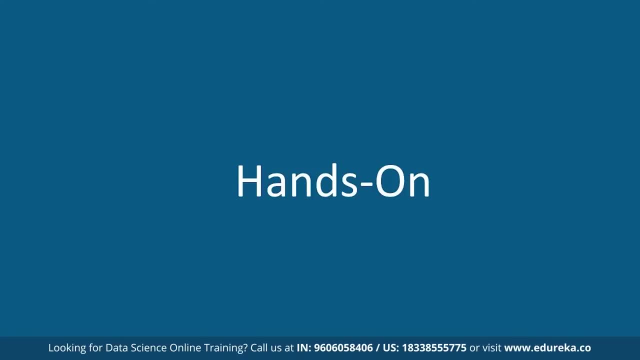 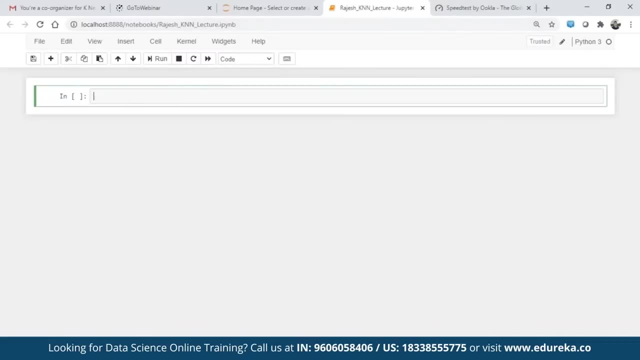 Okay, So to start the hands-on session, I'll go to this Jupiter notebook that I already have installed on my system and I have a certain code written, which we will take two examples. Both the examples are based on data sets which are available in the open source. 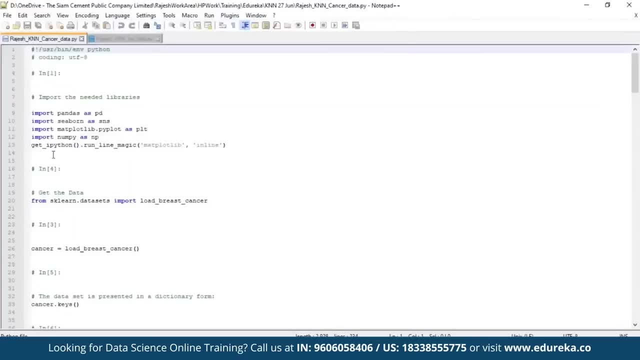 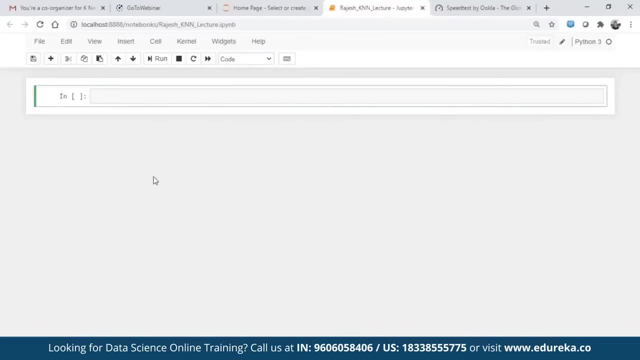 So you can easily get access to that data. So what we do is we start by importing the necessary libraries. so we import pandas, seaborn, numpy and matplotlib. basically, pandas and numpy are there for doing the data manipulation and also for storing data as matrices or as arrays. 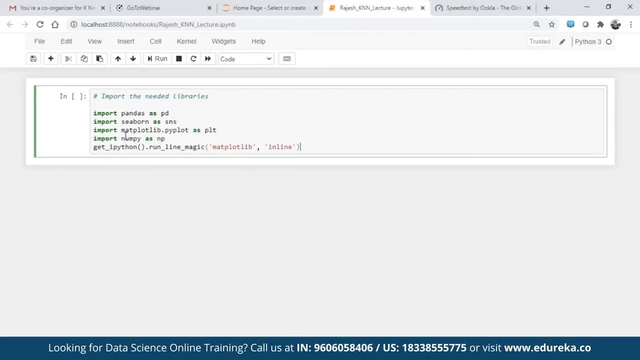 and and be able to perform some mathematical procedures on them. and then seaborn is basically used for plotting and matplotlib for plotting as well, And this line here get ipython just helps us to run the images That will be creating in line with Jupiter notebook, instead of opening up a new window. 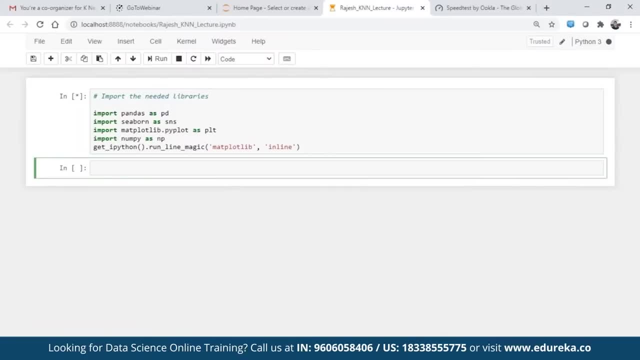 So let's run this, and what it will do is it will import all these packages for us which we are going to use, and then we will first import the breast cancer data There is available in your scikit-learn data sets. So we import that. 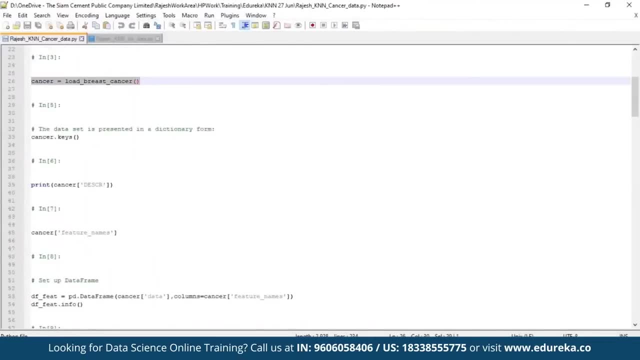 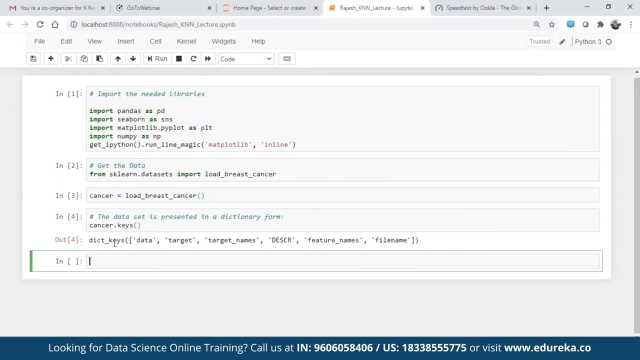 and then let's just initialize that data into a variable here called cancer. So cancer here represents all the load, the breast cancer data. And now we will. let's actually look at what this data is. It's a bunch of attributes in this dictionary here. 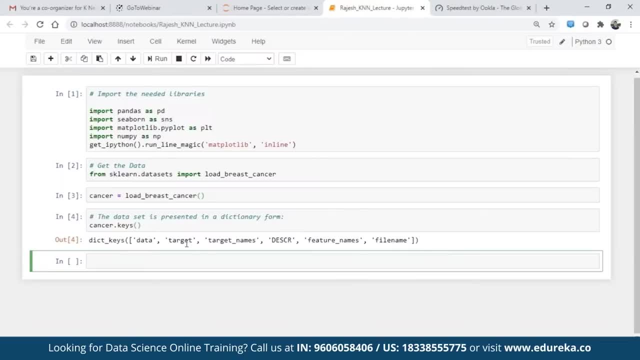 So you have data, the Target, which is basically nothing, but whether it is a cancer or not. So, whether it is malignant or benign, malignant means it's a bad cancer and benign means, well, it's just a tumor, It's not cancerous. Target's name description- feature names. 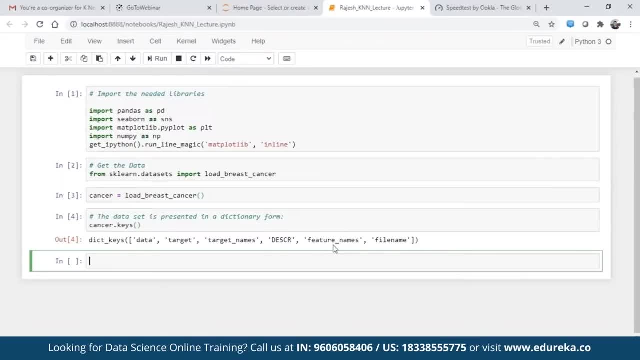 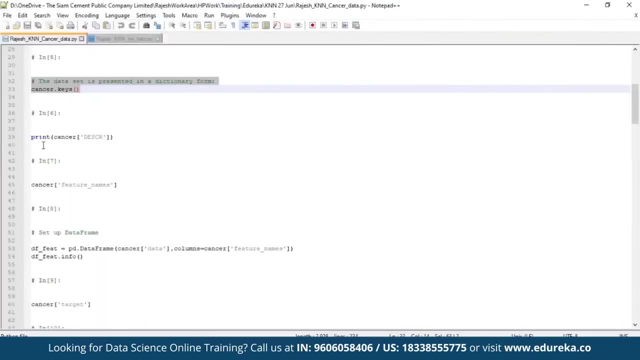 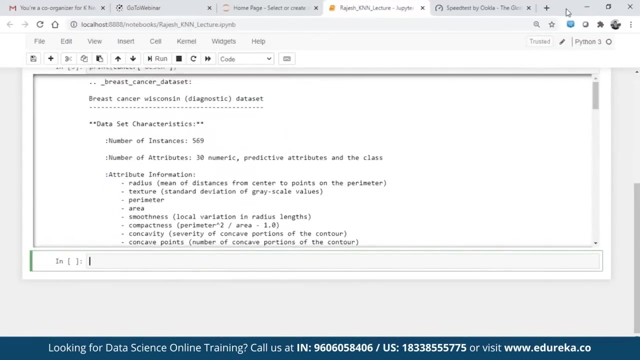 which is basically The features that will tell us whether a particular case belongs to cancerous or non-cancer, or malignant or benign, And then, actually, let's just print the description of this particular data here, So, as you can see, we can use this command. 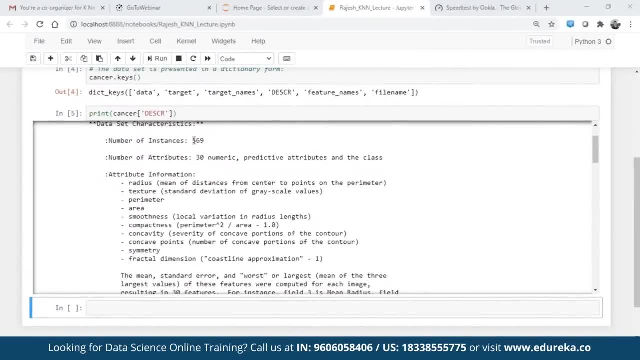 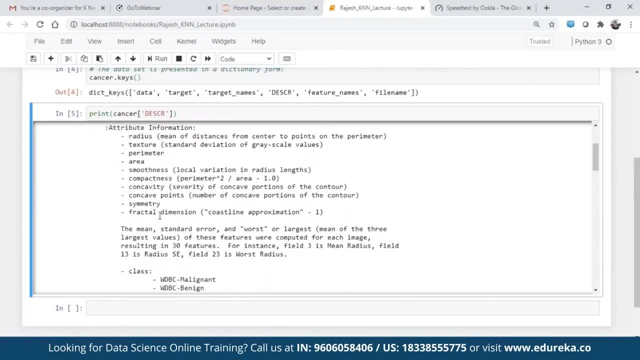 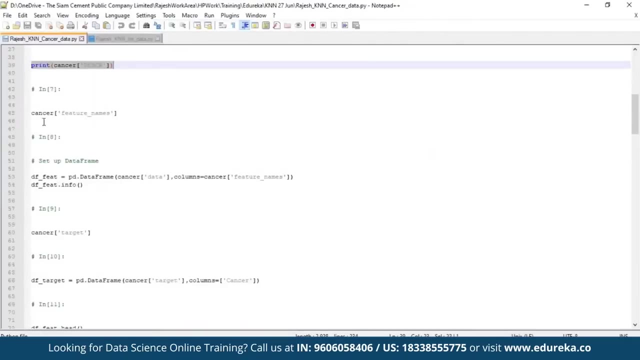 to print the description here. and then we see that there are 569 data points with about 30 attributes, and these attributes are radius, texture, parameter, Etc, and the max and min values of those are given here. And then now let's look at some of the feature names. 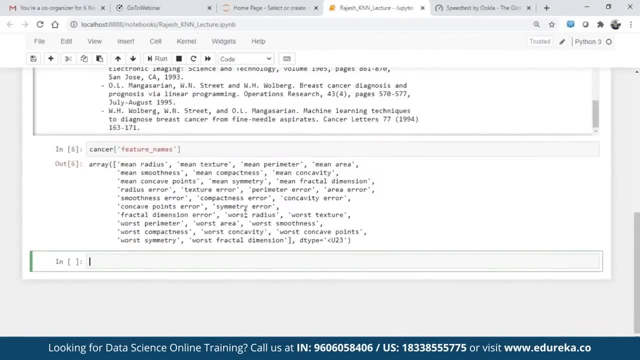 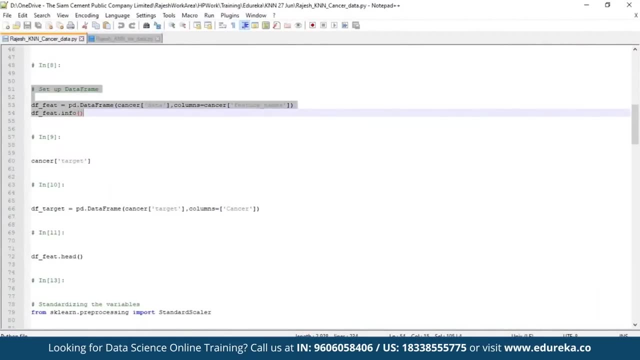 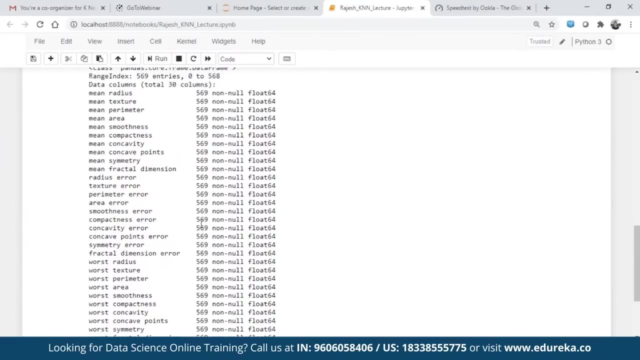 So these are the feature names: radius, texture and so on- And now let's actually set up a data frame of this particular data here, Using pandas, this function here. So there are 569 data points, And all these are basically your features, as we talked about. 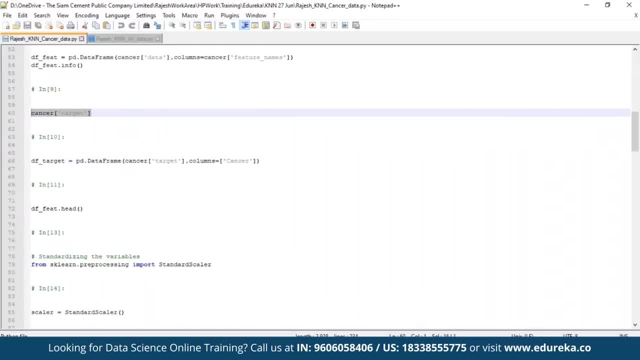 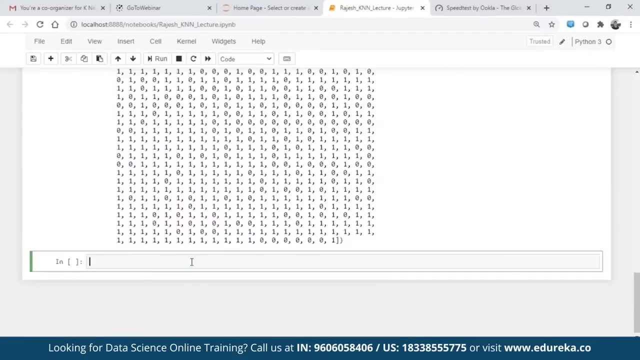 And let's look at the Target variable, which is nothing but whether it is telling us whether a particular data point belongs to malignant or benign. So 0 is cancerous and one is non-cancerous. And then we convert the Target into a data frame as well. 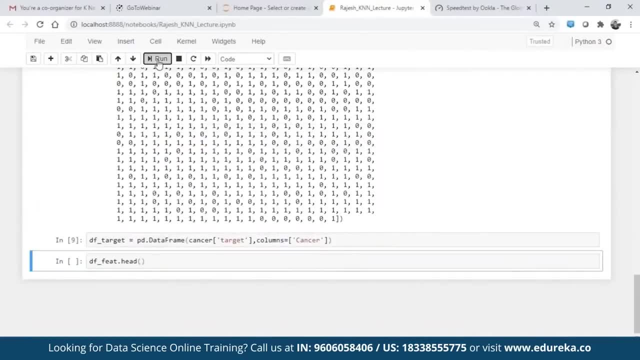 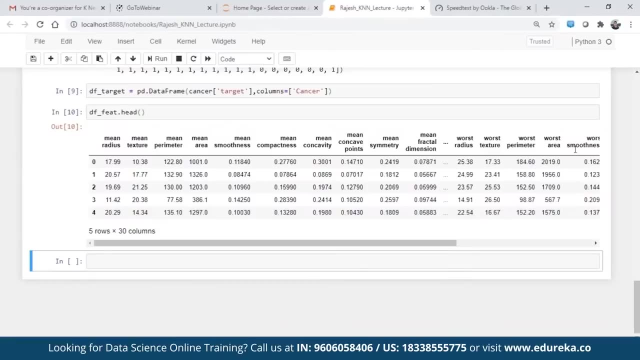 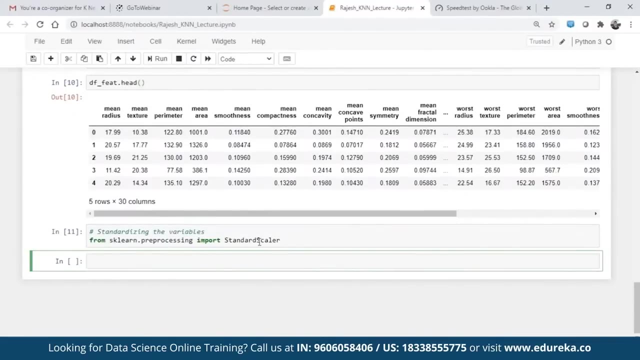 And then let's look at the couple of examples of how the data points look like. This is, you know, one row of the data points which, with all the several feature values that we have. So, basically, we use this package called standard scalar from scikit-learn for pre-processing. 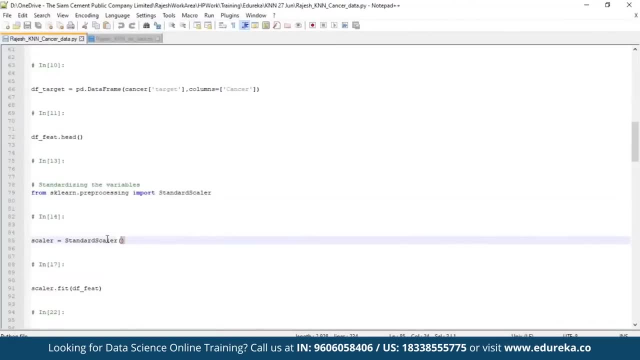 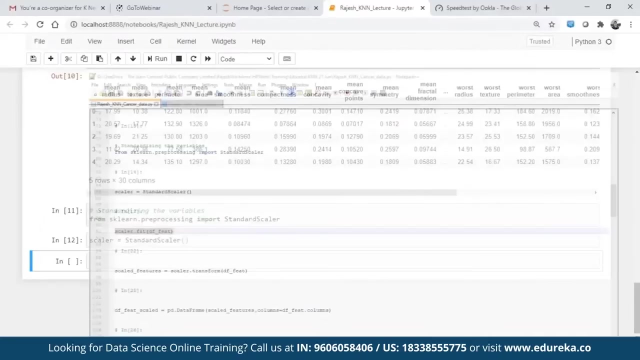 and for standardizing the variables, and we initialize this standard scalar into a variable called scalar. So standardizing is nothing but, you know, basically bringing all the samples to essentially the same Range, right? Because what might happen is some of the data point. 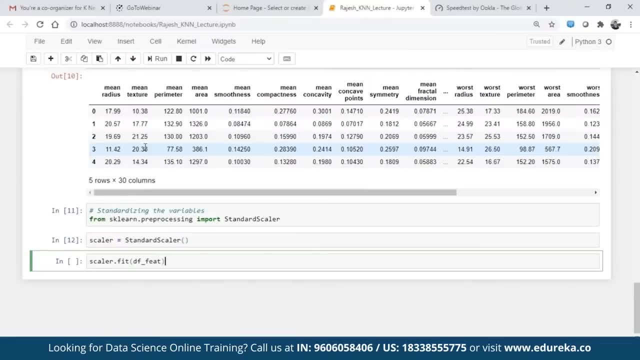 like, for example, temperature might be from 0 to 100 and some price might be from, let's say, thousand to a hundred thousand or whatever right. So the absolute values can can lead to some issues with respect to the prediction. Therefore we have to standardize it. 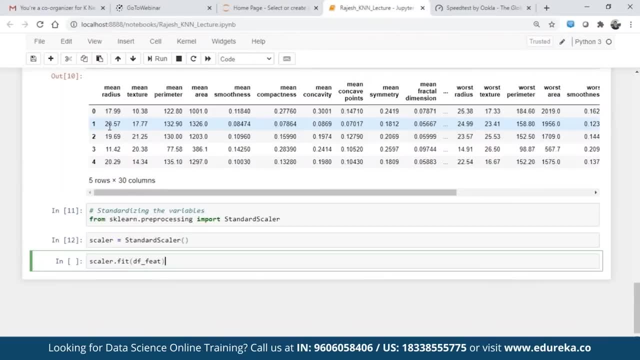 or bring it between, let's say, minus 1 and 1.. So, and then a mean of 0, right? So we have to bring everything to the same scale to be able to compare the samples. So we, first of all, we fit the this standardization. 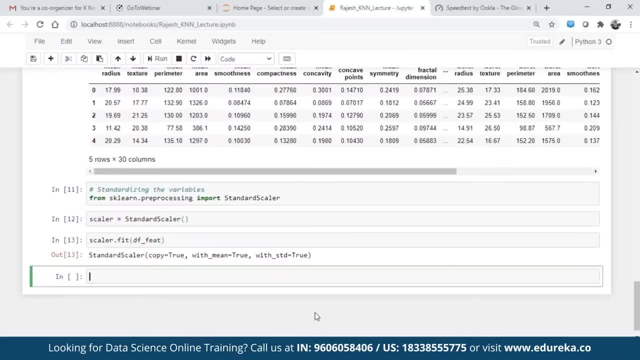 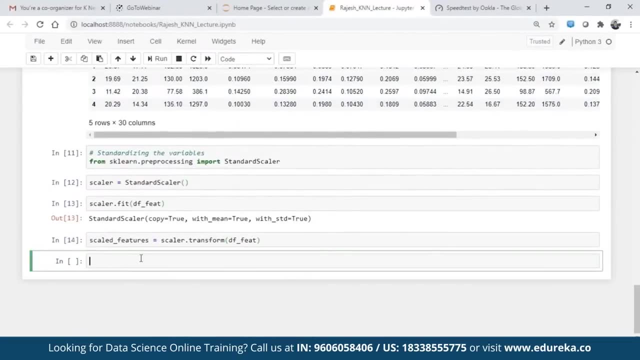 or normalization on the data set we have. and that is, we calculate the variance and and the means and then we actually apply it on the data set to transform it to the actual values, And then if we look at the scale values now. so let's look at the scale values. 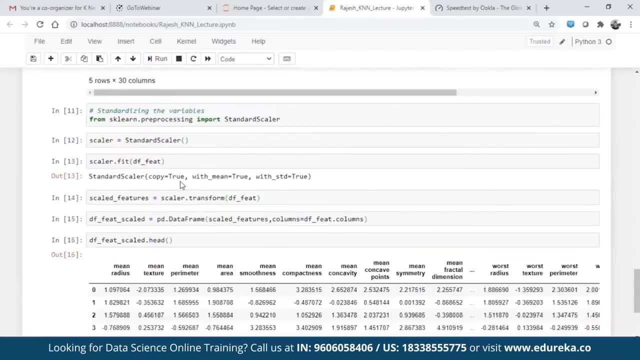 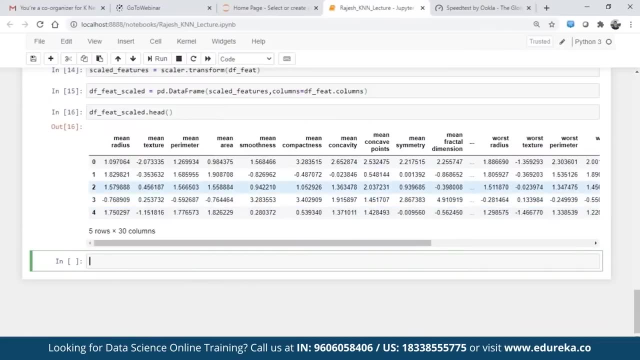 And this will give an example of the top five rows Here. so we can see now the values are between minus 1 and 1, or rather it is standardized essentially with the normal distribution, and then we divide this data into test and train. So basically we will train the model. 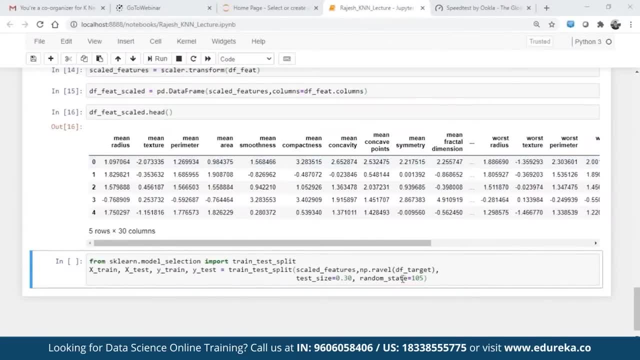 and then we will test it on a separate data set. If you use the same random state, you should be able to get the same result. Otherwise, you may get a different result here, and essentially we are keeping the testing size at 30, which means that we are dividing the entire data set. 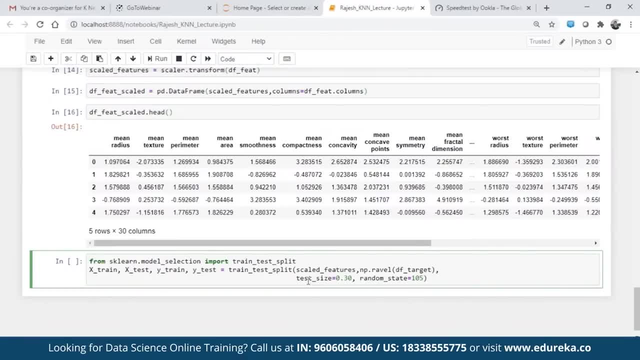 into two parts: the train part, which is having 70% of the data, and the test part, which is having 30% of the data. And again we are using this package called train test, split from the scikit-learn package. So we get the X and the Y's, which are basically nothing. 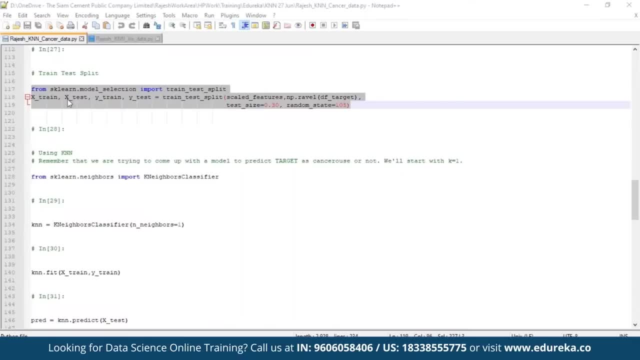 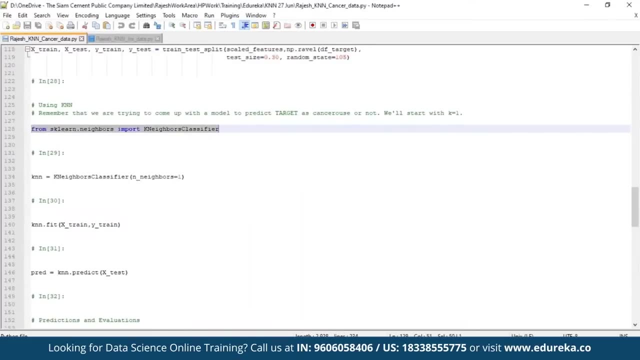 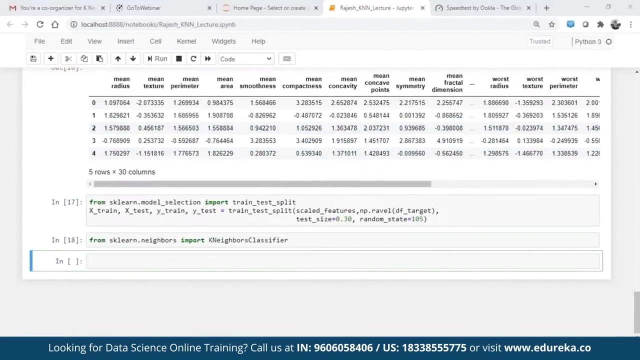 but your train and the X's are your predictors and Y is your predicted variable, whether it is cancerous or not. and then now let's import the K nearest neighbors classifier. This is that, the actual algorithm which we are importing from scikit-learn package. 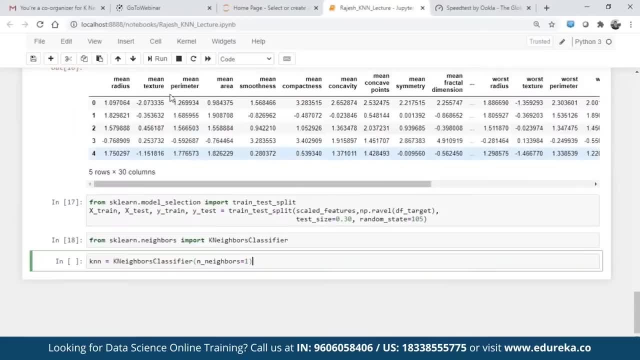 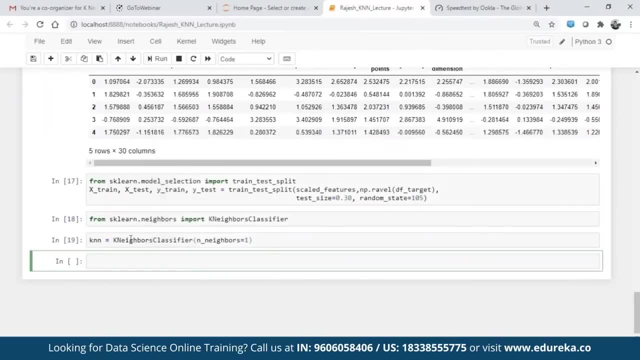 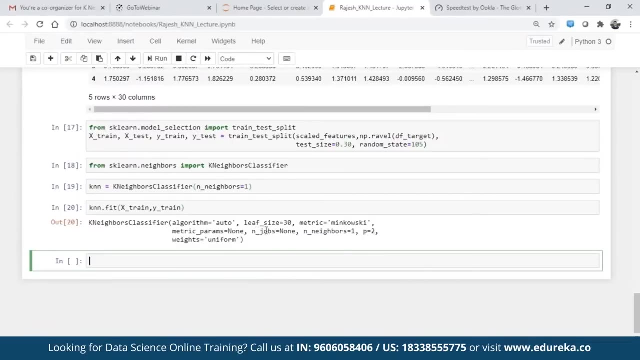 and now we initialize this particular algorithm and then we fit it on the data And some of the parameters, as you can see, is basically: what is the leaf size, and so on, so forth. the nearest and neighbors we are taking, So we are taking K is equal to 1 here, basically. 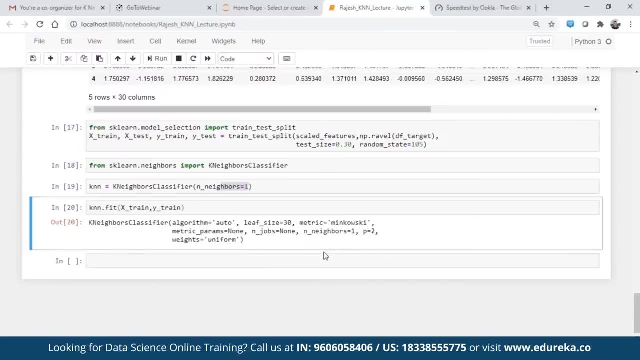 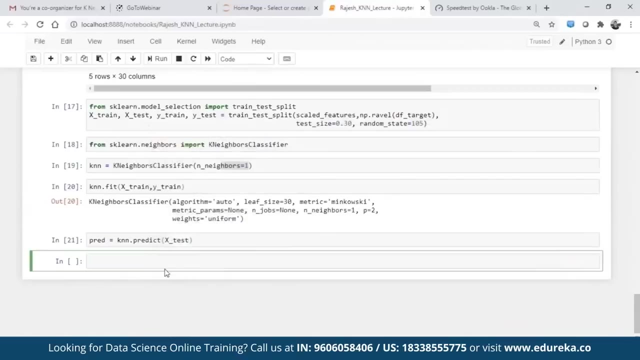 as of now. we will see the results based on that and then we will change it and see how the results vary. And we now run it on the bit, now try to predict it And then we will now try to evaluate what the results look like. 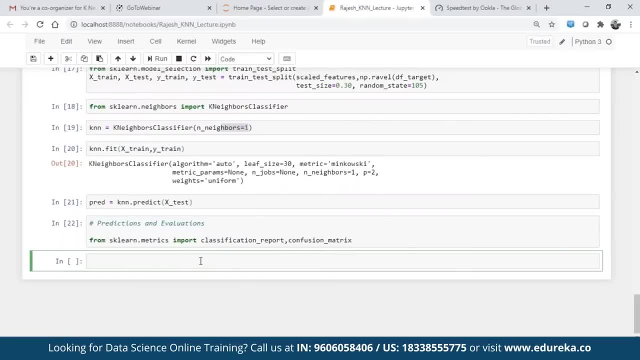 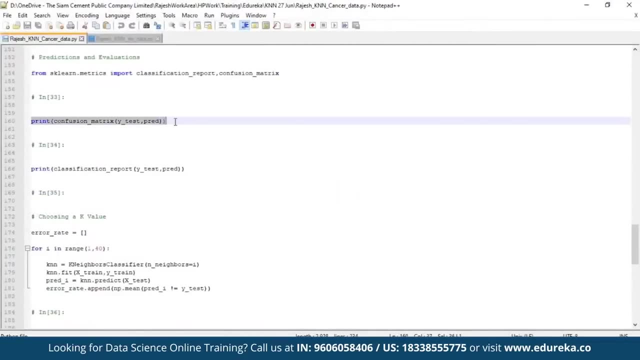 So we have imported the classification report and confusion Matrix, which is basically trying to see whether we were able to correctly classify The cancerous as cancerous and non-cancerous is, non-cancerous is or not. So we can see that this is the actual. 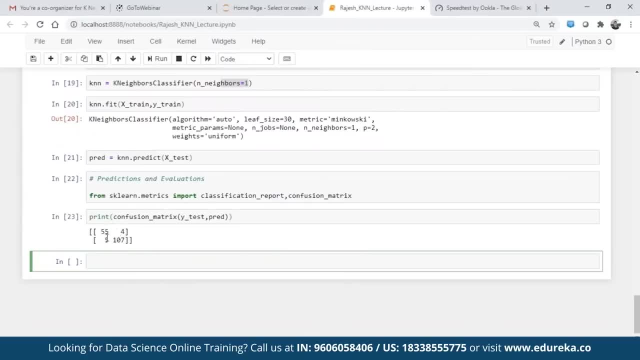 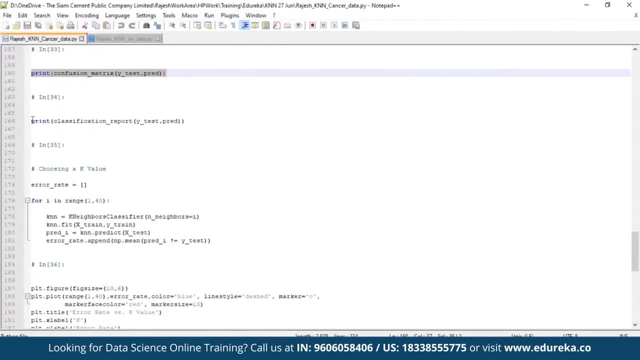 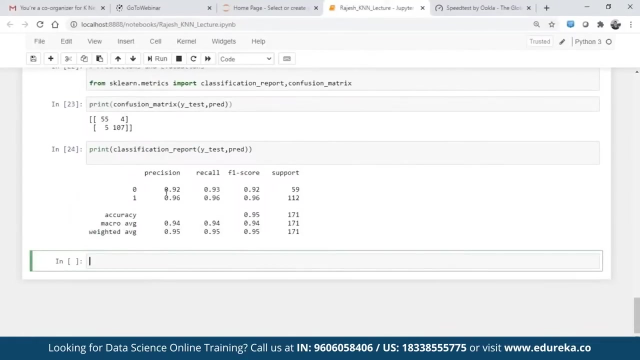 and this is the predicted. So basically, some data points here- 5 and 4- are classified wrongly, Otherwise all the others are classified well. So if we look at the accuracy- calculated accuracy actually- so we see that the precision which is true, alarm. 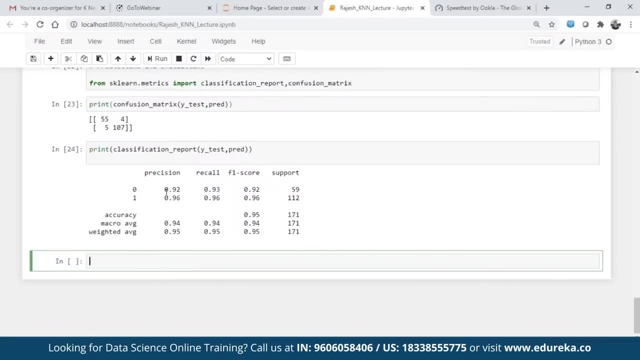 right, which is basically from the cancerous samples. How many were you able to To actually predict as cancerous? if you see, the accuracy is quite high: almost 94, 95%. and then the recall, which is from all of the cancerous samples. 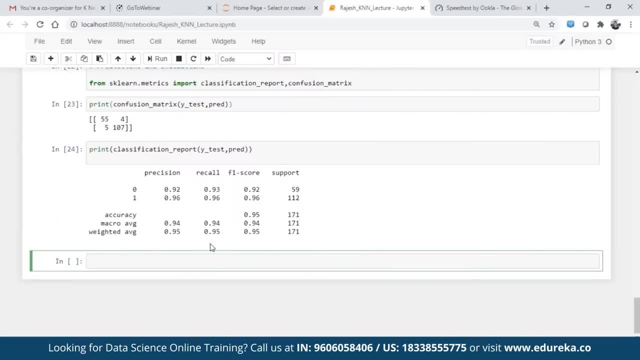 How many were you able to actually predict accurately is about again 94, 95%, and f1 score is nothing but a combination of both precision as well as recall, and that's quite good as well. So with K is equal to 1, you are able. 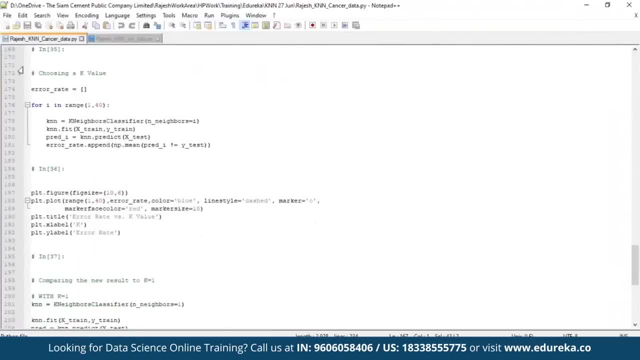 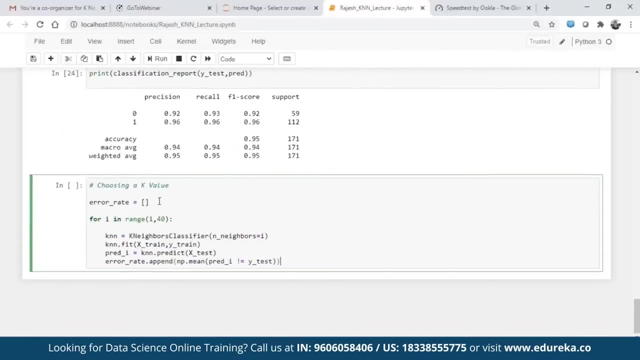 to get some- already some- good results. Now let's try to see how to choose the K value right. So this is basically nothing but a bunch of code that actually runs the K value from 1 to 40 and then tries to check the accuracy. 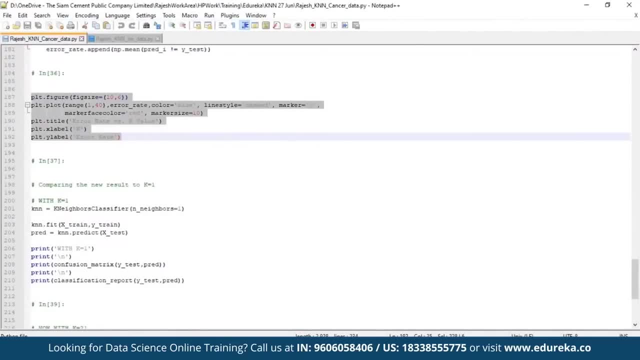 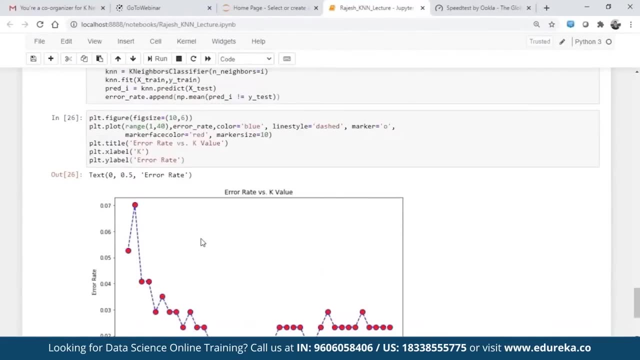 And this is just like doing a trial and error to see where we get the best results so that we can then use the best K value. So if you can see this particular plot here, after we plot the result from the running the trial and error from 1 to 40, we see: 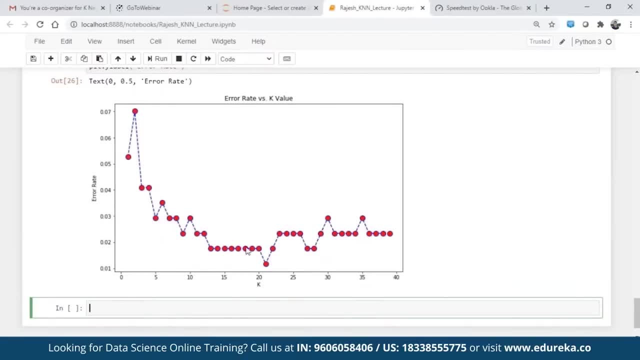 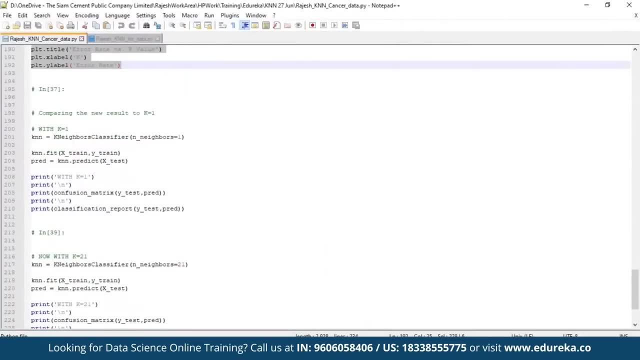 that the error actually starts decreasing. and somewhere around this K is equal to 21. we get the minimum value of error. So for us, the best K value is 21.. So now, if we compare the results between, K is equal to 1 and K is equal to 21,. 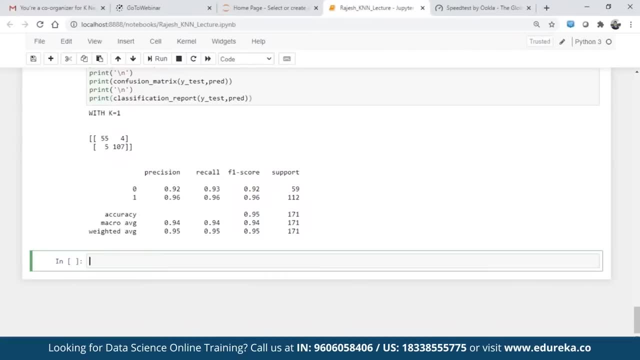 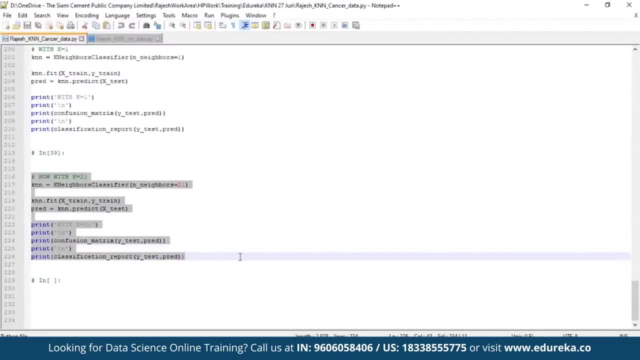 we should be able to see the prediction results. So, as you can say, this was the result: with K is equal to 1, which is we get about 94- 95% accuracy, and then with K is equal to 21.. We will see whether the accuracy improves, right. 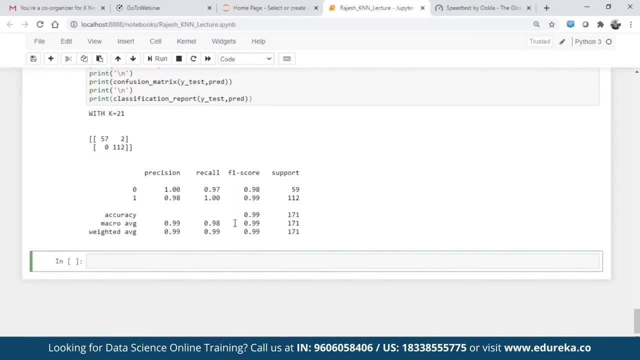 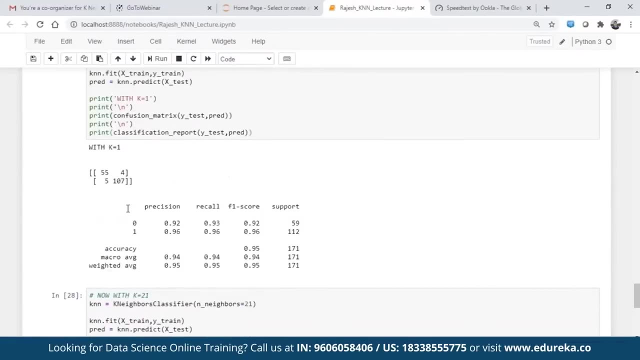 So we see that, yes, the accuracy has now gone up to almost 99%, which is we earlier had nine misclassified data points out of all of the points, and then here we have just two data points which are misclassified from the test data set. 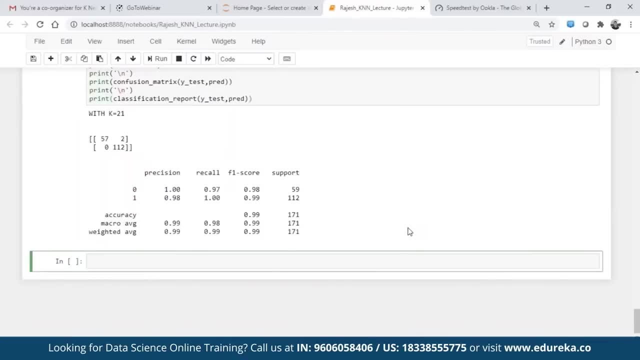 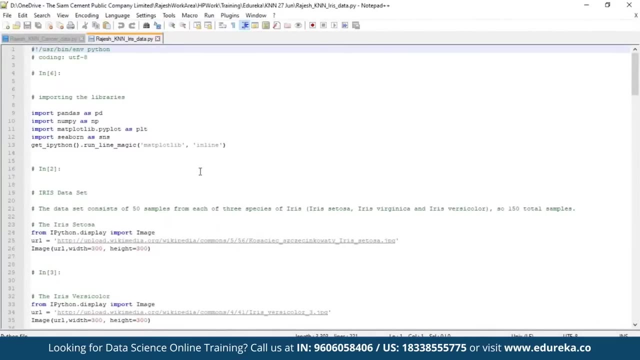 So now, this was one example of applying K and N on the cancer data set, which is available freely, And now let's look at another example, which is the iris data set, and again available freely as well. So iris is a type of flower and we will see. 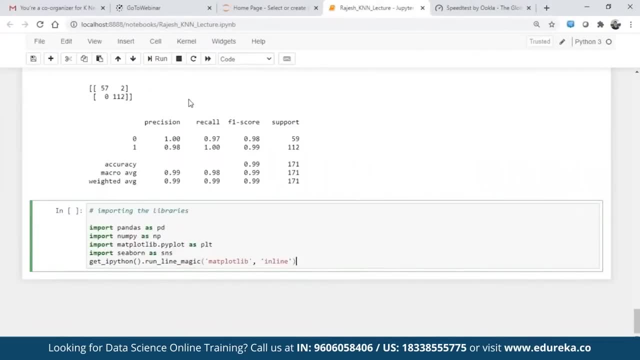 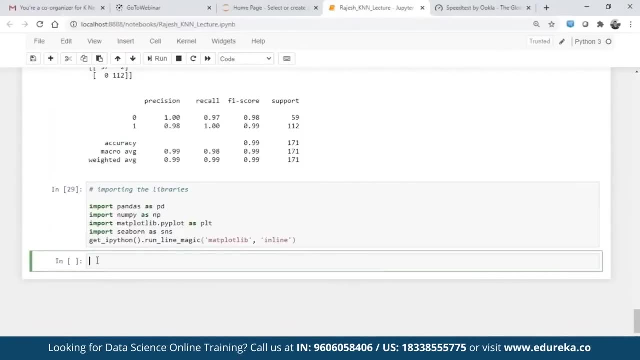 what flower is it? so just give me a moment here. So we again start by importing the necessary libraries and then we'll look at what this iris data set is. So the iris data set comprises of 50 samples of three species of iris flower. 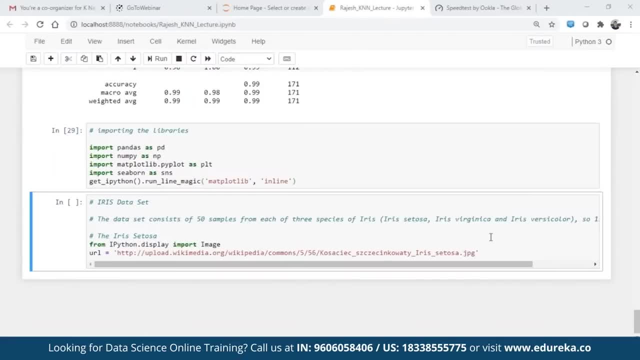 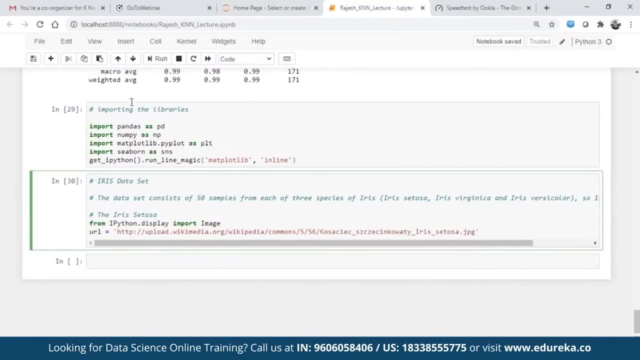 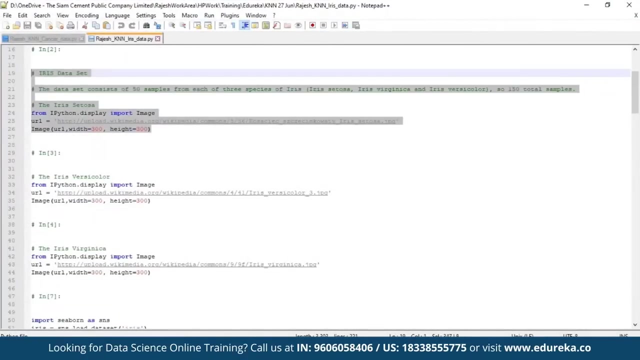 which is iris setosa, iris virginica and iris versicolor. These are the three types of iris flowers And if you run this basically, we will find that. Okay, sorry, we did not copy the entire read the code here, So it was giving an issue. 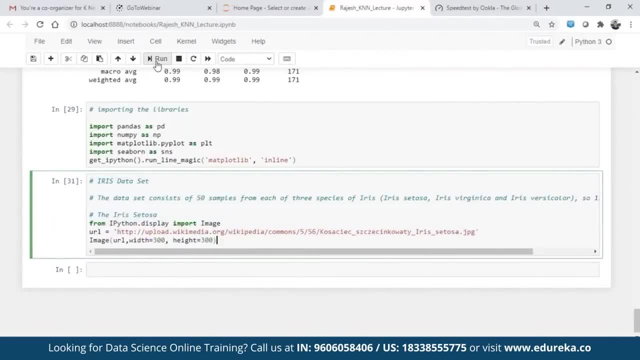 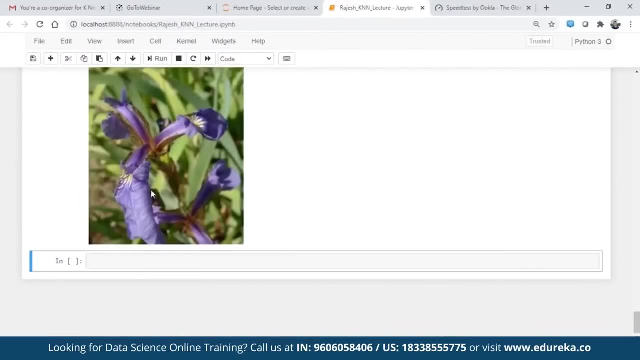 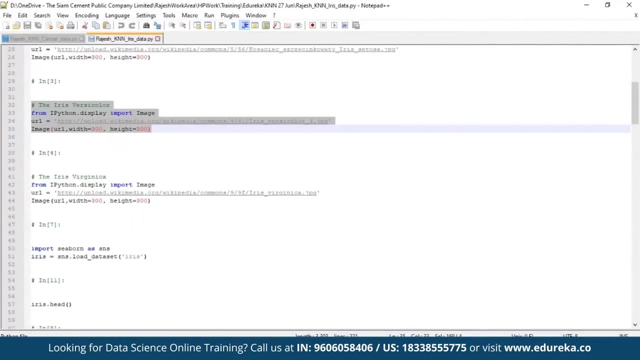 Let's just run it again, Okay. so we see that it is this particular flower which is iris setosa. So the iris setosa, you can see, and now let's look at the other two kinds of flowers here. So, which is iris versicolor? 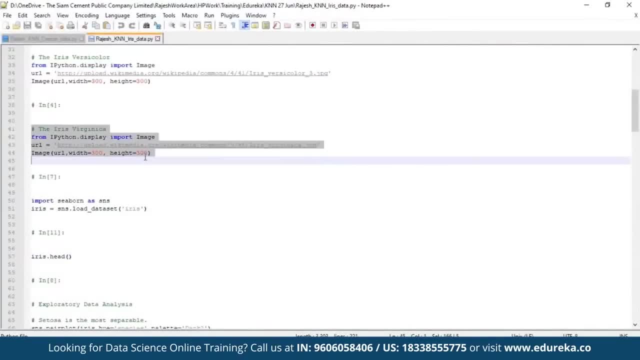 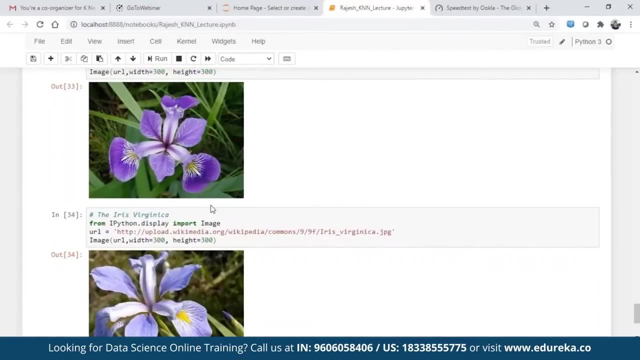 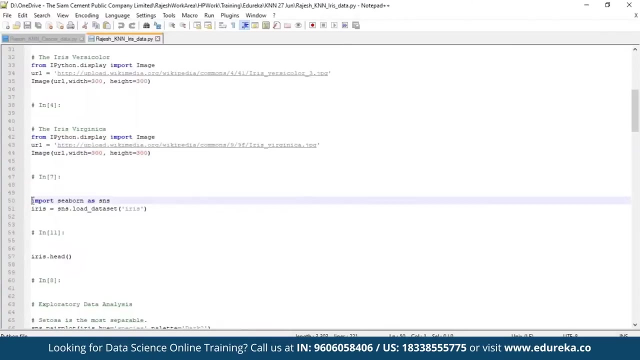 So this is iris versicolor, And then you have the iris virginica. So we see that this one is iris virginicas. So essentially, we now will import the sort of data set. We have already done that and we will now use the seaborn package. 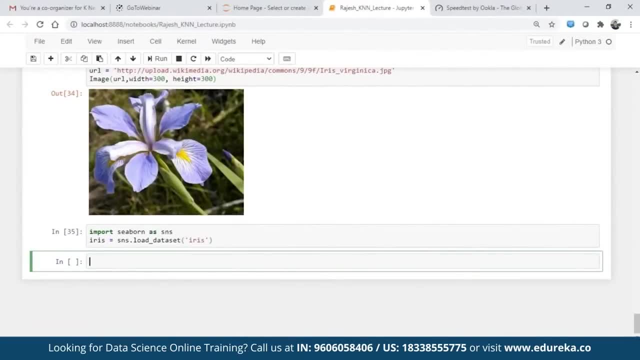 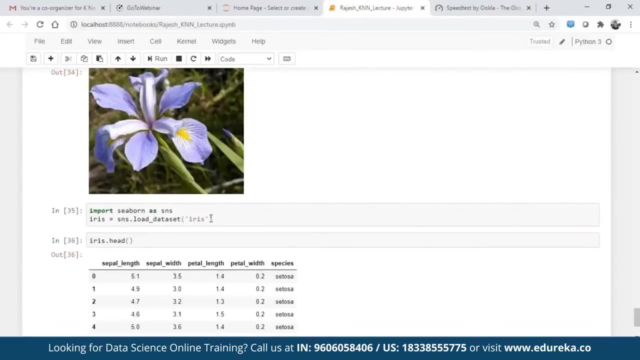 to actually plot some of this data and see how it looks like, Which is basically do some kind of exploring We data analysis. So, if we look at the data itself, so this is the top five rows from the data, right? So essentially, the data consists of: 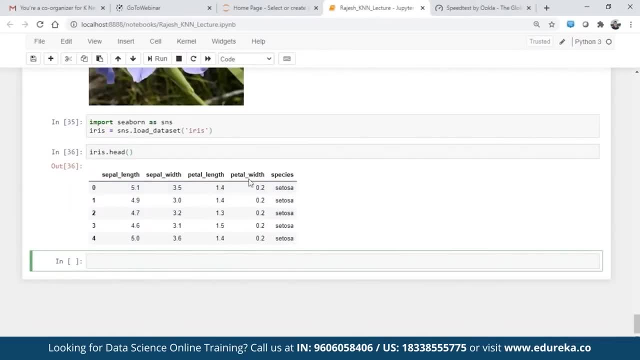 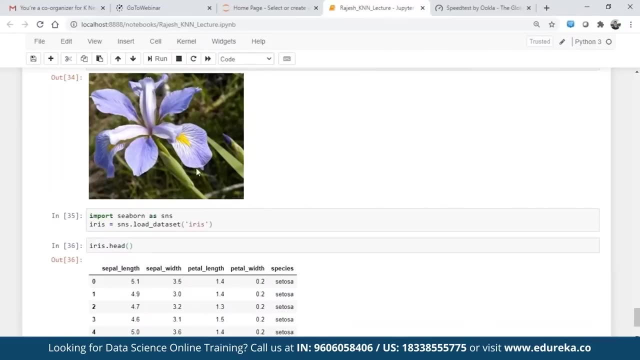 basically what is the sepal length, sepal weight, petal length and petal weight. and this is nothing but basically your petal is your. this colored part of the flower in the sepal is basically your green part here, right? So it is talking about one of what is the sepal and sepal. 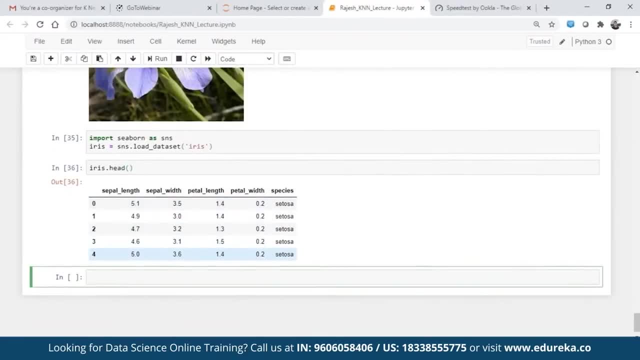 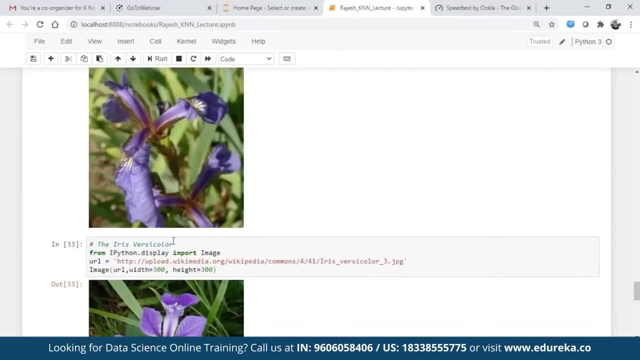 width and petal length and petal width of each of the species, whether it is setosa, virginica or versicolor, and we are. we will see whether we can use KNN to actually classify these, these flowers, into the data points, into these categories of flowers. 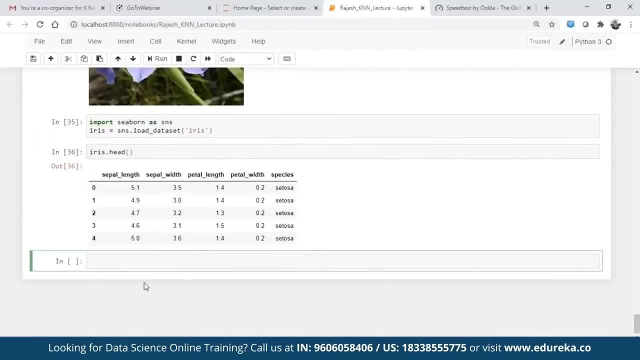 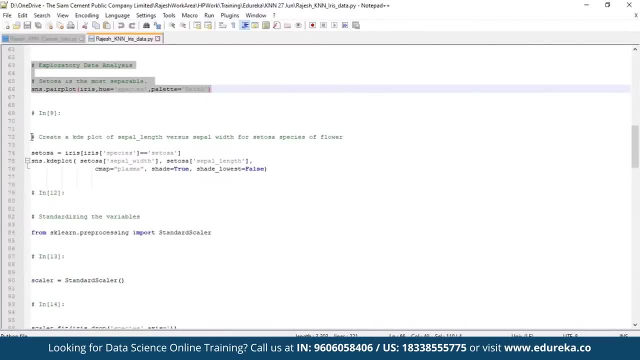 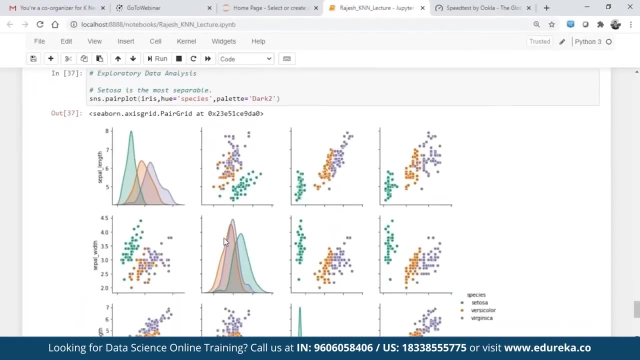 So let's do some quick exploratory data analysis on this. So we are running a pair plot on the data set and in the meantime I'll just copy another part of the code here. Okay, So now the plot has come up, So as we can see that the green is basically your setosa flower. 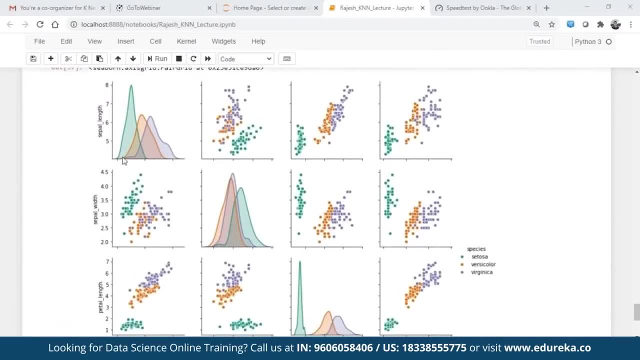 and we can see that this pair plot actually just plots the sepal length, sepal weight and petal and petal width of each of the samples of setosa versicolor and virginica and we see that the green dots which are the setosa flower, is actually quite 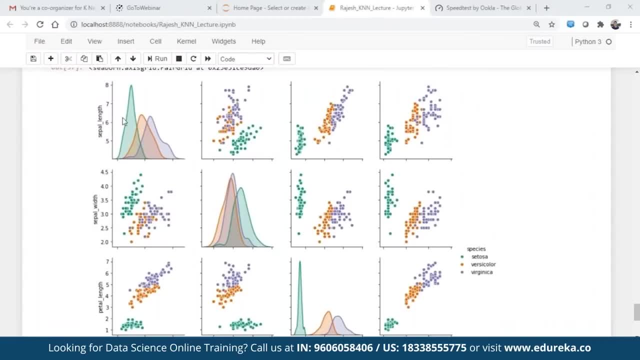 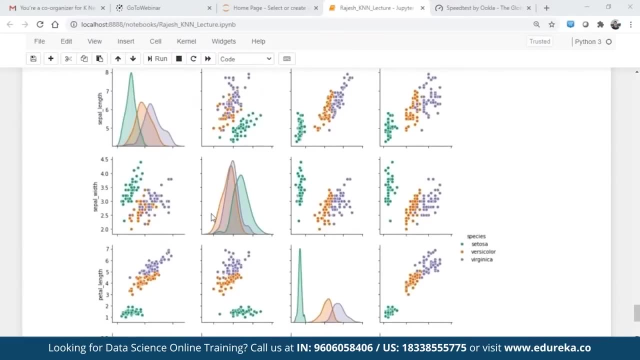 separable from the others. It's when you plot, let's say, for example, sepal length and petal length right, We see that this is quite separate from the other data point. So let's see whether you know we can actually be able to classify it using KNN. 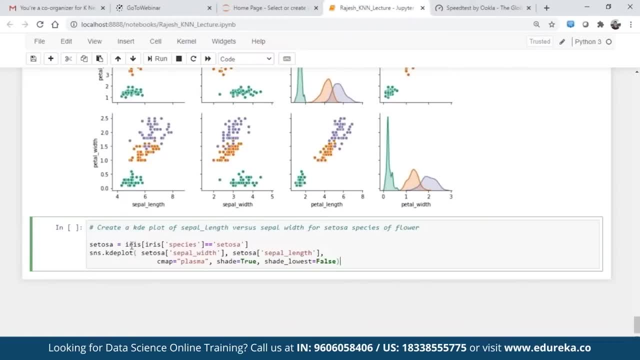 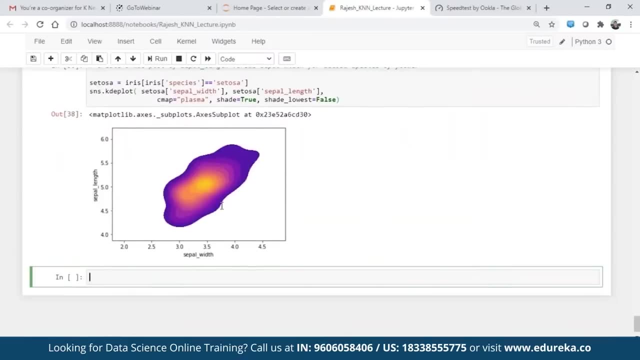 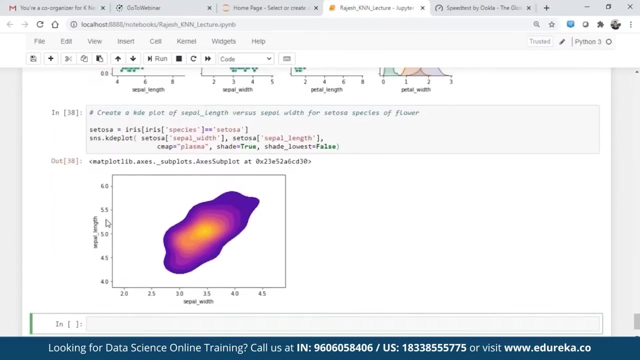 or not. and here we are running a kernel density estimation function on the setosa flower to check what kind of distribution it has. So this is the kernel density estimation plot using the SNS package, So only for the setosa flower. So if you plot the sepal length and sepal width we get something. 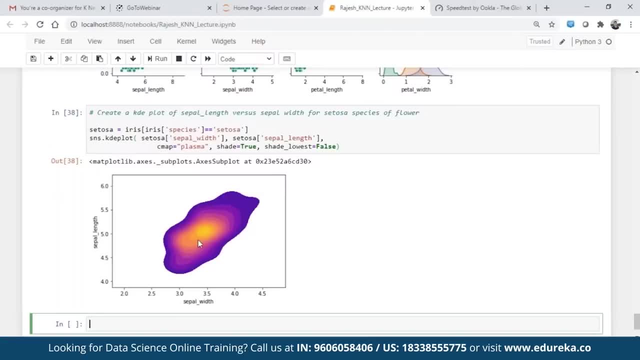 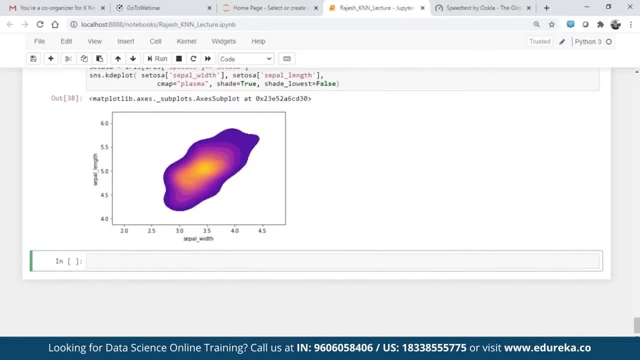 distribution like this. So essentially we see that the maximum centered around here and then there is a distribution as you can see here. So there's some kind of a linear relationship here. Okay, So now we will again do the same: standardization of the variables. 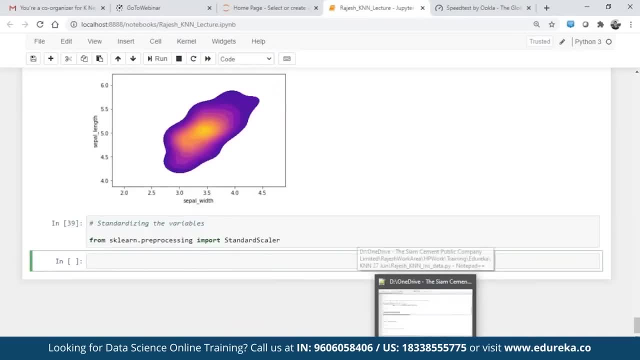 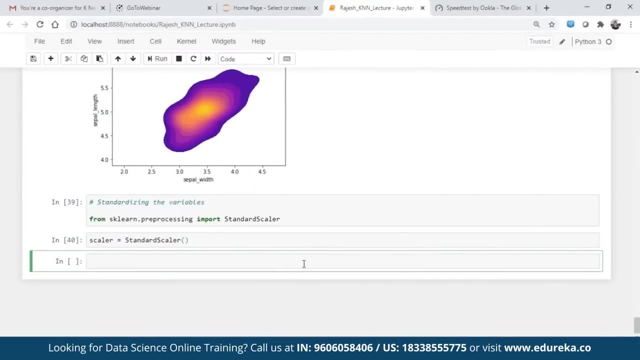 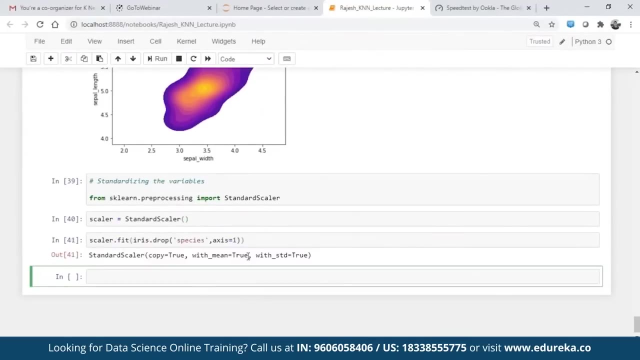 that we had done in the cancer data set case. So we are importing the standard scalar function from the scikit-learn pre-processing, So we will initialize that. so we are again basically doing the standardization or normalization Of the data and we will do the standardization. 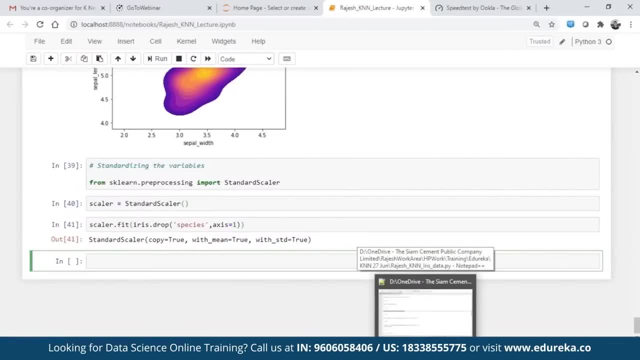 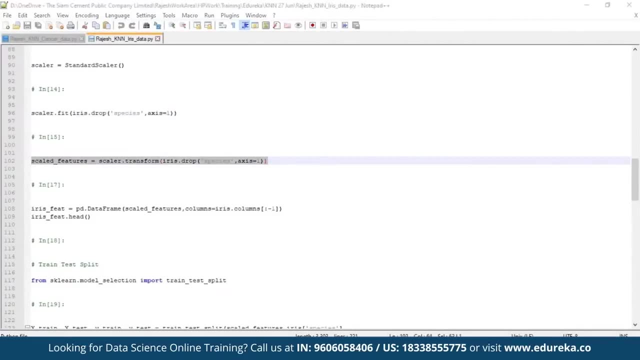 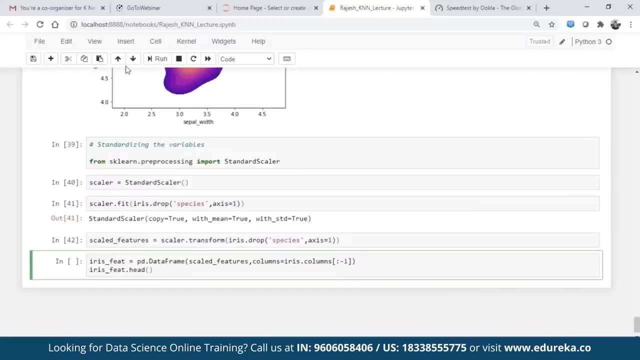 on everything except the species, which is a categorical value, right? So it's categorical whether it is which kind of flower it is. So we have removed that and then we have done the standardization or normalization on rest of the data. So we now convert this into a data frame, pandas data frame. 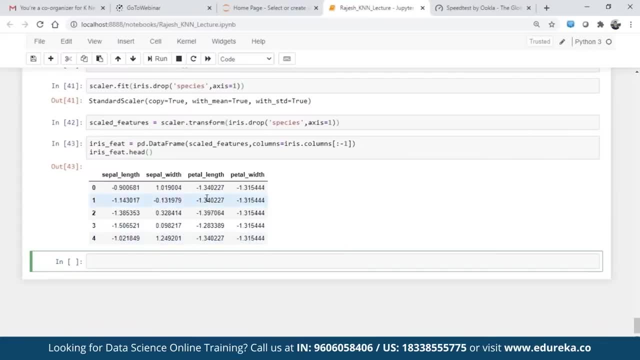 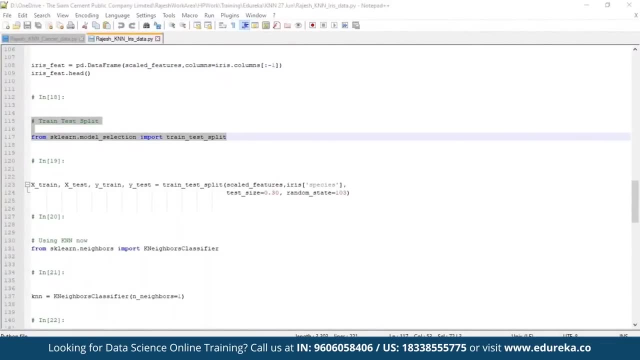 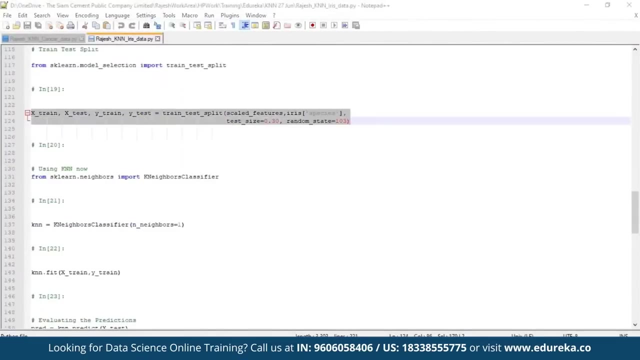 And if you look at the top five rows now it's all converted or transformed, So the values are now normally distributed, basically Okay. So now we divide the data again into train and test And we again have a training of about 70%. 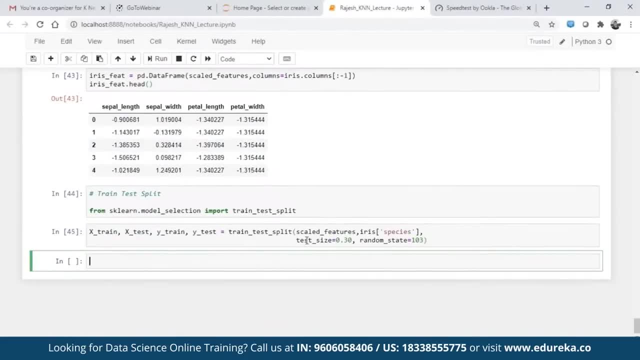 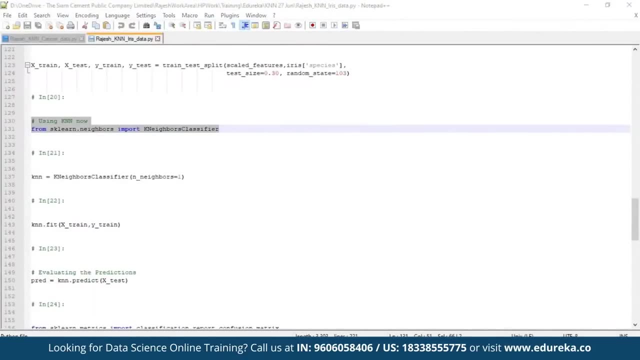 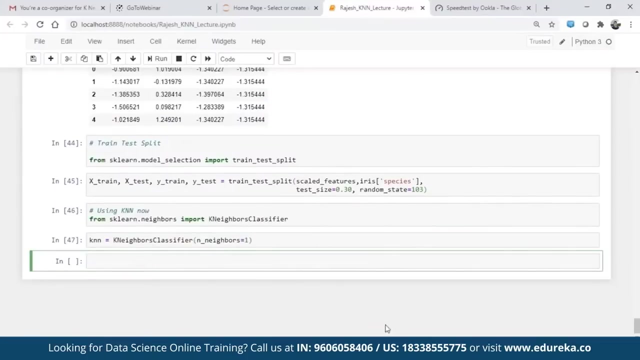 and test data set of about 30%. so we are dividing that entire data set into these buckets and we will now use KNN To see if we can use KNN to classify them. Again, the same and case is going to 1 and we will check the results. 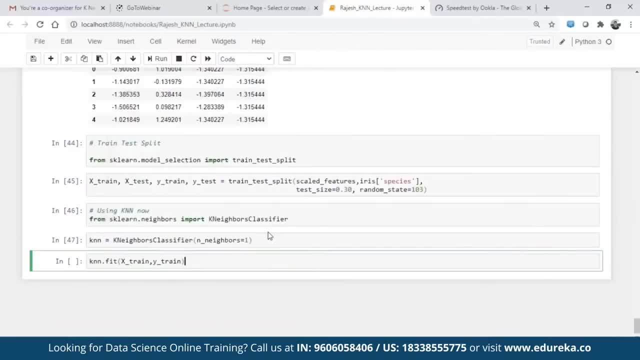 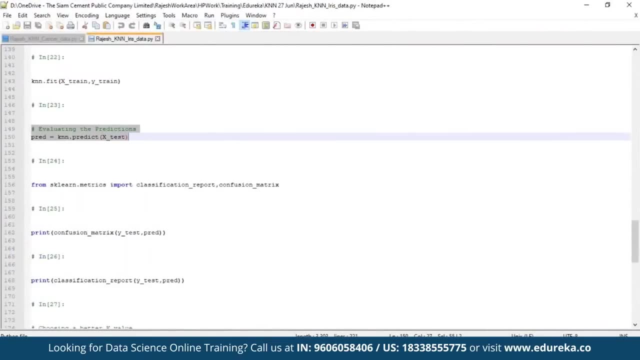 and then we will do a trial and error to check what is the best value of K. So here K is equal to 1. And now we are going to predict on the test data set and look at the results. So we are now importing the classification report. 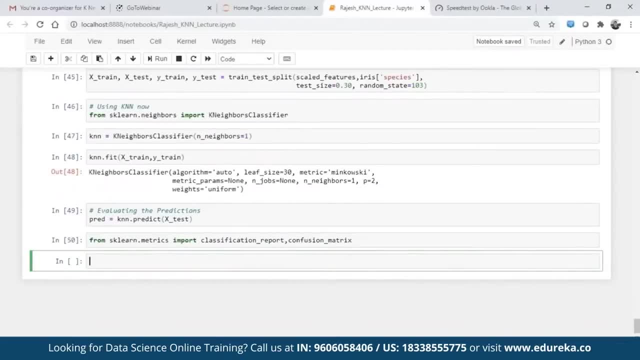 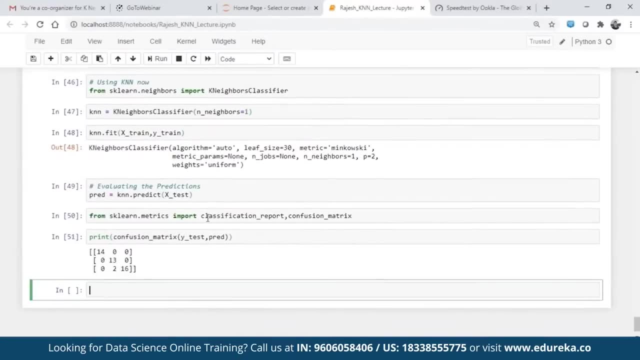 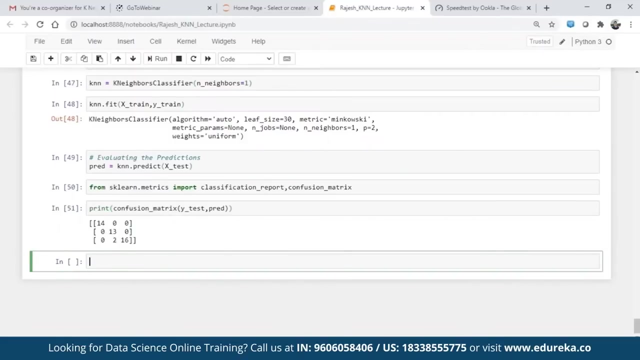 and the confusion Matrix. So if we look at the confusion matrix We see that kind of already We are getting quite good prediction. So just two misclassified points. And if we look at the accuracy, you see that the accuracy is quite high, around 96%. 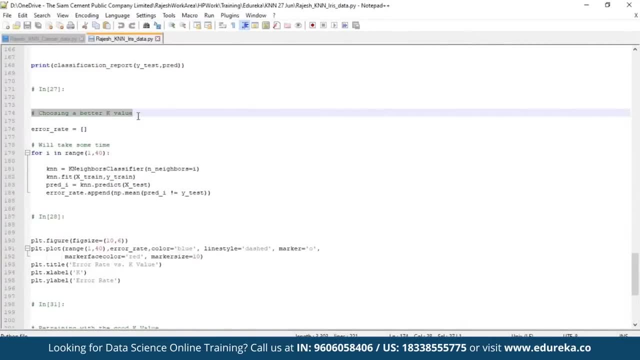 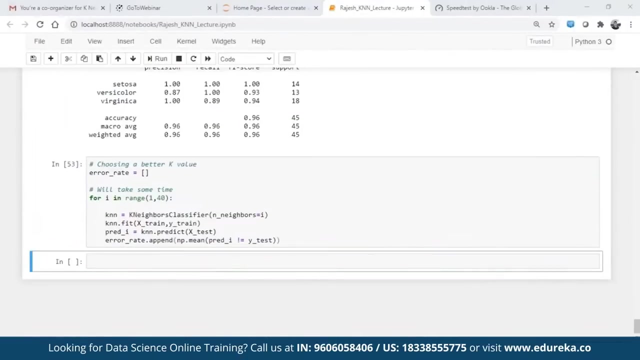 already. Now we choose, we have to see what is the best value of K. So essentially we will. we will again run K is going to 1 to 40 and check which is the best value. So let's plot the errors when we vary the K from 1 to 40. 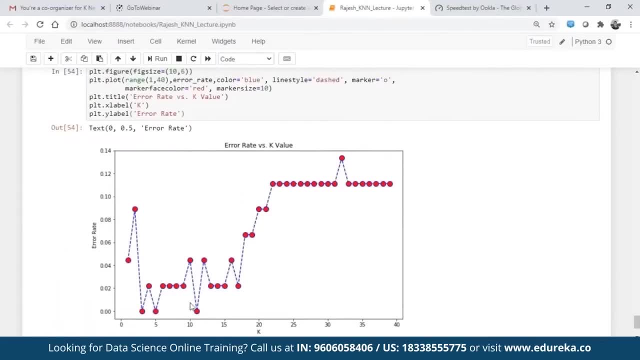 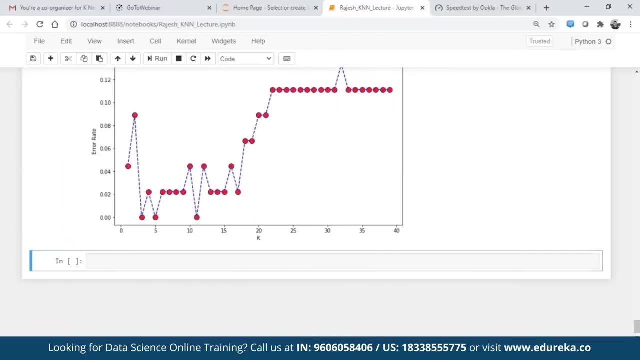 and we see that the actually the error decreases and then increases. So basically the error is minimum. with K is equal to, let's say, 3, or even 5 or maybe 11.. So let's choose one of these values. So let's say K is equal to 3. 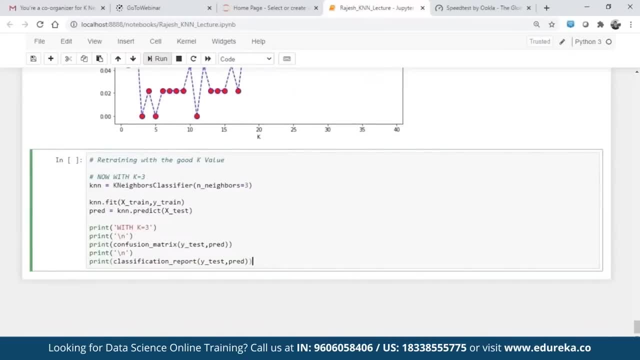 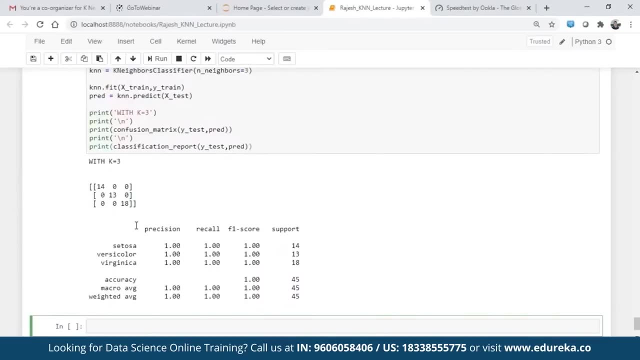 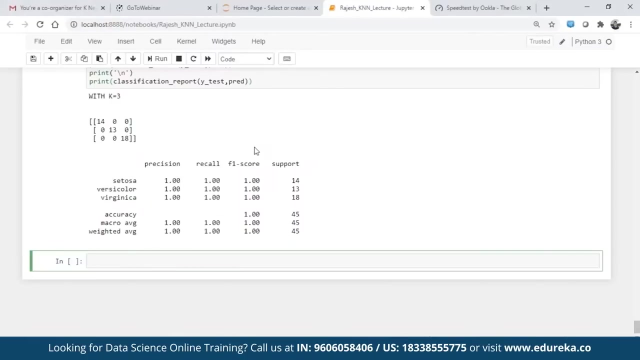 and let's see how the results look like. does it improve the accuracy or not? So we now see that even the two data points which are misclassified earlier is now classified properly. So the accuracy improves 200%. so that's the example of how you can choose K. 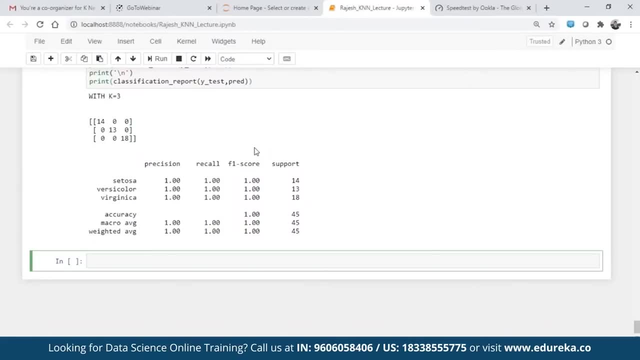 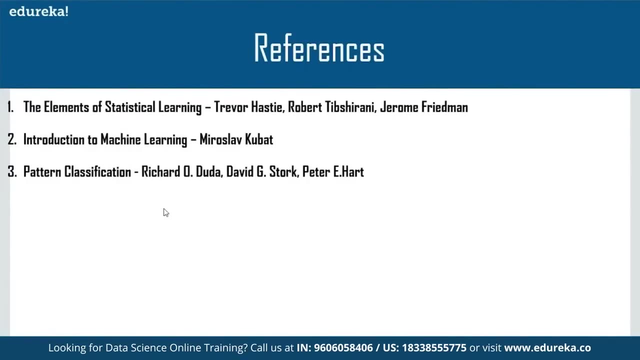 So we have covered the hands-on and now we will look at some of the references. So some of the references are basically these three textbooks here which I found quite good. Some of them are even available online So you can refer to them if you want to learn more about KNN. 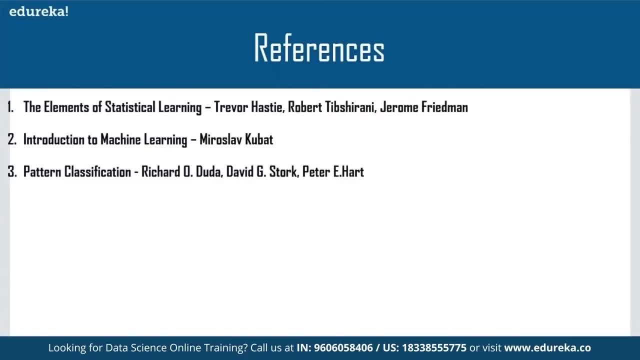 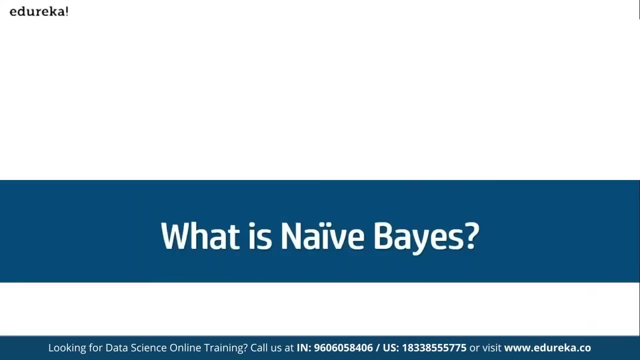 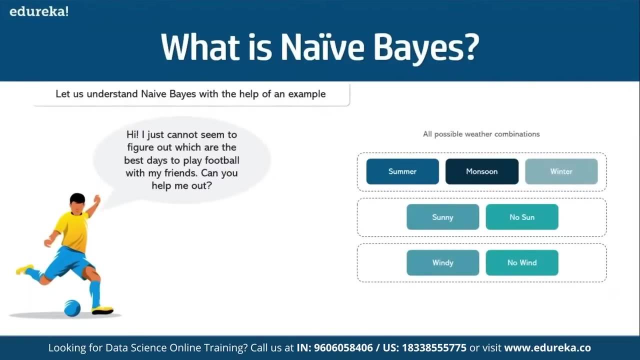 and also they are quite good references for some of the other techniques as well. So let us now talk about what is naive base. Okay, let us understand naive base with an example Here. I just cannot seem to figure out which are the best days. 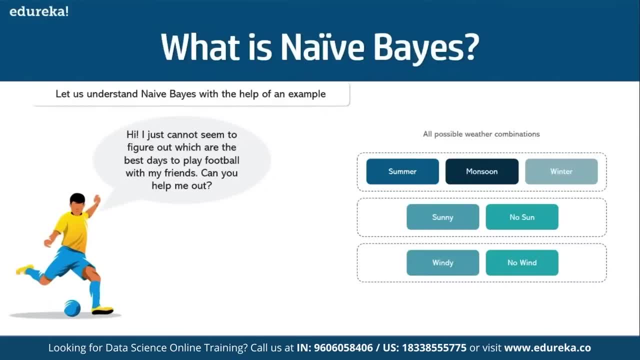 to play football with my friend. Can you please help us out? All possible conditions are given to us. There is summer, monsoon and winter, which is nothing but the outlook. Am I correct in saying that summer, monsoon and winter is nothing but the outlook? then we have sunny or not sunny. 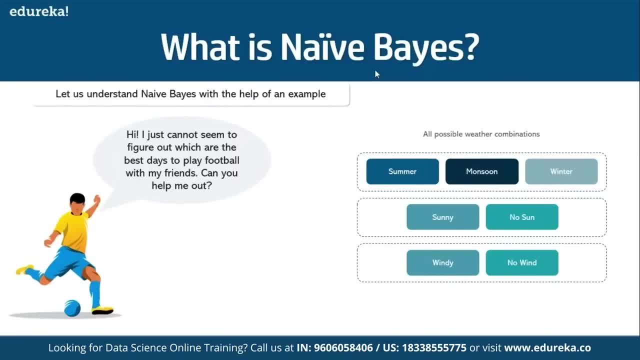 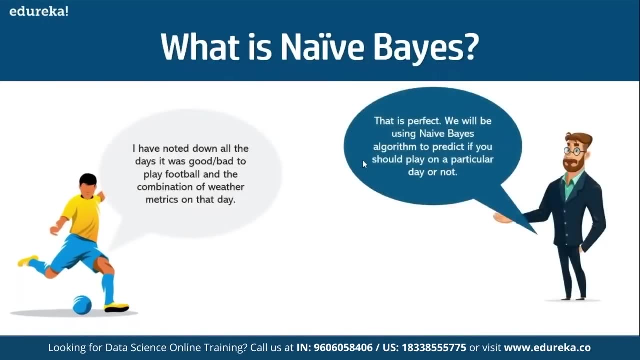 So that, basically, is the humidity right, and then we have windy or no Windy. that speaks about the winds. How are the winds right? So if you look at these combinations- okay, we will look at this using Navy bass on- how do we decide whether we can play or not? 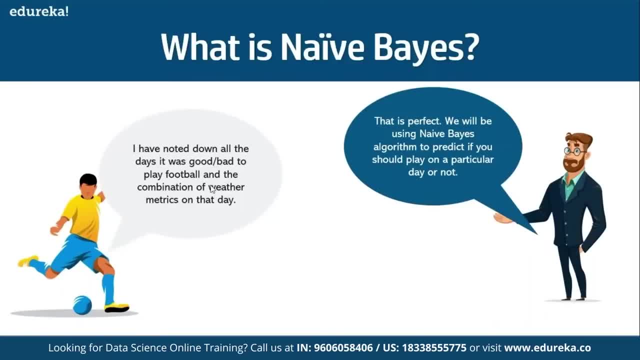 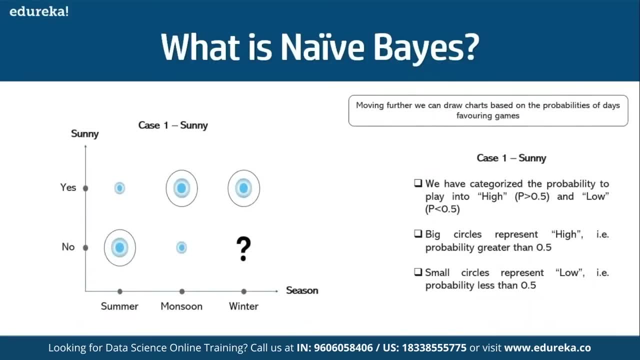 So, if I have noted down all the days, it was good, bad to play football and the combination of weather matrices on that day. That will be perfect. right, That is perfect, And we will be able to do Navy base classifiers using that. now Navy base classifier comes. 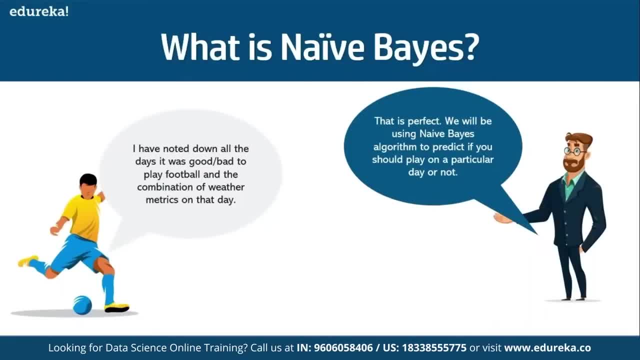 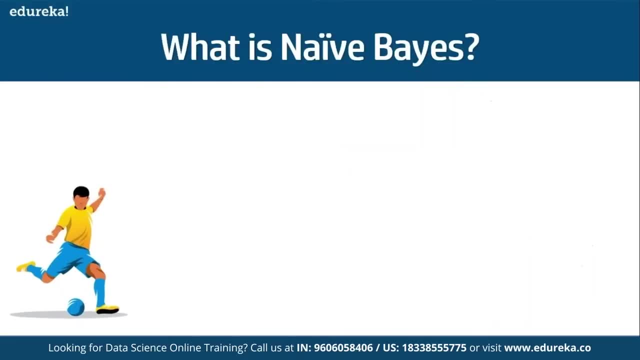 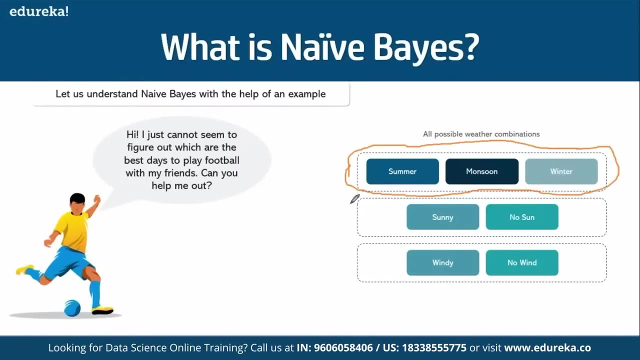 from the Navy base Here, and Navy base theorem is purely and purely based on the assumption of Independence. So what does it mean when I say Independence? What it means is that this variable has no relationship, No association with this variable. Now, when I talk about this in a linear context, obviously in summer you will see that we 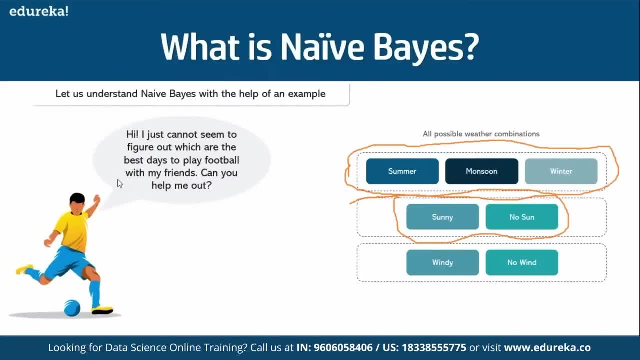 have more sunny days. Yes, So if you look at it from the correlation area, from the linear algebra concepts, linearly these two are correlated to each other. Am I correct in saying that obviously in monsoon we have less sunny days in winter? 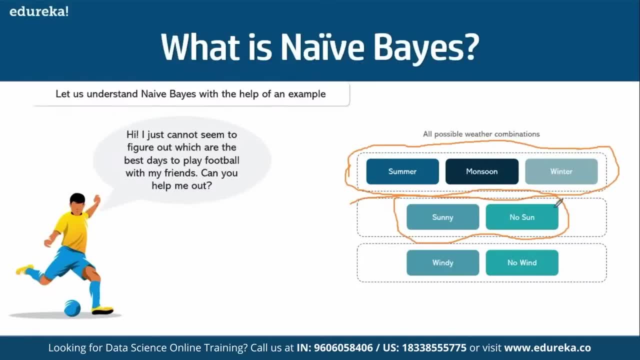 We further have less sunny days. Yeah, So although there is a relation, Navy buyers theorem says that all these variables are independent of each other. What does that mean, If this is causing any kind of an effect, if this is causing any kind of an impact? 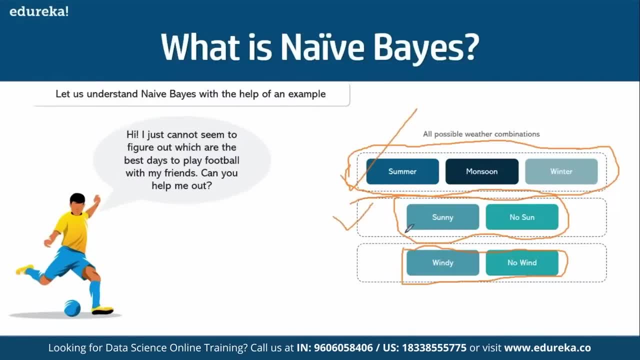 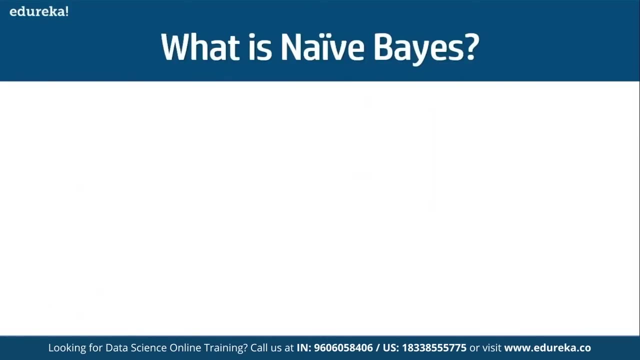 This should not matter. Okay, there is going to be no relationship. summer, monsoon, winter. It has its own weight, age, Okay, and it has nothing to do with the other conditions. Every condition is equally significant, All right. So what happens? 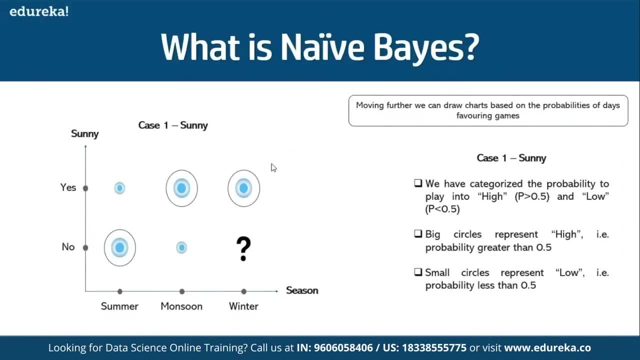 In Navy bars is we estimate the posterior probability of every event happening. here We calculate the posterior probability of an event happening. Okay, So here if you see, if you look at the sunny conditions, what we have done, sunny conditions, we have this distribution that there is no play happening in summer. 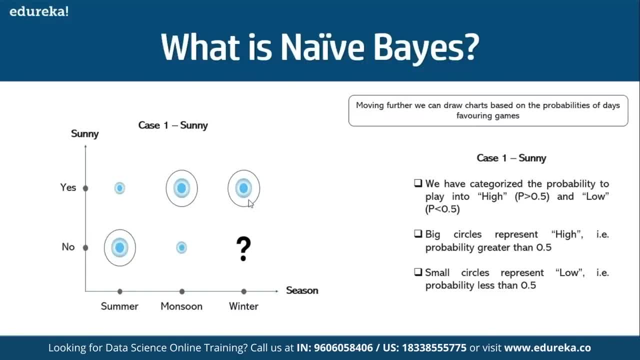 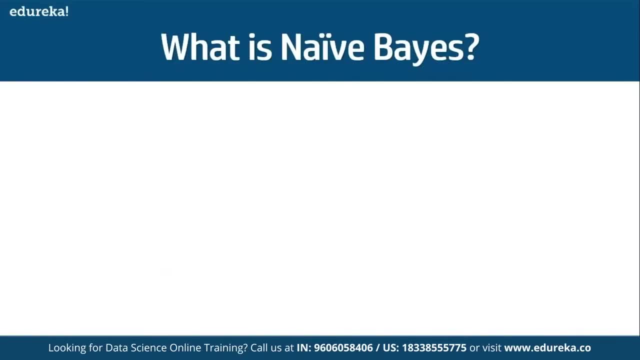 There is play happening in monsoon. There is play happening in winter, right? So base of the season, we are figuring that out. similarly, for windy conditions, We are doing that right again. Then we do it for a combination, right? Whether when windy conditions are yes and no, what happens to play? 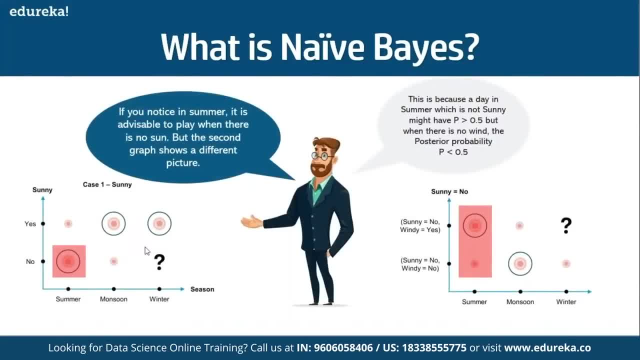 Okay, So here what? at the end of the day, What gets selected is the one which has a posterior probability of greater than 5.. Now, when I talk about posterior probability, what do I mean by posterior probability? Let me have a blank slide here. 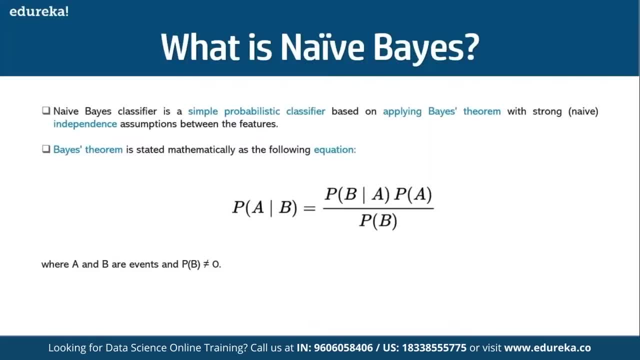 You? actually it's given, So I need not show you that. what is the simplistic probabilistic classifier here? What is the probability of an event a- happening given B? So, if you look at our problem context, what is it that we are trying to figure out? 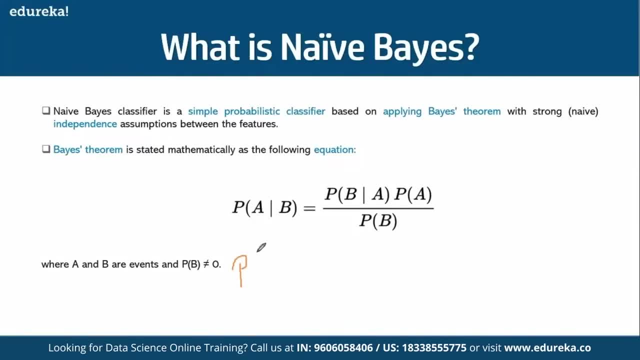 We are trying to figure out what is the probability of Play happening, given The outlook is sunny, Comma- The Winds Are normal And there is no rain On Any given day. on any given day when there is no rain, there is no wind and the outlook is sunny. 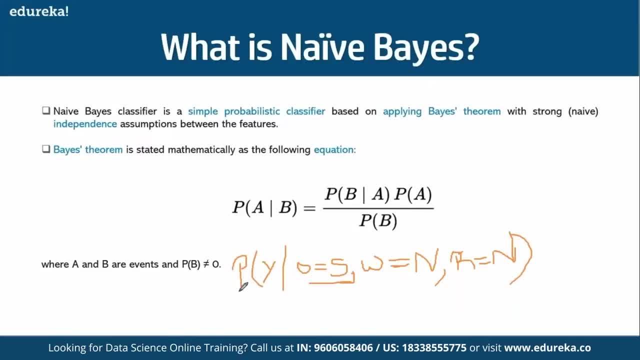 Whether play will happen or not. So what we end up doing is we calculate the posterior probability of play happening given these conditions. We also calculate the posterior probability of play not happening, Given these conditions, and then we normalize these probabilities Mathematically. 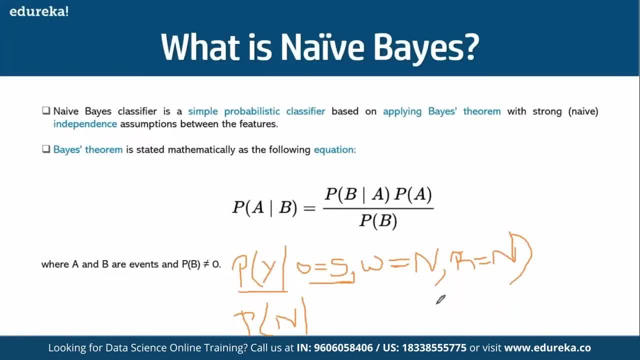 We do all of these calculations to figure out Navy bias. Okay, Now here see. here We are talking about one event. here We have three events. We have outlook, We have winds and we have rains. So what this becomes is probability of three independent events. 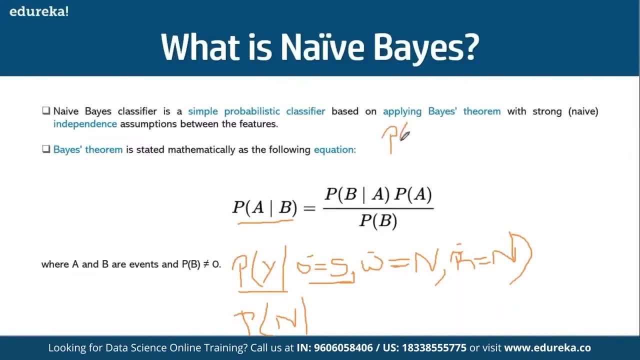 So what we will do? we figure out what is the probability of play happening, Given Outlook is sunny. We also figure out What is the probability of Play happening. Multiply this with the probability of wind. as no Given no, Then probability. 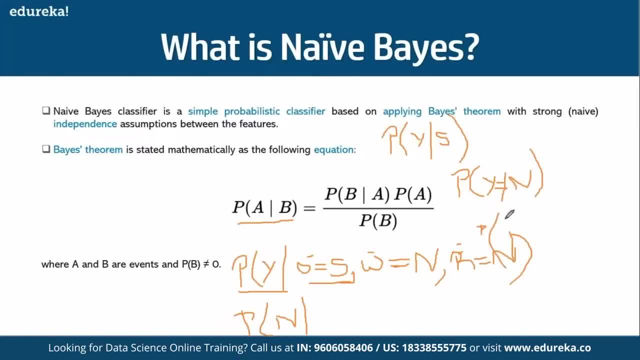 Probability of play happening, Given rain, is no, We figure out all the three independent probabilities multiplied. All right, This is what we do mathematically. This is what is done mathematically in Navy bias theorem. Ultimately, the posterior probability, The posterior probability, probability of an event. 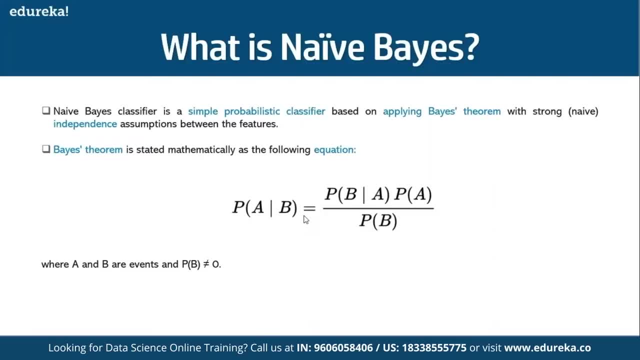 A happening given B conditions is calculated by first calculating the class probability. What is the class probability here? Probability of it raining given play was happening in that day. This is multiplied by the total probability of play happening and divided by the total probability of sunny conditions. 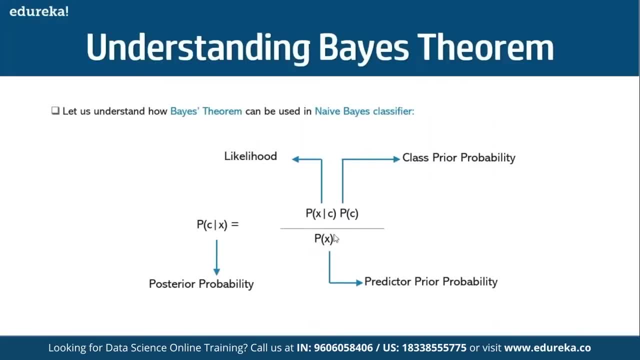 Here, as you see, this is the posterior probability, This is the class probability, Here is the predictors probability. This is the Outlook X, is the Outlook C, is what we are trying to predict. Right, and here is the likelihood. So how is this formulated into our table? 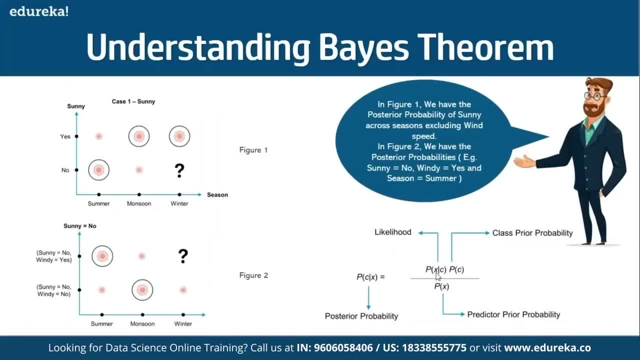 Now, if you correlate this to our graph, what will be the likelihood? What will be the likelihood of sunny conditions Given? play happens, Sunny conditions, play happens. 2 divided by 3, out of sorry. How many sunny conditions do we have? six? 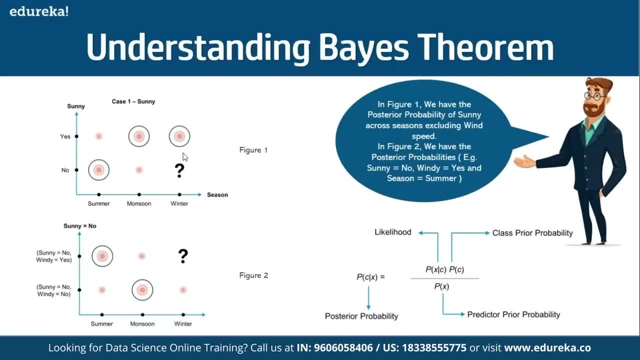 Conditions: in six conditions, How many days just play up in two days? 2 by 6, 1 by 3.. What is the class probability? So, of all the events that are given to us, how many days just play happen, Okay? 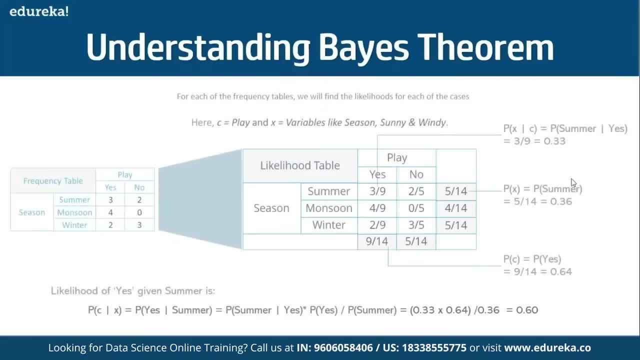 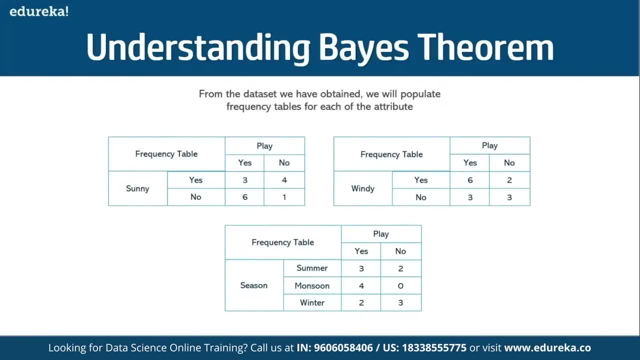 This is how this is calculated. So here you see, what we have done is- let me go back to the previous slide- Here you go. Okay, here What we have done is we have calculated this table. Now it speaks about the data set. 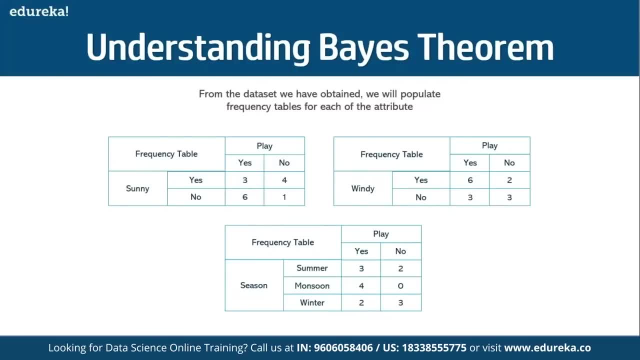 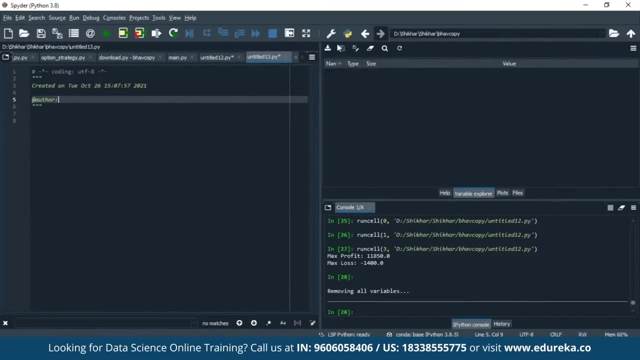 Where can you get this data set? You can look for golf play days data set online. You can look for golf play days data set. Okay, in this data set you will find all the data which is required for this Particular example to be done. 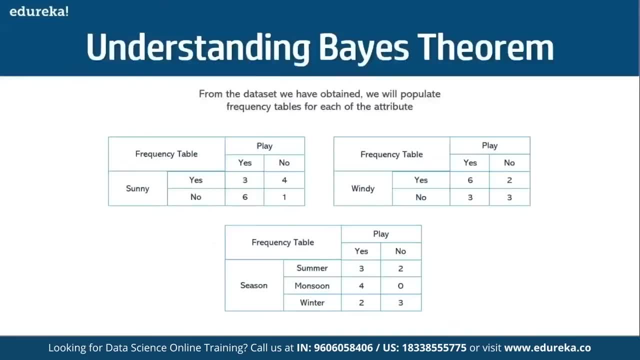 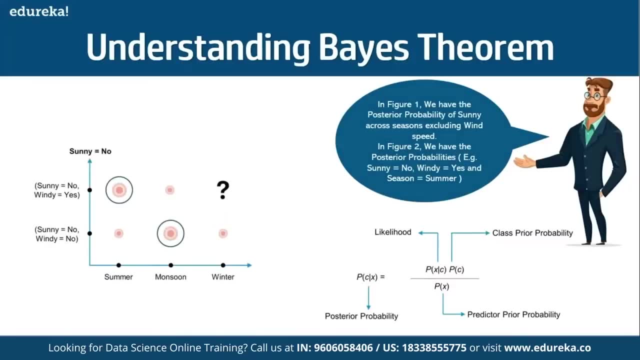 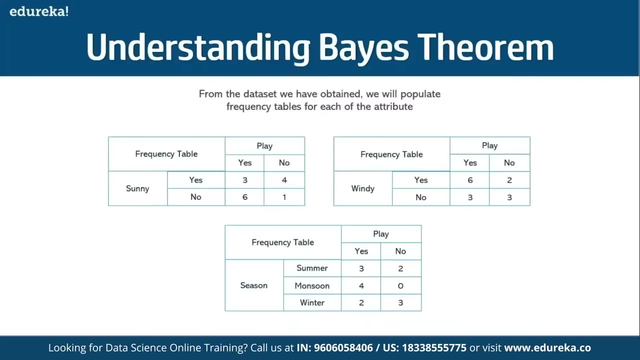 So what I will be doing is I will be doing this example, This Navy bias classification, with you in Python, All right, so whatever calculations are being done here, Okay, I will do the same activity in Python with pen and paper, and instead of doing this, 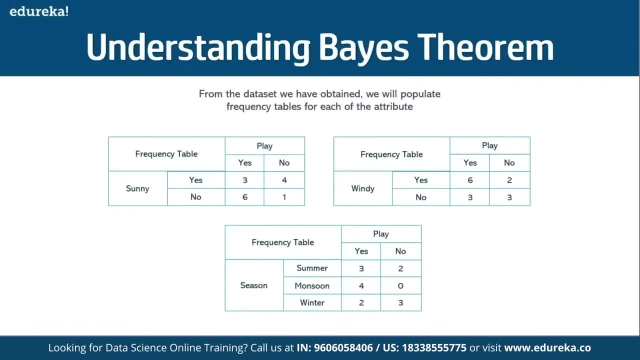 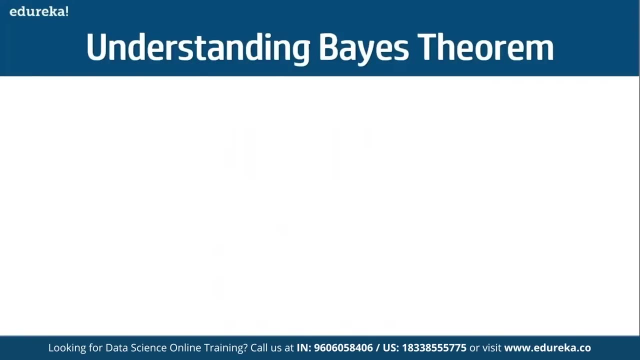 In a numeric way, where I'm doing a lot of probabilistic calculations. I will achieve this simply in Very limited lines of code, very limited lines of code with Python. Once I'm done that, I will come and explain this probability table to all of us. 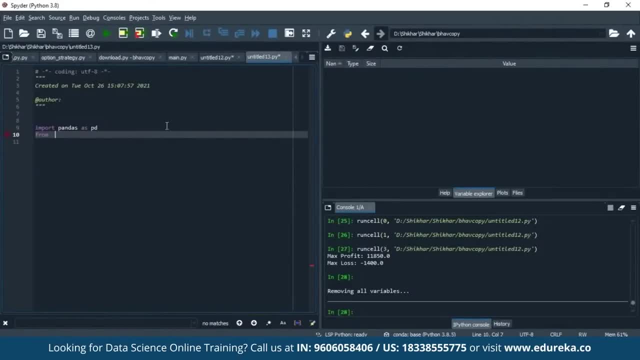 I'm going to use some basic libraries. All right, So here what I will be doing is using some very basic libraries for this activity. All right, So here what I will be doing is using some very basic libraries for this activity Done. 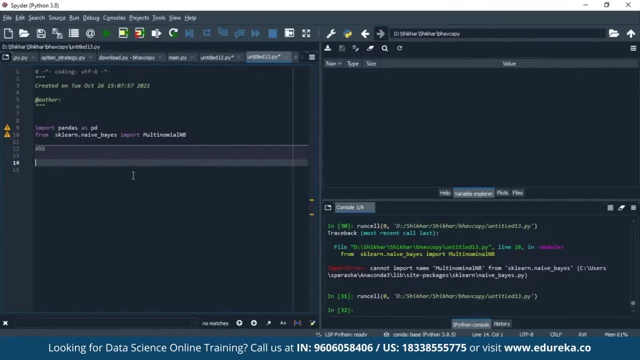 Now let me quickly go and read the data set. So for that, what I will do is click change my working directory. So for that, what I will do is click change my working directory. So for that, what I will do is click change my working directory. 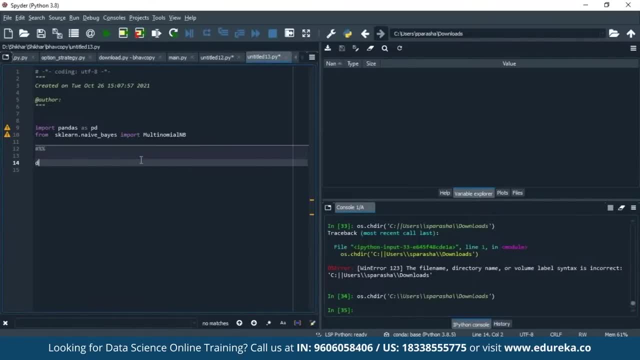 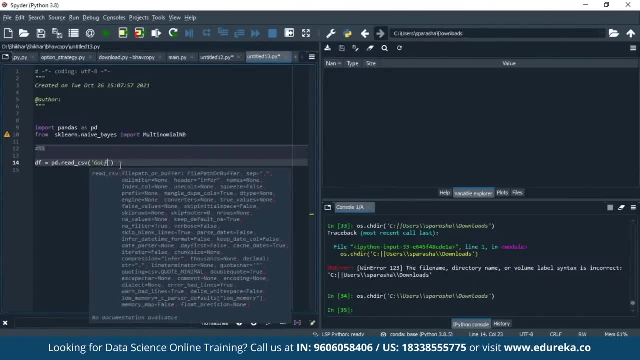 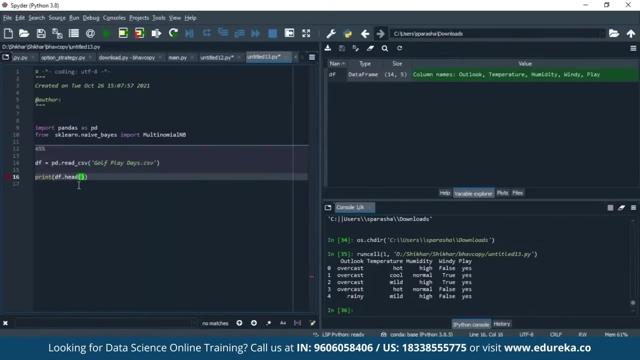 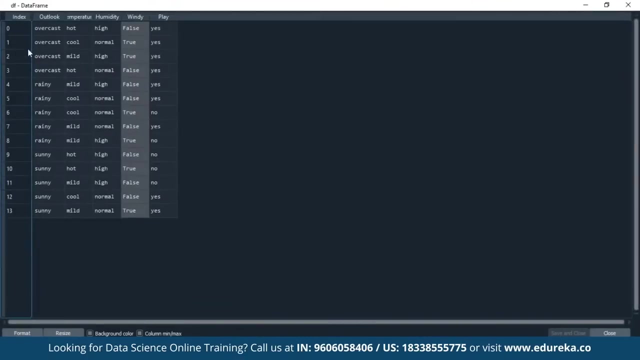 Here you go. This is the way I need your data set. And now let me quickly go and read my data. So my data frame is PD dot. If you look at this data set, in this data set you have 13- 14 days. in these 14 days, 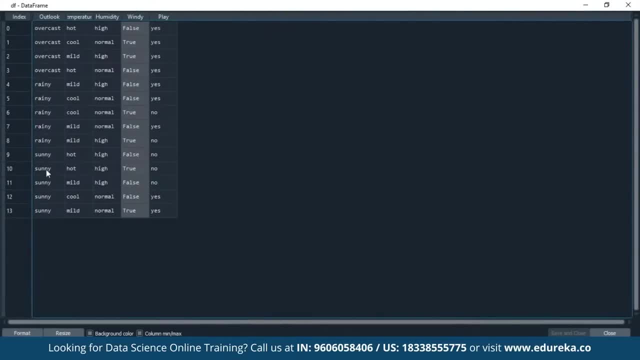 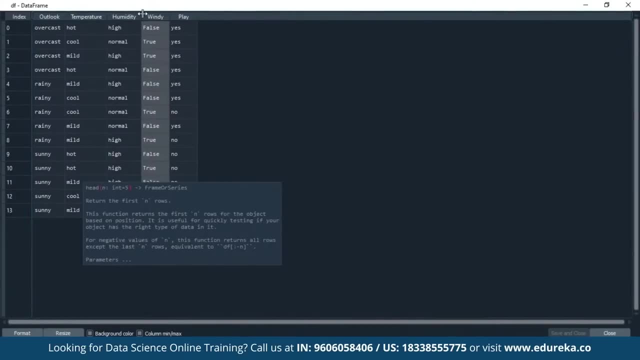 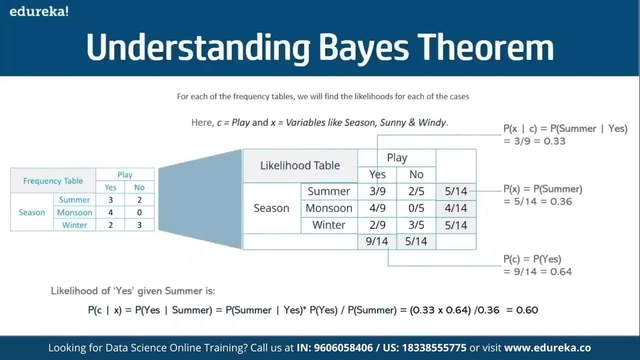 You have the outlook: overcast, rainy and sunny. you have temperature. temperature is hot, cool and mild. you have humidity, you have window and you have play right, So I will not be using okay, Let us use all four. in this example They are using only three variables, but in 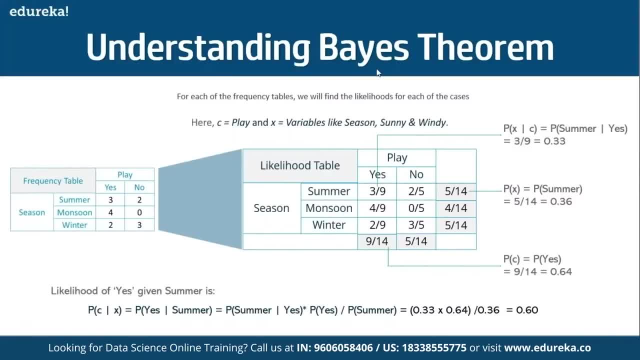 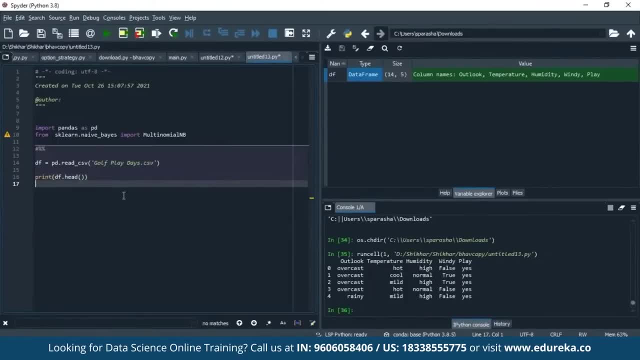 our hands-on. okay, in this hands-on, what I will be doing is I will be using all four variables. Let us do that, Okay? So before I do that, let me convert everything into a category. If you look at your data frame right now, it's not. everything is not into. 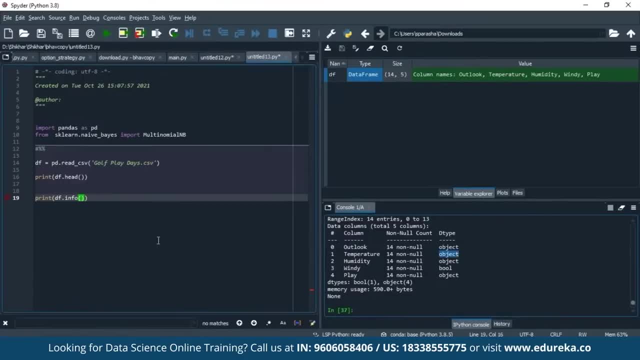 a categorical variable. Here you go see. Okay, so let me quickly go and convert everything into a category And once I have done this, let me create a new data frame in which I have everything as a category code, So that I have numbers. I'll show you what. what do I mean by this? 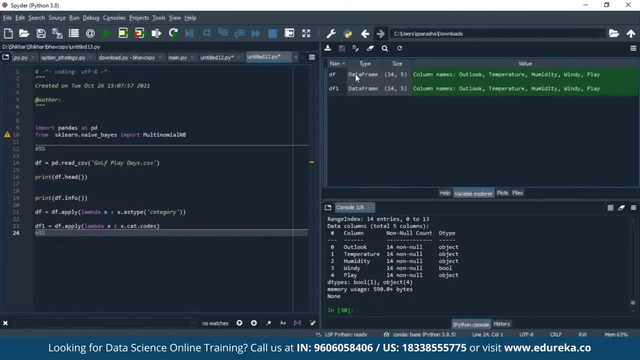 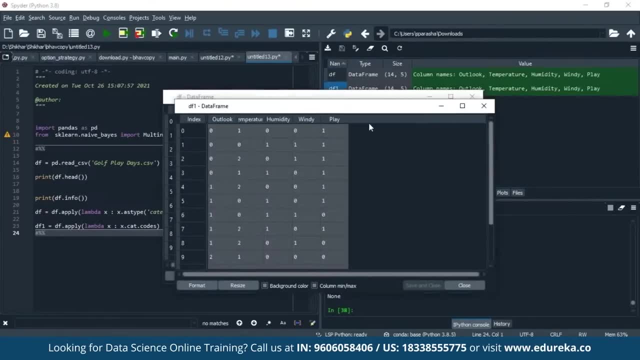 So let me execute this. Here you go, See. now I have two Data frames. in the first data frame I have all these values. These are now categorical variables. But in the second data frame I have all ones and zeros. So wherever you see, 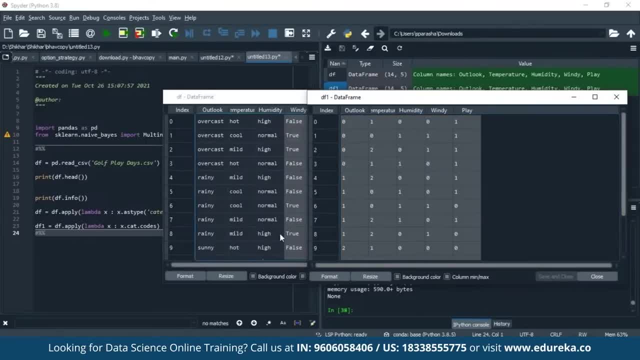 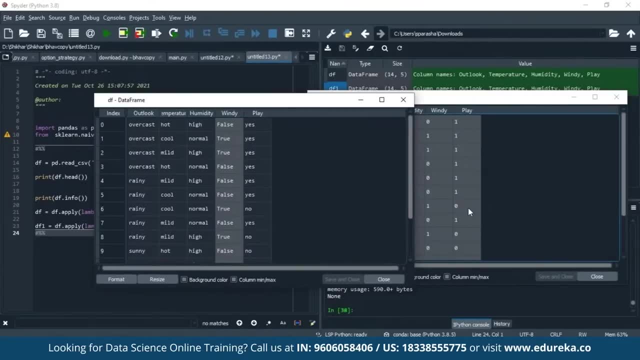 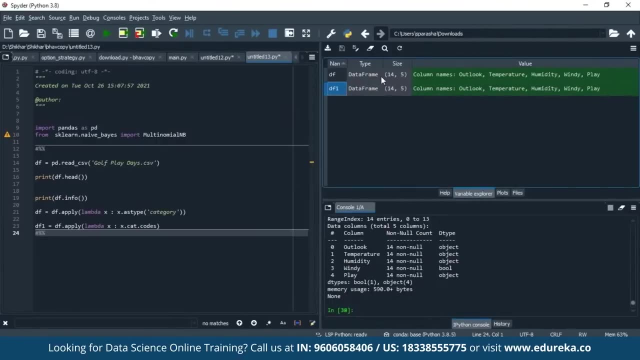 there is sunny conditions. Now I have a code to rainy conditions- code one. Similarly, when play happens, I have a one. when play does not happen, I have a zero. This is what I have done. This data frame is available online. 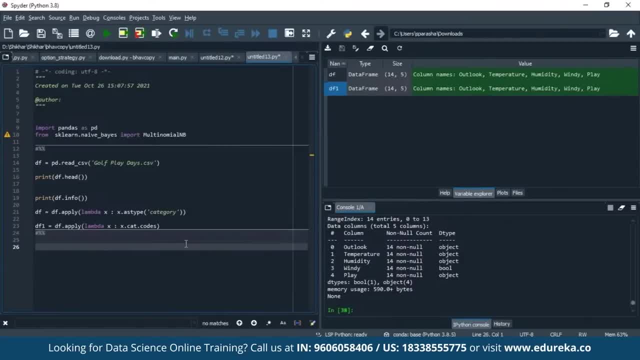 Okay, Get this data frame online. All right, Now my data frame is ready. So now what I'm going to do is I'm going to divide my data frame into training and testing. I have 14 records, So let's take 10 records for training. I will give 10 records as an input. 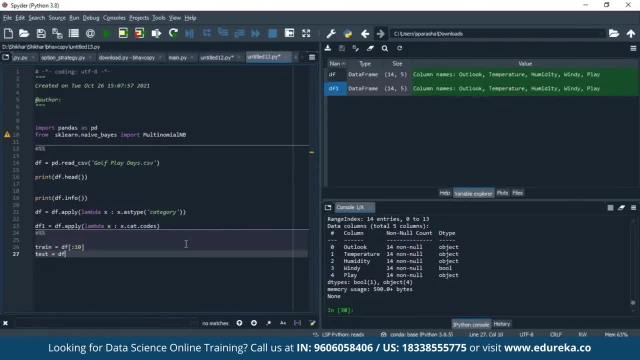 And I will give four records. last four records: Okay, Okay, Okay, Okay, As my tested data, All right. Uh, so now I will need to create my eggs and my wife. So how I will do that is, I'll say: 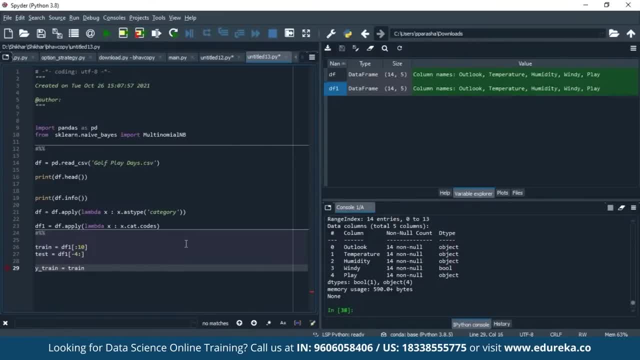 Y underscore train is equal to from train. I don't want the play variable. that play variable should be my wife, as simple as that. And I will say X underscore train is equal to three. Okay, And I will do the same thing for my test data. 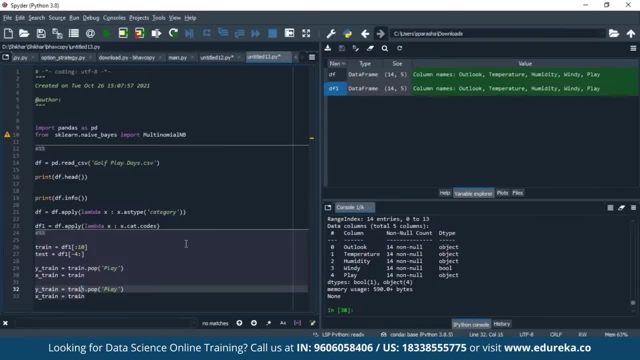 frame also. Now, those who are new to Python will find this a little bit strange. Please bear with me, But these are the only calculations, only steps which need to be performed every time you are trying to achieve Navy bias algorithm or any kind of an algorithm Right. So here, 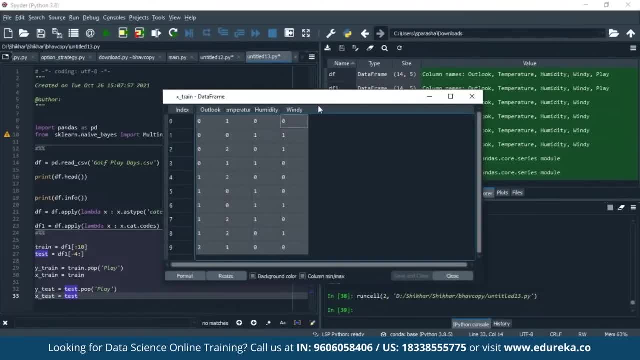 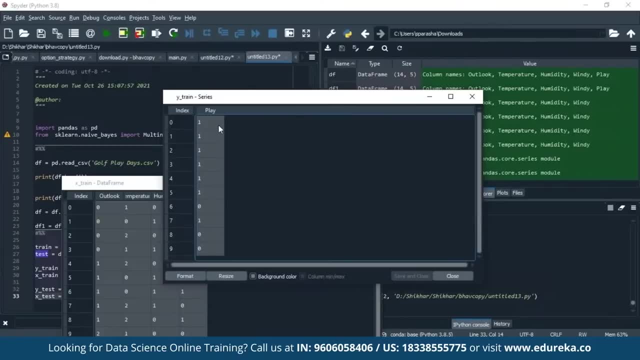 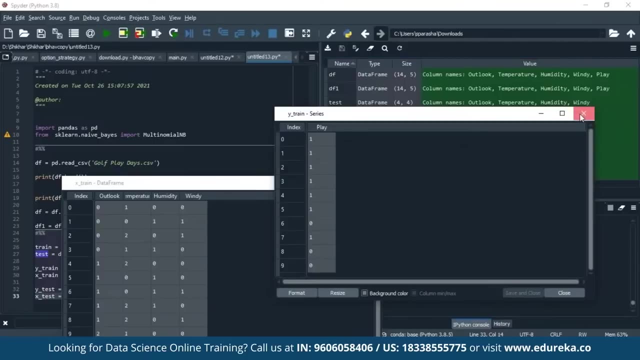 now, you see, this is my training data frame, in which play variable is not there. play variable is not there. This is my why- in which only play variable is there. This is my training data set. So both of them have 10 records with the matching index. Similarly, test data. 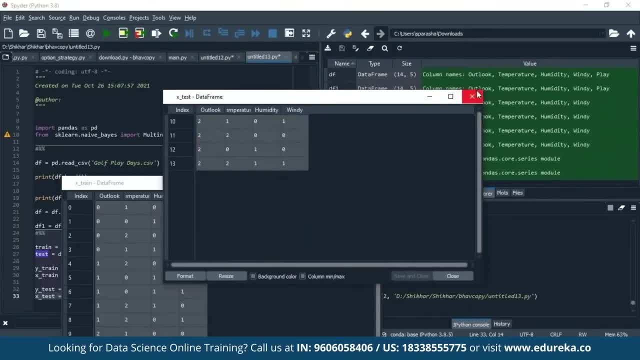 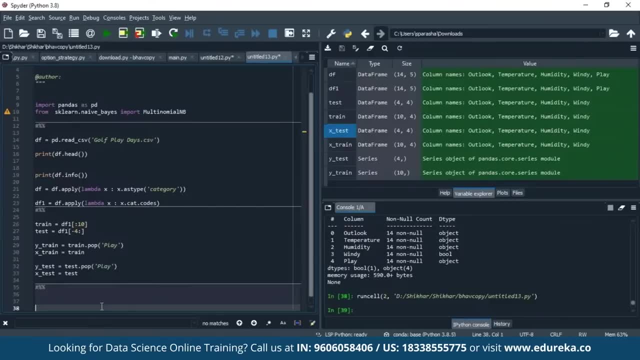 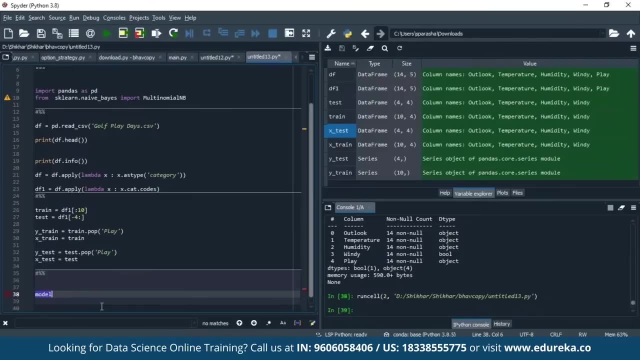 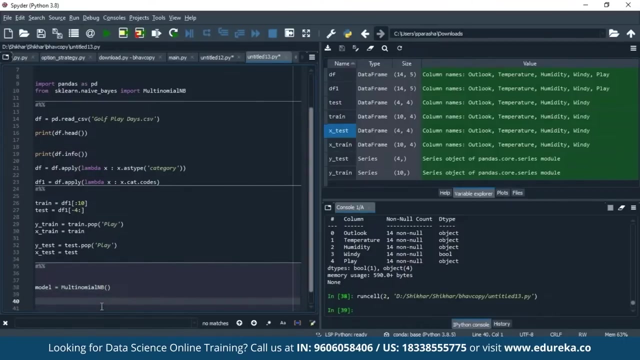 frame for records, for records with the matching index right, so that we know which data frame is where. Now, multinominal Navy bias. very simple, three lines of code and my model will be done. Okay, First I initialize my model. Here you go. I have initialized my model in this model. 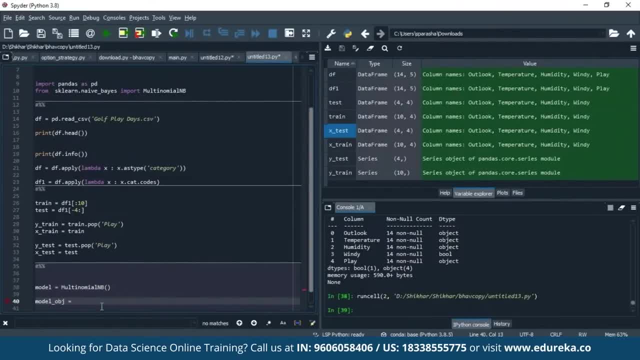 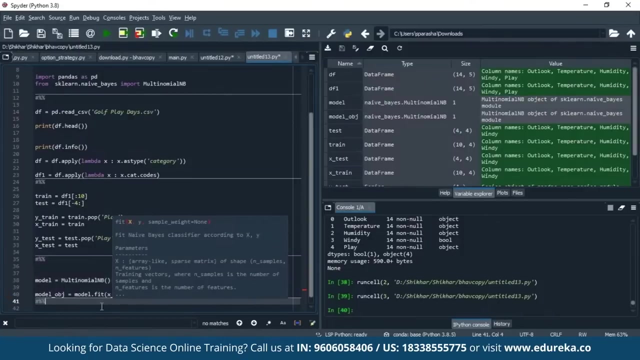 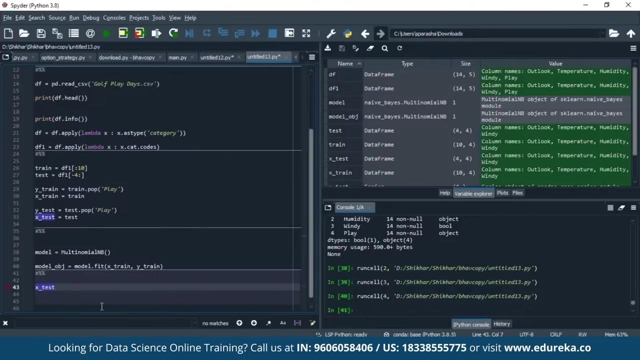 I fit my data in this model. I will fit my data So to do that. what I say is: fit X underscore train from my Y underscore train. done, Your model object is now ready And now you can simply get the classification outcomes. So we have in our test data frame, If you look. 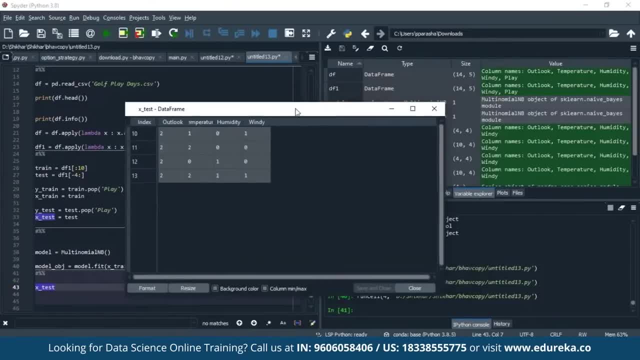 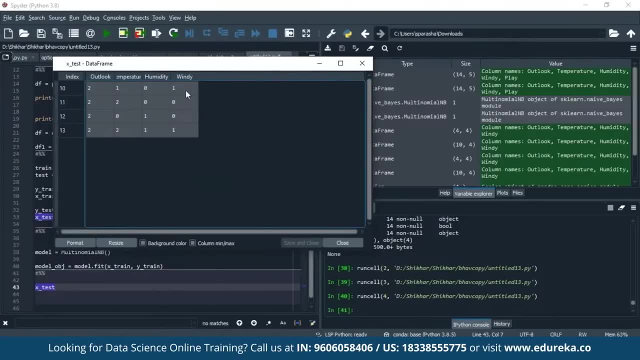 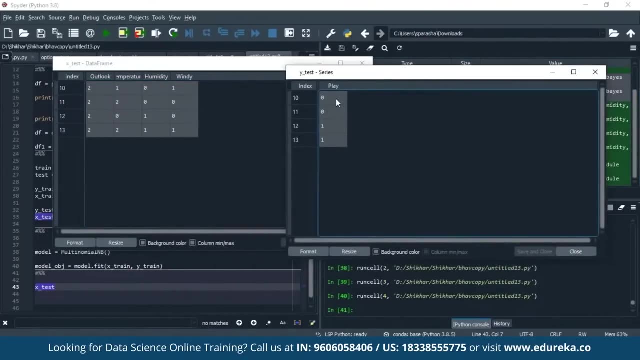 at our test data frame. this is our test data frame. We have three, four conditions. all four are sunny, high temperature, low humidity and windy Right. and if you look at their outcomes, these are their outcomes. on the first two days: plays not happening. on the next two days: plays happening. Let us look at what is the prediction of our 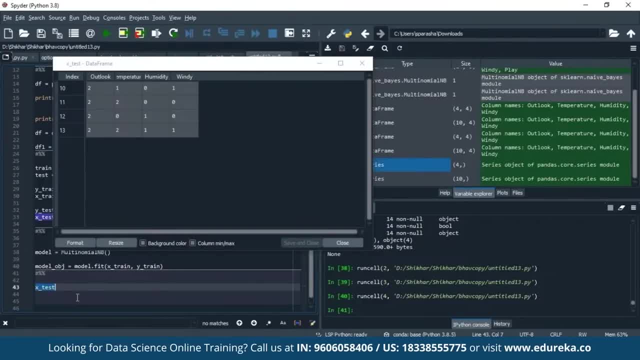 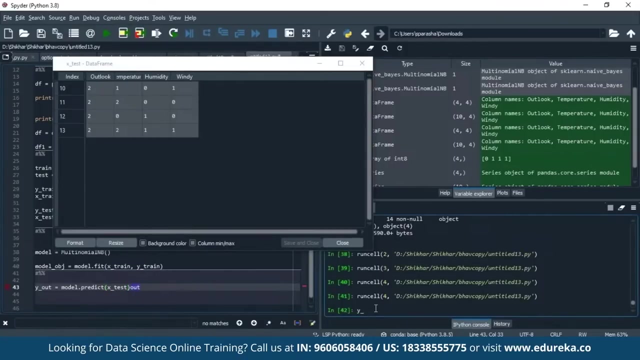 model for this. So to do that, what I simply do is X out is equal to model dot predict. to this I give my X underscore test. Here you go. Okay, Now you have your Y Y out variable. So this is the prediction for all the four inputs. 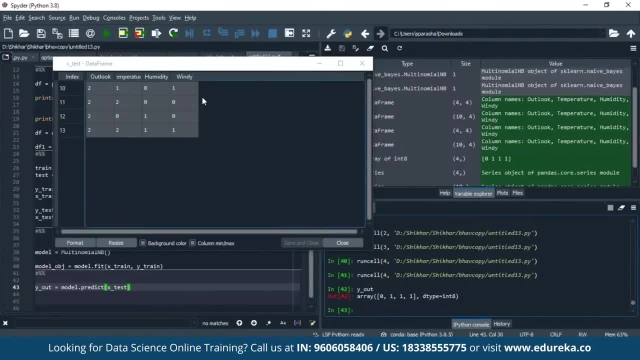 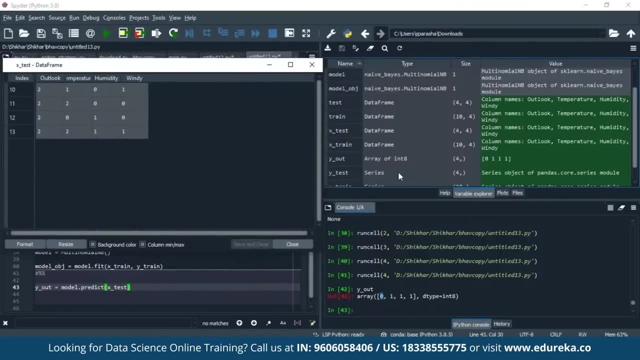 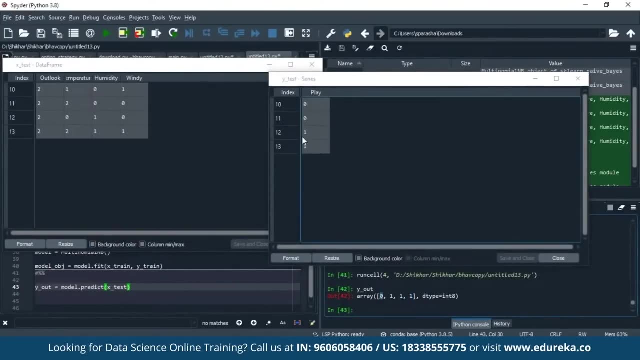 that you give and this is the prediction first day. first day, We say: play does not happen. Let us match it. Let us try to match it with our here. see, out of four records, three records. We are predicting correctly. three records, We are predicting correctly, If you want to. 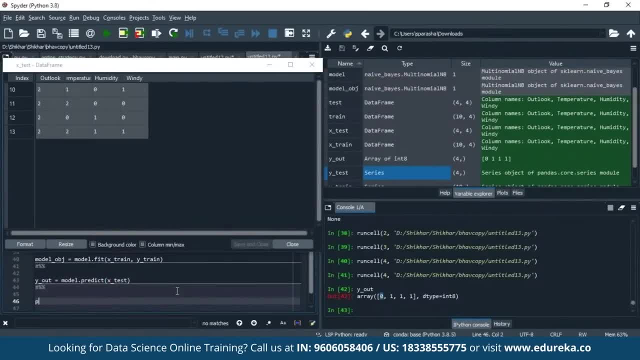 check, Check the accuracy. What is the accuracy of your model? What you can simply do is print. Let us print the accuracy on both training and testing. Training accuracy: How do I get the training accuracy? Very simple: model dot score. And here I give my X underscore train for my Y underscore train. 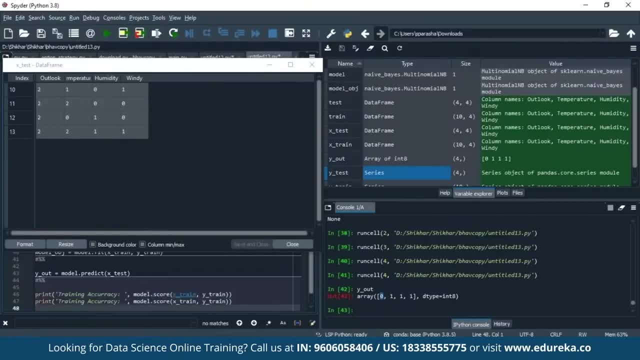 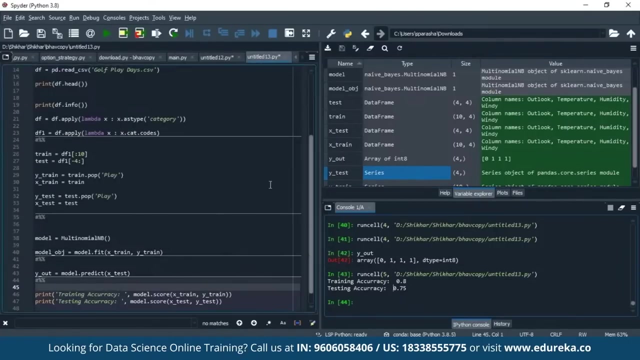 And then we do the testing accuracy also. Here you go. So here you can see, for our model training, We have 80% accuracy and for testing, we have 75% accuracy. Okay, So this is the advantage of doing this activity in Python. 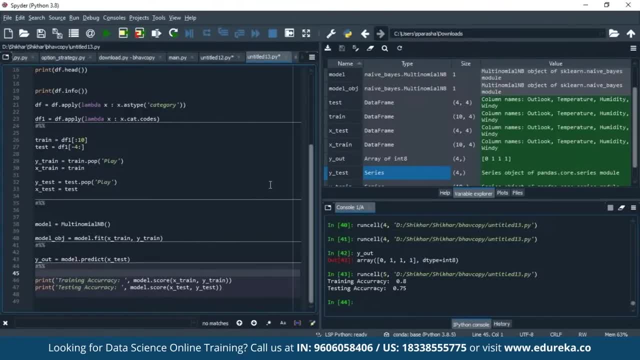 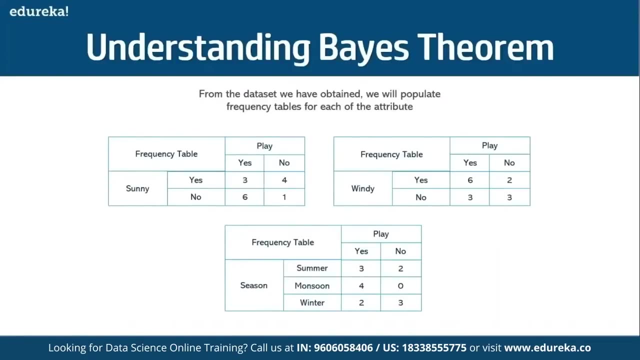 But what is happening in the back end? now let us go and also understand that, in terms of the knife bias classifier, we have successfully. we have successfully implemented the knife bias classifier in Python programming language. but here let us try to understand bias theorem. 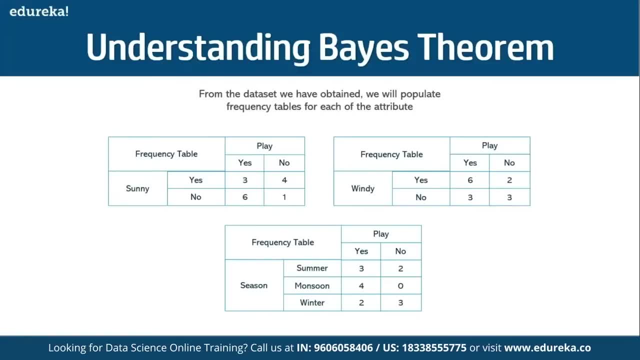 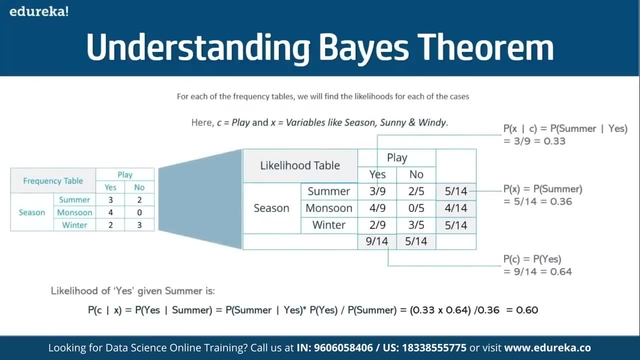 What is happening? So from this data set all the tabulated data frequency tables are calculated. Once the frequency tables are calculated, they are substituted in our formula to calculate the probabilistic scores. So what is the probability of Summer, given it is playing conditions total? 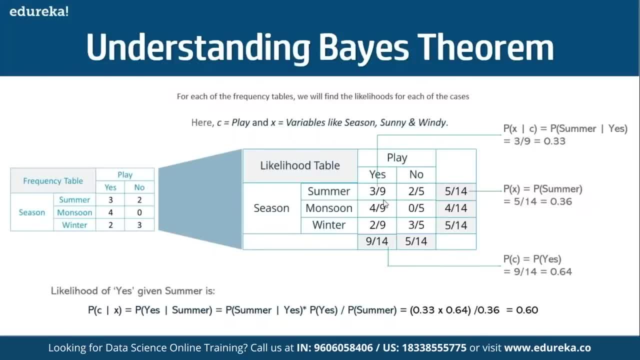 How many playing conditions are there? total: There are nine playing conditions. nine days play happened. that becomes our denominator. out of those days, How many days was summer is our numerator. That is how for this we get a probability of 0.33.. Then we calculate the class probability where we look at how many days was it summer out. 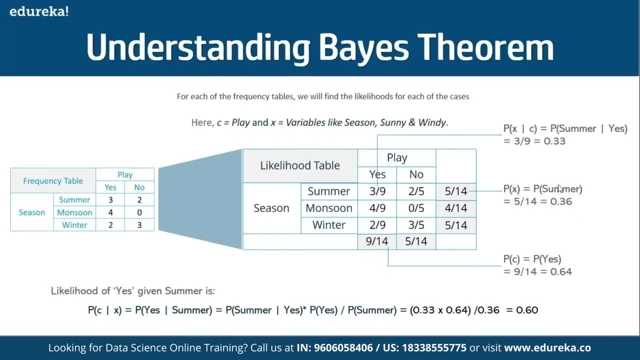 of total 14 days. five days was summer, So that's the probability and the class probability. That's the probability and the class probability is 0.64.. Put everything into our equation. put everything into our equation and this is what we get. 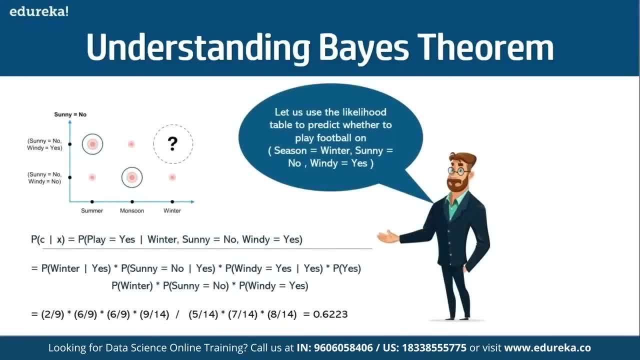 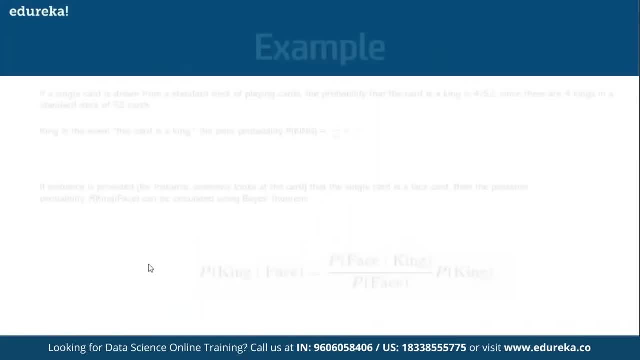 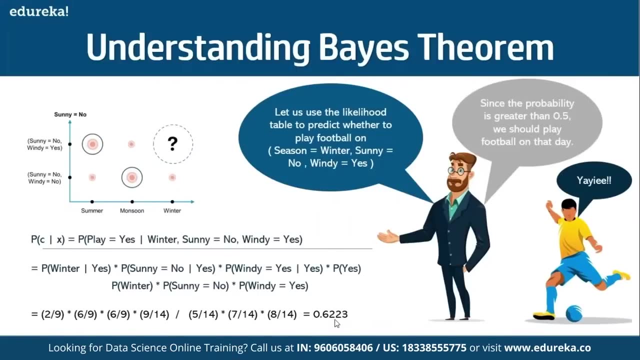 Okay, so we do this for each and every condition. So here we calculated for winter. All right, once we have done it for all three days- Winter, sunny and windy days- we substitute those here and that gives us the probability, which is more than 0.5 does. now we can say that if it is winter, sunny and conditions are sunny, 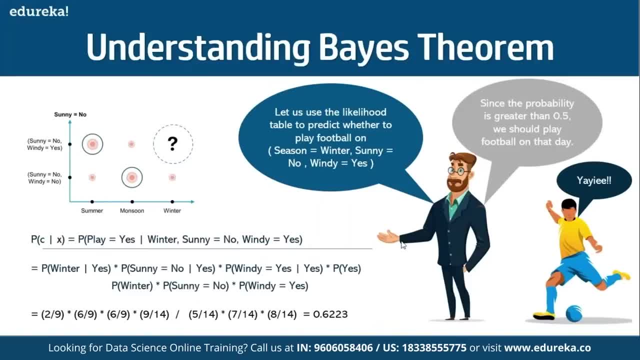 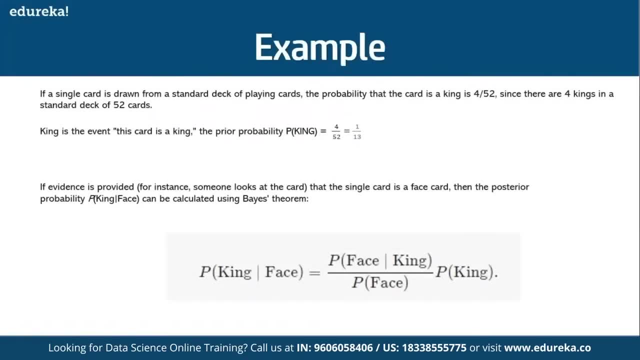 and there are winds. conditions are not sunny and there are winds, play can happen. Look at another example. If a single card is drawn from a standard deck of playing cards, the probability that card is a king is 4 by 52. since there are four kings in a standard deck, King is the event. 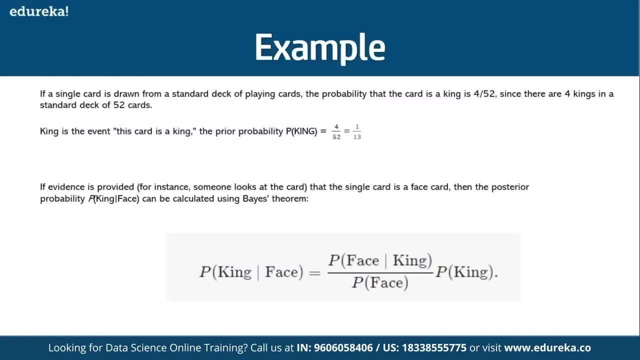 this card is a king. This is the event. the prior probability of this is 1 by 13. if evidence is provided- for instance someone looks at the card- that the single card is a face card, then the posterior probability can be calculated using bias theory. 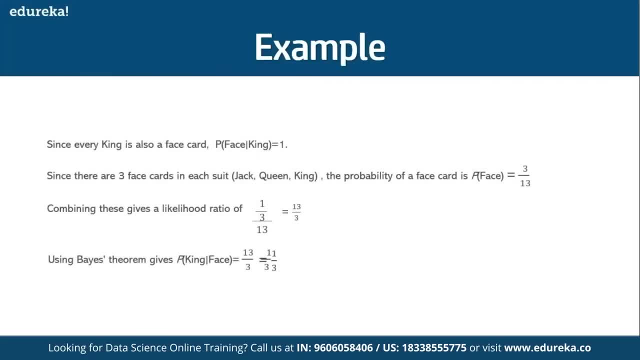 Okay, since everything is also a face card, the probability of face happening, given you getting a face card, given it's a king, is one. Since there are three face cards in each suit, All right, it's actually for Ace is also a face card. 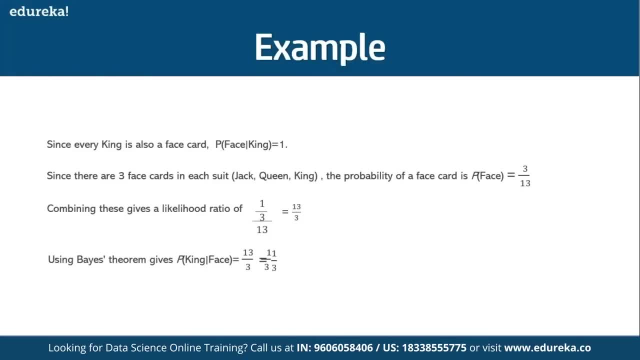 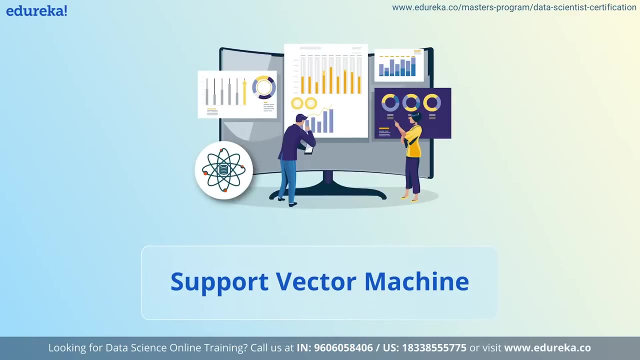 So it's Jack, King, Queen and Ace. the probability of the face card is 4 by 13.. Okay, So if you combine these three likelihoods, what you get is 13 by 4. so, using bias theorem, This is the probability that you get. 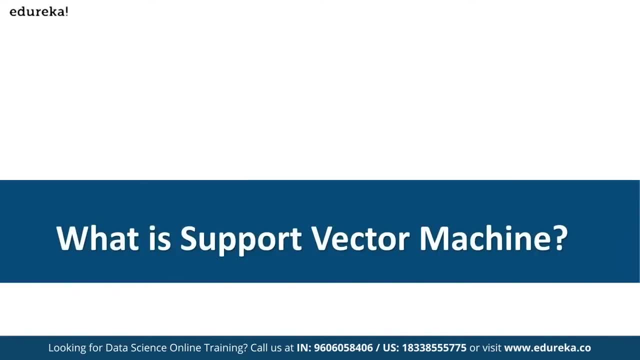 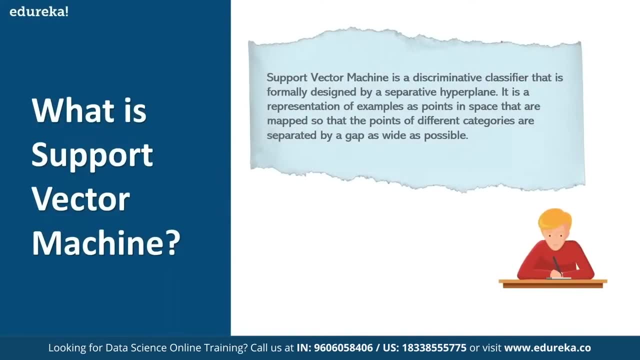 What is support Victor machine? Now, as you have seen already, support vector machine comes under supervised machine learning and we use it specifically for performing the task of classification. So support vector machine is a discriminative classifier that is formally designed by a separate hyper plane. 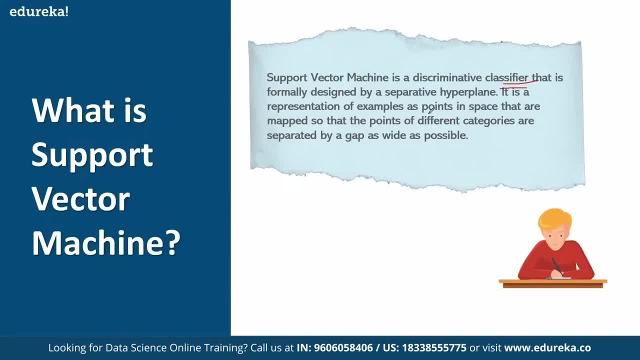 Okay, It is a representation of examples as points in a space that are mapped so that the points of different categories are separated by a gap As wide as possible. So in this case of the support vector machine, let's say I have some data points. 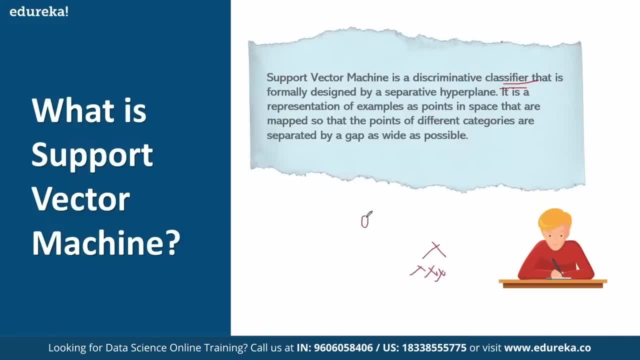 So there are some data points of X and there are data points of circle. Now this support vector machine is a type of machine learning algorithm where, if I have the collection of points, So here in this data points, I have two classes: one is X and the another one is circle. now 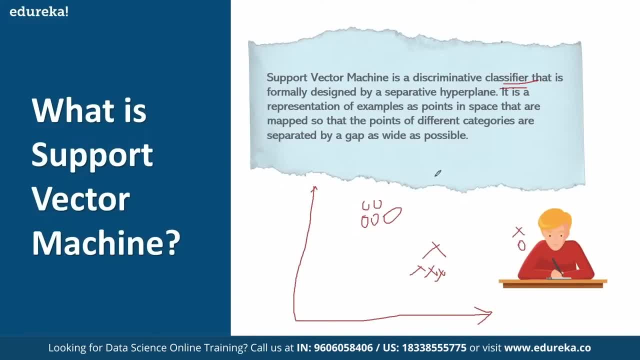 given this kind of data points, Okay, Given this kind of binary classification problem. So the expectation is, in case of support vector machine, I'm going to draw a hyper plane Which separates as much as possible. Okay, so I'm going to draw a hyper plane which separates these two classes as much as possible. 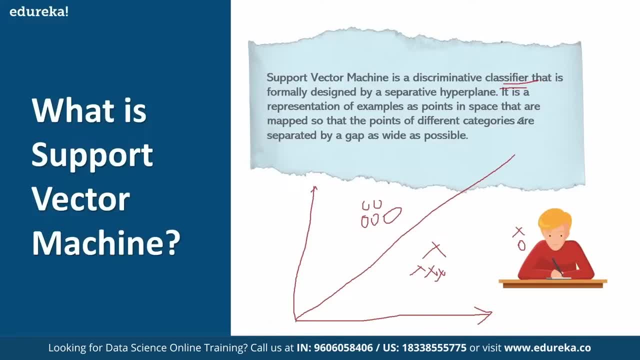 So it says that the I'm going to draw draw hyper plane And it will be separated by a gap as wide as possible. So that is the intuition behind support vector machine. Okay, now that you have an intuition behind what is support vector machine. 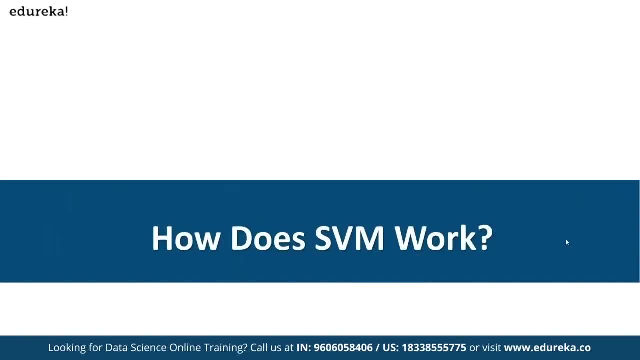 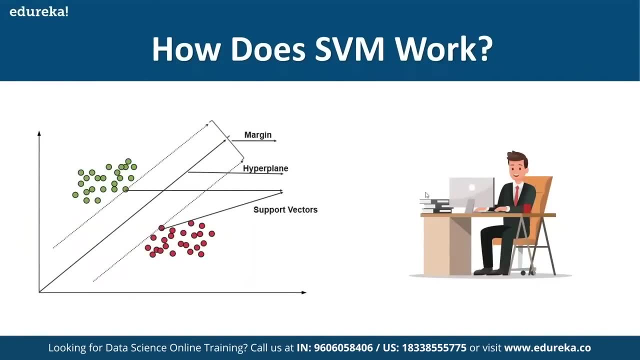 Let's understand, as how does this SVM, that is, support vector machine, would work? So in case of support vector machine? So here there is one more example. I have this set of points which is green, green curve- and I have another set of points which 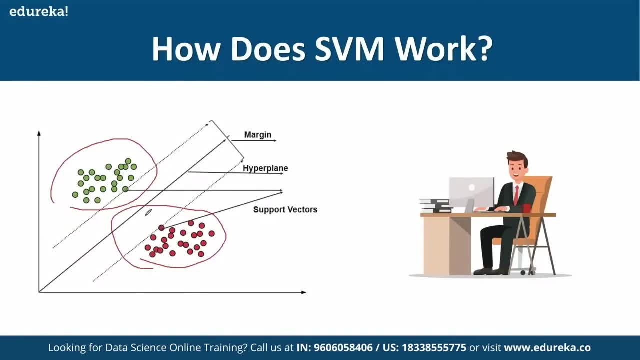 are in red color. So these two points are belonging to the different different classes. Now what I'm going to do is I'm going to draw a hyper plane which separates these two classes- data points- as much as possible, And when I'm drawing the hyper plane, I'll make sure that this hyper plane is as if this: 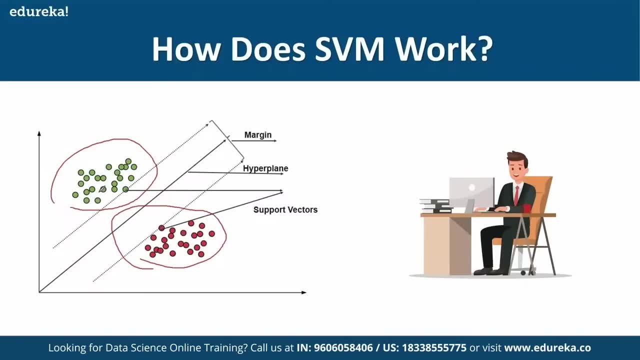 hyper plane is equidistant from my support vectors. Now, the support vectors is nothing But the point which is closer to my hyper plane. now, here, in this example that you're seeing, This data point and this data point are called as support vectors because these are the data. 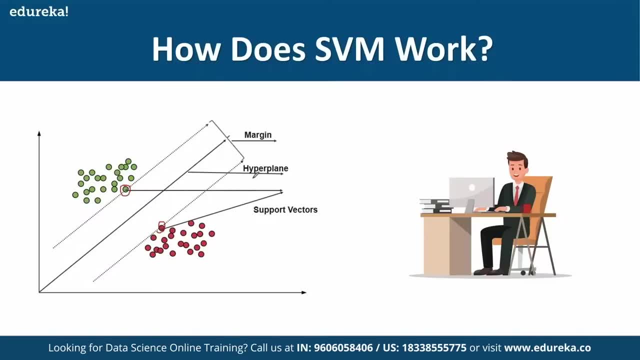 points which are nearest for my hyper plane that I'm just drawn in. if I am trying to make use of this SVM model, It is going to draw this kind of hyper plane to make sure that it is separating two classes, that two classes That we have over here in this example is red and green. 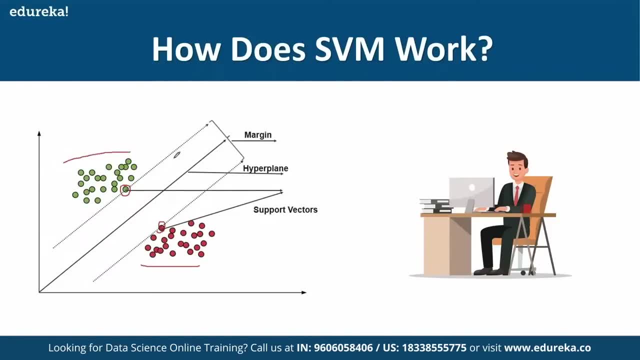 It is going to separate these two classes as much as possible and it will be equidistant from my support vectors- and the support vectors are nothing but the nearest point to my hyper plane- And that is how I'm going to separate between two classes when it comes to support vector. 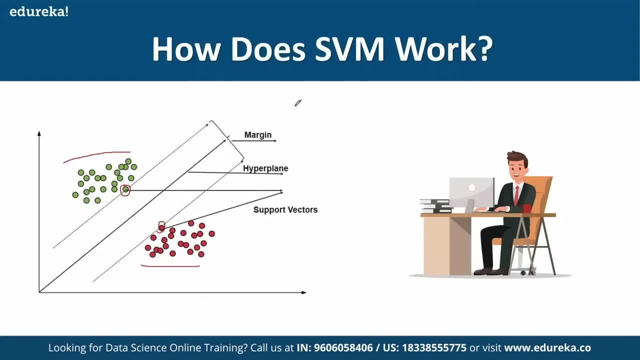 machines. Now here, in this example that you're currently seeing, the hyper plane that have just drawn- So this is a simple linear hyper plane- is like a straight line that I'm trying to draw if I want to separate two classes of data points. Now, apart from drawing this straight line, 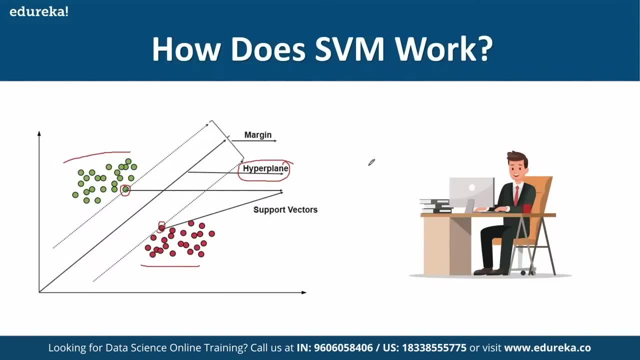 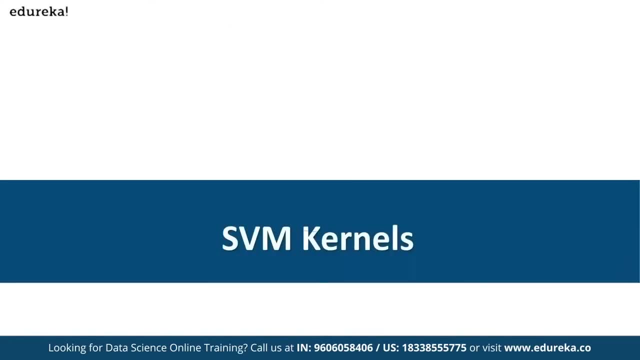 We also have other kind of lines as well which we can draw. So let's see how we can do that. So the types of line that we can draw or the hyper plane that we can draw is called as SVM kernels, that is, support vector machine. 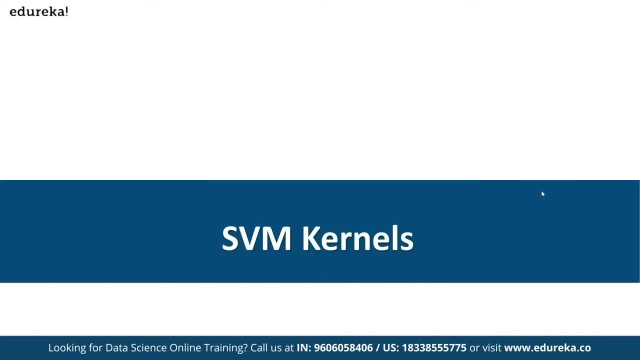 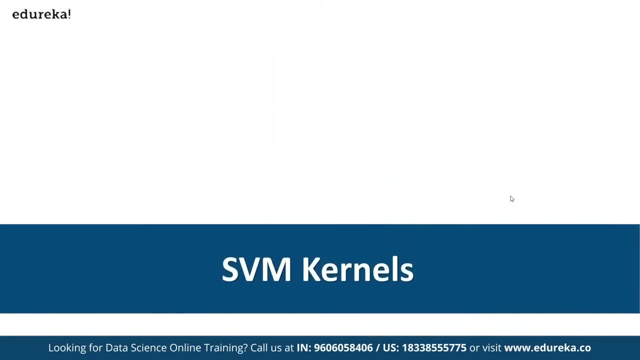 Kernels. the example that we have seen. It's an example for linear SVM kernels, So let's see What are the other types of kernels that we have. So, when it comes to SVM kernels, we have linear kernels, radial basis function kernel and along. 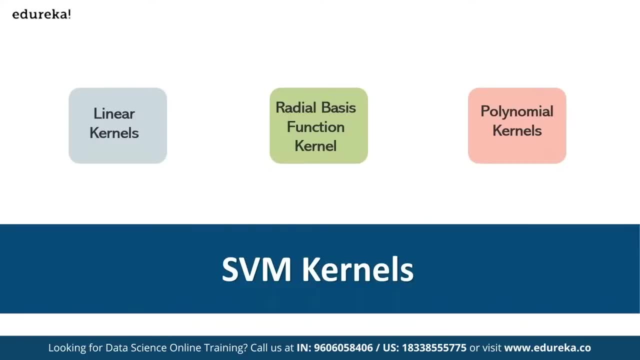 with that, We also have polynomial kernel. Now, in case of linear kernel, I'm going to draw a hyper plane which is like a straight line. in case of polynomial kernel, I can draw my hyper plane on the basis of polynomial function that I have created on. 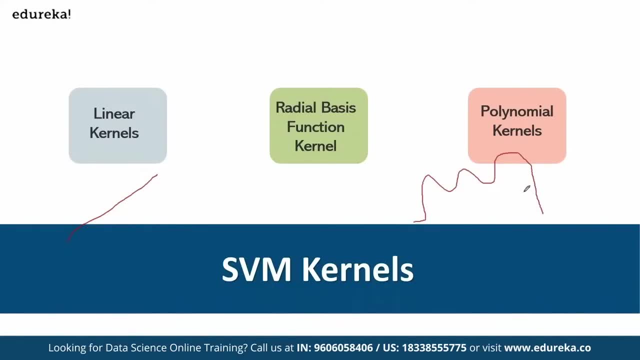 the basis of number of variables that I have and the degree that I have over there in case of polynomial and in case of radial basis function. So I'll make use of radial basis to separate my data points. Okay, so these three are the important kernels that we have in SVM and this is one of the 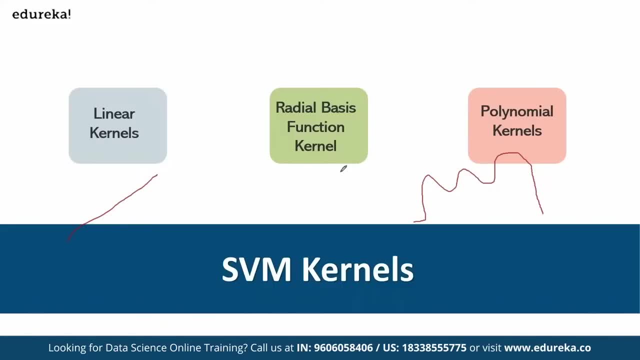 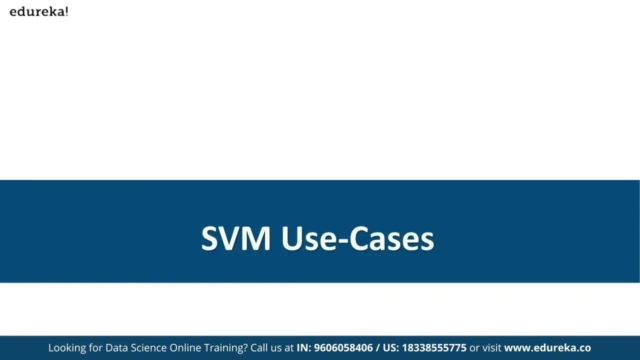 commonly asked interview question when it comes to the topic of support vector machines. Now let's look at some of the use cases, or the way we can do, where we can use this SVM to work. or let's look at some of the use cases where we can use this SVM. 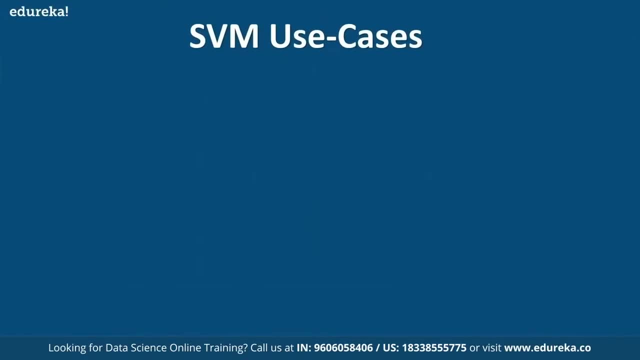 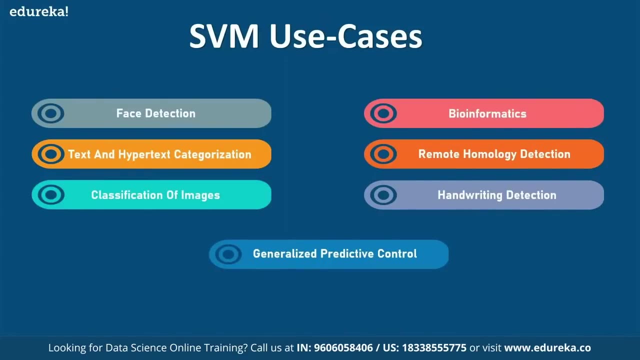 Okay, So we can use this SVM on many of the use cases. So, to name a few, we can use it in face detection. We can use it in text and hypertext categorization. We can use the SVM if I'm trying to classify any images I can make use in bioinformatics. 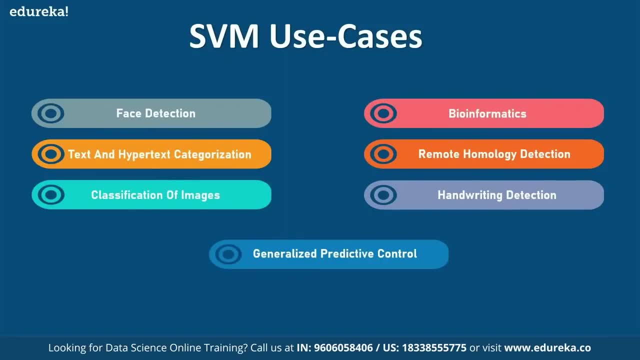 and if I'm trying to detect something, so I can in an example here- remote homology detection, handwriting detection or in general, we can make use of this generalized predictive control. So wherever we are dealing with the task of classification, we can use this SVM model. 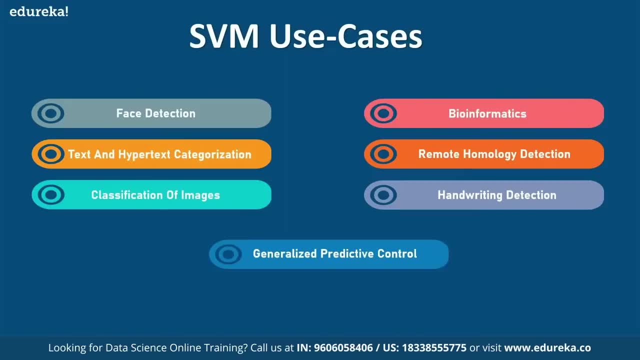 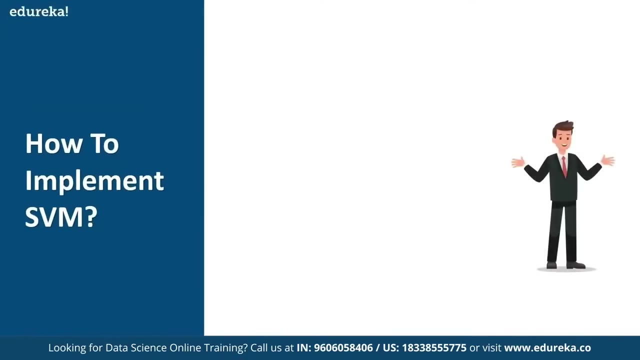 Okay, Now that we have a theoretical understanding as what is SVM and how it is actually going to look like and how it will be, Let's have a quick walkthrough as how we can implement this SVM. now to implement this SVM. These are the common steps that we are going to follow. 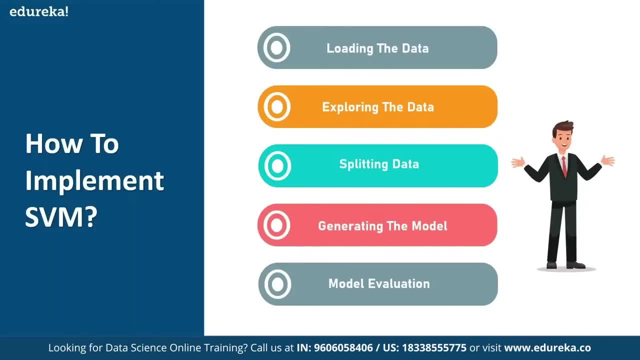 We are going to load the data, will explore the data, and once we have explored the data, We are going to split the data into two parts. The reason is simple: when I have training, So I'll be making use of my training data, and once my training is complete, 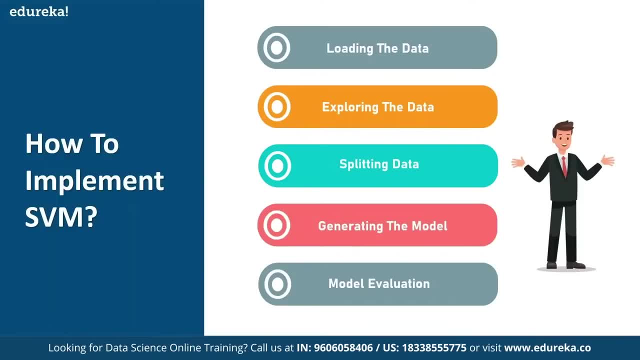 I'll check how my model has been trained with the help of my test data. So I'm going to split the data Now. once that is complete, we are going to train this SVM model and finally we can evaluate the model and observe as how model is working. 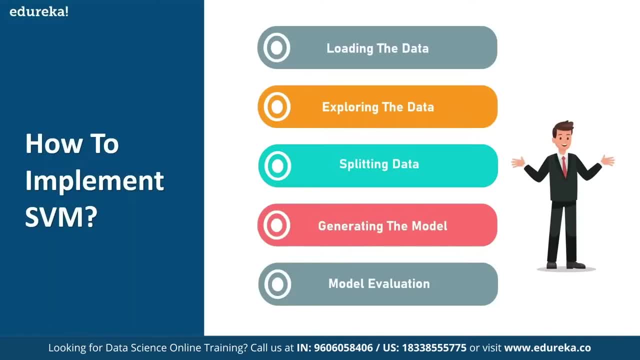 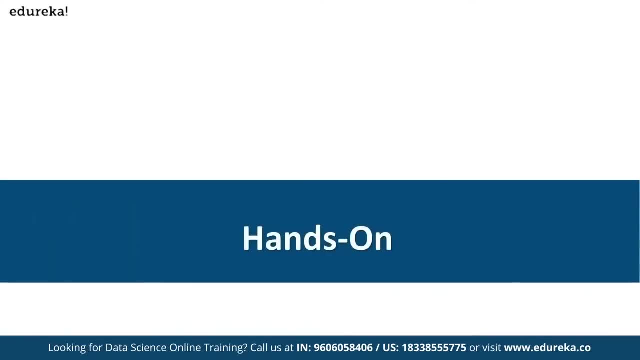 So this is the overview of the implementation of support vector machine. So let's do one thing: Let's walk it out and let's create the notebook in Google collab and let's see it in action as how we can implement this SVM. I'll come back to my Google collab. 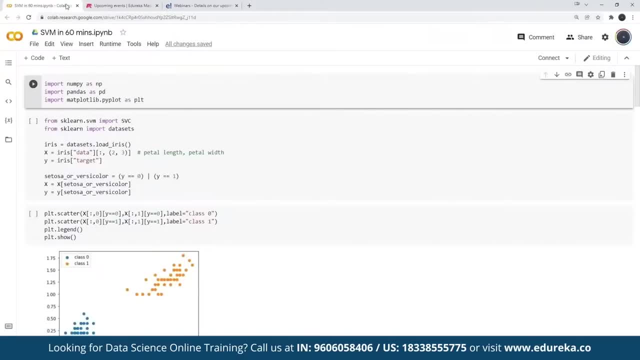 So this is the notebook that have already prepared, and I'll give you a walkthrough as we proceed along. now, here in my first cell, I'm importing my numpy library, pandas library- and along with that, for creation of plots, I'm importing My matplotlib library. 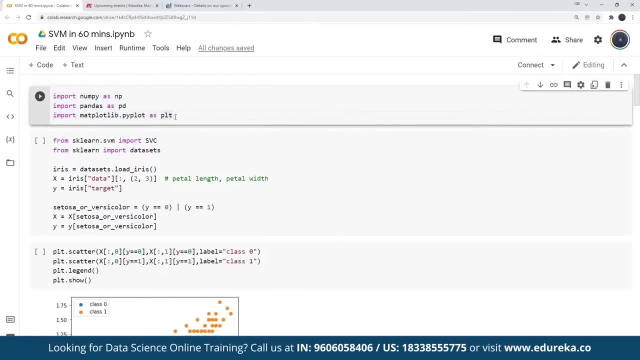 Now, if you are comfortable with seaborn, you can use the seaborn library as well. So in my example I'm just making use of matplotlib, because we are not interested in creation of visualization, but we want to understand as how model is being working. 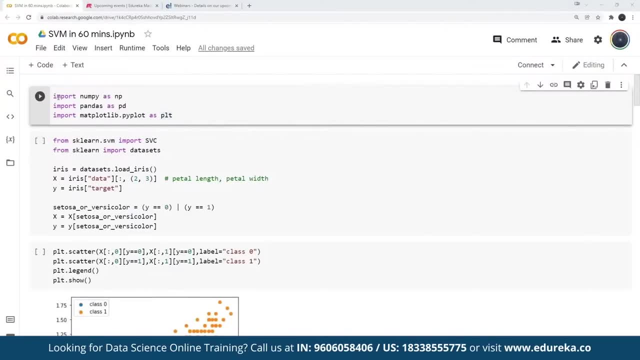 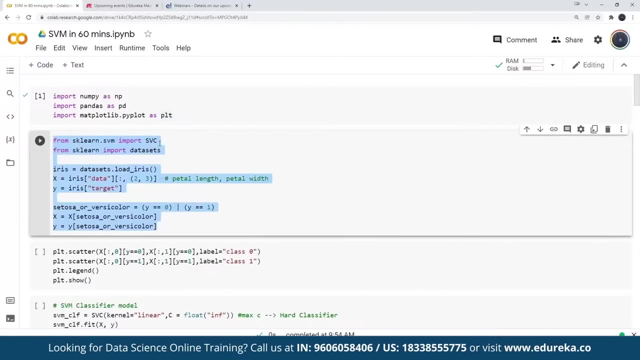 Okay, and I'm going to execute this cell. So this is going to take care of necessary imports. I'm importing my necessary libraries and once that is done here, I'm importing this SVM. So this SVM model is available inside my skill and library. 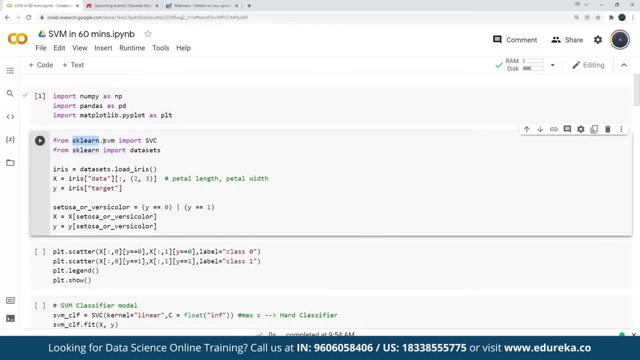 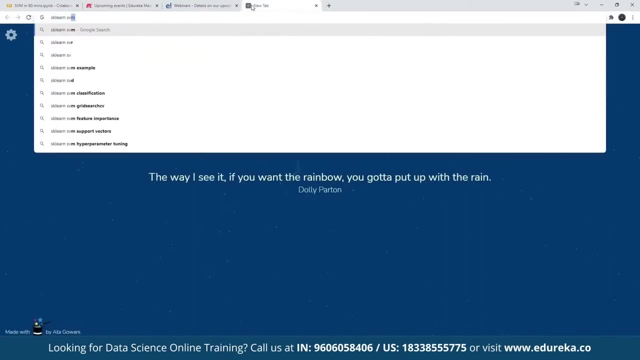 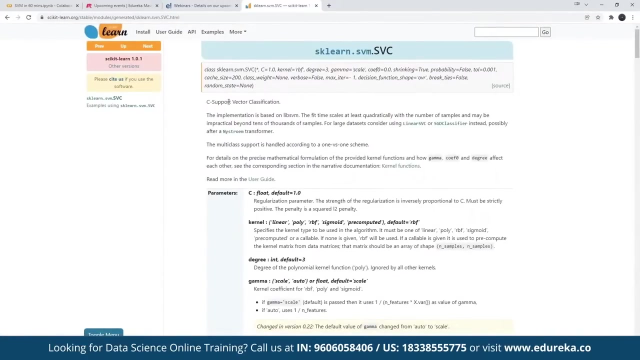 So I've mentioned as a skill and not SVM, and from a scale and out SVM, I'm importing my SVC. Okay, so I'm importing my SVC, So I'll show you what is this: SVC, SVM, SVC, So it's C means support vector classification. 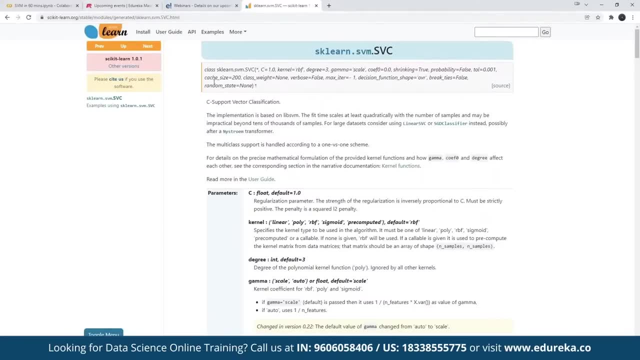 Okay, Now here, when I'm instantiating this SVC, I can mention what is the kernel that I want to use, and if I'm working with any polynomial kernel, then I can also mention what is the degree of polynomial that I want to use while performing the fit for my data set. 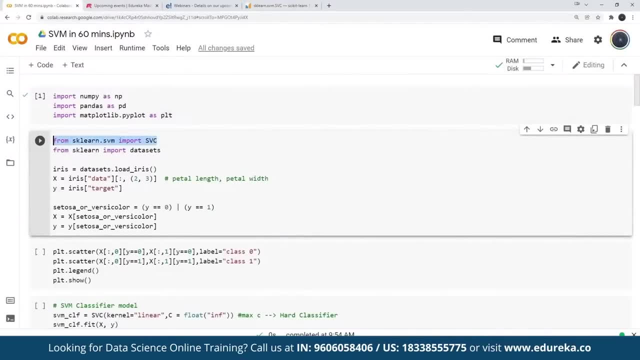 So I'm importing my SVC and along with that I'm also importing the data sets. So in the sk-none library itself we have a data set. So it skill and host already, like it actually skill and has many toy data set which will actually help us in our learning journey. 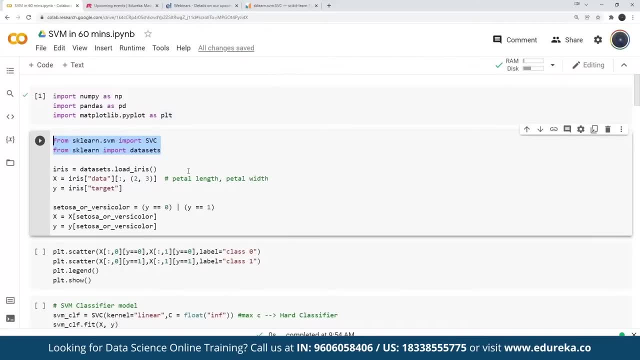 So we are going to use one of the data set, the famous iris data set. We use that for multi-class classification. So I'm going to load that iris data set and I'm just going to excite only two features. So the two features that I'm exciting is petal length and petal width. 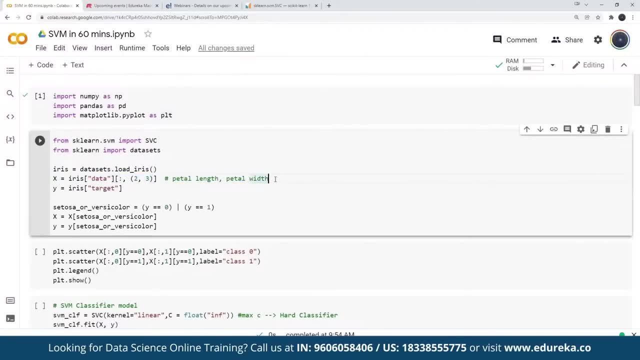 because I don't want to complicate it, I just want to visualize the data. So, in order to help in visualization, I'm just getting only two features of my given data and I'm separating my Y as iris target. So, whatever the target variable that I had, 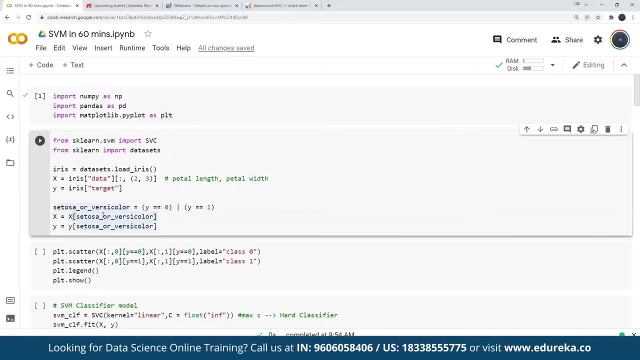 I'm assigning to my variable of Y. Then I'm going to do this: check whether it is setosa or versicolor. That means this default data set which is in multi-class classification. I'm just going to convert it into a binary classification task. 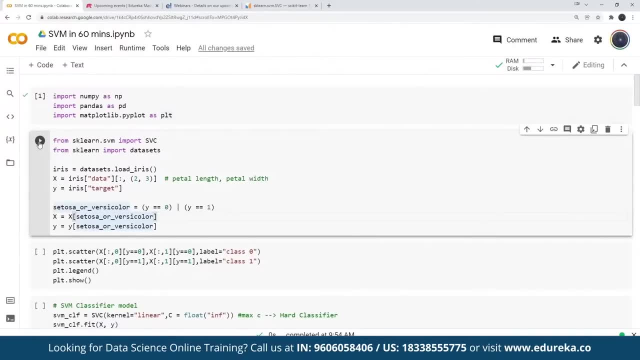 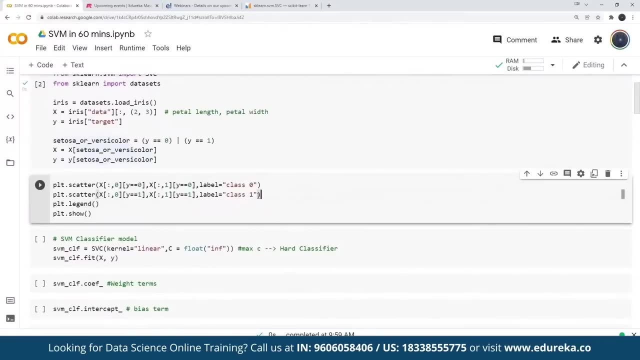 You'll get a better understanding once I execute this next cell. So this is going to prepare my data set, and once the data set is prepared, if I create a scatter plot. so I'm just creating the scatter plot to show us what and how my data set looks like. 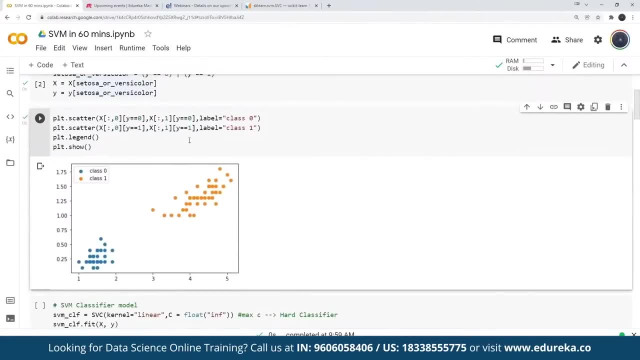 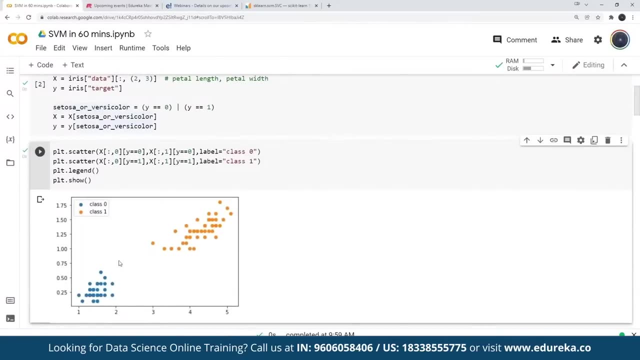 So this is how my data set looks like. on my x-axis, I think I'm having petal length. on my y-axis, I'm having petal width, and here the blue points refers to the class 0 and the orange points refers to the class of 1.. 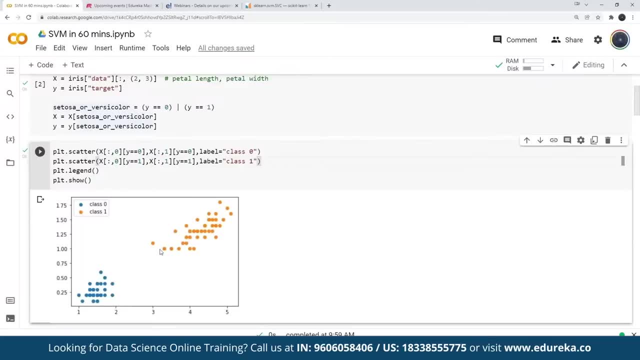 Okay, so this is how my data set looks like. You can clearly see that I have one set of points in one region and I have another set of points in another region. Now this is a classic example to understand about the SVM. How does it draw a hyperplane? 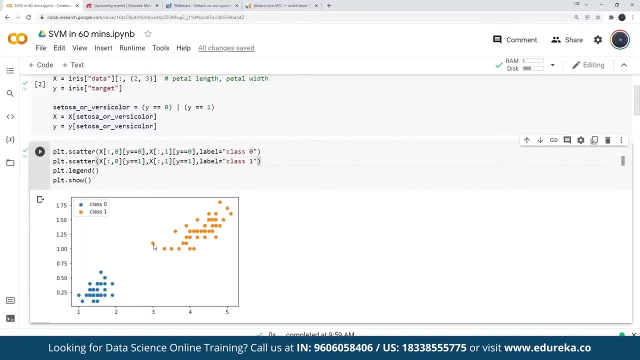 So we have the data set ready and, as I mentioned already, in order to fit this model. So when I say support vector machine, I'm going to draw a line. This line that I have drawn, it will be equidistant from my support vectors. 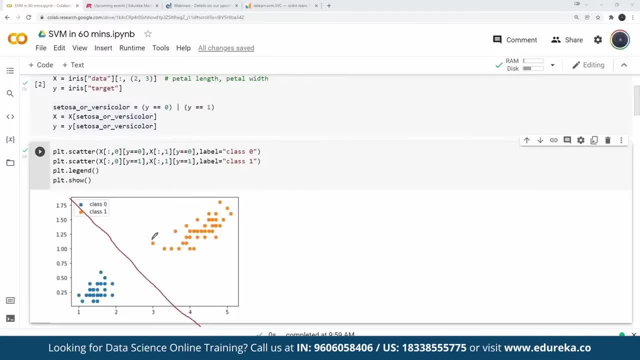 Now, here, in this example, the support vector is this: because this is the only point which is nearest to my line, And here I think this is the data point which is nearest to my SVM line, That is, this fisted line, hyperplane line. 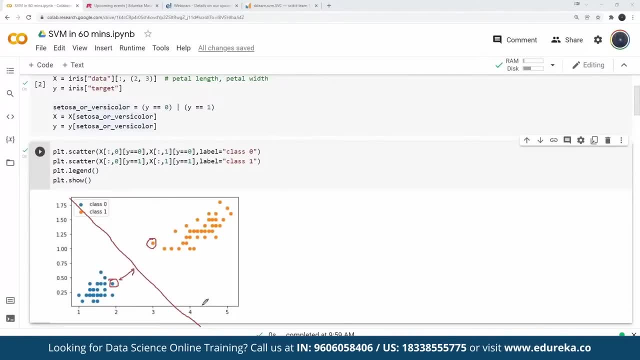 So I'll be placing this Hyperplane such that it is equidistant from the support vectors. That is how I'll be drawing this support vector line. So we now have an intuition. Let's see whether we get the same outcome as we are expecting. 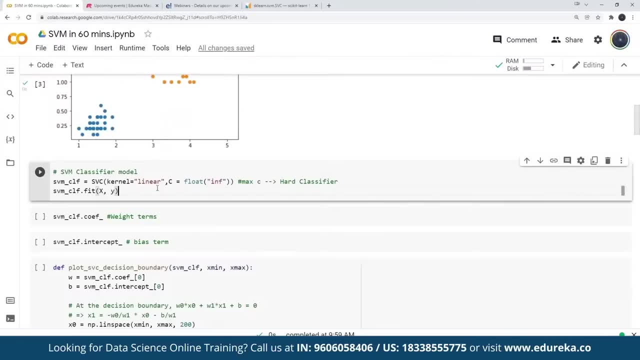 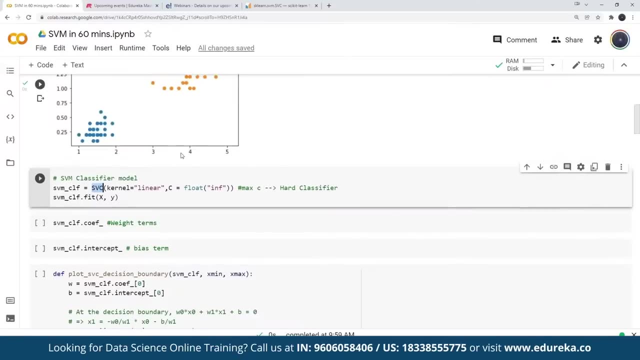 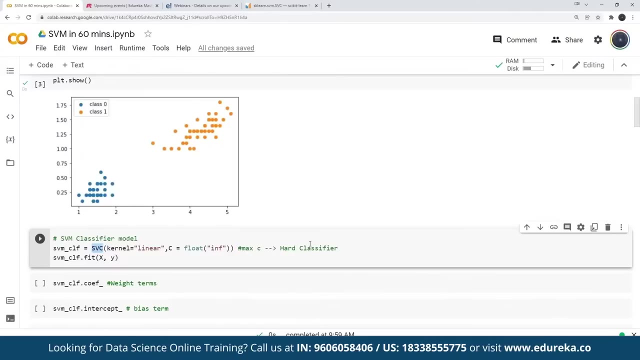 So here I'm initializing my model. So for initialization, I'm saying it as SVC: use the kernel as linear because I'm able to draw a line effectively We just seen- and I'm using the C as infinitive. That means it should be a hard classifier. 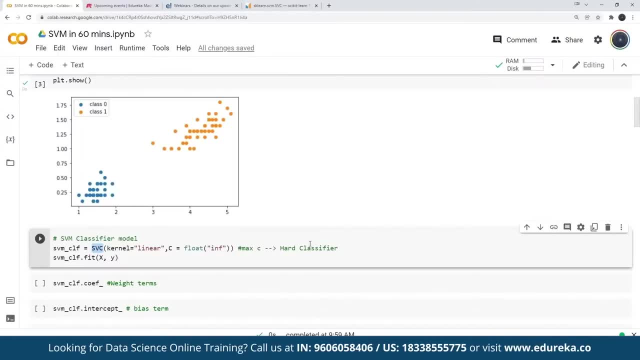 So hard classifier means I make, I want the hundred percent result. I mean I don't want any loose ends, I want to draw a line which passes, which clearly separates two classes. So I'm saying it as C, as infinity, to mention this as a hard classifier. 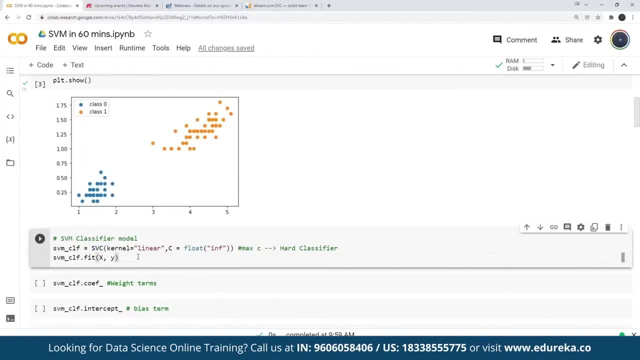 And once I initialize any model- here in the scenario SVM model- I am performing the fit on my data set. Now, this is the common flow that we follow whenever we are performing the fit, So we'll initialize the model and then we perform the fit on a data set. 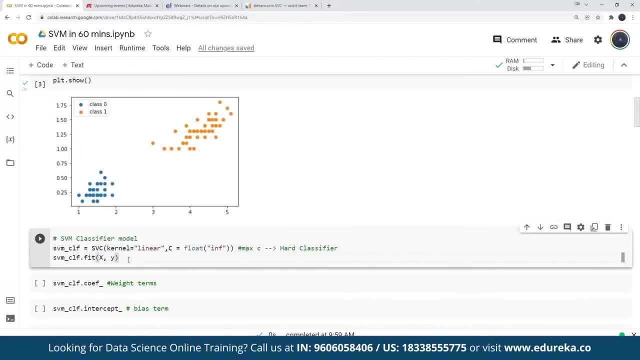 Now, since this SVM being a supervised machine learning model, I have to specify both my input X as well as my output Y. Hence SVM classifier dot fit X, comma Y. So this is going to perform the fit for my data set. I'll just execute this. 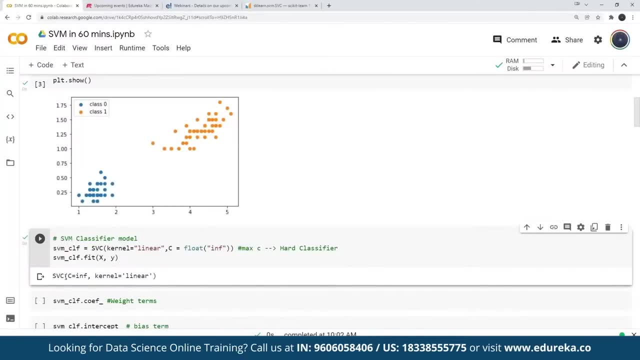 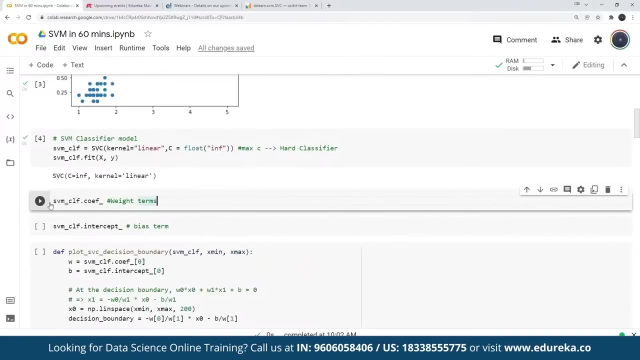 So this has performed the fit, and here it is giving me the confirmation, as this is the parameter that are being used to pop up the fit. Okay, Now, once I have drawn and once I have found this fit, next, if I want to display the weight terms, 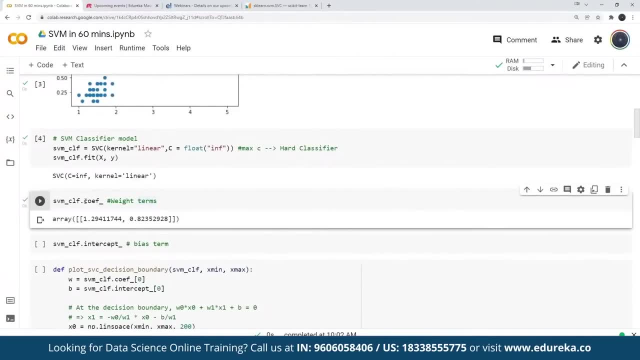 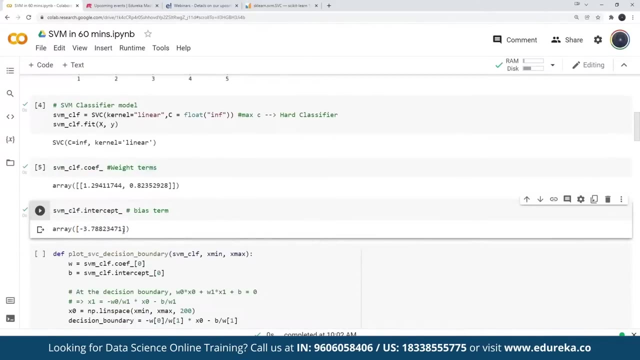 so I can say it as SVM classifier: dot coefficients. So these are the weight terms and if I want to display my bias, them or the intercept, it is minus 3.78.. Now this means the line that have just drawn. So that line has the, that line has the C term as, or the W not term as minus 3.78. 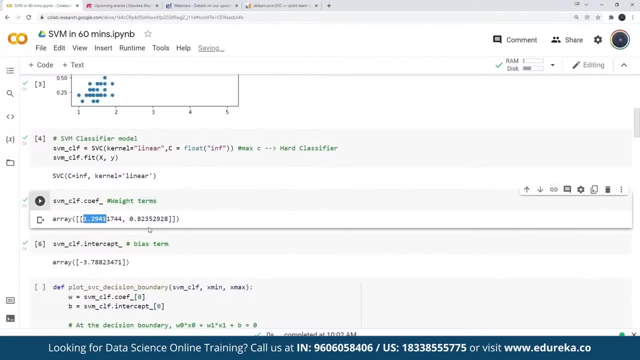 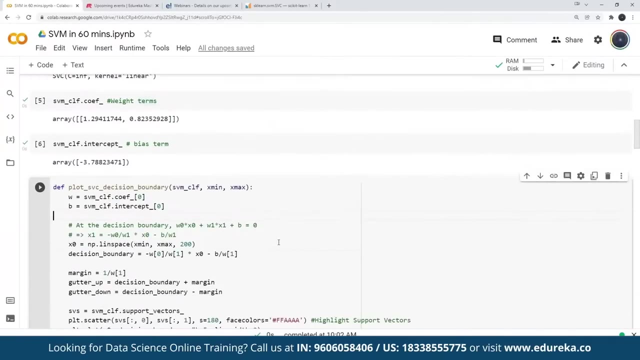 and W1, W2 are 1.29 and 0.82 respectively. So that's how that data is distributed for us. That's how the values has been found for our scenario. Next, in order to get the balance, for better visualization here: 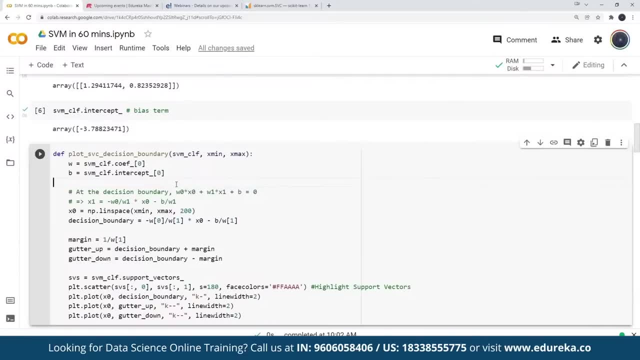 I have created a function that is called as plot SVC decision boundary, and this takes my SVM model. the X min and the X Max, Now W and B. I'm extracting from the coefficient and the intercept parameter that we have over here. So we are extracting from this at from this attributes. 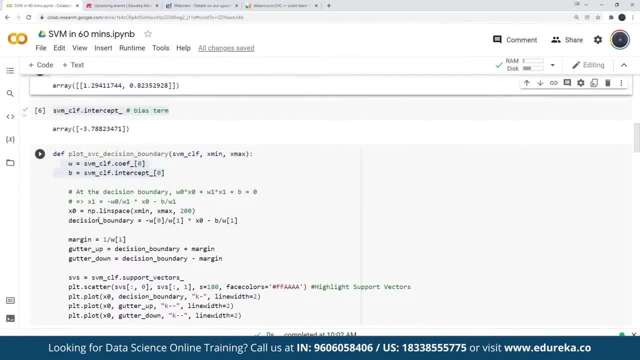 that we have from this model. And now, if I want to draw a decision boundary, so I need the set of points. So, in order to get the points, I'm saying it as X naught is equal to NB dot Linspace, X Max from X min. 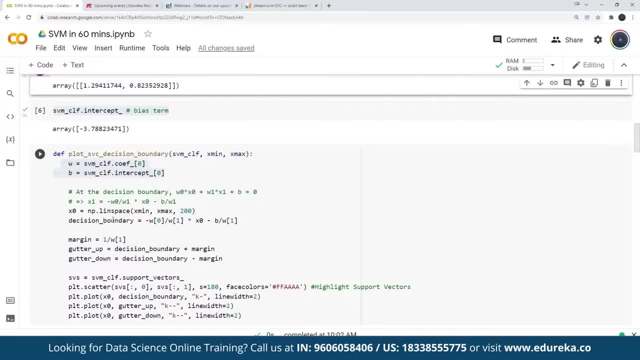 comma X, Max comma 200, and I'm specifying as how does my decision boundary should look like? my decision boundary is given by W, naught into X. naught plus W1 into X. 1 plus B is equal to 0.. So this is what my decision boundary would look like. 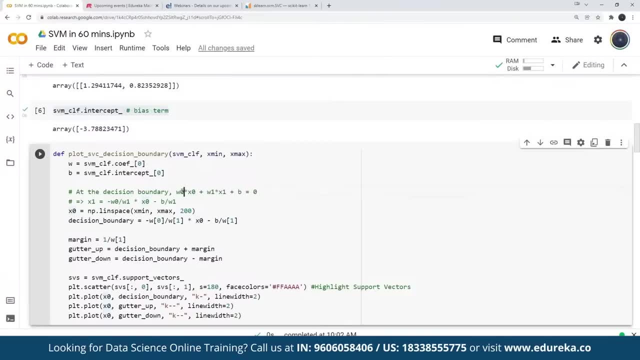 So I know what is X naught, I know W naught, I also have W1 and I also have B, So the only term that I do not have is my X 1.. Okay, So the only term that I do not have over here in this example is X 1. 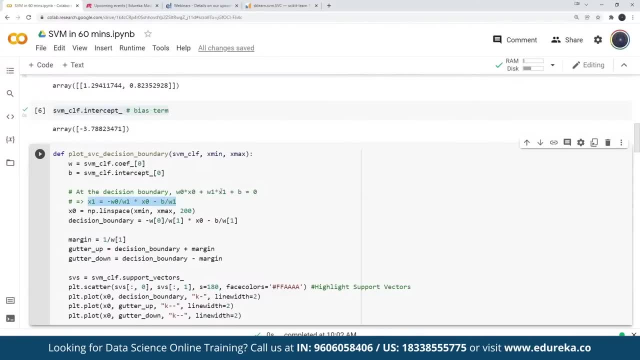 and the X 1 if I want it, So I just have to substitute it. So X 1 is equal to minus W 0 divided by W 1, into X naught minus B divided by W 1.. Now I am specifying the same equation over here for my X 2.. 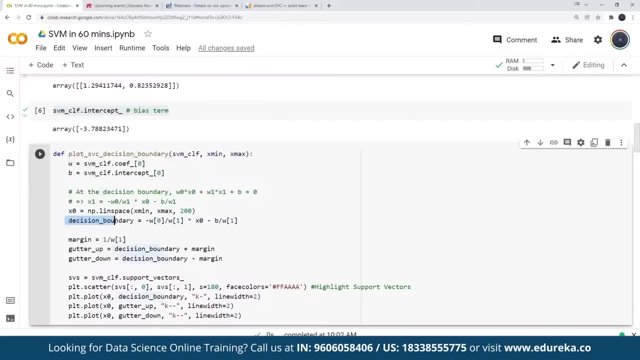 So my X naught and the decision boundary will give me the pair of input and output. Okay, Now, along with this, there is a property in SPM. Okay, So the property is given by whenever I have a margin. So that margin is given by 1 over W 1.. 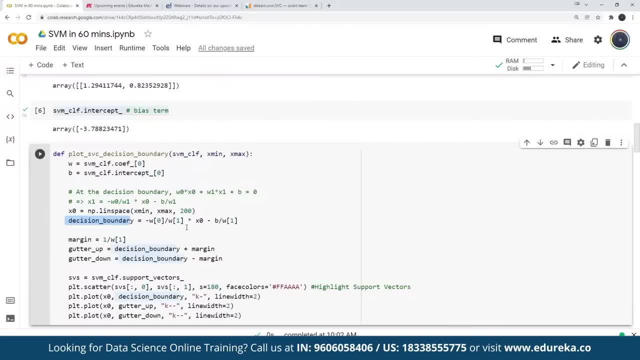 Okay, So the margin is nothing but the distance between my hyperplane and the support vector. So that is given by 1, by W 1.. Okay, Hence I have mentioned as gutter up and down. Gutter up means one line or the one line where the support vector lies. 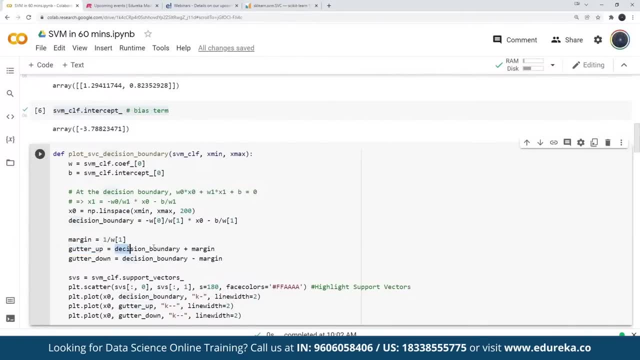 So that is given by decision boundary plus margin and one line below my support, One line below my hyperplane. That is where another support vector would lie. So I mentioned as decision boundary minus margin. Okay, Then I'm defining where exactly my support vector is. 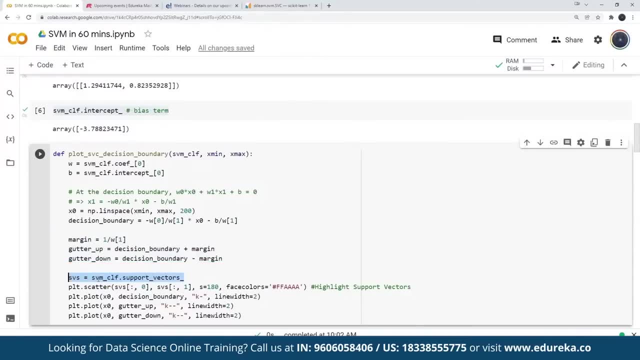 Where exactly my support vectors are present, My support vectors. I can access the support vector coordinates by saying it as by accessing the attribute of my train model: support underscore, vectors, underscore. Now I am specifying where exactly those support vectors are present with the help of a simple 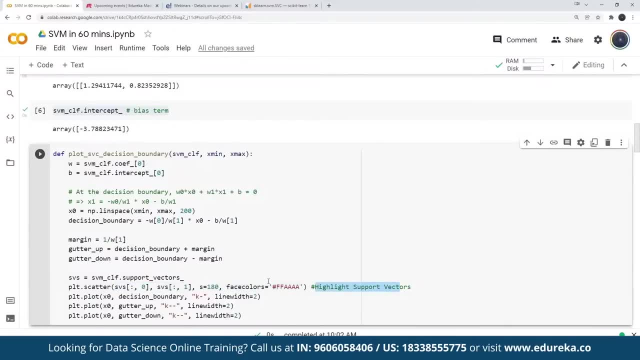 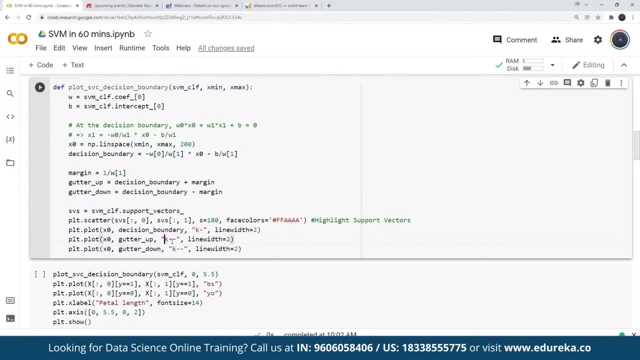 scatter plot by highlighting my support vectors and I'm specifying where exactly my decision boundary is present, And I'm also mentioning Where is my line, that is, gutter up and gutter down. So let's do one thing: I'll just execute this. This is going to create me a function. 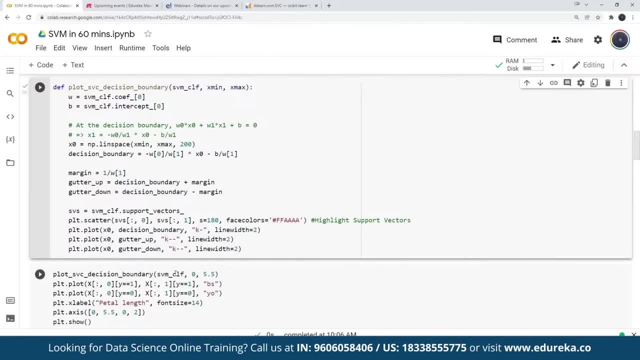 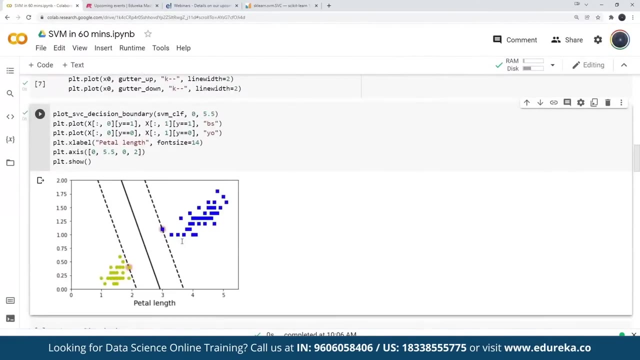 I'm going to call my function support vector machine classification, and I will specify my range of X and Y as here: Yeah, X min and X max as 0 comma 5.5.. I'll just execute this. So what we have done just now is we have created a function. 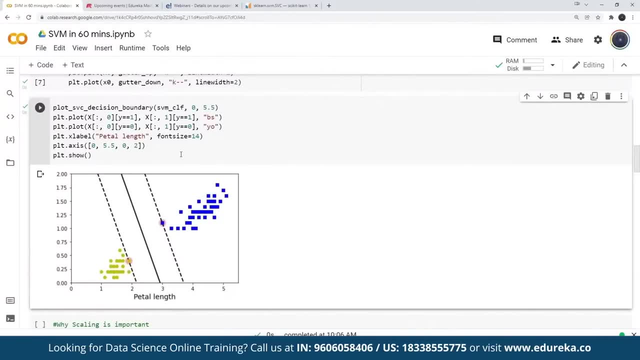 We have created this hyper plane, So the middle one, the solid line that you're seeing over here. So this solid line is called as your hyper plane and these points that you're seeing over here. So these two points which are highlighted, these two points are actually called as support. 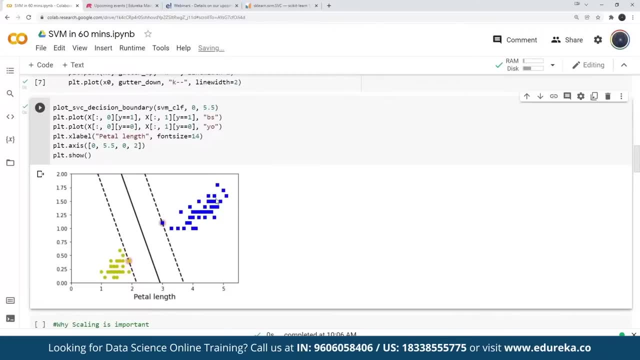 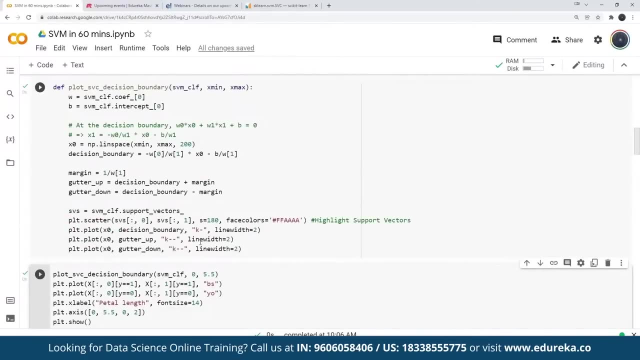 vectors. Okay, so this dotted line that you're seeing. so this dotted line refers to my gutter up and gutter down, which have found right here. Let's do one thing: I'll add some labels so that you'll get some more visualization in the plot itself. 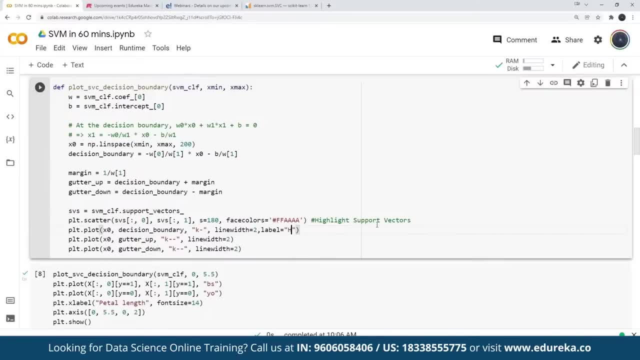 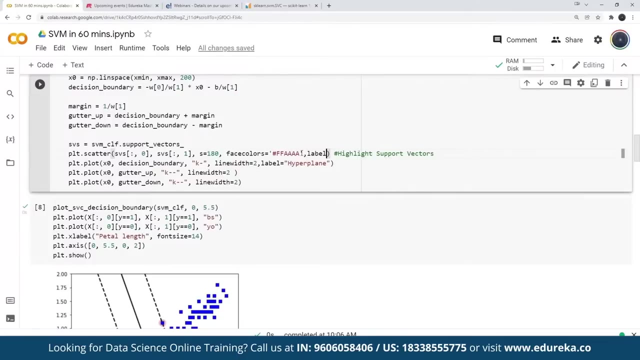 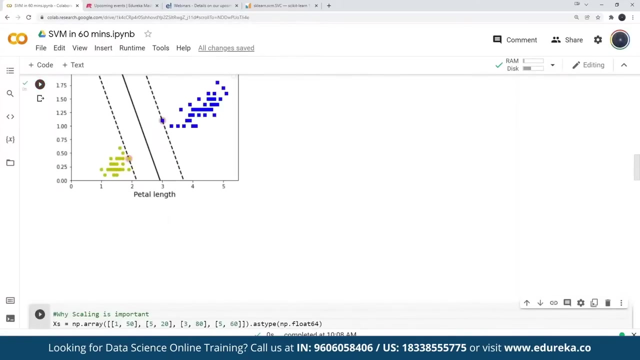 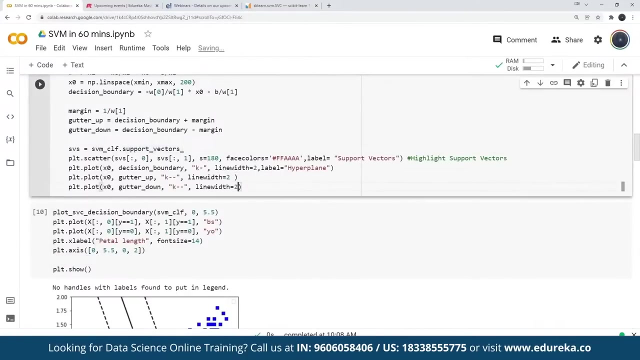 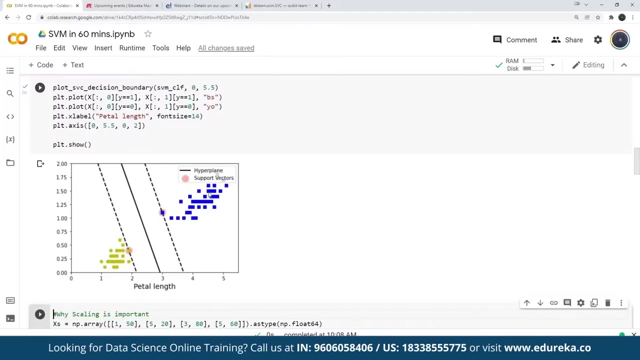 I'll say label and I'll mention it as hyper plane. Okay, and there is one more. Yeah, These are support vectors And I'll say PLD, not legend. So This clearly says which are all my hyper plane and which are all my support vectors. 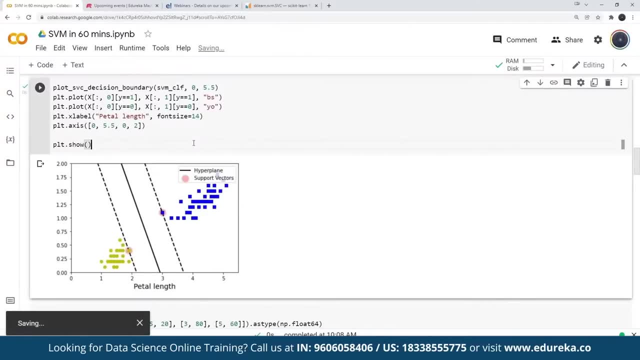 So this is the intuition behind support vector machines. So we'll be drawing a hyper plane which separates the points that we have. Okay, and whichever the point which is nearest to my hyper plane, We call that point as a support vector. now to access that support vector. 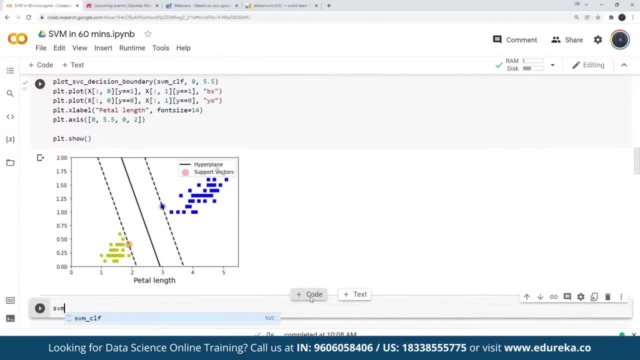 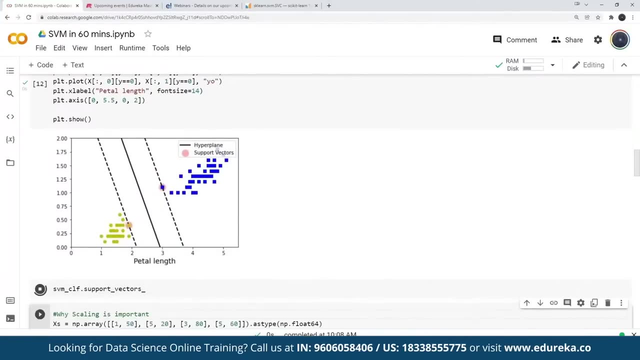 We make use of the attribute. So let's do one thing, Let's explore the same: the attributes, SVM, dot, support, underscore, vectors, underscore. So this is going to tell me where exactly my support vectors are present. So one point is given by 1.9, point 0.4.. 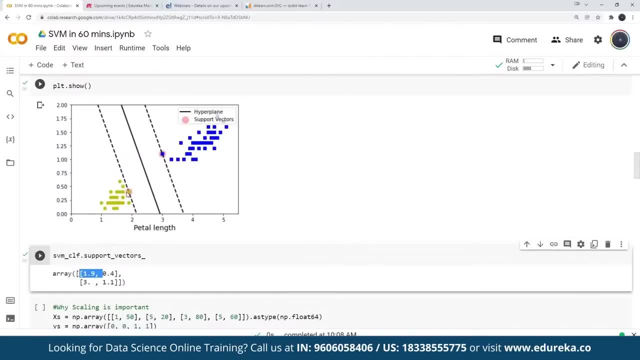 I think this is the point that I'm talking about. and the another support vector that we have is at the location 3 comma 1.1.. So 3 and 1.1.. This is where we have another support vector. So, using all these attributes, 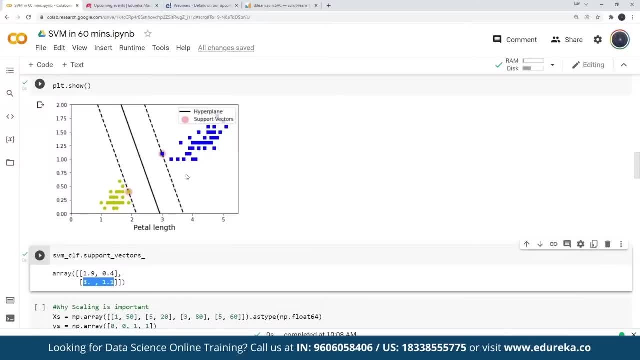 We have been able to create this, This visualization, Okay. Now, whenever we are working with the support vector machines, it's very important that we scale the data first. If I do not scale the data, I'll not be able to get a better fit of my SVM model. 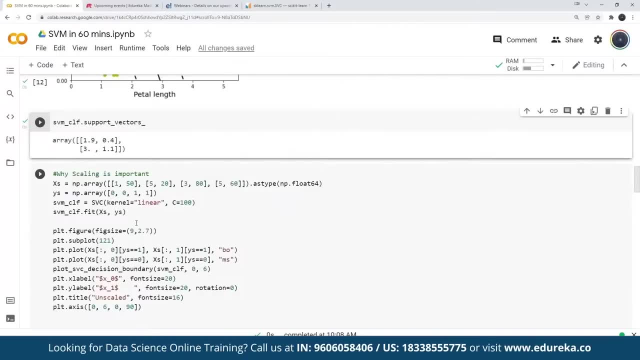 So here I've given one more example where I have my X is given as 1 comma 55 comma 23 comma 80, as you can clearly see. Okay, It's, it's not scaled. Okay, So I'm going to execute this cell. 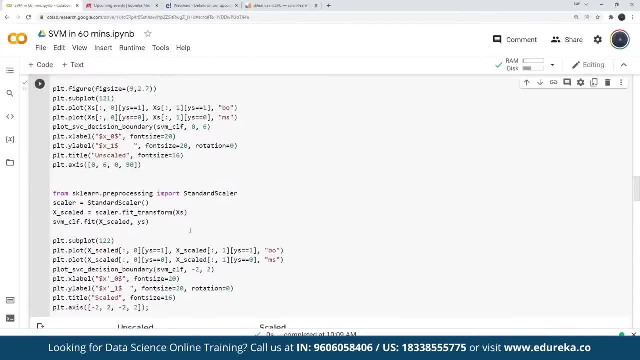 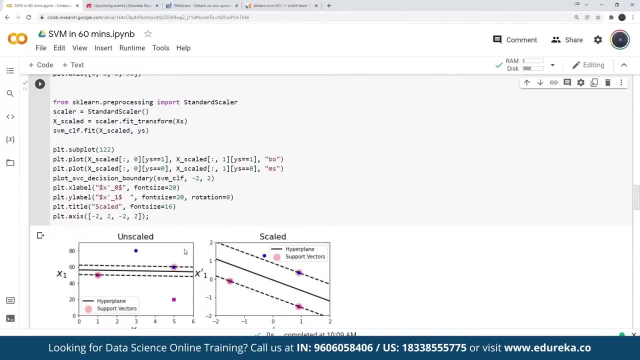 So this is going to tell me and give me a visualization as how the fit will be in case of scaled and unscaled. See, if it is unscaled, I'll. if it is not scaled, Okay, That means if it is unscaled, we can clearly see that the hyper plane that I'm drawing and the distance from my hyper plane. 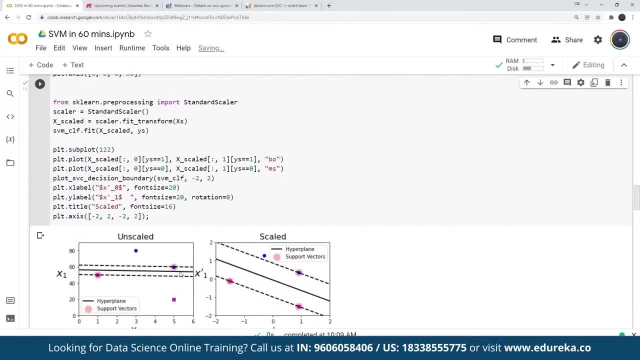 It's very close to each other, Very close to each other, And whenever I'm working it's. it will be difficult for me to separate those two data points, But if I scale them correctly. now, here for scaling I have made use of a scalar standard scalar. 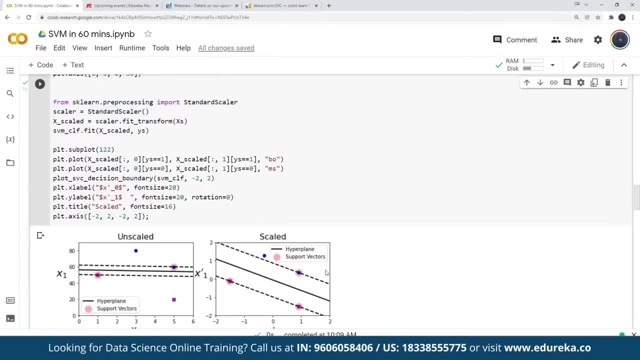 Now, if I scale it correctly, then in that scenario it will be easier for me and it would actually work better when I have scaled data. Okay, So this is about using the linear SVM model to perform the fit on my given data set. 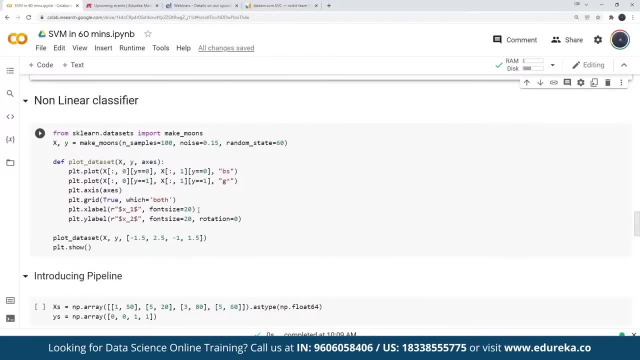 Now, if I go below, we have some more examples about nonlinear classifiers as well. Now, in order to test out the same here, I'm creating an example data set, and that data set that I'm generating is called as make moons data set. 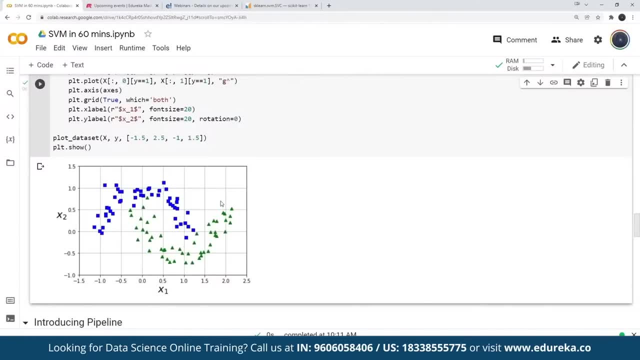 And this has been generated with the help of a skill and data set generator. Now, as you can clearly see, I cannot make use of linear classifier, So linear classifier is nothing but a classifier. Okay, which is an SVM model where I'm drawing or where I'm using a straight line to split my data points? 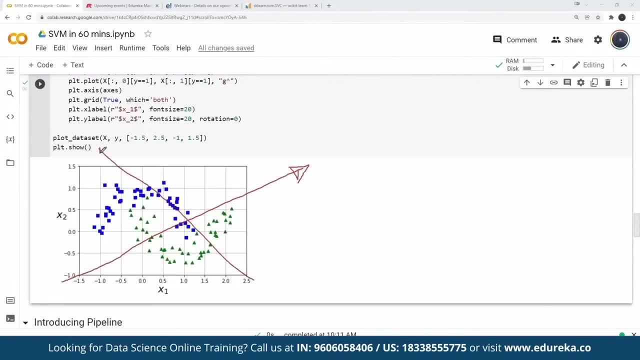 I can clearly see that I, wherever I join or wherever I try to draw a line over here, I cannot split the data in an effective manner. Now this brings us the challenge. Now, if I have a data set in this way Where I cannot linearly separate it, 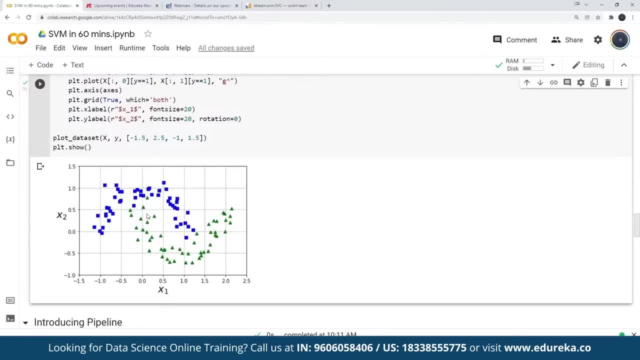 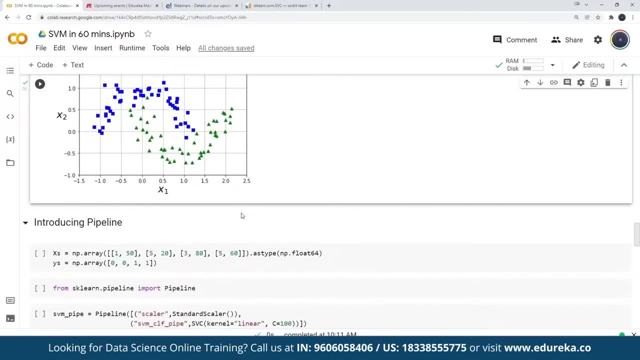 How can we go about and fit, perform the fit on our SVM model? So, in order to save us, we have a model that is called as SVM model and from that SVM model We can actually create a polynomial, polynomial kernel. so we can make use of polynomial kernel and using that polynomial kernel, 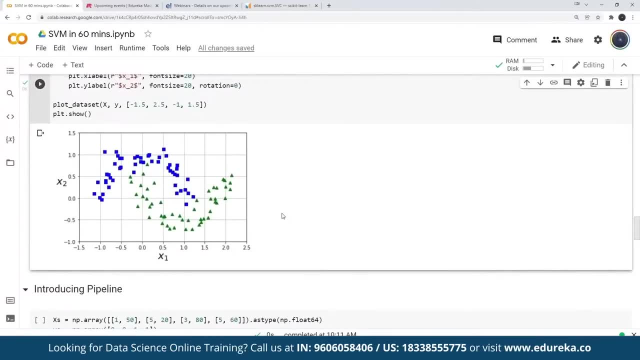 I can actually create it like this. I mean using polynomial kernel. I can perform polynomial kernel Regression, Or I can draw a line like this now to show you how it works: I'm getting some data like this, So this is some random data. 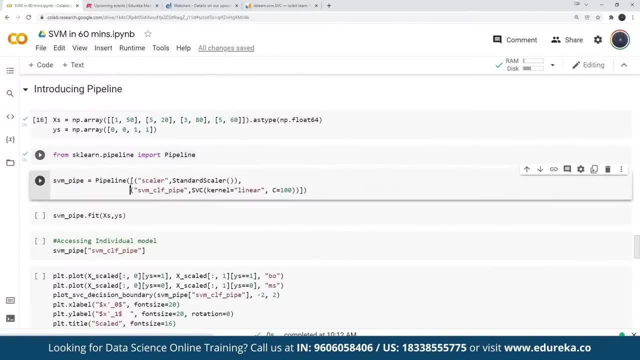 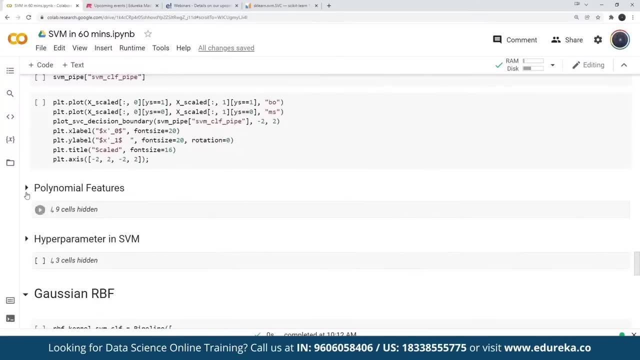 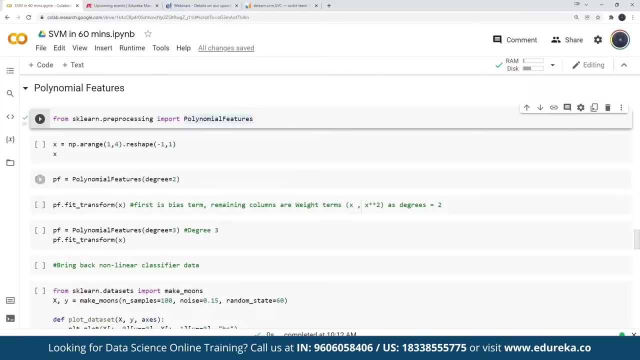 And I'm making use of pipeline, So this pipeline is going to take care of my standard scalar as well as kernel. I'll do one thing, I'll just come below. So this is what we are currently interested in. So here I'm importing the polynomial features. 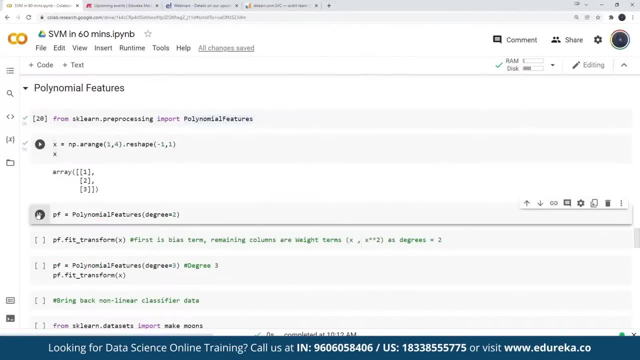 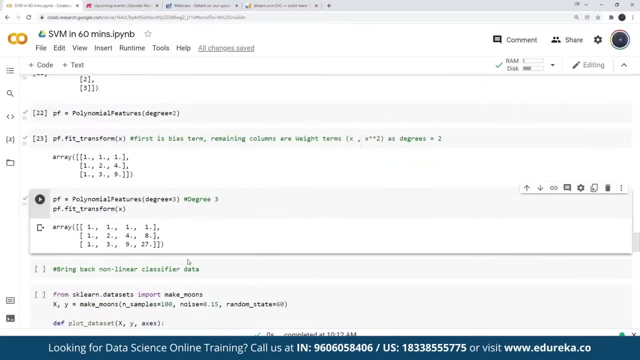 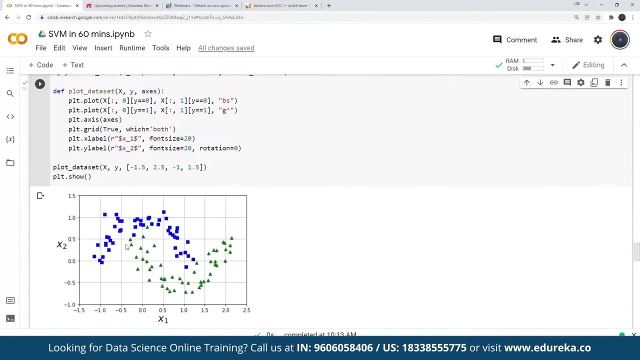 And I'm generating the polynomial Features for my data. I'm performing the fit and transform a polynomial data. That means I'm just modifying my existing data and I am sending it for my X. Okay, So this is how my pair of input, X and Y, looks like. 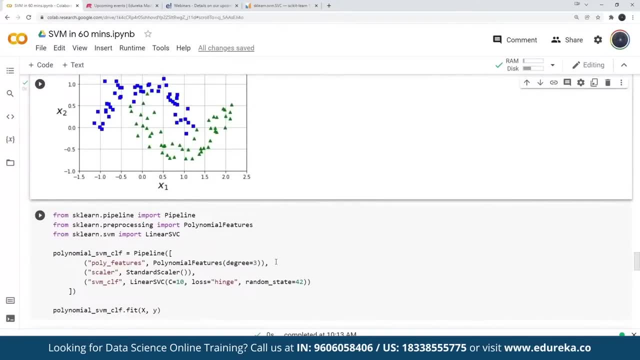 Now I'll use my X, I'm going to transform it with the help of my polynomial features, And then I'm going to scale it with the help of my standard scalar and I'm going to send it inside My classifier, that is, SPM classifier. 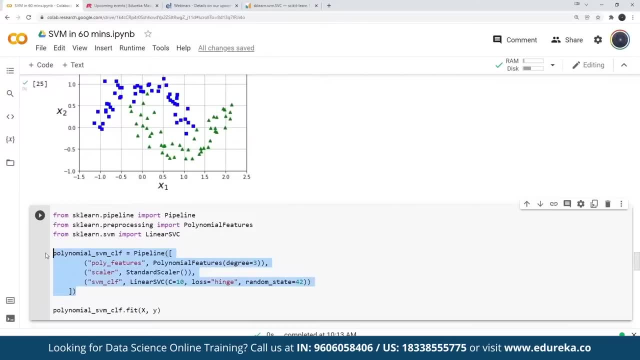 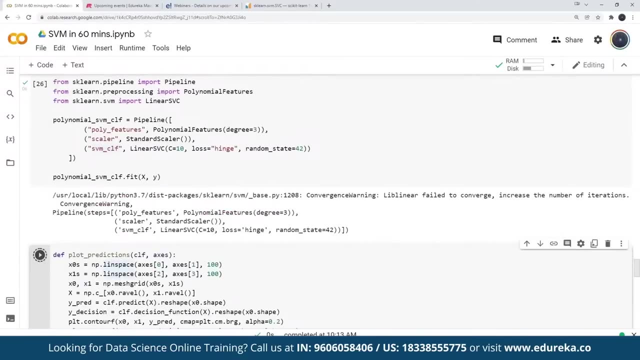 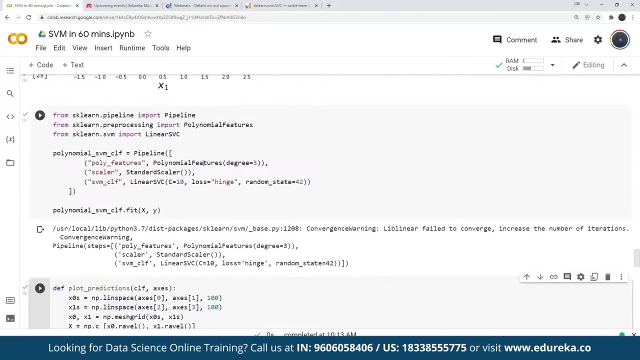 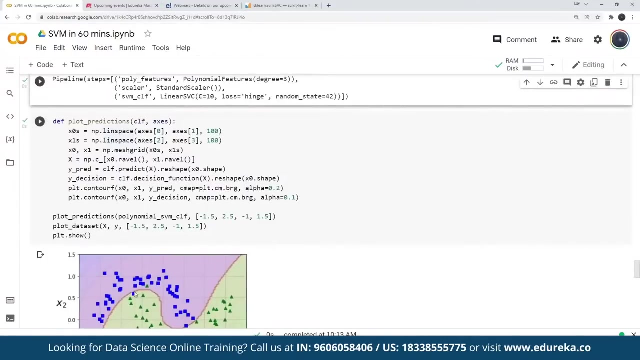 Okay, so I'm going to combine it together like this: Now observe what would happen And once that is complete, See with the help of my polynomial, polynomial features that have applied on my given linear data. So I have increased the degrees by which my model can learn. 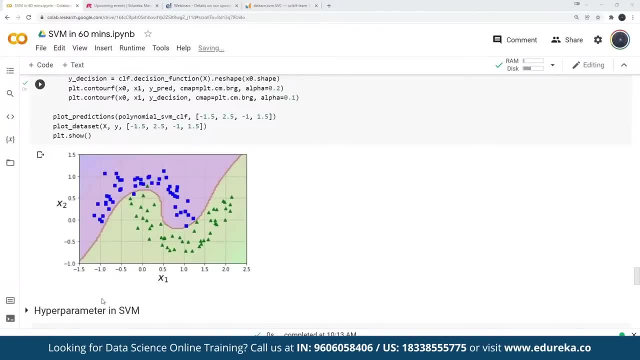 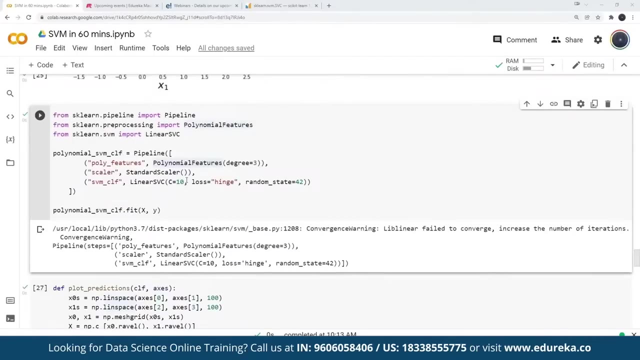 Now, instead of straight line, my model is also having the ability to learn this complex representation as well, Because I have increased the model complexity by adding my polynomial features And, while doing it, to make sure that we follow a clear path. So I have defined this skill as pipeline. 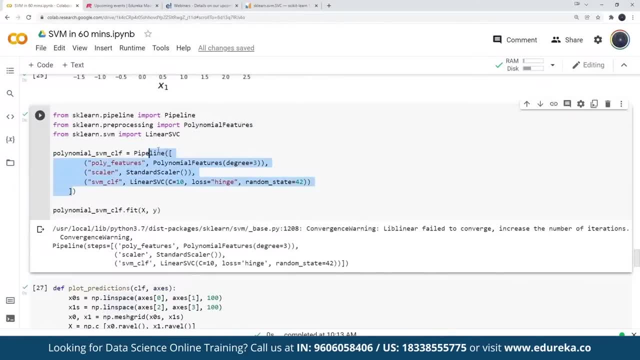 If you're new to data science, machine learning, I highly recommend you to learn this concept of a skill and pipeline. Now, this skill and pipeline helps us to combine multiple operations in a single call. So here we have created a pipeline. This pipeline is going to add some polynomial features for my input data. 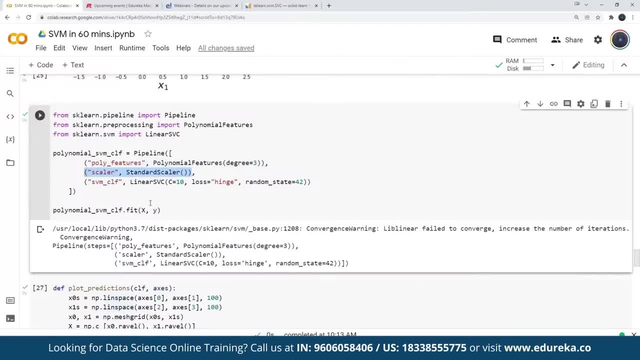 And on top of it, this is going to perform scaling, and then I'm going to perform this binomial classification using this SVM And, finally, I'm performing the fit on my data set. See when I perform the fit. it takes my input X and it's going to do all these activities. 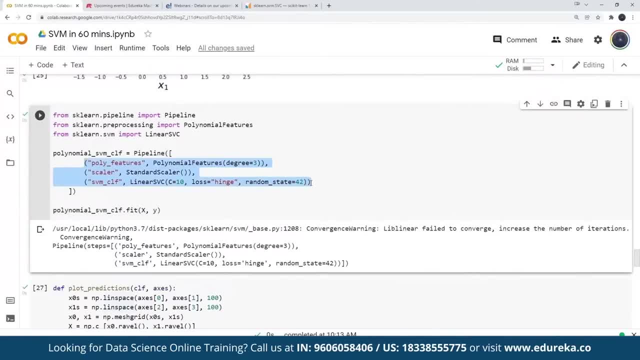 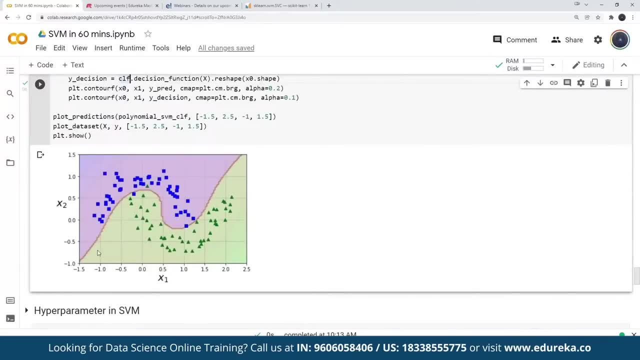 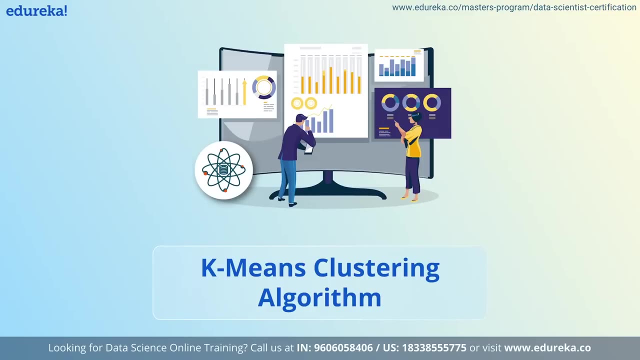 It is going to chain all these activities together And then it is going to perform the fit for my data Y Once the fit has been complete, so we can validate how my model is performing. So what is a clustering technique? Clustering technique is something that we will use it for grouping purpose. 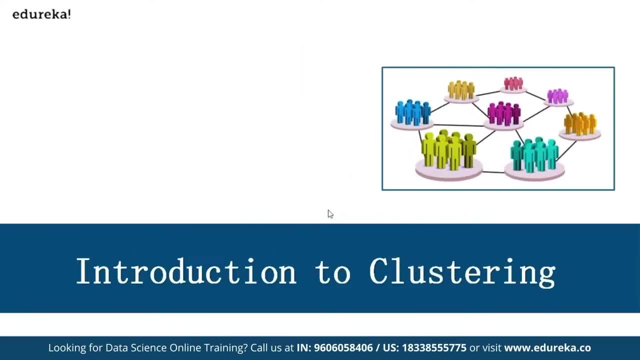 So, especially, there is a very easy way to understand what is clustering technique. You would have seen such a while we are going through a COVID-19 situation. the government has came up with creating some containment zones, As all of you must be knowing. 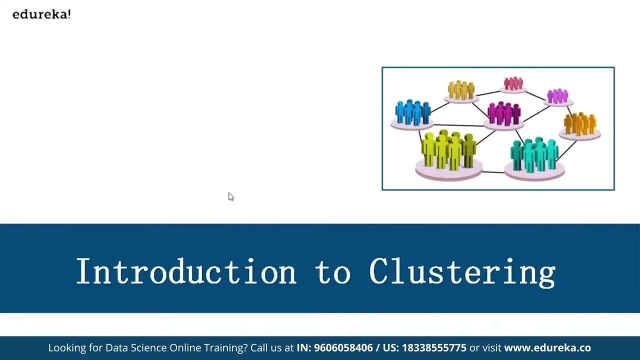 So how and what criteria government has taken that, okay, which area is supposed to be a containment zone or which area is supposed to be applied, with some restrictions on which areas can be, can be considered as normal? on what criteria that they have created? 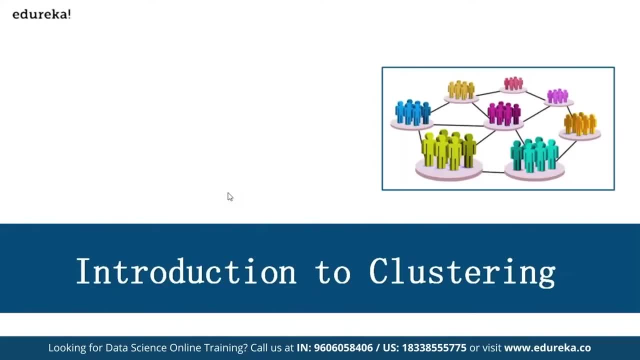 So that's what? using clustering technique, which means the governments- or when I say government means that the people who will be taking the final decision in such criteria, either prime minister, either the chief ministers of that particular state- will be taking decisions whether to go for a lockdown. 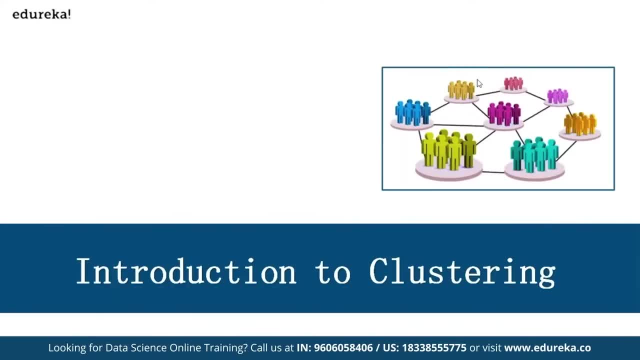 whether to not to go for lockdown, or which areas has to be considered as containment zones or non-containment zones. So those high level decisions are something which will be taken based on the clustering techniques, based on the clustering technique output which is generated by the these algorithms. 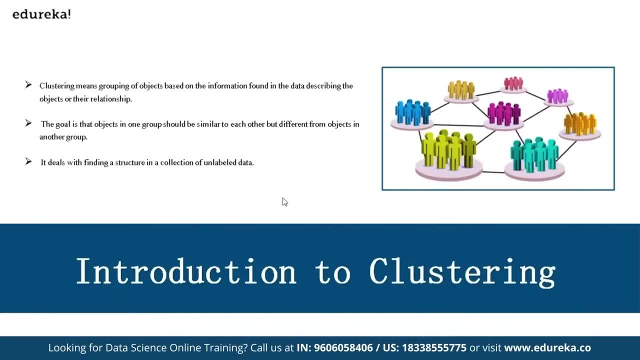 Based on a number of inputs. Okay, what is the population in a particular area? How many number of people are affected? How many number of hospitals which are present? How many number of people who are being recovered? So, likewise, based on these multiple criteria, 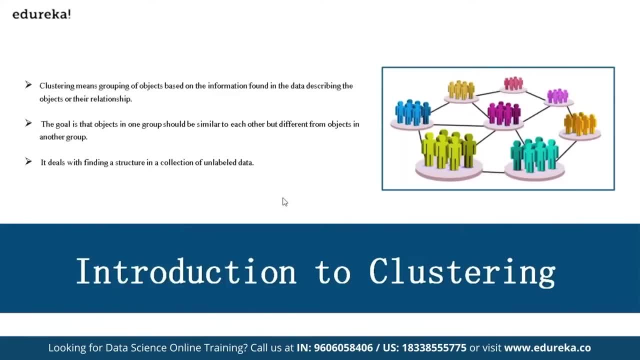 people will do some clustering technique on top of the data and, according to that, people will be segregated or the areas will be segregated, So that saying that, okay, these are the observations which belong to one cluster, These are the observations to belong to one cluster, like that. 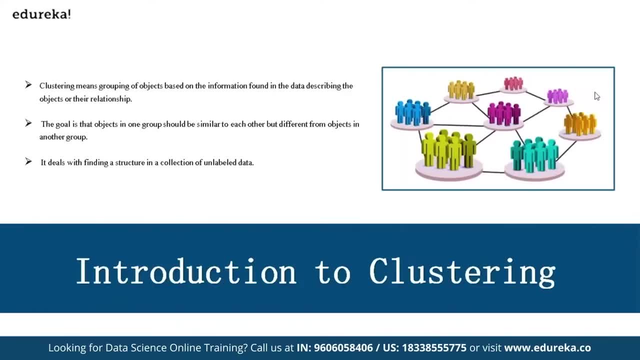 So that people can cluster them, which can make organizations to take decisions on a very high level. Okay, that's what is our clustering technique, which clustering technique output will contain the different different groups. It itself will group the different different components based on whatever the number of clusters that you want to generate. 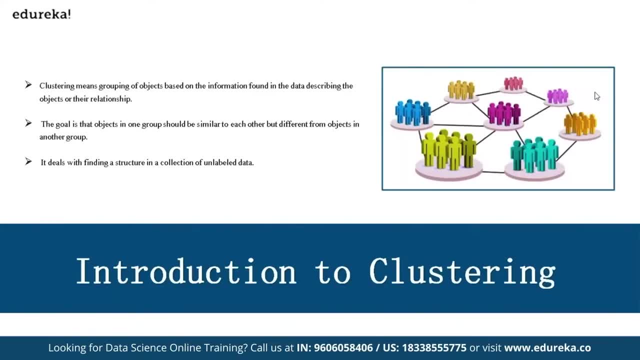 That may not give the direct output. on top of the generated output, People will be taking business related decisions. That's what is all about clustering techniques. Okay, so now what we will do. let's take an example of within clustering techniques. What are the different types of clustering techniques we have? 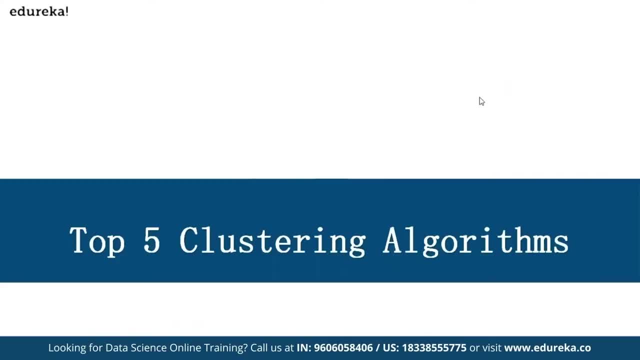 So there are multiple types of ways based on the type of output that we want to produce. There are multiple different types of clustering techniques we have, but out of which the let's try to understand about what are the very famous and most widely used clustering technique- algorithm- out of which we have something called K-means clustering algorithm. 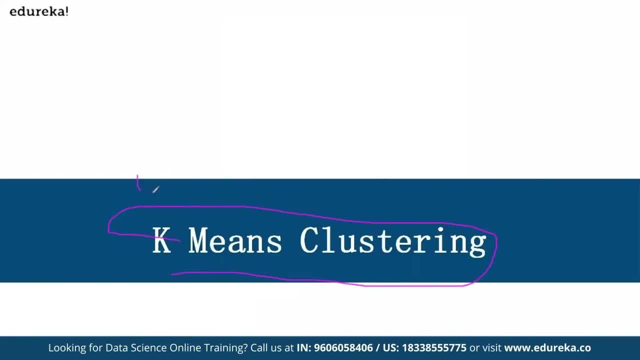 K-means clustering algorithm is one of the very famous and most widely used. More than 90% of the people will end up with using K-means clustering algorithm, which is very, very famous in clustering techniques. So what are these clustering techniques? 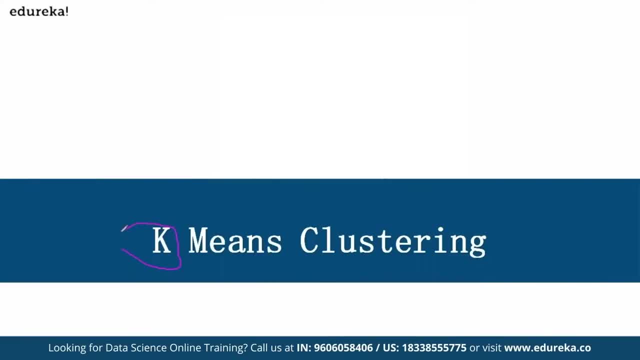 As I said, how this clustering technique will work. By default, K is nothing, but you are. you are supposed to. as a user, you are supposed to provide what is the input of K. It means wherever you see, there are multiple techniques that we have in machine learning, like K-means clustering technique. 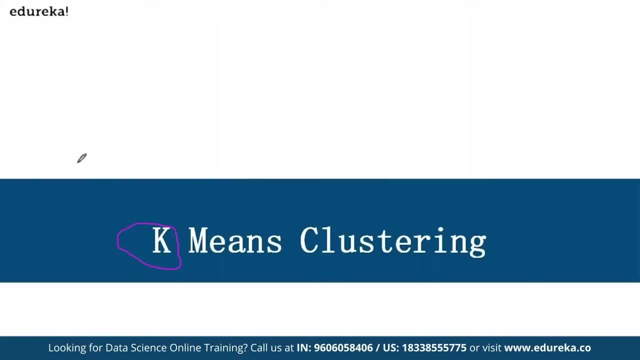 K-nearest-neighbor is one of the algorithm: K-fold cross validation. Likewise, wherever you see a notation called K, what does the K means? It's an input that you are supposed to provide. Always remember this: It's an input that you are supposed to provide to your algorithm. 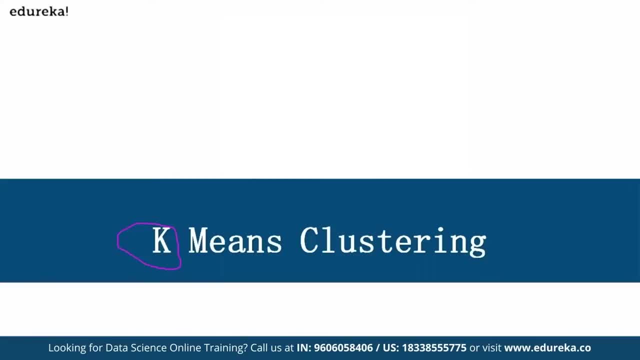 Your algorithm cannot identify that K value. Of course, everything else will be taken care by your algorithm, But whenever you see K, it means in K-means clustering. what is the meaning of K-means clustering? How many number of clusters that you want to provide? 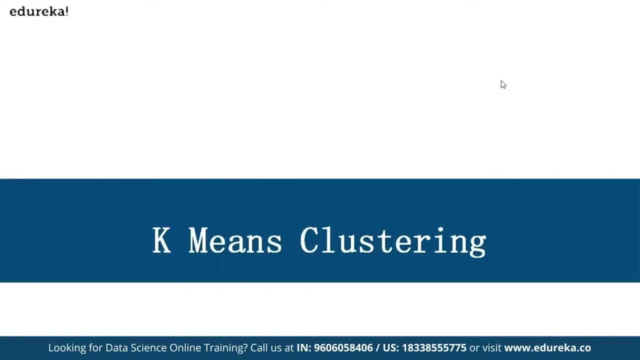 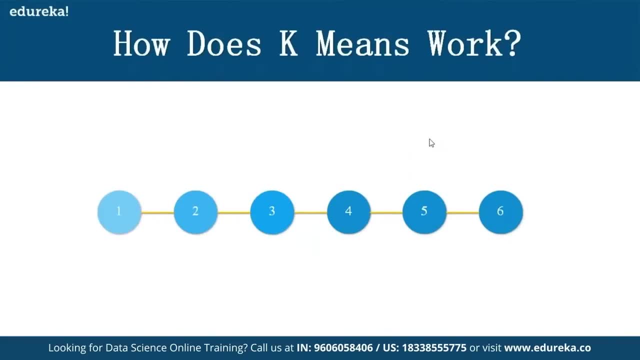 That is something that you have to input it to your algorithm. Here, the meaning of K is how many clusters that you want to generate. So how many clusters that you want to generate When you have a thousand observations, which are present, when you have a thousand input records, which are present in your historical data? 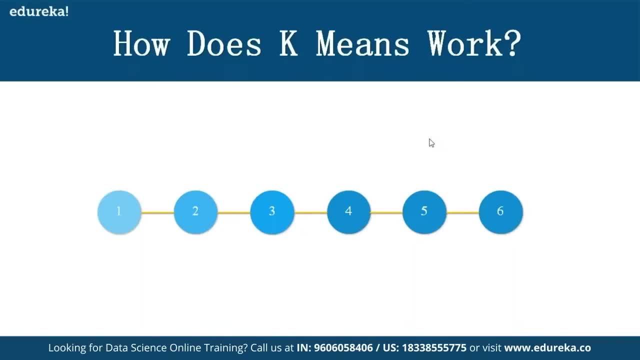 how many number of clusters that you want to provide. Do you want to go for one cluster? Obviously, one cluster means that the entire data set will be clustered as is. Do you want to create two clusters out of the data? Do you want to create three clusters out of the data? 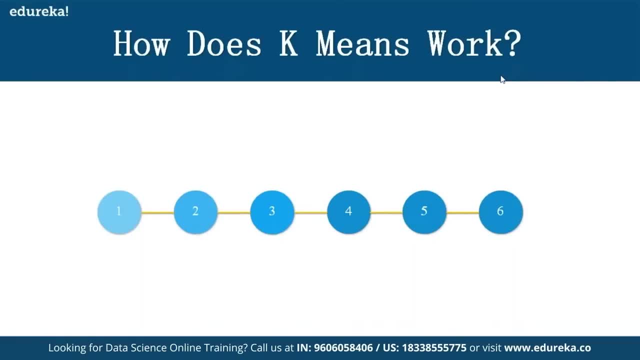 Four clusters, Five clusters. So how this can be done. There are multiple steps that are involved in generating K-means clustering algorithm. You can choose the number of clusters. This is nothing but your first step. You need to decide what is your. K is nothing but number of clusters that you want to produce. 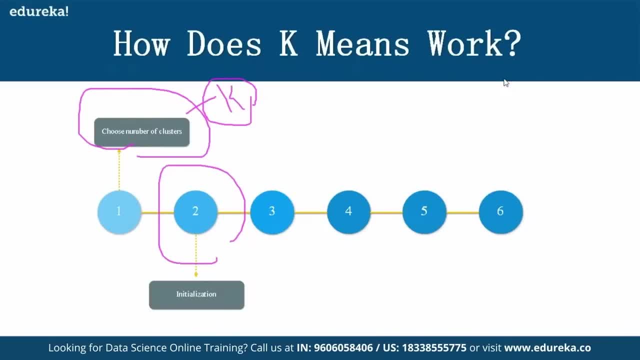 And then there is an initialization of centroids. will happen as a one time activity. So there is an initialization of centroids which will be declared. That will be used as your initial step for your machine And then assign the clusters, move the centroids and optimization. 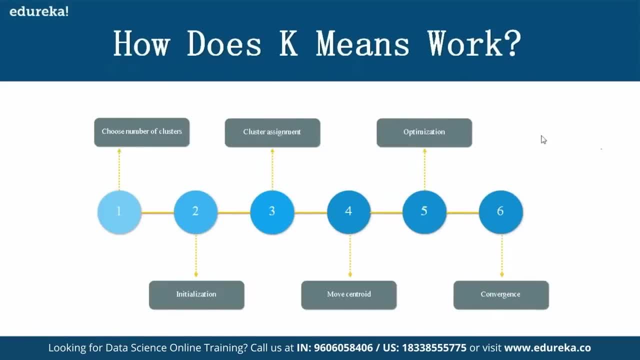 and then converge all the clusters into one component. Yes, I know it will be very difficult to understand by looking at this thing, So let me show you a very simple example how exactly to be done. Maybe let me take a simple diagram for you to show how exactly that's going to work. 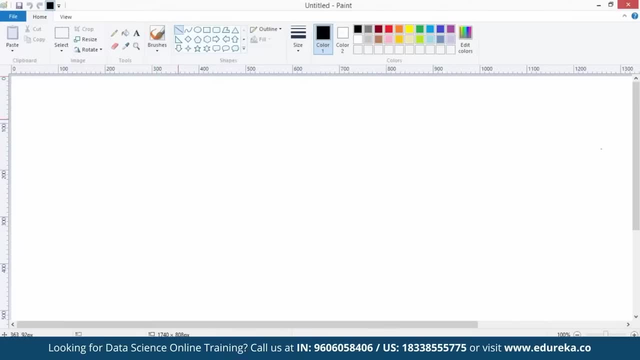 Okay, so let's say, for example, I'm going to take some historical data just to explain you on how exactly the K-means clustering algorithm will work. So what is that? it is written in the first step. So the choose a number of clusters. 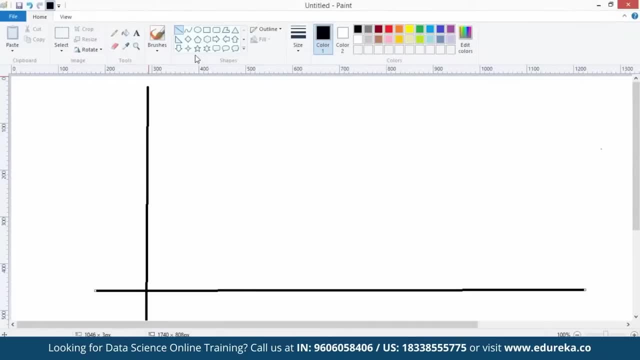 Now it means say, for example, we need to take some historical data. I'm considering some historical data here. Let's assume this is the historical data that we have. So, as you can see, there are multiple historical data points. As you can see, the first step, choose number of clusters, which means, let's assume to make this thing simple. 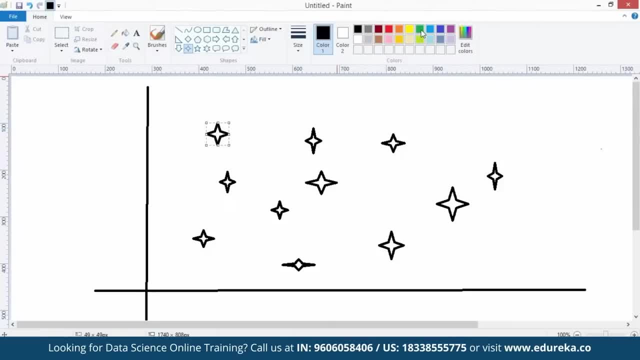 I'm going to choose that we want to have two clusters generated. Okay, so this is, which means we want to have two clusters created. So, because my number of clusters that I want to generate is two, I'm going to consider that there are two centroid which are present. 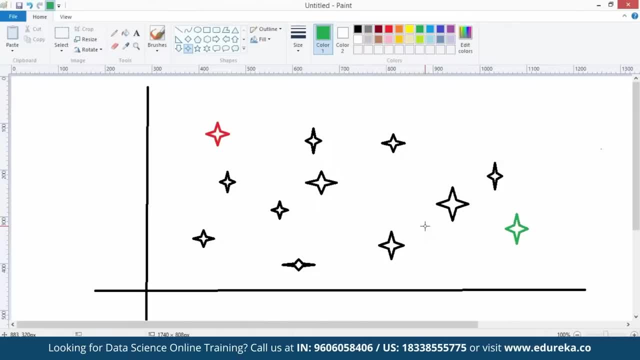 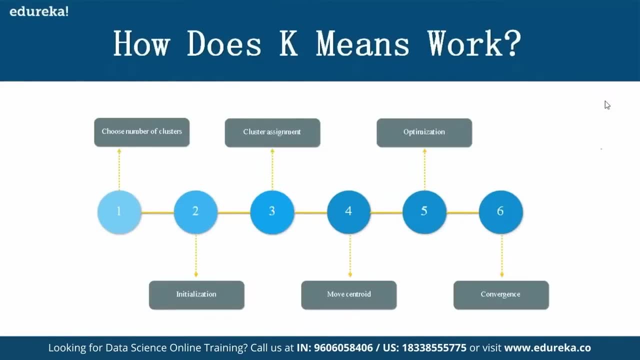 This is my first step: How this algorithm will do, How algorithm will come with the number of clusters. This is how it is. So first step is to choose the number of centroid and then initialize your centroid. That's the second step. So now what is the third step? 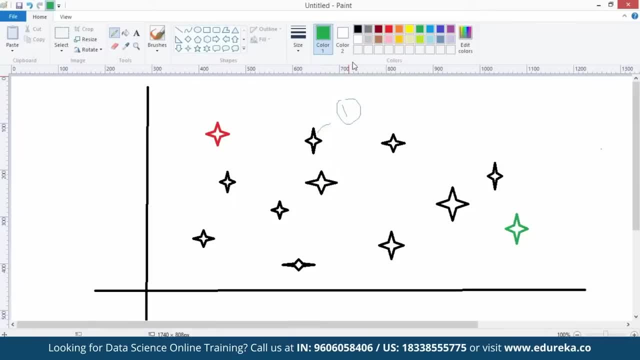 Let's assume this is observation number one. This is our data point one. So now what is the next step? We will take the distance from every observation to every centroid and every observation to every centroid. So this observation is more closer to red color. 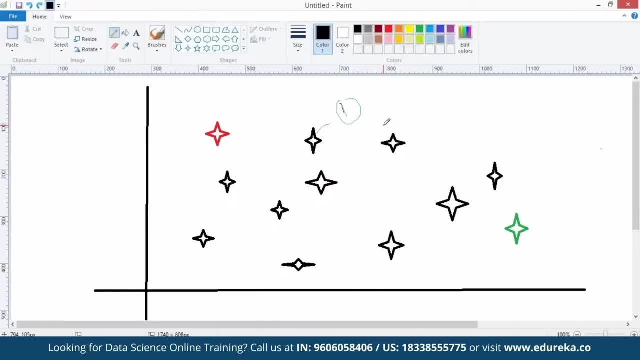 So now what happens? What is the next step? The algorithm will assign this particular observation one as a red color, for now, As considering that this belongs to red color. Likewise for the second observation. When the second observation appears, what is the distance from the second observation to both the centroid? 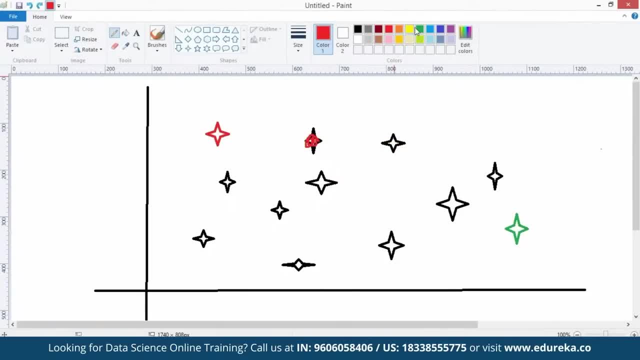 Now which one is more closer? I see green color is more closer, So now I'll mark this as green color. What if the distance is same, equal? So then the algorithm will force any of the observation to get into any of the centroid. 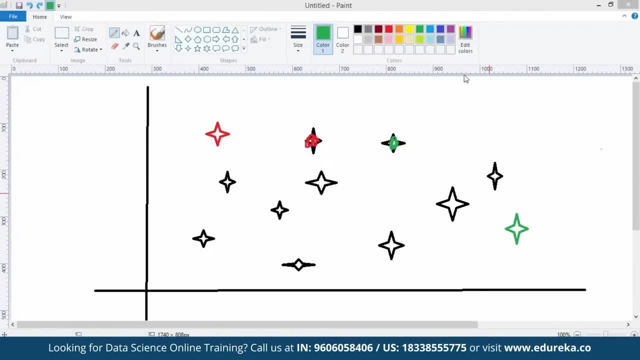 So number of centroid that you will choose based on the k value, as I said. Now you are going to. likewise, you will repeat the same process And whatever the observation which is more closer to whatever the centroid it is, you will mark them as with their so-called mark length. 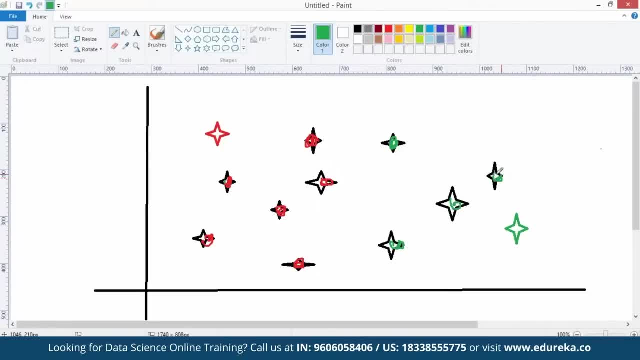 Now you are going to initially mark them as observations, either into green color, either into red color, So now these observations are now considered as green color observations And these observations are now considered as red color observations. This is step number one. What is the step number two? 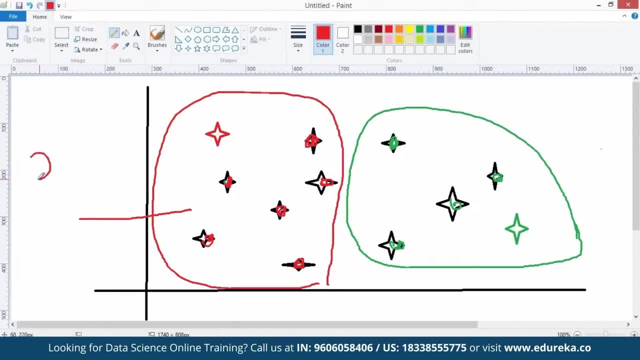 Step number two is segregate all these red color observations And take the average value of x and y coordinates And repeat the same process for calculating average coordinates of x and y coordinates for the green color observations. Take the average of all these observations. 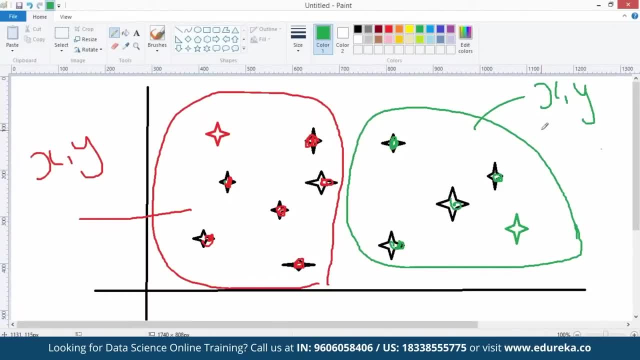 Calculate average And take all these observations. Take the average. You'll end up with getting a new centroid position called xy, Which means now you ended up with getting a new centroid in the initial Step that we have taken random centroid. Now you got the centroid that you can use based on the previous iteration. 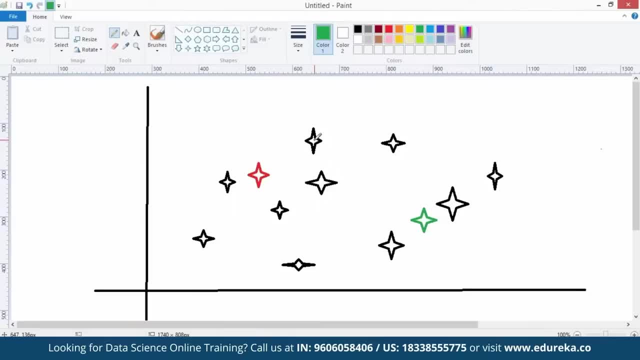 Now you end up with getting a new centroid. Again. you repeat the same process: Take the distance from every observation to every centroid And assign the observation based on the nearest of nearest distance, And continue to mark every observation either into red color or either green color or whatever it is. 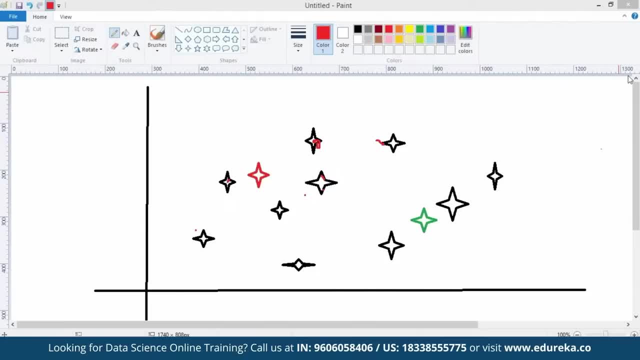 And you repeat the process until you will be able to see there will be no change applicable for your clusters. You repeat the process. It means in every step you might end up with changing your centroid. Every step will continue to change your centroid. Now the centroid might become like this: 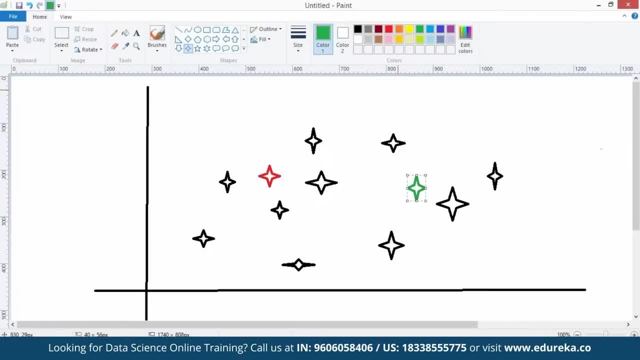 Then later your centroid will become like this. Likewise, your centroid will keep on moving. Initially you have taken it like this, But it might continue to move like this. Somewhere it will be fixed And after that there will be no change that you will notice if you repeat the same process. 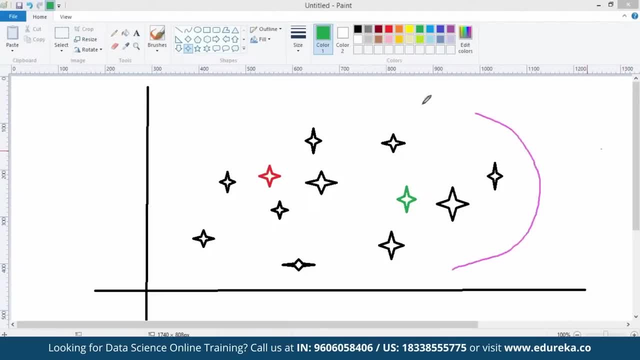 At this particular stage, whatever the observations which are grouped into green color, You will say like: these are the green color observations. Whatever the observations which are marked into red color, You will mark them as these are the observations which belong to red color. Likewise, you will segregate all these observations either into red color or green color. 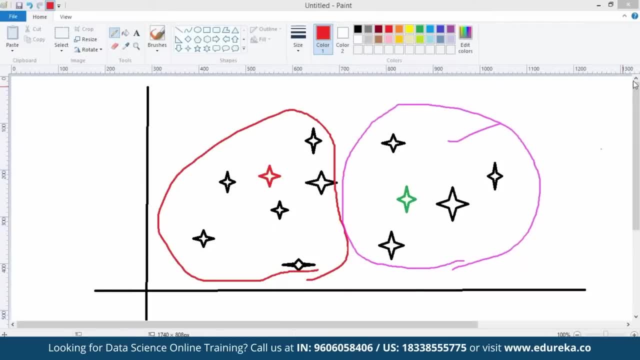 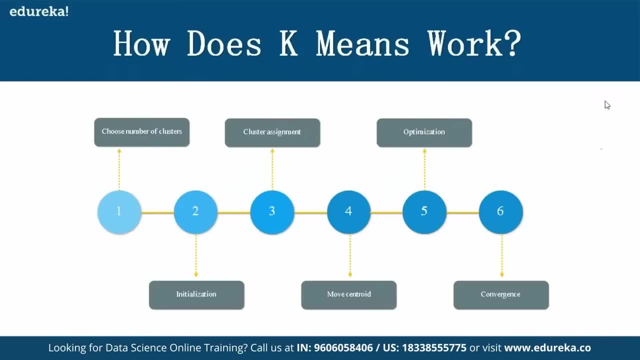 So you can generate these clustering techniques. That's how the k-means clustering algorithm will generate this algorithm output of using this algorithm. So now, likewise, there are multiple algorithms that we have. So, like when we talk about machine learning, So there are multiple types of algorithms that we have. 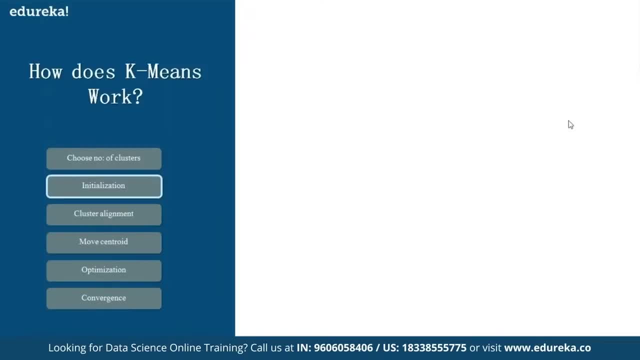 So like: how does the k-value will occur? So you are going to choose some randomly generated k-value And you will be choosing the number of k's over here And you can see that it will assign them based on the number of this easy most nearest distances. 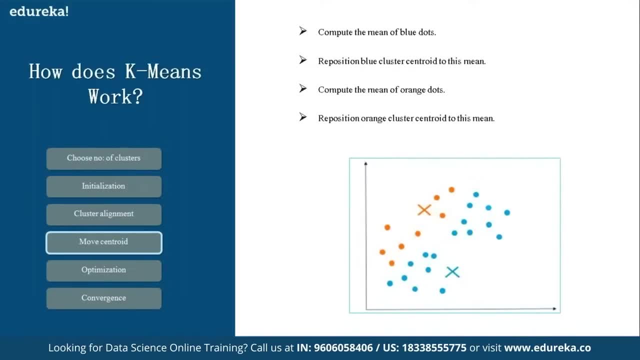 And according to that, it will change your centroids. Once you change your centroids, you will repeat the same process Until you are able to change that your centroids don't move further, And then, once it has been finalized, You will say, like there is a final cluster output that we can generate out of this. 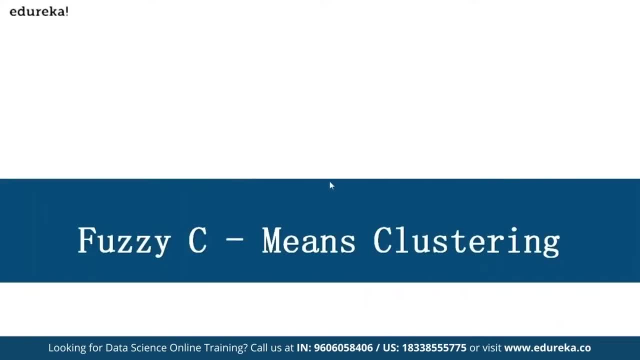 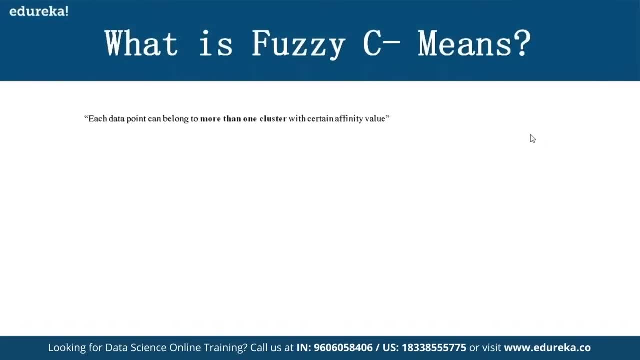 So, likewise, we also have different types of clustering techniques, And the second type of clustering technique that we have Is fuzzy or c-means clustering. So what is fuzzy or c-means clustering? The output will remain same. So c-means clustering means that there are places that one or two observations can belong to one or two different clusters. 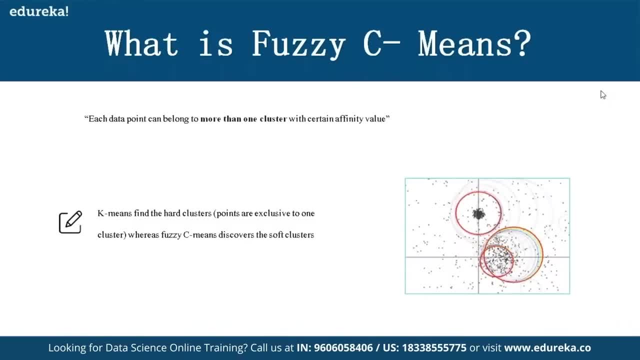 Like one or two different clusters, Which means usually the primary difference between your c-means and k-means clustering technique is, In case if there are any observations which are having equal amount of distance, Usually in k-means clustering, what we will do. 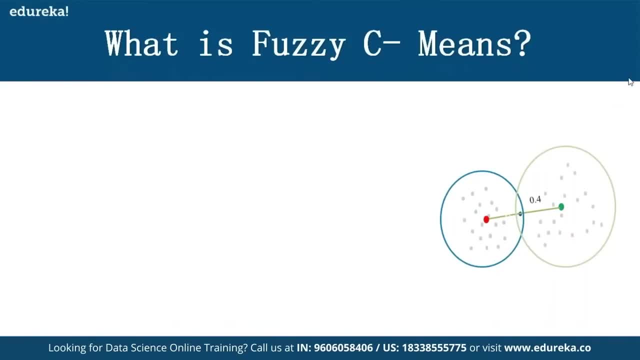 We will force this observation to be part of any of the cluster, But in c-means clustering Based on the distance that we see- There are chances that an observation can go to or can belong to one or two clusters. So it purely depends on the business use case. 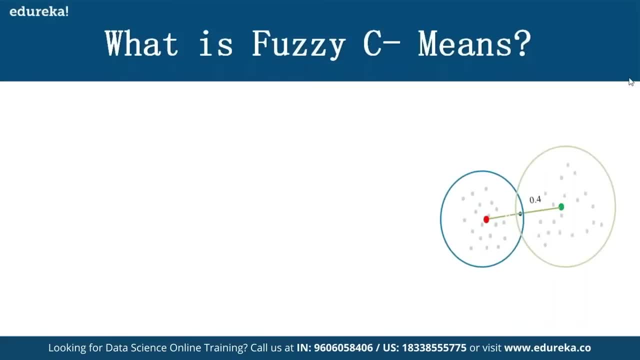 Who is going to decide to either to go for k-means clustering or c-means clustering, Based on our business outcome? So if people are going to decide whether to go for c-means clustering or k-means clustering, So there are n number of observations which might 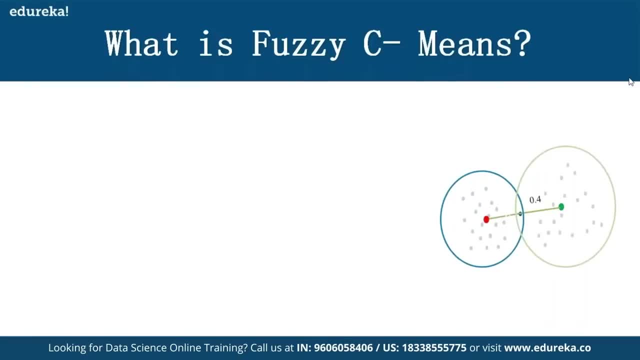 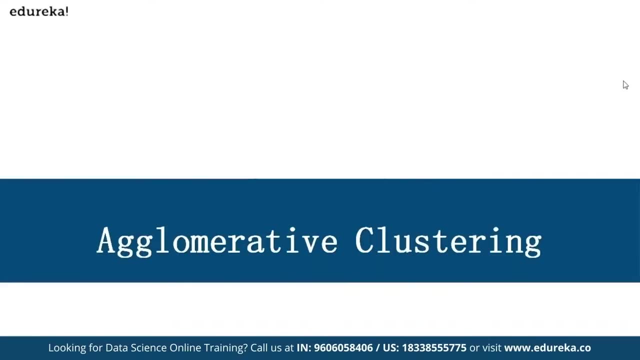 It's not mandatory- Which might can belong to one or more clusters that could happen. So the third: we agglomerate the clustering. So which is the third type of clustering technique that we have. So now, what is this agglomerative clustering? 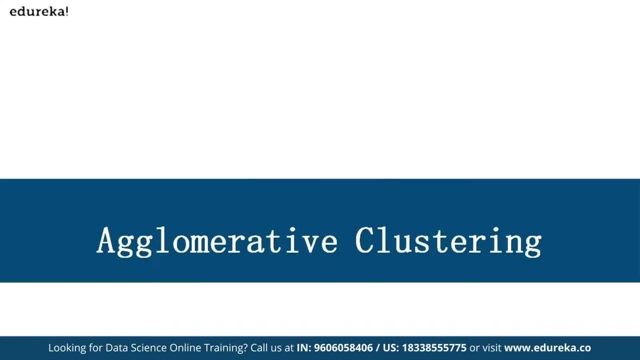 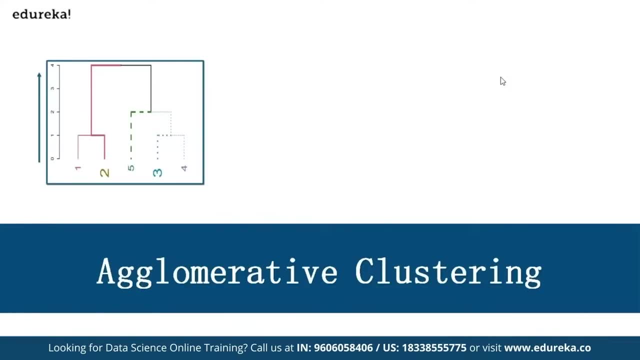 So this is what we also call it as hierarchical clustering. These clustering techniques are built using H-clustering. So what are this? So, based on the type of algorithm They will try to, There is a mathematical expression which are involved. So, considering the way how the data points are been segregated, 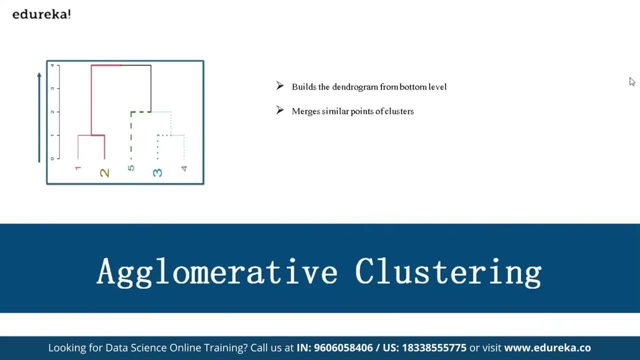 It will build a kind of dendrogram. So on top of this dendrogram, Your observations can be classified here like this, As you could see on the screen. You need to understand one thing When we are talking about unsupervised learning algorithms. 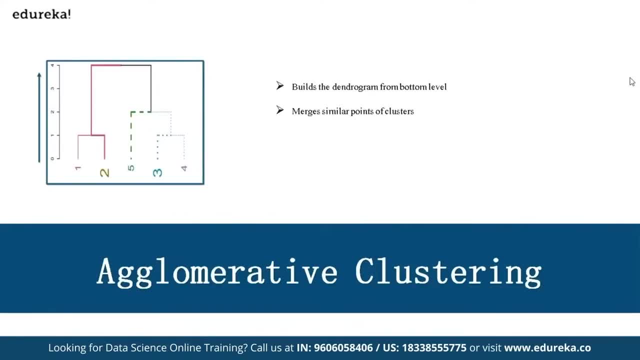 As I said, You may or may not have clarity on the data, Which means Your assumption is that, at the least level, You don't have clarity on the data. When you don't have clarity on the data, How can you say this is an outlay or this is not an outlay? 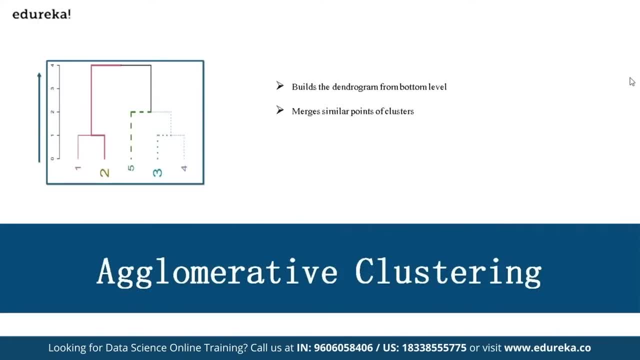 When you have clarity on the data, Especially when you are working on supervised learning algorithms- But you don't have output column, also How you will be able to evaluate, Because this is not been classified properly, This is not been clustered properly, Based on historical data. 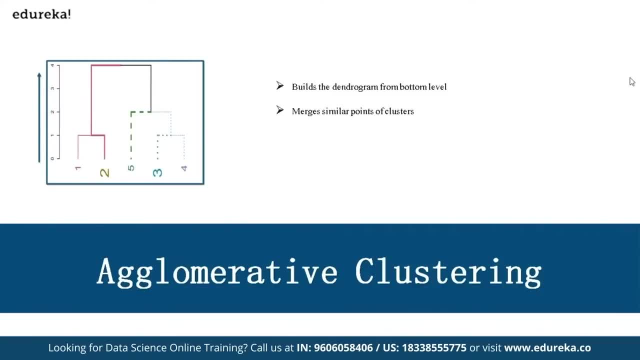 Because there is no output column. So those type of concepts are something Which you don't need to worry about. When you are working on unsupervised learning, They will be primarily. They will be constrained When you are working on supervised learning algorithms. 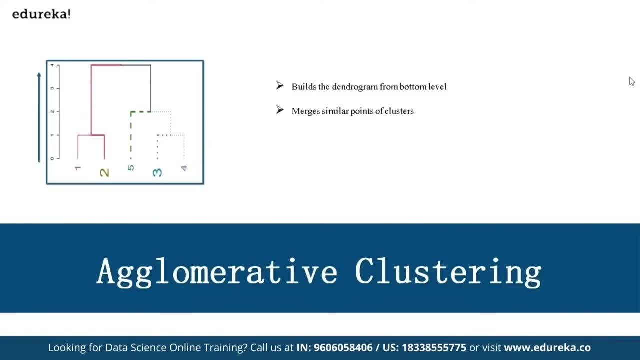 And, of course, in case, If you see that there are outliers which are present, Obviously it will be considered as any of the cluster. It belongs to the data, But anyhow, that's the characteristic of the data. You don't need to, You don't be taking care. 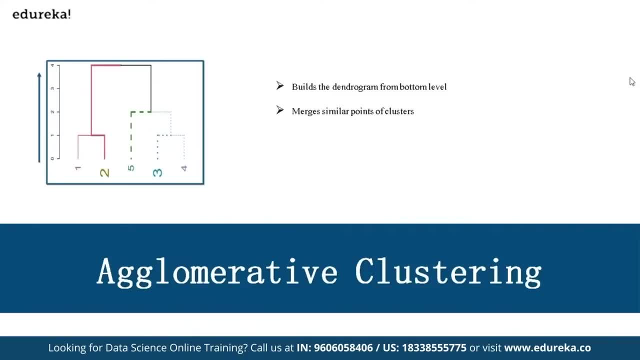 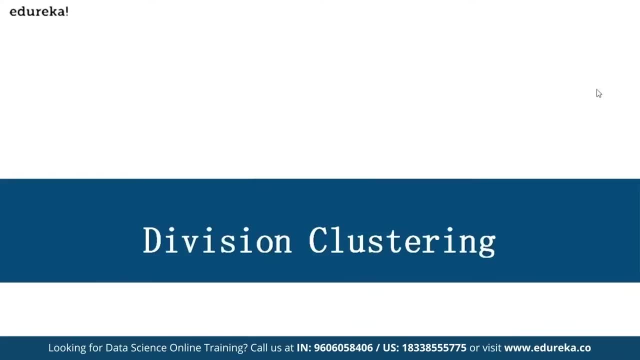 Because you might be killing the actual original values Which are present in the data. But you cannot expect that outlier can be recognized For all the cases that you have in unsupervised learning. So the next type of clustering technique That we have is division clustering. 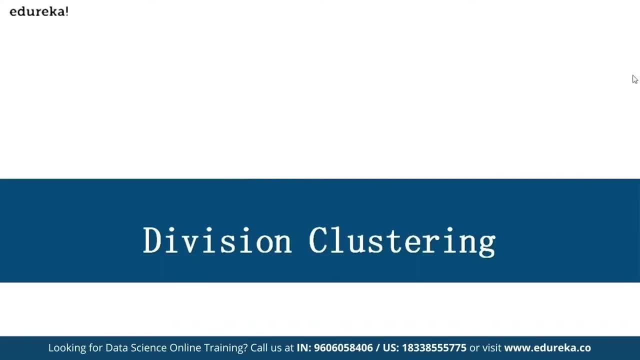 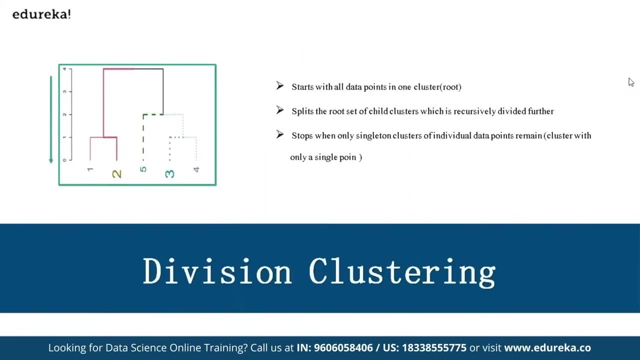 So what is this? division clustering, As the division clustering is, also Creates the data in a form of dendogram, But the difference is, You can see, that Starts with all data points in one cluster, Splits the route into child recursively. 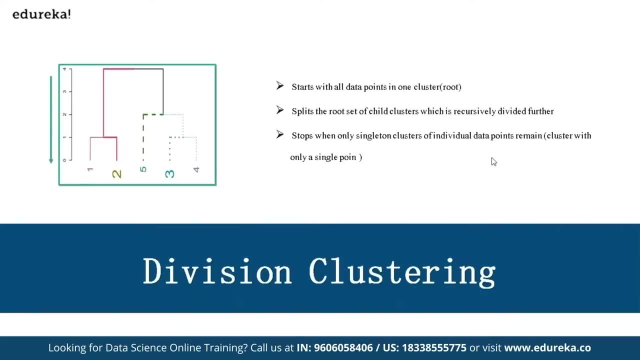 Based on the dendogram And stops when there is a singleton, clusters Which are created, Which means that for every cluster, There will be one observation which belongs to it. So likewise the clustering technique will work. Now there is one more technique that we have. 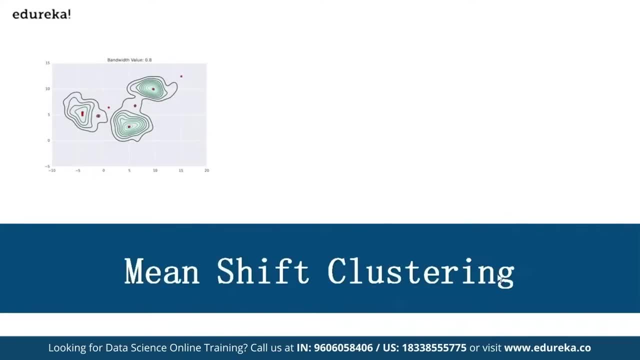 In terms of building a clustering technique. That's what we call the mean shift clustering. So what we will do, We'll take an average of every cluster that we have. What we will do, We'll end up with reducing their means into the. 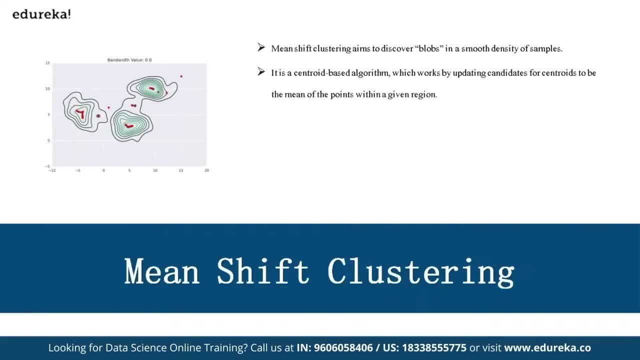 Into a single density of items And then we'll continue to repeat the process To see to that Which observations mean will belong to the same cluster And according to that We will continue to identify Which observation will belong to a cluster. 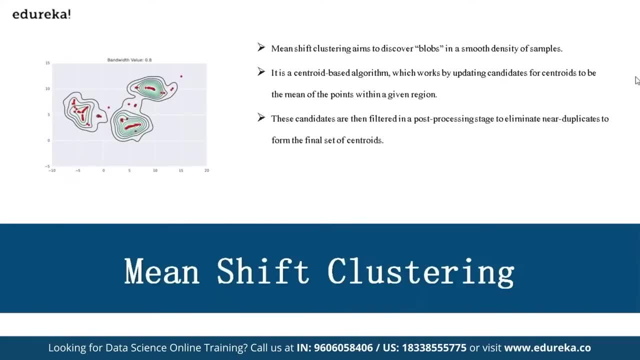 A particular cluster. So, likewise, We can apply different types of clustering technique That can help us to Trust of the data, Which is part of unsupervised learning. So now Let's jump into something called a small hands-on. Okay, 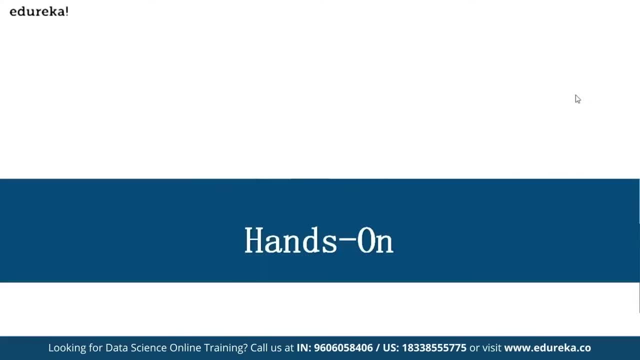 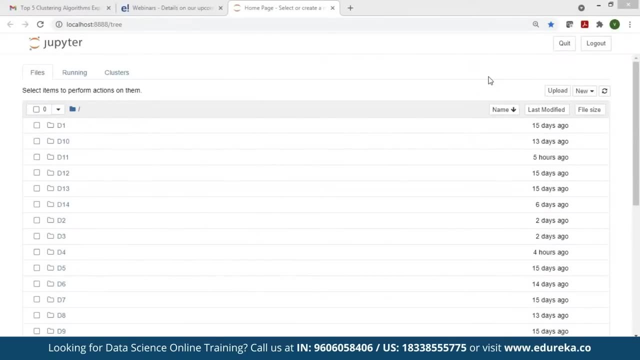 Let's take a small item example And we will see How do we build that particular A clustering technique on top of the data Using one of the simple data that we have In Jupyter notebook. Let me open. You can use kikit learn. 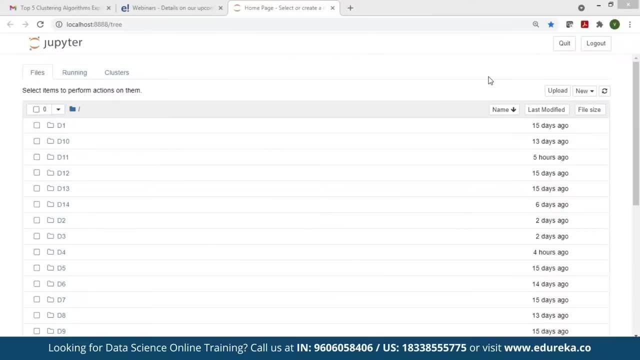 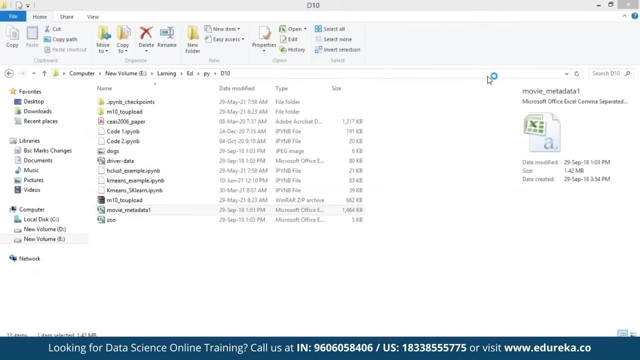 Using one of the example. Let me show you a data set that I'm going to use as well. So I'm what I'm going to do is I'm going to take this movie metadata information. Let me open this data set. I'm going to take this example of movie metadata. 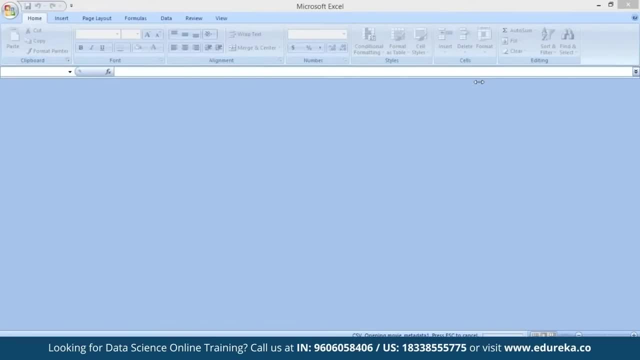 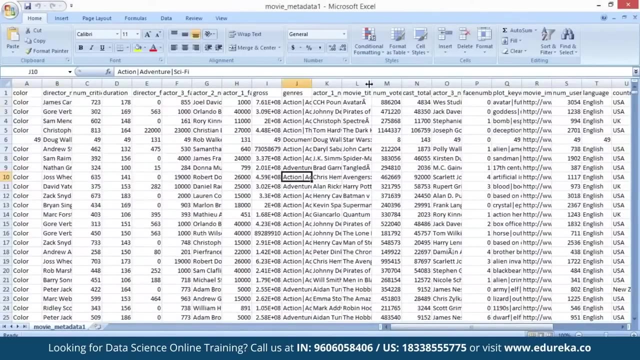 Information Where This data set has got a number of observations Which are present. Okay, Let me open this. Okay, You can see that there are a number of movies, Related information, As you can see the movie names. So, Avatar. 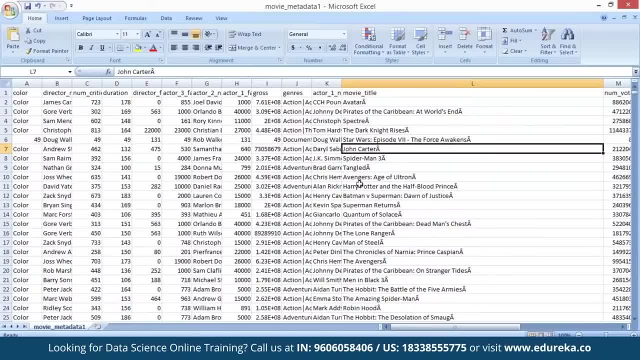 Pirates of the Caribbean Spectre, The Dark Knight, Star Wars, Etc. Etc. John Carter, Spiderman, 3. Tangled, Or etc. Etc. We have a lot of movies And about every movie We got a lot of information. 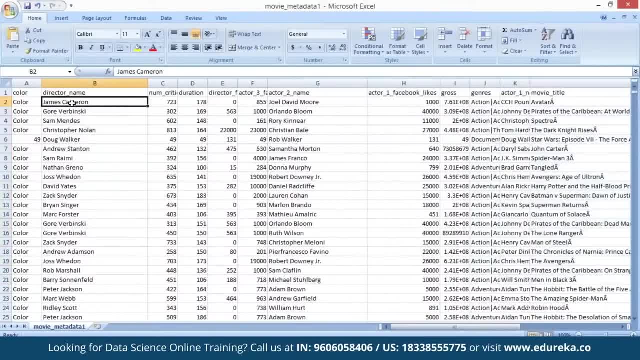 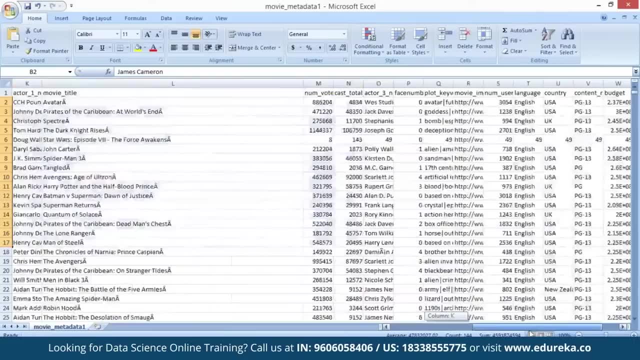 Which is present, Like Who is the director, Who is the actor Which is present As part of these, Whatever, Every observation. So now What we will do. We will try to Cluster these data points. You can see a lot of observations. 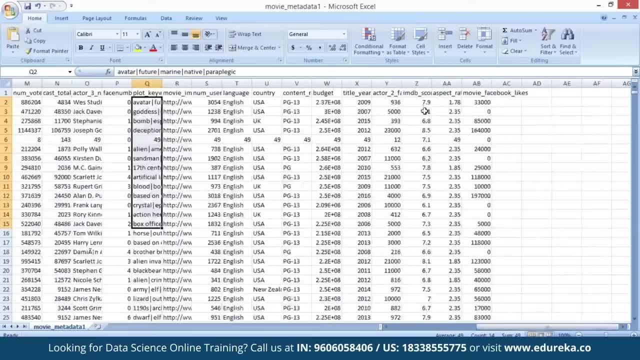 Which are given. What is the gross of the movie? What is the number of reviews? What is the IMDB rating? What is the So-called IMDB score? What is the movie span? What is the gross? What is the budget? 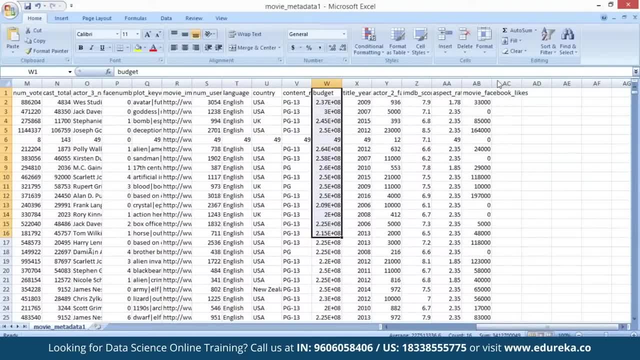 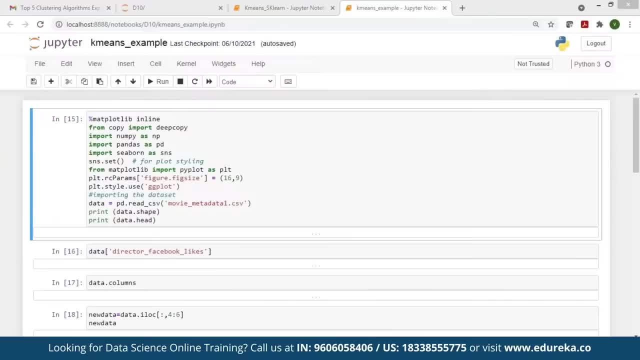 And everything. So now What I'll be doing. I'll be Reading this data set Using one of the pandas Library that we have. I'll be using something called pandas, As you can see. Read Pandas CSV. 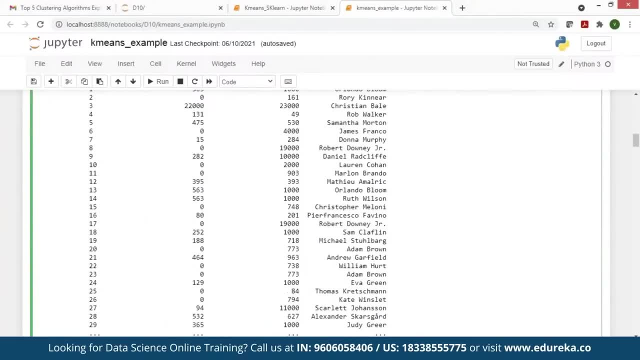 That I am able to read. I got a number of observations That are present. I cannot see that Director Facebook likes And actor 3 Facebook likes. So now, What is it I want to do is, Instead of building, 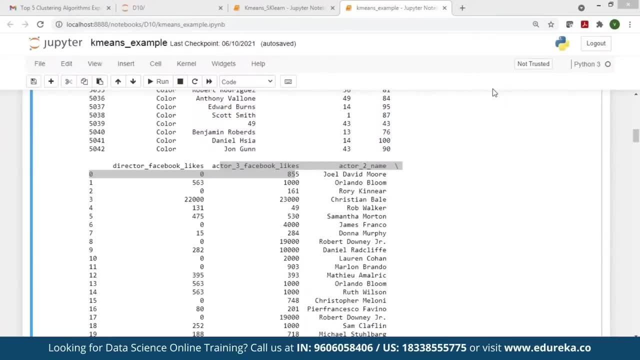 This clustering technique On top of every observation. So what I will do is I will take these columns Called Number of Facebook likes On director And number of actor Facebook likes Versus director Facebook likes, So where you can see that. 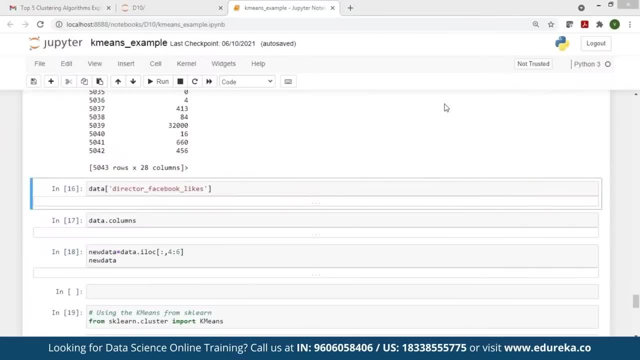 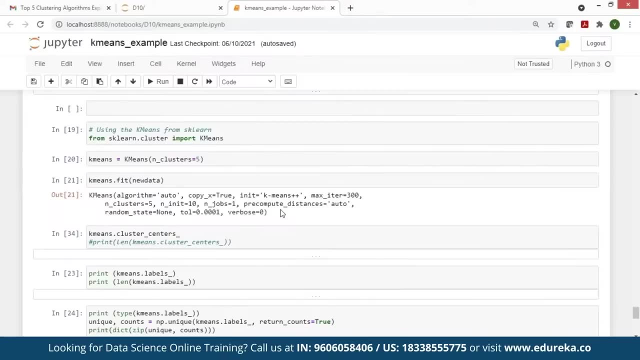 If I want to select A director Facebook likes Alone, I'll be able to choose this Director Facebook likes Alone. You can see For every movie You got that number of Director Facebook likes. If there are more Number of Facebook likes. 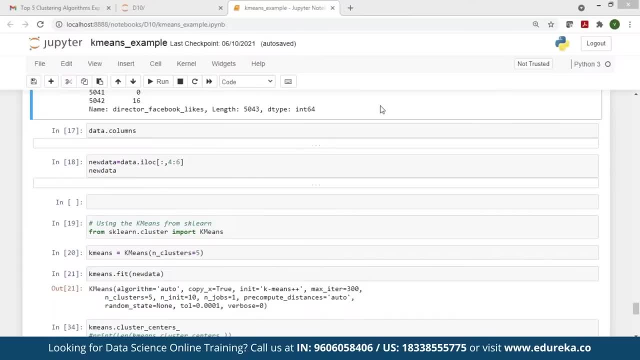 What does it mean? The director is Famous person, Or rather, If there are more Number of Facebook likes, The actor has got, Which means that The actor is very famous. That's what you can understand. So now You can see that. 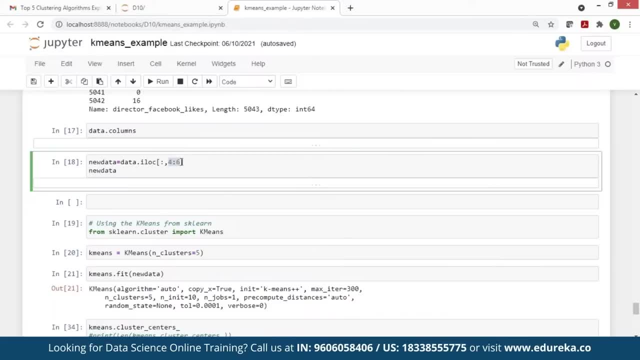 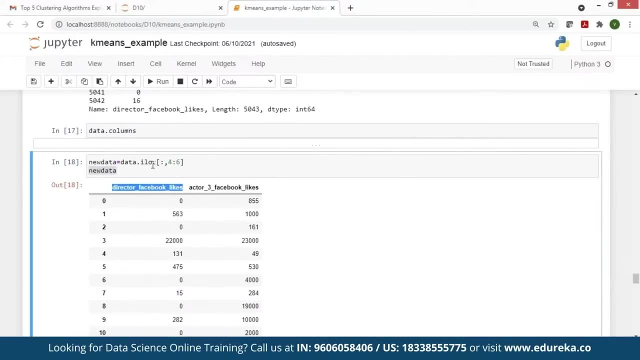 I'll try to extract These independent Components That we're talking about. I will extract All the records In all the Director. Facebook likes Versus Actor Facebook likes, Where I'm just going to form An object. 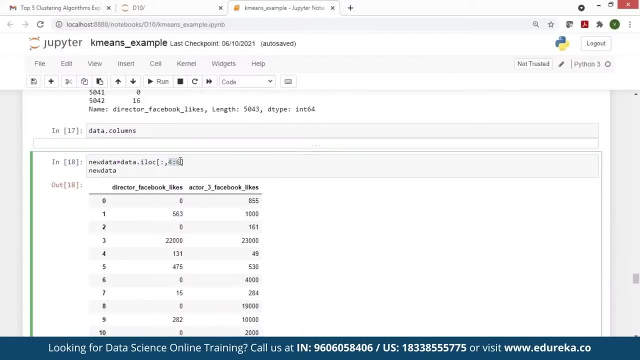 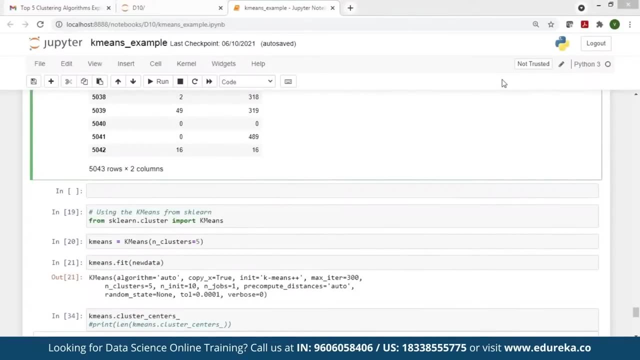 Called new data By applying some I location. I wanted to What other Column That I wanted to Using this I location Function. Now I got all the So So called Number of Director Facebook. 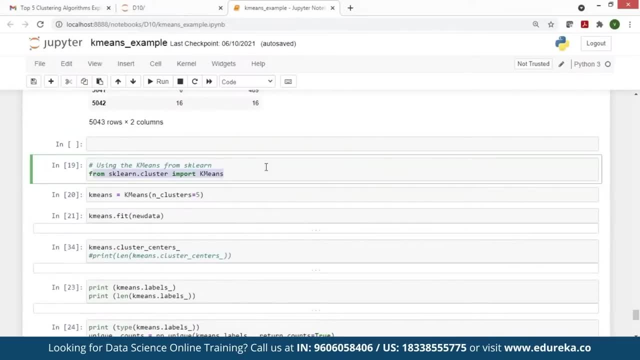 Like Actors. Actor Facebook. Like: We got Present As part Of this. Okay, So This has been Flooded Into An object Called K-means Clustering, And For This 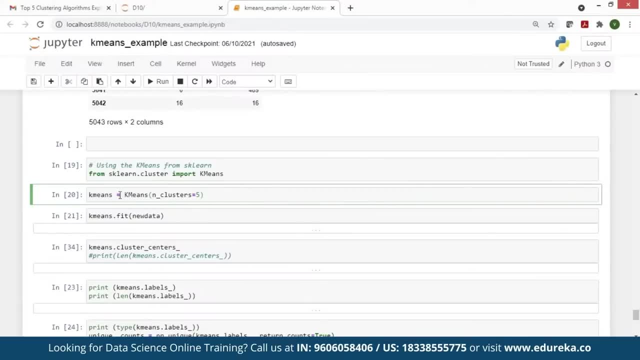 K-means Clustering. I'm Providing The C Is Equal To Number Of Clusters Is Equal To File. So Here, If You Are Aware Of, 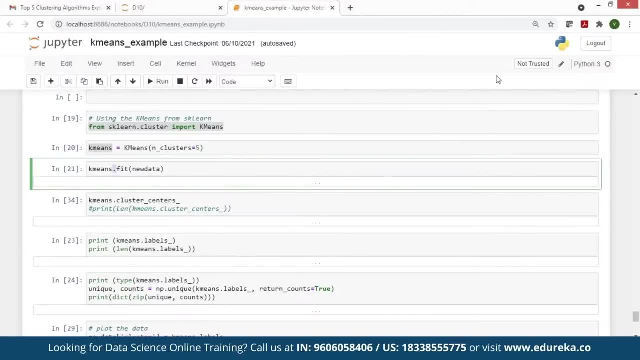 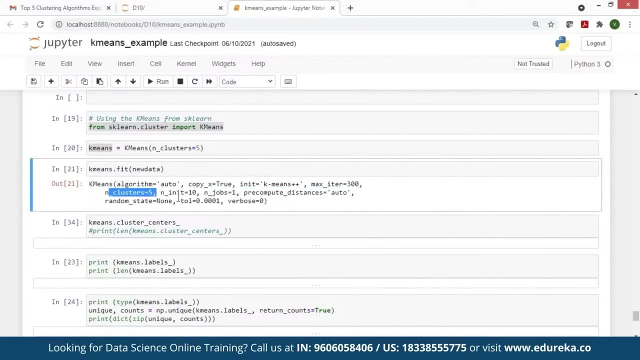 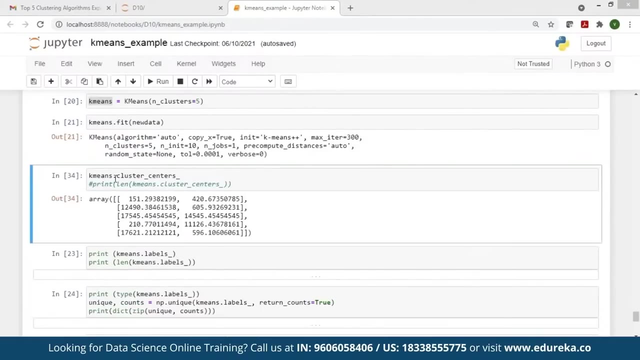 Object. It Is A Method That Is Going To Invoke What Supposed To Be The Process That Needs To Be Executed. That's Going To 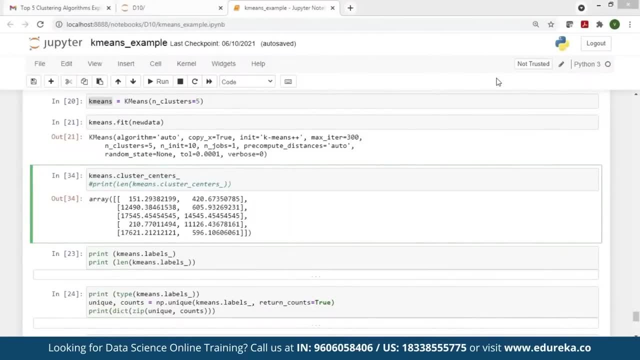 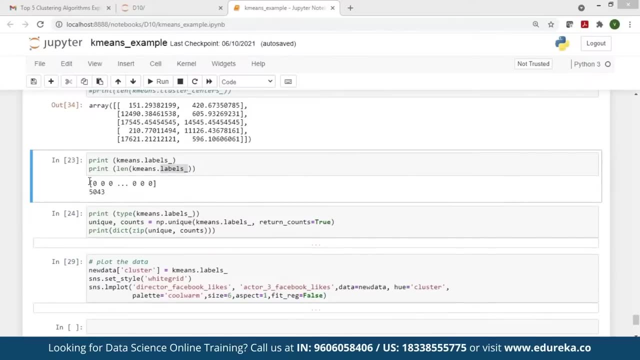 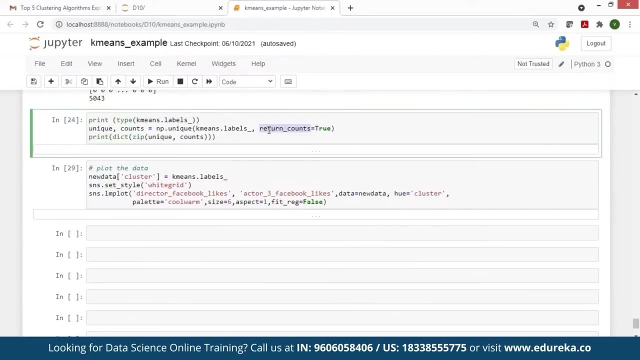 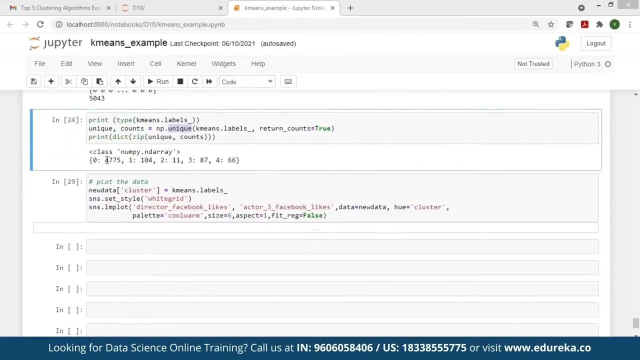 Build My Clustering Technique Algorithm By Print. What Is The Labels Which Are Generated? Labels Is Nothing Much. It Will Extract The Outcome You Can. 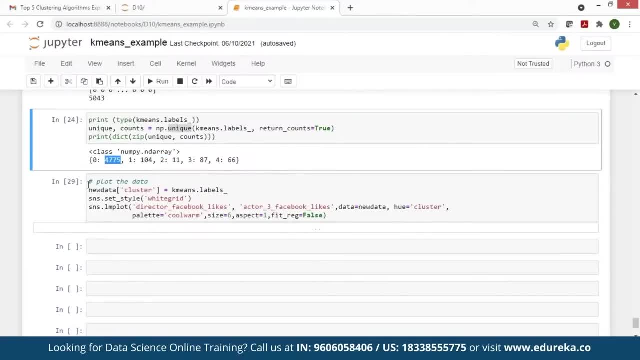 See That These Are The Labels, Numbers, Which Are Added To The Cluster. So The Data Properties Are Being Distributed And That's How The Clustering 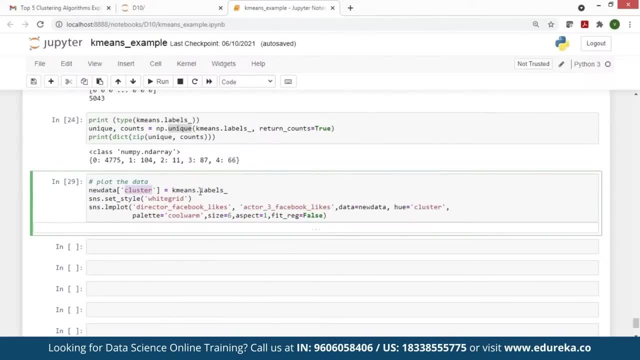 Technique Has Divided The Data Into A Cluster. Now You Can See What Is, Whatever The Column That I Call Director. As Facebook Life Works. 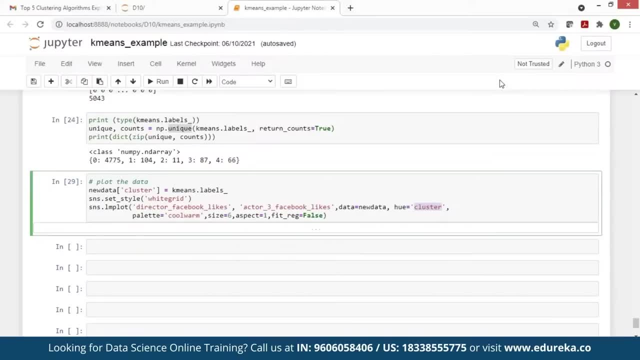 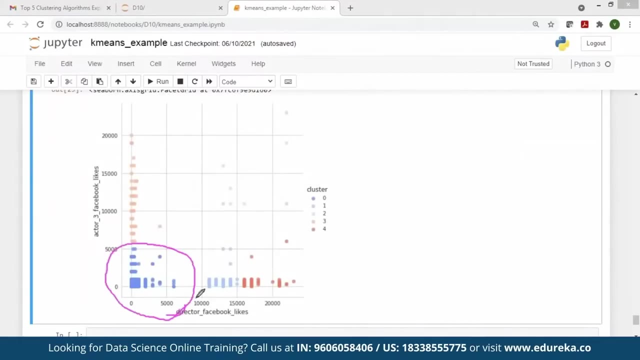 The Factor Facebook Life, And I'm Choosing This. Data Is Equal To New Data That Will Help Me To See How These Movies Are Been. 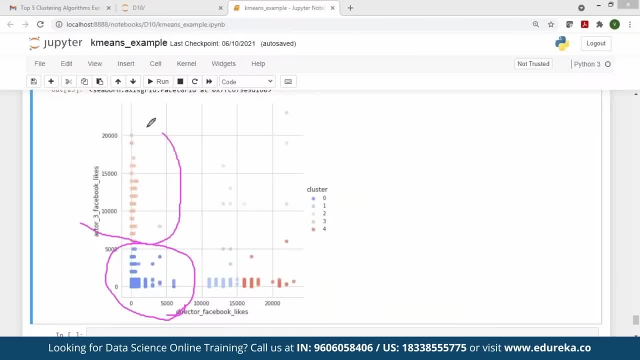 Segregated. I Can See These Movies Are Nothing But Cluster Number Zero One. This Is Nothing But Two, Number Three, Number Four, Like You Clearly. 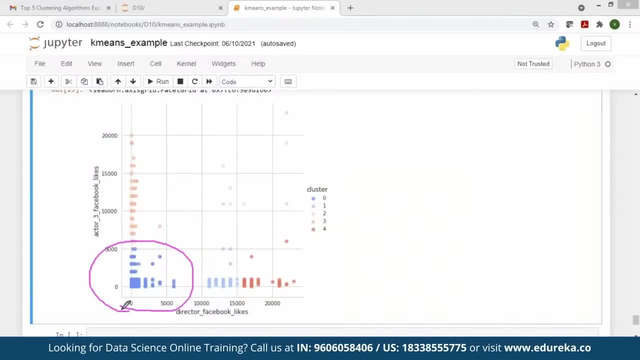 See That How The Cluster Has Came Up. The Movies Which Are Made By New People, With New Directors, New Actors Or New Directors Are Making. 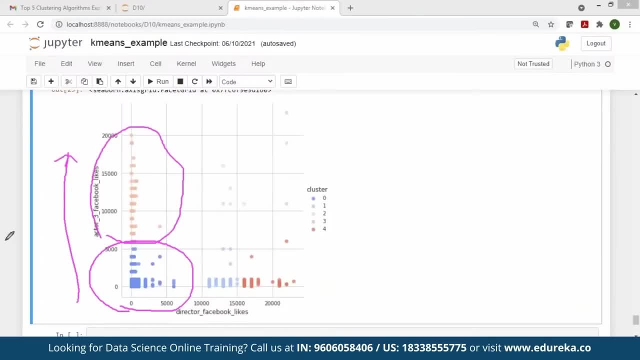 Film With New Directors. Very Famous Actors Are Making Films With New Actors And These Movies Are Something Where Average Fame Directors Are Making Films With. 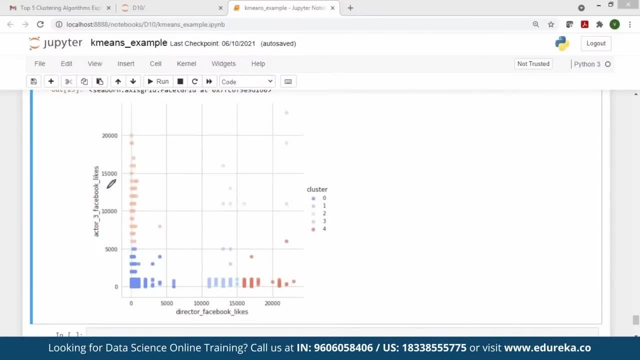 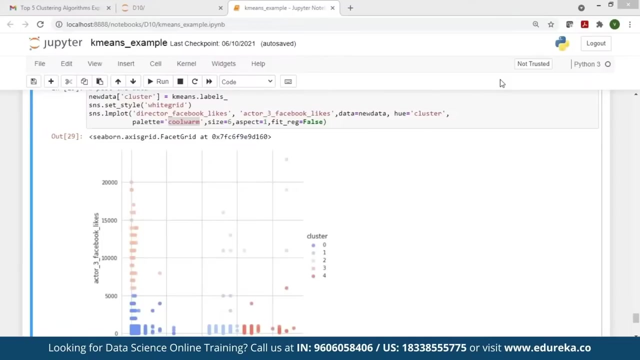 Some New Actors Is Organizing And Initialize At Huh, It Might Take Ố Longer Time For You To Segregated Every Comp nue Faeq. 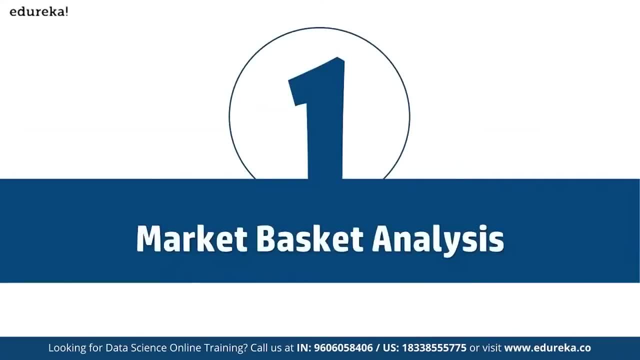 so it's a phenomenon called as the impulsive buying, and big retailers take advantage of machine learning and a priori algorithm to make sure that we tend to buy more, and that's what we have defined as a market basket analysis. now, first of all, let's discuss on that. so in today's world, the goal of any 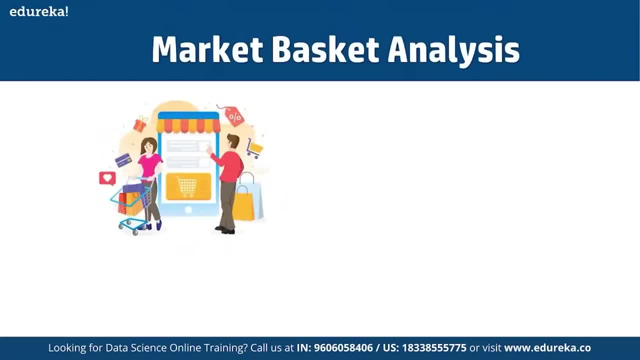 organization is to increase the revenue, and can this be done by pitching just one product at a time to the customer? the answer is clearly a no. hence the organization began mining data related to frequently bought items. so market basket analysis is one of the key techniques used by large retailers to 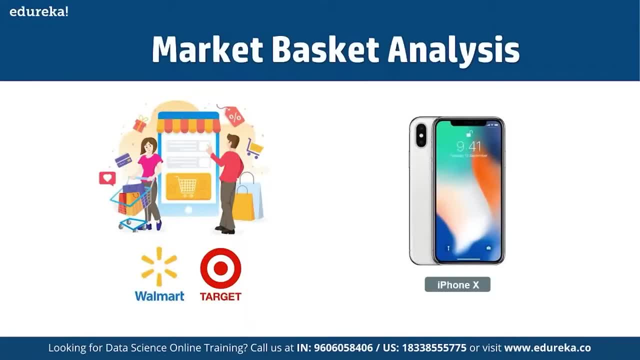 uncover associations between items, so they tend to find out the associations between items. so they tend to find out the associations between different items and products that can be sold together, which gives assisting in right product placement. typically it figures out what products are being bought together and organizations can place products in a similar manner. now 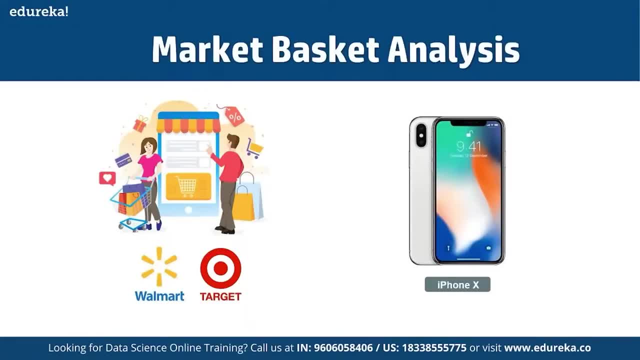 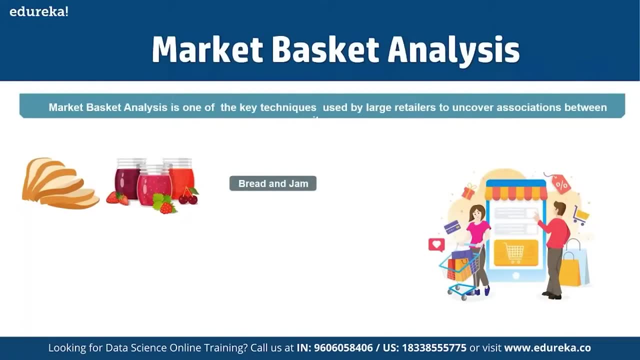 let's understand this better with an example. let's say we have people like people who buy bread usually buy butter too. so the marketing team at retail stores should target customers who buy bread and butter and provide them an offer to them so that they buy the third item, that we have eggs or any kind of Jam as well, correct? 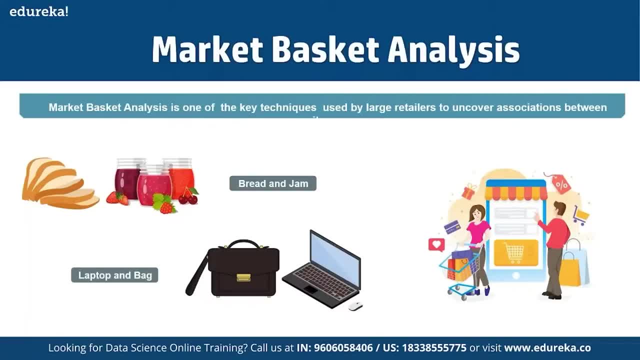 so if a customer buys bread and the butter and see a discount or an offer on eggs, they will be encouraged to spend more and buy the eggs. so this is what market basket analysis is all about. so this is a small example. let's say, if we take thousand, ten thousand items data. 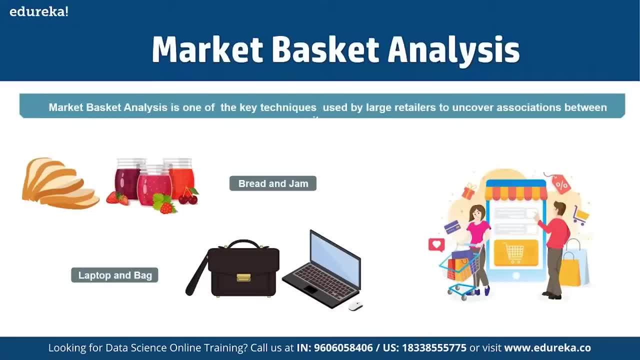 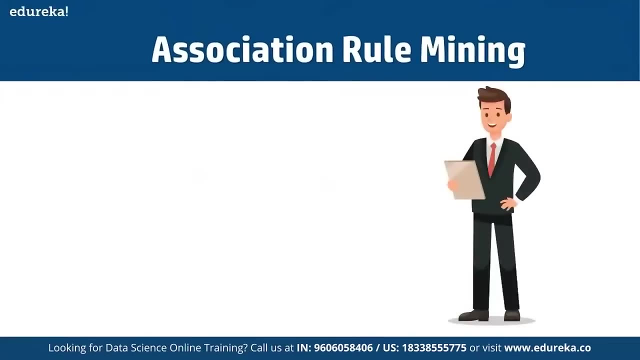 of our supermarket to a data scientist. just imagine the number of insights we can get out of it. and that is why association rules mining is also important to understand. so if we talk about association rule mining, then association rules can be thought of as an if-then relationship. 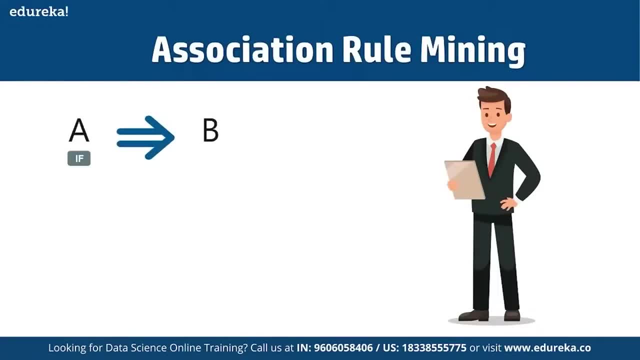 suppose we have an item a, so item a is bought by the customer and then the chances of an item b being picked by the customer to under the same transaction id is found out. so here we have simple if and then relationship. so there are two elements of these different rules. first of all we have the 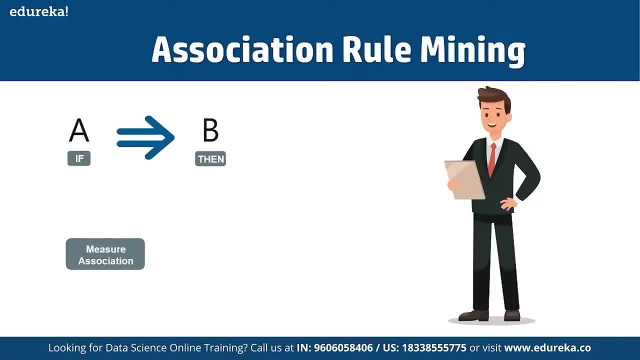 antecedent as an? if so, this is basically an item or a group of items that are typically found in the item sets or data sets, and then we have the consequent that is then so here, we have then, so then is basically used, for then it comes along as an item with an antecedent, or we can say a group of antecedents that we are. 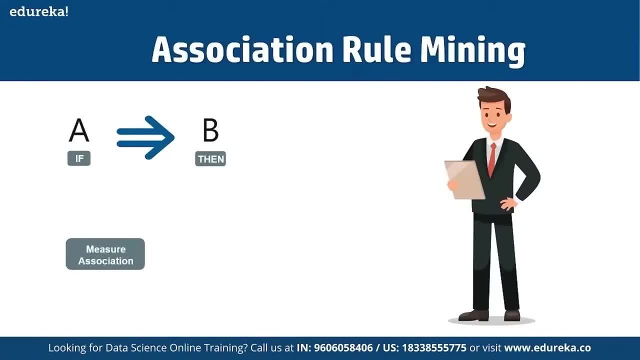 seeing and and this item we have discussed. it is basically an item or group of items that we found in item sets of data sets. now here comes a constraint. suppose we made a rule about an item use. we still have around 9999 items to consider for rule making, as we discussed. we have, we are 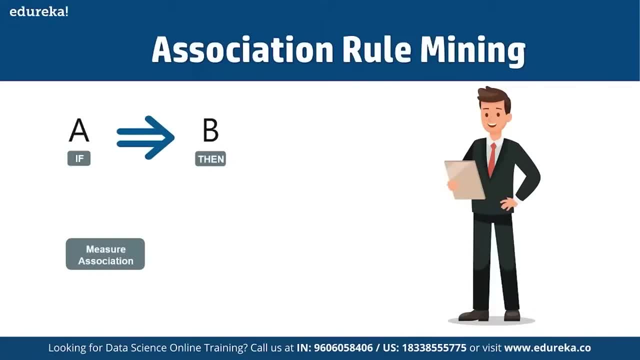 going to make use of 10 000 items. so this is where a priori algorithm comes into play, so that before we understand the apriori algorithm, let's understand the main mathematics involved here. so there are three ways to measure the association. we have support, confidence, and then we have lift, so which you can measure, the 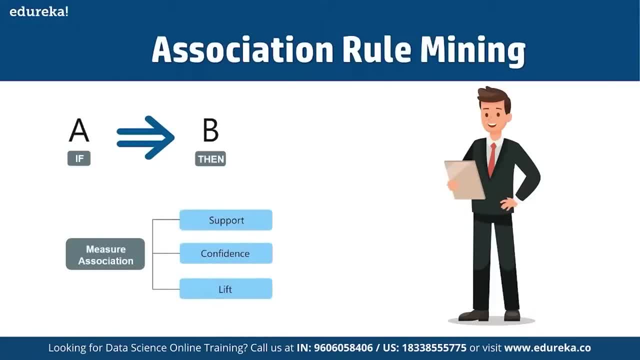 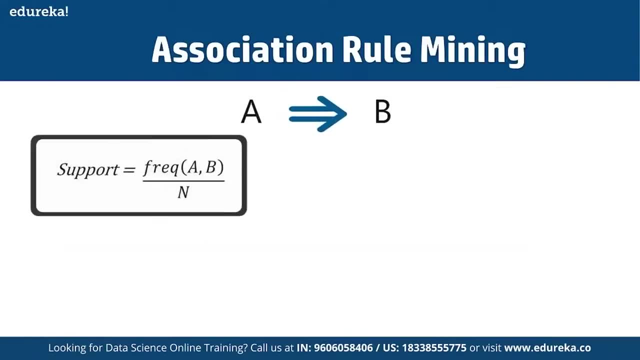 association. here you have support, confidence and lift. so support gives the fraction of transactions which contain item a. suppose if you talk about support here it is basically a frequent, the fraction of transactions which contains item a and b. so basically support tells us about the frequency. if they work against that, we can say frequently bought items or the combination of items spot. 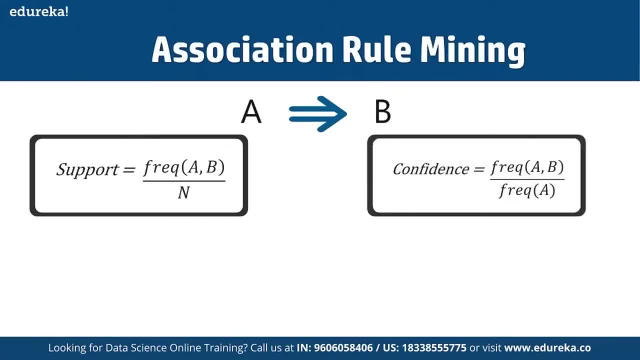 frequently by using a support. so with this we can filter out the items that have a low frequency. then we have confidence. so it tells us how often the items a and b are checked. the almost� occur together, given the number of times a occurs. So typically, let's say when we work with the a priori algorithm. 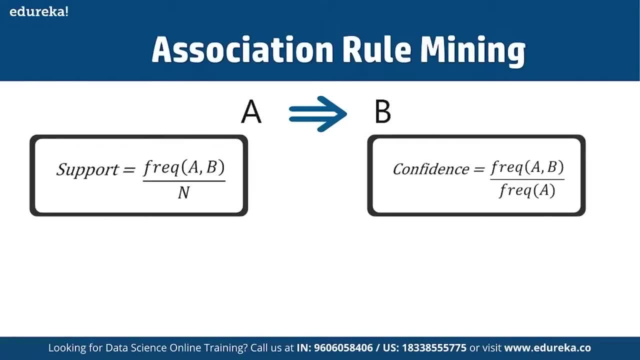 we define different terms accordingly, but how exactly we have to decide the value. That's the main question And, to be honest, there is not a specific way to define these terms. Suppose we have assigned the support value as 2.. Now, what is what exactly this means? 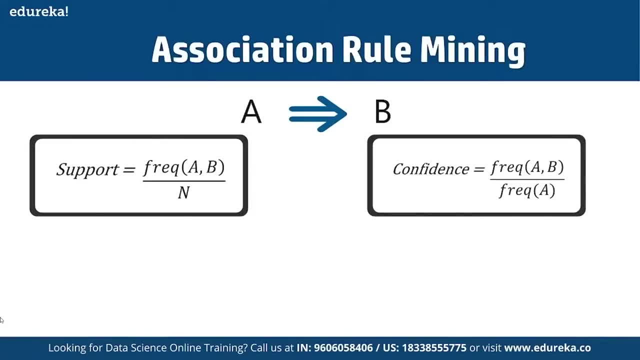 is until and unless the item frequency is not 2.. So here we define support as 2.. So until and unless the items frequency is not 2%, we will not consider that item for the a priori algorithm. So this makes sense as considering items. 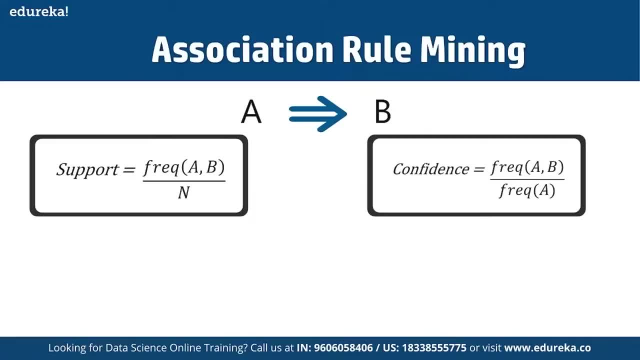 that are bought less frequently is a waste of time because, let's say, if only 2% of users are you are buying this item along with the item that they have bought, then obviously they cannot use it. We cannot even consider what is for the a priori algorithm. 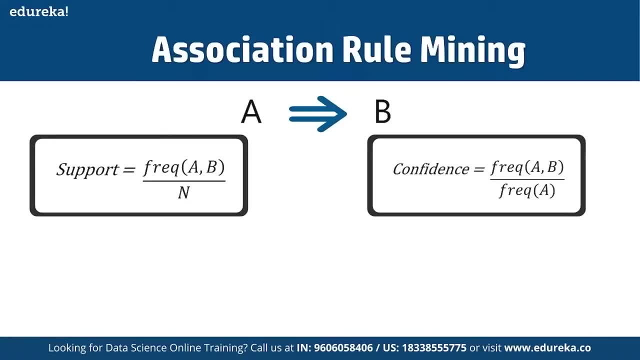 that we are going to work on here Now. suppose after filtering we still have around 5000 items left now creating Association rules for them is a practically impossible task for anyone, and this is where the concept of lift comes into play. So basically, lift indicates the strength of a rule. 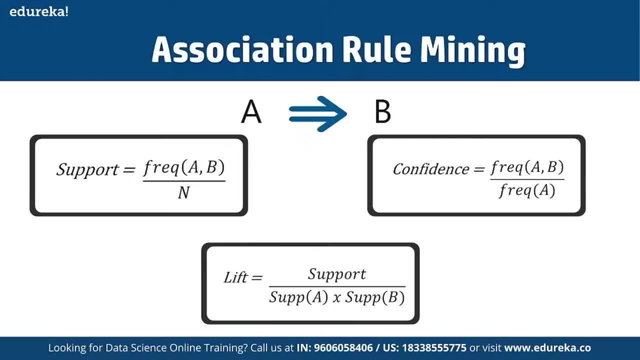 over the random occurrence of a and B and it basically tell us the strength of any given rule here. So for finding that out, we have simply divide by the support of a and then support of B. So focus on the denominator. It is the probability of the individual support values. 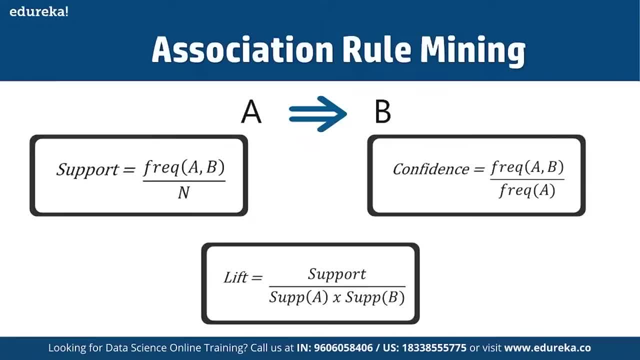 of a and B and not together. So lift explains the strength of a rule. So more the lift, more is a strength. Let's say a as opposed to. we can say for a is to be so, if a if, then relationship before. so if you talk about 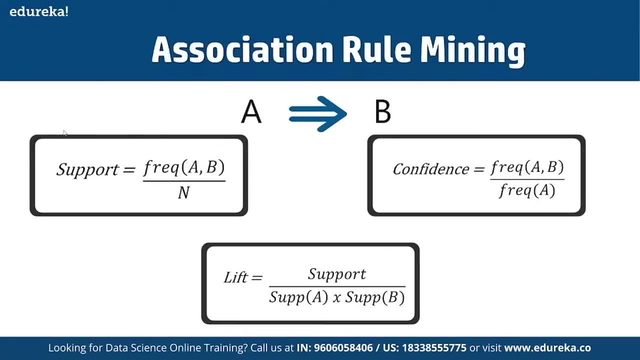 if then relationship for a- B, then that lift value is: for suppose let's say, for this reason the lift value is 4. here That means if you buy a, then the chance of buying B is 4 times if the lead value is 4, or we can say it's 4 times. 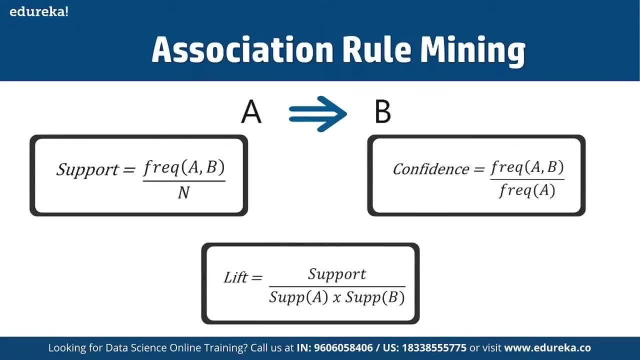 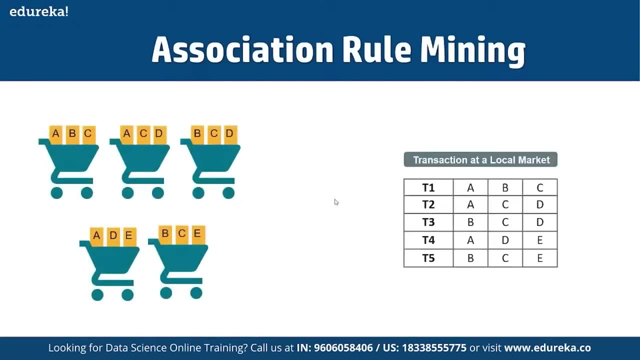 if the value here is 2, then it is 2 times, and so on. as a part of the lift, values are fine, So let's get started with the a priori algorithm and now let's see how exactly it works. All right, So now let's discuss on the concern. 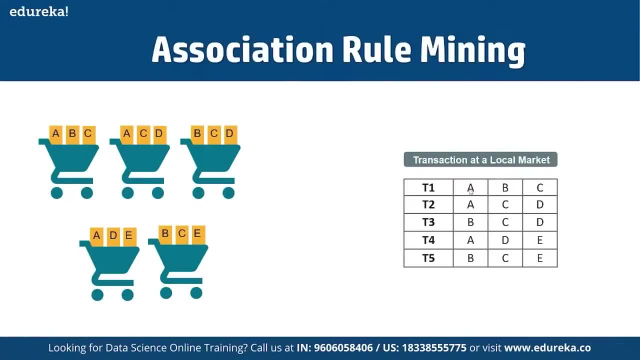 If this is what we discussed here- the transitions at our local market, and here we have ABC for a in transition to, we have a CD in transition 3, we have BCD in transition for, we have a de and then we have to transition 5.. 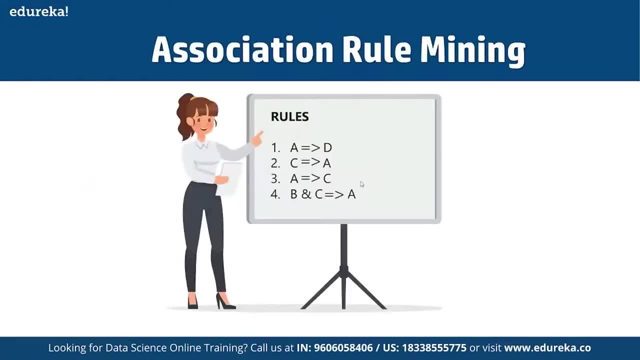 We have a BCD. So let's say here, If you find out the entire rules here- than a if a, and again they are going to purchase D. if they buy a seed, again they have option of going for a. if they buy a, then they have the option. 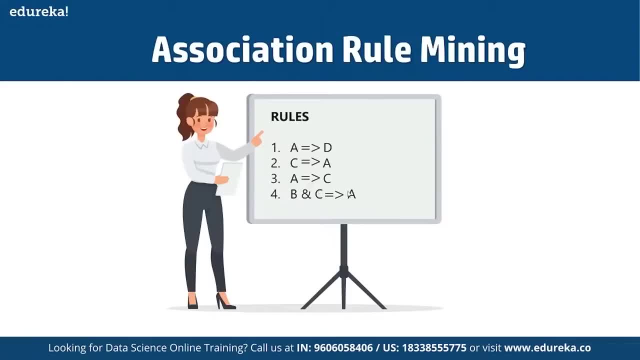 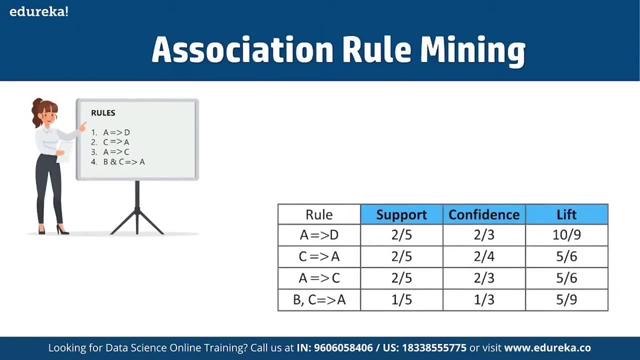 of going for C, and if they buy B and C together, then they are going to buy by a as well, And then, same way we can find out the support. So again for if a is for those who are purchasing a, the probability of buying D, it is some in terms of support. 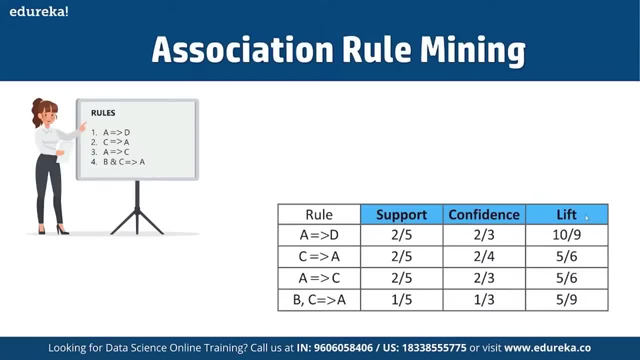 It is 2 by 5 in terms of confidence. It is 2 by 3 in terms of lift, It is 10 upon 9 way. as for see again for a, that means what is, what is a possibility that those who have purchased a seed will be buying a. so you can find the support. 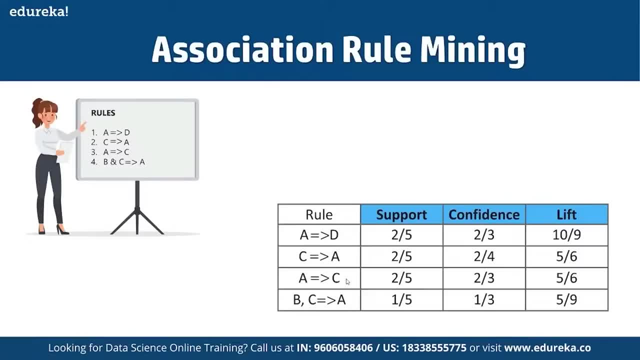 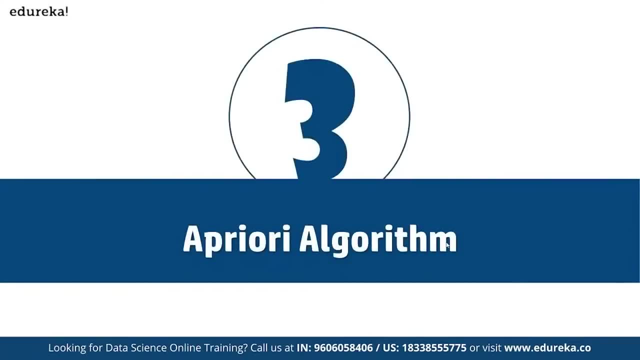 as 2 by 5 conference at 2 by 4 and lift us 5 by 6, same way for C and same way for BC and a. so we can see how the probability is going to be distributed as we first, as we find out the possibility. 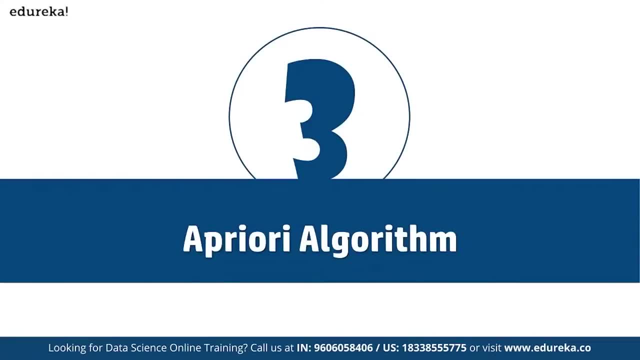 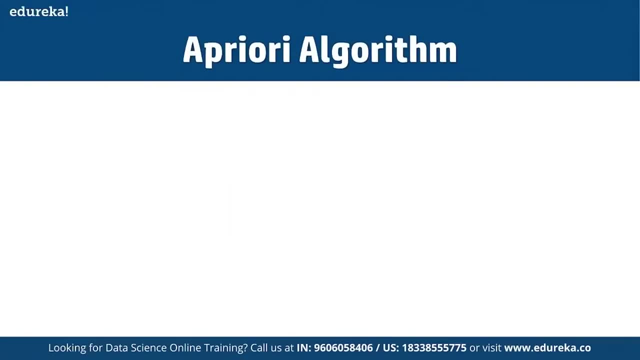 of one product to be bought over the other. All right, So now let's assume further on the a priori algorithm. but so a priori algorithm uses frequent item data sets- I guess item sets or data sets- to generate the association rules. So it is based on the concept that a subset of a frequent item set 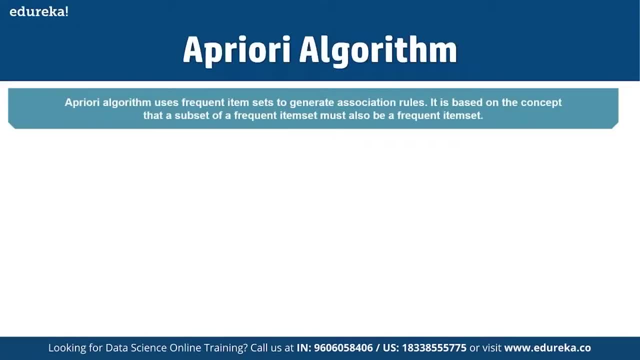 must also be frequent. item set must be a frequent item set, and frequent item set is an item set whose support value is greater than a threshold value that we have support. So we're getting what exactly a frequent item set is: It's an item set whose support value is greater. 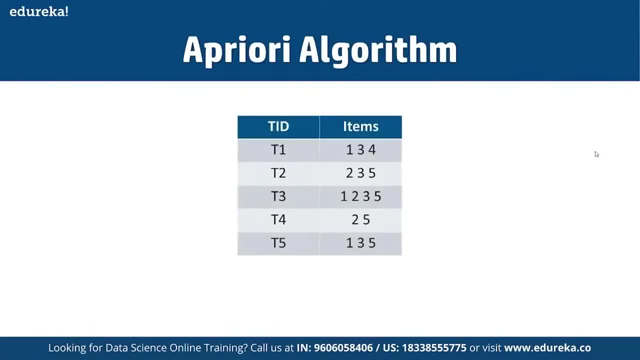 than a threshold value. All right. Now, if you talk about a simple example, here we can. let's say, we have the following data of a store here, So we have the transition ID here, and then we have nine items. So here we have. these one are transaction IDs. 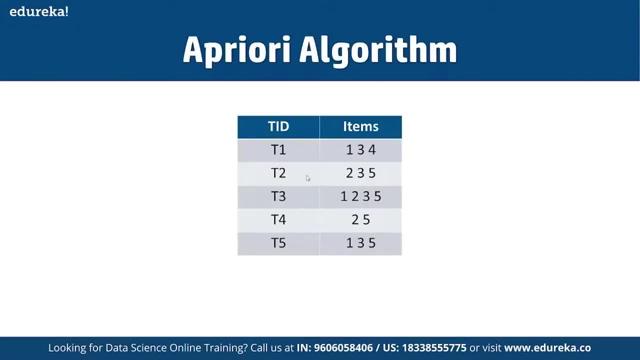 and here we have the items. So in transaction one we have 1, 3, 4, 2, 3, 5, 1, 2, 3, 5, 2, 5 and 1, 3, 5.. So if you talk about the first iteration now, 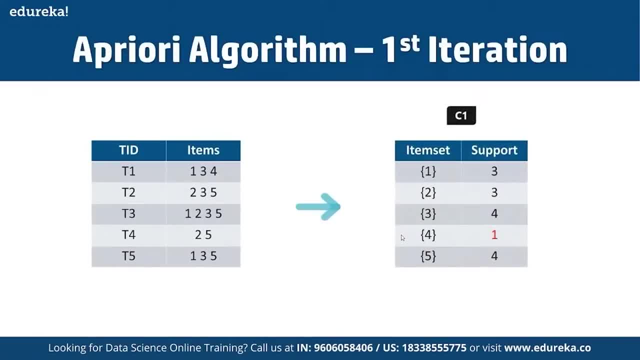 let's assume the support value is 2 and then we can create the item sets of the size 1 and calculate their support values as you can see here. So, as you can see, of the item 4 has a support value of 1 support value. 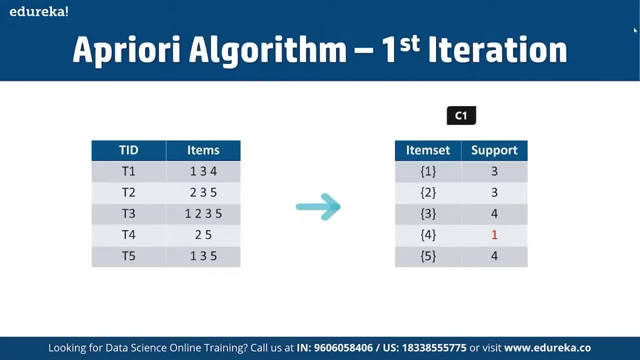 of 1 here, which is less than the minimum support value. So we are going to discard 4 in the upcoming iterations and we have the and that's how we can have the final table defined here as the FN. So here we are going to discard the value. 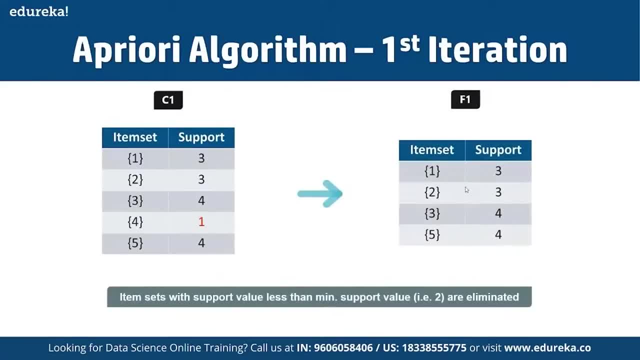 That's 4, and then we are going to have the final value to be giving given to us. So the item sets is support value less than minimum support value, That is, 2, are going to be eliminated. Next, we are going to create the item sets of size 2. 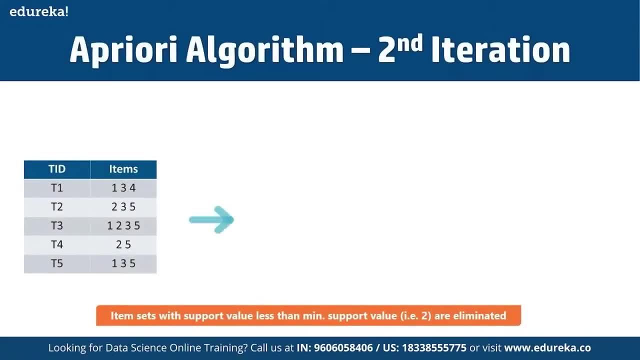 and calculate their support values. So all the combination of item sets in F1 are used in the iteration. So here we have C2 and then we have the F1. So basically here we are going to make use of the entire integration here and item sets having support less than 2 are eliminated again. 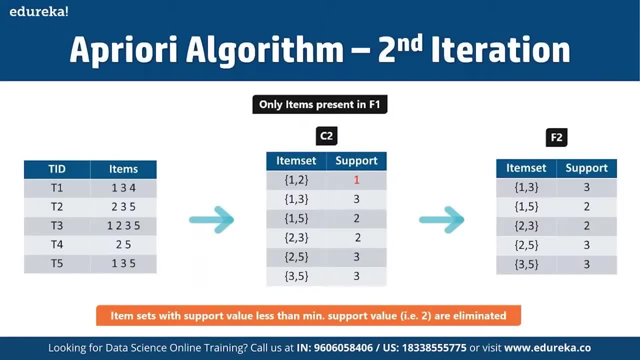 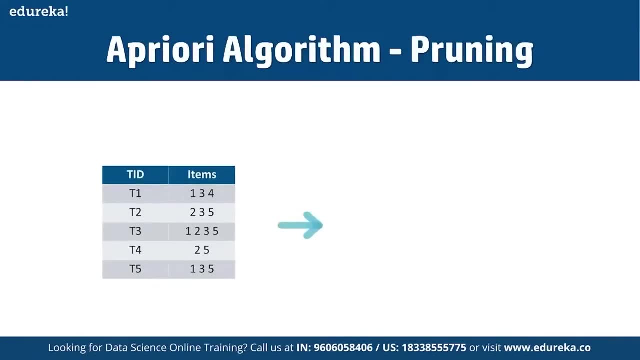 And in this case we have 1 and 2 right. So let's now understand what exactly we mean by printing and how it makes a Priory one of the best algorithms for finding the frequent item sets. So if you talk about pruning, then we are going to divide the item sets. 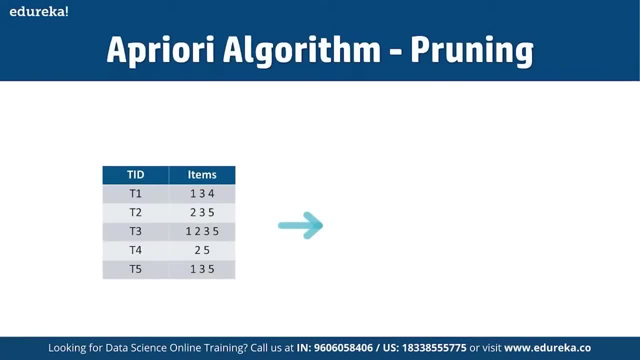 in C3 into subsets and eliminate the subsets that are having a support value less than 2 from this given item sets here. So here we are going to work on the third iteration. So we will discard 1, 2 and 3. we are going to discard 1, 2. 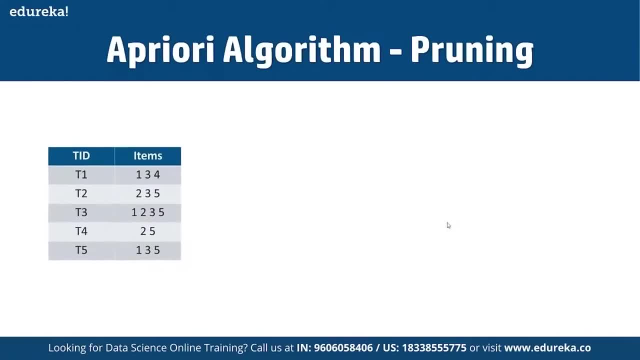 and 3, and 1, 2 and 5 as well. So they both, as they both contain 1 or 2, and this means again- and this is the main highlight of the Apriori algorithm. So again here we are going to discard 1 and 2. 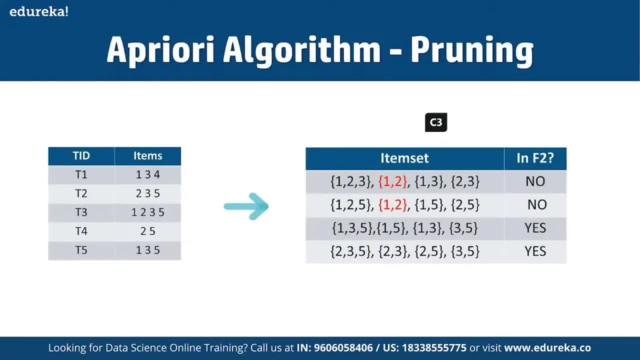 and this is the main highlight of this entire algorithm here, because again, the 1 and 2 is a common thing available in these, in these both data sets right. So this is the main highlight of Apriori algorithm here. And then, if you talk about the fourth iteration, 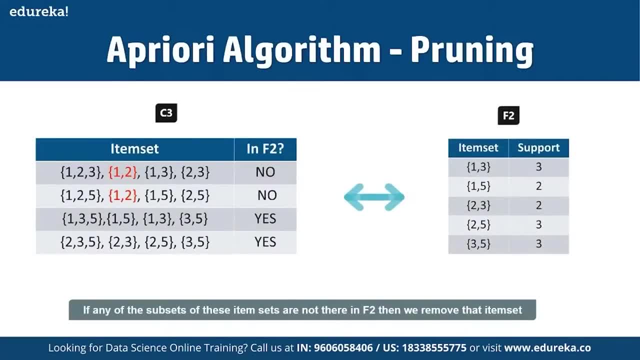 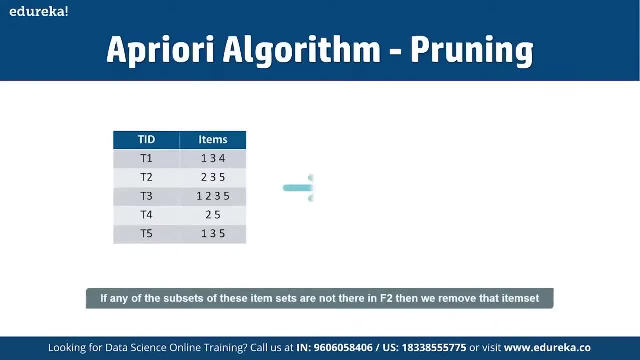 so if now, as you can see, if any of the subsets of these items are that are not in F2, then we are going to remove that particular item sets. And then, in terms of the fourth iteration, let's suppose here we have the transition ID. 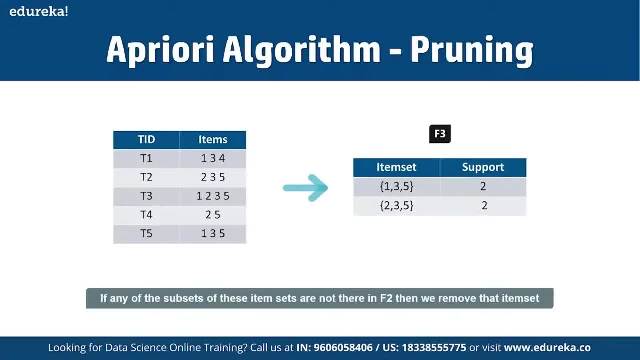 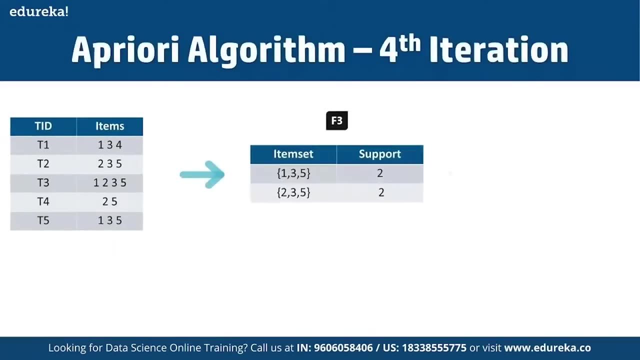 and here we have the item set And support available. So, since the support of this item set is going to be less than 2, so we will stop here and the final item sets will have is the F3 one. And now, still now, we have not calculated the confidence value yet. 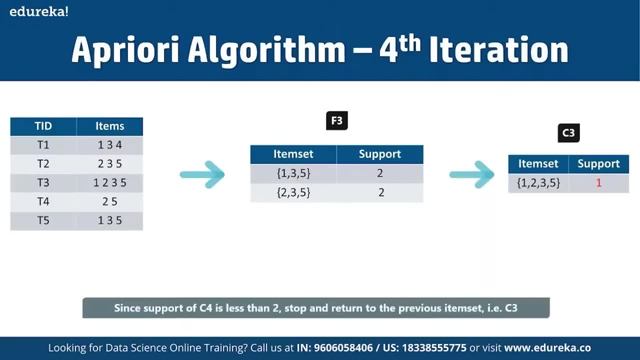 So again, this is something that we have to keep in mind. So with F3 we get the following item sets: That means for one we have 1, 3 and 5, and subsets are 1, 3, 1, 5.. 5, 3, 5, 1, 3 and 5.. 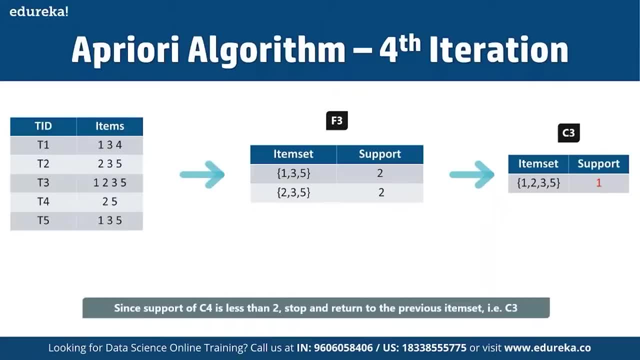 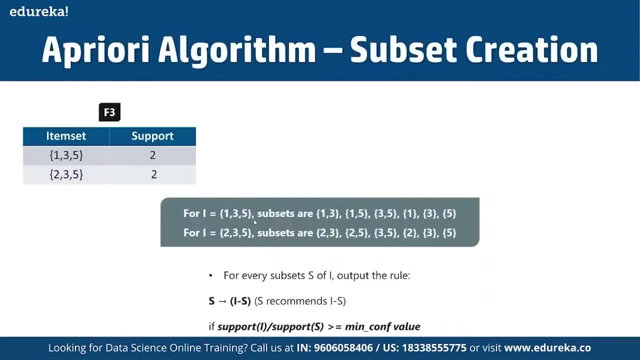 Whereas for item sets 1, again we have 2, 3, 2, 5, 3, 5, 2, 3 and 5 itself for the other time, itself available. So for one we have 1, 3, 5.. These are subsets of 1, 3, 1, 5, 3, 5, 1, 3 and 5, whereas 2, 3, 5 are subsets. 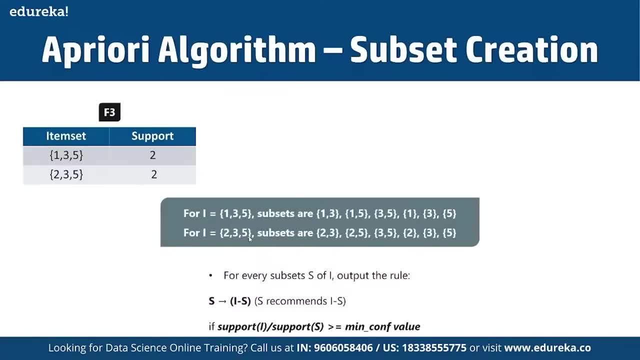 of 2, 3, 3, 5, 2, 5, 2, 3 and 5 right and for every subset of I. we have to find the output rule Now, when we are going for applying rules here, So we will create the rules and apply them on item set F3.. 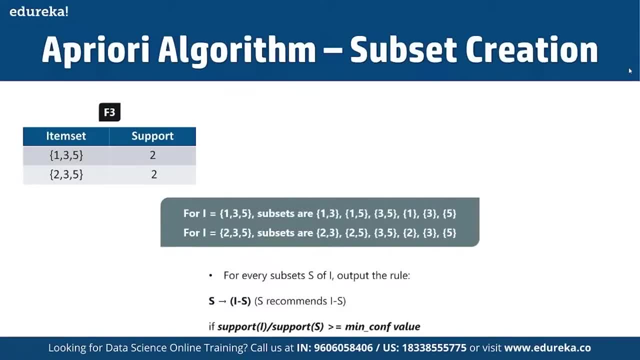 So now let's assume a minimum confidence value is 60%. so for every subset of whether that we have s of I, so are, the output rule is going to be: s is going to be recommended, So s is going to simply recommend is, and then we hit support: it is I. 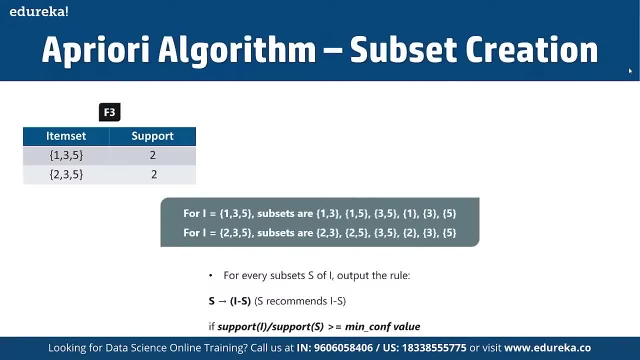 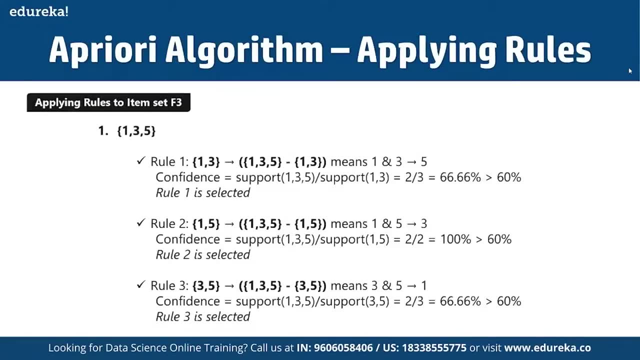 and then we can simply divide this by the support cell and to find the minimum Confidence value is going to be 25.. So your rule 1 here is 1, 3 is again a subject that means 1 and 3 will result to 5.. 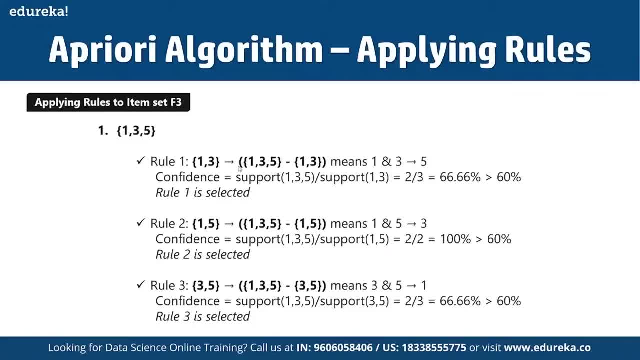 That means if a user is purchasing 1 and 3- both the items- then we have a good possibility of the customer going for the fifth item as well. So here the confidence is going to be. support 135 divided by a support: 1- 3, that is, 2 by 2.. 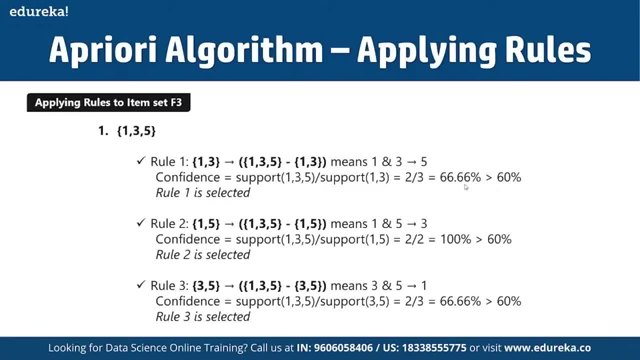 That is, 66.6 person is 60 person. So here rule 1 is going to be selected and in rule 2. We have 1, 5, 1, 3, 5 minus 1, 5. That means if the people, if someone is purchasing 1 and 5. 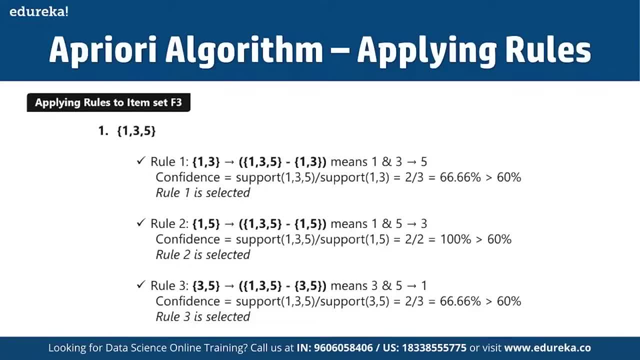 then they are going to have a good possibility of going for three as well, where we are going to see the confidence and support for finding the confidence. We are simply going to again subtract support for 1, 3, 5 by support of 1. 5 is 2 by 2 and this is going to simply be. 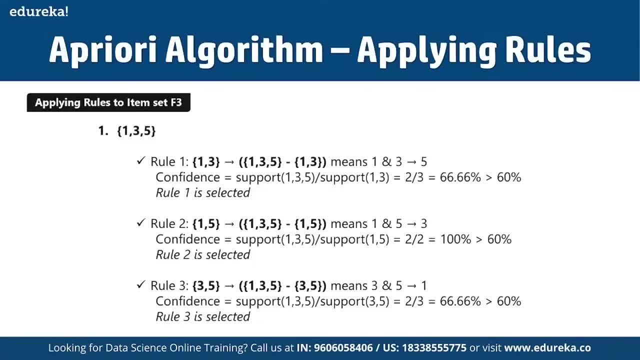 translated 100%, and which is much greater than 60% as well, and same way in rule 3.. We have 3: 5 1. 3, 5, 3.5.. That means here, if someone is going for purchasing 3 and 5. 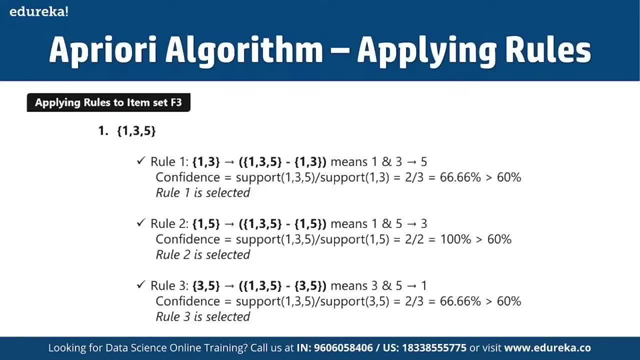 then they are, then they are going to high possibility of going for one as well. So here the conference is: support 135 divided by support 3, 5, that we get as 66.6%, and here the rule 3 is going to be selected here, as you can. 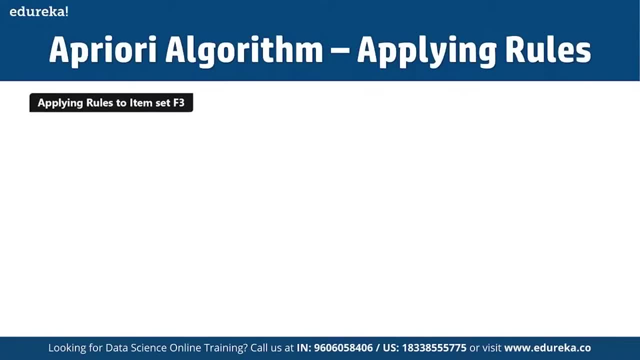 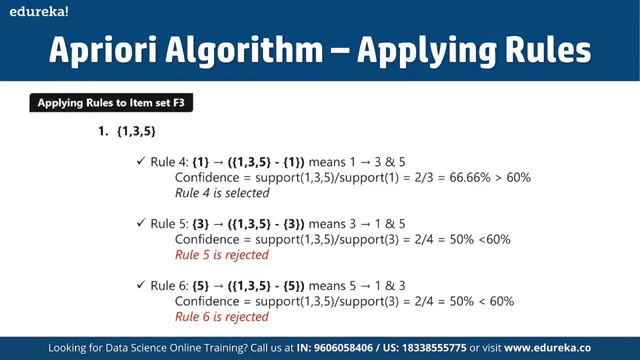 see here, Now, up right now. if you talk about the application of rules here now, when we are talking about this rule here, we can see whenever the confidence is going to be more than 60% to find him, Then this rule is going to be selected, as you can see here. 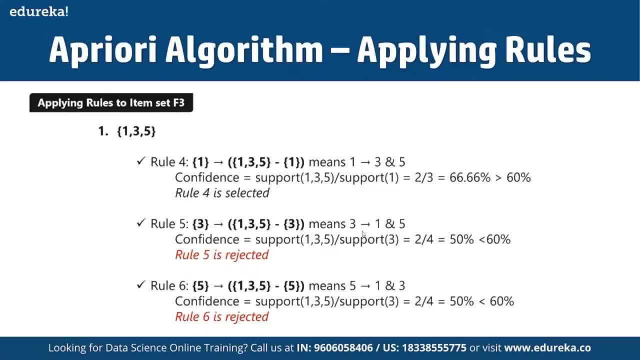 in this rule 5, where, what? where those who are purchasing three, they have a possibility of going for 1, 5, both. So here the confidence is less than 60%, which is why this is going to be rejected. same way for rule 6 as well. same way. 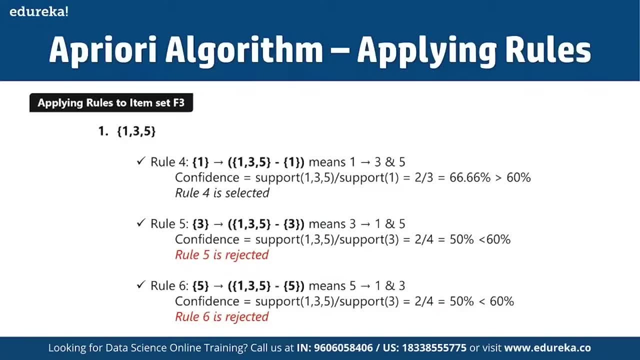 here for rule 6 as well, because here the confidence is going to be less than 60%. then that's why this is going to be rejected here. Okay, because again we have. we have assumed a minimum confidence level for 60% and wherever we are going to get the confidence, 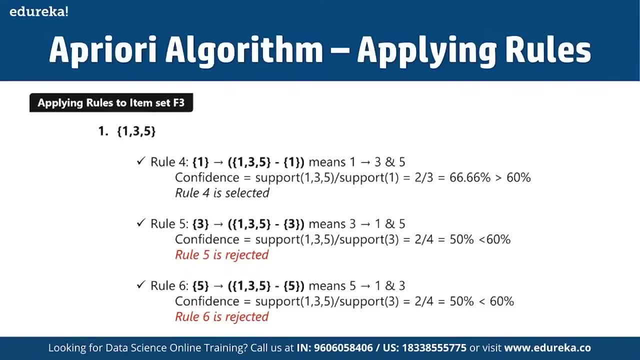 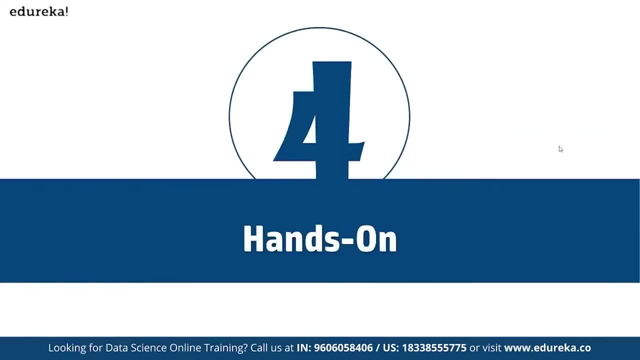 less than 60%, they simply going to reject that particular model here. All right. So first of all, that's how we have seen how we can create rules in a proprietary algorithms here, And the same steps can be implemented for this item set. 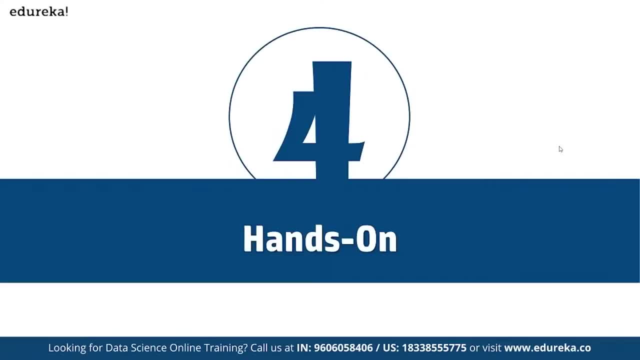 2, 3, 5, and then we are going to try it and see which rules are accepted and which rules are going to be rejected, and how we can implement the a priori algorithm in python. All right, so let's fetch some sample data sets here. 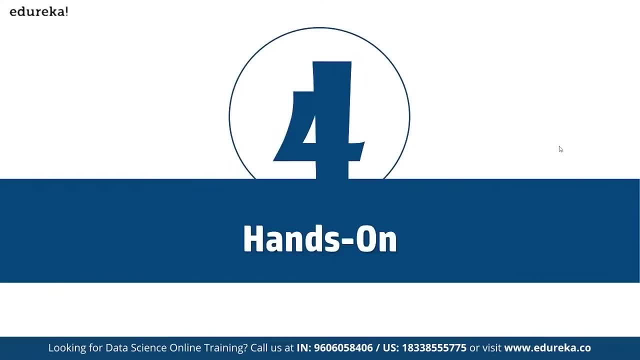 that we are going to work on. So to get started working on the actual analysis here, We are going to make use of the pie charm ID, so we can use any of the ID, Or we can also make use of the python hormone, ideally, to get started. 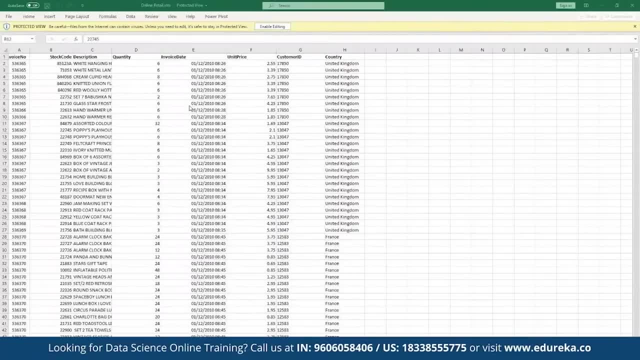 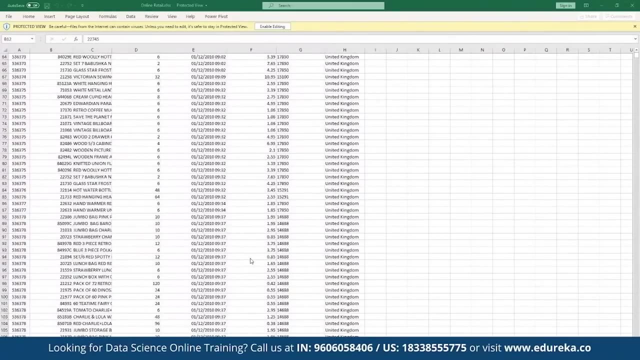 So we are going to make use of pie charm In this file will be having the access to the invoice number. We have the stock code, We have description, quantity, invoice date, unit price, customer ID and then we have the country. So this is a data point, that this is a file that we are going 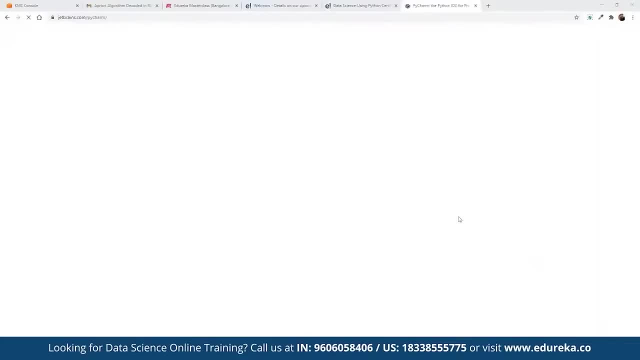 to work on, All right. So in the meantime we are also going to install pie charm as a main ID. So in case you want to work on python and we can make use of pie charm ID, which is one of the most popular IDs for getting started, 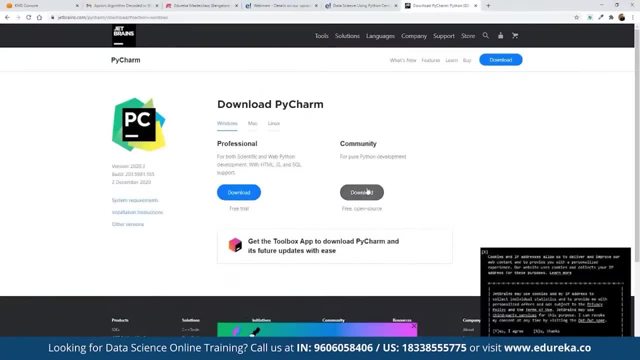 and pie charm is also offered as a free tool. Let me see how we get is also offered as a community tool here, So you can use it as a community tool in order to get started. So once we have the access to it, we can open this up. 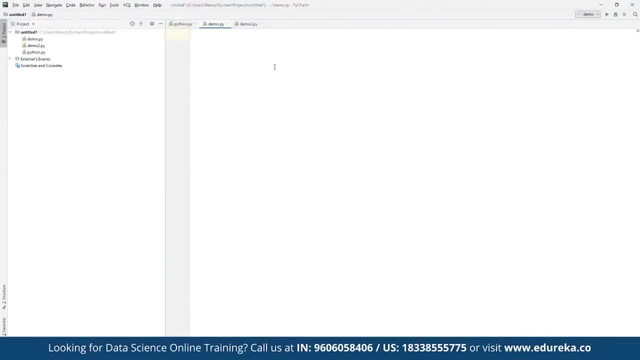 All right, So here we can get started first. First of all, we are going to work on the Pandas library. So here we are going to import Pandas And mlx10 libraries imported and to import and read the data set. So here we go, going to choose import. 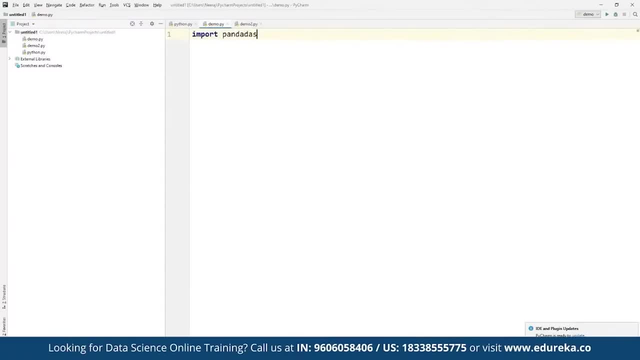 and then here we are going to find import pandas And from pandas as speedy. So here we go to import pandas as speedy and then we are going to use from mlx10.. We are going for frequent dot, frequent patterns, We are going to import a priori. 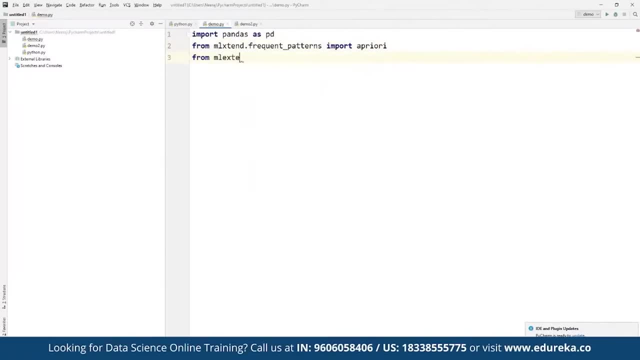 And then we are going To use the same from mlx10. Dot. frequent Underscore patterns. We are again going to import Association rules. They're going to pull up import Association rules and then we are going to create a data frame where we are going to make use of funders Diary. 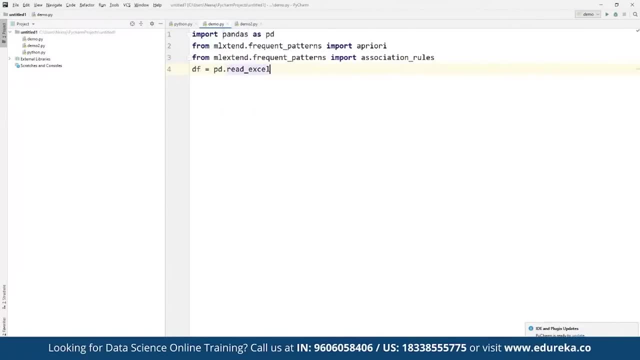 as PD dot read. and here we are going to read Excel file If it, if it is a CSE file that we define as read CSV And here we can define the path. suppose here The file is currently available in our users location and the users we have it in downloads. 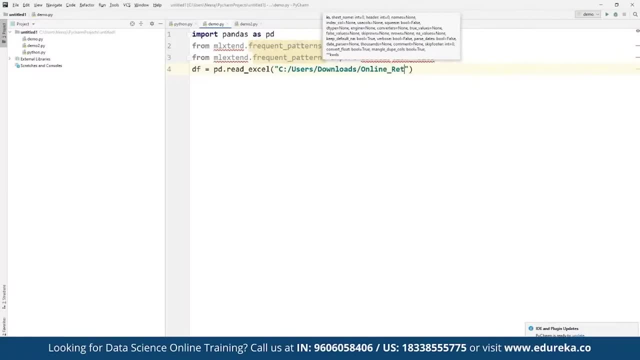 and by the name of online underscore retail. Dot Excel is 6.. So this is the free that we have currently imported here And, in case, suppose, some libraries are currently missing here, So we can import these libraries As in when acquired here. suppose if we, if something is missing here, 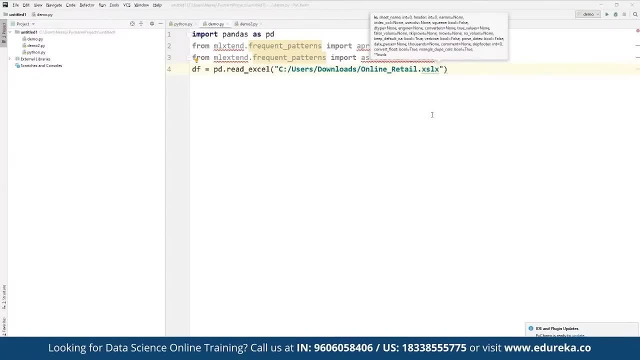 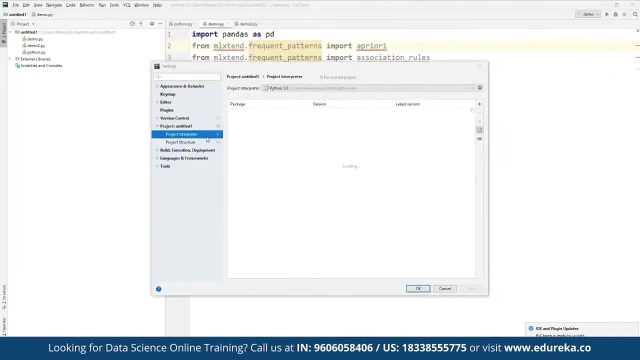 we can simply import these libraries in case they are not properly installed. So for installation of any new that we have we can go to file on a settings. here We have to go to project interpreter in case you want to add any specific library here. 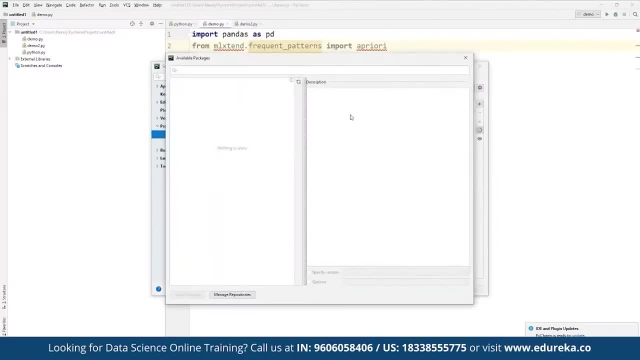 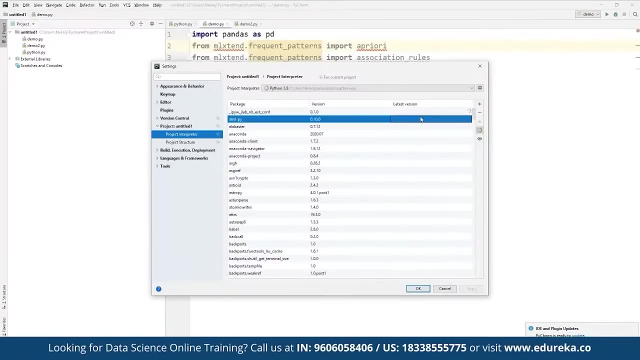 then we get simply click on plus and then we can choose which all library we want to add. here We can simply see the entire list of all the libraries currently installed here And now. if you want to start with more, then we can simply add more libraries. 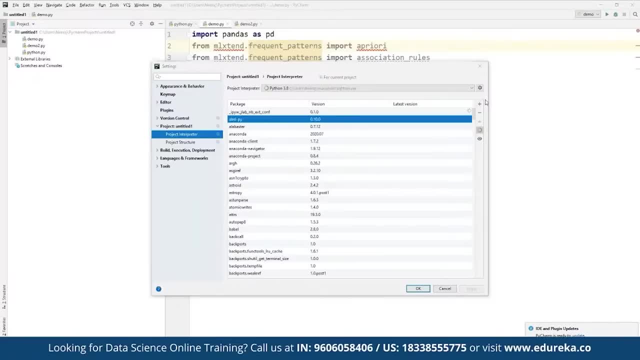 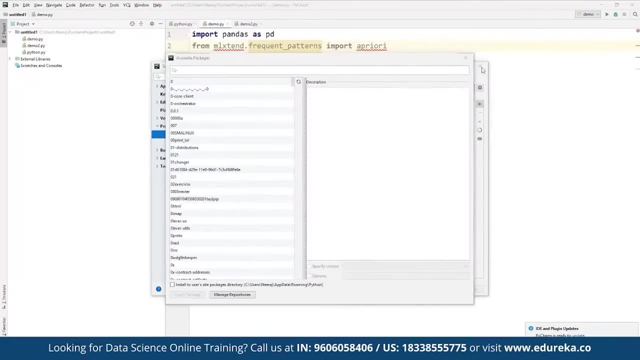 and then we can start deploying it one by one. So, for example, suppose if you want to install any specific library here, so here we can. so let's say, here We want to install the Apriori here. So I can see how you here. 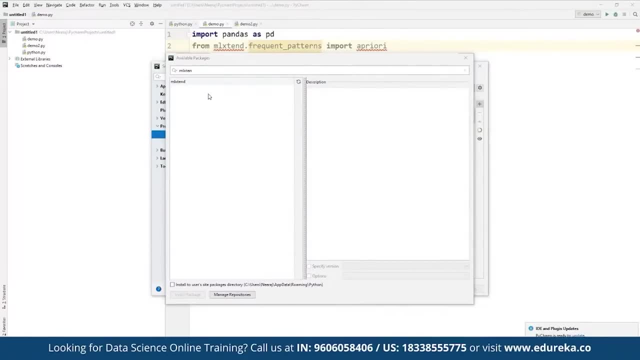 We can also import the image strength. So if this library is currently available, we can simply click on install package and this is going to be installed and stored in a system as a library. same way, If you are looking for Apriori here. 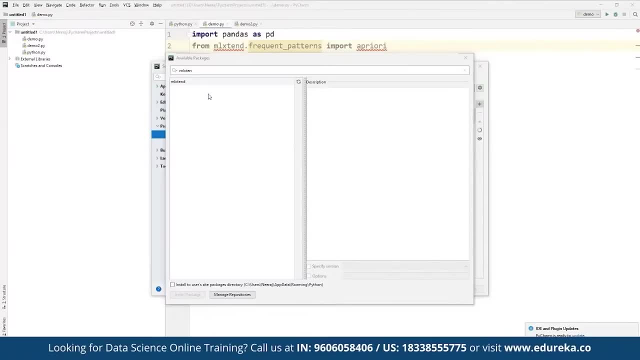 So here we can also use, because again, at the end we are going to use Apriori from the MSN that we have imported. So here we are going to install the other package as well. The first package for evanescent has been installed. 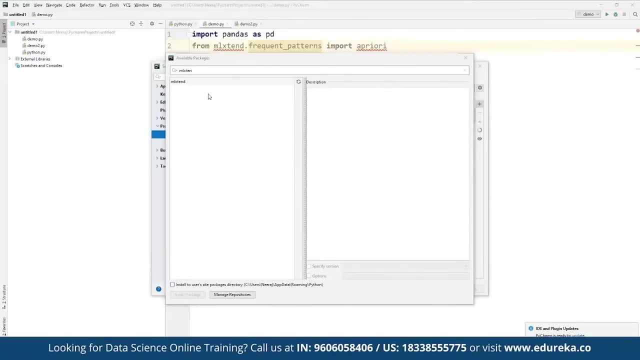 and now we are. and now if you want to install the other packages, then we can also install it. So in case we have missing some kind of library, that we can simply install it, or in case we are, you have not used those libraries, that we can simply use them one by one. 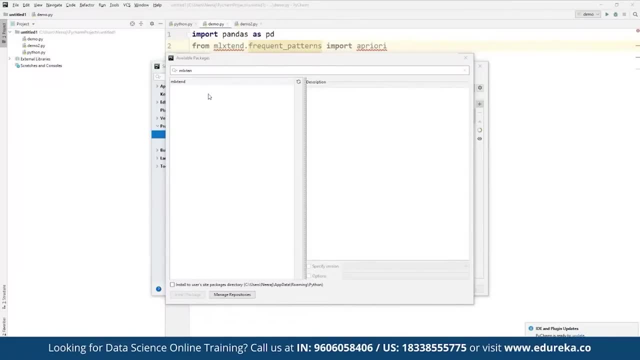 So, once we are done, we can simply come out. So, as you can see now where's the libraries have been properly installed and we will be able to see there is no error being shown here. And this is the path of the file: that where we have stored online retails dot XLS file. 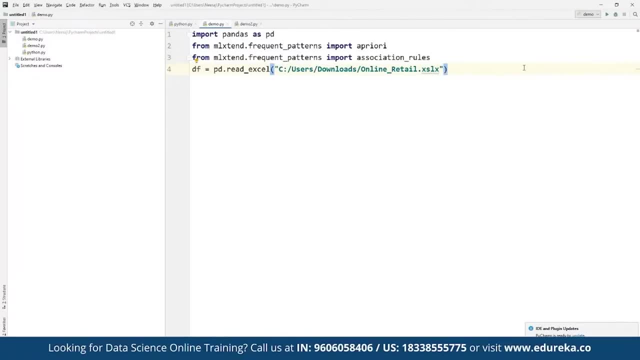 So just to confirm, we can confirm that we do have the file by the name of online retail, dot XLS X available here in a download directory. So once we have specified the file here and then we are going to simply use data frame. So in case we want to see the first few entries, 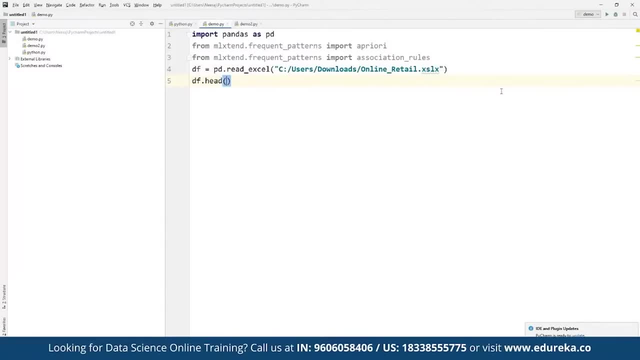 of the current data set that we have imported. So here we can simply define DF dot head and then, from the given path, The first two head is going to be returned back as a response. Now, once we are done, we can simply start applying it. 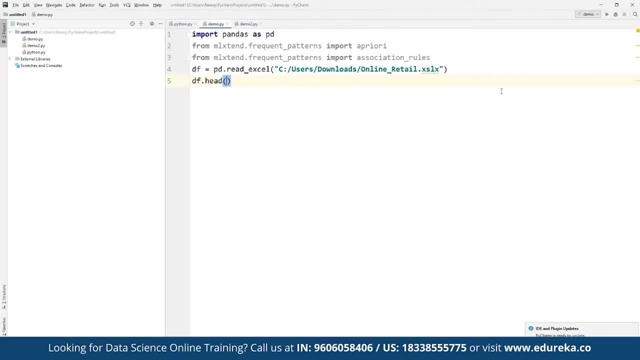 Now, once we have the access to the data set here, next step is going to be focus on data cleaning, which will include removing spaces from some of the descriptions that we have, and for that we are simply going to specify here We can, instead of using the data page, the data frame head here. 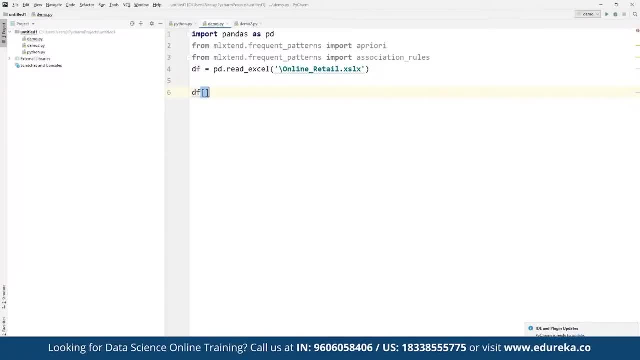 So now we are going to use the data frame and then from here we are going to add a short description. So here we can add a short description here. So basically, we are going to do work on data cleanup, which includes removing spaces from some of the descriptions. 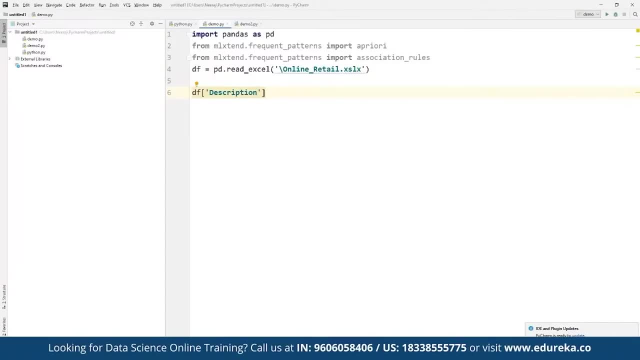 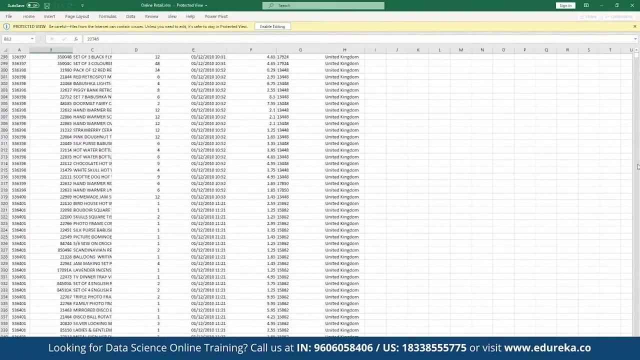 and then we are going to drop the rows that don't have invoice numbers and remove the credit transition as well. For example, suppose we have some rows where we don't have the, where we have blank transactions itself, right, We have some blank invoices. 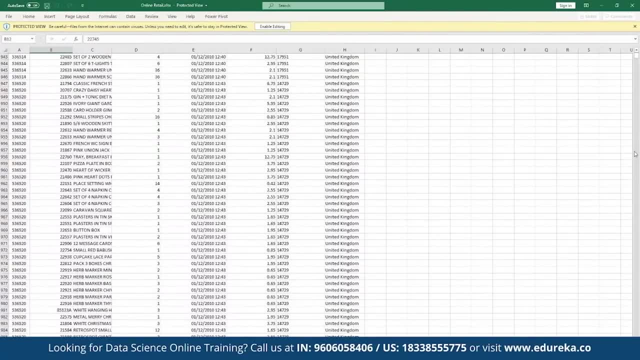 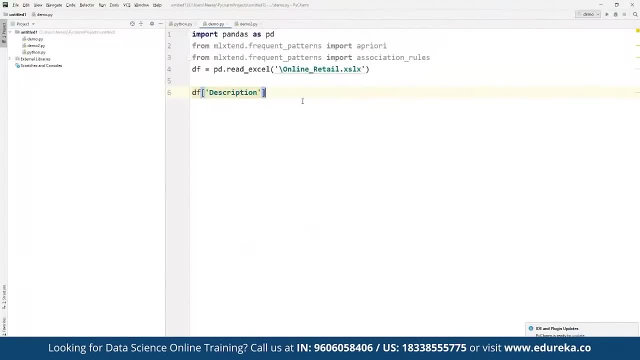 and then we have invoices numbers and remove the credit transition where we don't have any kind of invoice number face here. All right, So we have, we have to go in here, We have to work on removing those kind of anomalies. So here from the data frame: 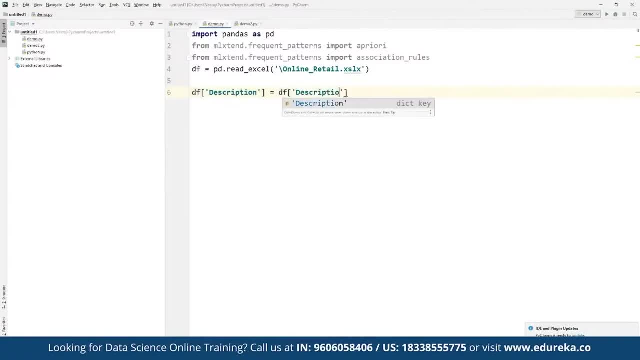 So here we can add parameter as description. Now, on a description, we are going to use a string function, Our string dot strip. So stream functions available under string. We're going to make use of it. And then same way from data frame. 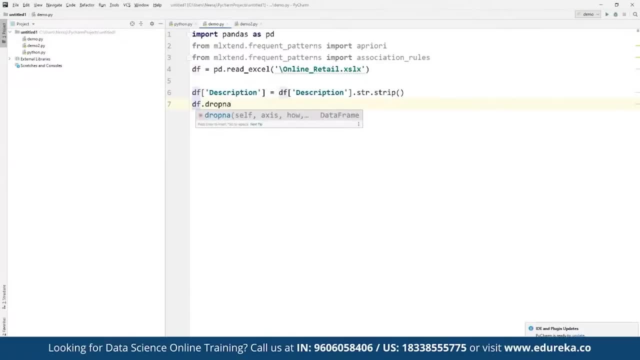 We are going to work on dropping. There we can find the values for X is equal to 0, and then the subset where the. what kind of values we have to drop? Do you have to define that parameter? where the invoice number Is going to be in place is going to be true. 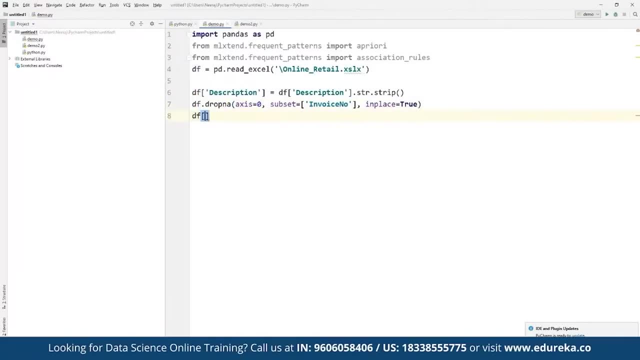 And then from data frame we can find the invoice frame, The invoice number, and then we can define it to be our data frame. where invoice number, again we are going to convert that to a string itself. So here we can define data frame and then the invoice number type. 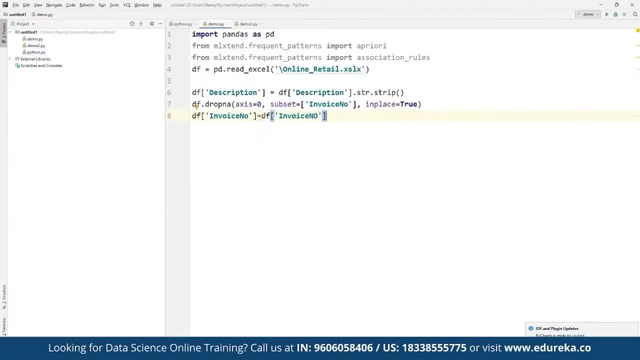 So here we have invoice number Dot, the AS type, and then we are going to the SD type of looking here We can keep it to AS type. So here we can define to be a string value. So here we can find to be a string. 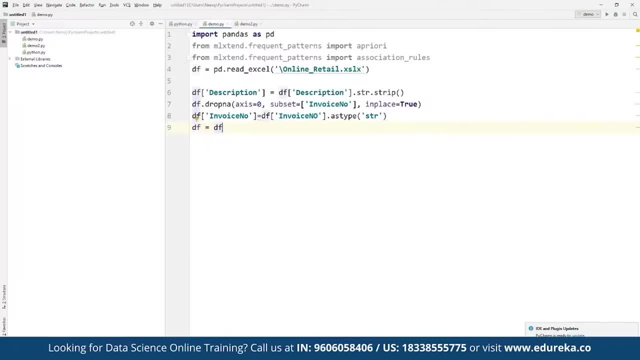 and then we can create a data frame where we can find data frame should be a value closer or get a value closer to data frame where we are going to find the invoice number. So here we have invoice number And then we can find this as a string point based on the 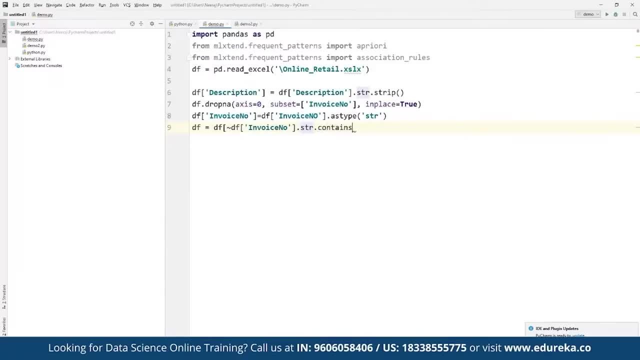 so here we are, string dot contains and then we can define wherever the value is C, wherever the value is C as a part of definition defined here, And then we are going to simply save it as a part of given data frame. So after we are done cleaning up, 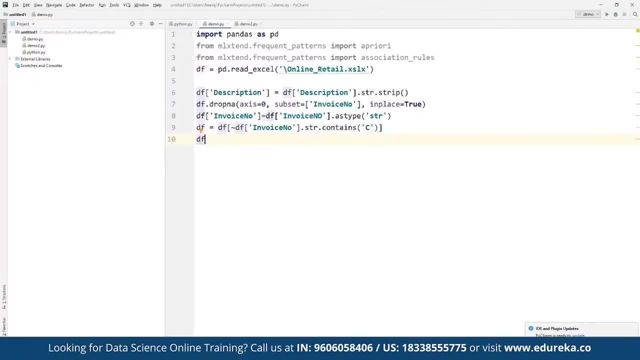 we need to consolidate the items into one transaction per row with each product. So, for the sake of keeping the data small, we are only going to look, you're only going to be looking at a sales for the for any specific country. So now, once we are done, 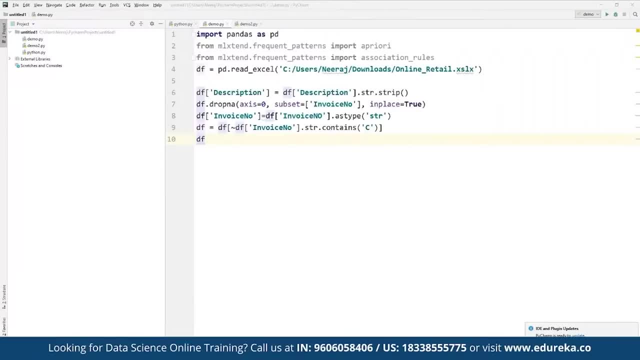 we are going to create and consolidate the items into one transactions per row with each product and, for the sake of keeping the data set small, we are going to look at the sales for a specific country. So for that, let's say here, we want to focus on one country data set here. 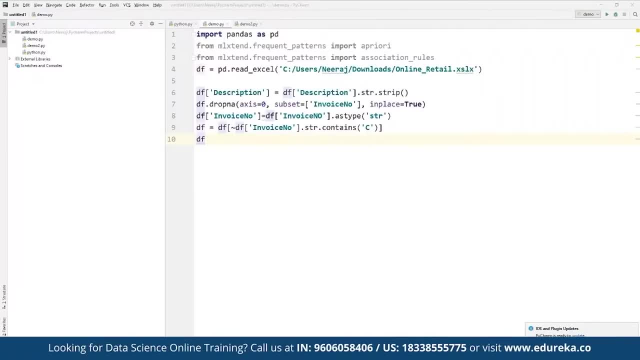 So here we can use basket and then in the basket part, here we can define multiple data Frames. for example, first of all we can define data frame and here we are going to use the same data frame and then we are going to segregate it for the base on the country itself. 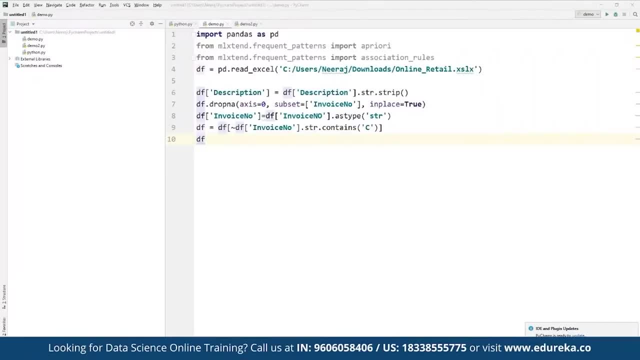 So here we can find country and then under country we can define which country we want to focus on. The country should be supposed, Let's say France, as a single country. So here we can define France as a country that we want to use for consolidation. 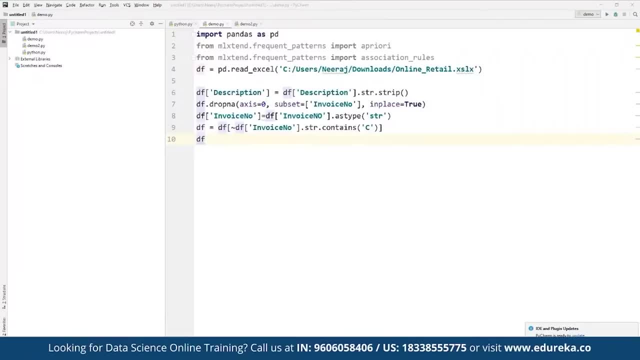 And then we are going to group. So here we can use group by the invoice number. So here we are going to find the invoice number for it. So here we have invoice number, and then we can add a short description here, So we can add: 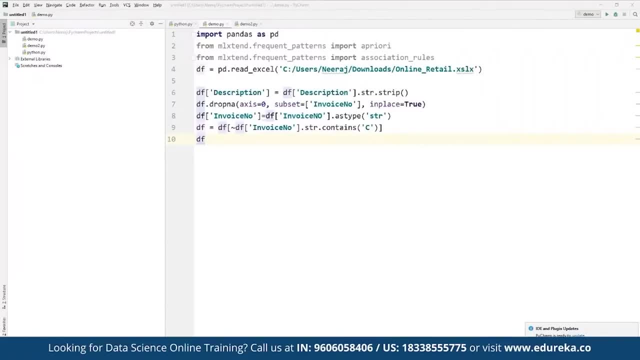 description and then, after we are done defining the description here, we can then define the quantity here. So here we can define quantity. and then, after quantity, we can define some. Let's put this on the line, just to what the confusion? so here we can define some. and 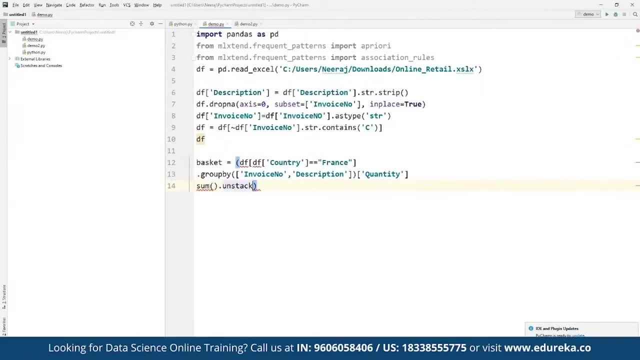 Then we can define unstack, dot reset. You miss one of the time. This is yes. So here we get to help you to define some. and Then we have defined unstack, and then we have define dot reset, dot reset and then the index value here. 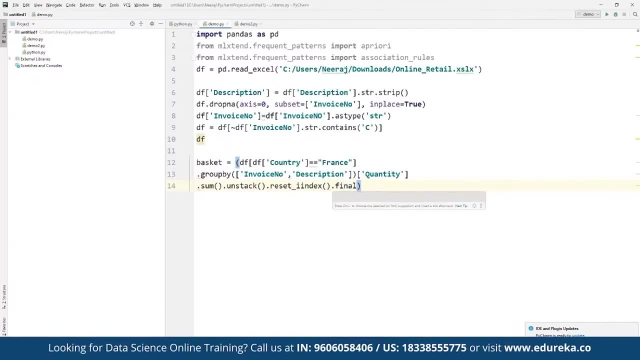 With the final any, with the final Orchid is a simple Fill color over with a simple fill, and then we can find it, the value, to be a simple zero, And then we can use set underscore index Where we can define for the invoice number. So here we have invoice. 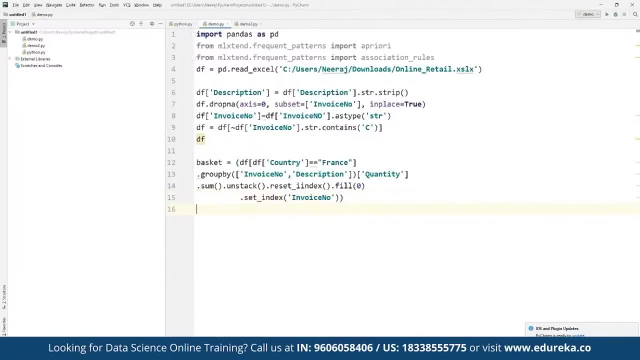 number define, And then we can define this for a basket. So basically, here we are going to define. So, basically, here we are going to define the Consolidation for the items into one transaction for over with each particular product, And the key, the number of provision, do we have? we, as focus our attention only for a for single concrete, so as in France. 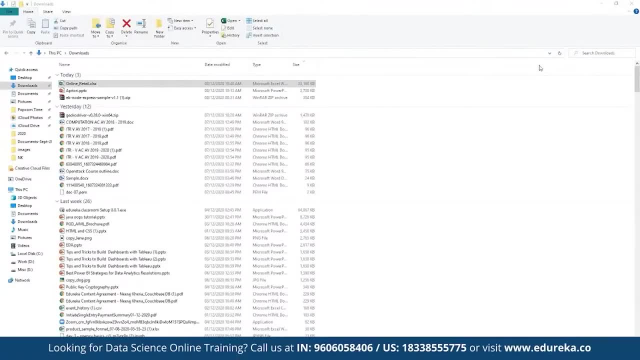 So afterwards, so after we are done with that part, next we have to work on Removing all the zeros. So basically, there are a lot of zeros in the data, But we also need to make sure that any positive values are converted to a 1 and anything less than 0 is also set to. 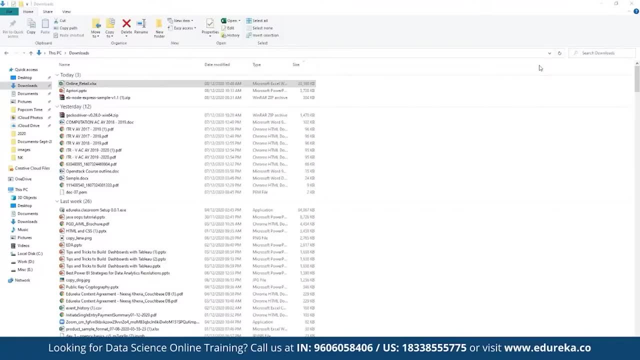 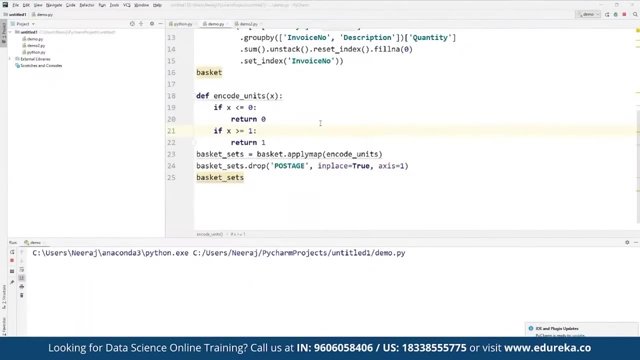 0. so for that we are going to make use of this. so basically, here we are now for converting that. here we are going to make the go ahead and Perform the encoding SSO. here we can define encoding units. So if X is less than or equals to 0, then we are going to turn 0, and if X is greater than or equals to 1, 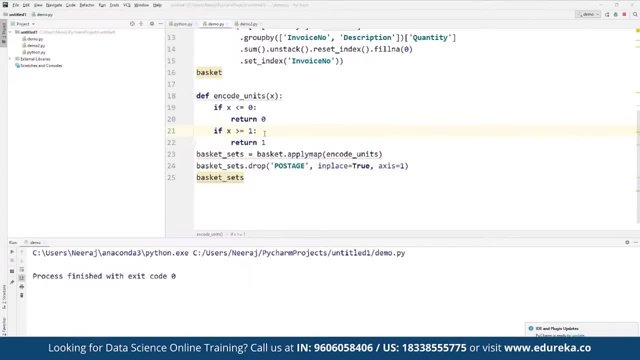 Then it is going to turn 1, Where we are going to define the basket sets and the basket applied map in code units And then we are going to use, simply use the drop Posted and place set up to be true here. So basically, here we are going to simply work on first of all. 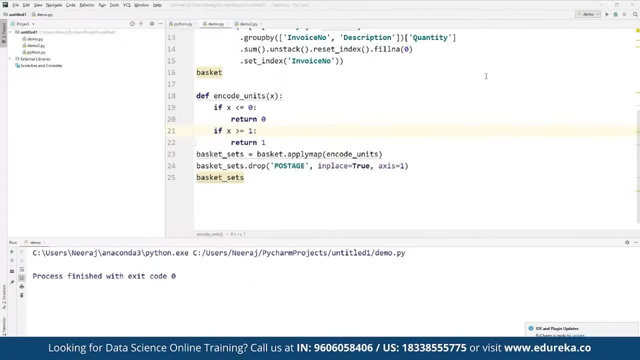 roaming, removing all the anomalies here and Then, if there are a lot of zeros in the data, We also have to make sure that any positive values is converted to 1 and anything less than 0 is also subpoena. that what we had done here and then we are going to generate a frequent item set. 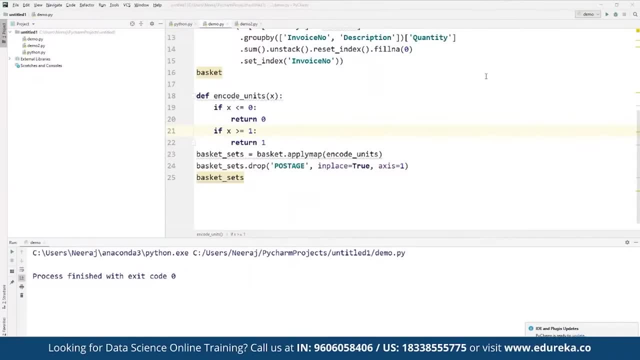 that have support value of at least seven person, and this number is chosen so that we don't, so that we can get close enough and we don't observe any kind of errors. me or we don't get any, it any errors thrown, and here we can generate the frequent 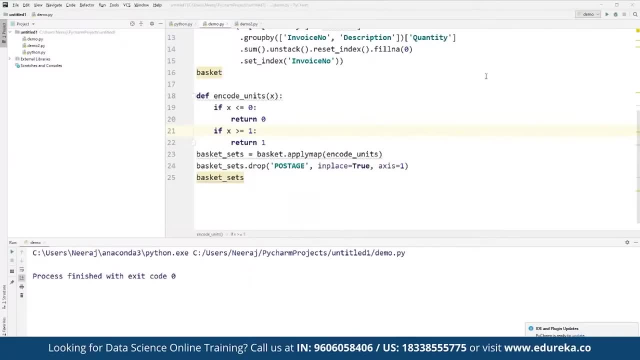 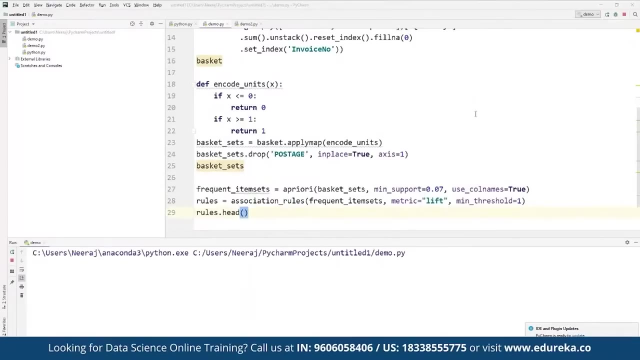 generate the rules with the corresponding support, confidence and lift. So for doing that, we can make use of frequent item set. So here we are going to find frequent- I frequent- item sets where we are going to find the RPOE from basket set. minimum support should be 0.7. 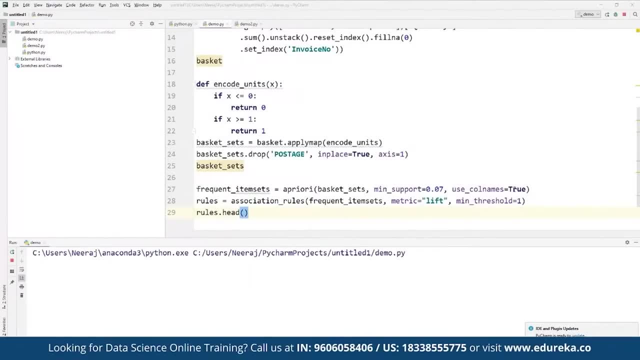 and the call length that are going to be used is should be true, and the rules here define should be for association rules, where we want to find the metric as lift and the minimum threshold to be set to one, And then we are going to filter the data frame. 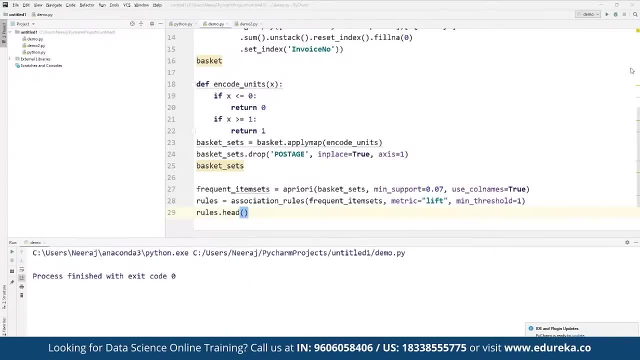 using standard pandas code for a large lift and high contact. So here we can see that the output value is 0.8 and then if we run this and we'll be able to see the output directly in the section altogether. So here we can simply run the rules and then if 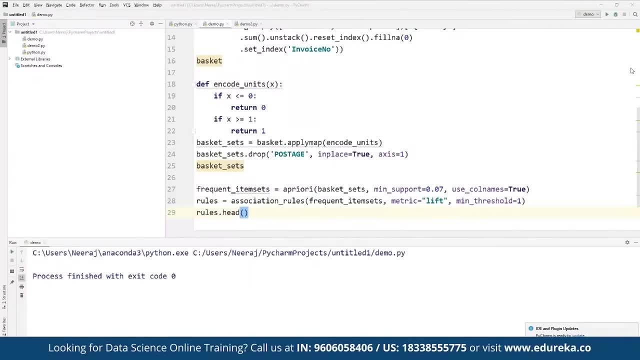 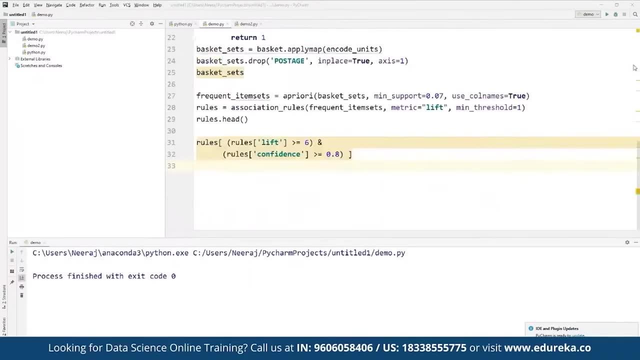 you run rules. here we can define rules for lift- It is going to be defined as a value greater than six- and the rules where confidence value is going to be 0.8 altogether. So that's how we can make use of the RPOE algorithm. 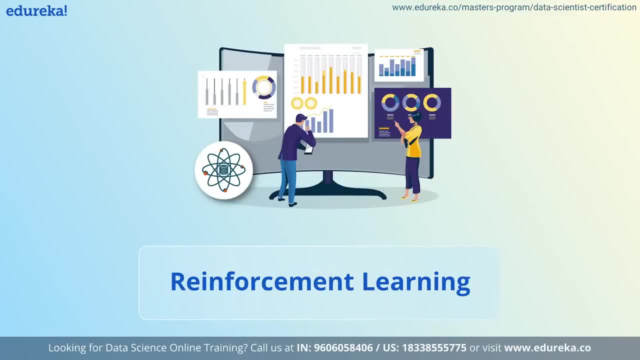 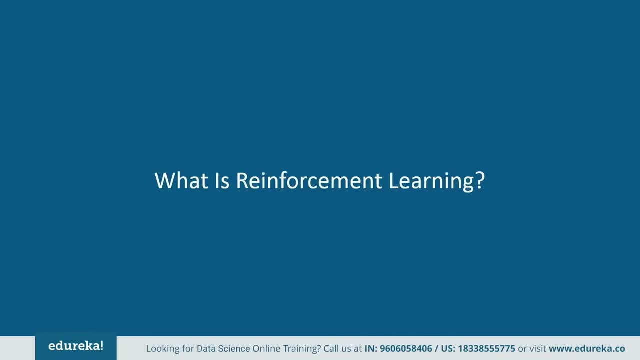 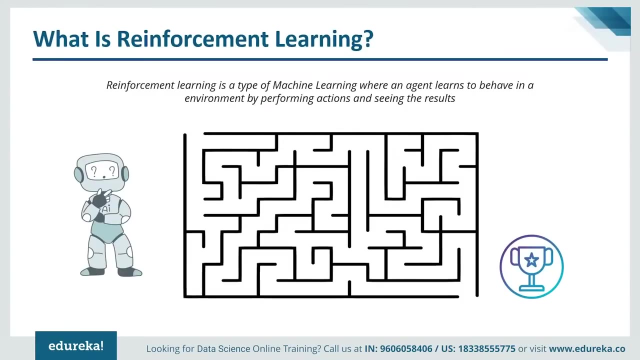 here. So let's look at some other examples and let's define what reinforcement learning really is. So, guys, reinforcement learning is a part of machine learning, where an agent is put in an environment and he learns to behave in this environment by performing certain actions. 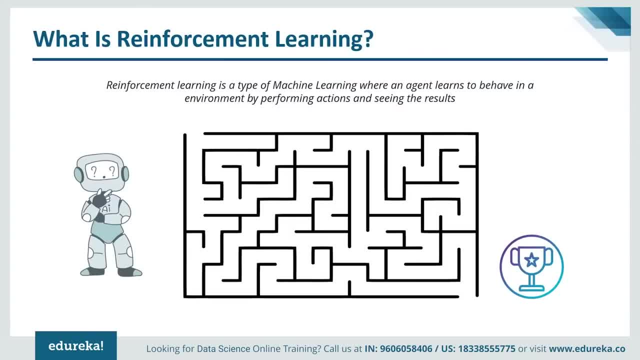 Okay, so it basically performs actions and it either gets the rewards on the actions or it gets a punishment. and observing the reward which it gets from those actions, Reinforcement learning is all about taking an appropriate action in order to maximize the reward in a particular situation. 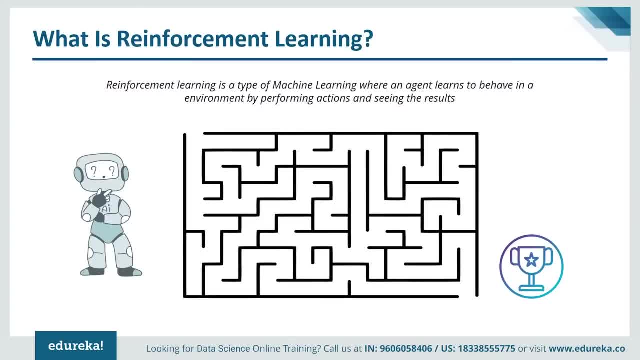 So, guys, in supervised learning, the training data comprises of the input and the expected output, and so the model is trained with the expected output itself. But when it comes to reinforcement learning, there is no expected output. here The reinforcement agent decides what actions to take. 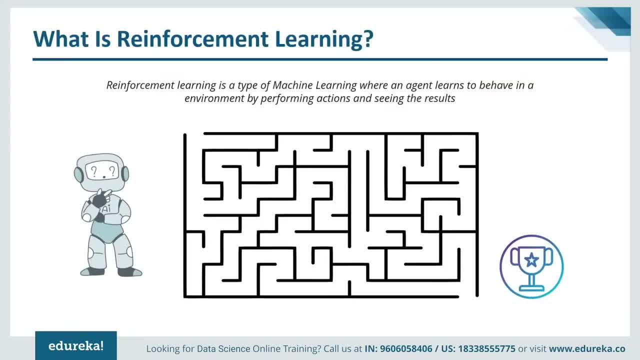 in order to perform a given task. in the absence of a training data set, It is bound to learn from its experience itself. Alright, so reinforcement learning is all about an agent who's put in an unknown environment and he's going to use a hit-and-trial. 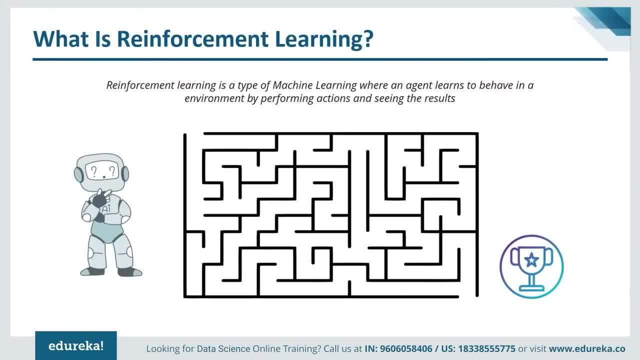 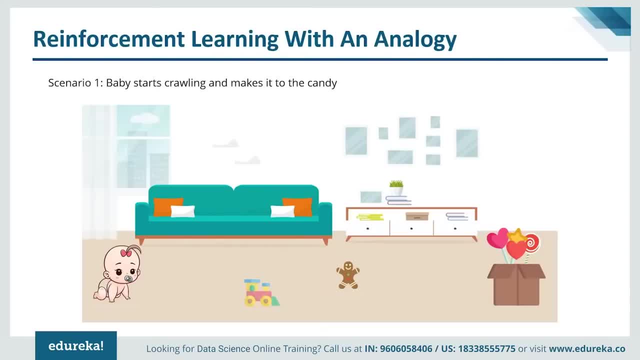 method in order to figure out the environment and then come up with an outcome. Okay, Now let's look at reinforcement learning with an analogy. So consider a scenario wherein a baby is learning how to walk. This scenario can go about in two ways. 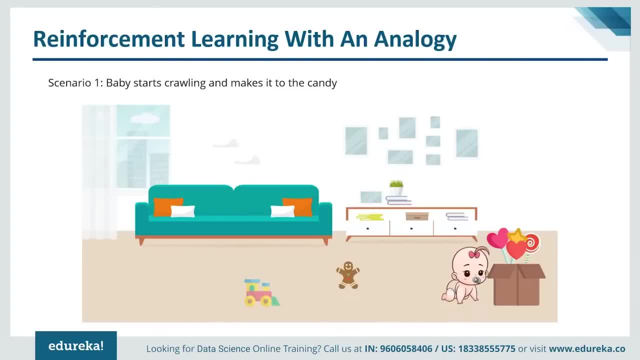 Now, in the first case, the baby starts walking and makes it to the candy. Here, the candy is basically the reward it's going to get. So, since the candy is the end goal, the baby is happy, It's positive. Okay, so the baby is happy and it gets a reward. 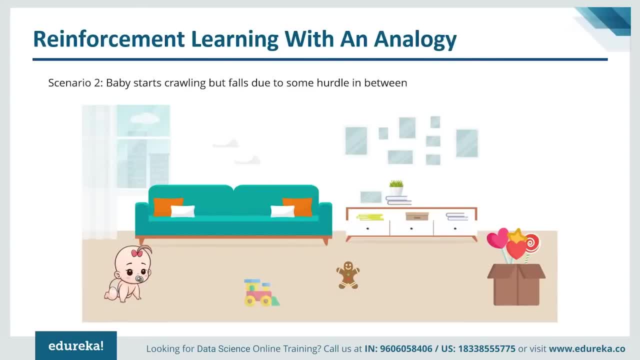 It a set of candies. Now, another way in which this could go is that the baby starts walking but falls due to some hurdle in between. the baby gets hurt and it doesn't get any candy, and obviously the baby is sad. So this is a negative reward. 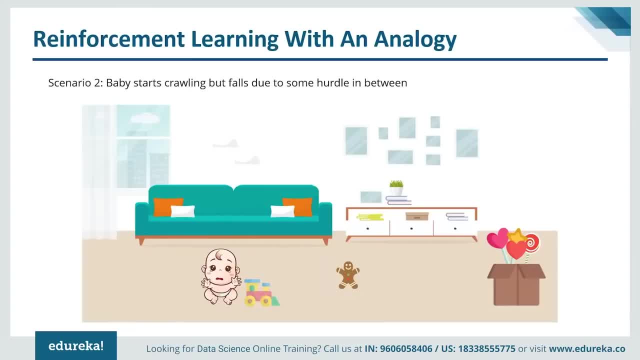 Okay. or you can say this is a setback. So, just like how we humans learn from our mistakes by trial and error, reinforcement learning is also similar, Okay. So we have an agent which is basically the baby and a reward which is the candy over here. 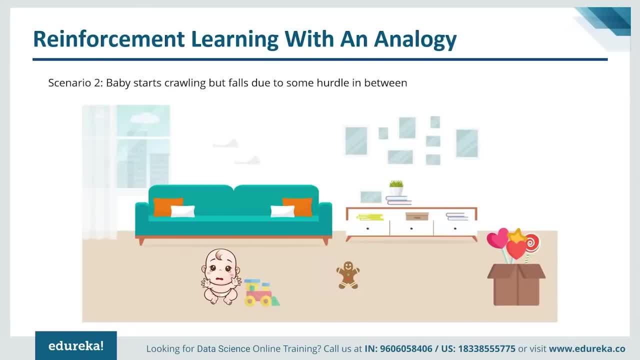 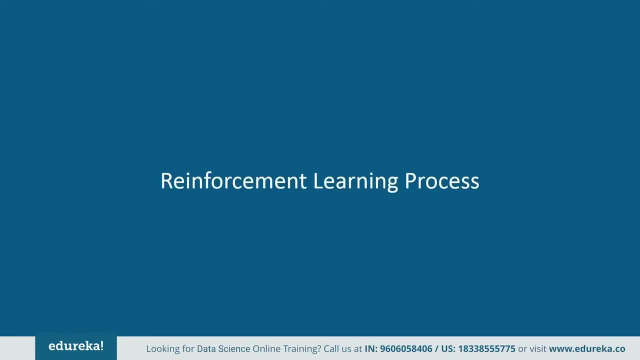 Okay, and with many hurdles in between, The agent is supposed to find the best possible path to reach the reward. So, guys, I hope you all are clear with the reinforcement learning. Now let's look at the reinforcement learning process. So, generally, a reinforcement learning system has two main 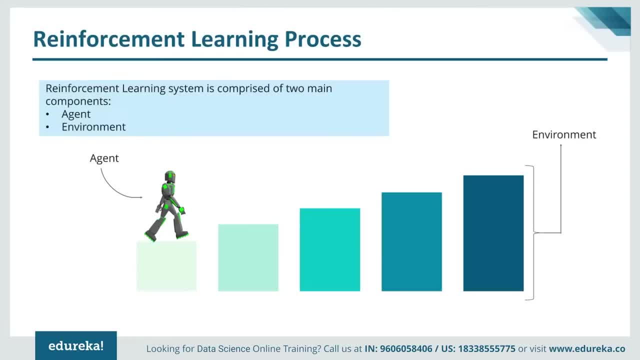 components. All right, The first is an agent and the second one is an environment. Now, in the previous case, we saw that the agent was a baby and the environment was a living room wherein the baby was crawling. Okay, the environment is the setting that the agent is acting. 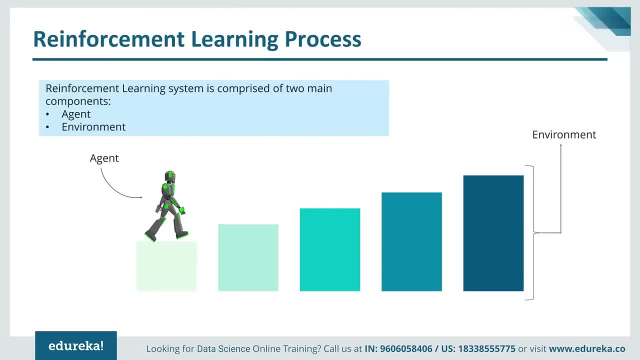 on, and the agent over here Represents the reinforcement learning algorithm. So, guys, the reinforcement learning process starts when the environment sends a state to the agent, and then the agent will take some actions based on the observations. in turn, The environment will send the next state and the respective 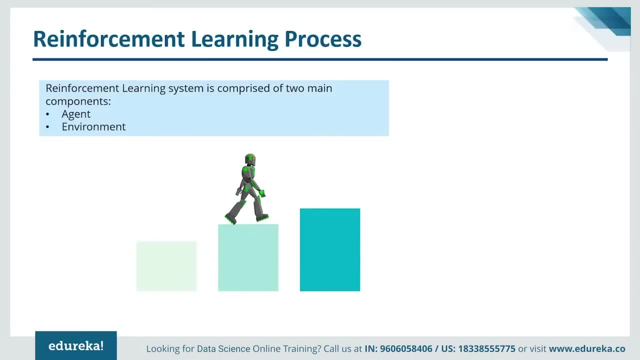 reward back to the agent. The agent will update its knowledge with the reward returned by the environment, and it uses that to evaluate its previous action. So, guys, this loop keeps continuing until the environment sends a terminal state, Which means that the agent has accomplished all his tasks. 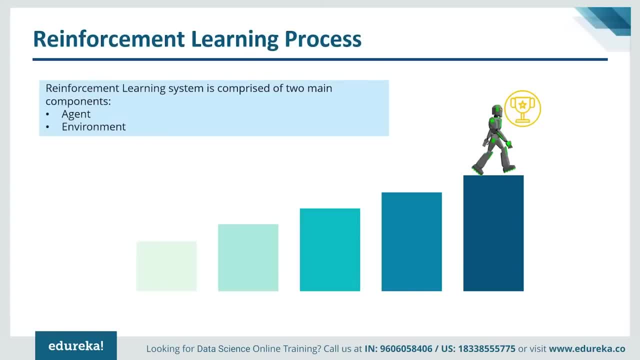 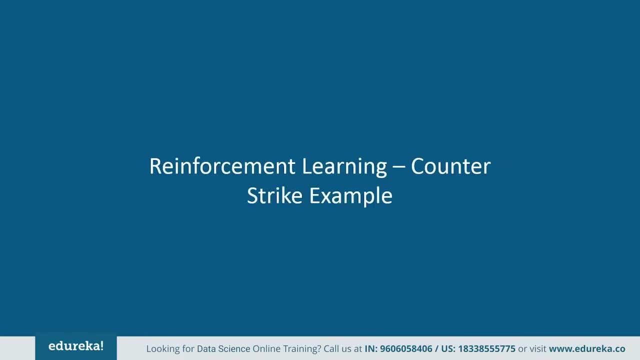 and he finally gets the reward. Okay, This is exactly what was depicted in this scenario, So the agent keeps climbing up ladders until he reaches his reward. to understand this better, Let's suppose that our agent is learning to play counter-strike. 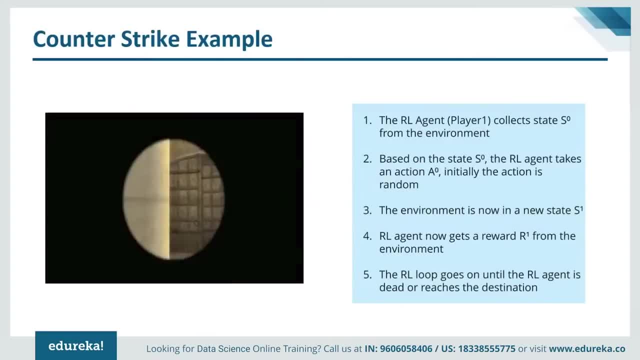 Okay, So let's break it down now. Initially, the RL agent, which is basically the player, player one, Let's say it's the player one who is trying to learn how to play the game. Okay, he collects some state from the environment. 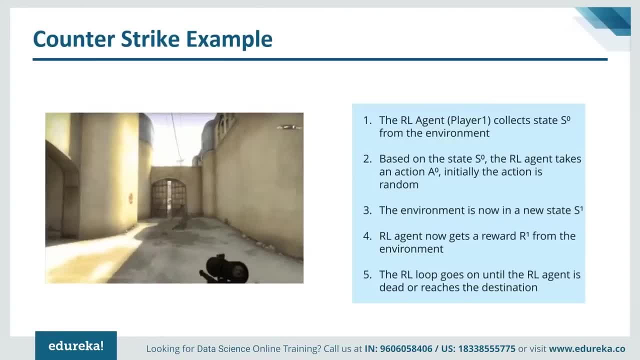 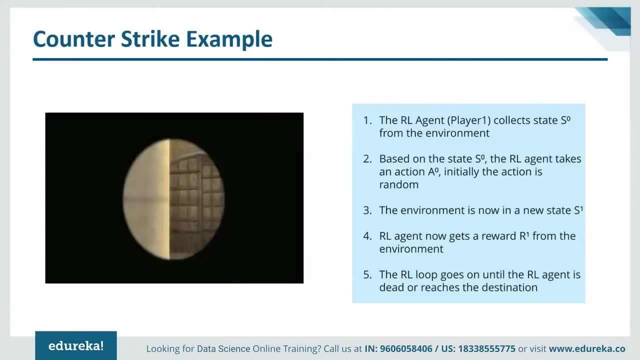 Okay, This could be the first state of counter-strike. Now, based on this state, the agent will take some action. Okay, and this action can be anything that causes a result. So if the player moves left or right, it's also considered as. 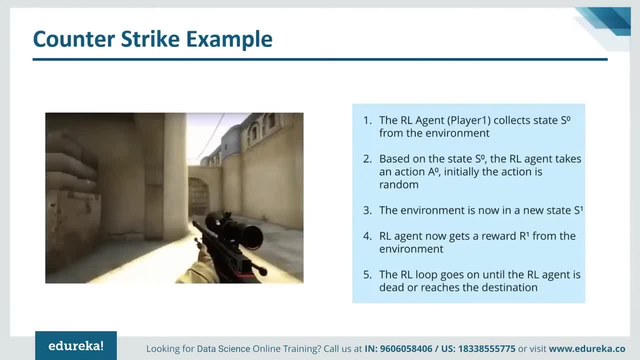 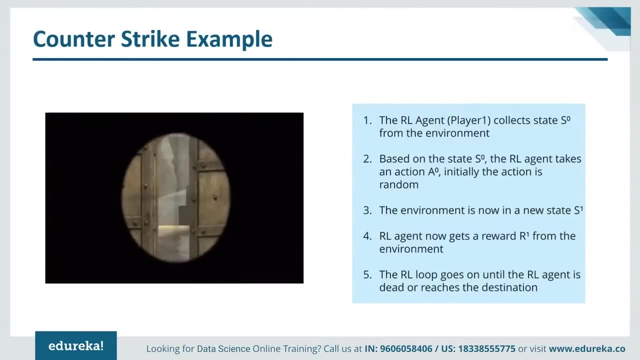 an action. Okay, So initially the action is going to be random because obviously the first time you pick up counter-strike you're not going to be a master at it, So you're going to try with different actions and you're just going to pick up a random action in the beginning. 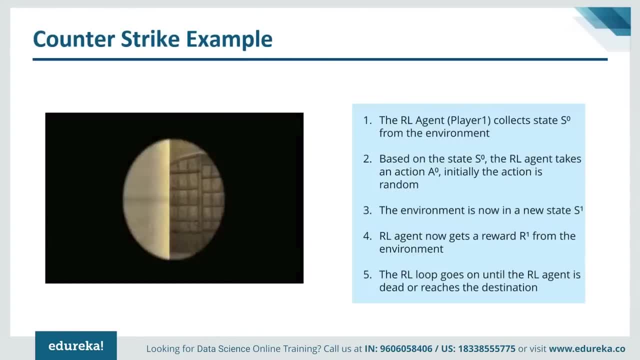 Now the environment is going to give a new state. So after clearing that, the environment is now going to give a new state to the agent Or to the player. So maybe he's cross stage one now he's in stage two. So now the player will get a reward- R1- from the environment. 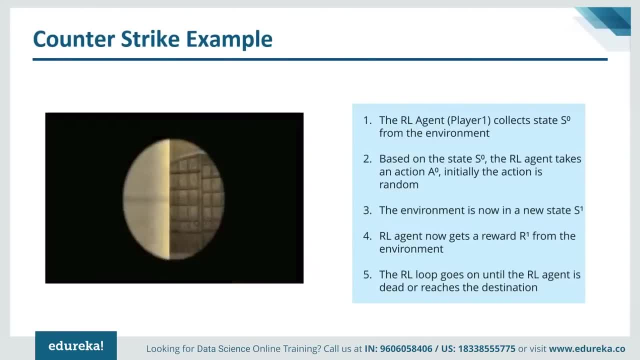 because it cleared stage one. So this reward can be anything. it can be additional points or coins or anything like that, Okay. So basically, this loop keeps going on until the player is dead or reaches the destination- Okay, and it continuously outputs a sequence of states actions. 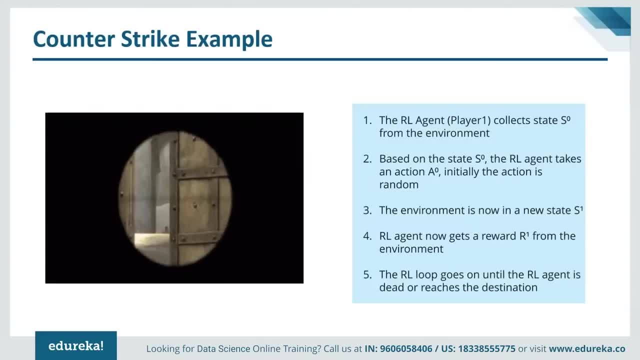 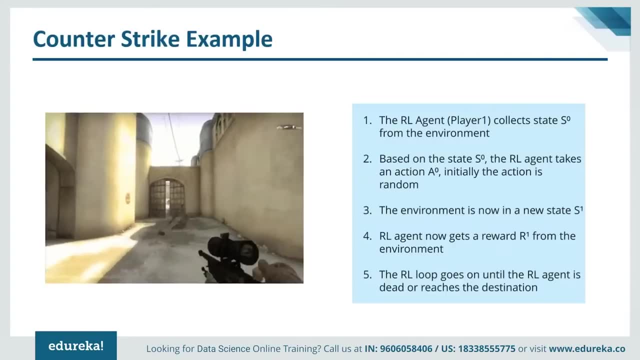 and rewards. So, guys, this was a small example to show you how reinforcement learning process works. So you start with an initial state and once the player clears that state, he gets a reward. after that, the environment will give another stage to the player and after it clears that state, 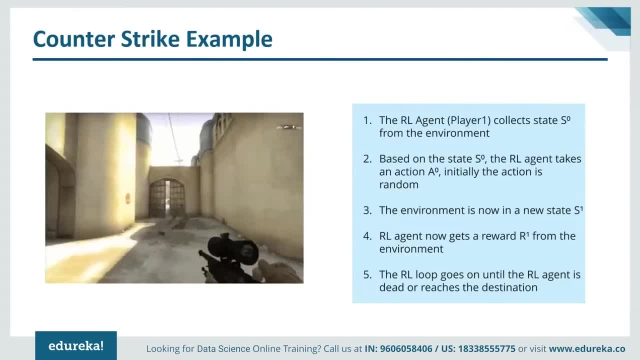 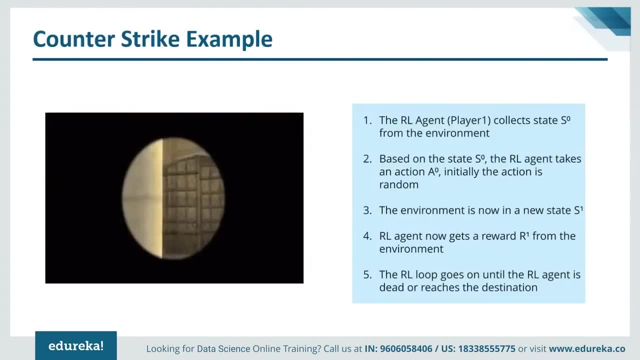 it's going to get another reward, and it's going to keep happening until the player reaches his destination. All right, So, guys, I hope this is clear. now Let's move on and look at the reinforcement learning definitions. So there are a few concepts that you should be aware of while 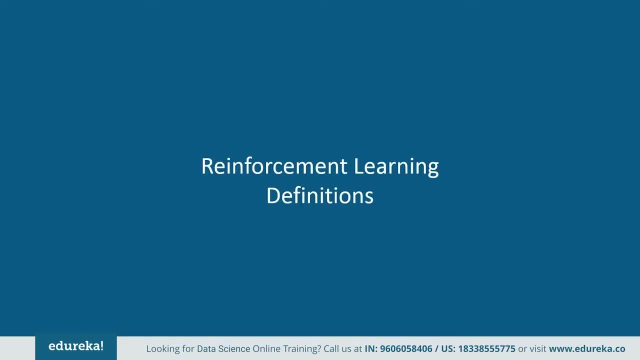 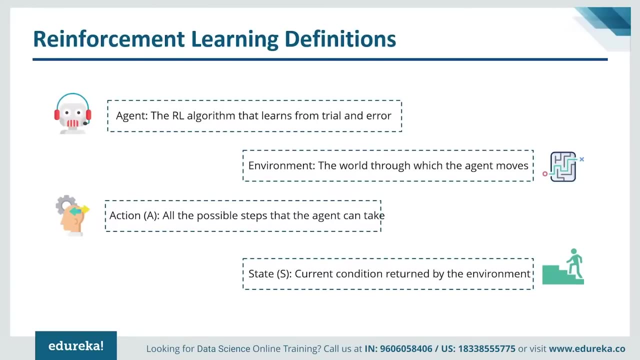 studying reinforcement learning. Let's look at those definitions over here. So first we have the agent. Now an agent is basically the reinforcement learning algorithm that learns from trial and error. Okay, so an agent takes actions like, for example, a soldier in counter-strike navigating through the game. 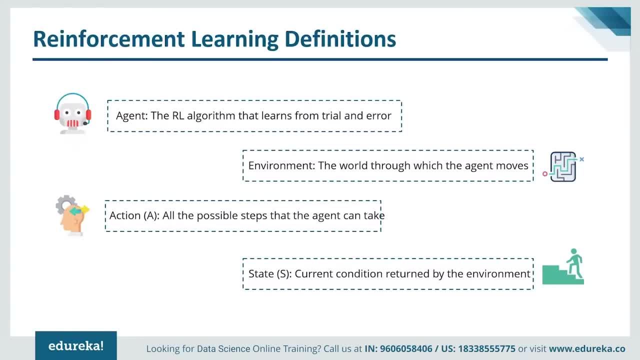 That's also an action. Okay, if he moves left, right or if he shoots at somebody, that's also an action. Okay. so the agent is responsible for taking actions in the environment. Now, the environment is the whole counter-strike game. Okay, it's basically the world through which the agent moves. 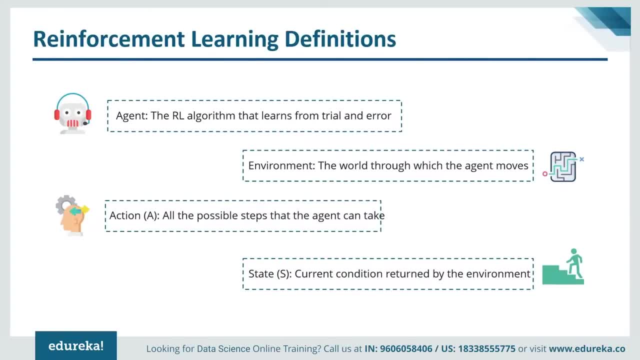 the environment, takes the agents current state and action as input and it returns the agents reward and its next state as output. All right, Next we have action. now all the possible steps that an agent can take are called actions. So, like I said, it can be moving right, left or shooting, or any. 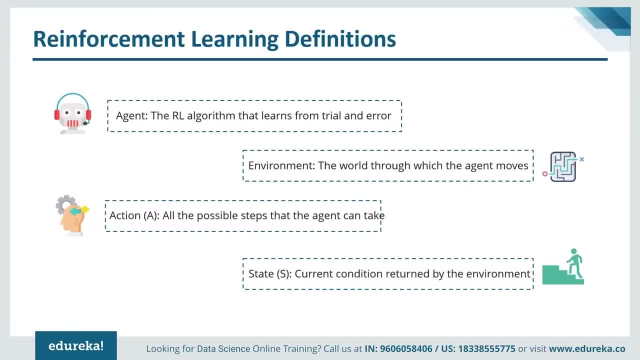 of that. All right. then we have state. now, state is basically the current condition returned by the environment. So, whichever state you are in, if you are in state one or if you're in state to, that represents your current condition, All right. Next, we have reward. 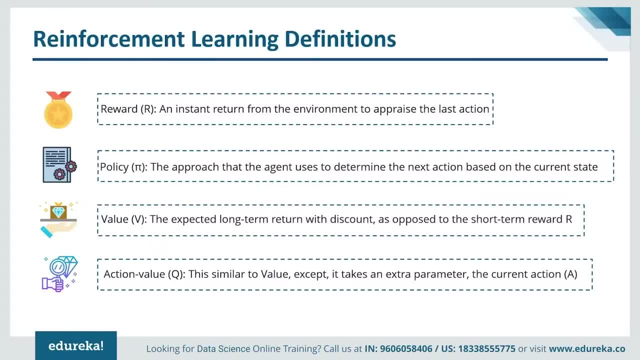 A reward is basically an instant return from the environment to appraise your last action. Okay, so it can be anything like coins or it can be additional points. So basically, a reward is given to an agent after it clears the specific stages. next we have policy. policy is basically the 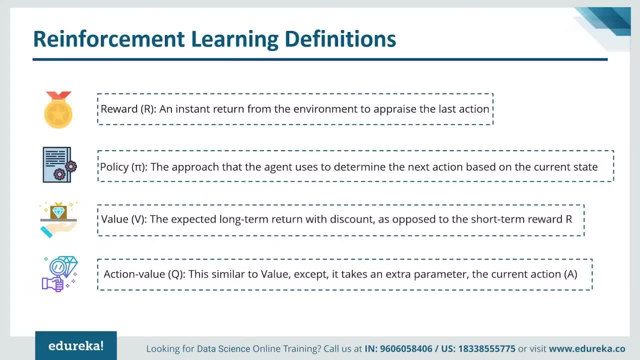 strategy that the agent uses to find out his next action based on his current state policy is just the strategy with which you approach the game. then we have value. now value is the expected long-term return with discount. So value and action value can be a little bit confusing for you. 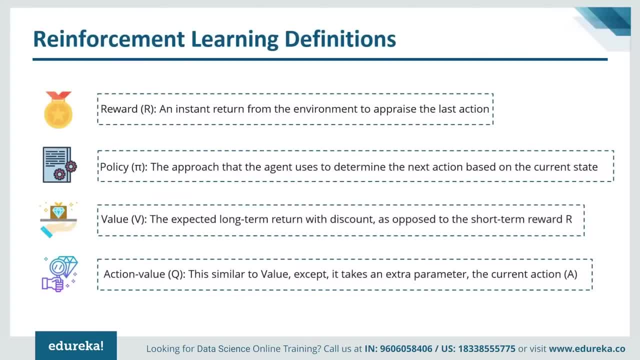 right now, But as we move further you'll understand what I'm talking about. Okay, So value is basically the long-term return that you get with discount. Okay, discount I'll explain in the further slides. then we have action value now. action value is also known as Q value. 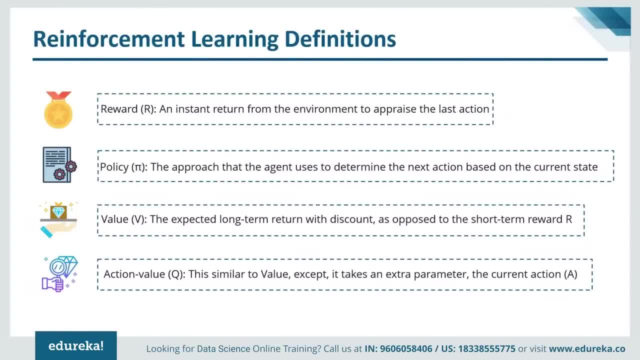 Okay, It's very similar to value, except that it takes an extra parameter, which is the current action. So basically, here you'll find out the Q value, depending on the particular action that you took. All right, So guys, don't get confused with value and action value. 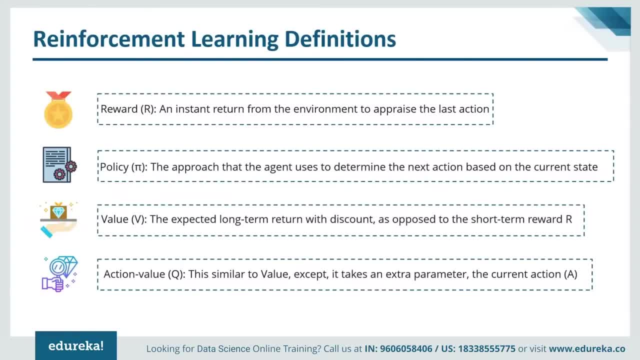 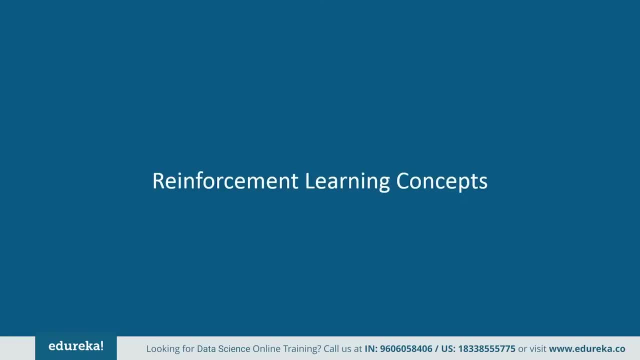 We look at examples in the further slides and you'll understand this better. Okay, So, guys, make sure that you're familiar with these terms, because you'll be seeing a lot of these terms in the further slides. All right now, before we move any further. 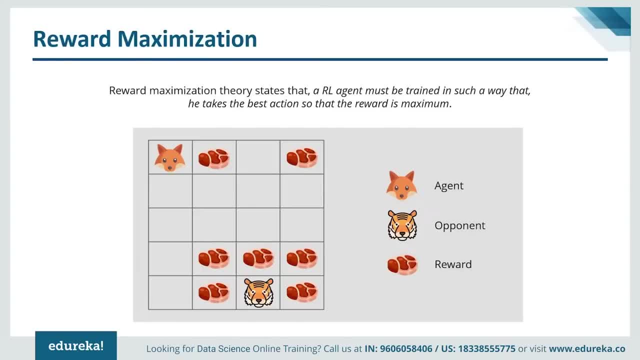 I'd like to discuss a few more concepts. Okay, So first we'll discuss the reward maximization. So, if you haven't already realized it, the basic aim of the RL agent is to maximize the reward. Now, How does that happen? Let's try to understand this in depth. 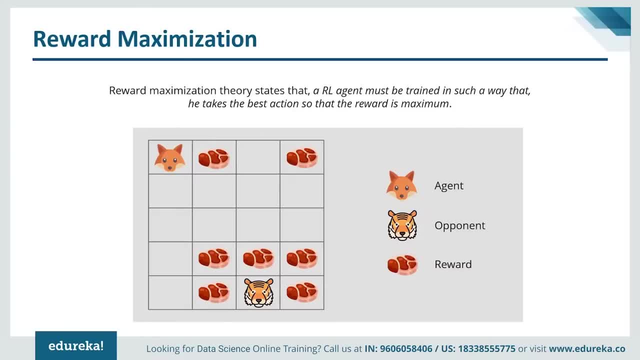 So the agent must be trained in such a way that he takes the best action so that the reward is maximum, because the end goal of reinforcement learning is to maximize your reward based on a set of actions. So let me explain this with a small game. 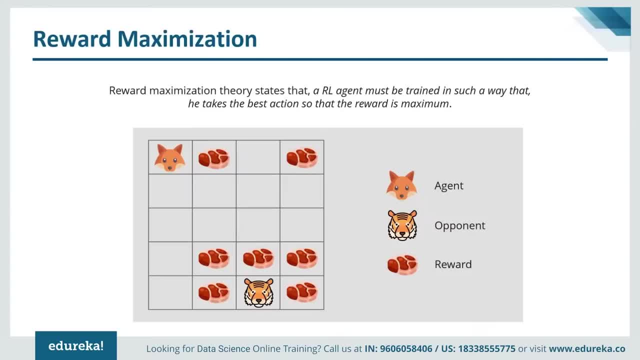 Now in the figure you can see there is a fox, There's some meat and there's a tiger. So our agent is basically the Fox, and his end goal is to eat the maximum amount of meat before being eaten by the tiger. Now, since the Fox is a clever fellow, 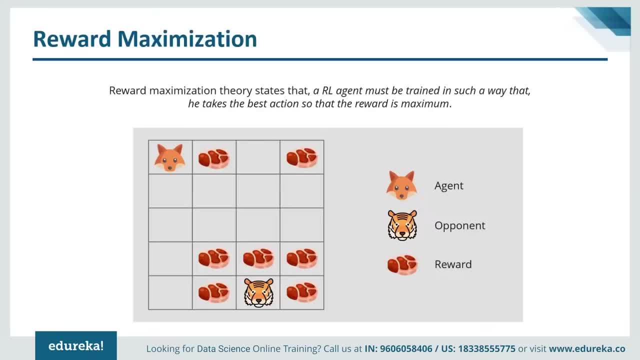 He eats the meat that is closer to him, rather than the meat which is closer to the tiger. Now, this is because the closer he is to the tiger, the higher are his chances of getting killed. So, because of this, the rewards which are near the tiger, even if 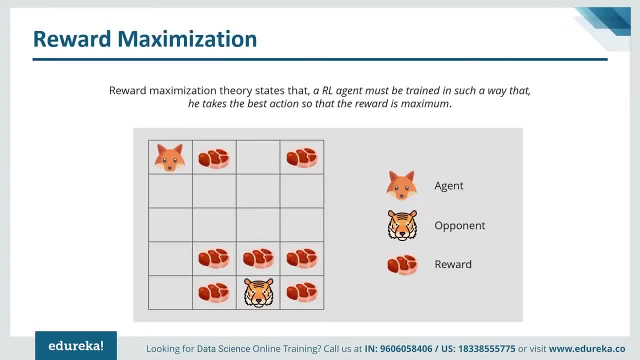 they are bigger meat chunks, they will be discounted. So this is exactly what discounting means. So our agent is not going to eat the meat chunks which are closer to the tiger because of the risk All right now, even though the meat chunks might be larger. 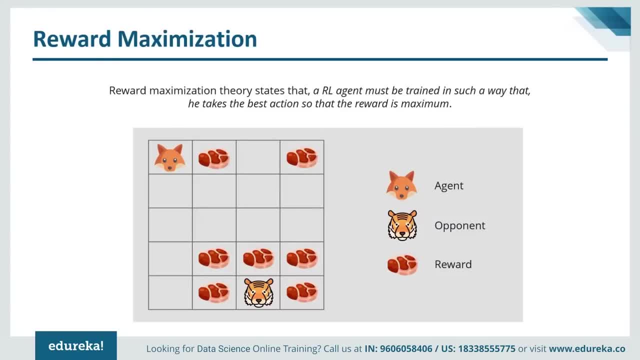 He does not want to take the chances of getting killed. Okay, This is called discounting. Okay, This is where you discount, because you improvise and you just eat the meat which are closer to you, instead of taking risks and eating the meat which are closer to your opponent. 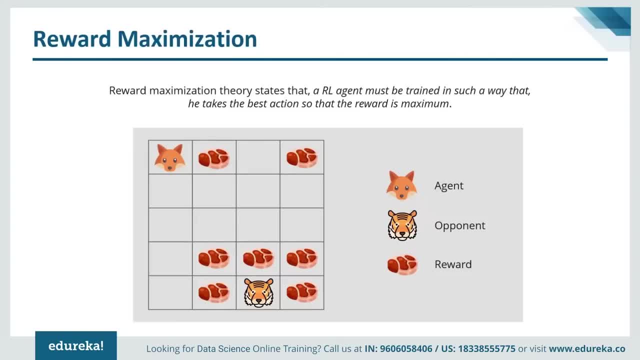 All right. Now the discounting of reward works based on a value called gamma. will be discussing gamma in our further slides, But, in short, the value of gamma is between 0 and 1.. Okay, So the smaller the gamma, the larger is the discount value. 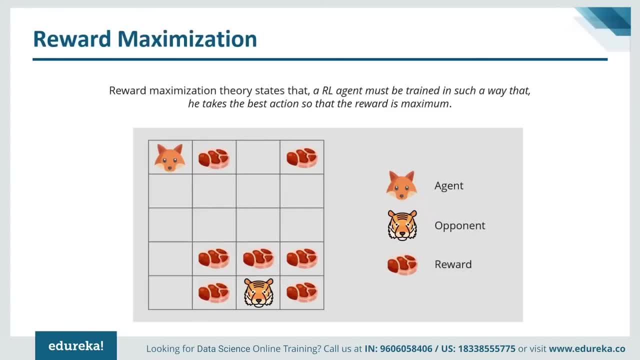 Okay. So if the gamma value is lesser, it means that the agent Is not going to explore and he's not going to try and eat the meat chunks which are closer to the tiger. Okay, but if the gamma value is closer to 1, it means that our 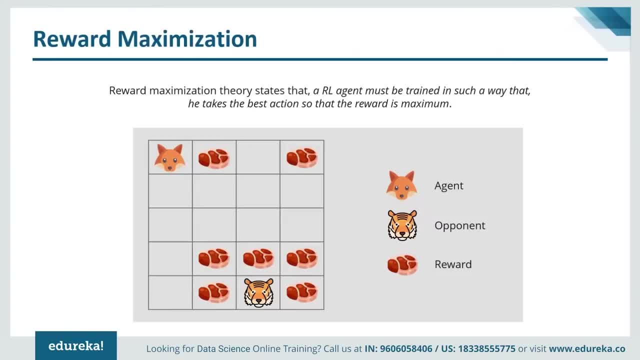 agent is actually going to explore and it's going to try and eat the meat chunks which are closer to the tiger. All right Now. I'll be explaining this in depth in the further slides, So don't worry if you haven't got a clear concept yet. but 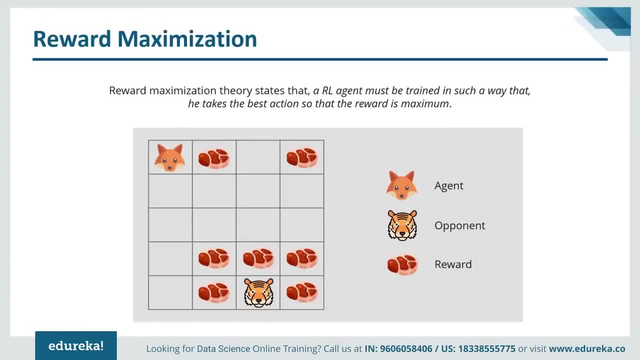 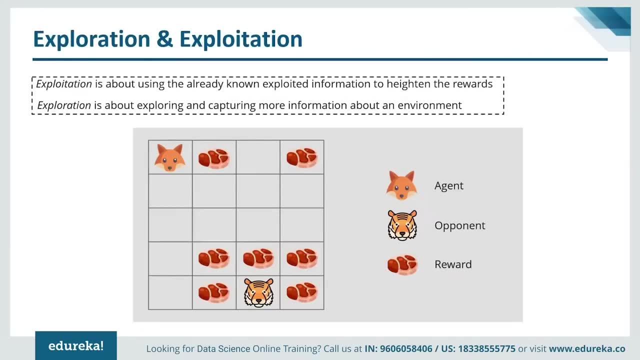 just understand that reward maximization is a very important step when it comes to reinforcement learning, because the agent has to collect maximum rewards by the end of the game. All right, Now let's look at another concept, which is called exploration and exploitation. So exploration, like the name suggests, is about exploring, and 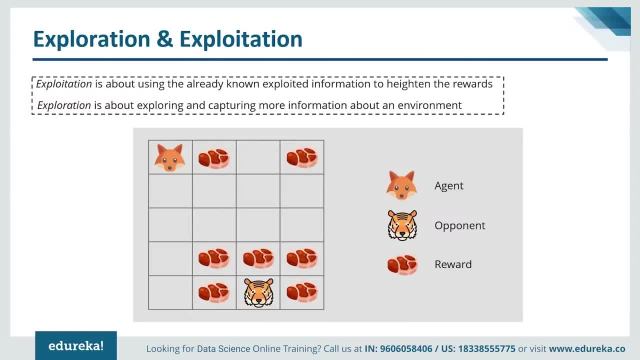 capturing more information about an environment. On the other hand, exploitation is about using the already known, exploited information to heighten the rewards. So, guys, consider the fox and tiger example that we discussed now here. the Fox eats only the meat chunks which are close to him, but he does not eat the meat chunks which are closer to. 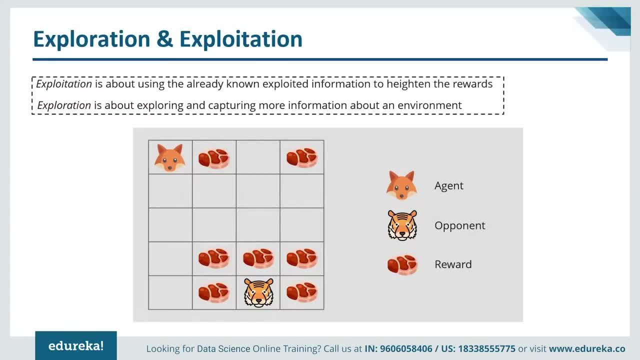 the tiger. Okay, even though they might give him More rewards, He does not eat them. If the Fox only focuses on the closest rewards, he will never reach the big chunks of meat. Okay, This is what exploitation is about. You're just going to use the currently known information and 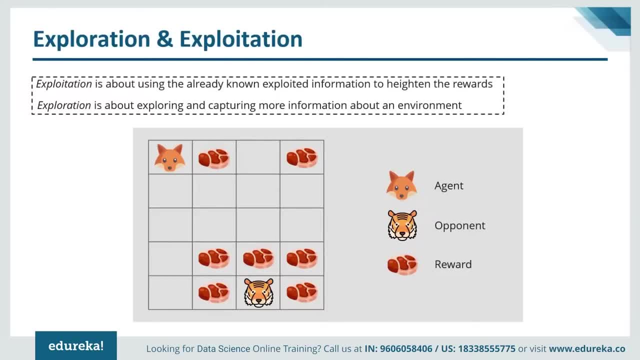 you're going to try and get rewards based on that information, But if the Fox decides to explore a bit, it can find the bigger reward, which is the big chunks of meat. This is exactly what exploration is, So the agent is not going to stick to one corner instead. 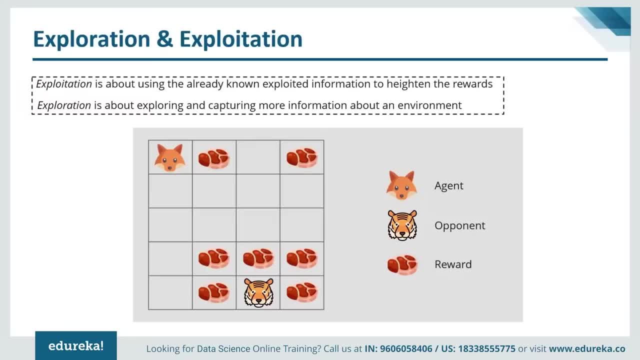 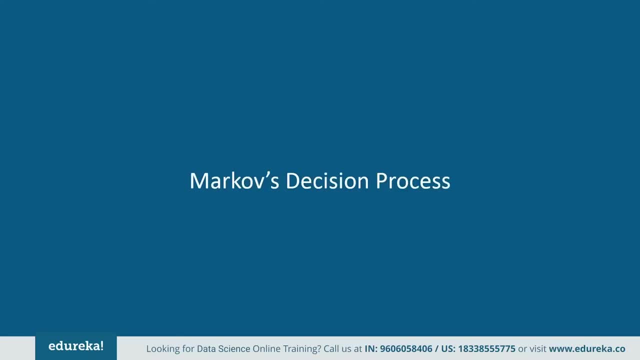 He's going to explore the entire environment And try and collect bigger rewards. All right, So, guys, I hope you all are clear with exploration and exploitation. Now let's look at the markers decision process. So, guys, this is basically a mathematical approach for mapping. 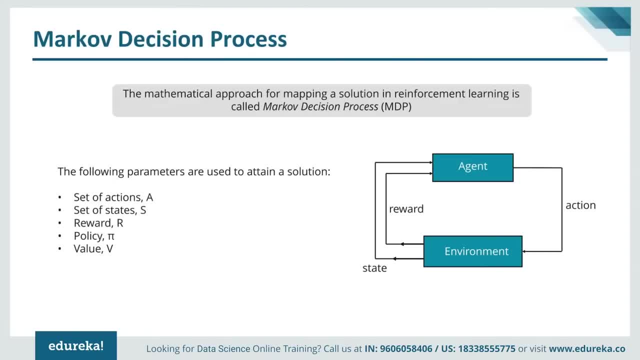 a solution in reinforcement learning. in a way, The purpose of reinforcement learning is to solve a mark of decision process. Okay, So there are a few parameters that are used to get to the solution. So the parameters include the set of actions, the set of states. 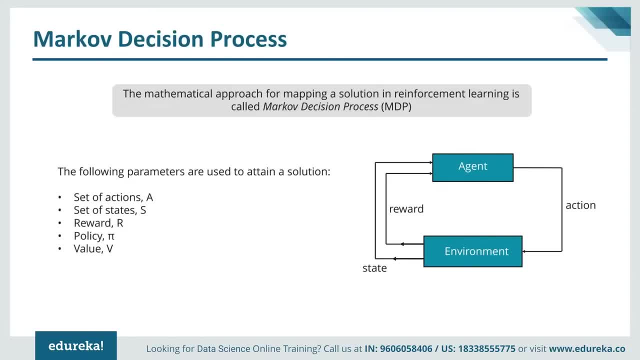 the rewards, The policy that you're taking to approach the problem and the value that you get. Okay, So, to sum it up, the agent must take an action A to transition from a start state to the end state S. While doing so, the agent will receive a reward R for each. 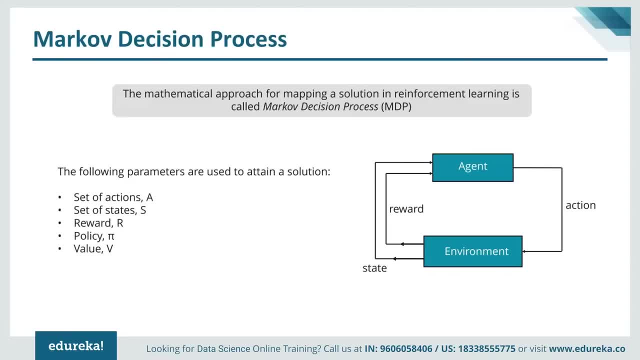 action that he takes. So, guys, a series of actions taken by the agent define the policy, or it defines the approach, and the rewards that are collected define the value. So the main goal here is to maximize the rewards by choosing the optimum policy. All right, 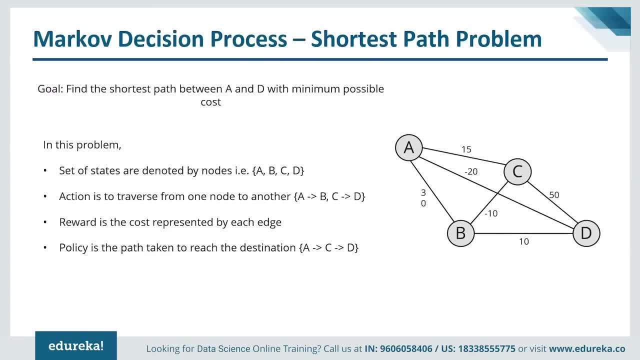 Now let's try to understand this with the help of the shortest path problem. I'm sure a lot of you might have gone through this problem when you were in college. So, guys, look at the graph over here. So our aim here is to find the shortest path between A and D. 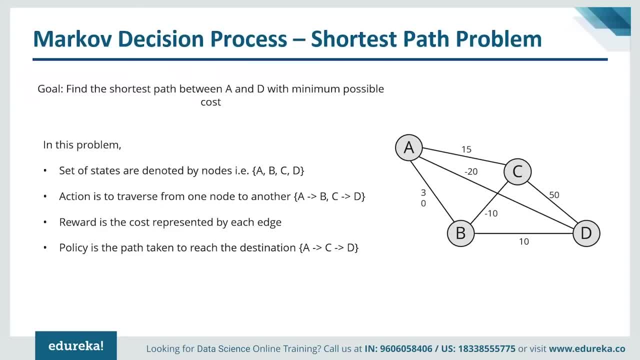 with minimum possible cost. So the value that you see on each of these edges basically denotes the cost. So if I want to go from A to C, it's going to cost me 15 points. Okay, So let's look at how this is done. 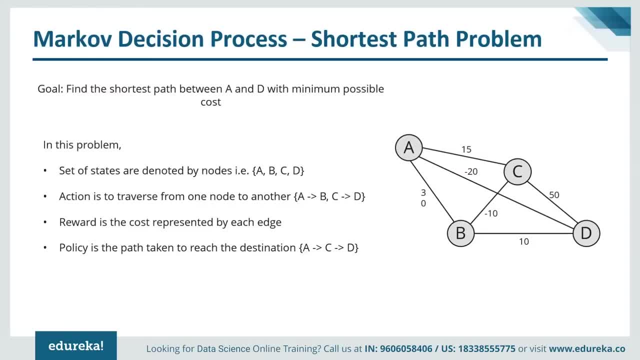 Now, before we move and look at the problem, in this problem, the set of states are denoted by the nodes, which is ABCD, and the action is to traverse from one node to the other. So if I'm going from A to B, that's an action. similarly, A to 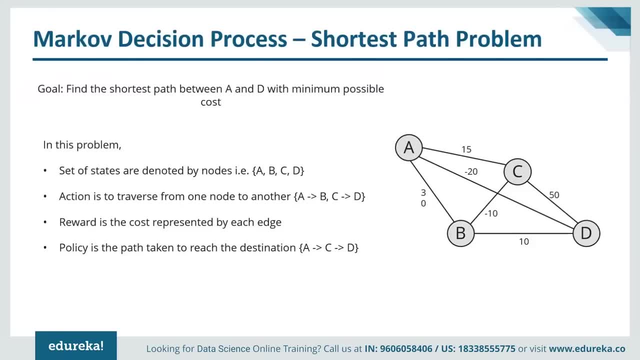 C. That's an action, Okay. the reward is basically the cost, which is represented by each edge over here. All right, Now the policy is basically the path that I choose to reach the destination. So let's say I choose a CD. 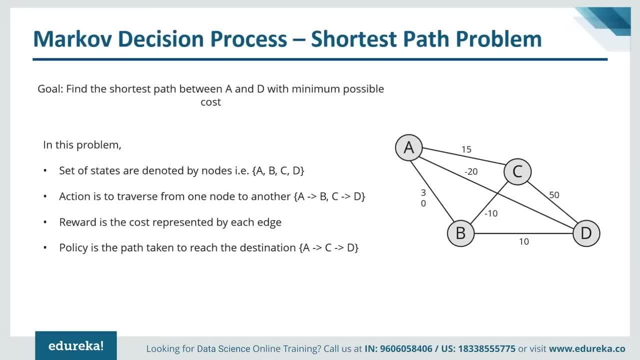 Okay, that's one policy. in order to get to D, I'm choosing A CD, which is a policy. Okay, It's basically how I'm approaching the problem. So, guys, here you can start off at node A and you can take baby. 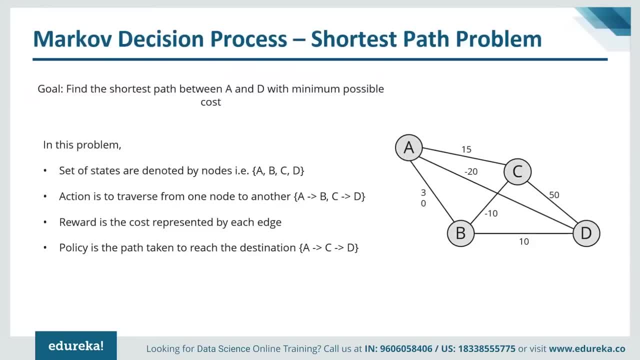 steps to your destination Now. initially you're clueless, So you can just take the next possible node which is visible to you. So, guys, feel smart enough. You're going to choose A to C instead of ABCD or ABD. All right. 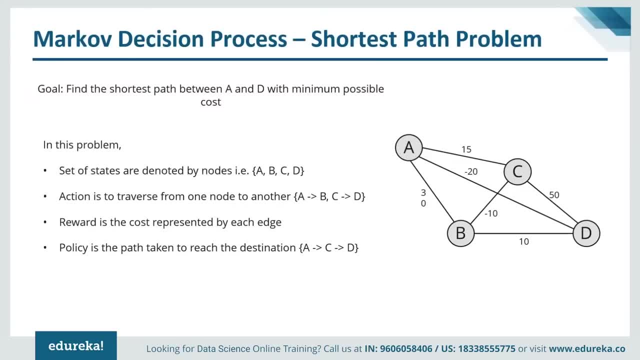 So now, if you're at node C, you want to traverse to node D. You must again choose a wise path. All right, you just have to calculate which path has the highest cost or which path will give you the maximum rewards. So, guys, this is a simple problem which is trying to calculate. 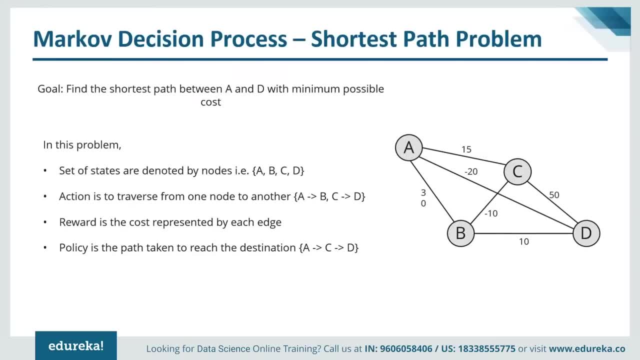 the shortest path between A and D by traversing through these nodes. So if I traverse from ACD, it gives me the maximum reward. Okay, It gives me 65, which is more than any other policy would give me. Okay. So if I go from ABD, it would be 40. when you compare this to: 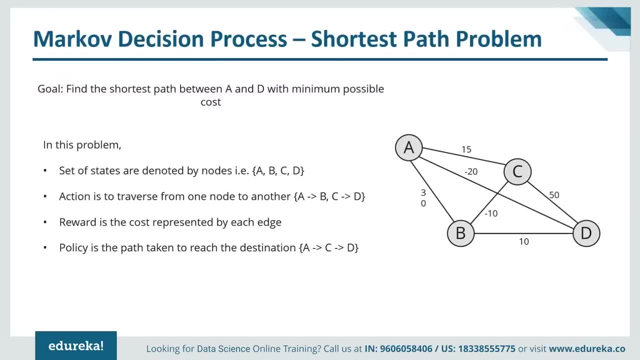 ACD. it gives me more rewards, So obviously I'm going to go with ACD. Okay, So, guys, was a simple In order to understand how Markov decision process works. All right, So, guys, I want to ask you a question. 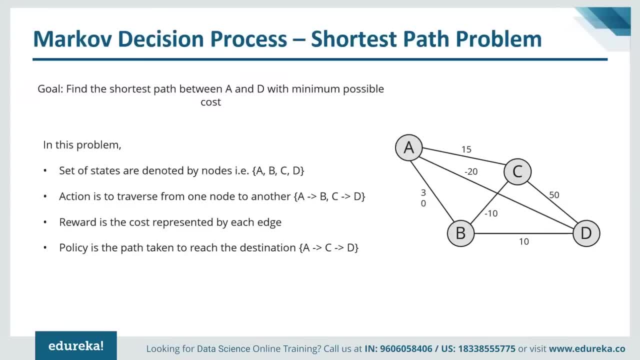 What do you think I did here? Did I perform exploration or did I perform exploitation? Now, the policy for the above example is of exploitation, because we didn't explore the other nodes. Okay, We just selected three nodes and we traverse through them. So that's why this is called exploitation. 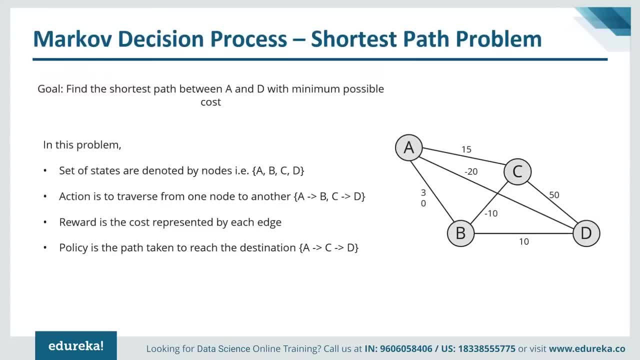 We must always explore the different nodes so that we can find a more optimal policy. But in this case, obviously ACD has the highest reward and we're going with a CD. but generally it's not so simple. There are a lot of nodes. 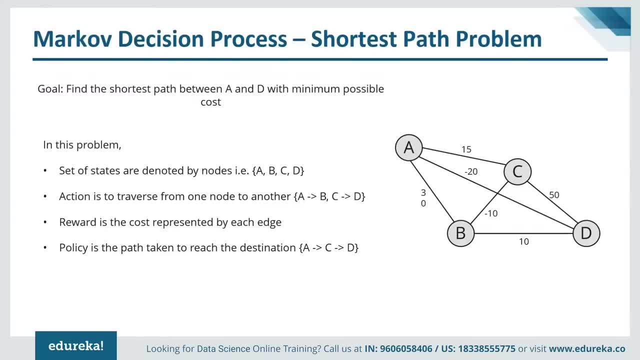 There are hundreds of nodes to Traverse and they're like 50: 60 policies. Okay, 50, 60 different policies. So you make sure you explore through all the policies and then decide on an optimum policy which will give you a maximum reward. 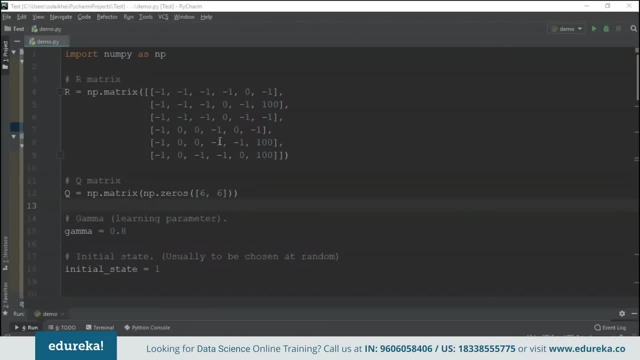 So, guys, this is our code and this is executed in python, and I'm assuming that all of you have a good background in python. Okay, if you don't understand python very well, I'm going to leave a link in the description. You can check out that video on python and then maybe come. 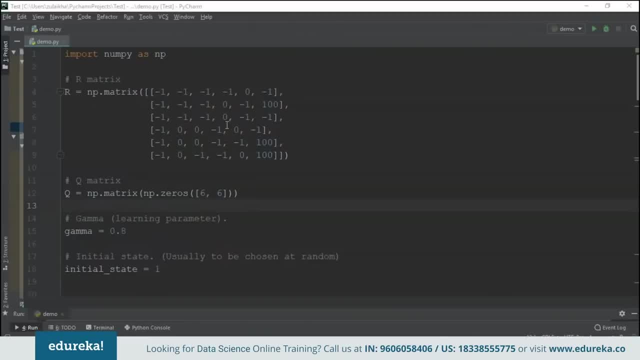 back to this later, Okay, but I'll be explaining the code to you anyway. but I'm not going to spend a lot of time explaining each and every line of code, because I'm assuming that you know python, Okay? So let's look at the first line of code over here. 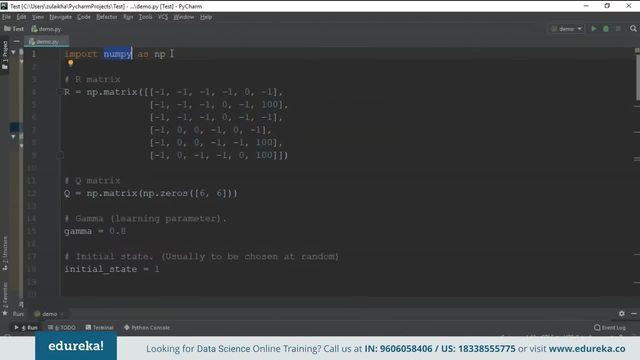 So what we're going to do is we're going to import numpy. Okay, numpy is basically a python library for adding support for large multi-dimensional arrays and matrices, and it's basically for computing mathematical functions. Okay, So first we're going to import that. after that we're going to 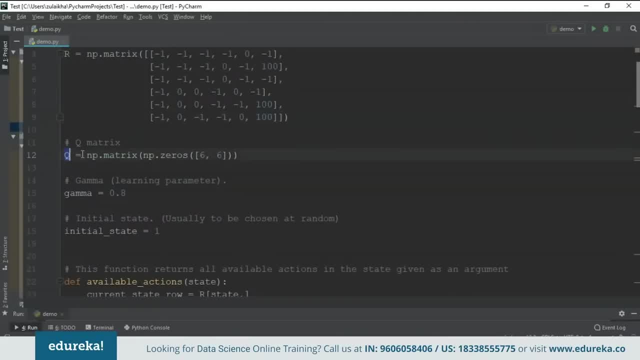 create the R matrix. Okay, So this is the R matrix. next, We're going to create a Q matrix, and it's a 6 into 6 matrix, because obviously we have six states, starting from 0 to 5.. Okay, and we're going to initialize the value to 0. 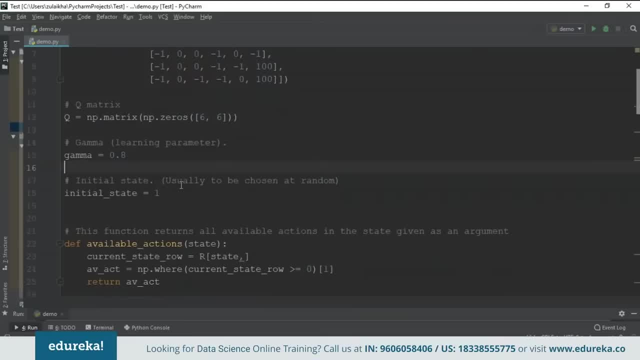 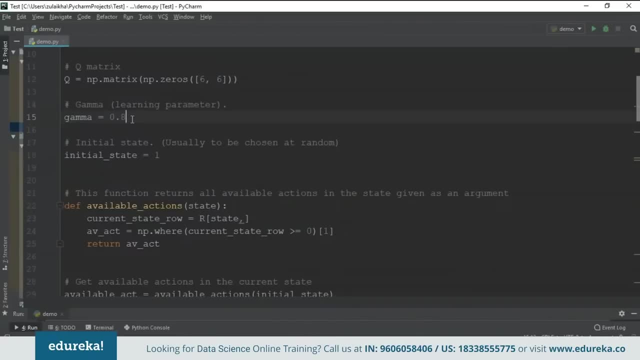 So, basically, the Q matrix is going to be initialized to 0 over here, All right. after that we're setting the gamma parameter to 0.8.. So, guys, you can play with this parameter and you know, move it to 0.9 or move it lower to 0.8.. 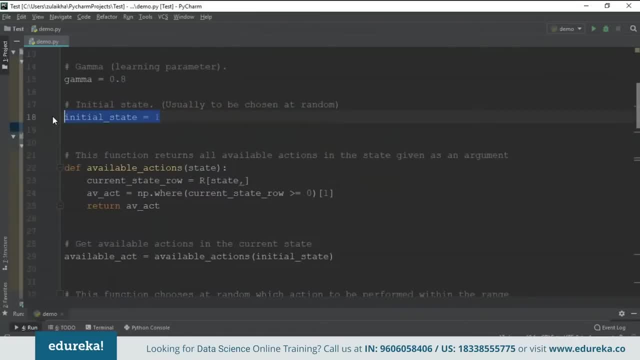 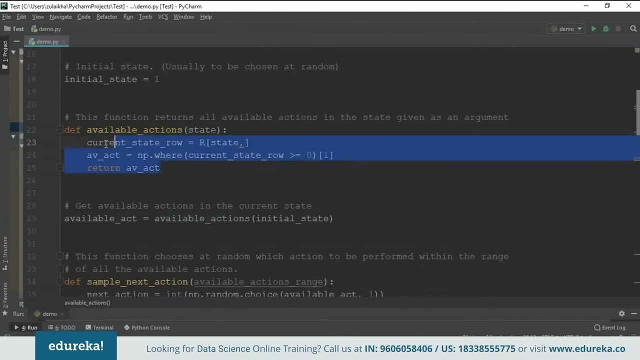 Okay, you can see what happens then. then we'll set an initial stage. Okay, initial stage is set as one. after that, We're defining a function called available actions. Okay, So basically, what we're doing here is: since our initial state is one, we're going to check our row number one. 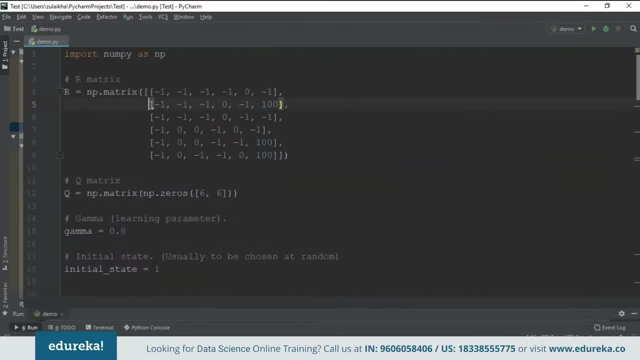 Okay, this is our row number one. Okay, this is row number zero, This is row number one, and so on. So we're going to check the row number one and we're going to find the values which are greater than or equal to 0, because 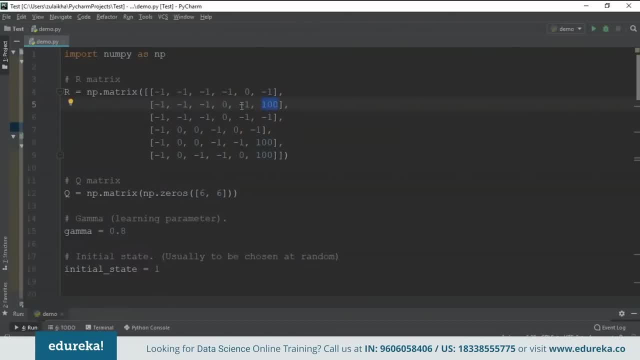 these values Basically- Basically represent the nodes that we can travel to. now, if you select minus one, you can't traverse to minus one. Okay, I explained this earlier. the minus one represents all the nodes that we can travel to, but we can travel to these. 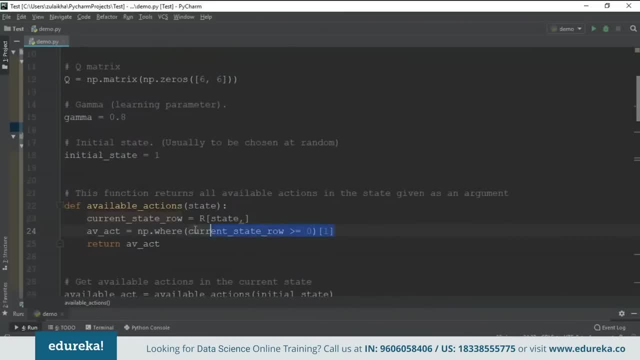 nodes. Okay, So basically over here we're checking all the values which are equal to 0 or greater than 0. these will be our available actions, So if our initial state is one, we can travel to other states whose value is equal to 0 or greater than 0, and this is stored. 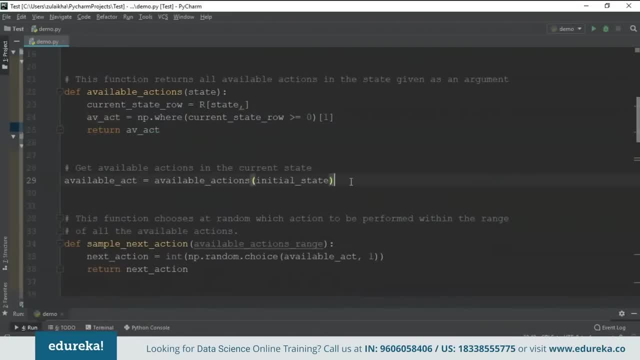 in this Variable called available act. All right, Now, this will basically get the available actions in the current state. Okay, So we're just storing the possible actions in this available act variable over here. So basically over here, since our initial state is one, we're. 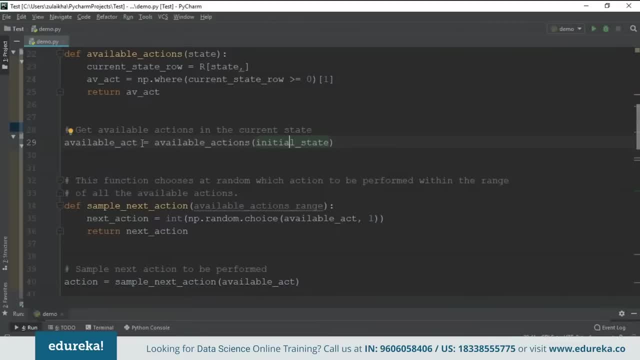 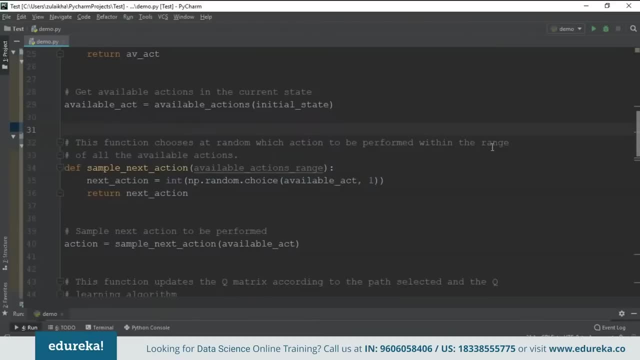 going to find out the next possible states We can go to. okay, that is stored in the available act variable. Now, next is this: function chooses at random which action to be performed within the range. So, if you remember over here. so, guys, initially, 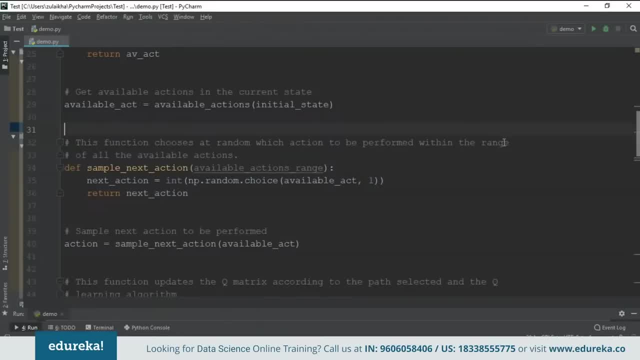 We are in stage number one. Okay, our available actions is to go to stage number three or stage number five. Sorry, room number three or room number five. Okay. Now, randomly, we need to choose one room, So for that we're using this line of code: 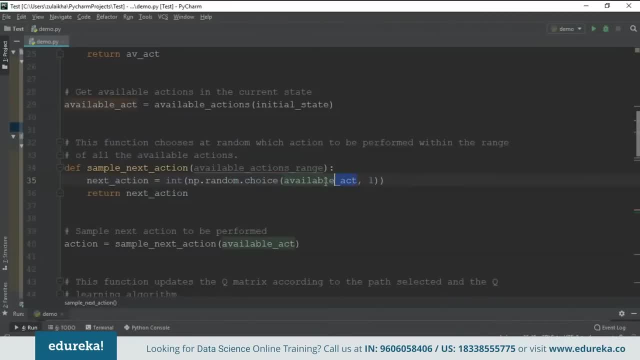 Okay. So here we are randomly going to choose one of the actions from the available act. this available act, Like I said earlier, stores all our possible actions. Okay, from the initial state. Okay. So once it chooses an action, it's going to store it in next. 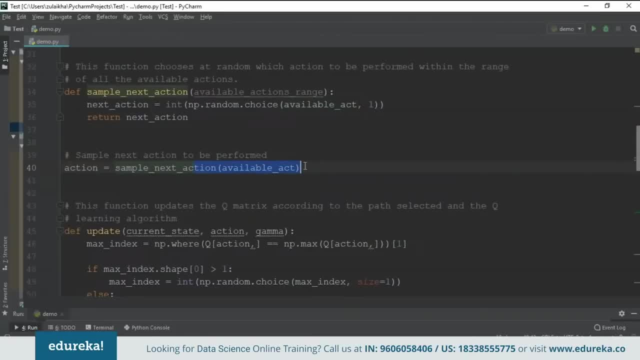 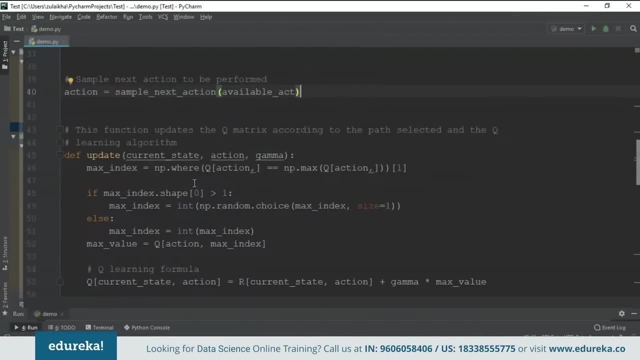 action. So, guys, this action will represent the next available action to take now. next is our Q matrix. Remember this formula that we used? So, guys, this formula that we use is what we're going to calculate in the next few lines of code. 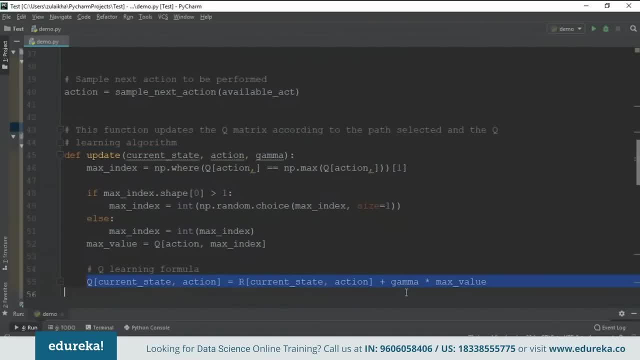 So in this block of code we're just executing and computing the value of Q. Okay, this is our formula for computing the value of Q, current state comma action, our current state comma action, gamma into the maximum value. So here, basically, we're going to calculate the maximum. 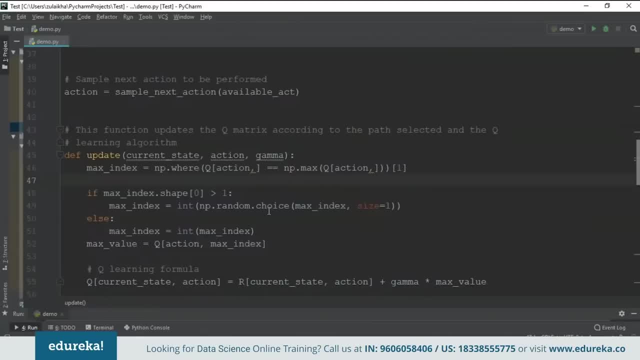 index, meaning that we're going to check which of the possible actions will give us the maximum Q value. All right, if you remember in our explanation over here, this value of your Max Q of 5 comma 1, 5 comma 4 and 5 comma 5, we. 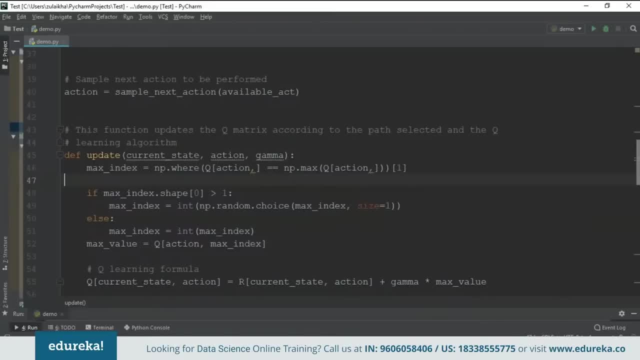 had to choose a maximum Q value that we get from these three. So basically, that's exactly what we're doing in this line of code: We're calculating the index which gives us the maximum value. after we finish computing the value of Q, We'll just have to. 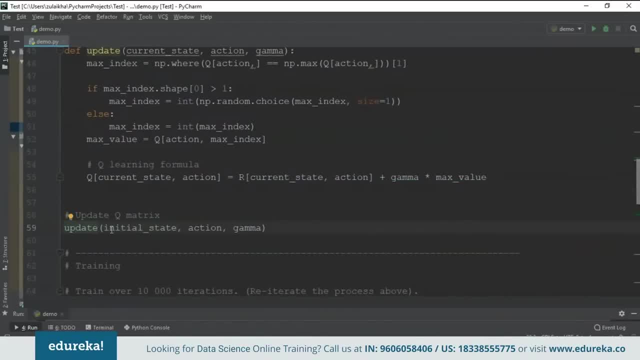 Update our Matrix. after that, we'll be updating the Q value and we'll be choosing a new initial state. Okay, So this is the update function that is defined over here. Okay, So I've just called the function over here. So, guys, this whole set of code will just calculate the Q value. 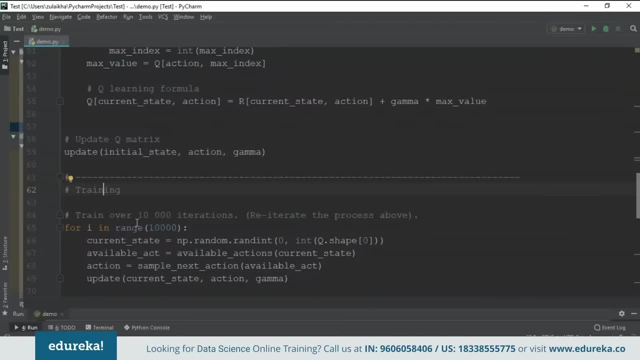 Okay, This is exactly what we did in our examples. after that We have the training phase. So, guys remember, the more you train an algorithm, the better it's going to learn. Okay, So over here I have provided around 10,000 iterations. 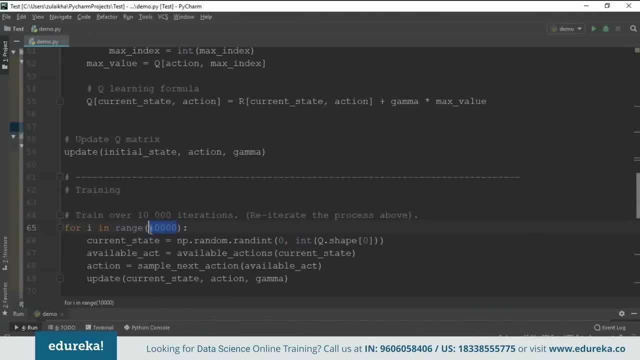 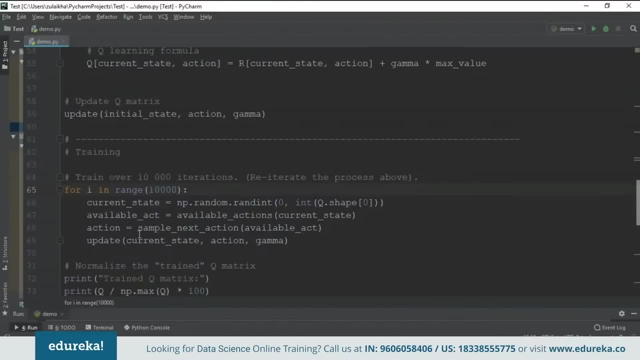 Okay, so my range is 10,000 iterations, Meaning that my agent will take 10,000 possible scenarios and it will go through 10,000 iterations to find out the best policy. So you're exactly what I'm doing is I'm choosing the current. 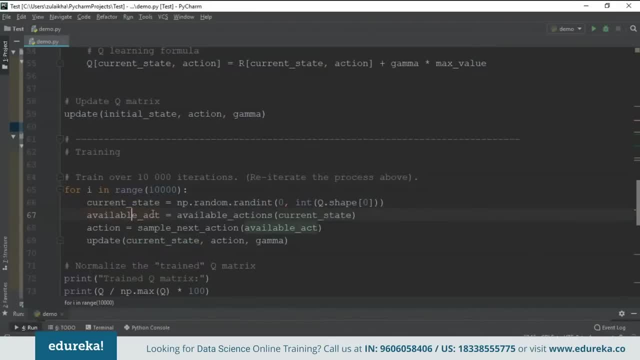 state randomly. after that I'm choosing the available action from the current state. So either I can go to stage 3 or state 5, then I'm calculating the next action and then I'm finally updating the value in the Q matrix and next we just normalize the Q matrix. 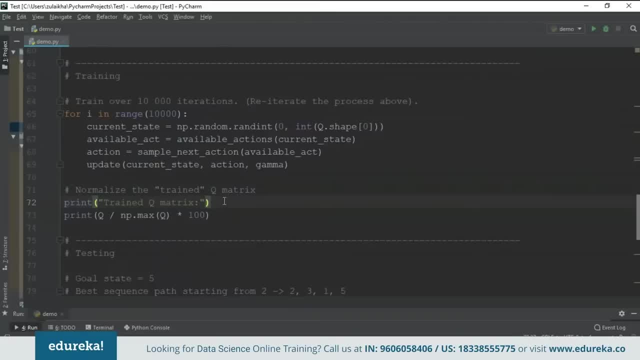 So sometimes in our Q matrix the value might exceed- Okay, Let's say it exceeded to 500, 600.. So that time you want to normalize the matrix, Okay, We want to bring it down a little bit. Okay, because larger numbers we won't be able to understand and 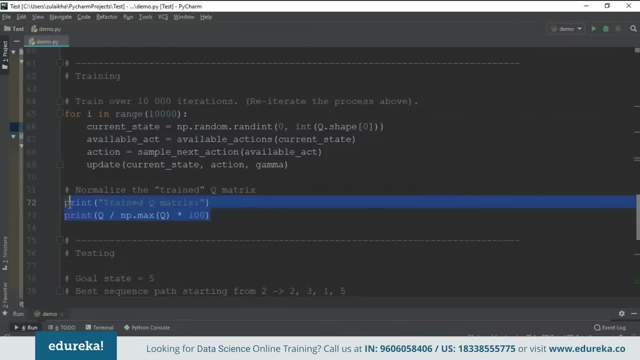 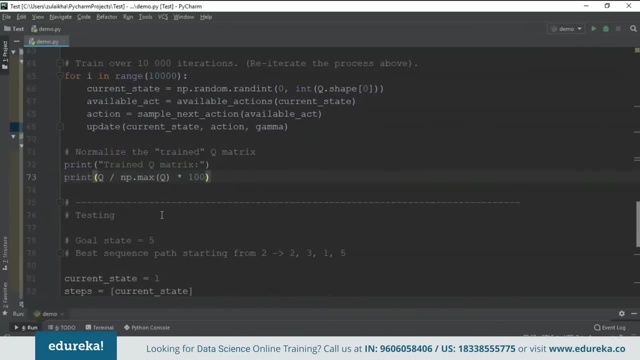 computation will be very hard on larger numbers. That's why we perform normalization. You're taking your calculated value and you're dividing it with the maximum Q value into hundred. All right, so you're normalizing it over here. So, guys, this is the testing phase. 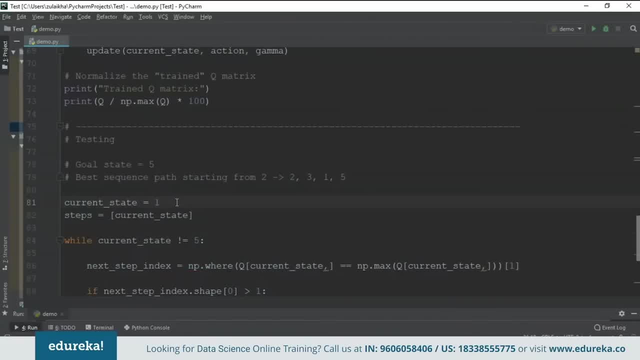 Okay, here You'll just randomly set a current state and you won't given any other data, because you've already trained Our model. Okay, you're going to give a current state. then you're going to tell your agent that. listen, you're in room number one. 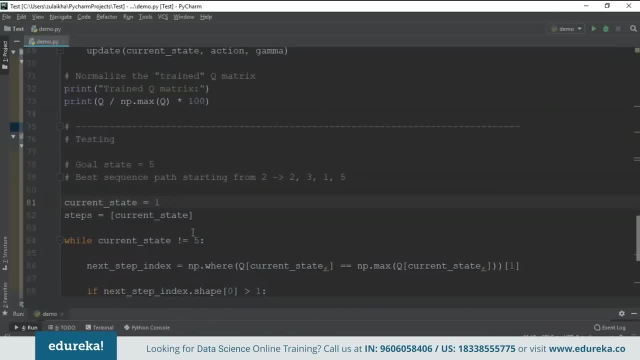 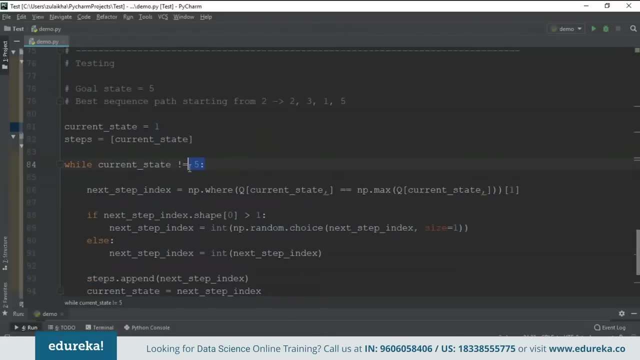 Now you need to go to room number five. Okay, so he has to figure out how to go to room number five, because we've trained him now. All right, So here we've set the current state to one, and we need to make sure that it's not equal to five, because five is the end goal. 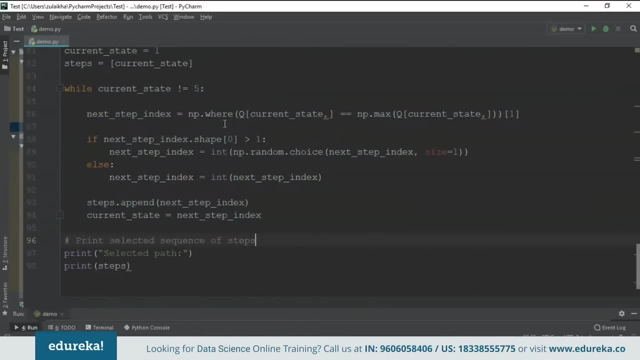 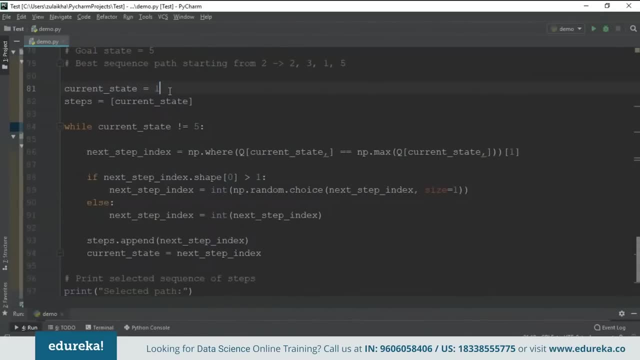 So, guys, this is the same loop that we executed earlier, So we're going to do the same iterations again. Now, if I run this entire code, let's look at the result. So our current state here, with chosen As one: Okay, and if we go back to our Matrix, you can see that there. 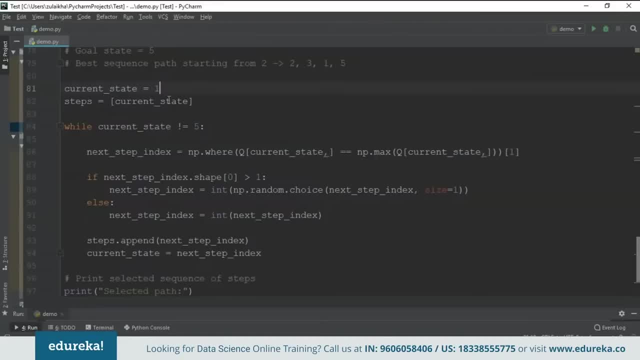 is a direct link from one to five, which means that the route that the agent should take is one to five. Okay, directly It should go from one to five because it will get the maximum reward, like that. Okay, Let's see if that's happening. 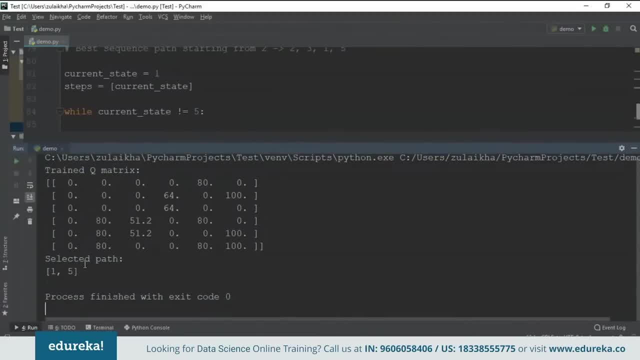 So if I run this, it should give me a direct path from one to five. Okay, that's exactly what happened. So this is a selected path, So directly from one to five. it went, and it calculated The entire Q matrix for me. 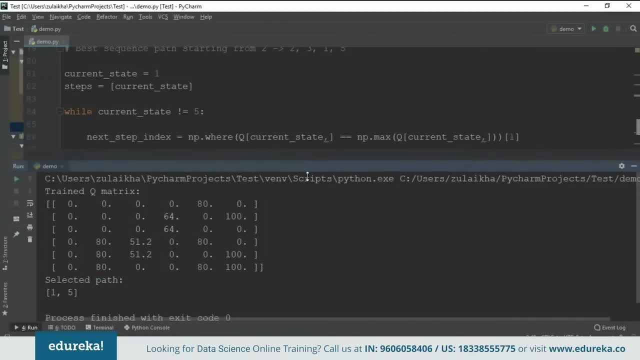 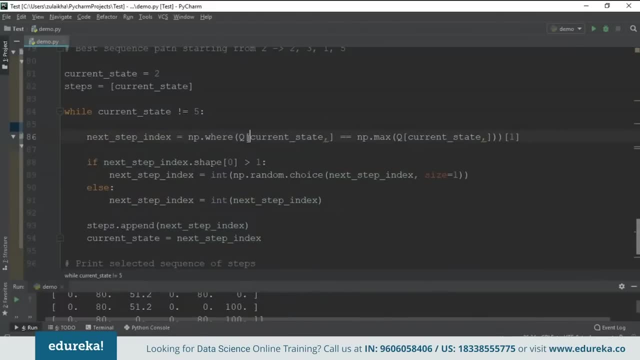 So, guys, this is exactly how it works. Now, let's try to set the initial stage as, let's say, two. So if I set the initial stage as two and if I try to run the code, let's see the path that it gives. 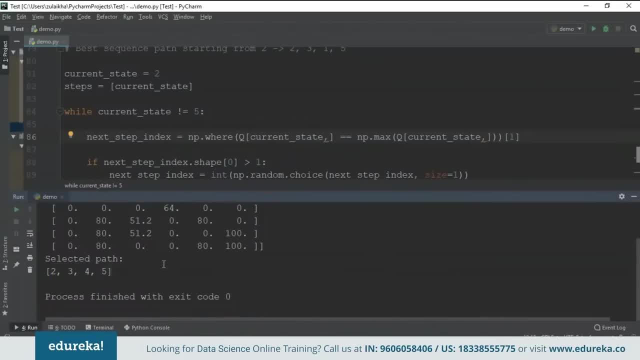 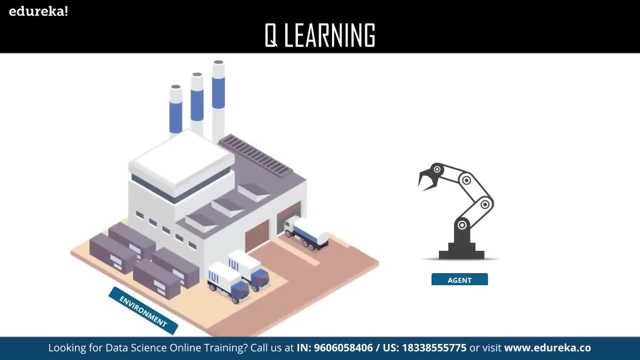 So the selected path is two, three, four, five. Now it chose this path because it's giving us the maximum reward from this path. Okay, This is the Q matrix that it calculated and this is the selected path Now for a robot, and environment is a place where it has been. 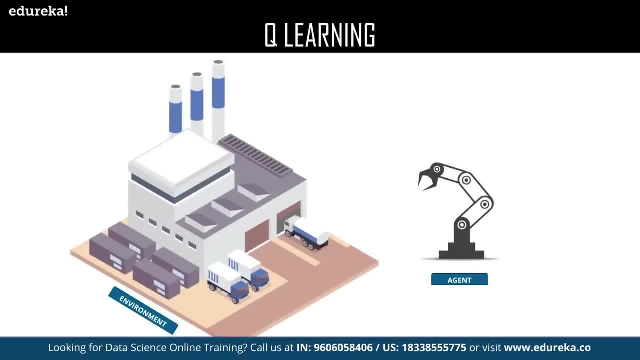 put to use. Now, remember, this robot is itself the agent. For example, an automobile factory where a robot is used to move materials from one place to another. Now, the task we discussed just now have a property in common. Now, these tasks involve an environment and expect the agent. 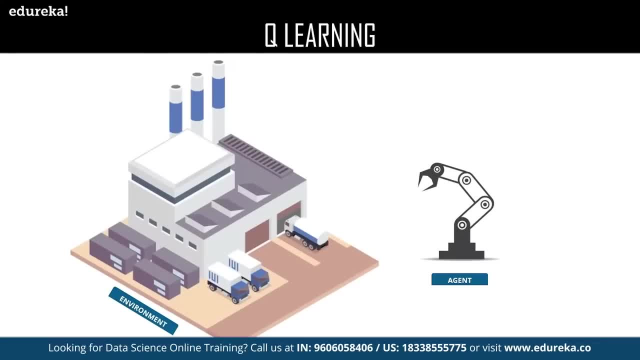 to learn from the environment. Now this is where traditional machine learning Fails, and hence the need for reinforcement learning. Now it is good to have an established overview of the problem that is to be solved using the Q learning or the reinforcement learning. 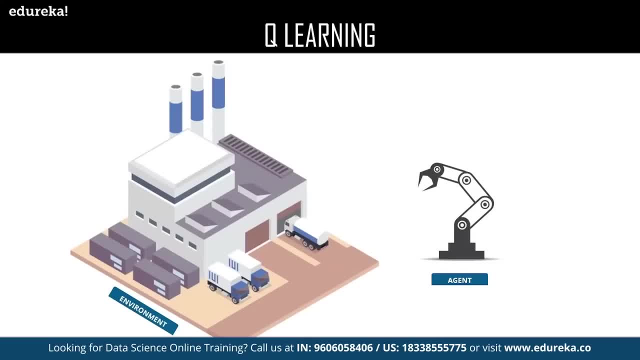 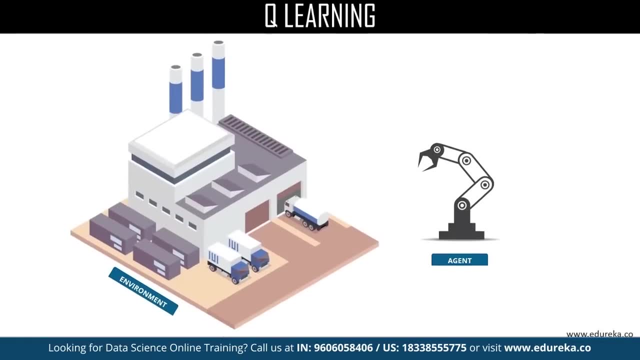 So it helps to define the main components of a reinforcement learning solution, That is, the agent, environment, action, rewards and States. So let's suppose we are to build a few autonomous robots for an automobile building factory. Now these robots will help the factory personal by conveying 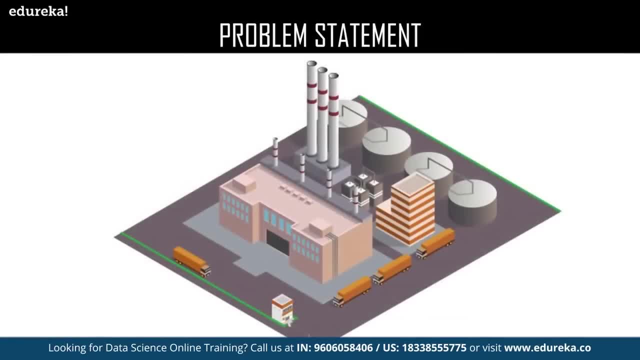 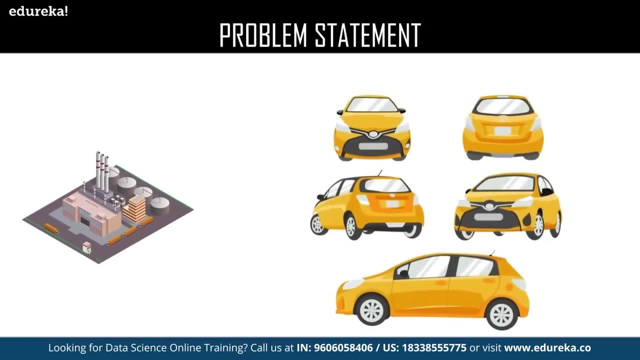 them the necessary parts That they would need in order to build the car. Now these different parts are located at nine different positions within the factory warehouse. The car part include these chassis, wheels, dashboard, the engine and so on, and the factory workers have prioritized the location. 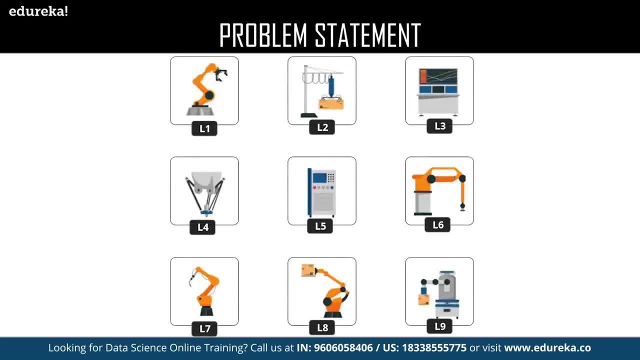 that contains the body or the chassis to be the topmost, but they have provided the priorities for other locations as well, which we will look into the moment that these locations within the factory look somewhat like this. So, as you can see, here we have L1, L2, L3, all of these stations. 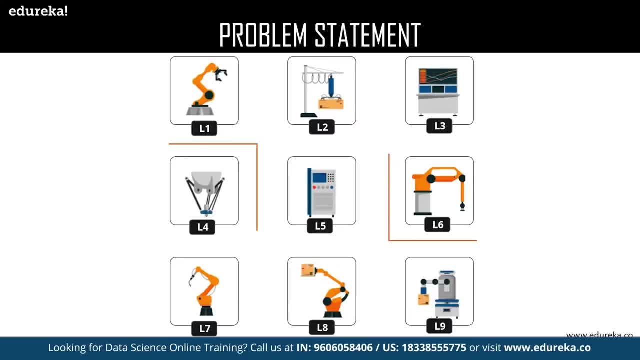 Now one thing: you might notice here that there are little obstacle present in between the locations. So L6 is the top priority location. that contains the chassis for preparing the car bodies. Now the task is to enable the robots so that they can find the shortest route from any given location to another location on. 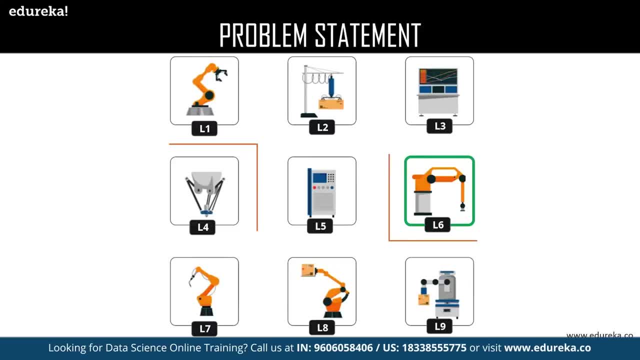 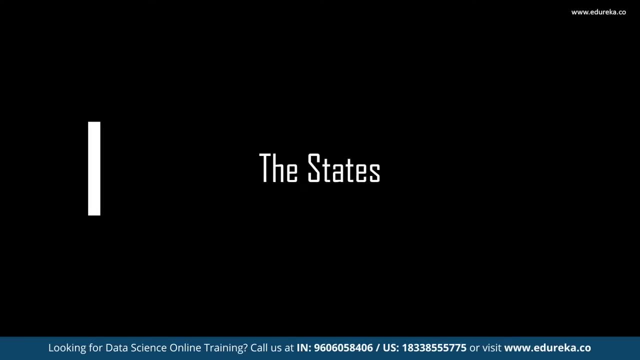 their own. Now the agents in this case are the robots. the environment is the automobile factory warehouse. So let's talk about the states. The states are the location in which a particular robot is present in the particular instance of time, which will denote its states. the machines understand numbers rather than letters. 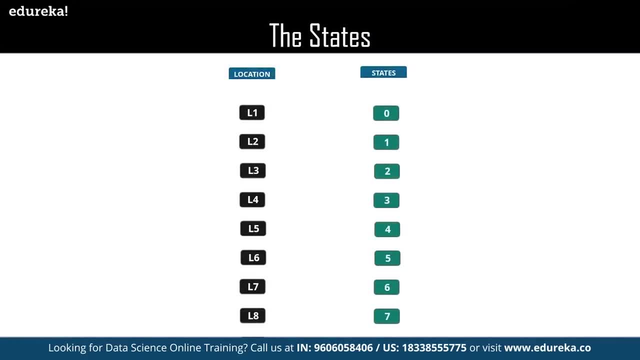 So let's map the location codes to number. So, as you can see here we have mapped location L1 to the state 0, L2 and 1 and so on. We have L8 as state 7 and N line at state 8.. 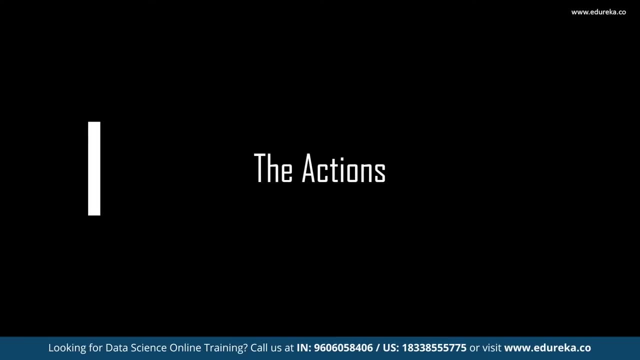 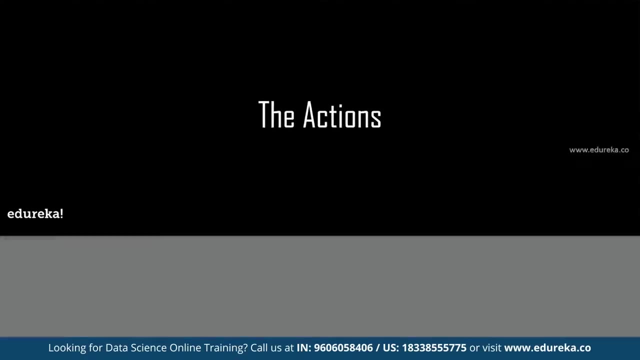 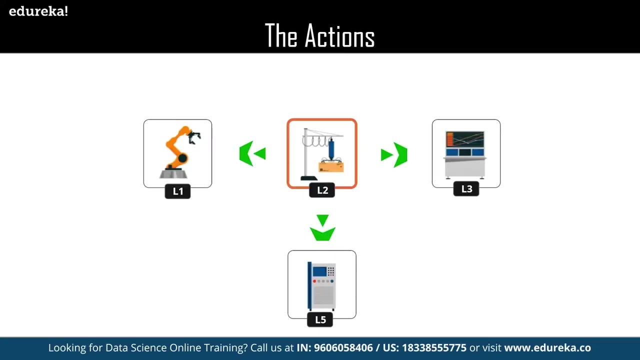 Well, next, what we're going to talk about are the actions. So in our example, the action will be the direct location that a robot can go from a particular location. right? Consider a robot that is at L2 location and the direct locations to which it can move are L5, L1 and L3.. 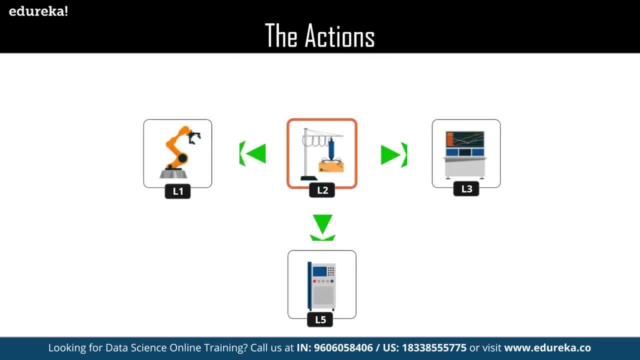 Now the figure here may come in handy to visualize this. now, as you might have already guessed, the set of actions here is nothing but the set of all possible states of the robot. for each location, the set of actions That a robot can take will be different. 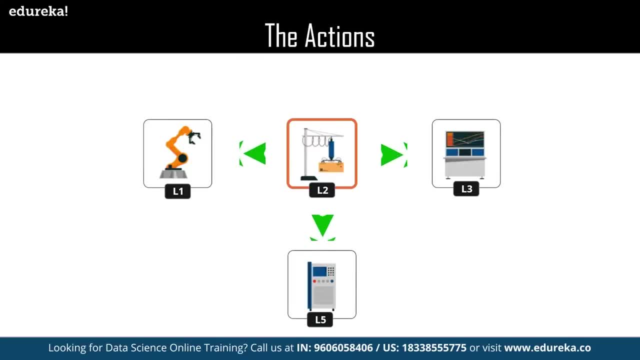 For example, the set of actions will change if the robot is in L1 rather than L2.. So if the robot is in L1, it can only go to L4 and L2 directly. Now that we are done with the states and the actions, 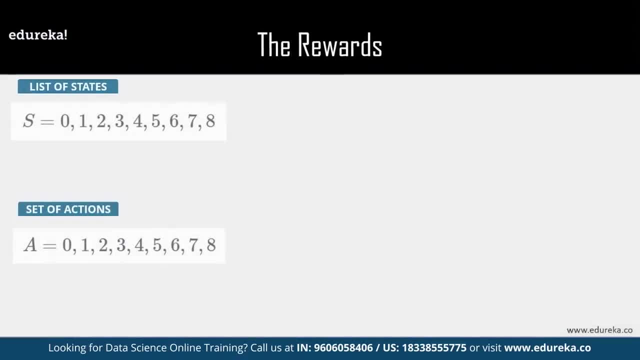 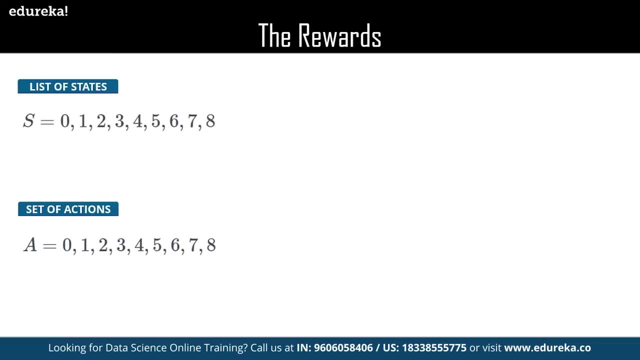 Let's talk about the rewards. So the states are basically 0, 1, 2, 3, 4 and the actions are also 0, 1, 2, 3, 4 up till 8.. Now the rewards now will be given to a robot if a location which 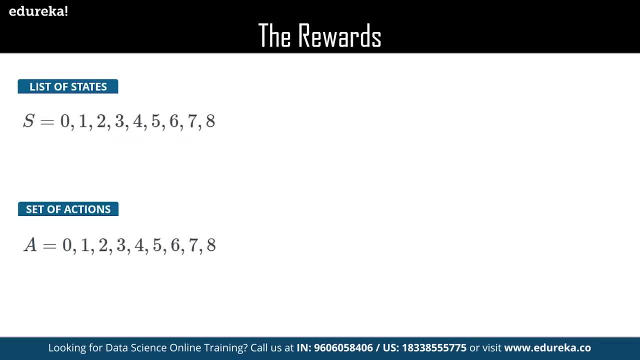 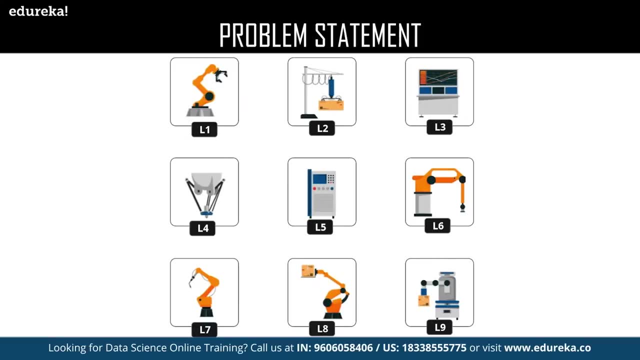 is the state Is directly reachable from a particular location. So let's take an example. Suppose L9 is directly reachable from L8, right. So if a robot goes from L8 to L9 and vice-versa, it will be rewarded by 1, and if a location is not directly reachable from 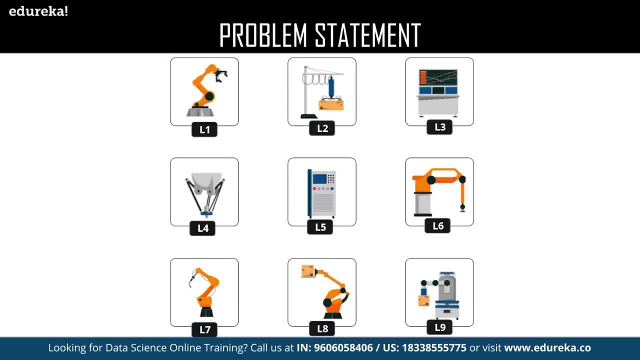 a particular location. we do not give any reward, a reward of 0. now. the reward is just a number here and nothing else. it enables the robots to make sense of the movements, helping them in deciding what locations are directly reachable and what are not. now, with this queue, 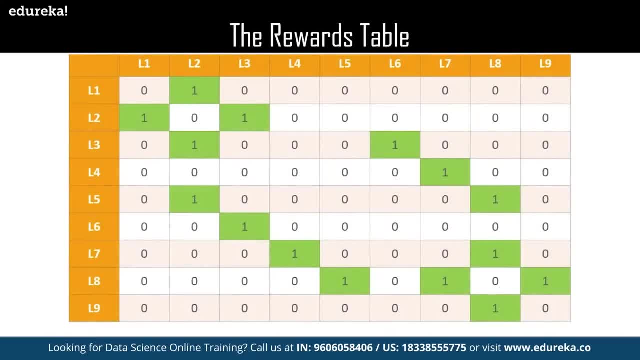 We can construct a reward table which contains all the reward values, mapping between all possible states. So, as you can see, here in the table, the positions which are marked green have a positive reward and, as you can see here we have all the possible rewards that a robot can get by moving. 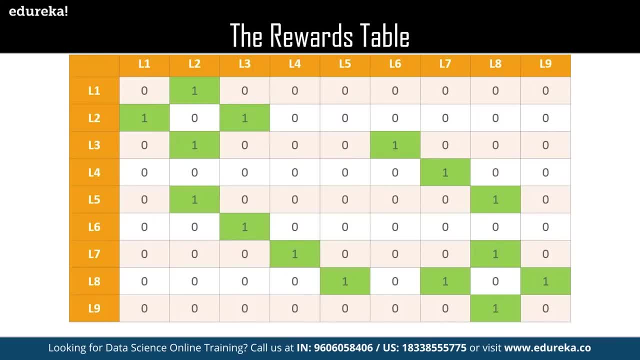 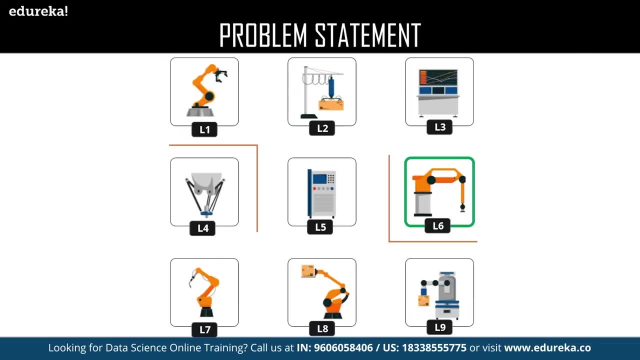 in between the different states. now comes an interesting decision. Now remember that the factory administrator prioritize L6 to be the topmost. So how do we incorporate this fact in the above table? Now, this is done by associating the topmost priority location. 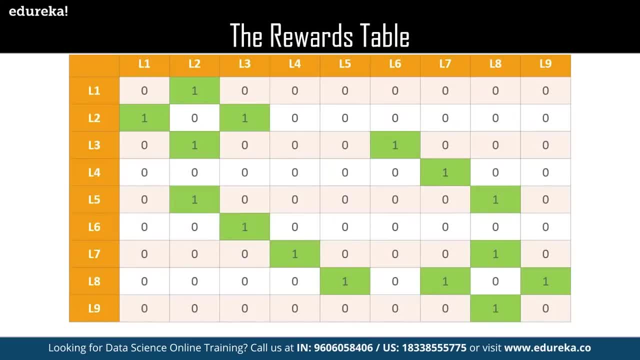 with a very high reward than the usual ones. So let's put 999 in the cell L6, L6. now the table of rewards with the higher reward for the topmost location looks something like this: We have now formally defined all the vital components for the. 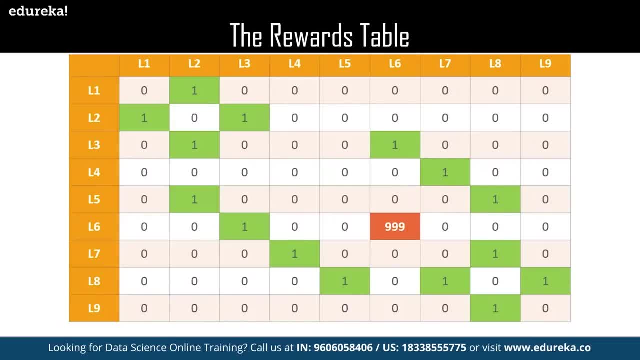 solution. We are aiming for the problem discussed. Now. you will shift gears a bit and study some of the fundamental concepts that prevail in the world of reinforcement learning and Q learning. So first of all we'll start with the Bellman equation. 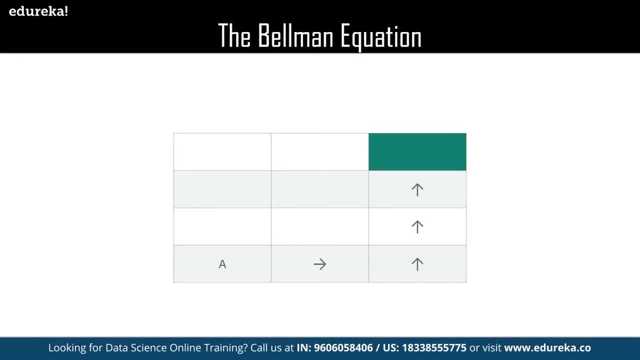 Now consider the following square of rooms, which is analogous to the actual environment from our original problem, but without the barriers. now suppose a robot needs to go to the room marked in the green from its current position a using the specified direction. Now, how can we enable the robot to do this programmatically? 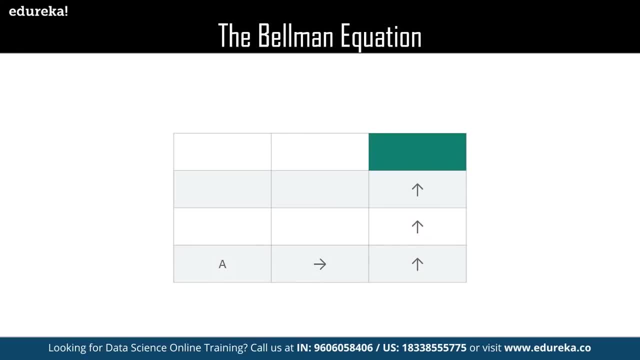 One idea would be introduced, some kind of a footprint which the robot will be able to follow. now here a constant Value is specified in each of the rooms which will come along the robots way if it follows the direction specified above now. in this way, if it starts at location a, it will be able to scan. 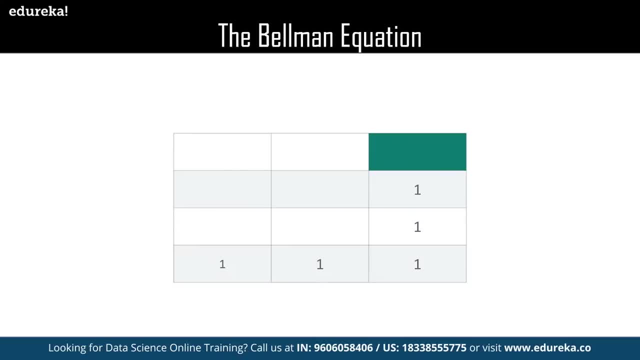 through this constant value and will move accordingly. but this will only work if the direction is prefix and the robot always starts at the location a. now consider: the robot starts at this location rather than its previous one. Now, the robot now sees footprints in two different directions. 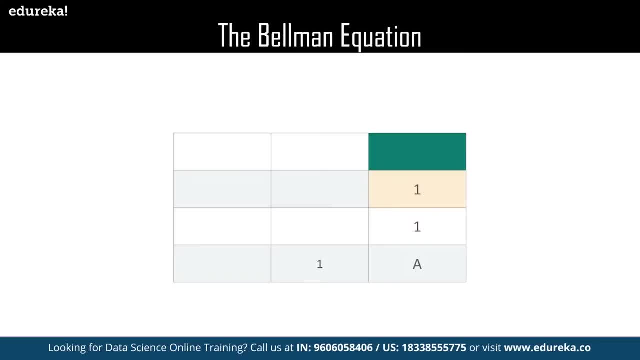 It is therefore Able to decide which way to go in order to get the destination, which is the green room. It happens primarily because the robot does not have a way to remember the directions to proceed, So our job now is to enable the robot with the memory. 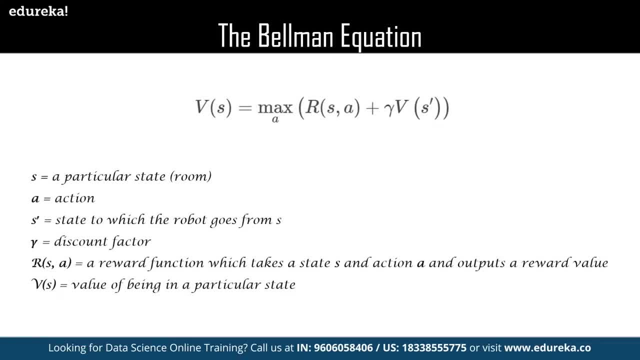 Now, this is where the Bellman equation comes into play. So, as you can see here, the main reason of the Bellman equation is to enable the robot with the memory. That's the thing we're going to use. So the equation goes something like this: V of S gives maximum. 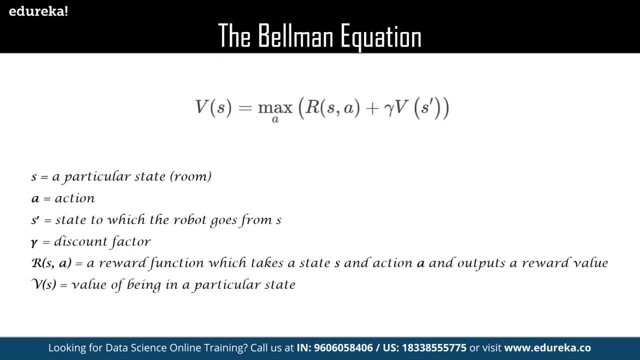 of a, R of S, comma a plus gamma of Vs dash, where s is a particular state which is a room, a is the action moving between the rooms s, dash is the state to which the robot goes from s and gamma is the discount factor. 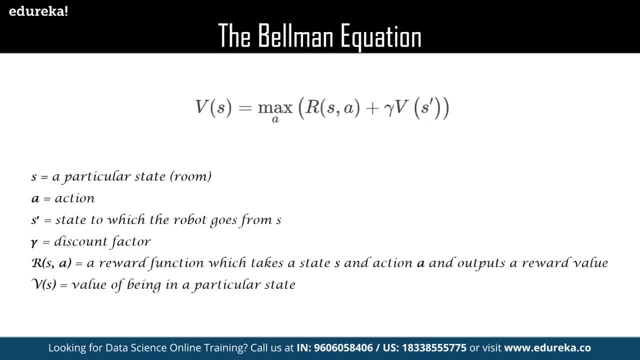 Now we'll get into it in a moment. and obviously R of S, comma a, is a reward function which takes a state s and action a and outputs the reward. now, V of S is the value of being in a particular state, which is the footprint. 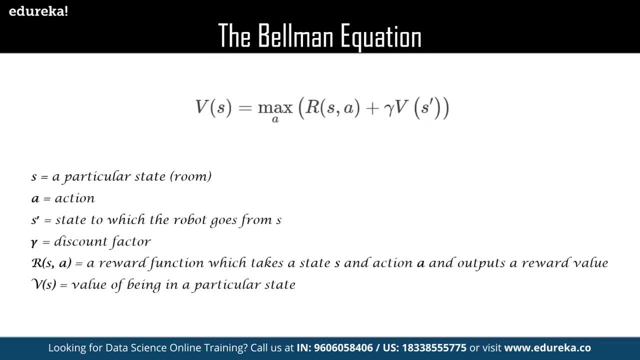 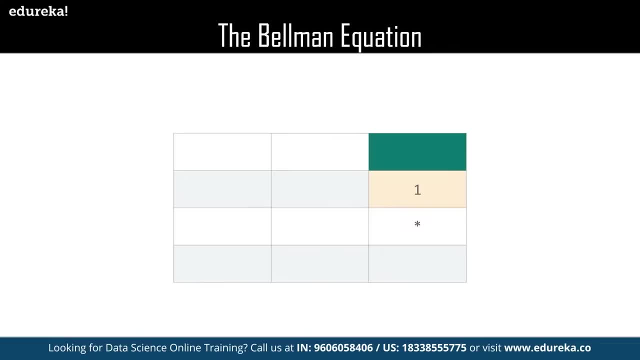 Now We consider all the possible actions and take the one that yields the maximum value. Now there is one constraint, However, regarding the value footprint, that is the room marked in the yellow just below the green room. It will always have the value of one to denote. that is one of. 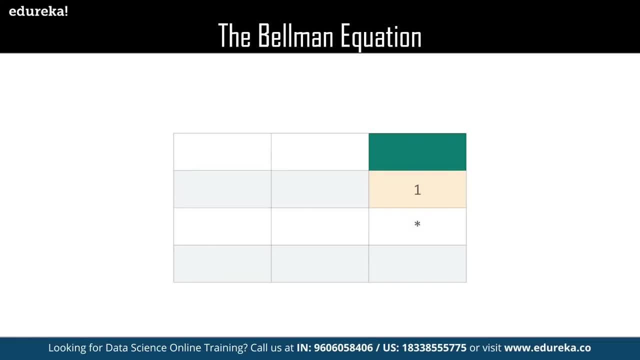 the nearest room adjacent to the green room. Now, this is also to ensure that a robot gets a reward when it goes from a yellow room to the green room. Let's see how to make sense of the equation which we have here. So let's assume 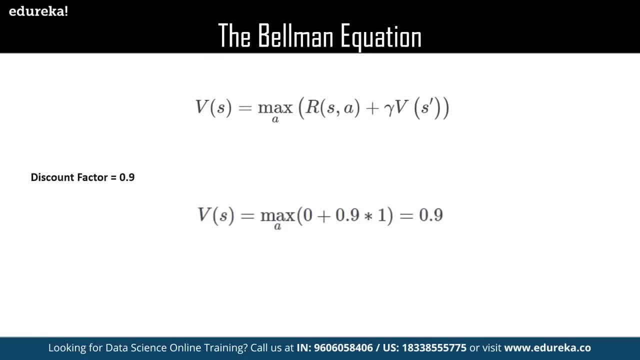 A discount factor of 0.9. as we remember, gamma is the discount value or the discount factor, So let's take it 0.9.. Now for the room which is marked just below the one, or the yellow room which is the asterisk mark for this room. 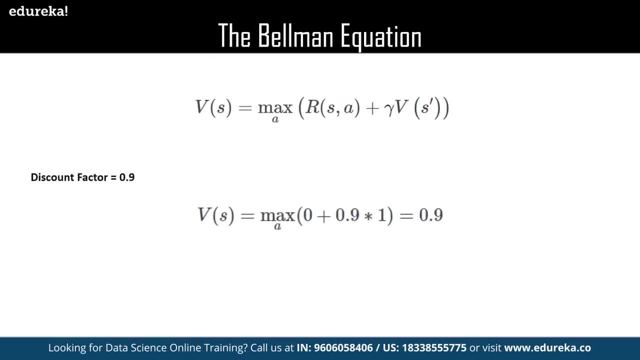 What will be the V of S? that is, the value of being in a particular state. So for this V of S would be something like: maximum of a will take 0, which is the initial of our s comma, a plus 0.9, which. 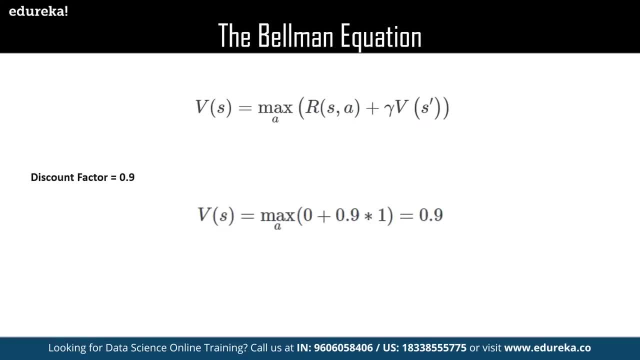 is gamma into one That gives us 0.9.. Now here the robot will not get any reward for going to a state marked in yellow. Hence the R s comma a is 0 here, for the robot knows the value of being in the yellow room. 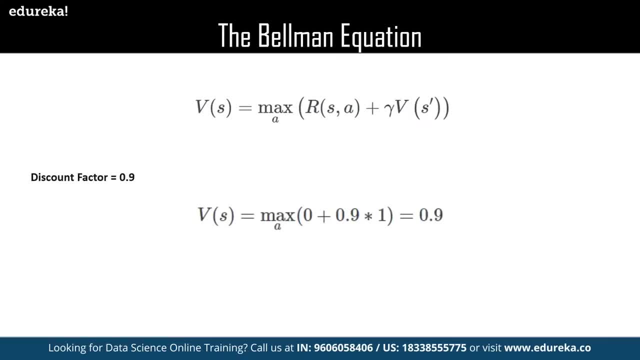 Hence V of S dash is one. following this for the other states, We should get 0.9.. Then again, if we put 0.9 in this equation, we get 0.81, then 0.729.. And then we again. 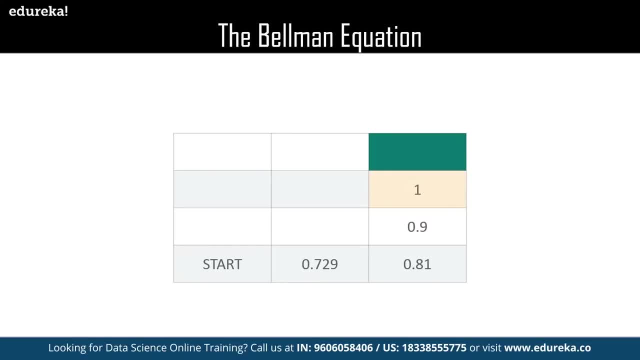 The starting point. So this is how the table looks, with some value footprints computed from the Bellman equation, and a couple of things to notice. here is that the max function helps the robot to always choose the state that gives it the maximum value of being in that state. 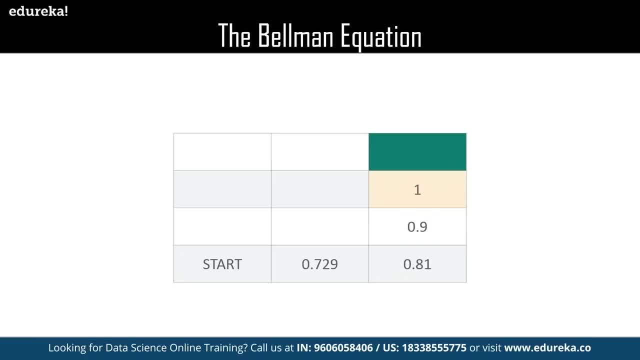 Now the discount factor gamma notifies the robot about how far it is from the destination. This is typically specified by the developer of the algorithm that would be installed in the robot. Now the other states Can also be given their respective values in a similar way. 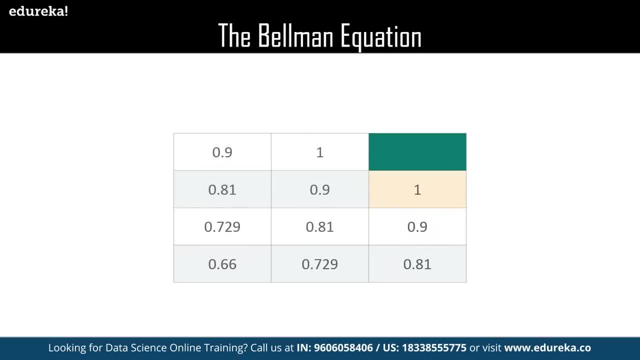 So, as you can see here, the boxes adjacent to the green one have one, and if we move away from one, we get 0.9, 0.81, 0.729 and finally we reach 0.66. now the robot now can proceed its way through the 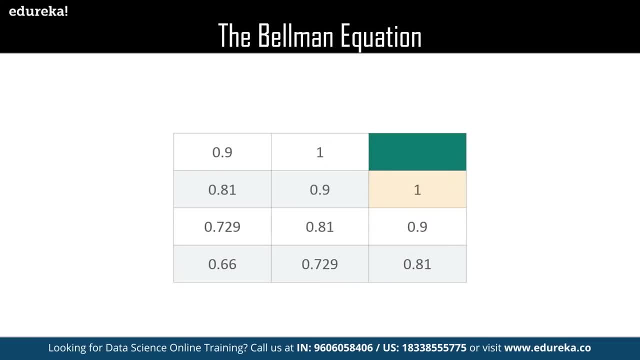 green room utilizing these value footprints, even if it's dropped at any arbitrary room in the given location. now, if a robot lands up in the highlighted Blue area, it will still find two options to choose from, but eventually either of the paths will be good enough for the robot. 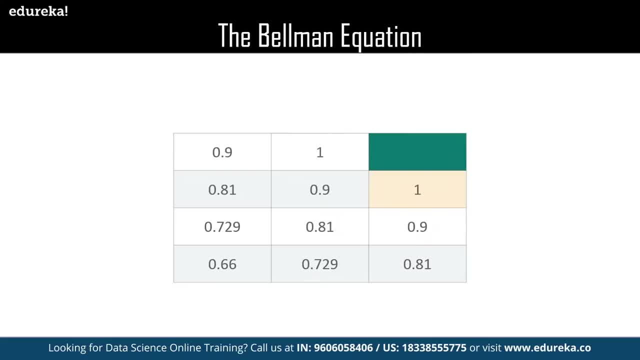 to take because of the way the value footprints are now laid out. Now, one thing to note here is that the Bellman equation is one of the key equations in the world of reinforcement learning and Q learning. So if we think realistically, our surroundings do not always 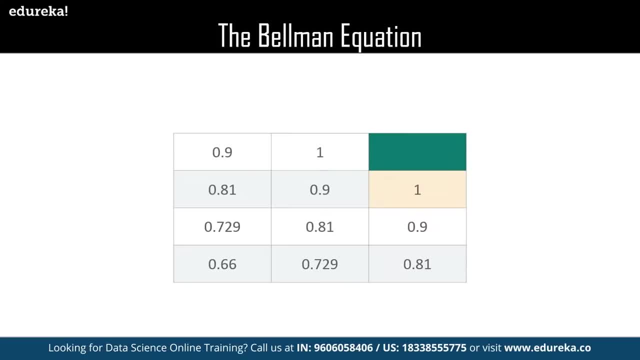 work in the way we expect. there is always a bit of stochasticity involved in it, But this applies to robot As well. Sometimes it might so happen that the robots machinery got corrupted. Sometimes the robot may come across some hindrance on its way. 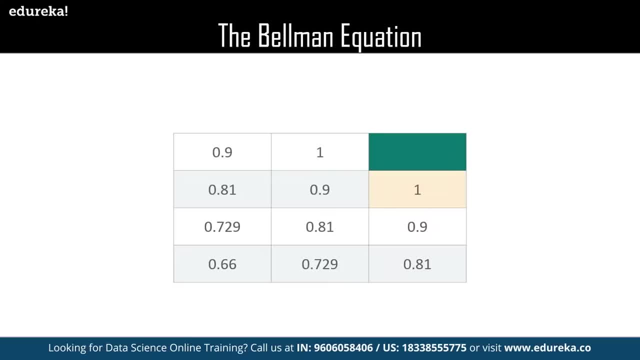 which may not be known to it beforehand, right, and sometimes even if the robot knows that it needs to take the right turn, it will not. so how do we introduce the stochasticity in our case? now, here comes the mark of decision process. but consider: the robot is currently in the red room and it needs to go to the 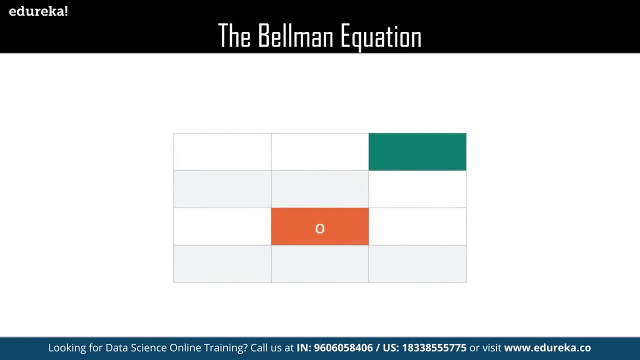 green room Now. Let's now consider The robot has a slight chance of dysfunctioning and might take the left or the right or the bottom turn, instead of taking the upper turn, in order to get to the green room from where it is now, which is the red room. 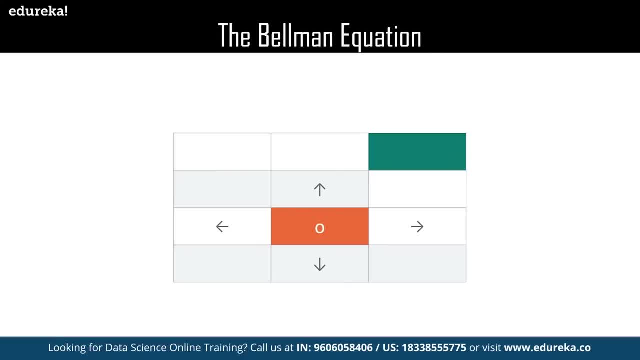 Now The question is: how do we enable the robot to handle this when it is out in the given environment right now? this is a situation where the decision-making regarding which turn is to be taken is partly random and partly under the control of the robot. now. 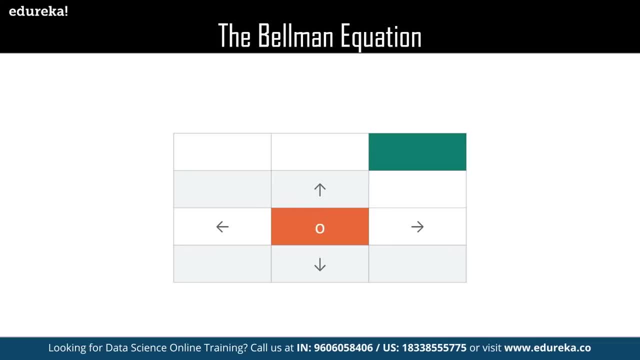 partly random, because we are Not sure when exactly the robot mind dysfunctional and partly under the control of the robot, because it is still making a decision of taking a turn right on its own and with the help of the program embedded into it. So a mark of decision process is a discrete time stochastic. 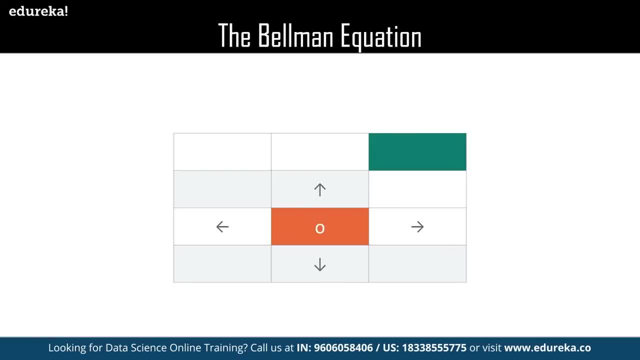 control process. It provides a mathematical framework for modeling decision-making in situations where the outcomes are partly random and partly under the control of the decision maker. now we need to give this concept a mathematical Shape, most likely an equation, which then can be taken further. 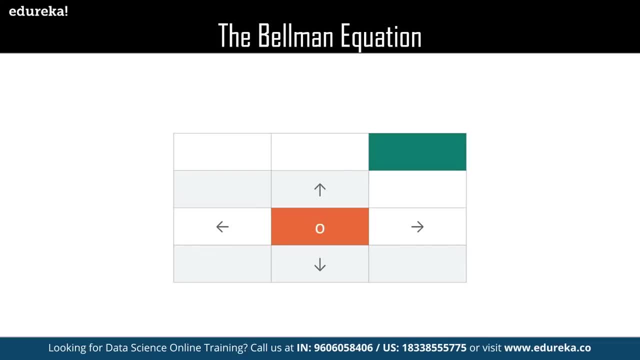 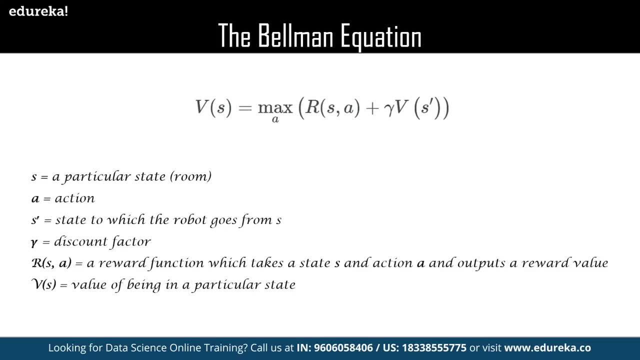 now you might be surprised that we can do this with the help of the Bellman equation, with a few minor tweaks. So if we have a look at the original Bellman equation, V of x is equal to maximum of our s comma a plus gamma V of s dash. 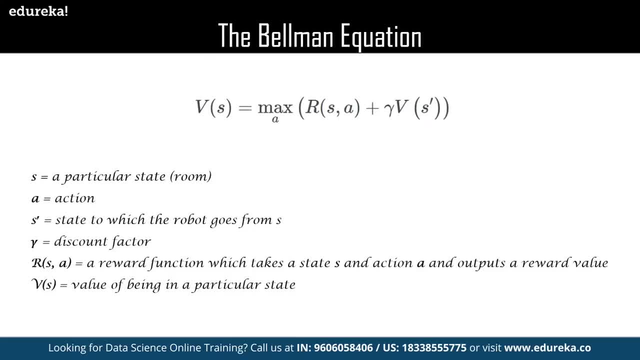 what needs to be changed in the above equation so that we can introduce some amount of randomness here? As long as we are not sure when the robot might not take the expected Turn, we are then also not sure in which room it might end up in. 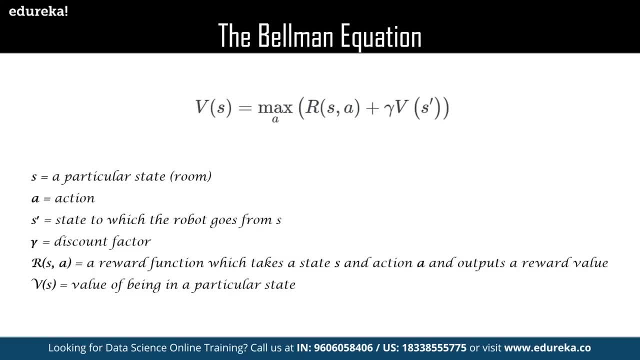 which is nothing but the room. it moves from its current room at this point, according to the equation, We are not sure of the s dash, which is the next state, or the room, but we do know all the probable turns the robot might take now in order to incorporate each of those probabilities into the above. 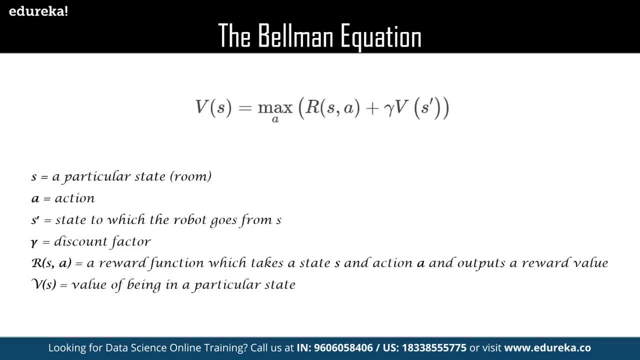 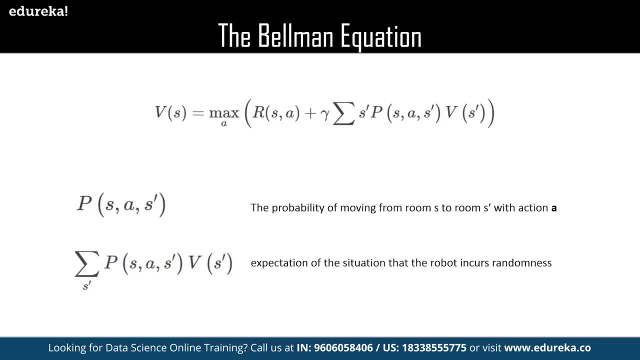 equation. We need to associate a probability with each of the turns to quantify the robot. if it has got any explicit, is chance of taking this turn Now. if we do so, we get: PS is equal to maximum of our s comma a plus gamma into summation of s dash, P, s comma a comma s dash into V of s. 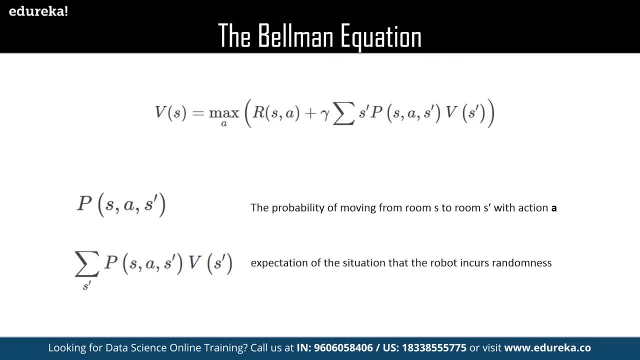 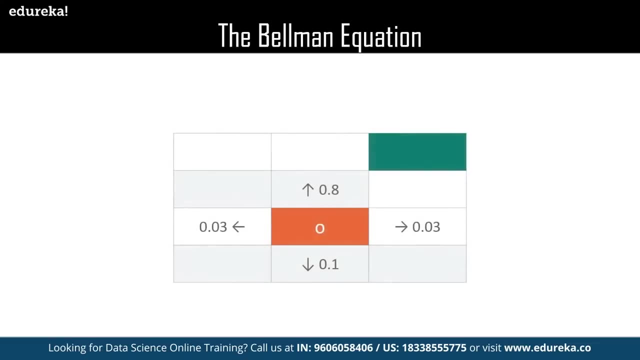 dash. Now the PS a and s dash is the probability of moving from room s to s dash with the action a, and the submission here is the expectation of the situation that the robot incurs, which is the randomness. Now let's take a look at this example here. 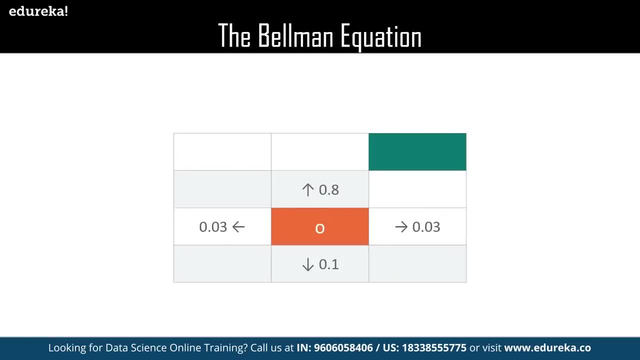 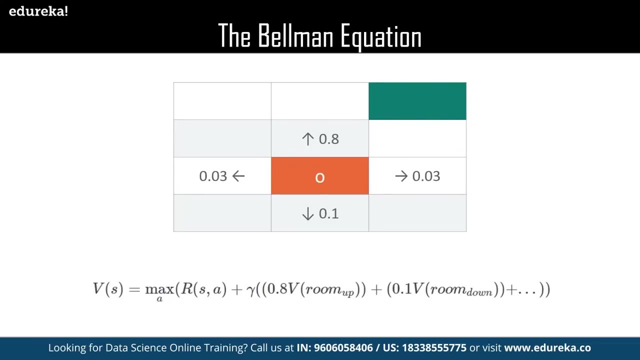 So when we associate the probabilities to each of these stones, we essentially mean that there is an 80% chance that the robot will take the upper turn. Now, if you put all the required values in our equation, we get: V of s is equal to maximum of r of s, comma a plus gamma of 0.8 into V of. 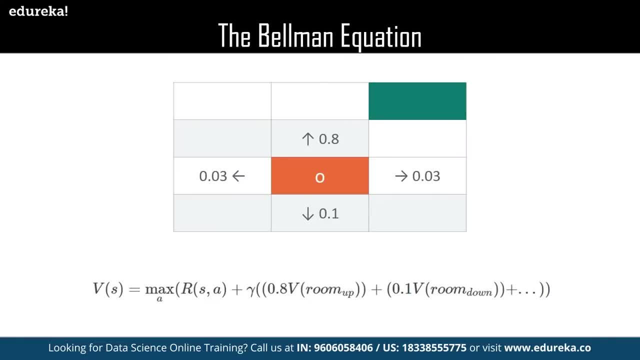 room up plus 0.1. Into V of room down, 0.03 into room of V of room left plus 0.03 into V of room right now. note that the value of footprints will not change due to the fact that we are incorporating stochastically here. but 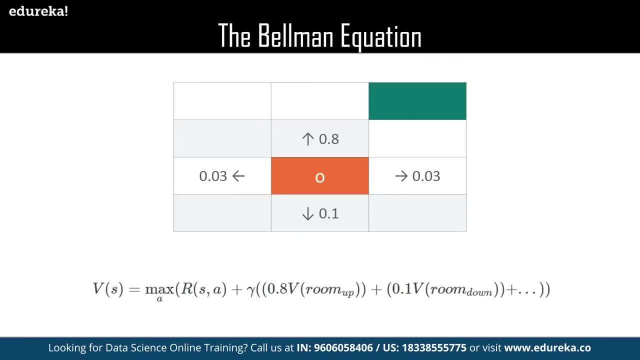 this time we will not calculate those value footprints. instead, We will let the robot to figure it out. now, up until this point, We have not considered about rewarding the robot for its action of going into a particular room. We are only rewarding The robot when it gets to the destination. 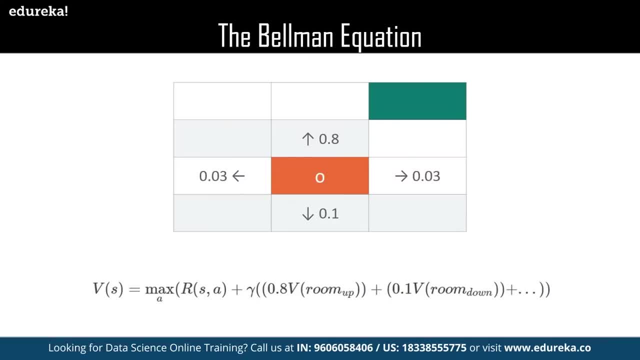 Now, ideally there should be a reward for each action The robot takes to help it better assess the quality of the actions. but the rewards need not to be always be the same. but it is much better than having some amount of reward for the actions than having 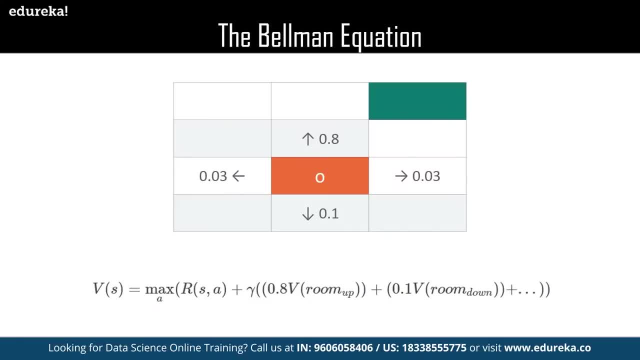 no rewards at all, right, And this idea is known as the living penalty. in reality, The reward system can be very complex, and particularly modeling sparse rewards is an active Area of research in the domain of reinforcement learning. So by now we have got the equation which we have is so what? 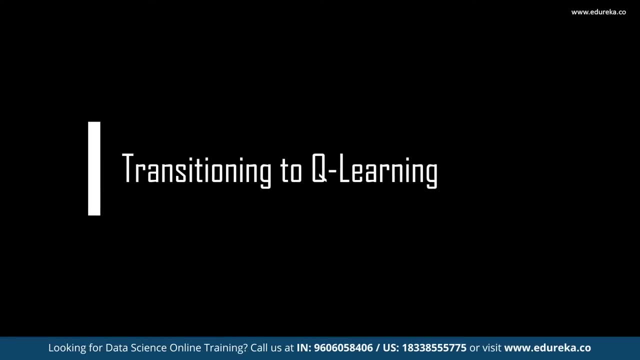 we're going to do is now transition to Q learning. So this equation gives us the value of going to a particular state, taking the stochasticity of the environment into account. Now we have also learned, very briefly, about the idea of living penalty, which deals with associating each move of the robot 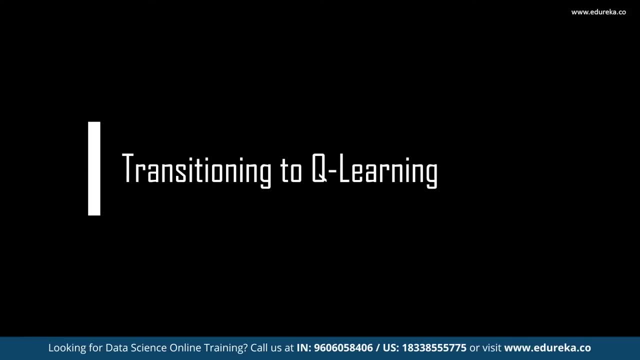 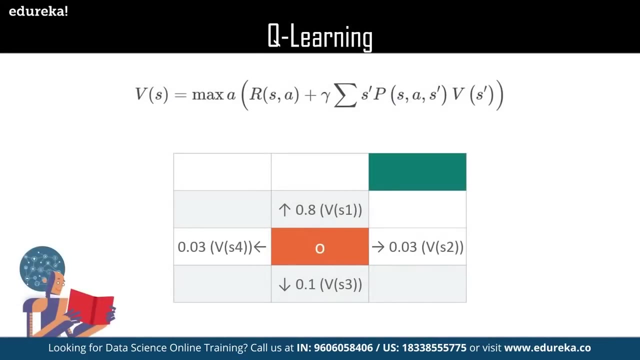 with a reward. So Q learning possesses an idea of assessing the quality Of an action that is taken to move to a state, rather than determining the possible value of the state which is being moved to. so earlier we had 0.8 into V of S1, 0.03 into V of S2, 0.1 into V of S3, and so on. 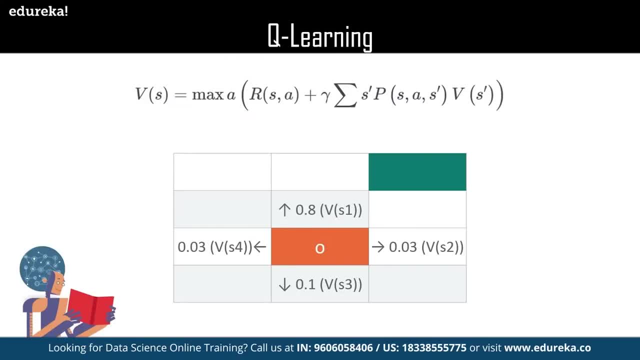 Now, if you incorporate the idea of assessing the quality of the action for moving to a certain state, so the environment with the agent and the quality of the action will look something like this: So, instead of 0.8, V of S1 will have Q of S1, A1 will have Q of S2, A2 Q of S3.. 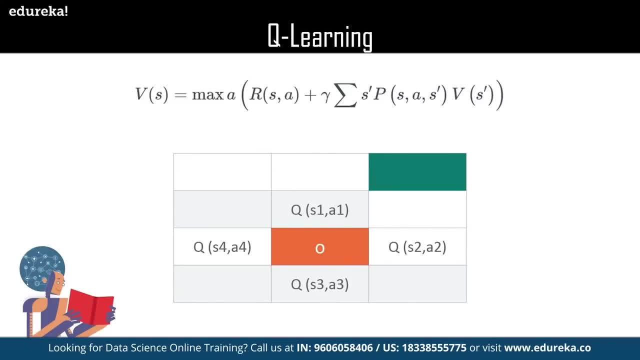 Now the robot now has four different states to choose from and along with that there are four different actions, also for the current state it is in. So how do we calculate Q of S? A, that is the cumulative quality of the possible actions the robot might take. 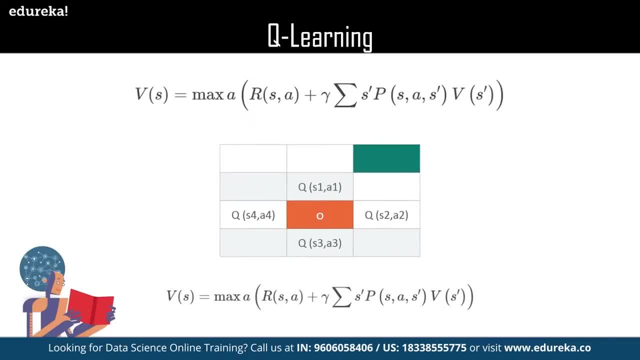 So let's break it down now from the equation: V of S Equals maximum of A R S, comma A plus gamma summation S dash, P, S, A S dash into V of S dash. If we discard the maximum function, we have R S of A plus. 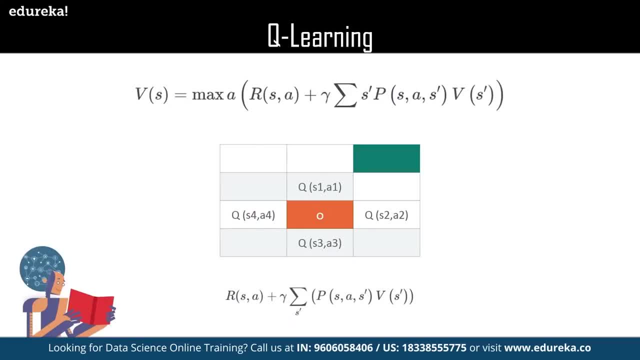 gamma into summation P and V. Now, essentially, in the equation that produces V of S, we are considering all possible actions and all possible states from the current state that the robot is in, And then we are taking the maximum value caused by taking a. 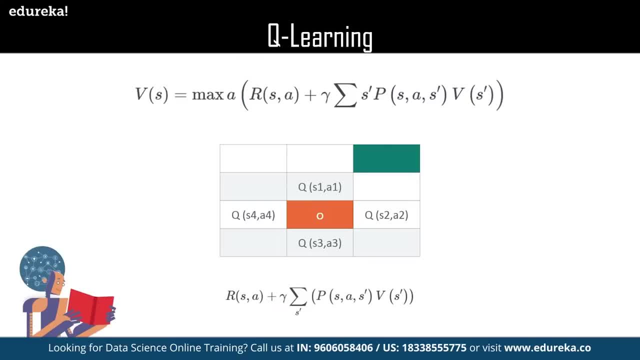 certain action and the equation produces a value footprint which is for just one possible action. In fact we can think of it as the quality of the action. So Q of S comma A is equal to R S comma A, plus gamma of summation P and V. 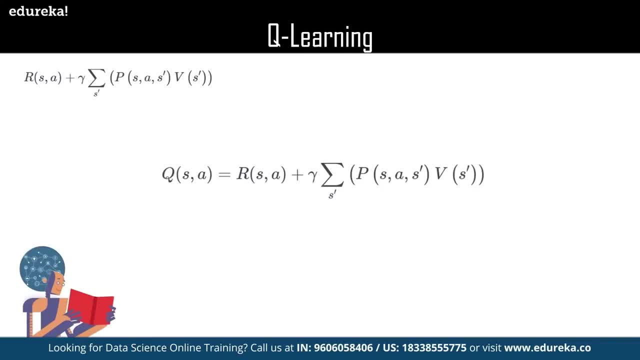 Now that we have got an equation to quantify the quality of a particular action, We are going to make a little adjustment in the equation. We can now say that V of S Is the maximum of all the possible values of Q of S. comma A right. 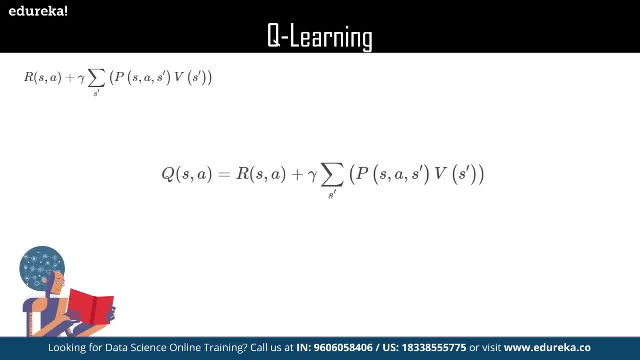 So let's utilize this fact and replace V of S dash as a function of Q. So Q S comma A becomes R of S comma A, plus gamma of summation P, S A S dash and maximum of the Q S dash A dash. So the equation of V is now turned into an equation of Q. 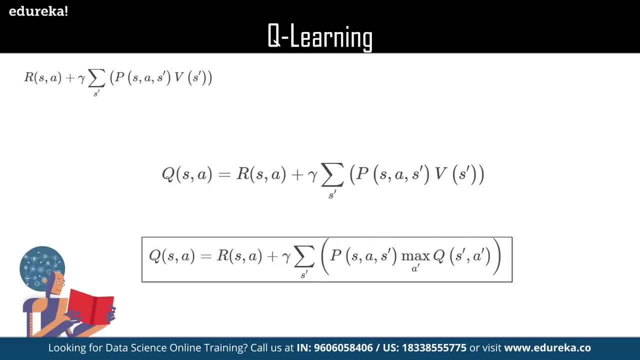 which is the quality. But why would we do that Now? this is done to ease our calculations, because now we have only one function, Q, which is also the core of the dynamic programming language. We have only one function, Q to calculate, and R of S comma A. 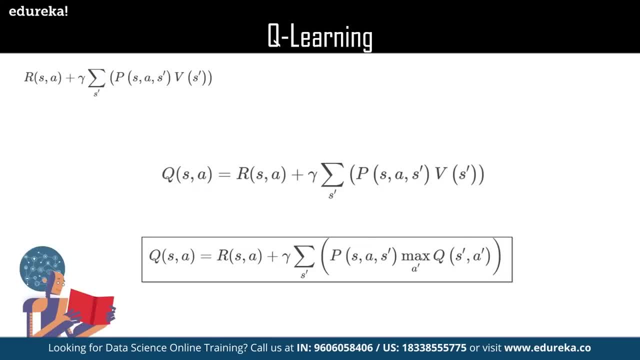 is a quantified metric which produces reward of moving to a certain state. Now the qualities of the actions are called the Q values and from now on we will refer to the value footprints as the Q values. An important piece of the puzzle Is the temporal difference. 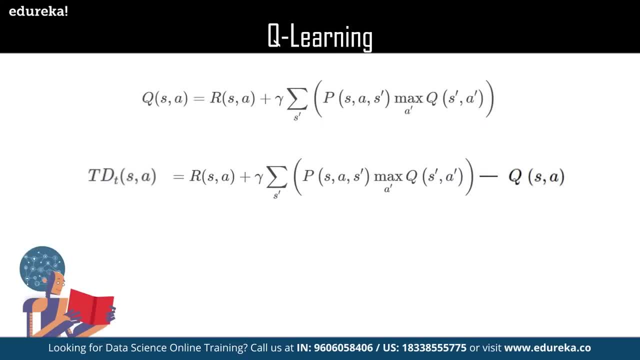 Now, temporal difference is the component that will help the robot calculate the Q values with respect to the changes in the environment over time. So consider: our robot is currently in the mark state and it wants to move to the upper state. One thing to note that here is that the robot already knows. 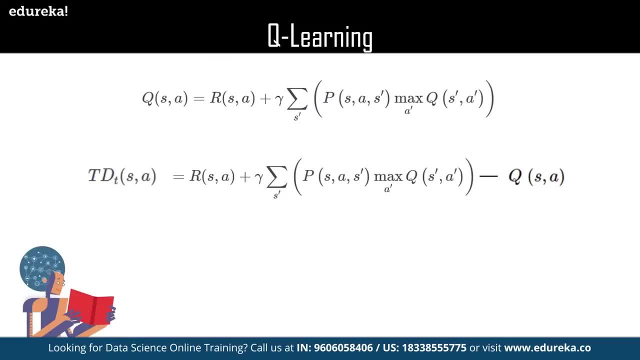 the Q value of making the action that is, moving to the upper state, and we know that the environment is stochastic in nature- and the reward that the robot will get after moving to the upper state. So the new Q will be different from an earlier observation. 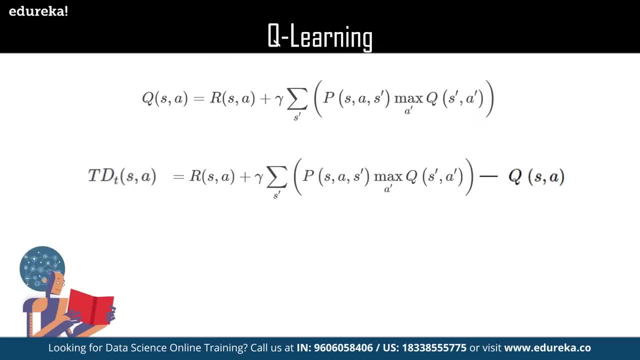 So how do we capture this change, the real difference? We calculate the new Q S comma A with the same formula and subtract the previously known Q S A from it. So this will in turn give us the new Q A. Now the equation that we just derived gives the temporal difference. 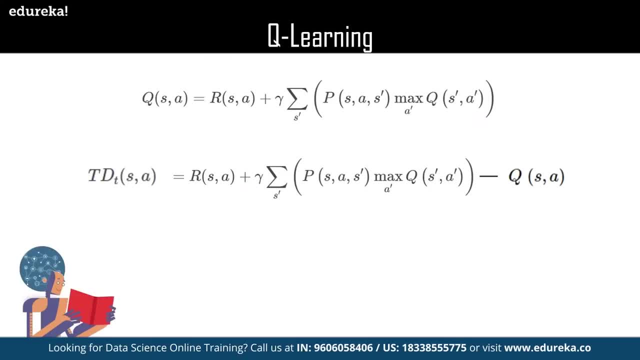 in the Q values, which further helps to capture the random changes in the environment which may impose. Now the new Q S comma A is updated as the following: So Q T of S comma A is equal to Q T minus 1 S comma A plus alpha. 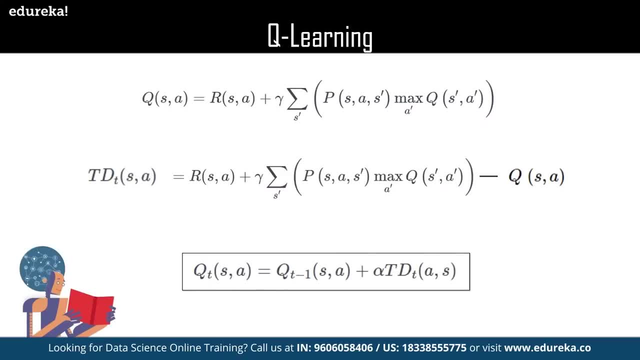 T D T of A comma S. Now here, alpha is the learning rate, which controls how quickly the robot adapts to the random changes imposed by the environment. The Q T S comma A is the current state Q value and the Q T minus 1 S comma A is the previously recorded Q value. 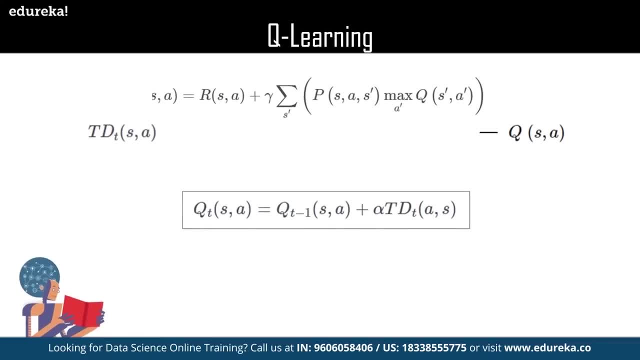 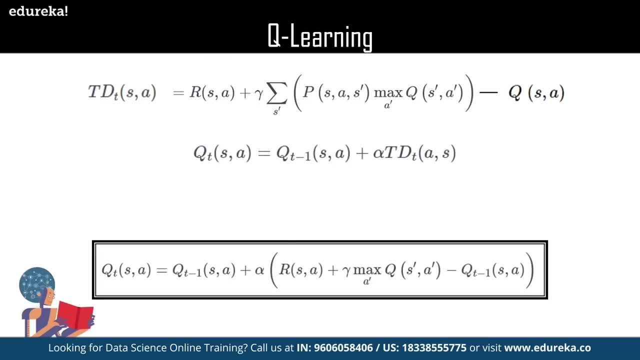 So if you replace the T D S comma A with its full form Equation, we should get: Q T of S comma A is equal to Q T minus 1 of S comma A plus alpha into R of S comma A plus gamma. maximum of Q S dash A, dash minus Q T minus 1 S comma A. 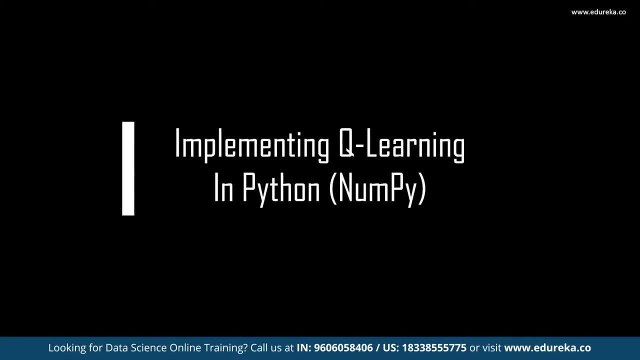 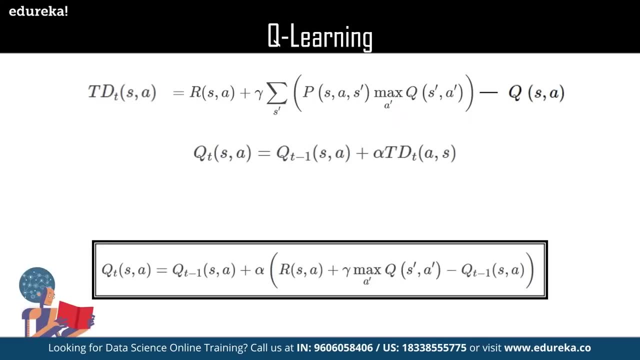 Now that we have all the little pieces of Q learning together, Let's move forward to its implementation part. Now, this is the final equation of Q learning, right? So let's see how we can implement this and obtain The best path for any robot to take now to implement the algorithm. 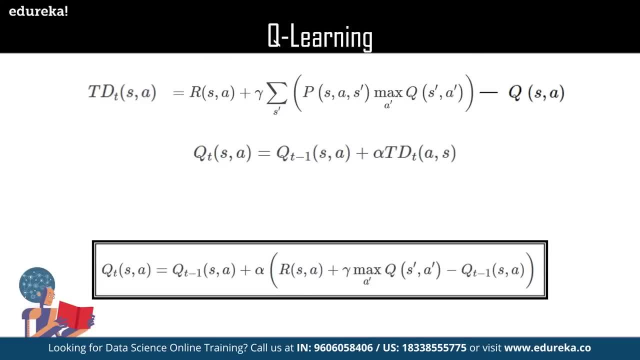 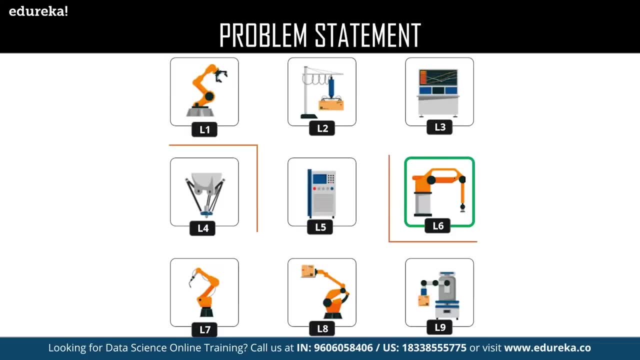 We need to understand the warehouse location and how that can be mapped to different states. So let's start by recollecting the sample environment. So, as you can see, here we have L1, L2, L3 to L9 and, as you can, 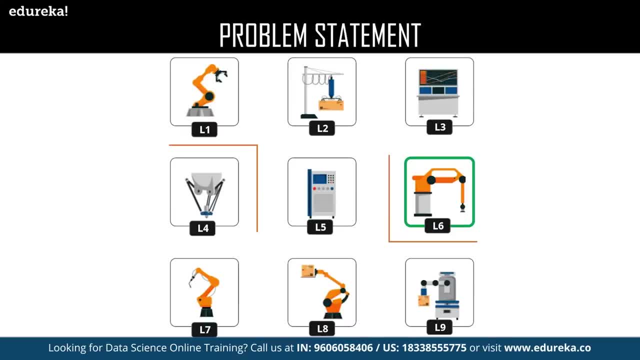 see, here we have certain borders also. So first of all, let's map each of the above locations in the warehouse to numbers or the states, so that it will ease our calculations, right. So what I'm going to do is create a new python3 file in the 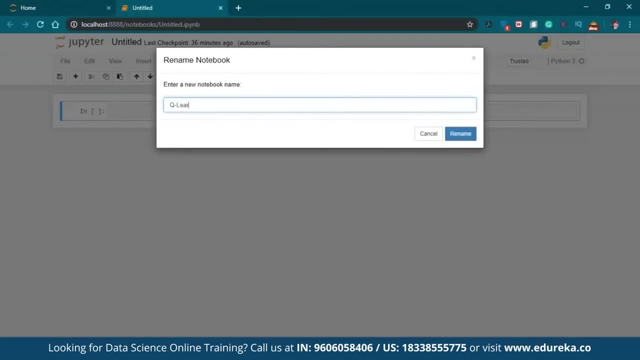 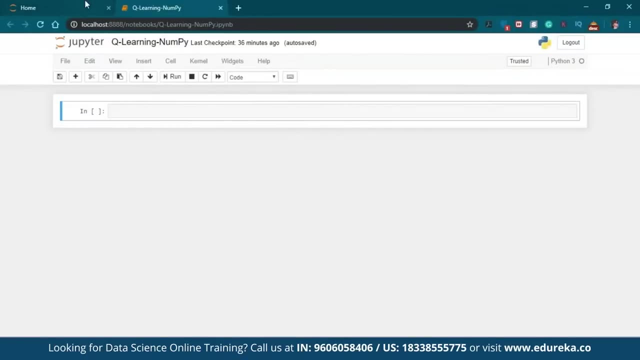 Jupyter notebook, and I'll name it as Q learning NumPy. Okay, so let's define the states, But before that, what we need to do is import NumPy, because we're going to use NumPy for this purpose, and let's initialize the. 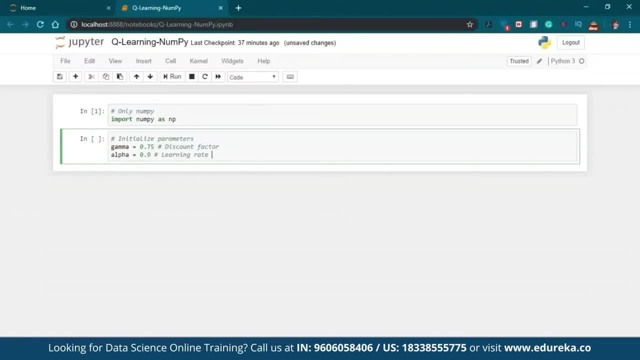 parameters, that is, the gamma and alpha parameters. So gamma is 0.75,, which is the discount Factor, whereas alpha is 0.9,, which is the learning rate. And that's what we're going to do: is define the states and map. 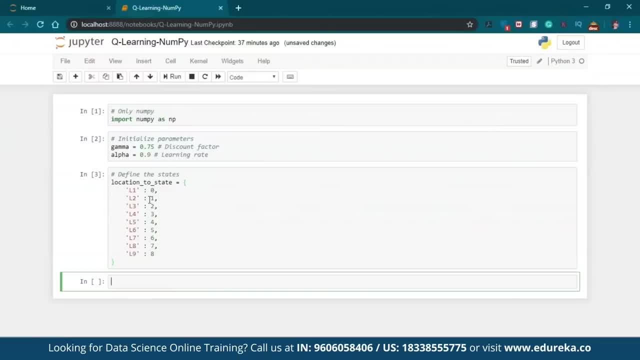 it to numbers. So, as I mentioned earlier, L1 is 0 and till L9, we have defined the states in the numerical form. Now the next step is to define the actions, which is, as mentioned above, represent the transition to the next state. 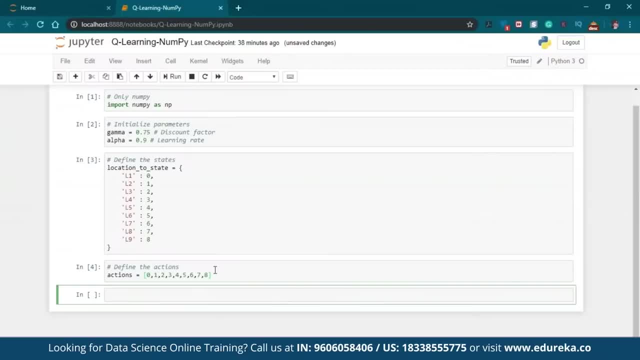 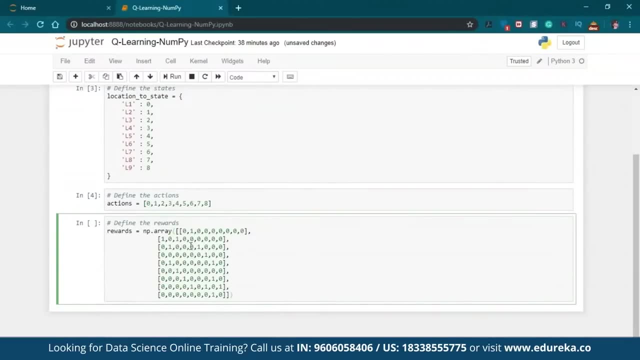 So, as you can see, here we have an array of actions from 0 to 8.. Now what we're going to do is define the reward Table. So, as you can see, it's the same Matrix that we created just now. that has showed you just now. 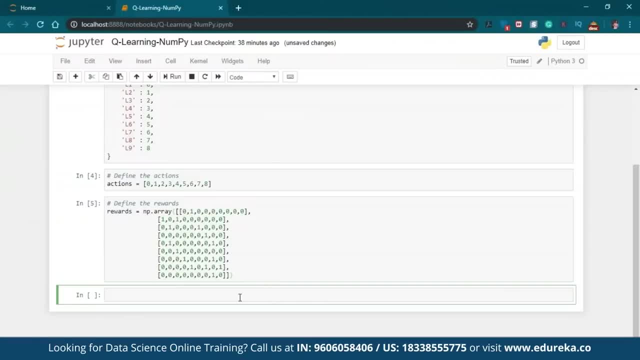 Now, if you understood it correctly, there isn't any real barrier limitation as depicted in the image. For example, the transition L4 to L1 is allowed, but the reward will be 0. to discourage that path or in tough situation, What we do is add a minus on there so that it gets a negative. 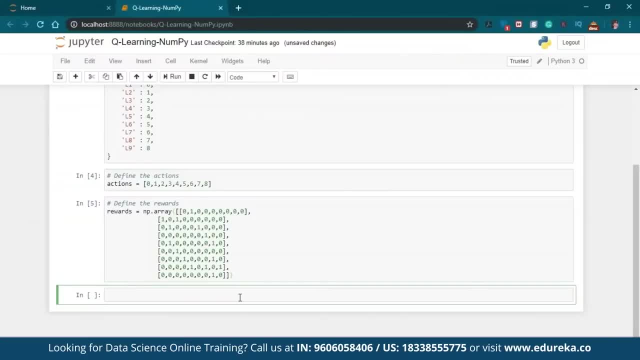 reward. Now, in the above code snippet, as you can see, We took each of the states and put once in the respective state that are directly reachable from the certain state. Now, if you refer to that reward table once again what we created. 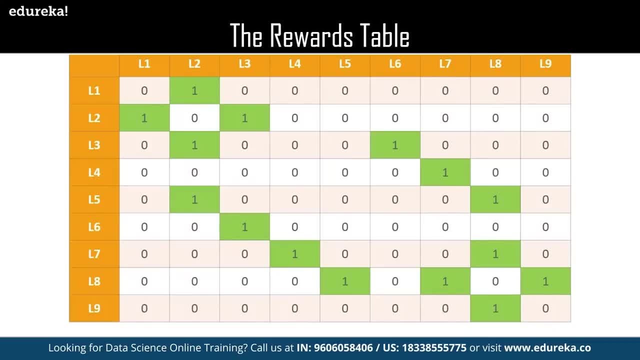 the above array construction will be easy to understand. But one thing to note here is that we did not consider the top priority location L6 yet. We would also need an inverse mapping from the states back to its original location, and it will be cleaner when we reach to the utter. 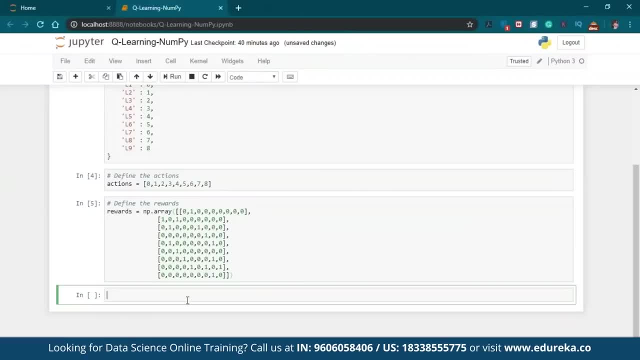 depths of the algorithms. So for that we need to add a minus on that. What we're going to do is have the inverse map, location, state to location. We will take the distinct state and location and convert it back. Now what we'll do is: we'll not define a function, get optimal. 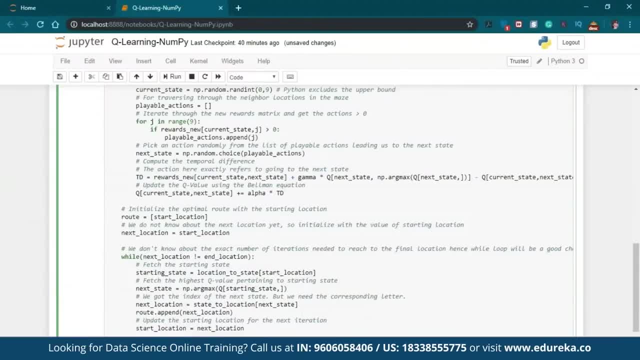 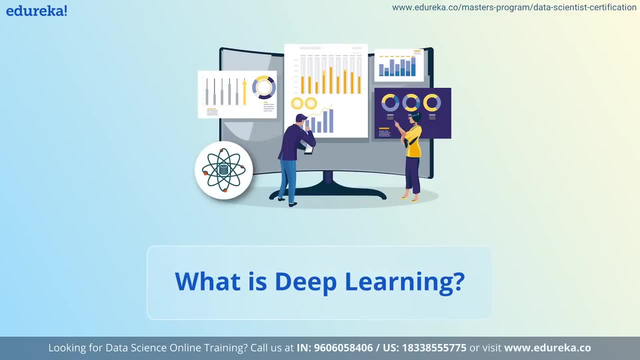 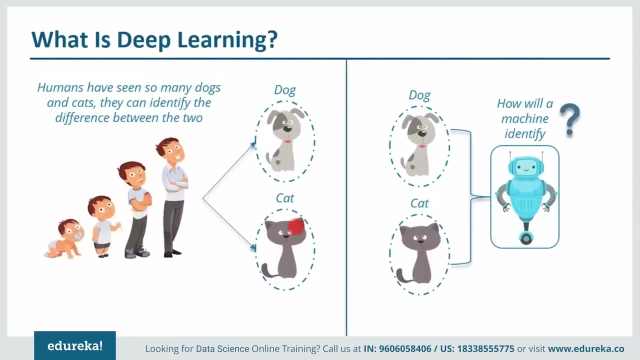 which is to get optimal route, which will have a start location and an end location. So, guys, let us understand deep learning with an analogy. So how do you think our brain is able to identify the difference between a dog and a cat? 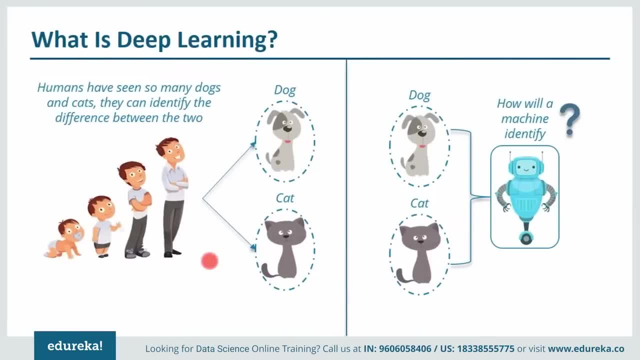 The reason is, since the day we are born, we are actually seeing different types of cats and dogs in our day-to-day life And because of that we are able to identify the difference or spot the difference between the two, that is, dog and a cat. 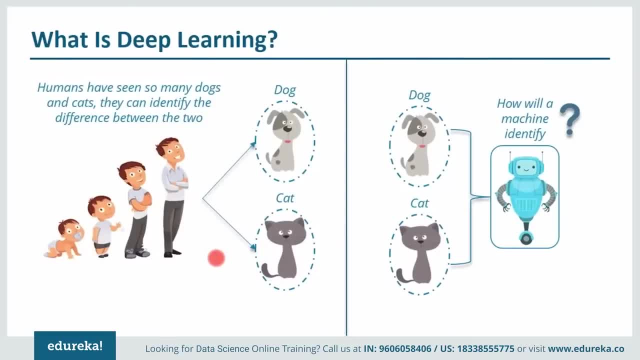 Even if we see different types of cats and dogs, we still know which is a cat and which is a dog. So this is because we have seen a lot of cats and dogs in our entire life. But what if I want a machine to do that task for me? 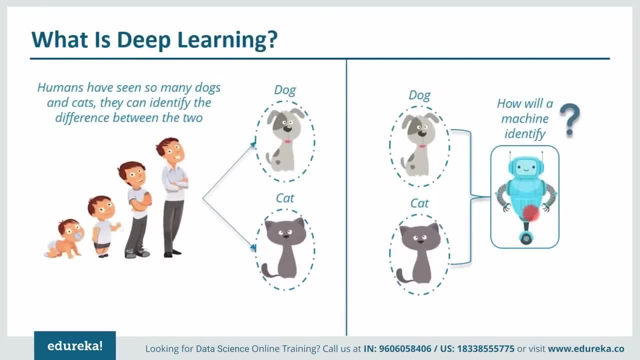 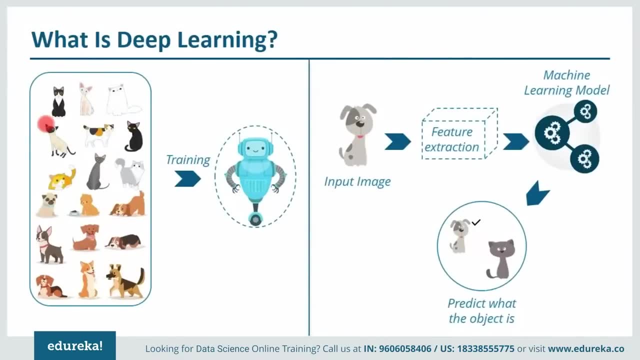 So how will a machine identify whether the given Image is of a dog or a cat? So one way of doing that is we can train our machine to a lot of images, or a lot of images of different cats and dogs, that is, different breeds of cats and dogs. 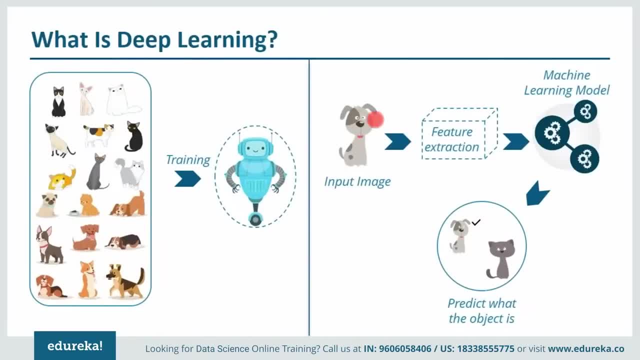 And then what will happen once our training is done? we can provide it with an input image. then we'll manually extract certain features, features like nose, whiskers, colors, edges- It can be anything- The important features, which actually helps us in classifying whether. 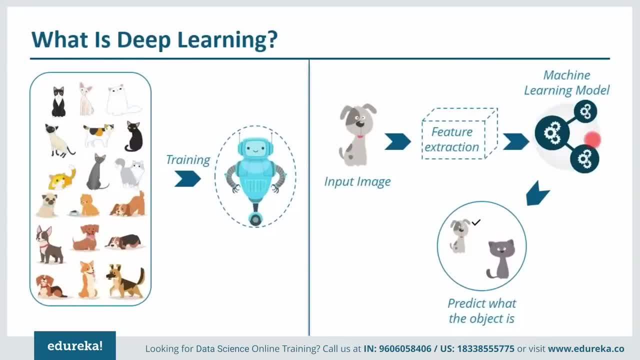 the input Image is a cat or a dog, Then we make a machine learning model with that and once it is done, our machine learning model is able to predict whether the input image is of a cat or a dog. But if you notice here, one very big disadvantage with this is we have 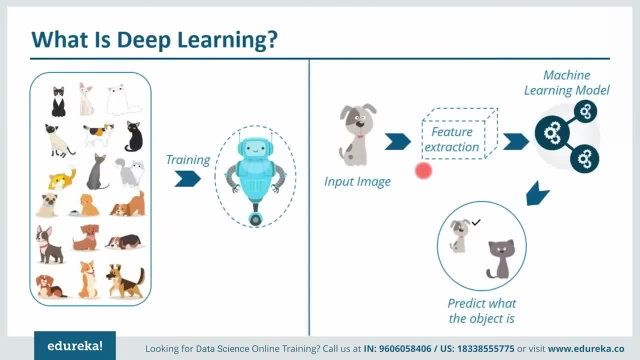 to manually extract features, features such as nose whiskers, all those features. We have to manually extract it and provide it to our machine learning model. and trust me guys, in every scenario It is not possible. if you have large number of inputs, You cannot do that. 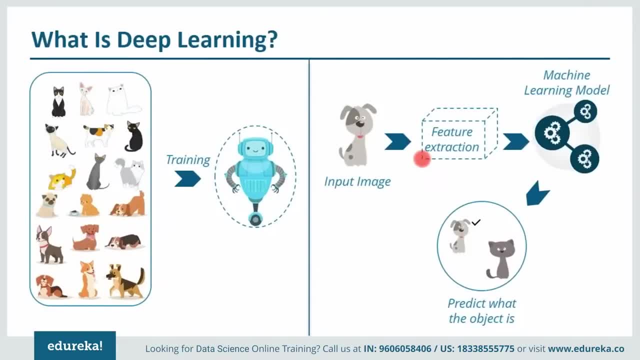 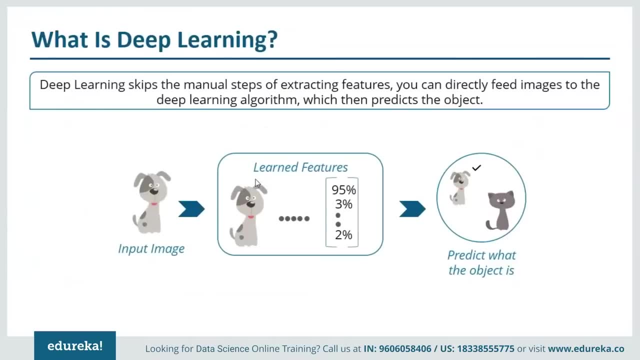 You cannot manually extract the features or basically, you can say columns which are important for you in order to predict what the object is right, and that led to the evolution of deep learning. So what happens in deep learning? We skip the manual step of feature extraction. 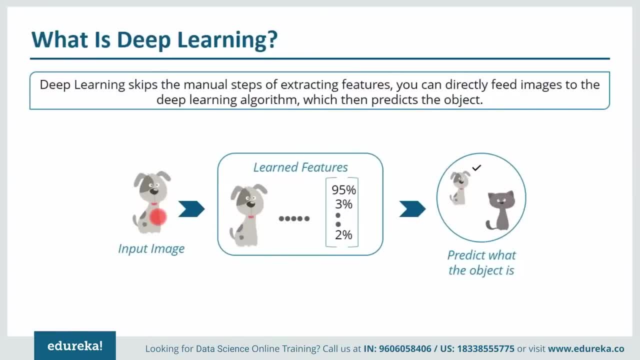 So what we do? we directly take the input image and feed it to our deep learning algorithm, and because of that, what happens? whatever features are we already manually provided. apart from that, there might be many other features which are important, For example, if our features don't include the length of the neck, and that is one of 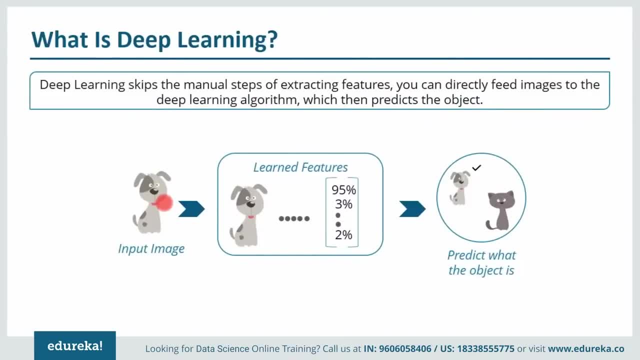 the major feature in order to identify or classify whether it is a cat or a dog. now what will happen? our algorithm will automatically determine that feature and will take into consideration, and then it will classify whether the input image is a cat or a dog. So what happens here? 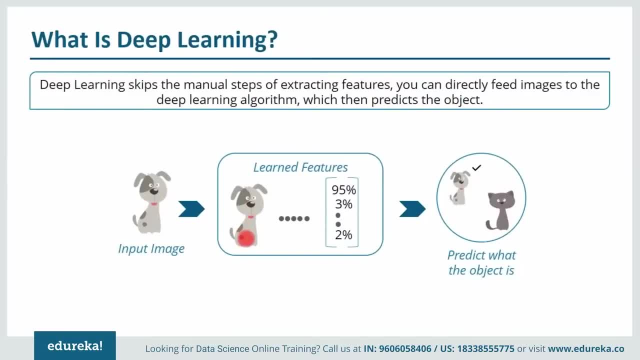 We provide an input image of a dog and then it will automatically learn certain features, Even if you don't provide it with those features, and after that it will give us the probability and according to this particular scenario, It says: 95% chances of being a dog, 3% chances of some other animals. 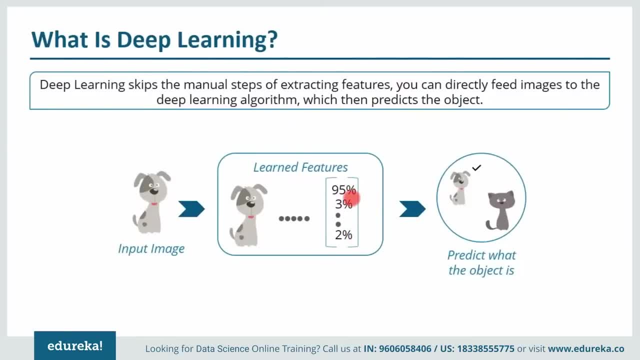 similarly 2% chances of some other animals. So, since the highest probability goes with the dog, so the prediction says that the object or the input image is nothing but a dog. fine guys, So we'll move forward and we'll understand how exactly deep learning. 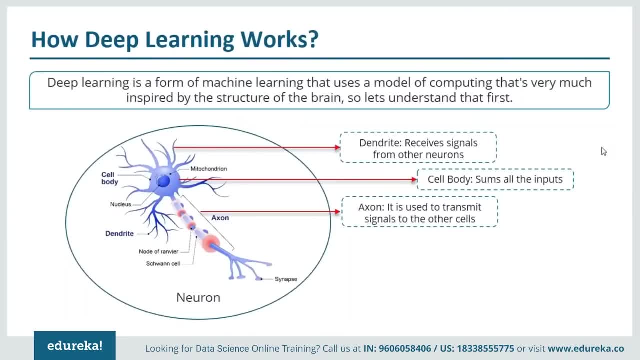 works. So the motivation behind deep learning is nothing but the human brain, as we have seen in the previous analogy as well What we are trying to do. We are trying to mimic the human brain, We are trying to mimic the way we think. 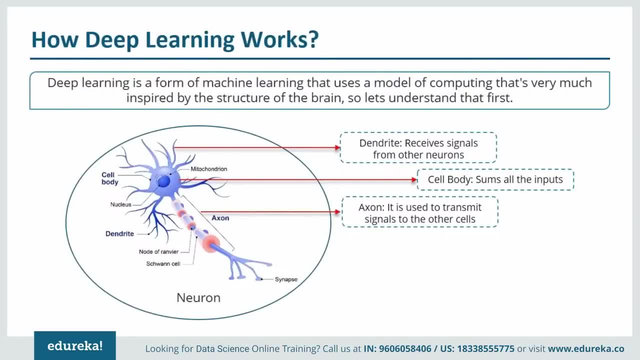 The way we take decisions, the way we solve problems. We are trying to make sure that we have a system that can mimic our own brain. So obviously the motivation for deep learning has to be our brain and how our brain work with the help of our brain cells. 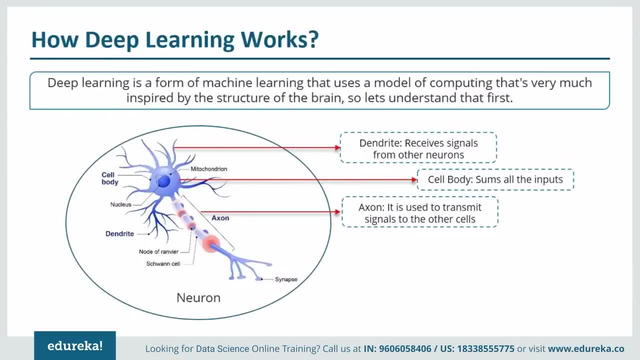 which we call neuron. Now let us understand how a neuron works and let me tell you, guys, This is what we think how a neuron works. This is what our studies tell us. So yeah, so these are called dendrites. So dendrites receive signals from other neurons and then it passes. 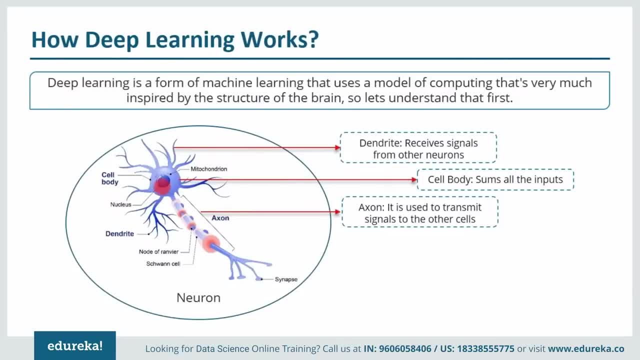 those signals to the cell body. Now, this cell body is where we perform Certain function. It can be a Sigma function. That's what we believe. We believe it performs Sigma function. that is nothing but sums all the inputs. then, through Exxon, what happens? these signals are: 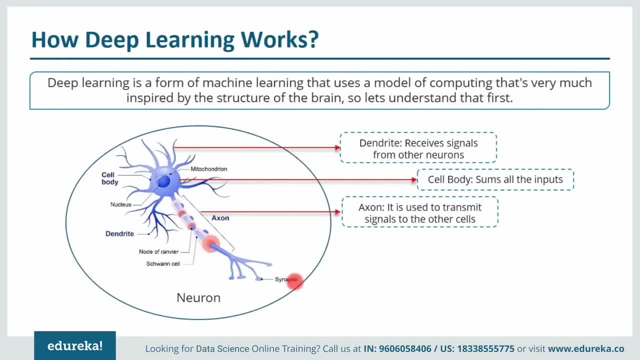 fired to the next neuron, and the next neuron is present at some distance, and that distance is nothing but synapse. So it fires only when the signals coming from the cell body exceeds a particular limit. then only the cell or this neuron will fire the signals to the next neuron. and this is how the neuron at the brain 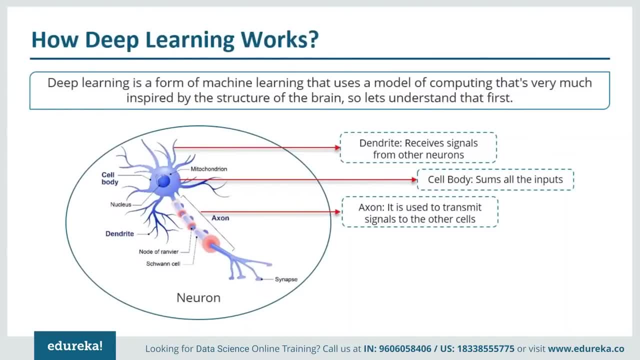 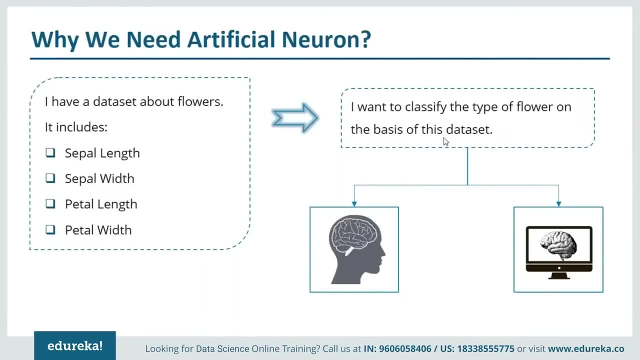 cell works And we take the same process forward and we try to create artificial neurons. So let us understand why we need artificial neurons. with an example. So I have a data set of flowers, say, and that data set includes sepal length, sepal width, petal length and petal width. 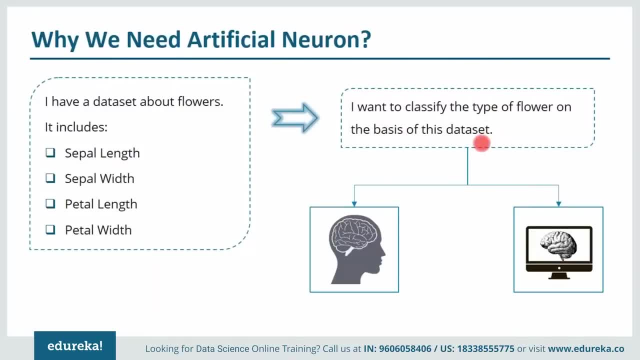 Now what I want to do. I want to classify the type of flower on the basis of this data set. Now there are two options: either I can do it manually- I can look at the flower manually and determine by its color- or any means, and I can. 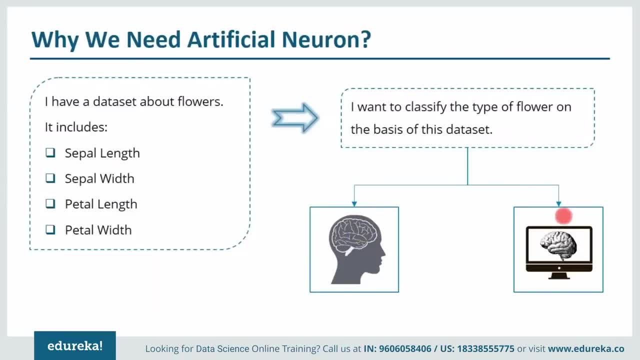 identify what sort of a flower It is, or I can train a machine to do that. Now let me tell you the problem with doing this process manually. First of all, there might be millions of inputs that will be given to you and for a human brain to perform. that particular task is next to. 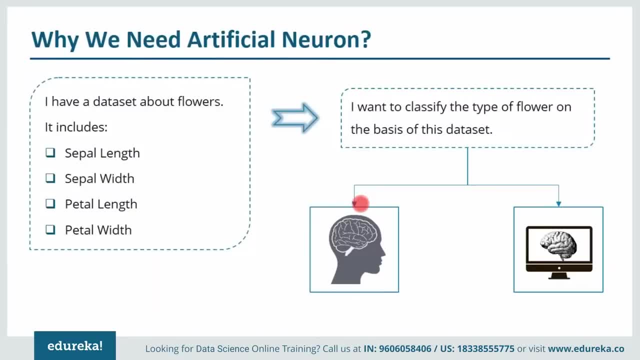 impossible. and at the same time, we always get tired at some point of time, right, So we cannot just continue working for a long period of time in single stretch. and the third point is human error risk, which is always there. So these are a few limitations with the human brain. 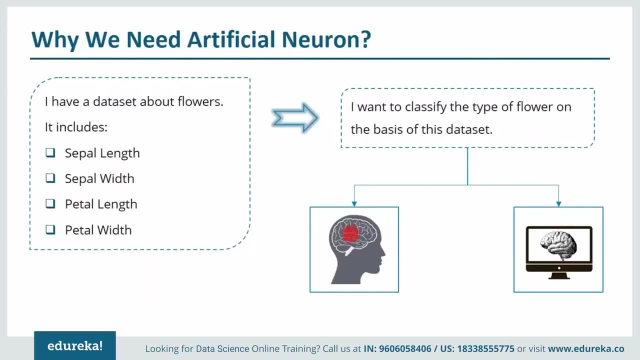 So what we can do: we can train a machine to do That task for us, or we can put our brain inside a machine so that it can classify the flowers for us. So with this, what will happen? the machine will never get tired and and will make better predictions as well. 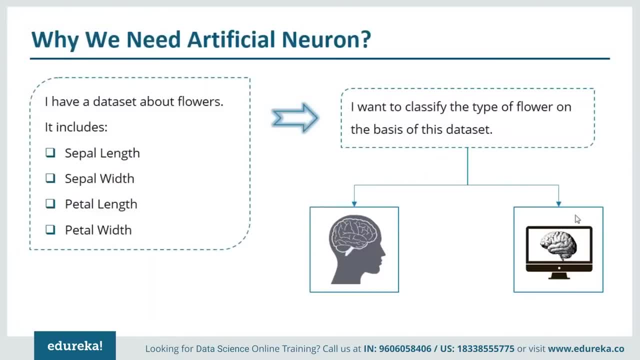 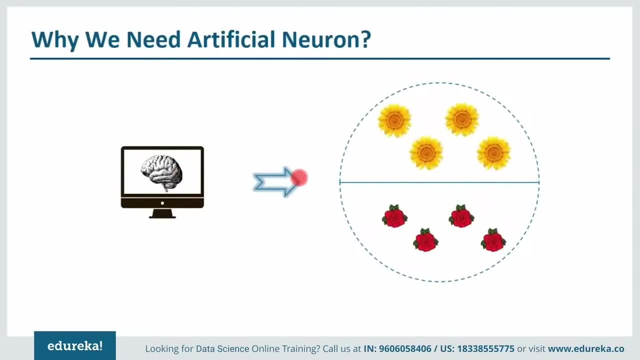 So this is why we create artificial neurons, so that there's a system present that can mimic our brain, and this is what exactly happens. So this particular artificial neuron can actually classify the flowers, or you can say, can divide the flowers on the basis of certain features. 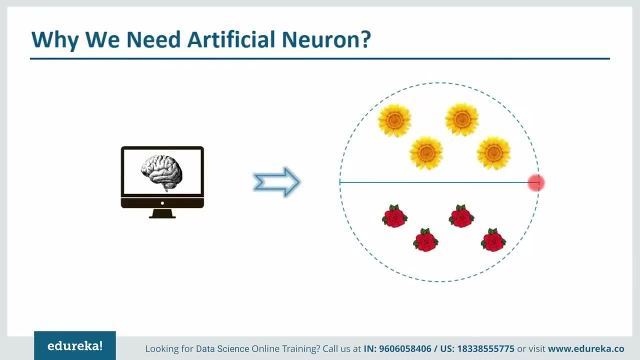 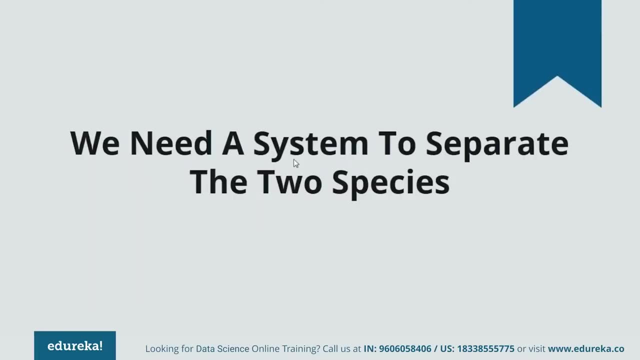 in our case It is separate length, separate width, petal length And petal width, so on that basis it can classify the two flowers. So what we need here, we need some sort of a system that can actually separate the two species. and what is that system is nothing but an. 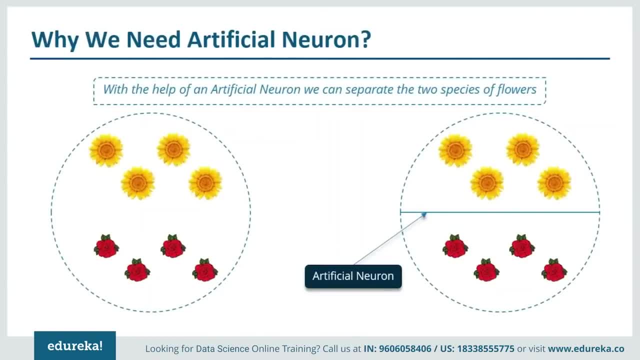 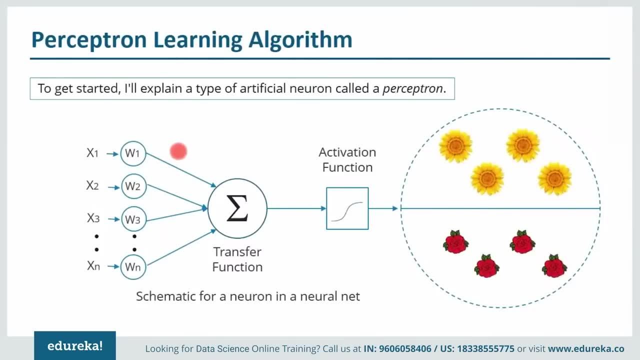 artificial neuron. So we need artificial neuron and one type of artificial neuron is a perception. Now let me explain you perception with the flow diagram that is there in front of your screen. Now, over here, what happens? we have set of inputs like x1, x2, dash, dash, dash. 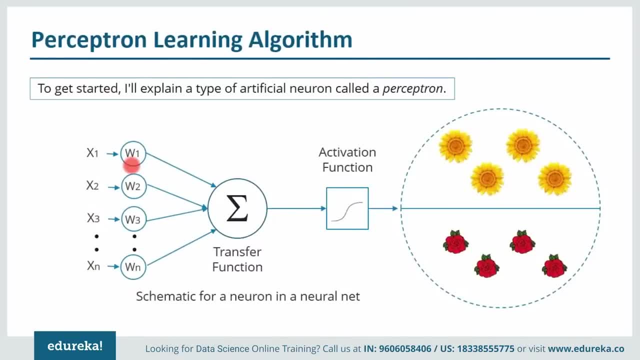 till xn. Now these inputs will be multiplied with their corresponding weights, which is w1, w2, w3 till wn in our case. Now these weights actually define how important our input is. So the value of weight is high. We know that this particular input is very, very important for us. after, 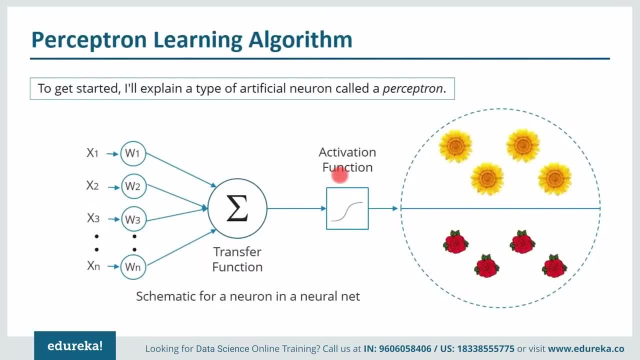 multiplication. All of these are sum together and then it is fed to an activation function. Now, the reason of using activation function is to provide a threshold value. So if our signal is above that threshold value, a neuron- or you can say our perceptron- will fire, else it won't fire. 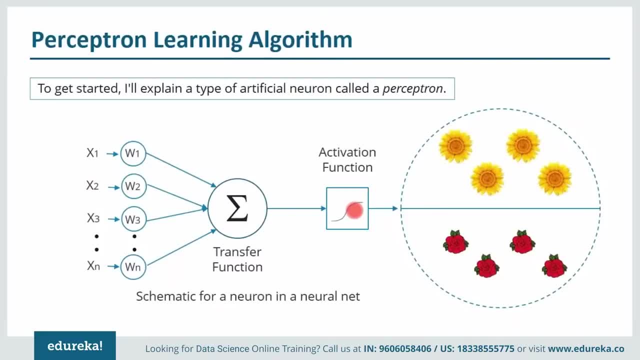 So that is the reason Why we use an activation function. There can be different types of activation function. that can be sigmoid, They can be step function, sign function, depending on our use case. We define the activation function Now. the main idea was to define an algorithm in order to learn the values. 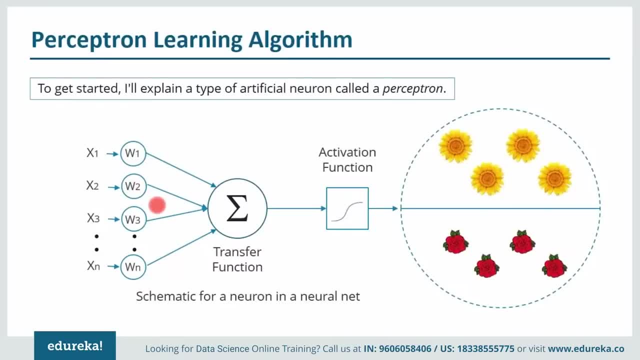 of the weights, which are w1, w2, w3 in our case, to learn the values of the weights that are then multiplied with the input features in order to make a decision whether a neuron fires or not, in context of pattern classification, which is in our case. 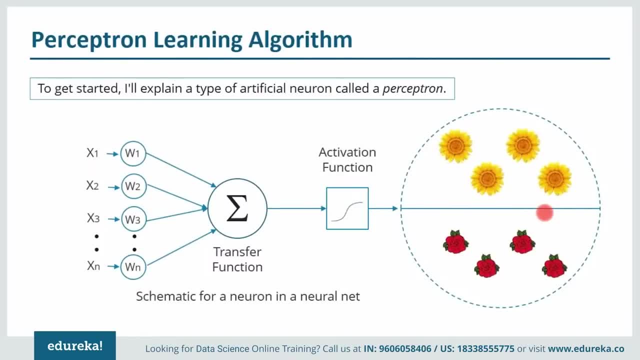 Flowers. so we are trying to classify the two species of flowers. such an algorithm could be useful to determine if a sample belongs to one class or one type of a species, or another class or another type of the flower. We can even call perceptron as a single layer binary linear classifier, to be. 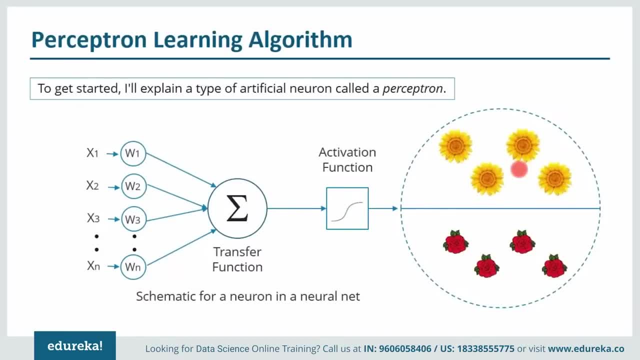 more specific, because it is able to classify inputs which are linearly separable, and our main task here is to predict to which of the two possible categories a certain data point belongs, Based on a set of input variables. Now there's an algorithm on which it works. 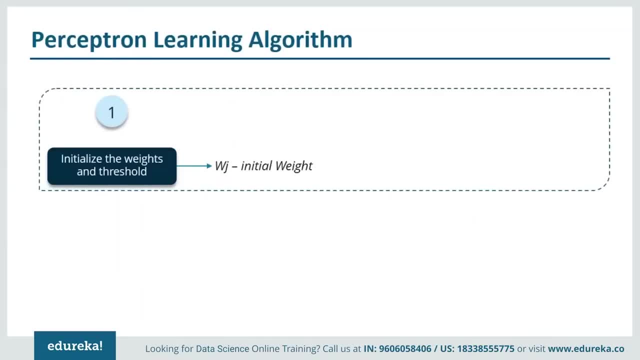 So let me explain you that. so the first thing we do is we initialize the weights and the threshold. now, these weights can actually be a small number or a random number, and it can even be zero, So it depends on the use case that we have. then what we do: we provide the input. 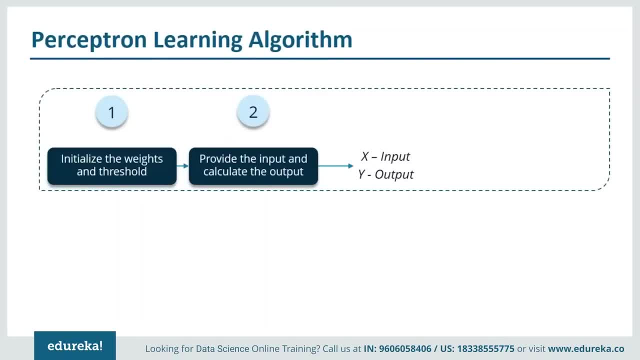 and then we calculate the output. now, when we are training our model or we are training our artificial neuron, We have the output values for a particular set of inputs. So we know the output value. but what we do, We give the input and we see what will be the output of our particular neuron. 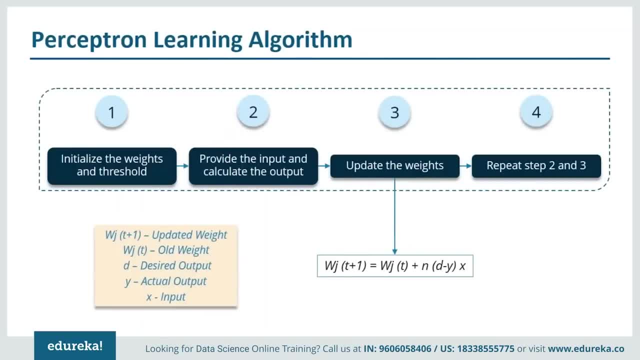 and, accordingly, we need to update the weights in order to reduce the loss, or you can say, in order to reduce the difference between the actual output and the desired output. So what happens? Let me tell you that. so we need to update the weight. So how we are going to update the weight is, we can say: the new weight is equal. 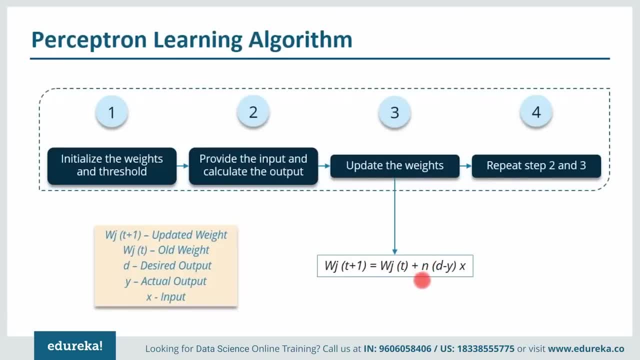 to the old weight plus the learning rate. learning rate will discuss about it later in the session, But generally we choose learning rate somewhere between 0.5 to 0.01.. After that, what happens? we find the difference between the desired output and the actual output, and then we multiply it with the input. 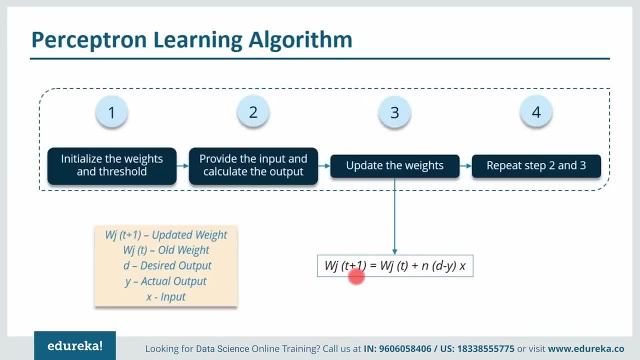 So on that basis, we get a new weight. So this is how we update the weights and then what happens? we repeat the steps two and three. So we are going to repeat the steps two and three, that is, we are going to apply this new weight again. 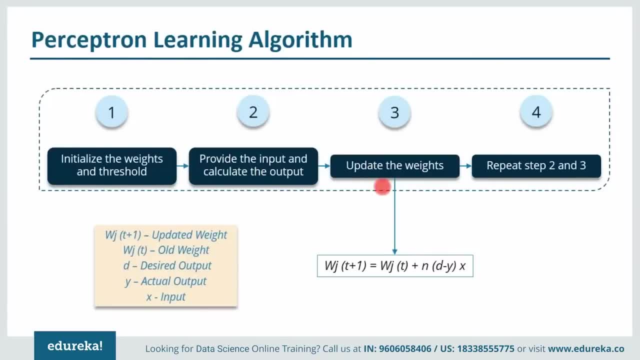 We are going to calculate the output again, We are going to compare it with the desired output and if it matches, then it's fine. Otherwise we are going to update it again. So this is how the whole perceptron learning algorithm works. fine, So we'll move forward and we'll see the various types of activation functions. 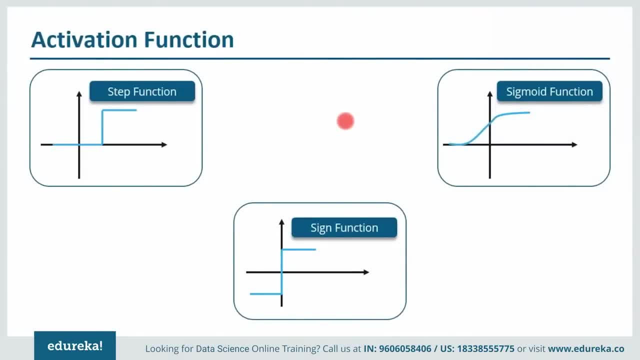 So these are the various types of activation functions that we use, Although there can be many more activation functions. again I'm telling it depends on your use case. So we have a step function. So if our output is actually above this particular value, then only a neuron. 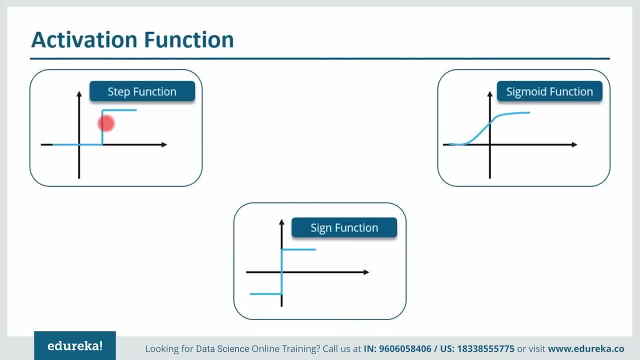 will fire, or you can say the output will be plus one, or if it's less than this particular value, then we'll have no output, or we'll say zero output. similarly for the sigmoid function as well, and same goes for sine function. So let us move forward and we'll focus on various applications of this perceptron. 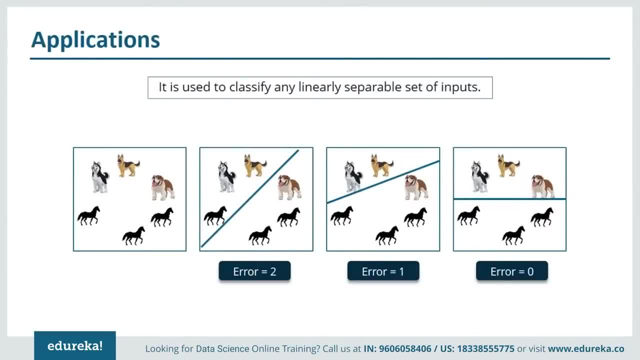 Now, as I've told you earlier as well, it can be used to classify any linearly separable set of inputs. Now let me explain to you with the diagram that is there in front of your screen. So we have different types of dogs and we have horses and we want a line that 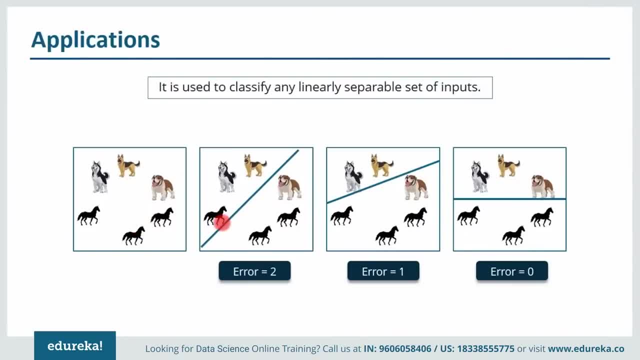 can separate these two. So our first iteration will produce this sort of a line. but here we can notice that we have error here, as we have classified horse one of the horses- as a dog and a dog As a horse. So error is two here. 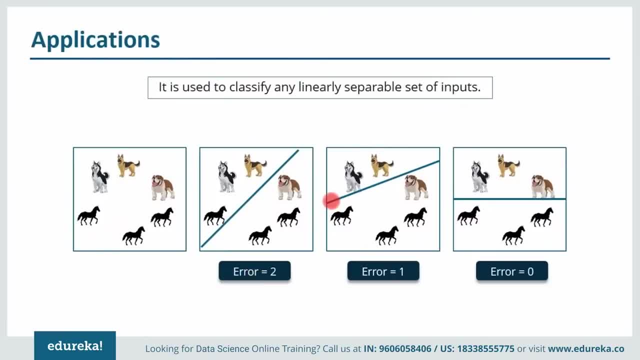 Similarly, we now what happens. we have updated the weights. now, after updating the weight, what happens? our error has reduced. So what happens now? We have actually classified all the horses correctly, but one dog we have classified wrong and we have considered it as a horse. 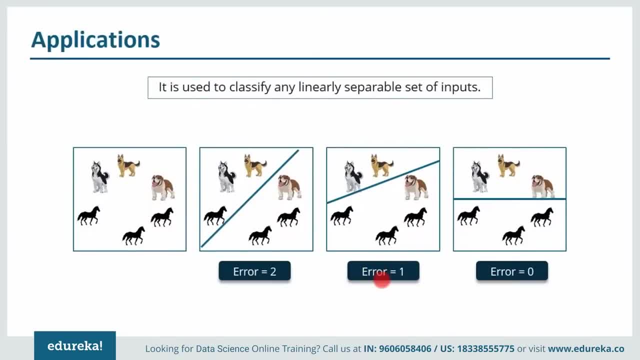 So our error becomes one once again. what will happen? if you can remember, the step two and three of a perceptron learning algorithm will be done, and then, after that, our weights will be updated and our desired output will become equal to our actual output and we get a. 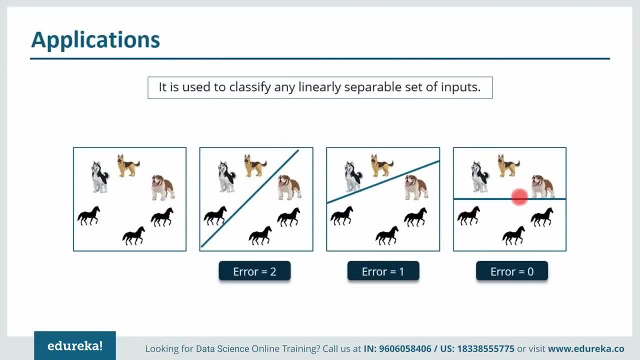 line Something like this: So what we have now? we have properly classified dogs and horses, So this line separates both of them. This is how we can actually use a single layer perceptron in order to classify any linearly separable set of inputs. 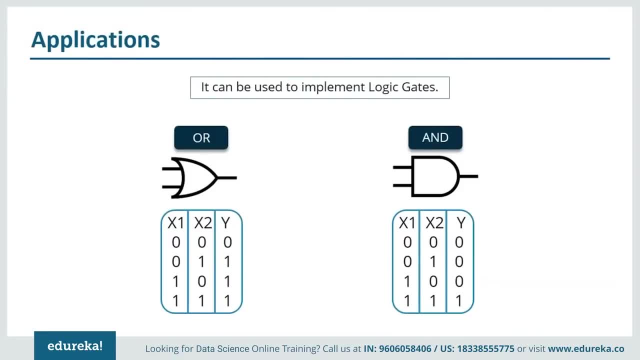 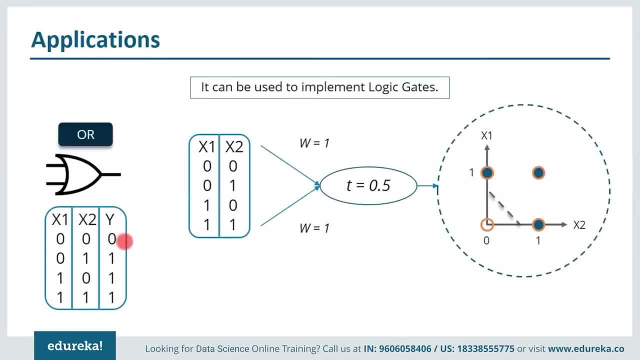 Now we can even use it in order to implement a logic. gates, that is, or, and, and. now let me tell you how you can do that. first, We'll look at our gate. now, in our gate, What happens here is the truth table, truth table. 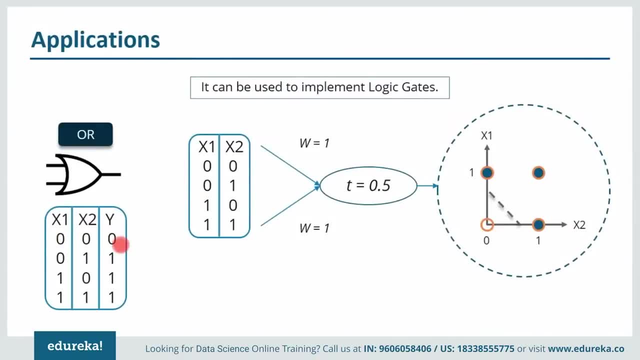 According to that, we have two inputs, x1 and x2.. So if both are zero, we get a zero. if any one of the input is high, or any one of the input is one, we get the output as one. So what we need to do is we need to make sure that our weights are present in 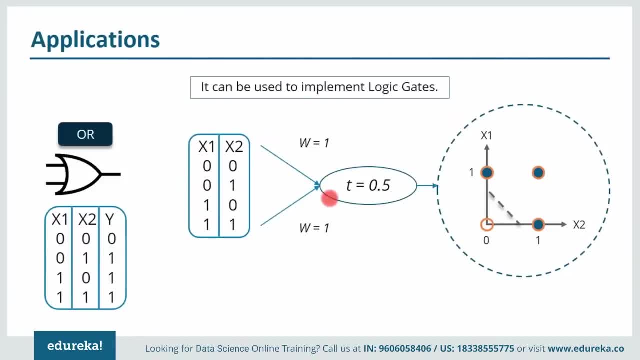 such a way that we get the same output. So how we have done that, when the value of weight is equal to one, and then we provide the input x1 and x2, after passing through this activation function, we get this sort of a graph, which is the graph for our order: a gate. 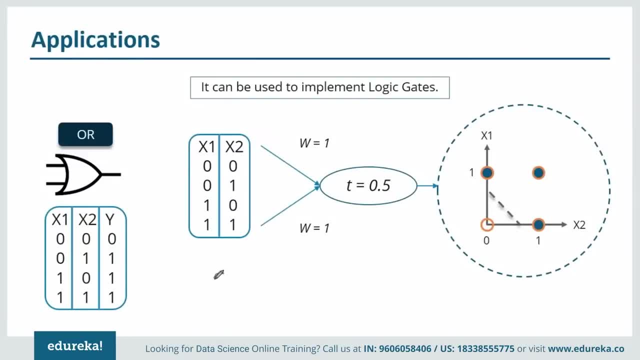 Now we have x1 and x2 as inputs, So we provide first input as zero, x1, and this also has zero. So 0 into 0 is again 0, 0 into 0 is 0, and then we passes through this activation function. 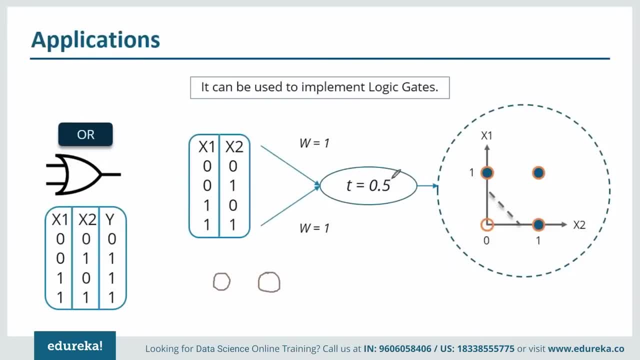 Now we need to make sure that whatever value that comes here should be greater than 0.5. Then only our neuron, or the perception, will fire, But since this value is actually less than 0.5. So the neuron won't fire and our output will be 0, as you can see it over here. 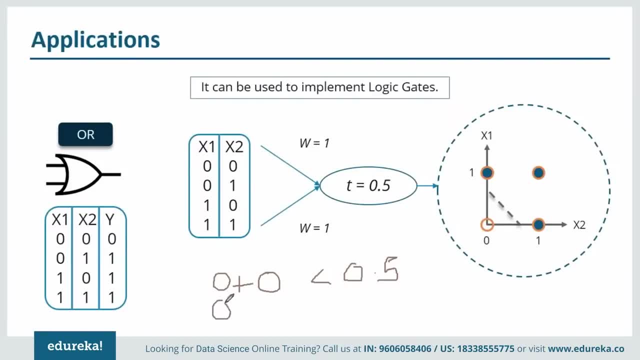 Now let's take the other set of inputs. Now our x1 is 0.. And our x2 is 1.. So 1 into 1 will what will be obviously 1.. Now, in this case, our output is bigger than 0.5.. 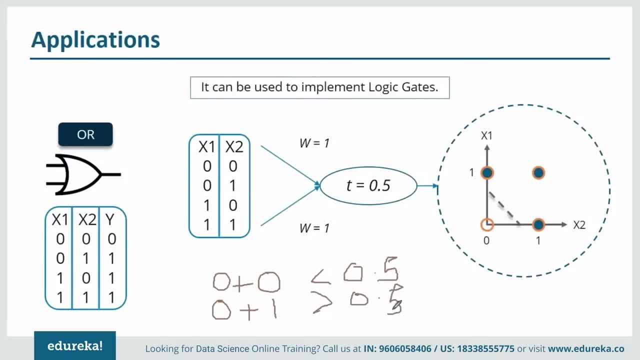 Then what will happen? our neuron will fire and we'll get 1, the output 1 here, as you can see it in the graph. Similarly, when my x1 is 1 and x2 is 0, in that case also, our output is greater than 0.5- our neuron will fire. 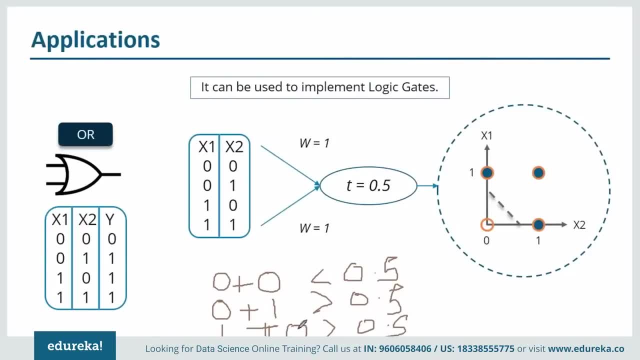 and we'll get this sort of a graph when I talk about 1- 1.. Then our output Will be 2, which is greater than 0.5.. So we get an output that is 1, and this is how we get the graph. 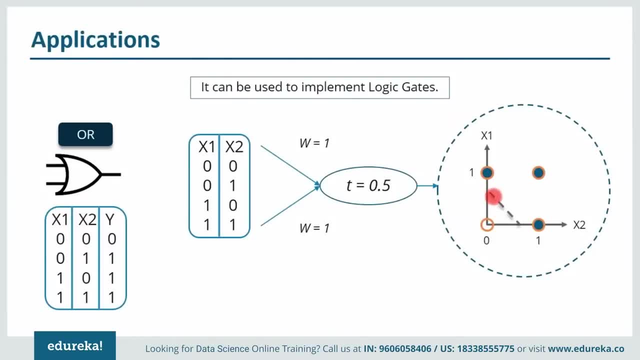 And now, if you notice, with the help of the single-layer perceptron, we are able to classify the ones and zeros. So this line, anything above this line, is actually 1 and anything below this line We have zeros. So this is how we are able to classify, or able to implement or gate. 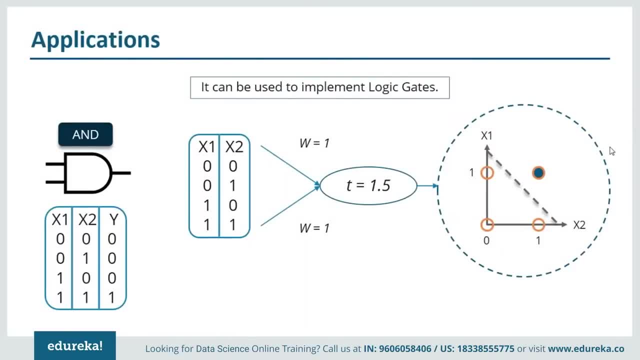 Similarly when I talk about and gate as well. So there's a difference in the truth table of and gate in and gate what happens. we need to make sure that both of our neurons will fire. So this is how we are able to classify, or able to implement or gate. 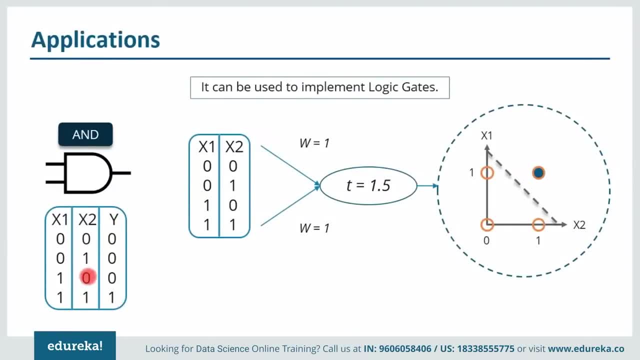 So that both of our inputs are high in order to get a high out. If any of the input is low, we get a low output, And that's the reason we choose an activation function that is 1.5,, which means that if our value or the output is about 1.5,. 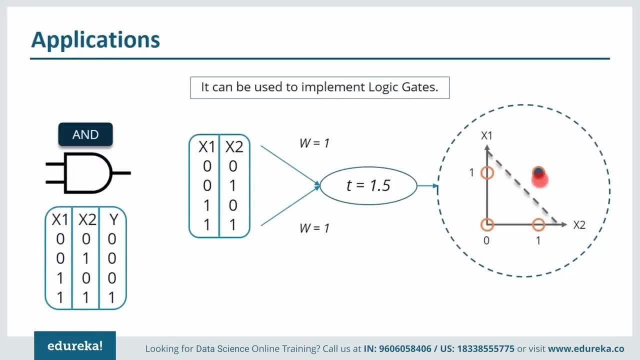 then only our neuron will fire and we'll get one here. And there's only one case, that is when both the inputs are high. So when both the inputs are I. so x1 is 1, x2 is 1, we get something which is 2, which is obviously greater than 0.5.. 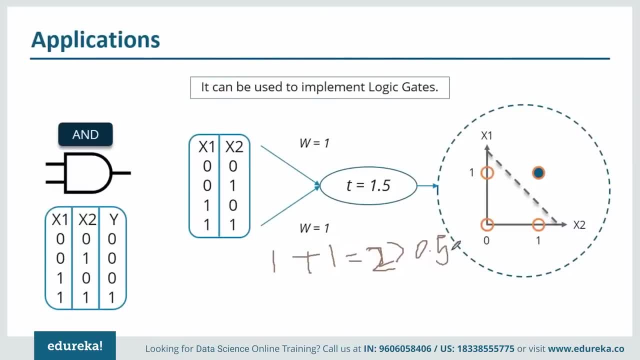 This is how it is. So 1 plus 1, 2, which is obviously greater than 0.5.. So what we get we are neuron fires and we get one here, but for the rest of the inputs, all will be less than 1.5.. 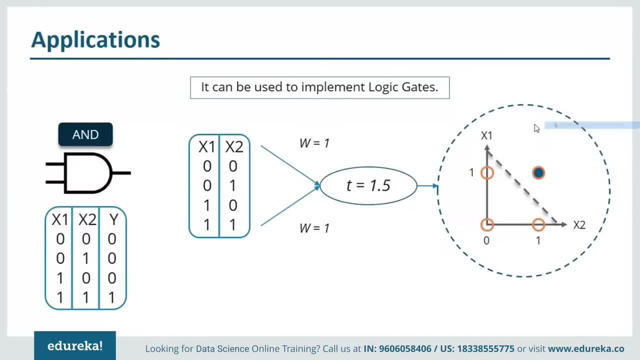 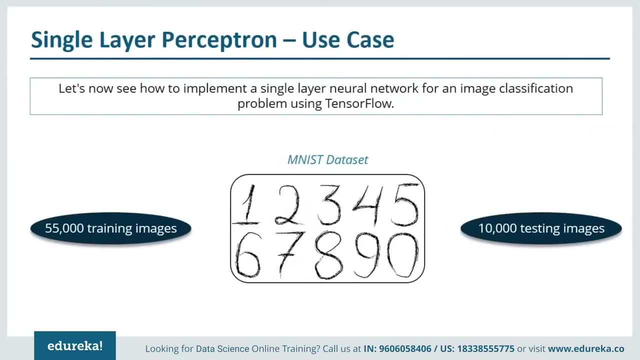 So that is why our neuron doesn't fire and we get a 0 output. This is how we can implement and and or gate. So let's move forward, guys, and we'll actually understand a use case, that is, of MNIST data set. The reason for using MNIST data set is because it is already clean and will be a perfect example for this. 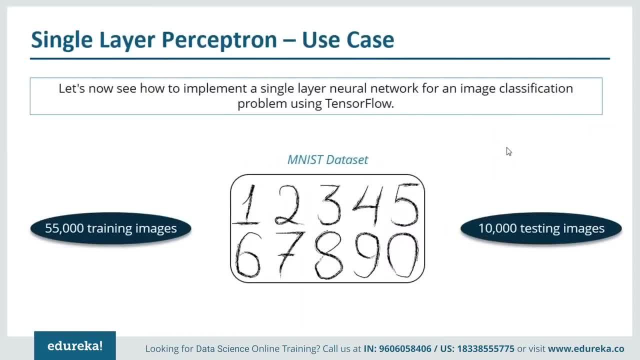 Now what this MNIST data set contains. It basically contains handwritten digits from 0 to 9, and in that data set we have 50,000 training images along with 10,000 testing images. So we will train our model with those 55,000 training images. 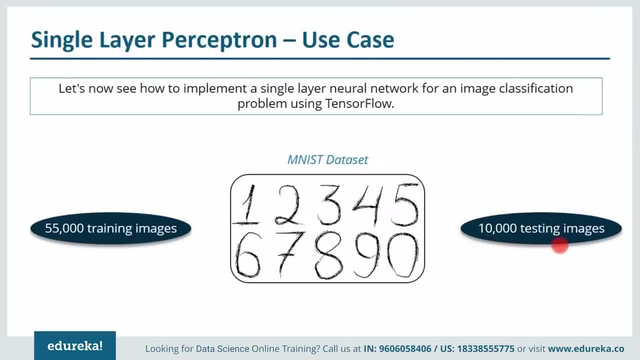 and then we are going to test the accuracy of a model with the help of those 10,000 testing images. and for all of this, we need to understand first What exactly is tensorflow. So let's move forward, guys, and understand what exactly is tensorflow. 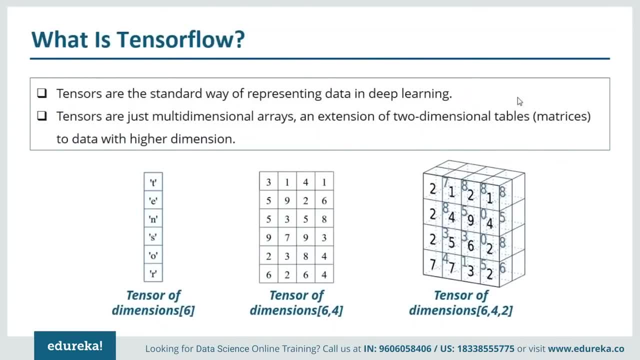 Now, what is tensorflow? As I've told you earlier as well, We use this tensorflow library in order to implement deep learning models, and the way the data is represented in the deep learning model is called tensors. Now, what are tensors? Now, tensors are just the multi-dimensional arrays. 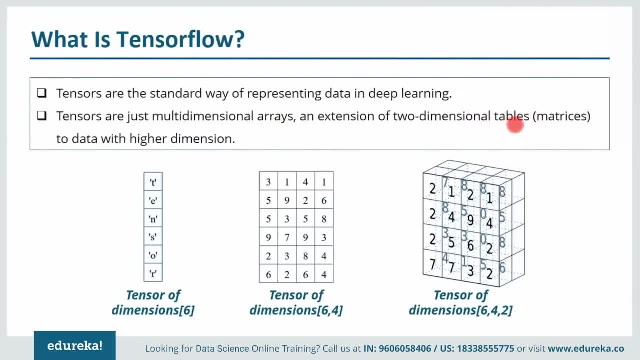 or you can say an extension of two-dimensional tables, matrices, to data with high dimension. Now let me explain you with the examples that are there in front of your screen. So this particular data is nothing but a tensor of dimension 6, because we have six rows. 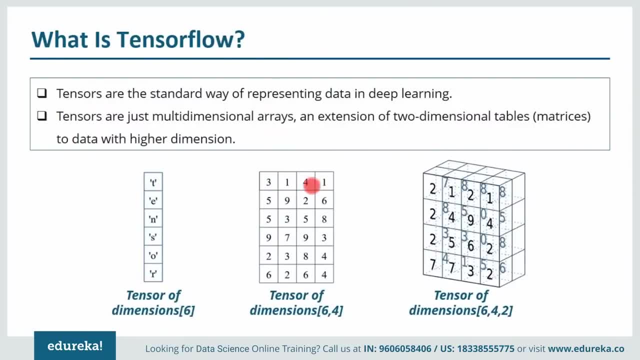 And we have only one single column. now over here We have four columns as well as six rows, So this becomes a tensor of dimension 6 comma 4, similarly over here as well. So we have another dimension, that is the third dimension, in which we have two values. 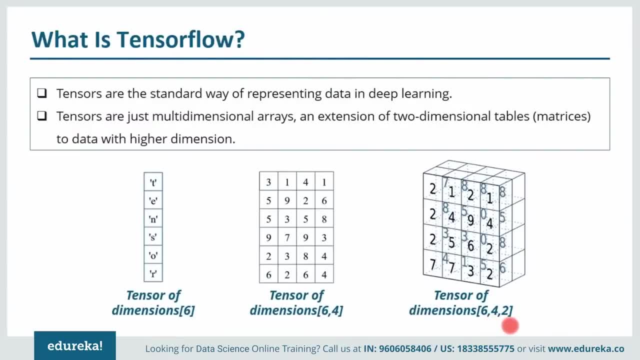 So we consider this as a tensor of dimension 6, 4 and 2.. So this is nothing but a way of representing data in tensorflow. Now, if you consider the tensorflow library at its core, it is nothing but a library that performs Matrix manipulation. 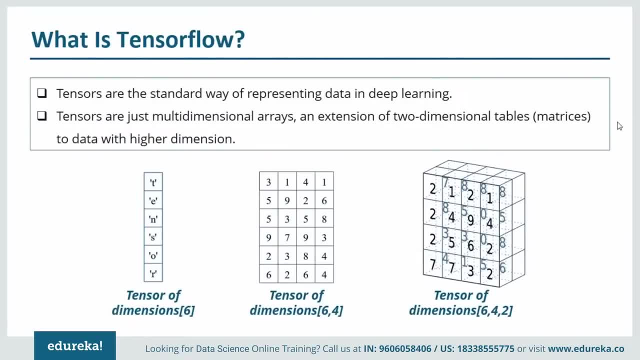 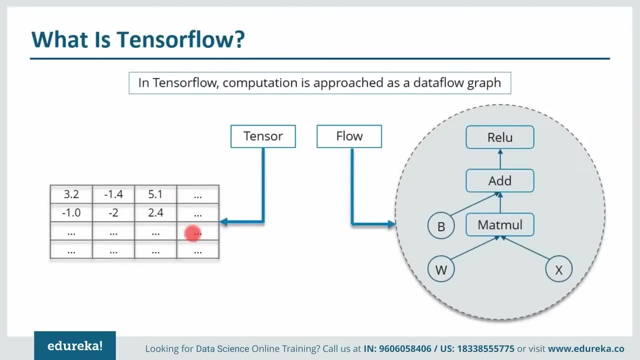 That is what tensorflow is. Now let us move forward and understand tensorflow in a bit detail. So, as the name tells, that, it consists of two words: tensor as well as flow. Now we understood what exactly tensor is. Now, when I talk about flow, it is nothing but a data flow graph. 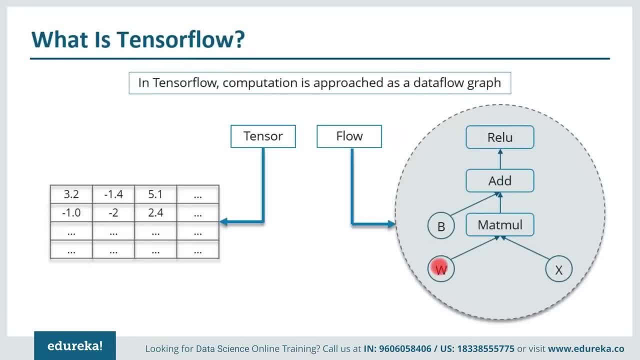 So let me just give you an example that is there in front of your screen. So we talked about weights and inputs. So we provide these weights and inputs and we perform a matrix multiplication. So the weight is one tensor, X input is one tensor. 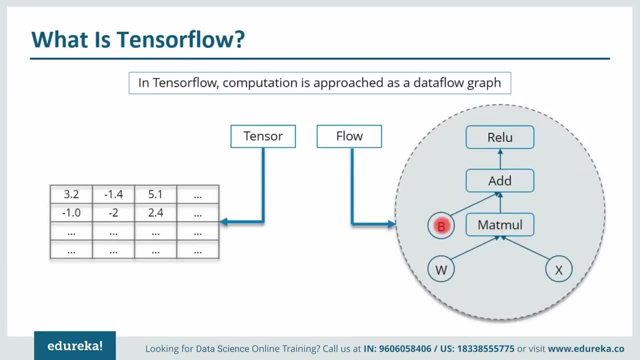 Then we perform Matrix multiplication. after that We add a bias. then what we do? we add all of these. So what is this? This is nothing but the Sigma function in the perceptron that we have seen. Then we pass it through an activation function, and the name of that activation function is: 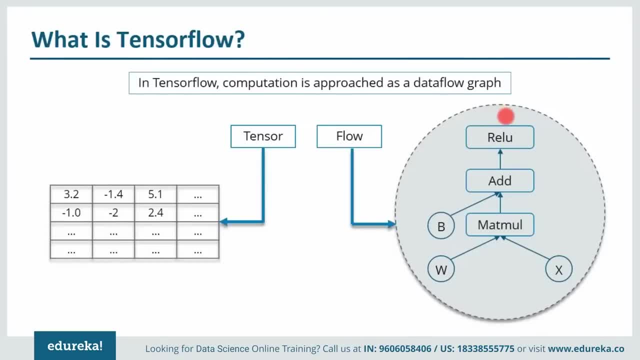 RELU or RELU, what you can say it and then our neuron will fire. So this is nothing but a flow, or you can say a data flow graph. Now let us understand few code basics of tensorflow. So we'll move forward and understand the code basics of tensorflow. 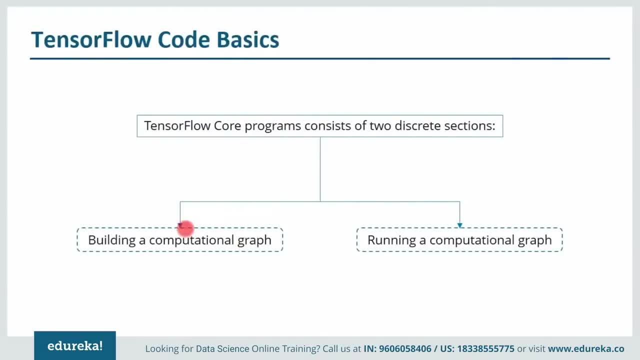 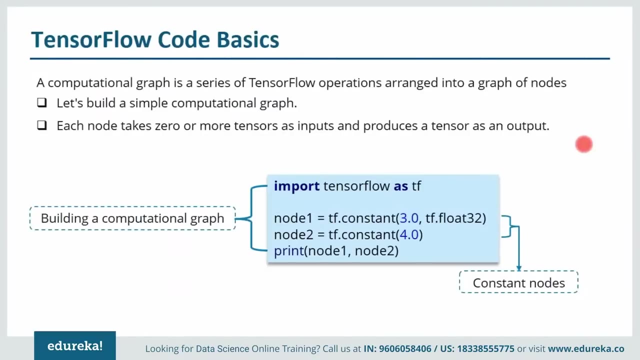 Now the tensorflow programs actually consists Of two parts. one is building a computational graph and another is running a computational graph. So we'll first understand how to build a computational graph. Now you can think of a computational graph as a network of nodes and with each node known as an operation. 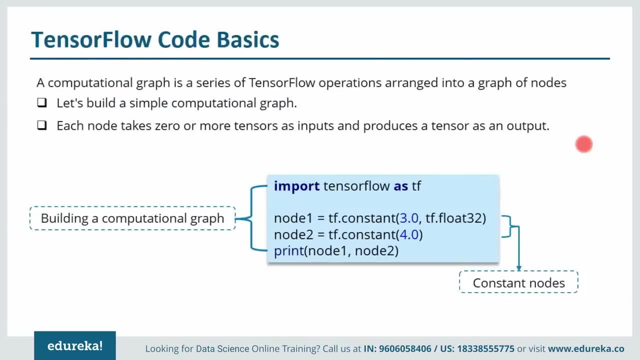 and running some function that can be as simple as addition or subtraction, or it can be as complex as, say, some multivariate equation. Now let me explain it to you with the code that is there in front of your screen. So the first thing you do, you import. 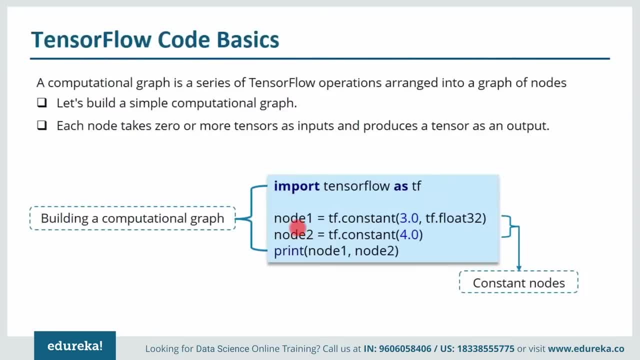 The tensorflow library. then what do you do? you define two nodes and these nodes are constants. So we'll call that function, will call it as TF dot constant and will provide a value that is 3, and it is nothing but a float number of 32 bits. 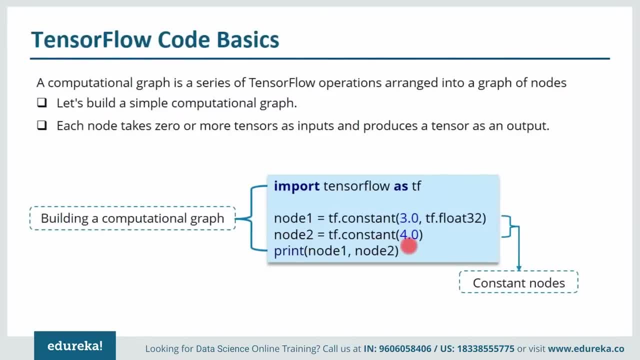 Similarly, we defined one more node, which is a constant, and it contains value 4.. So these are nothing but your constant nodes. This is basically what computational graph is. So, basically, we have built a computational graph and in this graph, each node takes: 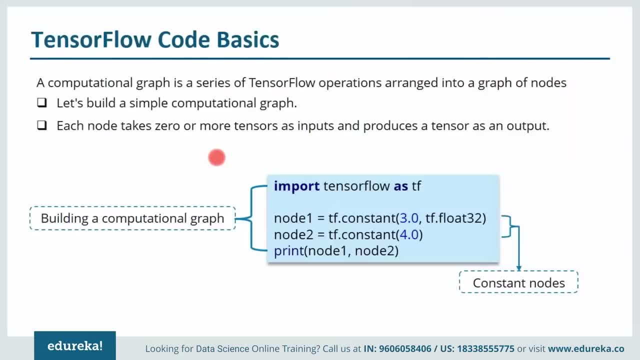 Zero or more tensors as inputs and produces a tensor as an output, and one type of node is a constant- that I've told you earlier as well- And these tensorflow constants. it takes no inputs and it outputs a value which is stored internally. Now what I'll do? I'll actually execute this in my pie chart. 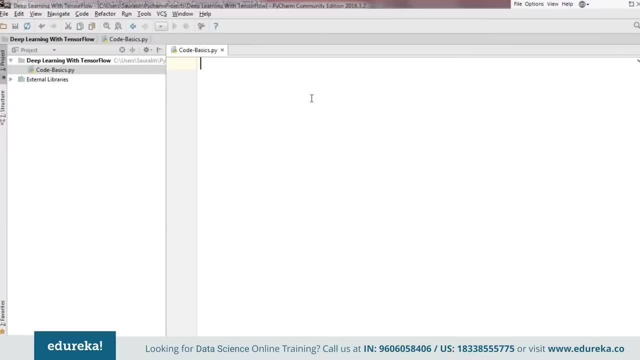 So for that I'll open it. So this is my pie charm, guys, and I've already installed tensorflow. So the first thing that I need to do is import the tensorflow library. for that I'm going to type in here: import TensorFlow as TF. 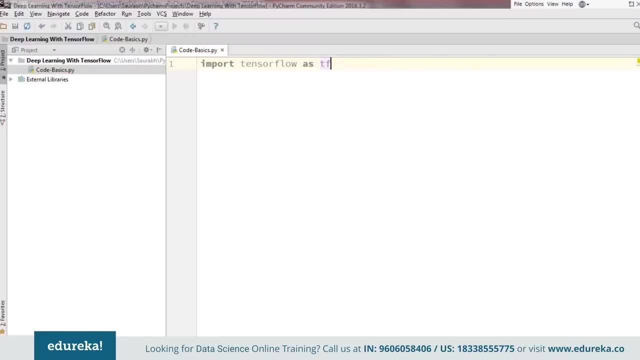 So if you are familiar with the python basics, you know what it means actually. So I am importing tensorflow library and in order to call that, I'm going to use the word TF. So after that, I'm going to define my node 1 and node 2, which are constant nodes. 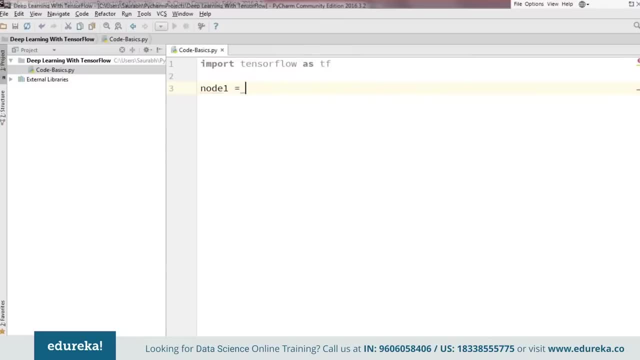 So for that I'm going to type in here node 1, equal to TF dot constant, And then I'm going to define the constant value in this. So it will be 3. And it will be a float value of TF dot, float of 32 bit. 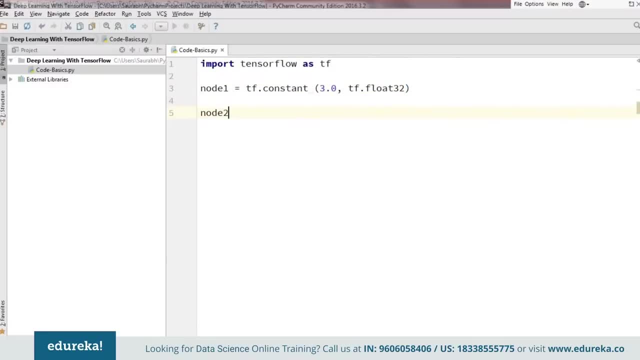 All right, and now I'm going to define my second constant node. So I'll type in here node 2: TF dot constant. I'll put 4 in here and 4, that's it. And so the TF dot float 32 will be present implicitly. 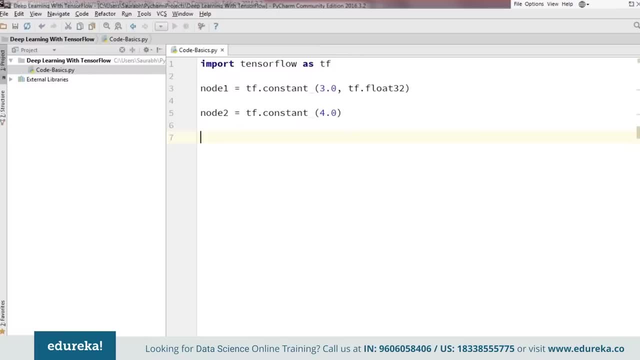 I don't need to do that again and again. So I have created a computational graph here. So what if I print it Now? so let us see what will be the output. node 1: comma. node 2.. Let's go ahead and run this and see what happens. 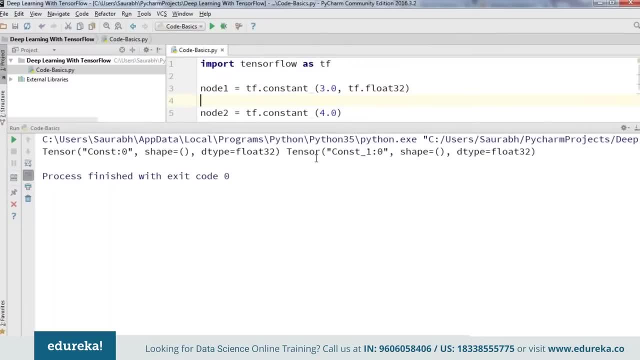 If you notice here that printing the nodes does not output the values 3 and 4, you might be expecting that right, that it should print 3 and 4. but instead they are nodes that, when evaluated, would produce 3 and 4 respectively. So to actually evaluate the nodes, what we need to do is we need to run this computational graph. 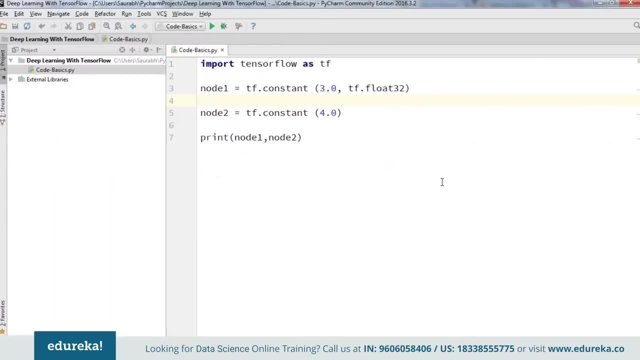 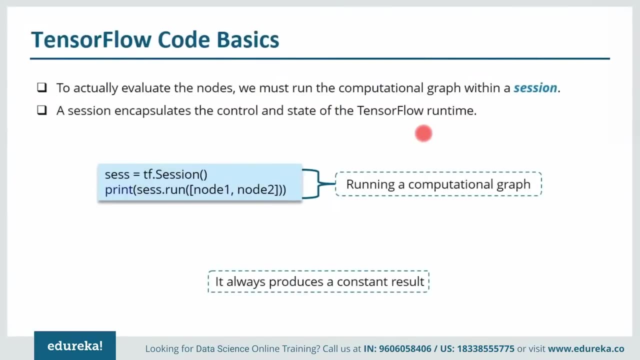 So let me show you that. for that I'm again going to open The slides. So, since I've told you earlier as well, we need to actually run this computational graph within a session. And what is this session? It's session actually encapsulates the control and state of the tensorflow runtime. 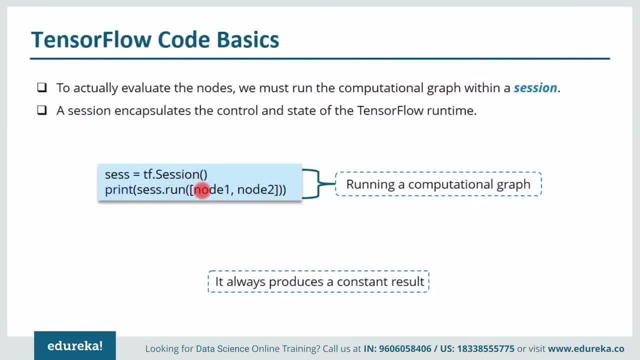 Now the code that is there in front of your screen. what it will do? It will actually create a session object and then it invokes its run method to run enough of the computational graph in order to evaluate node 1 and node 2. and how it does that? by running the computational graph in a session. 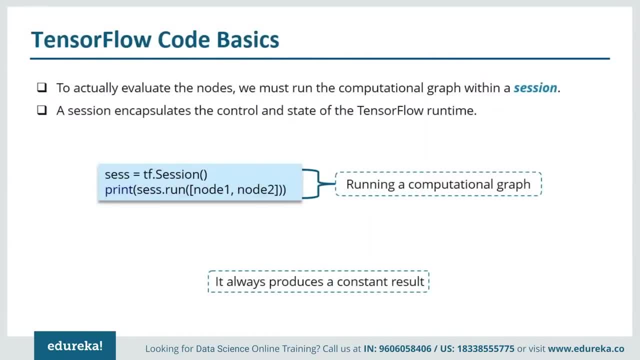 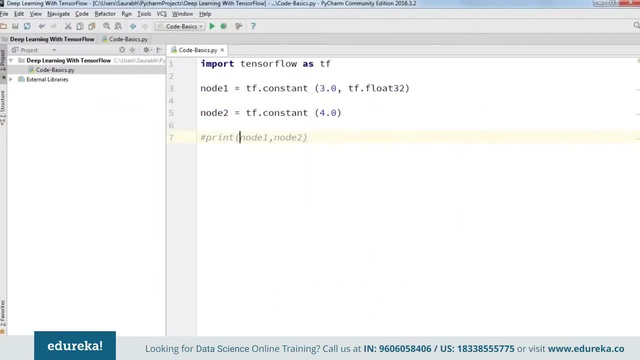 So now let me show it to you practically how it happens. So again, I'm going to open my pie charm. This is my pie charm, guys. So let me first comment this print statement, and now I'm going to run a session, So for that I'm going to type in here, says equal to TF dot session. and now I'm going to print it. 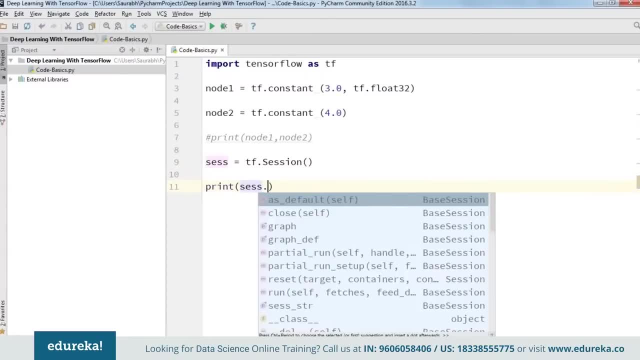 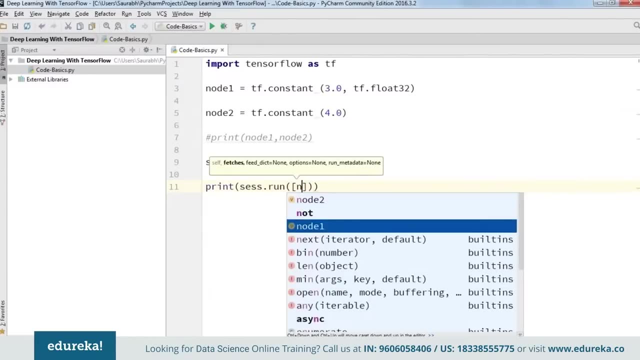 So for that I'm going to type in: print says dot run and what I want to run. I want to run node 1 and node 2.. So I'm going to type Type in here and node 1 comma, node 2.. 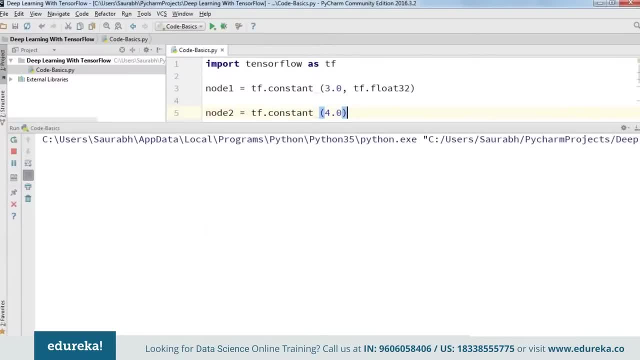 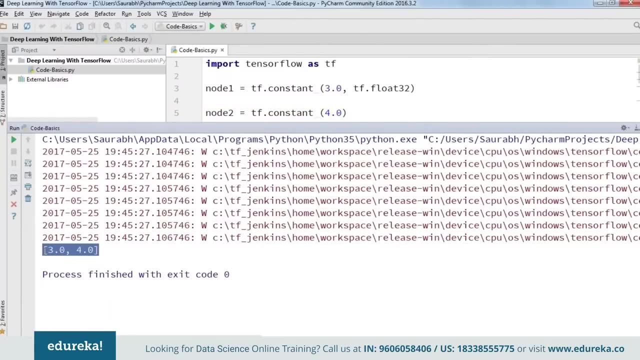 That's all. and now, when I run this, it will actually give me the value 3 and 4. and yup, it does, it gives me the value 3 and 4.. So what we did? we first build a computational graph. We first saw how to build a basically a computational graph, and then we understood that these all are nodes. 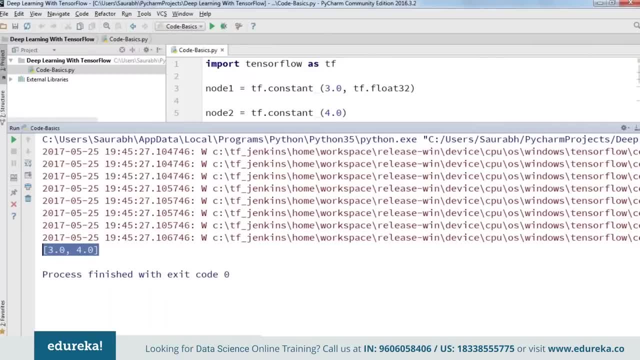 So, in order to get their value, we need to evaluate those nodes, and how we can do that? by running the computational graph inside a session And then, finally, when we run that session, we get the output 3 and 4, which is nothing but the values of those nodes. 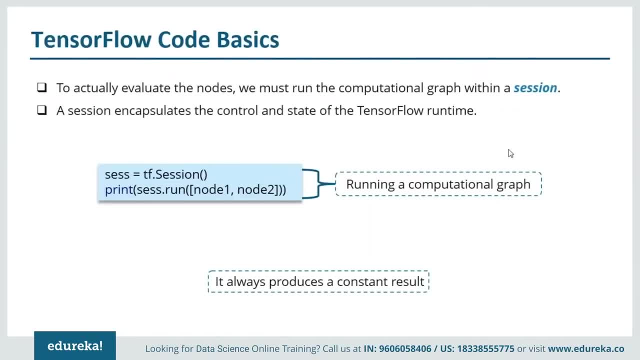 And the one thing that you must have noticed here is that it will always produce a constant result, right? So how to actually avoid that? So we saw how to run a computational graph as well. Now let me explain it to you with one more example. 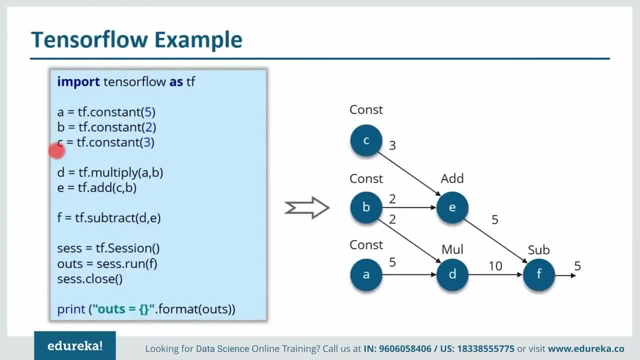 So this is one example in which we take three constant nodes, a, b and c, and we perform certain operations like multiplication, addition and subtraction, And then we run the session and then we finally close it. And this is the diagram How it looks like. so we have three constant nodes: c, b, a. a contains value 5, b contains 2. similarly, c contains 3. first, 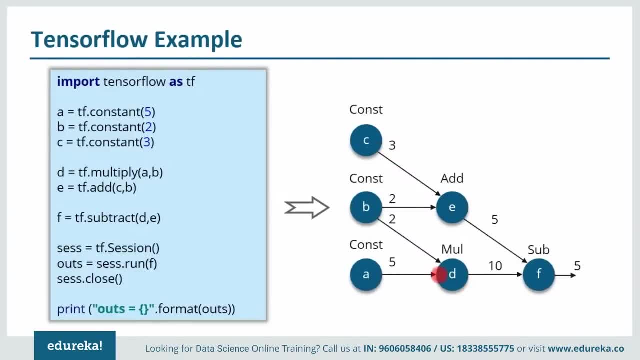 We add c and b, then we add b and a, then we get two other nodes, that is, e and d, and then from that e and d, What we are going to do is we are going to subtract both of them and then we get the final output. 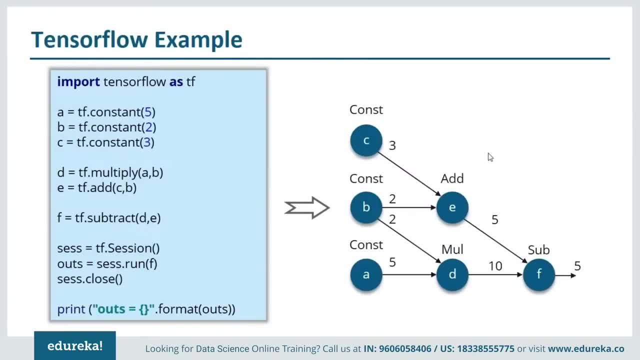 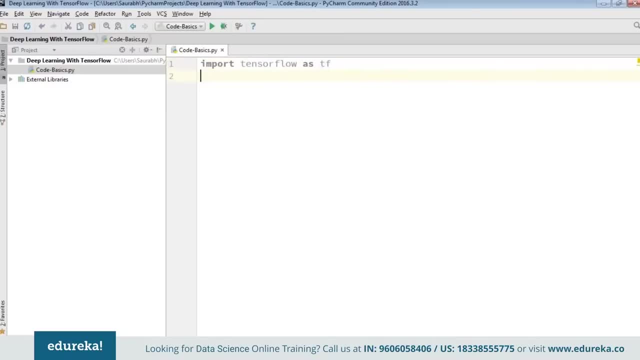 Now let me go ahead and execute this practically in my pie charm. So this is my pie charm again, guys. First thing I need to do is import tensorflow as t, F. Then we are going to find the three constant nodes. So first is a, a equals to t, f, dot constant and the value that will be there in a will be five. 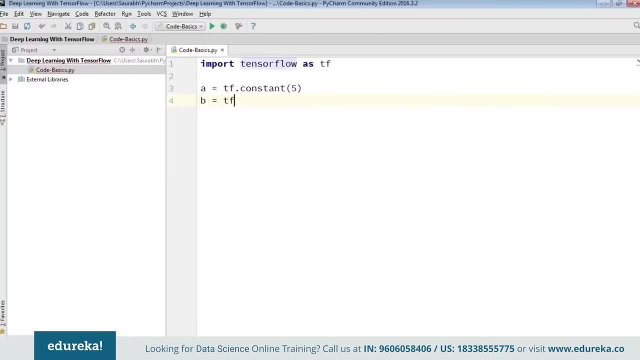 Then I'm going to find one more constant node that will be b, t, f dot constant, and the value that will be there in it will be two. And then I'm going to find the last constant node and t- f dot constant. The value that will be there is three. 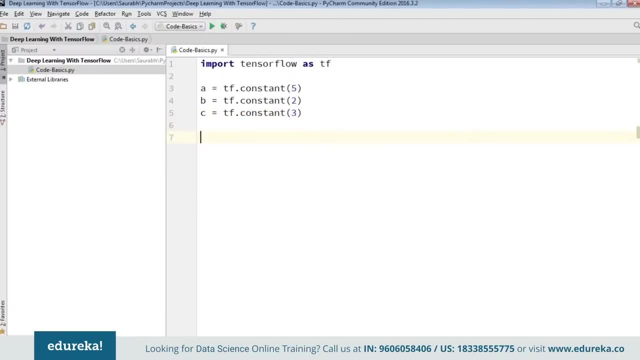 All right. So we have three constant nodes and now we are going to perform certain operations in them. for that I'm going to find one node- Let it be d- which will be equal to t, f, dot. multiply So the two nodes that we want to multiply, so that will be a comma b. 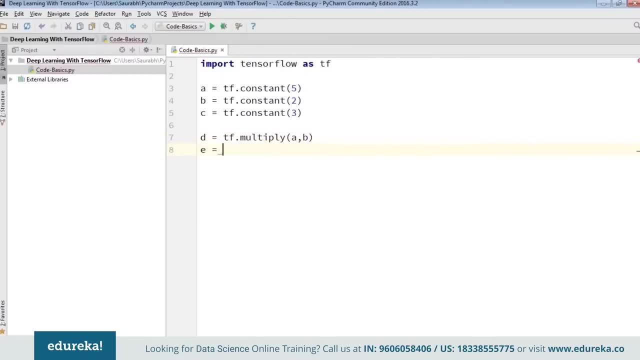 And then there will be one more node in order to perform some operation that is addition to t, f, dot, add, add c and b. And then we're going to find one more node, Let it be f, and inside that node We're going to perform the subtraction operation: t, f, dot, subtract d and e. 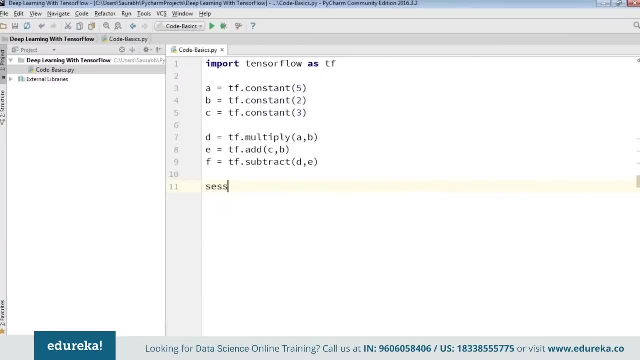 So we have built our computational graph. Now we need to run it, and you know the process of doing that. says is equals to t f dot session. Then we are going to define a variable- Let it be O, U, T, S, outs, whatever name that you want to give in- and just type in a says a dot, run f. 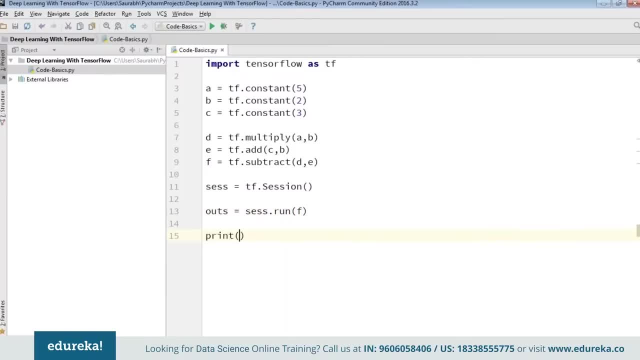 Let's see if that happens or not, And then we're going to print it. for that I'm going to type in here, print out. Let's go ahead and run this and see what happens. So we have got the value 5, which is correct, because if you notice our presentation as well, 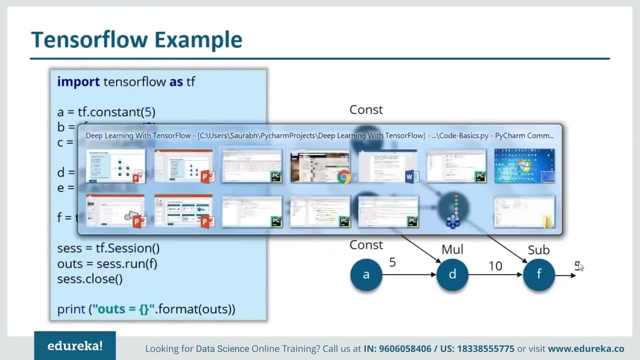 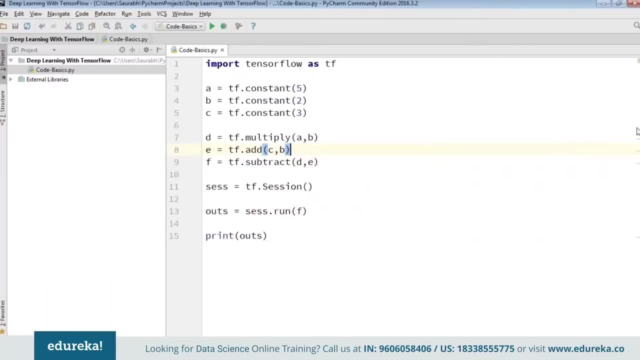 let me open it for you over here. We also we get the value If I similar to our implementation and pie charm as well. So this is how you can actually build a computational graph and run a computational graph. I've given you an example now, guys. 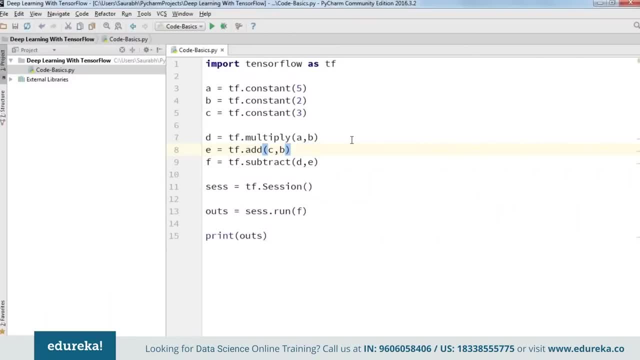 let us move forward. because these are all the constant nodes. What if I want to change the value that is there in the node? So for that we don't use a constant nodes, for that We use placeholders and variables. Let me explain it to you first. 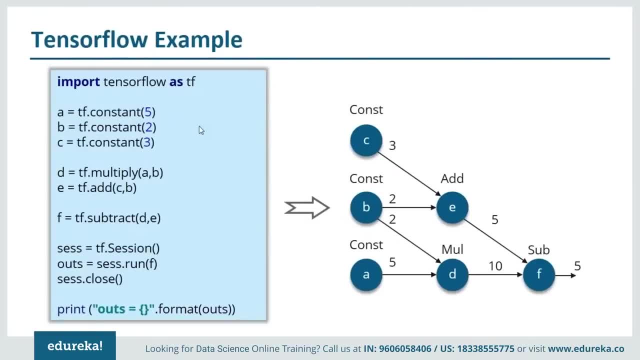 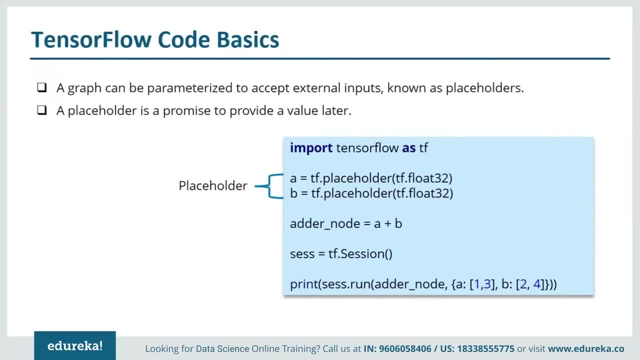 I'll open my slides. So, since these are all constant nodes, we cannot perform any operation. Once we have provided a value, it will remain constant. So, basically, a graph can be parameterized, Except external inputs as well. And what are these? 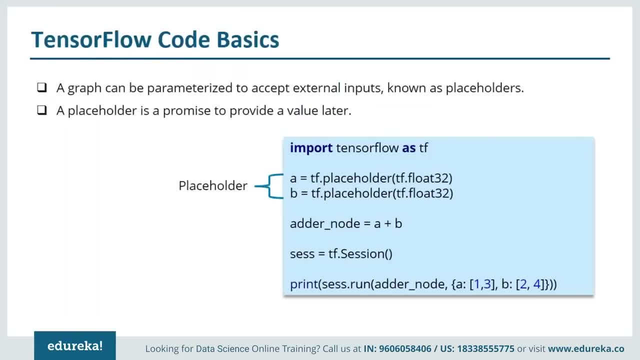 These are nothing but your placeholders, and these placeholders is basically a promise to provide values later. So there's an example that is there in front of your screen Over here. These three lines are bit like a function or a lambda, in which we define a two input parameters, A and B. 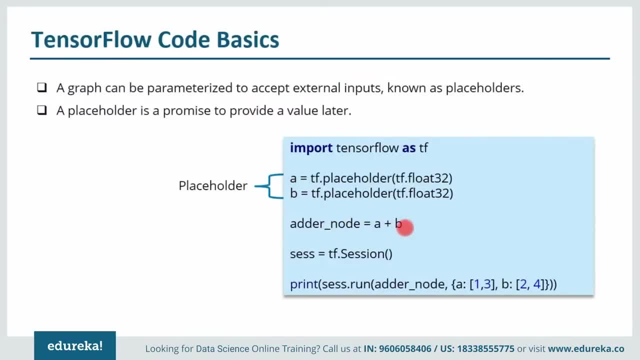 and then an operation possible in them. So we have actually performing addition, So we can evaluate this graph with multiple inputs by using feed underscore dict parameter. As you can see, we are doing it here, So we are actually passing all these values to our placeholders here. 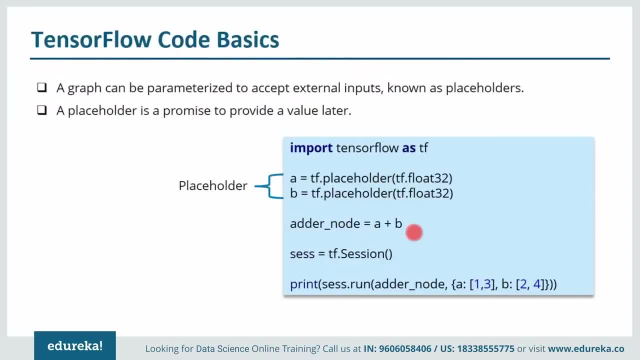 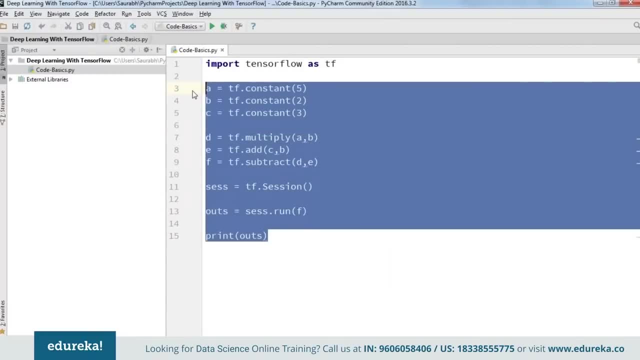 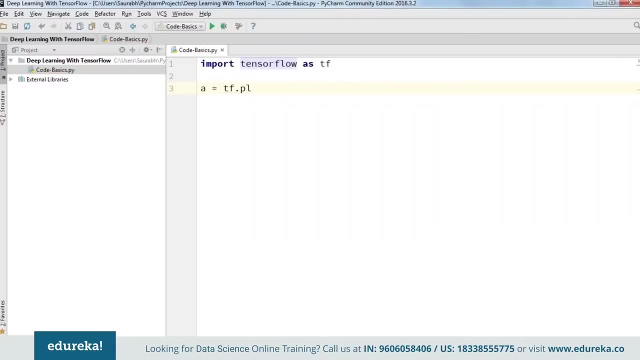 So these all values will be passed and, accordingly, will get the output. So let me show you practically how it happens. So I'm going to open my pie charm once more, I'll remove all of this. and yeah, so the first placeholder, I'm going to name it as a TF, a dot placeholder, and what sort of a placeholder it will be. 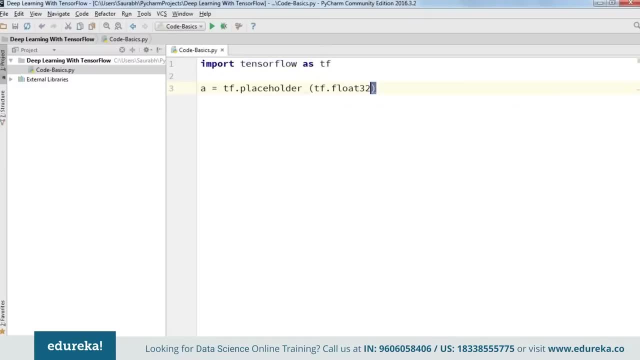 So I'll consider it as Load number of 32 bits. Similarly, I'm going to Define one more variable as well. I'm going to name it as B. Then I'm going to Define an operation that I'm going to perform them. 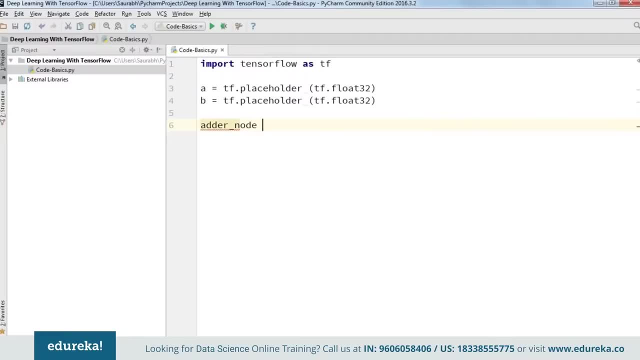 So I'm just going to type in here: adder, underscore, node equals to a plus B, And now our placeholders are currently empty, So that, totally earlier as well, placeholders are nothing but a promise in order to feed values later. So this is how we have built a computational graph. 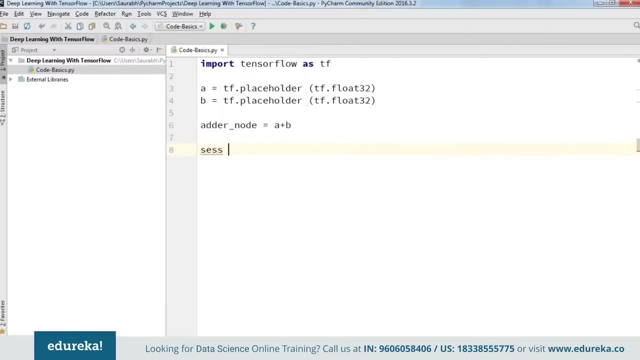 Now our next step Is to start a session, so for that I'm going to type in a assess equals to TF, a dot session, Right, Since these placeholders are currently empty, and we know that these placeholders are nothing but a promise, in order to provide them with certain values later. 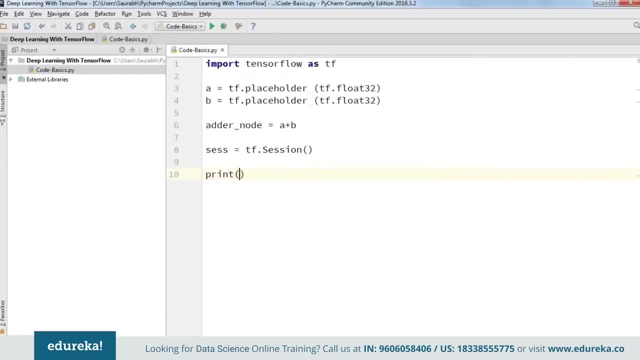 So let's go ahead and provide the values, or you can say a list of values. So I'm going to type in here: print says dot, run, Adder, underscore node, And then the values that I'm going to feed in. So basically, 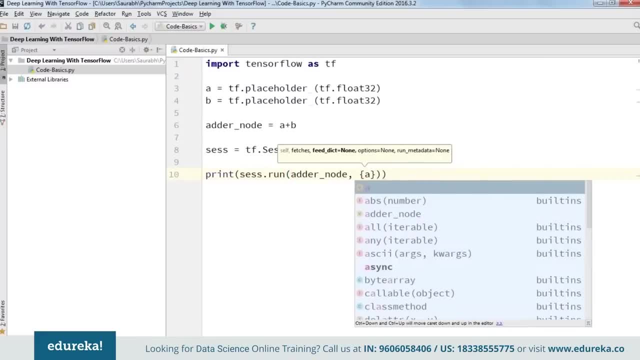 I'm going to feed in a dictionary: A colon, 3: a colon, a list of integer values between 1 to 3, and one more will be B colon, a list of integer values between 2 and 4.. All right, so this is done. 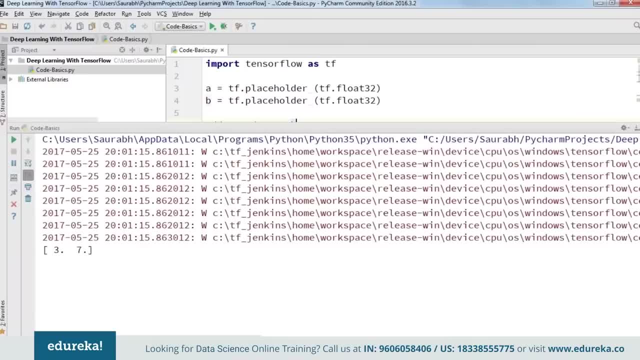 Now let us go ahead and execute this and see what happens. So we have got the output of 3 and 7.. So basically, if you add 1 and 2, you get 3. similarly, you add 3 and 4, you get 7.. 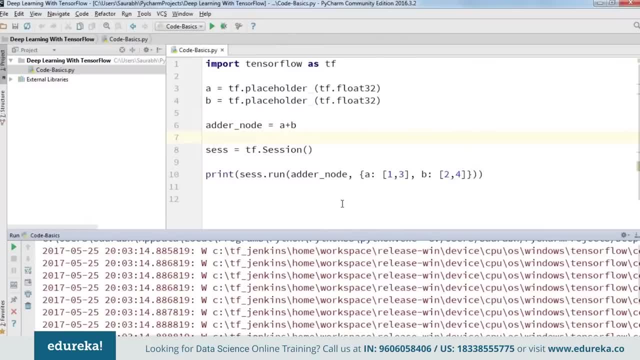 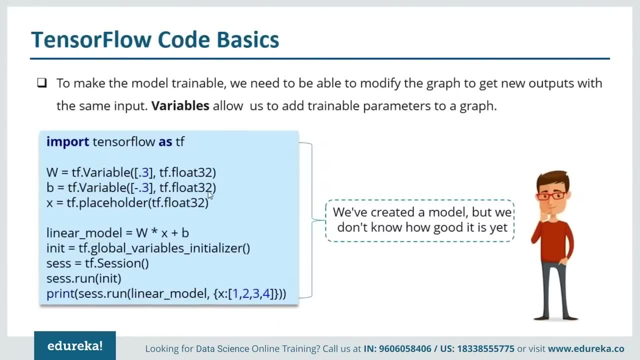 It's pretty easy mathematics, But my main focus was to make sure that you understand what our placeholders. So we understood what exactly our placeholders. now the time to understand what our variables. So basically, in deep learning, We typically want a model that can take arbitrary inputs. now, in order to make the model trainable. 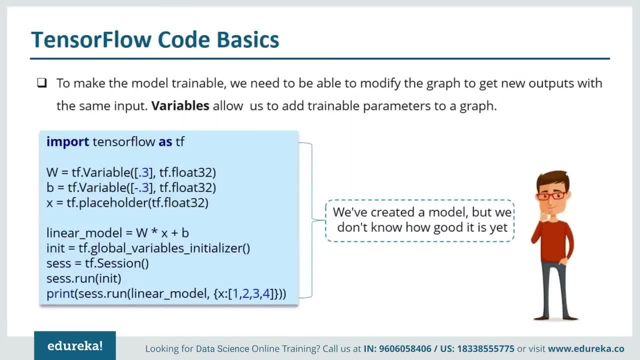 We do able to modify the graph to get new outputs with the same input. And what helps us to do that? variables basically allows us to add a trainable parameters to our game Graph. So, in order to declare variables, what we do is you can refer the code that is there in front of your screen. 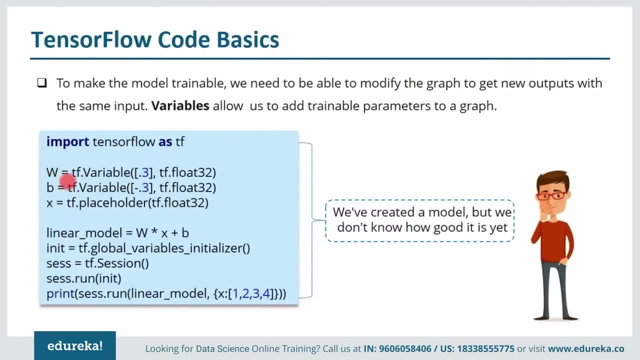 So we have taken two variables in one placeholder and the first variable has a value 0.3.. The other variable has minus 0.3 and the placeholder obviously it will remain empty and then later on we feed in some values to it. Then we create a linear model. 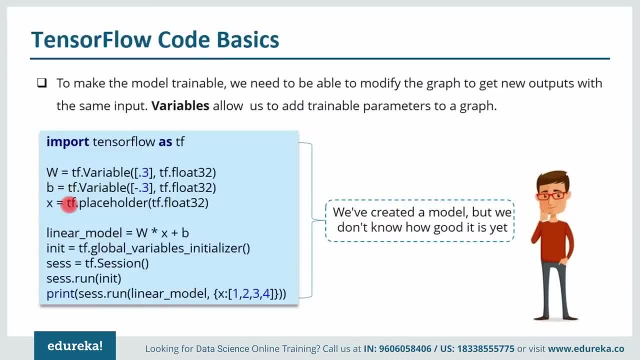 or you can say some operation in which we are going to multiply this W with X and then we are going to add a bias or a B value to it. Then what we need to do is we need to initialize all the variables in the tensorflow program. 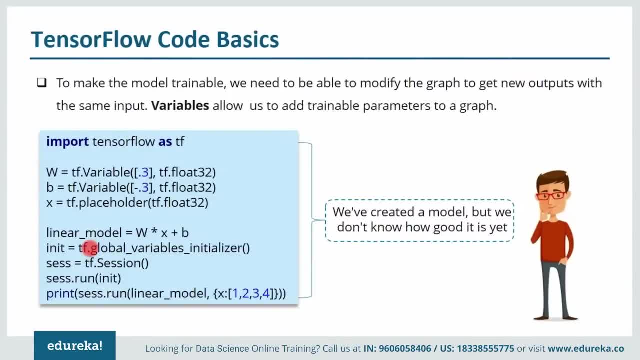 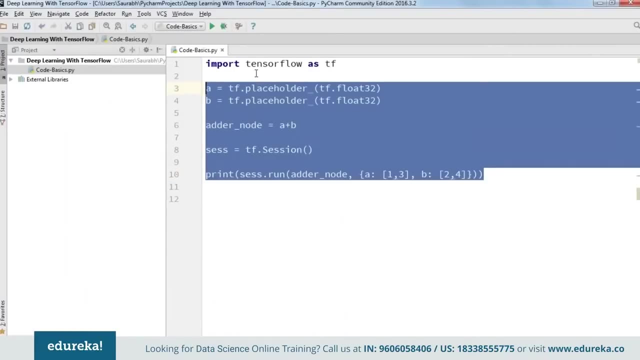 So for that you must explicitly called a special operation, which is a TF dot- global variable initializer, and then just directly run the session. Now let us go ahead and execute this practically, guys. Let me remove all of this. Yeah, so our first variable will be a W and we are going to call in a TF dot variable. 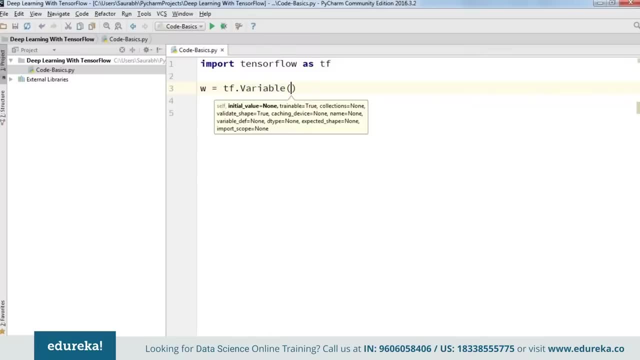 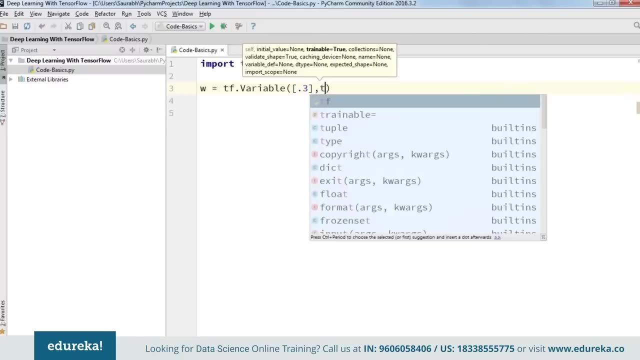 And in that variable we are going to store a value which is 0.3.. And it is of a float type 32-bit. So just type in here: TF dot, float 32.. Yeah, then we are going to define one more variable. 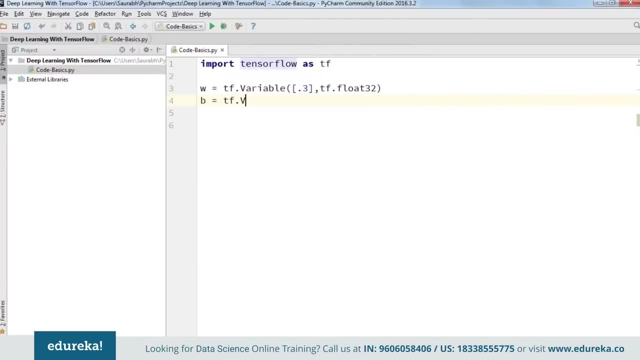 Let it be B. So I'm going to type in a TF dot variable And the value of this variable will be minus of 0.3.. Again, it is float type of 32-bit, So just type in that TF dot, float 32.. 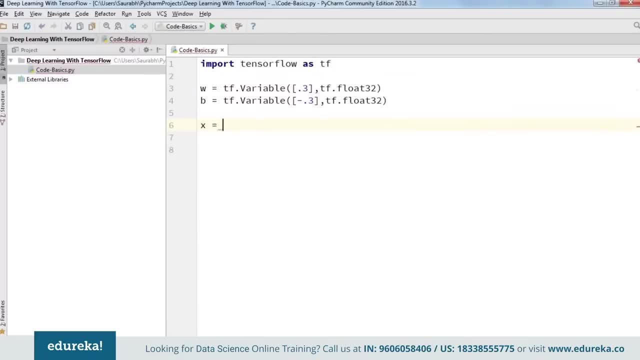 Now I'm going to define a placeholder that is X, X is equals to TF dot placeholder And it is again a float type 32-bit And then some operation that we are going to perform. So I'm going to type in here linear underscore model equal to W multiplied by our X value. 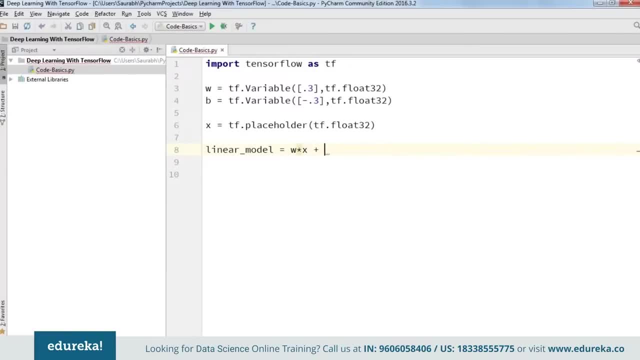 That is a placeholder, And then we want to add a bias to it or B value to it. All right. Now, as we have seen earlier as well, in order to initialize constants, we call TF dot constant and their value will never change. But, by contrast, variables are not initialized when you call TF dot variable. 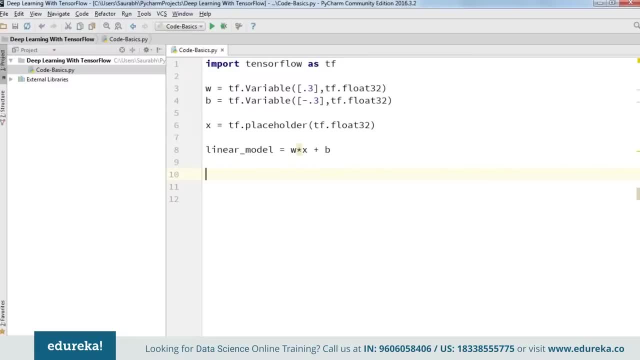 So to initialize all the variables in the tensorflow program, what you need to do is you need to explicitly call a special operation And how you're going to do it. just type in here: INET equal to TF. dot. global Underscore variables. 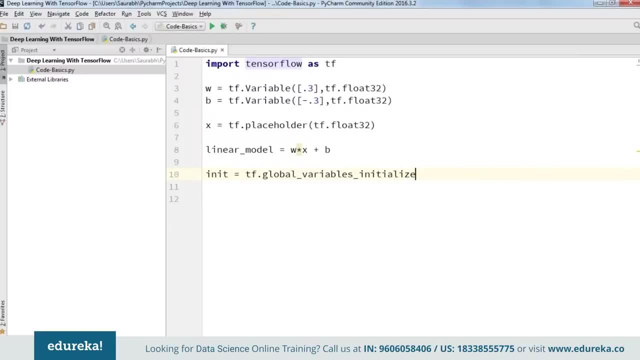 Underscore initializer. That's all, And then we're going to run a session. So you know the process says is equals to TF dot session- INET. Now let's print it, and before that, what we need to do is need to provide the X placeholder with some values. 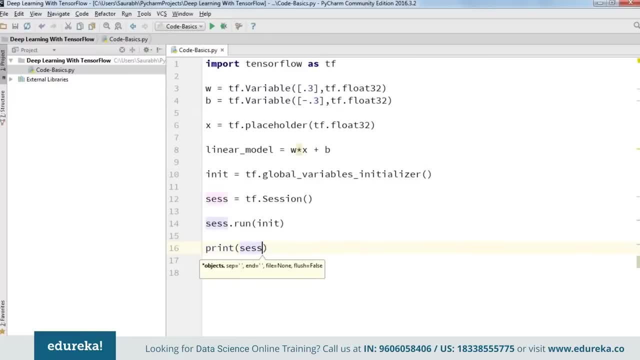 We'll actually going to do that at the print statement itself, So I'm going to type it: says dot run, Run what run? a linear model And the values that we are going to pass in. X will be a dictionary again, And let me show you how you can do that. 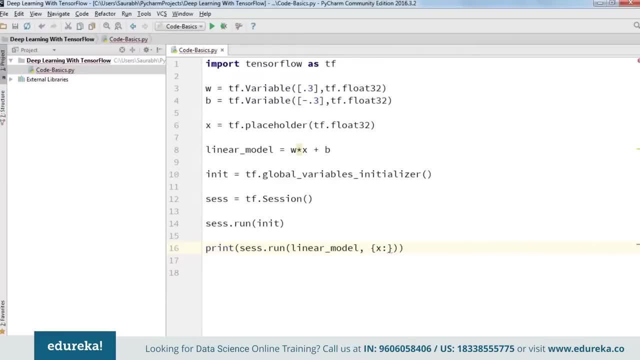 So X, a colon, and it will be a list of values from 1 comma, 2 comma, 3 comma, 4.. Yeah, that's all, and we are going to run it now. So this is how we get the output. It's simple mathematics. 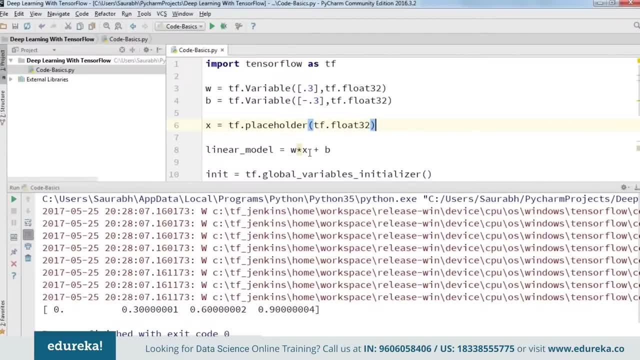 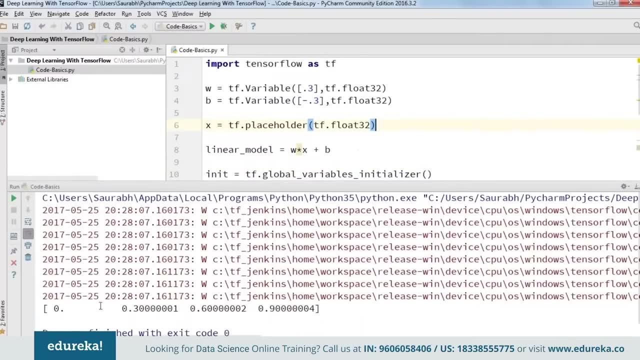 What we have? the first value of W will be 0.3 and the first value of a B will be a minus 0.3 and the first value of X will be 1.. So it will be 3 minus 3, which is again 0, similarly for other values as well. 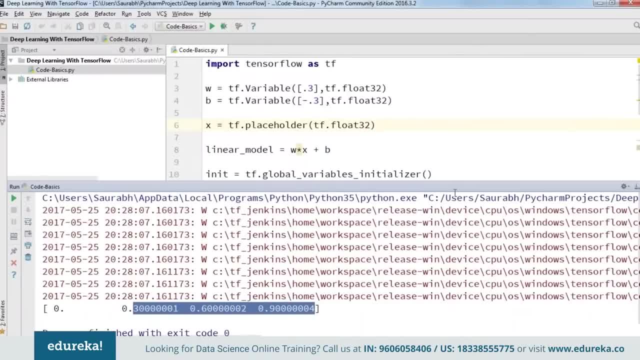 You can calculate it. It's absolutely correct. So what we have done? we have created a model, but we don't know how good it is yet, So let's see how we can actually evaluate that. for that I'm again going to open my slides. 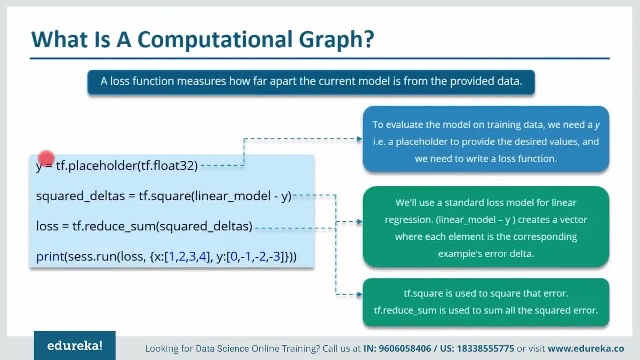 So now, in order to evaluate the model on the training data, we need a placeholder Why, as you can see in front of your screen, to provide the desired values and we need to write a loss function. So this placeholder Y will actually be provided with the desired values for each set of inputs. 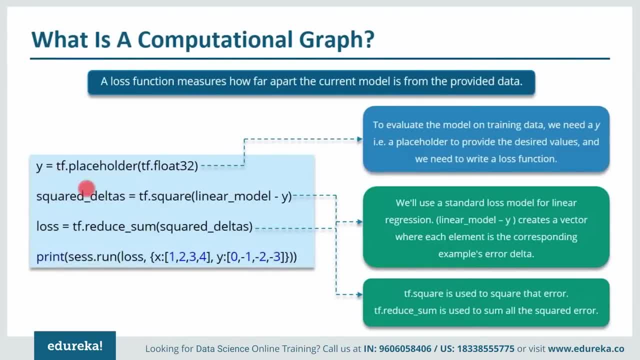 and then we're going to calculate the loss function. And how are we going to do that? We're going to minus the actual output with the desired output and then we are going to do the square of it. after that We're going to sum all of these square deltas and then we're going to define one single. 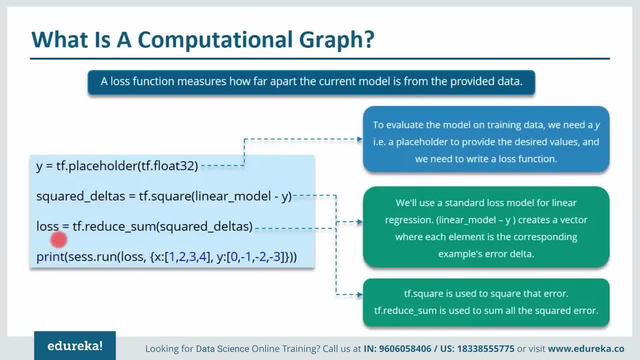 scalar as loss. So this is how we are actually going to calculate the loss, And then, after that, we need to provide the values to X and Y placeholders. So what I'm going to do, I'm going to open my pie charm and then I'm going to show you. 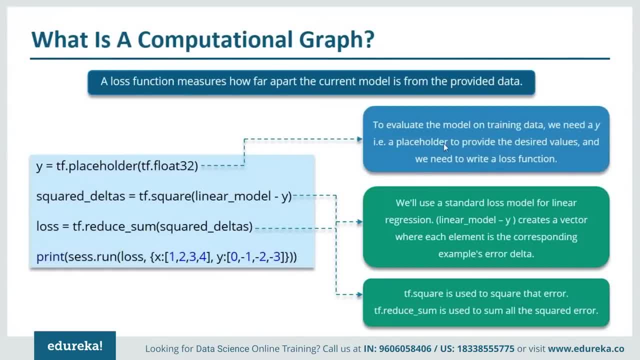 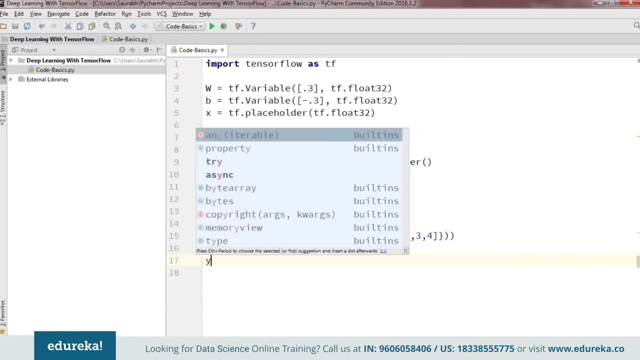 how correct our model is on the basis of the values that we provide to Y placeholder. So, guys, this is my pie charm again. And since here I what I'm going to do is I'm going to define a placeholder first. Y is equals to TF dot- placeholder, TF dot- float 32.. 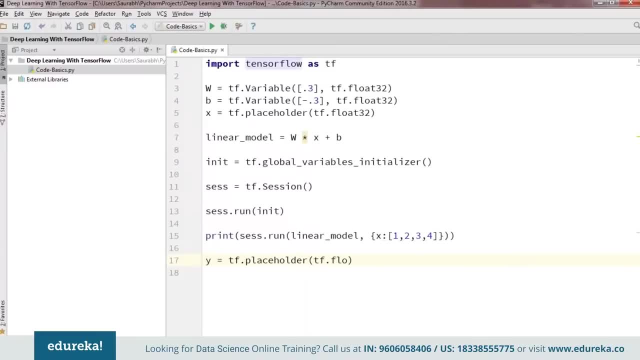 So I'm going to type in a TF dot float 32 square Delta. TF dot square the actual output minus the desired output and then I'm going to sum all those losses. or you can say square deltas, TF dot reduce underscore sum. So I'm going to type in here: square deltas. 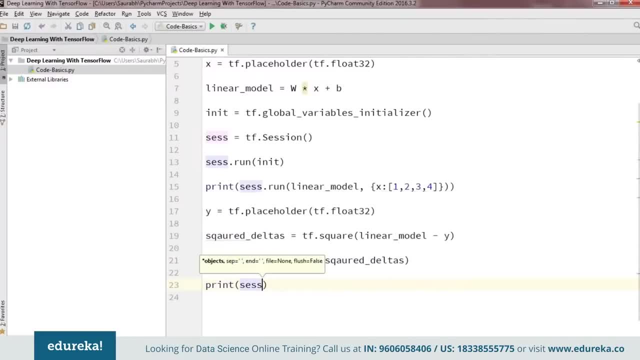 Then finally print it. So I'm going to type in: says dot run Loss X, colon 1 comma 2 comma 3 comma 4.. 0 comma minus 1 comma minus 2 comma minus 3, and that's all and we are good to go. 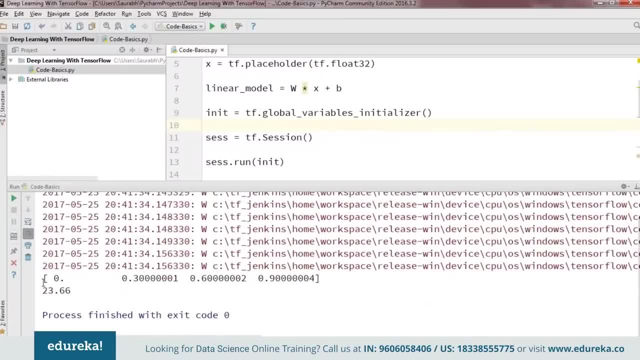 Let's run it and see what will be the loss. So the loss is 23.66,, which is very, very bad. Now our next step is to realize how to actually reduce this loss. So let's go ahead with that. I'm going to open my slides once more. 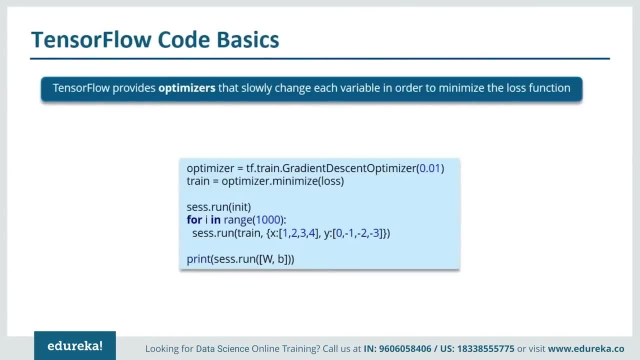 Now, in order to reduce this loss, TensorFlow provides optimizers that slowly change each variable in order to minimize the loss function, And the simplest optimizer is gradient descent. In order to do that, we have to call the function called TF dot gradients. So, as you can see it in the code itself, 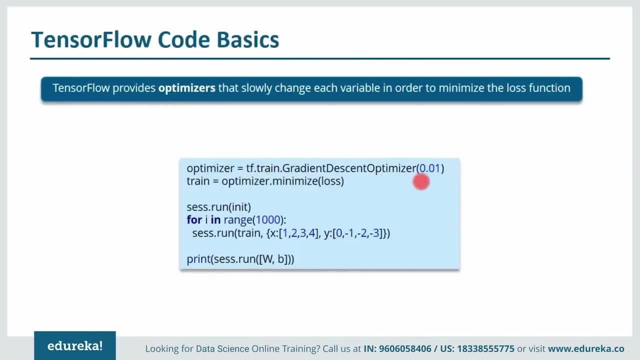 So we have a TF, dot train, Dot gradient descent optimizer, and this is nothing but the learning rate 0.01. then train equals to optimizer, dot minimize the loss. So we're going to call this optimizer, which is nothing but the gradient descent optimizer, in order to minimize the loss, and then we are going to run it. 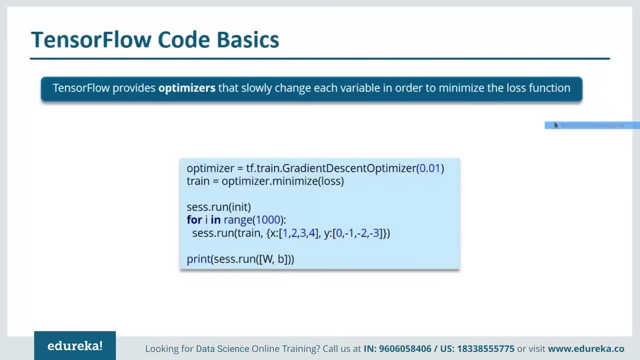 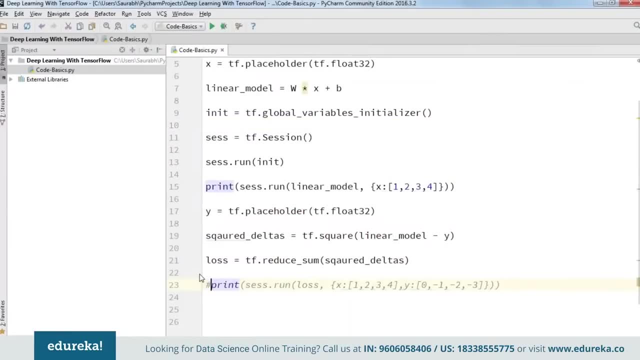 So let's see if that happens or not. So for that again I'm going to open my pie charm, And over here let me first comment this print statement, and now I'm going to type in here: Optimizer equals to TF, dot train. 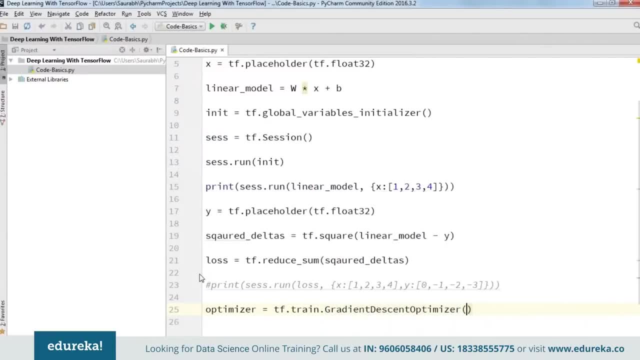 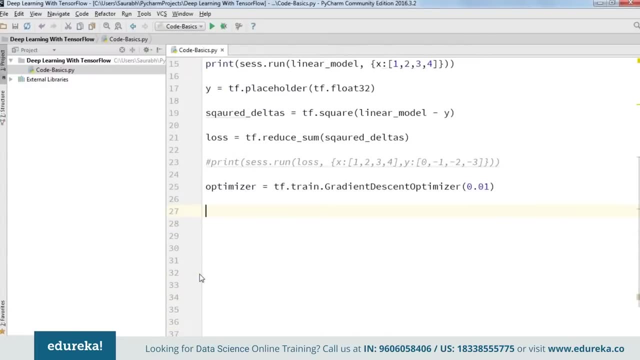 Gradient descent optimizer And the learning rate will be 0.01. and, guys, let me tell you, this is just an introductory session to TensorFlow and deep learning. So all the modules that we have discussed in the beginning will be covered in detail. So whatever topics are there in those modules will be covered in detail. 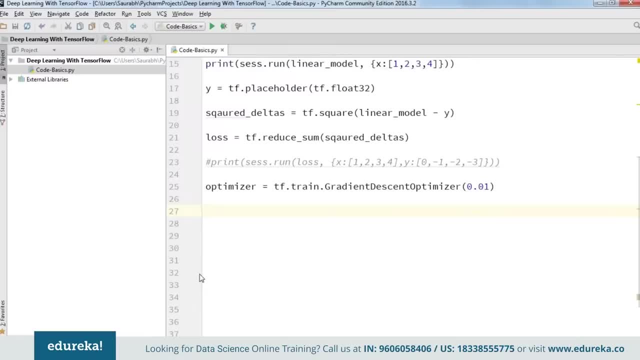 So you don't need to worry about it. So I'm just giving you a general introduction and overview Of how things work in TensorFlow. All these things, all these gradient descent optimizers, All these things will be discussed in detail in the upcoming sessions. 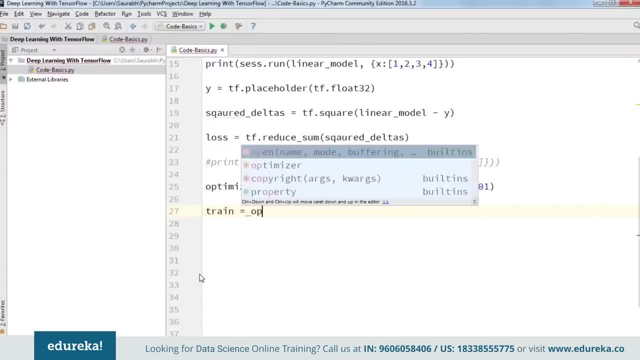 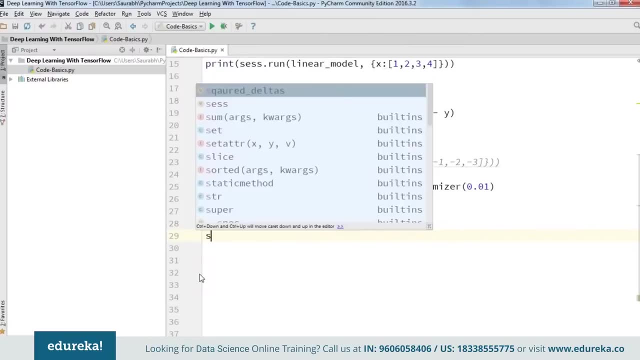 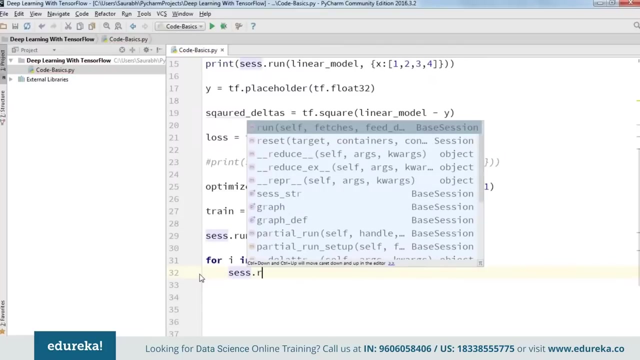 Now I'm going to type in here: train equal to optimizer dot minimize loss. And then now let's go ahead and run. this says dot run, Inet Says dot run, and we're going to feed in values to our X and Y placeholders. 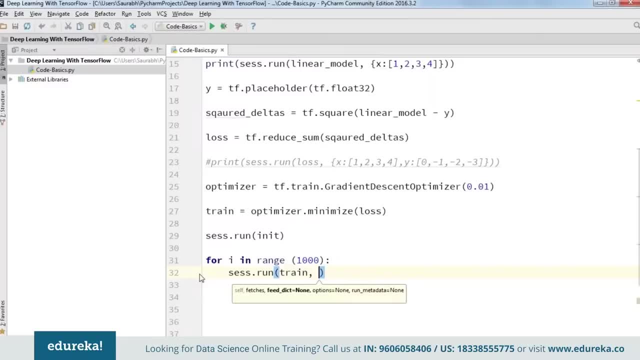 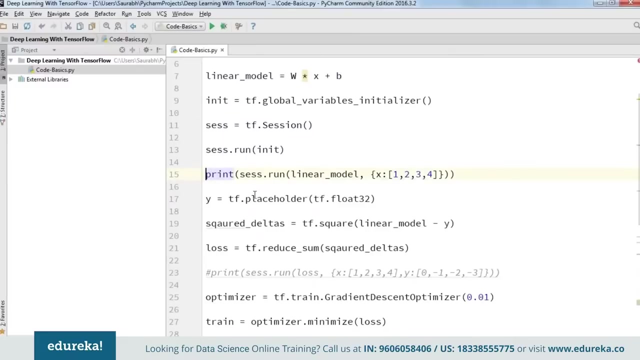 Train comma X will have values 1, 2, 3, 4. And Y will have values 0 comma minus 1 comma minus 2 comma minus 3.. Print Says: dot run W comma P. Now let me first go ahead and comment these lines. 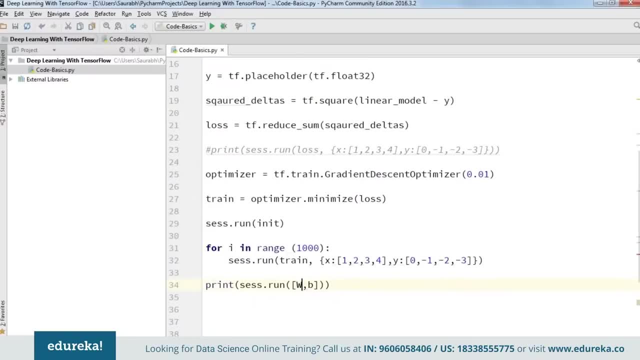 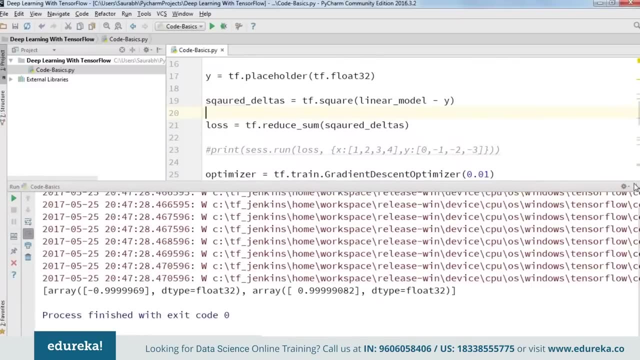 All right, so I've just made a mistake here. This is in uppercase W, and yeah. so now we are good to go and let's run this and see what happens. So these are our final model Parameters. So the value of a W will be around a point: nine, nine, nine, nine, six, nine. 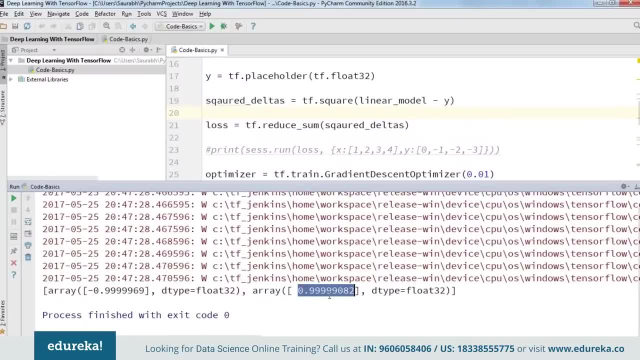 and the value of our B will be around a point nine, nine, nine, nine zero eight two. So this is how we actually build a model, and then we evaluate how good it is And then we try to optimize it in the best way possible. So I've just given you a general overview of how things works in TensorFlow. 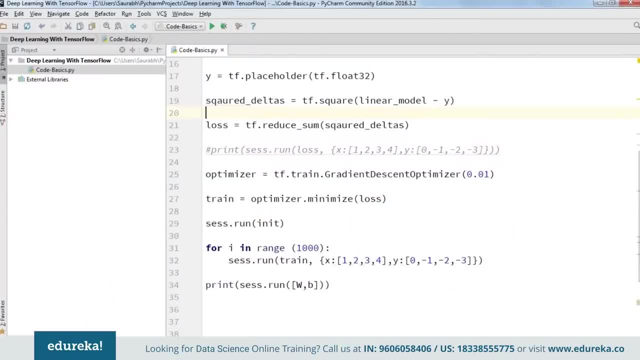 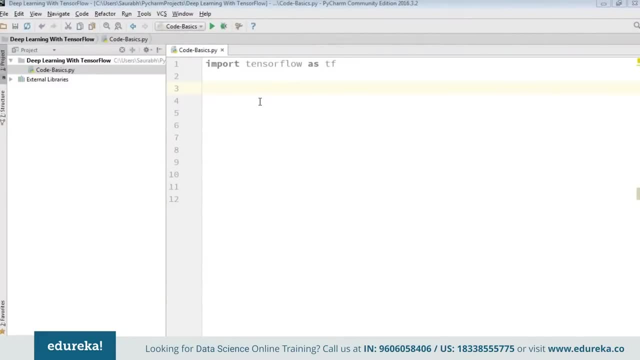 So now is the time to actually implement the and and or gate that I was talking about at the beginning of the session. So for that, let me first remove all of this. Now, in order to implement and gate, our training data should consist of: the truth table for and gate. 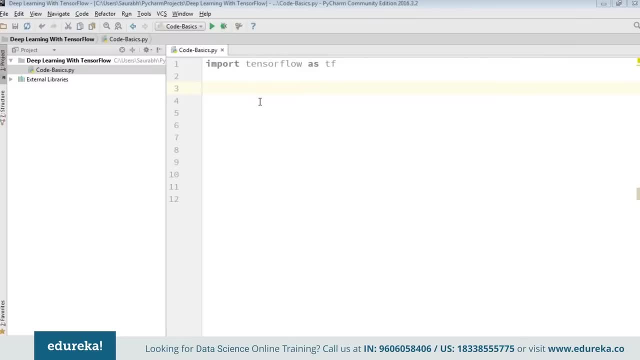 and we know that truth table and we know that if any of the input is low, then the output will be low, and and if both the inputs are high, then output will be high. One thing to note here, guys, is that the bias is implemented by adding an extra value of one to all the training examples. 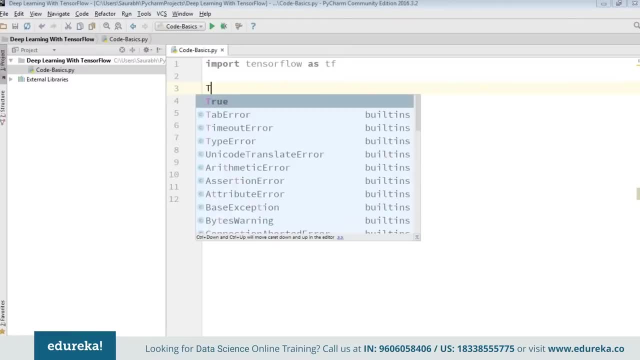 So yeah, enough of the explanation, Let's go ahead and code it. So I'm going to type in here: T comma F equal to one point, Comma minus one point, and bias will always be one. So I'm going to type in here: bias is equals to one point zero. and now I'm going to provide the training data. 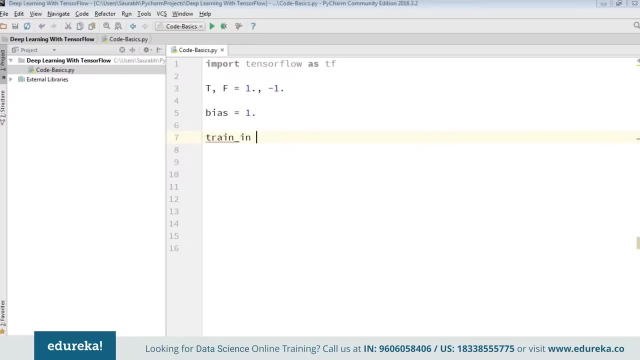 So for that I'm going to type in train underscore in equal to: if one input is true and the another input is also true, Then we have bias. Then again, if one input is true, the other input is false, Then also we have bias. 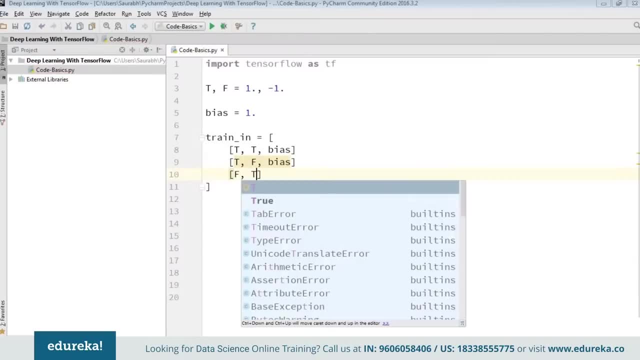 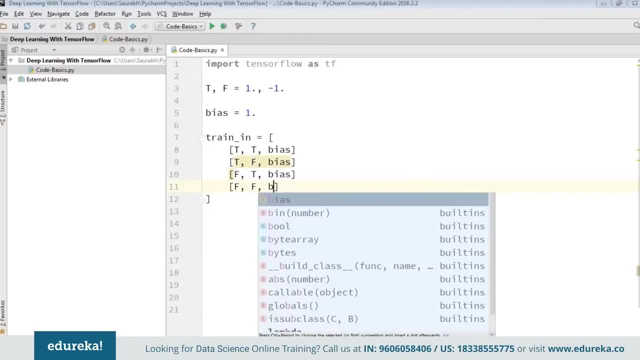 Similarly, one input is false, Another input is true, Then we have bias, And then, finally, when both the inputs are false or zero, then we have bias. right, This is our training data and the train out will type in here as the output. 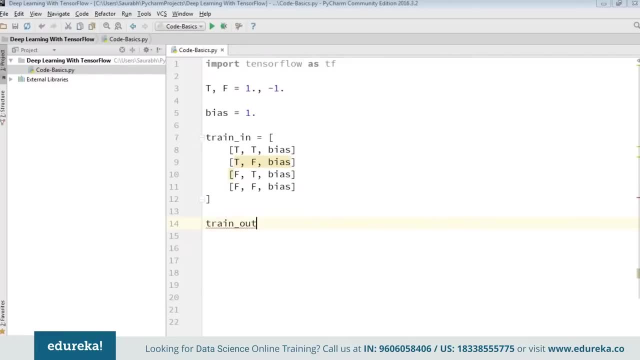 Basically, train underscore out will be equal to: So yeah, if both the inputs are true, or both the inputs are one and output is true. Oops, I forgot our comma everywhere. Let me just go ahead and do that. Yeah, so if both the inputs are true. 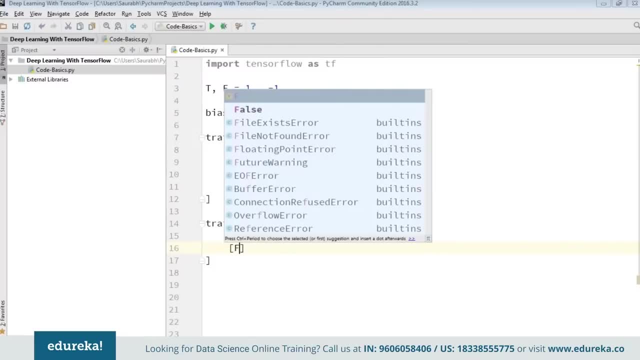 the output will be true. If any of the input is for, the output will be false. So I'm just going to type in here: falls everywhere, because there's only one condition in which we have the true output. All right, so this is done now. 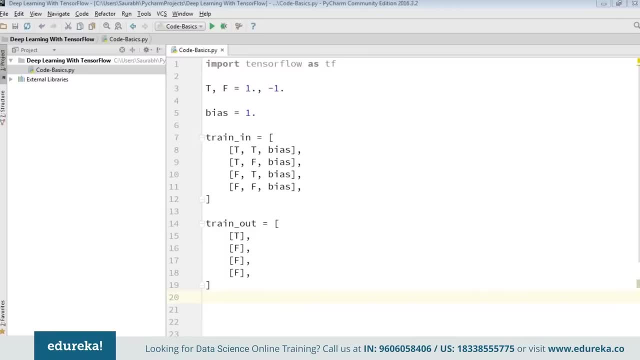 Now, as we know that tensorflow works by building a model out of empty tensors, then plugging in known values and evaluating the model, like we have done in the previous example, Since the training data that we have provided will remain constant, The only special tensorflow object we have to worry about in this case is our three cross one tensors of vectors. 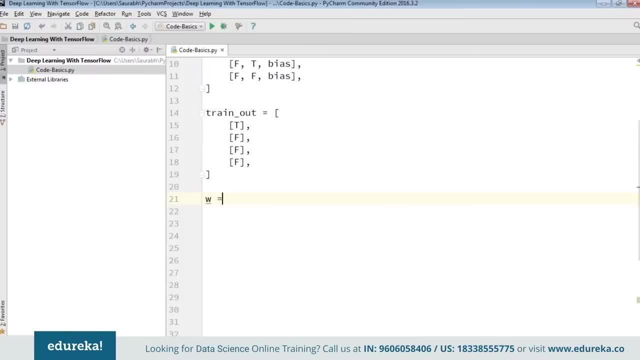 And now what are we going to do? We're going to define a variable and we are going to put in some random values in it. So I'm just going to type in TF a dot variable and generate the random function: TF dot- random underscore normal. 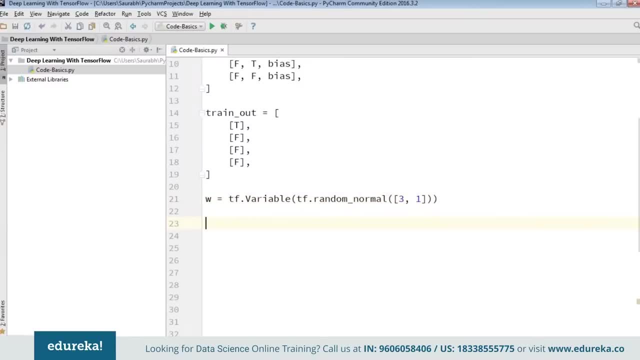 Three comma one. Now what it is? it is basically a variable, So its value may be changed on each evaluation of the model as we train, with all values initialized to normally distributed random numbers. Now that we have our training data and weight tensor, 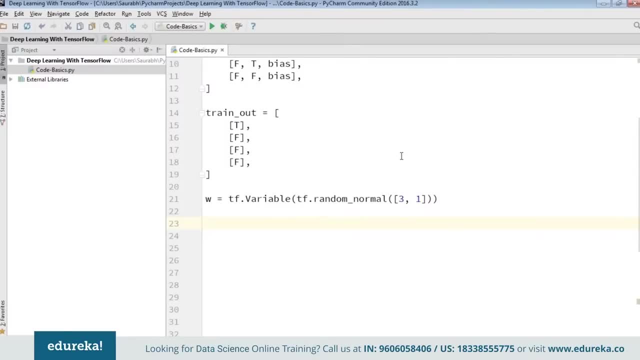 we have everything needed to build a model using tensorflow. So what we need to do, we need to define an activation function and we're going to define a step activation function or step function. So for that, what I'm going to write here is a function: step. 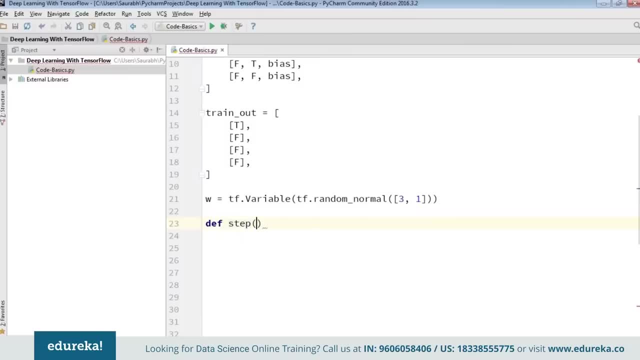 We're going to define our own step function, although you can use the predefined function as well. That totally depends on you. I'm going to type in here: is greater equal to TF, dot greater X, comma zero. Then we're going to define one more variable as float. 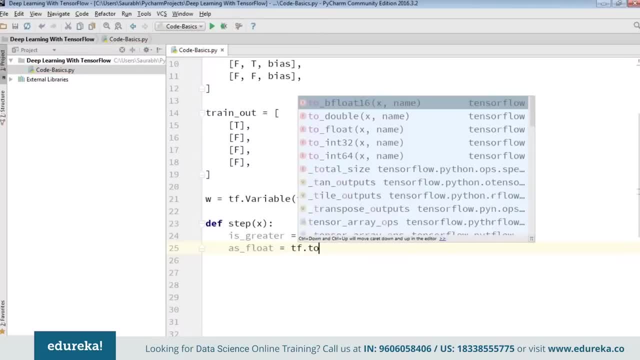 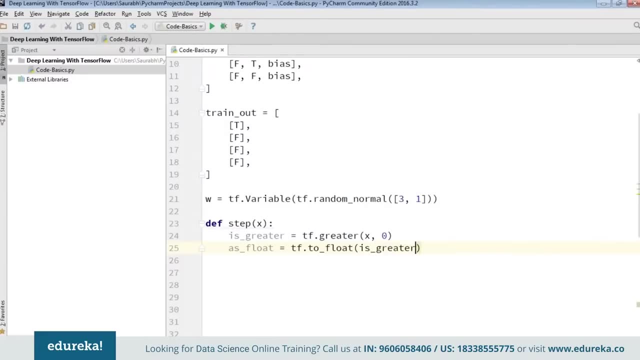 TF a dot to Underscore float Is underscore greater, Then we're going to define one more variable, doubled equal to TF a dot. multiply As underscore float comma two, Then return TF dot subtract Double comma one. So now this is how we have defined our step function. 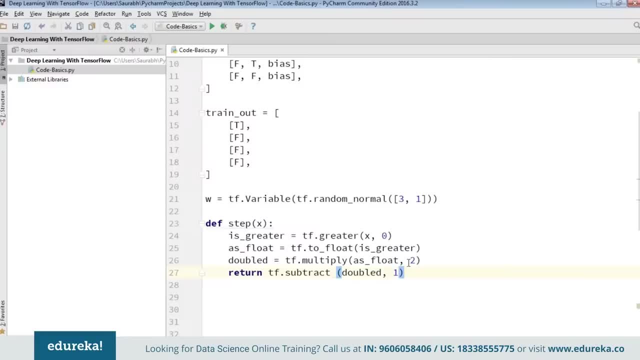 So with the step function defined, the output error and the mean squared error of our model can be calculated in one short line each. Let me show you how you can do that. So just type in here output equal to call that function. that is step. 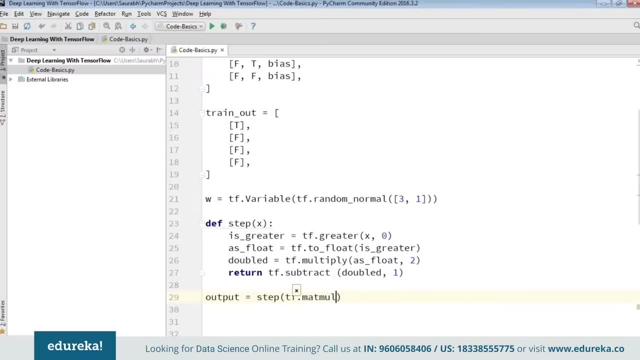 TF dot matrix multiplication matmul Train Underscore in Comma W. Now for error. we're going to type in here: error equals to TF dot subtract Train underscore out Comma output. And for mean squared error I'm going to type in here: MSC. 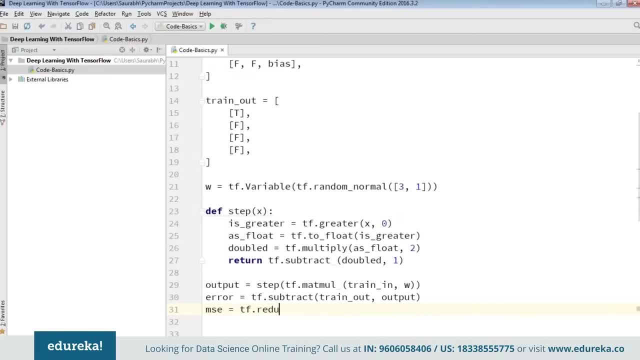 Equals to TF dot reduce, Underscore, mean, TF dot square, And then error. Now the evaluation of certain tensor functions can also update the values of variables, like a tensor of weights W. So in our case, basically we're going to update the weights W. 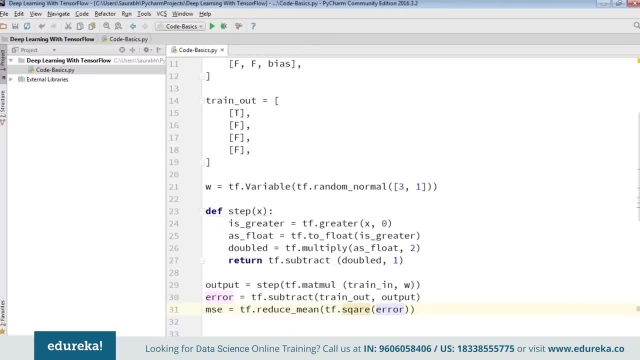 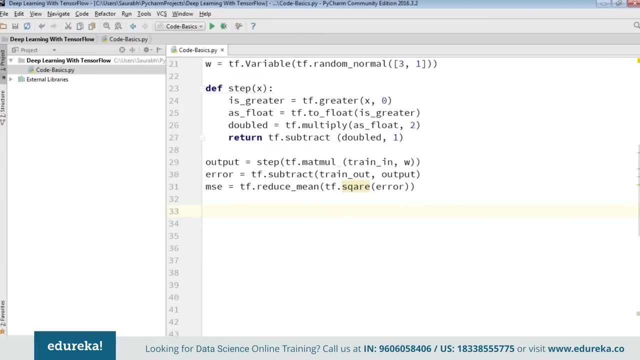 So first we calculate the desired adjustment based on error, Then we add it to W. Now let me show you how we'll do that. So, if you can recall, we have done that in the previous example as well, where we were updating the weights and bias. 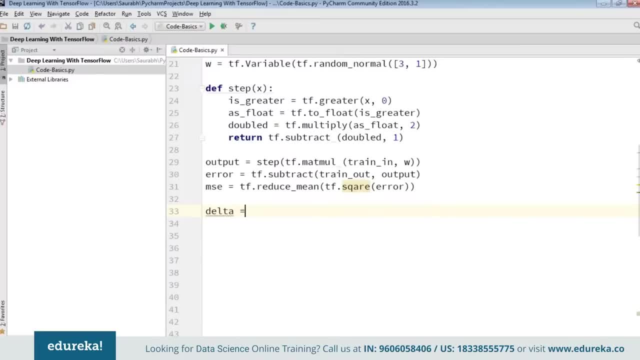 So now I'm going to type in here: Delta is equals to TF, dot matmul. or you can say matrix multiplication: Train underscore in Comma: error Comma transpose underscore a Equals to true. Then we're going to type in here: train equal to. 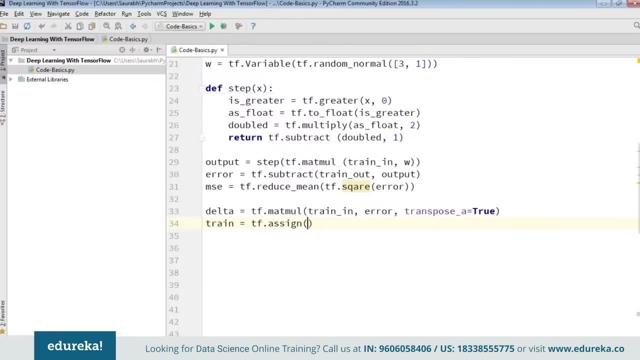 TF Dot. assign W comma TF dot. add W comma Delta, The first matrix multiplication, and then we're going to add it all. The model has to be evaluated by tensorflow session, which we have seen earlier as well. But before that, 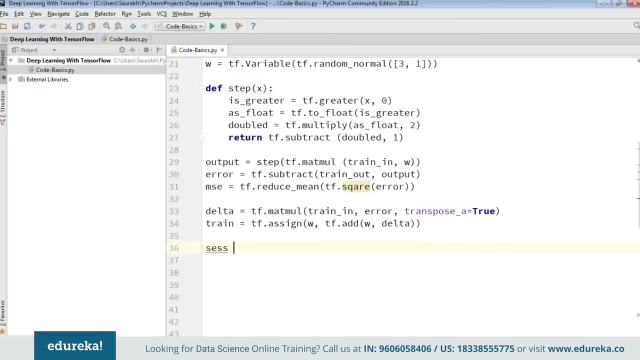 we also need to initialize all the variables. So first let me just type in here: says equals to TF dot session. And then I'm going to type in here: Access dot. run, TF dot. initialize- Underscore all variables. So now what our next task is in order to perform various iterations. 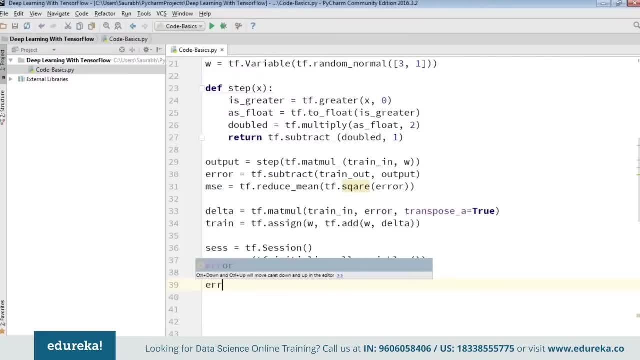 so that we get zero error. So what we're going to do, we're going to define a variable ERR and our target. So, basically, our ERR is nothing but error, which can be equal to one or zero, Because we are using binary output. 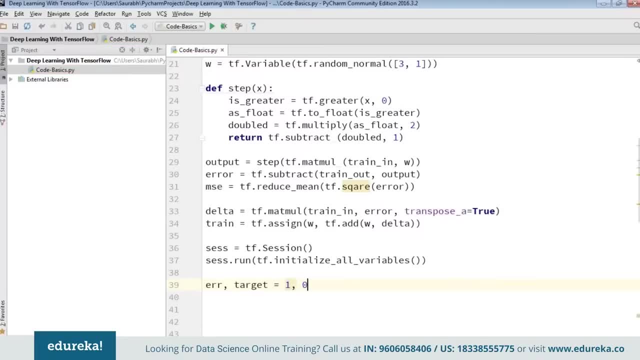 So our error can be one, and our target is to make it as zero right now. Next, what we're going to do, we're going to define a park Now. you can consider right now a park as nothing but the number of cycles. 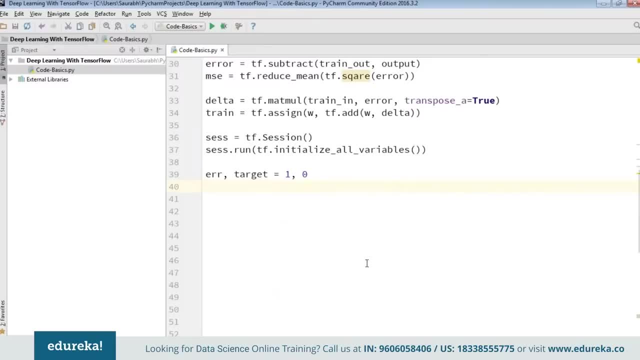 or you can say number of iterations that will be required in order to reach the desired output, or you can say: in order to reduce the error to zero. So I'm just going to define that, So I'm going to type in here: a park, or you can give whatever variable name. 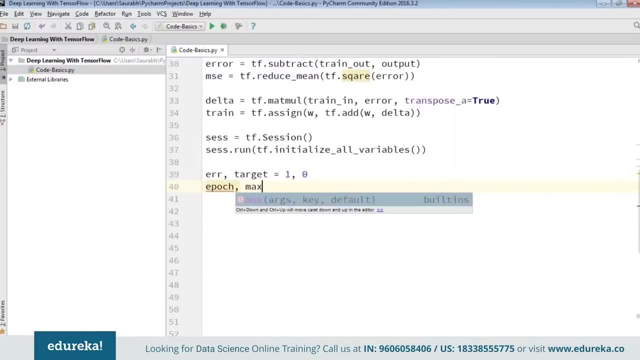 you want, and I'm going to type in here: Max underscore: A park Equal to zero comma 10, which means that our it will start from the zero I park and our maximum value of a park will be 10.. Now 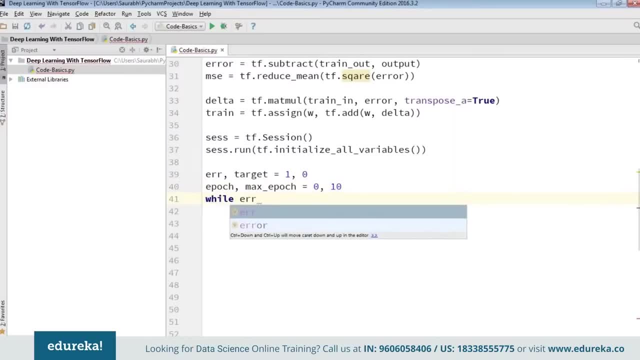 I'm going to define. while ERR should be is greater than target And a park is less than maximum, a park- Increase the value of a park. Why one? Then they'll type in: ERR Says dot run, Mean squared error, comma train. 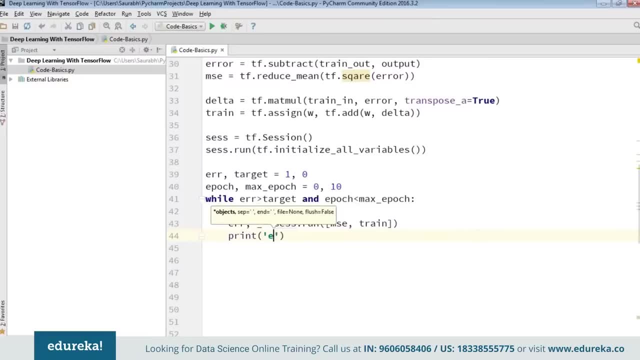 And let's just finally print it and see what happens. Print a park, Mean squared error, Colon ERR. So basically, what it will print? it will print the cycles or a park and the error with respect to that particular cycle. So let us go ahead and execute this and see what happens. 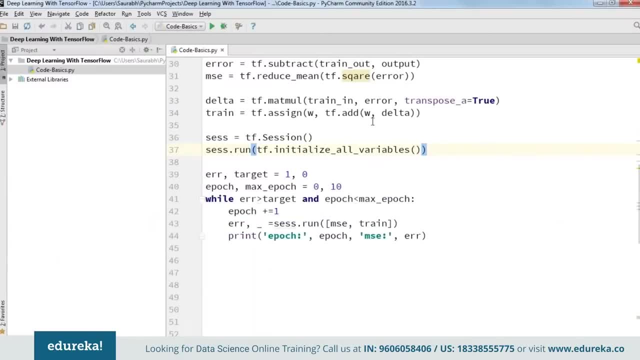 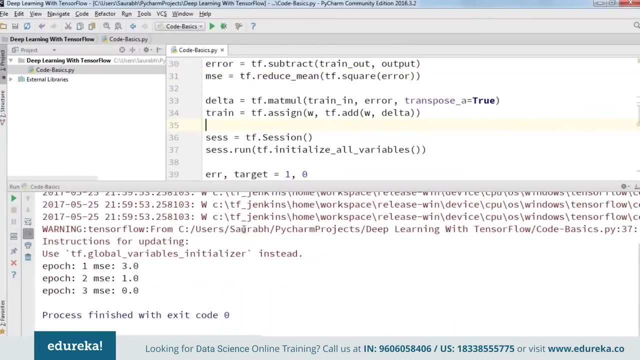 Oops, I've typed the spelling of square wrong. Pardon me for that. I'm just going to make it right now. SQ, you are e? All right, let's go ahead and execute it once more. So yeah, in three epochs. 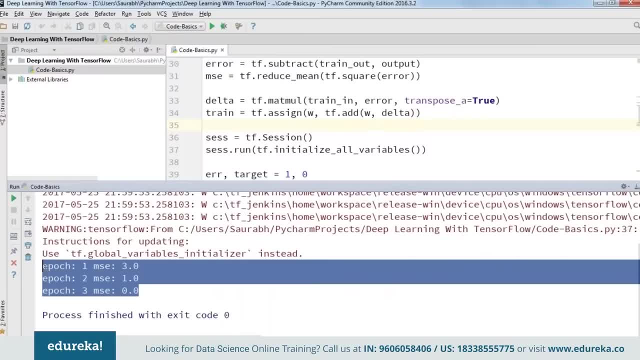 we got the value of mean squared error as zero. That means it took us three iterations in order to reduce the output to zero. So this is how you can actually implement a logic gate. or you can say: this is how you can actually classify the high and low. 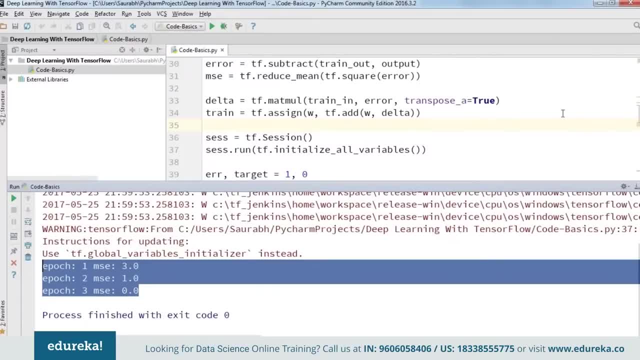 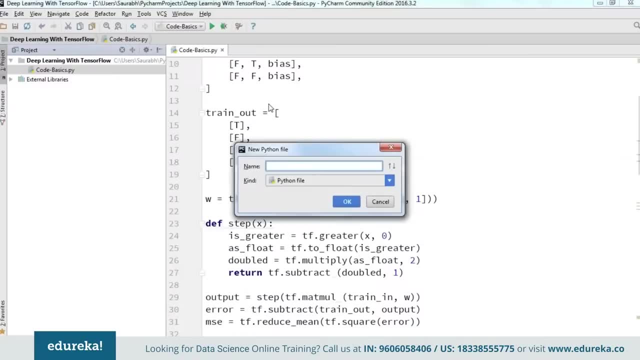 Outputs of a particular logic gate using single-layer perception. Similarly, you can do that for all gate as well. So what I'm going to do? I'm going to create a new python file and I'm going to name it as MNIST. 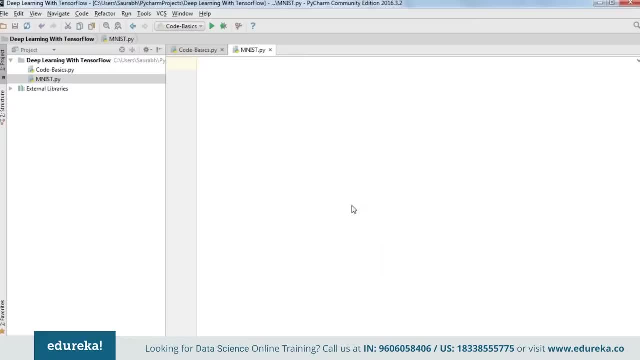 which is nothing but the data set on which we are going to perform the classification of handwritten digits. So we're going to execute a use case and we have told you earlier as well. in this MNIST data set, We have handwritten digits between from 0 to 9 and it has 55,000 training sets as well as 10,000 test sets. 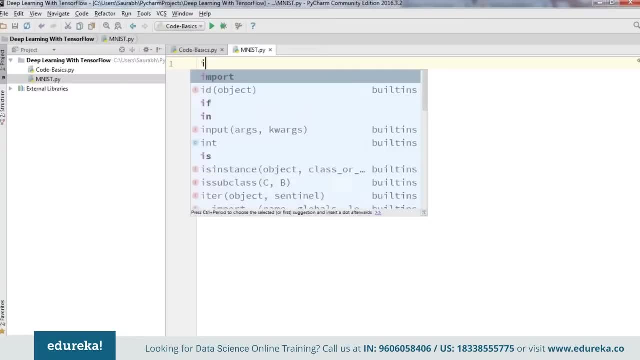 So let's go ahead with that. The first thing I'm going to do is download the data set, But before that let me just import tensorflow library as TF. and yeah, now let us download the data set. So for that I'm going to type in from tensorflowexamplestutorialmnist: import input underscore data. 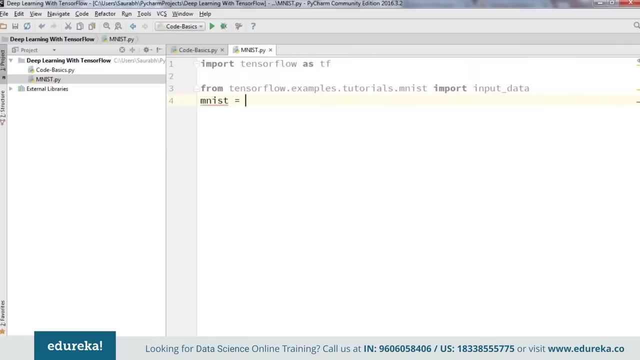 And now I'm going to type in here: MNIST is equals to input underscore data And this underscore data dot read data sets. Type in here: MNIST underscore data. Comma 1. underscore hot equals to true. Now here, MNIST is nothing but a lightweight class. 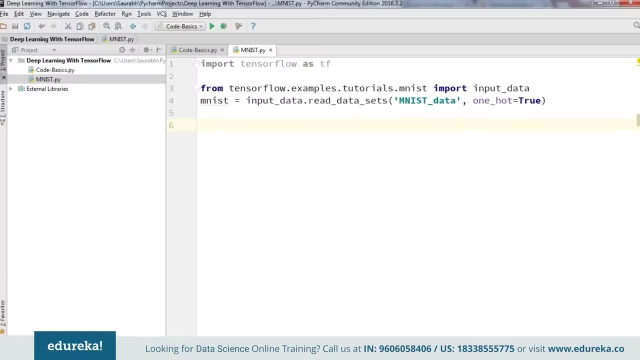 which stores the training, validation and testing sets as and numpy Y address. And when I talk about this, one hot equals to true, is nothing but one hot encoding. Now let me tell you what one hot encoding is. So for that, let me just comment few lines. 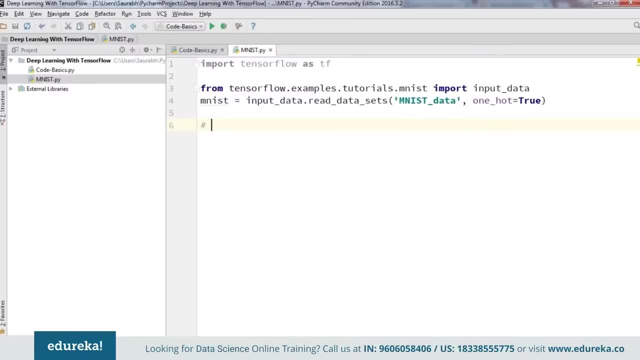 So one hot encoding means that if I'm classifying something as a 7, so if I classify that my digit is 7, so how am I going to represent that? So I'm going to type in here: 0, 1, 2, 3, 4, 5, 6, 7th. a bit will be active. 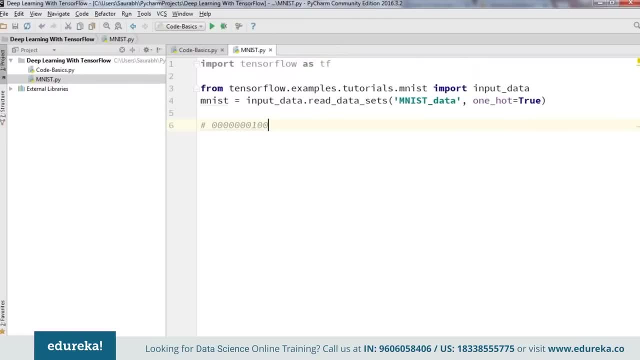 So I'm going to type in there one, then eight and then nine. Similarly, if I want to represent, say, that my digit is 2, so I'm going to type in 0, 1. on the second digit, I'm going to type in here as one and the rest all zeros. 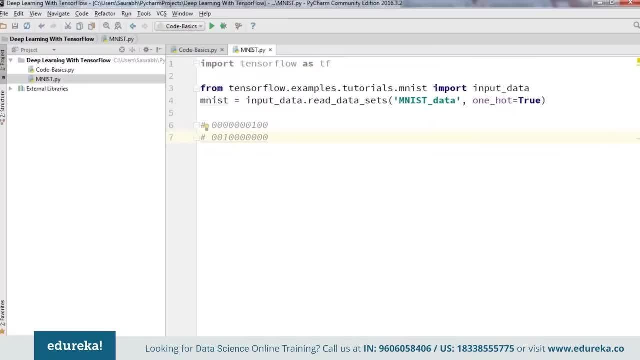 So I hope you got the concept of what exactly one hot encoding is. So it's like only one output is active at a time. That's all. So our next step is to start the session, like we do every time. So I'm going to type in here: says equals to TF dot interactive session. 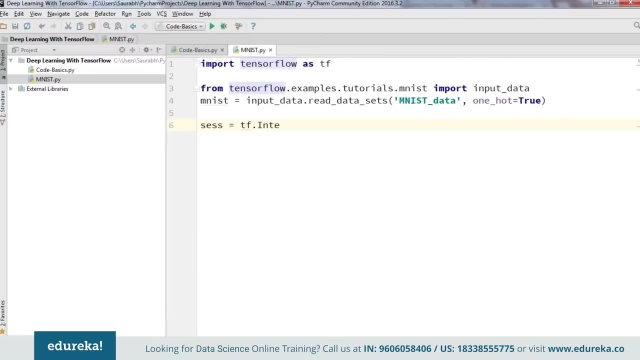 So I'm just going to type in here: interactive session, Yeah, And now we are going to do, we're going to build the computation graph by creating nodes for the input images and target output classes. So for that I'm going to define some placeholders for that. 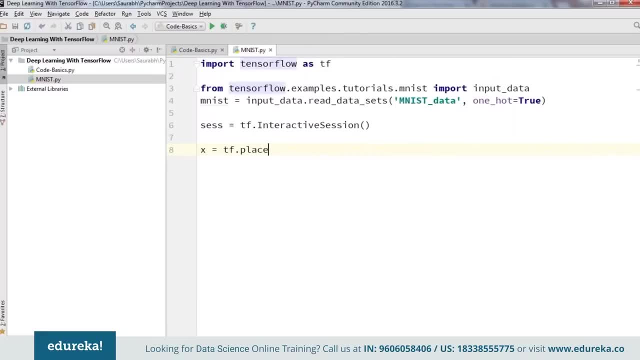 I'm going to type in: X is equals to TF, dot, placeholder, TF dot, floor 32.. And the shape will be none comma 784.. Now the input images X will consist of 2D tensors of floating-point numbers. Here we assign it a shape of say none comma 784, as you can see. 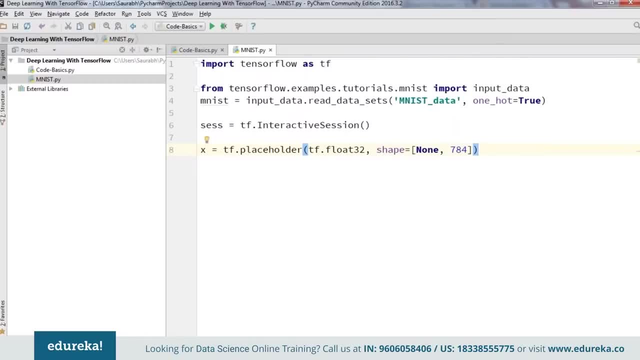 So where 784 is the dimensionality of single flattened, 28 by 28 pixel MNIST image of handwritten digits. And what none indicates? It indicates that the first dimension corresponding to the batch size can be of any size. Means the first dimension can be of any size. 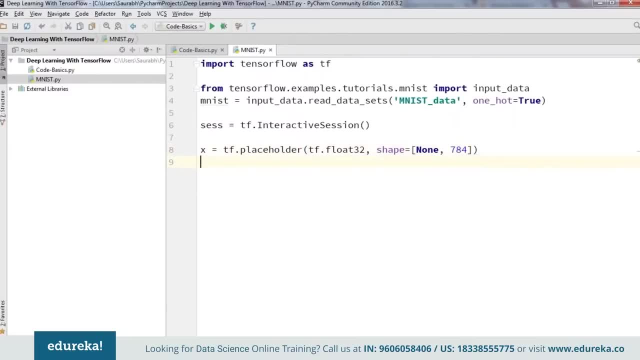 We are not putting any restrictions on that. Now I'm going to define the variable Y, which will nothing, which will be nothing but our real labels, or you can say the desired output placeholder, and I'm going to type in here: TF, dot, float 32.. 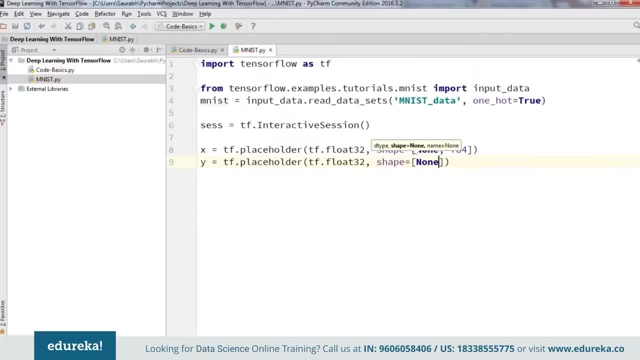 And I'm going to define the shape, which will be none comma 10, because we have 10 classes. And similarly, Y is also a 2D array where each row is one hot 10 dimensional vector indicating which digit class the corresponding MNIST image belongs to. 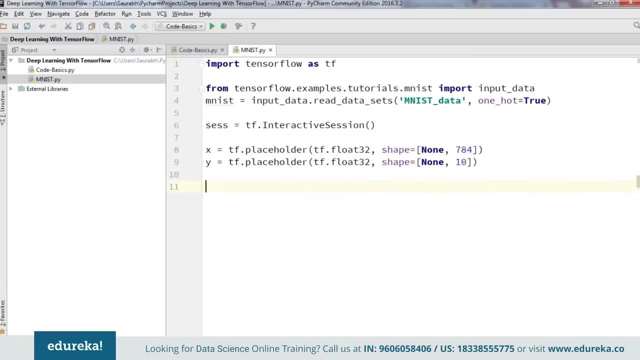 And now next step is to define weight and biases for our model, like we have done in the previous example. So we could imagine treating these like additional inputs, but tensorflow has even a better way to handle them, and what it is? it is nothing but variables. 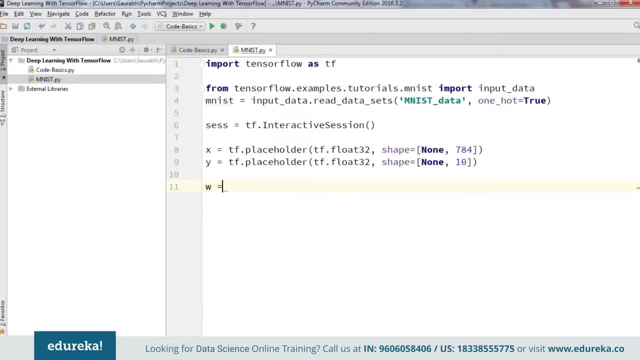 So let us go ahead and do that. I'm going to type in here W- TF dot variables, TF dot zeros. I'm going to initialize it to zeros and the shape will be a 784 comma 10.. So it's like 28 cross, 28 pixels and a 10 classes. 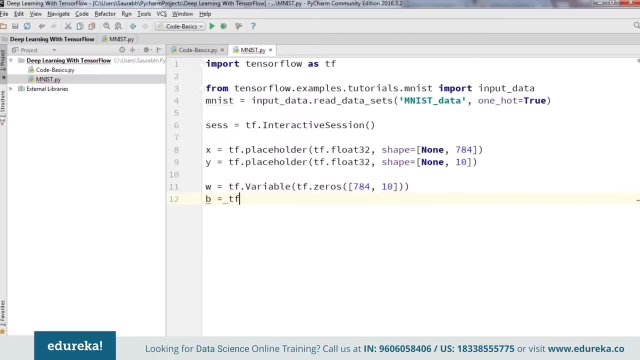 Similarly when I talk about bias. so it will be TF dot variable. TF dot zeros. initialize it to zeros and the shape will be 10.. We pass the initial value for each parameter in the call to TF dot variable. Now over here, as we can see that we initialize both W and B as tensors full of zeros. 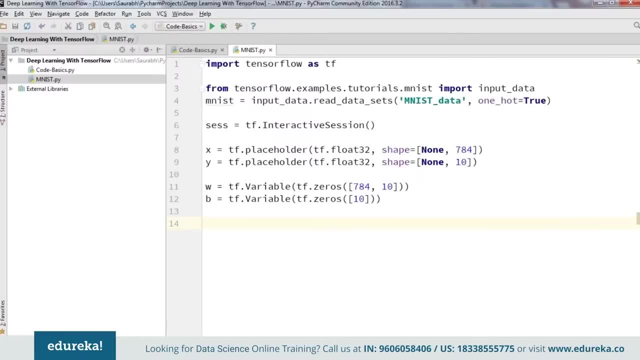 and W is a 784 cross 10 matrix because we have 784 input features and 10 outputs. And when I talk about bias B, it is a 10 dimensional vector because we have 10 classes And we have learned that before we can use variables in a session. 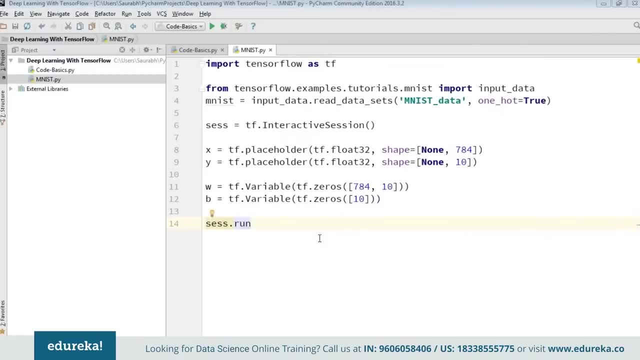 We need to first initialize it. So we're going to type it here: says a dot run, and after that I'm going to type in TF, dot. global underscore variables- Underscore initializer. All right, so we have initialized all the variables. 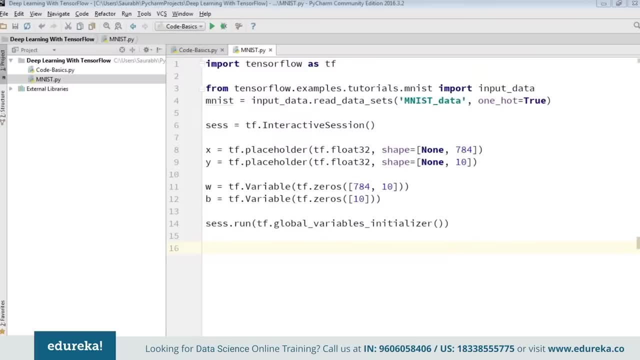 So our next task is to predict the class and the loss function. So we can now implement a regression model. It takes only one line. We multiply the vectorized input image X by the weight matrix W And add the bias. So for that I'm just going to type in here: Y equal to TF, dot matma. 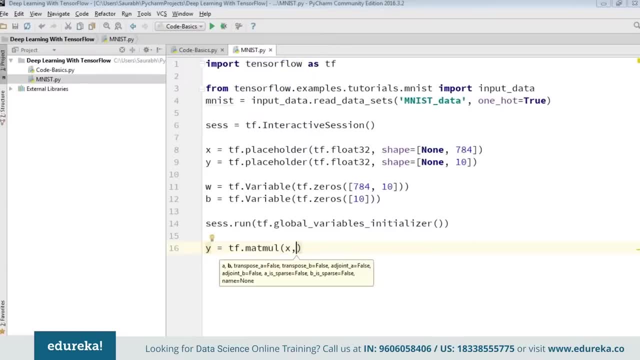 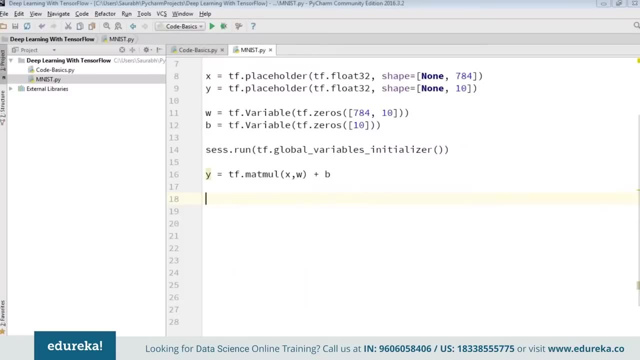 That is nothing but matrix multiplication X, comma, W plus B. All right, So now we can specify a loss function very easily. So the loss indicates how bad the models prediction was on single example. We try to minimize that while training across all the examples. 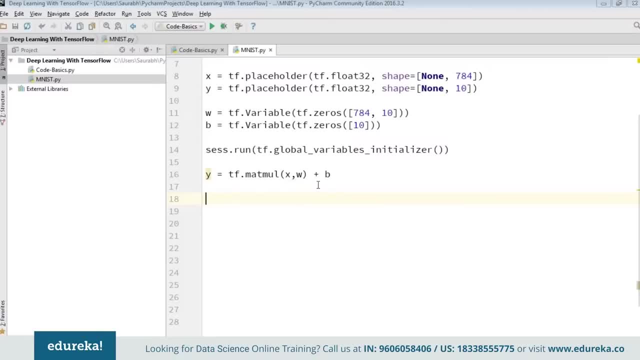 So now we can specify a loss function. now loss indicates How bad the models prediction was on a single example and we try to minimize that while training across all the examples. Now, here our loss function will be cross entropy, or you can say the difference between the actual output and the predicted output. 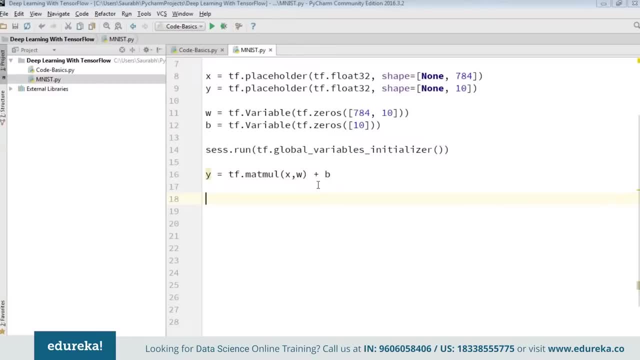 So for that, what I'm going to do, I'm going to you make use of softmax cross entropy function. So here the loss will be the difference between the target output and the actual output. So, for that, what I'm going to do is I'm just going to type in here a variable name. 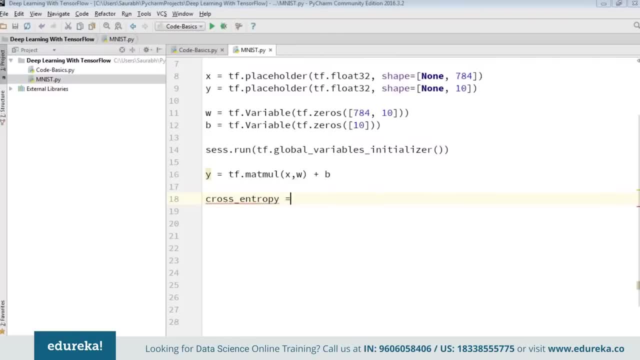 I'm going to name it as cross entropy. And yeah, entropy equals to tf dot, reduce, underscore, mean. And then just type in here. Let me just enter the next line: tf dot, nn, dot, softmax, underscore, cross entropy with logits. And now over here. 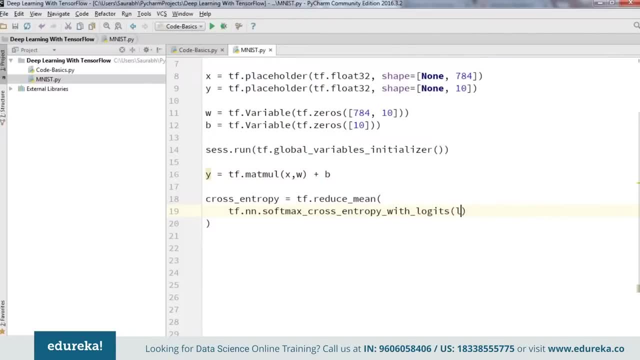 I'm going to type in first our target output, which will be labels equals to Y, comma, our actual output, So it'll be logits. It's is equals to Y. that's all So over here. let me just give you a brief idea. 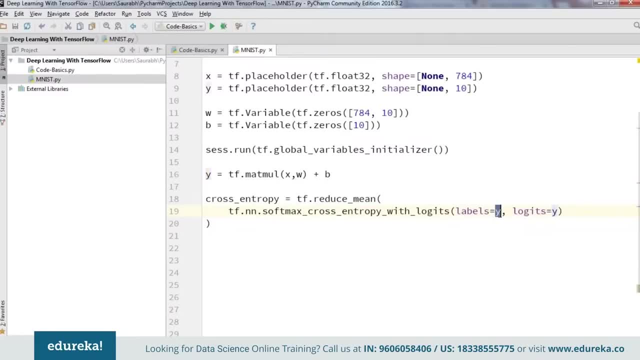 What is happening? So labels is equals to Y means that this is our target output and this is the actual output. So it will be, will name it as Y underscore, And so what exactly is happening? It will calculate the difference between the target output and for the actual output. for all the examples: 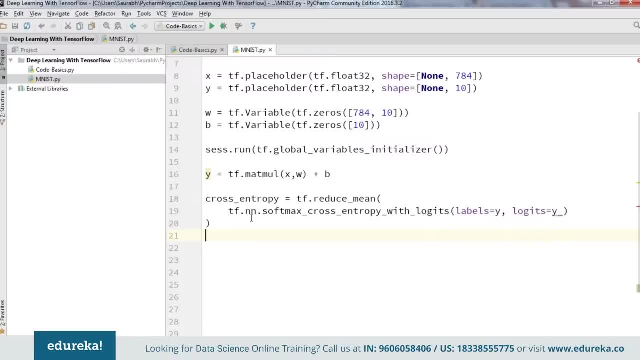 then it is going to sum all of them and then find out the mean. So this is what, basically, this cross entropy variable will do, Now that we have defined our model and training loss function. It is straightforward: We're going to train using tensorflow. 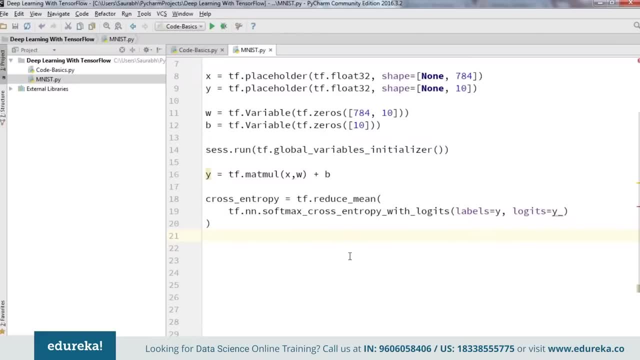 Now we need to train our model, So tensorflow has a wide variety of built-in optimization algorithms, as I've told you earlier as well, And for this example, we'll use steepest gradient descent with a length of about 0.5 to descend the cross entropy. 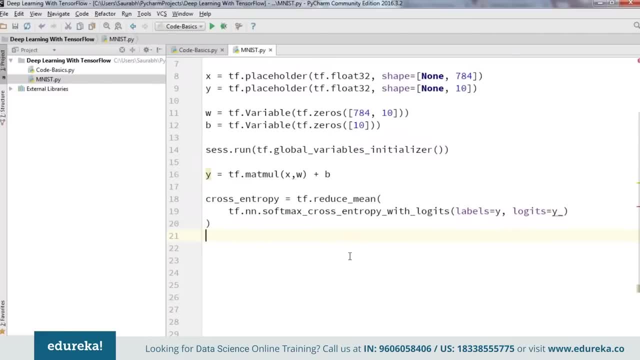 So basically we're going to use a 0.5 learning rate or you can say the step length. So for that I'm going to type in here: train underscore, step equal to tf dot, train Dot, Gradient descent optimizer and the step will be 0.5 and minimize a loss. 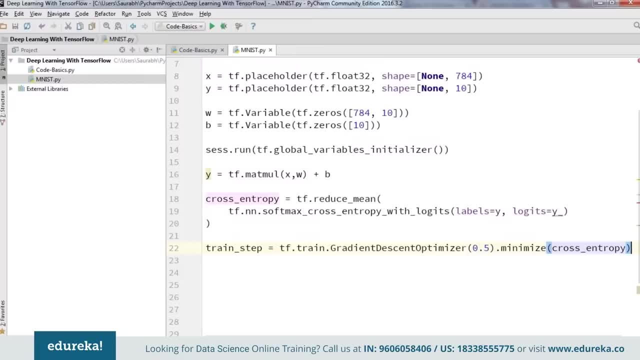 So minimize cross entropy. That's it. So what this one line basically will do, it will minimize the cross entropy, which is nothing but the loss function that we have defined. now, in the next step, What we are going to do, We are going to load hundred training examples in each training iteration. 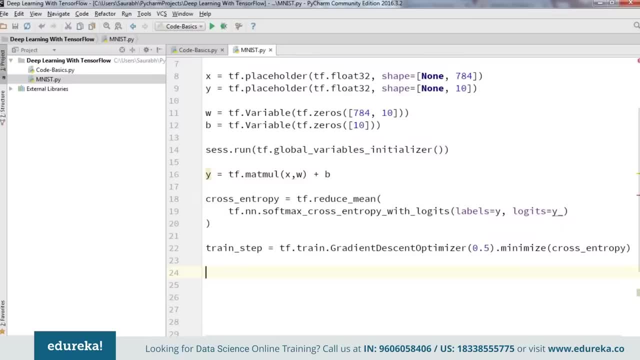 So each time the training iteration happens, it will take hundred examples. We then run the train underscore Step operation, which is nothing, but to reduce the error using feed underscore dict, which is nothing, but we are going to feed the real values to our placeholder. 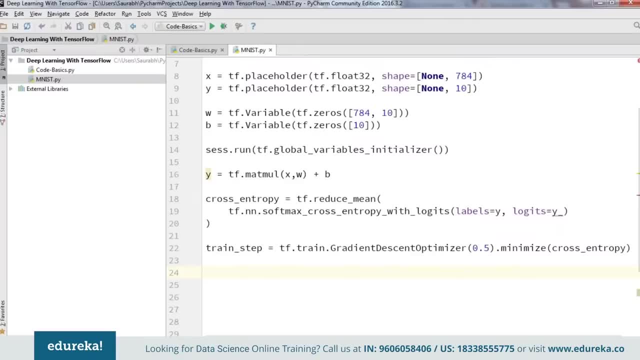 Why now? next, what we are going to do? We're going to load a hundred training examples in each training iterations, which means that for each iteration will take hundred training examples and will run the train underscore step operation, which is nothing but the optimizer here and after that. 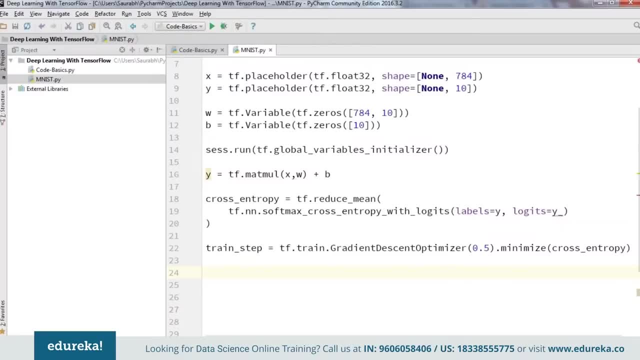 we are going to use a feed underscore dict to replace the placeholder tensors X and Y with the training examples. So basically, X will contain the input images And Y will contain the actual outputs, or you can say the desired outputs. for that I'm going to type in here for underscore in range thousand. 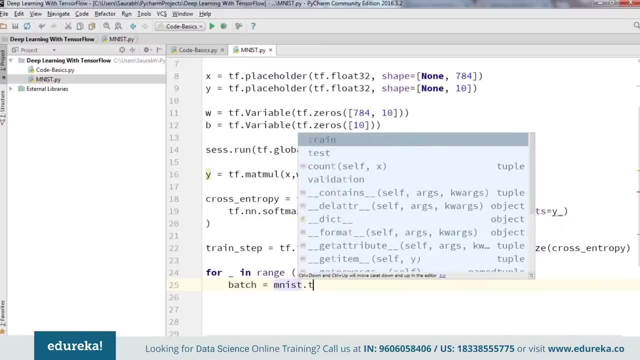 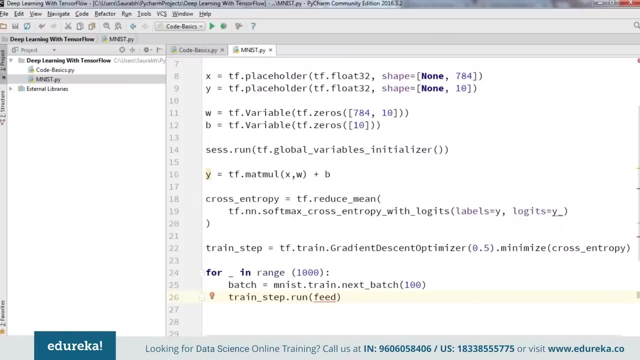 Batch equals to MNIST dot train dot Next. underscore batch hundred. train. underscore step dot run. and I'm going to feed in the values to X and Y variable feed. underscore dict equal to X colon Batch zero. comma Y colon batch one. That's it. 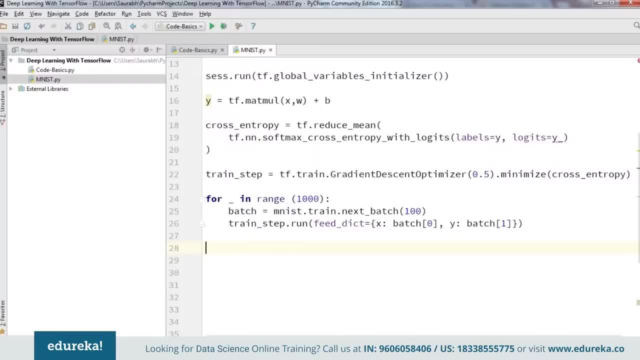 Now we need to evaluate our model. We need to figure out how well our model is doing, and for that I'm going to make use of TF dot argmax function. Now, this TF dot argmax function, Let me tell you how it works. first, 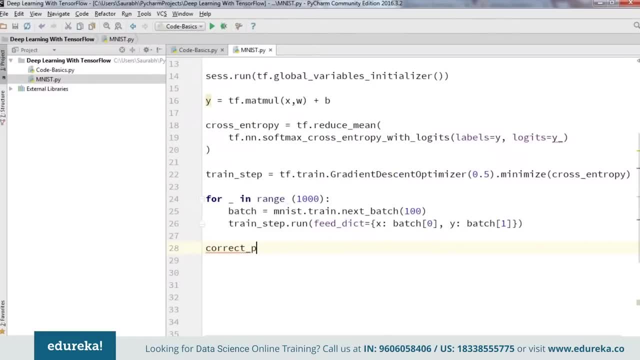 I'm going to type in here: Correct Underscore prediction Equals to: TF dot. equal TF dot argmax Y underscore comma one, Comma TF dot argmax Y, comma one. So basically, this TF dot argmax of Y underscore comma one is a label. 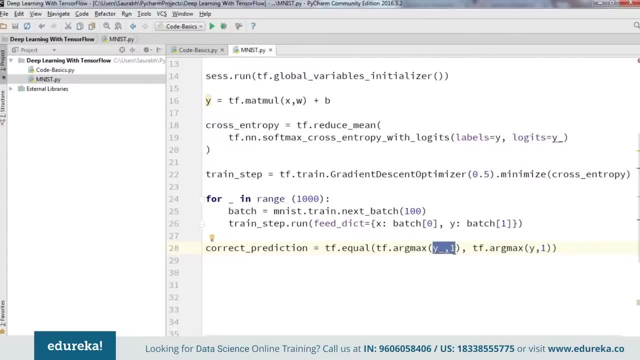 Our model things is most likely. for each input That means it is a predicted value, While TF dot argmax of Y, comma one is a true label. It is there in our data set present already and we know that it is true. So what we are doing? they're using TF dot equal function to check if our actual prediction matches the desired prediction. 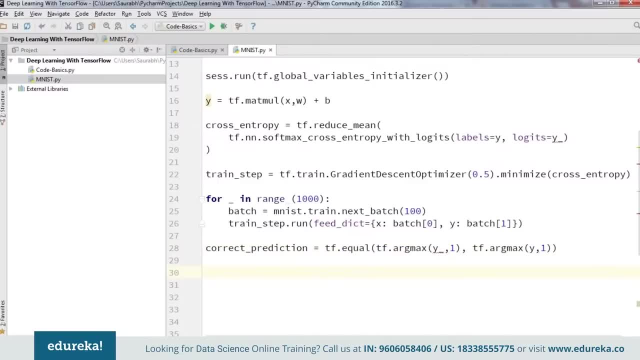 This is how it is working. So now what we're going to do? we're going to calculate the accuracy to determine what fraction are correct. We cast a floating point numbers and then take the mean repeat. So now I'm going to define a variable. 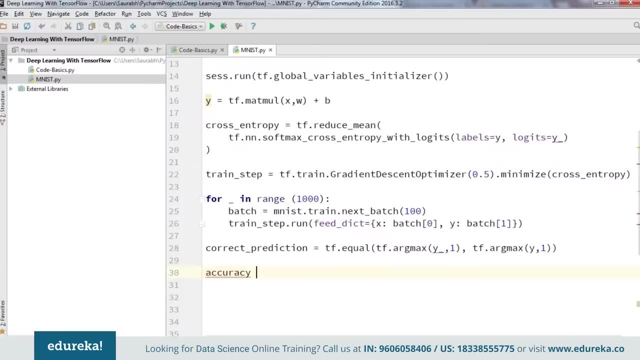 For accuracy. So just going to type in: accuracy equals to: TF: dot. reduce underscore mean TF, dot. cast correct underscore. prediction Comma: a: TF a dot, float 32.. And what we can do? finally, we can evaluate our accuracy on the test data and this should give us accuracy of about 90%. 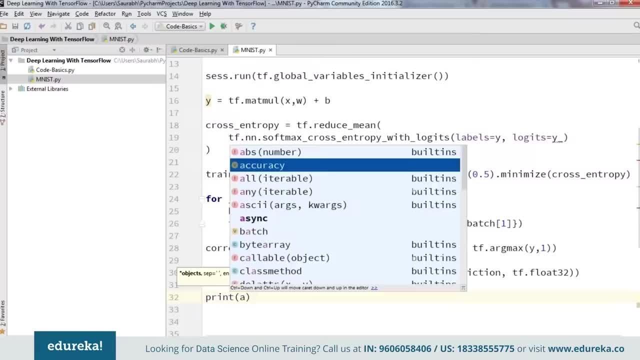 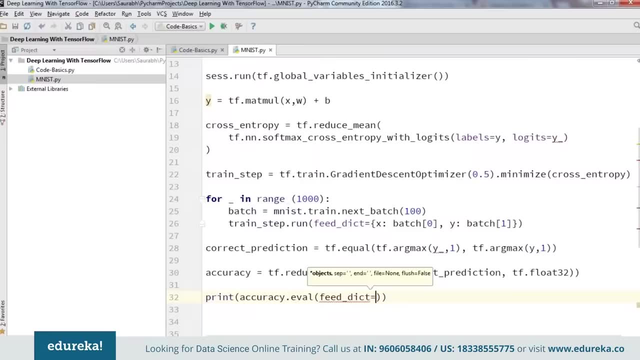 So let us see if that happens. I'm going to type in here: print: Accuracy dot- evaluate eval feed. underscore dict: Equal to X colon MNIST dot test dot images. Comma Y colon MNIST dot- test dot labels. That's it, guys, and I've done a mistake here instead of Y. 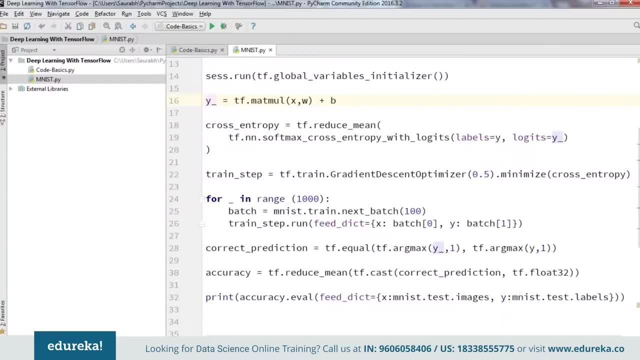 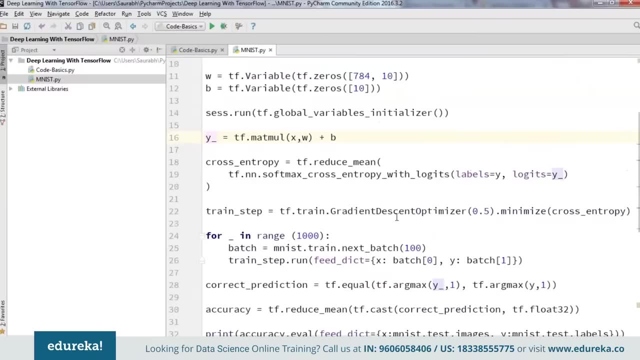 It will be Y Underscore, because this is our predicted value, not the actual value, and why we have considered as actual value and this Y underscore will be our predicted values. This is the mistake that I made. So, yeah, now I think the code looks pretty fine to me and we can go ahead and run this. 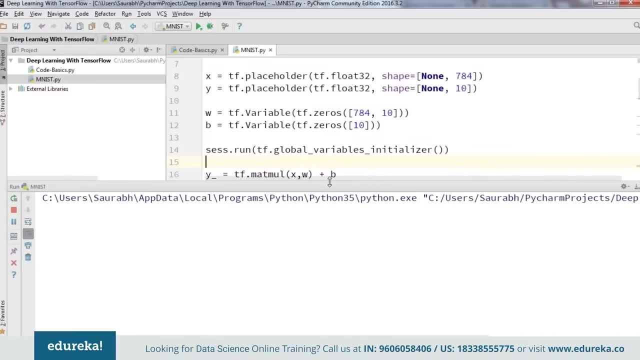 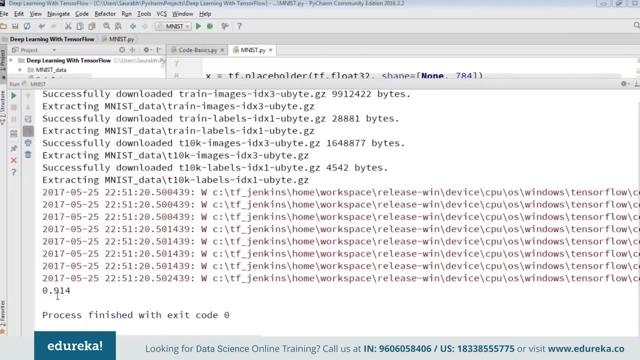 Let us see what happens when we run this. So, guys, it is complete now, and this is the accuracy of a model which is 91.4%, And which is pretty bad, though, when you talk about a data set like MNIST, but yeah, with a single layer. 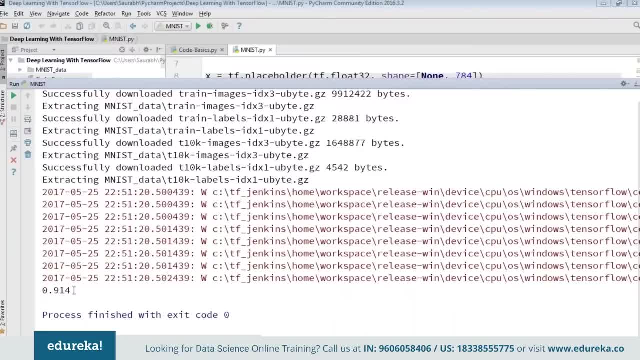 which is very, very good. So we have got an accuracy of around 92% on the MNIST data set, which means that whatever the test data sets were there, that is like 10,000 test images. So on those test images, whatever the prediction our model has made, are 91.4% correct. 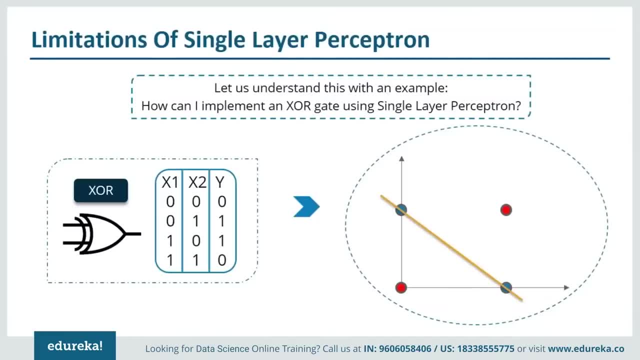 So now there are certain limitations of single layer perceptron. Let us understand that. So, in order to understand that, we will take an example. So we have an XOR gate here and this is a truth table. So, according to this truth table, 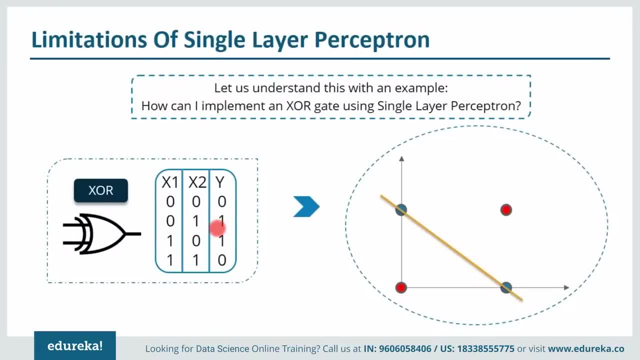 if any one of the input is high, then the output is high, and if both the inputs are low, output is low, and if both the inputs are high, output is low. So how can you classify the high and the low outputs with a single line? 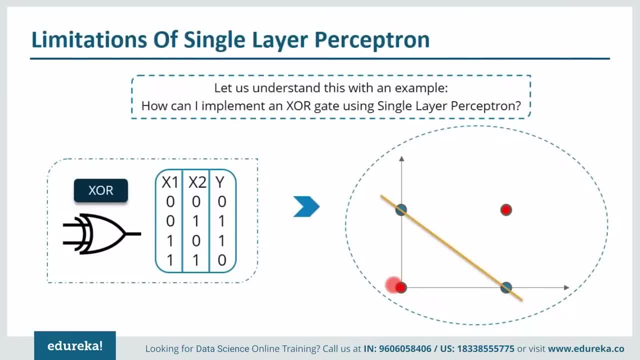 Definitely you can't, if you see the points. So one point is here, one is here, here and here, and which? these two points are high outputs and these two are low. So how can you classify with a single line? Definitely you can't. So now what's the answer to this? 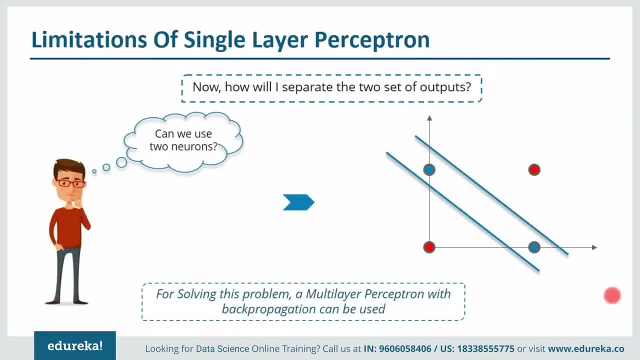 What if we use multiple neurons? using multiple neurons, We can have two lines that can separate it. Now we can solve this problem if we have multiple neurons. So if we use two neurons, we can have two lines and that can actually separate the high outputs as well as the low outputs. 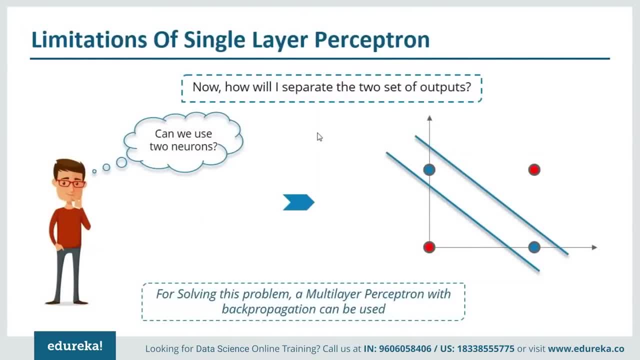 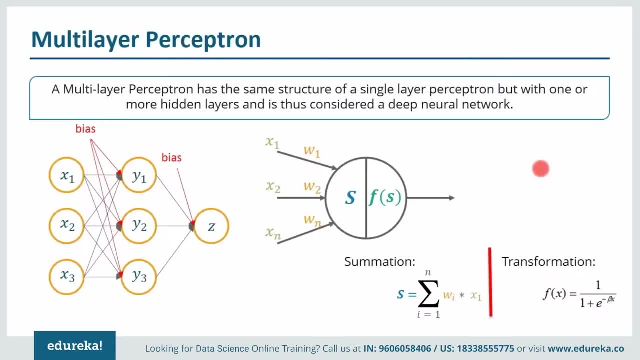 So this is where we use multi-layer perceptron with back propagation. So what are multi-layer perceptron, multi-layer perceptions? They have the same structure like the single-layer perceptron. The only difference is they have more than one hidden layer. So let me explain it to you with an example. 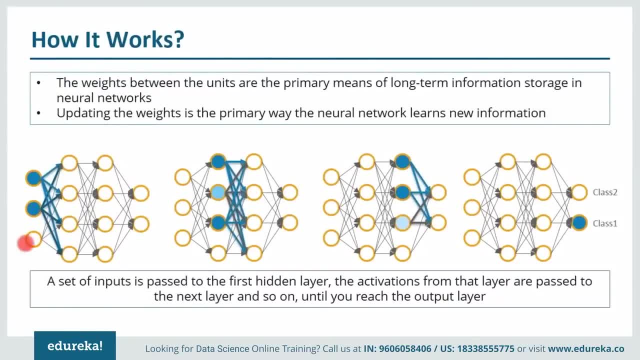 So this is how a typical multi-layer perceptron looks like. So we have input layer, We have two hidden layers and we have one output layer as well. Now, typically, each of these input layers are connected to the next hidden layer. Each neuron is connected to the next neuron present at the adjacent layer. 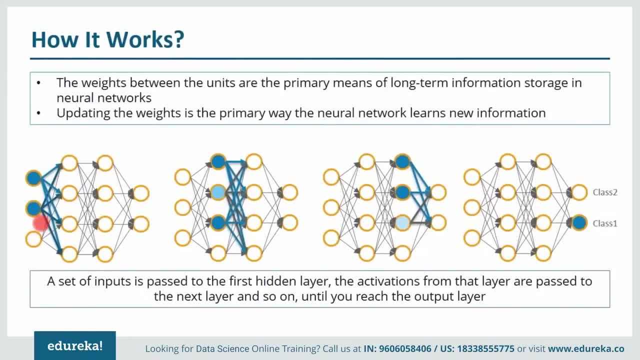 but the neurons of the same layer are not connected to each other. Now what happens? a set of inputs are passed to these input layers and the output of this input layer will be passed to the first input layer And the output of this input layer will be passed to the first input layer. 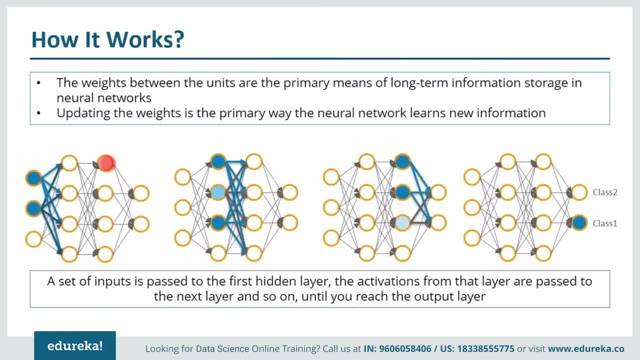 Then, after activation function of the first hidden layer, the output will be passed to the next hidden layer as the input and similarly, finally, we get the output. Now you must be thinking how the model learns from here. So the basically, the model learns by updating the weights, and the algorithm that it uses is called back propagation. 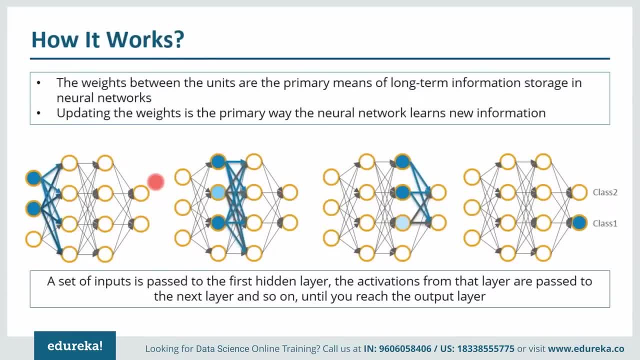 So the back propagation algorithm helps the model to learn and update the weights in order to increase the efficiencies. So basically, at this process of from input layer to the output layer is called a feed forward process And then, when we back, propagate it in order to increase the efficiency or accuracy so that we can update the weights. that is called as a back propagation. 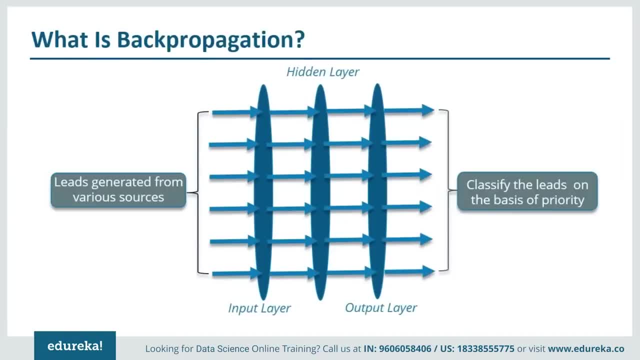 So let us move forward and understand what exactly is back propagation. So what is back propagation? Now let us understand this with an example. So we'll take the inputs as the leads generated from various sources, And my aim is to classify the leads on the basis of the priority. 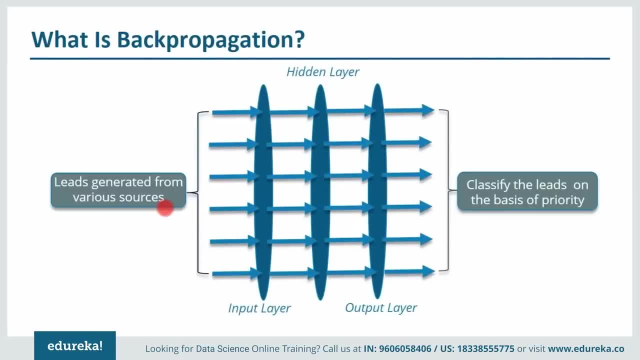 So there might be certain leads which won't make it that much difference to me, Whereas compared to the other leads. So in that case I need to make sure the leads which are important gets the highest amount of weight. How am I going to do that? 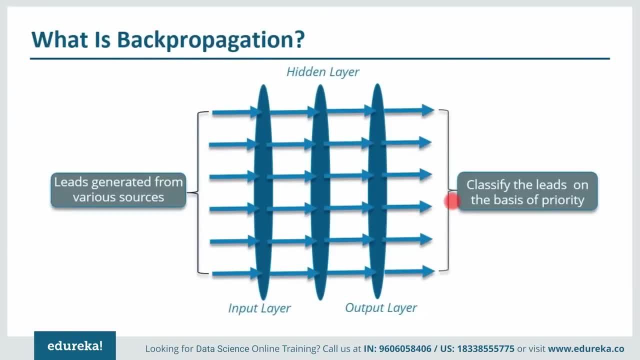 First we'll see the output that, accordingly, will calculate the error and, based on that error, We are going to update the way, and this process is nothing but your back propagation. in a nutshell, I can say right, Although the algorithm is pretty complex. 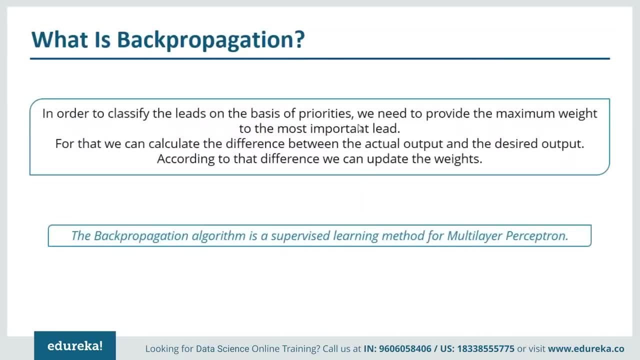 but yeah, this is basically what happens. So, in order to classify the leads in the basis of priorities, we need to provide the maximum weight to the most importantly. and how are we going to do that? We're going to compare the actual output and the desired output and, according to the difference, 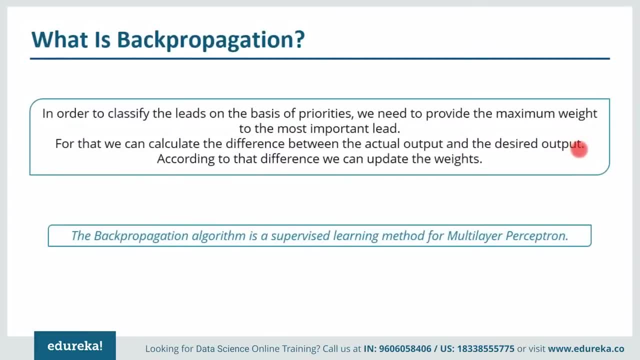 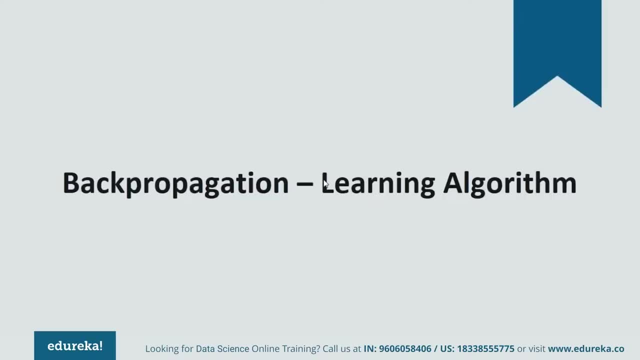 we can update the weights. So what is back propagation? So back propagation is nothing but a supervised learning algorithm for multi-layer perceptron. Now let us understand what exactly is this algorithm. Let us understand this with an example that is there in front of your screen. 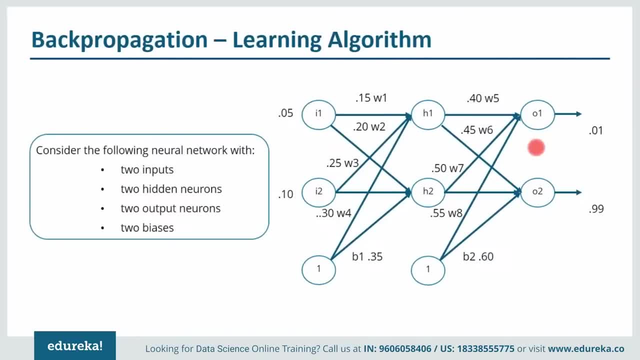 So these two are our input neurons, These two are our hidden neurons and these two are our output neurons. Now our aim is to get point zero one and point nine nine as our output and at the same time, we have inputs as point zero five and point one zero. 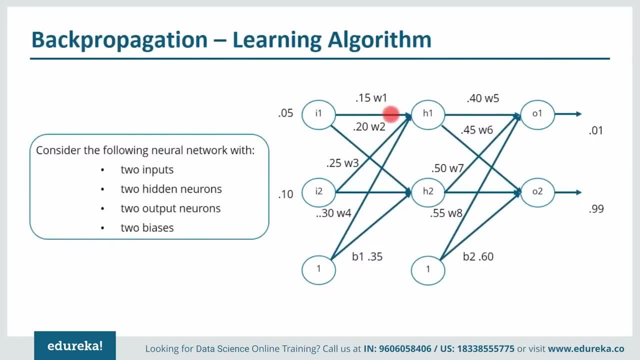 Initially, we take the weights as we can see it here. So point one: five w one, point two: zero w two. So these are the weights. plus we have two biases as well. Now what we need to do is we need to make sure that we have weights in such a way that we get output as point zero one and point nine nine. 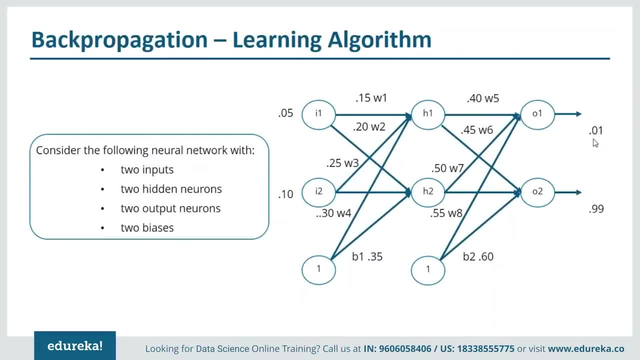 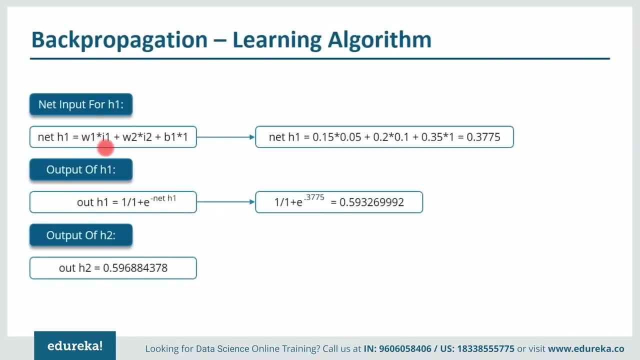 But let us see if we get that same output. when we provide these kind of weights, The net input for this particular H1 will be what It will be: W1 into I1.. That is the first input, plus W2 into I2, plus B1.. 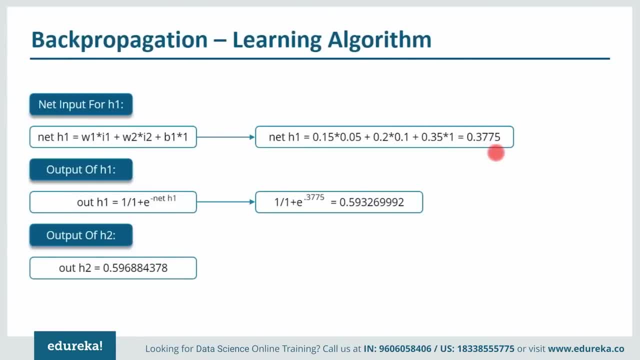 One into one, which gives us the answer as point three, double seven, five. Similarly, the output for H1 will be nothing but the activation function, the output and after the activation function. and we are using her sigmoid function because our brain also uses a sigmoid functions. 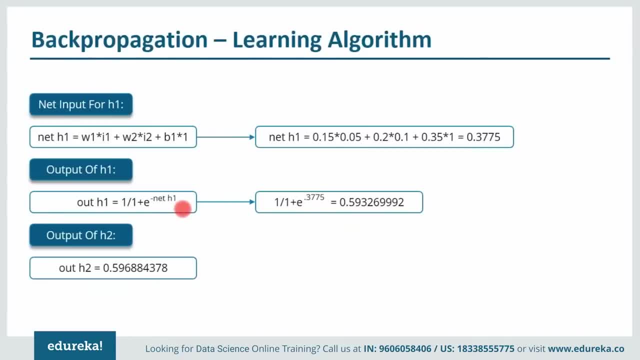 That's what we believe in. and at the same time it is easily differentiable, And if you differentiate it twice you get the same number. So the output of H1 will be point five nine something. So let me go back. So the output of this particular H1 will be point five nine something. 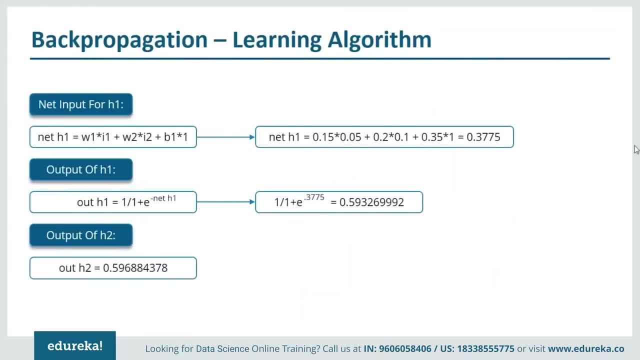 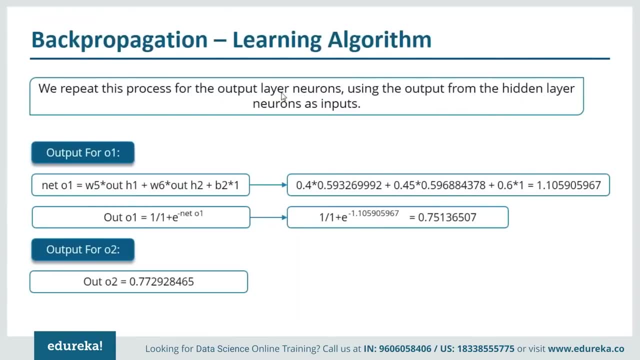 Then we're going to calculate the output of H2 as well, Similarly, and we get the output as point five, nine, six, double, eight, four, three, seven, eight. next up, We are going to repeat the process for the output layer neurons as well. So for the output layer the net input will be W5 into out of H1, W6 into out of H2 plus B2.. 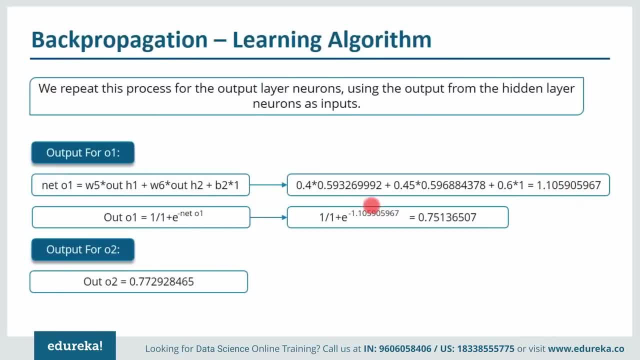 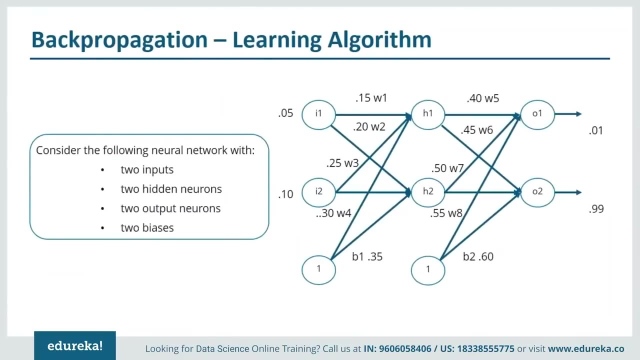 That is the bias. So we get the output somewhere like this, and then the net output for out O1 will be after the activation function, which will be point seven five one. similarly, the output for O2. Will be point seven seven. Now, if you notice that this is not the desired output, our desired output was point zero one and point nine nine. 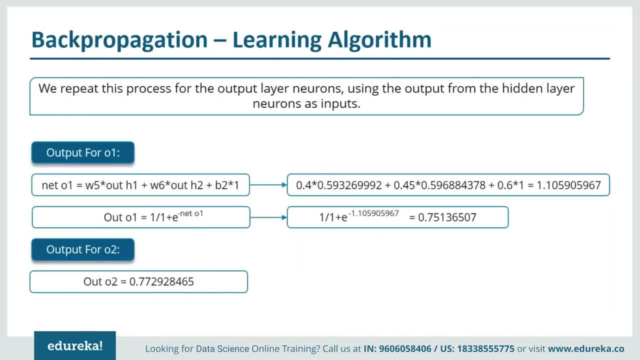 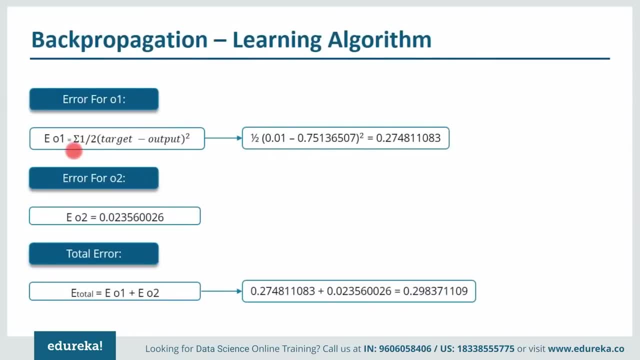 What we got. instead, we got point seven five and point seven seven. So what we need to do, we need to update the weight. So for that we're going to calculate the error now. error for output: O1 is nothing but the Sigma of one by two. target minus output. whole square target is nothing but your desired output. 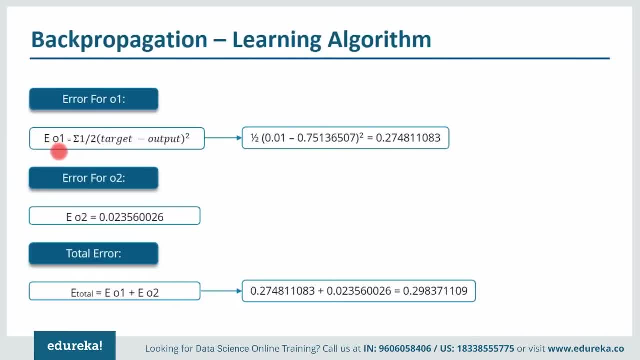 and output is your actual output. So your error of output of O1 neuron Will be point two, seven, eight. similarly, for O2 will be point zero, two, three. So the total error comes down to point two nine something next up. We need to update the weight so as to decrease this error. 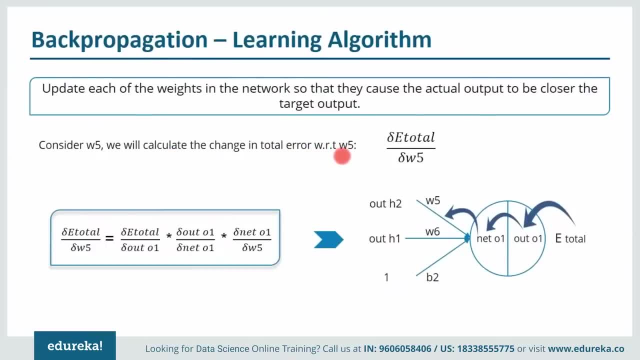 Now what we're going to do. We're going to first calculate the change in total error with respect to any of the random weight. will take W5, for example, just to show you. so we're going to calculate the change in the total error when we change with respect. 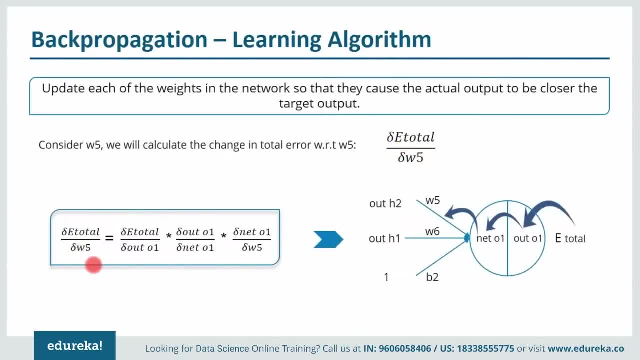 to the weight W5.. So we're going to apply a chain rule here. So using partial derivative, We're going to calculate E total by Delta of auto, one into Delta of auto, one by Delta of NATO, one, and then Delta of NATO, one by Delta. 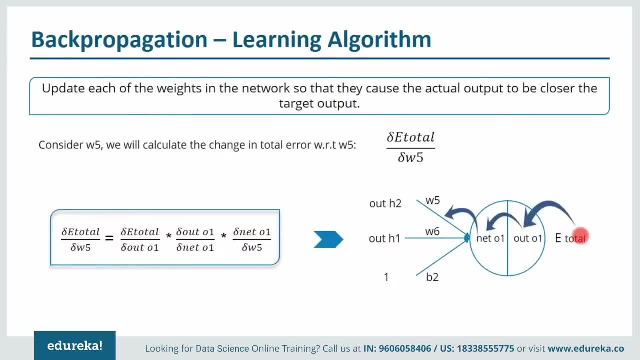 of W5. as you can see it from this particular example as well: E total, change in E total with respect to auto one, change in auto one with respect to NATO one and change in NATO one with respect to W5.. We're going to multiply that and we're going to get this particular term, and let us see how we do that. 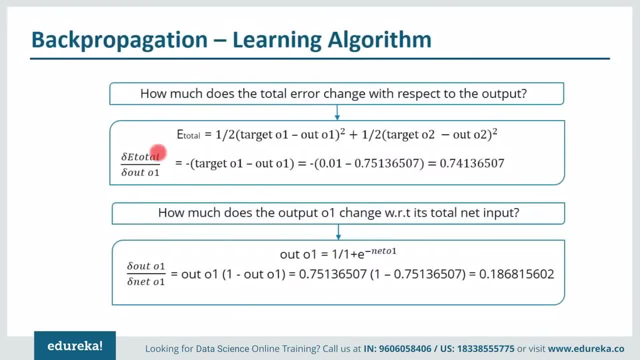 So how much the total error change with respect to the output, E total by E out one. We're going to calculate it. It came around point seven four one. Similarly, We're going to calculate how much this output, or one, change with respect to the net output. 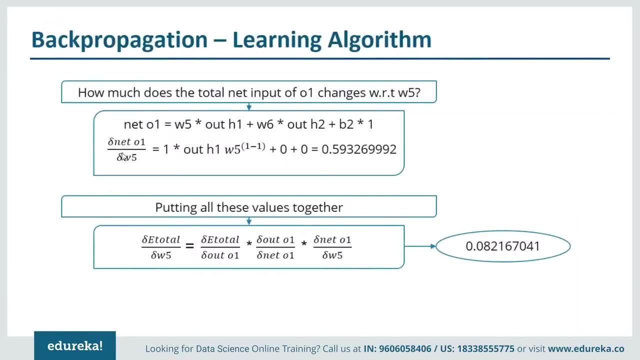 and we get this. after that, We're going to calculate it for net output change with respect to W5.. Also, we got this and then, finally, what we did: we put all these values together and we found out to change in the error with respect to the change in weight W5. 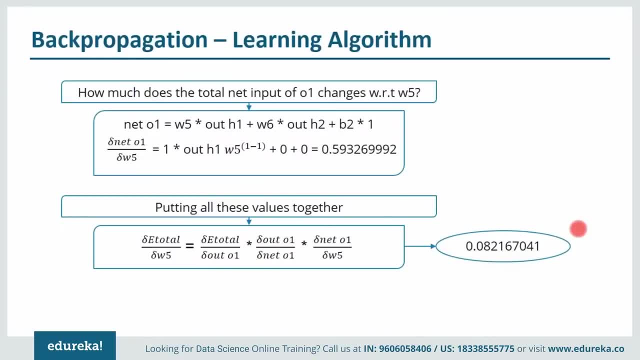 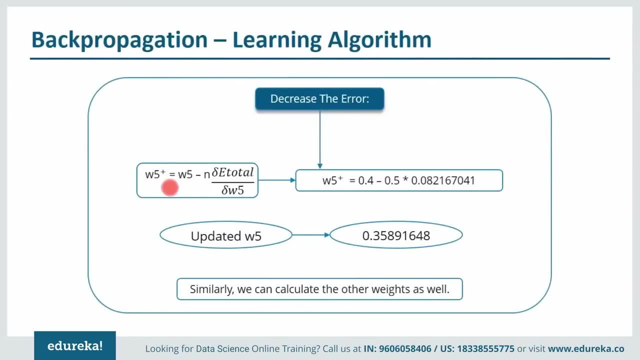 which came to up around point zero eight two one. six seven zero four one. Now is the time to update the weight. So how are we going to update the weight? First thing we need to do is we need to follow this formula, So W5.. 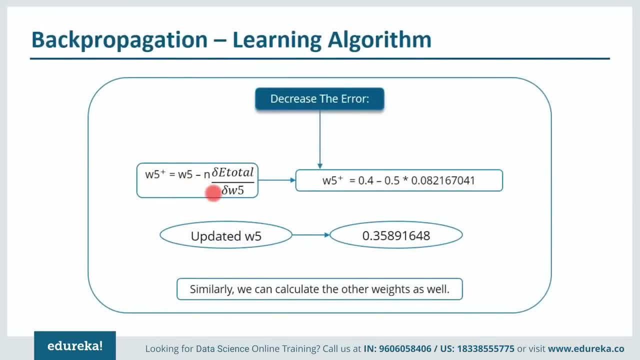 Plus is nothing but the updated weight, which is equal to W5, minus the learning rate into Delta of E, total by Delta of W5.. So which came to around a point: three, five, eight, nine, one, six, four, eight. similarly we can calculate the other weights as well. 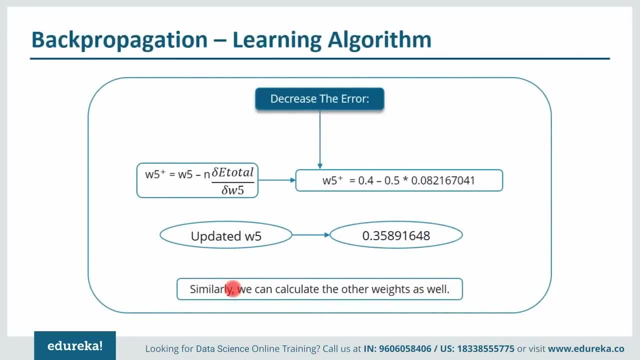 So we're going to repeat the same process and we're going to calculate the other weights as well. Then again we're going to see how much is the loss. if still the loss prevails, then we're going to repeat the same back propagation learning algorithm again, for all the ways. 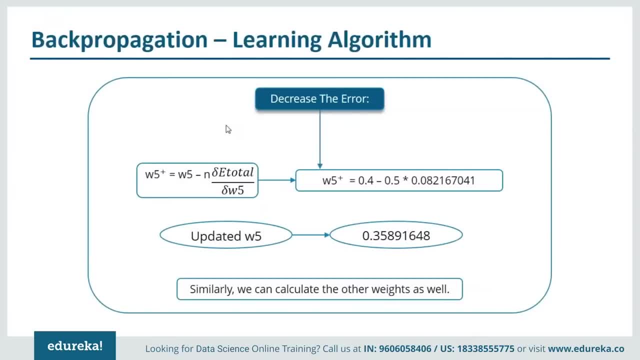 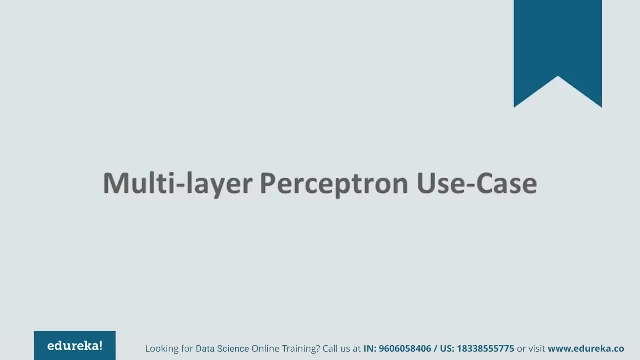 So this process will keep on repeating. So this is our back. propagation actually works. So now what I'm going to do? I'm going to make use of the same MNIST data set and I'm going to increase the efficiency of that data set by 97 to 99% with the help of multi-layer perceptron. 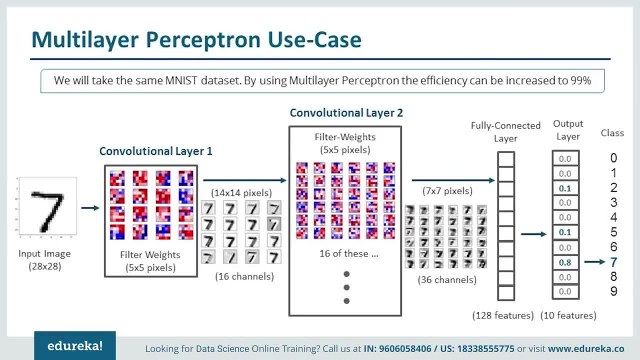 So, guys, let us go ahead with that. So, guys, as I've told you earlier, is where we are going to use the same MNIST data set which we have used in the single layer perceptron. So I'm going to perform a classification using multi-layer convolutional networks. 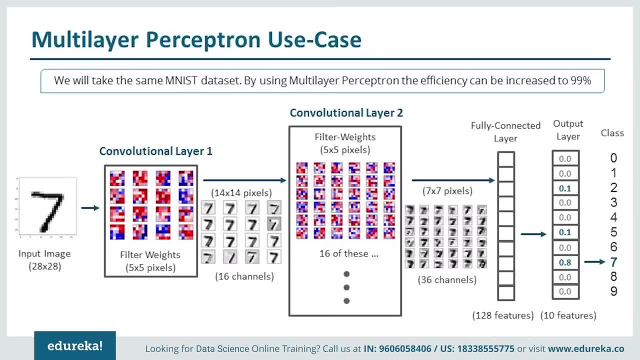 Now, what are convolutional networks? Basically, these networks Are used in order to classify images. So, basically, what I'm doing is I'm just trying to show you that- how we can increase the efficiency using the convolutional neural networks. You don't have to go in much detail about it, because we'll be learning about it in the upcoming modules. 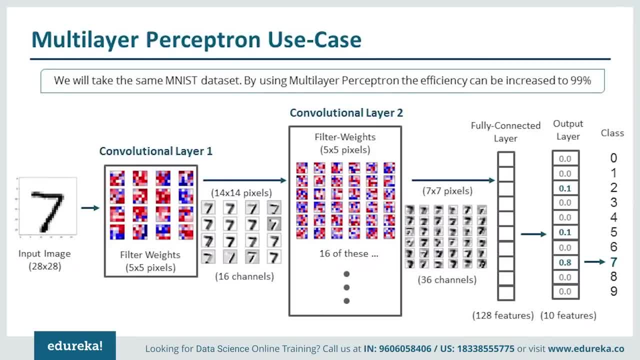 I'm just giving you a general overview, or you can say a taste of how things work in convolutional neural networks. So we give an input image to this convolutional network, Then this input image is processed in the first convolutional layer using the filter weights. 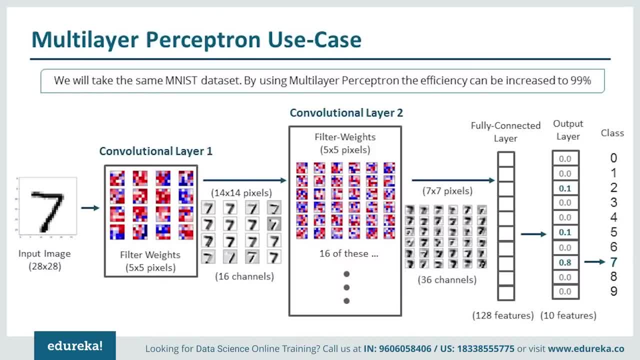 Now this result in 16 new images, One for each filter in the convolutional layer. The images are also down sampled, So the image resolution is decreased from 28 cross 28 to 14 cross 14.. Now these 16 smaller images, and from the first convolutional layer, are then processed in the second convolutional layer. 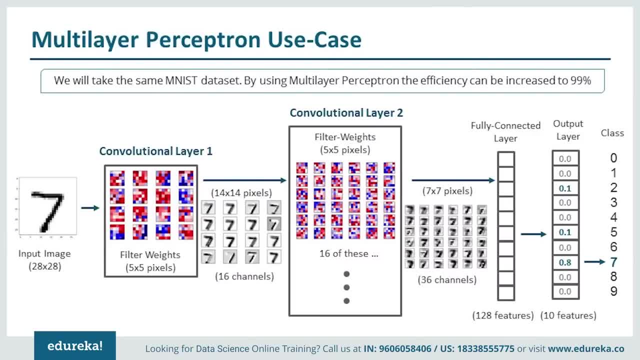 We need filter weights for each of these 16 channels and we need filter weights for each output channel of this layer. Now there are total 36 output channels. So there are total of 16 cross 36, equal to around 576 filters In the second convolutional layer. 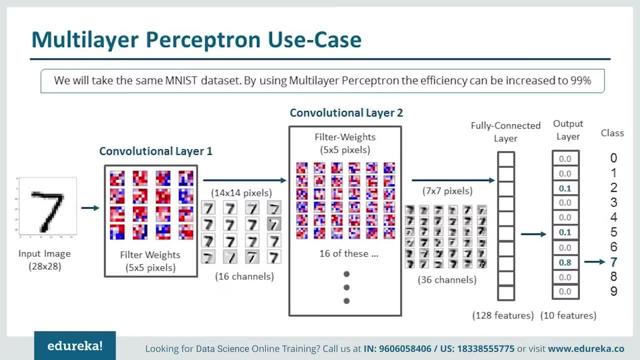 Now the resulting images are down, sampled again to 7 cross 7 pixels. The output of the second convolutional layer is 36 images of 7 cross 7 pixels each. Now these are then flattened to a single vector of length- 7 cross, 7 cross 36, which is 1764. 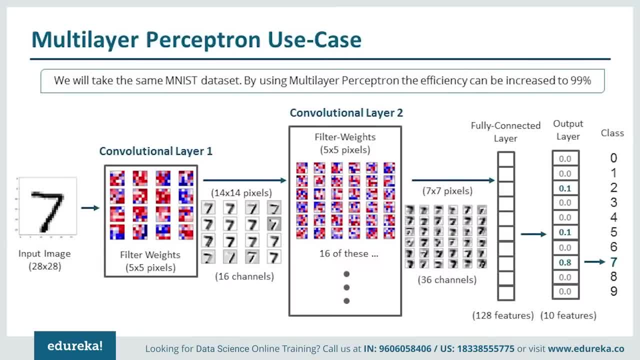 Which is used as the input to a fully connected layer with 128 neurons, And this feeds into another fully connected layer with 10 neurons, One for each of the classes, Which is used to determine the class of the image, that is, which number is depicted in the image. 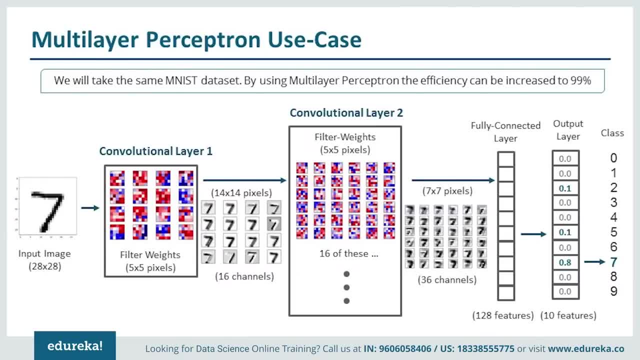 So whatever number that we provide in. So basically the output layer, or you can say the last layer or the fully connected layer with 10 neurons, is used to determine the class or which digit is the input image of. Now, the input image depicts the number 7, and the four copies of the images are shown here. 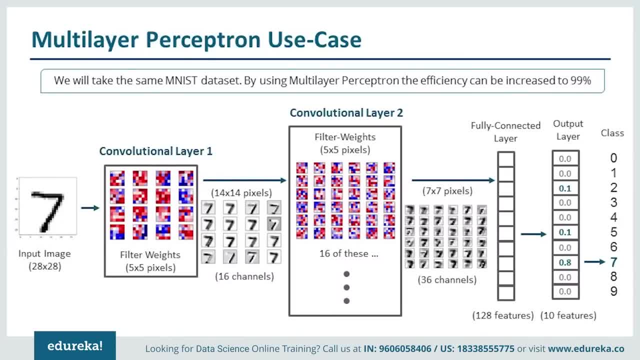 So, basically what happens, whatever filter we have in each layer, it will be present on the image pixels. So there'll be a dot product of the filter and the image pixel behind that. So we'll get A dot product there. We are going to repeat that same process in each of these layers and for each of these layers and for each of these images, and we are calculating the dot product. 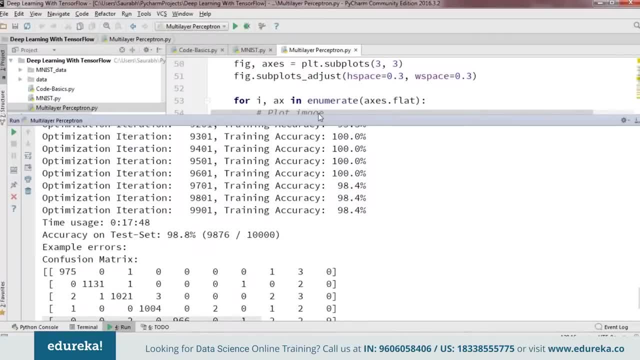 So let me just show you that we can increase the efficiencies. So I have already done the code and it will take time if I do it right now. So this is what the efficiency we ended up with. So it is 98.8 percent. 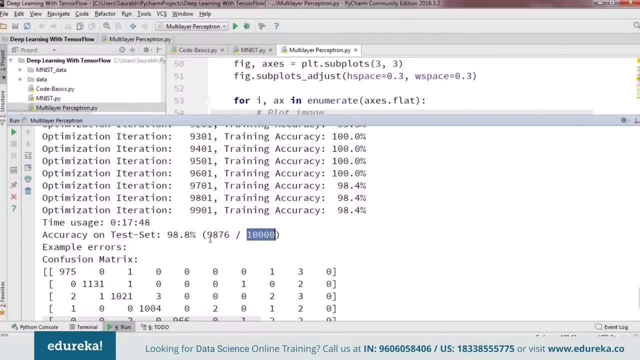 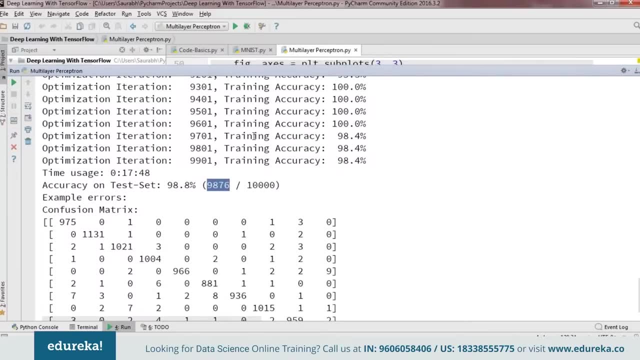 So, on the test sets, we had around 10,000 test samples, out of which we predicted 9876 correctly, So which is pretty good Actually, if you see so it because in the single layer perceptron example that we took, we were getting accuracy of around 92%, but here we are getting around 99%, which is actually very good. 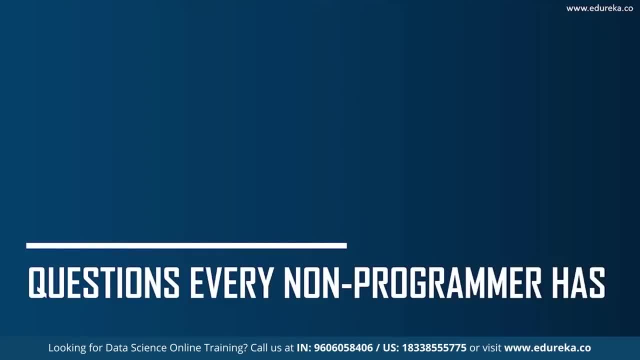 So now let's move on and discuss a couple of questions that every non-programmer usually has right about data science and machine learning. Now, guys, data science, artificial intelligence and machine learning might seem intimidating, But it isn't actually as complex as you might think. right, many of the tools that have been developed over the last decade or so have all helped to make artificial intelligence and machine learning more accessible to engineers with varying degrees of experience and knowledge. 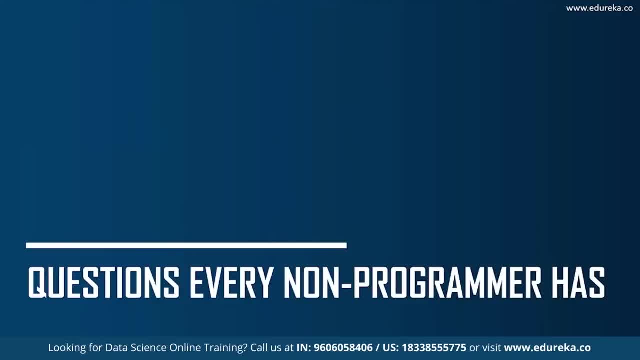 And today we've got to a stage where it's now accessible even to people who have barely written a line of code in their life. Now that's very exciting, But if you're completely new to the field, it can be challenging To know how to get started now as a beginner. 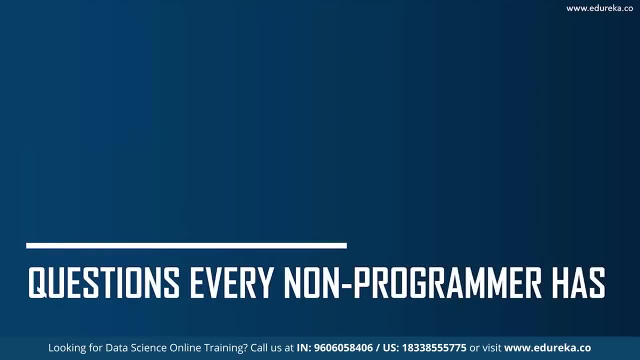 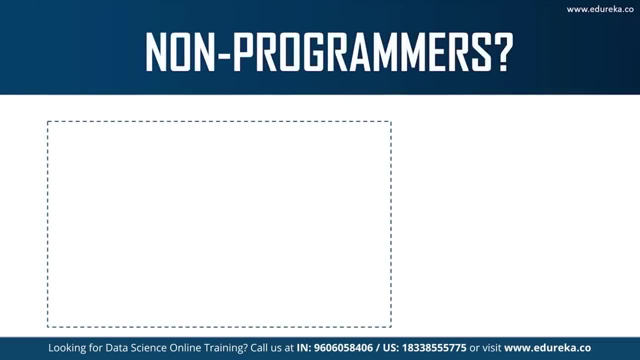 It's natural to have a lot of questions regarding data science and machine learning, So I'll be addressing the top three frequently asked questions by beginners or by non-programmers. What exactly do I mean by non-programmers? and so a non-programmer can be anyone from a software tester who's basically working on an automated tool. 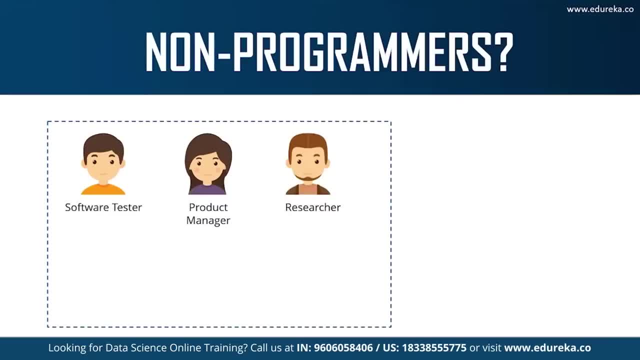 It can be a product manager. It can be a researcher who's creating content. It can be a content writer. It can be a student who has just graduated Or somebody who's still studying. It can be a marketing consultant. Basically, you can be from any background and still take up data science and machine learning. 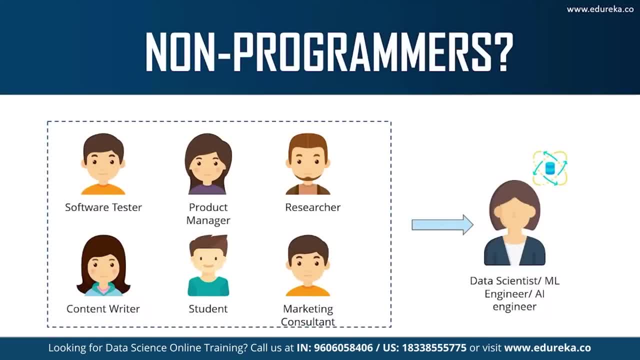 Now, if you want to get into the depth of the field, then obviously you do require programming languages, But, however, if you just want to start off and you cannot do programming at all, There are a couple of tools that I'll be discussing today, and these tools do not require you to have any prior programming knowledge. 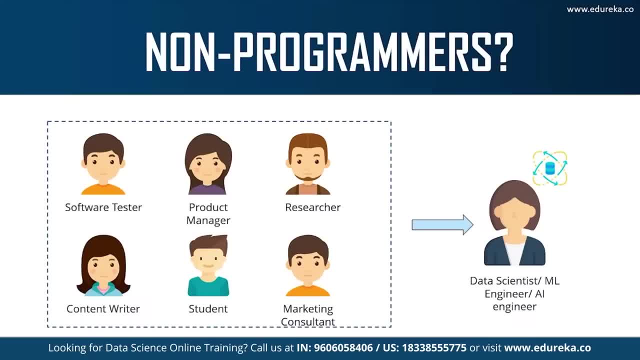 Now, in the further slides you will see me discuss about these tools. I'll be mentioning a couple of them. I'll be mentioning a couple of features to y'all. Now let me answer a couple of questions which are very frequently asked. 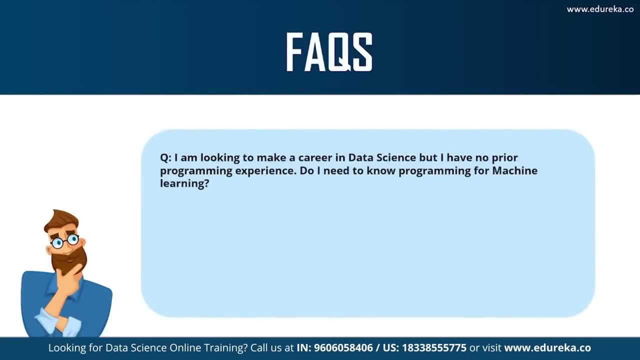 The first question that I usually get is: people tell me that I'm looking to make a career in data science, but I have no prior programming experience. Do I need to know programming for machine learning and data science? Now, in a nutshell, let me tell you that the answer to this question is yes. 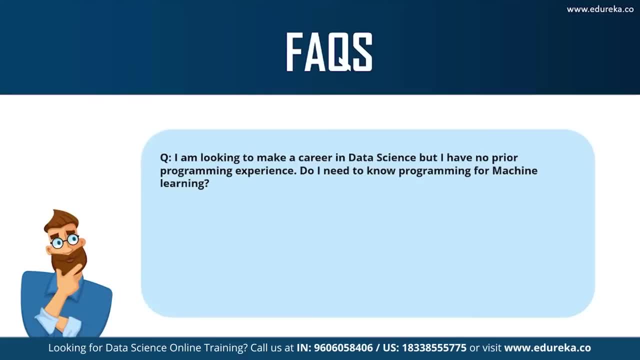 Okay, if you want a career in machine learning, then having some form of programming knowledge always helps, But let me tell you that programming is just a part of machine learning. So if you're looking to make a career out of it, I'd say that it is important for you to know the different programming languages like Python, at least to get started. 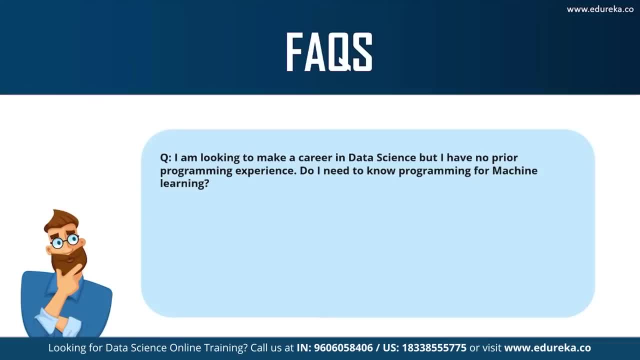 But due to recent breakthroughs, there are a lot of machine learning and data science tools that do not require you to have the programming necessity. right, You do not have to know programming languages, But if you ask me personally, then I'd say that you still have to learn programming languages, because only then you know how the entire process works. 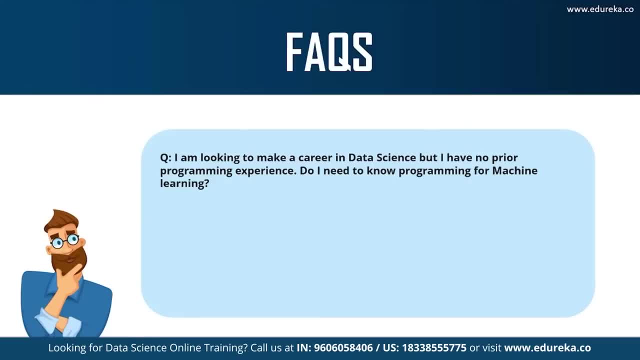 You know how machine learning really works because you're implementing it through code. Now another question is: are there any tools that can help me with data science and machine learning without knowing any programming language? Okay, the answer to this is a simple yes, And there are a lot of tools in the market these days that will help you get started with machine learning. 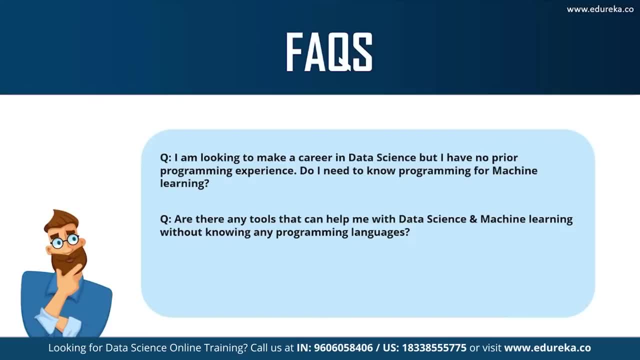 So these are especially useful for business applications of machine learning like predictive modeling, statistical analysis and so on. So there are a lot of tools and I'll be discussing a lot of those tools in the upcoming slides And so, don't worry, We'll talk more about the tools in the further slides. 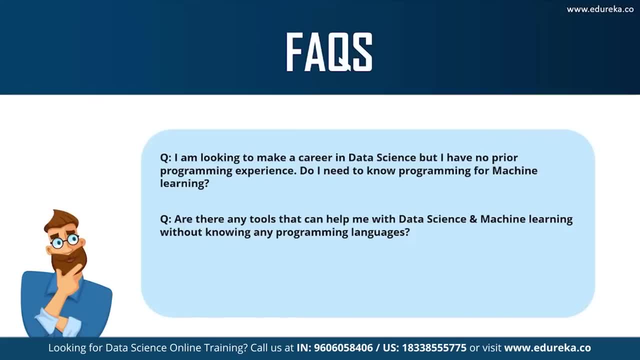 Another question is: do I need to know advanced mathematics or do I need to know advanced statistics in order to learn data science and machine learning? Now, this question depends on what exactly you're looking for, And if you really want to go in depth into the field of data science and machine learning, and if you want to understand the why behind the working of machine learning, then you need to know advanced mathematics. 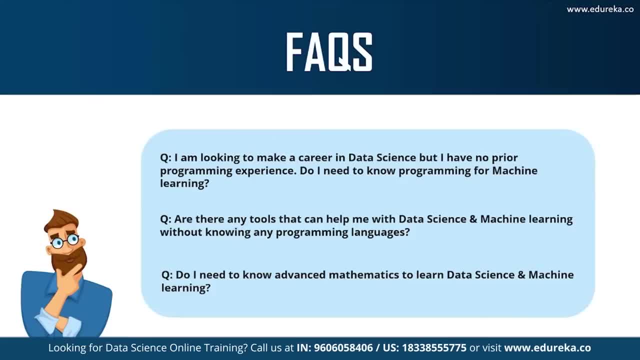 And if you really want to go in depth into the field of data science and machine learning algorithms, which is very fundamental to understanding machine learning, then I'd say that yes, you do need to learn mathematics. Advanced mathematics is basically, you have to have really good understanding of statistics, because statistical analysis plays a very important role in machine learning and data science. 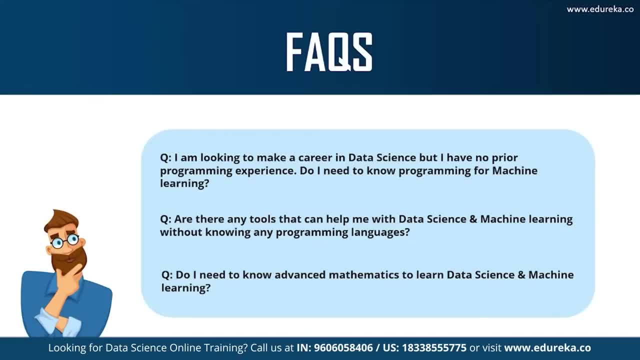 So a lot of topics under mathematics, which include probability. Of course, there is statistics and linear algebra. These topics can help you know more about machine learning algorithms and about data science, And about the different methods and techniques that are used to derive information from data. 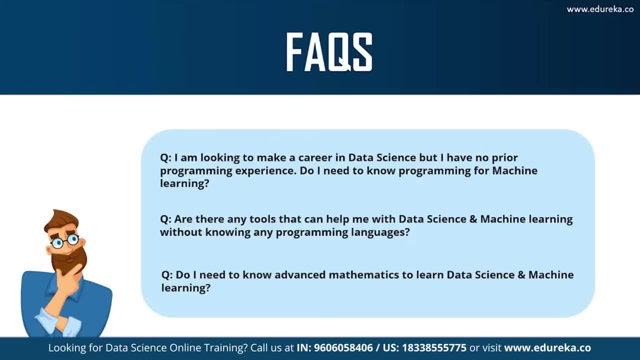 Now, not knowing advanced math is not an excuse to not learning machine learning. So, to sum it up for you, if you want to go in depth into machine learning and data science, then knowing advanced mathematics is a prerequisite, because it will help you understand the algorithms, the formulas, how the learning is done and many other machine learning concepts. 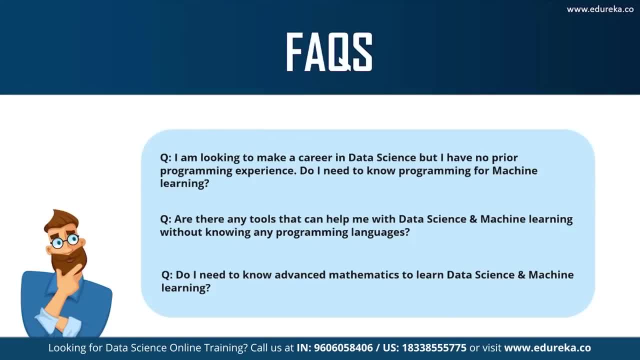 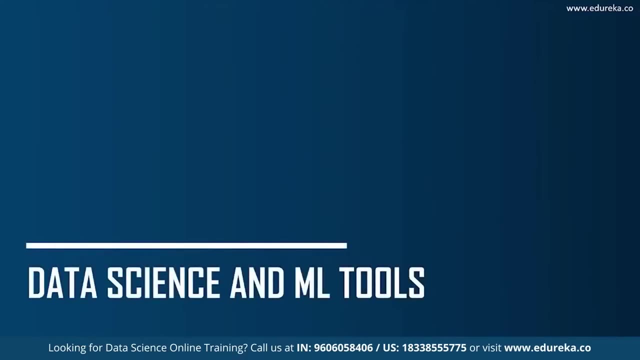 Right. So for now, let's move on and let's look At why exactly anybody should go for these data science and ML tools, And so we just looked at a couple of questions that non-programmers have. Now let's look at how you all can get started and why you should go for data science and ML tools. 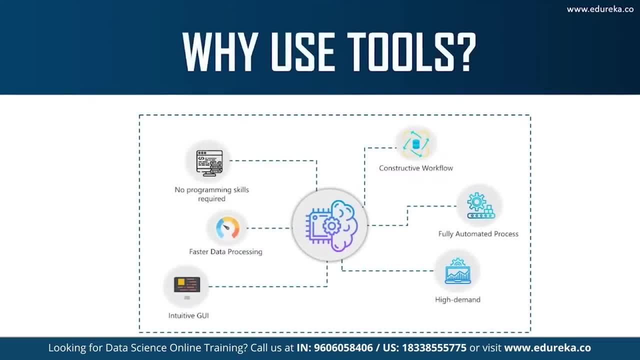 Now. the first reason is that you don't require programming skills to use data science and machine learning tools. Now, this is especially advantages to all of you non-IT professionals who don't have experience with programming in Python or in R. Another reason is that they provide a very interactive user interface which is very easy to use, and you know, you can learn very quickly by using that UI. 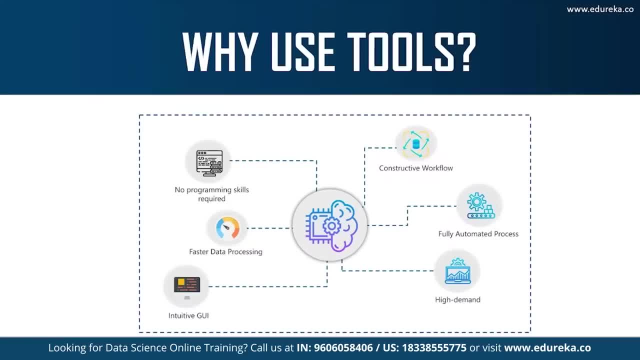 Now, another reason is that these tools provide- you can say- a very constructive way to define the entire data science workflow, and then you can implement it without worrying about any coding bugs or any errors. Right? So, given the fact that these tools don't require you to do any sort of coding, 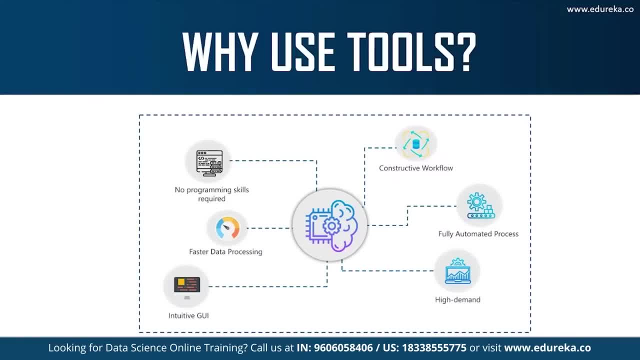 It's faster and easier To process data and to build strong machine learning models. Also, all the processes that are involved in the workflow are automated and they require minimal human intervention. So basically, all the processes are mostly drag-and-drop right. Whatever you want, whatever model you want, is just basic drag-and-drop in these tools. 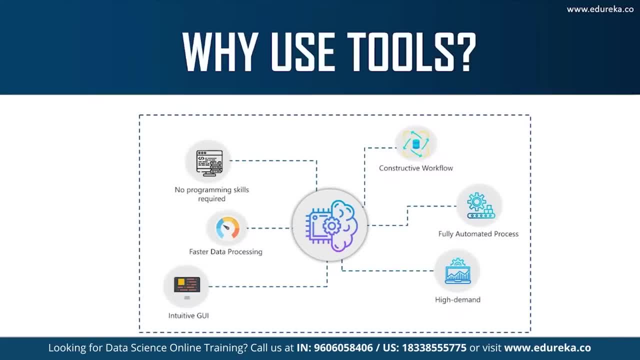 All you have to do is drag the modules that you want in your workflow Now. Another reason is that many data-driven companies have adapted to these data science tools and and they started looking for professionals who are able to handle and manage such tools. A lot of companies that are taking up professionals who have knowledge of ML tools, like IBM Watson and so on. 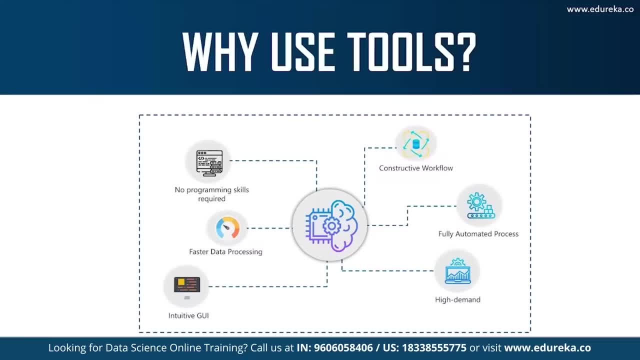 So, guys, those were a couple of advantages of using data science and machine learning tools. Now let's take a look at the top tools that any non-programmer can use in order to get started with data science and ML. So guys know that this list is in no particular order, right? 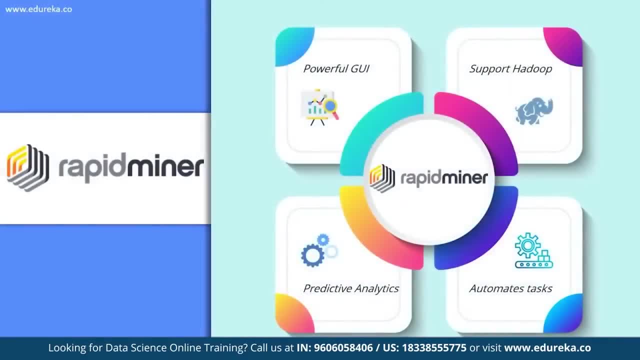 I have not ranked them according to the tools, So the first tool is RapidMiner. Now, it's no surprise that RapidMiner made it to this list, One of the most widely used data science and ML tools, preferred by not only beginners who are not well equipped with programming skills. 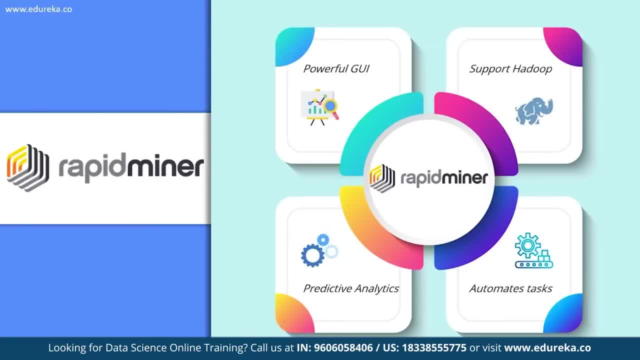 but it is also preferred by experienced data scientist. RapidMiner is the all-in-one tool that takes care of the entire data science workflow, from data processing to data modeling and even deployment. So if you're from a non-technical background, RapidMiner is one of the best tools for you. 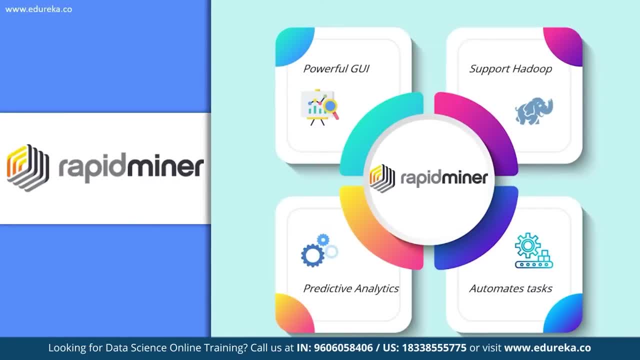 And it provides a very strong and a very interactive UI that only requires you to dump the data. There is literally no coding required, right? So all you have to do is you just have to dump the data into the tool and it will build predictive models and machine learning models that use complex and convoluted algorithms in order to achieve precise outputs. 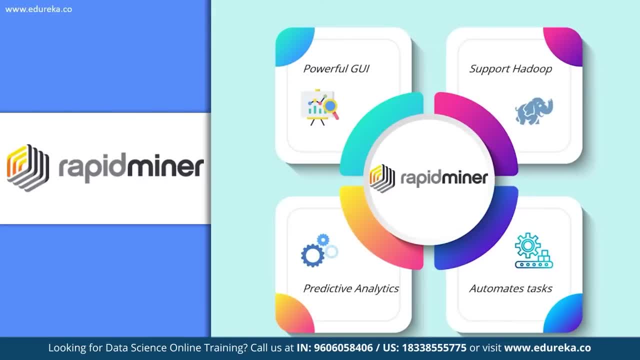 Now let me discuss a couple of features of RapidMiner. So, like I said that it provides a powerful visual programming environment, right, You can perform a lot of data visualization through this tool. It also comes with an inbuilt RapidMiner Hadoop that allows you to integrate with Hadoop frameworks for data mining and analysis- right? 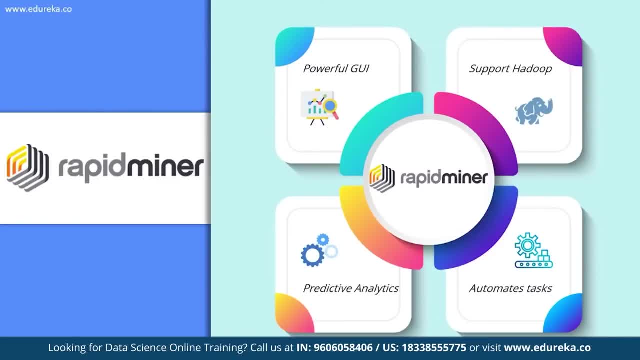 So having Hadoop support is very important because it helps in big data analytics, So you can dump all your data into the Hadoop framework And then perform analytics, and all of that through RapidMiner. Apart from that, it supports any data format and it also performs top-class predictive analytics by expertly cleaning the data right. 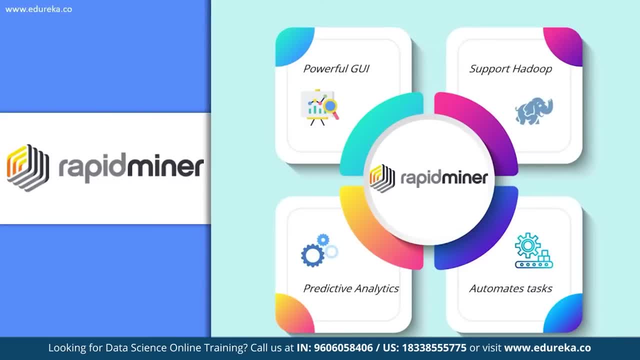 So data cleaning and data wrangling is done very easily through RapidMiner right. It uses programming constructs that automate all the high-level tasks, such as data modeling, So data modeling is also automated on RapidMiner. You don't have to code. 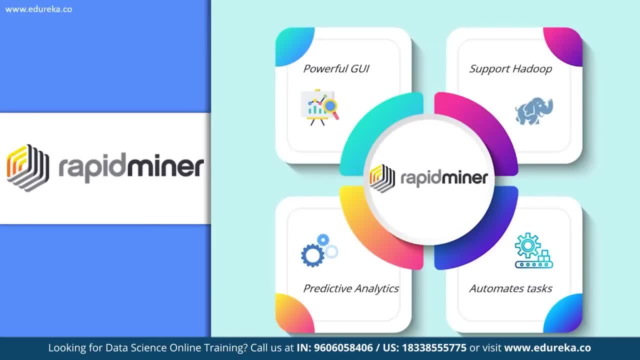 A single line. you just have to dump the data into the tool and do a couple of drag-and-drops, and that's it right. So RapidMiner is known as one of the best tools for data science and ML. So now let's look at our next tool, which is data robot. 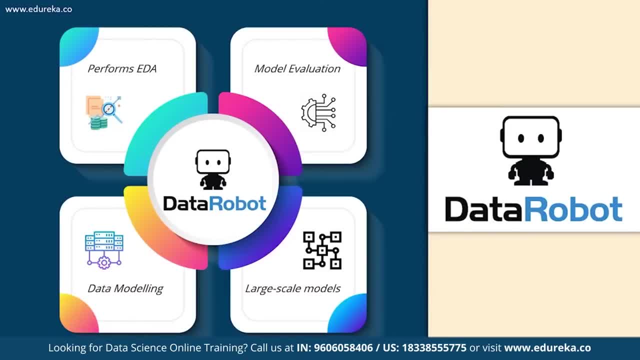 Now, data robot is an automated machine learning platform which builds precise projective models in order to perform extensive data analysis. It is known as one of the best tools for data mining and feature extractions. So professionals with less programming experience go for data robot because it is considered to be one of the most simple tools for data analysis. 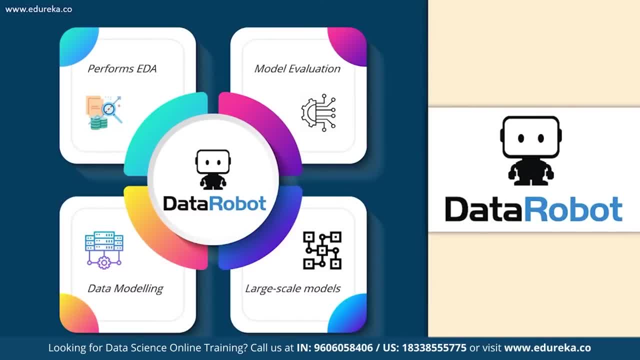 So, just like RapidMiner, data robot is also a single platform that can be used to build an end-to-end data science solution. right, It uses the best practices in creating solutions that can be used to model real-world business cases and can be used to solve real-world complex problems. 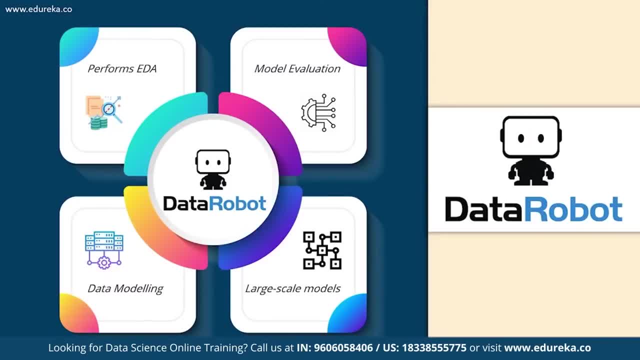 So, coming to the features of data robot, it automatically identifies the most significant features and it builds a model around these data features. right So? data modeling is done very easily when it comes to data robot. right So, guys, data modeling basically involves you to build a model that can help in predicting your output. 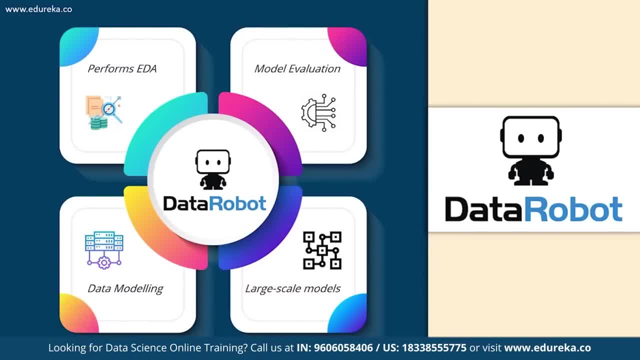 Now this model basically takes in all the important features that are needed to predict your output. This entire process is automated in data robot. Another thing is that it runs the data on different machine learning models and it'll check which model provides the most accurate outcome. 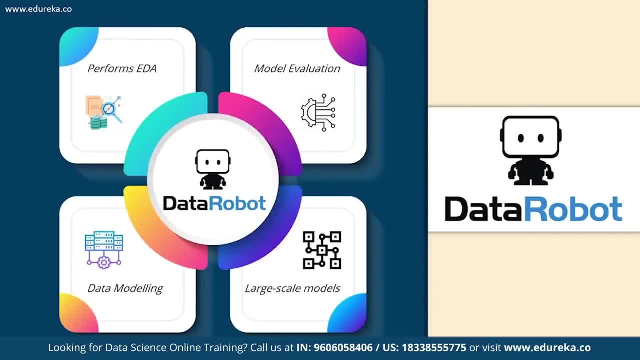 And so basically uses test cases. It has different, different models and it tests where your accuracy is maximum. Also, it is very fast in building, training and testing predictive models, in performing text mining, data scaling and so on. These are other additional features. 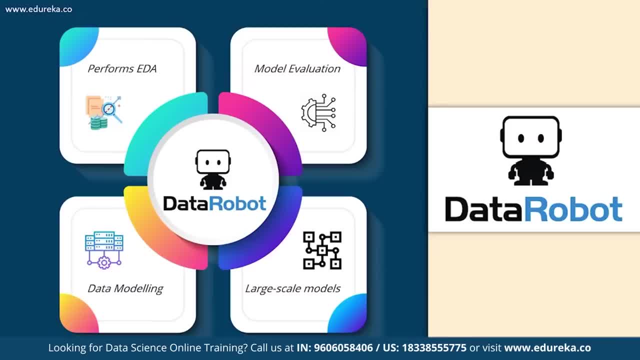 It can also run large-scale data science projects, and it is also known for incorporating model evaluation methods like parameter tuning and so on. right, So model evaluation is also easily carried out on data robot. So basically, your end-to-end data science process and machine learning process is covered by the single tool. 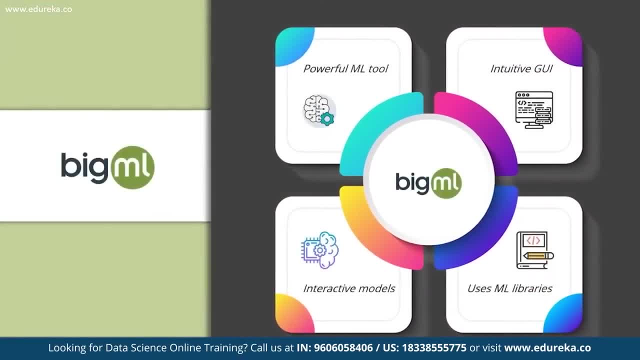 Now let's move on and discuss another tool, which is BigML. So BigML, you can see that it eases the process of developing machine learning and data science models By providing readily available constructs that help in classification, regression and clustering problems. 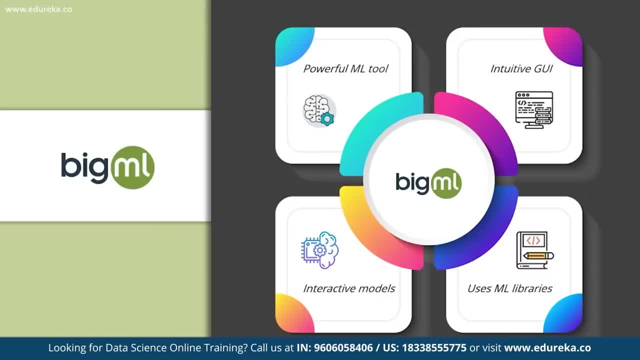 Right. It incorporates a wide range of machine learning algorithms and it helps to build a strong model without much human intervention. This lets you focus on important tasks like improving your decision-making process and so on. Right, So some features include that it is a very detailed and comprehensive machine learning tool. 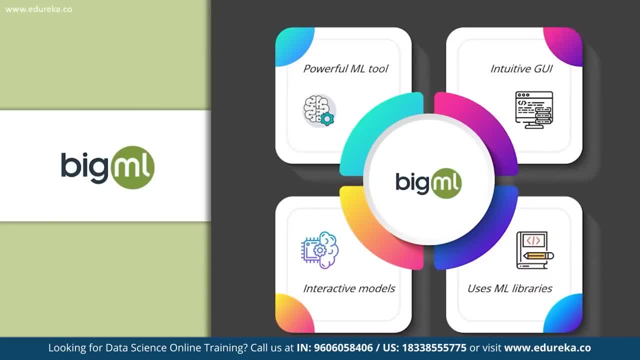 That supports the most complex machine learning algorithms, involving full support for supervised and unsupervised learning, which basically involves anomaly detection, association, mining, regression, clustering and classification. Another feature is that it provides a simple web interface and APIs that can be set up in a fraction of the time that it takes for traditional systems. 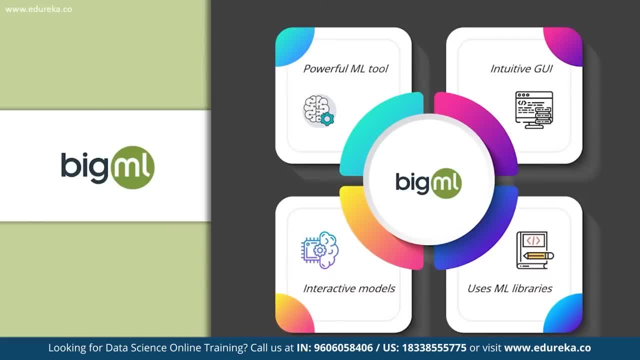 So comparatively, it's extremely, extremely fast. It also creates visually interactive predictive models that make it easy to find correlations among the different features in your data Right. So data visualization is also a pretty important role in data science, and BigML really helps in creating such visualizations. 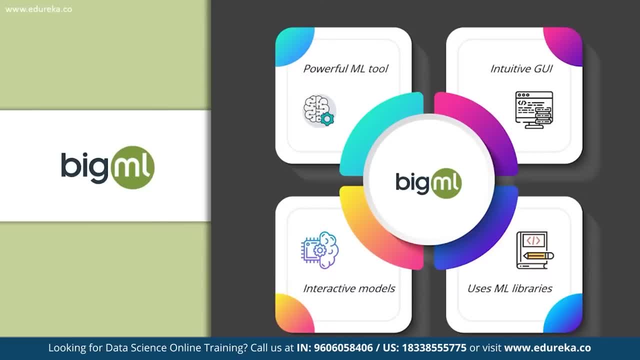 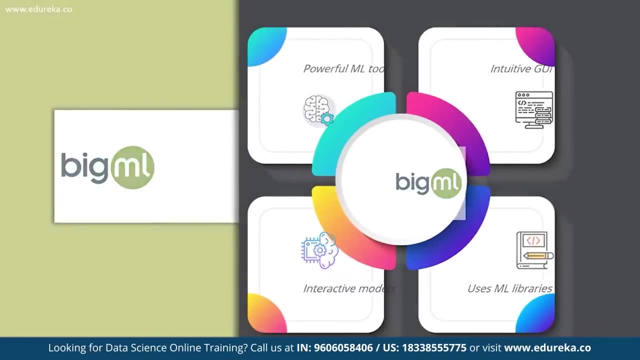 which help you understand the dependencies between your features in your data. Apart from that, it also incorporates bindings and libraries of the most popular data science languages like Python and Java Right, So it has support for all of these languages. So that was about BigML. 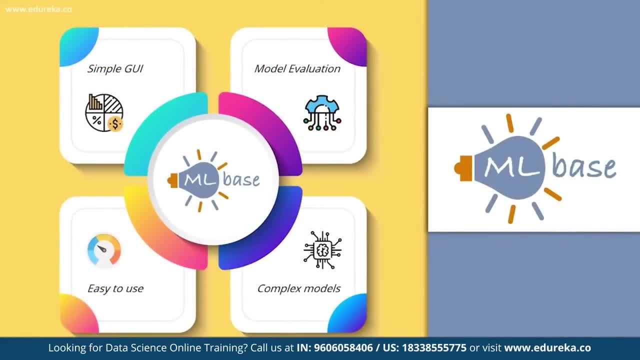 Now let's look at another tool called MLBase, or machine learning base. So MLBase is again an open-source tool that is one of the best platforms used to create large-scale machine learning projects. Now, before I tell you the features of MLBase, 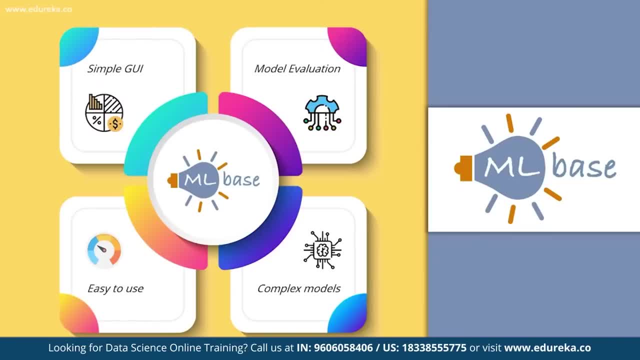 let me tell you that there are three main components in this tool. So there's something known as ML optimizer, and the main purpose of this optimizer is to automate the entire machine learning pipeline construction. After that, we have something known as MLI. Now, MLI is an API that is focused on developing algorithms and performing feature extractions for any sort of difficult or any sort of high-level computation. 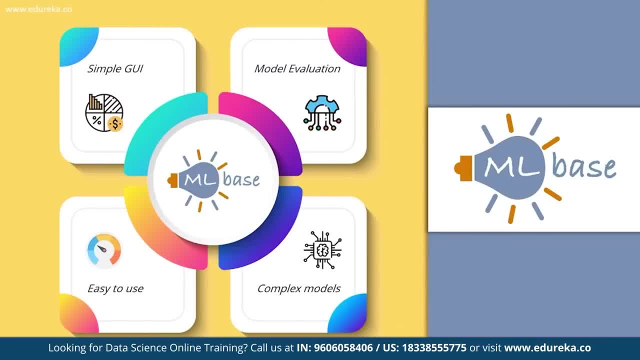 Then another component is the ML lib, or machine learning library. It is Apache Spark's very own machine learning library that is currently supported by the Sparks community. So it basically supports Apache Sparks machine learning library, right? So now let me tell you a couple of features of MLBase. 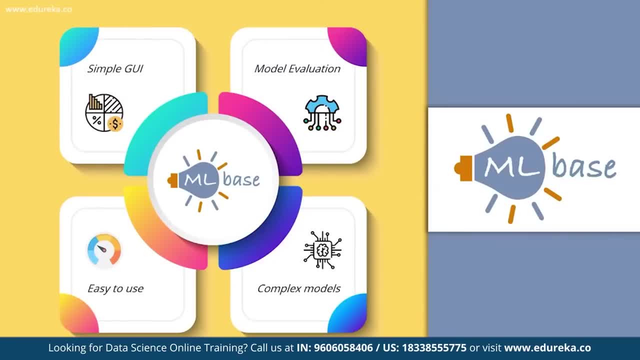 So, like I mentioned, it provides a very simple UI for developing machine learning models, predictive models and all of that Right? So, guys, having a good user interface actually pretty important when it comes to these tools, because you need to easily understand and you need to easily grasp what exactly is happening. 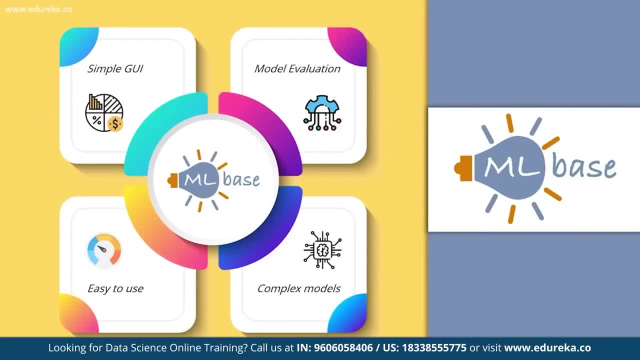 How exactly You get it going to build a model, how you're going to add data, what features you're going to select in order to build a model, how you're going to make your model better through parameter tuning, cross validation and all of that. so it's important to have a very simple ui that will make everything. 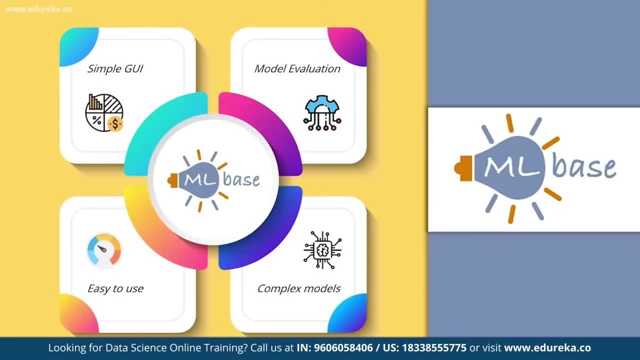 look easier and more understandable, and that is easily achieved through ml base right. i think it has one of the simplest ui among a lot of other tools. now, another feature is model evaluation right, so it basically learns and it tests this data on different learning algorithms to find. 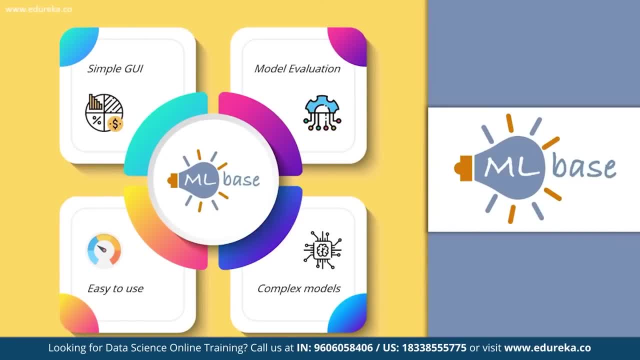 out which model gives the best accuracy, right. so basically it compares our accuracy on different models. it runs your data on different models. another feature is easy to use. so, like i said that, the ui of this tool is extremely simple and extremely understandable. so non-programmers who 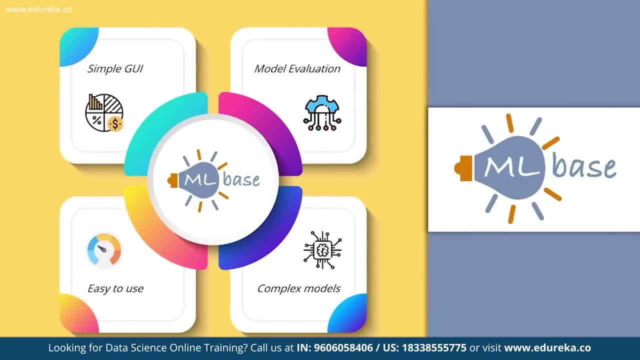 are new to data science or who are new to this whole machine learning process. they can easily scale data science modules because of how easy and how simple the tool is to use. apart from that, it can scale more large and more convoluted projects much more effectively than. 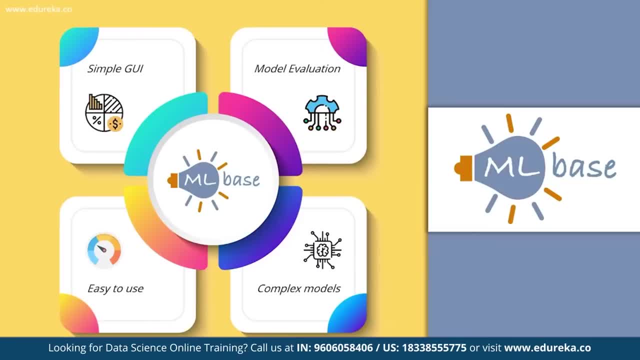 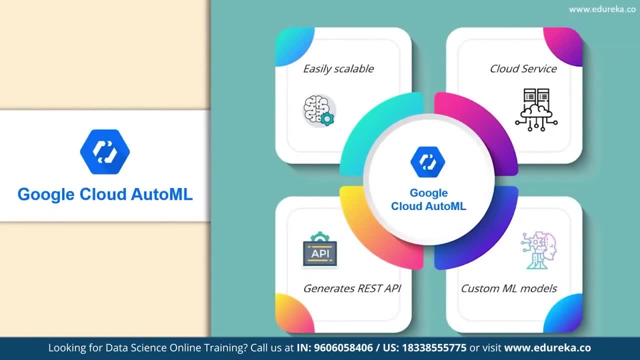 any other traditional system. so that was all about ml base. so now let's discuss the next tool, which is google cloud auto ml. now, google cloud auto ml is a platform of machine learning products that allows a lot of professionals with a limited experience to do a lot of machine learning and to do a lot of machine learning and to do a lot of. 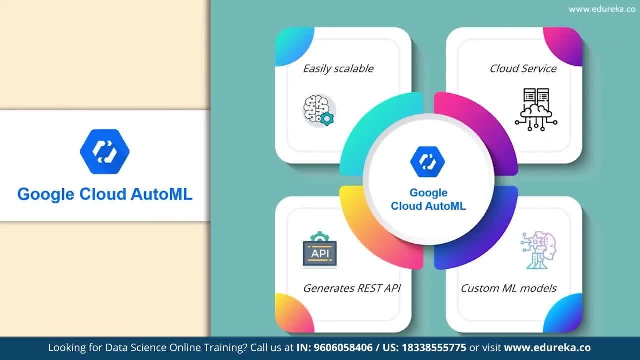 experience in data science to train high-end models which are specific to their business needs. so this cloud auto ml tool is one of the best machine learning platforms, with over 10 years of trained google research constructs to help you build predictive models. so let me discuss some of 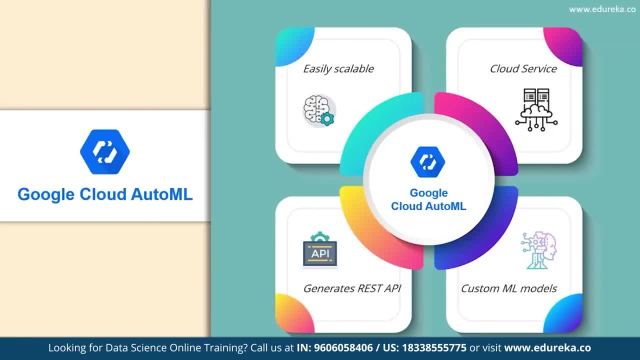 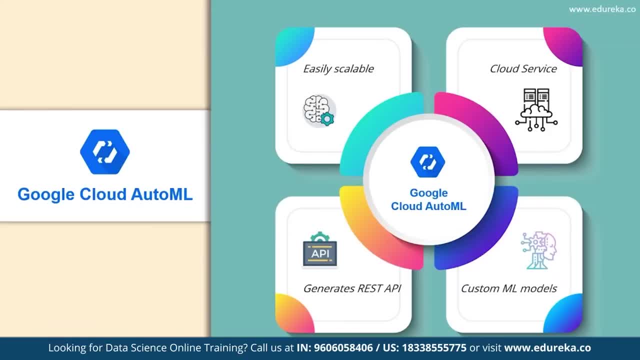 easy to use for people who do not have experience in ml and data science, and it comes with a lot of documentation. it comes with a lot of tutorials, so one of the best features of this tool is that any person with minimal expertise or limited information in the field of machine learning 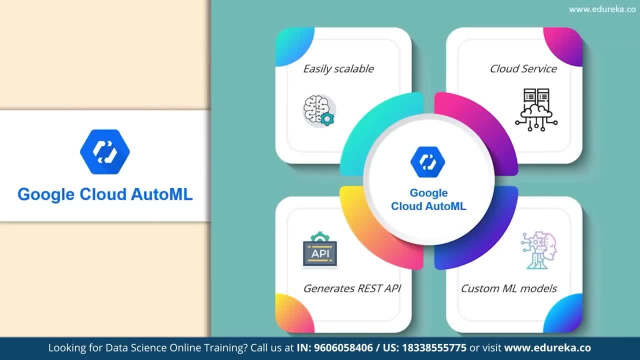 they can easily use the tool and build high level machine learning models. right so, this tool has a lot of documentation. it comes with a lot of tutorials, so it's one of the easiest tools to use and it supports a lot of people from different back backgrounds. right so, if you're not very aware with data science and ml, it has a very detailed 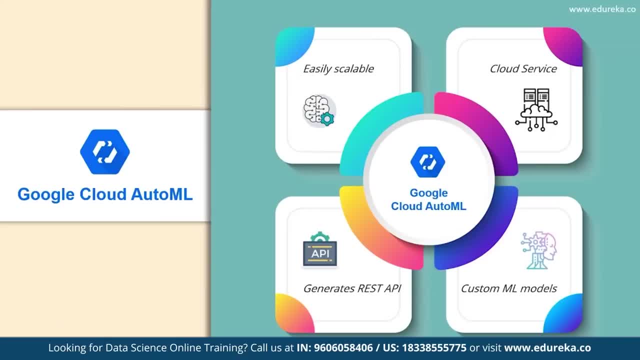 and a very comprehensive approach to the entire process, so this is one of the best tools for a beginner, i would say. also, apart from that, it has a fully fledged integration with many other google cloud services, which will help you in data mining and data storage. right, these are very important. 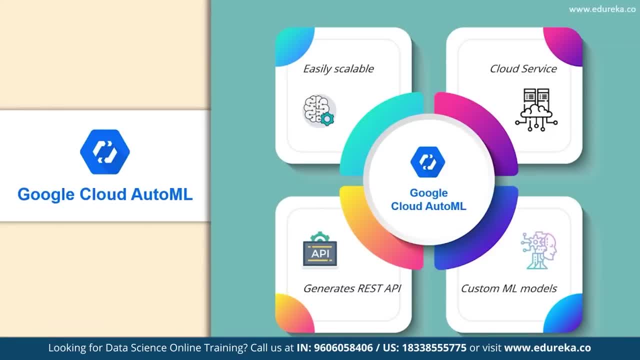 parts of data science and ml. it also generates a rest api while making predictions about the output. so having apis also help you connect with other tools. it also provides a very simple ui to create custom machine learning models that can be trained, that can be tested, improved and deployed through. 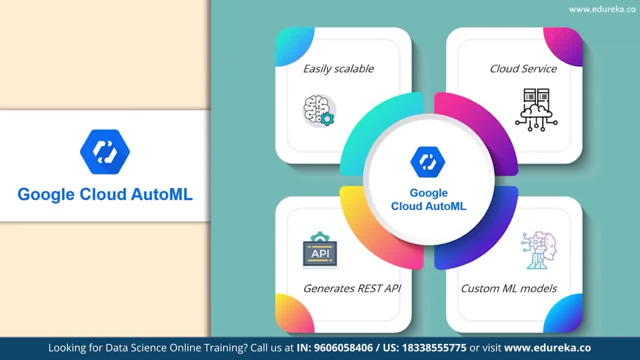 the same platform. right again, it's an end-to-end solution to data science. it provides the entire data science workflow and it is quite easy to use. moving on to the next tool, we have auto vika. now. this is one of my favorite tools when it comes to machine learning and data science. 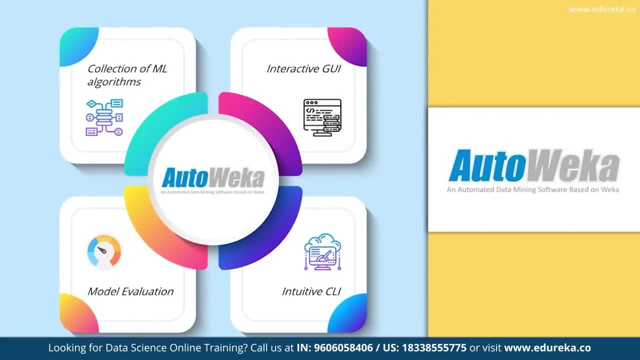 it is an open source ui based tool which is ideal for beginners because it provides a very intuitive interface for performing all your data science related tasks. so, apart from having a simple ui, it supports automated data processing. it performs very extensive eda supervised and unsupervised learning algorithms. all of this is covered in the tool. 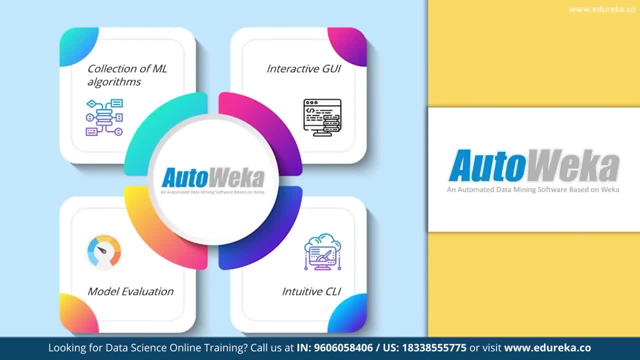 right. i think this is one of the best tools for beginners and also if you want to go in more depth about data science and ml, i feel like this is one of the best tools, right. it's perfect for newbies who are just getting started with data science and ml also. 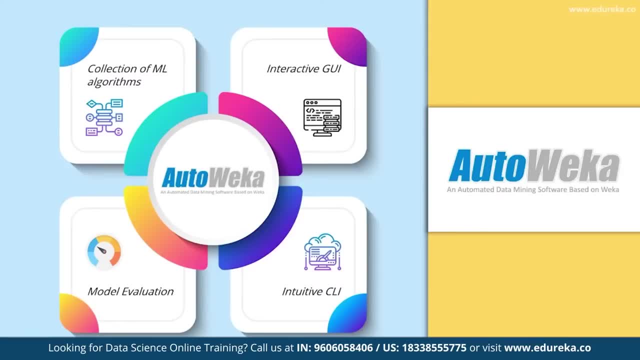 it has a huge community of developers who are kind enough to publish tutorials and research papers about using this tool. so actually, this tool is preferred by a lot of developers as well. so i'm aware of a couple of data scientists who use python and r and who also use autoveka, because 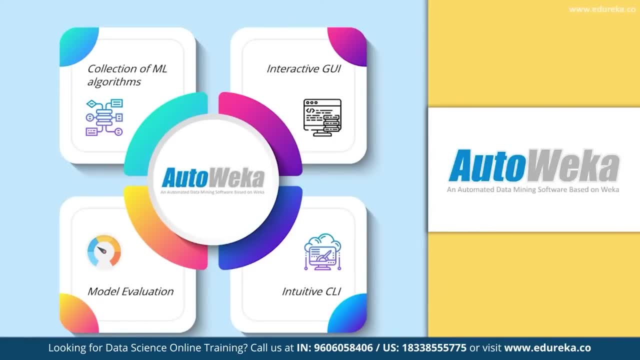 they find it extremely easy and they find it a very strong tool. so thank you so much for watching these videosdirrlikeonme. i will see you next time, bye, bye. tool for building machine learning models. Now let me tell you a couple of features of the tool. 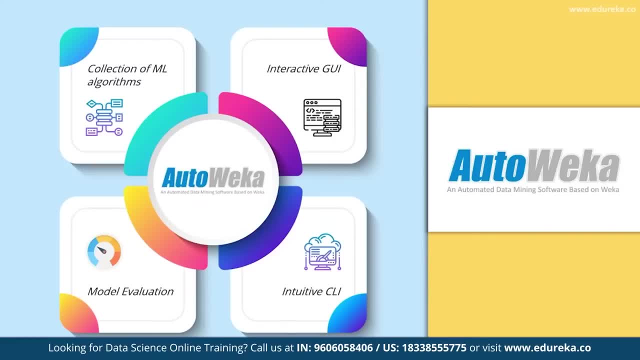 So Weka provides a huge range of machine learning algorithms So you can perform classification, you can perform regression, clustering, anomaly detection, association mining, data mining and all of that right. It also provides a very interactive graphical interface to perform. 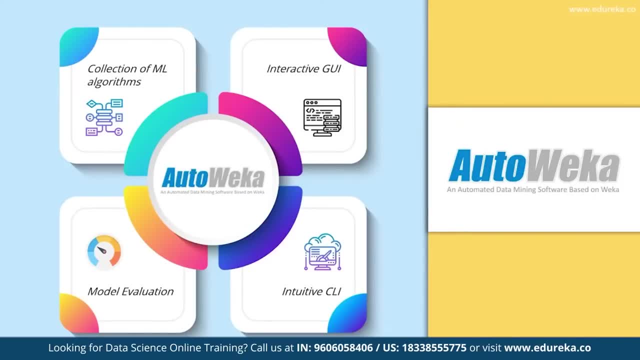 data mining tasks, to perform data analysis and EDA, and so on. Another feature is that it allows developers to test their models on varied set of possible test cases and it helps in providing the model that gives the most precise output right. So, like a lot of the other tools that I, 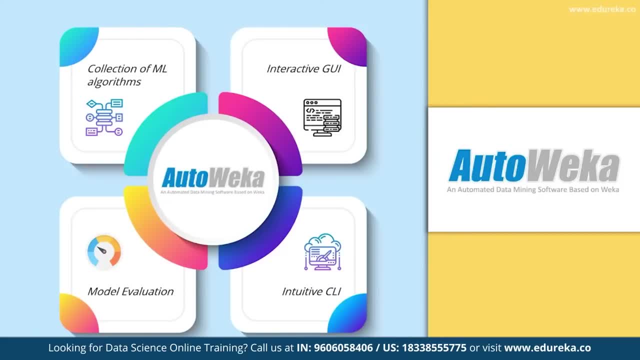 mentioned in this list. this tool also helps in model evaluation right. Basically, it tests your data on different models and it chooses which model is the most accurate or gives you the most precise output. So it helps you to perform data mining tasks, to perform data analysis and EDA. 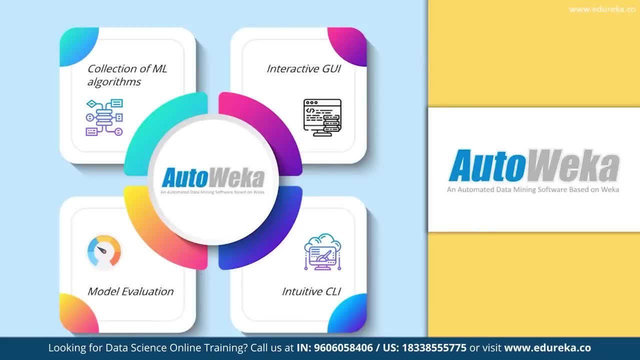 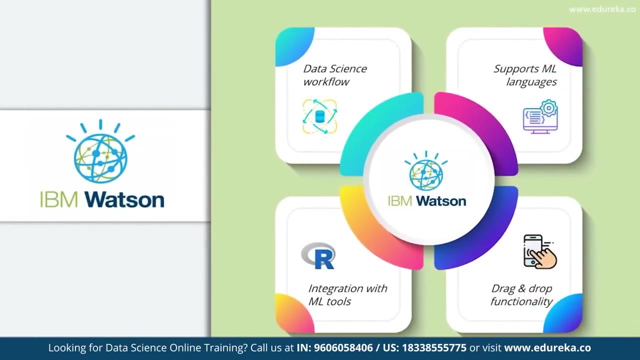 and so on. Apart from that, it also comes with a simple yet a very intuitive command line interface to run basic commands right. So, guys, these were a couple of features of AutoWeka. Now let's move on and look at the next tool, which is IBM Watson Studio. So we're all aware. 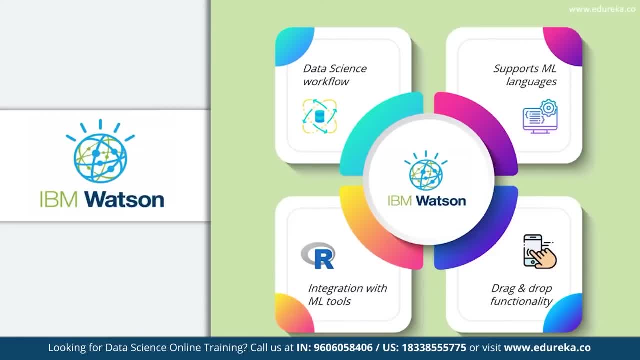 of how much IBM has contributed to this AI-driven world. So IBM is actually known as the number one contributor in contributing a lot of tools, concepts, technologies which reward the AI and data science, And so, like most service provided by IBM, IBM Watson Studio is again. 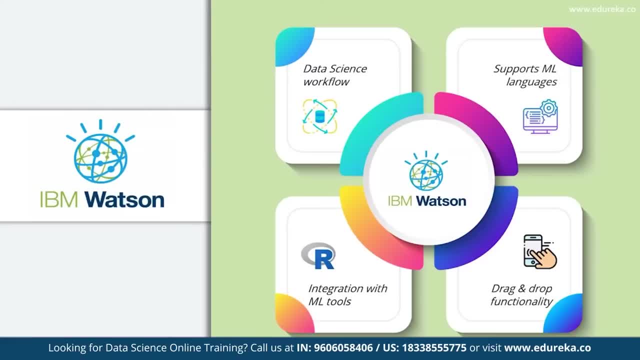 an AI-based tool which is used for extensive data analysis. It is used for machine learning, data science and so on. right, There are a lot of organizations actually which make use of IBM Watson. It also comes in a lot of healthcare sectors. There's also a particular tool created. 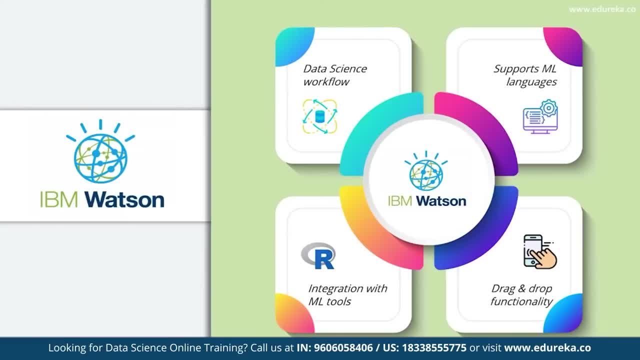 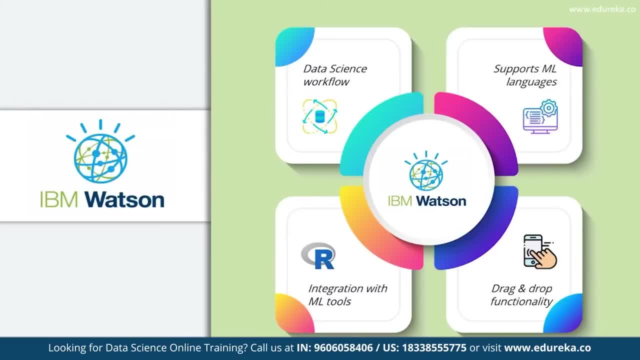 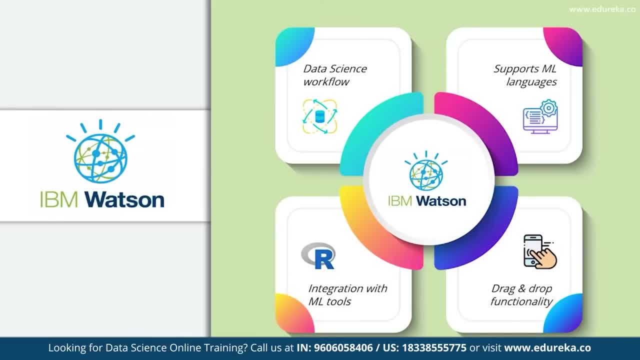 recognized in the market. let's take a look at a couple of features of IBM Watson. One feature is that it provides support to perform data preparation, exploration and modeling within a span of a few minutes, and the entire process is automated right, So it's a very quick tool. 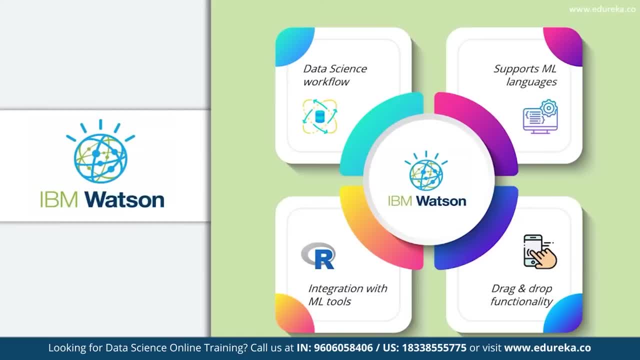 which can perform your entire end-to-end process in a couple of minutes. It also supports multiple data science languages and tools such as Python 3 notebooks. It supports Jython scripting, SPSS modulars and data refinery, So it provides support for all these. 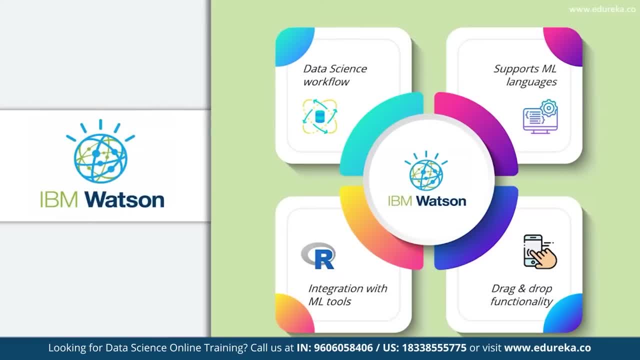 languages. Now for coders and data scientists: it offers integration with RStudio, with Scala, with Python and so on. You can say that IBM Watson is a more advanced tool, right? So a lot of data scientists and a lot of coders actually make use of this tool, right Apart. 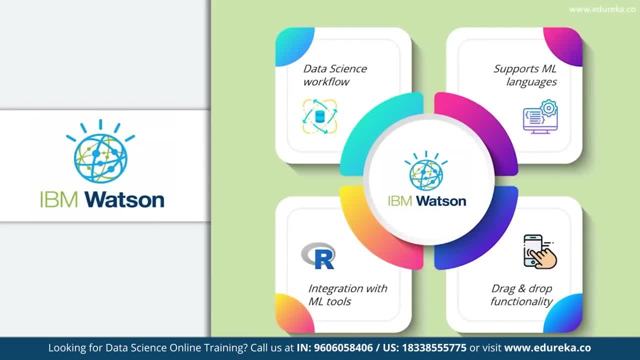 from being automated. it also provides support for the different programming languages, like R and Python. Another feature is that it uses the SPSS modular. that provides drag and drop functionality, and this is quite simple, because it lets you explore data and build strong models very easily. 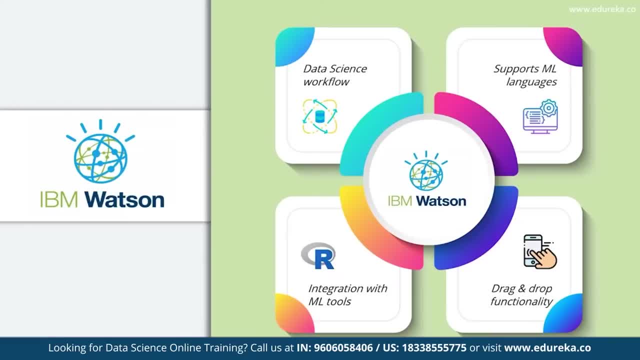 right. All you have to do is drag and drop, right. So, guys, those were a couple of features of IBM Watson. So I'd say IBM Watson is a more advanced tool. It provides support for all the different languages that come under the name of IBM Watson. So I'd say IBM Watson is a more advanced tool. 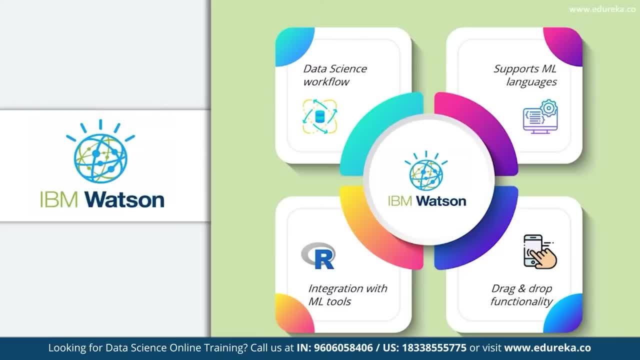 Data science right. It has a really good data analysis support. So the EDA that is performed in this tool is really good. It helps in extracting the most significant variables and then it builds a model on that variable. So, guys, that was a little bit about IBM Watson Studio. Now let's. 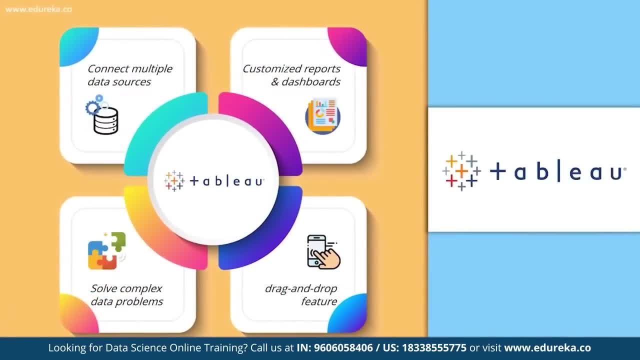 look at our next tool, which is Tableau. Now, Tableau is known as the most popular data visualization tool in the market. It allows you to break down raw, unformatted data into a processable and understandable format. This tool is mainly 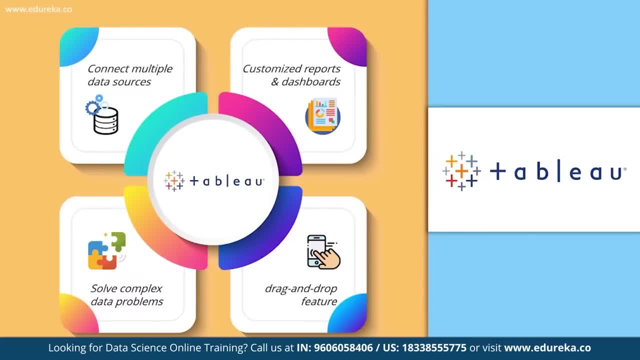 focused on data visualization. right, You can also perform a lot of data analysis also on the tool, but it is one of the best tools for data visualizations. A lot of high-end companies, a lot of data-driven companies, make use of this tool to see their business growth and to visualize. 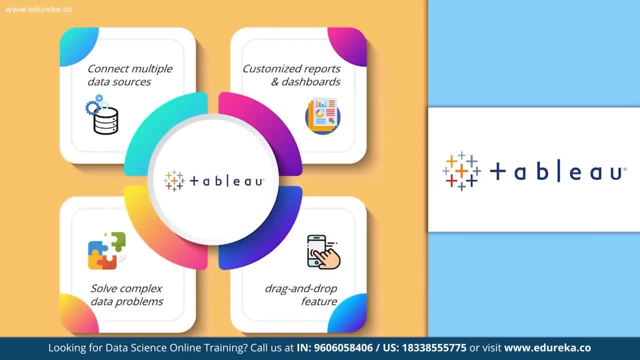 and analyze their data. So let me tell you a couple of features of Tableau. Tableau desktop feature: it allows you to create customized reports and dashboards that help you get real-time updates right. It can also connect to multiple data sources and it can visualize. 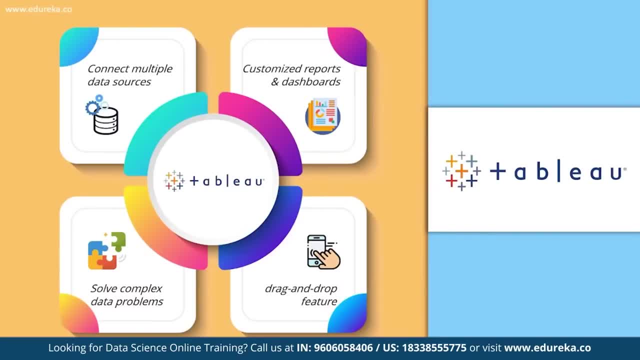 a huge amount of data to find a lot of correlations and patterns in data, right? So that's what data visualization is important for: It's for understanding the correlations in your data, So it can connect to different data sources and then it can perform data visualization. 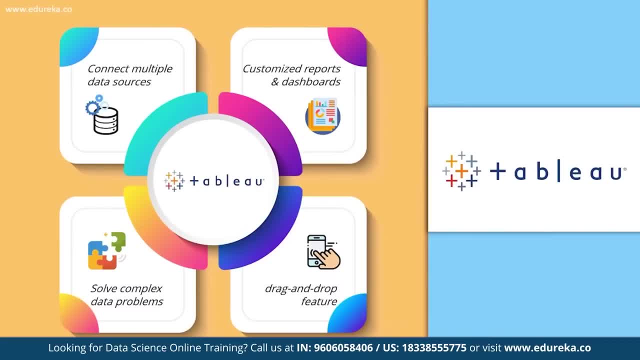 So, apart from this, Tableau also provides cross-database join functionality, which allows you to create calculated fields and join tables. Basically, this entire process will help in solving complex data-driven problems, right? So, guys, this is a very advanced tool for data science. 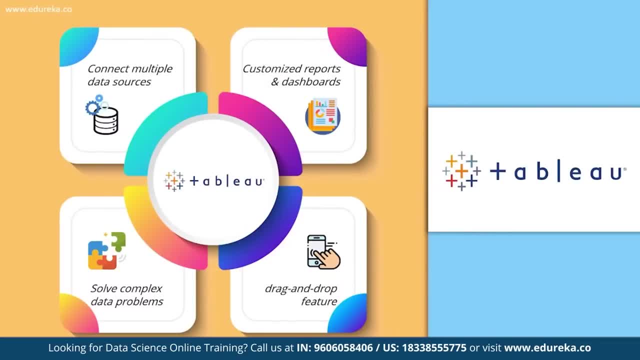 It goes in-depth with the entire data and it tries to bring out the best features and the most significant features in your data through graphs and through plots. Now, apart from that, it is a very intuitive tool. It uses the drag-and-drop feature to derive useful insights and perform data analysis. 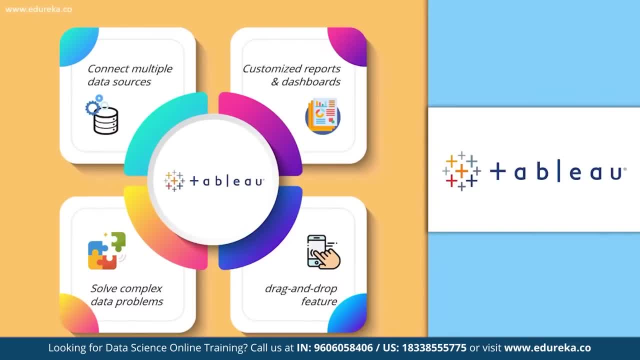 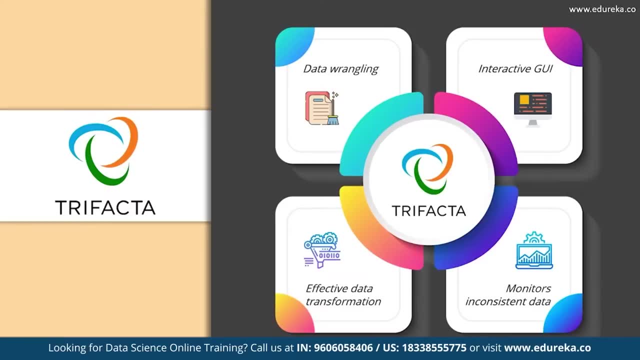 So those were a couple of features of Tableau. Now let's move on and discuss Drafacta. Now, Drafacta is an enterprise data wrangling platform that help you understand what exactly is in your data and how it can be useful for different analytic explorations- The key to identifying 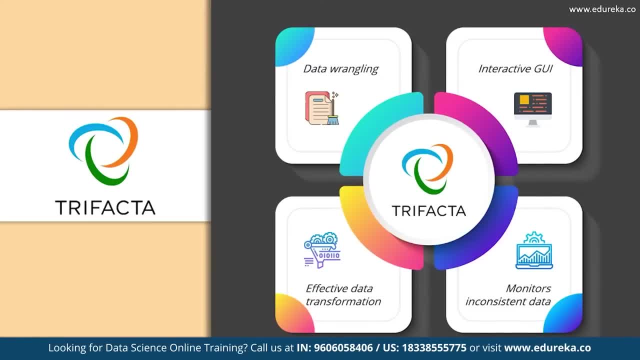 the value in your data. So Drafacta is actually considered the best tool for performing data wrangling, data cleaning and analysis. Now, data wrangling and cleaning is one of the important features of Drafacta. So let's understand a few features of Drafacta. So 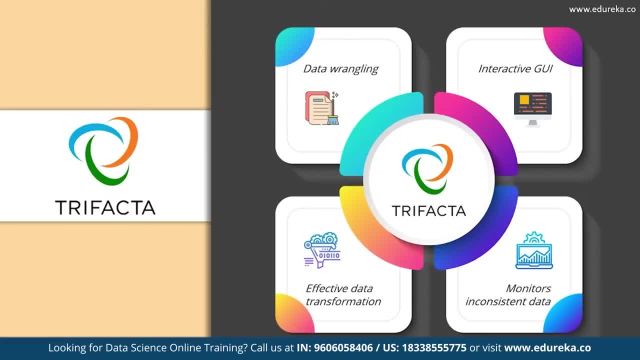 basically, Drafacta allows you to connect to multiple data sources, irrespective of where the data lives, And so you can have connections with various data sources. It also provides a very interactive UI for understanding the data, to not only derive the most significant data. 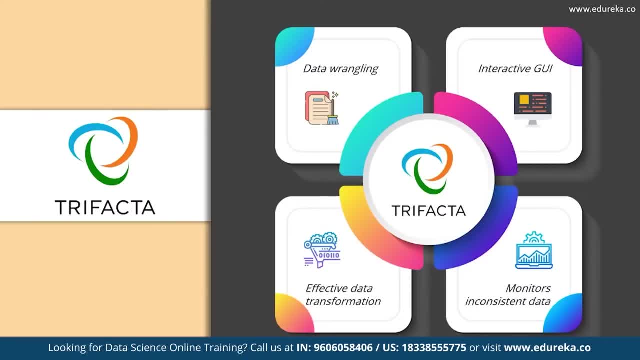 but also to remove unnecessary or any sort of redundant variables. Apart from that, it provides visual guidance, machine learning workflows and feedback that will guide you in assessing the data and performing any sort of data transformation. It is also very good at monitoring your data, So 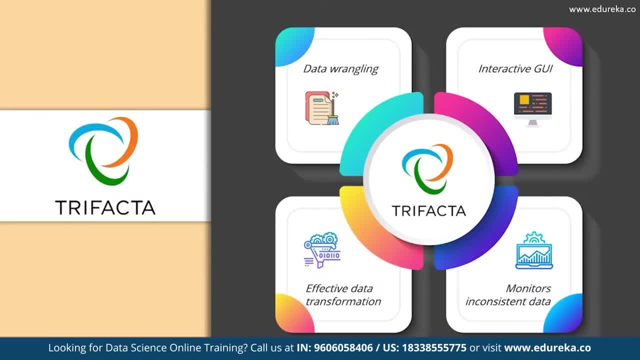 it monitors the inconsistencies in data and it removes any sort of null values or any missing values and make sure that data normalization is performed so that you can monitor the data and make sure that you avoid any sort of biasness in the output right, So it's mainly for data. 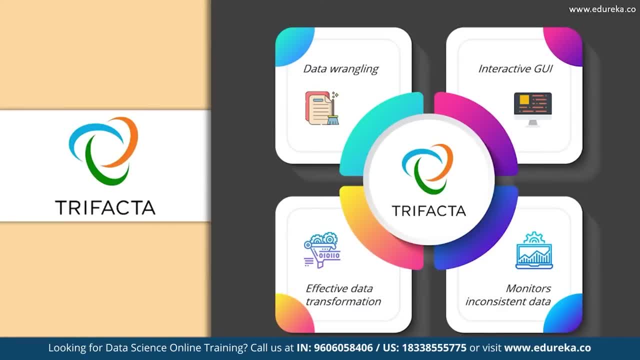 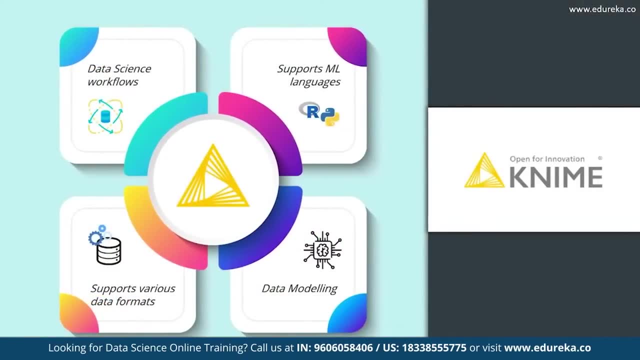 preparation. I would say Drafacta is a very good tool for data preparation, data wrangling and so on. So that was all about Drafacta. So now let's discuss the last tool for the day, which is: 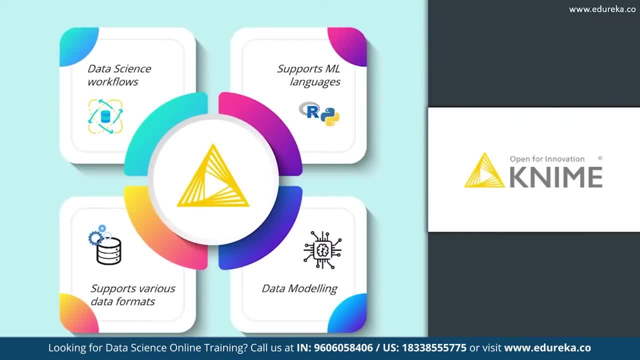 KNIME Now again. KNIME is an open-source data analytics platform which is aimed at creating out-of-the-box data science and machine learning applications. right So, building data science applications involves a lot of data science and machine learning applications, right So? 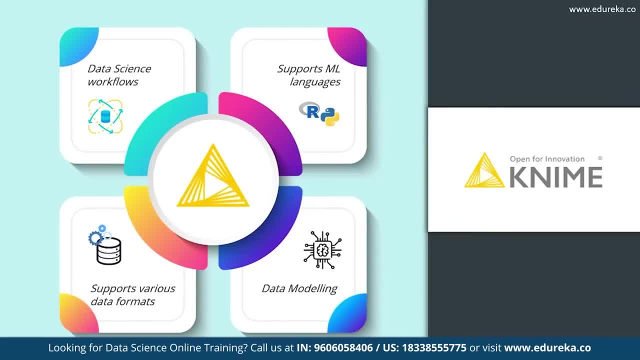 it involves a lot of tasks, right. It involves data processing, data wrangling, EDA and all of that. So this tool basically makes sure that this entire process is fully automated. right, It provides a very interactive and a very intuitive user interface which makes it easy to understand. 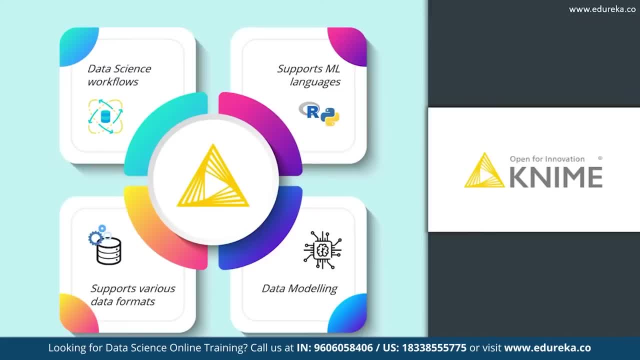 the whole data science methodology. A few features of KNIME include that it can be used to build an end-to-end data science workflow without any coding, So you just have to drag and drop the modules. It can be used to build an end-to-end data science workflow without any coding, So 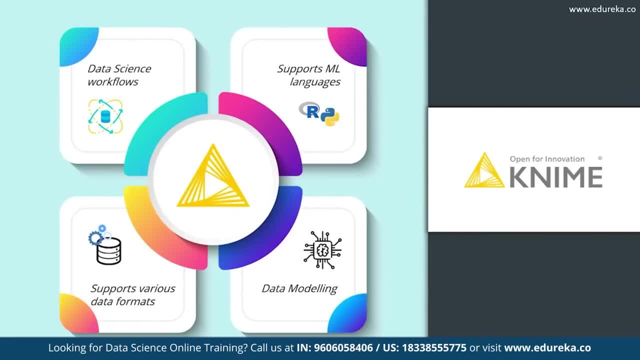 it also provides support to embed tools from different domains, including scripting in R, in Python, and it also provides APIs to integrate with Apache Hadoop right. So it has support for all the important tools that are needed in data science- Apache Hadoop- it also provides support. 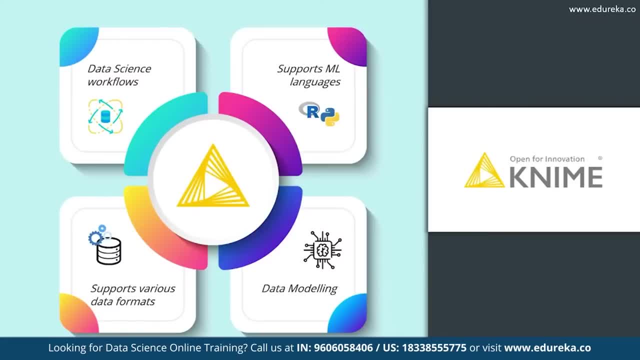 if you want to code in R and Python. It is also compatible with various data sourcing formats, which include simple text formats such as CSV files, PDF, XLS and so on. It is also compatible with unstructured data formats, including images, GIFs and so on. Another feature is that it 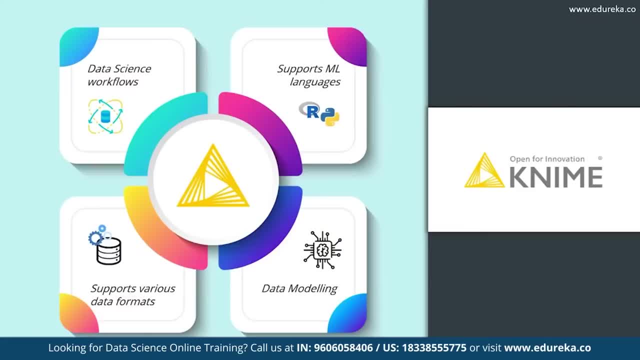 provides full-fed support for performing data wrangling, feature extraction, normalization, data modeling, model evaluation, and it even allows you to create interactive visualizations. So, like I said, it covers the entire data science process, end-to-end KNIME is actually one of my. 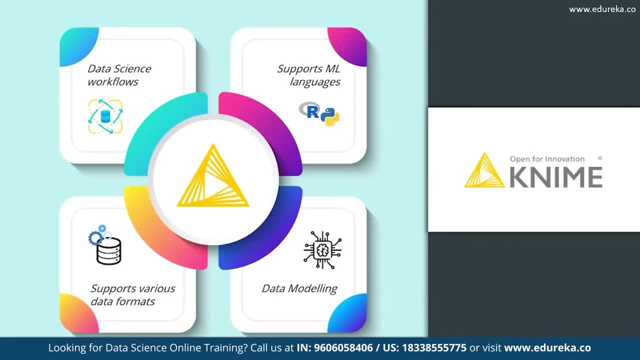 favorite tools as well. right, It is used for the entire data science workflow and actually it's a very understandable tool. It performs data analysis in a very in-depth manner, and I feel like the fact that it supports machine learning languages is very good, because 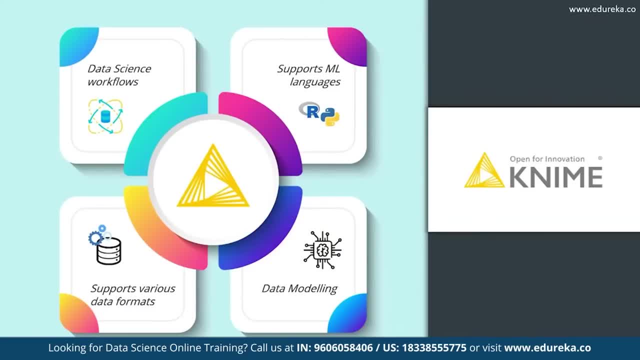 not only can non-IT professionals and programmers go for this tool, even data scientists can go for this tool. There are actually a lot of data scientists that make use of KNIME in order to perform EDA and all of that. So, guys, those were the top tools for data science and machine learning. 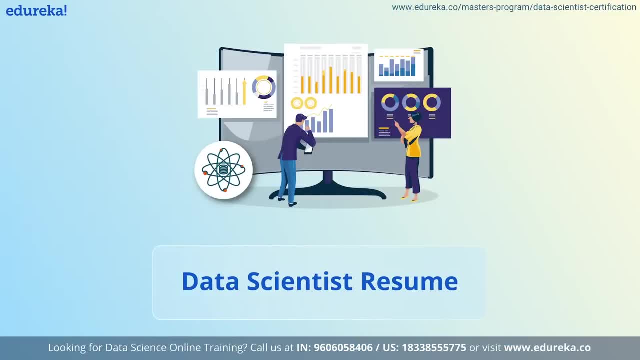 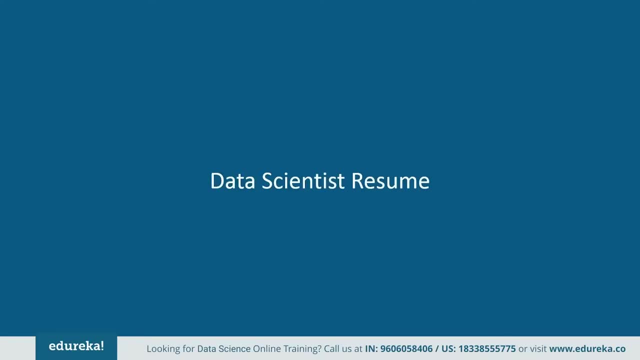 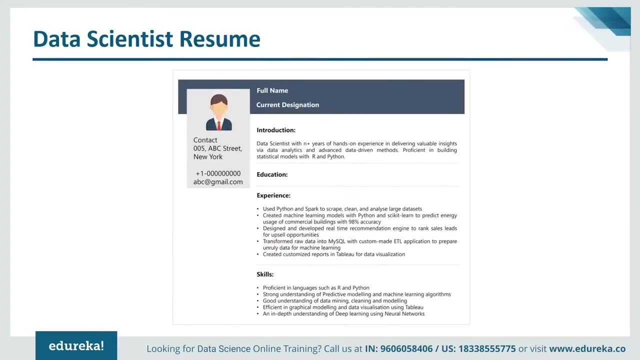 if you are a non-programmer Now let's move on and look at a data scientist sample resume. So I created a sample resume in order to make you understand what exactly you should put in your resume. So an introduction is very necessary. Make sure it's a simple and a short introduction, but also make sure that it 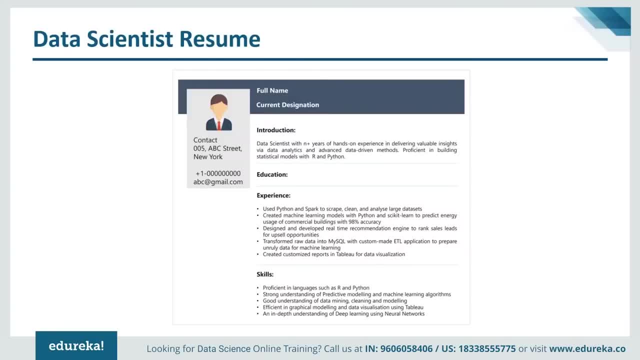 draws attention. Make sure you sneak in your skills and your experience in the introduction, So I've written that a data scientist with n plus years of experience should be able to do this. So I have hands-on experience in delivering valuable insights via data analytics and advanced 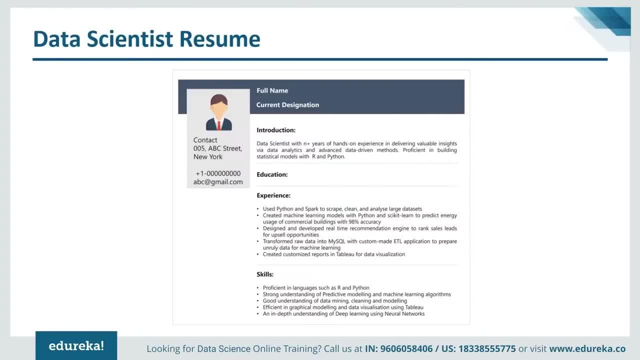 data-driven methods, Also proficient in building statistical models using R and Python. So here I've not only mentioned my experience, I've also mentioned a few skills. okay, Now the education field. I'll let you guys deal with it. Y'all can fill out the education field according to your. 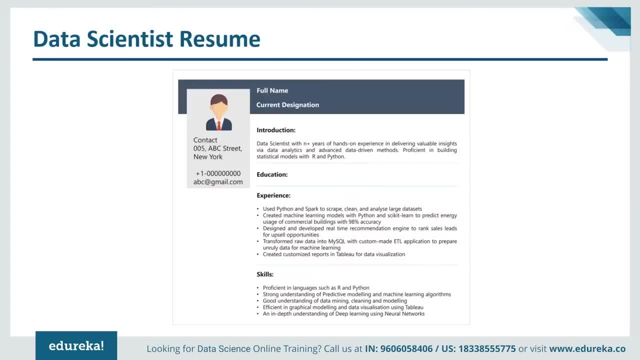 education. Now, within the experience field, you have to list down all the projects that you've done, all the data science-related projects, Whether it's text mining, whether it is NLP, whether it is predictive modeling, whether it's building machine learning algorithms, deep learning algorithms, anything. You have to mention all your. 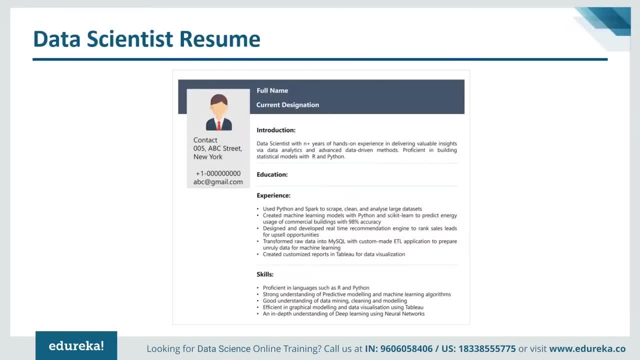 data science projects in your experience field. Here I mentioned I've used Python and Spark to scrape, clean and analyze large data sets, all right, So I'm basically saying that I have good enough information about the data lifecycle, I know how to clean and I know how to analyze and. 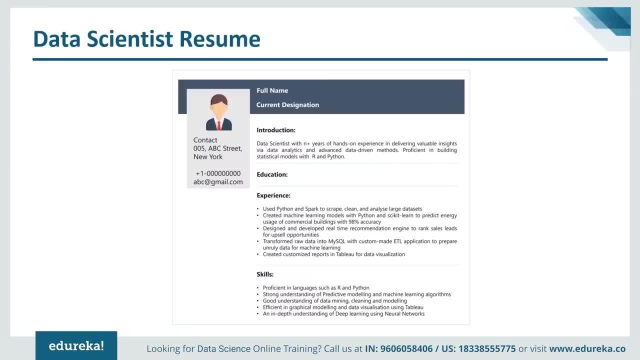 explore data sets. Then I've said, created machine learning models with Python, and I've also mentioned that I've created a model that is used to predict energy usage of commercial buildings with 98% accuracy. Now, guys, mentioning your projects is very. 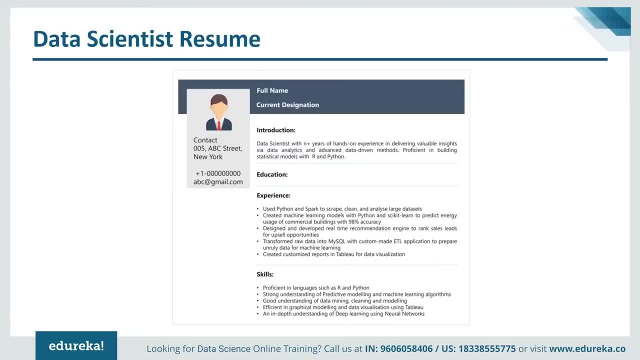 important. all right, Because that's the only proof of your capability. So you have to impress your interviewer over here. You have to show him all the projects you've done and you know how they have changed or contributed to your company. So next, I've mentioned design and develop real-time. 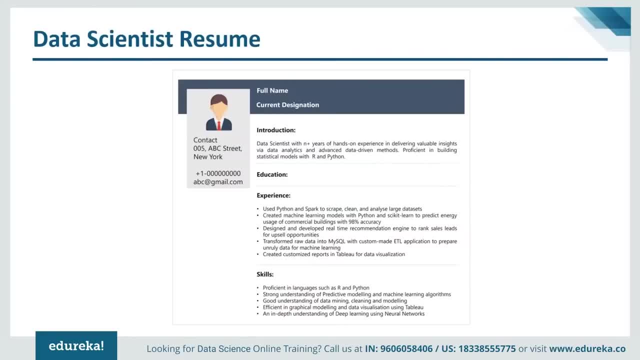 recommendation engines and then transformed raw data into MySQL. and finally, I've mentioned expertise in Tableau for data visualization. So, guys, make sure you don't skip data visualization. There are a lot of data scientists who don't pay much attention to data visualization. Data visualization is one of the 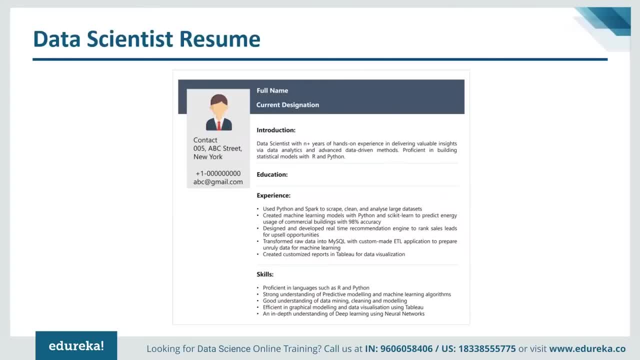 most important aspects of a data lifecycle, because here you're showing the stats and you're trying to show the growth in the company or how a particular variable or how a particular product is affecting the business. Okay, that you can clearly show using data visualization. Then I've mentioned a few skills. 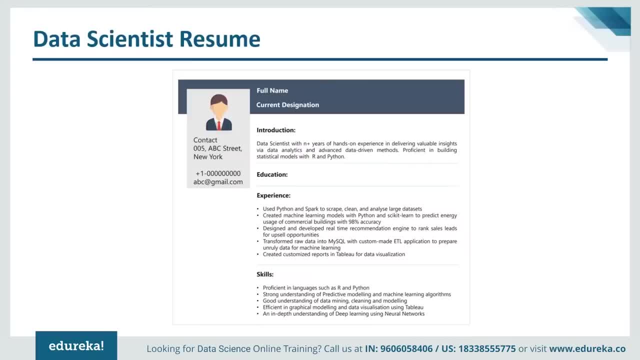 Here I've mentioned proficient in languages such as R and Python. Now, this has to be your number one skill, okay, You have to know R and Python very well. Then there is strong understanding of predictive modeling and machine learning algorithms, which I mentioned earlier. okay, 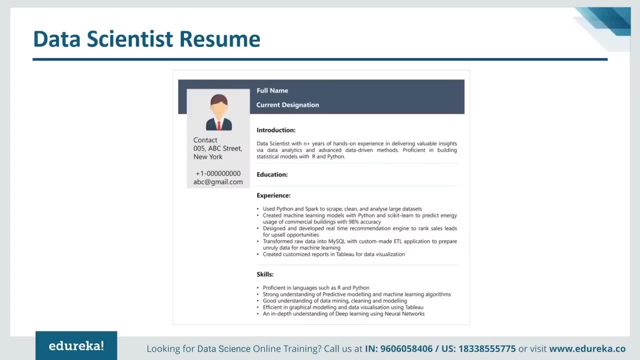 Machine learning algorithms and predictive modeling are very, very important. Predictive modeling is nothing but using machine learning algorithms in order to predict an outcome. okay, Good understanding of data mining, cleaning and modeling. Again, here I'm trying to mention the 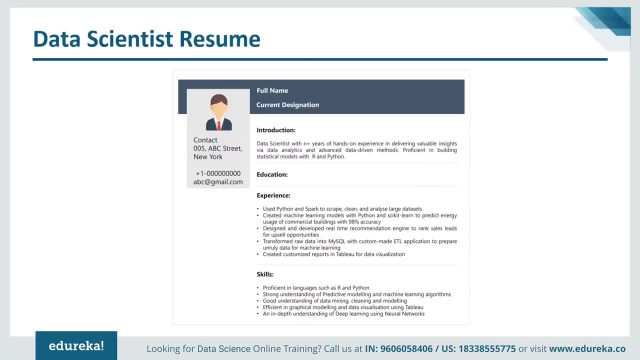 data lifecycle. and then, I've said, efficient in graphical modeling and data visualization using Tableau and an in-depth understanding of deep learning using neural networks. So, guys, this was the entire data scientist resume. Now I'll just give you a few key points that you should keep in. 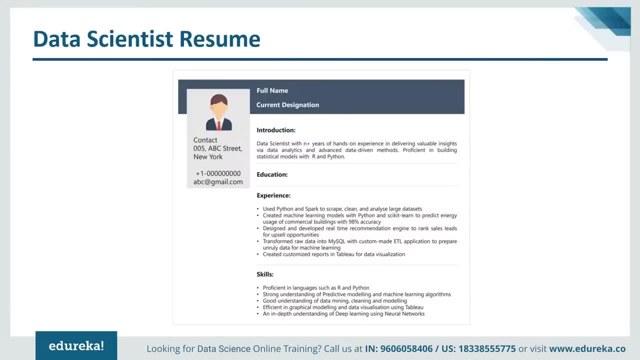 mind while you're building your resume. So first of all, try and state your career objective. okay, Make it clear and precise. State exactly what you're applying for and where your interest lies Now. within the educational qualification, you can mention your bachelor degree, your master's degree and usually people. 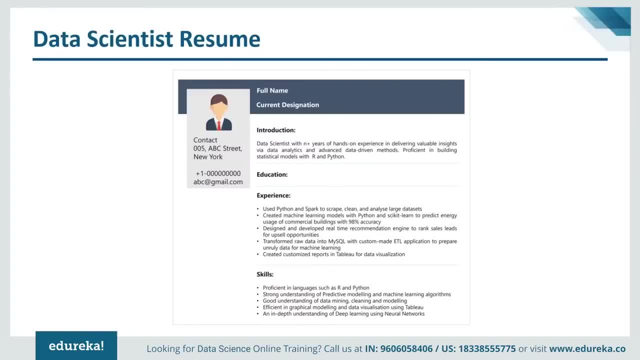 with the background of computer science or statistics are preferred, all right, But I'm not saying that it's necessary. There are a lot of data scientists who don't have a matching or an equivalent data scientist degree. It's not a prerequisite, but mostly people with a computer. 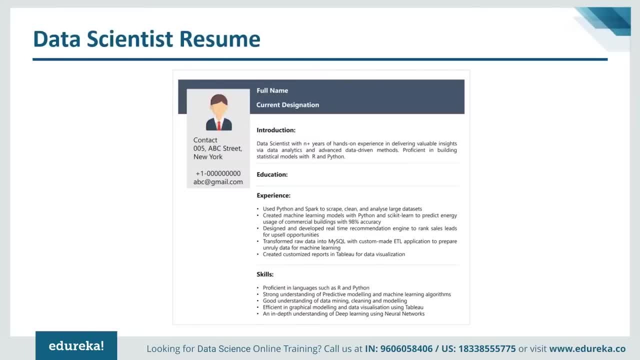 science or a statistics background are preferred. all right, Now, next, you can mention your professional experience. So basically, in your experience, you can mention your contributions to the company. okay, You can write about machine learning models that you created and you can see. 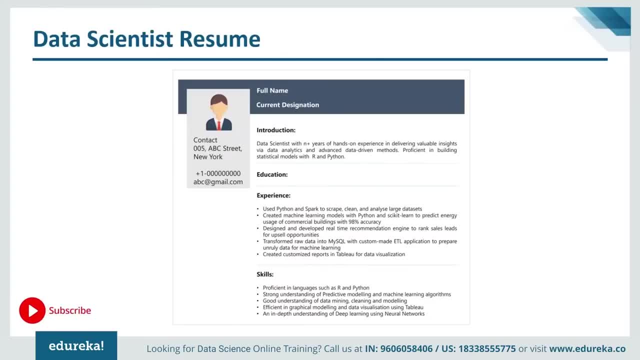 how it solved the business problem and how it benefited your organization. After that, you can mention your technical and your non-technical skills. Now, what are technical skills? Now, guys, technical skills are the practical abilities acquired from working on real-time projects and working. 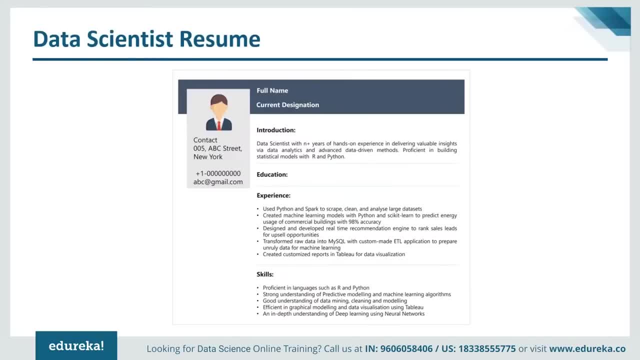 on field, okay. So basically, you have to prove your technical skills. So you have to prove your capabilities by listing out your skills. So make sure you list out all your technical and all your relevant skills only in this, okay, Because this is the best way to impress your interviewer by. 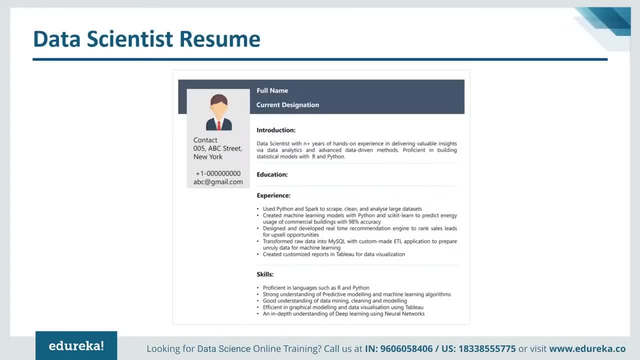 telling him how much you know and how much you've worked on, and therefore you know, these many tools or these many technologies. Now, in the non-technical skills, you can impress your interviewer by showing him how strong your communication skills are and how strong your. 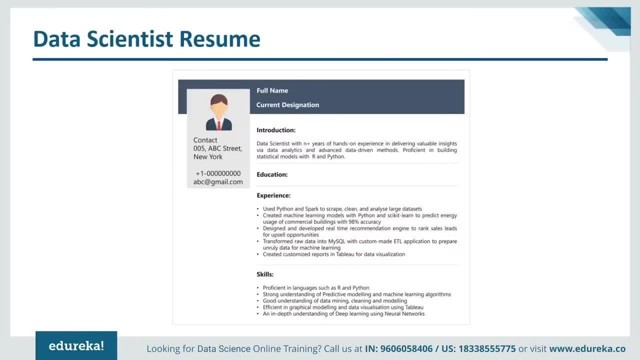 intellect or your analytical thinking is okay, Because a data scientist is not somebody who is an hardcore programmer. You have to have very good business acumen. You have to have very good communication skills, because you're handling a business okay. A data scientist is going to talk. 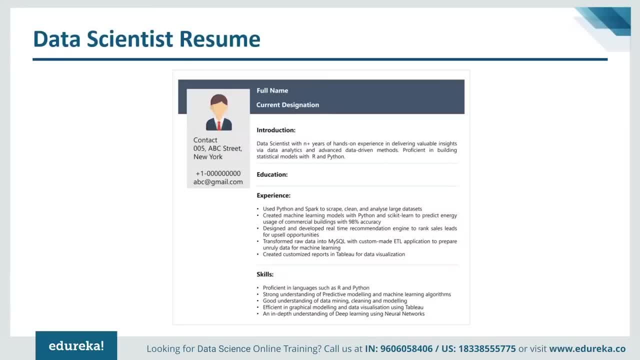 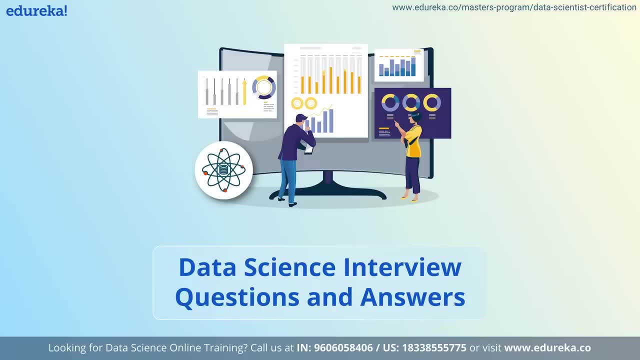 to other stakeholders, communicate their company stats to other stakeholders. So data scientist has to have excellent communication skills. So let's start with the questions here directly. We'll, in the beginning, start to focus on some of the things that you've learned in the past, So let's start with the questions here directly. 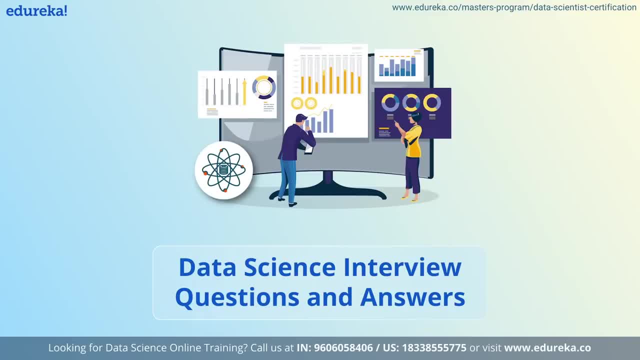 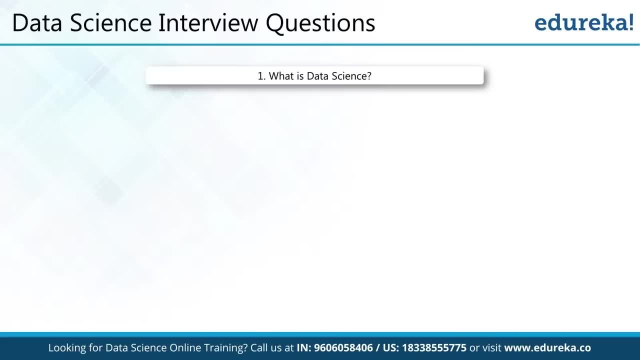 We'll, in the beginning, start to focus on some of the fundamental questions, which is more for you to understand what is data science? than like a particular interviewer asking you that question. For instance, many people wonder what data science is all about, right, Though there are many online. 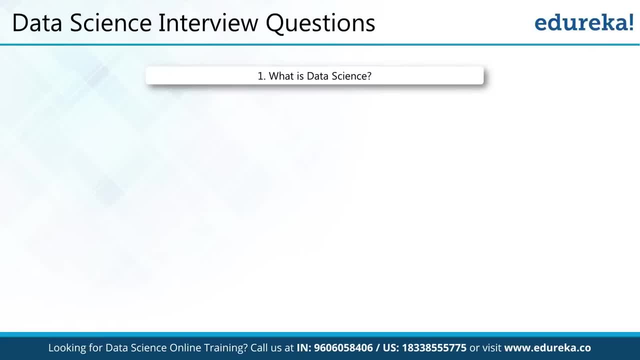 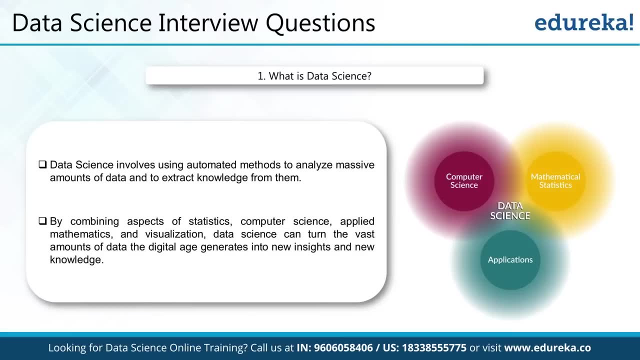 sources and blogs, which describes data science in a very nutshell. this is what it boils down to right, A person who is very good in understanding the computer algorithms, a person who understands the statistics and a person who is very good in understanding the data science and a person who 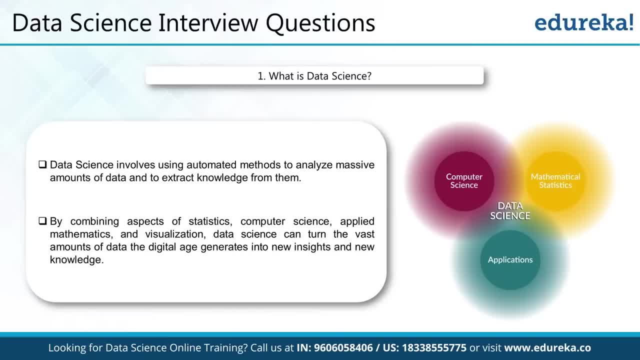 understands the statistics and mathematical ideas and applying these two knowledges from the computer science and mathematics into a particular application, right A business application where somebody sees a value coming out from the data. So how do you apply that? So that's how kind of 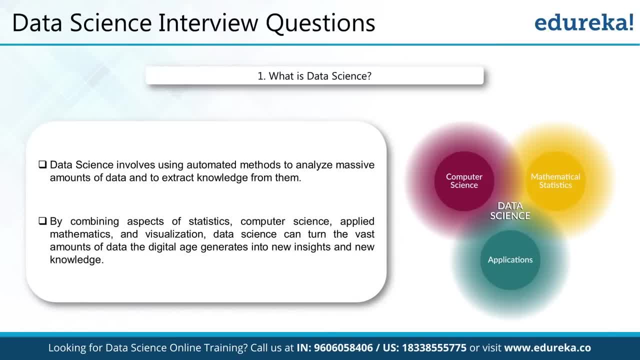 data science approaches. So when you combine these two powerful concepts coming in from computer science and mathematics on a real-world application, the sort of outcome that comes from a particular data science project goes in a direction where it's not just about the data science, it's about the 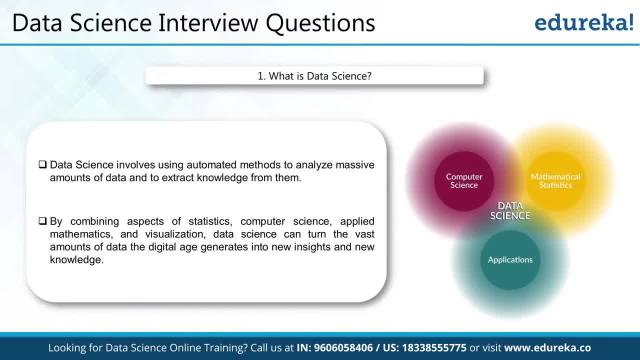 data science project goes in a direction where it's not just about the data science project, goes in a direction where people see a return on investment, right. So the people you bring in, the technology, you bring in the ideas you are working on, all of it should kind of give you some return on the investment you have. 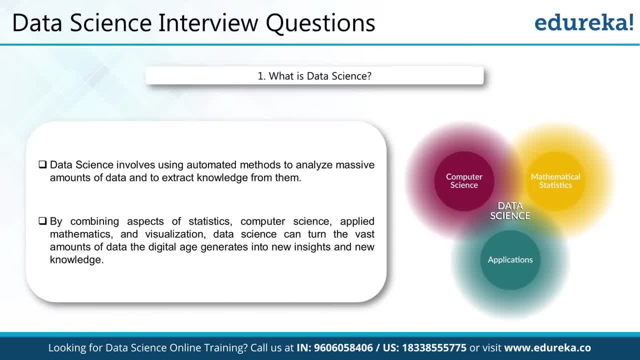 put in. So that's where industries are started to looking at data science. So various subjects which are very important for you to know: statistics, computer science, applied mathematics, and then subjects like linear algebra, calculus and a few more right. So fundamentally from computer science. 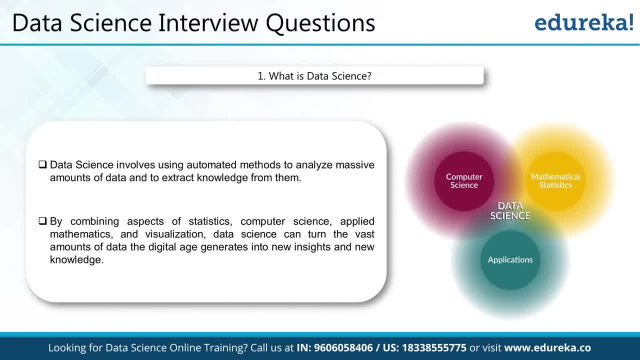 algorithms and data structures might be very useful from the mathematics or statistics and things like calculus, linear algebra, matrix, factorization and concepts like that, And from the application. it is more from your experiences from the industry If you have worked for retail. 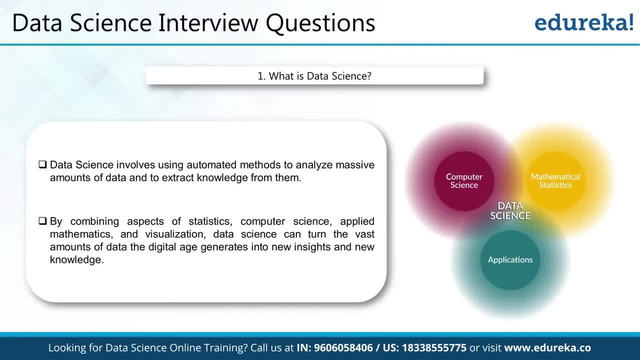 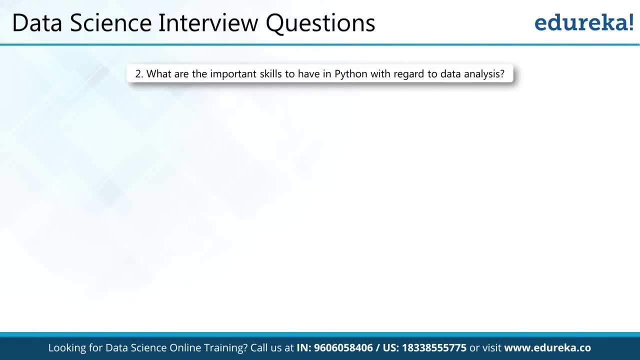 you know how the business process in retail works, right? So people often also ask from the technology end, do we need any sort of experiences in Python language, right? Python or whatever like, for example, R programming as well? So Python is one of the most looked out. 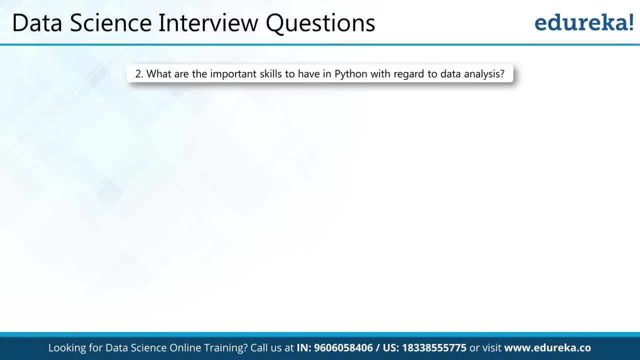 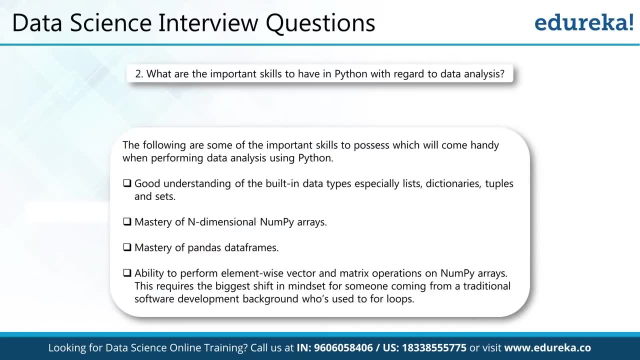 for kind of programming skills, particularly when you want to build solutions in data science domain And with availability of libraries like NumPy Pandas, Python has now established its ground very strongly in giving a very robust framework for designing data science solutions And, in particular, things which it has. 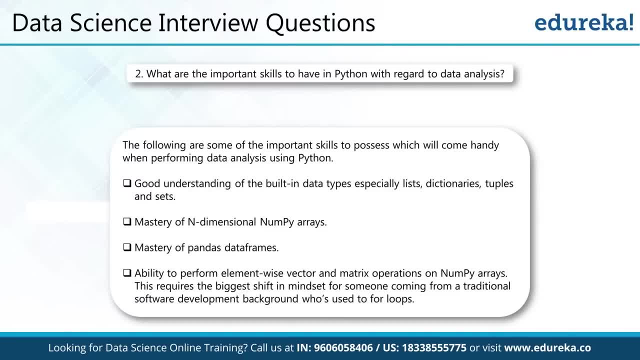 like list, dictionaries, tuples and stats are one of its own sort of one of its capabilities, which sets Python in its own league of programming languages suitable for upcoming out with data science solutions. So there are many more other libraries as well, apart from this, for building machine learning algorithms. 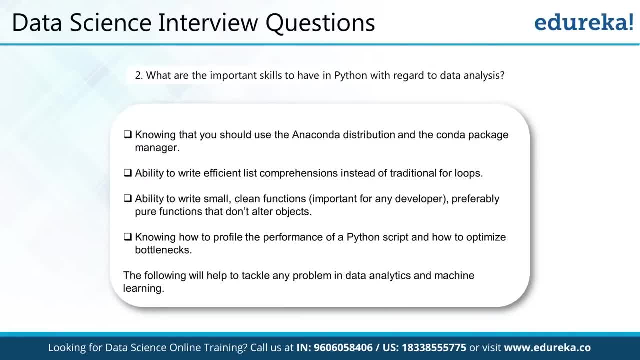 But these are some common libraries that you would not really find people using it, And also with distributions like Anaconda. Python has shown its capabilities even for a production grade solutioning right, Wherein you make sure that all the dependencies that one particular library has. 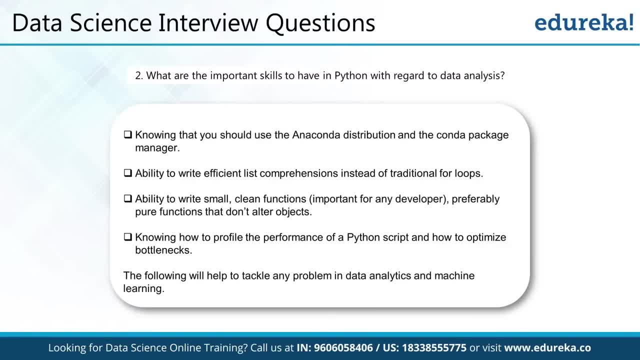 for building a data science solution is all in one place, So quite a popular programming language in the recent kind of happenings, Although R programming is also equally good in terms of producing a quick prototype for most of your modeling tasks. But Python is moving itself into a production grade. 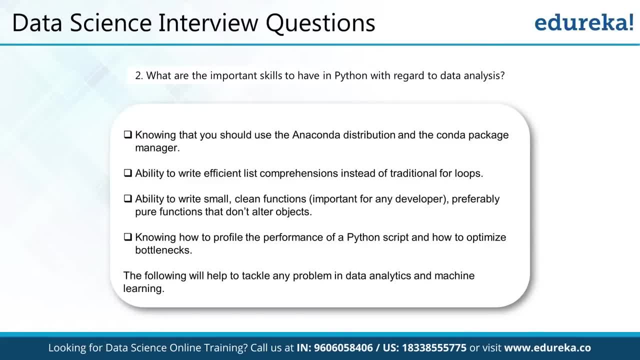 where things can be deployed after the sort of prototype into a production environment and it can phase the customers from day one. So that sort of capabilities are coming up with Python, right. So let's talk something a bit more specific with the data, right? 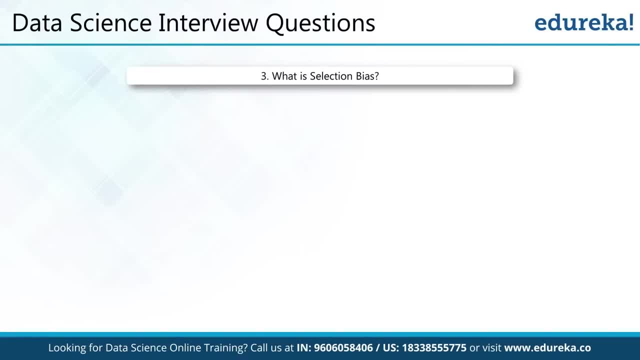 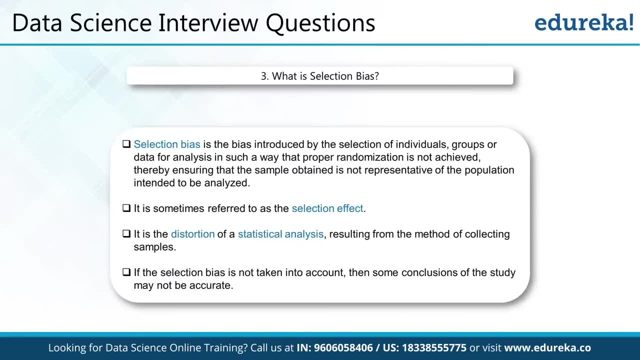 So when people are doing any sort of data analysis, they normally face something that we know by the name selection bias, right? So what is actually a selection bias? The fundamental place where you start doing a data analysis is by selecting a representative sample. 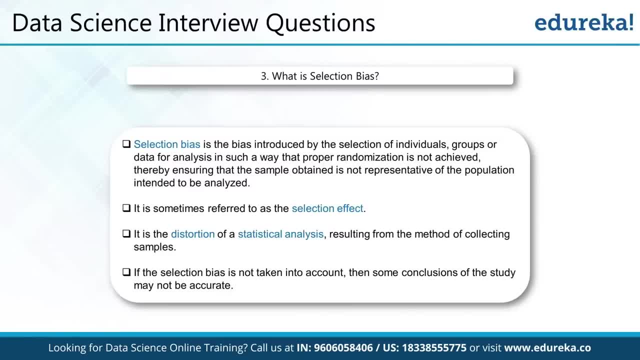 So that's where we like normally start doing any analysis. So when you like working for a company which has, let's say, one billion records in their databases, like one billion is like very, very large number which represents various customers data, or it might also be, depending on which feature. 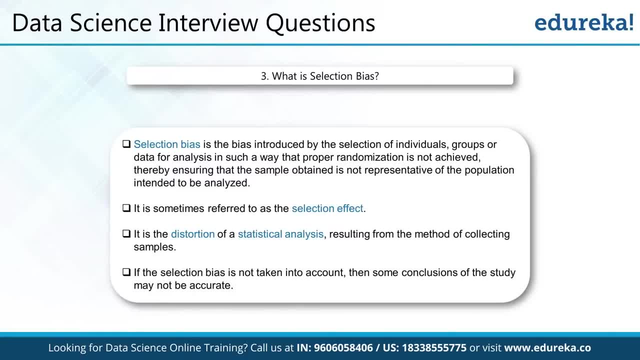 you are working on and so on. So if you collect all of those, it might very easily come to one billion records, which is nothing but in a structured form, number of rows. So with that, an enormous amount of volume in the data. this is that you take up might have to have a lot of filters. 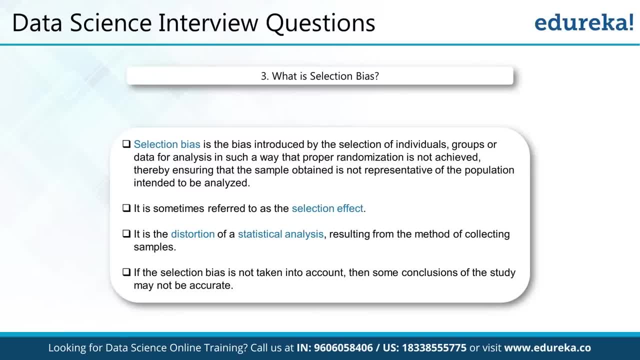 like saying: I only want to analyze a particular feature in my products. let's say right, And I only want my customers from XYZ region, which is, let's say, top four region or top five regions, So you might like put many features or filters like this: 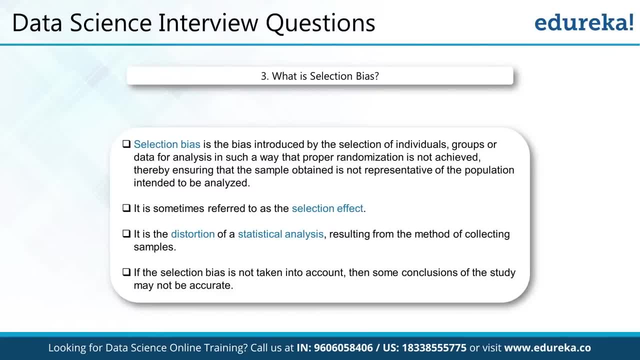 But later on, if you would like to do a kind of an analysis which covers most of your customer base, right There comes the tricky situation of not being able to use the entire volume of one billion records. at the same time. you want to do a really good study or analysis. 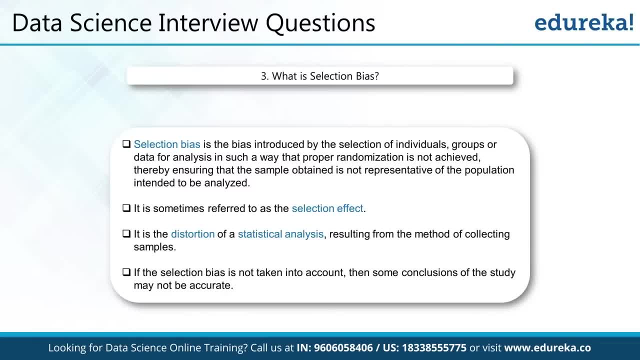 based on what data you have. So in statistics we normally use this idea of doing a kind of a randomized selection, right? So with this randomized selection, we make sure that out of these one billion records we are choosing a small subset, let's say of one million. 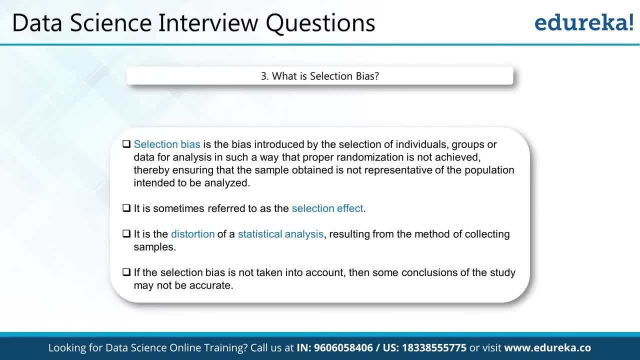 which is a true representation of the entire population. right, But what happens with this is, while we do this one million record, selection based way, there are chances that you might have certain bias in the analysis, obviously because you're not using the entire population. 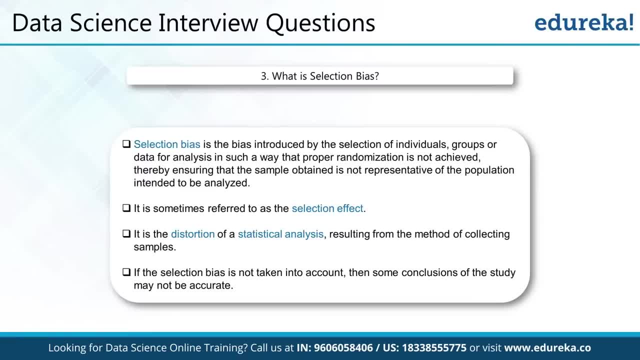 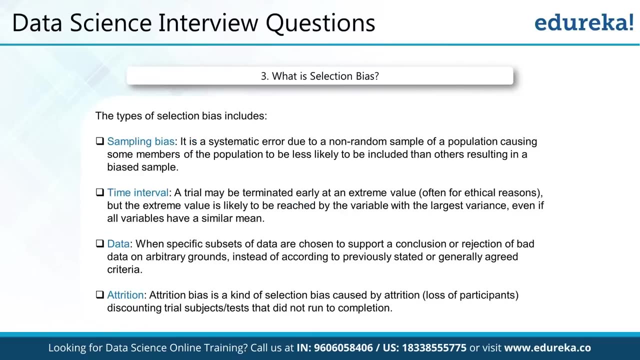 So selection bias- is this particular sort of a characteristics while you are doing a sampling on a large population of data? Very common example for this is if you want to do a exit poll analysis of particular election even before the election results are coming up and you have not chosen a representative sample. 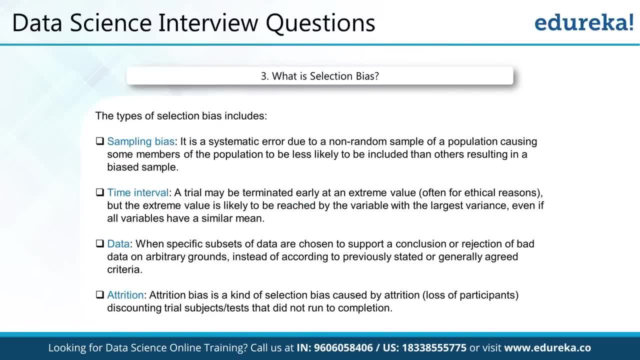 for doing that exit poll analysis right. By that you- I mean you- only have one million records. you only have asked some questions for a selective view from the particular constituency and they have an opinion towards one candidate, but that doesn't represent. 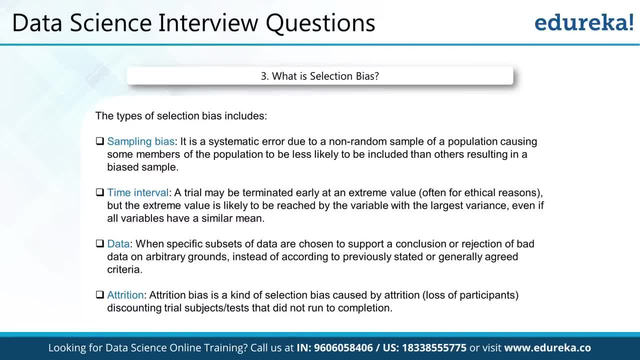 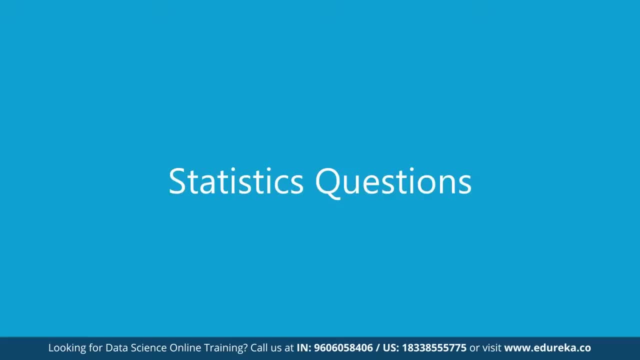 the entire opinion of the population in that constituency. So selection bias is like very important to handle and most of the time people employ things like randomized selection or selection sampling techniques like stratified sampling and so on. So by that you can minimize this selection bias. 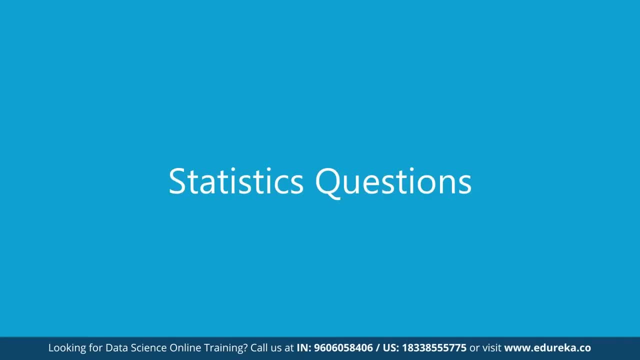 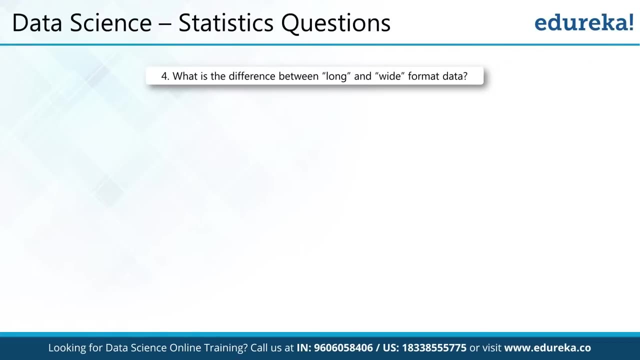 So these are some very generic questions. So let's start With some sort of statistical questions and also how to deal with different types of data. Okay, so doing any sort of data with a structured information. So structured information I mean there are many rows. 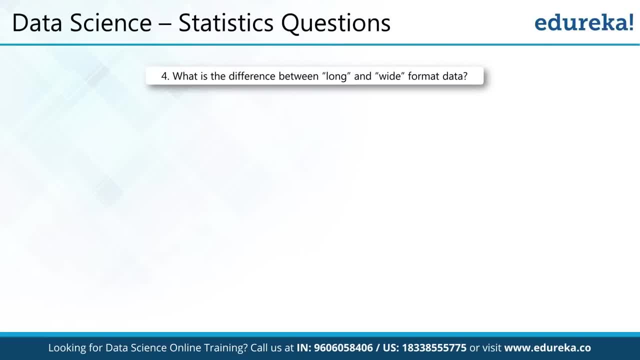 and like many columns, and it looks more like a tabular data, right? So with such a data in place, there are, like these, two different formats, one saying the long and the wide. So let me like show you an example. here You have a record of two customers. 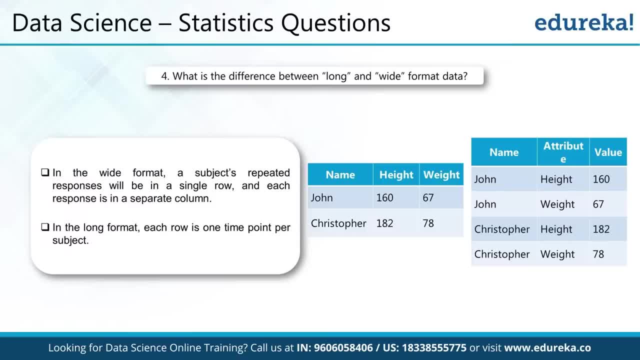 And you store just two values, which is the height and the weight. So these are like in columns. So with these two customers, these height and weight being a separate column, is one format, like a long format. Let's say, transform this by having only one particular column. 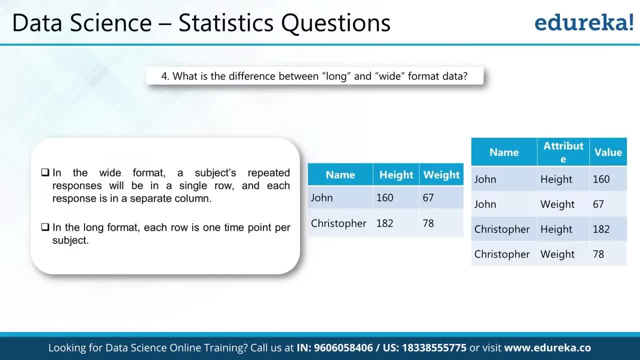 which will say attribute. By that I will bring in these two columns as one column, by calling that as an attribute, and put the values in one column. So this sort of format is called the long one. What really happens is, instead of having two separate columns, 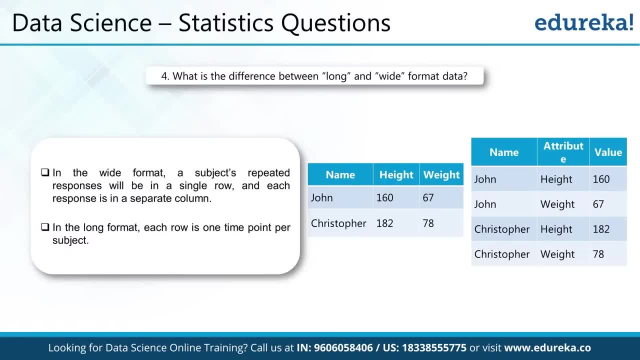 for two of your attributes, you put both of those into one column, And by doing that, there are a lot of benefits with respect to the task you have in your hand, particularly in data visualization. Certain data visualizations would need you to not put your attributes as a separate column. 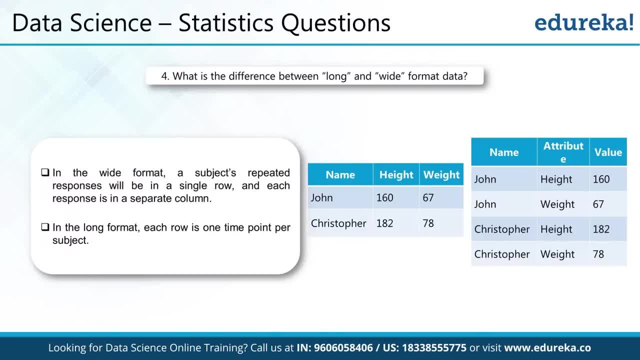 but rather as the one column which can have the attribute names, So which might then go into building your legends right. So these kind of techniques, these kind of techniques are kind of very common formats between like the long and the wide, and very frequently will people like deal with. 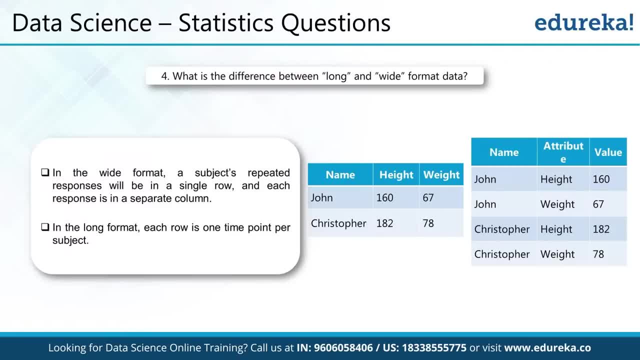 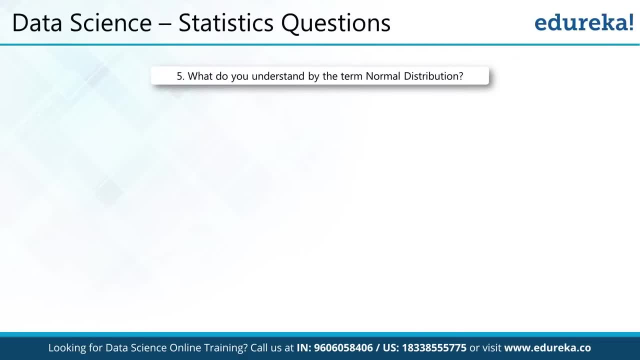 both these data formats, depending on what task they are doing, particularly when we are building the visualization dashboards. Okay, talking a bit more on the data analysis perspective, people like know that in stats, normal distribution kind of is that one like the godfather of the distributions. 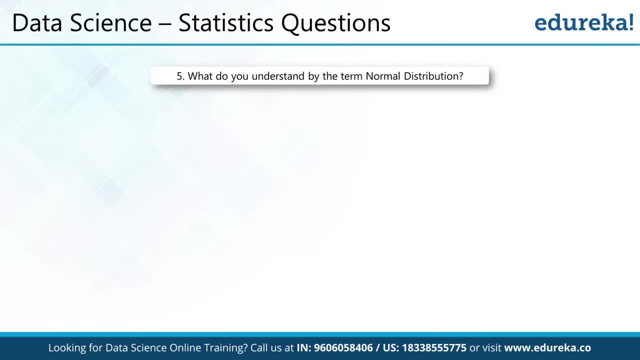 You have many distributions which normally people try to see if is present in my data or not. but the moment people kind of see normal distribution coming up in any data, things are kind of a bit easy to understand And in typical case any distribution. 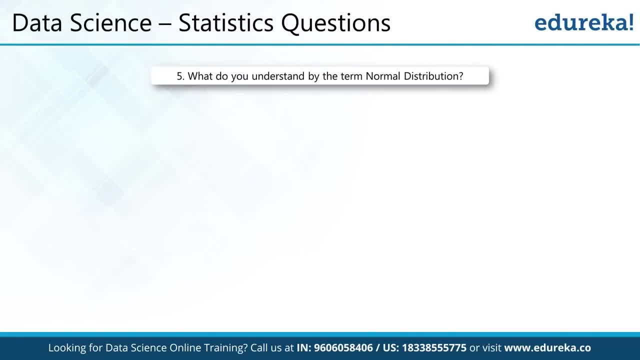 any data distribution that you would like to find out. given data for analysis, it gives us a lot of characteristics around what the data is about. If I'm, let's say, analyzing the salaries of the employees in my company, right, I might see that there are some employees. 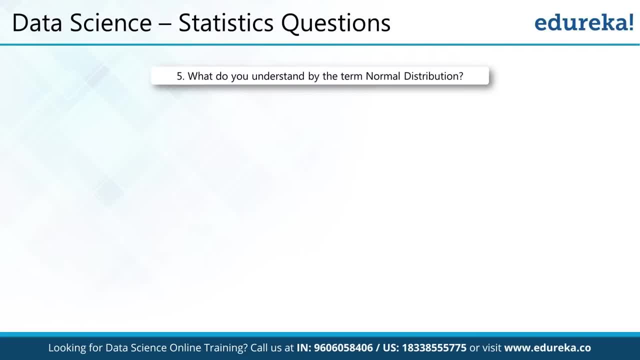 who are in like that thick crust in the center where majority of the people are sitting with a moderate level of salary ranges, And then there are these sort of extremes on the left and the right. So you are like very commonly people refer, whenever you talk about salaries, towards the bell curve. 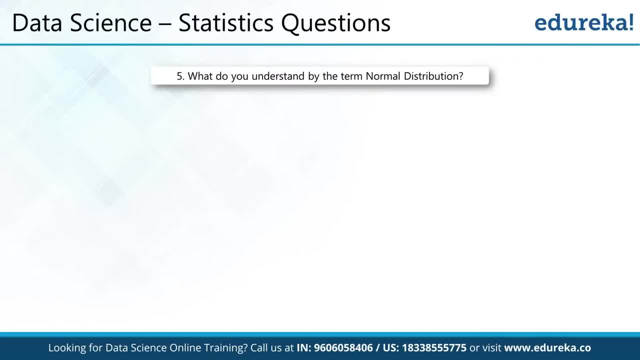 and then they start talking about top 25% of your performers and my company, the bottom 25 and the middle one which your like, our sort of performance team, the normal performance. so this sort of bell curve distribution is very commonly understood and, as 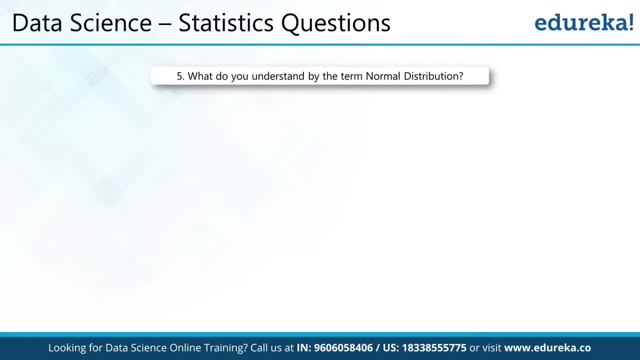 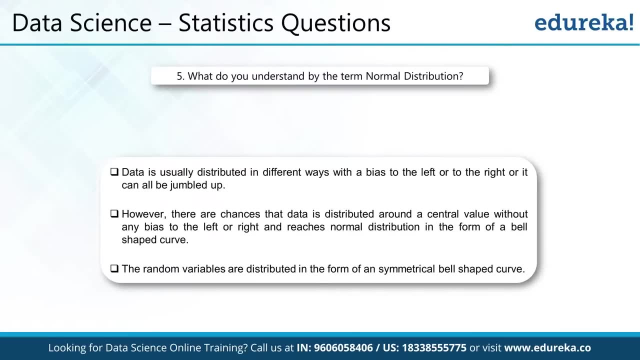 well as used in doing many data analysis. so is the other distributions as well, but normal distribution has its own significance. so when somebody asks you around anything, around not normal distribution, the first thing you should visualize is the symmetrical bell-shaped curve right, and the moment you get that bell-shaped curve in your imagination, start thinking of. 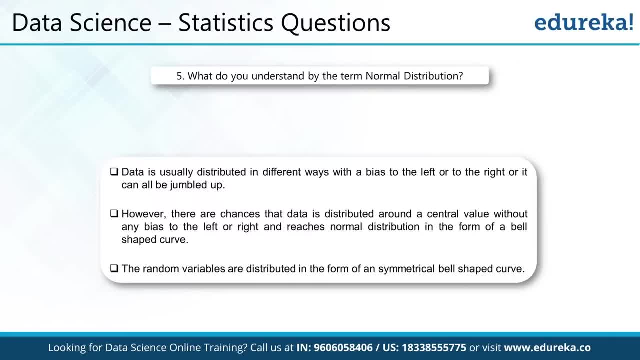 certain properties, like what is the mean of a normal distribution, what is the standard deviation of a normal distribution and, in particular, a special case of normal distribution which we call the standard normal distribution. so in that standard normal distribution, we know, the mean is exactly 0 all the time and the standard deviation is exactly 1 right. 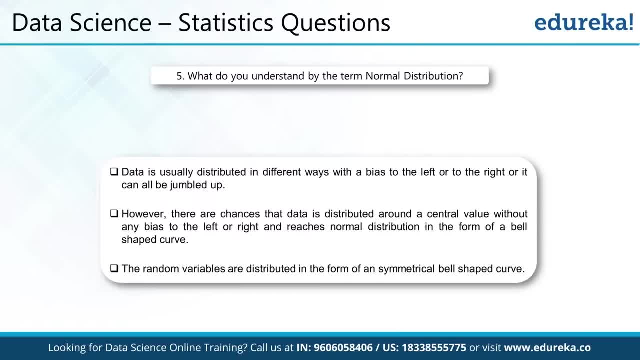 so there are different places where normal distributions are kind of used, and if you are comfortable with ideas like center limit theorem or the law of law, of law of the law of large numbers, you might want to relate that as well to normal distribution, particularly the center limit theorem. right, but the idea is a distribution which is symmetrical around. 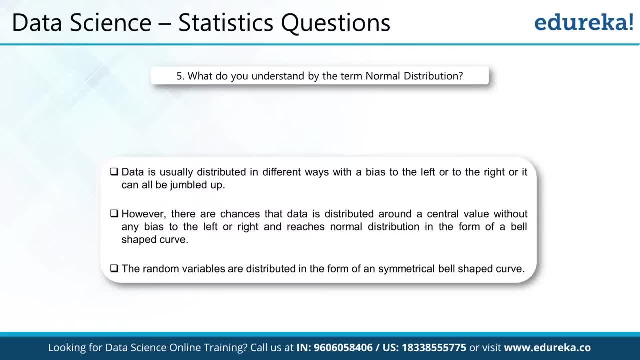 the mean. so that's what a normal distribution is. so, depending on which variable you are trying to analyze, even a given data set, whether it could be like an employee's salary or your sales in a for a business of yours right, or your number of, let's say, interactions of the 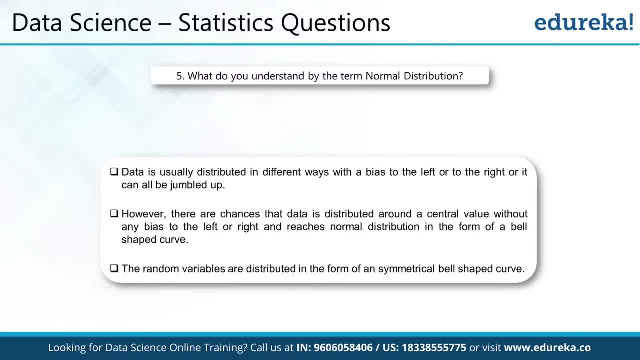 customers on your project. So any variable that you define can have a symmetrical bell-shaped distribution, which we normally refer by normal distribution, and the moment we understand that something follows a normal distribution, all these properties of that distribution is like revealed. so that's sort of the importance of doing any analysis around the distribution of data and normal. 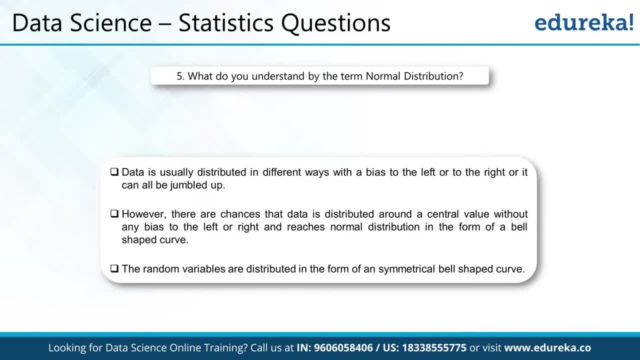 distribution like very common one and in many statistical techniques in even model building exercises. if you have anything in a normal distribution, many other possibilities of a applying certain modeling techniques comes out evidently there and also there are many other modeling techniques in stats and machine learning where there is an fundamental assumption. 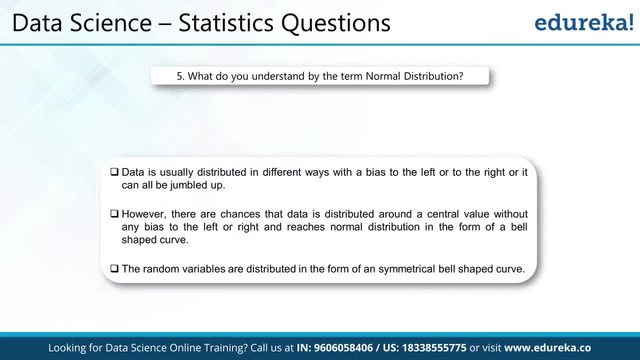 that things should follow a normal distribution. if it is not following, then the model is wrong. there are many use cases of for knowing what normal distribution is, but in simple terms it's a symmetrical bell-shaped curve right a b testing. so quite a popular approach, people. 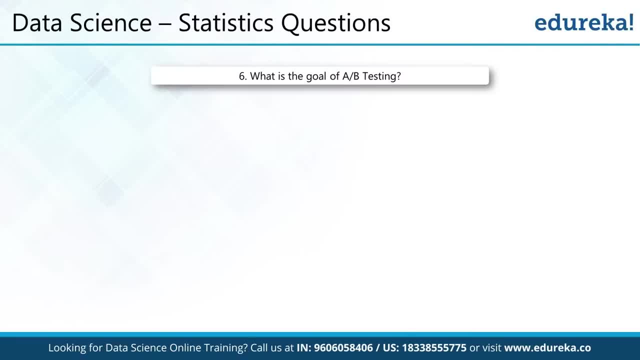 particularly who are working with product right, and what happens is When you are, as a company, having lot many features inside a product. for instance, if LinkedIn is a company which has a web page, right, it has lot of features inside that. you have some jobs portal in LinkedIn. you have places where you can connect to your professionals in the similar industry. you can also read about the post people are doing in the portal and so on. so there are different places in the website with many features. so what happens is if LinkedIn, as a company, is looking for some changes. 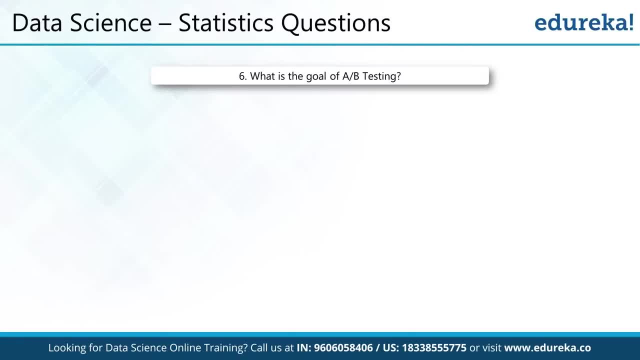 For instance, changing the entire websites, design in aesthetics. design and aesthetics are changing one particular feature inside their website, right? These changes are normally accompanied by sort of a process called a b testing. so what happens? as an analyst, you might be working with LinkedIn and say on a fine day, they might come out with a new feature, a new design or new sort of changes in their website. so you as a person would tell: okay, this is my framework for testing this new change. 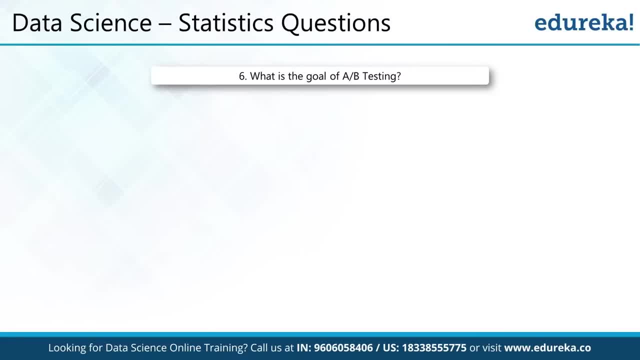 So you as a person would tell: okay, this is my framework for testing this new change by defining a metric. so my metric would be in simple terms saying: if I change this website from A to B, is my number of footprints on the website going to go down or not? so this: 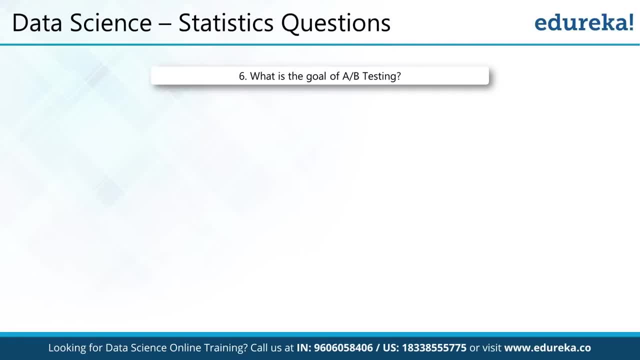 is my metric, and if I successfully establish the fact that, after rolling out this new website, my number of customers who are going to visit my website is not going to go down, I can be confident that. okay, fine, this works. now roll out this new feature. so, in this framework, 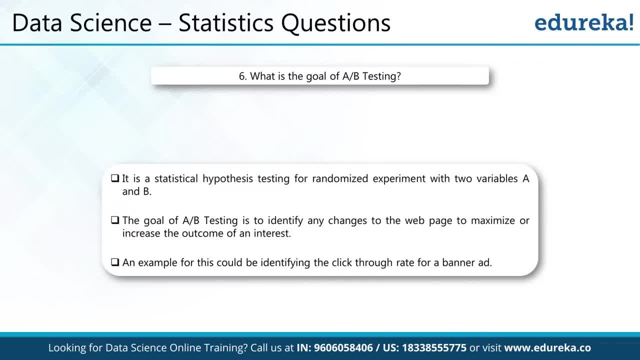 we normally have two set of users to identify the particular risk associated with getting this new feature into the platform and in which we, in a randomized way, put one user group and expose them to an older website and another user group and expose them to the newer new features, right or the new website. and when we compare the results of a particular 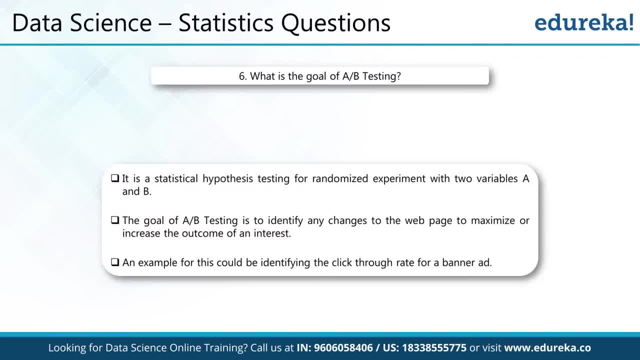 metric, like the number of clicks or the number of purchases and so on. we should be able to see that the metrics are not going to be the same as the metrics that we are seeing in the data, and we should be able to see that these two groups are either exactly the same. 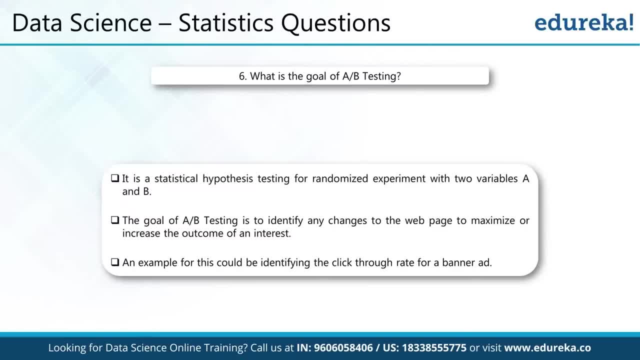 or quite different. and if it is on the negative side of the difference, we say the feature is not good. and even if, when the difference is not at all there, we say: even if we bring this new feature, nothing is going to happen. so this A-B testing framework is quite robust. 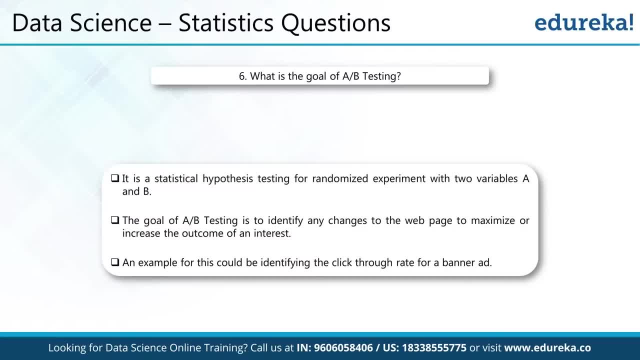 in its own way. right, and a very common question: if you have like worked as data analyst or if you are expecting to be like sitting for this data analyst kind of work and you are doing this kind of a role, knowing A-B testing framework is very important, ok, so sometimes 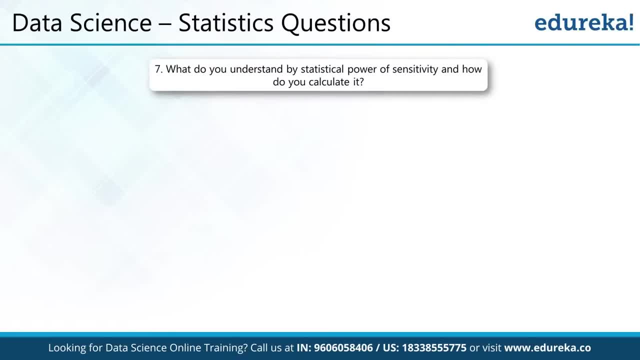 also, when you do these kind of A-B testing sort of analysis, people normally come out with sort of saying: what should be the sample size of my users whom I should be getting to participate in my A-B testing framework? or also when you are building some models. 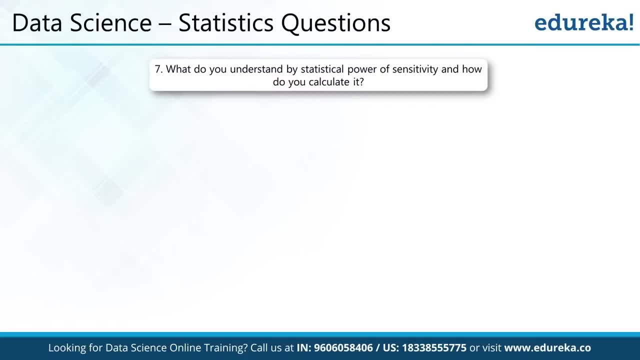 you might see that there are certain statistical measures which has to be evaluated and then evaluated by the end of model building exercise, like if you are building a machine learning model, let's say, and you want to see if the those metrics on which I am evaluating are. 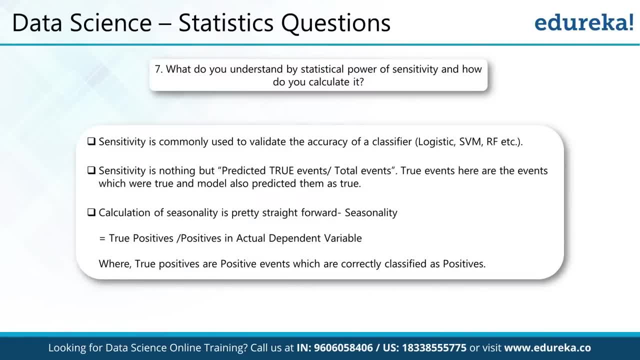 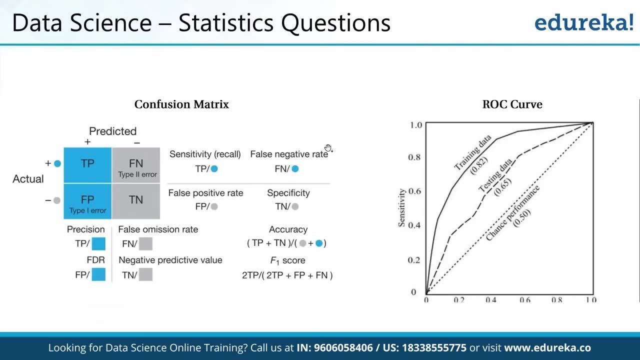 really good or not right? so in that sensitivity is one of those methods, or like metrics, which we normally evaluate, and I am going to show you some, something that we normally refer by the name confusion matrix. so I will spend some time explaining this and then come to 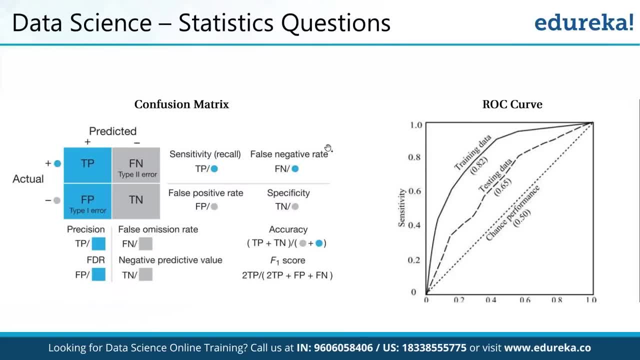 what we mean by like sensitivity. So let's say you are building A model, right, a model for predicting whether a particular customer is going to purchase from my platform within one month or not, right? so very simple problem statement, which might include many variables that we would bring in and then finally build this model saying: 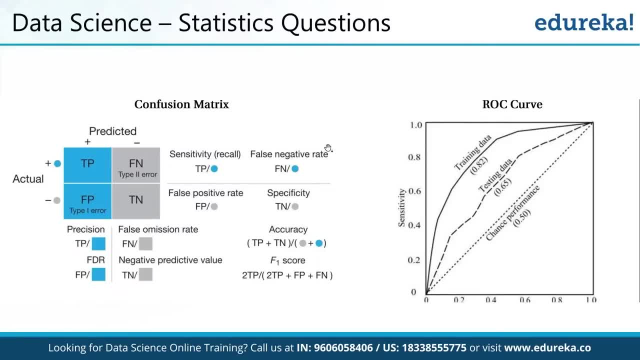 ok, this is my final model, which says, with 90% accuracy whether my customer is going to buy from my platform- let's say, an online e-commerce platform- within next month or not. so this is my model. so now, as you, without going into the details of the model, let's: 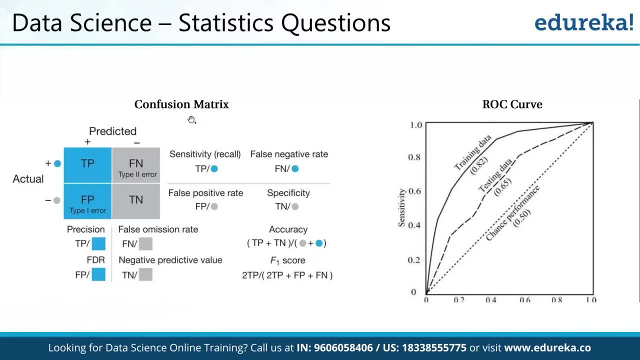 assume That after you build the model, you have got the results. so while we analyze and evaluate what the result is all about, we might come out with a confusion matrix. so what it says. so obviously, when you are building a model which follows a supervised way of learning, 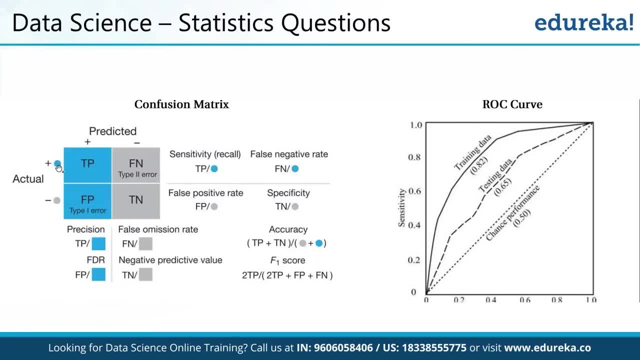 you will see from the historical data after people have purchased in the platform within next one month, whether they are buying or not. so I can obviously create a really good training data set right Which will contain the information after people. let's do the first transaction with me in. 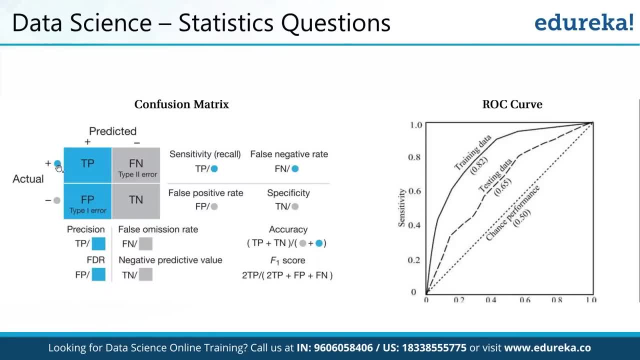 next one month, whether they are buying the next product or not. so with that data set I train my model, and the wave confusion matrix puts that is by saying: my actual data says something and you have predicted something right. so let's kind of get into the details. 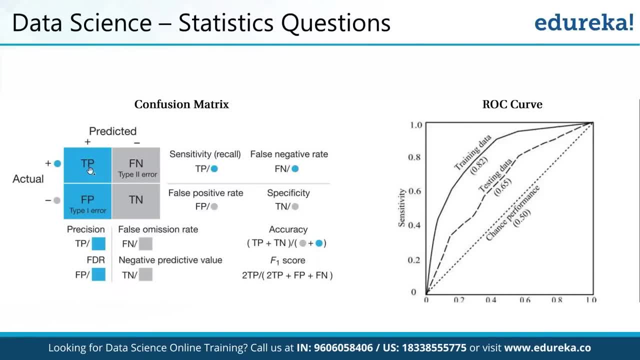 of that. so this particular box which says my actual data, says the customer will buy and you are also predicting the same. so this we call the true, positive. The prediction is actually true, right in a positive direction, saying the purchase happened now like moved or diagonally opposite to this TP, which is this TN, which is true, negative. 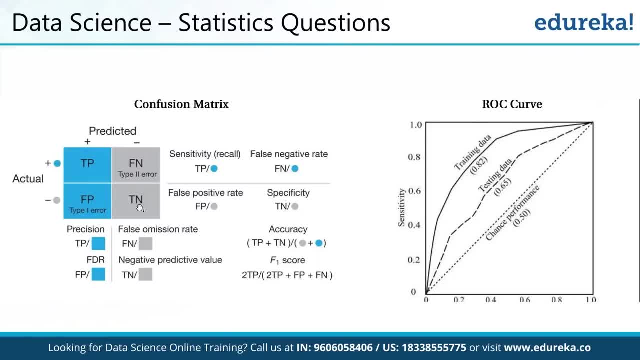 which means the prediction of your model saying the customer will not buy is actually matching with the actual data as well. right? so both of these values, the true positive and the true negatives- for the two cases is the right predictions from your model. but consider the off diagonal elements, the false negative and the false positive and these two cases. this 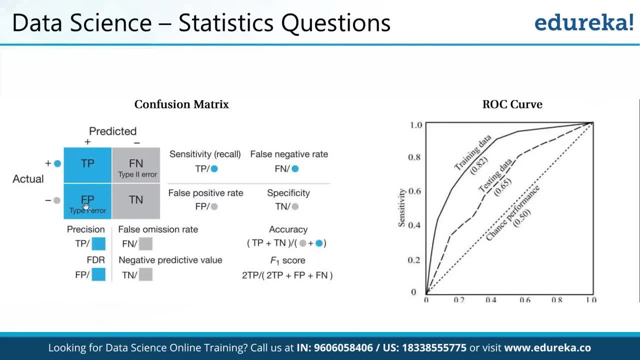 is sort of an error. why? because your actual data says the customer is not going to buy. in this case, let's say: but your prediction says he is going to buy, so the prediction is actually positive, whereas the actual data is on the negative side. so this is a false. 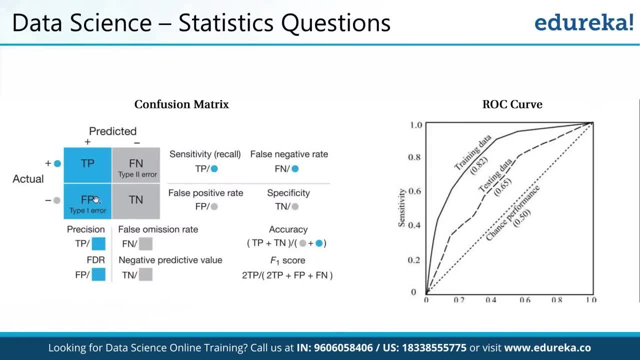 prediction right. so you have your, in this case your FP, which is the false positive cases, and on the off diagonal element, If you look at this one, which is FN, which is your false negative, for the cases where you are predicting the customer is not going to buy, but in the actual data it says that 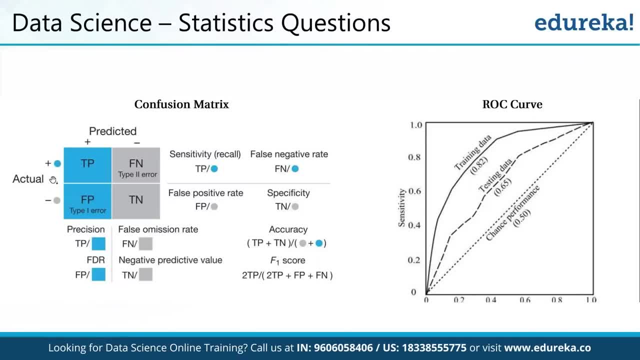 customer actually has brought the product. so in this case the model is wrong. so the type 1 and type 2 errors needs to be taken care of when you are building any machine learning model. if these errors are low, then your model is going to move towards that 100%. 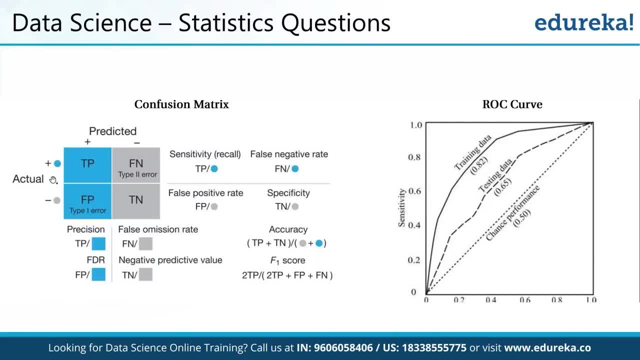 accuracy mark. but normally any machine learning model has its own limitations. so particularly there is one metric which we refer by calling sensitivity. so what happens is these true positives and true negatives needs to be controlled, right, if my model is very good in true positive ones, like the positive cases of when the customer is buying, but it is doing very bad job when 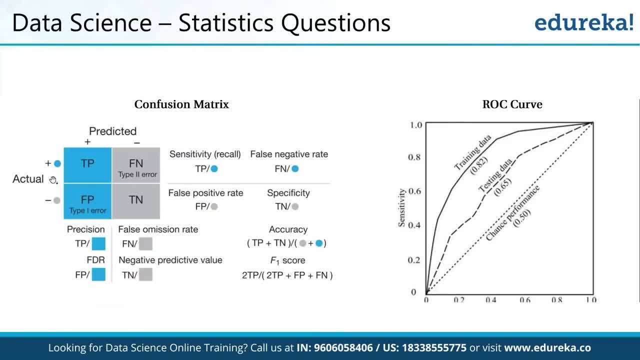 the customer is not buying. the cases in which the customer is not buying, then the model has some sort of issues. right, it is doing only good in one place but doing very bad on the other case. so I need to find out that by some metric. So sensitivity: 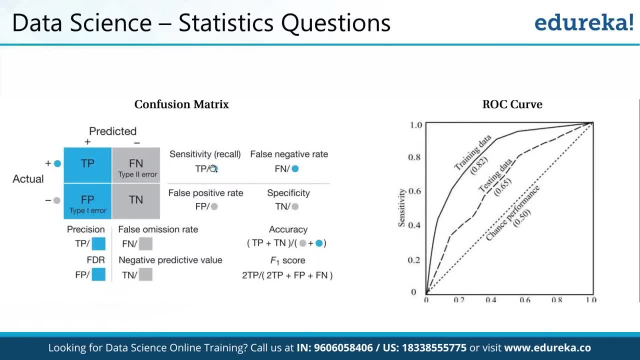 So sensitivity- help us to find that out- which is, in simple terms, is a ratio between the true positive in the denominator. we have all the cases of positive predictions. so imagine now if the type 1 error is going to grow, my sensitivity is going to come down. so if my 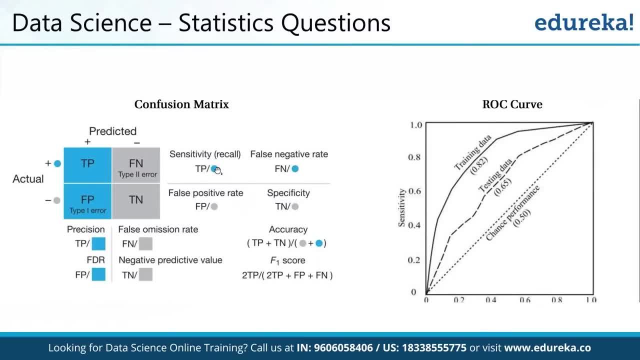 true, positives are like very high, the sensitivity will also be high. so this is sort of what we call the statistical power. if this sensitivity is really good, I would say that my positive cases are predicted well. And the exact opposite of this sensitivity is what we know by specificity. so we need 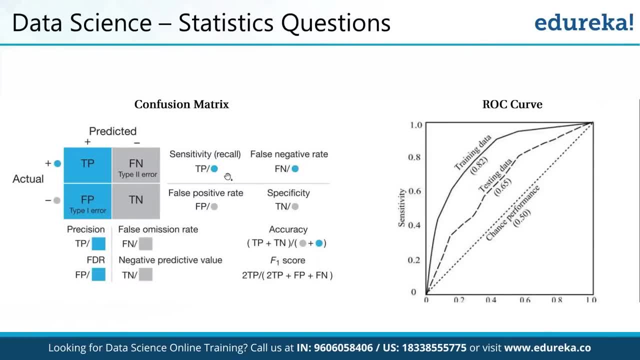 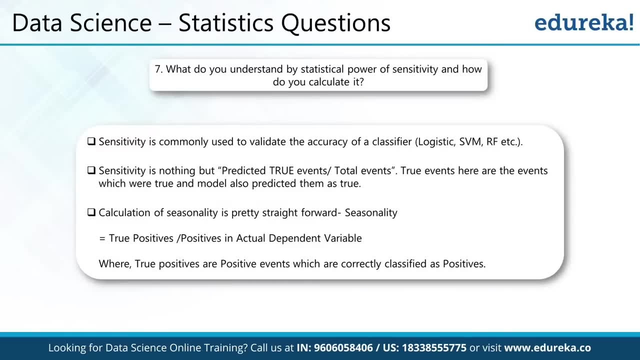 to make sure that in a very good machine modeling, model sensitivity and specificity- both are balanced right. so in very simple terms, this is what it will be like. mean here the ratio of true positive by total positive events there and, as I mentioned, both of these- sensitivity and specificity- play a good role when you want to evaluate a model's output right and 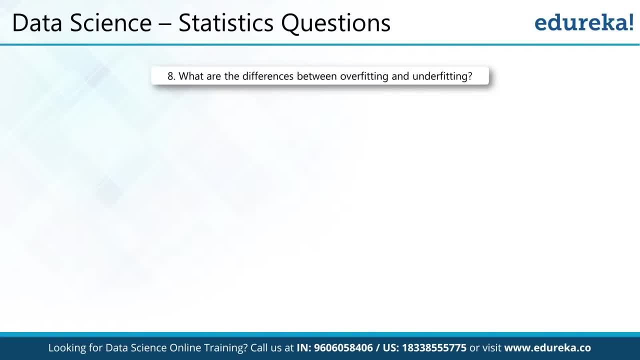 one more common problem, so these questions might be immediately following one another. when people ask You about sensitivity and specificity, as you know, it's about the machine learning models output. right when the model is done, you understand whether the model is good or not. so in those 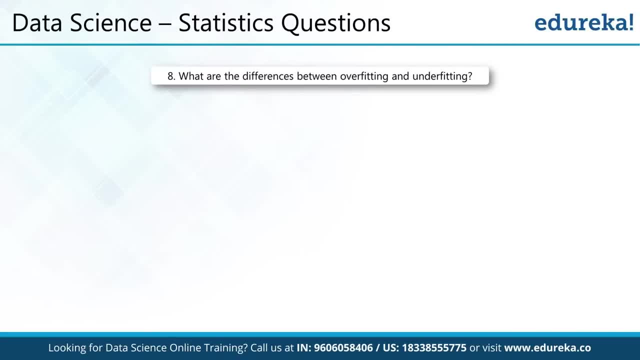 cases we also come across some kind of issues like overfitting and underfitting, given machine learning model, right. so these words are very common and the idea is: depending on the complexity of your model, you might see that you want to adapt very sort of exactly to your data. 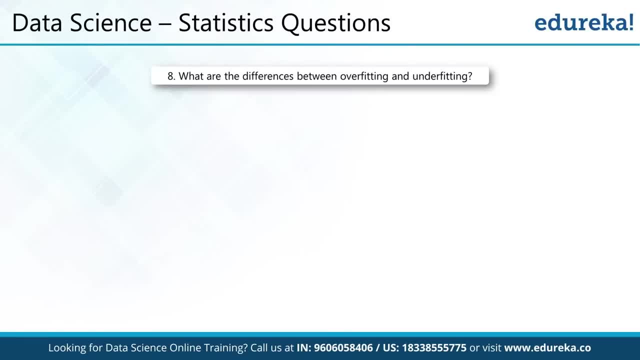 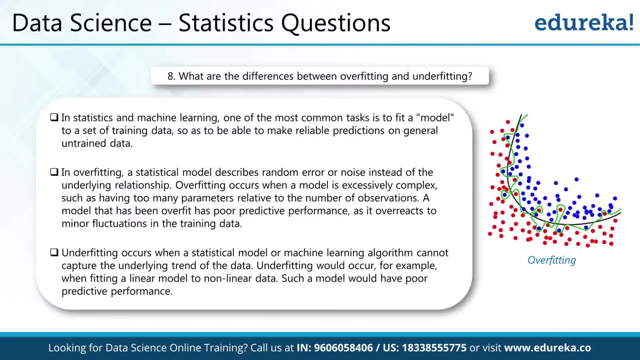 points. So you might want to do a generalization. so for instance here, if I have these red and blue dots here right and if I draw a curve like this which separates the red from the blue, and when this separation happens, I am building actually a classifier using some. 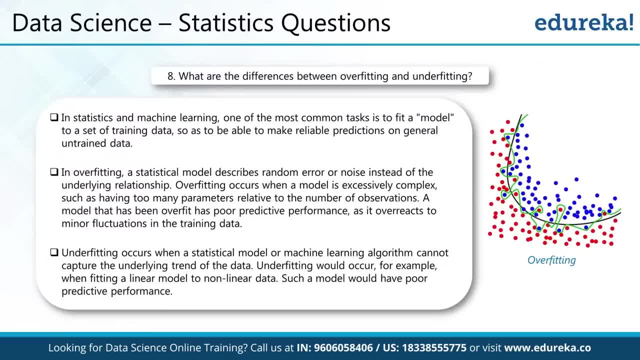 sort of modeling technique. but now imagine, by drawing a smooth curve like the one which is given in black, you might be over generalizing it right, by which I mean There might be some red dots on the other side of this boundary. you can obviously see that, but the moment I am kind of a bit more flexible by drawing this green boundary, which 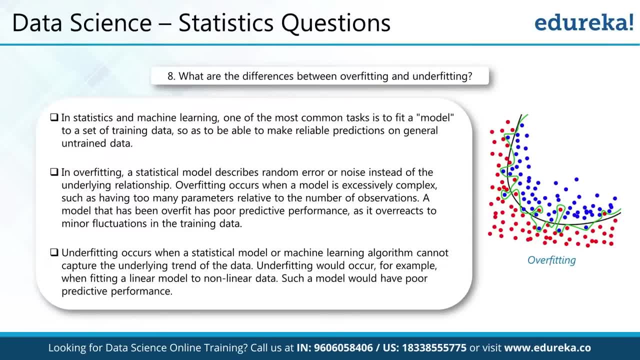 actually covers all that issues which is coming out with these red dots on the other side of the boundary. So this green boundary has, like, taken care of that. but the problem when we are building any model right, The idea is: How do you generalize to the pattern found in the data? 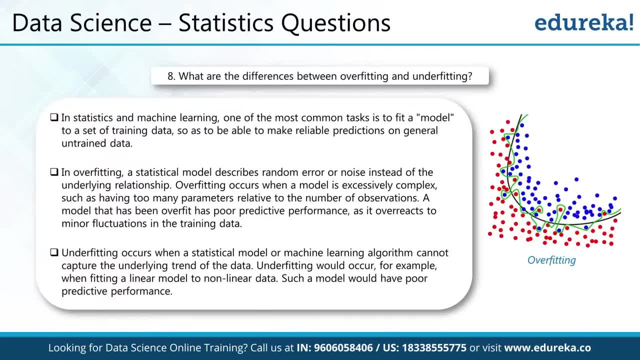 So if you don't do that generalization, well, you are under fitting. but if you do that generalization like too specific, you are over fitting. So this curve might be represented by some polynomial right, but that zigzag kind of a polynomial might be bit more complex than a smooth curve like the one which is shown. 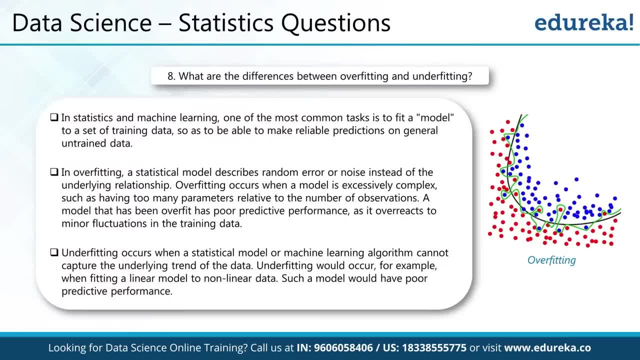 in the black. So you need to be very careful when you are building a model. particularly in the cases of regression models, Where it is represented by a line and a portion, You need to make sure that the polynomial is not so complex at the same time, not so. 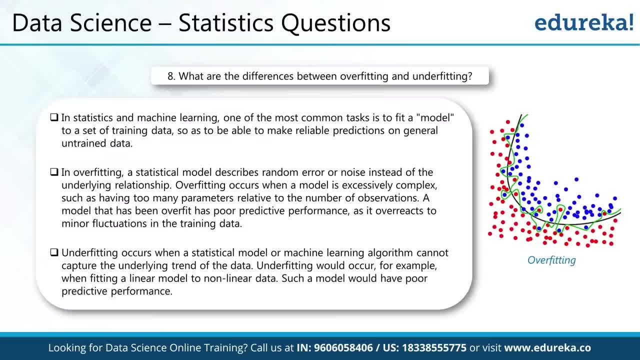 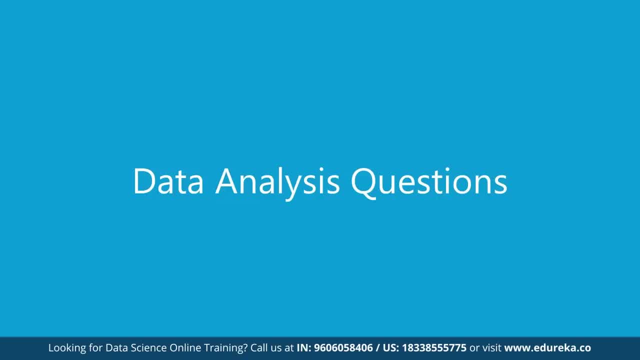 simple, then you will either end up in an over fitting situation versus an under fitting situation, So we need to have a good balance between these two right? So, in summary, when kind of statistical questions comes in, it would mostly covering things like some basic statistical properties as you would be like very aware of, like things like standard. 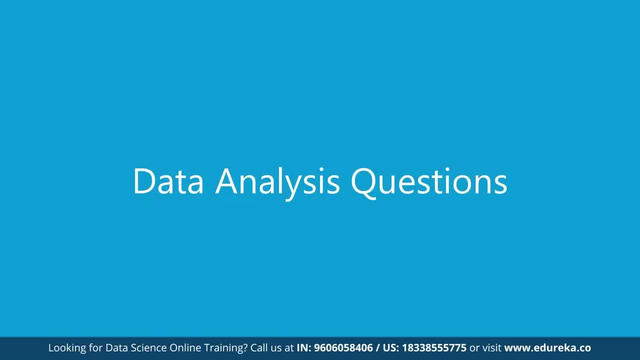 deviation Averages, How to interpret median, How to interpret quartiles right- The first quartile, second quartile and so on. And what do you mean by percentiles right? These are some basic questions. A bit more complex in nature might be discussions around sensitivity, over fitting, under fitting. 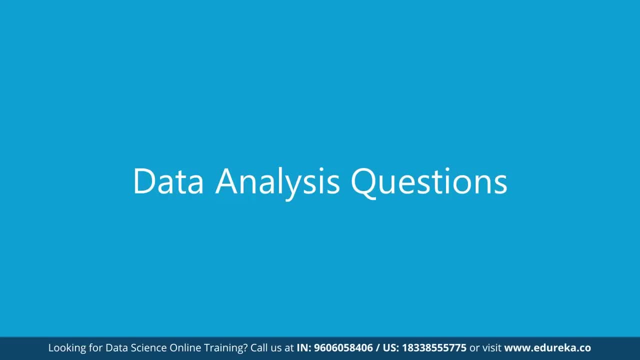 These are like statistical ideas, So you want to prepare, maybe from basics level, using the properties like standard deviation mean and so on, Till things like over fitting, under fitting, standard deviation mean and so on, Till things like over fitting, under fitting, standard deviation mean and so on. 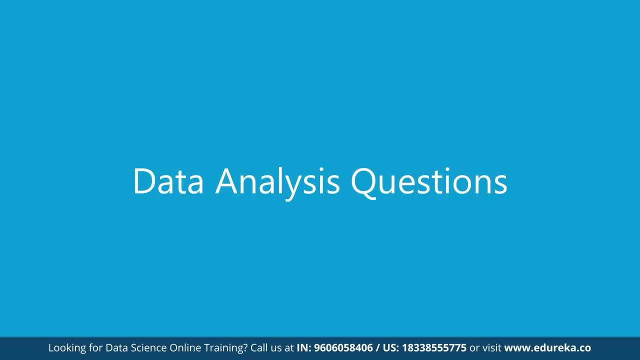 Under fitting statistical desensitivity and specificity kind of ideas. So that will make your crown a bit more stronger when you are going for the interviews then these are atleast the bare minimum for you to understand in the statistical concepts, right. Even anything less than that you might like face some difficulties in the interviews. 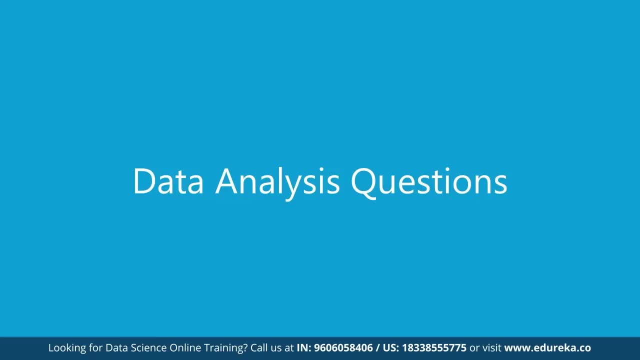 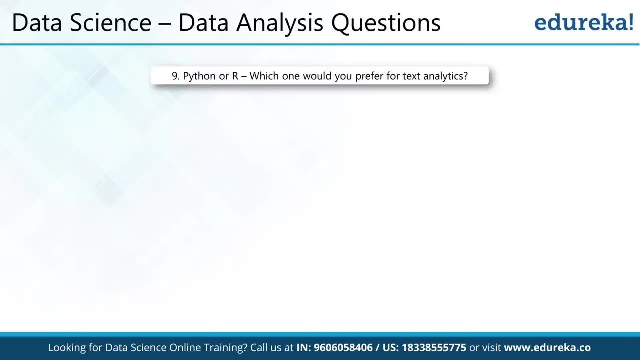 But lets also talk about now questions which are related a bit more on data analysis. So lets see what kind of data analysis questions which might pop up- Fantastic that's will actually. you killed that idea provision or anything like that in the interview. okay, so some generic questions like this. people normally do analysis on structured 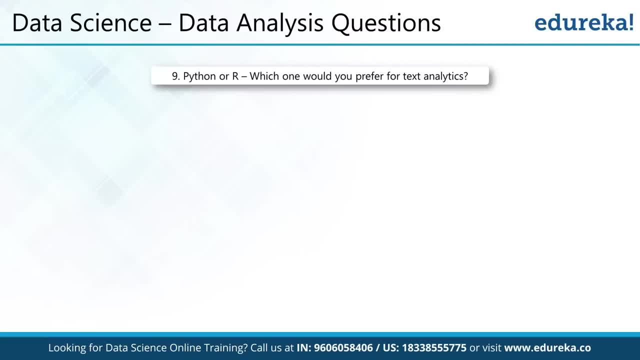 data which is in rows and columns, but there might be cases when the data is not so well structured and those places the data might be textual, for instance in twitter, right, if you're doing any sort of algorithms like sentiment analysis- quite commonly known algorithms- so in that case the 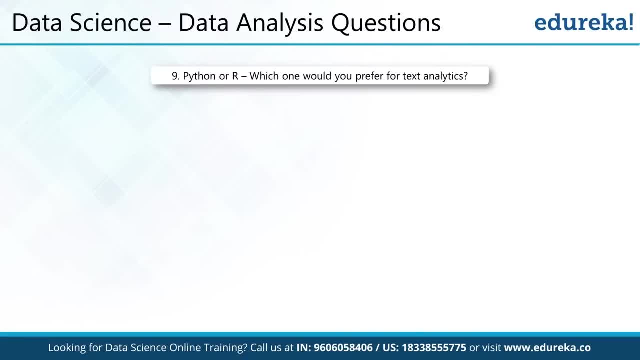 sentiment analysis could be for a brand, for a election campaign or maybe something else around your product features and so on. so text analytics in its own are really large domain, and in python as well as r there are number of libraries, so in particular r has libraries like tm. right the text. 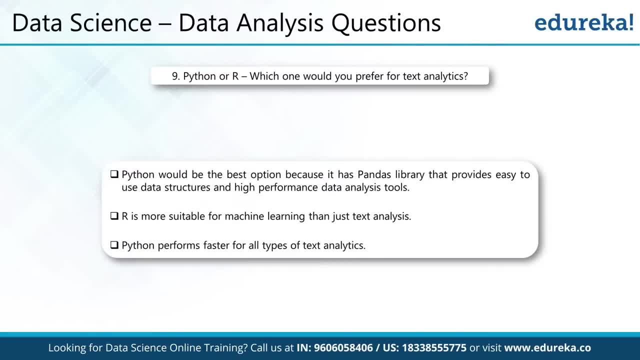 mining package, python as well. we have packages like pandas, packages like the numpy ones right, and also packages like nltk, which is the numpy package, which is the numpy package, which is the build only for a natural language processing so it can deal with many different sort of text. 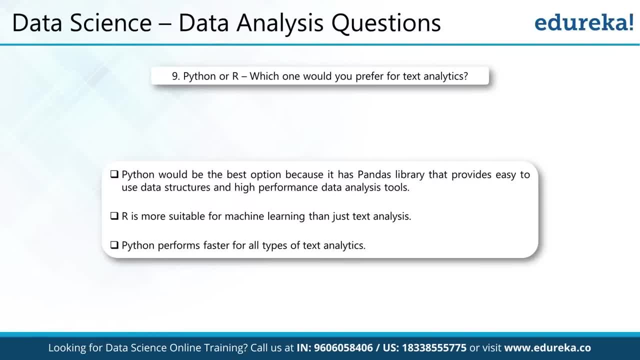 mining approaches or text analytics approaches. so in comparison, if you talk about, as i said, the robustness in python is much more than in r, but in terms of features both are powerful enough with the libraries and packages that it offers. right, one of the fundamental sort of starting. 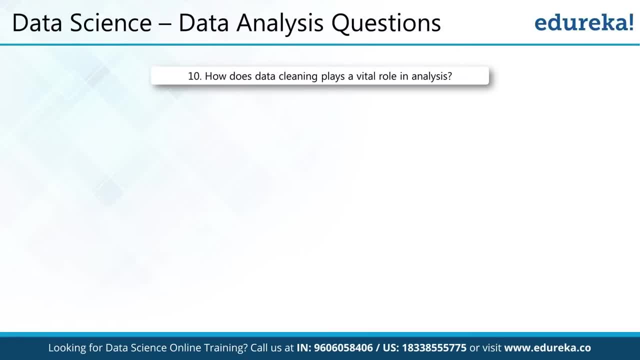 place when you do any analysis. so when you are given a data set and you are asked to do some sort of basic analysis of what that data tells you, maybe typically, you are given a data set and you are asked to do some sort of basic analysis of what that data tells you, maybe typically, 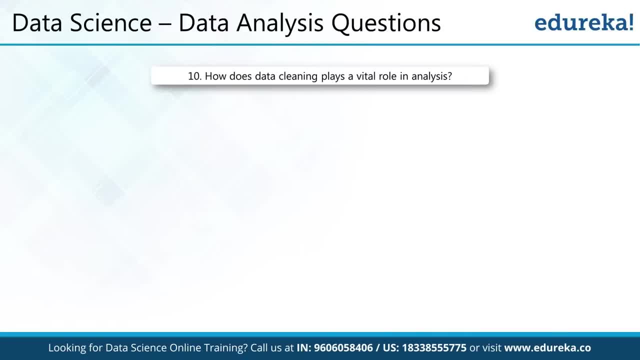 you are given a data set and you are asked to do some sort of basic analysis of what that data tells you, maybe typically of questions like: i am a retail business and my sales in a particular region is going down, so this is an analysis that is affected out of you and you need to dig through in understanding what. 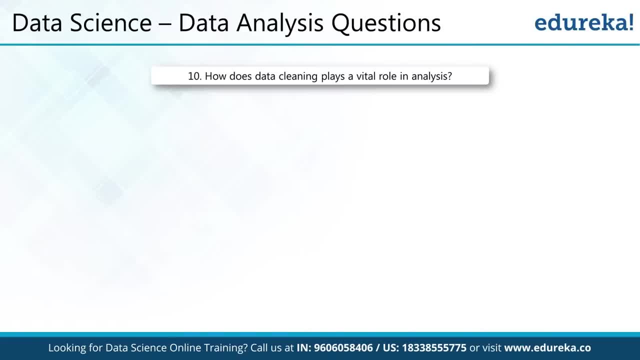 really is the problem in the sales going down. so if this is sort of the data, this, which is given to you, you might want to first look at the transactional data which is present in the system. then you might also want to go to outside of your network. maybe you might get the sentiments of your customers. 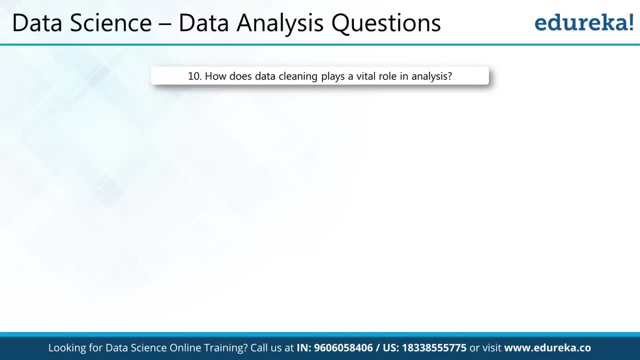 from social media platforms and so on. so there will be different sources of data that you will collect, but often times collecting the data is not only the task. and but often times collecting the data is not only the task- right, and not like only building a model or 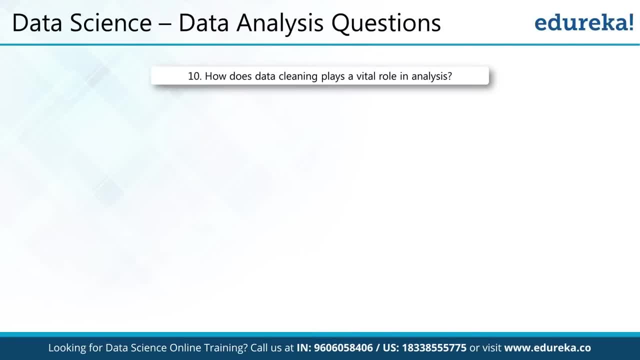 doing statistical analysis might like come very later in the stage, but what comes before that, after you have collected the data, is to make sure that the integrity of the data is maintained. you get rid of all the unwanted noise from the data and then finally prepare the data for doing the. 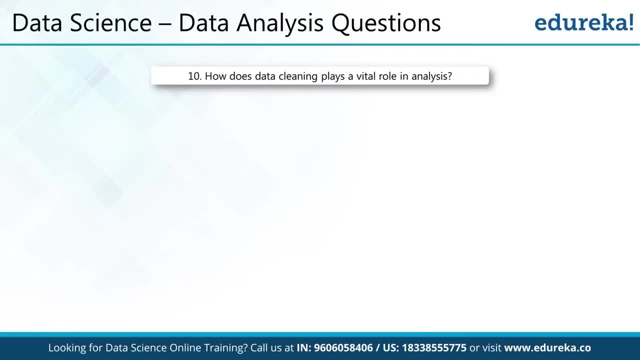 sort of modeling exercise or doing descriptive analytics on top of it. so this cleaning, cleaning and understanding the data, doing a lot of explorations with plot in essence takes close to 70 to 80 percent of your time in any data analysis task. so if your company maintains the data in a very 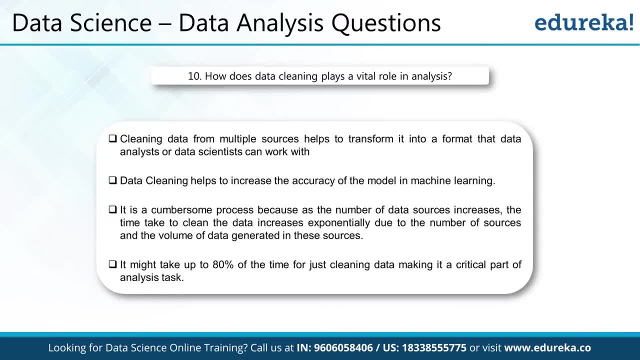 well structured way, this kind of heavy time which we spend on data analysis might be ready or the data cleaning might be reduced. otherwise, you need to like take this up for any new project that you take up which for which the data is not available in prior or you don't. 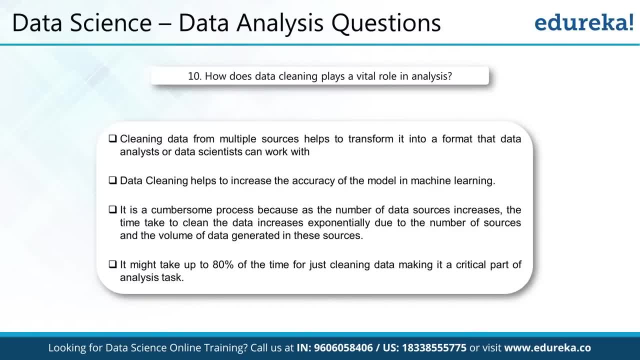 have, like any pipeline, which do this cleaning. you have to write it down of your own. so very, very important. if you don't do the cleaning part and understanding the data well, the analysis or the models that you build might end up giving you a very, very bad performance right. 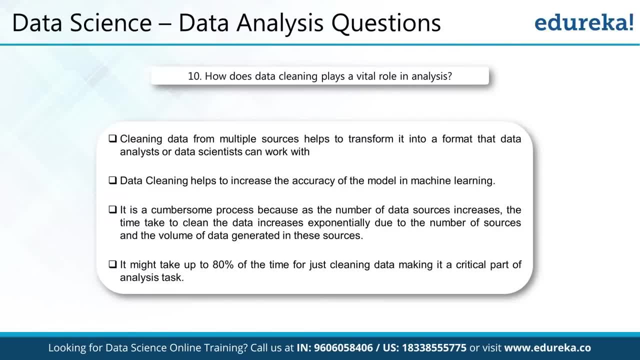 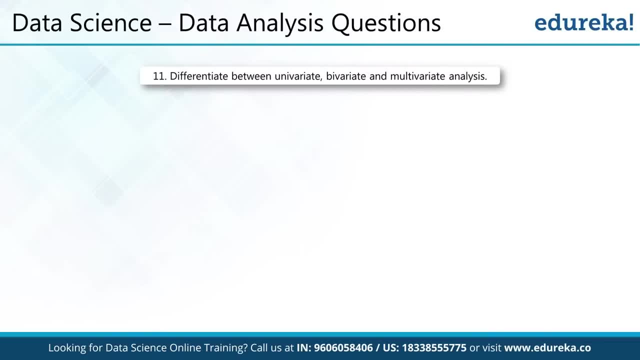 so very important. as I said, 80% of the time people normally spend on this task right, and often times When you are analyzing things like the example I told my sales are going down. what do I do? it is not possible to come out with such answers to complex problems like this with just one. 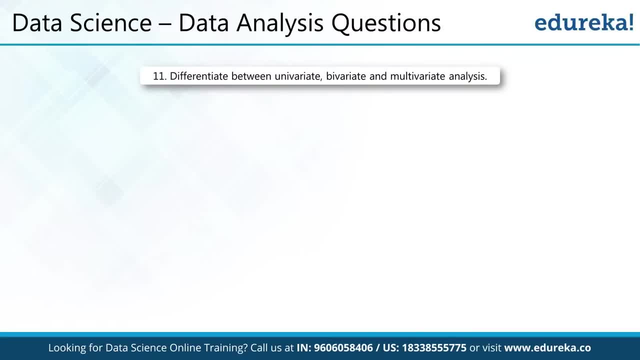 variable right. so you might also want sometimes to move beyond one variable and talk about, let's say, how to do multivariate or bivariate kind of analysis. so often times this question comes up where you like ask to distinguish between this univariate, bivariate and multivariate. 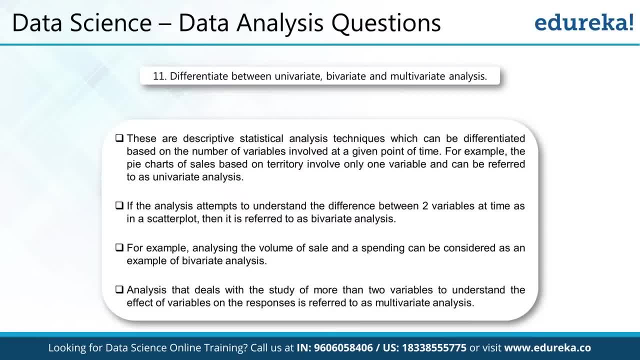 bivariate analysis, and the idea is very simple: in any sort of analysis it is not only one variable which kind of decides the end output of your analysis, but there are multiple factors involved. so when there are multiple factors involved, you might also want to look at things. 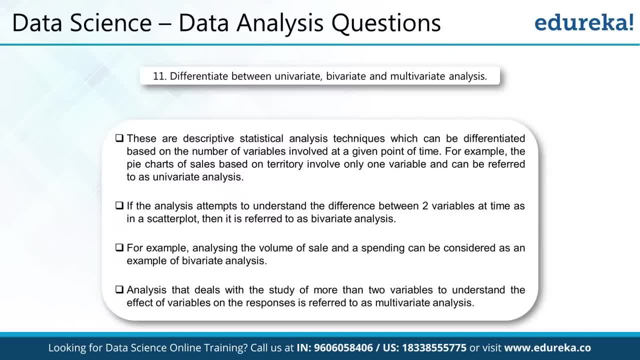 like correlation. there are multiple variables. you want to see if there is any correlation between these things. sales are going down, but because of what? is it because my sales representatives are not going to the market, or is it my products are bad, Or is there some other reasons? so with all the variables in one place, you might want. 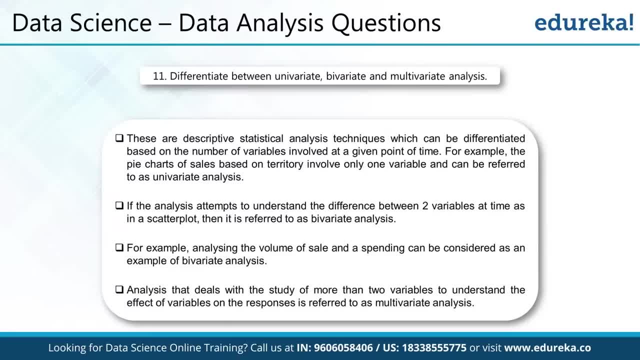 to go and dig deeper to see if there is any relationships coming in the variables or not. and when we collectively get all these variables together and do some sort of coherent analysis around the problem, you come out with a really crisp answers to what you are trying to analyze. 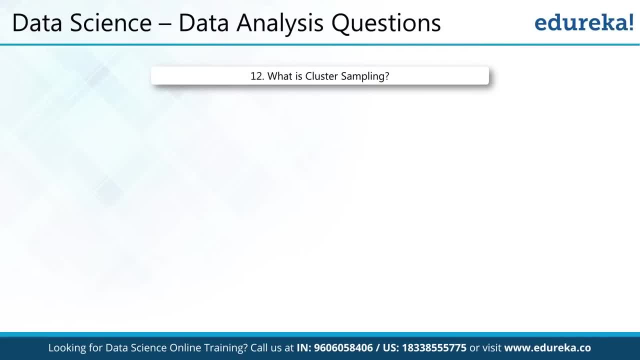 right and moving on. there is also times when people do some sort of grouping right with the data. You do a sampling right, you get a data set in your system or in whichever servers you are doing the analysis. but in that there might be lot, many number of times when even the 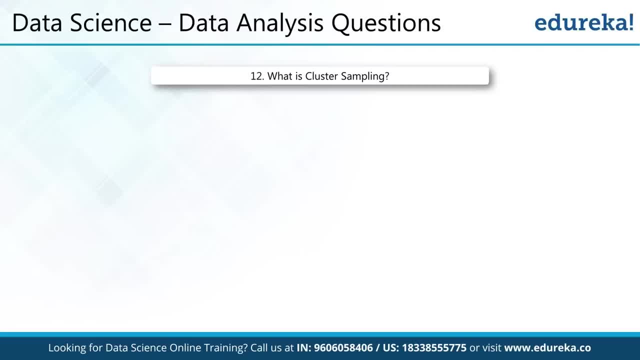 randomized sampling of getting the true representative from the population like that might not work well, right? so in those cases you might want to do some sort of systematic sampling, or maybe a cluster based sampling as well, wherein you might decide to say: I want to analyze the issue with only five regions. 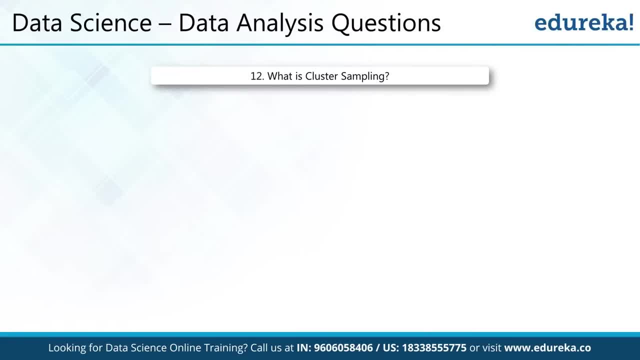 In my mind and with the five regions I'm going to form different clusters or in the systematic sampling. you might also want to say that with the five regions that I have got, I might want to analyze only for one product right which is not doing that good in the sales. so these 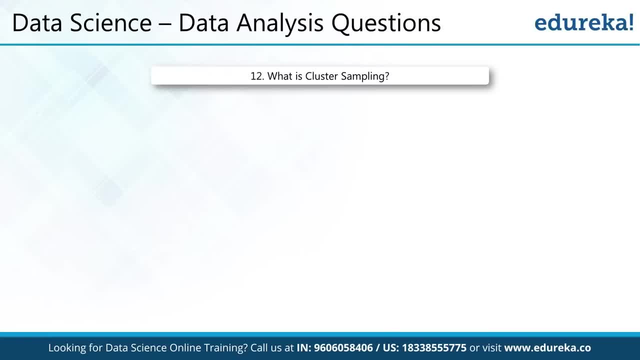 kind of sampling techniques like the cluster based one or the systematic sampling techniques- and there are different names for this- people might be able to give a very good interpretation of what really went wrong, In whichever sort of analysis you are doing. so one example is like sales going down, but 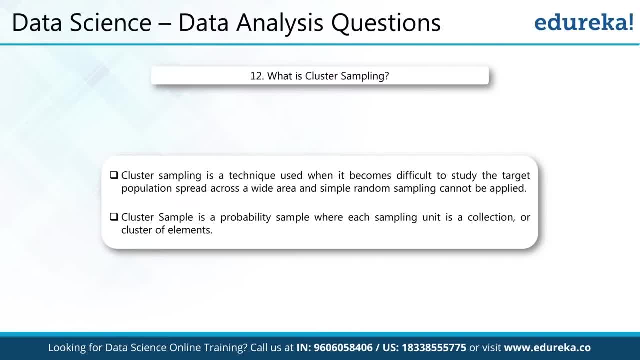 you can adapt this to other analysis as well, but the idea is, instead of doing a randomized sampling, by which we are not very sure which kind of data is coming in the data set you want to use for analysis, but if you did a cluster based, cluster systematic sampling- 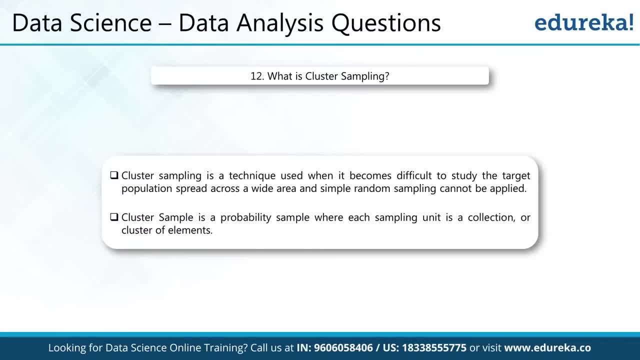 you know exactly which cluster, which sort of regions in this example. you are like analyzing and in the end of the analysis you will be very able to say this is not like a randomized sample that I have taken, but from these five regions. so there are many different ways of 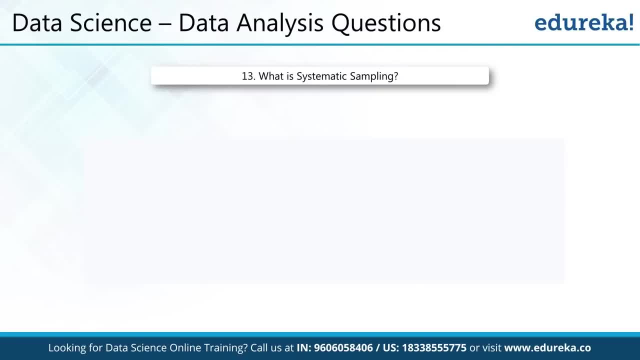 doing clustering, Cluster or sort of the systematic sampling which kind of helps in this particular final end results of your, and I will to put your end results in the right perspectives, right, instead of doing a randomized sampling. okay, one more, quite a useful sort of an idea kind. 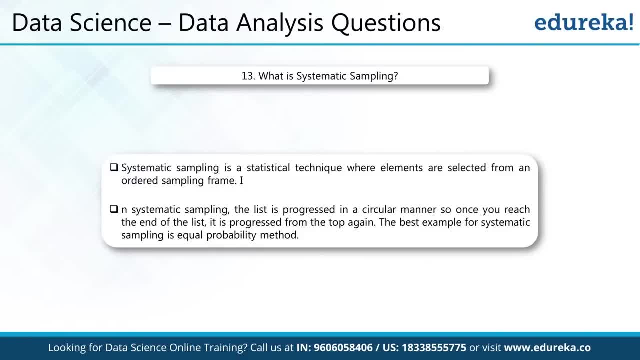 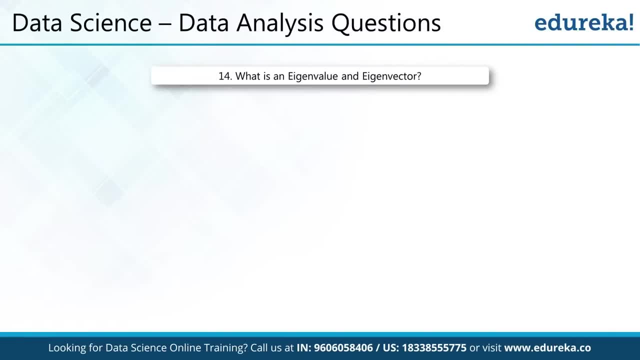 of related to what we earlier saw between moving from one variable to multiple variables- right and Egan value and Egan vectors, kind of a concept borrowed from linear algebra- helps us To bring in some in some way a linear combination of different variables together, for instance, 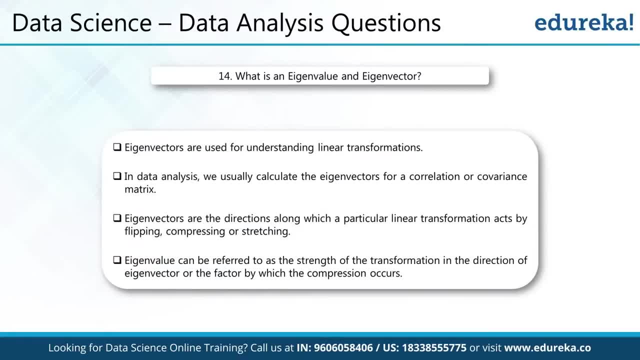 in some complex analysis it might happen so that, given a data set, it might have many columns, right? let's assume you have a data set with 1 million rows and let's assume 10,000 columns, so, and these 10,000 columns are some features. there are complex problems like that, but in 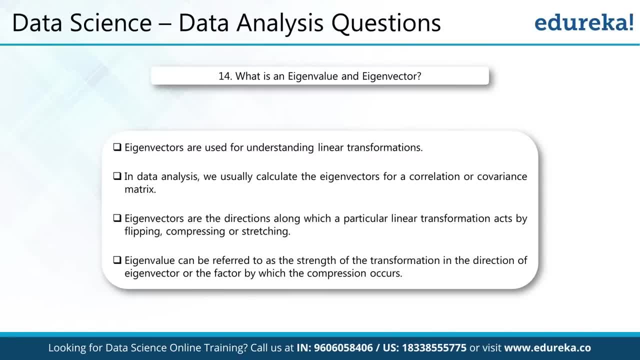 most often, like most of the time, Not all the 10,000 variables Are useful, right, the input variables. so what we can do is we might want to transform this data set in a lower dimensional space, by which we mean this: 10,000 columns can be reduced. 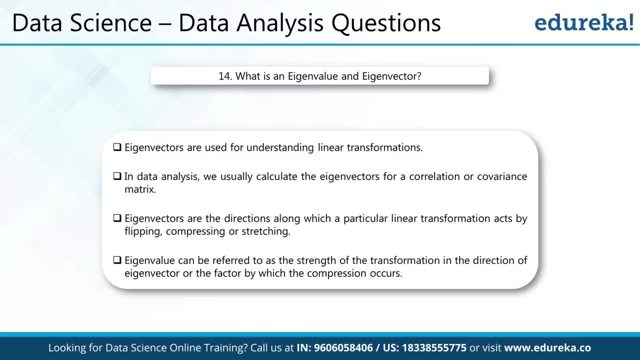 to, let's say, only 100 columns, right? so Egan value and Egan vectors, are these ideas which helps us in this transformation? and the idea is, can this hundred variables be represented as some sort of linear combinations of the 10,000 variables? and if I am able to do that, 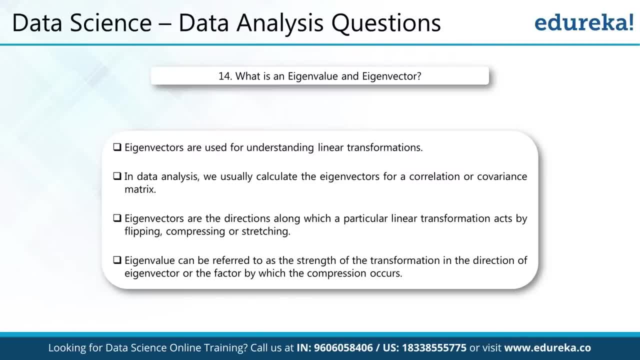 my dimensionality is reduced, the time I take to do the analysis is kind of also reduced and the representability, which will come with only 100 variables, will go up right. so quite a powerful idea. Egan values and the Egan vectors. and, as I said, the Egan vectors is kind of. 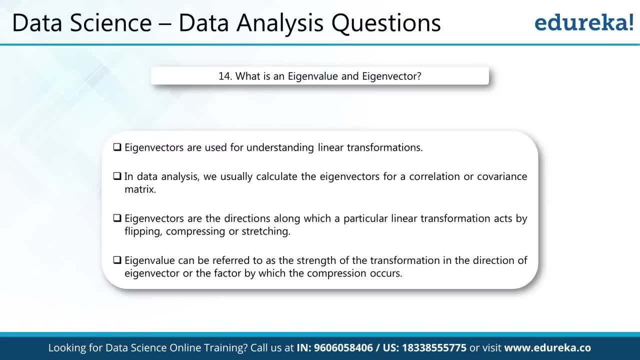 that linear combinations of many kind of variables there and this calculations around Egan vectors, normally happens For A correlation or a covariance kind of a matrix which, as you know, the measure. correlation is also about how to two variables are related or how strongly two variables are correlated. 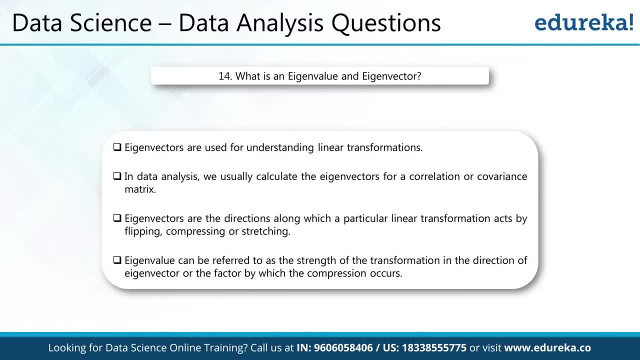 right, so that's why we are also saying this: Egan vectors can help us to compress the sort of data that we have, right, and that's because of one Egan vector can be representing a hundred column, a hundred variables together, right? so that's sort of how it works. so quite a. 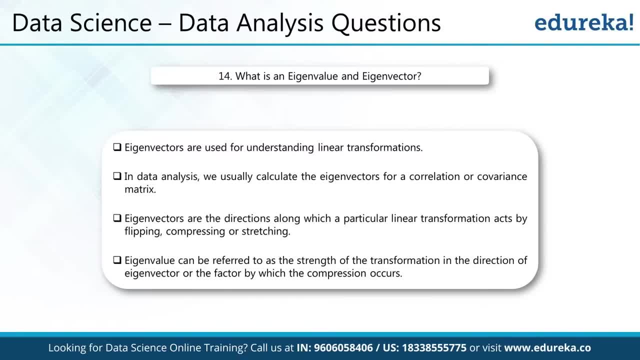 powerful idea and commonly used methods For reducing the dimensions of an enlarged data set like the PCA, a principal component. analysis is actually based on like in value and eigenvectors. so if somebody asks you about eigenvalue and eigenvectors in an interview, also talk about the PCA, principal component. 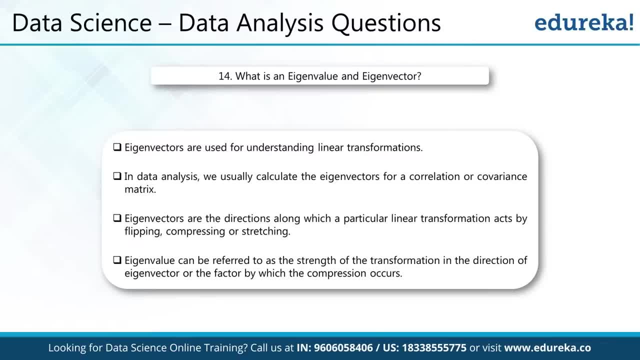 analysis which is actually based on these two concepts. so that gives them a good idea to the interview view. you let you know about the eigenvalues and eigenvectors and you are also able to think of its application, like in PCA right. So we talked about this false positive and the false negative cases in our confusion. 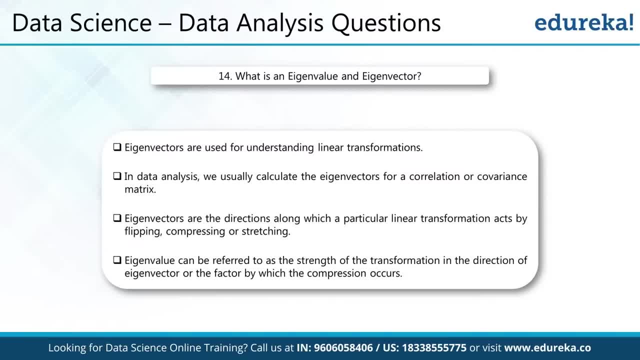 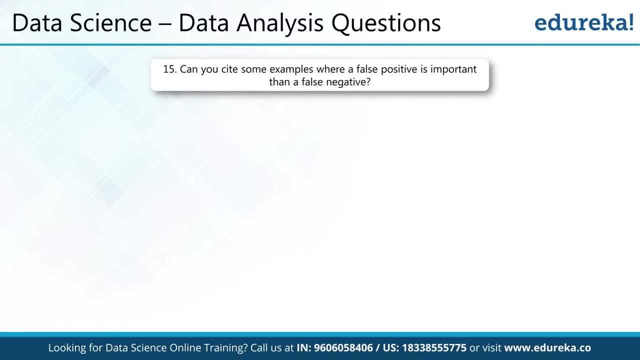 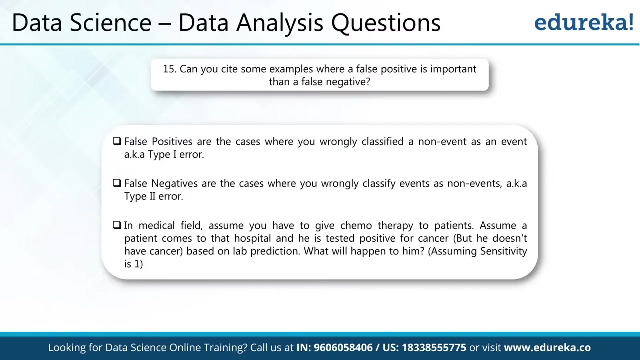 matrix example. so this is exactly the same. you also talked about the type 1 and type 2 error. okay so, but let's now also drill further and say examples or kind of scenario when the false positives are important, in scenarios where the false negatives are sort. 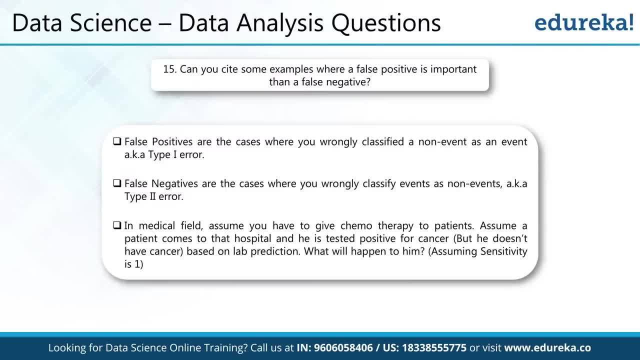 of important and the. by the term importance we mean: are we like allowed to do this mistake? if you are building a machine learning model, are we even allowed to do a mistake on either of the cases, the positive or the negatives? so for instance, here, if I take an example, 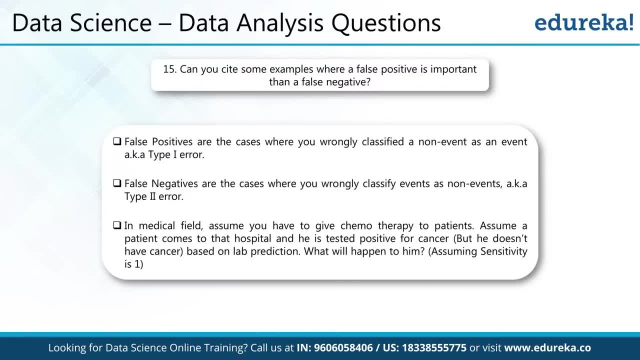 in a medical domain Where we have, let's say, a process called chemotherapy which is normally given to cancer patients, which is a radio active kind of a therapy which kills the cancerous cells. right, so it is very focused sort of a therapy on the cancerous cells. so what will happen if? 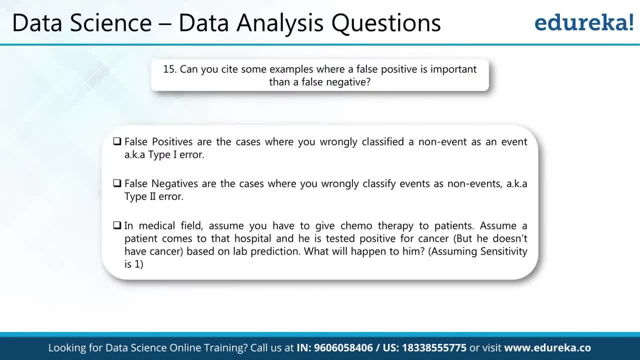 you like, predict. let's say you are building a model for detecting cancers, right given a CT image, And this model would obviously not be 100% accurate. So let's say you are building a model for detecting cancers, right given a CT image, and the average treating rate is 100%. 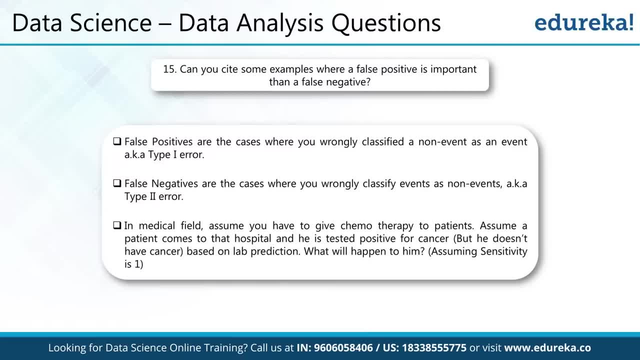 Say my person correct, I she learning model has its limitations, but you are here required to predict this: whether a patient has cancer or not, and based on that, radiologist might decide that whether the chemotherapy is right for this patient or not. But imagine now if you have predicted somebody to be positive for cancer, but the patient 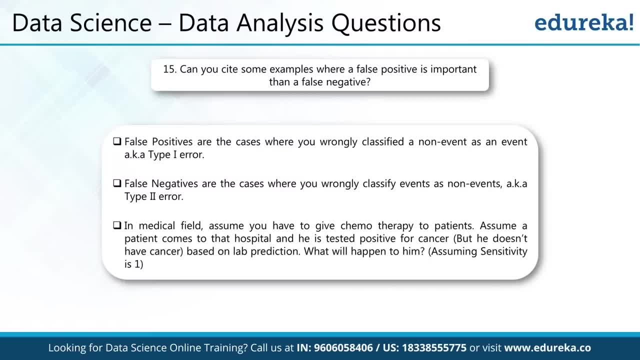 is actually not having the cancer there, right? so in those cases you might end up saying let's go ahead with the chemotherapy. but the side effects of chemotherapy are like very, very adverse right, because you are giving these therapies on the healthy cells if the patient is not having the cancers. so in these 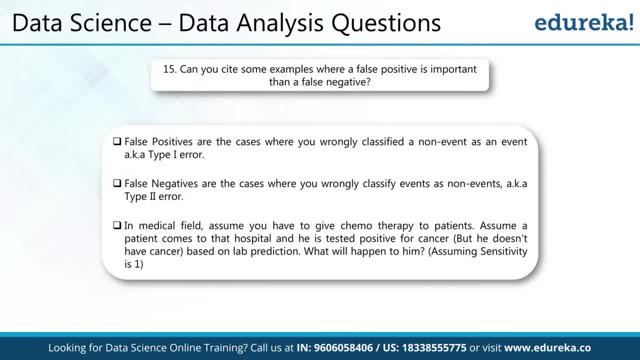 cases, sort of the false positives, becomes a bit more important. so it will be absolutely fine if your model says the patient doesn't have cancer, if even if there is, like this, slight possibility of cancer present in the cells of the patients, but in that case you are not like. 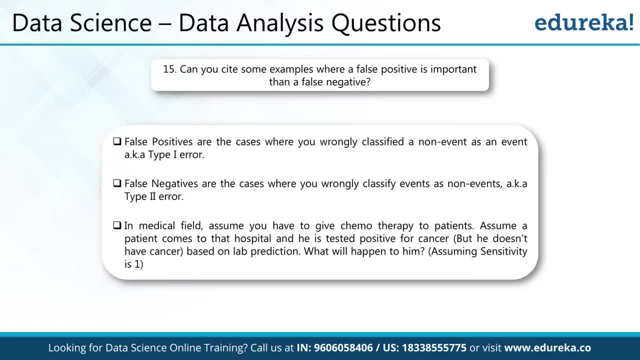 exposing the patient with a chemotherapy there, right, which is like more harmful than saying that the patient doesn't have the cancer, right? so in these cases, the false negative- though the false negative itself is not so good in this case, but at least with this particular example, the false positive gets the importance than the false negative, but both are bad, as you know, right. 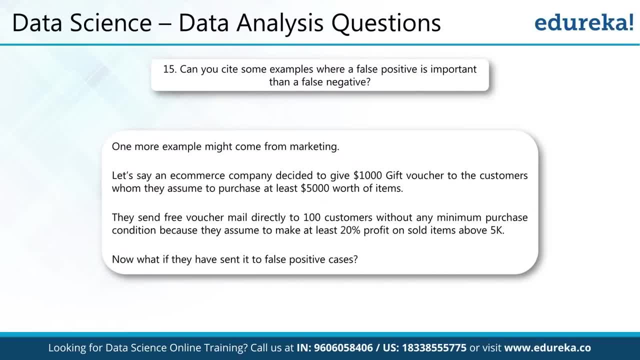 from the confusion matrix discussions. so in simple terms, it is better to not expose the patient with a false positive with a treatment like this, chemotherapy like treatment you. then it is like much better than saying you don't have cancers. okay. and a very similar example in some other context might also come up. so if you would like to think of some other examples in the 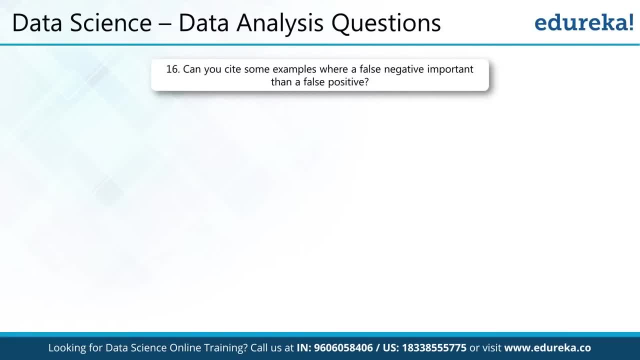 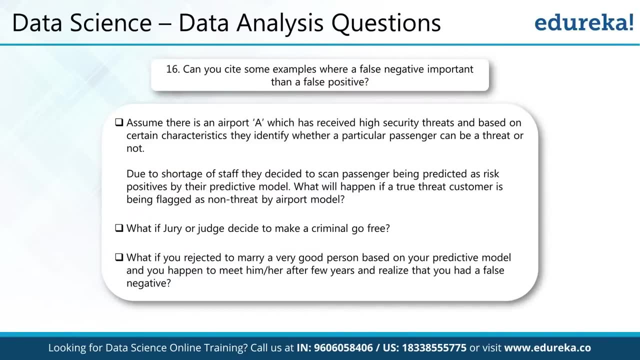 same context. okay, so where is the other case now, which is the false negative? right? so we talked about the false positives importance, but there might be also cases where false negative might become a bit more important there, and for examples like this: if you are, let's say, building a model, 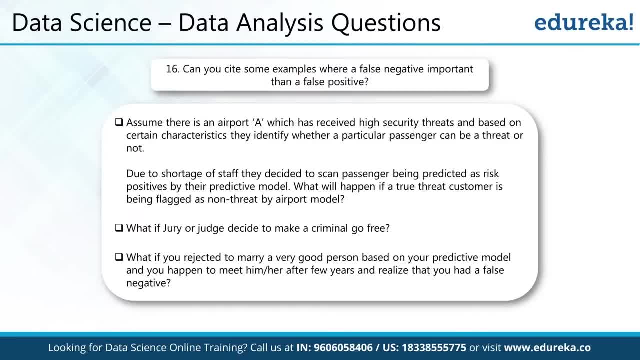 where you want to convict a particular criminal basis, all the records and the arguments which has happened in the court. right, and let's see what would happen if you make a criminal go free. right, because your model says it's false, negative, the, though the person is actually a criminal, but because your model 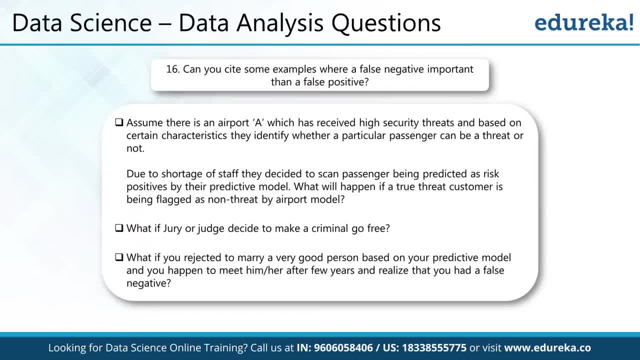 predicted. based on all the evidences you had, the person is not a criminal. so you are letting a criminal like walk free in society. so that kind of is more harmful than convicting that person, and maybe for a prolonged period of time you might also want to get more evidences and build a stronger case. so 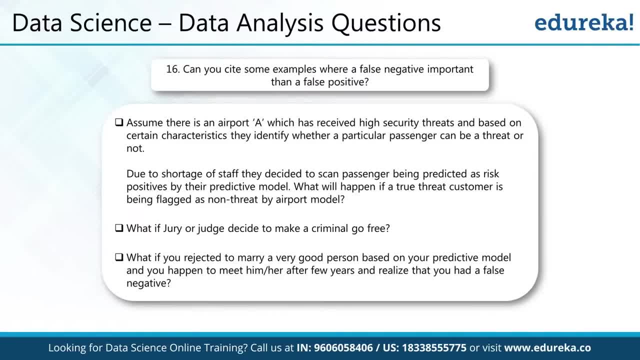 it is fine to keep a suspect in behind the bars for a longer period, then letting the suspect go free there when we like. know that there it might be a case of a criminal going free from the judicial systems there, right? so in these cases the other case becomes more important. so keep in mind, it is very 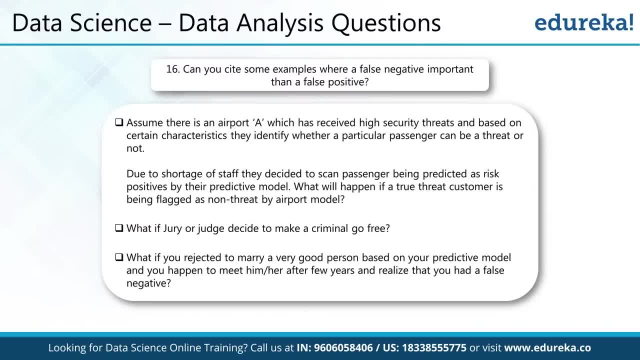 easy to get yourself confused between this false, negative and positive. but if you keep an example in mind, always and like don't give any room for confusion, there, though it is, a confusion matrix will be based on which these two ideas comes in. you will be able, at every time, put these examples in front and talk from that. so if you start, 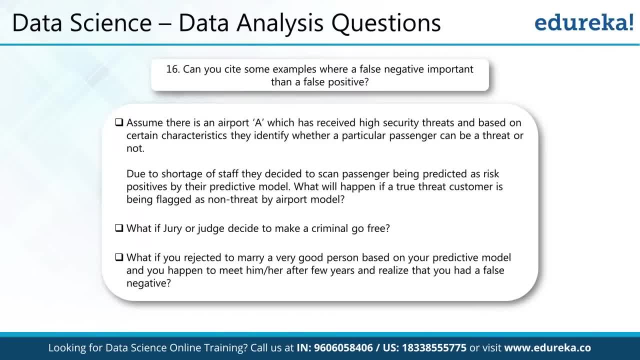 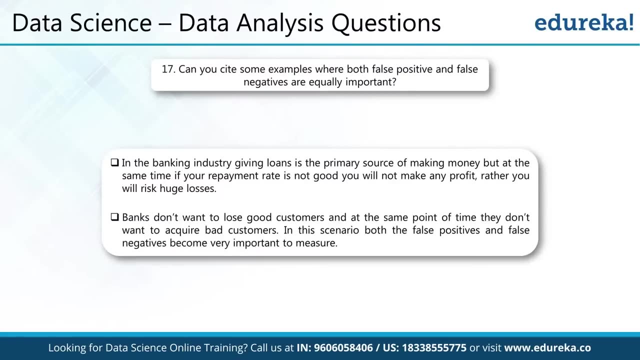 to explain what false negative is in terms of the formula, you might get confused, but if you take an example and then explain, things are much more clear for you as well as the person who is hearing that in the interview. right, and in cases when both are important, typically the one which relates to 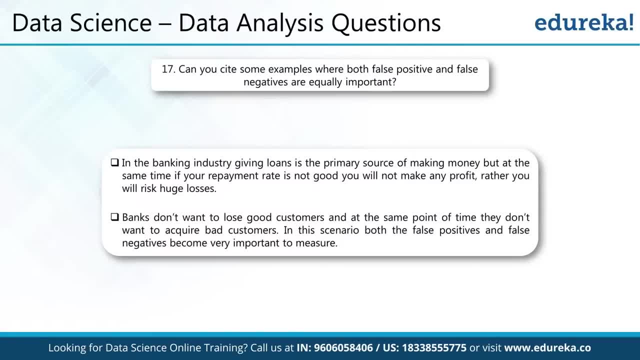 you banking industry, you are building up a model which will decide whether to give a loan to a person or not, basis many of the input attributes, that around which you have like collected the application from the customer. but here you say, if the customer is really good and you are missing the opportunity there of not. 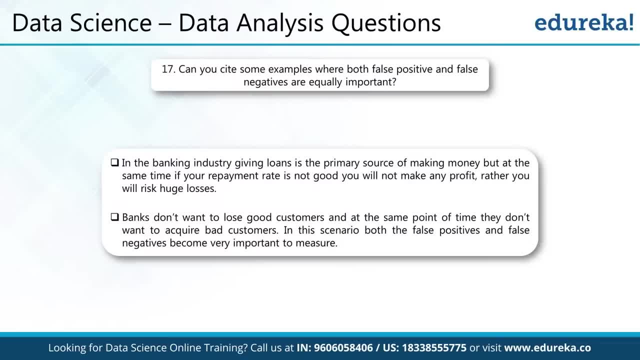 giving the loan versus the customer is really bad in terms of its, his or her credit history, and you are giving the loan in both the cases. in one case, you are losing the business. in the other cases, you are taking a risk in which you will lose your money right. so in this case and in 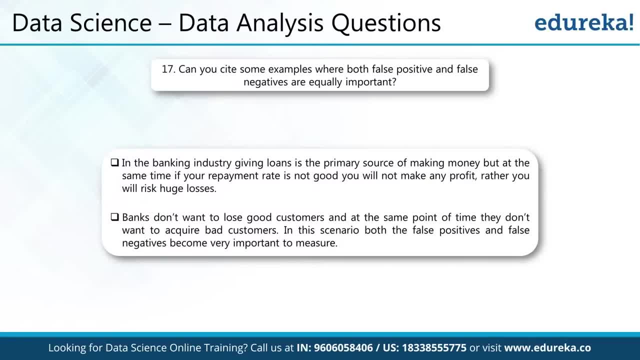 this example. both kind of has an equal role. so if you are positive or false negatives are in, either of this is high. you will end up losing some chunk of your money there. keep these three examples in mind and every time you get to like here, false positive, false negatives- things should not be like. 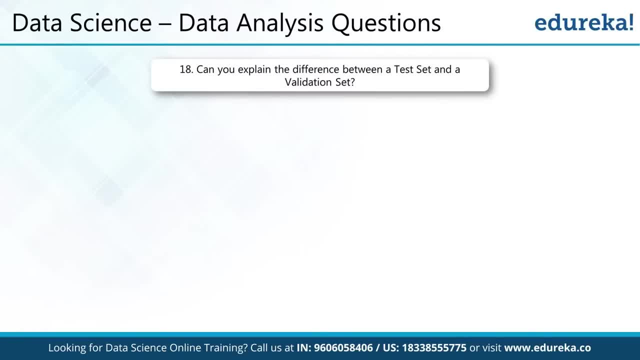 confusing at all. okay, so now let's also talk about building a machine learning model. so so far we have discussed about what happens after building the model. but let's step one, like get one step back and see how do we normally build a machine learning model and what kind of processes we normally follow. so when we 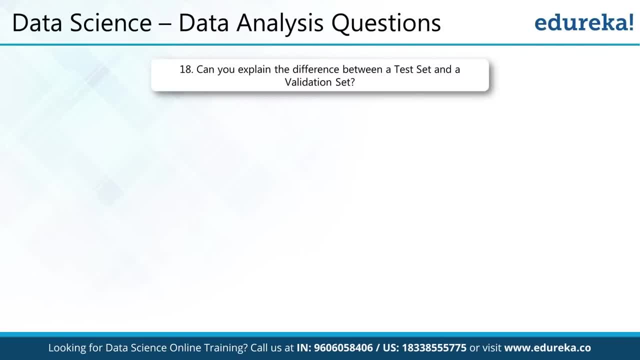 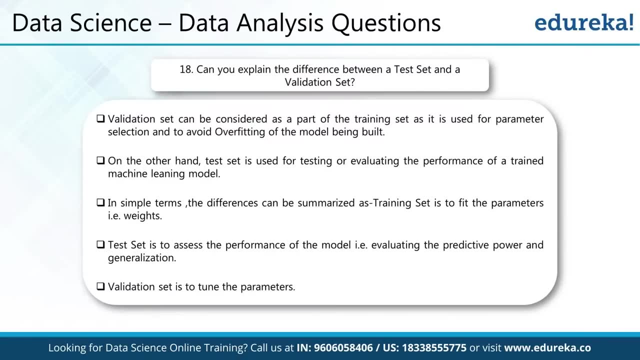 are like building a machine learning model. we know that we need to. given a data set, we need to divide it into different buckets or different parts. so the commonly known divisions that we like have is your training data, right then. we also divide the data into something called test data, and sometimes 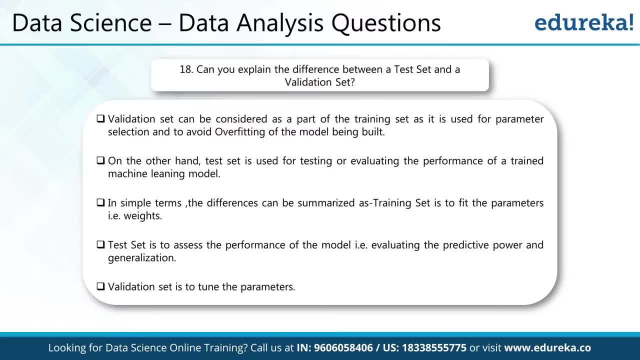 we will also divide the or keep one portion of your large data set, which is called the validation data. so oftentimes people confuse between the test data and the validation data, right? so what happens is in the training process. there are certain models wherein, while you are training, you will use the training data, obviously, but in the 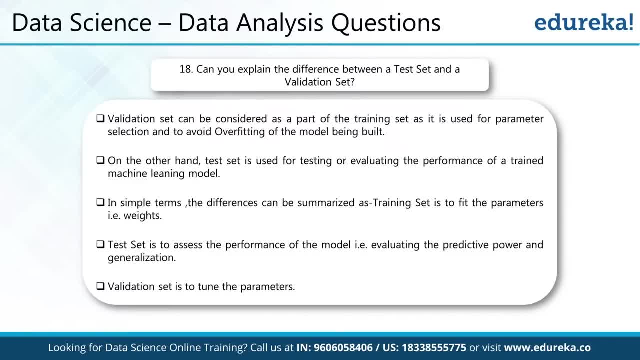 process of training. you can also involve something like a validation step right which will make sure that during the process there is one part dedicatedly given for the validation of the model, which is called the validation step model, and when the model is done, you might see that the final model is well. 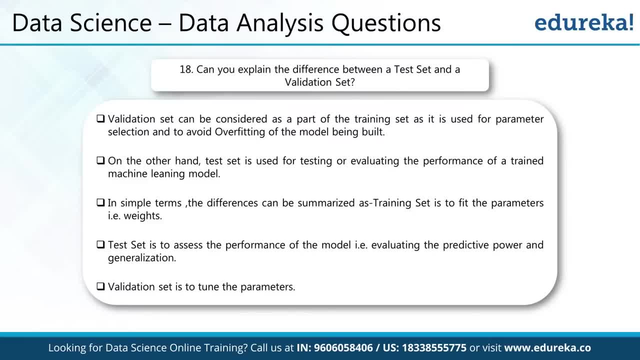 trained on the data, at the same time validated. but when the model is completely done, then only you get into a process that we call testing, right? so you can imagine like this: you have a data of thousand records. you keep some seven hundred records for training, hundred record for validation and the 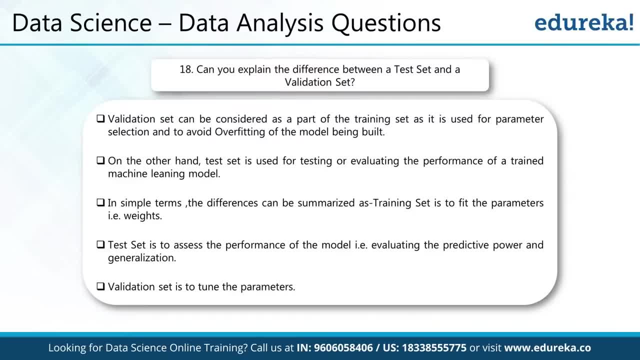 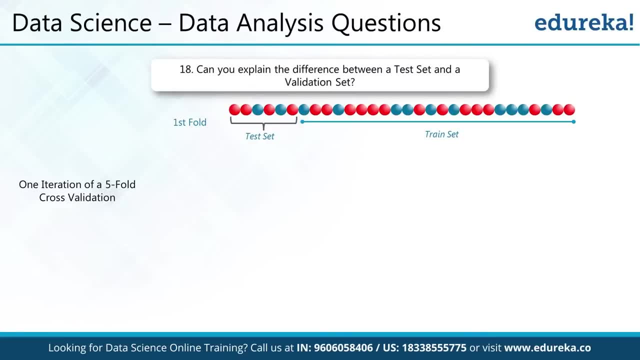 remaining two hundred records for testing. so there are three splits, right? if I would like to explain this with an example, this is how it will happen. so there is a process called k-fold cross-validation in which k can be any number like between five and ten. mostly there are like standards saying five fold cross. 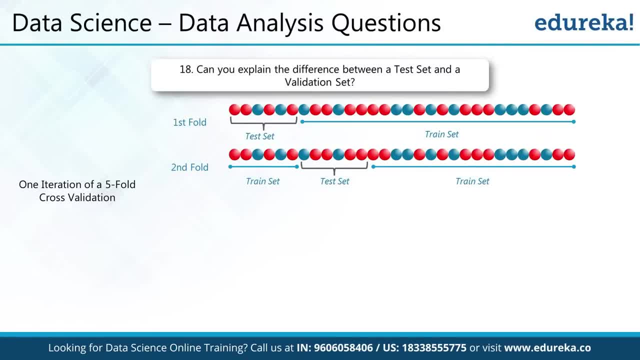 validation or ten fold cross validation, and the idea is, when you are building your model, you will work with a training set right and a validation set in which a small portion of the data you keep for validation and the rest you use for training. so what you see here- test set- can be like replaced with a validation. 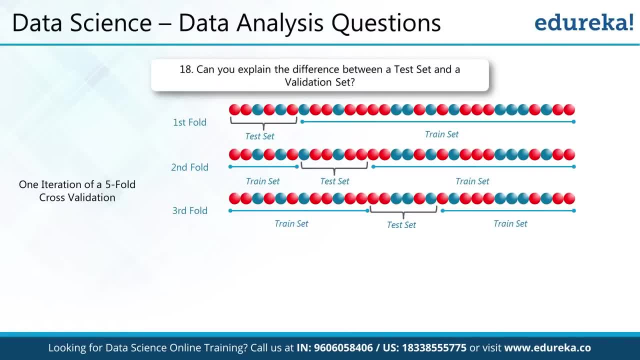 set right and you can see that this is a rolling sort of subset and you keep changing it in each fold. so you go for the first fold of the iteration. you keep one validation set and the rest of it is the training set and the next fold you. 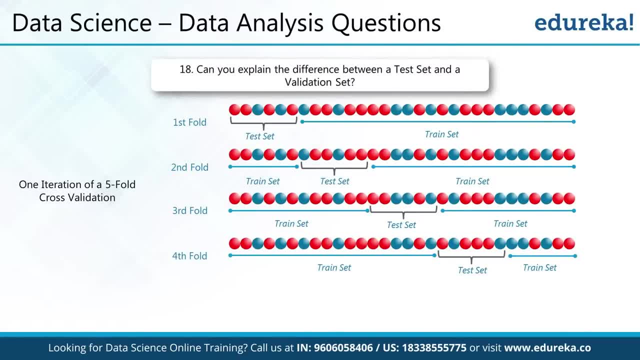 move this window to another subset and the rest is training data and so on. and when this model is done, using this k-fold cross-validation approach, in the end you will get a model which you can then use on the testing data to see if the accuracies are good or not. so this kind 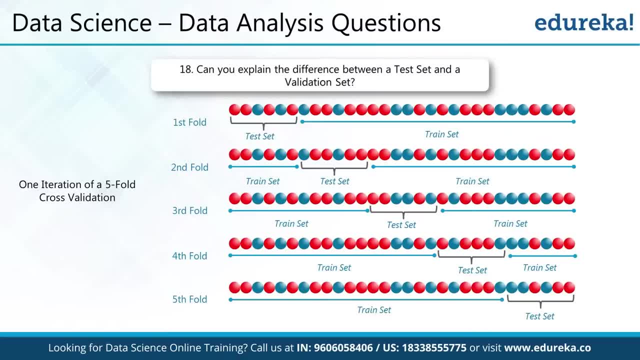 of brings in a lot of performance improvements. people have also found validation set to be an really good way of tuning the parameters in many machine learning models. as you might know, there are something called parameters, typically in the neural network models, and these parameters need to be tuned as the model is a kind of proceeding, so we cannot use the testing. 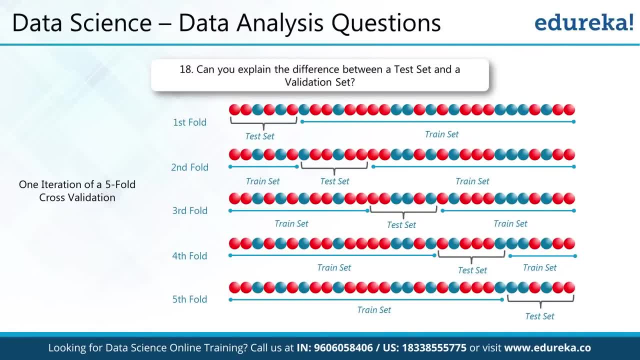 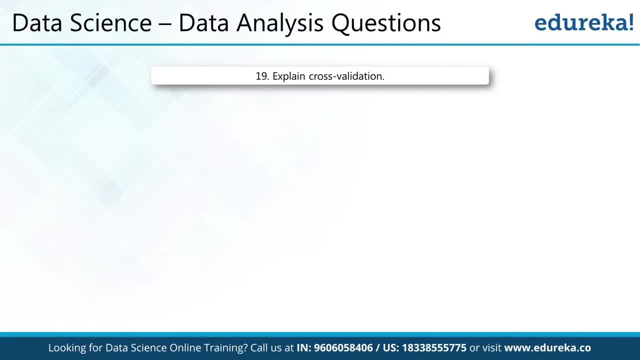 data set for tuning this parameter. so validation set kind of comes very handy in those cases, right? so we just talked about the cross validation. so when you keep moving this validation set in each of the fold- first fold, second fold, third fold- and the validation set is keep changing, you kind of do this process of 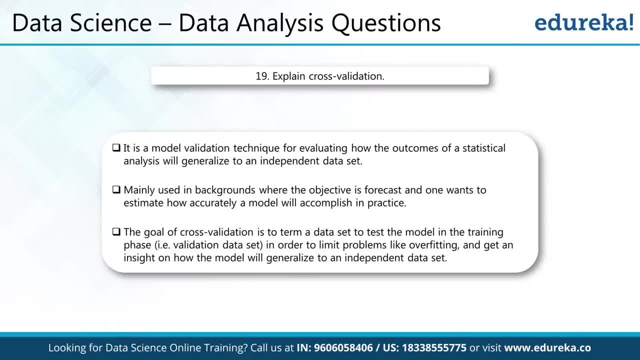 cross validation right, and the idea behind doing cross validation is is to see how well is your final model generalizes to the data that you have. so, independent of which data you use for training, your model should generalize because oftentimes it happens when you train your machine learning model it 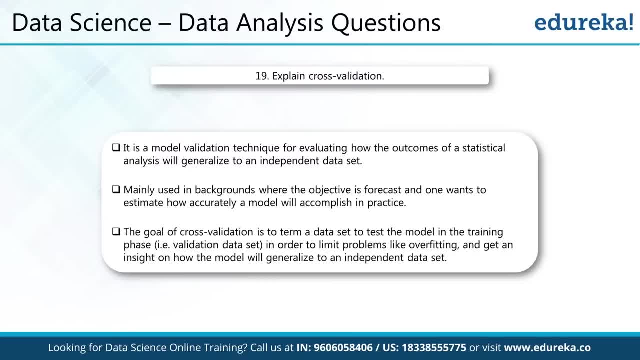 works very good in the training part, but when it comes to the testing the model does very bad. the same problem with the overfitting and the under fitting cases. so in this approach of cross validation you have made sure that your tray model has trained on various subsets of the data right and in the process we also 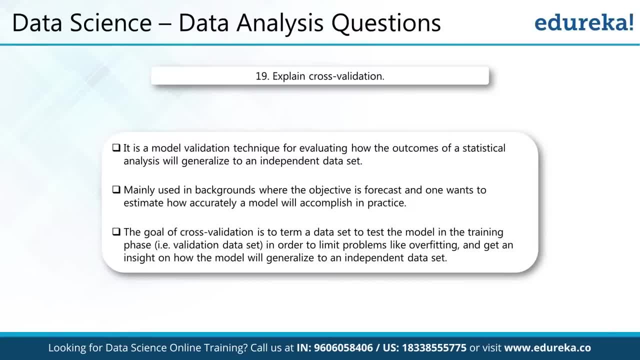 have this small validation set so that every stage of the cross validation process you are able to use a different subset. so that means you have to have a means. you have trained your model very well so irrespective of which data you use, your model is going to do well in the testing cases. so that's how cross 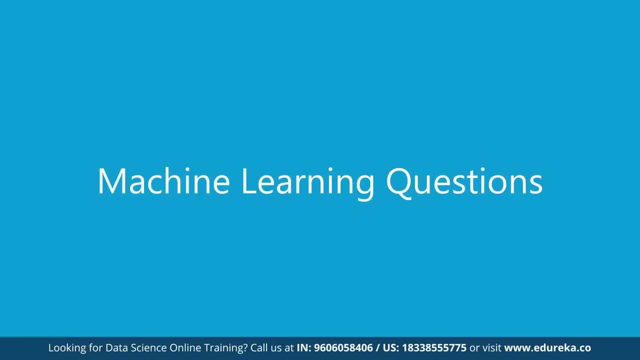 validation brings in the capabilities. okay, so with the two pillars, like the statistical analysis and the basic data analysis, I hope you are getting some sense of how people ask a particular question, coming from either the model building perspective or from normal data analysis perspective. right, so we're. 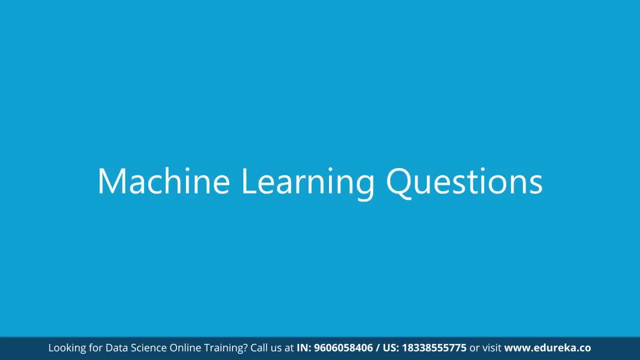 going to know now go a bit more deeper into questions which might relate directly to machine learning. so these are all. the most questions that you have seen so far are either saying how do we do analysis after the model is built or how do we normally perform simple data analysis like a be testing frameworks. 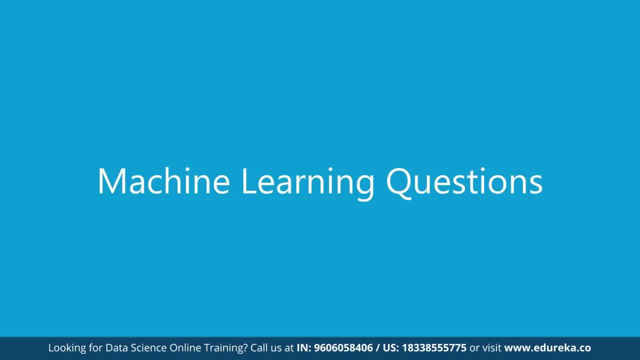 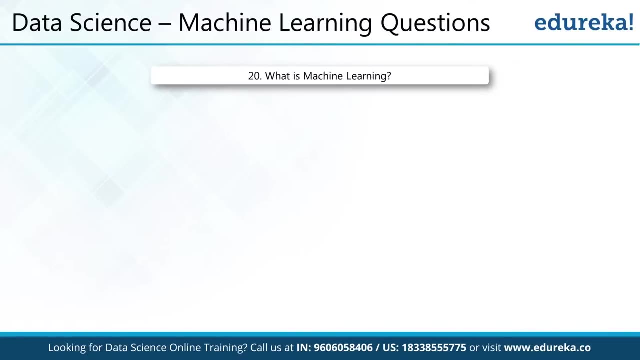 and so on. but what if you are asked something very particularly from a machine learning domain? right? so the next set of questions will cover those part. like people might also start with the basics, like what do you mean by machine learning? so the idea, I think, must be very clear. you were given a set. 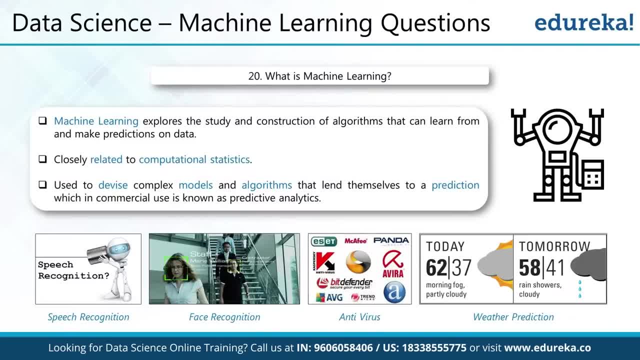 of data points particular to a given domain, right, and you would like to build a learning algorithm which will take the historical data and predict something for the future. so, as we talked about many examples, finding whether a convict is actually convict or not, like predicting if, given the evidence is if, 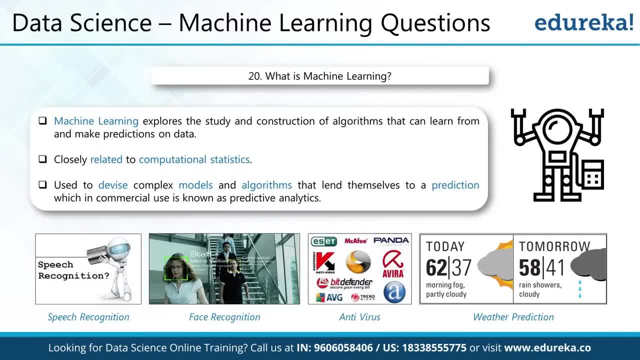 person is, is a convict there or not? or predicting whether we should be giving a loan to a customer or not. right, predicting the onset of cancer in a given patients by using the given patients historical records, and so on. and now this algorithms are now even becoming more complex, like it is starting to work on speech data face. 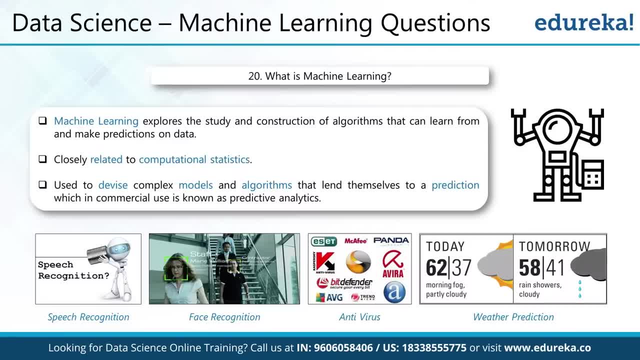 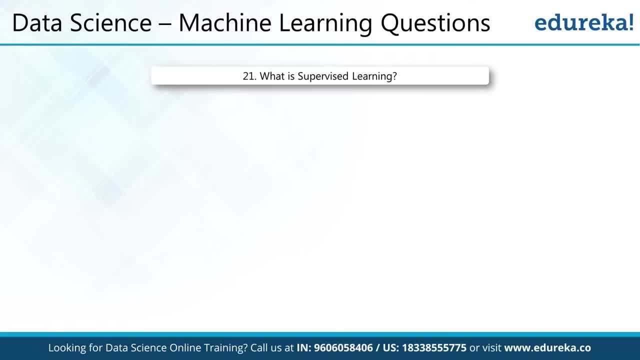 data, which are mostly used for biometric authentication systems. right so many use cases coming up from various industries, right so in machine learning, the most commonly used two types of learning: the supervised and the unsupervised learning. there are, like, two other types as well: the semi. 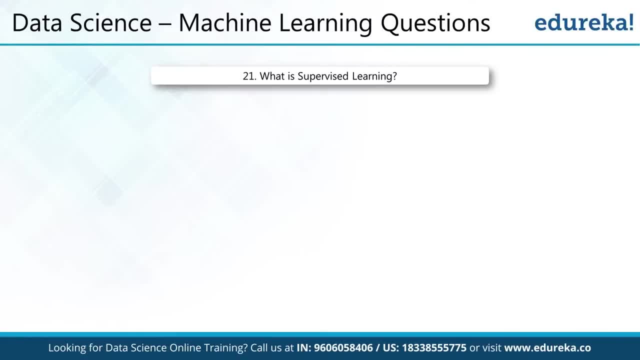 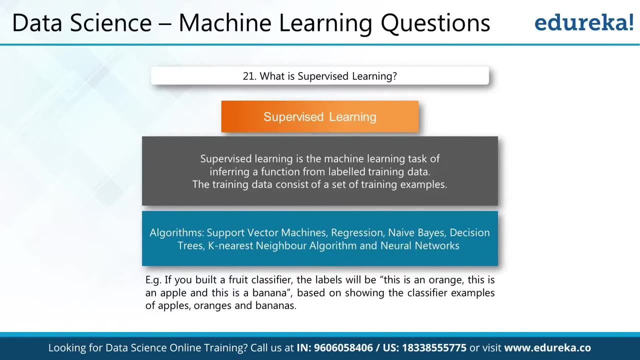 supervised and the reinforcement learning. and the idea is around: if you are given a set of input attributes, do you have a label which can help to learn the input attributes around any data points that you have or you don't have, right? so if you have, then the approach could be a supervised learning approach. 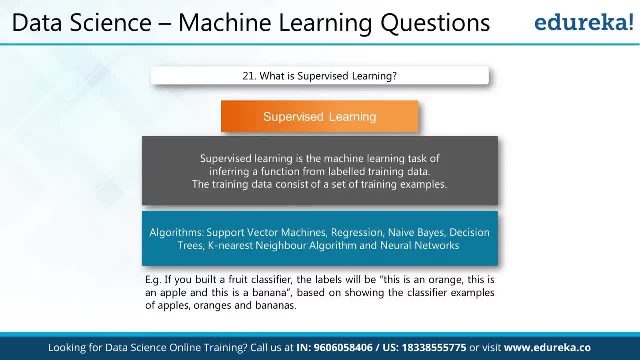 versus. if you don't have, then the approach is more and unsupervised. so some examples of the algorithms are like support vector, machine regression, a base decision trees. all of these are the supervised learning algorithms. so, in a very simple terms, if I say you are given an input, attributes for 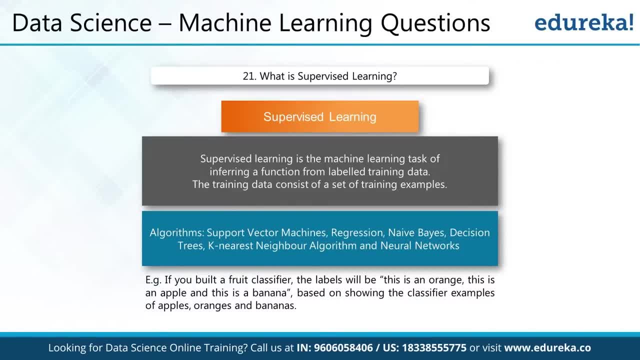 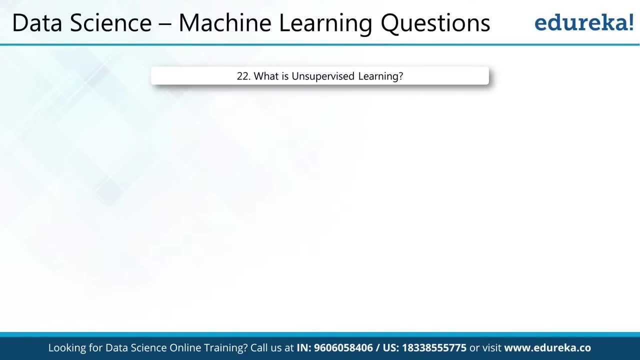 identifying. let's assume a sort of given an image of different fruits based on the characteristics of the fruit. can you like identify whether it is apples, bananas or the oranges? so if I am given that label with me, the model will run, keeping in mind that, given these characteristics, this is an apple. this is. 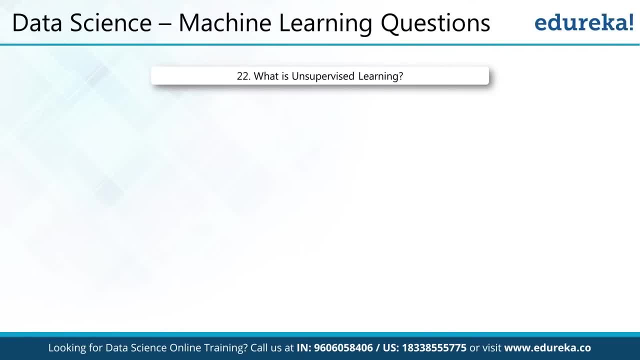 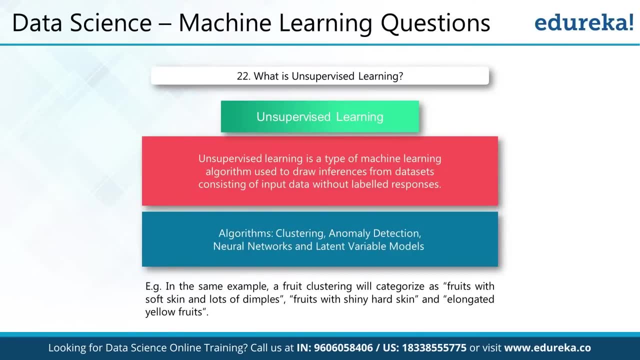 an orange and this is a banana. but in the other case, if you go for a clustering approach where such a label of saying that it is of apple, banana and orange is not available, then we might just simply segregate the data points with the input features, maybe with color. 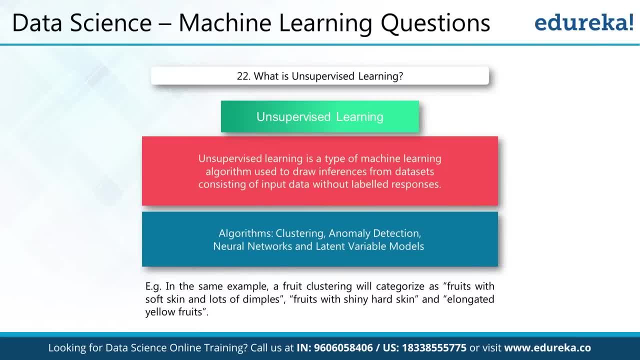 with texture or with the shape. right. with that, we can maybe say that particular fruit with this shape is, like you know, into a bucket which we can like call banana or another kind of a spherical shape. it might be apple or an orange. so, depending on the presence of a label, we can say either to use supervised or an. 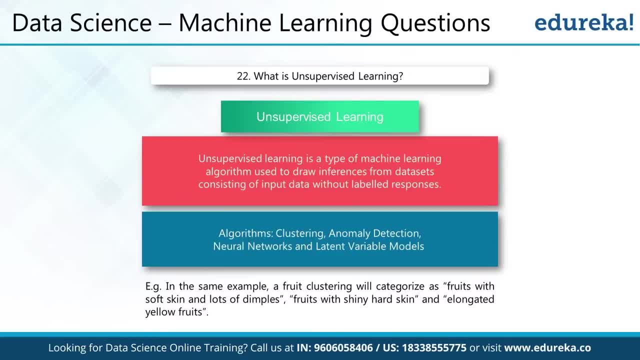 unsupervised learning, and both of these approaches are quite common, and sometimes there are certain algorithms which can have the both ways. it can also learn an unsupervised manner and the supervised manner, so depending on how you model the problem, the fundamental difference comes from the fact on 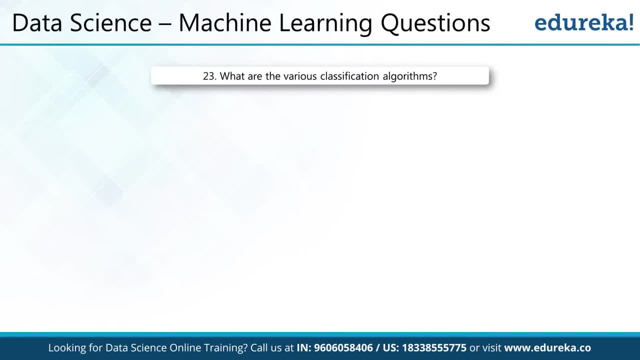 whether we have the label or not. okay, so when we talk about the supervised learning algorithms- other name for supervised learning- is kind of one of the types in the supervised learning algorithms, is classification right and the classification is around, given a set of input attributes, and the label is like categories right, for instance, if it is. 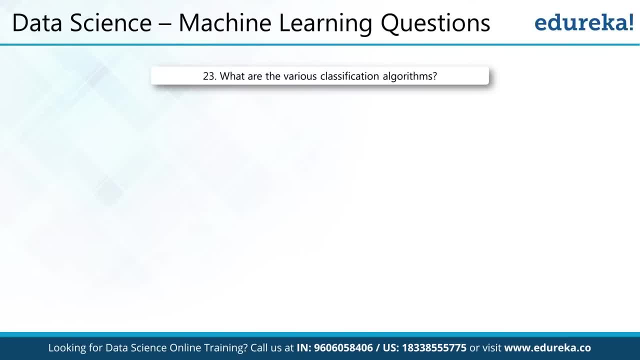 fruit- bananas, Apple and oranges- like if it is a customer whom we want to predict into either kind of a defaulter type or a good customer. so the classes are two like one, which is saying the customer is going to be a defaulter, the other says the customer is. 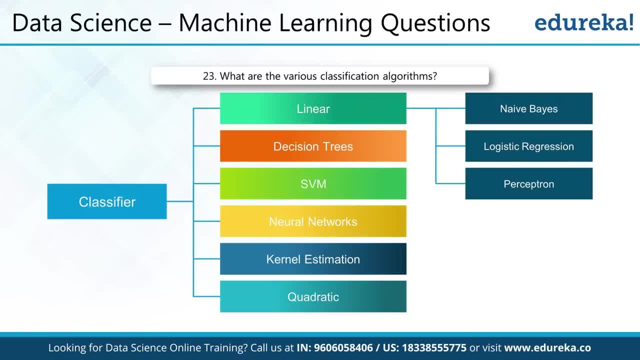 going to be a good customer. same is true for when you want to build and classification algorithm for detecting cancer- whether the patient has a cancer or not, has a cancer right- or if you want to detect, let's say, a malicious content or a malicious file, which might be a virus chosen, or worm or something else. 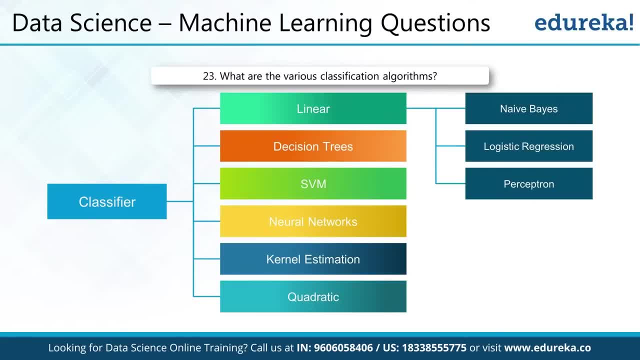 right. so in that case the classes are now many, so more than one class can also be there. but the fundamental idea is we are following a supervised learning algorithm, but the type of problem we are solving is a classification problem. so instead of saying the classification algorithm is a classification problem, so 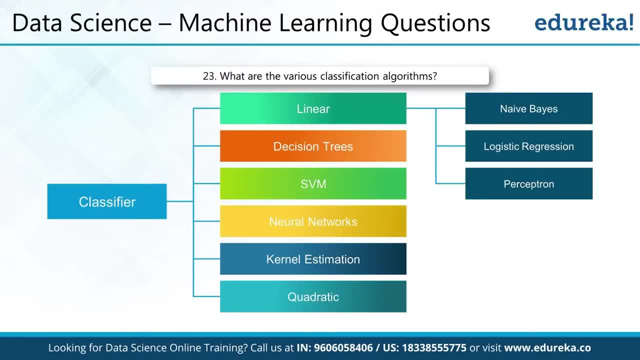 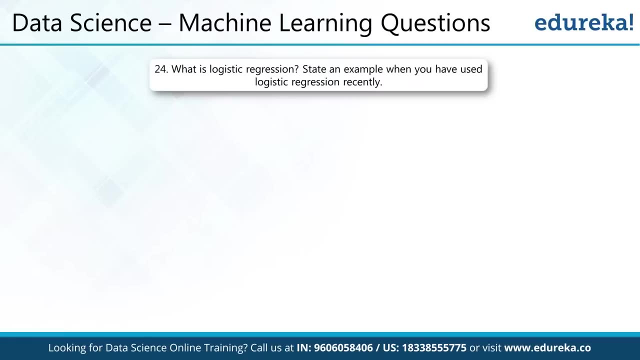 instead of saying the classification algorithm, we can also say it's a classification problem using supervised learning algorithm. so these are the various types of classification algorithms, like the linear regression decision tree, then you have the support vector machines and so on. right, so now let's talk about one of the types of classification algorithm called the. 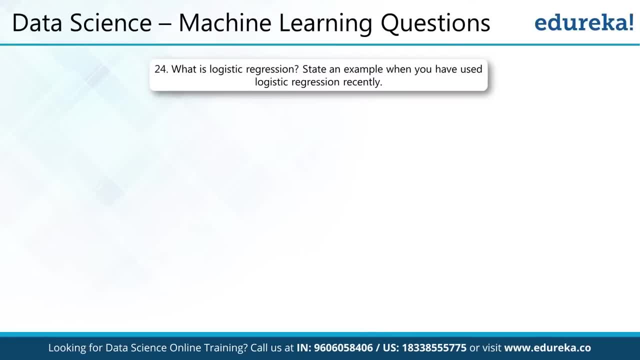 logistic regression right. so very commonly used algorithms and banks or companies as big as like American Express, so sort of, have leveraged the logistic regression algorithms to quite a extent and they have like built a really really robust implementations of these algorithms, particularly in banking sector cases like predicting whether a customer is going to be a default or or not, given if 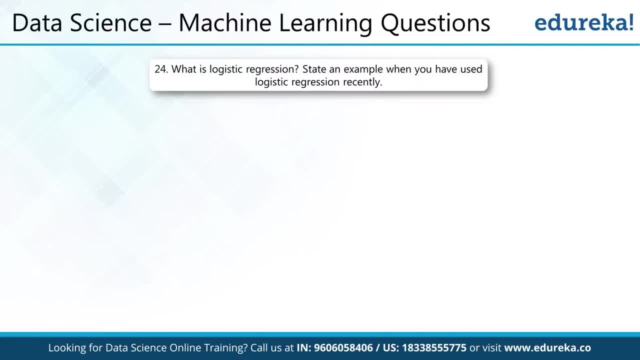 I issue the customer a credit card or give a loan right. these kind of decisions can very well robustly be taken from a logistic regression algorithm, and these algorithms are best suited for two class problems or a a binary problem, right where you have either- why yes or no- quite a common. 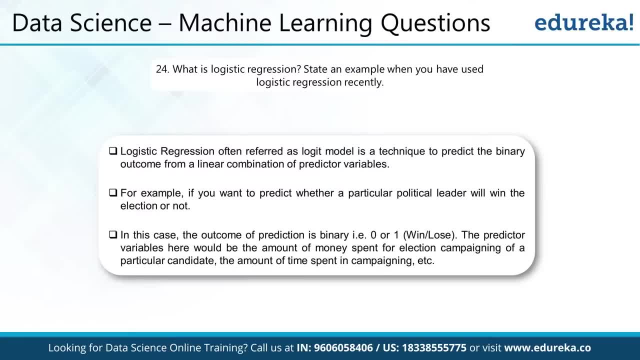 technique, as I mentioned, and in all the possible cases wherever you have these binary classes of problems, you might use a logistic regression: a political leader winning a collection or not, somebody getting a success in an examination or not and, as I mentioned, whether to give a loan to a customer basis, whether he or 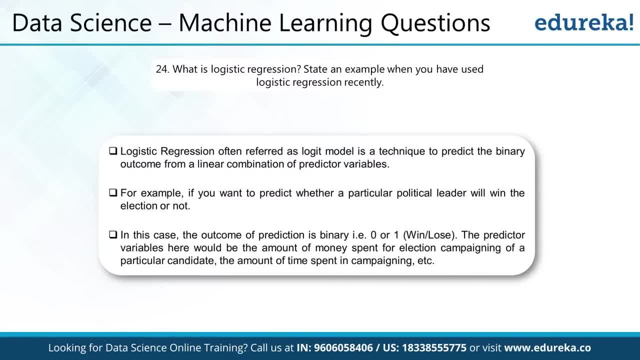 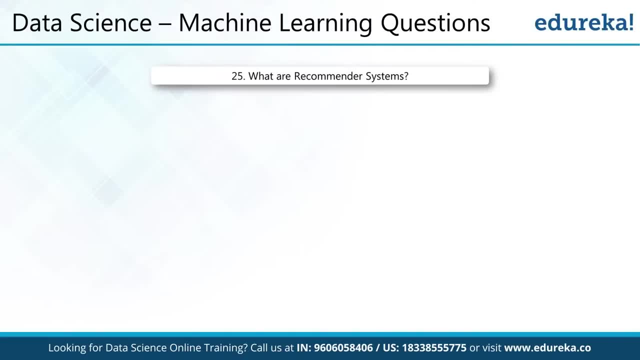 she or is going to become a defaulter or not, and many of these like binary types. so keep in mind logistic regression works best for classification problems with two class. so one of another. widely used algorithms like the recommender systems and like I think, this particular algorithm doesn't. 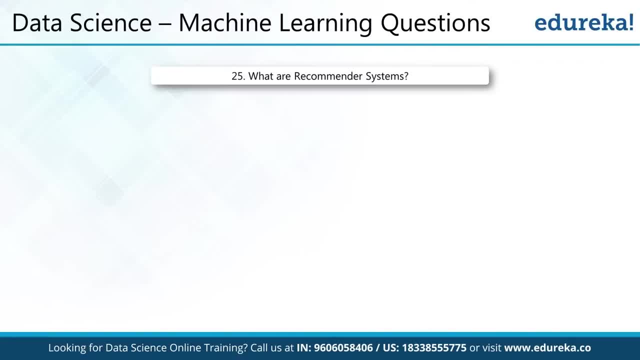 need introduction. so this is that common nowadays. take an example in Amazon you have a product which you are browsing, the products which comes in bottom of the widget which says you may also like, or customers who brought this also brought this right. so these sort of recommendations is actually from recommender system which is running in. 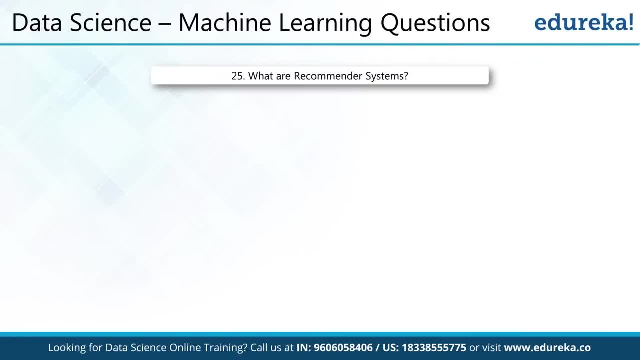 the back end, if you like. take YouTube example: if you watch one video, the next video is like- starts to come, one after the other. that again is a recommender system working in behind the scene. or if you take Netflix, if you watch a particular movie, it starts to adapt right to a movie which you might like. 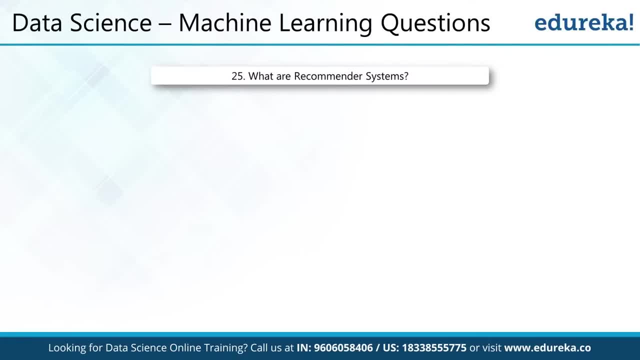 Netflix also uses recommender system. the applications are like coming more and more as sophisticated systems are building in. right, Facebook uses it for recommending friends. right, you have a set of friends and, based on your data coming from the contact mail list, Facebook starts to curate friend suggestions. there and all. 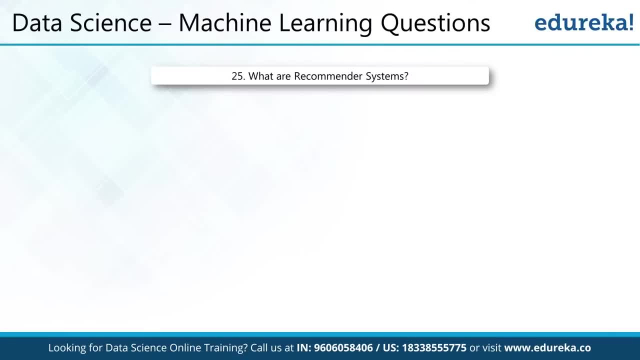 of these are algorithms which might benefit the business in some way or the other. for Amazon it is. if you give a recommendation below a page, people might buy one more than one product in a transaction for Facebook. they will grow their network of people and they will be able to get more and more products in a transaction for Facebook. they will grow their network of people. 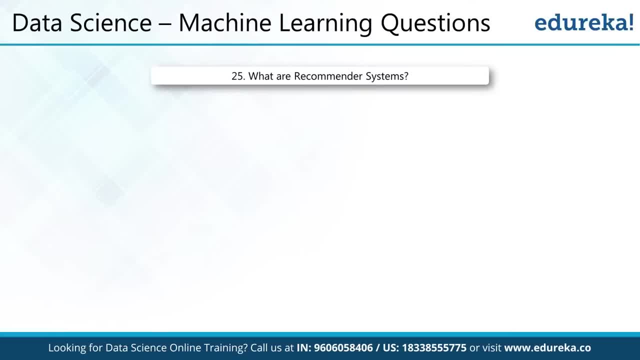 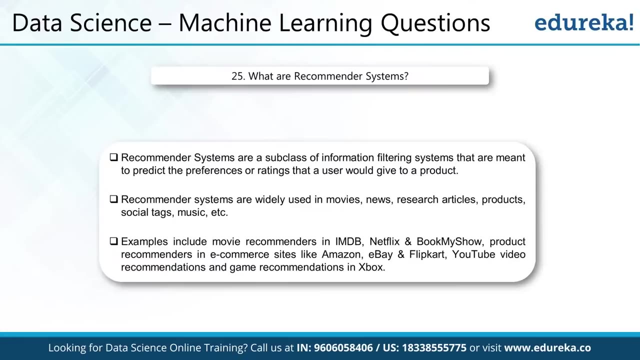 right. their connection between the users are going to go stronger and hence, obviously, the kind of ads that Kufa is Facebook wants to sell will also starts to grow right and more our users, more the connections, more is the sort of interactions. you know about the connections as well as the behaviors. 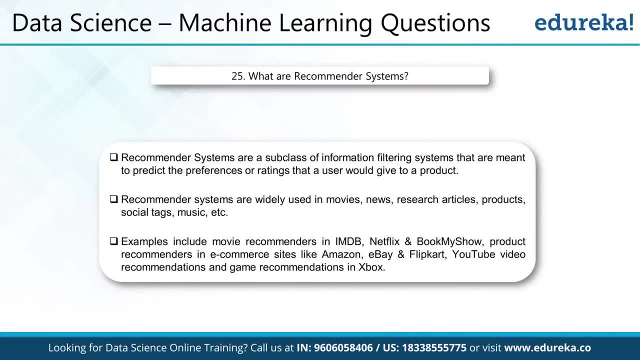 that people show in a social network. so the fundamental idea behind all these recommender systems is to get a meaningful comparison between two users or between two items right for Amazon, between any two products. what's the similarity? if the similarity is really high, recommend that product to the for a given product in. 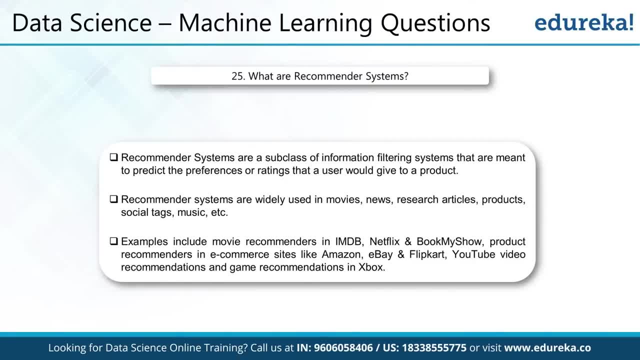 consideration. or if you find that two users are very similar in, let's say, Facebook, you might want to show to each other that you have another friend whom you might want to connect right. so there are, like many such use cases, which comes out the moment you get into the deeper understanding of recommender. 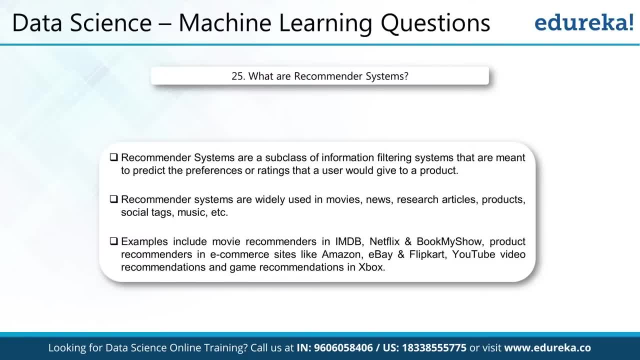 system. but the fundamental idea is: how do I compare two items? the items might be product, people, movies and so on- and how do we compare two users in simple terms? so this is what a recommendation system works on. so there are quite famous examples, like the collaborative filtering approaches- user-based collaborative filtering. 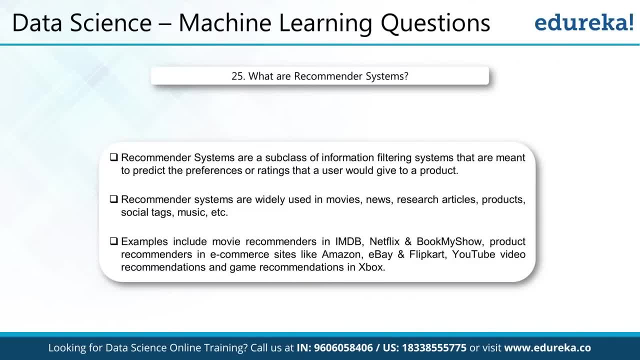 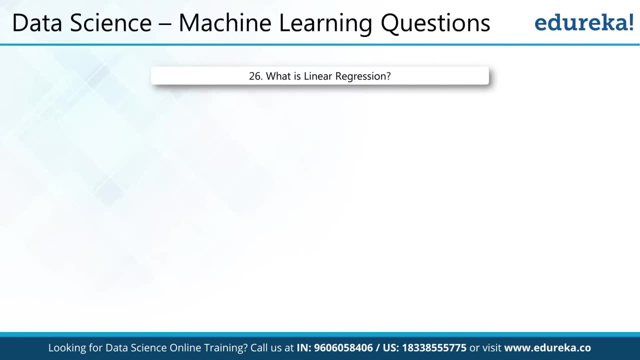 algorithms or the item-based collaborative filtering algorithms. both of the algorithms are quite commonly used in recommender systems and nowadays people have also moved on to latin factor-based models like the svd, singular value decompositions and many others. so we talked about classification problem and then we said logistic regression is a binary class problem, right, so you? 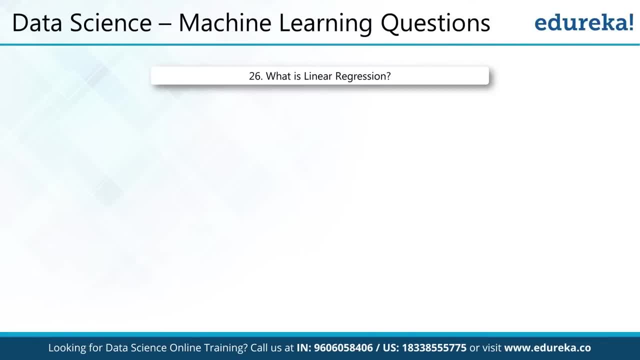 might also be asked something around linear regressions. so what if i don't want to have a class of a particular user or a patient or something like that, right? but instead, if i would ask you, can you give me a crisp value instead of a class, right? so when i'm like classifying a given 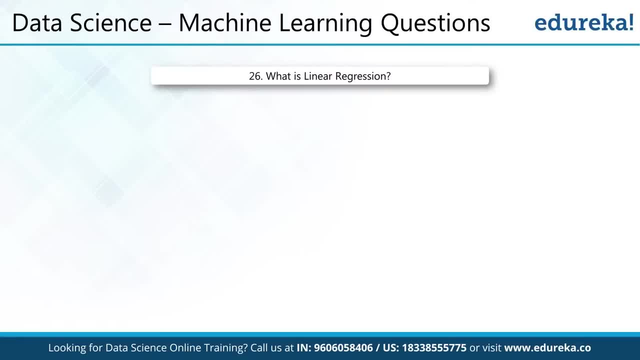 file into you a good bad, in which bad can be virus, worms, trousers. these are the classes. but if i don't want class but rather, for example, if i want to know the exact value of a house in a particular locality in my city, how do i calculate that right? so linear regression models in machine learning. 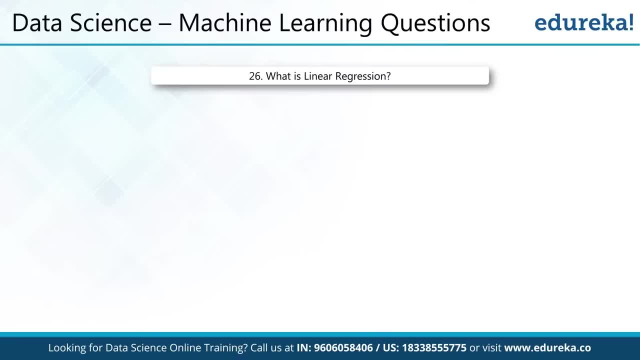 is one such technique which can regress over a given input data, which might include the properties of the houses, like number of bedrooms, the area in square feet and so on, and finally predict a value, a crisp value, which will be exactly in terms of, let's say, dollar or, uh, in any other. 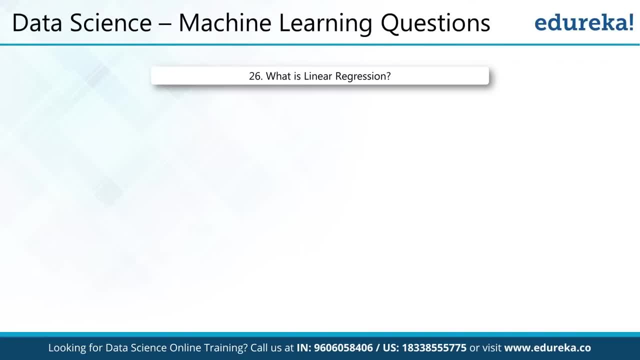 currency, the value of the price, and the idea is, once again, that you have a training data with you which has labels. so from the past data, i know that, given these attributes of the house, what should be the idle price of a house? i'll use that as my training data and then build my model for future. 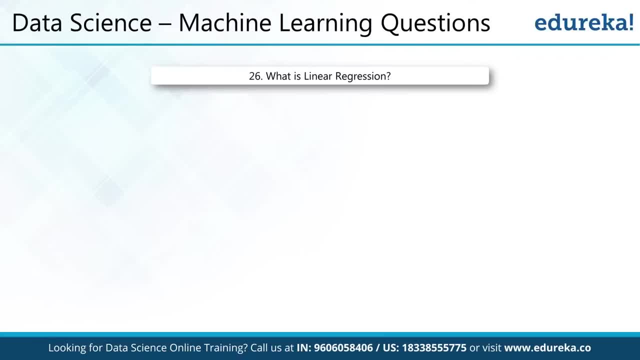 so now, with any such similar pattern in any data which is going to be coming in future for maybe a new property which is built in some kind of model like a house, with which we can do some kind of, say, XYZ location, I can use the model and predict, exactly because these features. 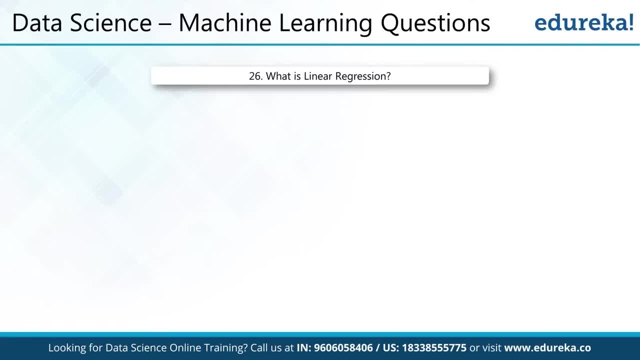 are somewhere similar in that locality the prices might be, you know, in a particular range. so a model like linear regression will learn those patterns in the given input attributes and try to predict the price of the house. right, and the idea is, if I have a set of data points, I want to build a very generic. 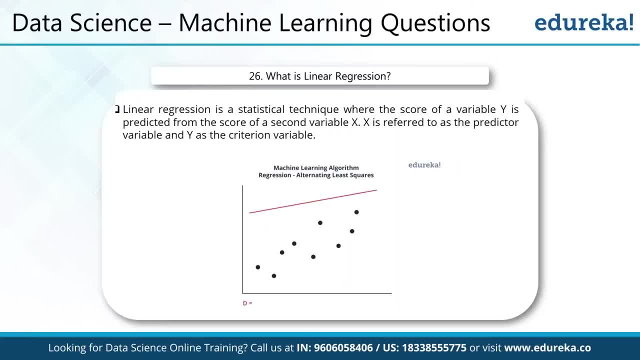 model, like drawing this line which is as close as to all the points, right, so you can like draw infinitely many number of points if you are given a set of data points like this in a two-dimensional space, but the one which is the shortest or the closest to the points is the best line. so the red line which you see here, 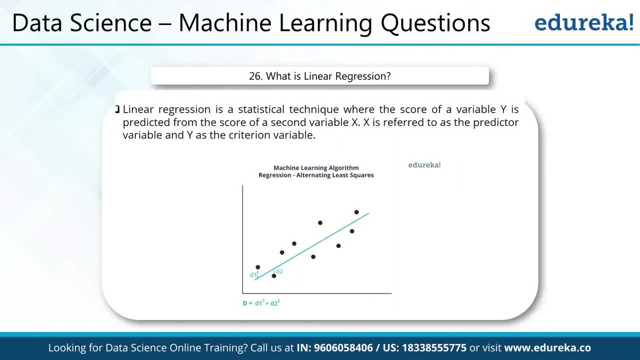 is like far away from all these points, right. so this is not a best line, but if I see this blue line which is very close to all the data points, is like one of the best lines which I can get from this points, right. so the idea here is to fit. 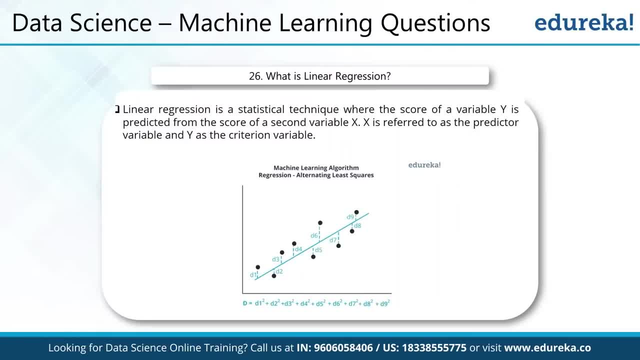 a line, passing through as closely as possible to all the data points that I have and minimize these so-called the error, which is nothing but the summation of all the data points that I have, and minimize these so-called the summation of all the data points that I have and minimize these so-called the. 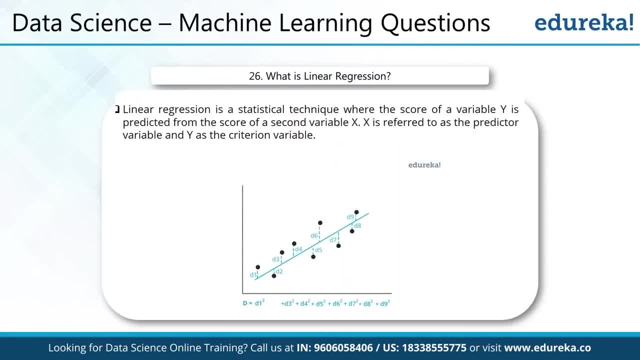 distances right. so there are simple linear regression ideas and the fundamental idea that we are following here is your variables are having a linear relationship, which means with the increase of one variable, the other also increases. but if you have a pattern which is not so linear in shape, like if 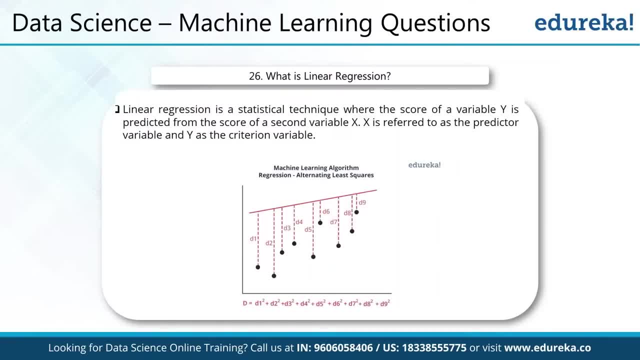 you are like, not able to draw a generic line, but the representation or the sort of points are aligned in a way that you can only create a model which is polynomial. so if you are able to draw a generic line, but the representation or the sort of points are aligned in a way that you can only create a model which is 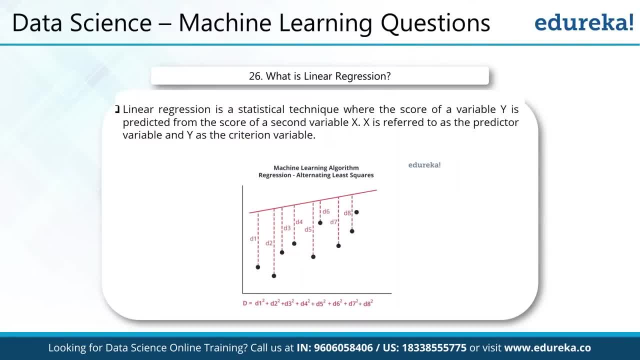 polynomial. so if you are able to draw a generic line, but the representation or the sort of points are aligned in a way that you can only create a model which is polynomial, so in that case linear regression will not be so useful because the relationship is not linear anymore, right? so in that case you might. 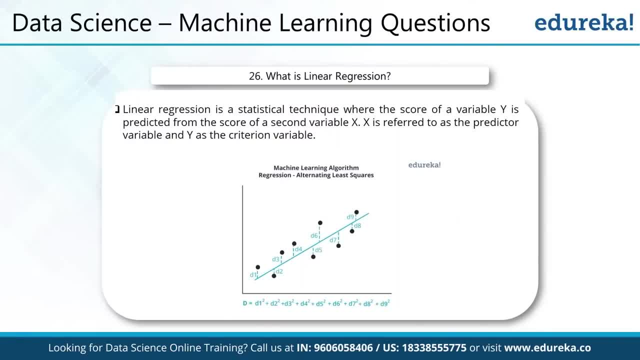 want to go for some other regression approach, maybe like a polynomial regression which has a nonlinear relationship between the independent attributes. so quite a common approach and it has, like a really large chunk of its explanation coming from the statistical ideas. statistical ideas like hypothesis testing, p-values, confidence intervals and so on. so it's. 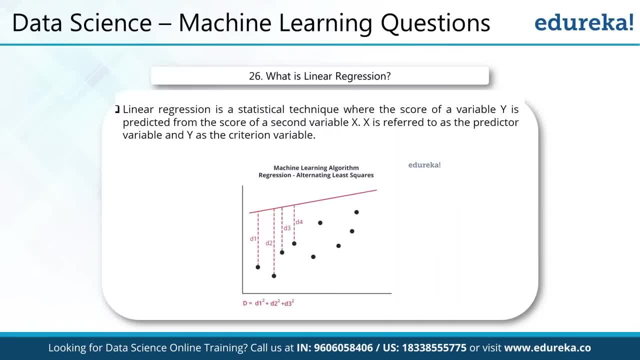 if somebody is asking you around linear regression, it would be to start with saying how you are build a linear regression model right, and then you might give some examples of it. so, at best, if you're not comfortable with these ideas like p-value or hypothesis testings, you might want to refresh that. 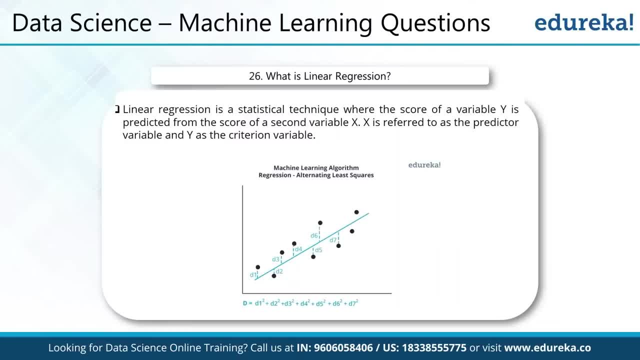 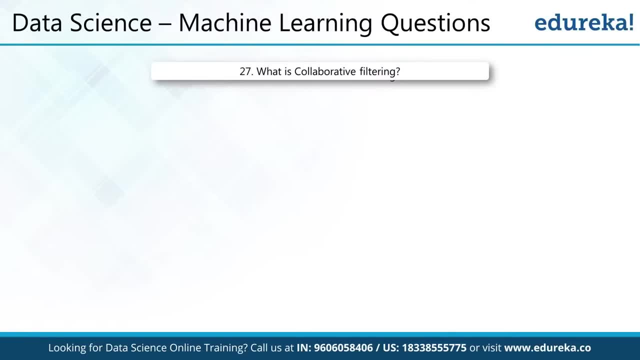 before you like, go for any interview, because if linear regression comes up, these concepts needs to be a bit more explained, right? so when I talked about the recommendation algorithm, I mentioned something about collaborative filters, right? the user-based collaborative filtering or the item based collaborative filtering? so these are the two commonly. 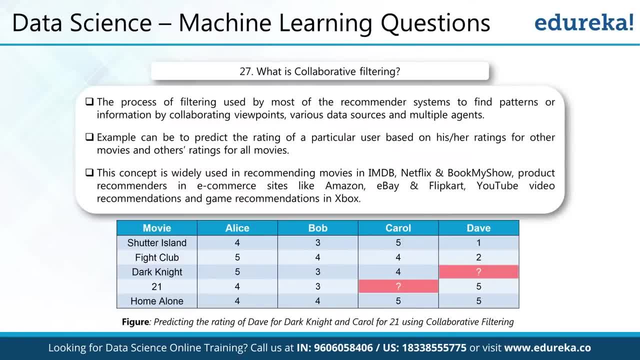 used sort of recommendation algorithms right, normally referred to as item based, so IBCF and the UBCF as idea, as I mentioned, is to compare to users or to compare to movies or, let's say, items in particular. so the item can be anything- a product, a movie or a person and the sort of weight bills. the model is given lot of users and their 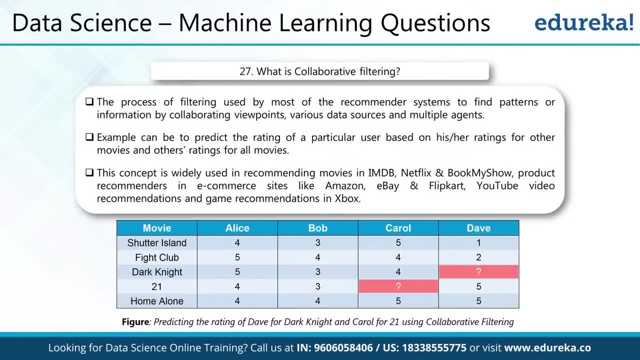 particular, let's say in this example the rating to a movie. we now need to find out: can we recommend for some users, based on the behaviors of other users or their ratings to the movie, some suitable movies or not? so for example here for Carol: Carol has not seen the movie 21, right, so there is a question mark there. 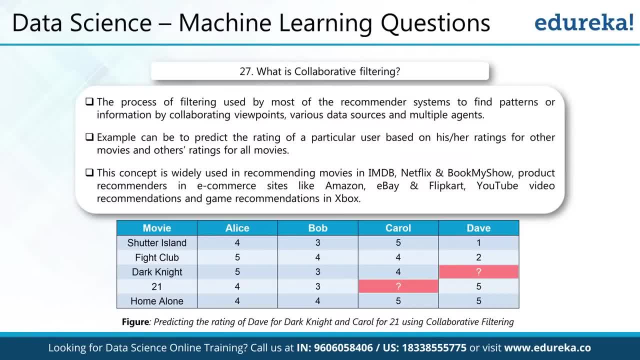 so can I predict this value? if it comes to be, let's say, like close to 2, I won't recommend the movie. but if it comes to, let's say, somewhere 3, 4 or 5, yep, the model says yes, recommend this movie to Carol. okay, so one more fundamental. 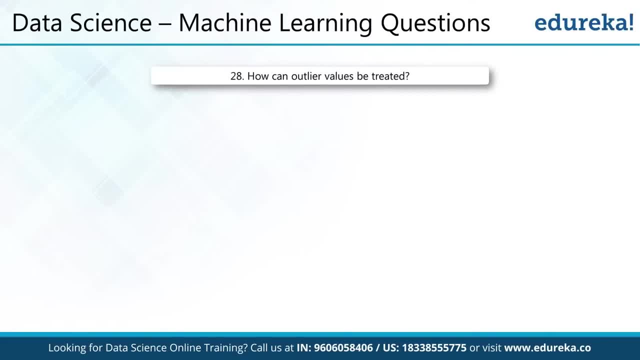 problems on when you build the models. so, as I mentioned in the earlier discussions, that when we are doing some analysis with the data after you collect the data there requires a lot of cleaning right and exploration as well. so in that process of cleaning and exploring the data sets, you might often find there are 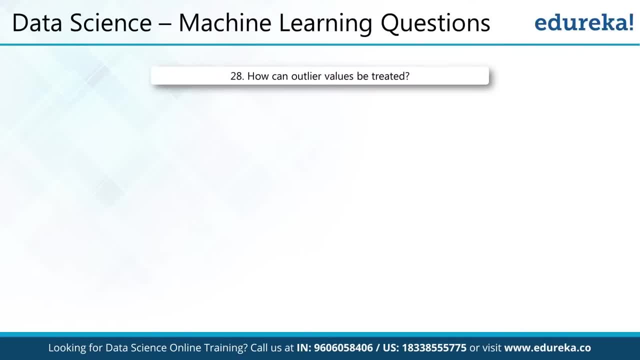 some extreme points. so, for instance, if I am building a regression model for predicting the house prices, and there is this one house price and there is this one house price and there is this one house price with somebody has sort of able to sell for a very high price by means of maybe. 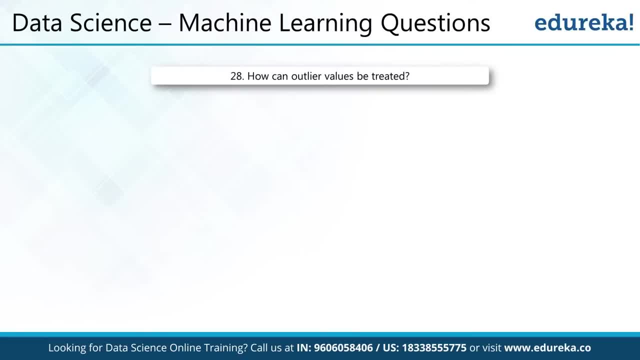 some auction or some other sort of marketing gimmick there. the point might mislead the model to predict or get itself towards that outlier point. right, so we don't want to like move towards an outlier point, but we need to deal it separately. so if you don't have a better explanation for why that outlier is in, 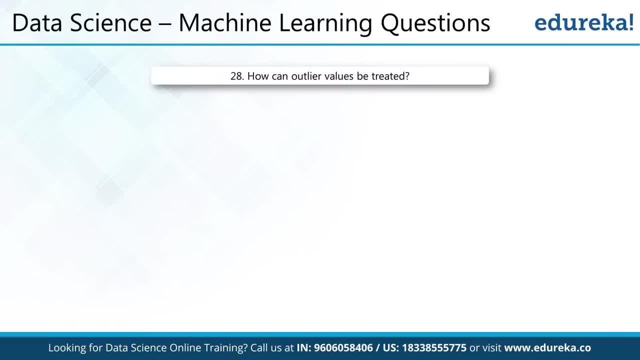 terms of an input attribute, better is to remove it. so, for instance, if I am like analyzing any data in an e-commerce world where I am going through all the products and the sales that the product has seen in last one week, and on the last one week there was a particular day when a kind of a sales day was there. 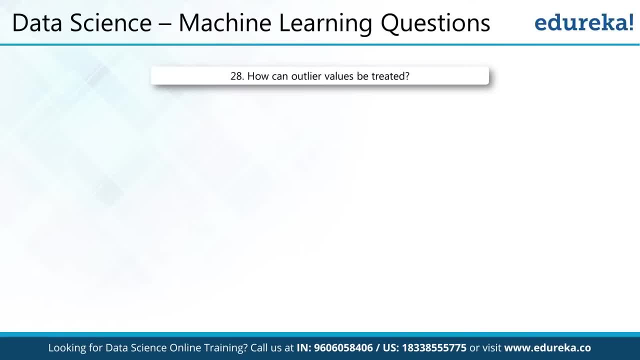 like nowadays, e-commerce companies do this a lot, but in those sales days, you would obviously expect that the products purchase is going to go very high, right, but does that mean that it's an outlier to me? not, because if I am able to explain an outlier by saying that this was a discount day, I might be able to. 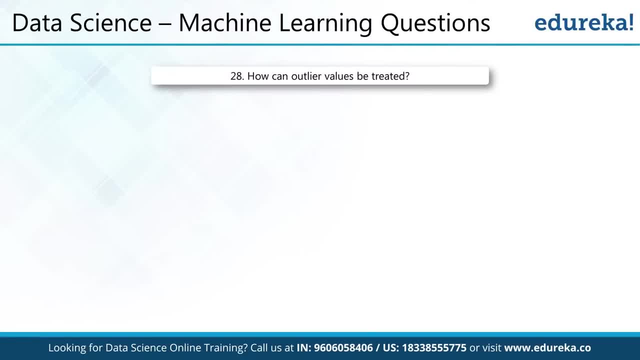 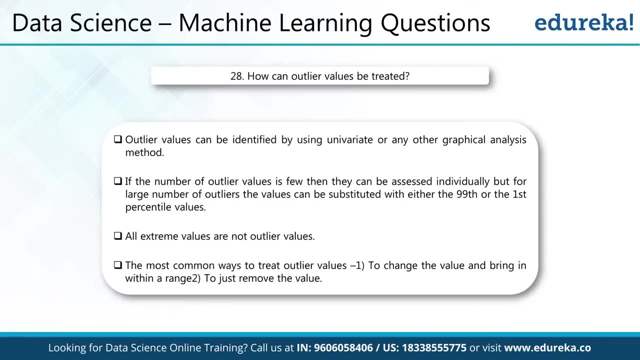 handle it separately. either I can like simply take all those points which are for the discounts day or sales day and keep it separately, or if I would like to have the variable, like saying whether the given day is a sales day, and keep the outlier as well, then the analysis goes in a different direction. so it's 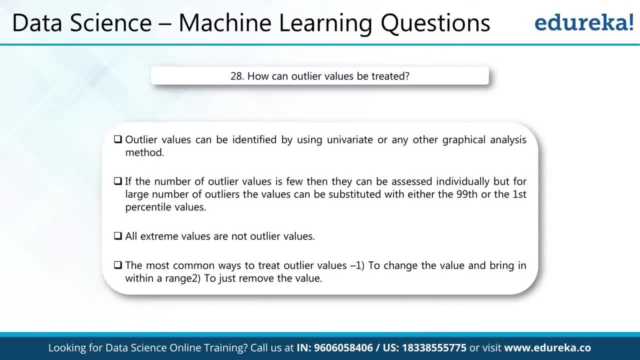 important you handle the outlier before you start to build your model or do any analysis. otherwise your insights or your models output might totally give you a different direction and there are very different ways to handle the outliers. so some people use approaches like removing any data points, which is like outside of the range of mean plus 3. 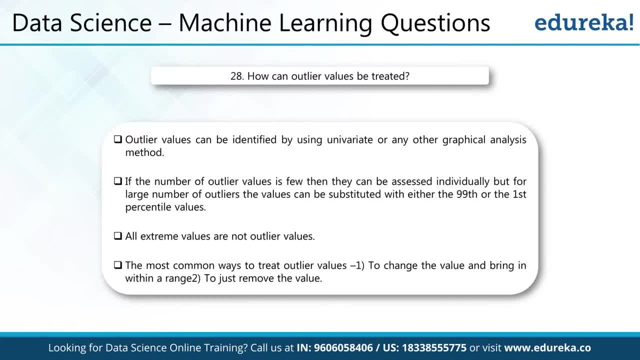 standard deviation right, or sometimes people also use the percentile way of doing it. any point which is greater than the ninety ninth percentile can be like removed. so these are like you are removing the toppers from the data points of yours of, let's say, a SAT examination or a CAT examination. so the 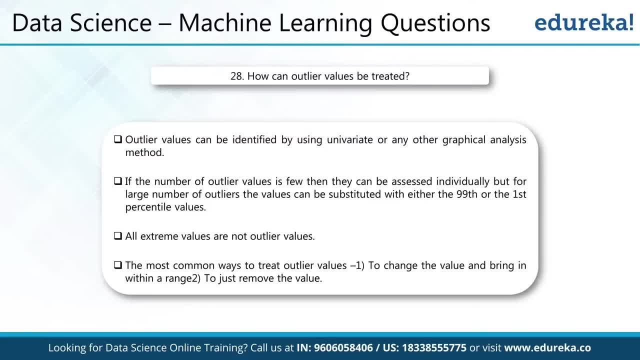 are sometimes can cause certain issues in explaining the model. so you can obviously imagine this in very intuitive terms. also, if you have a set of first course for candidates who appeared for an examination and there was one outlier candidate who scored really, really high, so do you have a way of explaining that? 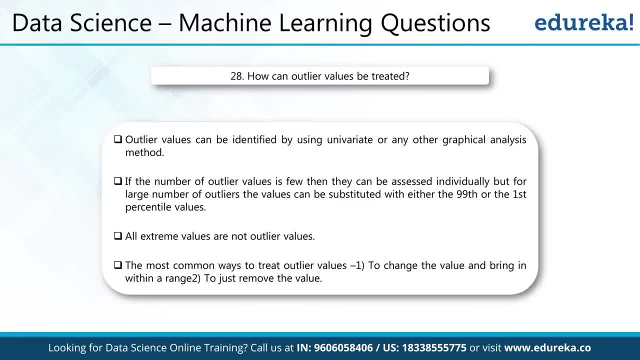 outlier. you might be simply calling that person a talented person, but does that like? explain the model may be difficult, right? so better is to keep those exceptional cases separate and do the analysis with the rest of it, so which gives you the good pattern or good insight from a data. so that's how you 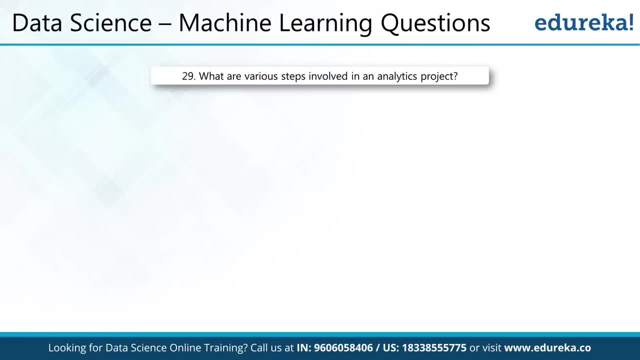 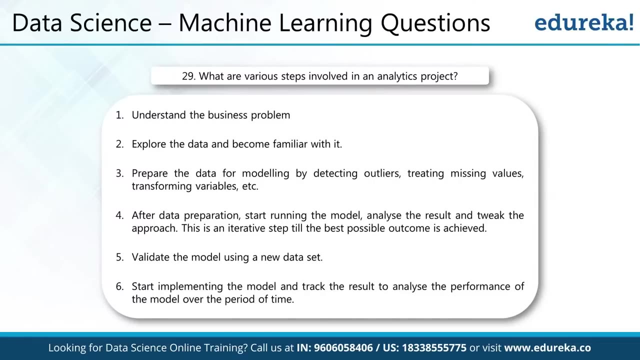 like normally handle an outlier right, and this quite often is an important question to answer that: if you are given an analytics project with lot of data, how do you normally approach it right? in typical cases, the first step is to really go deep dive into the problem in hand, and the problem needs to be defined. 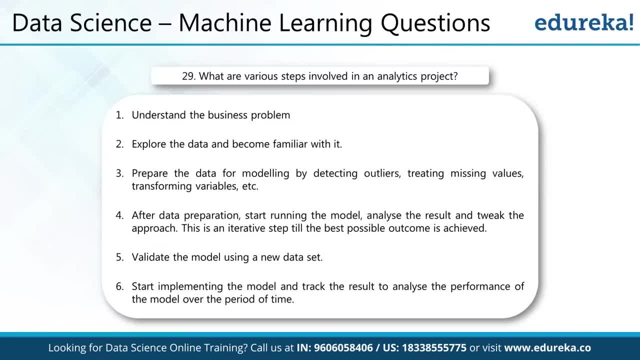 very crisply. so no, never define a problem which is broad in sense. so, for example, if you are building a model for customer segmentation using a clustering approach, so instead of saying build a customer segmentation model for all the categories of products, that can be like a broad problem. but if I say 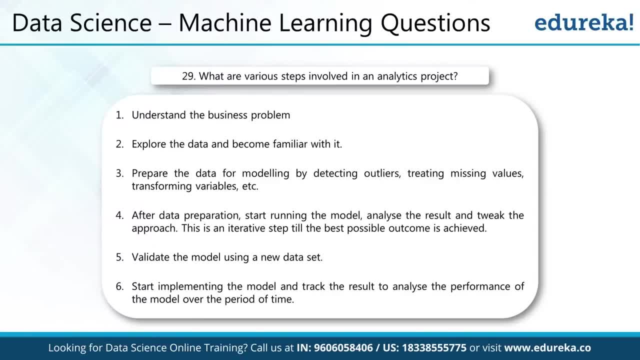 build a customer segmentation model only for fashion category of products, right then the problem becomes crisp. so defining a problem statement and it's understanding is the foremost task. and then comes the kind of exercise of exploring the data in which you will identify outliers, missing values and if you need any. 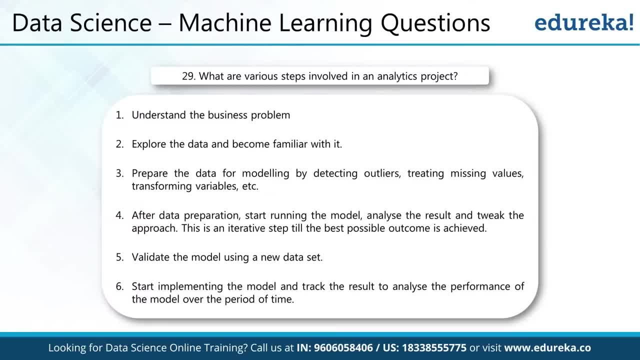 transformations like converting from a log format to a wide format or the vice versa. you do all that steps in the second and the third step and once we have found out that the data is very good, now, after we have removed all the outliers and the missing values and 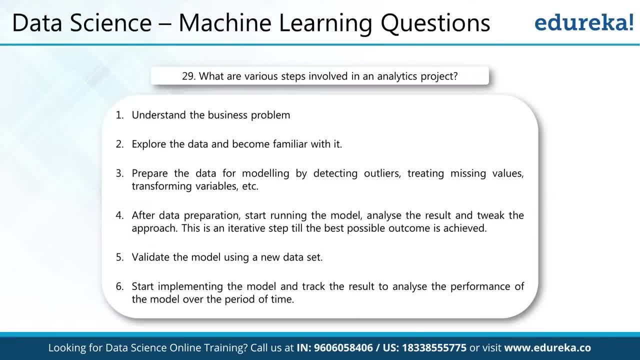 so on. you then start to understand certain relationship like given input attributes relate in some way or the other right. so this is a stage where you start to prepare for any further insight building exercise. or like model building exercise. and let's say, if you build the model in this step, the immediate step is to validate it right, whether the model 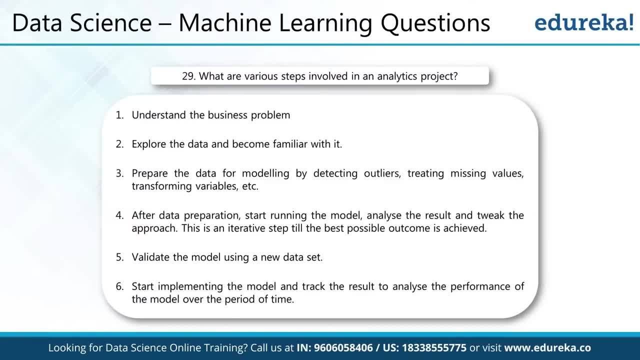 is really good or not, by using a testing data. right, and once, let's say, all of these is done and you are either coming out with a insight or a model, you would like to see, in long term, how this model is going to perform. so it might happen. so, because every model is not static, 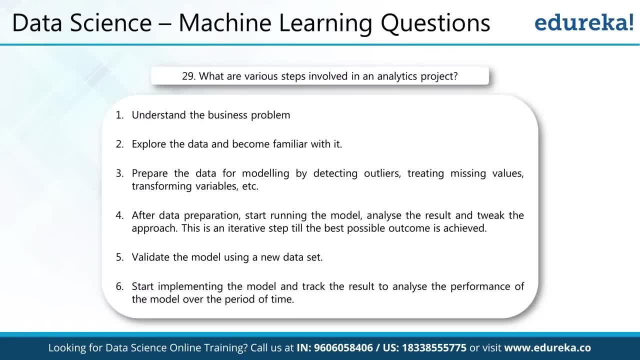 your data is growing on daily basis, So if you want to build a really robust model on a growing times, it should append. the model should update based on the new data which is available right. so over a period of time you should track and analyze how good the model is performing on a real world data and 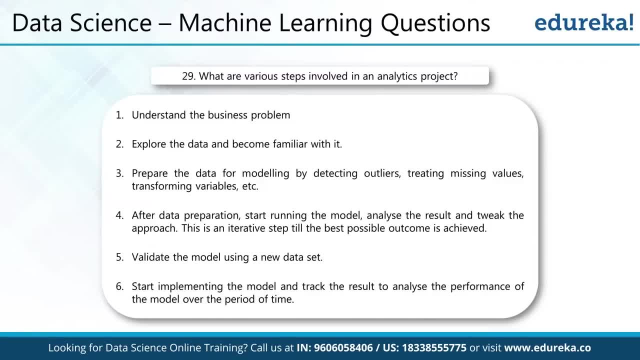 if the performance is going down, then it's time to retrain the model and maybe come out with an updated model on the data that you are already given right. okay, so one more task. as I was explaining in the cleaning process, how do we treat the missing values? 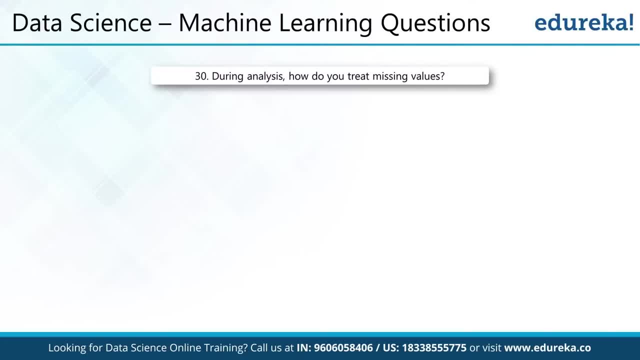 So there are quite a number of techniques to do that. so, for instance, if you have an attribute- let's say age right- and you are analyzing this age in various segment of people- people who are teenagers, people who are professionals, people who are still in their college and 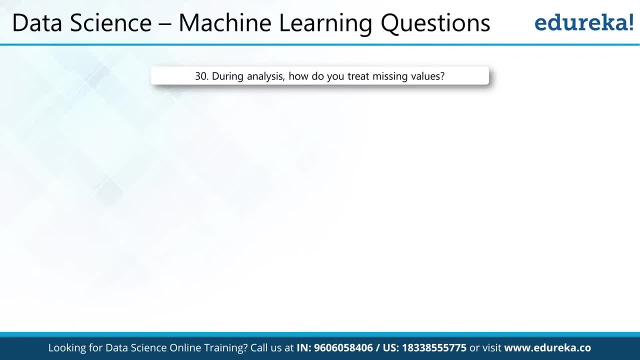 so on, right. and there is one value missing in one of these categories of people, let's say teenagers. so if the age is missing, because I know I am analyzing a group of people who are teenagers by looking at the average age In the teenage group, right, I can maybe impute a value. so instead of discarding the entire, 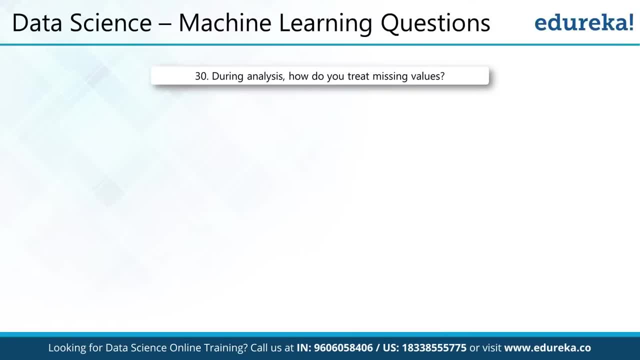 row because I don't have the value of age. I might be able to impute it by some simple measures like this: calculating the average in that group and putting the value there, which will not be completely wrong, because I know there is a very strong evidence: teenagers. 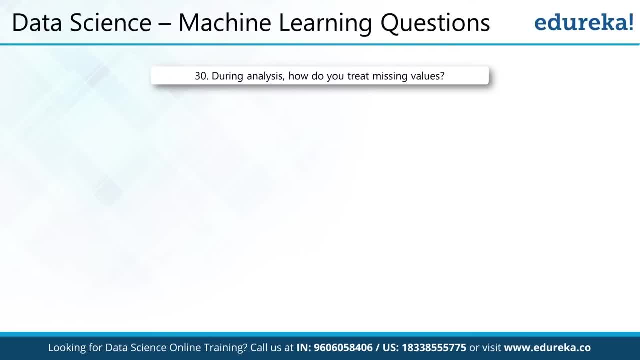 would be more or less in the range of, let's say, 16 to 20, right, even if I am wrong in my average calculation, it might not be so high. It might be like This: plus or minus one or two years, so which I am like, fine with if I want to keep my data. 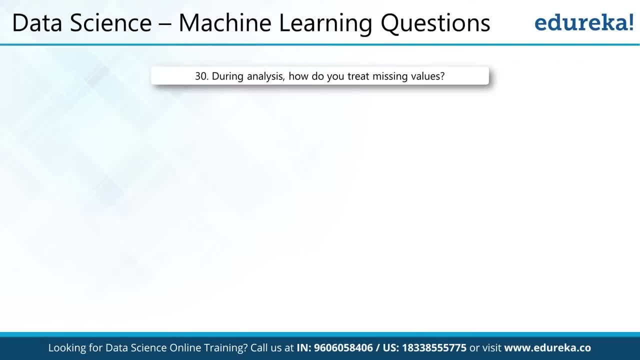 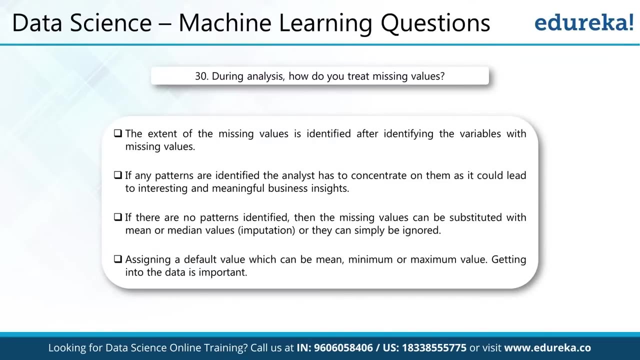 retained, and you might see that in your many applications. sometimes having a kind of discarding a particular row because of missing values might be very costly, because the data is limited in number. so that's why people normally do this at a sort of mean minimum or maximum. 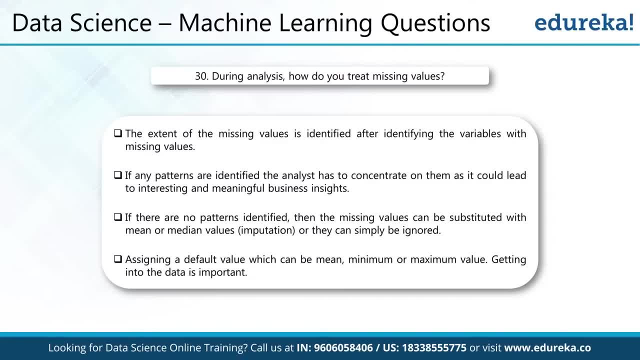 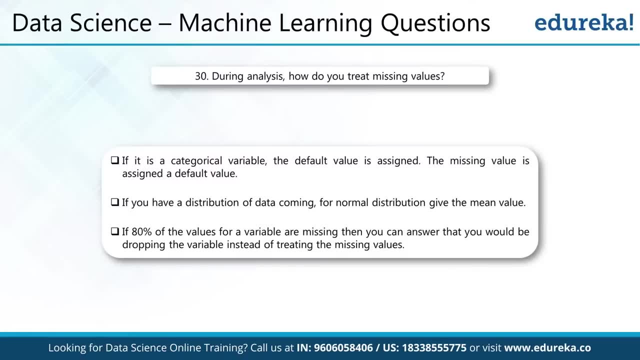 kind of a value, or they also calculate the average and impute the value there. so there can be some other pattern based Imputation also possible. but I'll just give you an example. and in other cases, if nothing is possible by putting a value, if everything is going to be misleading, then better, better. 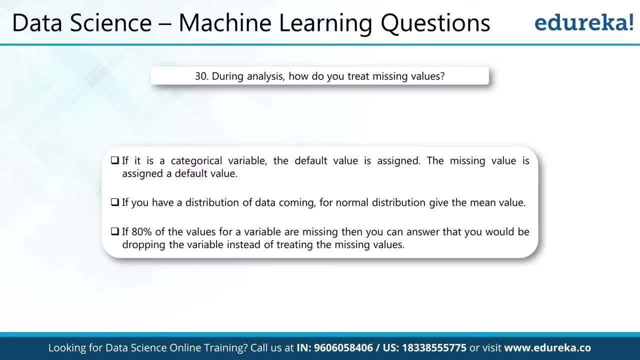 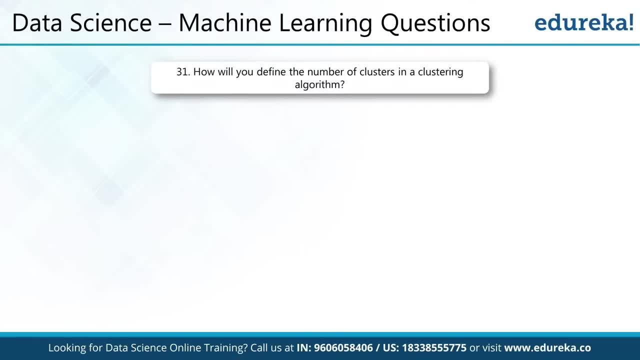 is to like remove that, but that can only be done if you have a surplus of data with you. if not, then be cautious of removing any values, particularly the missing ones. okay, so this question particularly pertains to a machine learning algorithm called k-means right every. 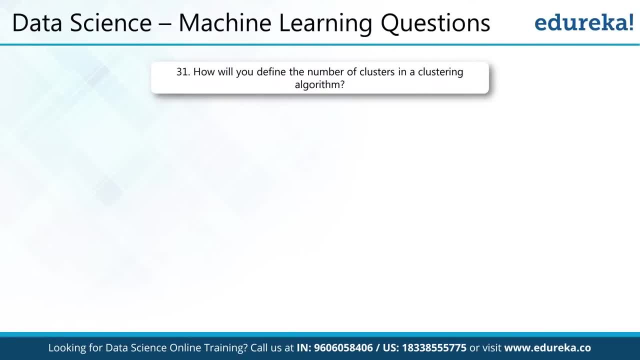 time you run the algorithm you have to define what should be the value of k. So there are approaches like elbow curve, which plots the kind of a plot scatter plot between the x-axis, which is the number of clusters, versus y-axis, which is the WSS, or within sum. 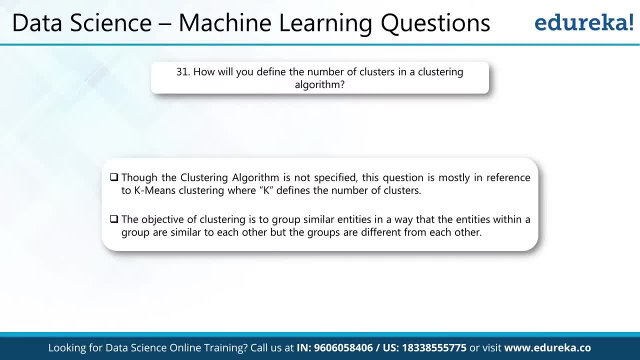 of square, which is also known by the name distortion. the idea is, when we are building the k-means clustering algorithm, if we find at one point- if you like, keep increasing the value of k, then one point- we find that the distortion is low, which means the distance. 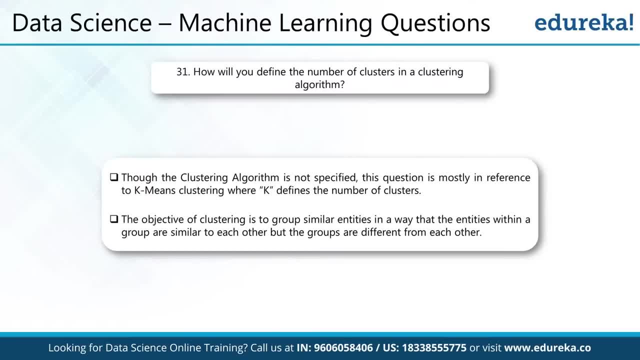 between The data points within a cluster is as close as possible and the distances between two cluster points, like a point in cluster one and a point in cluster two, is as far as possible. so that's the case. then the distortion will be like very low. but if your points inside 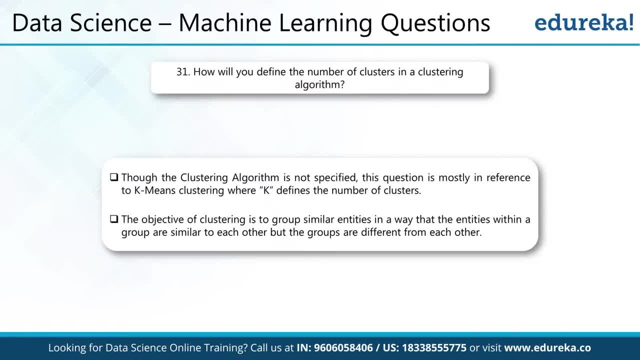 a cluster itself is very spread out and your clusters are very close to each other, then the distortion is going to be very high. so in those cases the value of k needs to be maybe further increased, and at one point using an idea called an elbow curve, which would 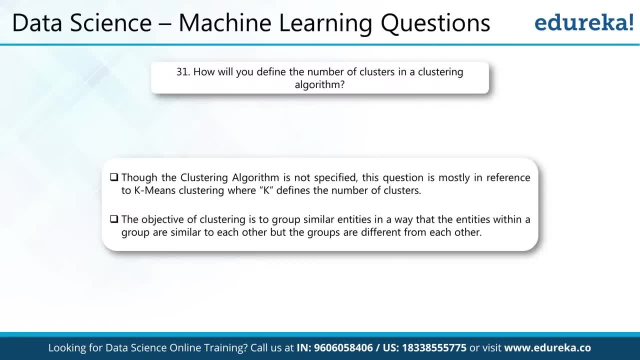 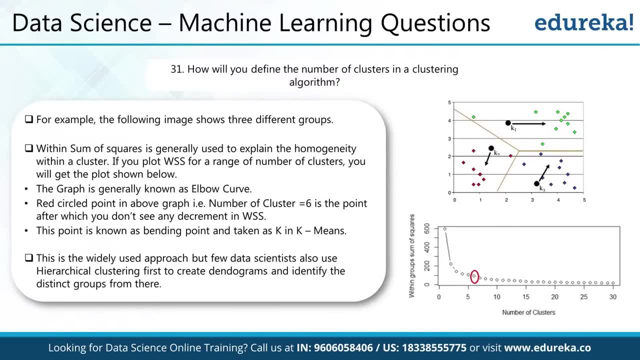 show you a small kink from where there is a sharp dip in the distortion values, and that is an appropriate value for k, while we are building a k-means algorithm. So this is how it looks like, so you can see. here, the x-axis is the number of clusters. 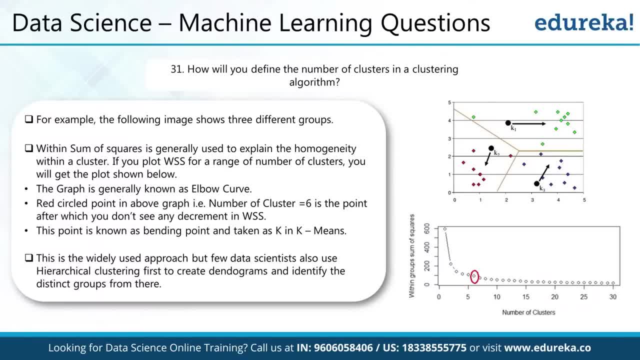 and your y-axis is your within group of sums of square and at one point you can see there is a sharp dip here. here and after this point, which is like circled in red, the values sort of almost saturates. so this may be, I can use as the appropriate value of k, which is the 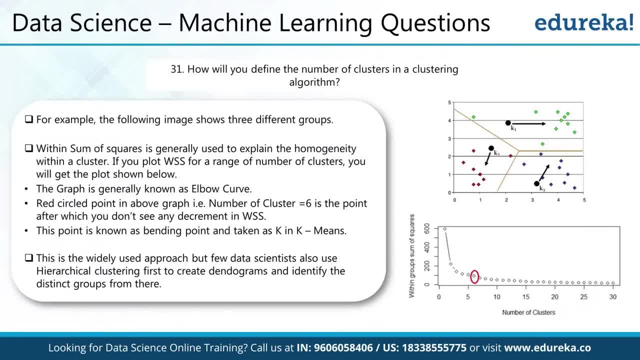 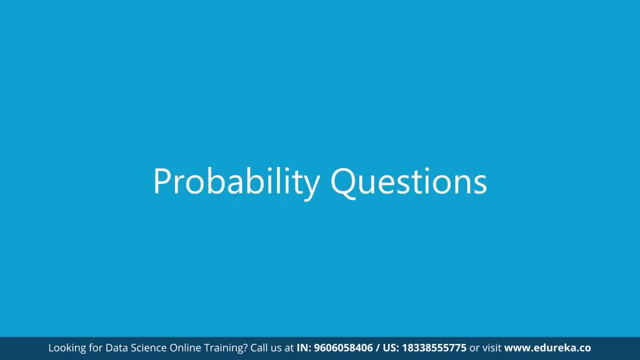 appropriate value of k, so value of k can be like 6 in this case. so I hope you are now getting comfortable with questions around data analysis, statistics and even the machine learning part. so the next pillar, which might very closely be associated with statistics as well, is around probability, right, so it is like in sometimes in most of the standard. 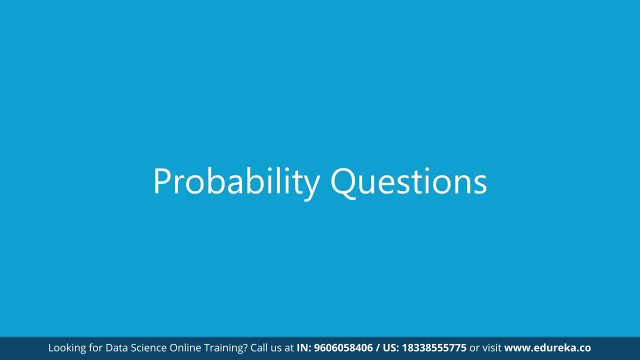 literature, probability and statistics comes together, it is now inseparable anytime. so in the Naive Bayes algorithm like this is one of the machine learning algorithm which is based on the Bayes theorem. probability ideas are quite a lot used and there are some really niche probability concepts, like the probability graph models, which is actually based on the 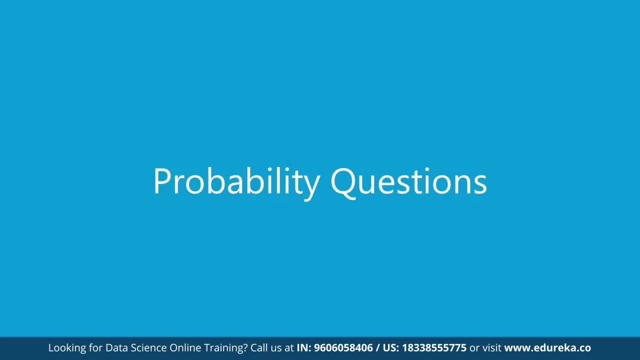 basics coming from Bayes theorem and the fundamental properties around probability. I will not go to that detail of probability in interview questions. if you have an expertise around probability and probability graph models or Naive Bayes kind of algorithms, I will not feel like confident to speak about it. but most of the time the probability questions. 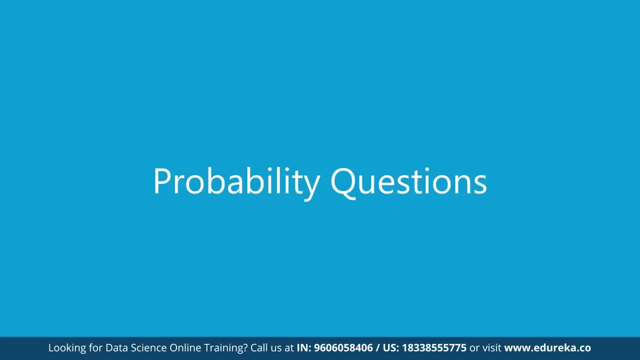 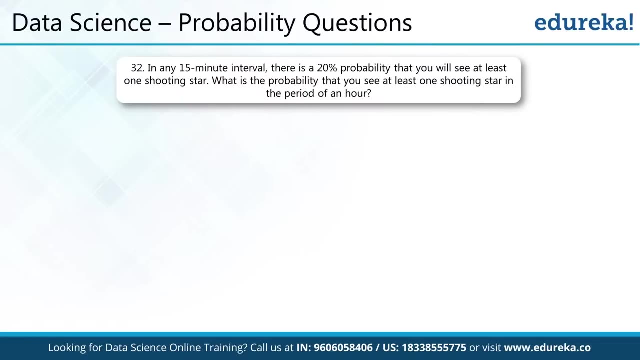 are quite basics and fundamentals, like the one which is asked in interviews, depending on, obviously, in which place you are giving the interview at. so let us also like see some sort of approach in attacking a probability problems. ok, so I will like read it out for you what the problem is here. so it says in any 15 minute interval there is a 20% probability. 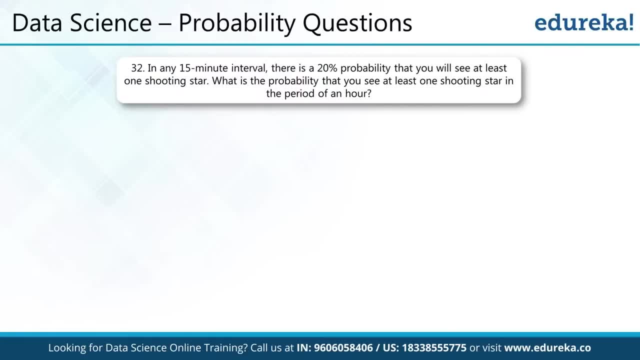 that you will see a shooting star, Like a good example, rather. so what is the probability that you see at least one shooting star in a period of an hour? so there is unknown information given to us that every 15 minute interval there is this 20% probability you will see at least one star. so we now want 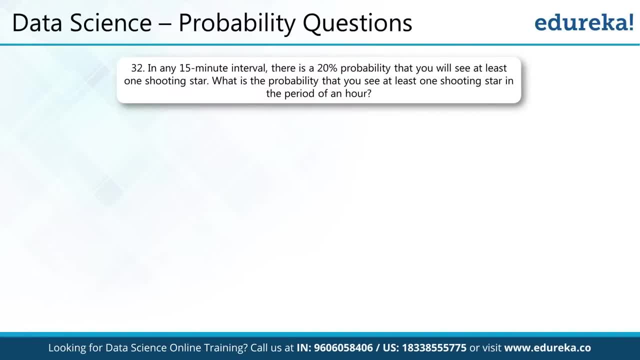